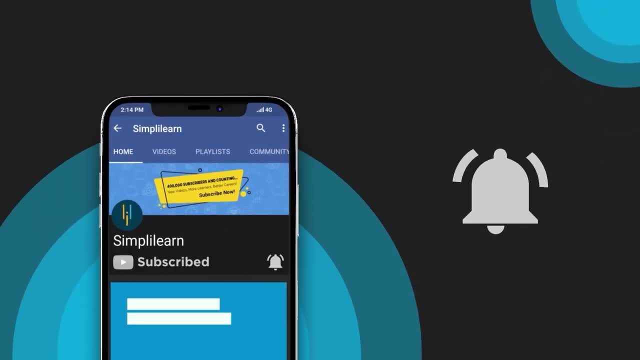 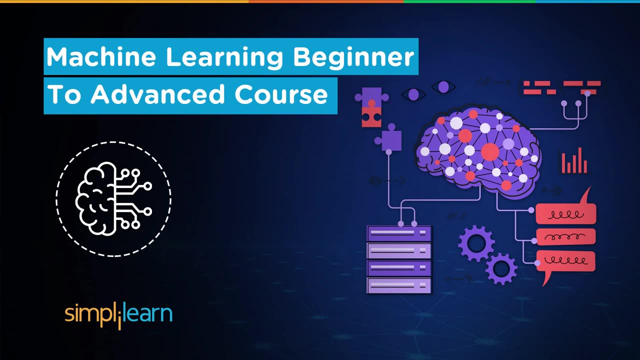 Hello everyone, welcome to this fantastic machine learning beginner to advance full course by simply learn. But before we begin, if you enjoy watching these videos and find them interesting, subscribe to our channel, as we bring you the best videos daily. Also, hit the bell icon to never miss any updates from simply learn. So let's get started. We. 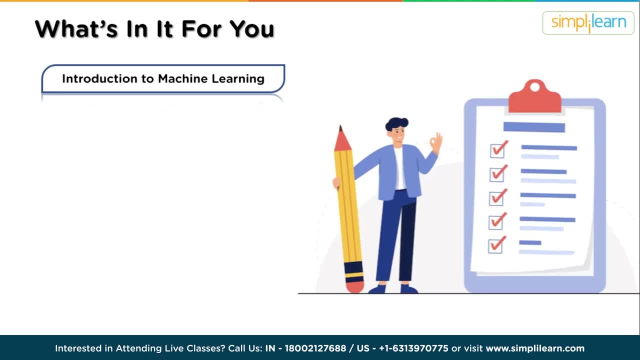 will brief you with machine learning introduction. After that we will see the types of machine learning. Forward, we will cover machine learning roadmap, skills required for machine learning engineers and the top applications and projects for machine learning. We will walk you through. 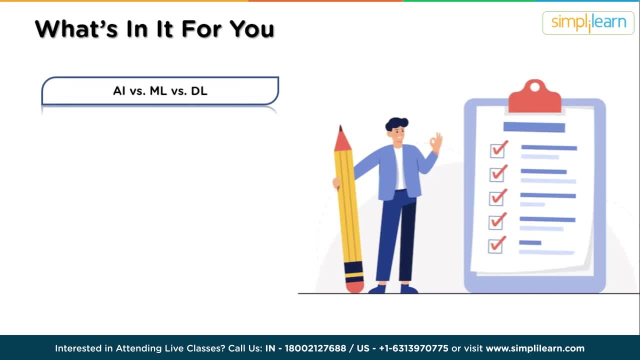 some fantastic concepts like AI versus ML versus DL. By proceeding with the course, we will teach you different machine learning algorithms like linear regression, logistic regression and many more. We will walk you through unique projects like fake news detection, object detection and 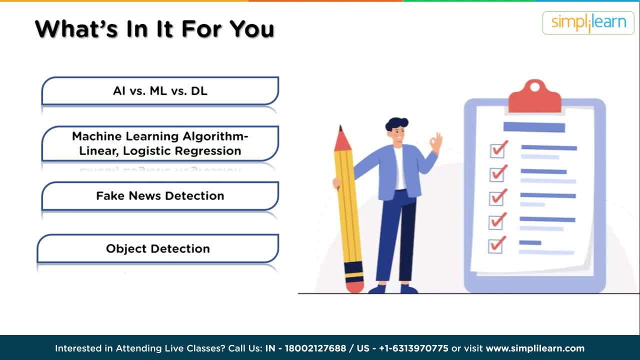 many more. These projects will serve you as the finest portfolios for your future interviews. Speaking of interviews, we have covered you long with most frequently asked machine learning interview questions to help you crack the most challenging interviews. But before we begin to understand what machine learning is, if you want to become an AI expert and 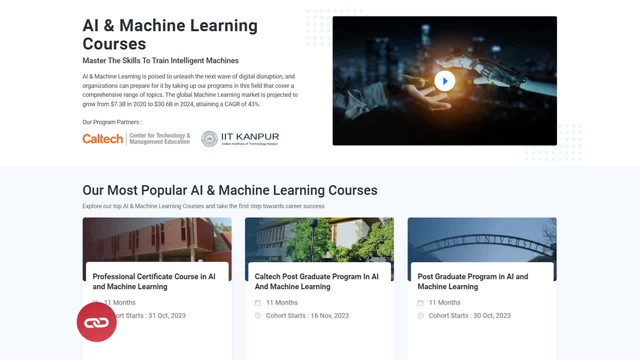 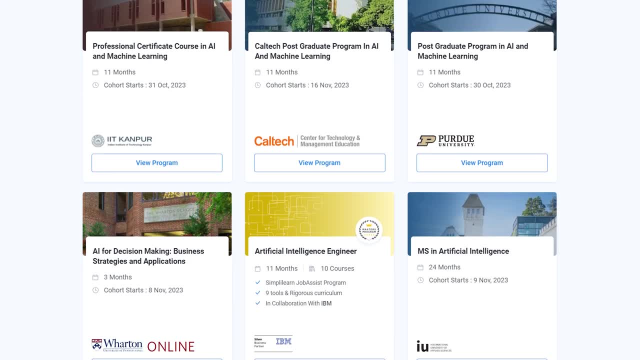 gain handsome salary packages. look at the wide range of AI ML courses by simply learn in collaboration with top universities across the globe. By enrolling in any of these certification programs, you will gain expertise in skills like generative AI, prompt engineering, chat. 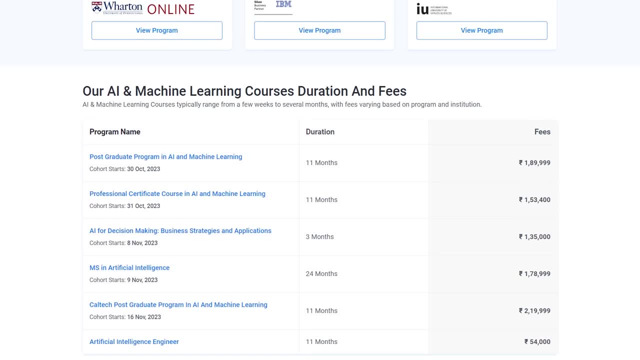 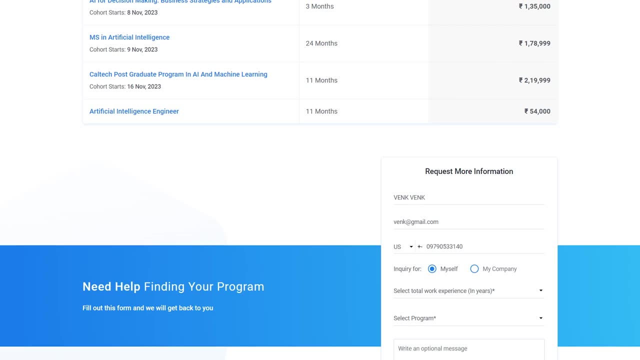 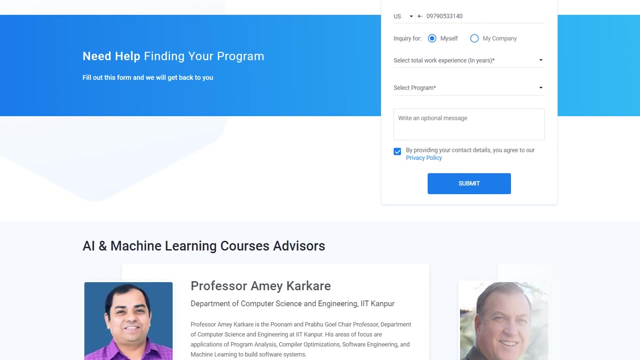 GPT, explainable AI, machine learning algorithms, supervised and unsupervised learning, model training and optimization, And there's much more on the list. With hands-on experience in the tools like ChatGPT, DALI, Python, OpenCV and TensorFlow, you will catch the eyes of. 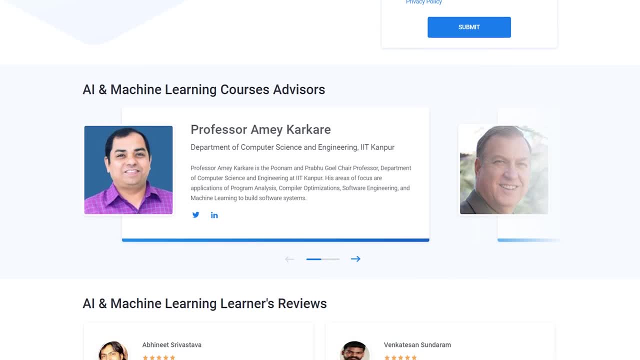 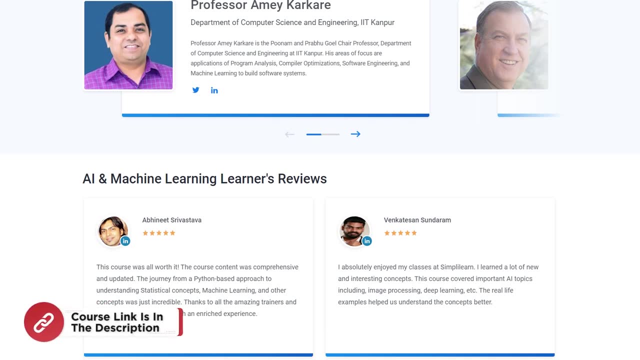 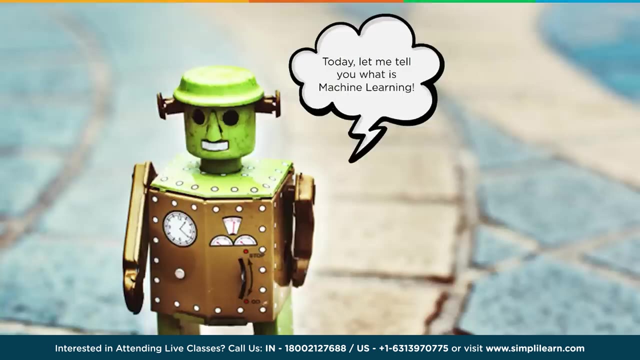 top recruiters. So what are you waiting for? Hurry up and enroll now. An year of experience is preferred to enroll in these courses. Find the course link in the description box. With that in mind, over to our training experts. Here we have our. it looks a little bit like Frankenstein, our Frankenstein-looking robot. 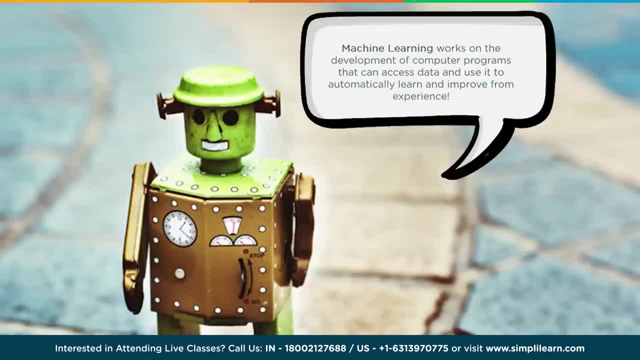 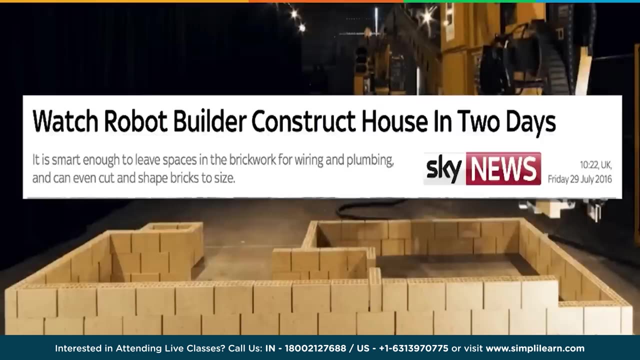 Today, let me tell you what is machine learning, Machine learning. machine learning is the technology that works on the development of computer programs that can access data and use it to automatically learn and improve from experience. Watch a robot builder construct a house in two days. This was back in July 29th 2016,. so that's pretty impressive, this. 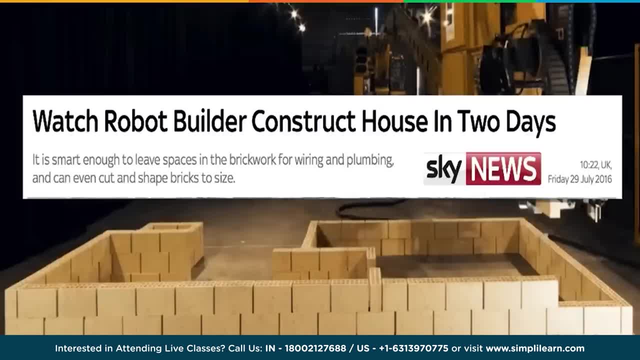 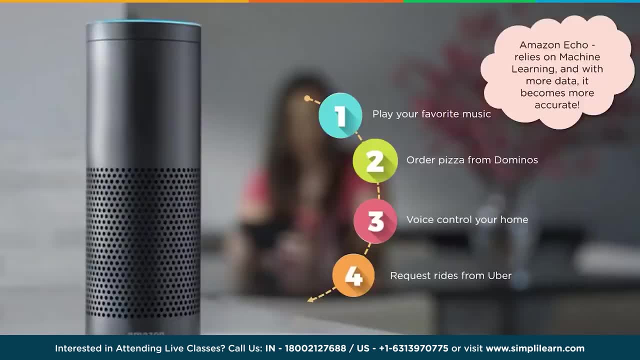 amount of time to continue to grow in its development And it's smart enough to leave spaces in the brickwork for wiring and plumbing, and can even cut and shape bricks to size Amazon. Echo relies on machine learning And with more data it becomes easier to learn. 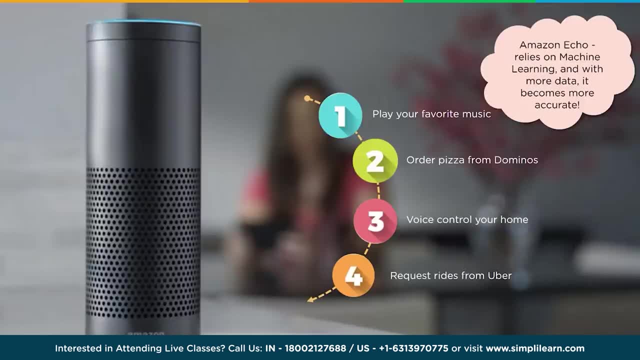 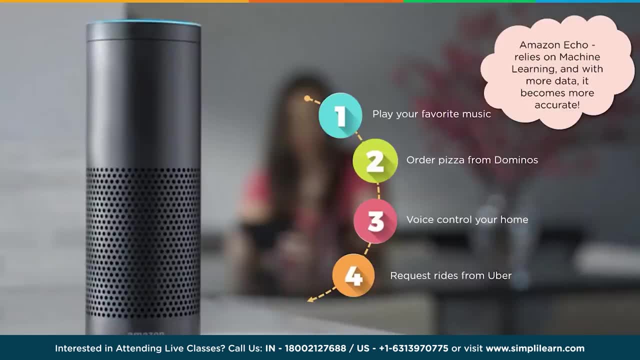 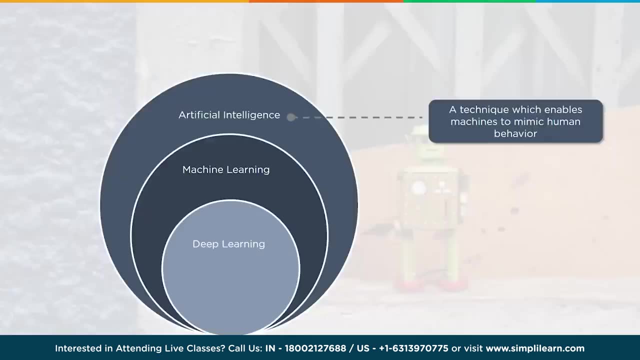 Play your favorite music, Order pizza from Domino's Voice, control your home. Request rides from Uber. Have you ever wondered the difference between AI- machine learning- and deep learning- Artificial intelligence- a technique which enables machines to mimic human behavior? This is really important, because this is how we are able to gauge how well our computations. 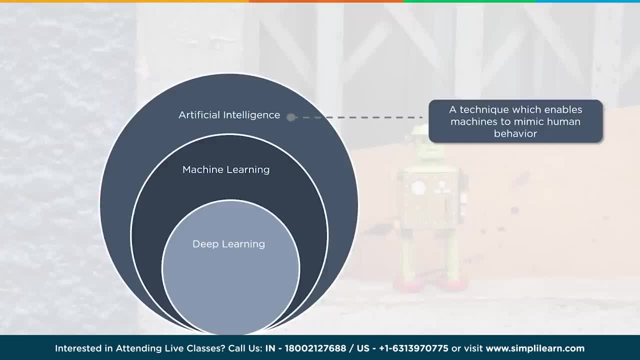 or what we're working on works, is the fact that we're mimicking human behavior. We're using this to replace human work and make it more efficient and make it more streamlined and more accurate, And so the center of artificial intelligence is the big picture of all this put together. 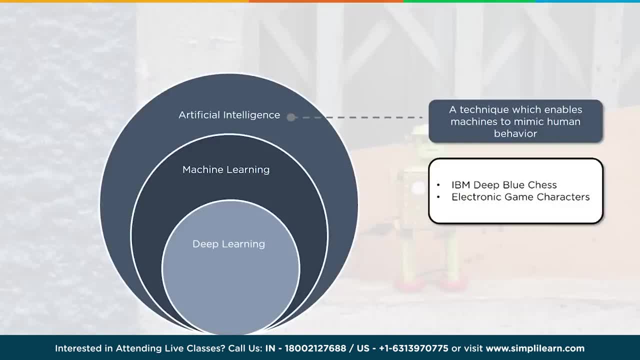 IBM deep blue chess electronic game characters. Those are just a couple examples of artificial intelligence. Machine learning, a technique which uses statistical methods enabling machines to learn from their past data. So this means if you have your input from last time and you have your. 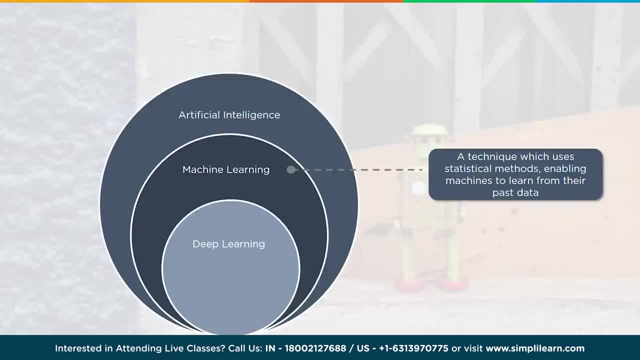 answer. you use that to help prove the next guess. it makes for the correct answer. IBM Watson, Google search algorithm, email spam filters- These are all part of machine learning. And then deep learning, which is a subset of machine learning, composing algorithms that allow a model to train itself, and 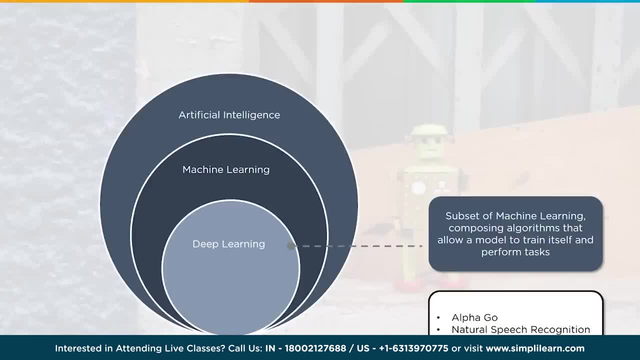 perform tasks- AlphaGo, natural speech recognition- These are a couple examples. Deep learning is associated with tools like neural networks, where it's kind of a black box. As it learns, it changes all these things that are, as a human, we'd have a very hard time tracking, And it's able to come up. 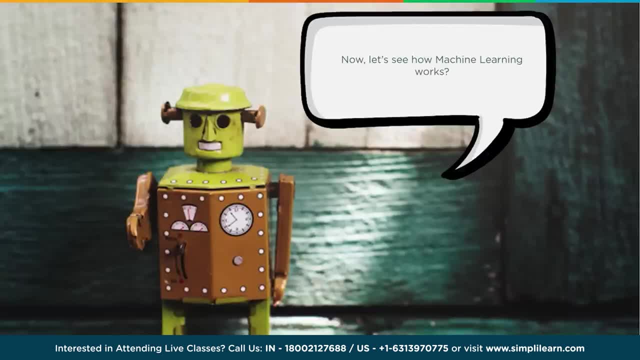 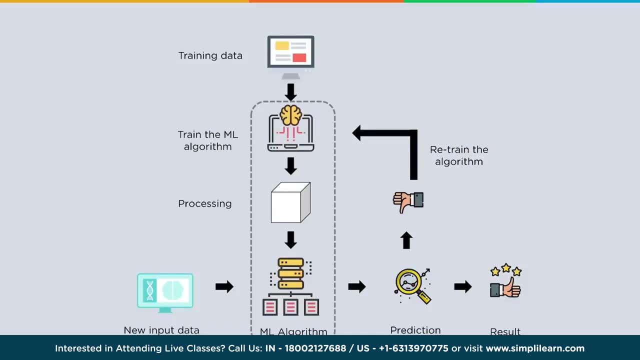 with an answer from that. Now let's see how machine learning works. First we start with training the data. Once we've trained the data, the train, we go into the machine learning algorithm, which then puts the data into a processing, which then goes down to machine- another machine learning. 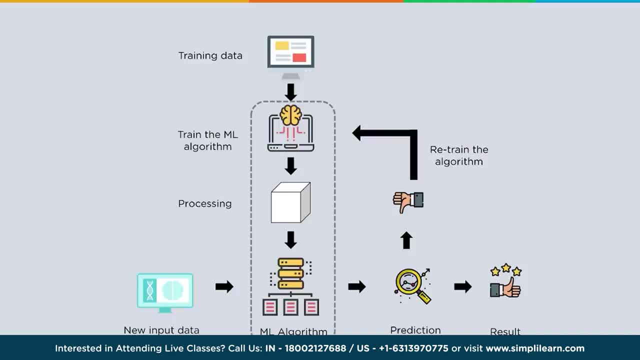 algorithm And then we take new data- because you have to test whatever you did and make sure it works correctly- and we put that into the same algorithm. Once we do that, we check our prediction, we check our results And, from the prediction, if we've set aside some training data and we find 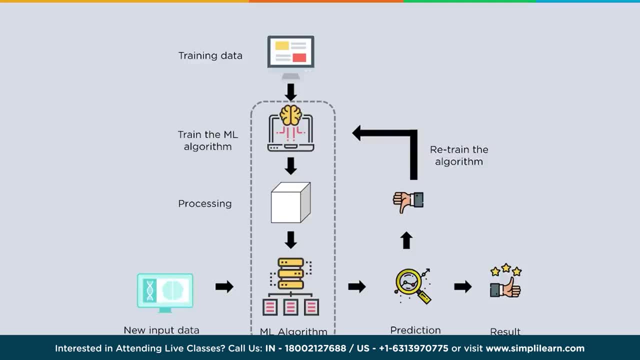 out, it didn't do a good job predicting it and it gets a thumbs down, as you see. then we go back to the beginning and we retrain the algorithm, And a lot of times it's not just about getting the wrong answer, it's about continually trying to get a better answer. So you'll see, the first time you 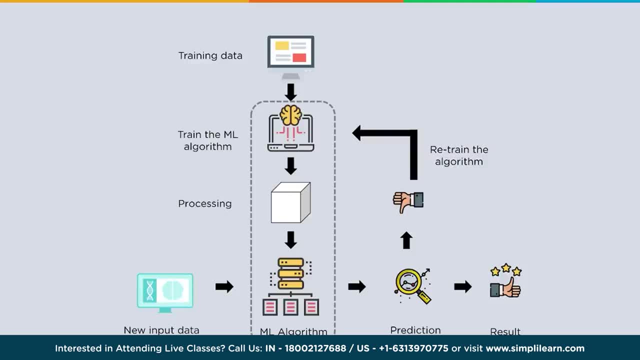 might be like: oh, this is not the answer I want, depending on what domain you're working in, whether it's medical, economical, business, stocks, whatever. You try out your model and if it's not giving you it, if you think you can get a better answer, you retrain it And you keep doing that until you get. 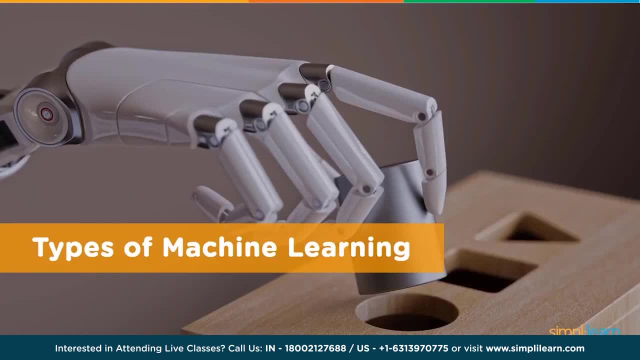 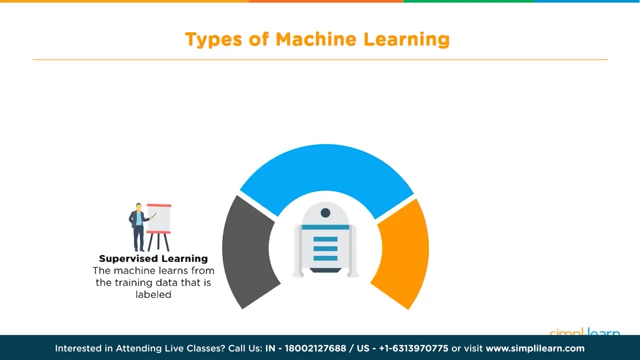 the best answer you can. Now let's look into the types of machine learning. Machine learning is primarily of three types. First one is supervised machine learning. As the name suggests, you have to supervise your machine learning while you train it to work on its own. It requires labeled training. 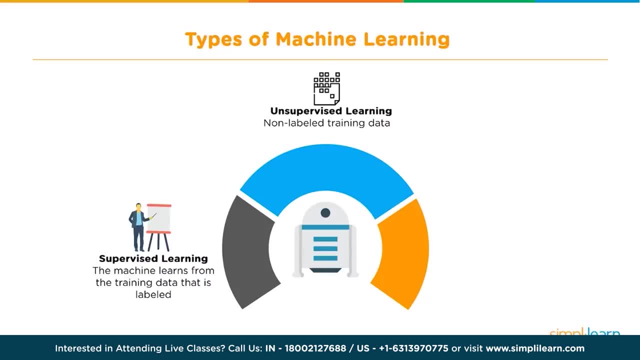 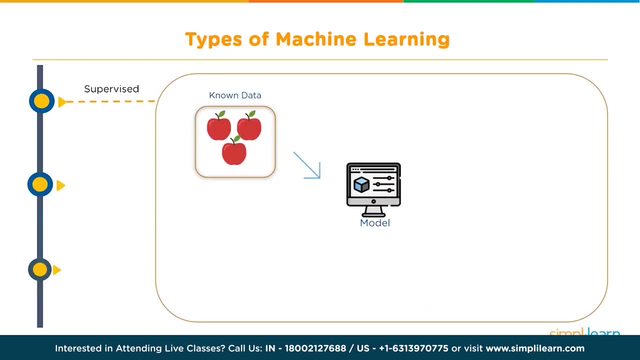 data. Next up is unsupervised learning, wherein there will be training data but it won't be trained. There is reinforcement learning, wherein the system learns on its own. Let's talk about all these types in detail. Let's try to understand how supervised learning works. Look at the pictures. very, very. 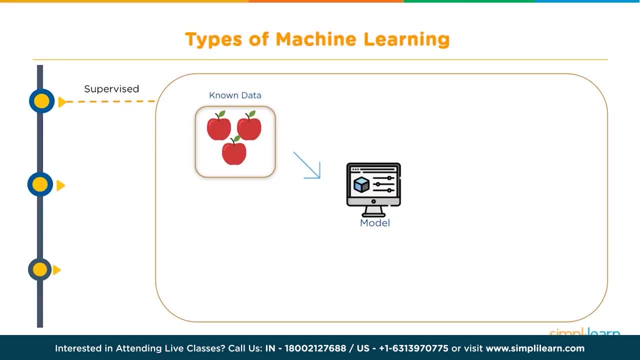 carefully. The monitor depicts the model or the system that we are going to train. This is how the training is done. We provide a data set that contains pictures of a kind of a fruit, say an apple. Then we provide another data set which lets the model know that these pictures were that of a fruit called apple. 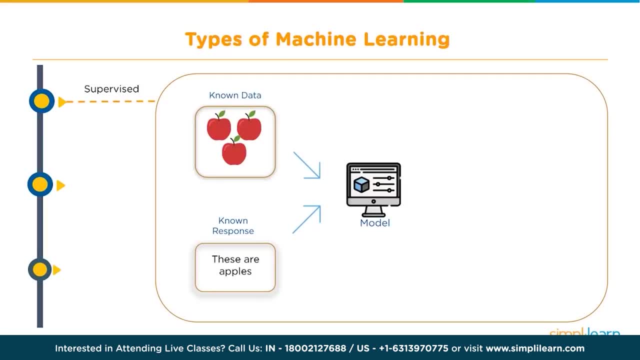 This ends the training phase. Now what we will do is we provide a new set of data which only contains pictures of apple. Now here comes the fun part: The system can actually tell you what fruit it is, And it will remember this and apply this knowledge in future as well. That's how supervised learning 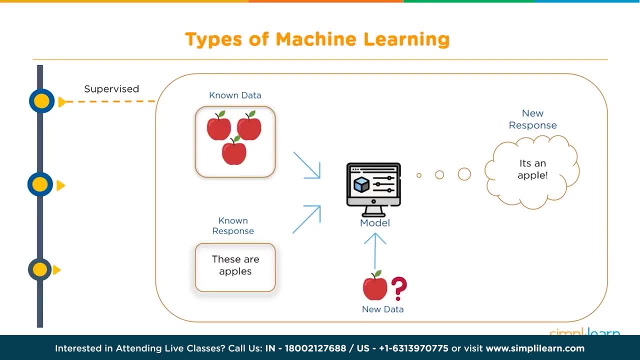 works. You are training the model to do a certain kind of an operation on its own. This kind of a model is generally used into filtering spam mails from your email accounts as well. Yes, surprise, aren't you? So let's move on to unsupervised learning. now Let's say we have a data set which is 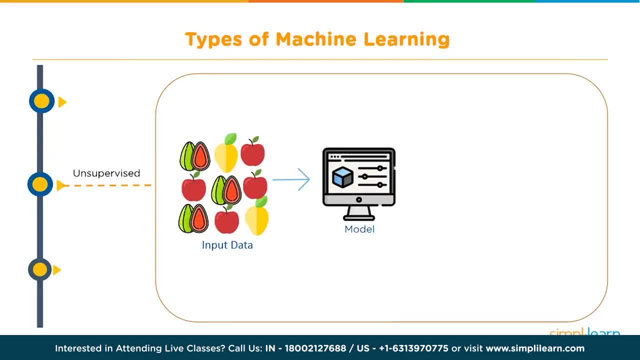 cluttered. In this case, we have a collection of pictures of different fruits. We feed these data to the model and the model analyzes the data to figure out patterns in it. In the end, it categorizes the photos into three types, as you can see in the image, based on their similarities. 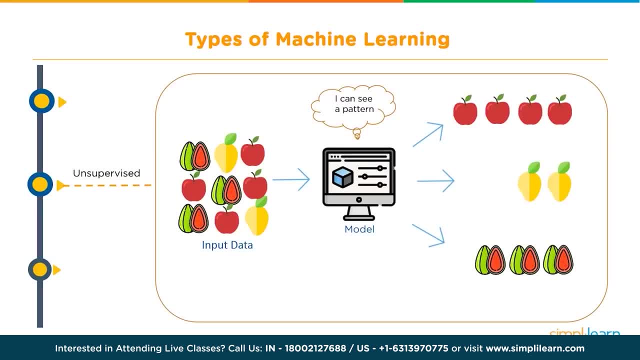 So you provide the data to the system and let the system do the rest of the work. Simple, isn't it? This kind of a model is used by Flipkart to figure out the products that are well suited for you. Honestly speaking, this is my 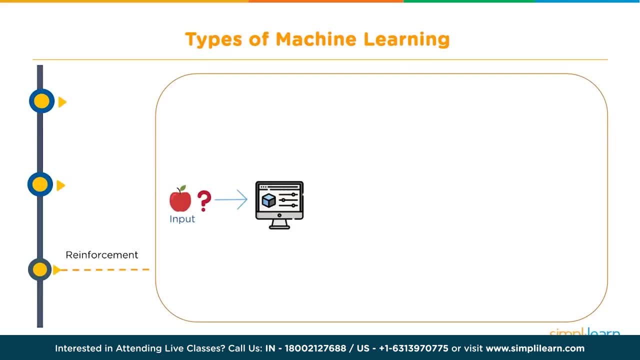 favorite type of machine learning out of all the three, And this type has been widely shown in most of the sci-fi movies lately. Let's find out how it works. Imagine a newborn baby. You put a burning candle in front of the baby. The baby does not know that if it touches the flame, its fingers. 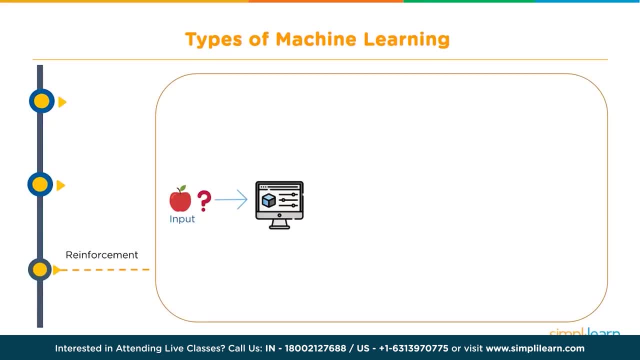 might get burned, So it does that anyway and gets hurt. The next time you put that candle in front of the baby, it will remember what happened the last time and would not repeat what it did. That's exactly how reinforcement learning works. 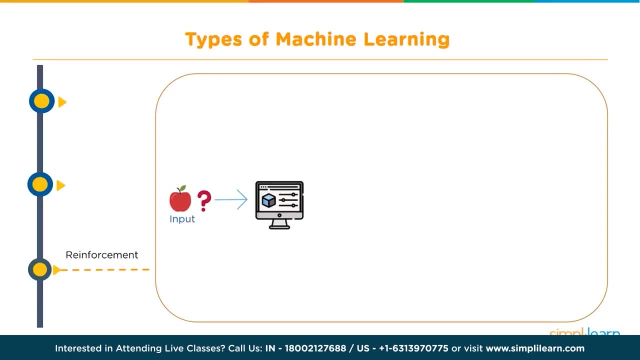 We provide the machine with a data set wherein we ask it to identify a particular kind of a fruit, In this case an apple. So what it does? as a response, it tells us that it's a mango, But, as we all know, it's a completely wrong answer. So, as a feedback, we tell the system that it's. 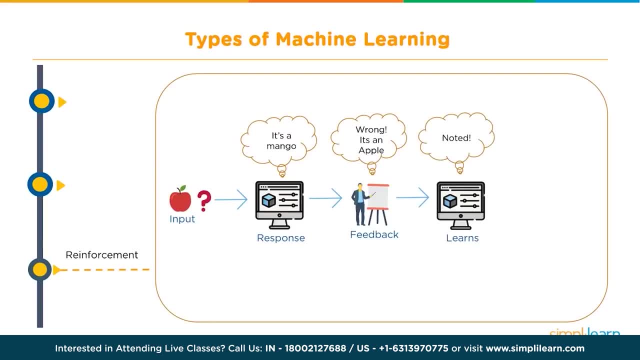 wrong. It's not a mango, it's an apple. What it does, it learns from the feedback and keeps that in mind When the next time when we ask a same question, it gives us the right answer. It is able to tell us that it's actually an apple. 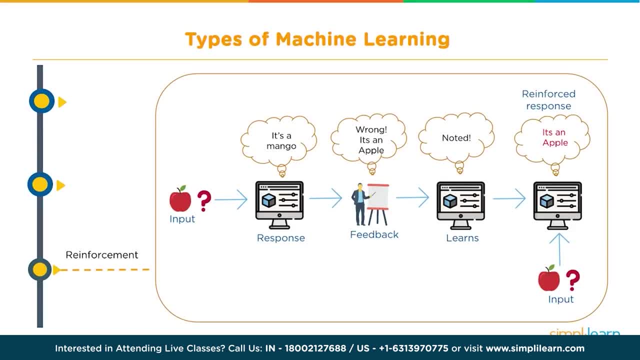 That is a reinforced response. So that's how reinforcement learning works. It learns from its mistakes and experiences. This model is used in games like Prince of Persia or Assassin's Creed or FIFA, wherein the level of difficulty increases as you get better with the games. 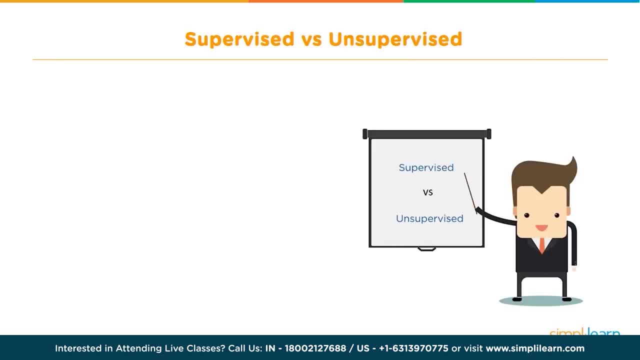 Just to make it more clear for you, let's look at a comparison between supervised and unsupervised learning. Firstly, the data involved in case of supervised learning is labeled. As we mentioned in the examples previously, we provide the system with a photo of an apple. 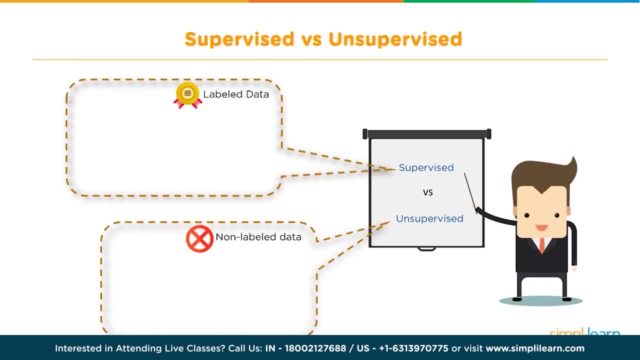 and let the system know that this is actually an apple. That is called labeled data, So the system learns from the labeled data and makes future predictions. Now, unsupervised learning does not require any kind of labeled data, because its work is to look for patterns in the input data. 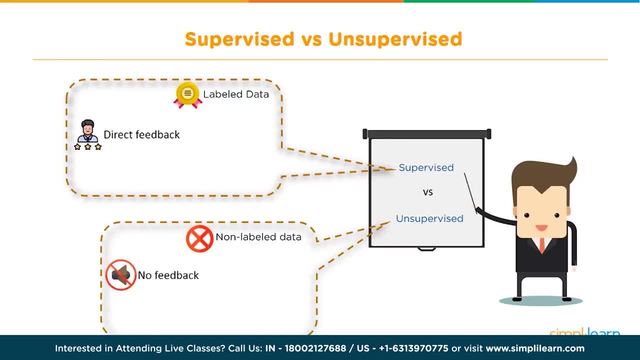 You can organize it. The next point is that you get a feedback. in case of supervised learning, That is, once you get the output. the system tends to remember that and uses it for the next operation. That does not happen for unsupervised learning. 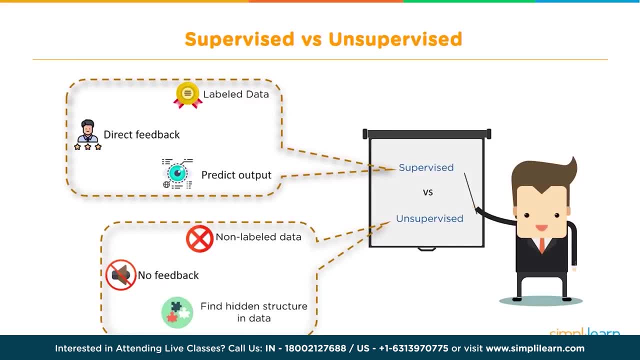 And the last point is that supervised learning is mostly used to predict data, whereas unsupervised learning is used to find out hidden patterns or structures in data. I think this would have made a lot of things clear for you regarding supervised and unsupervised. 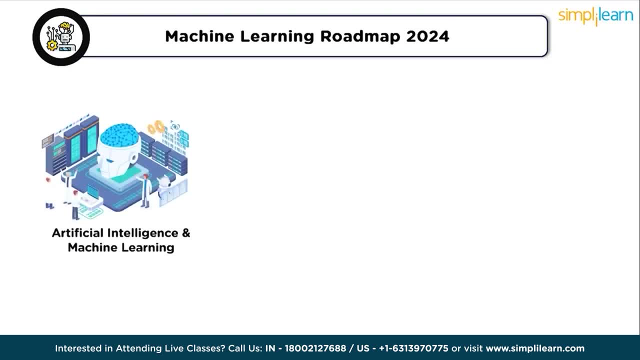 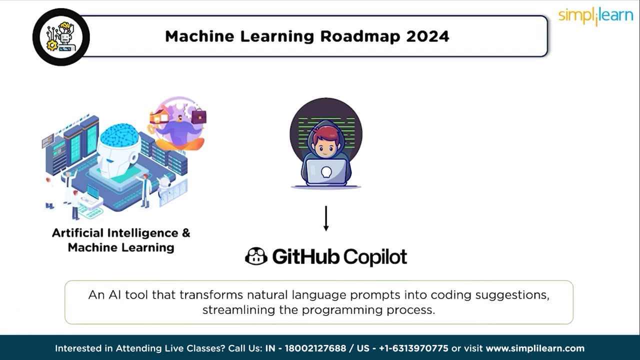 learning. In recent years, artificial intelligence and machine learning have permeated every aspect of our lives. If you are a programmer, chances are you have begun utilizing GitHub's Copilot, an AI tool that transforms natural language prompts into coding suggestions, streamlining the programming. 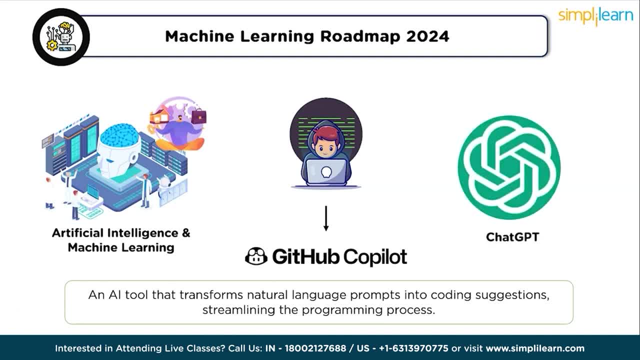 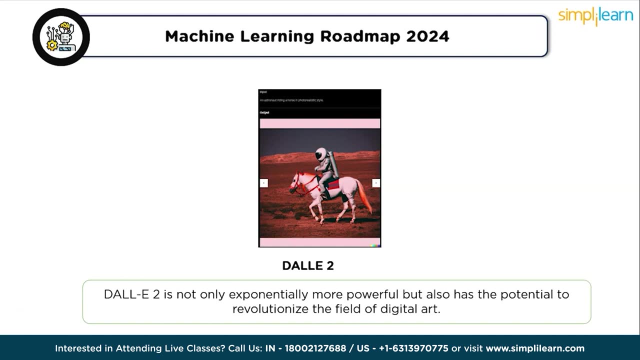 process. As a writer, you may have encountered OpenAI's GPT-3 or similar autoregressive language models that leverage deep learning to generate text resembling human language. Many of us are familiar with OpenAIcom. OpenAI has dedicated a few hours to experimenting with DALE2, the AIML-powered text-to-image generator. 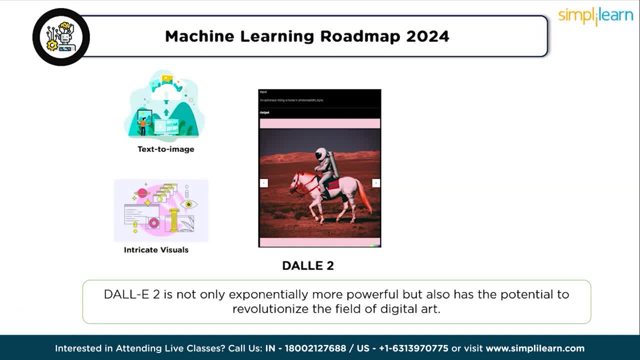 capable of producing intricate visuals based on the most unusual requests. Not only is DALE2 exponentially more powerful, but it also has the potential to revolutionize the field of digital art. Consider its impact on a digital artist, illustrator or graphic designer career. 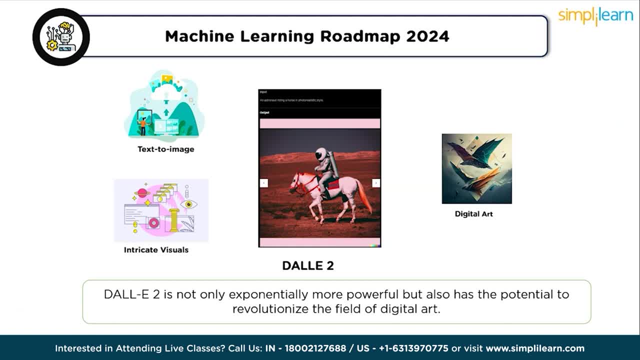 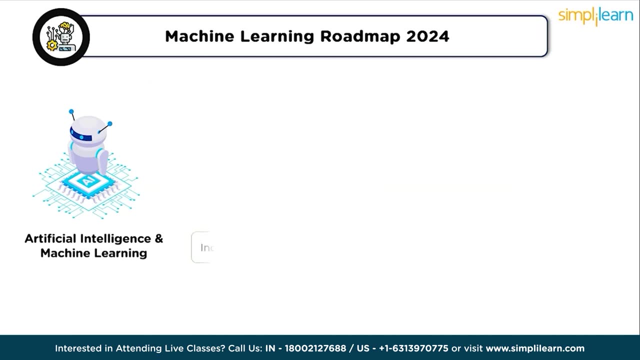 Imagine creating a highly realistic image within seconds using an app. These techniques can be used to create a digital image. These technologies have significant real-world applications with far-reaching implications. Let me tell you some fascinating facts about machine learning. According to recent studies, machine learning-related job postings have increased by a staggering. 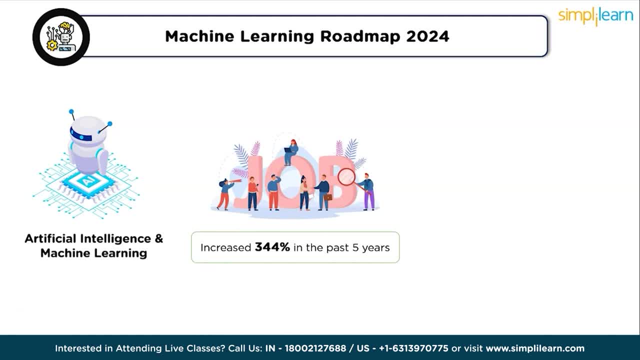 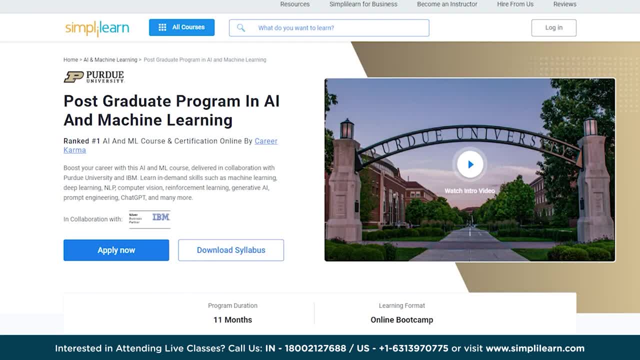 The average salary is about 800,000 per day in India and about 600,000 per week in disorder in India. Accelerate your career in AI and ML with our comprehensive postgraduate program in AI and machine learning. Gain expertise in machine learning, deep learning, NLP, computer vision and reinforcement. 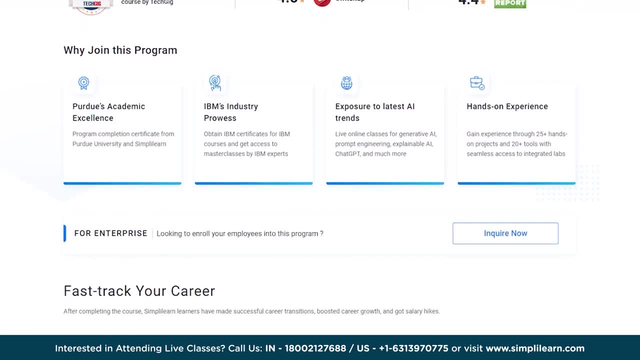 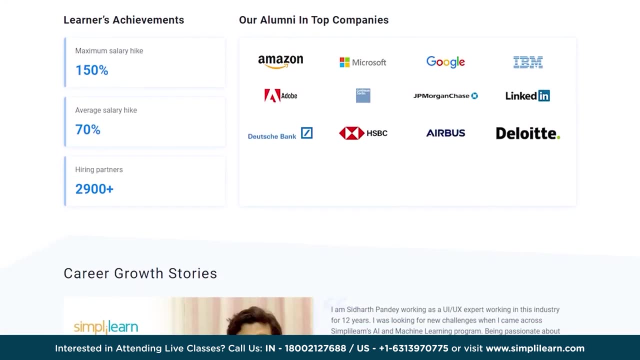 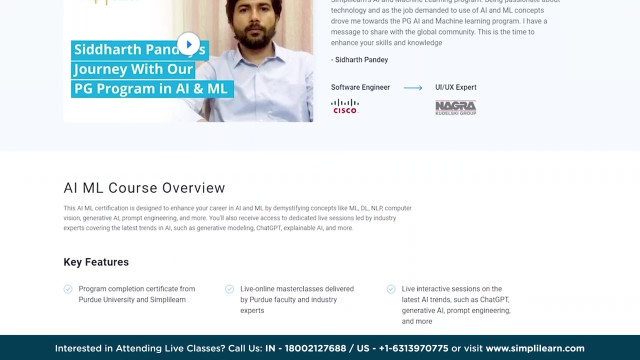 learning. You will receive a prestigious certificate, exclusive alumni membership and hackathons and ask-me-anything sessions by IBM, With three capstone and 25-plus industry projects using real datasets from Twitter, Uber and more. you will gain practical experience, master classes by purdue faculty and ibm experts ensure 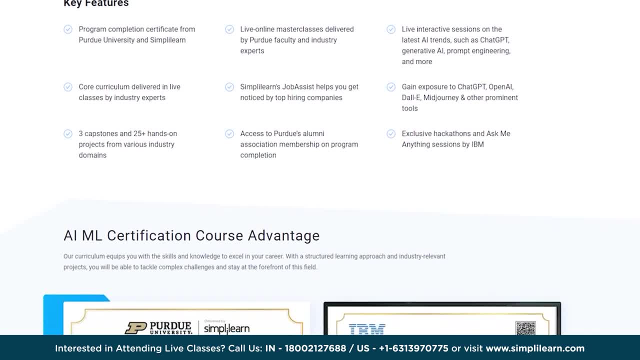 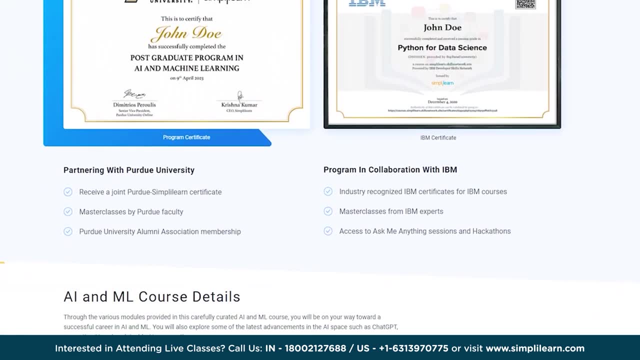 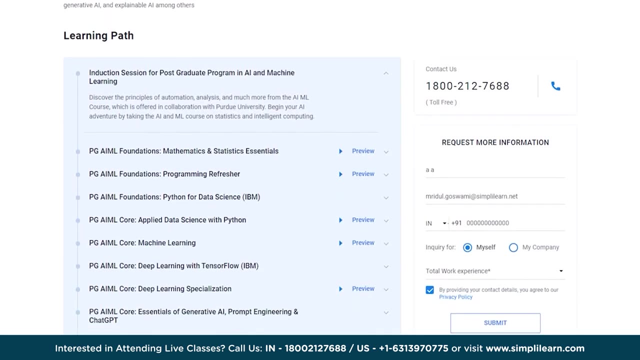 top-notch education simply learns. job assist helps you get noticed by leading companies, live sessions on ai trends like chat, gpt, generative ai and explainable ai. this program covers statistics, python, supervised and unsupervised learning, nlp, neural networks, computer vision, gans, keras, tensorflow and many more skills and roll now and unlock exciting. 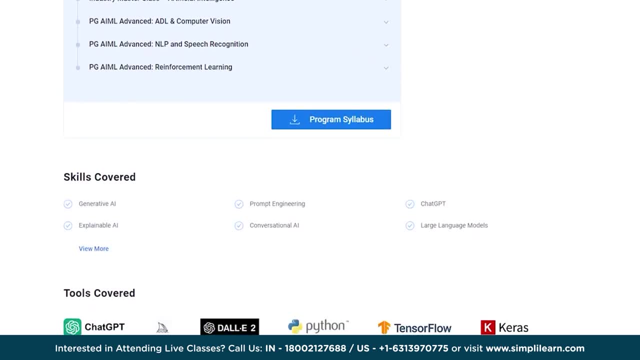 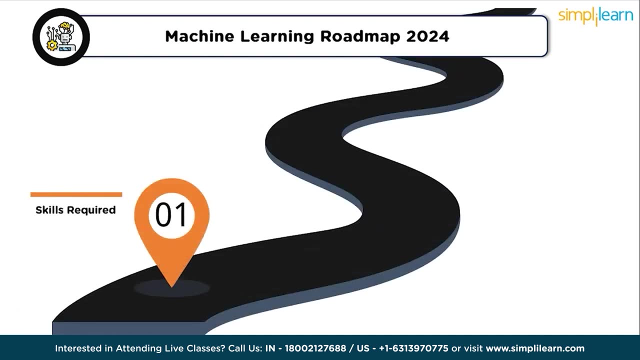 ai and ml opportunities. the link is mentioned in the description box below. with that having said now, here is a comprehensive step-by-step guide to learning machine learning. number one is skills required. number two: job roles in ml. number third company is hiring ml engineers. and the number four: 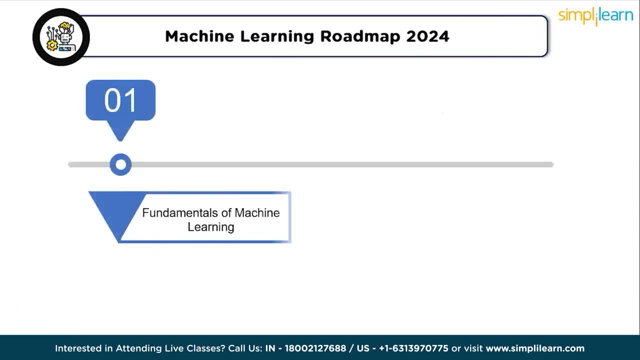 is future scope of ml? now, starting with the number one, that is, fundamentals of machine learning. familiarize yourself with the fundamentals of machine learning. you are familiarized with the different elements, varieties and regulations pertaining to operating a car. it is essential to delve into the fundamentals of machine learning to understand what lies. 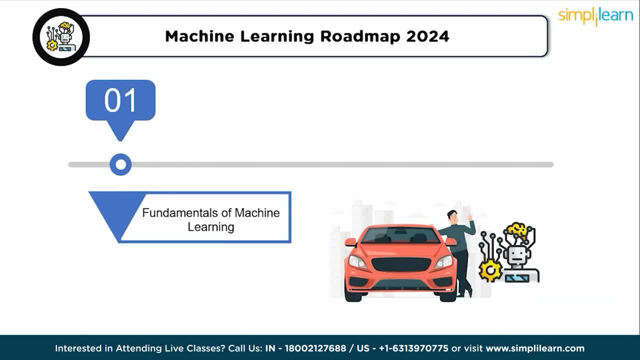 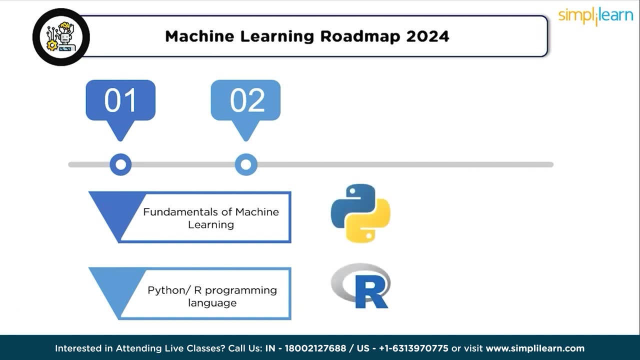 ahead and the required knowledge now moving to number two, that is, acquiring proficiency in python, or our programming language. to excel in the field of artificial intelligence and machine learning, it is crucial to develop a strong command of python and other software applications for machine learning. both python and r are widely used in the data science community. 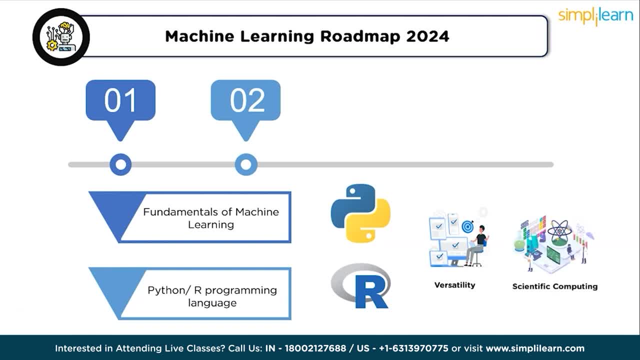 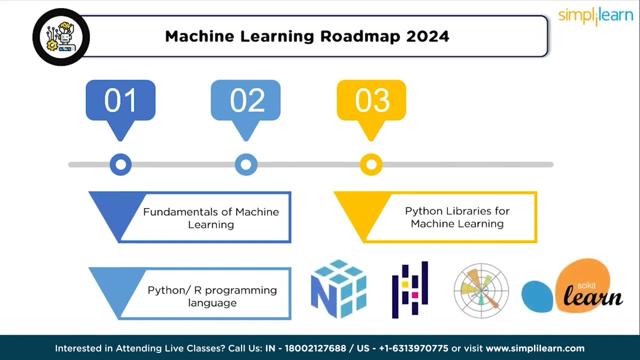 due to their versatility and extensive libraries for scientific computing. so now moving on to the third step, that is, gain knowledge of essential python libraries for machine learning. once you have acquired proficiency in python as part of a machine learning journey, the subsequent step involves familiarizing yourself with essential python libraries, crucial for working with python. 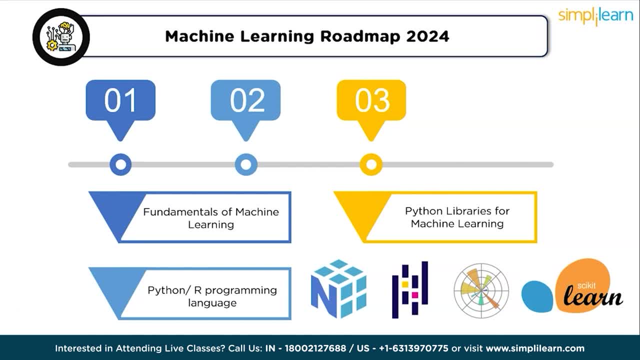 with data and implementing machine learning solutions. The key python libraries that you should learn for machine learning are numpy, pandas, matplotlib and scikit-learn. Now moving to step 4, that is, learn and implement various machine learning algorithms After gaining proficiency in python as part of our machine learning journey. the subsequent 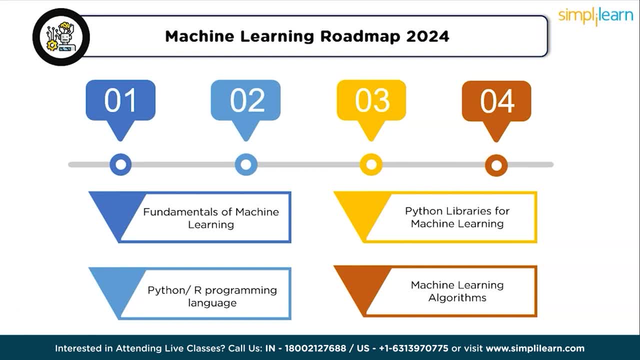 milestone involves learning various machine learning algorithms and their implementation using python. Listed below are some of the key machine learning algorithms that are essential to learning: 1. Linear regression, 2. Logistic regression, 3. Passive aggression. 4. Naive Bayes. 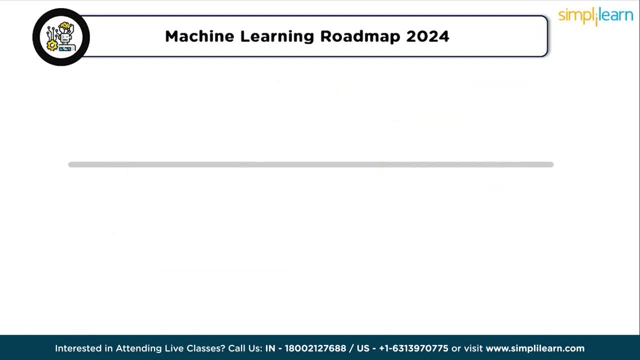 5. Support vector machines. Now, moving to step 5, master the concepts and implementation of neural networks. Once you have acquired knowledge of python and machine learning algorithms, the next significant step in the machine learning roadmap is to learn neural network architectures and 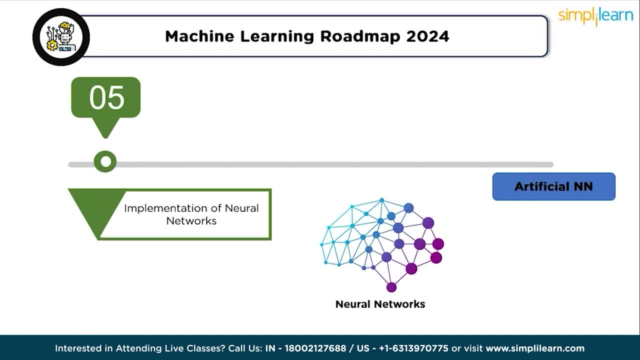 their implementation. Outlined below are several crucial neural network architectures that are essential to learning: 1. Artificial neural networks, 2. CNN, 3. RNNN, 4. Long short term memory. Now moving to step 6, that is, engage hands-on projects to apply your knowledge and reinforce. 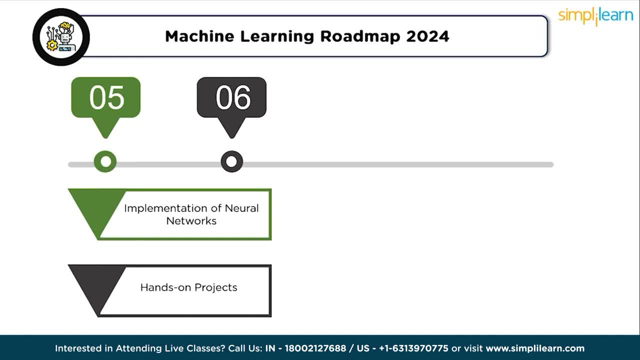 your understanding. After acquiring knowledge of python, machine learning algorithms and neural network architectures, the next crucial step is the machine learning roadmap and is to gain practical experience by working on projects that allow you to apply what you have learned. The first project is iris. flower classification number 2: California house price prediction. 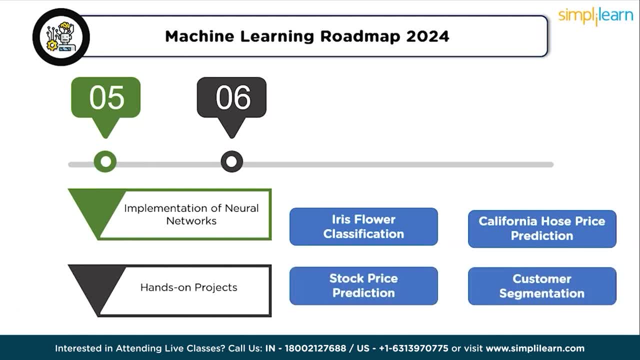 number 3: stock price prediction. number 4: customer segmentation. Now we'll move to job roles in machine learning. Machine learning, as highlighted earlier, has gained immense popularity for its ability to elevate human efforts. It has enhanced machine performance through autonomous learning. 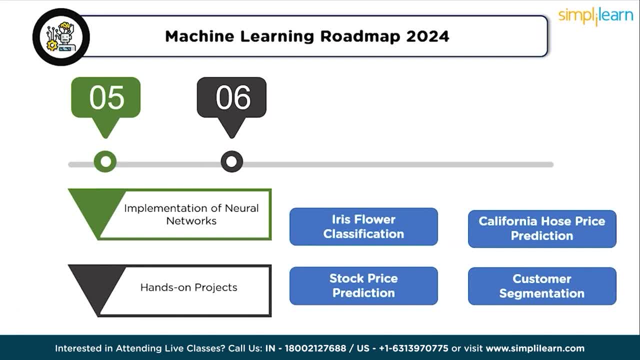 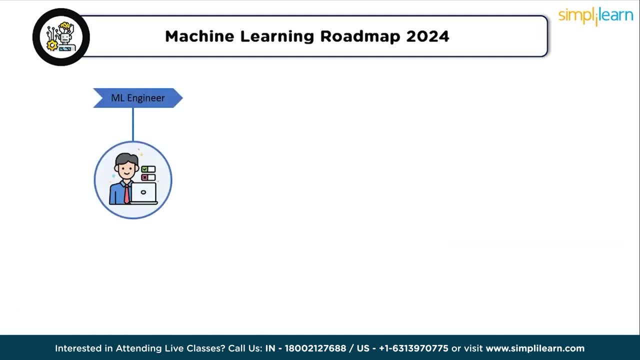 This popularity has resulted in lucrative and sought-after career options within the field, including roles like machine learning engineer. So the duty of a machine learning engineer encompasses the creation, construction and deployment of machine learning models, Collaborating closely with data scientists and software engineers, they participate in. 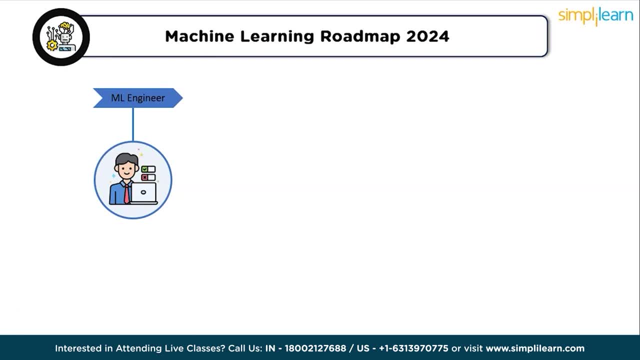 the development and execution of machine learning systems. According to Glaston, XML engineers can earn up to $150,000 in US and 11 lakhs per annum in India. Now moving to data scientist. The role of a data scientist involves gathering, scrutinizing and interpreting extensive datasets. 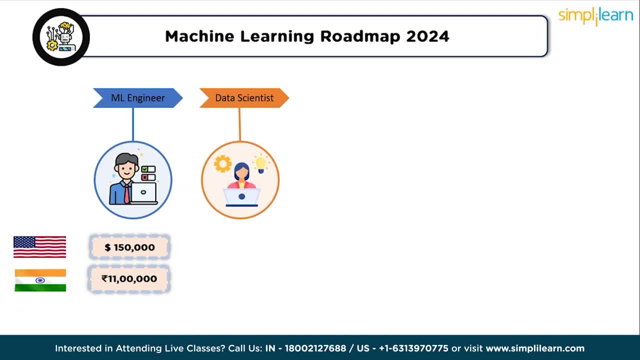 Leveraging machine learning algorithms, they uncover patterns and glean insights from the data, Utilizing this knowledge to inform decisions and address challenges. According to Glaston, Data scientists earn $145,000 in US and $155,000 in China. Now moving to NLP engineers. 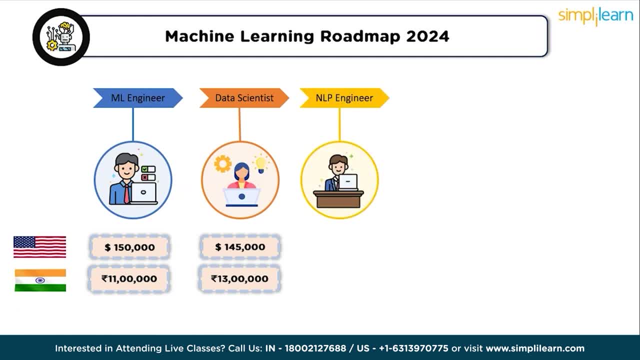 Their special duties may vary based on the role and sector, But as outlined by Freelancer Map, an NLP engineer typically engages in tasks such as designing natural language processing systems and addressing speech patterns and AI speech recognition. According to Glaston, an NLP engineer can earn $120,000 in US and 10 lakhs per annum. 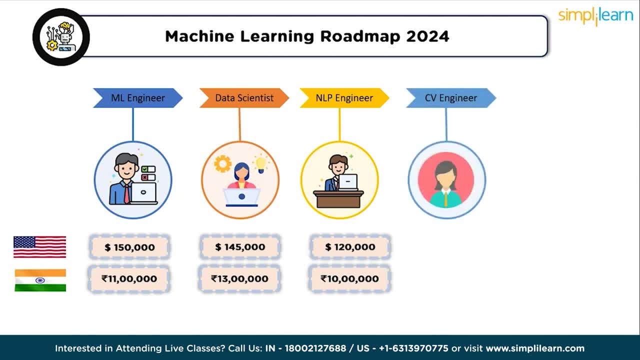 in India. Now moving to computer vision engineer. Engineers specializing in computer vision operate within the realm of computer vision, employing machine learning to empower computers to comprehend and interpret visual data from their surroundings. Their responsibilities include tasks such as image and video analysis and object detection. 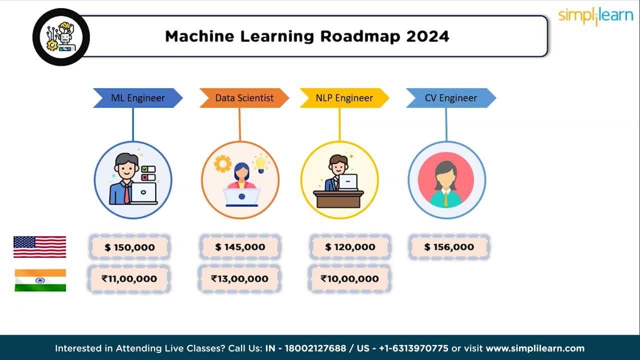 According to Glaston CV, engineers earn $156,000 in US and 8 lakhs per annum in India. Now moving to business intelligence developer. The main role of a BI developer is to develop, deploy and maintain BI tools and interfaces. 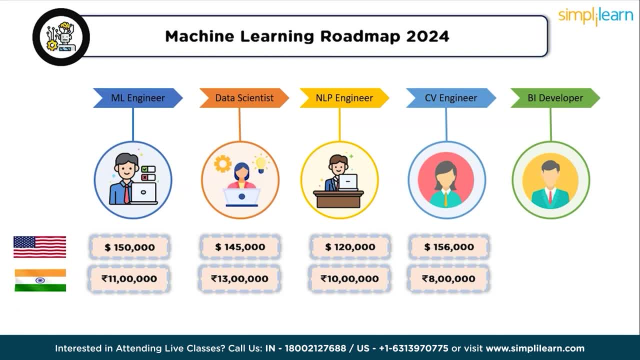 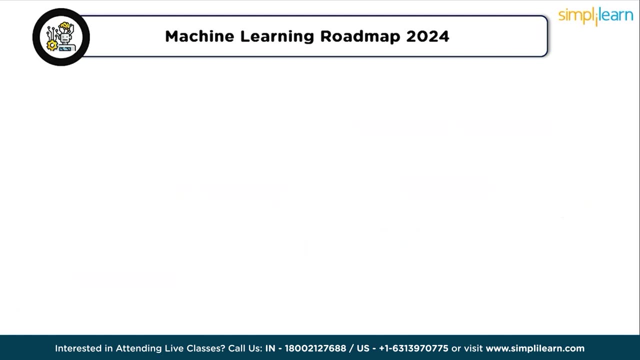 They are also responsible for simplifying highly technical language and complex information into layman's terms for everyone else in the company to understand. According to Glaston, business intelligence developers earn $105,000 in US and 7 lakhs per annum in India. 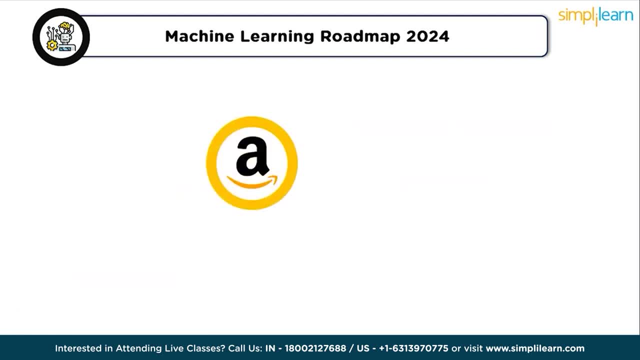 Now we'll see the top companies hiring for machine learning engineers. Number one is Amazon, then we have Accenture, Google, Apple, Intel. So these are the top hiring companies that hire machine learning engineers. Now we'll talk about the future of machine learning. 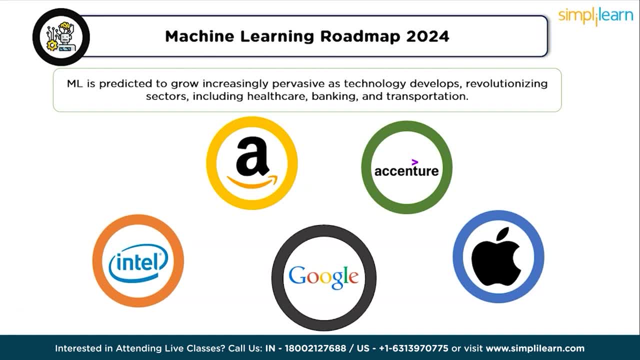 Machine learning has a bright future but faces several difficulties. ML is predicted to grow increasingly pervasive as technology develops, revolutionizing sectors including healthcare, banking and transportation. The work market will change due to the development of new technologies. In the future, ML is expected to be one of the leading companies in the world. 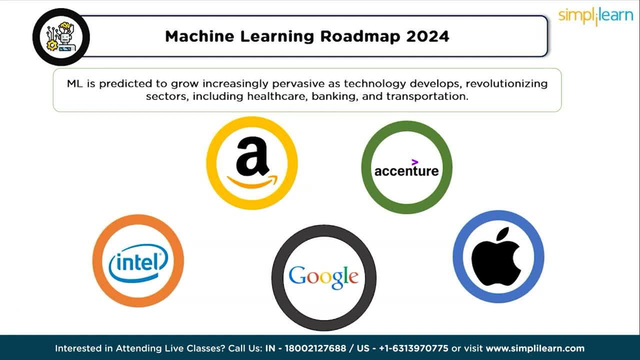 In the future, ML is expected to be one of the leading companies in the world. What does this mean? Last but not least, it means that the industry is moving very far toward AI-driven automation, necessitating a new position and skills, And with this we have come to the end of this video. 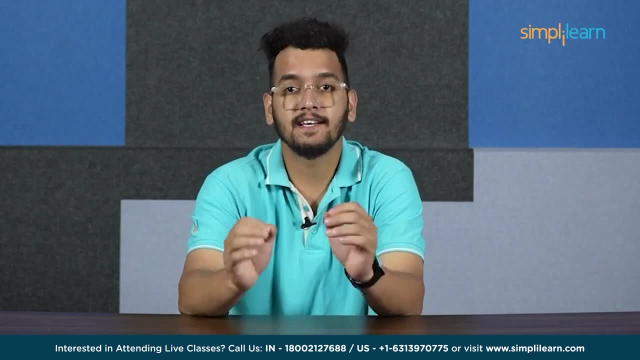 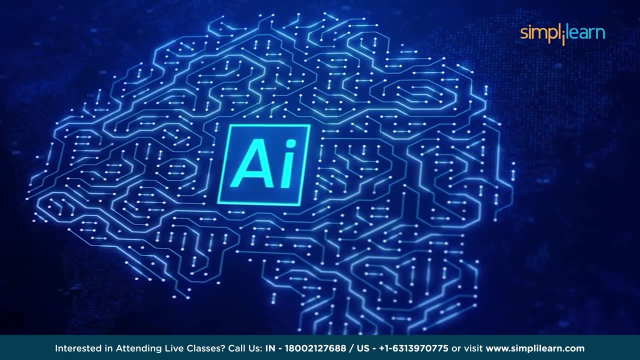 I hope you found this video informative and interesting. Let us begin. Hello Everyone, And welcome to our video on Skills Required for an ML Engineer. Machin3e learning has been the talk of the town lately. Every organization has realized the potential of machine learning. 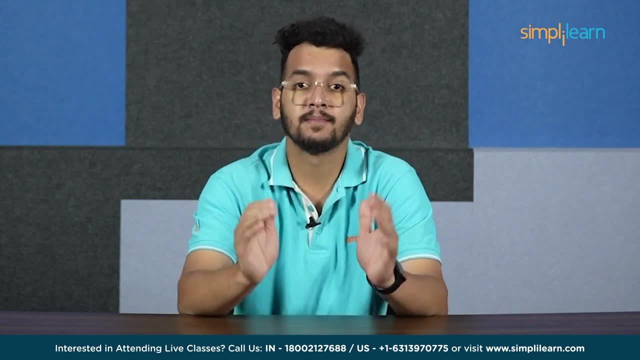 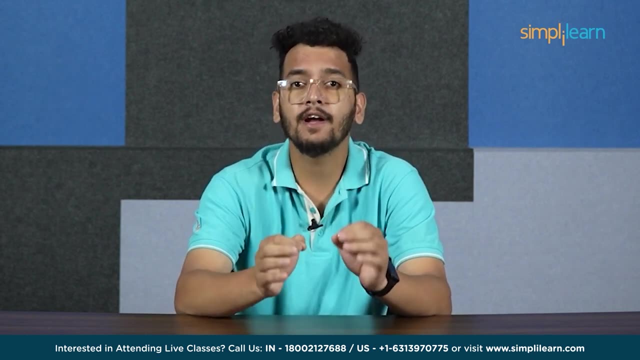 It is improving their business objectives and achieving its enterprise goals. Its growth process leads to visions of danelling- ό família learning jobs and upskilling themselves in the field of machine learning. you can take up this growing opportunity in the field of machine learning and utilize it to lend yourself a. 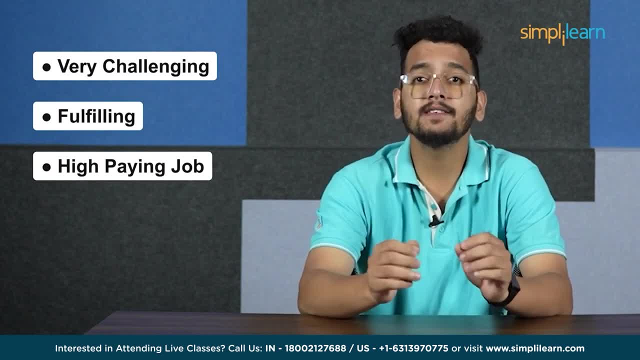 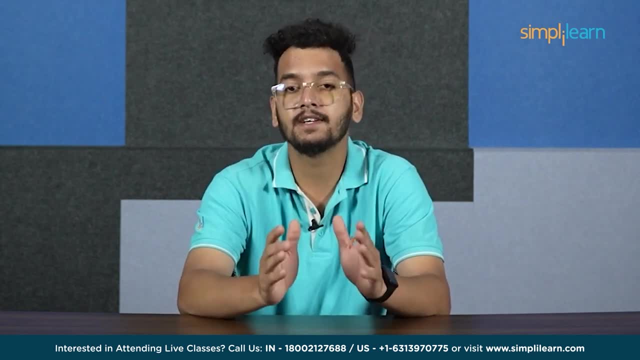 very challenging, fulfilling and high paying job. in this video, we will be breaking down in complete detail each and every skill that you would need in order to crack the machine learning engineer job interview. well, ml is not just a passing trend. it's a seismic shift that is reshaping our world. 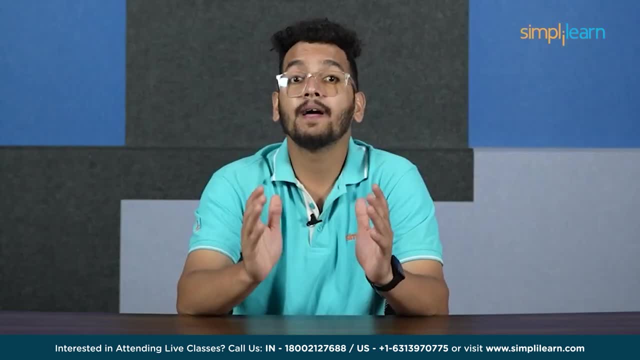 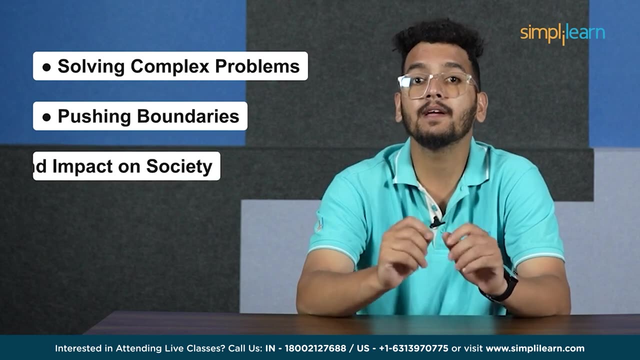 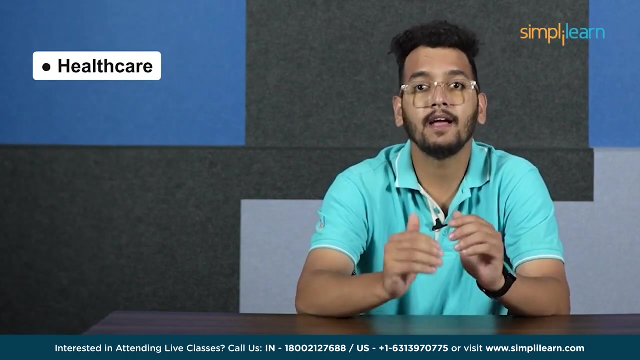 and creating new avenues for innovation and discovery. so by embracing a career in ml, you become part of dynamic field that thrives on solving complex problem, pushing boundaries and making a profound impact on society. so the demand for ml professional is skyrocketing across industries, from healthcare and finance to entertainment and transportation organizations. 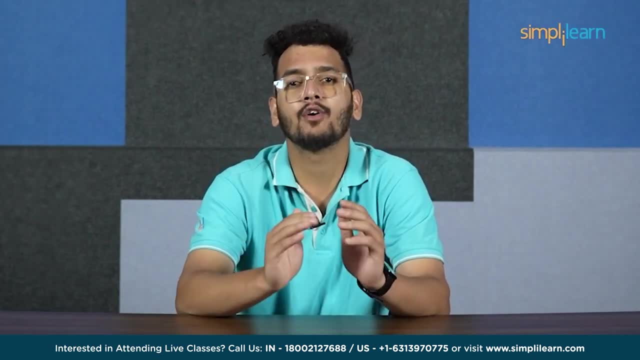 are actively seeking talented individuals who can harness the power of ai to drive their business forward. but what skill does it takes to become an ml engineer and create new avenues for innovation and discovery? so by embracing a career in ml, you become part of dynamic field that thrives on solving complex problem, pushing boundaries and making a 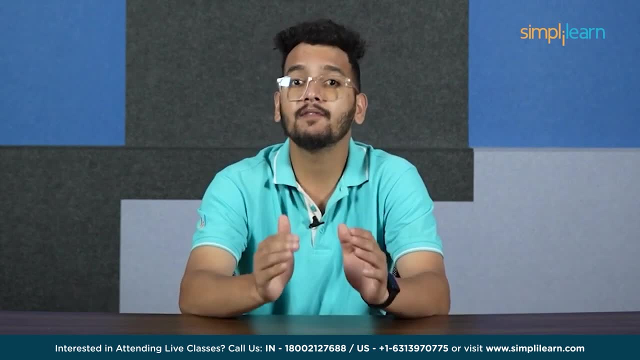 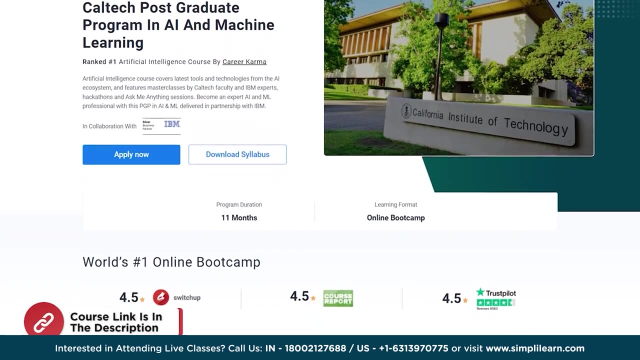 career in ml engineer. how can you embark on this thrilling journey? we have the answers to all your questions. also accelerate your career in ai and ml with our comprehensive postgraduate program in ai and machine learning. gain expertise in machine learning, deep learning, nlp, computer vision and. 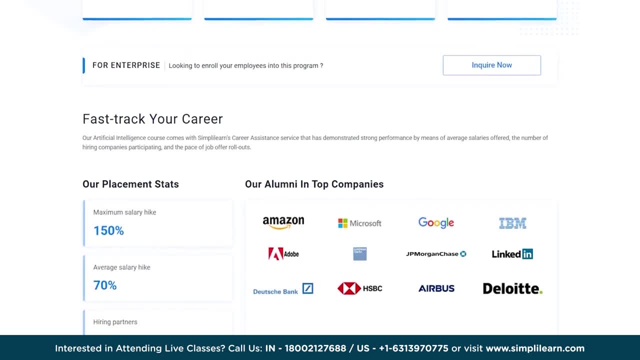 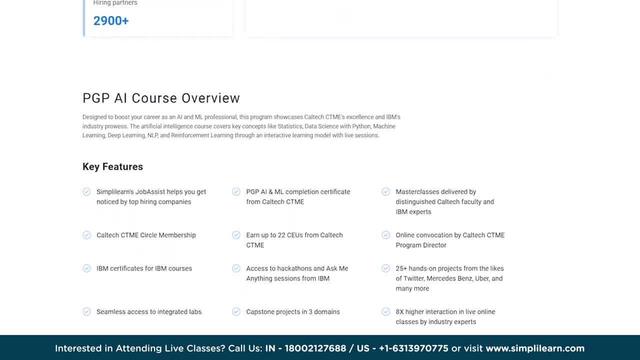 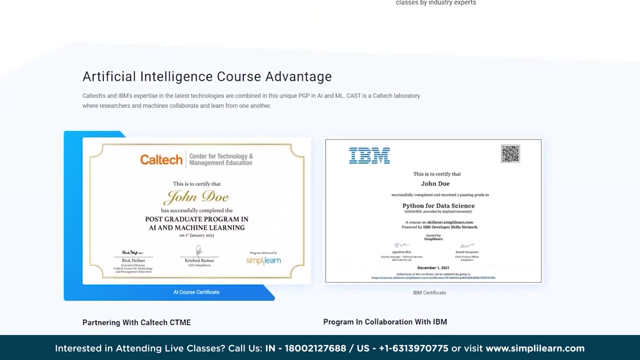 reinforcement learning. you will receive a prestigious certificate, exclusive alumni membership and- ask me anything- sessions by ibm, with three capstone projects and 25 plus industry projects using real data set from twitter, uber and more. you will gain practical experience. master classes by caltech faculty and ibm experts. 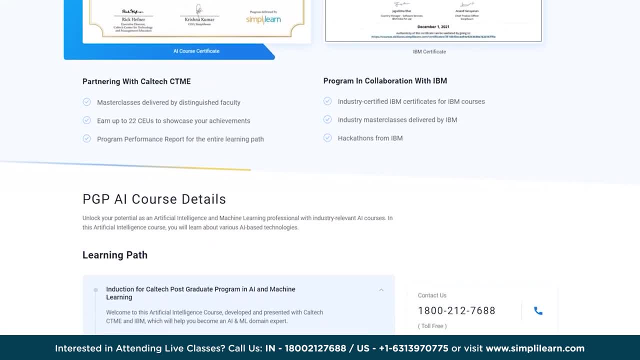 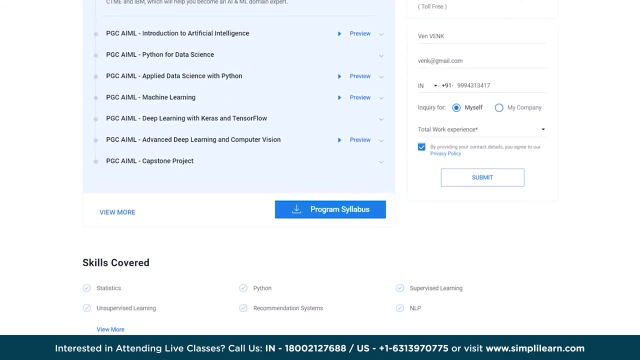 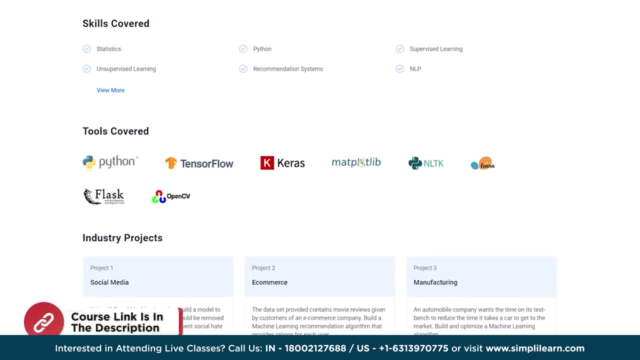 ensure top-notch education simply learns: job assist. help you get noticed by leading companies. this program covers python, supervised and supervised learning, nlp, neural networks, computer visions, gans, keras, tensorflow and many more other skills. so enroll now and unlock exciting ai and ml opportunities. the link is in the description box below, so without any further delay, let's get started. 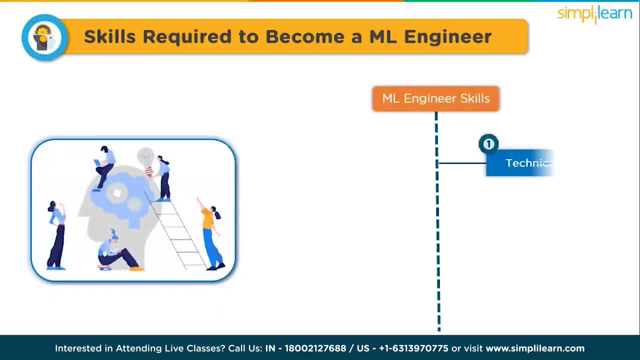 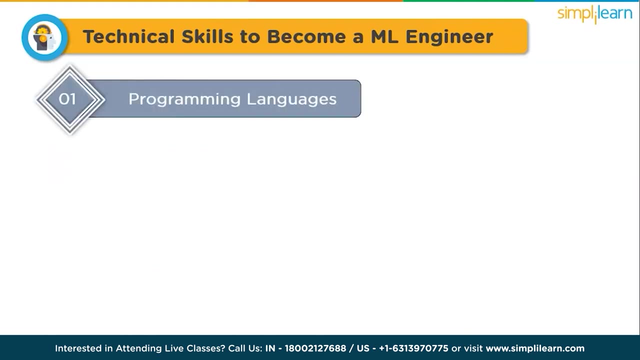 to become a machine learning engineer you need a combination of technical skills, non-technical skills and some bonus skills. so here are some essential skills required to pursue a career as an ml engineer. so first we will talk about some technical skills to become a ml engineer. so first one in the list is programming languages. strong programming skills are 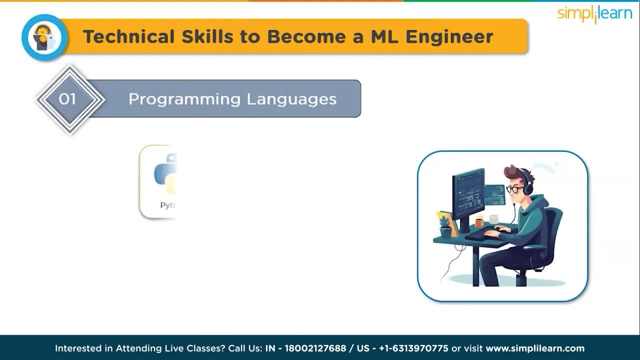 essential. you should be proficient in at least one programming languages, such as python or r. python is widely used in the ml community due to its rich libraries, that is, numpy, pandas, tensorflow and pytorch. that supports ml tasks, and the second on the list is machine learning algorithms and techniques. you should have a solid understanding of various ml algorithms, such 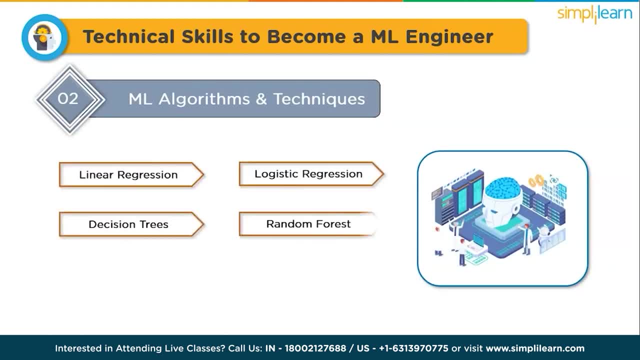 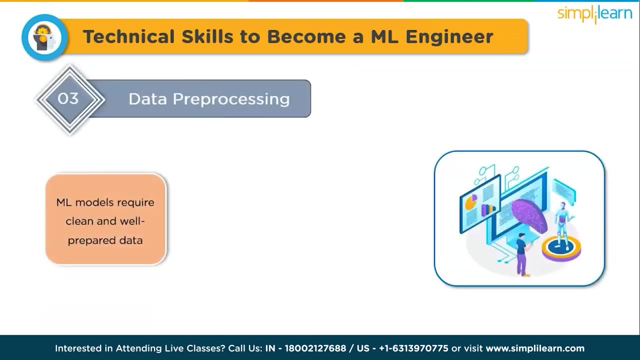 as linear regression, logistic regression, decision trees, random forest neural network and deep learning. familiarize yourself with the principles behind these algorithms, their pros and cons and when to use them. so third one on the list is data pre-processing. ml models require clean and well prepared data. you should know. 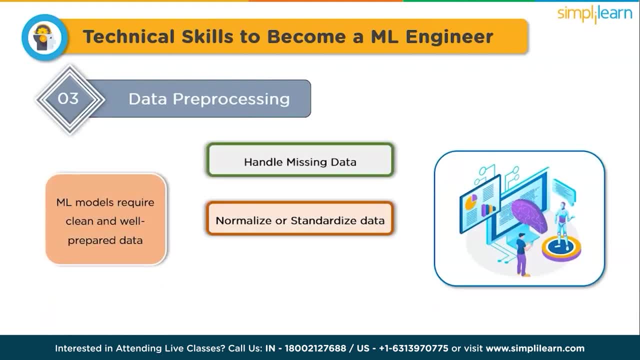 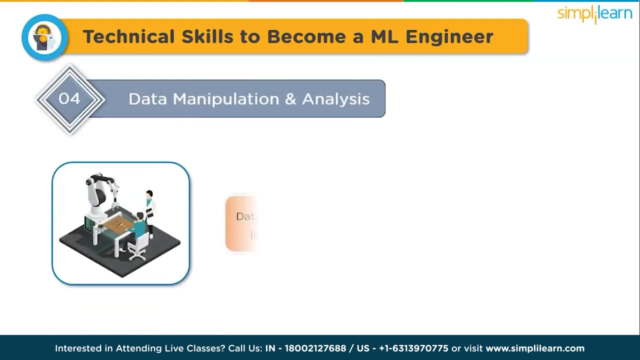 how to handle missing data, deal with normalized and standardized data and the final is perform feature engineering. understanding data pre-processing technique is crucial for effective ml model training. and the fourth one is data manipulation and analysis. data is the foundation of ml model. you should be skilled in the data manipulation and analysis using libraries like 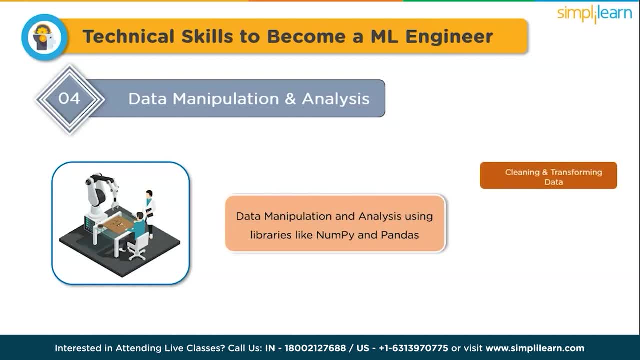 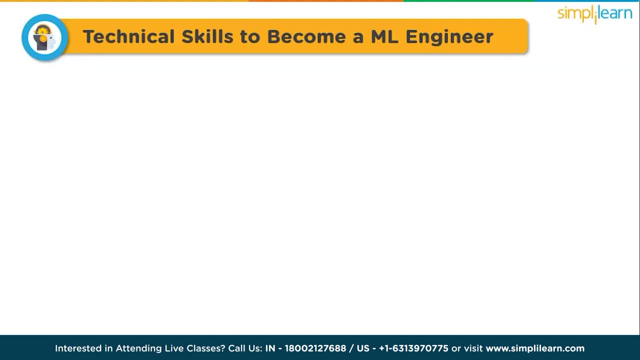 numpy and pandas. this includes cleaning and transforming data, exploratory data analysis, which is eda, and understanding the statistics of the data. and the fifth one is machine learning libraries and frameworks. familiarity with popular ml libraries and framework is essential. some some commonly used one include numpy, pandas, tensorflow. 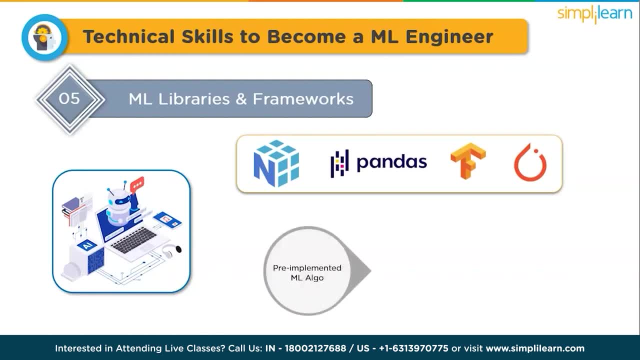 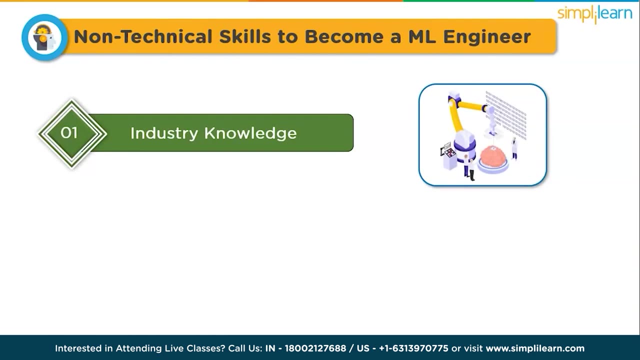 and python. these library provide pre-implemented ml algorithms, neural network architectures and tools for model training and evaluation. now that we have seen the technical machine learning engineering skills, let us have a look at the non-technical machine learning skills. so the first machine learning projects that effectively tackle genuine challenges are likely to achieve great 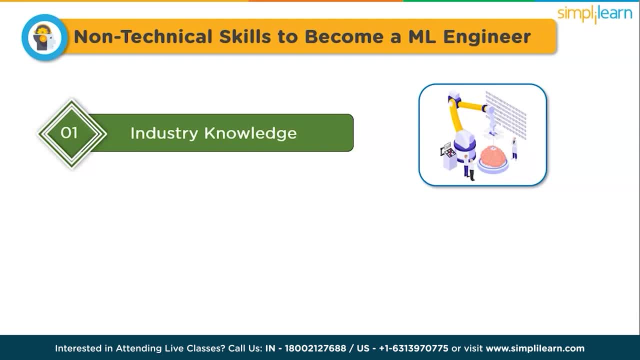 success. regardless of the industry you are involved in, it is crucial to have a comprehensive understanding of its operation and identify ways to optimize business outcomes. and the second one on the list is effective communication. effective communication plays a crucial role in facilitating these interactions. companies seeking skilled ml engineer value candidates who can effectively 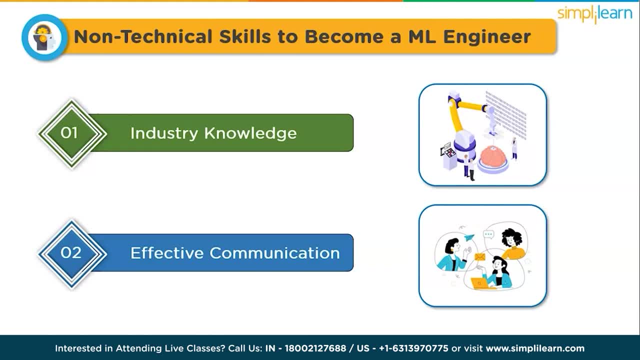 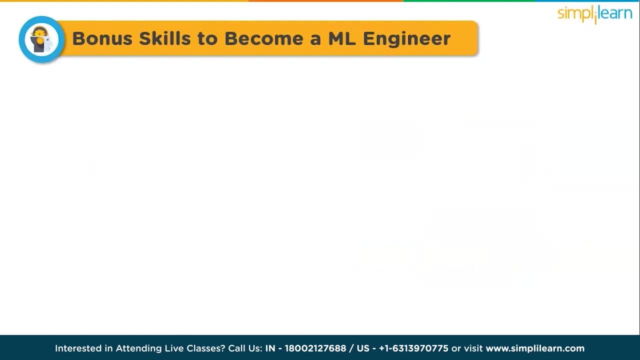 convey technical discoveries to non-technical terms like marketing or sales, demonstrating clarity and fluency in their explanation. moving forward, let's see some bonus skills to become a ml engineer. the first one on the list is reinforcement learning. in 2023, reinforcement learning emerged as a catalyst for numerous captivating advancement in deep learning. 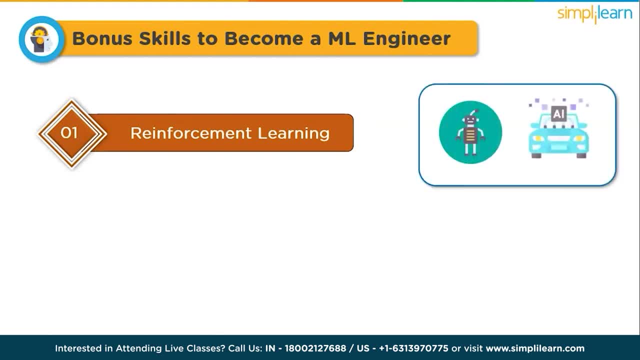 and artificial intelligence to pursue a career in robotics, self-driving cars or any other ai related field. it is crucial to comprehend this concept. and the second on the list is computer vision. computer vision and machine learning are fundamental computer science that can independently fuel highly advanced system relying on cv and ml algorithm. 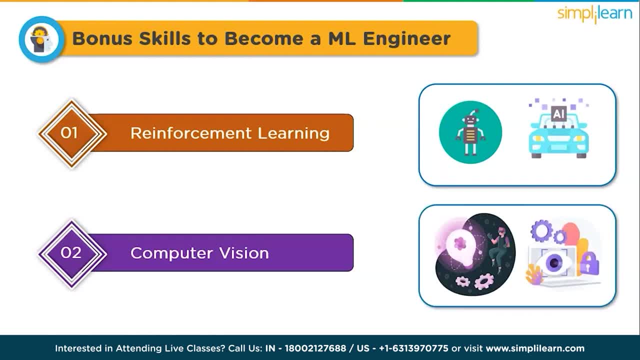 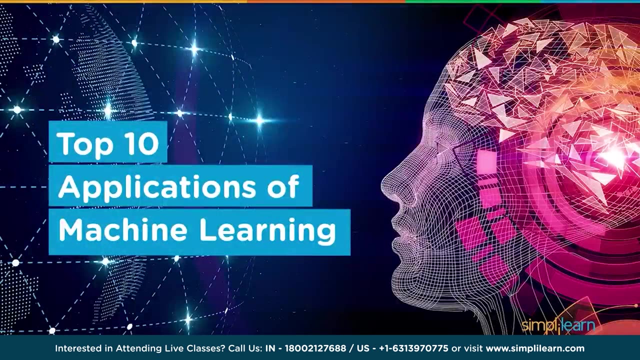 however, the combination has a potential to unlock the greater even possibilities and achievements. so remember that the field of ml is constantly evolving, so continuous learning and staying updated with the latest development and the research papers are essential to be the practical. machine learning has improved our lives in a number of wonderful ways. today let's talk about 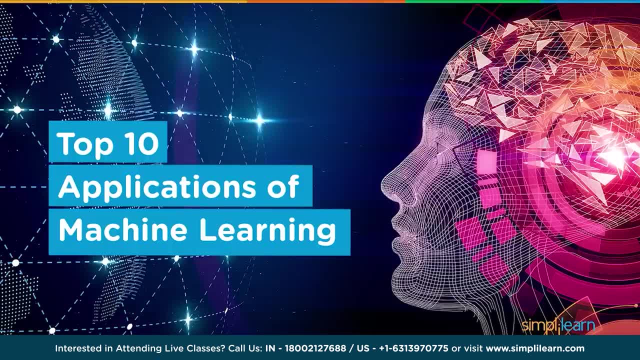 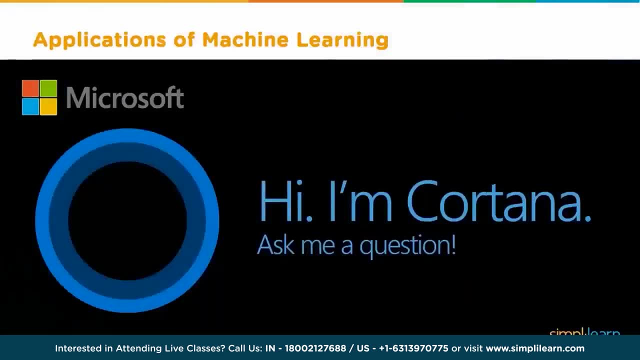 some of these i'm rahul from simply learn, and today we are going to talk about some of these. i'm rahul, and these are the top 10 applications of machine learning. first, let's talk about virtual personal assistants: google assistant, alexa cortana and siri. now, we've all used one of these, at least at some. 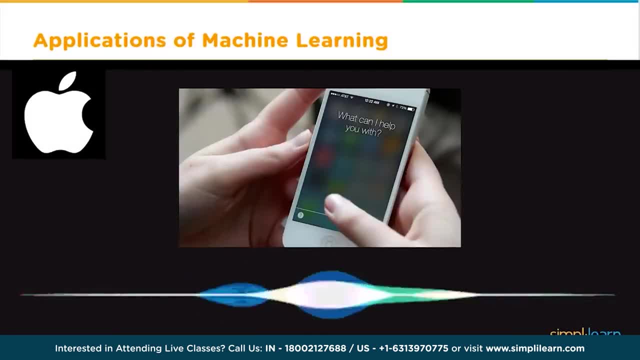 point in our lives. now. these help improve our lives in a great number of ways. for example, you could tell them to call someone, you could tell them to play some music. you could tell them to even schedule an appointment. so how do these things actually work? first, they record whatever you're. 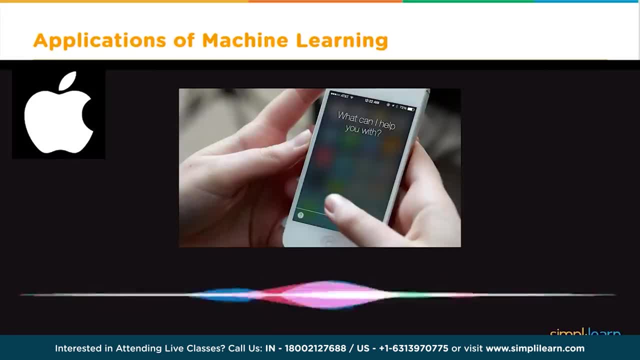 saying: send it over to a server which is usually in a cloud, decode it with the help of machine, then provide you with an output. so if you ever notice that these systems don't work very well without the internet, that's because the server couldn't be contacted. next let's talk about 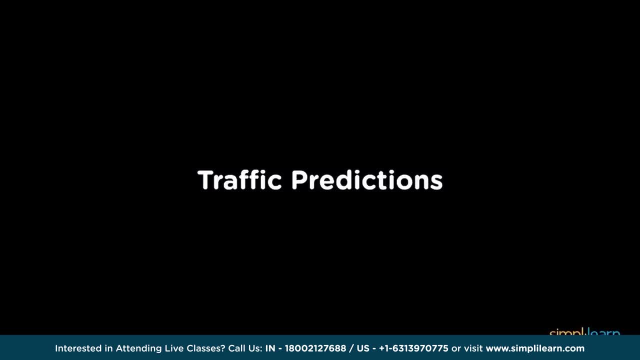 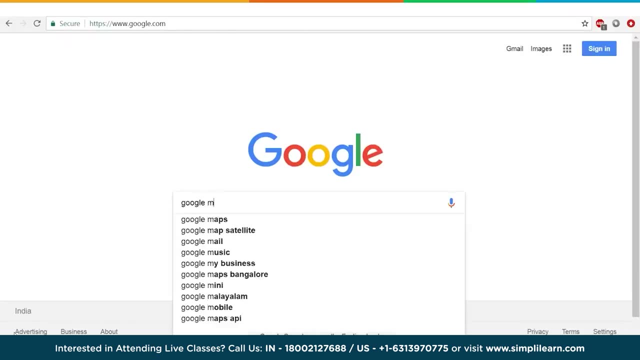 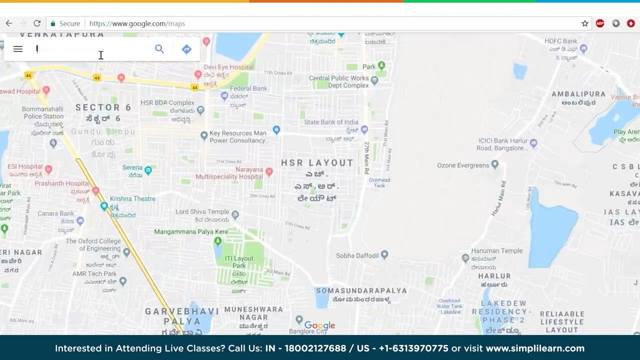 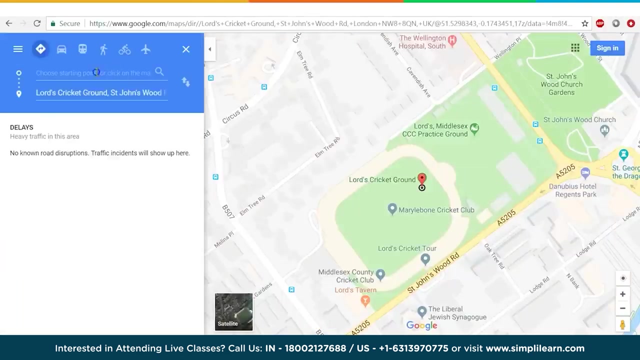 traffic predictions now say i wanted to travel from buckingham palace to lord's cricket ground, the first thing i would probably do is to get on google maps, so search it and let's put it here. so here we have, the path you should take to get to lord's cricket ground. now, here the map is a. 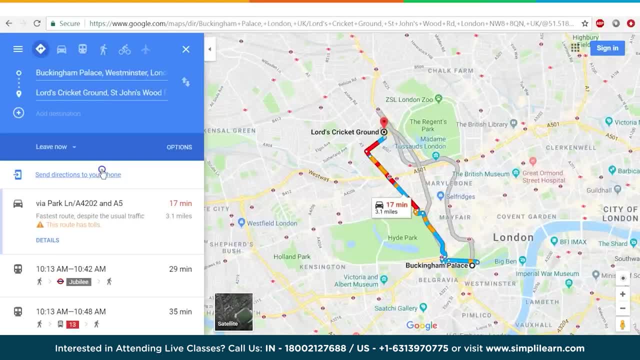 combination of red, yellow and blue, but the blue regions signify a clear road, that is, you won't encounter traffic there. yellow indicate that they are slightly congested and red means they're heavily congested. so let's look at the map- a different version of the same map- and here as i 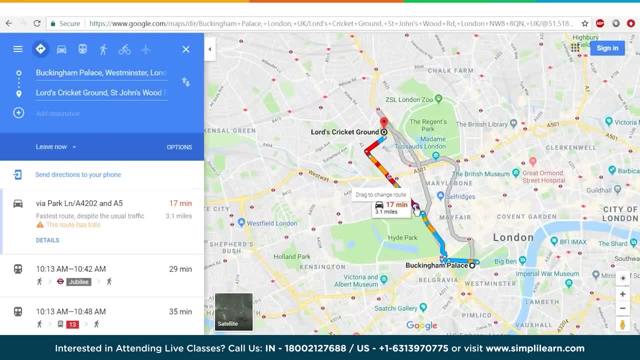 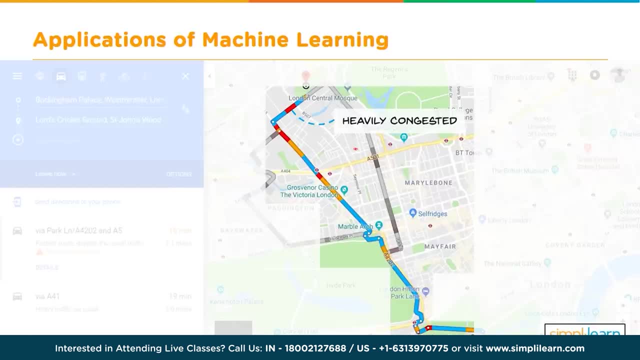 said earlier, the map is a combination of red, yellow and blue, but the blue regions signify a clear road, that is, you won't encounter traffic there. the yellow indicate that they are slightly congested. so here, as i told you before, red means heavily congested, yellow means slow moving and 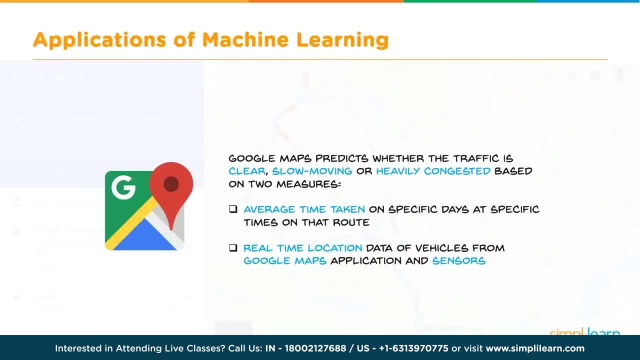 blue means clear, so how exactly is google able to tell you that the traffic is clear, slow moving or heavily congested? so this is with the help of machine learning and with the help of two important measures. first is the average time that's taken on specific days at specific times. 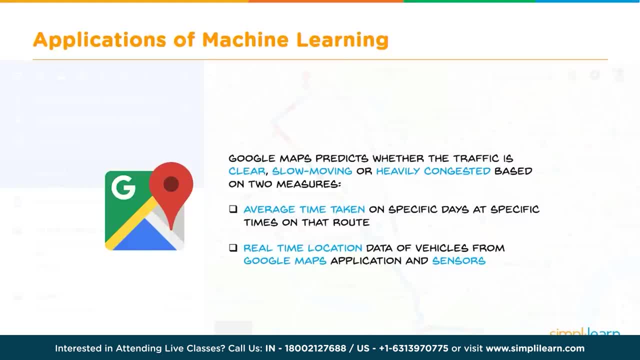 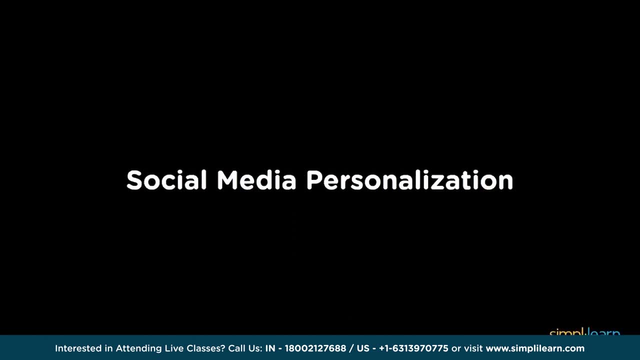 on that route. the second one is the real-time location data of vehicles from google maps and with the help of sensors. some of the other popular map services are bing maps, mapsme, and here we go. next up, we have social media personalization. so, say, i want to buy a drone and i'm on amazon, and 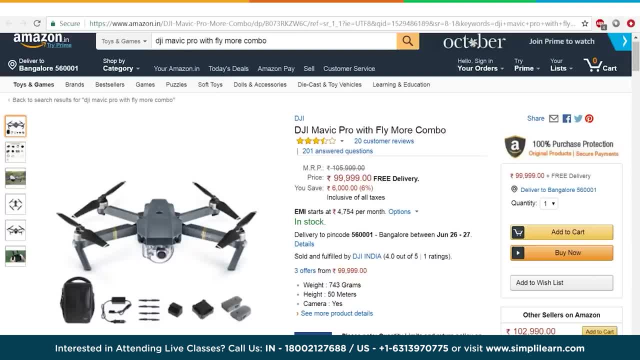 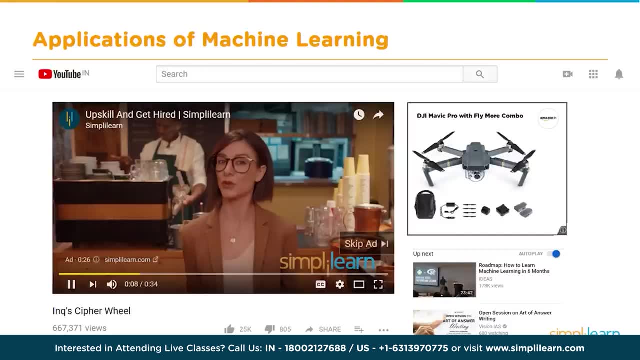 i want to buy a dji mavic pro. the thing is it's close to one lab, so i don't want to buy it right now, but the next time i'm on facebook i'll see an advertisement for the product. next time i'm on youtube, i'll see an advertisement. even on instagram i'll see an advertisement. so here, with the help of 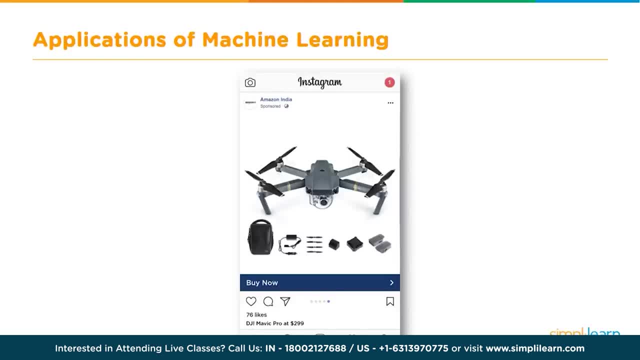 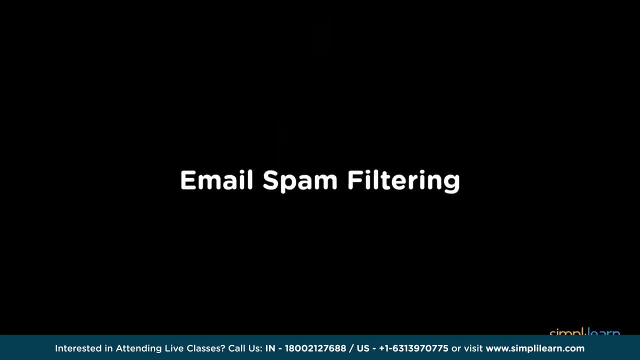 machine learning, google has understood that i'm interested in this particular product. hence it's targeting me with these advertisements. this is also with the help of machine learning. let's talk now. this is a spam that's in my inbox now. how does gmail know what spam and what's not spam? so 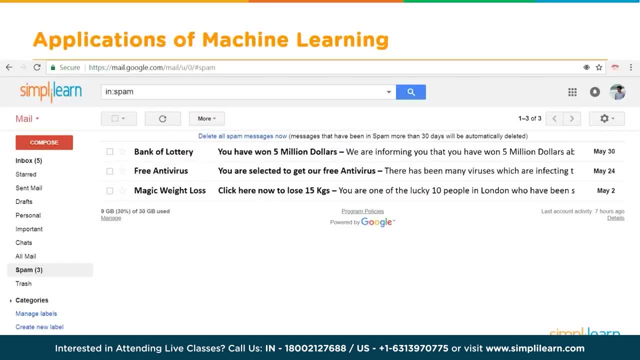 gmail has an entire collection of emails which have already been labeled as spam or not spam, so after analyzing this data, gmail is able to find some characteristics like the word lottery or winner. from then on, any new email that comes to your inbox goes through a few spam filters. 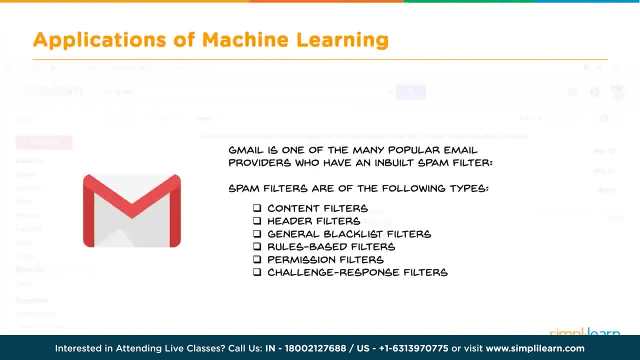 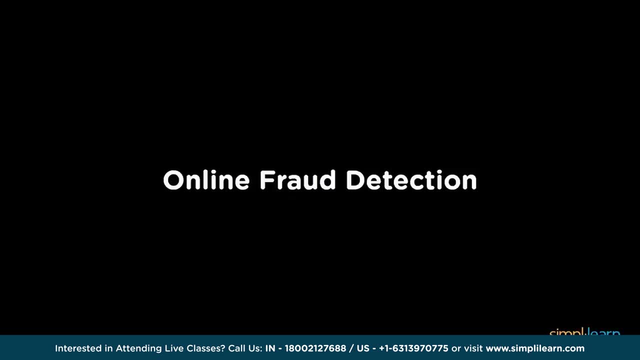 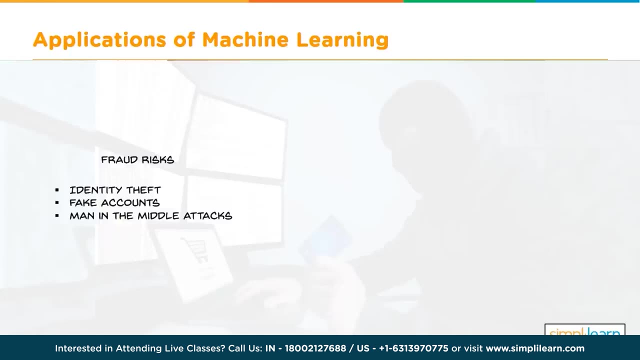 to decide whether it's spam or not. now, some of the popular spam filters that gmail uses is content filters, header filters, general blacklist filters and so on. we have online fraud detection. now there are several ways that online fraud can take place. for example, there's identity theft, where they steal your identity. fake accounts, where these 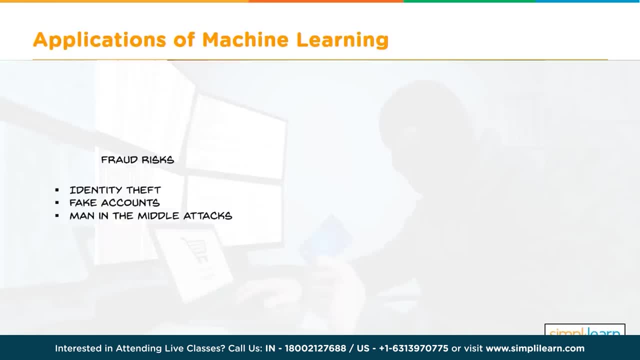 accounts only last for how long the transaction takes place and stop existing after that. and man in the middle attacks where they steal your money while the transaction is taking place. the feed forward neural network helps determine whether a transaction is genuine or fraudulent. so what happens with feed forward neural networks are that the outputs are converted into hash. 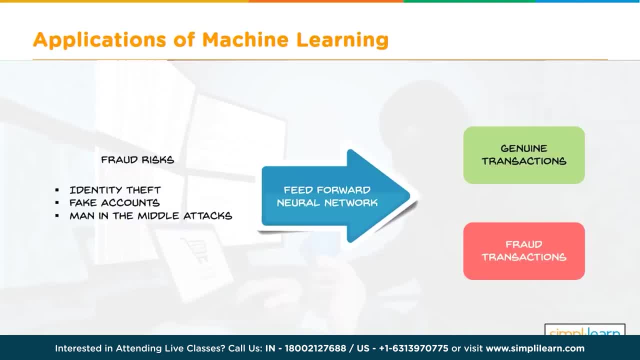 values, and these values become the inputs for the next round. so for every real transaction that takes place, there's a specific pattern. a fraudulent transaction would stand out because of the significant changes that it would cause with the hash values. stock market trading. machine learning is used extensively when it comes to stock market trading. 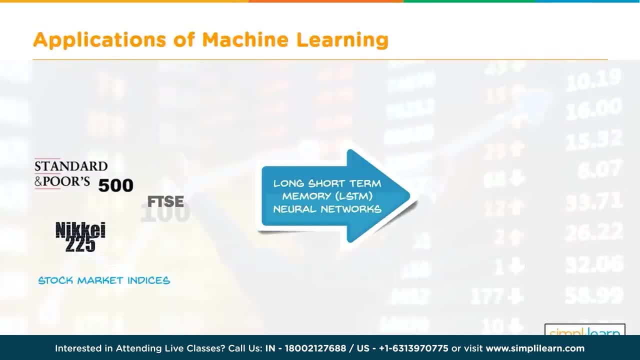 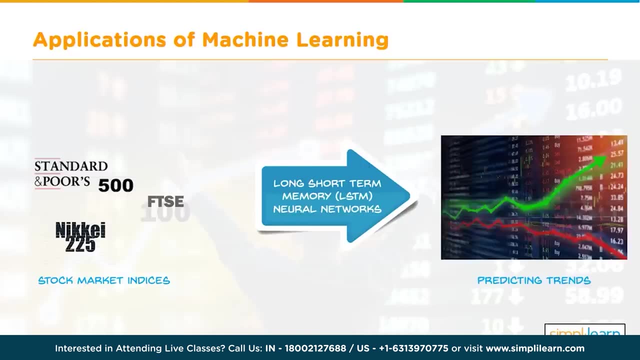 now you have stock market indices like nikai. they use long short-term memory neural networks. now these are used to classify, process and predict data when there are time lags of unknown size and duration. now this is used to predict stock market trends. assistive medical technology: now. 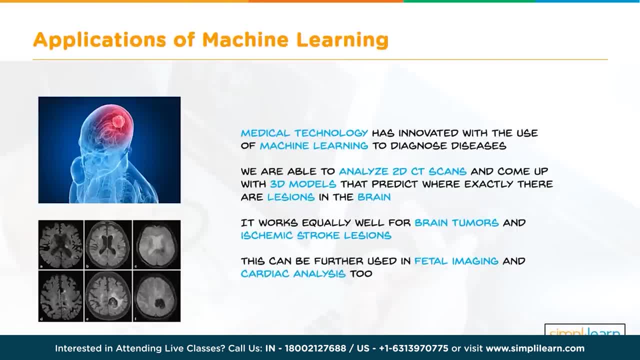 medical technology has been innovated. with the help of medical technology, we've been able to use machine learning. diagnosing diseases has been easier, from which we can create 3d models that can predict where exactly there are lesions in the brain. it works just as well for brain tumors. 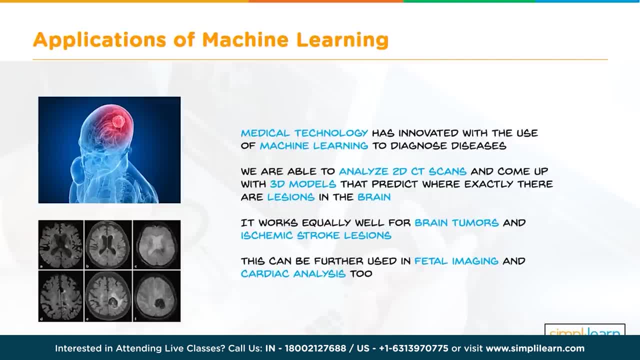 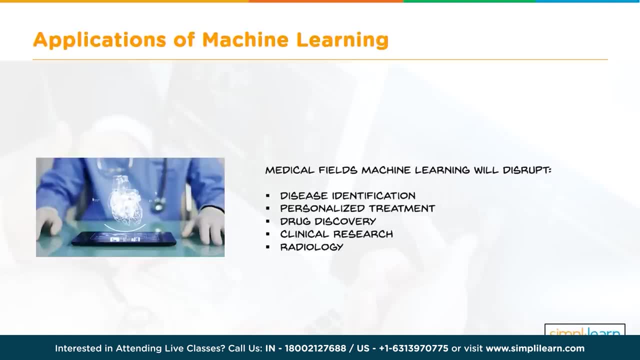 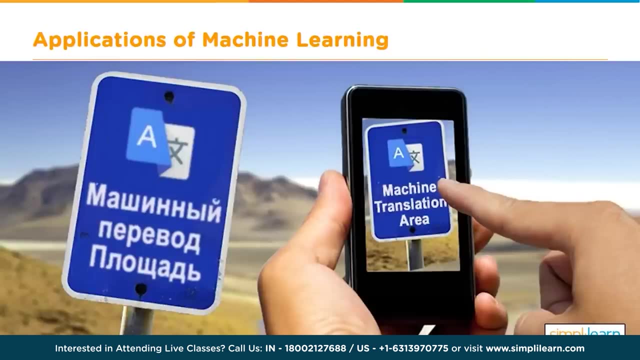 and ischemic stroke lesions. they can also be used in fetal imaging and cardiac analysis. now, some of the medical fields that machine learning will help assist in is disease identification, personalized treatment, drug discovery, clinical research and radiology, and finally, we have automatic translation. now say: you're in a foreign country and you see billboards. 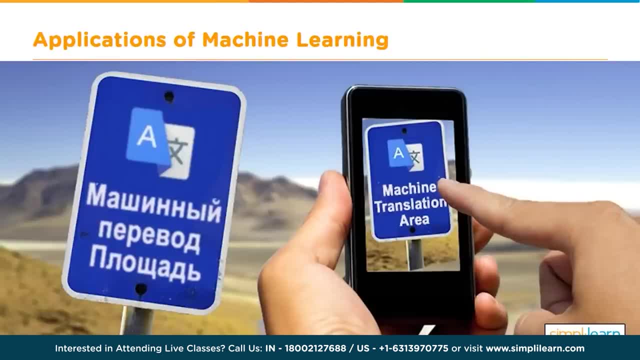 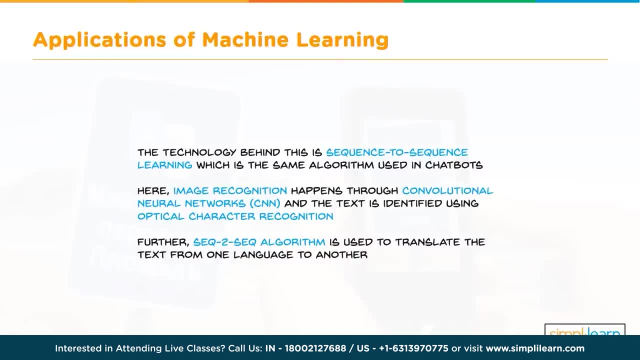 and signs that you don't understand. that's where automatic translation comes of help. now, how does automatic translation actually work? the technology behind it is the same as the sequence of sequence learning, which is the same thing that's used with chatbots. here, the image recognition happens using convolutional neural networks and the text is identified using optical. 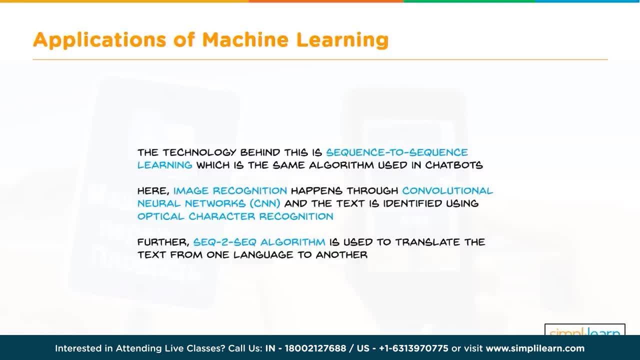 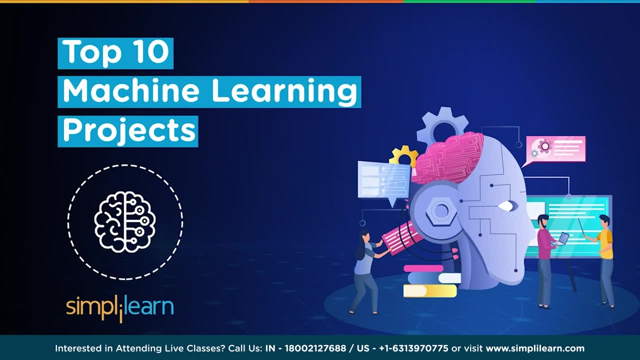 character recognition. furthermore, the sequence sequence algorithm is also used to translate the text from one language to the other. finding a suitable job in the field of machine learning is becoming increasingly difficult. the ideal way to display your machine learning skill is in the form of portfolio of data science and machine learning projects. a solid portfolio of projects. 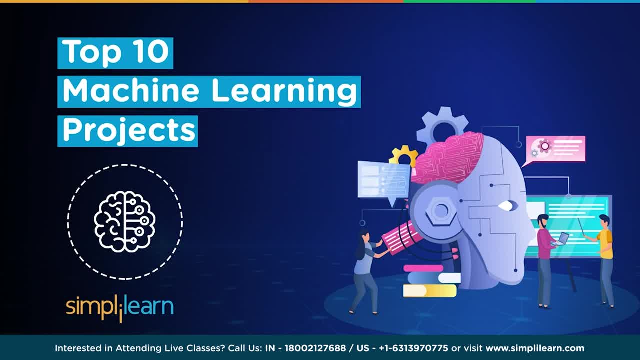 straight that you can utilize those machine learning skills in your profile as well. projects like movie documentation system, fake news detection and many more are the best way to improve your early programming skills. you may have the knowledge, but putting it to the use what is keep you competitive. 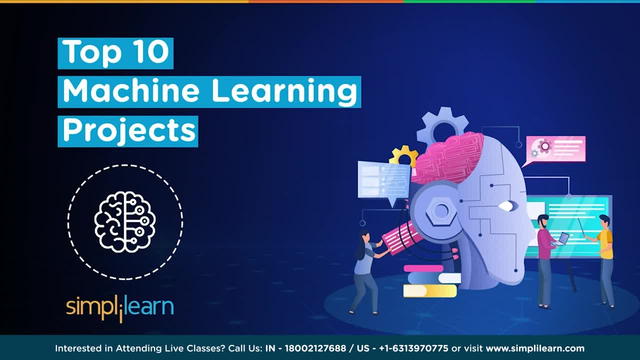 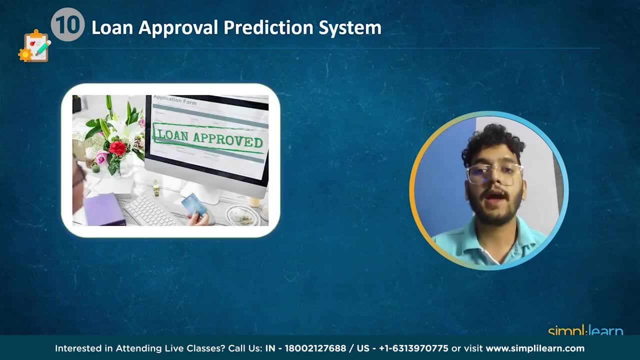 here are 10 machine learning projects that can increase your portfolio and enable you to acquire a job as a machine learning engineer. at number 10, we have loan approval prediction system. in this machine learning project, we will analyze and make prediction about the loan approval process of any person. this is a classification problem in which we must determine the 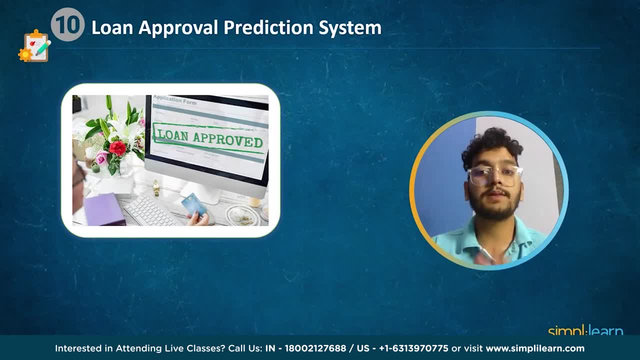 mind whether or not the loan will be approved. a classification problem is a predictive modeling problem that predict a class label for a given example of input data. some classification problem include spam email, cancer detection, sentiment analysis and many more. you can check the project link from the description box below to understand classification problem and how to build a loan. 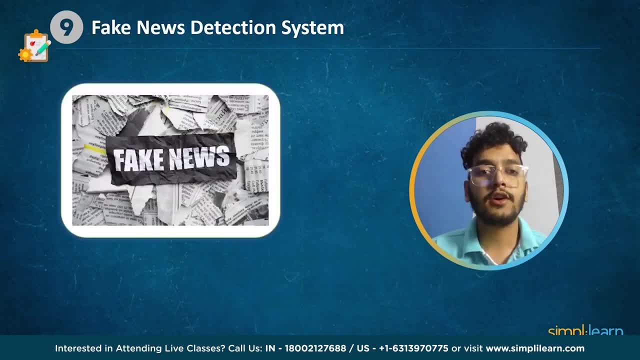 prediction system. at number nine, we have fake news detection system. do you believe in everything you read in social media? isn't it true that not all news is true? but how will you recognize fake news? answer: you will able to tell the difference between real and fake news by practicing this. 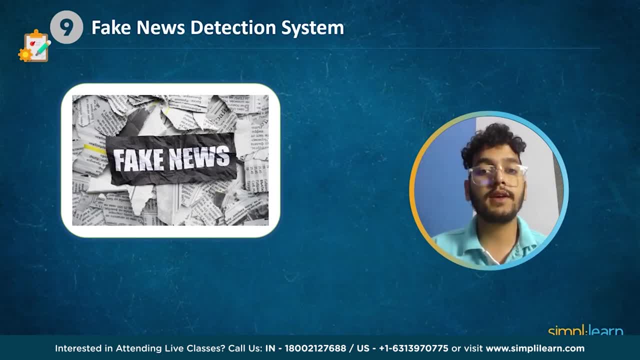 project of detecting face new. this ml project for detecting fake news is concerned with the fake news and the true news on our data set. we create our tf id vectorizer with s killer. the model is then fitted using a passive aggressive classifier that has been initialized. finally, the accuracy. 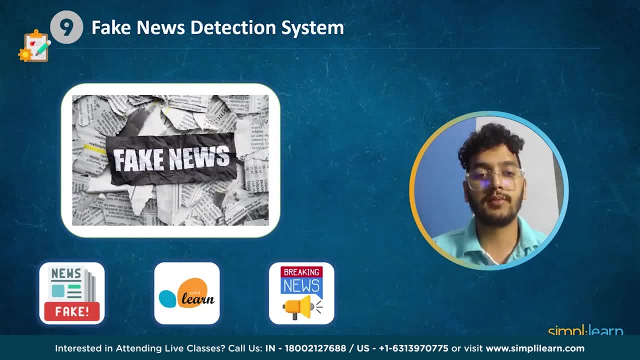 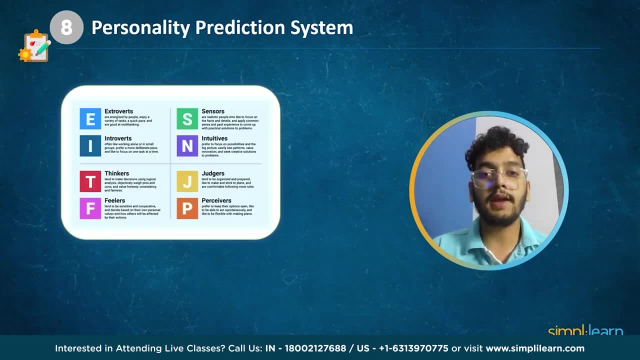 score and the confusion matrix indicate how well our model performs the link for the project in the description box below. at number eight, we have personality prediction system. the idea is based on an individual personality using machine learning techniques. a person personality influences both his personal and professional life. nowadays, many companies are shortlisting applicants. 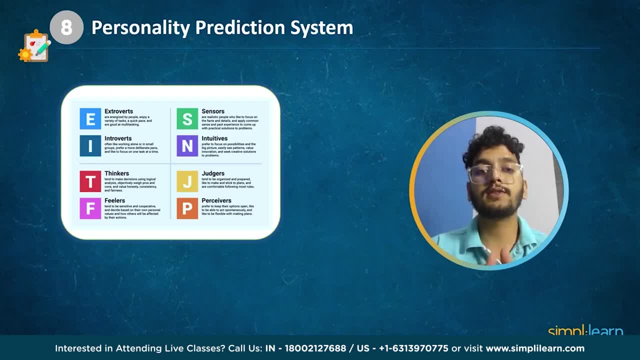 based on their personality, which increases job efficiency because the person is working on what he is good at rather than what is compelled to do. in our study, we attempted to combine personality prediction system using machine learning techniques such as svd name base and logistic regression to predict a person. personality and talent prediction using phrase frequency. 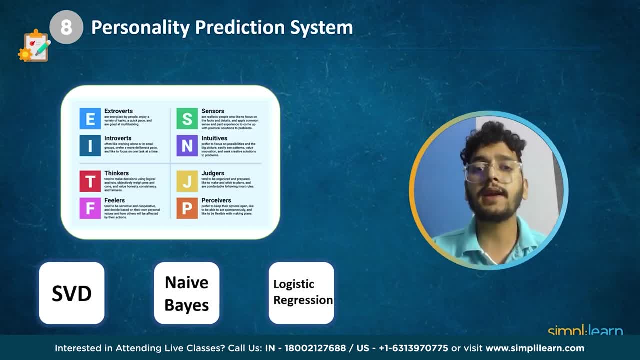 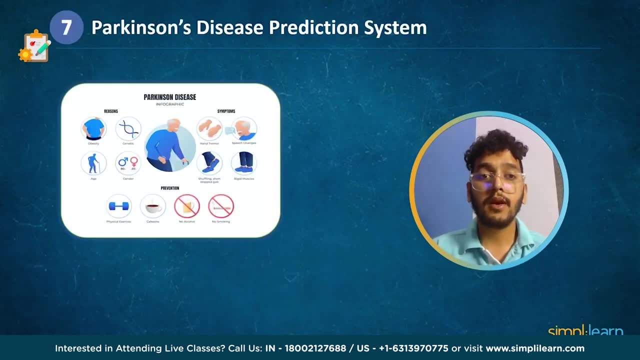 this model or method allow users to recognize their personality and technical abilities easily. to learn about more this project, check the link in the description box below. at number seven we have parkinson disease system. parkinson disease is a progressive central nervous system element that affects movement and cause tremors and stiffness. it comprises five stages and affects 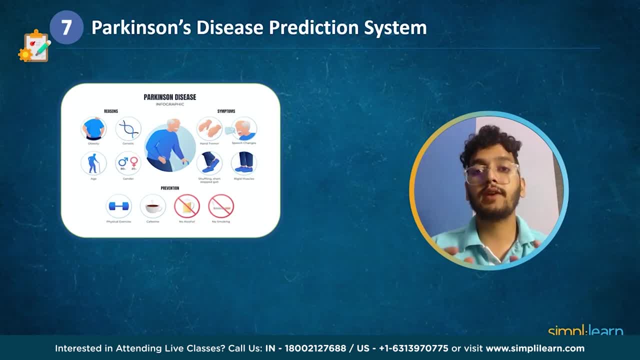 more than one million worldwide each other in this machine learning project we will develop an svm model using python modules, scikit-learn, numpy and pandas and svm. we will import the data, extract the features and label and scale the features, split the data, set, design and influence model and calculate the model accuracy and at the end we will check the parkinson disease. 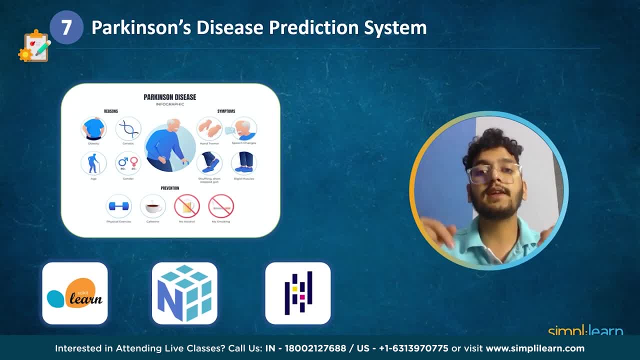 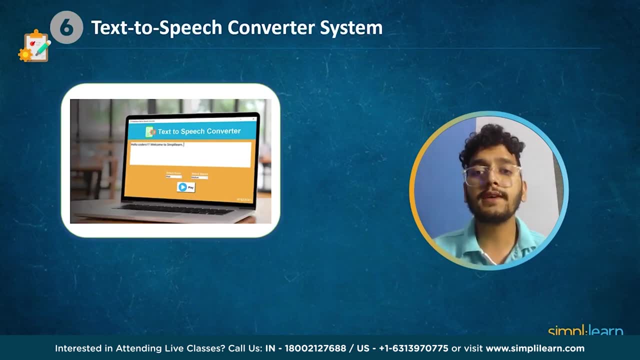 for the individual to learn about more this project, check the link in the description box below. at number six we have text-to-speech converter application. the machine learning domain of audio is undoubtedly cutting as right now the majority of the application available today are the commercial. the community is building several audio specific open source. 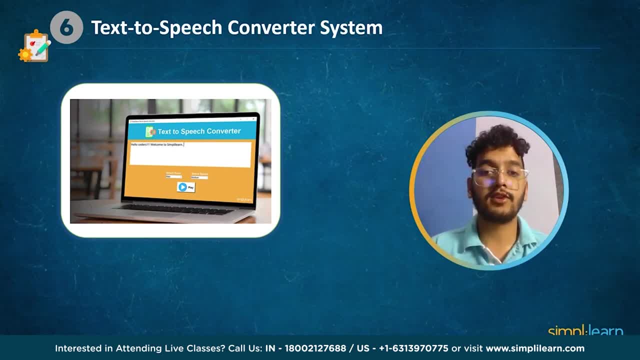 framework and algorithm. other text-to-speech applications are available. for this project we will utilize py ttsx3. py tt ss3 is a python text-to-speech conversion library. it operates offline unlike other libraries and is compatible with python 2 and python 3.. before api, various pre-trained models were accessible in python. 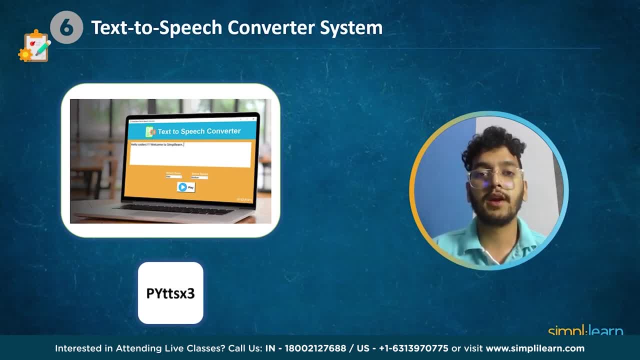 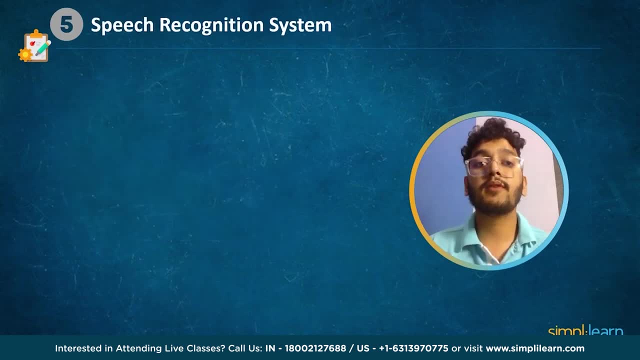 but changing the voice of volume was often difficult. it also needed additional computational power. to learn more about this project, check the link in the description box below. at number five, we have a speech recognition system. speech recognition system is a feature of python. speech recognition, often known as speech to text, is the capacity of a machine or program to 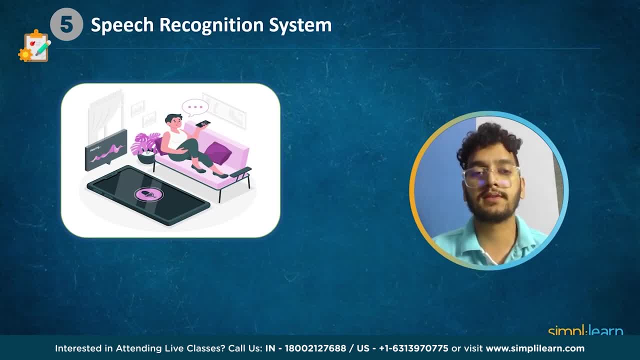 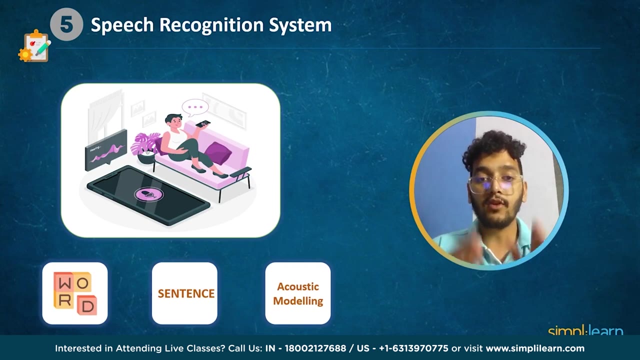 recognize and transfer word spoken aloud into readable text. mls speech recognition uses algorithms that model speech in terms of both language and sound to extract the more important parts of the speech, such as words, sentences, and acoustic modeling is used to identify the phenomes and the phonetics on the speech. for this project, we will utilize py- tt sx3. py- tt- sx3 is a python. 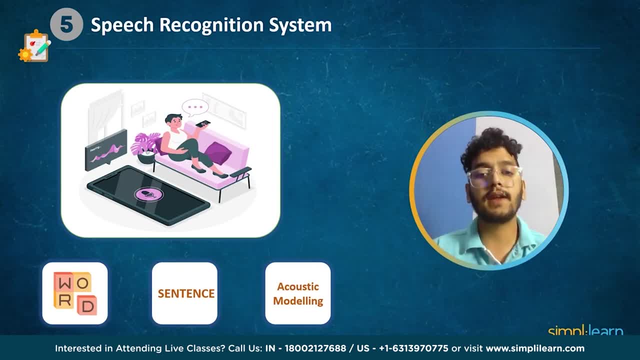 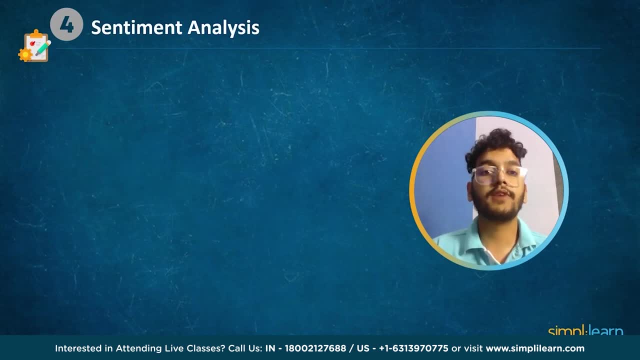 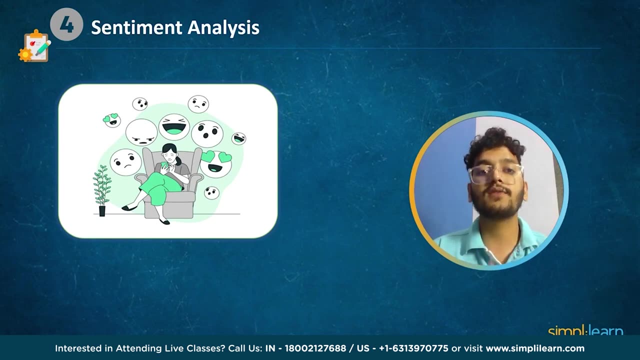 text-to-speech conversion library. it operates offline, unlike other speech recognition systems, and is compatible with python 2 and python 3. to learn more about this project, check the link in the description box below. at number four, we have sentiment analysis. sentiment analysis, also known as opinion mining, is a straightforward process of determining the author's feeling about a text. what 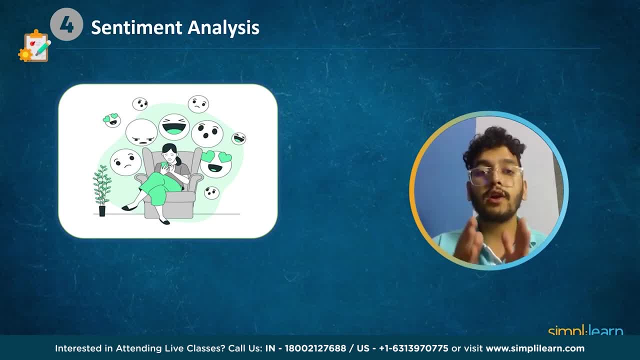 was the user intention when he or she wrote something. to determine what could be personal information, we employ a variety of natural language processing and text analysis technology. we must detect, extract and quantify such information from the text to enable classification. In this project we will use the Amazon customer review dataset for the sentiment analysis. 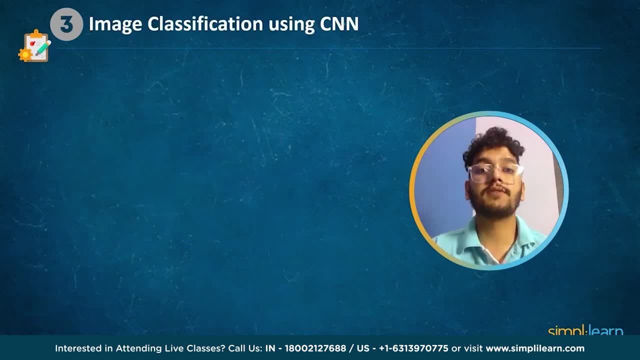 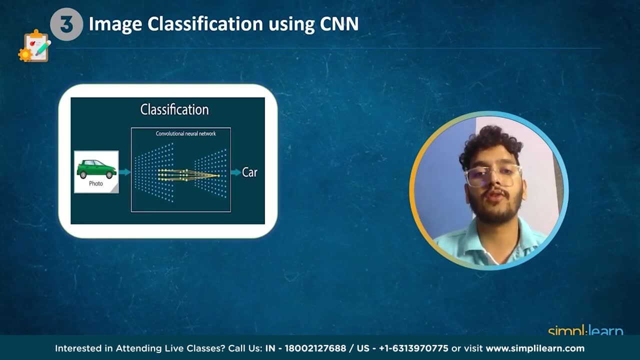 Check the link in the description box below. At number 3, we have image classification using CNN. Deep learning is a booming field. currently, Most projects and problem statements use deep learning and any sort of work. Many of you, like myself, would choose a conventional neural network as a deep learning technique. 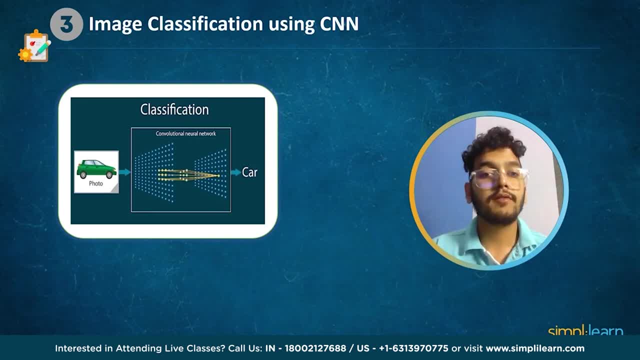 for answering any computer vision problem statement. In this project we will use CNN to develop an image processing project and learn about its capabilities and why it has become so popular. We will go over each stage of creating our CNN model and our first spectacular project. 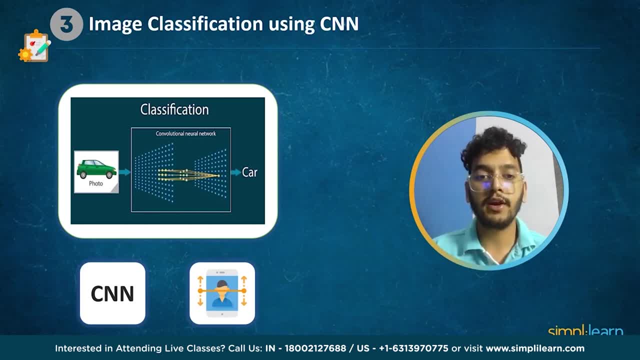 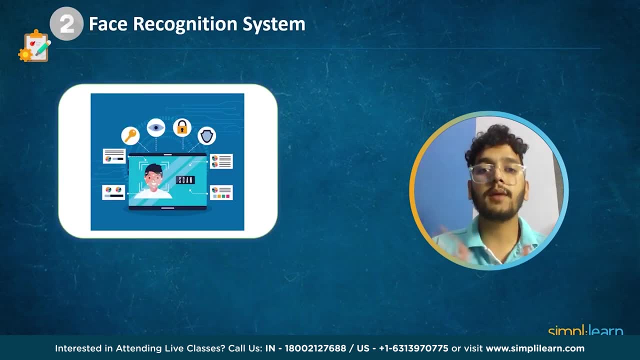 We will use the CFR-10 dataset for image classification in this project. To learn more about this project, check the link in the description box below. At number 2, we have face recognition system. Currently, technology absolutely amazes people with incredible inventions that make life. 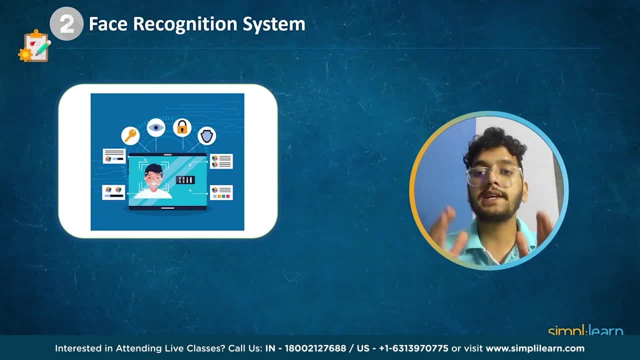 easier and more comfortable. Face recognition has shown to be the least intrusive and fastest form of the biometric verification over time. This project will use OpenCV and face recognition recognition libraries to create a face detection system. opencv provides a real-time computer vision. 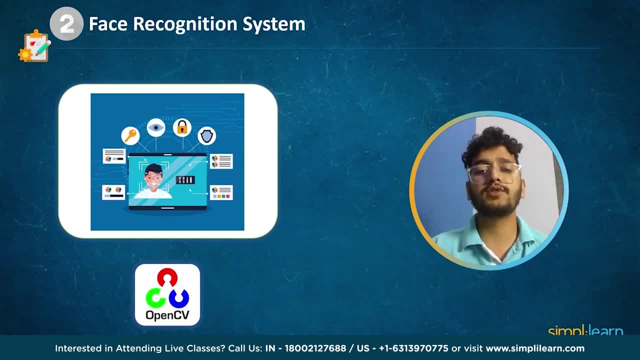 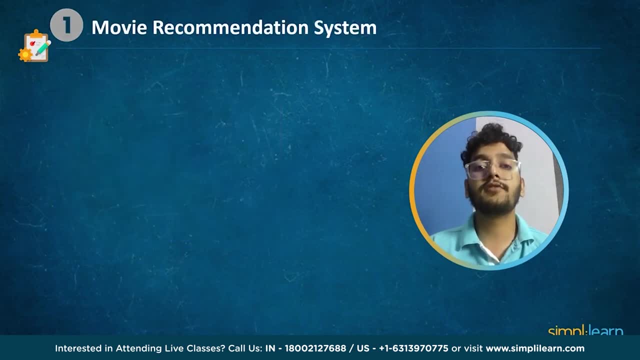 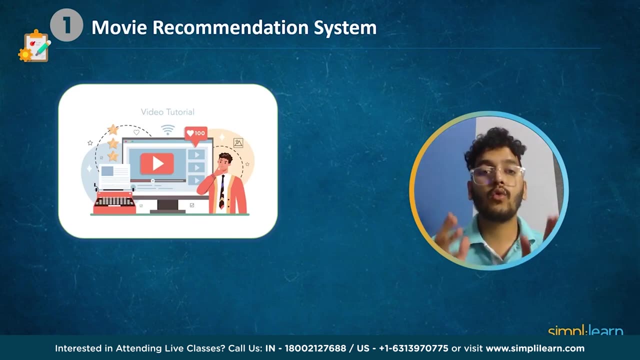 tool library and hardware. we can create amazing real-time projects using opencv. to learn how to create face recognition system for you, check the link in the description box below. and last but not the least, we have movie recommendation system. almost everyone today use technology to stream movies and television show, while figuring out what to stream next can be disheartening. 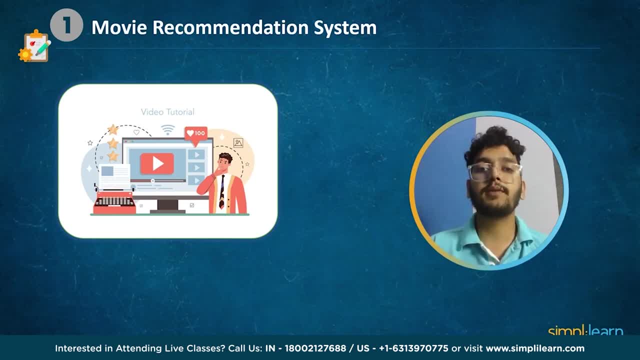 recommendation are often made based on a viewer history and preferences. this is done through a machine learning and can be a fun and the easy project for the beginners. new programmers can practice by coding in either python or r and with the data from the movie lens data set generated. 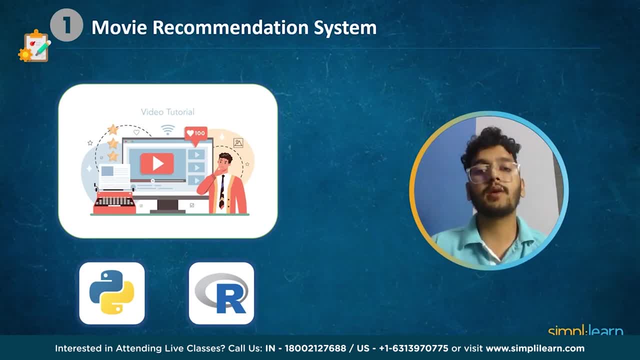 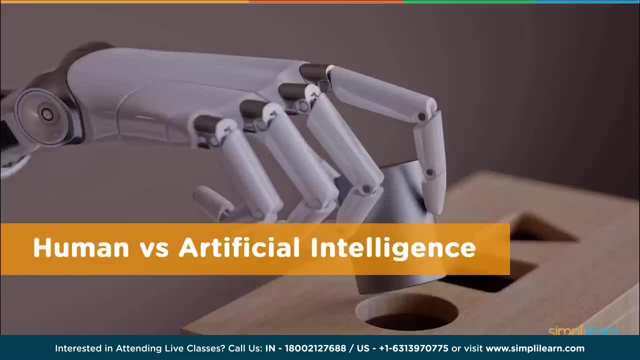 by the more than 6 000 users to learn how to create movie recommendation system for yourself or for your loved ones. check the project in the description box below. human versus artificial intelligence: humans are amazing. let's just face it. we're amazing creatures. we're all over the planet. 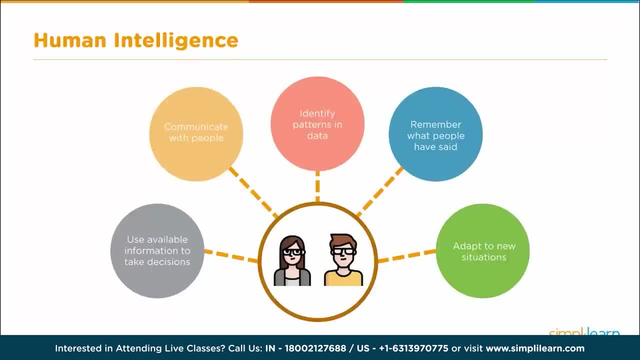 we're exploring every nick chinook. we've gone to the moon, we've gone into outer space. we're just amazing creatures. we're able to use the available information to make decisions, to communicate with other people, identify patterns and data. remember what people have said: adapt to new situations. so let's take. 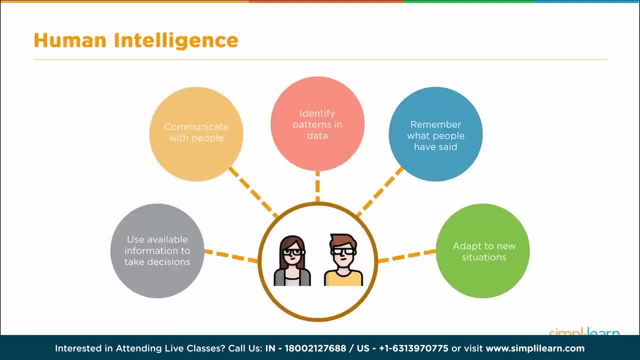 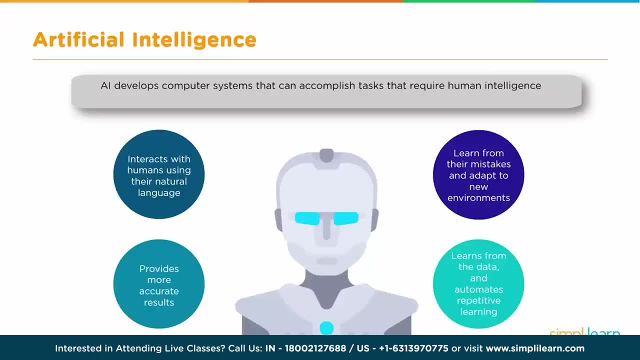 a look at this so you can get a picture. you're a human being, so you know what it's like to be human. let's take a look at artificial intelligence versus the human. artificial intelligence develops computer systems that can accomplish tasks that require human intelligence and artificial intelligence. 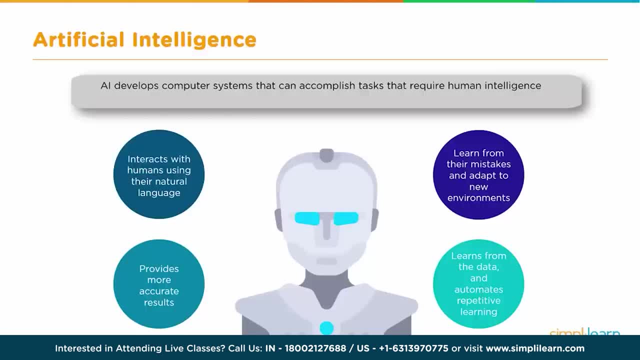 requires human intelligence, so we're looking at this. one of the things that computers can do is they can provide more accurate results. this is very important. recently, i did a project on cancer whereas identifying markers, and, as a human being, you look at that and you might be looking at all the different images. 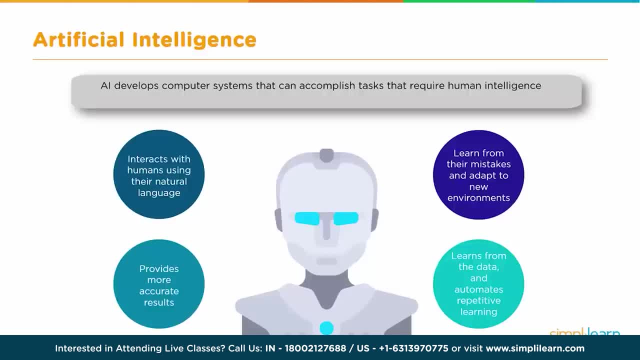 in the data that comes off of them and say: i like this person, so i want to give them a very good um outlook. And the next person you might not like? so you want to give them a bad outlook. Well, with artificial intelligence, you're going to get a consistent prediction of what's going to come out. 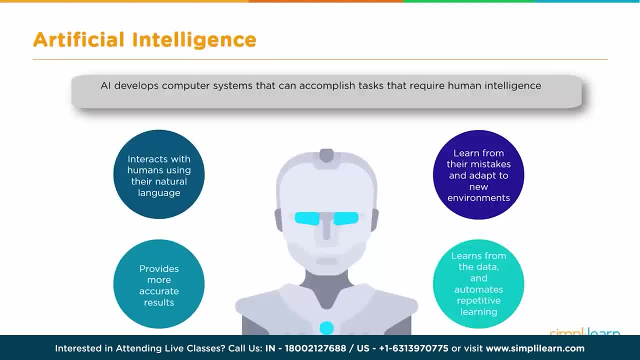 It interacts with humans using their natural language. We've seen that as probably the biggest development feature right now. that's in the commercial market that everybody gets to use. As we saw with the example of Alexa, They learn from their mistakes and adapt to new environments. 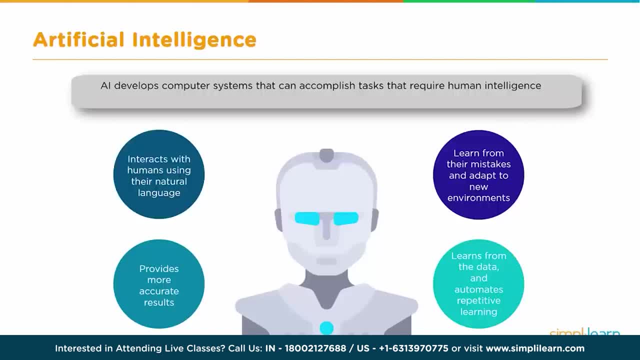 So we see this slowly coming in more and more, And they learn from the data and automate repetitive learning. And repetitive learning has a lot to do with the neural networks. You have to program thousands upon thousands of pictures in there And it's all automated. 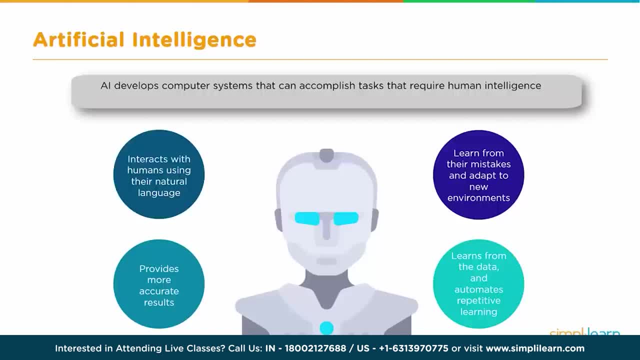 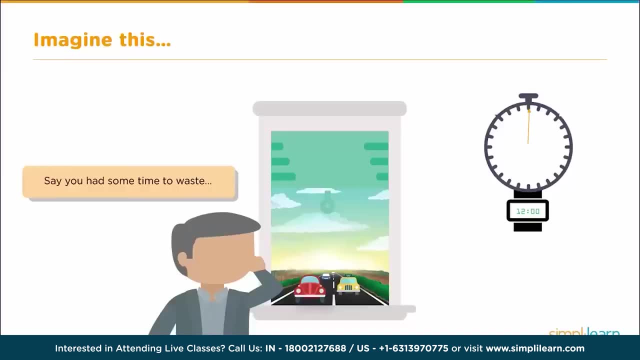 So, as today's computers evolve, it's very quick and easy and affordable to do this. What is machine learning and deep learning all about? Imagine this: Say you had some time to waste- Not that any of us really have a lot of time anymore to just waste in today's world. 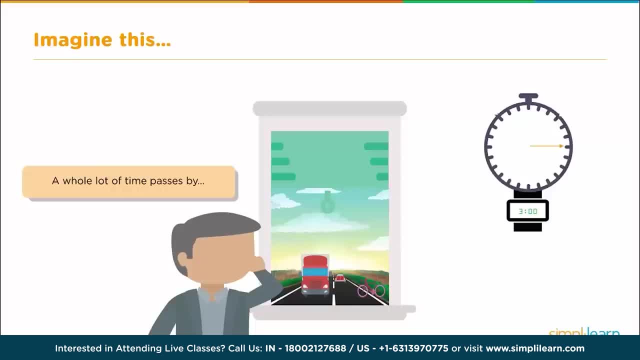 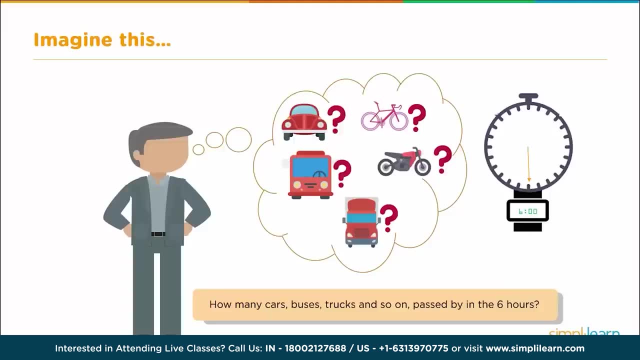 And you're sitting by the road And you have a whole lot of time And a whole lot of time. A whole lot of time passes by. Here's a few hours And suddenly you wonder how many cars, buses, trucks and so on passed by in the six hours. 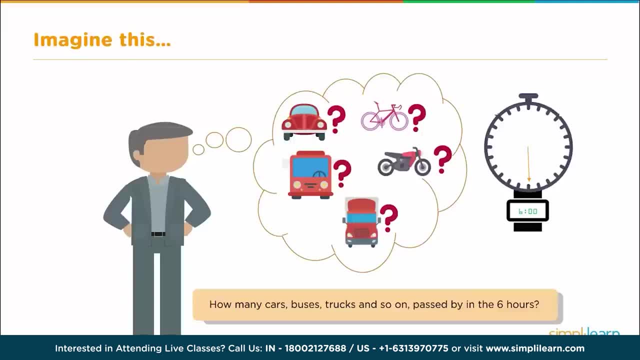 Now, chances are you're not going to sit by the road for six hours and count buses, cars and trucks, Unless you're working for the city and you're trying to do city planning And you want to know: hey, do we need to add a new truck route? 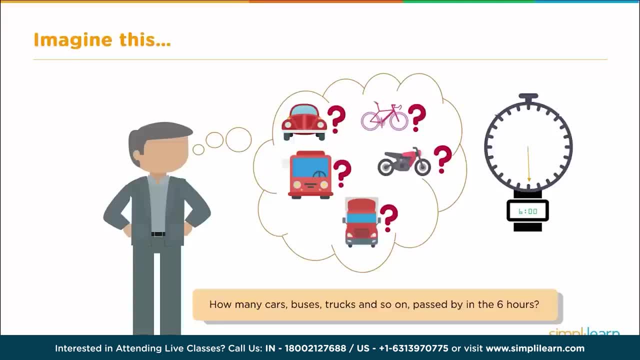 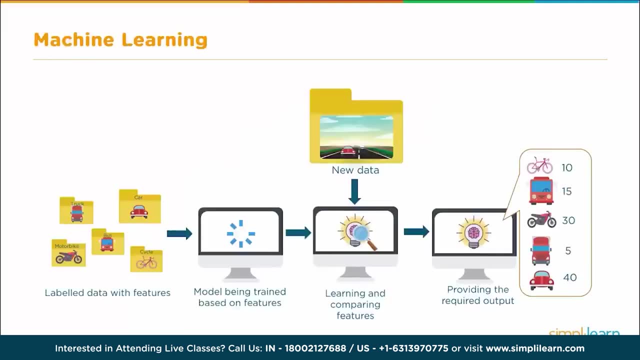 Maybe we need a bicycle lane because we have a lot of bicyclists here, That kind of thing, So maybe city planning would be great for this Machine learning. Well, the way machine learning works. Machine learning works is we have labeled data with features. 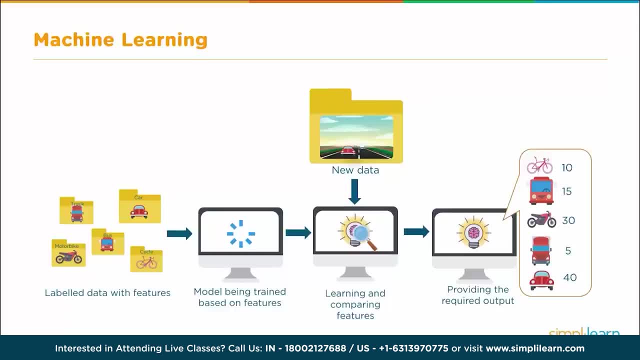 Okay, So you have a truck or a car, a motorcycle, a bus or a bicycle And each one of those are labeled. It comes in And, based on those labels and comparing those features, it gives you an answer: It's a bicycle. 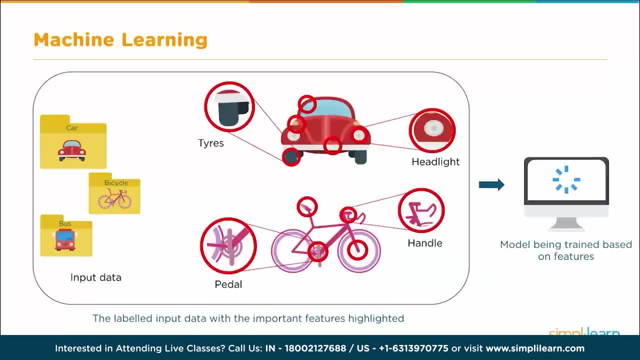 It's a truck, It's a motorcycle. Let's look a little bit more in depth on this. In the model here, it actually the features we're looking at would be like the tires. Someone sits there and figures out What a tire looks like. 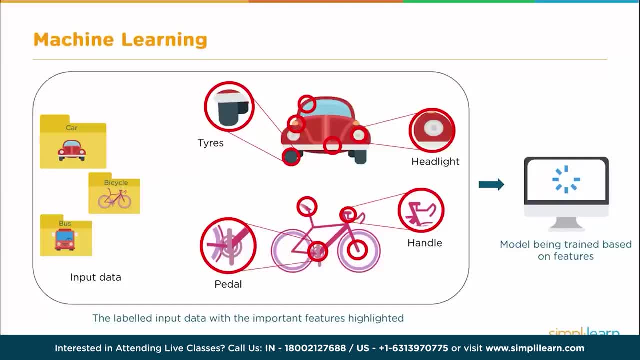 It takes a lot of work If you try to figure the difference between a car tire, a bicycle tire, a motorcycle tire. So in the machine learning field this could take a long time if you're going to do each individual aspect of a car. 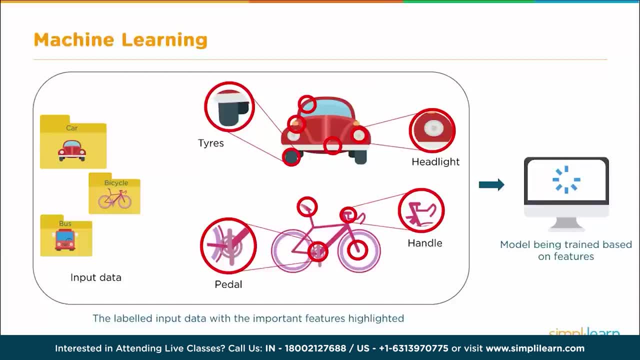 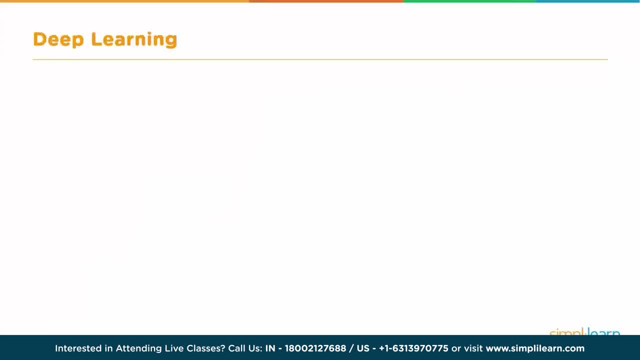 And try to get a result on there, And that's what they did do. This is still used on smaller amounts of data, where you figure out what those features are and then you label them- Deep learning. So with deep learning, One of our solutions is to take a very large unlabeled data set and we put that into a training model using artificial neural networks. 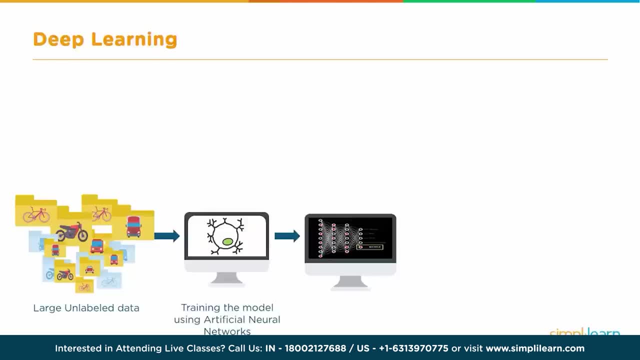 And then that goes into the neural network itself. when we create a neural network and you'll see, the arrows are actually kind of backward, but which actually is a nice point, because when we train the neural network we put the bicycle in and then it comes back and says, if it's a truck? it comes back and says, well, you need to change that to bicycle, and then it changes all those weights, going backward. 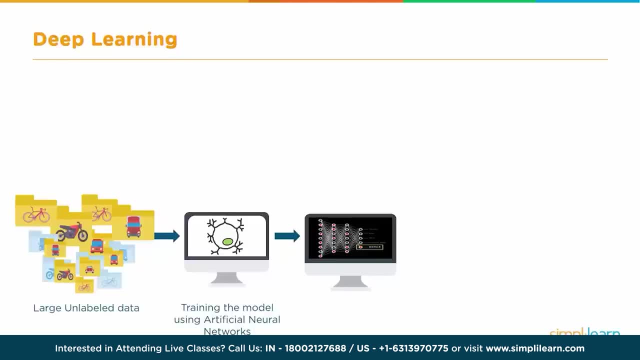 They call it back propagation and let it know it's a bicycle and that's how it learns. Once you've trained the neural network, you then put the new data in and they call this testing the model. So you need to have some data you've kept off to the side where you know the answer to. 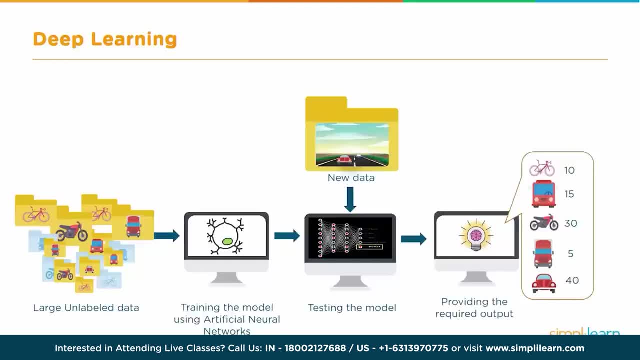 And you take that and you provide the required output and you say, okay, is this? is this neural network working correctly? Did it identify a bike as a bike, a truck as a truck, a motorcycle as a motorcycle? Let's just take a little closer look at that. 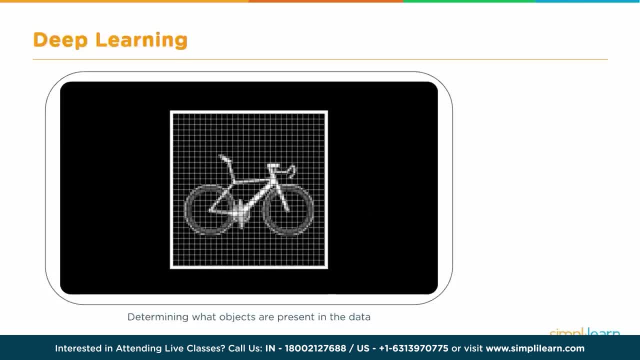 Determining what objects are present in the data. So How does deep learning do this? And here we have the image of the bike. It's 28 by 28 pixels. That's a lot of information there. Could you imagine trying to guess that this is a bicycle image by looking at each one of those pixels and trying to figure out what's around it? 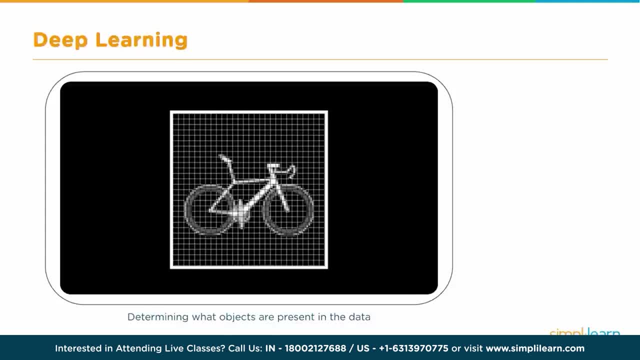 And we actually do that as human beings. It's pretty amazing. We know what a bicycle is And even though it comes in as all this information and what this looks like is the image comes in, it converts it into a bunch of different nodes. 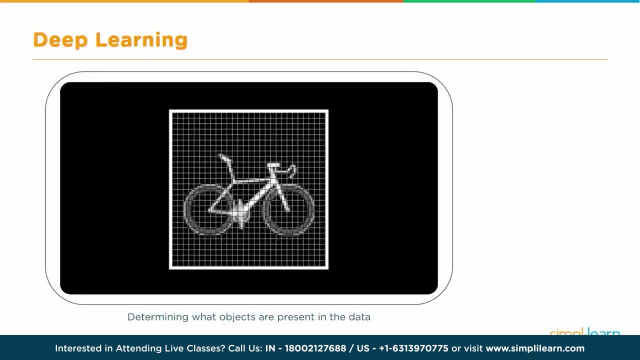 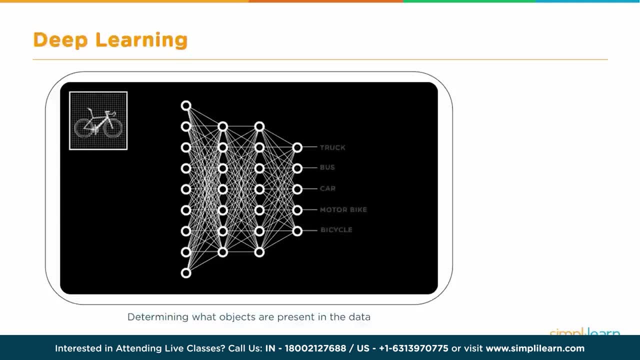 In this case, there's a lot More than what they show here And it goes through these different layers and outcomes. This is okay. This is a bicycle. A lot of times they call this the magic black box. Why? Because as we watch it go across here all these weights and all the math behind this, and it's not. it's a little complicated on the math side. 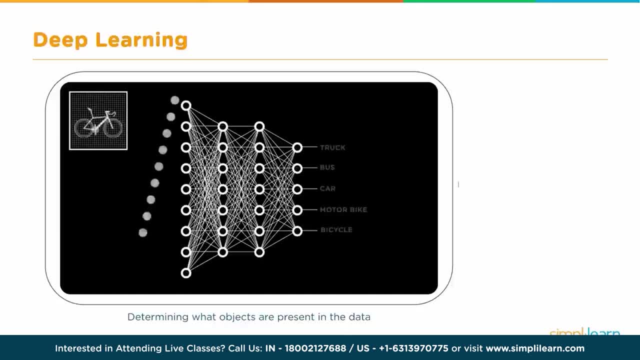 You really don't need to know that when you're programming or doing working with the deep learning. But it's like magic. You don't know. You really can't figure out what's going to come out by looking. what's in each one of those dots and each one of those lines are firing and what's going to come out. 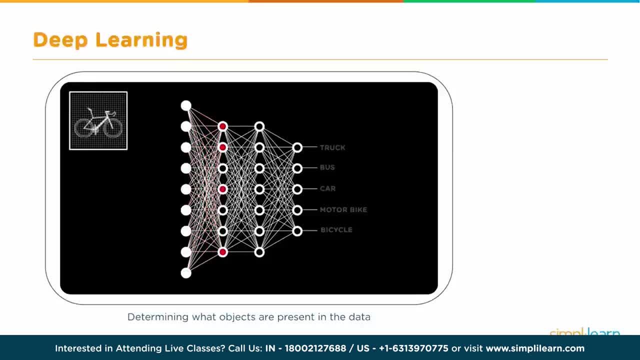 What's going in between them. So we like to call it the magic box. So that's where deep learning comes in. And in the end it comes up and you have this whole neural network comes up and it says, okay, we fire all these different pixels and we connects all these different dots and gives them different weights. 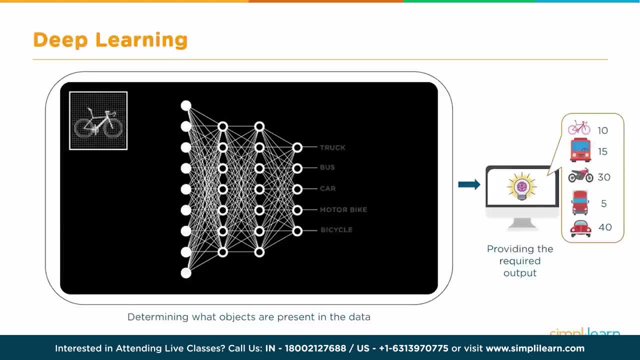 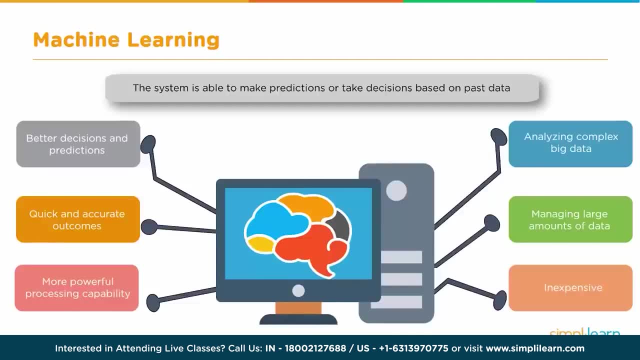 And it says, okay, this is a bicycle, And that's how we determine what the object is present in the data. with deep learning, Machine learning, We're going to take a step into machine learning here and you'll see how these fit together in a minute. 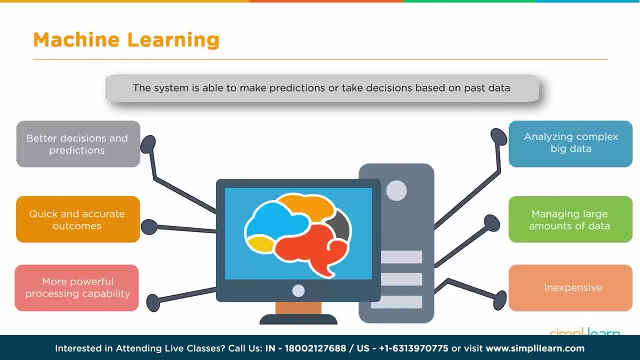 The system is able to make predictions Or take decisions based on past data. That's very important for machine learning is that we're looking at stuff and, based on what's been there before, we're creating a decision on there. We're creating something out of there. 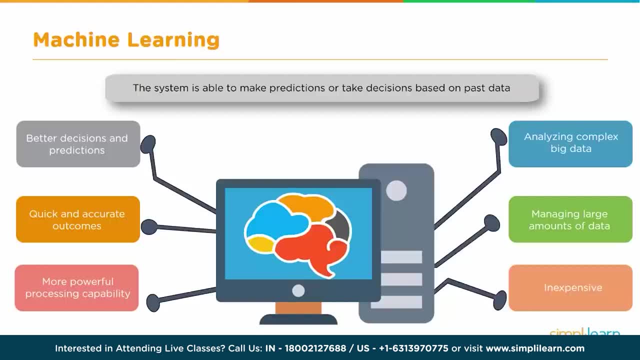 We're coloring a beach ball. We're telling you what the weather is in Chicago. What's nice about machine learning is a very powerful processing capability. It's quick and accurate outcomes, So you get results right away Once you program the system. 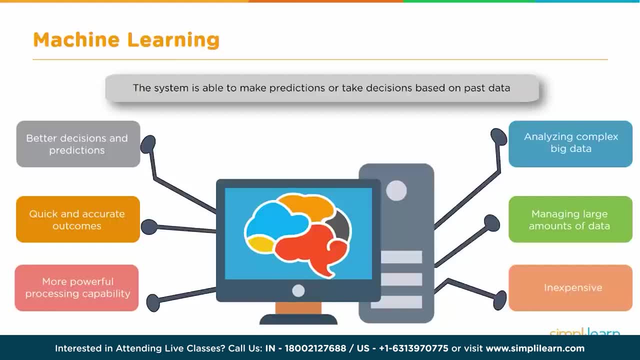 The results are very fast And the decisions and predictions are better. They're more accurate. They're consistent. You can analyze very large amounts of data. Some of these data things that they're analyzing now are petabytes and terabytes of data. 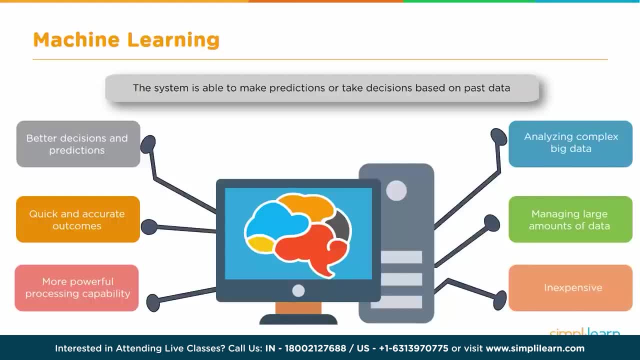 It would take hundreds of people, hundreds of years, to go through some of this data and do the same thing that the machine learning can do in a very short period of time. And it's inexpensive compared to hiring hundreds of people. So because a very affordable way to move into the future. 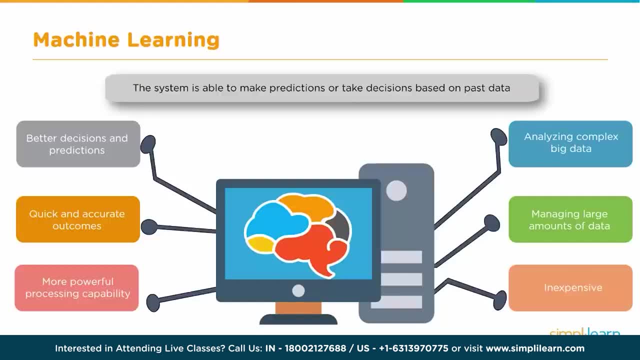 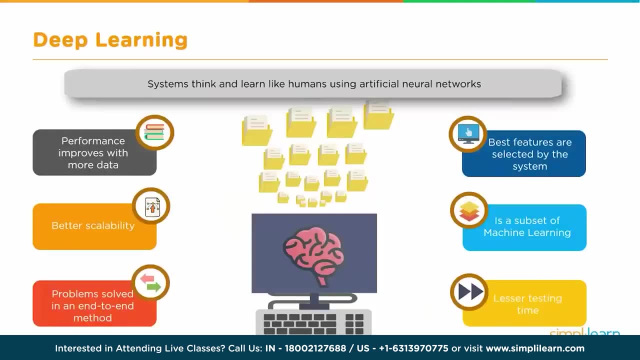 It's very expensive compared to hiring hundreds of people. So because a very affordable way to move into the future. It's very expensive compared to hiring hundreds of people. So because a very affordable way to move into the future As to apply the machine learning to whatever businesses you're working on and deep learning systems think and learn like humans using artificial neural networks. 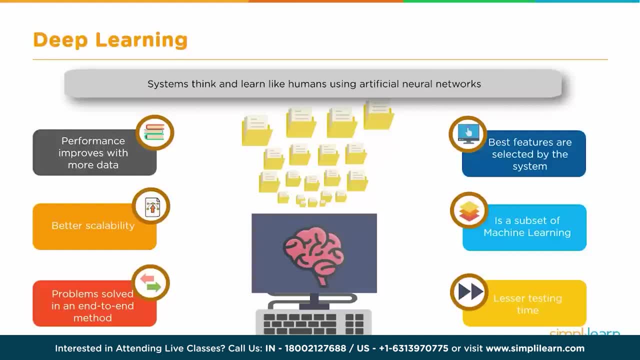 Again, it's like a magic box, So perhaps a real job prop hyung here in Southern California. Performance improves with more data, So the more data that deep learning gets, the more it gives you better results. A scalability- So it's easy to say it's global- might be understood as Scalability. 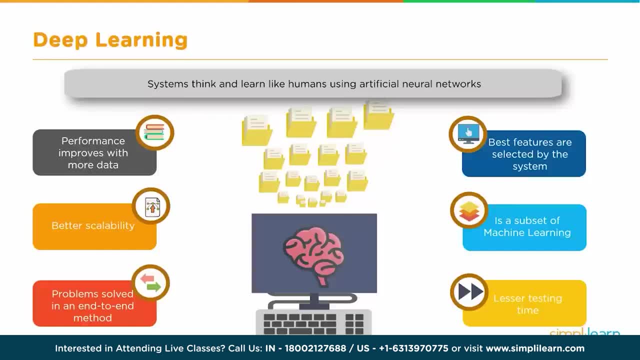 So you can scale it up, You can scale it down, You can increase what you're looking at. So Right now I've solved all the manipulations specifically with the rich data. That's working not just for my computer actions here at NASA. 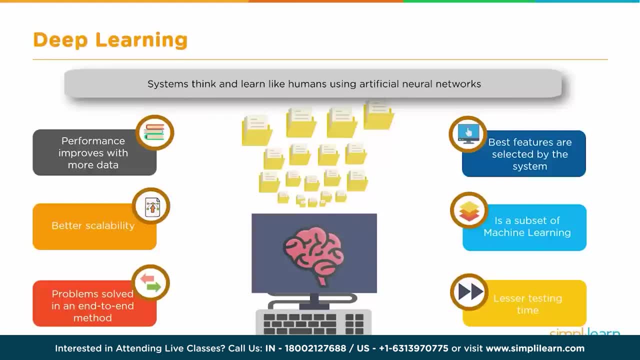 Currently, you know, we're limited by the amount of computer processing students that have access to our system, by the amount of computer processing power as to how big that can get. but that envelope continually gets pushed every day on what it can do. Problem solved in an end-to-end method. so instead of 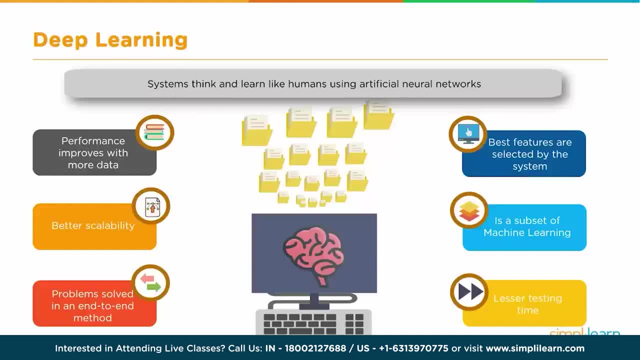 having to break it apart and you have the first piece coming in and you identify tires and the second piece is identifying labeling, handlebars, and then you bring that together that if it has handlebars and tires it's a bicycle and if it has something that looks like a large square it's. 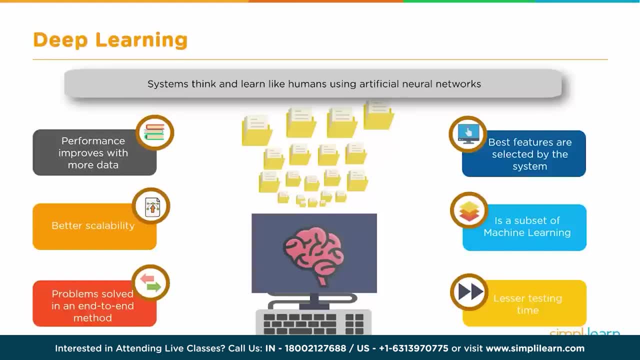 probably a truck. The neural networks does this all in one network. you don't really know what's going on in all those weights and all those little bubbles, but it does it pretty much in one package. that's why the neural network systems are so big nowadays and coming into their own Best features. 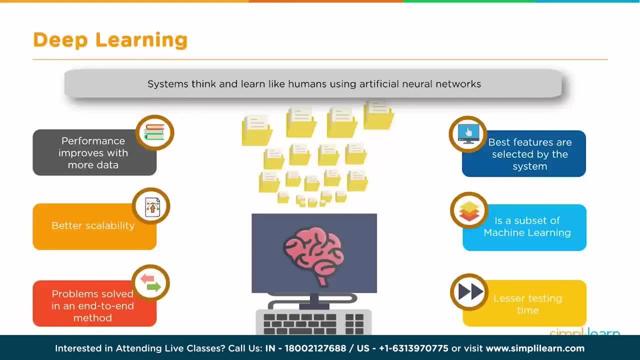 are selected by the system, and this is important. they kind of put it on a bullet on the side here. it's a subset of machine learning. this is important. we talk about deep learning. it is a form of machine learning. There's lots of other forms of machine learning- data analysis- but this is the newest and biggest. 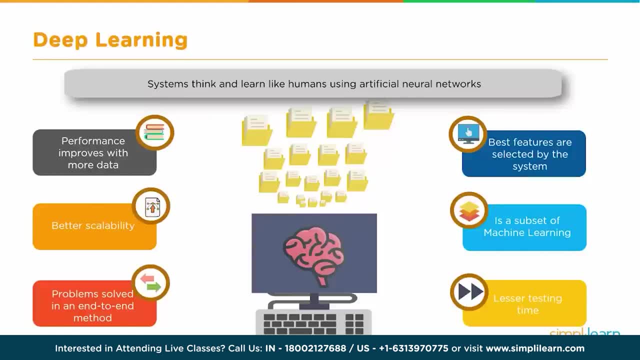 thing that they apply to a lot of different packages and they use all the other machine learning tools available to work with it. and it's very fast to test. you put in your information, you then have your group of tests and then you held some aside. you see how does it do. it's very quick. 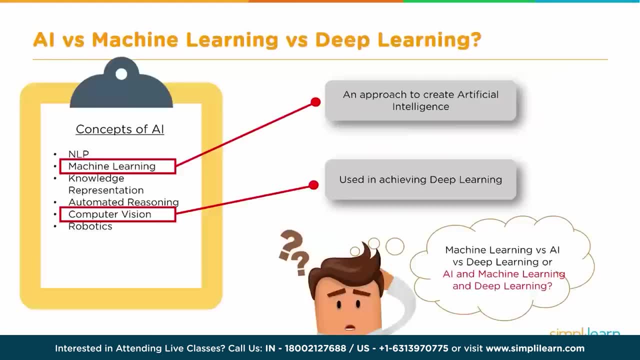 to test it and see what's going on with your deep learning and your neural network. Are they really all that different? AI versus machine learning, Machine learning versus deep learning- concepts of AI. so we have concepts of AI. you'll see: natural language processing, machine learning, an approach to create artificial intelligence. so it's one of 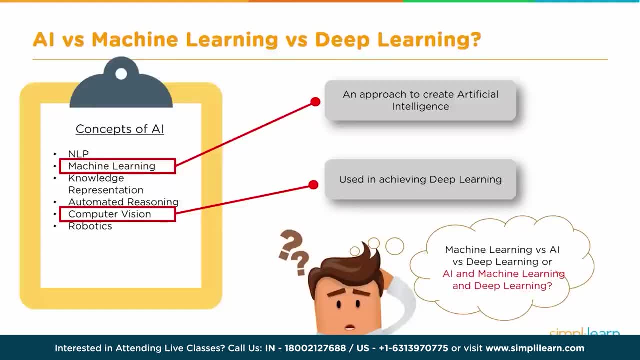 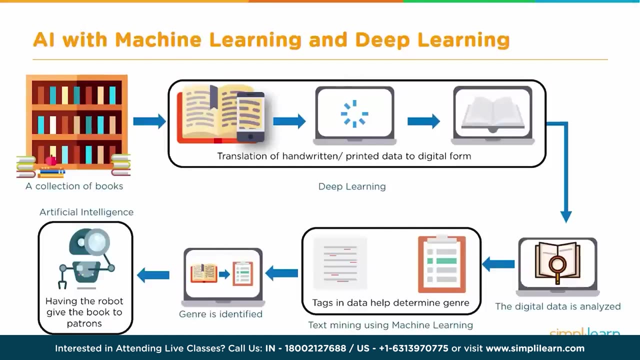 the subsets of artificial intelligence: knowledge representation, automated reasoning, computer vision, robotics, machine learning versus AI versus deep learning, or AI and machine learning and deep learning. so we look at this: we have AI with machine learning and AI with machine learning, So we're going to put them all together. we find out that AI is a big picture. we have a collection of 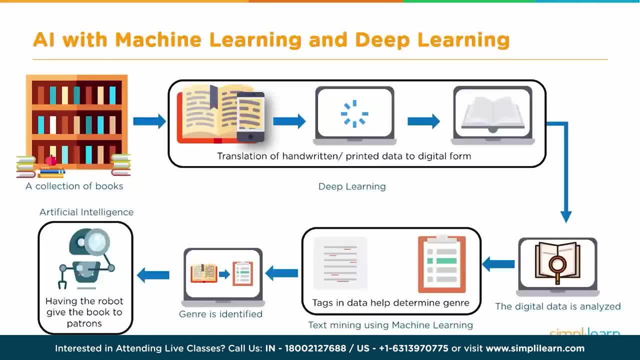 books. that goes through some deep learning. the digital data is analyzed. text mining comes through the particular book you're looking for. maybe it's a genre of books as identified and in this case we have a robot that goes and gives a book to the patron. I have yet to be at a library that has a 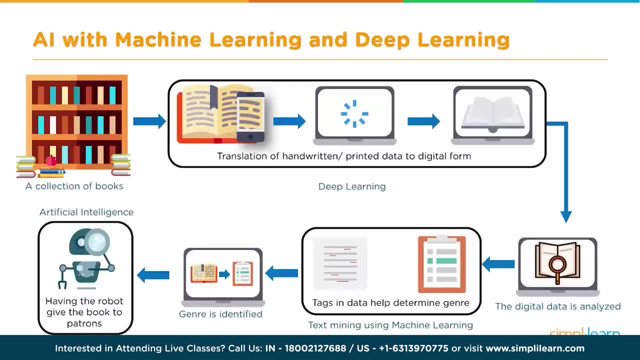 robot. bring me a book, but that will be cool when it happens, cause we'll look at some of the pieces that we have to talk about a robot. bring me a book, but that will be cool when it happens. you have your own robot at a library that's offering you a look at some of the pieces, but you're not going to have your own robot or a group that's offering you a book. 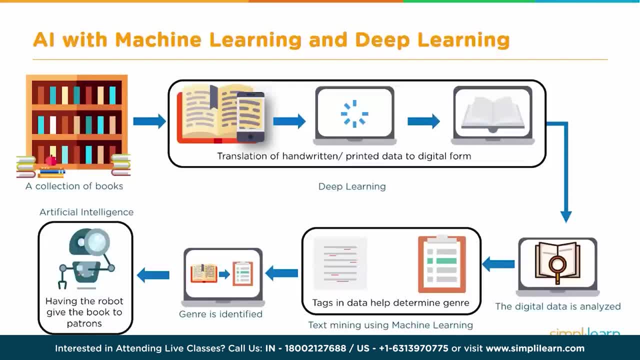 So we'll look at some of the pieces here. This information goes into as far as this example: the translation of the handwritten printed data to digital form. That's pretty hard to do. That's pretty hard to go in there and translate hundreds and hundreds of books. 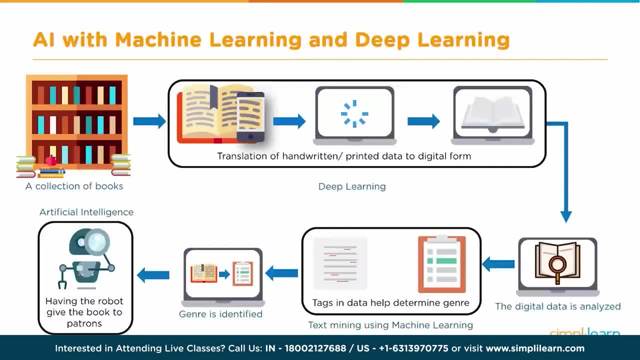 and understand what they're trying to say if you've never read them. So in this case we used a deep learning, because you can already use examples where they've already classified a lot of books and then they can compare those texts and say: 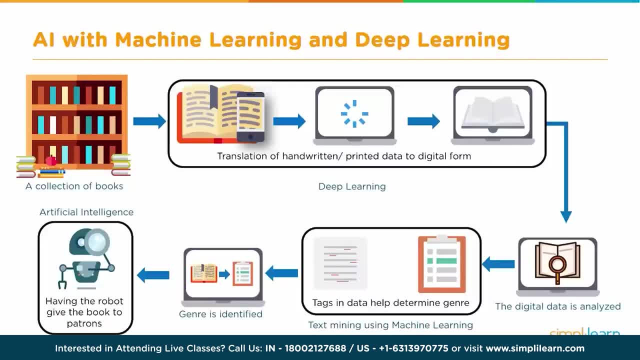 oh okay, this is a book on automotive repair. This is a book on robotic building. The digital data is then analyzed. Then we have more text mining using machine learning. So maybe we'd use a different program to do a basic classify what you're looking for. 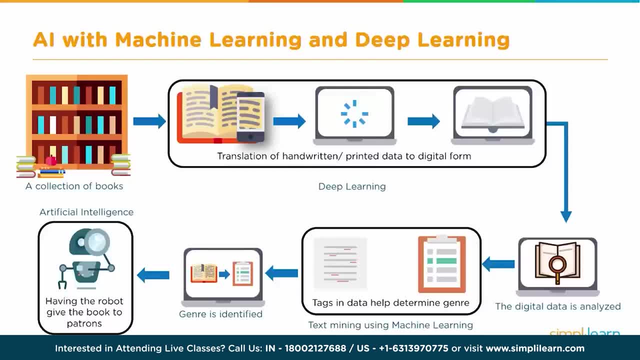 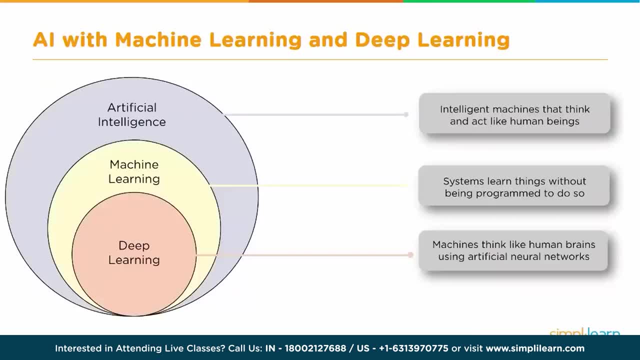 and say: oh, you're looking for auto repair and computers, So you're looking for automated cars. Once it's identified, then of course it brings you the book. So here's a nice summation. Here's a nice summation of what we were just talking about. 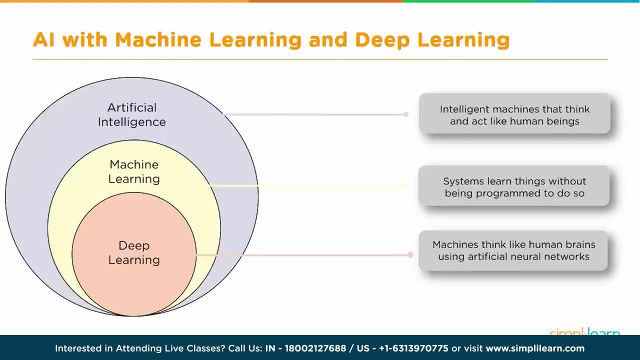 AI with machine learning and deep learning. Deep learning is a subset of machine learning, which is a subset of artificial intelligence, So you can look at artificial intelligence as the big picture. How does this compare to the human experience? in either doing the same thing as a human, we do? 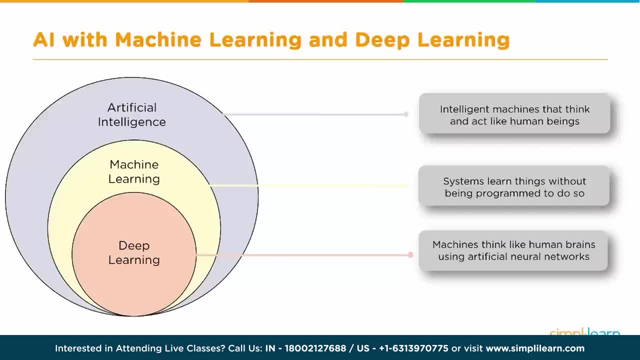 or does it better than us? And machine learning, which has a lot of tools, is something that learns from data past experiences. It's programming, It comes in there and it says, hey, we already had these five things happen. The sixth one should be about the same. 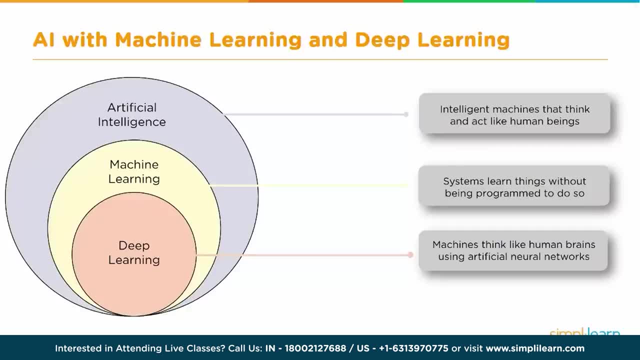 And then there's a lot of tools in machine learning, but deep learning, then, is a very specific tool in machine learning. It's the artificial neural network which handles large amounts of data and is able to take huge pools of experiences, pictures and ideas. 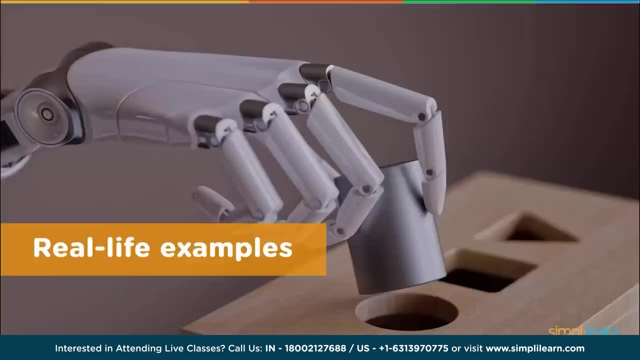 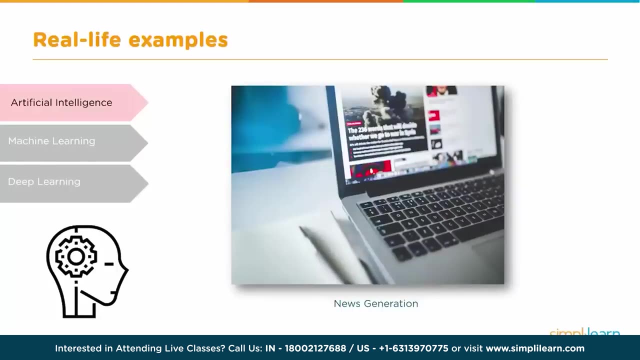 and bring them together. Real life examples: Artificial intelligence, News generation- Very common nowadays is: it goes through there and finds the news articles, or generates the news based upon the news feeds, or the back end coming in and says: okay, let's give you the actual news based on this. 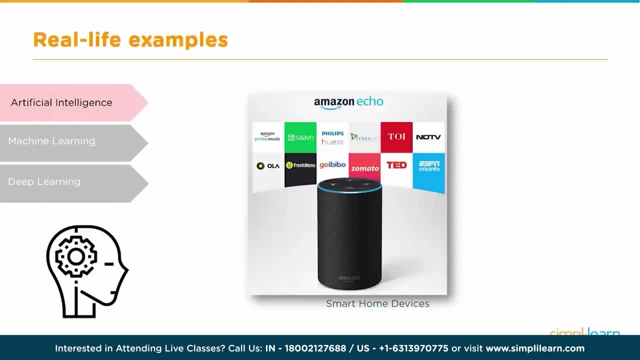 There's all the different things: Amazon Echo. They have a number of different Prime Music on there. Of course, there's also the Google Command and there's also Cortana. There's tons of smart home devices now where we can ask it to turn the TV on. 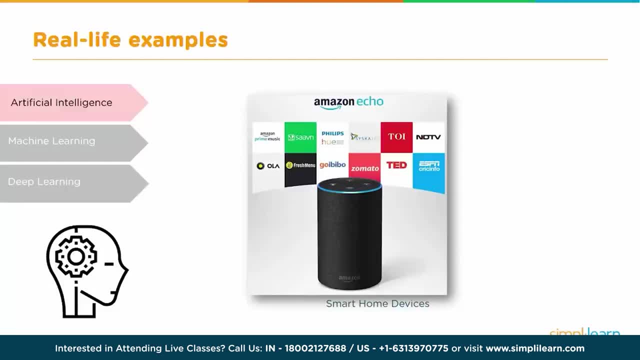 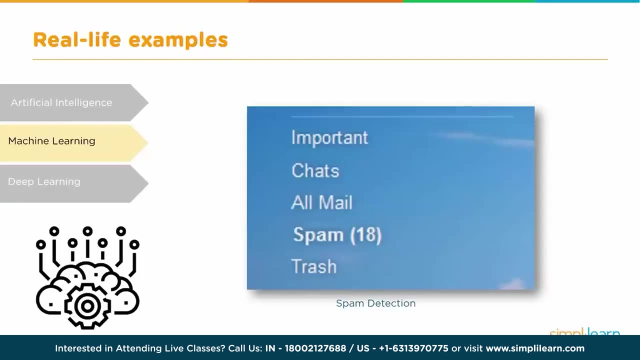 Or play music. for us, That's all artificial intelligence From front to back. you're having a human experience with these computers and these objects that are connected to the processing. Machine learning, Spam detection- Very common Machine learning- doesn't really have the human interaction part. 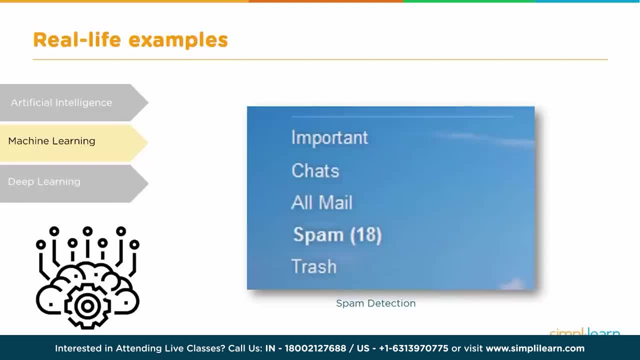 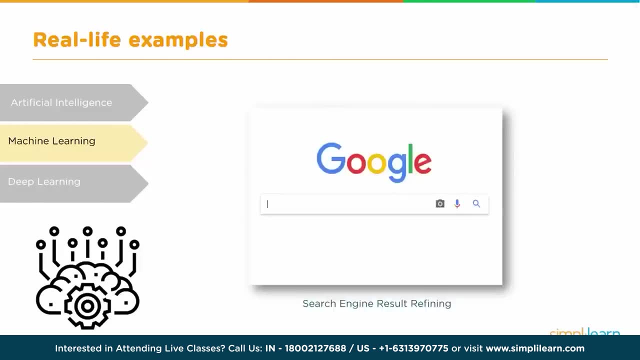 So this is the part where it goes and says: okay, that's a spam, That's not a spam, And it puts it in your spam folder. Search engine result refining- Another example of machine learning, whereas it looks at your different results. 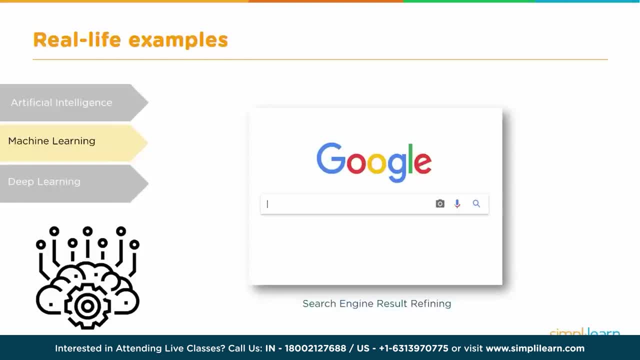 and it is able to categorize them as far as this had the most hits. This is the least viewed. This has five stars, You know. however, they want to weight it All. good examples of machine learning, And then the deep learning. 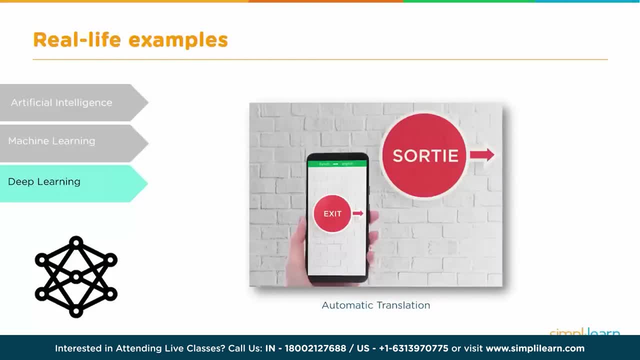 Deep learning. another example is: is you have like an exit sign? In this case it's translating it into French: Sortie. I hope I said that right Neural network has been programmed with all these different words and images And so it's able to look at the exit in the middle and it goes okay. 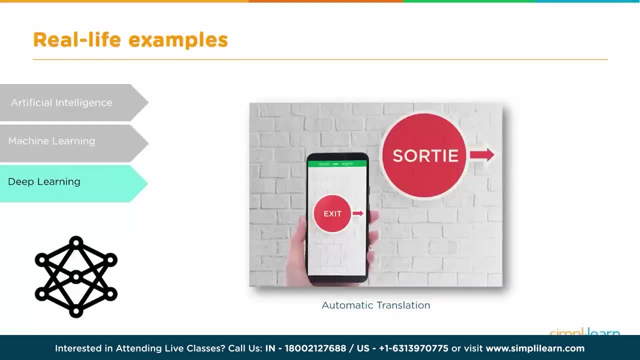 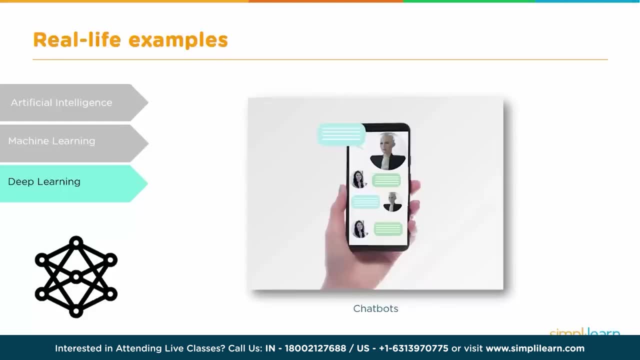 we want to know what that is in French And it's able to push that out in French and learn how to do that. And then we have chat bots. I remember when Microsoft first had their little paperclip Boy. that was like a long time ago. 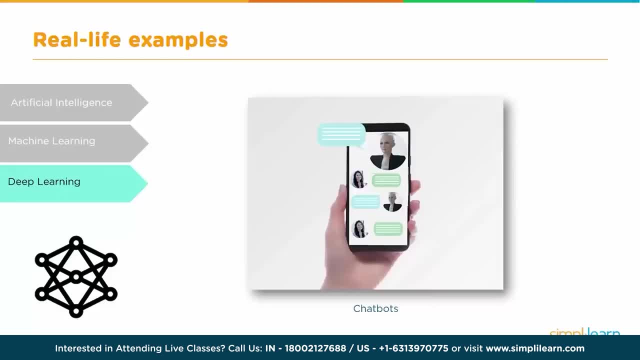 They came up and you would type in there and chat with it. These are growing. You know, it's nice to just be able to ask a question And it comes up and gives you the answer And instead of it being were you just doing a search on certain words. 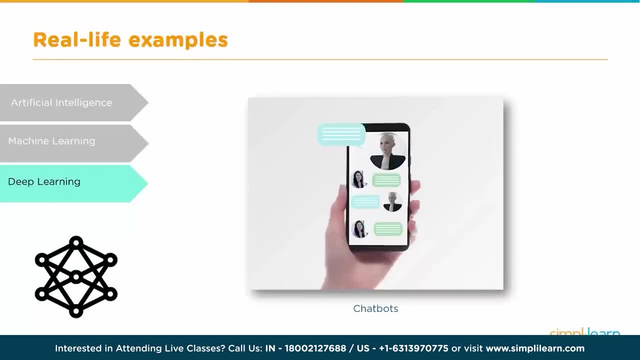 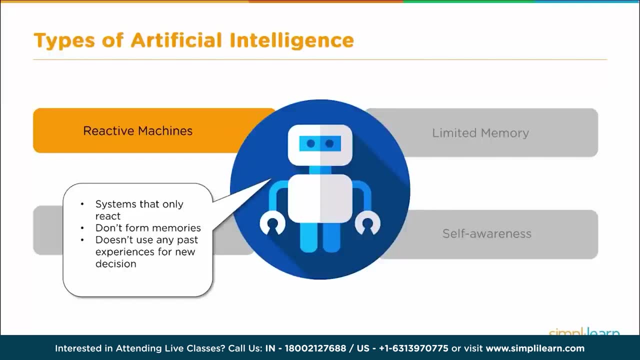 it's now able to start linking those words together and form a sentence in that chat box. Types of AI and machine learning- Types of artificial intelligence. This and the next few slides are really important. So one of the types of artificial intelligence is reactive machines. 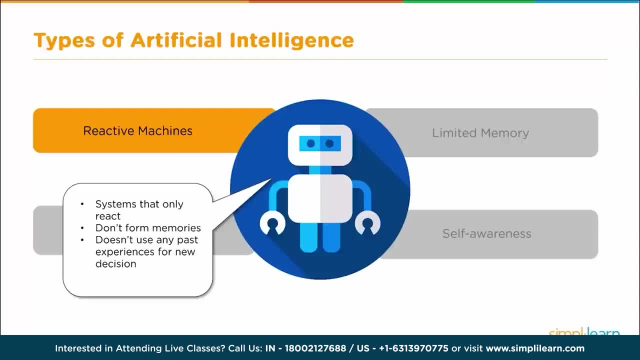 Systems that only react. They don't form memories, They don't have past experiences. They have something that happens to them And they react to it. My washing machine is one of those. If I put a ton of clothes in it and they get all clumped on one side. 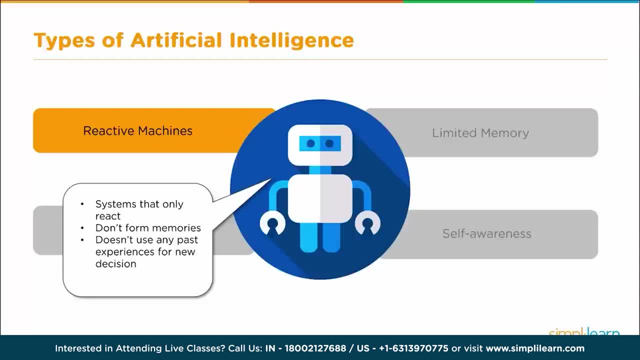 it automatically adds a weight to re-center it, So that my washing machine is actually a reactive machine, working with whatever the load is and keeps it nice, And so when it spins it doesn't go thumping against the side. Limited memory: Another form of artificial intelligence. 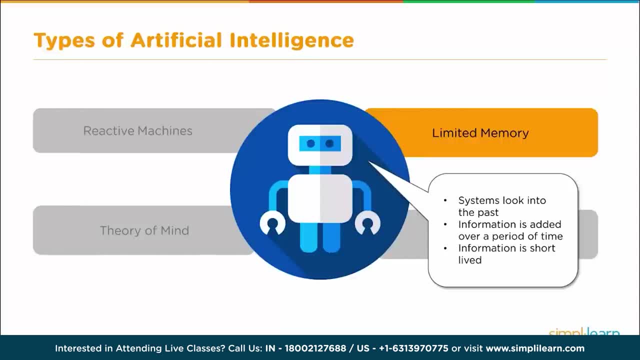 Systems. look into the past. Information is added over a period of time And information is short-lived. When we're talking about this and you look at like a neural network that's been programmed to identify cars, it doesn't remember all those pictures. 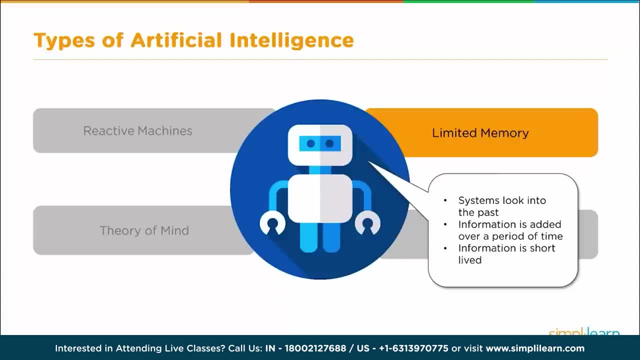 It has no memory as far as the hundreds of pictures you process through it. All it has is: this is the pattern I used to identify cars as the final output for that neural network we looked at. So when they talk about limited memory, this is what they're talking about. 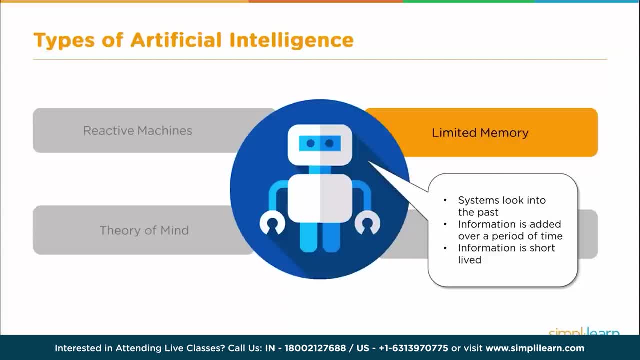 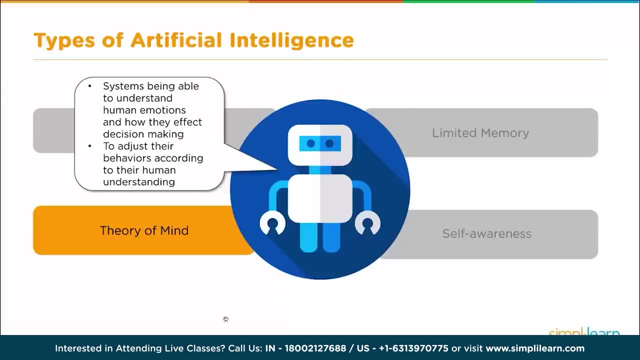 They're talking about. I've created this based on all these things, but I'm not going to remember any one specifically Theory of mind Systems being able to understand human emotions and how they affect decision making, to adjust their behaviors according to their human understanding. 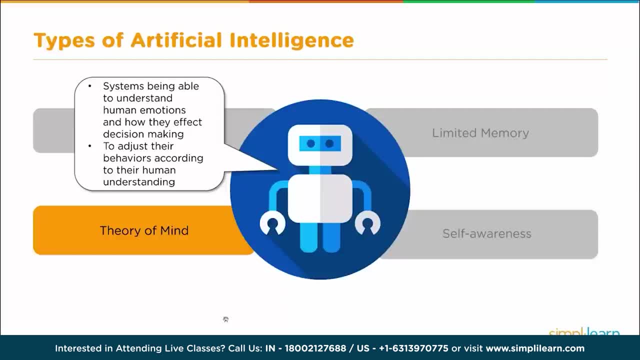 This is important because this is our page mark. This is how we know whether it is an artificial intelligence or not. Is it interacting with humans in a way that we can understand? Without that interaction, it's just an object. So we talk about theory of mind. we really understand how it interfaces. 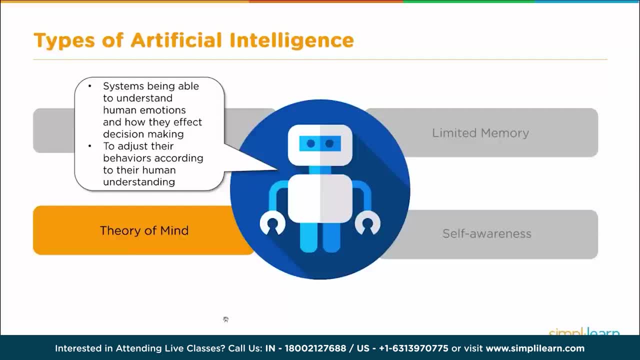 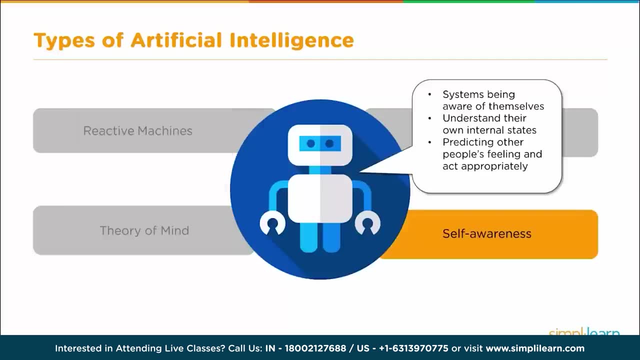 that whole. if you're in web development, user experience would be the term I would put in there. So the theory of mind would be user experience. How is the whole UI connected together? And one of the final things as we get into artificial intelligence is systems being aware. 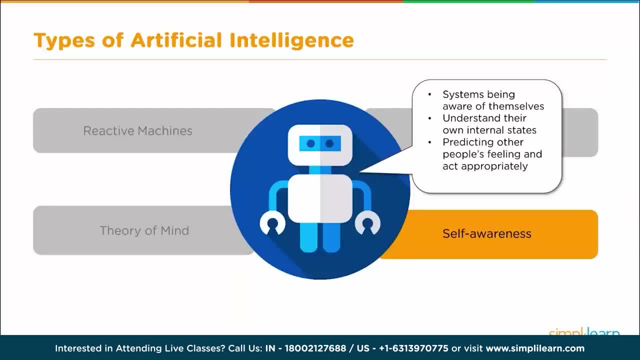 of themselves understanding their internal states and predicting other people's feelings and act appropriately. So as artificial intelligence continues to progress, we see ones that are trying to understand well what makes people happy. How would they increase our happiness? How would they keep themselves from breaking down if something's broken inside? 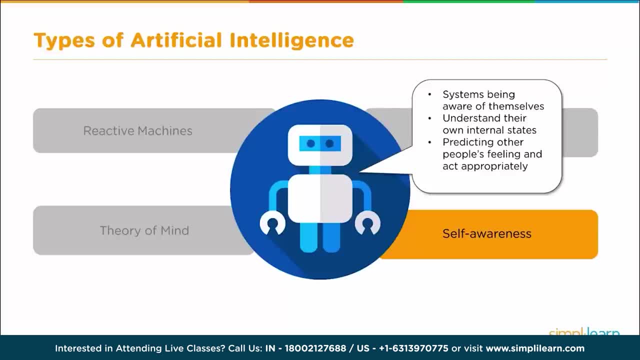 They have that self-awareness to be able to fix it And, just based on all that information, predicting which action would work the best. What would help people If I know that you're having a cup of coffee first thing in the morning is what makes you happy. 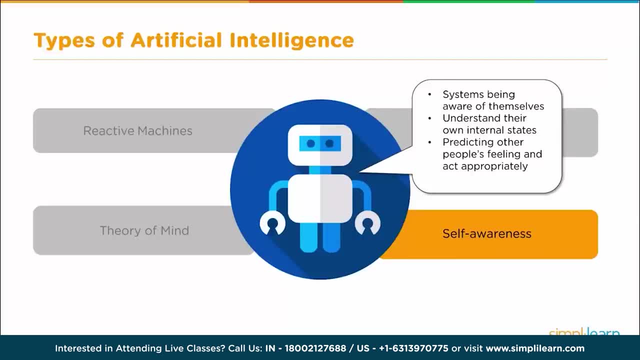 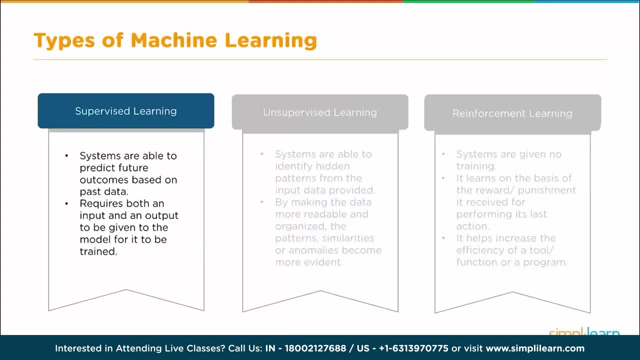 as a robot, I might make you a cup of coffee every morning at the same time to help your life and help you grow. That would be the self-awareness is being able to know all those different things, Types of machine learning And, like I said on the last slide, this is very important. 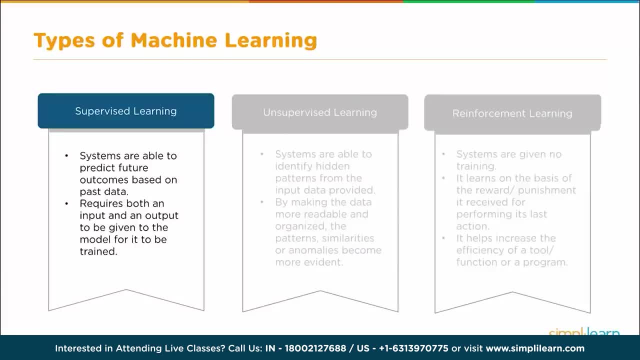 This is very important If you decide to go in and get certified in machine learning or know more about it. these are the three primary types of machine learning. The first one is supervised learning Systems are able to predict future outcome based on past data. 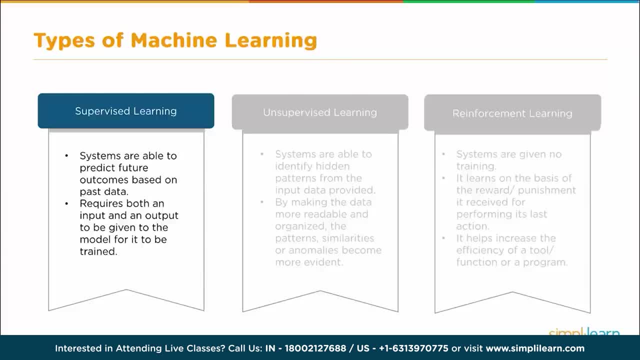 Requires both an input and an output to be given to the model for it to be trained. So in this case we're looking at anything where you have 100 images of a bicycle and those 100 images you know are bicycle, so they're pre-set. 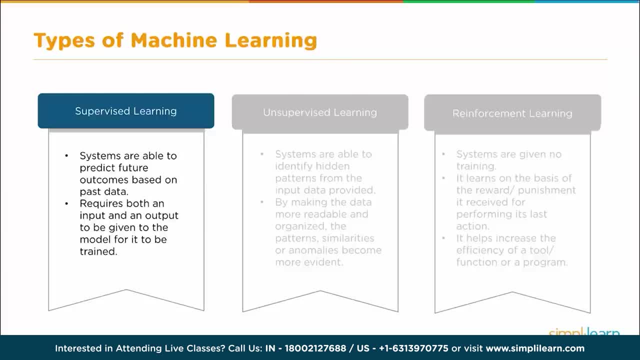 Someone already looked at all 100 images and said: these are pictures of bicycles And so the computer learns from those. and then it's given another picture, and maybe the next picture is a bicycle, and it says: oh, that resembles all these other bicycles, so it's a bicycle. 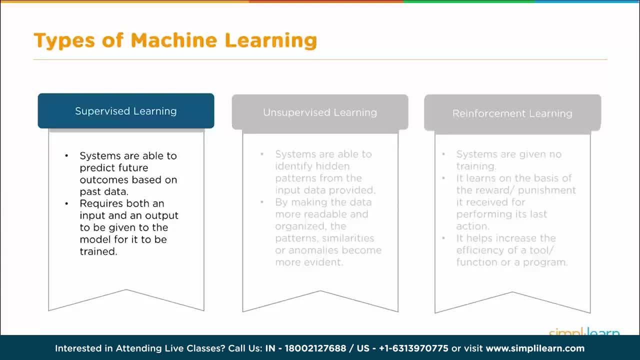 And the next one's a car and it says, eh, it's not a bicycle, That would be supervised learning, because we had to train it, We had to supervise it. Unsupervised learning Systems are able to identify hidden patterns. 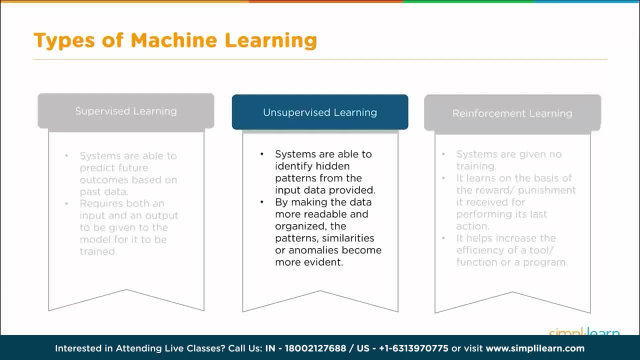 from the input data provided. by making the data more readable and organized, The patterns, similarities or anomalies become more evident. You'll heard the term cluster. How do you cluster things together? Some of these things go together. Some of these don't. 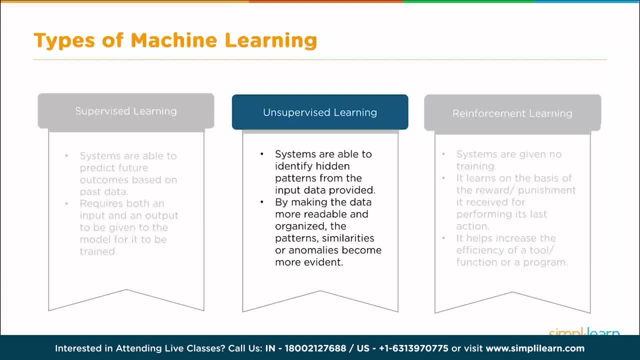 This is unsupervised, where it can look at an image and start pulling the different pieces of the image out because they aren't the same. The human, all the parts of the human, are not the same as a fuzzy tree behind them. 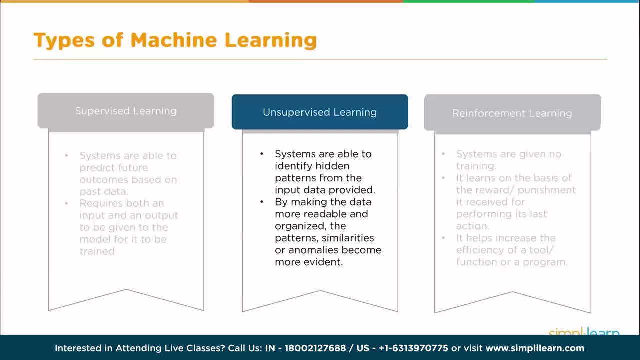 because it's slightly out of focus, which is not the same as the beach ball. It's unsupervised, because we never told it what a beach ball was, We never told it what the human was and we never told it that those were trees. 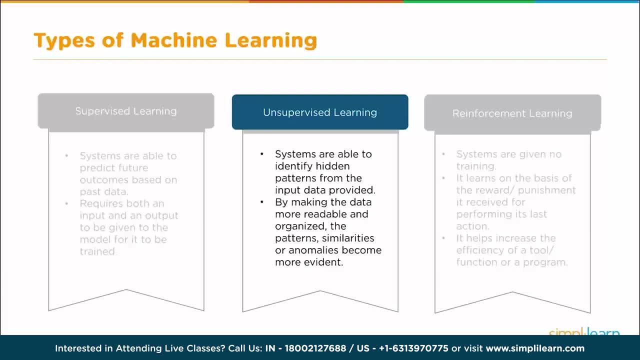 All we told it was: hey, separate this picture by things that don't match and things that do match and come together. And finally there's reinforcement. learning Systems are given no training. It learns on the basis of the reward punishment it received for performing its last action. 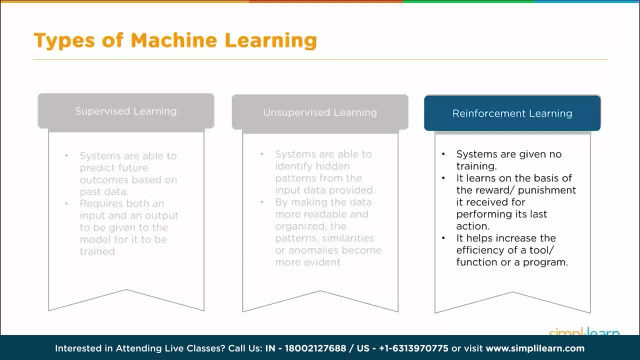 It helps increase the efficiency of a tool, function or a program. Reinforced learning or reinforcement learning is kind of you give it a yes or no. Yes, you gave me the right response, No, you didn't. And then it looks at that and says, oh, okay, so based on this data coming in, 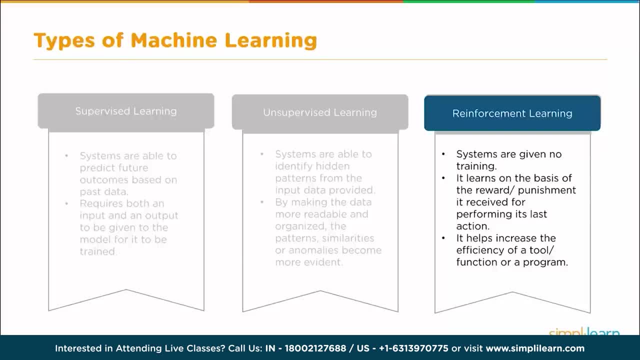 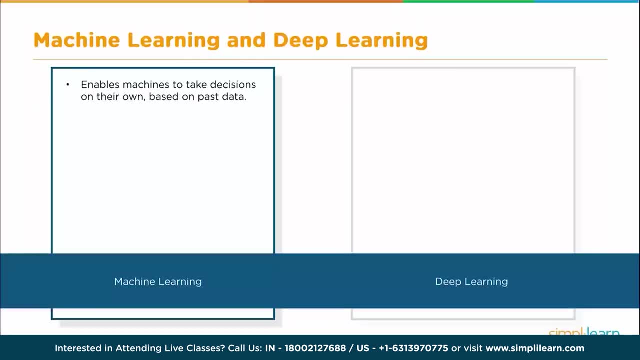 what I gave you was a wrong response, so next time I'll give you a different one, Comparing machine learning and deep learning. So remember that deep learning is a subcategory of machine learning, So it's one of the many tools. 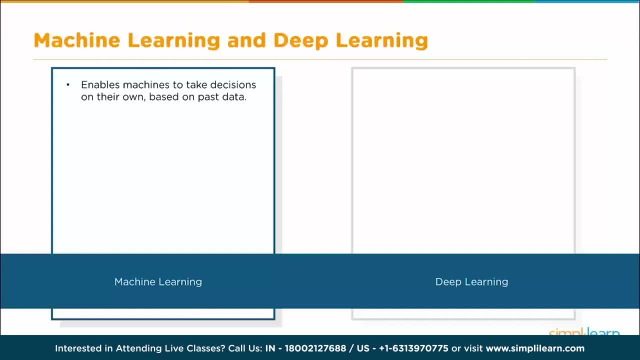 And so we're grouping a ton of machine learning tools all together. Linear regression k-means clustering. there's all kinds of cool tools out there you can use, And machine learning enables machines to take decisions, to make decisions on their own based on past data. 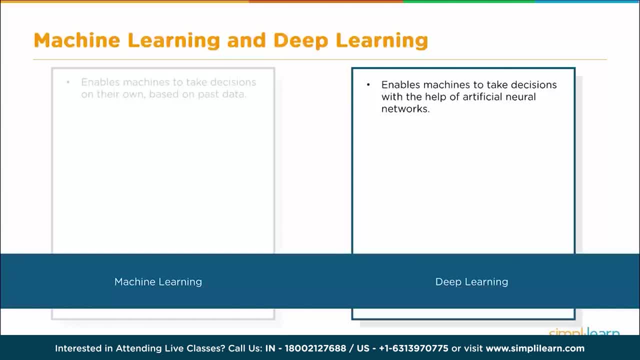 Enables machines to make decisions with the help of artificial neural networks. So it's doing the same thing, but we're using an artificial neural network, as opposed to one of the more traditional machine learning tools Needs only a small amount of training data. This is very important. 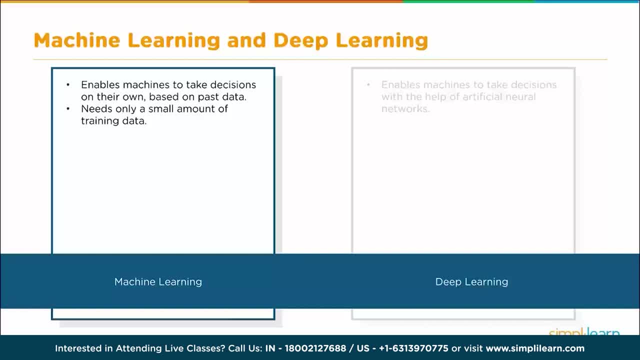 When you're talking about machine learning, they're usually not talking about huge amounts of data. We're talking about, maybe, your spreadsheet from your business And your totals for the end of the year. When you're talking about neural networks, you usually need a large amount of data to train the data. 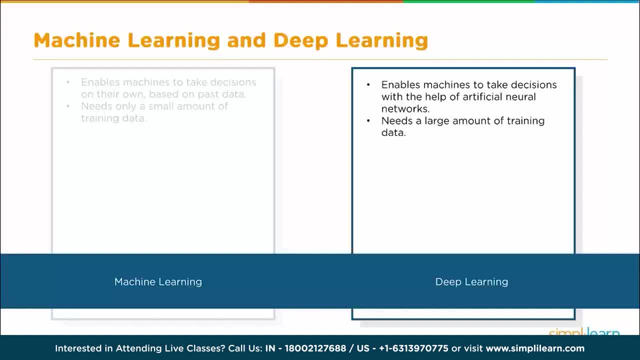 So there's a lot of training involved. If you have under 500 points of data, that's probably not going to go into machine learning. Or maybe you have, like in the case of one of the things, 500 points of data and 30 different fields. 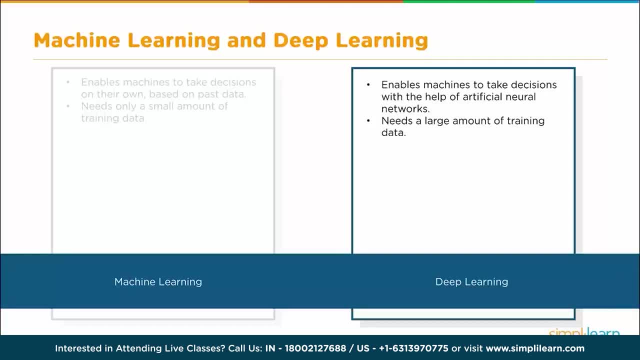 It starts getting really confusing there in artificial intelligence or machine learning And the deep learning aspect really shines when you get to that larger data. that's really complex, Works well on low-end systems, So a lot of the machine learning tools out there you can run on your laptop with no problem and do the calculations there. 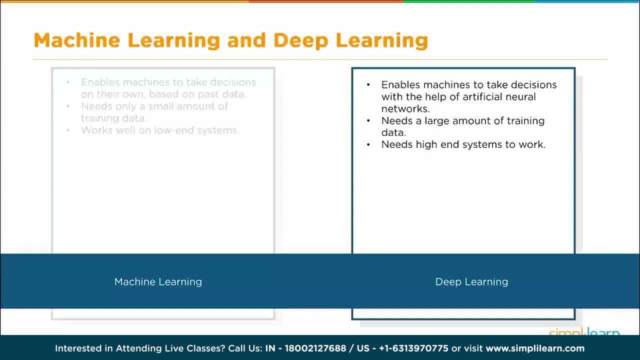 Where with the machine learning, it usually needs a higher-end system to work. It takes a lot more processing power to build those neural networks and to train them. It goes through a lot of data. We're talking about the general machine learning tools. 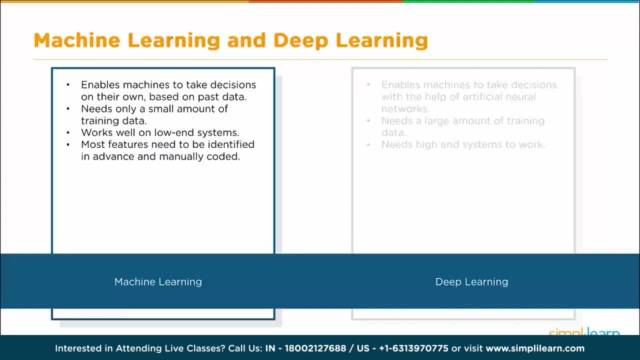 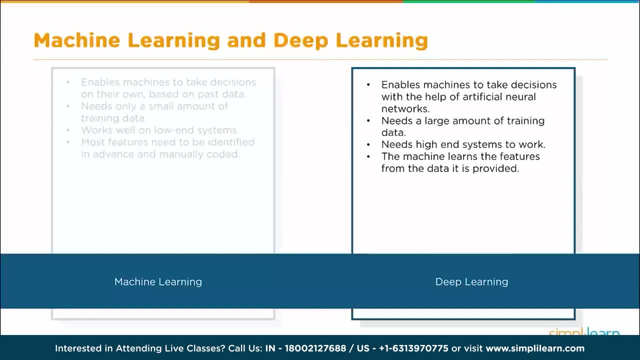 Most features need to be identified in advanced and manually coded, So there's a lot of human work on here. The machine learning tools: The machine learns the features from the data it is provided. So again, it's like a magic box. You don't have to know what a tire is. 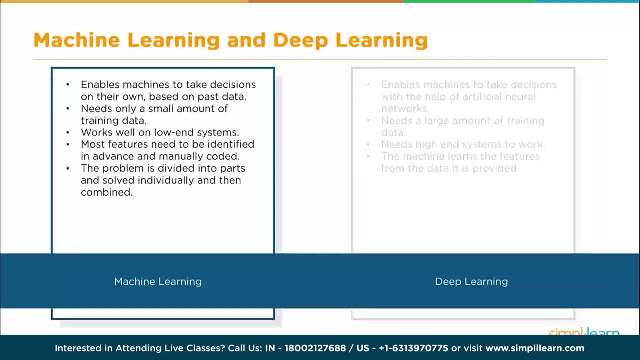 It figures it out for you. The problem is divided into parts and solved individually and then combined. So in machine learning you usually have all these different tools and use different tools for different parts, And the problem is solved in an end-to-end manner. 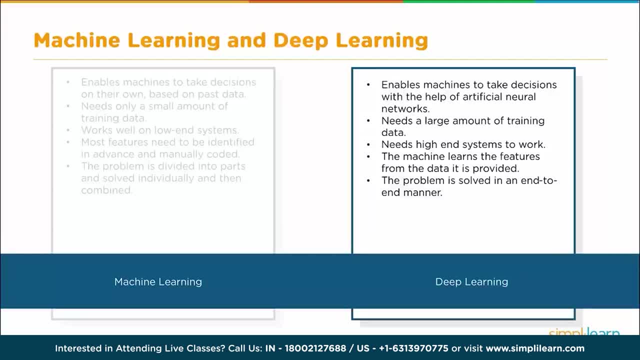 So you only have one neural network or two neural networks. that is, bringing the data in and putting it out. It's not going through a lot of different processes together. And remember, you can put machine learning and deep learning together So you don't always have just the deep learning solving the problem. 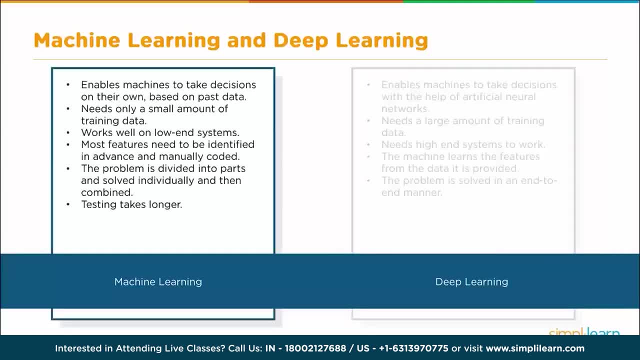 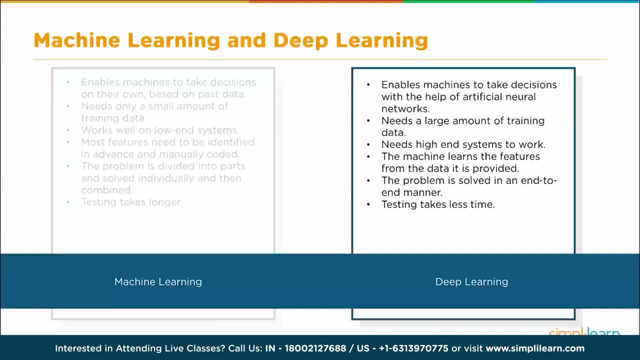 You might have it solving one piece of the puzzle. With regular machine learning and most machine learning tools out there. they take longer to test and understand how they work And with the deep learning it's pretty quick. Once you build that neural network, you test it and you know. 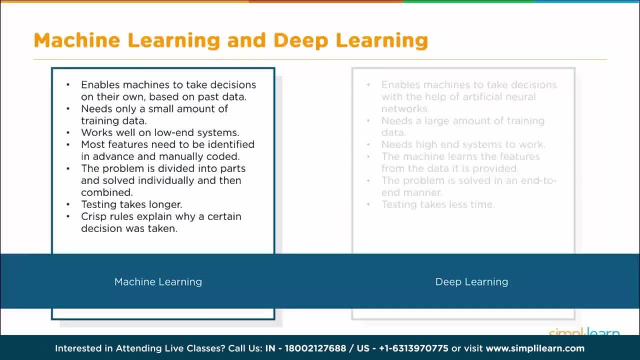 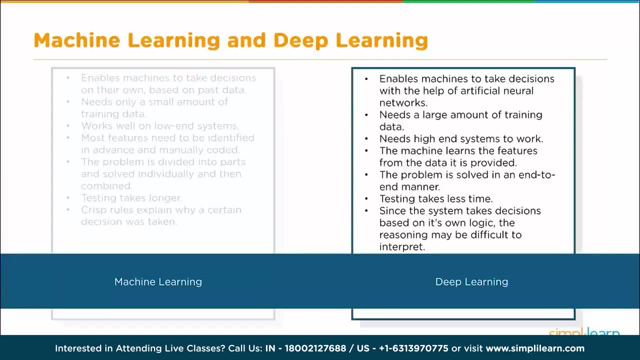 So we're dealing with very crisp rules, limited resources. You have to really explain how the decision was made When you use most machine learning tools, But when you use the deep learning tool inside the machine learning tools, the system takes care of it based on its own logic and reasoning. 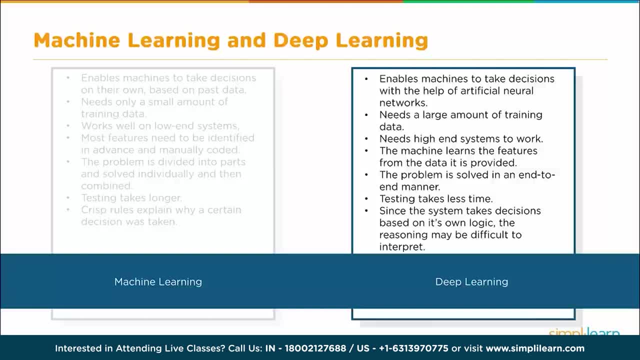 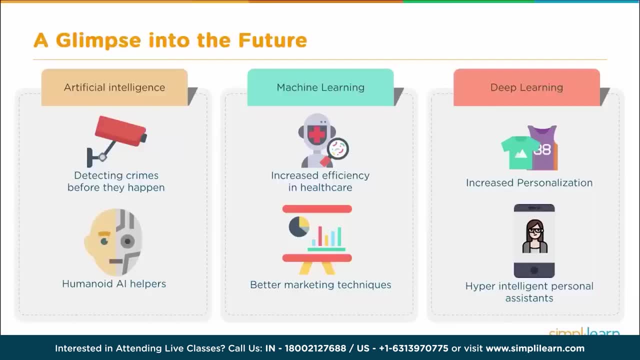 And again, it's like a magic black box. You really don't know how it came up with the answer. You just know it came up with the right answer. A glimpse into the future. So a quick glimpse into the future: Artificial intelligence. 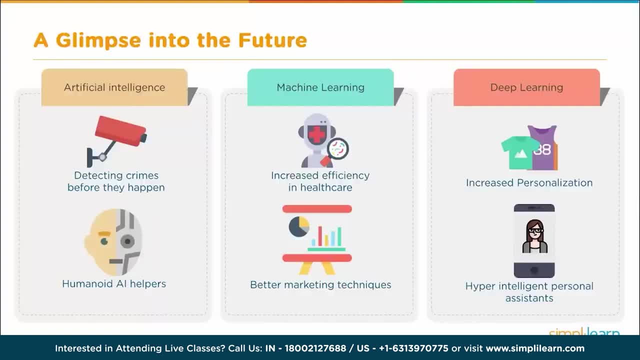 Be using it to detecting crimes before they happen. Humanoid AI helpers, which we already have a lot of, It'll be more and more. Maybe it'll actually be androids. That'd be cool to have an android that comes and gets stuff out of my fridge for me. 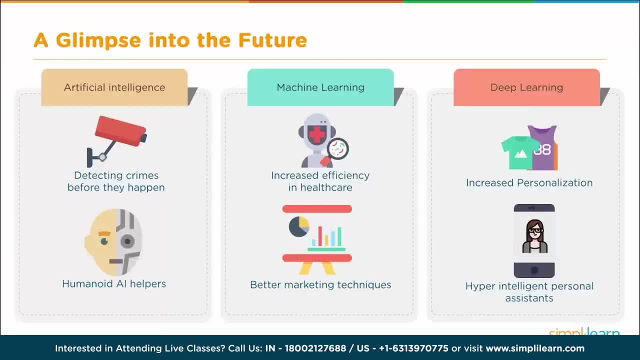 Machine learning, Increasing efficiency in healthcare- That's really big in all the forms of machine learning, Better marketing techniques- Any of these things if we get into the sciences it's just off the scale. Machine learning and artificial intelligence go everywhere. 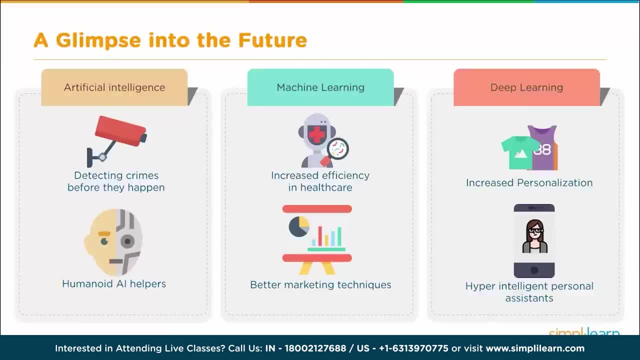 And then the subcategory deep learning: Increased personalization. So what's really nice about the deep learning is it's going to start now catering to you. That'll be one of the things we see more and more of, And we'll have more of a hyper intelligent personal assistant. 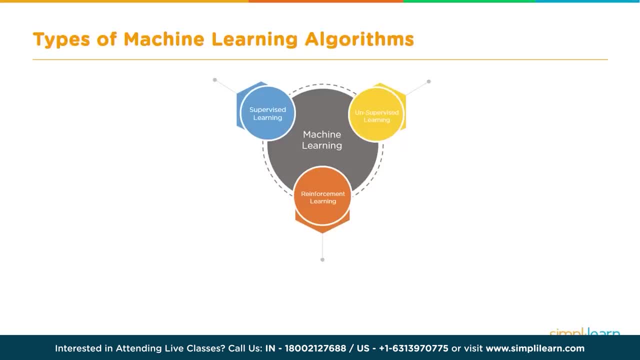 I'm excited about that. What are the different types of machine learning algorithms? Machine learning algorithms are broadly classified into three types: The supervised learning, unsupervised learning and reinforcement learning. Supervised learning in turn consists of techniques like regression and classification. 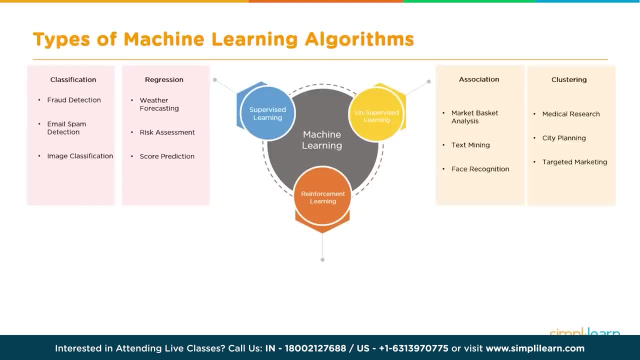 And unsupervised learning. These techniques, like association and clustering And reinforcement learning, is a recently developed technique And it is very popular in gaming. Some of you must have heard about AlphaGo, So this was developed using reinforcement learning. Primary difference between supervised learning and unsupervised learning: 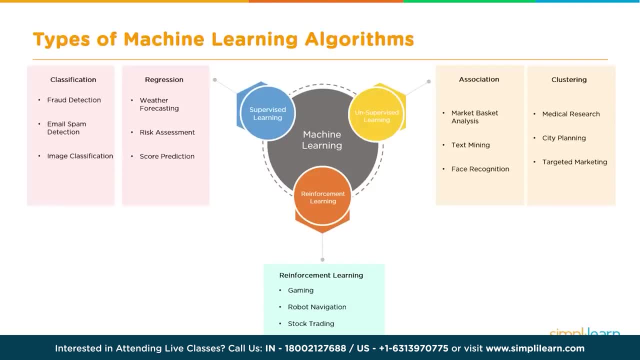 Supervised learning is used when we have historical data and we have labeled data, Which means that we know how the data is classified. So we know the classes We are doing classification, Or we know the values when we are doing regression. So if we have historical data with these values, 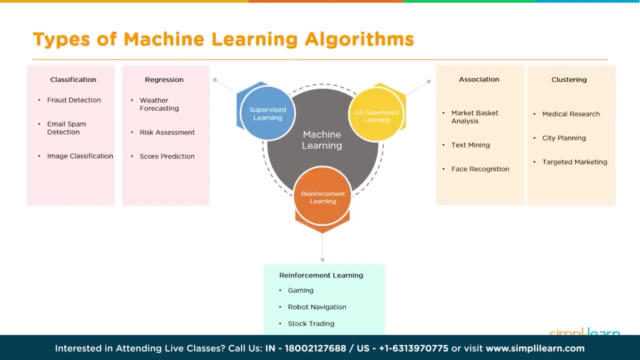 Which are known as labels. Then we use supervised learning. In case of unsupervised learning, We do not have past labeled data, Historical labeled data, So we use techniques like association and clustering To maybe form clusters or new classes maybe, And then we move from there. 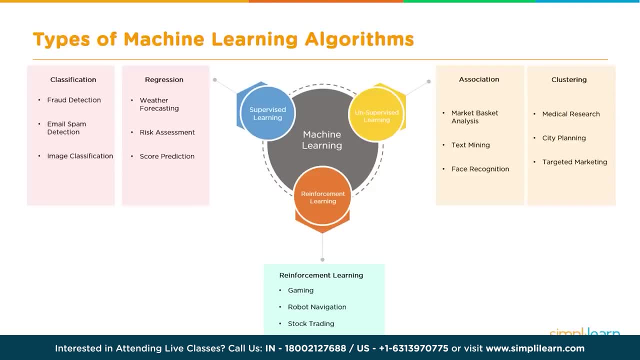 In case of reinforcement learning, The system learns pretty much from scratch. There is an agent and there is an environment. The agent is given a certain target And it is rewarded when it is moving towards that target And it is penalized if it is moving in a direction which is not achieving that target. 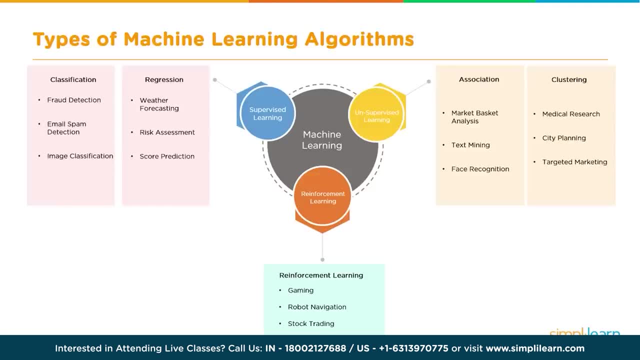 So it's more like a carrot and stick model. So what is the difference between these three types of algorithms? Supervised algorithms or supervised learning algorithms Are used When you have a specific target value That you would like to predict. The target could be categorical. 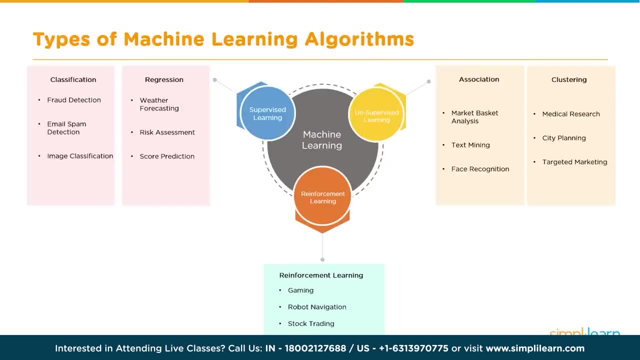 Having two or more possible outcomes, or classes, If you will. That is what is classification, Or the target could be a value which can be measured, And that's where we use regression, Like, for example, weather forecasting. You want to find the temperature. 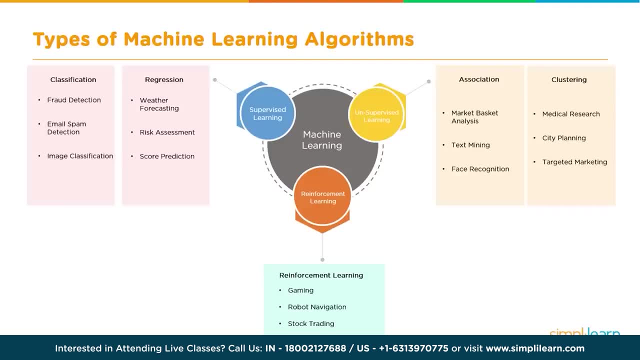 Whereas in classification You want to find out whether this is a fraud Or not a fraud, Or if it is email spam, Whether it is spam Or not a spam. So that is a classification example. So, if you know, Or this is known as labeled information- 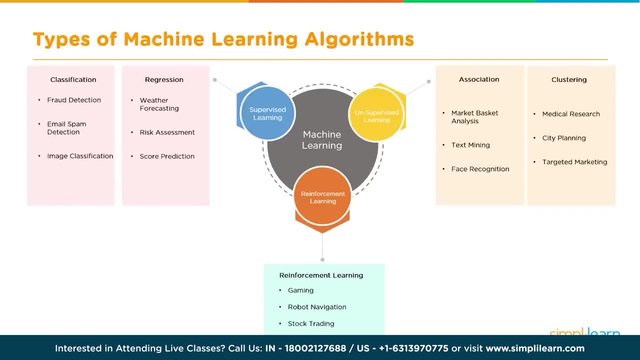 If you have the labeled information, Then you use supervised learning. In case of unsupervised learning, We have input data, But we don't have the labels Or what the output is supposed to be. So that is when we use unsupervised learning techniques. 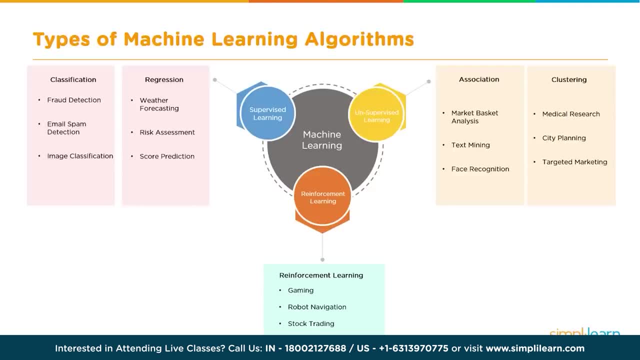 Like clustering and association, And we try to analyze the data. In case of reinforcement learning, It allows the agent to automatically determine the ideal behavior Within a specific context, And it has to do this to maximize the performance, Like, for example, playing a game. 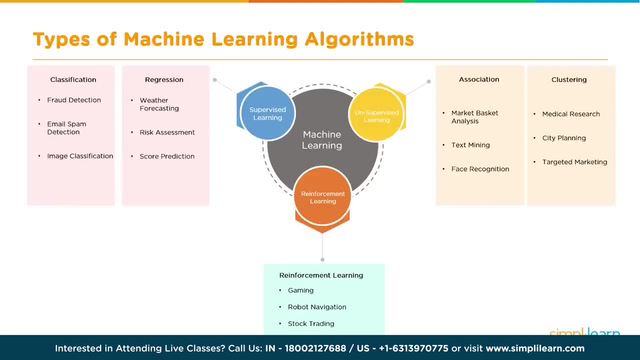 So the agent is told that you need to score the maximum score possible without losing lives. So that is a target that is given to the agent And it is allowed to learn from scratch. Play the game itself multiple times And slowly it will learn the behavior. 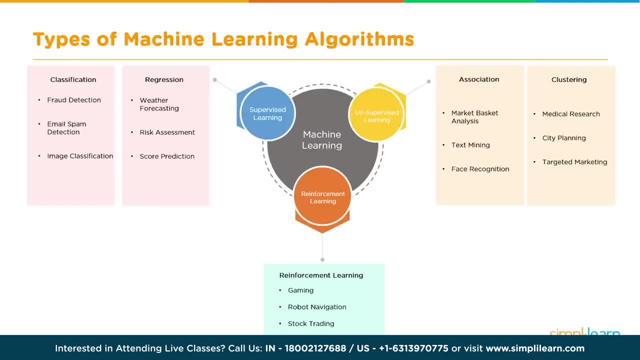 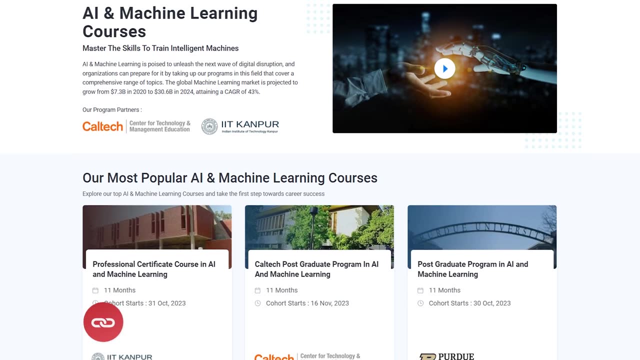 Which will increase the score And keep the lives to the maximum. If you want to become an AI expert And gain handsome salary packages, Look at the wide range of AI ML courses by SimpliLearn, In collaboration with top universities across the globe. 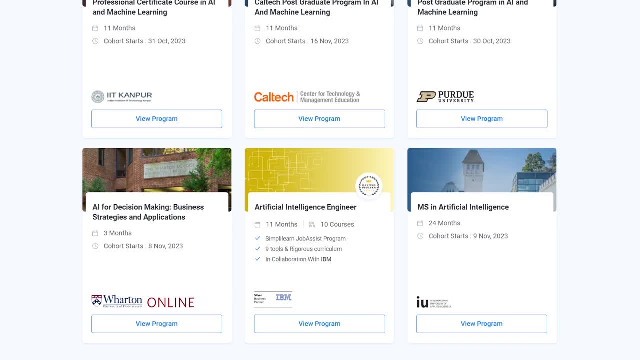 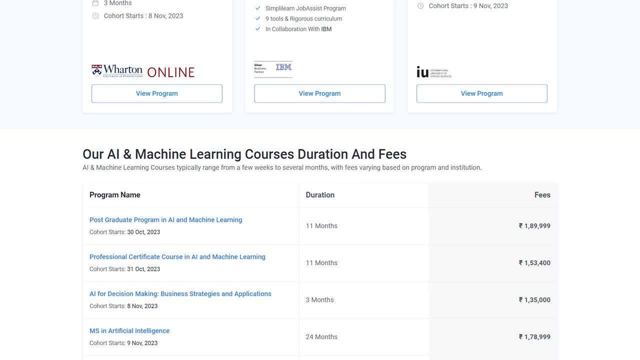 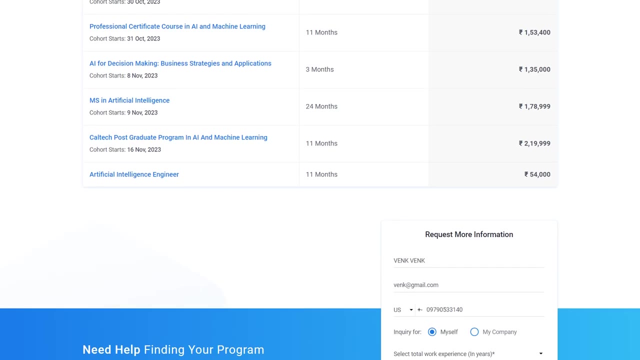 By enrolling in any of these certification programs, You will gain expertise in skills like generative AI, Prompt engineering, Chat, GPT, Explainable AI, Machine learning algorithms, Supervised and unsupervised learning, Model training And optimization, And there is much more on the list. 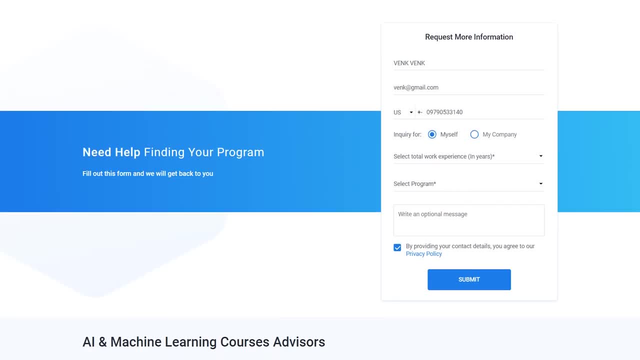 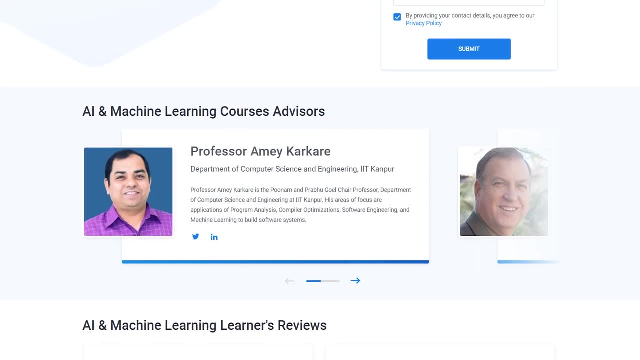 With hands-on experience in the tools like Chat, GPT, DALI, Python, OpenCV And TensorFlow, You will catch the eyes of top recruiters. So what are you waiting for? Hurry up and enroll now. An year of experience is preferred to enroll in these courses. 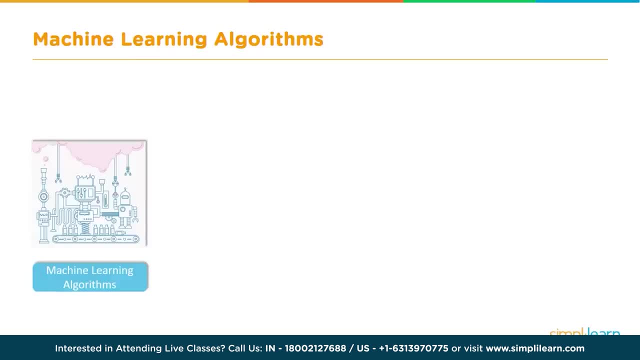 Find the course link in the description box. When we look at a different machine learning algorithms, We can divide them into three areas: Supervised, Unsupervised, Reinforcement. We are only going to look at supervised today. Unsupervised means we don't have the answers. 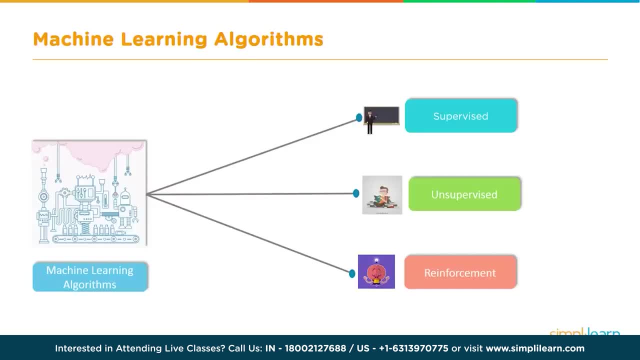 We are just grouping things. Reinforcement is where we give positive and negative feedback To our algorithm, to program it, And it doesn't have the information until after the fact. But today we are just looking at supervised, Because that is where linear regression fits in. 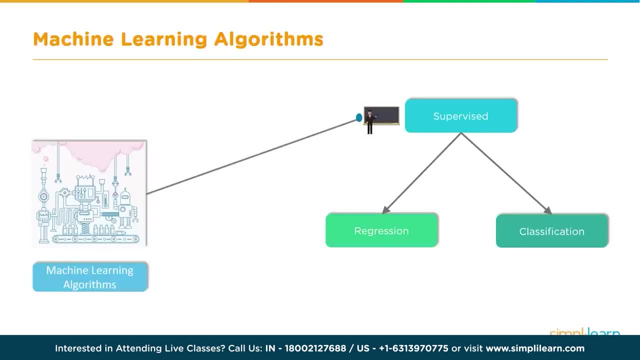 In supervised data. We have our data already there And our answers for a group And then we use that to program our model And come up with an answer. The two most common uses for that Is through the regression and classification. Now we are doing linear regression. 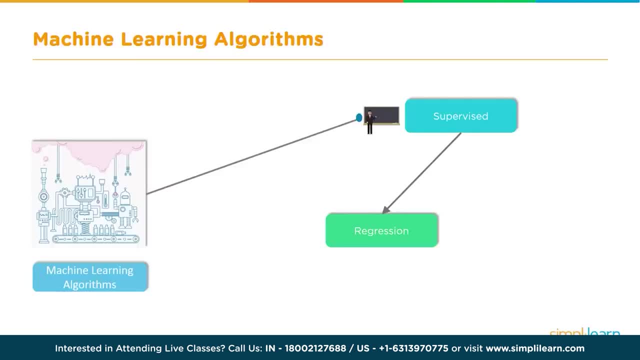 So we are just going to focus on the regression side And in the regression We have simple linear regression, We have multiple linear regression And we have polynomial linear regression. Now, on these three, Simple linear regression is the examples we have looked at so far. 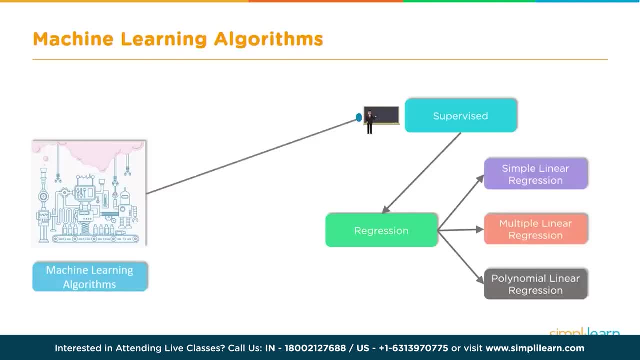 Where we have a lot of data And we draw a straight line through it. Multiple linear regression Means we have multiple variables. Remember where we had the rainfall and the crops. We might add additional variables in there, Like how much food do we give our crops? 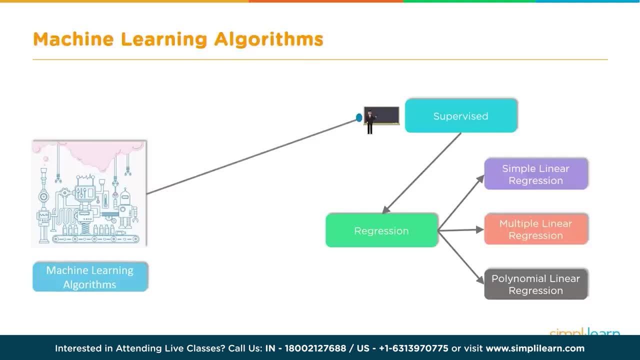 When do we harvest them? Those would be additional information Add into our model And that is why it would be multiple linear regression. And finally, we have polynomial linear regression, That is, instead of drawing a line, We can draw a curved line through it. 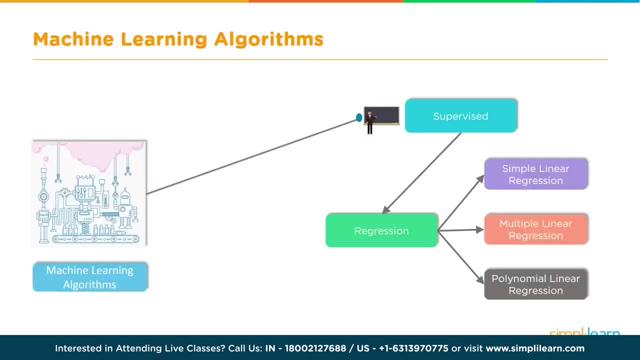 Now that you see where regression model Fits into the machine learning algorithms- And we are specifically looking at linear regression- Let's go ahead and take a look At applications for linear regression. Let's look at a few applications Of linear regression. 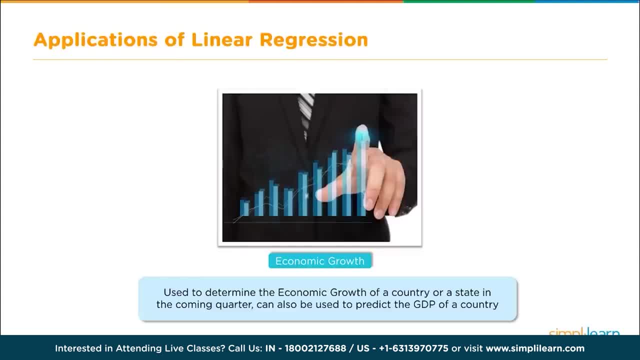 Economic growth, Used to determine the economic growth Of a country or a state In the coming quarter, Can also be used to predict the GDP of a country. Product price Can be used to predict what would be the price Of a product in the future. 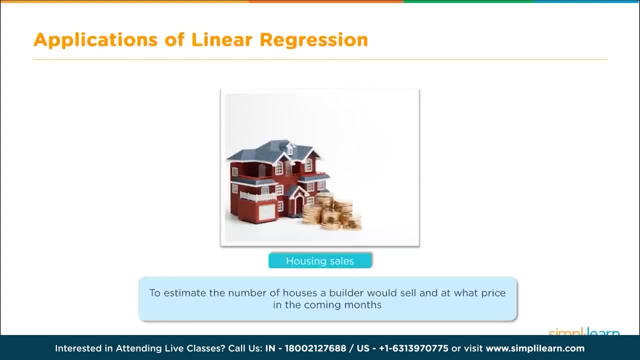 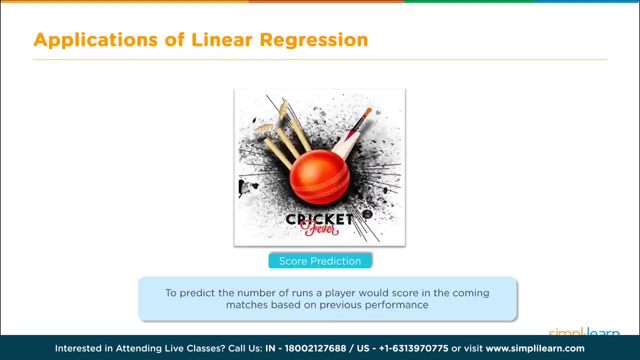 We can guess whether it is going to go up or down. Or should I buy today Housing sales To estimate the number of houses A builder would sell And what price, in the coming months? Score predictions, Cricket fever: To predict the number of runs. 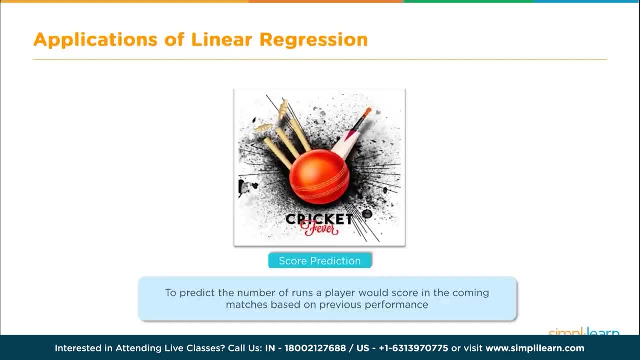 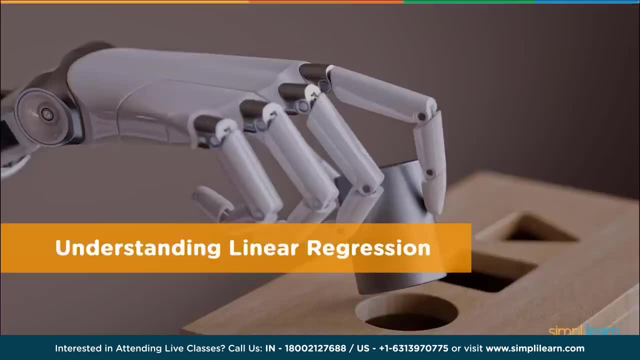 A player would score in the coming matches Based on the previous performance. I am sure you can figure out other applications You could use linear regression for. So let's jump in And let's understand linear regression And dig into the theory. 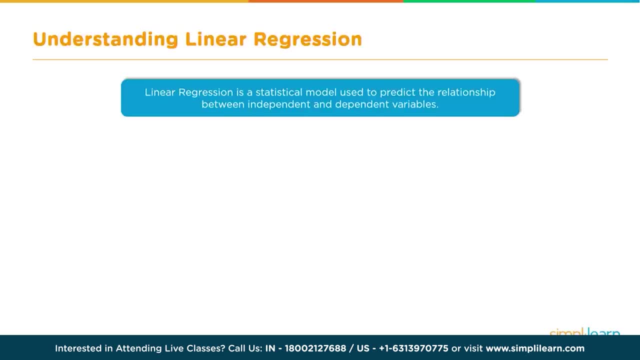 Understanding linear regression. Linear regression Is a statistical model Used to predict the relationship Between independent and dependent variables By examining two factors. The first important one Is which variables in particular Are significant predictors of the outcome variable, And the second one: 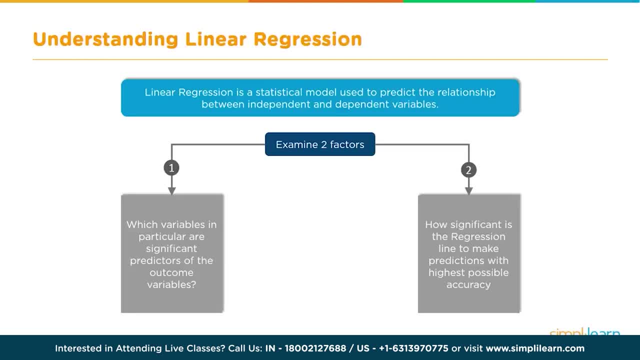 That we need to look at closely Is how significant is the regression line To make predictions with the highest possible accuracy. If it's inaccurate, We can't use it. So it's very important we find out the most accurate line we can get. 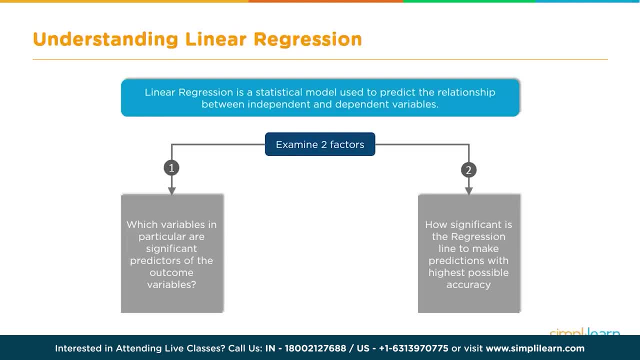 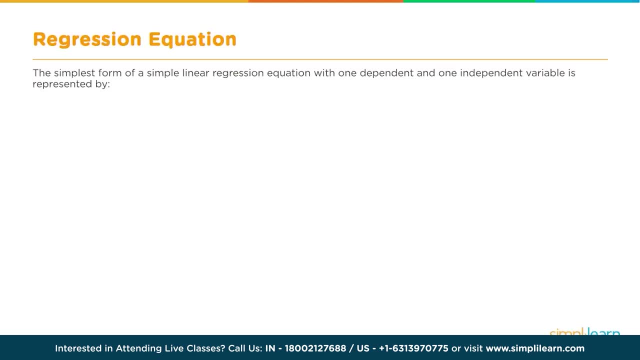 Since linear regression Is based on drawing a line through data, We're going to jump back And take a look at some Euclidean geometry. The simplest form Of a simple linear regression equation With one dependent And one independent variable Is represented by y equals. 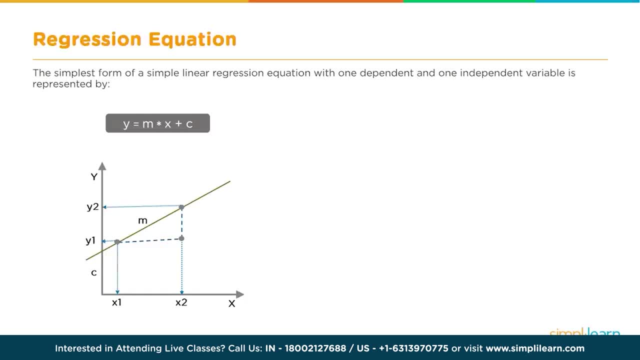 M times x plus c. And if you look at our model here, We plotted two points on here: X1 and y1.. X2 and y2.. Y being the dependent variable, Remember that from before- And x being the independent variable. 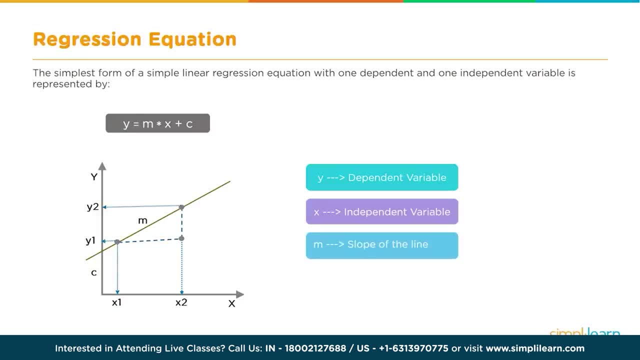 So y depends on whatever x is. M, in this case, Is the line Where m equals the difference In the y2 minus y1. And x2 minus x1. And finally we have c, Which is the coefficient of the line. 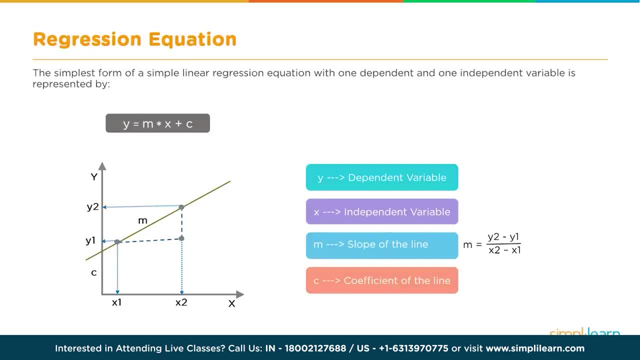 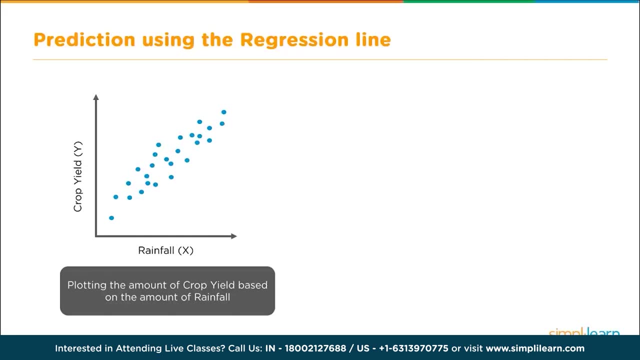 Or where it happens to cross the zero axis. Let's go back And look at an example we used earlier Of linear regression. We're going to go back to plotting the amount of crop yield Based on the amount of rainfall, And here we have our rainfall. 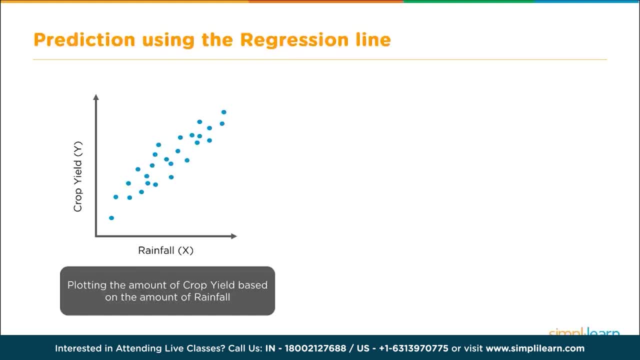 Remember, we cannot change rainfall And we have our crop yield Which is dependent on the rainfall. So we have our independent And our dependent variables. We're going to take this and draw a line through it As best we can through the middle of the data. 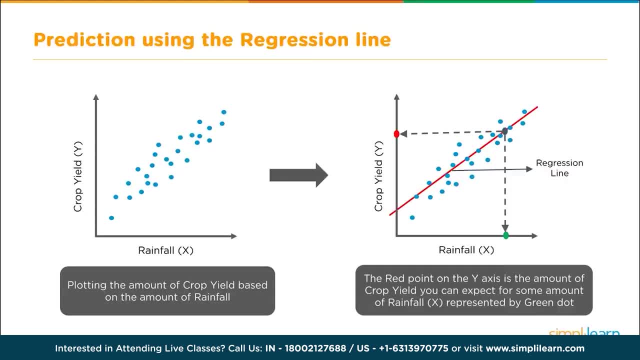 And then we look at that, We put the red point on the y-axis Is the amount of crop yield you can expect For the amount of rainfall Represented by the green dot. So if we have an idea what the rainfall is for this year, 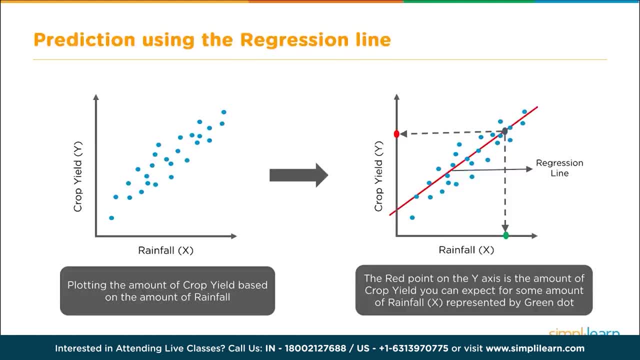 And what's going on. Then we can guess how good our crops are going to be. And we've created a nice line right through the middle To give us a nice mathematical formula. So let's take a look And see what the math looks like behind this. 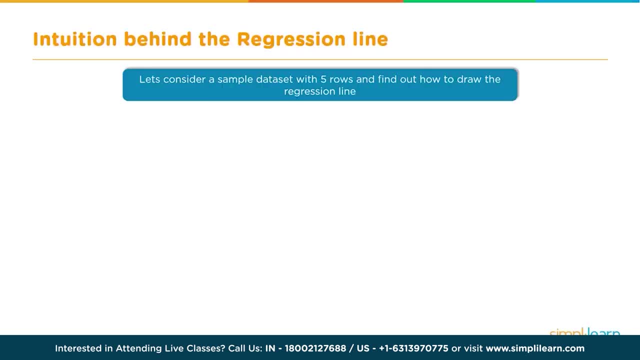 Let's look at the intuition behind the regression line. Now, before we dive into the math And the formulas that go behind this And what's going on behind the scenes, I want you to note That when we get into the case study, 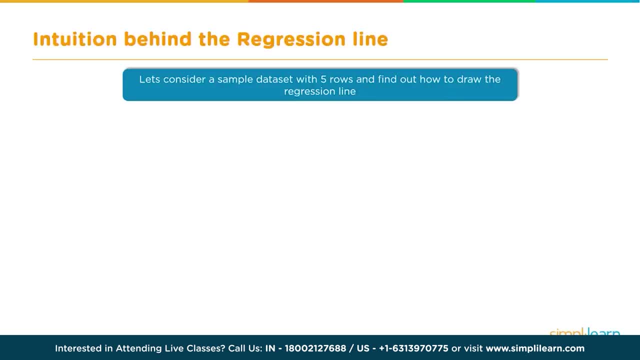 And we actually apply some python script, That this math that you're going to see here Is already done automatically for you. You don't have to have it memorized. It is, however, Good to have an idea what's going on. So if people reference a different method, 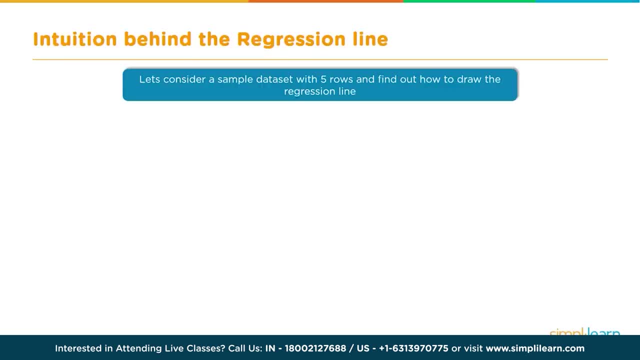 Or different terms. You'll know what they're talking about. Let's consider a sample data set With five rows And find out how to draw the regression line. We're only going to do five rows Because if we did like the rainfall, 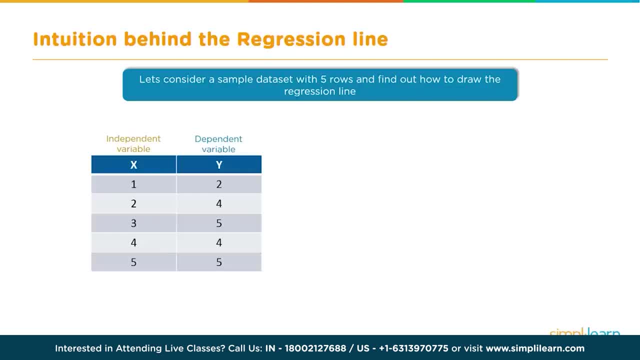 With hundreds of points of data That would be very hard to see what's going on with the mathematics. So we'll go ahead and create our own two sets of data And we have our independent variable x And our dependent variable y. And when x was one? 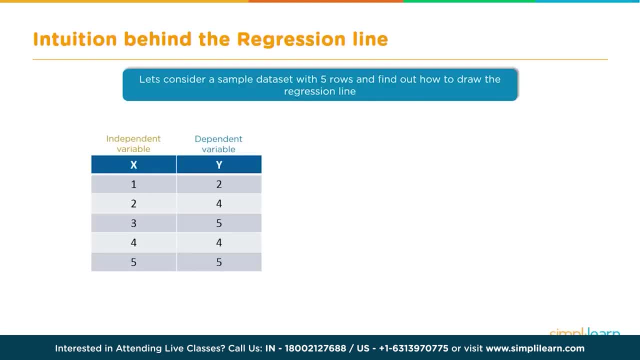 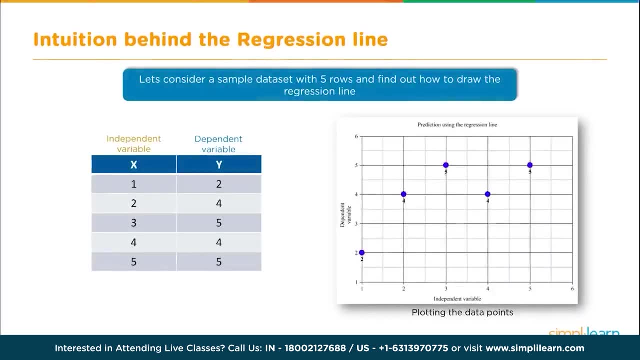 We got: y equals two When x was two, When y was four, And so on and so on. If we go ahead and plot this data on a graph, We can see how it forms a nice line. through the middle You can see where it's kind of grouped. 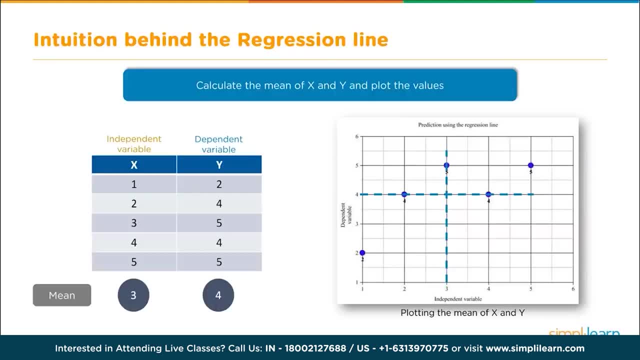 Going upwards to the right. The next thing we want to know Is what the means is Of each of the data coming in, The x and the y. The means doesn't mean anything other than the average, So we add up all the numbers. 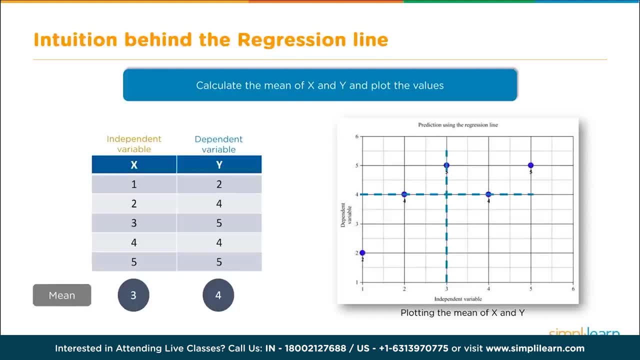 And divide by the total. So one plus two plus three plus four plus five Over five equals three, Four. If we go ahead and plot the means on the graph, We'll see we get three comma four, Which draws a nice line down the middle. 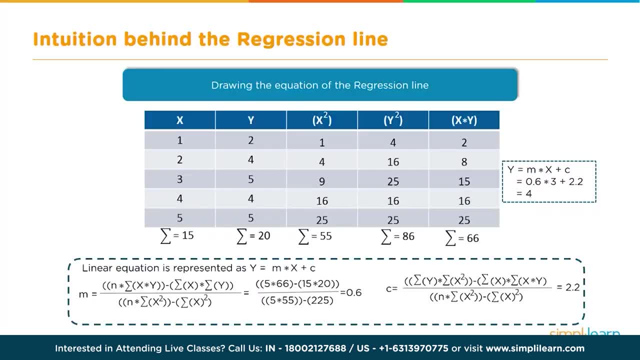 A good estimate Here. we're going to dig deeper into the math Behind the regression line. Now remember before I said, You don't have to have all these formulas memorized Or fully understand them, Even though we're going to go into a little more detail of how it works. 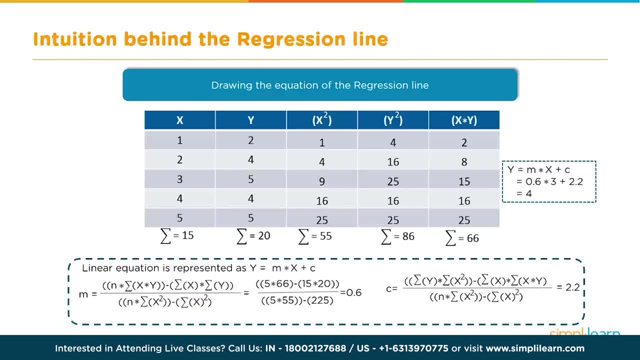 And if you're not a math wiz And you don't know, if you've never seen the sigma character before, Which looks a little bit like an e That's opened up. That just means summation. That's all that is. 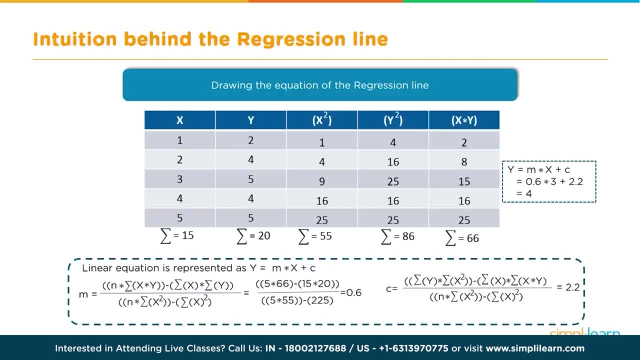 So when you see the sigma character It just means we're adding everything in that row, And for computers this is great Because as a programmer You can easily iterate through each of the xy points And create all the information you need. So in the top half you can see where we've broken that down into pieces. 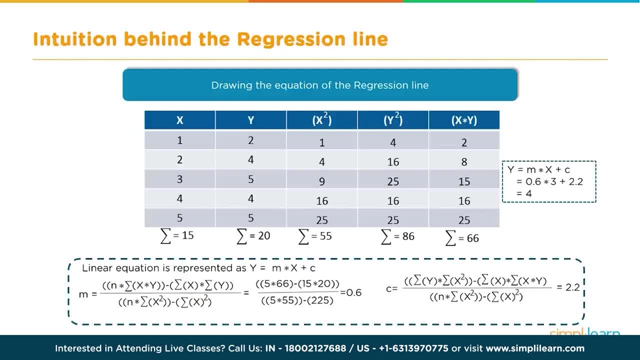 And, as it goes through the first two points, It computes the squared value of x, The squared value of y And x times y, And then it takes all of x and adds them up, All of y adds them up, And so on, and so on. 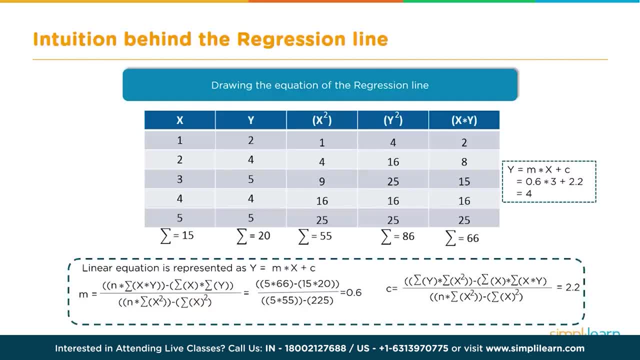 And you can see we have. The sum is equal to 15.. The sum is equal to 20.. All the way up to x times y, Where the sum equals 66. This all comes from our formula for calculating a straight line. 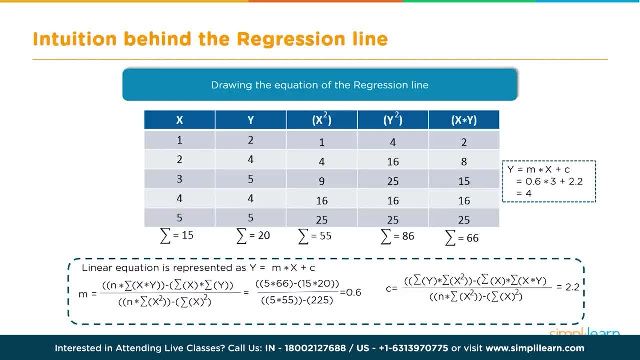 Where y equals the slope times, x Plus the coefficient c. So we go down below And we're going to compute more like the averages of these And we're going to explain exactly what that is in just a minute And where that information comes from. 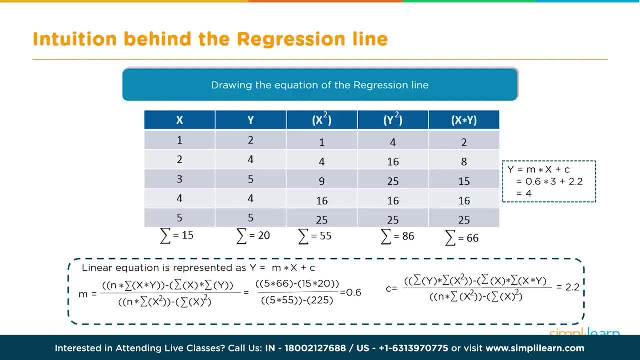 It's called the square means error, But we'll go into that in detail in a few minutes. All you need to do is look at the formula And see how we've gone about computing it Line by line, Instead of trying to have a huge 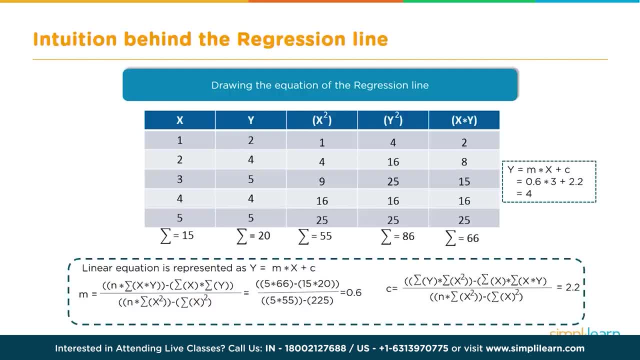 Set of numbers Pushed into it And down here you'll see where the slope m Equals And the top part. if you read through the brackets You have the number of data points Times the sum Of x times y, Which we computed one line at a time there. 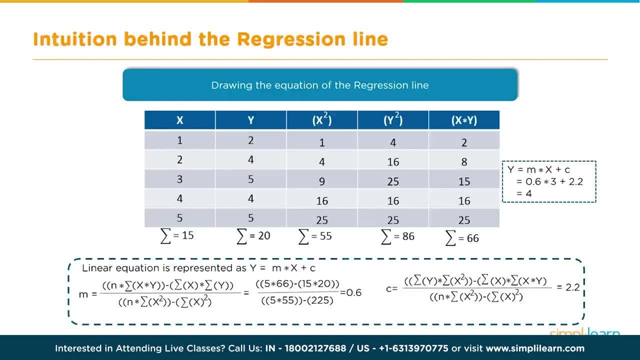 And that's just the 66. And take all that Times the sum of x, Times the sum of y, And those have both been computed, So you have 15 times 20.. And on the bottom we have the number of lines. 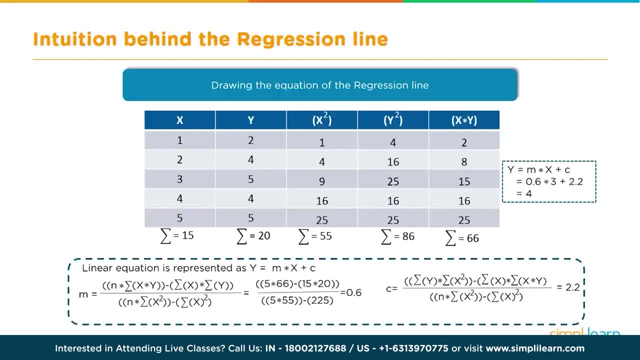 Times the sum of x squared, Easily computed as 86 for the sum Minus. I'll take all that and subtract The sum of x squared And we end up as we come across with our formula. You can plug in all those numbers. 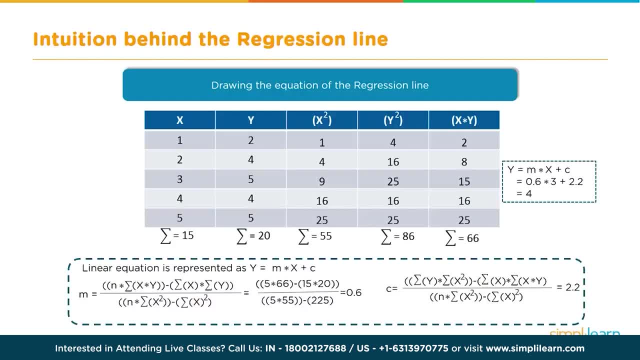 Which is very easy to do on the computer. You don't have to do the math on a piece of paper or calculator And you'll get a slope of .6. And you'll get a coefficient If you continue to follow through that formula. 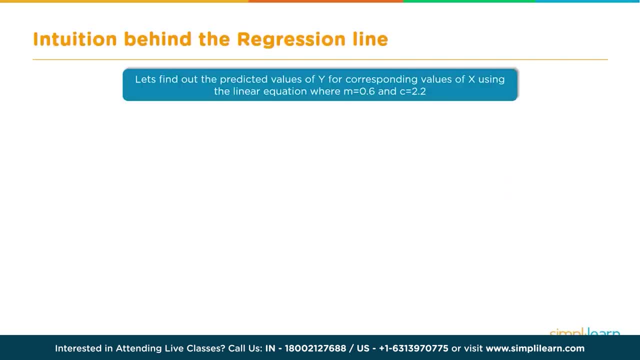 You'll see, it comes out as equal to 2.2.. Continuing deeper into what's going behind the scenes, Let's find out the predicted values of y For corresponding values of x Using the linear equation, Where m equals .6.. 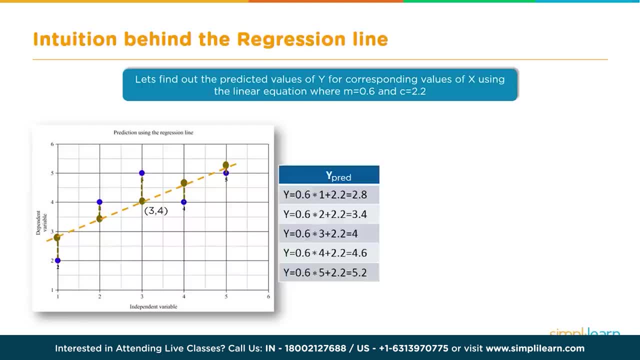 And c equals 2.2.. We're going to take these values And we're going to go ahead and plot them. We're going to predict them. So y equals .6 times where x equals 1.. Plus 2.2 equals 2.8.. 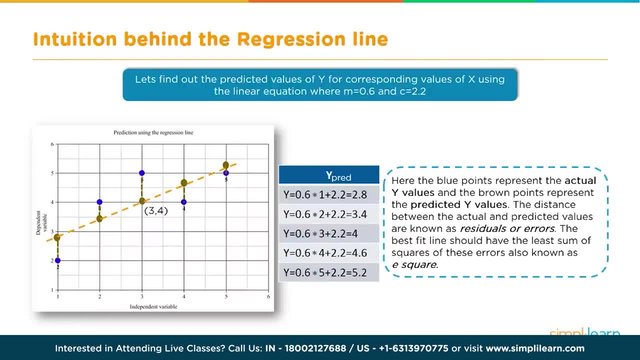 So on and so on. The red points represent the actual y values And the brown points represent the predicted y values. Based on the model we created, The distance between the actual and predicted values Is known as residuals or errors. The best fit line should have the least sum of squares. 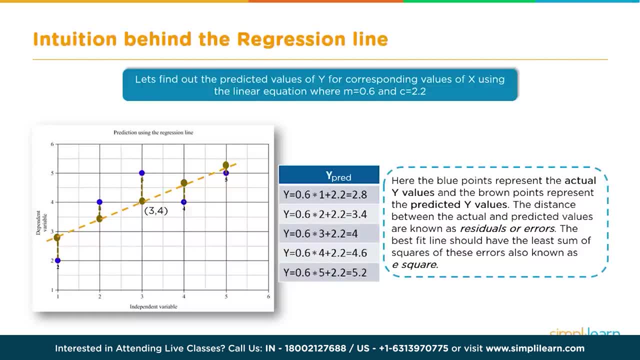 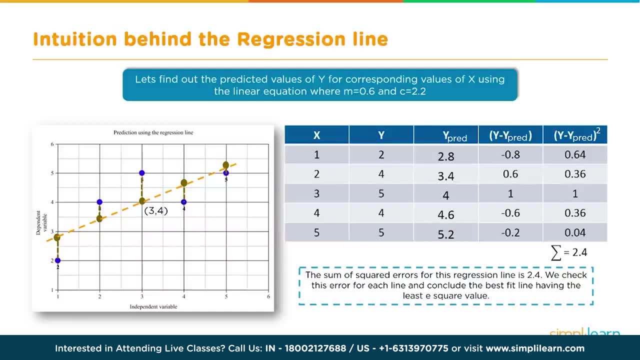 Of these errors, Also known as e squared. If we put these into a nice chart Where you can see x And you can see y, What the actual values were, And you can see y predicted, You can easily see where we take y minus y predicted. 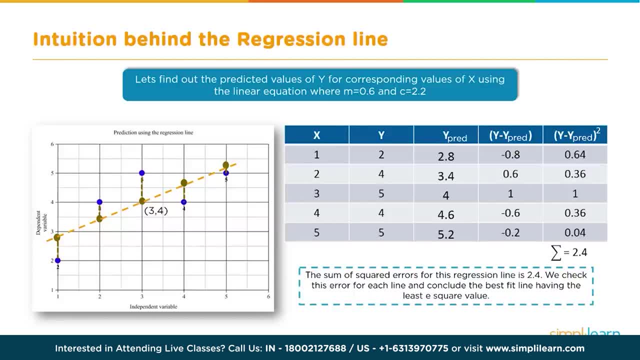 And you can see where we take y minus y predicted And we get an answer. What is the difference between those two? And if we square that Y minus y prediction squared, We can then sum those squared values. That's where we get the .64.. 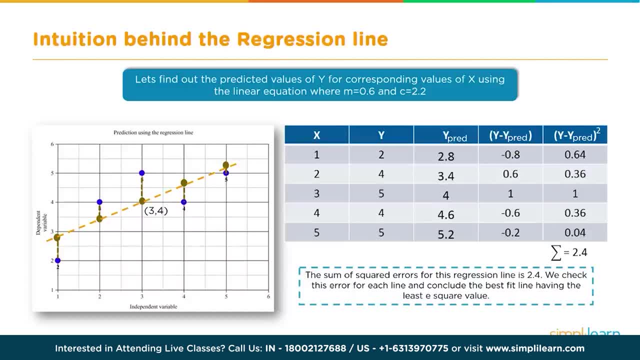 Plus the .36 plus 1. All the way down until we have a summation equals 2.4.. So the sum of squared errors For this regression line is 2.4.. We check this error for each line And conclude the best fit line. 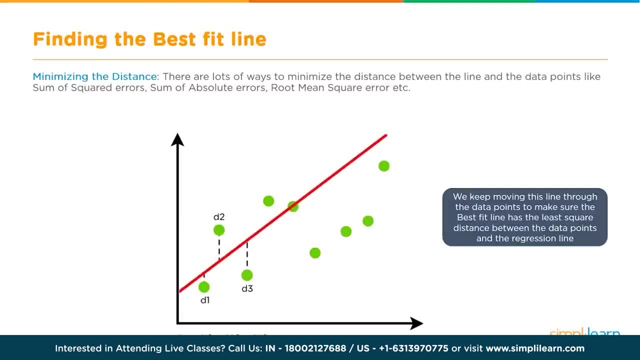 Having the least e squared value In a nice graphical representation. We can see here That we are moving this line Through the data points To make sure the best fit line Has the least squared distance Between the data points And the regression line. 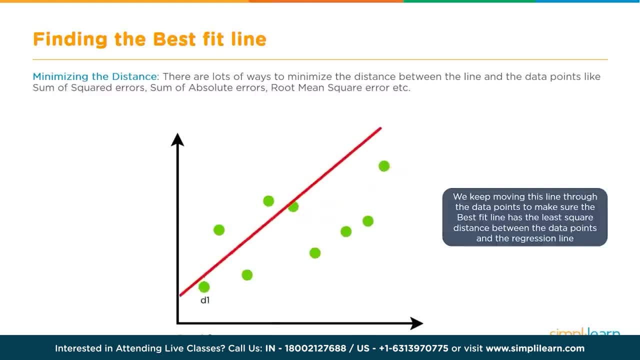 Now we only looked at the most commonly used formula For minimizing the distance. There are lots of ways to minimize the distance Between the line and the data points, Like sum of squared errors, Sum of absolute errors, Root mean square error, Etc. 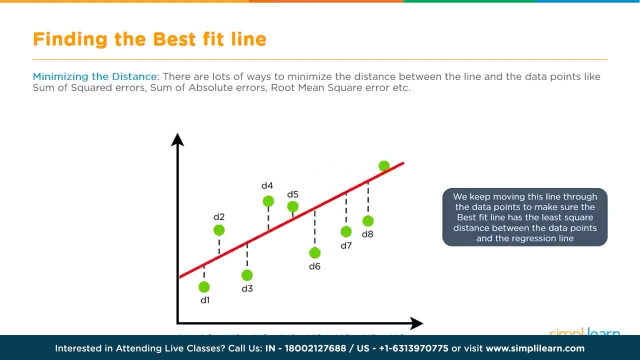 What you want to take away from this, From computer programming And iterating through the data, Calculate the different parts of it. That way, these complicated formulas you see, With the different summations and absolute values, Are easily computed one piece at a time. 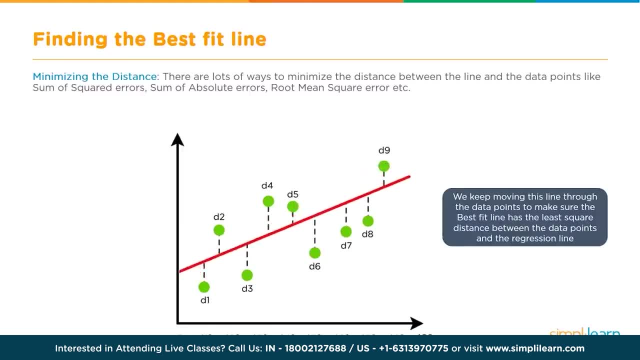 Up until this point, We have only been looking at two values: X and Y. Well, in the real world, It is very rare that you only have two values When you are figuring out a solution. So let's move on to the next topic. 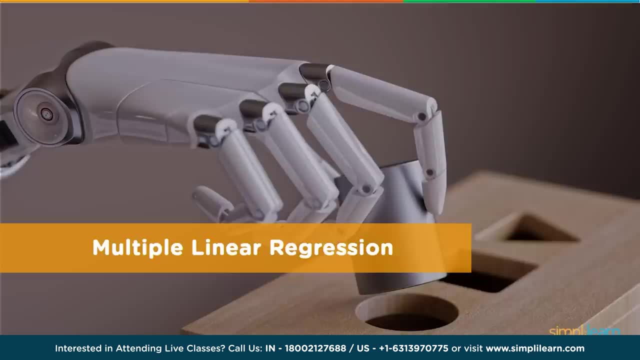 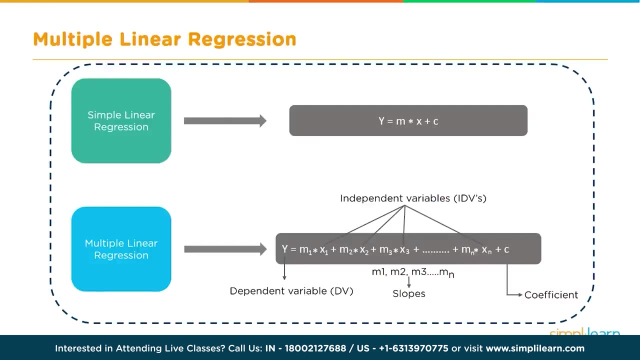 Multiple linear regression. What happens when you have multiple inputs? So in multiple linear regression We have. Well, we will start with the simple linear regression Where we had Y equals M plus X plus C And we are trying to find the value of Y. 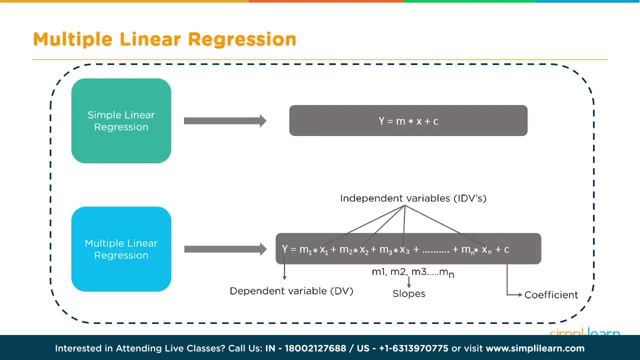 Now, with multiple linear regression, We have multiple variables coming in. So instead of having just X, We have X1, X2, X3.. And instead of having just one slope, Each variable has its own slope Attached to it, As you can see here. 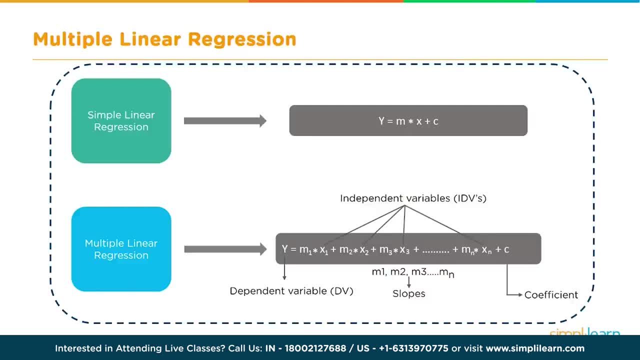 We have M1, M2, M3. And we just have the single coefficient. So when you are dealing with multiple linear regression, You basically take your single linear regression And you spread it out. So you have: Y equals M1 times X1. 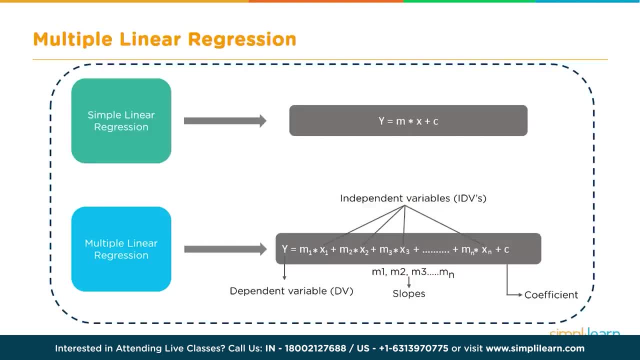 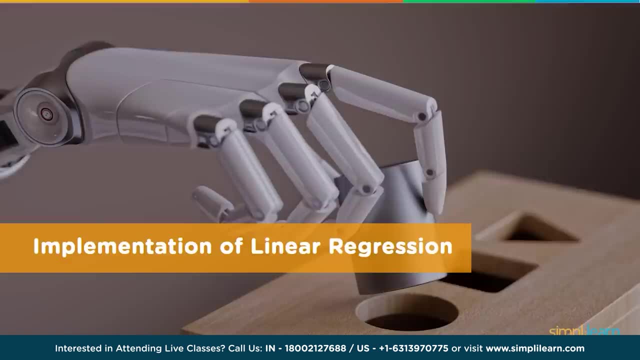 Plus M2 times X2.. So on all the way to M to the nth, X to the nth, And then you add your coefficient on there. Implementation of linear regression. Now we get into my favorite part. Let's understand how multiple linear regression works. 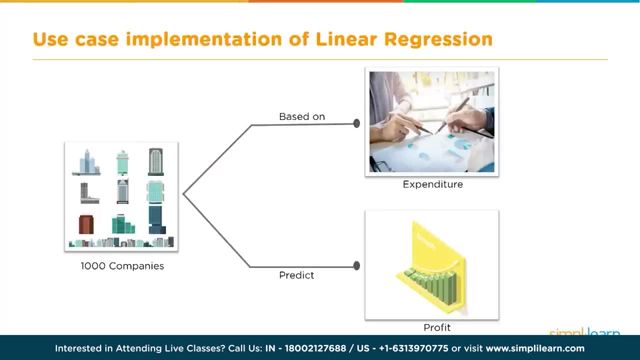 By implementing it in Python. If you remember before, We're going to start a company And, just based on its R&D, Trying to figure out its profit, We're going to start looking at the expenditure of the company. We're going to go back to that. 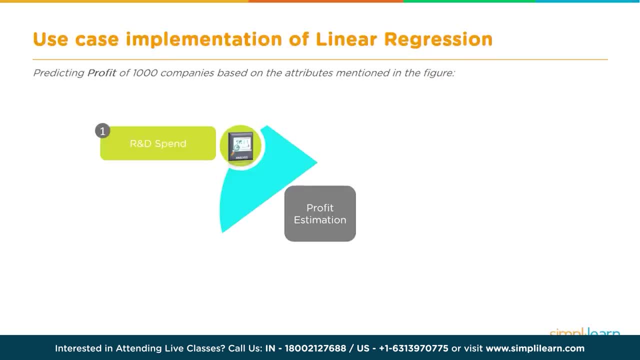 And we're going to predict its profit. But instead of predicting it just on the R&D, We're going to look at other factors Like administration costs, Marketing costs And so on, And from there We're going to see if we can figure out what the profit of that company is going to be. 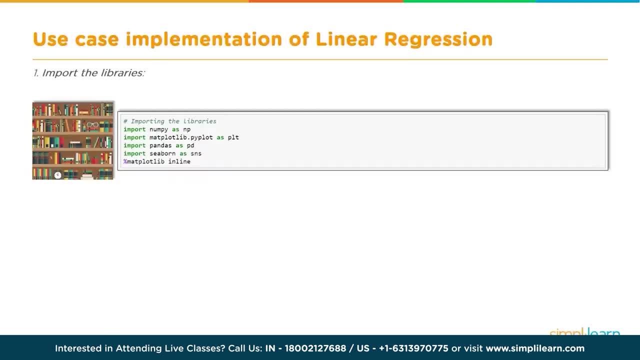 To start our coding. Before we do any kind of linear regression, We're going to take a look at the data To see what we're playing with. Then we'll go ahead and format the data to the format we need To be able to run it in the linear regression model. 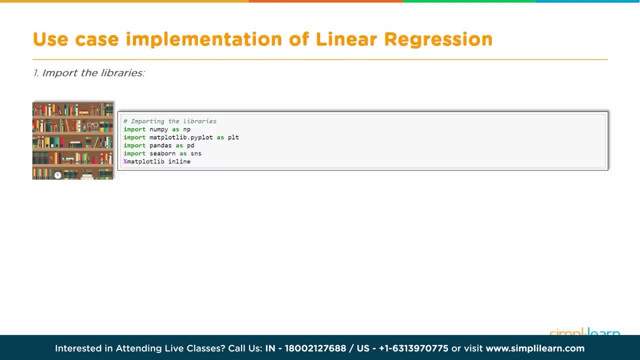 And then from there We'll go ahead and solve it And just see how valid our solution is. So let's start with importing the basic libraries Now. I'm going to be doing this in Anaconda Jupyter Notebook, A very popular IDE. 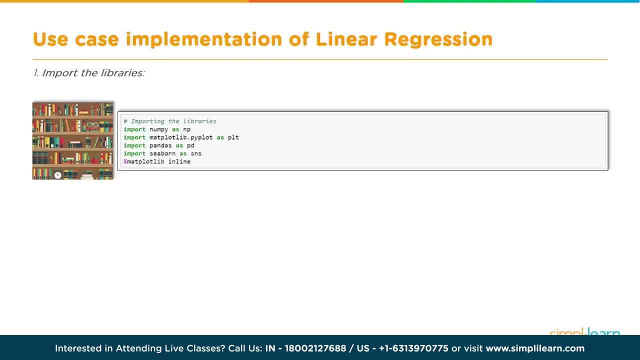 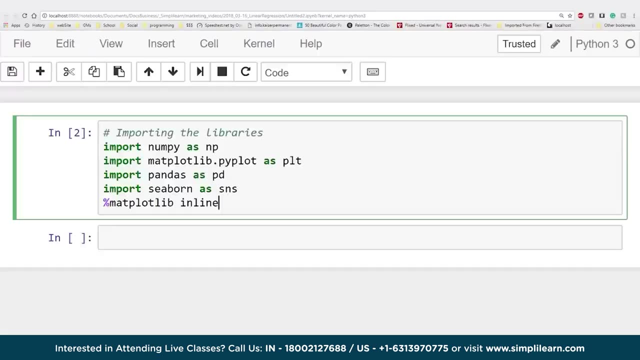 I enjoy it because it's such a visual to look at And so easy to use. Just any IDE for Python will work just fine for this, So break out your favorite Python IDE. So here we are in our Jupyter Notebook. Let me go ahead and paste our 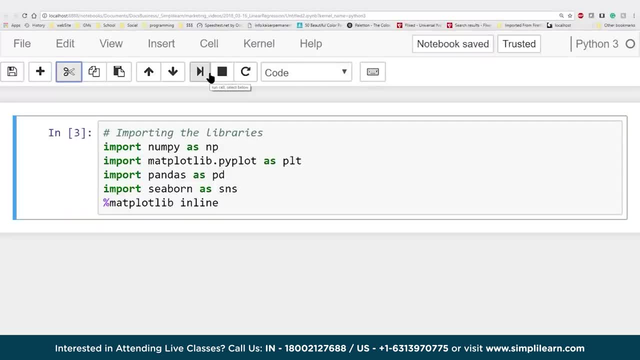 First piece of code in there And let's walk through what libraries we're importing. First we're going to import numpy As np And then I want you to skip one line and look at Import pandas as pd. These are very common tools that you need with most of your linear regression. 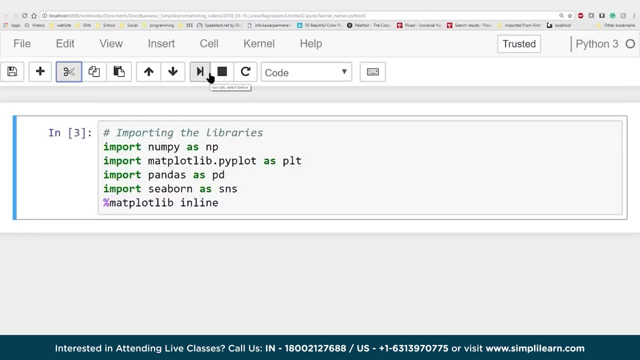 The numpy, Which stands for number. Python Is usually denoted as np And you have to almost have that for your sklearn toolbox, So you always import that right off the beginning, Pandas, Although you don't have to have it for your sklearn libraries. 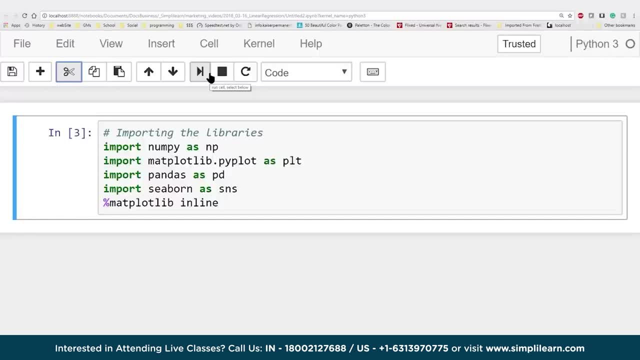 It does such a wonderful job of importing data, Setting it up into a data frame So we can manipulate it rather easily, And it has a lot of tools also in addition to that, So we usually like to use the pandas when we can. 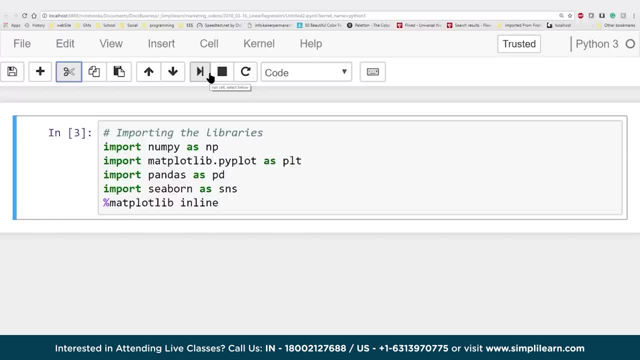 And I'll show you what that looks like. The other three lines Are for us to get a visual of this data And take a look at it. So we're going to import matplotlibrarypyplot As plt And then seaborn as sns. 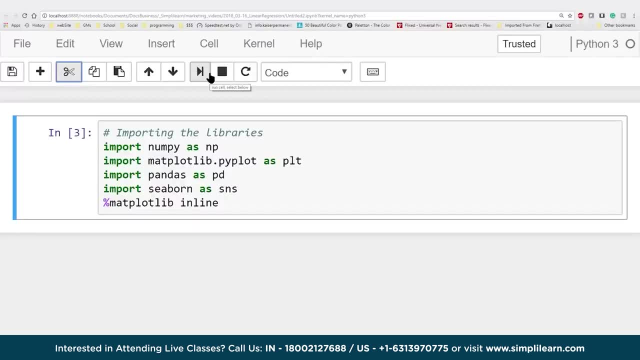 Seaborn works with the matplotlibrary, So you have to always import matplotlibrarypyplot And then seaborn sits on top of it And we'll take a look at what that looks like. You could use any of your own Plotting libraries you want. 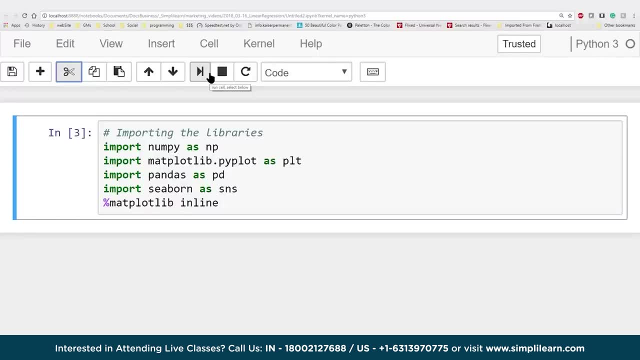 There's all kinds of ways to look at the data. These are just very common ones. And the seaborn is so easy to use. It just looks beautiful. It's a nice representation that you can actually take and show somebody. And the final line: 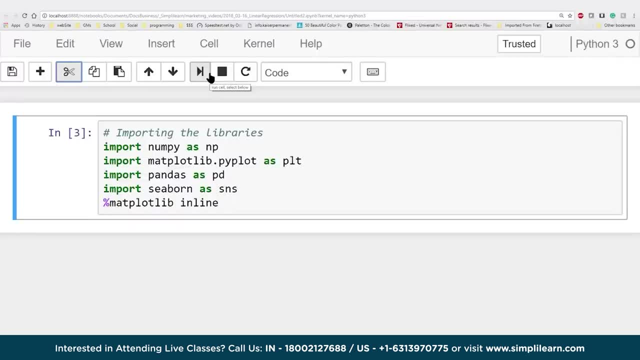 Is the ambersign matplotlibrary inline. That is only because I'm doing an inline IDE. My interface in the anaconda jupyter notebook Requires I put that in there Or you're not going to see the graph when it comes up. 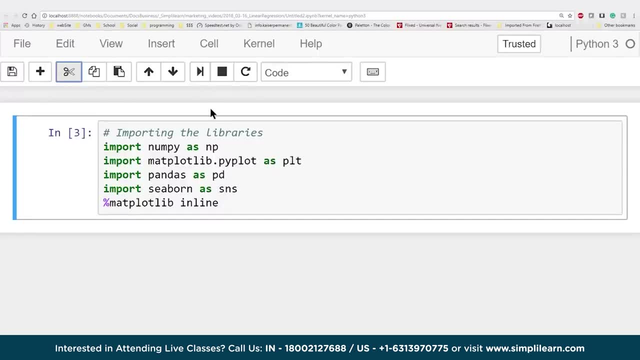 Let's go ahead and run this. It's not going to be that interesting Because we're just setting up variables- In fact, it's not going to do anything That we can see- But it is importing these different libraries and setup The next step. 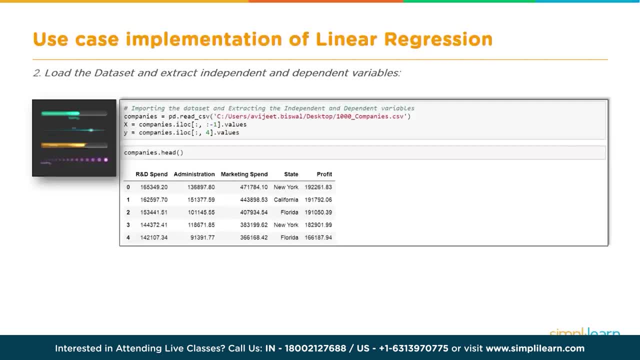 Is load the dataset And extract independent and dependent variables. Now here in the slide You'll see companies equals pdreadcsv And it has a long line there With the file at the end: Companiescsv. You're going to have to change this. 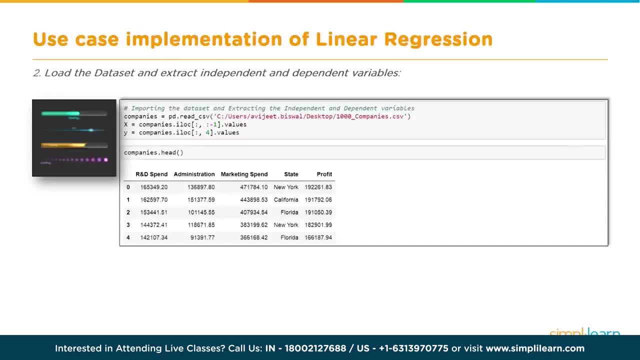 To fit whatever setup you have And the file itself You can request. Just go down to the commentary below this video And put a note in there And simply learn. will try to get in contact with you And supply you with that file. 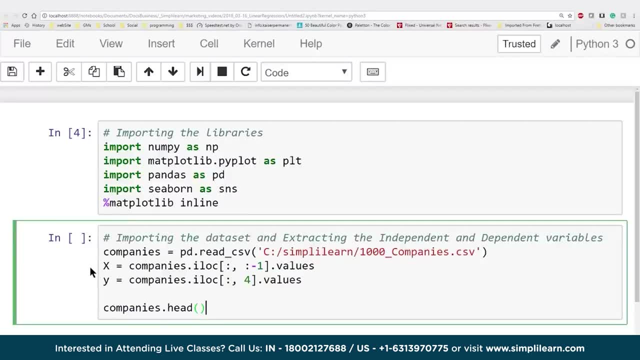 So you can try this coding yourself. So we're going to add this code in here And we're going to see that I have Companies equals pdreadercsv And I've changed this path to match my computer. C colon slash. simply learn slash 1000. 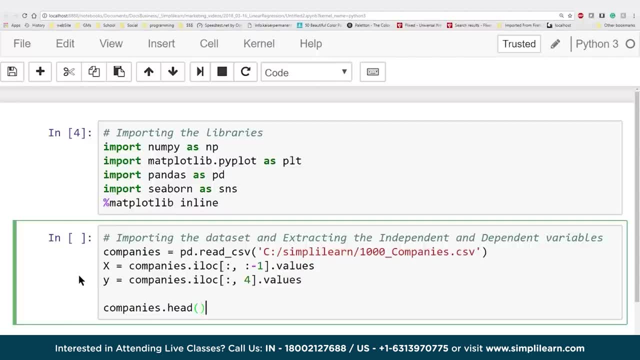 And then below there We're going to set the x equals to companies Under the i location And because this is companies is a pd dataset, I can use this nice notation that says: Take every row, That's what the colon, The first colon, is comma. 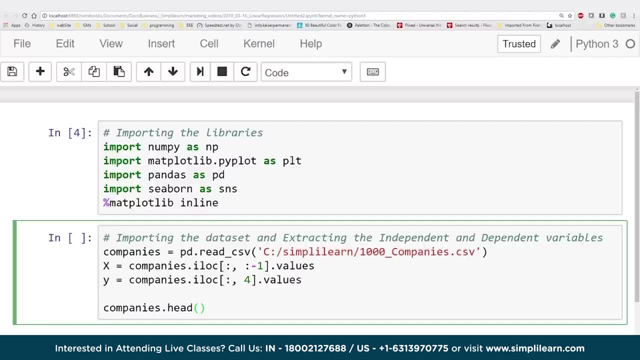 Except for the last column. That's what the second part is, Where we have a colon minus one And we want the values set into there. So x is no longer a dataset, A pandas dataset, But we can easily extract the data. 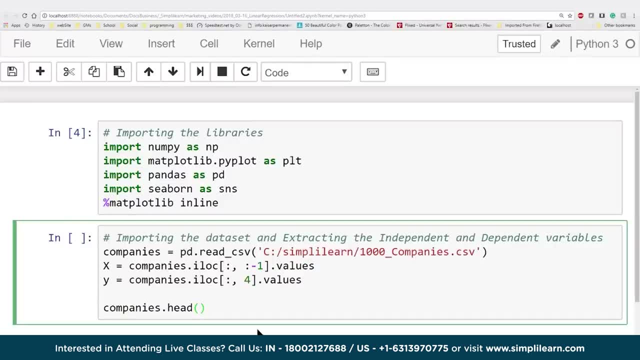 Into the last row. Well, the question is going to be: What are we actually looking at? So let's go ahead and take a look at that, And we're going to look at the companies dot head, Which lists the first five rows of data. 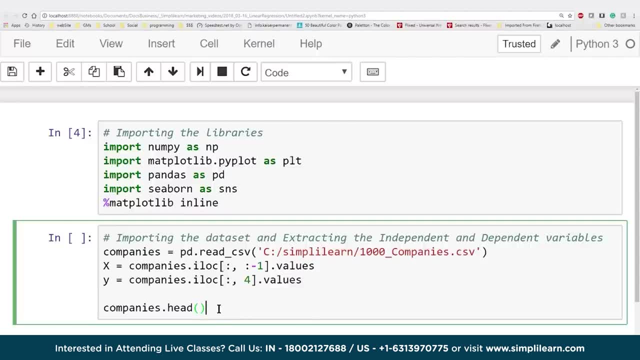 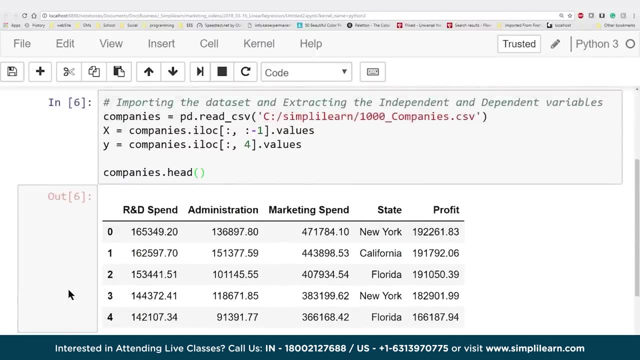 And I'll open up the file in just a second So you can see where that's coming from. But let's look at the data in here. As far as the way the pandas sees it, When I hit run, You'll see it breaks it out into a nice setup. 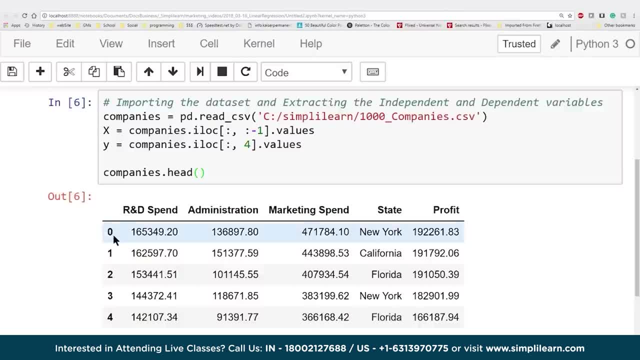 This is what pandas- One of the things pandas is really good about- Is. it looks just like an excel spreadsheet- We don't start with one, So it shows the first five rows: Zero, one, two, three, four, And then it shows your different columns. 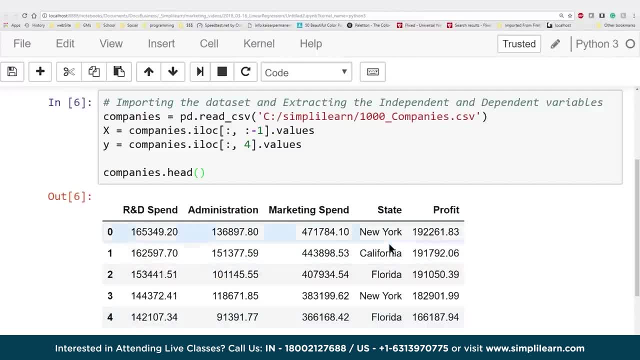 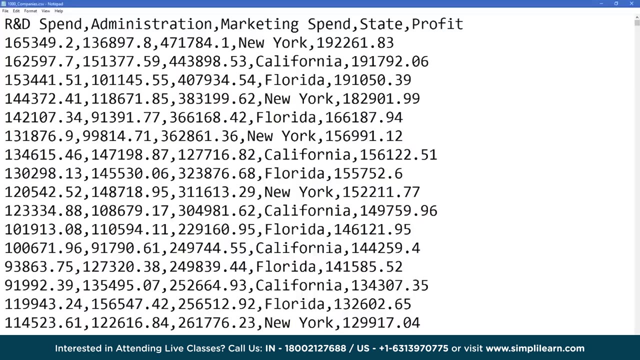 R and D spend Administration, Marketing spend, State Profit. It even notes that the top are column names. It was never told that, But pandas is able to recognize a lot of things That they're not the same as the data rows. 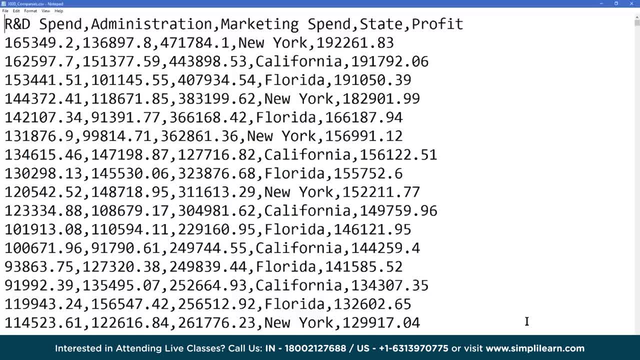 Why don't we go ahead and open this file up in a csv So you can actually see the raw data? D spend Administration, Marketing, spend State, Profit, Carries, return. I don't know about you, But I'd go crazy trying to read files like this. 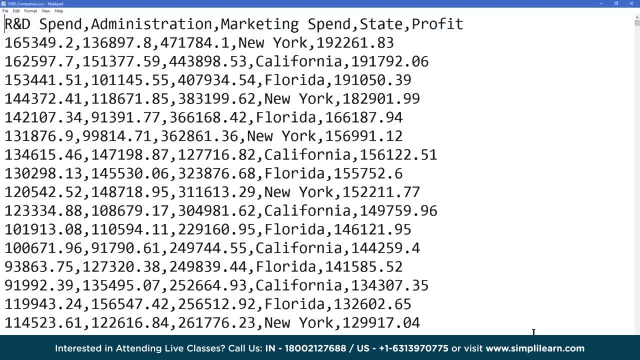 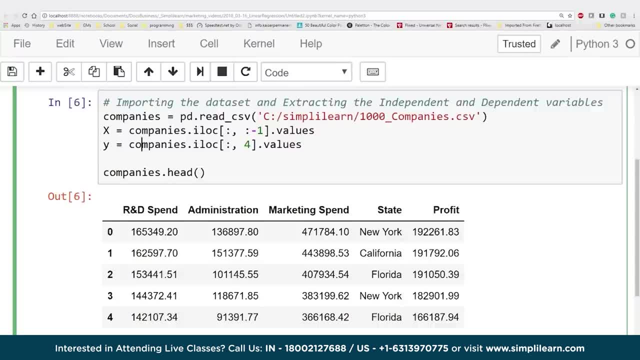 That's why we use the pandas. You could also open this up in an excel And it would separate it, Since it is a comma separated variable file. But we don't want to look at this one. We want to look at something we can read rather easily. 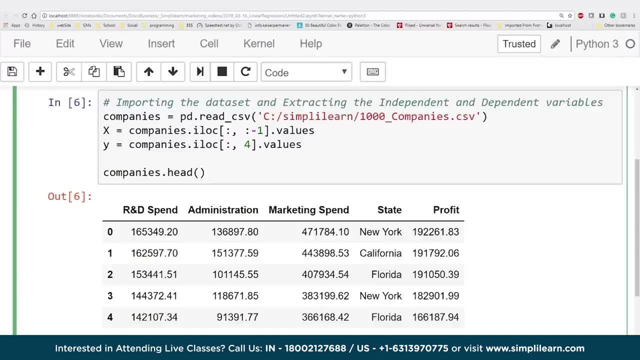 Maybe you're an expert in business And investments And you understand what $165,349.20.. Compared to the administration cost Of $136,897.80.. So on and so on- Helps to create the profit Of $192,261.83.. 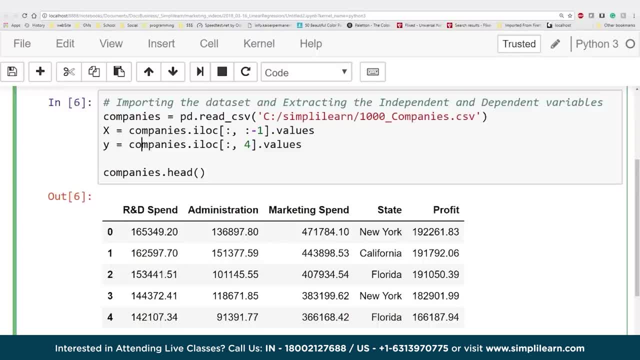 That makes no sense to me whatsoever, No pun intended. So let's flip back here And take a look at our next set of code, Where we're going to graph it So we can get a better understanding of our data And what it means. 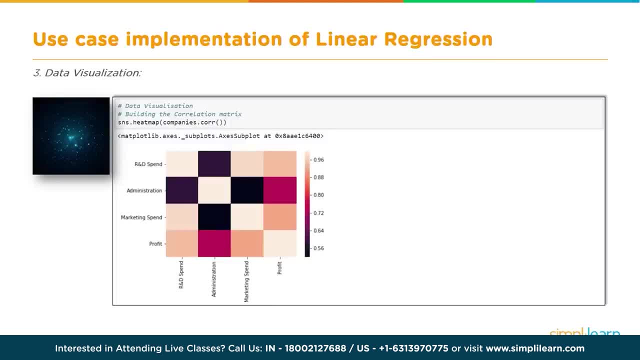 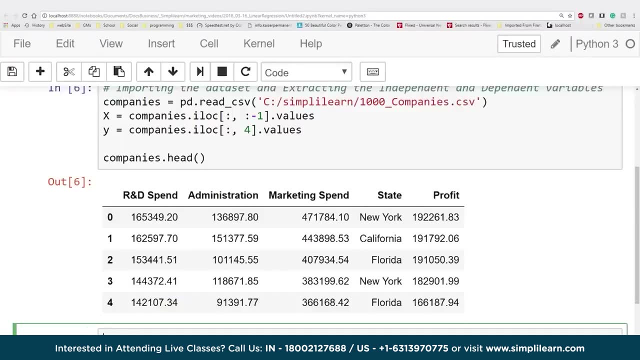 So at this point We're going to use a single line of code To get a lot of information, So we can see where we're going with this. Let's go ahead and paste that into our notebook And see what we got going. 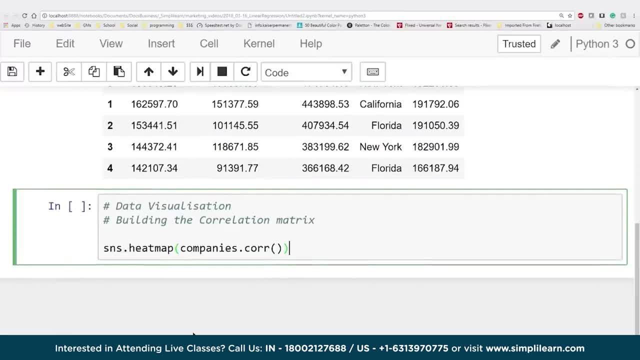 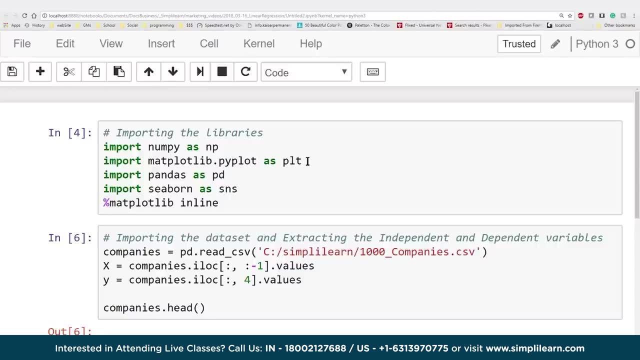 So we have the visualization And again we're using SNS, Which is pandas, As you can see. we imported the matplotlibrarypyplot As PLT, Which then the seaborn uses, And we imported the seaborn as SNS, And then that final line of code. 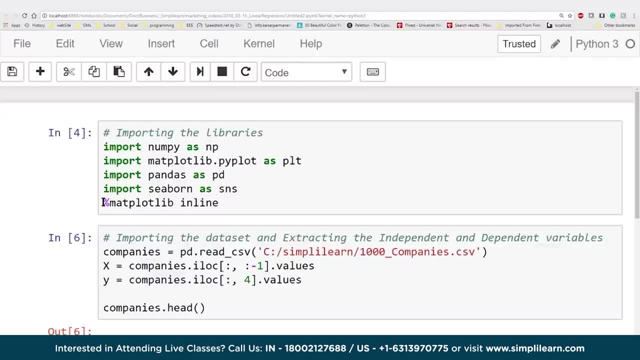 Helps us show this, Our inline coding. Without this it wouldn't display And you could display it to a file and other means, And that's the matplotlibrary inline with the amber sign at the beginning. So here we come down to the single line of code. 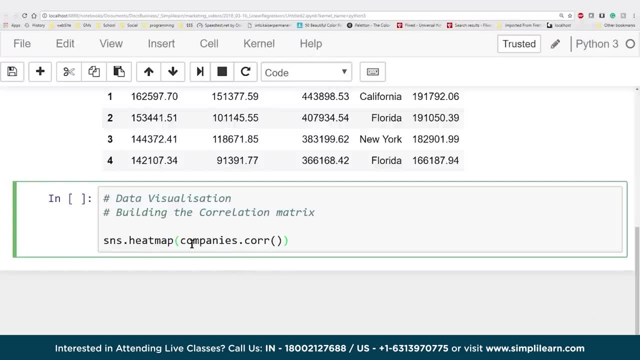 Seaborn is great Because it actually recognizes the panda data frame. So I can just take the Companiescore for coordinates And I can put that right into the seaborn. And when we run this We get this beautiful plot. And let's just take a look at what this plot means. 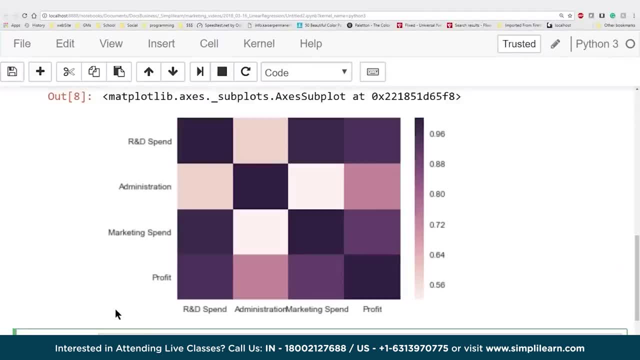 If you look at this plot On mine, It's a little bit more purplish and blue Than the original one. We have the columns and the rows, We have R&D spending, We have administration, We have marketing spending and profit. 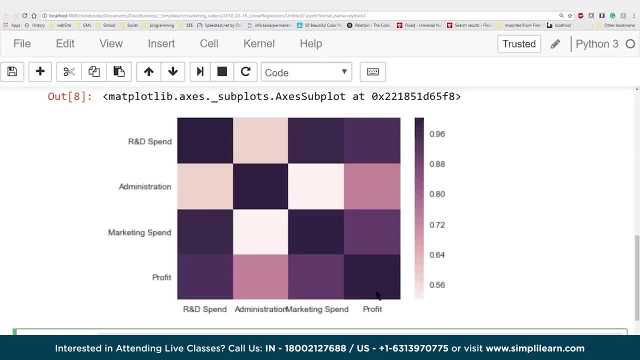 And if you cross index any two of these, Since we're interested in profit, If you cross index profit with profit, It's going to show up If you look at the scale on the right Way, up in the dark. Why? Because those are the same data. 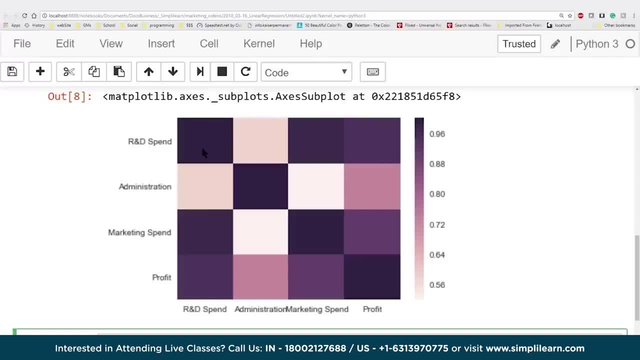 They have an exact correspondence And if you look down the middle, You get this dark row, Or dark diagonal row. That shows that this is the highest corresponding data. That's exactly the same And as it becomes lighter, There's less connections between the data. 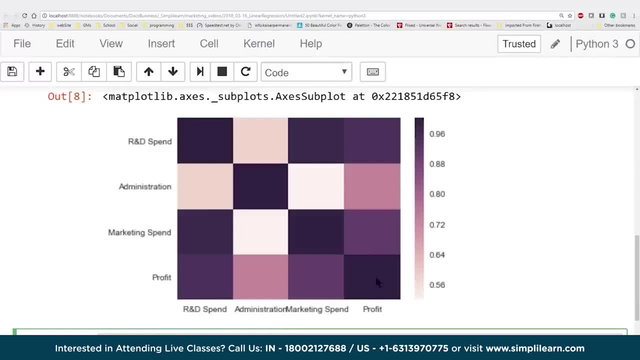 So we can see with profit, Obviously profit is the same as profit. And next, it has a very high correlation With R&D spending, Which we looked at earlier, And it has a slightly less connection to marketing spending And even less to how much money we put into the administration. 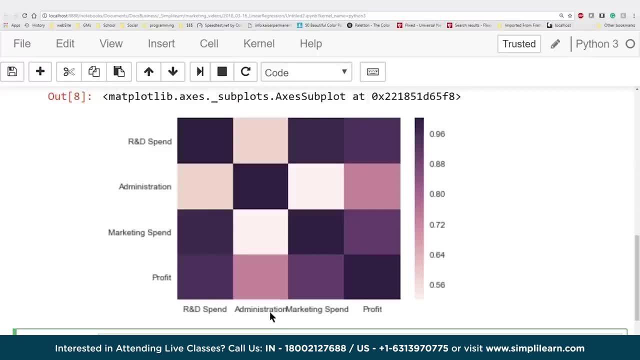 So, now that we have a nice Look at the data, Let's go ahead and dig in And create some actual, useful linear regression models So that we can predict values And have a better profit Now that we've taken a look at the visualization of this data. 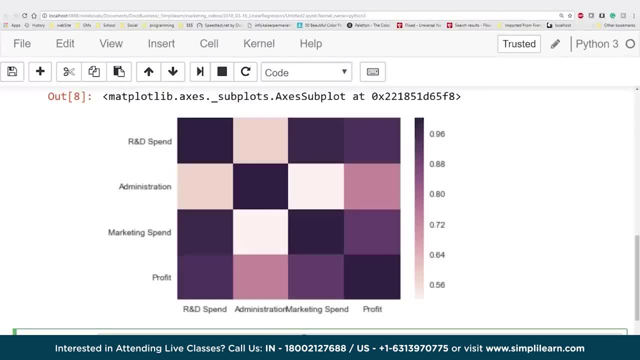 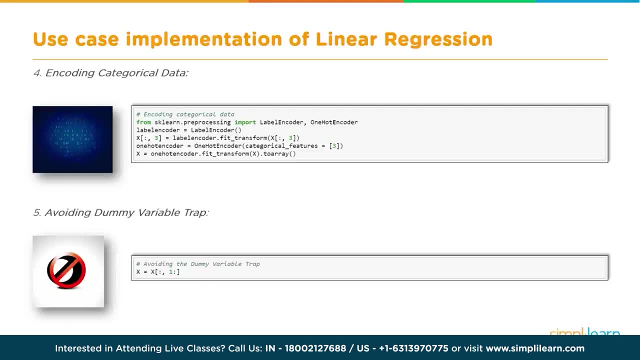 We're going to move onto the next step. Instead of just having a pretty picture, We need to generate some hard data, Some hard values. So let's see what that looks like. We're going to set up our linear regression model In two steps. 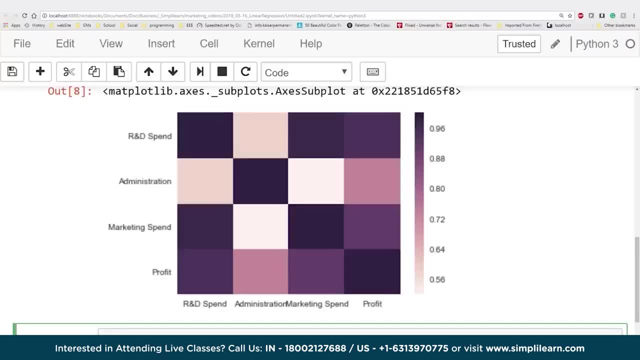 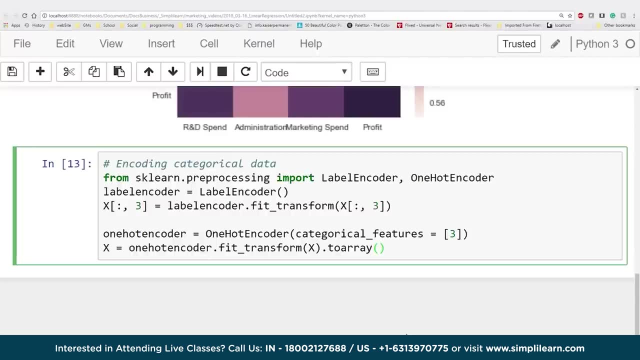 The first one is we need to prepare some of our data So it fits correctly. We're going to import this code into our Jupyter notebook And what we're bringing in Is we're going to bring in the sklearn pre-processing Where we're going to import the label encoder. 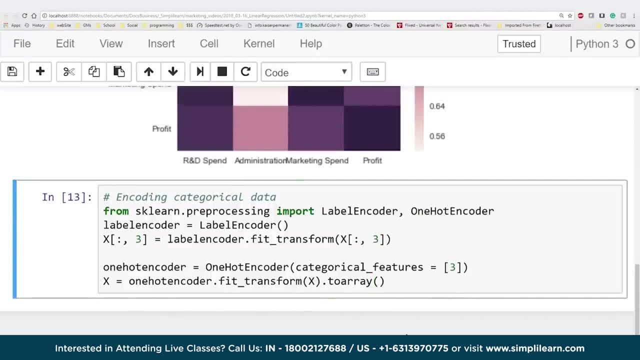 And the one hot encoder To use the label encoder, We're going to create a variable called label encoder And set it equal to capital L label, Capital E encoder. This creates a class that we can reuse For transferring the labels back and forth. 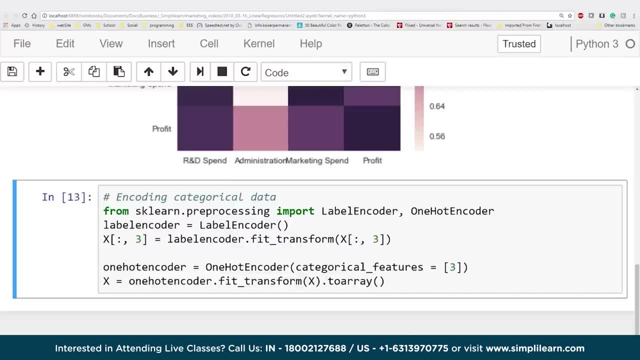 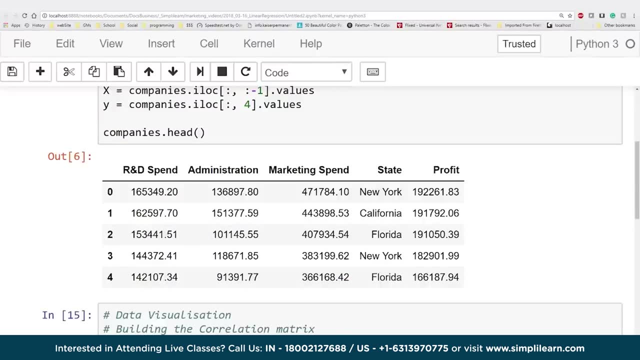 Now about now, you should ask: What labels are we talking about? Let's go take a look at the data we processed before And see what I'm talking about here. So we did the companies dot head And we printed the top five rows of data. 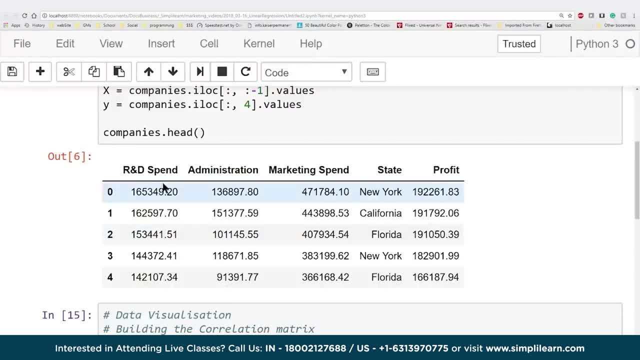 We have our columns going across. We have column zero, Which is R&D spending, Column one, which is administration, Column two, which is marketing spending, And column three is state, And you'll see under state We have New York, California, Florida. 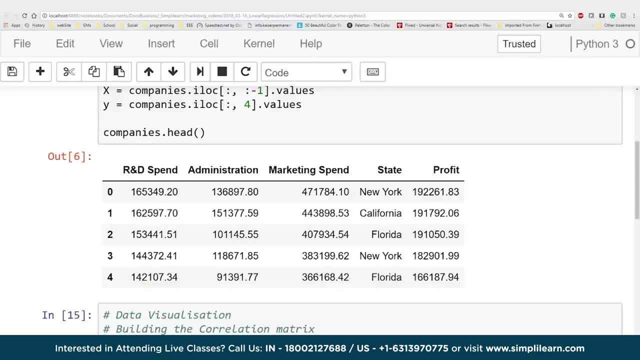 Now to do a linear regression model. It doesn't know how to process New York. It knows how to process a number. So the first thing we're going to do Is we're going to change that: New York, California and Florida. 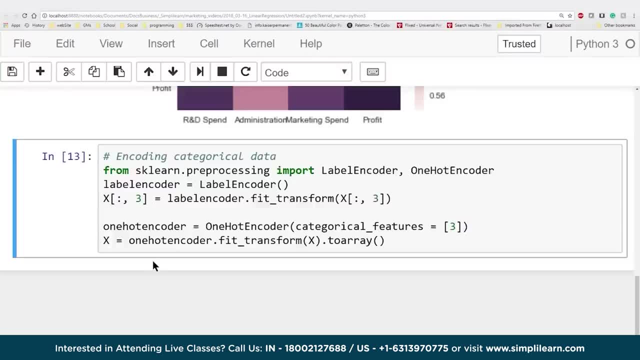 We're going to change those to numbers. That's what this line of code does here. X equals. And then it has the colon comma three in brackets, The first part. the colon comma Means that we're going to look at all the different rows. 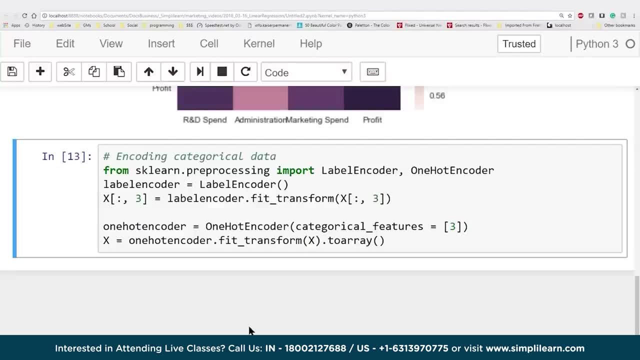 So we're going to keep them all together. But the only row we're going to edit Is the third row And in there we're going to take the label coder And we're going to fit and transform the X. Also the third row. 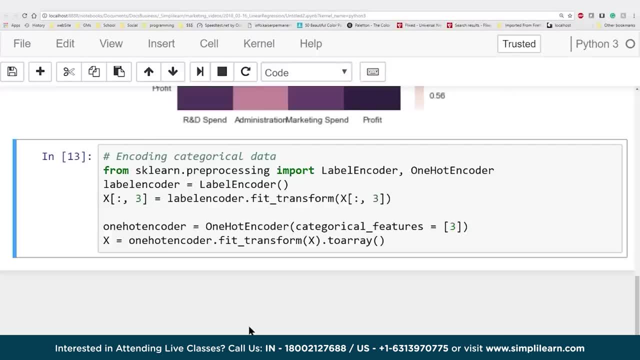 So we're going to take that third row And we're going to set it equal to a transformation That tells it that instead of having a New York, It has a zero or a one or a two, And then, finally, We need to do a one hot encoder. 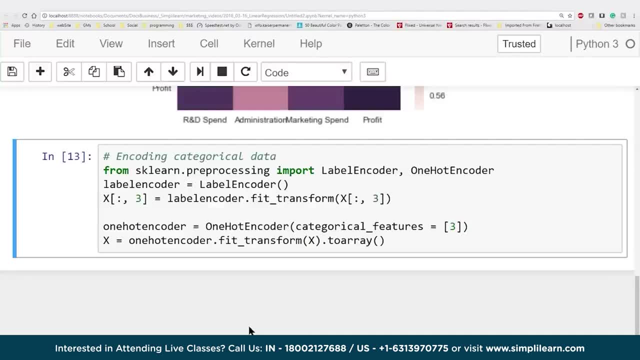 Which equals one hot encoder. Categorical features equals three. And then we take the X And we go ahead and do that: equal to one hot encoder. Fit, transform X to array. This final transformation Preps our data for us, So it's completely set the way we need it. 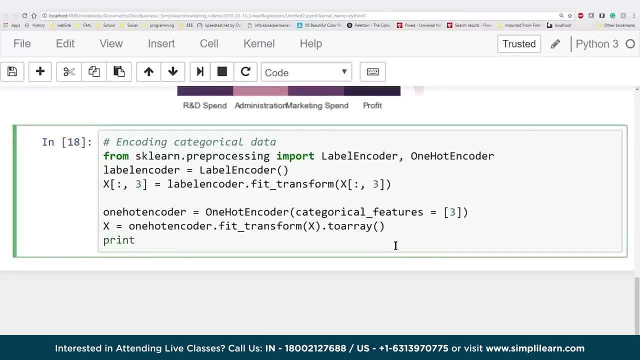 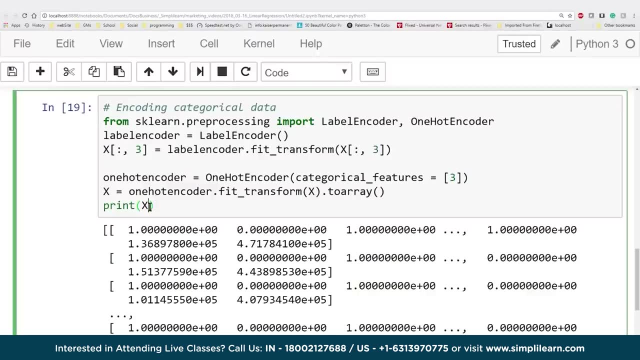 As just a row of numbers. Even though it's not in here, Let's go ahead and print X And see what it's doing. You'll see you have an array of arrays And then each array is a row of numbers. And if I go ahead and just do row zero, 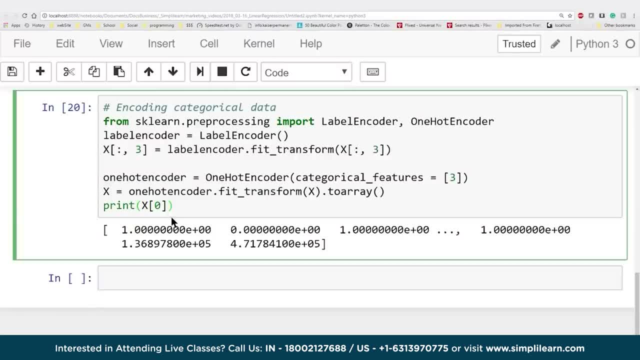 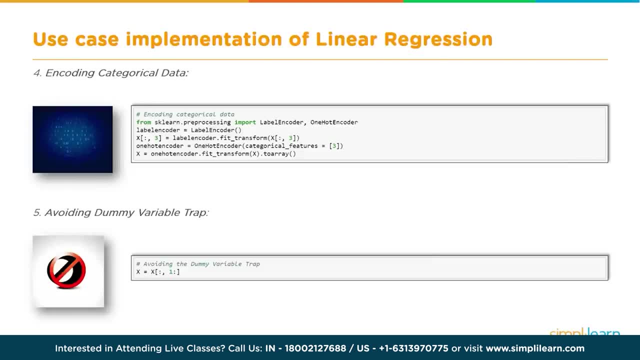 You'll see, I have a nice organized row of numbers That the computer now understands. We'll go ahead and take this out there, Because it doesn't mean a whole lot to us. It's just a row of numbers. Next, on setting up our data, 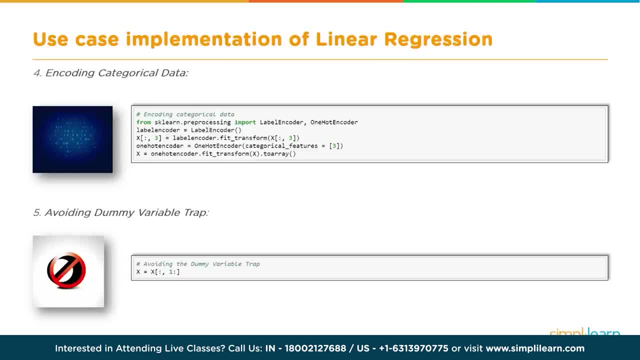 We have avoiding dummy variable trap. This is very important. Why? Because the computer has automatically transformed Our header into the setup From all these different variables. So when we did the encoder, The encoder created two columns And what we need to do. 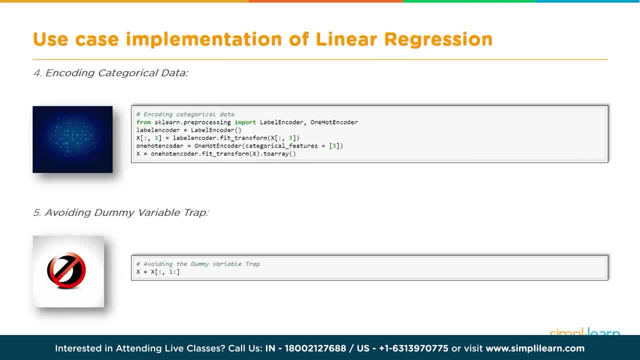 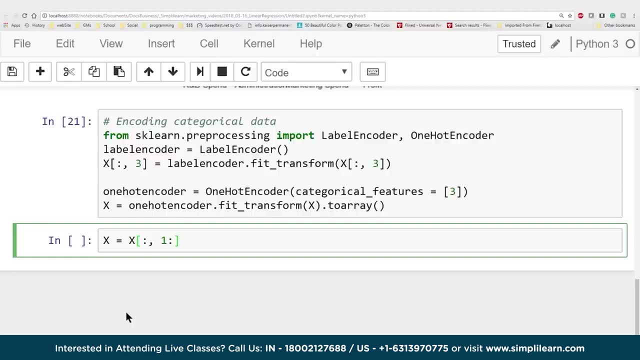 Is: just have the one, Because it has both the variable and the name. That's what this piece of code does here. Let's go ahead and paste this in here. We have X equals X, colon, comma, one colon. All this is doing. 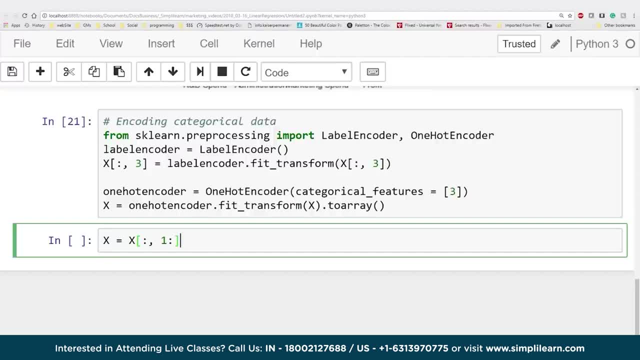 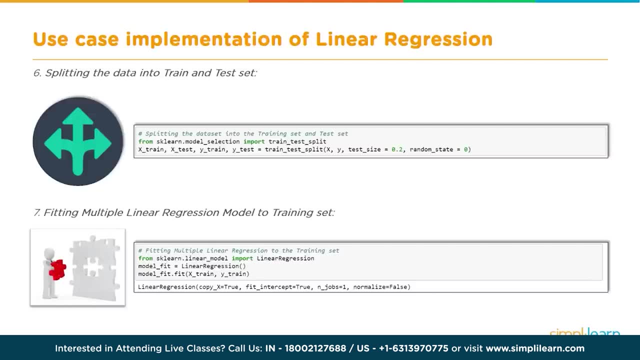 Is removing that one extra Column we put in there When we did our one hot encoder And our label encoding. Let's go ahead and run that And let's see what that looks like here, And we're going to do that in two steps. 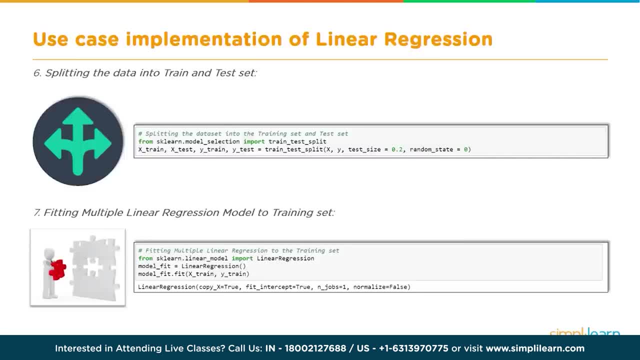 The first step Is going to be in splitting the data. Now, whenever we create A predictive model of data, We always want to split it up. So we have a training set And we have a testing set. That's very important. 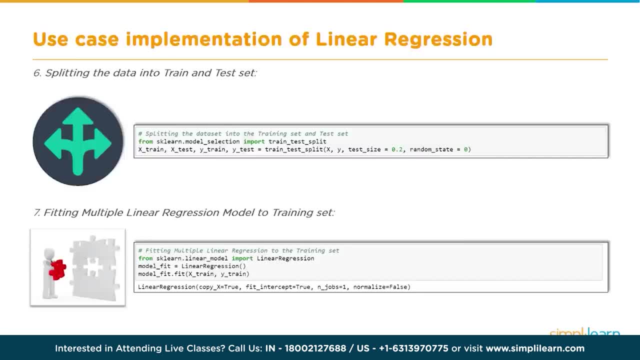 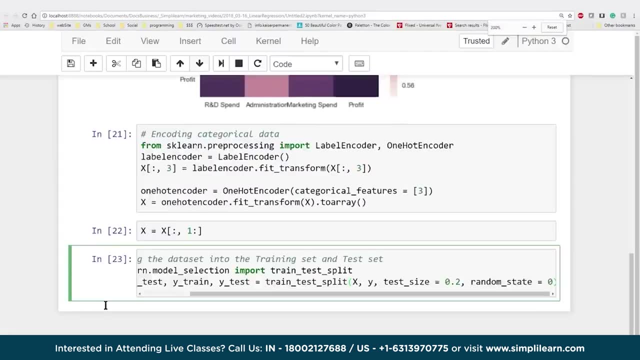 Otherwise we'd be very unethical- without testing it To see how good our fit is, And then we'll go ahead and create our multiple linear regression model And train it And set it up. Let's go ahead and shrink it down a size or two. 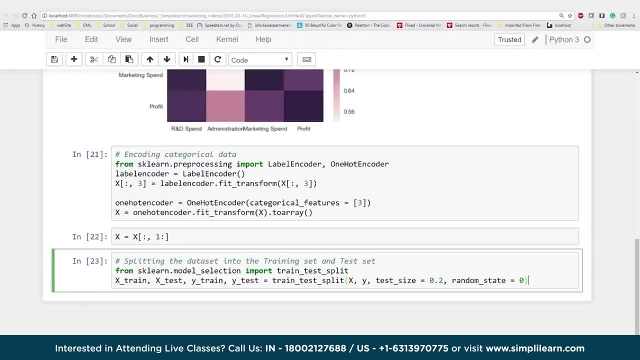 So it all fits on one line. So from the sklearn module selection We're going to import train test split And you'll see that we've created Four completely different variables. We have capital X train. Capital X test, Smaller case, Y train. 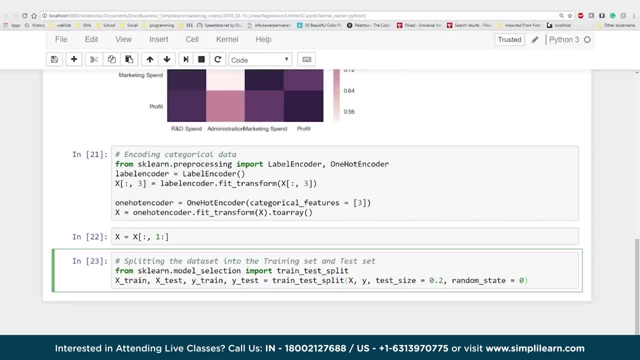 Smaller case, Y test. That is the standard way That they usually reference these. When we're doing different models, You usually see that a capital X. You see the train and the test. What this is Is X. is our data going in? 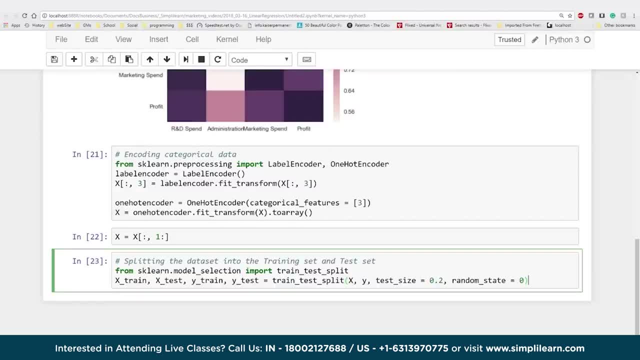 That's our R&D spin, Our administration, Our marketing, And then Y, which we're training, is the answer. That's the profit, Because we want to know the profit of an unknown entity. That's what we're going to shoot for in this tutorial. 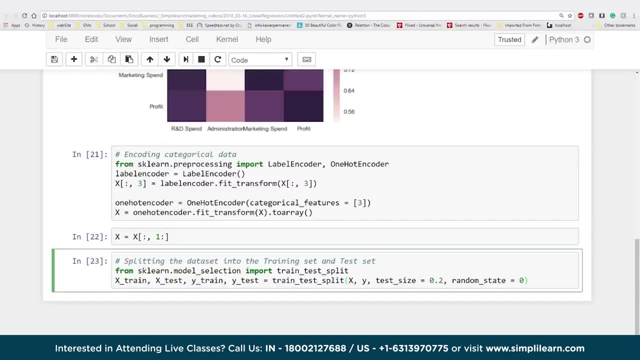 The next part, Train test split. We take X and we take Y. We've already created those. X has the columns with the data in it And Y has a column with profit in it. That means 20%, So 20% of the rows are going to be tested. 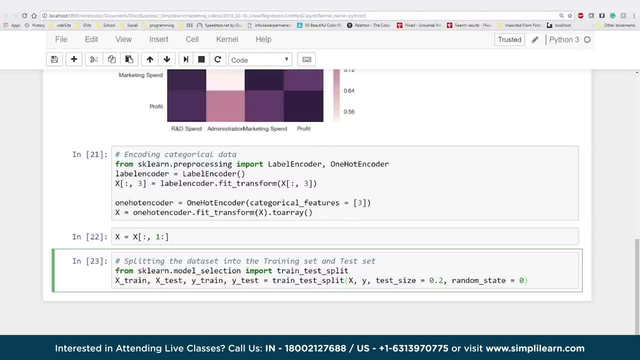 We're going to put them off to the side. So since we're using 1000 lines of data, That means that 200 of those lines We're going to hold off to the side to test for later, And then the random state equals 0.. 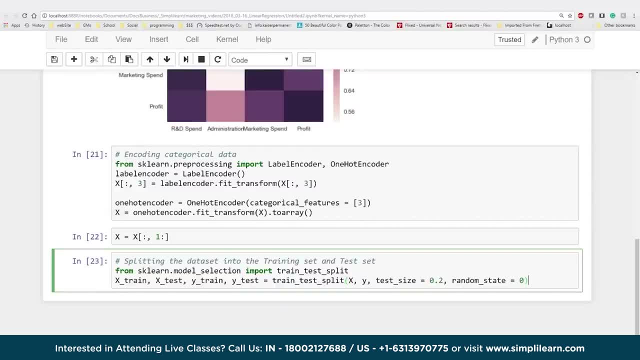 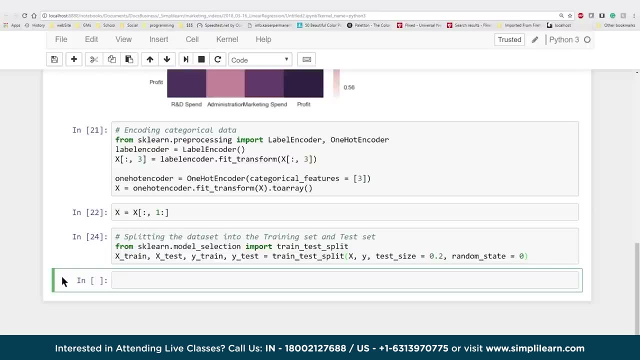 We're going to randomize which ones it picks To hold off to the side. We'll go ahead and run this. It's not overly exciting because it's setting up our variables, But the next step is The next step. we actually create our linear regression model. 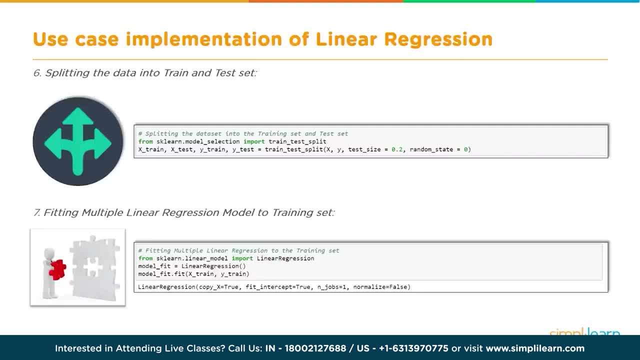 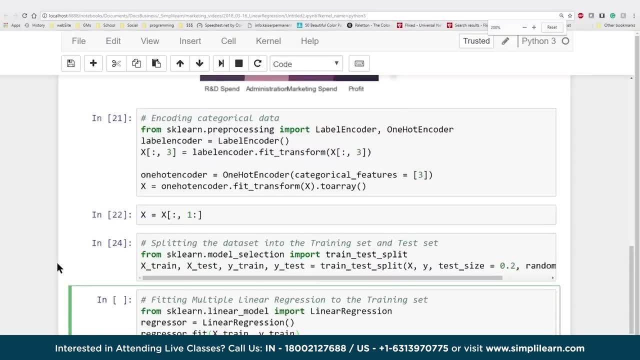 Now that we got to the linear regression model, We get that next piece of the puzzle. Let's go ahead and put that code in there and walk through it. So here we go, We're going to paste it in there And let's go ahead. and since this is a shorter line of code, 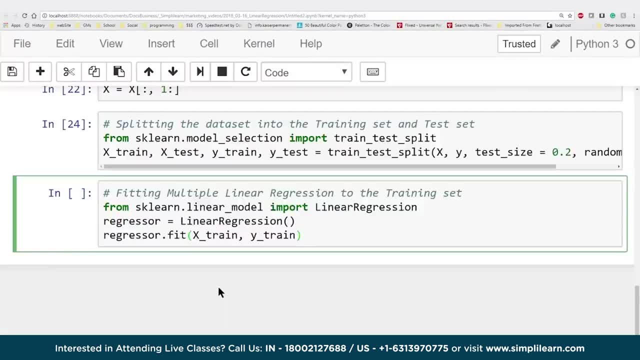 Let's zoom up there so we can get a good look. And we have from the sklearnlinear-model. We're going to import linear regression Now. I don't know if you recall from earlier When we were doing all the math. Let's go ahead and flip back there and take a look at that. 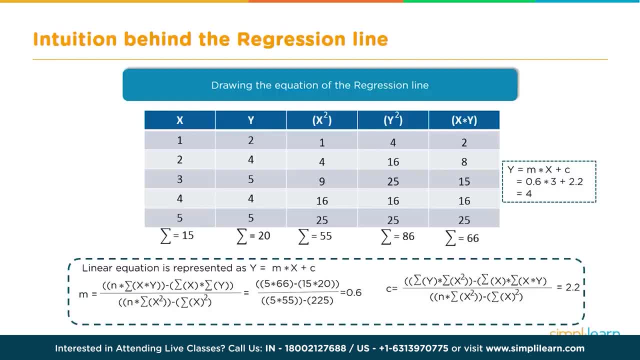 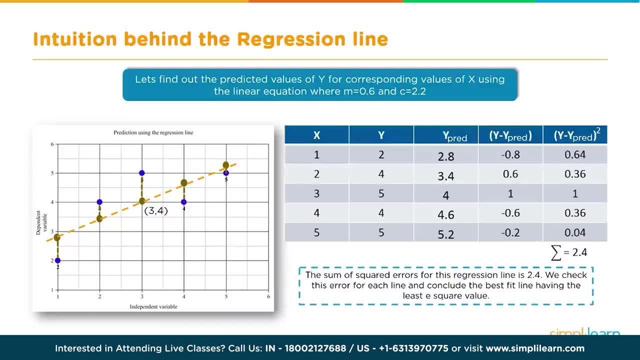 Do you remember this, Where we had this long formula on the bottom And we were doing all this sumization, And then we also looked at Setting it up with the different lines, And then we also looked all the way down to Multiple linear regression. 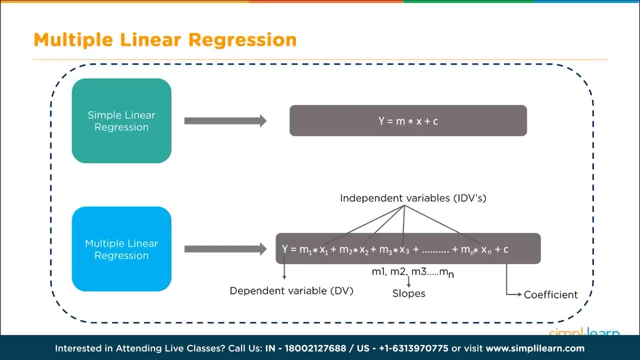 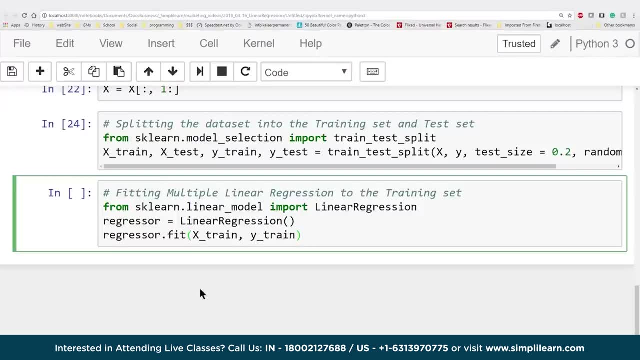 Where we're adding all those formulas together. All of that is wrapped up in this one section. So what's going on here Is I'm going to create a variable called regressor, And the regressor equals the linear regression. That's the linear regression model. 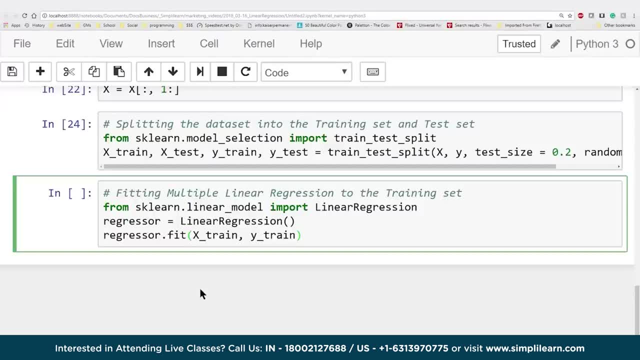 That has all that math built in, So we don't have to have it all memorized Or have to compute it individually. And then we do the regressorfit. In this case we do xtrain And ytrain. That's the training data. 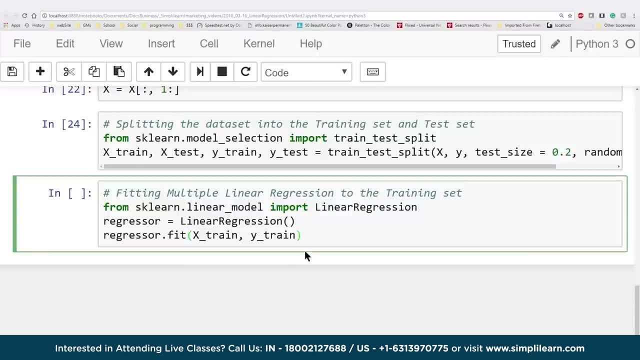 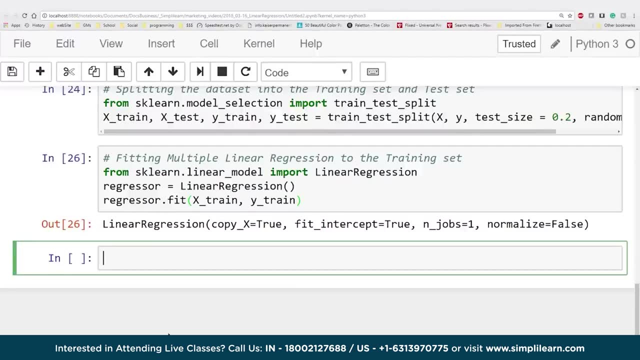 X being the data in And y being profit, What we're looking at And this does all that math for us. So within one click and one line, We've created the whole linear regression model And we fit the data to the linear regression model. 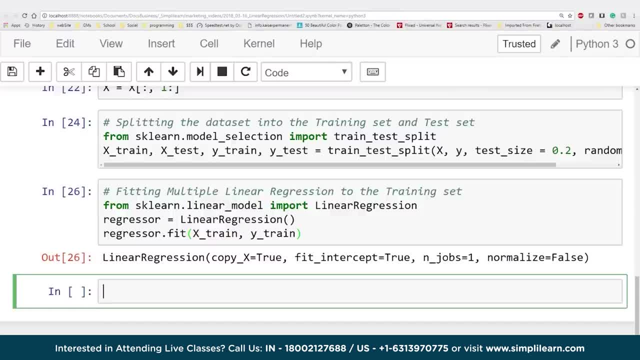 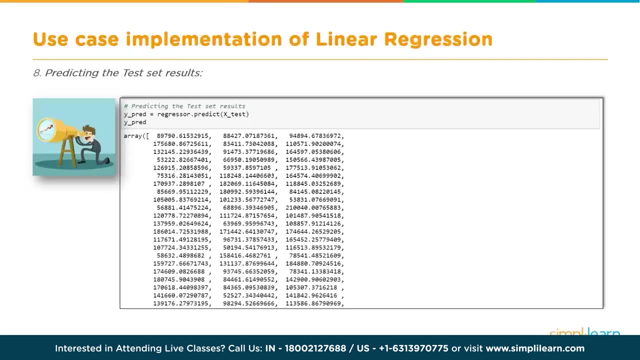 And you can see that when I run the regressor It gives an output: Linear regression. It says copy: x equals true, Fit intercept equals true, In jobs equals one. Normalize equals false. Let's go ahead and use it. And if you remember, 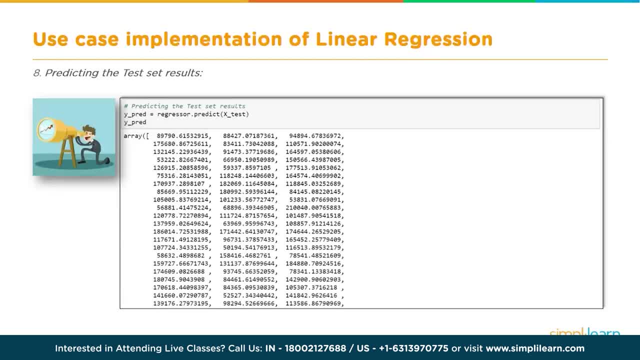 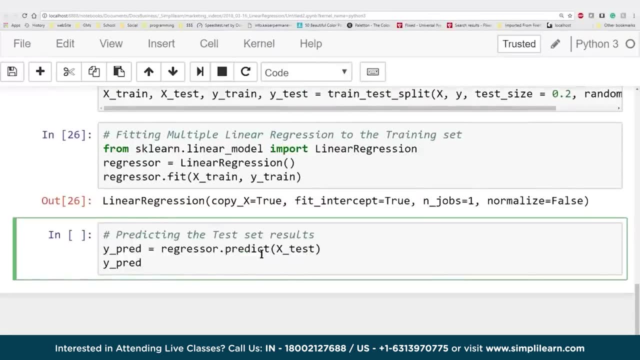 We kept a bunch of data aside. So we're going to do a ypredict variable And we're going to put in the xtest And let's see what that looks like. Scroll up a little bit, Paste that in here. Predicting the test set results. 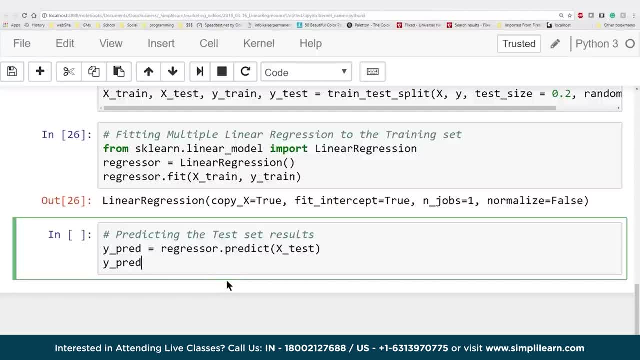 So here we have ypredict equals, regressorpredict, xtest going in And this gives us ypredict. Now, because I'm in Jupyter inline, I can just put the variable up there And when I hit the run button It will print that array out. 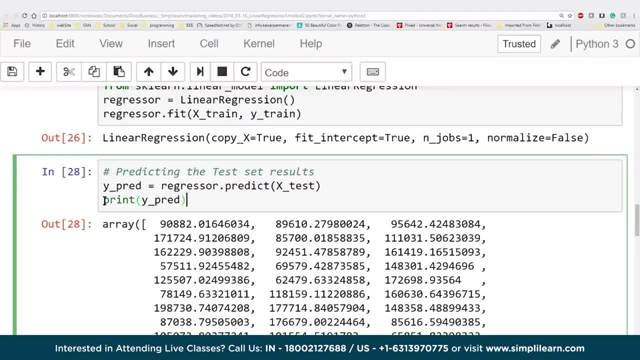 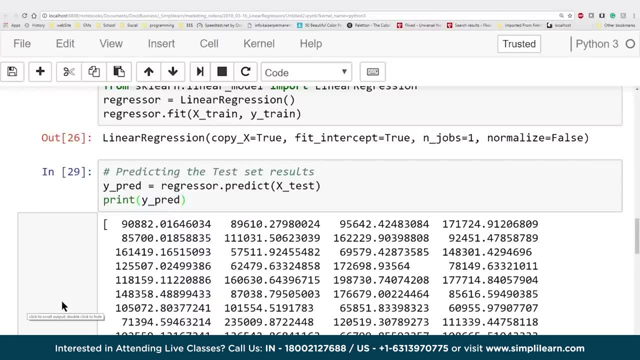 I could have just as easily done print ypredict. So if you're in a different IDE, That's not an inline setup Like the Jupyter notebook- You can do it this way: Print ypredict And you'll see that for the 200 different test variables. 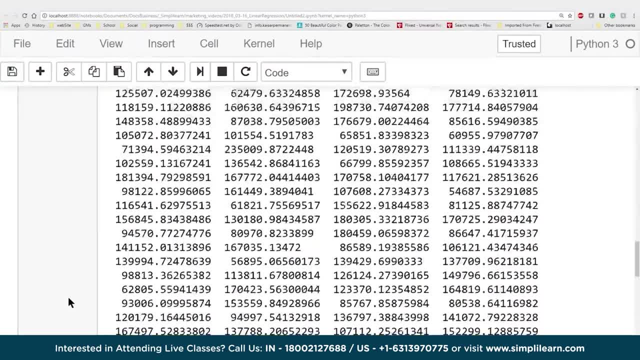 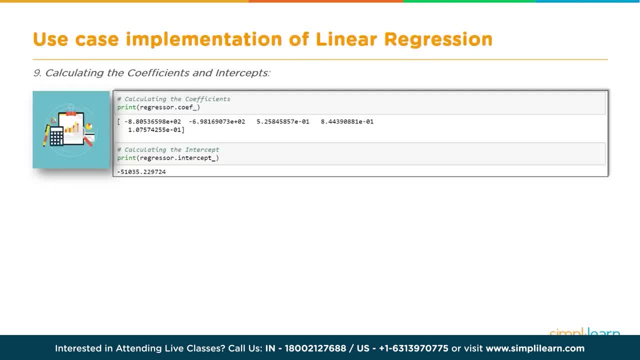 We kept off to the side. It's going to produce 200 answers. This is what it says. the profit are for those 200 predictions. But let's don't stop there. Let's keep going and take a couple. look, We're going to take just a short detail here. 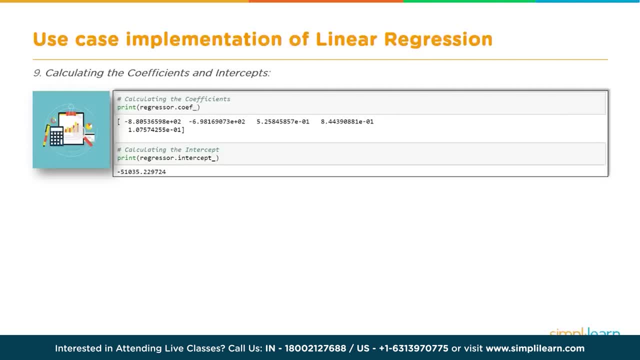 And calculating the coefficients and the intercepts. This gives us a quick flash At what's going on behind the line. We're going to take a short detour here And we're going to be calculating the coefficients and intercepts So you can see what those look like. 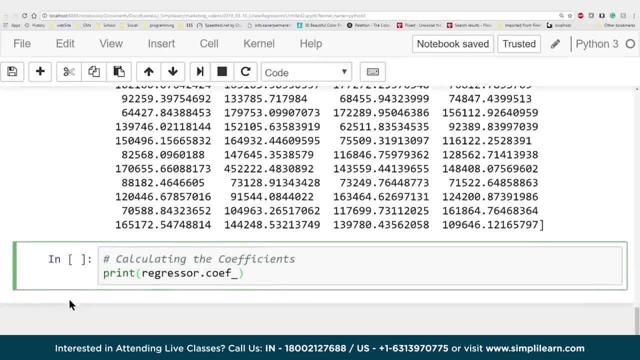 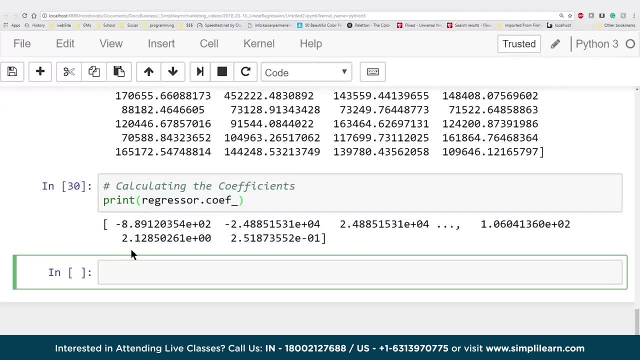 What's really nice About our regressor we created Is it already has the coefficients for us. We can simply just print Regressorcoefficient. When I run this, You'll see our coefficients here And if we can do the regressor coefficient. 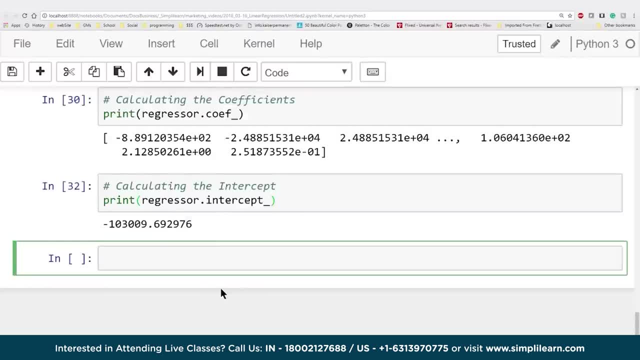 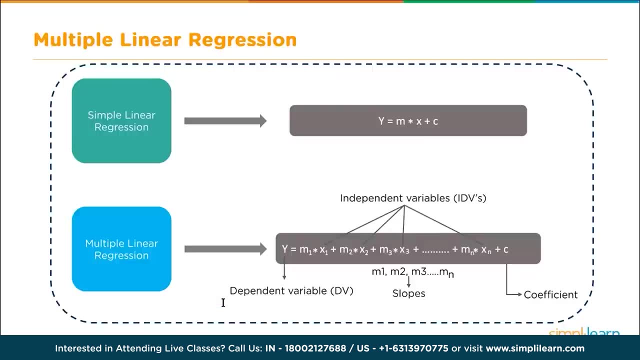 We can also do the regressor intercept. Let's run that and take a look at that. This all came from the multiple regression model. We'll flip over so you can remember Where this is going into and where it's coming from. You can see the formula down here. 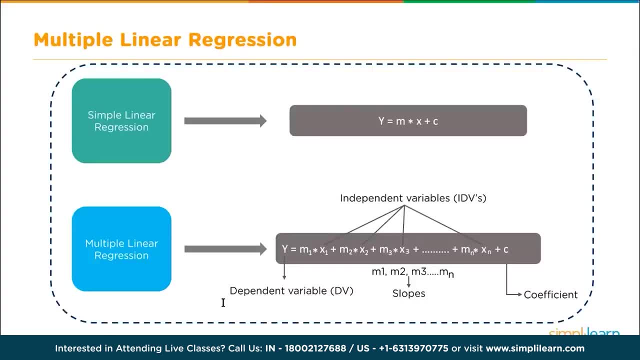 Where y equals m1 times x1.. Plus m2 times x2.. And so on and so on, Plus c the coefficient, So these variables fit right into this formula. Y equals slope 1 times column 1 variable, Plus slope 2 times column 2 variable. 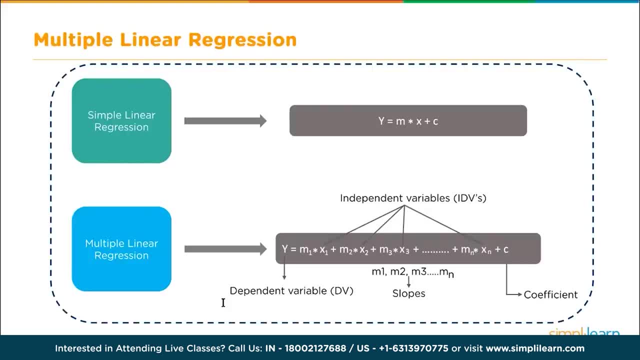 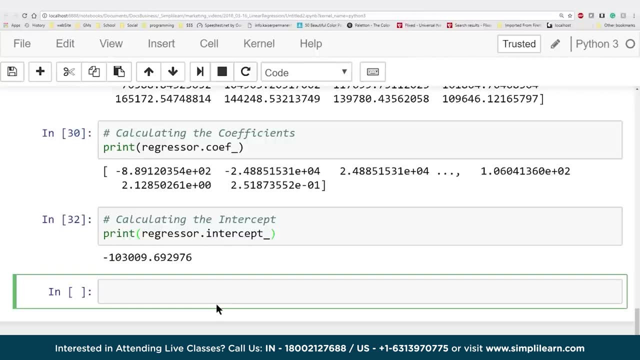 All the way to the m, to the n And x to the n plus c the coefficient, Or in this case You have minus 8.89 to the power of 2.. Etc, Etc Times, the first column And the second column. 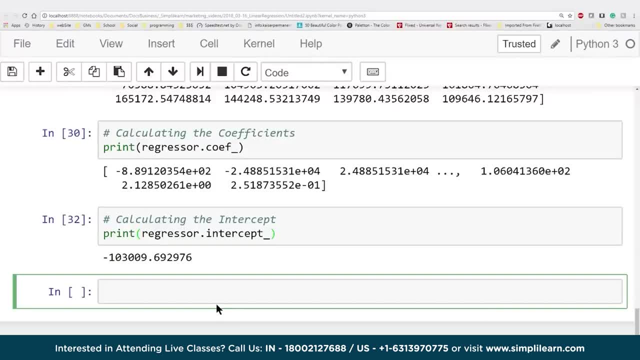 And the third column, And then our intercept is the minus 103009 point. Boy, it gets kind of complicated when you look at it. This is why we don't do this by hand anymore. This is why we have the computer To make these calculations easy to understand. 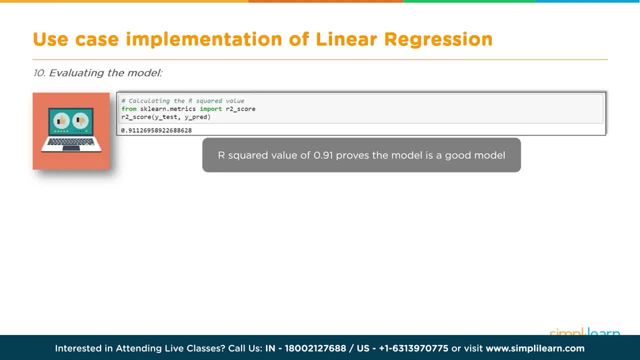 And calculate. Now, I told you that was a short detour And we're coming towards the end of our script. As you remember, from the beginning I said, if we're going to divide this information, We have to make sure it's a valid model. 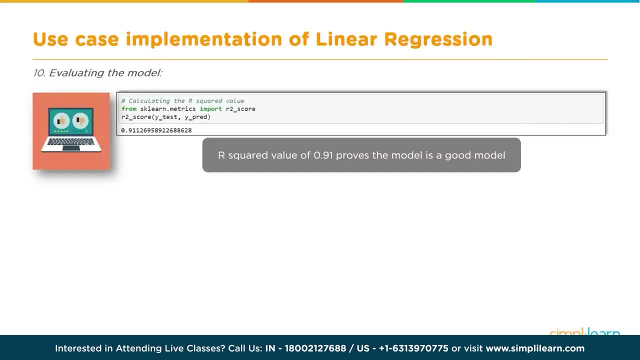 That this model works And understand how good it works. So calculating the r squared value: That's what we're going to use To predict how good our prediction is. And let's take a look at what that looks like in code. And so we're going to use this. 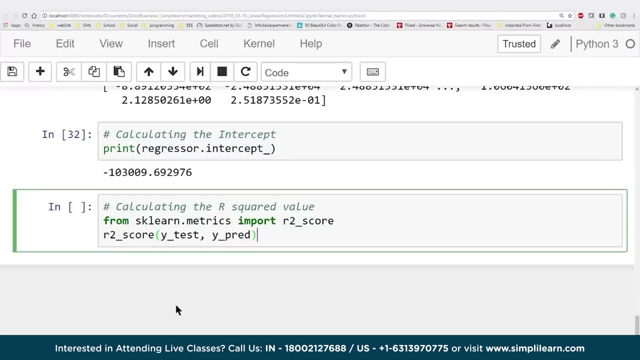 From sklearnmetrics. We're going to import r2 score. That's the r squared value. We're looking at the error. So in the r2 score We take our y test Versus our y predict, Because the actual values we're testing. 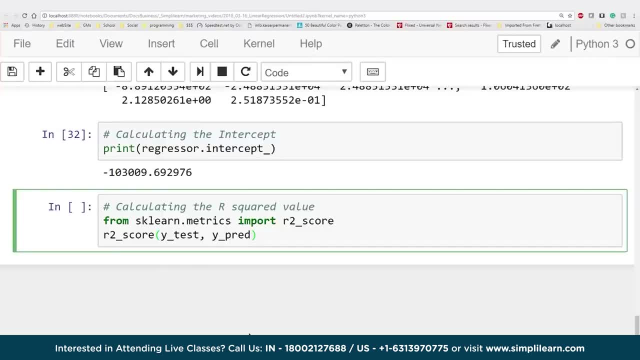 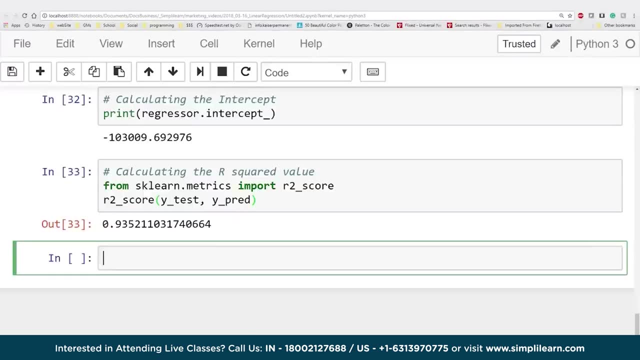 That was the one that was given to us. That we know are true. The y predict of those 200 values Is what we think it was true And when we go ahead and run this We see we get a .9352.. 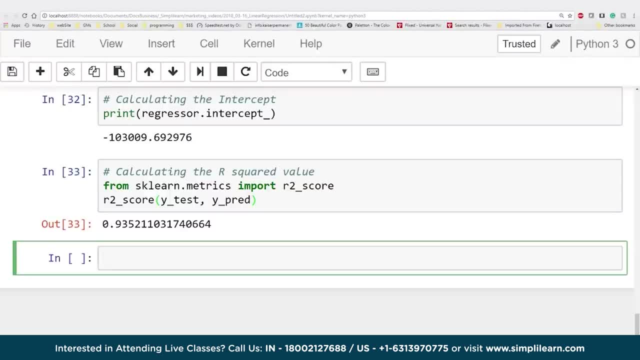 That's the r2 score. Now, it's not exactly a straight percentage, So it's not saying it's 93% correct, But you do want that in the upper 90s. Oh and higher Shows that this is a very valid prediction. 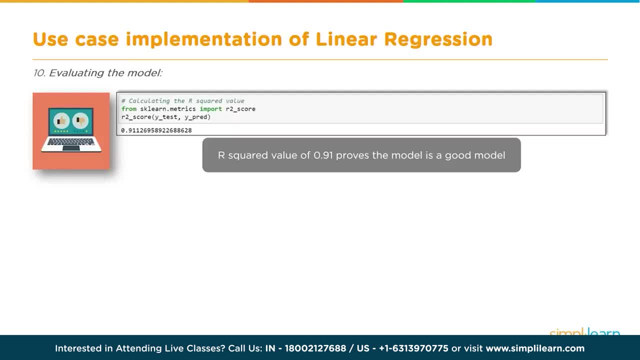 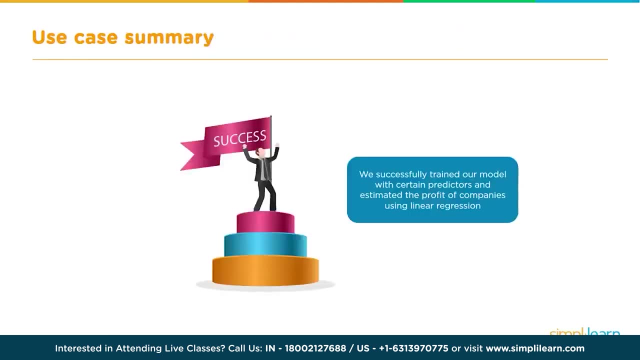 Based on the r2 score And if r squared value of .91.. .92 as we got on our model Because, remember, it does have a random generation involved. This proves the model is a good model, Which means success Yay. 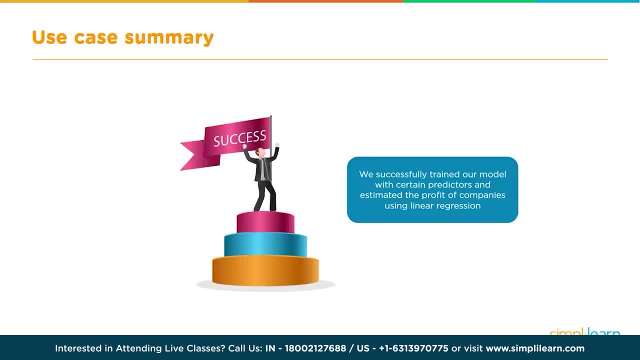 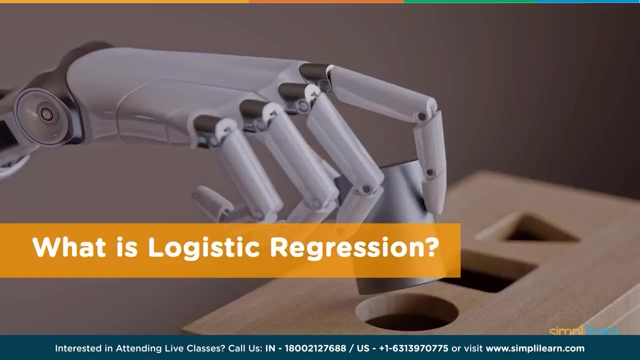 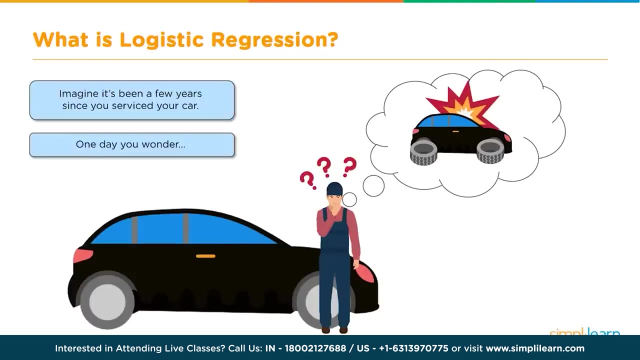 We successfully trained our model with certain predictors And estimated the profit of the companies Using linear regression. So now that we have a successful Linear regression model, Alright, what is logistic regression? As I mentioned earlier, Logistic regression is an algorithm For performing binary classification. 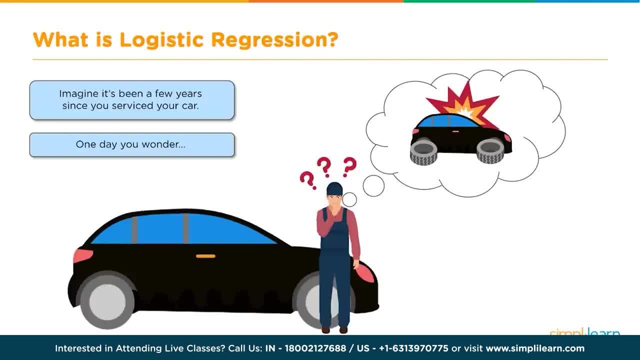 So let's take an example, Let's see how this works. Let's say your car has not been serviced For quite a few years And now you want to find out If it's going to break down in the near future. So this is like a classification problem. 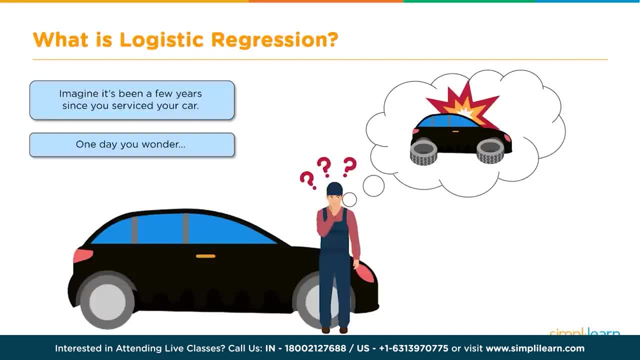 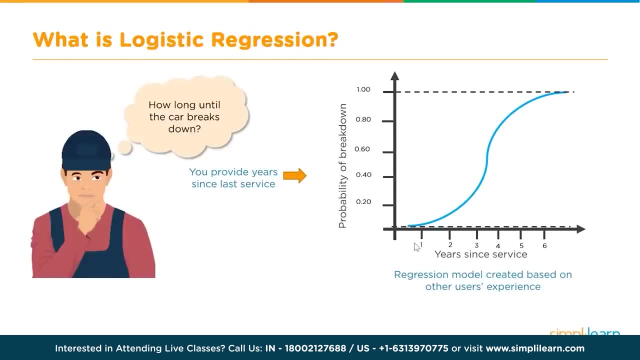 Find out whether your car will break down Or not. So how are we going to perform this classification? So here's how it looks. If we plot the information Along the x and y axis, X is the number of years Since the last service was performed. 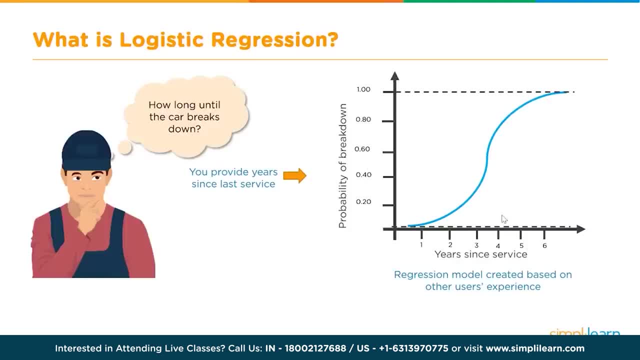 And y is the probability Of your car breaking down. And let's say, this information was This data rather Was collected from several car users. It's not just your car, But several car users. So that is our labeled data. So the data has been collected. 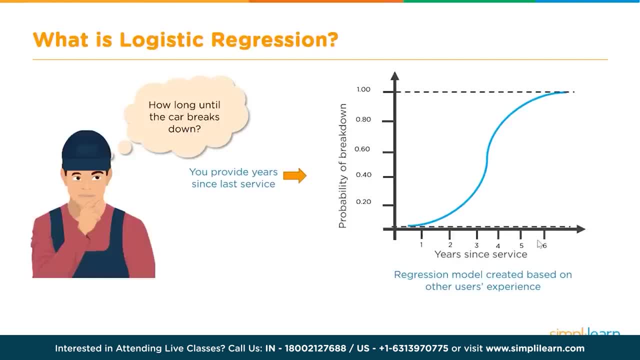 And for the number of years And when the car broke down And what was the probability, And that has been plotted Along x and y axis. So this provides an idea. From this graph We can find out whether Your car will break down or not. 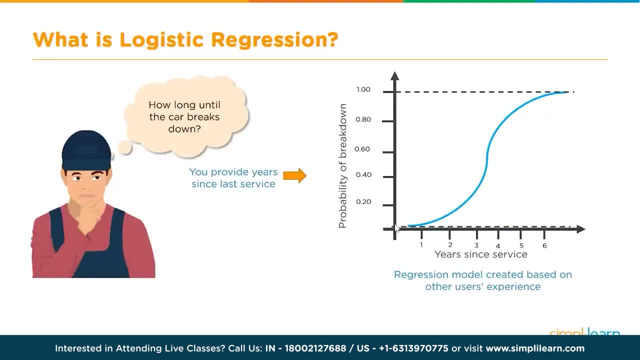 We'll see how. So, first of all, The probability can go from 0 to 1.. As you are aware, Probability can be between 0 and 1. And, as we can imagine, It is intuitive as well As the number of years are. On the lower side, Maybe 1 year, 2 years or 3 years Till after the service. The chances of your car breaking down Are very limited. The probability of your car breaking down. The probability of your car breaking down. 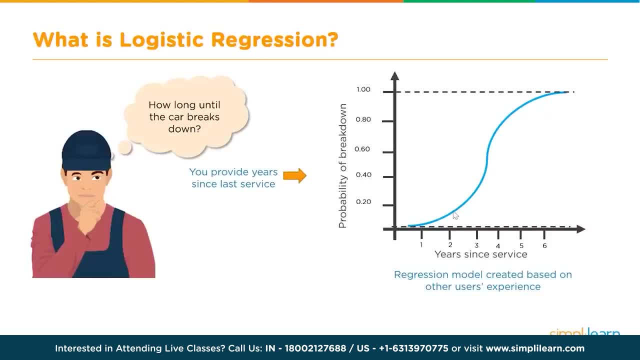 Within 2 years of your last service Are 0.1 probability. Similarly, 3 years is maybe 0.3., And so on. But as the number of years increases, Let's say if it was 6 or 7 years. 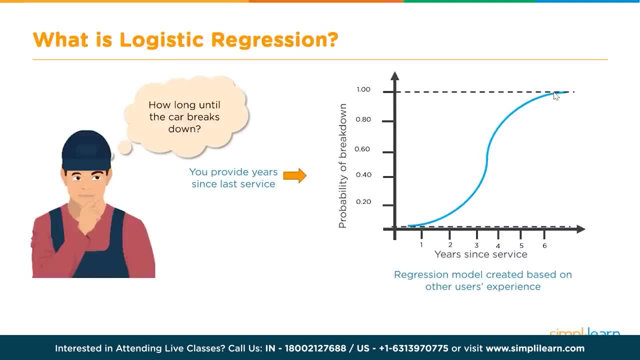 There is almost a certainty That your car is going to break down. That is what this graph shows. So this is an example of an application Of the classification algorithm, And we will see in little details How exactly A discrete regression is applied here. 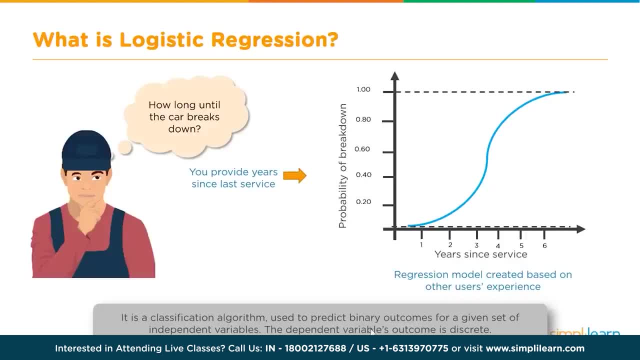 One more thing needs to be added here Is that the dependent variables outcome Is discrete. So if we are talking about Whether the car is going to break down or not, So that is a discrete value, The why that we are talking about. 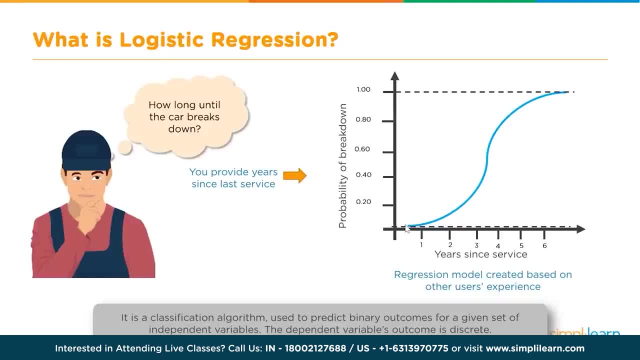 The dependent variable that we are talking about. What we are looking at is Whether the car is going to break down or not, Yes or no. That is what we are talking about. So here the outcome is discrete, Not a continuous value. 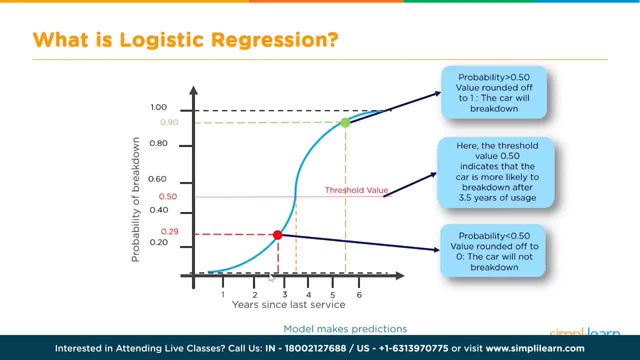 So this is how the logistic regression curve looks. Let me explain a little bit What exactly, How exactly we are going to Determine the class, The outcome, rather So, for a logistic regression curve, A threshold has to be set, Saying that: 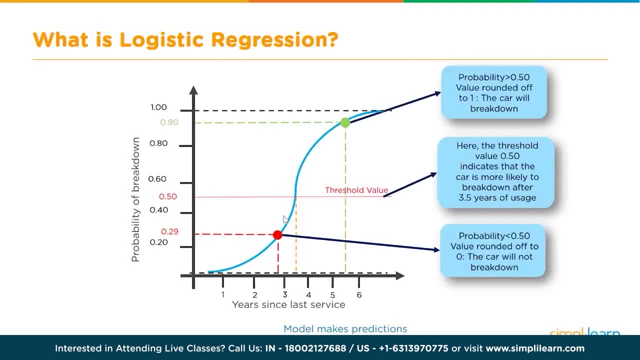 Because this is a probability calculation. Remember, this is a probability calculation And the probability itself Will not be 0 or 1.. But based on the probability, We need to decide What it should be. So there has to be a threshold. 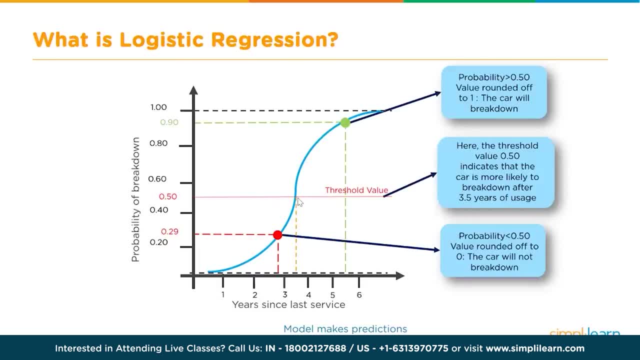 Like, for example, 0.5 can be the threshold. Let's say in this case: So any value of the probability below 0.5. Is considered to be 0. And any value above 0.5. Is considered to be 1.. 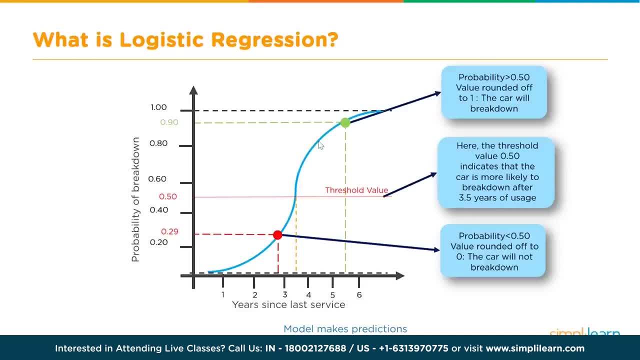 So an output of, Let's say, 0.8. Will mean that the car will break down, So that is considered as an output of 1.. And let's say An output of 0.29. Is considered as 0.. 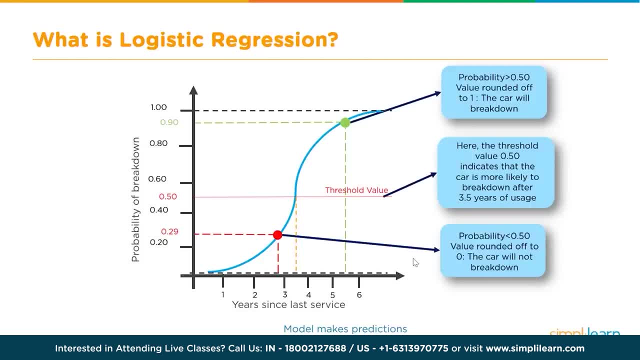 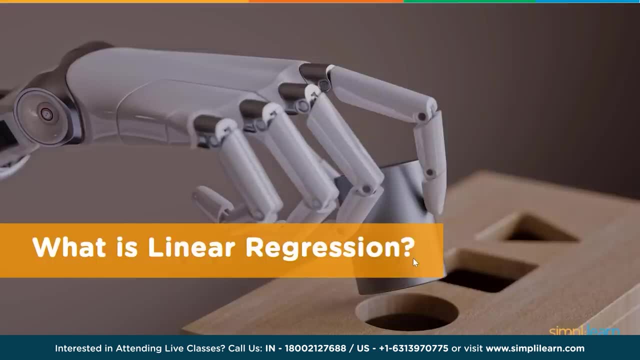 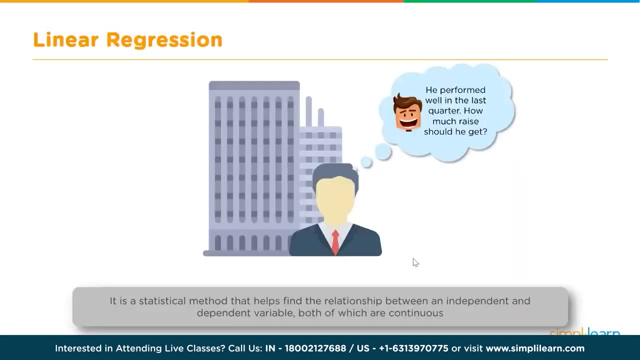 And the car will not break down. So that is the way logistic regression works. Now let's do a quick comparison Between logistic regression And linear regression, Because they both have the term Regression in them, So it can cause confusion. So let's try to remove that confusion. 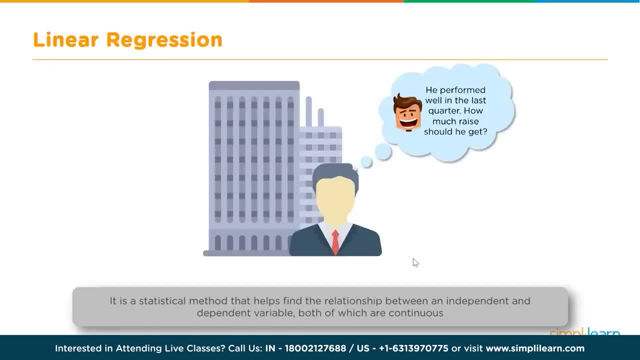 So what is linear regression? Linear regression is a process, Is once again an algorithm For supervised learning. However, here you are going to find A continuous value. It could be the price Of a real estate property, It could be your hike. 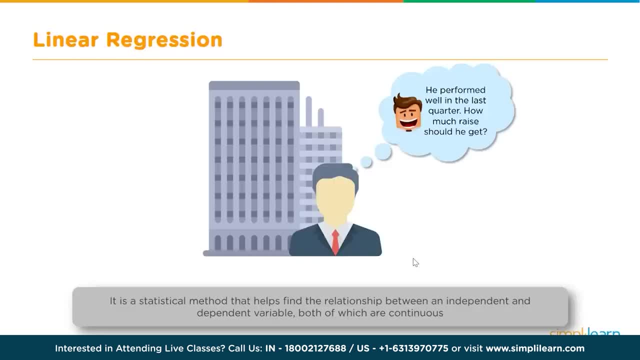 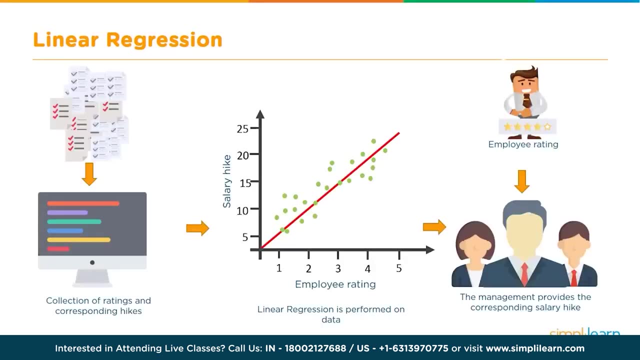 How much hike you are going to get, Or it could be a stock price. These are all continuous values. These are not discrete Compared to a yes or no kind of response That we are looking for in logistic regression. So this is one example of a linear regression. 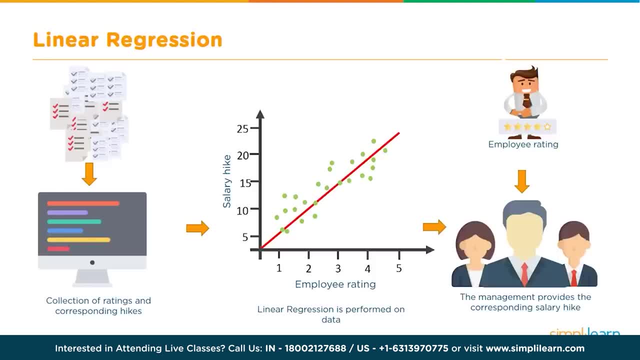 Let's say, the HR team of a company Tries to find out What should be the salary hike of an employee, So they collect all the details Of their existing employees, What has been given, And that is the labeled information That is available. 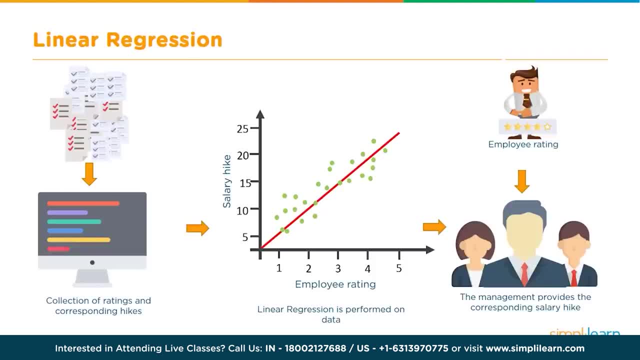 And the system learns from this. It is trained And it learns from this labeled information So that when a new employee's information is fed, Based on the rating, It will determine what should be the hike. So this is a linear regression problem. 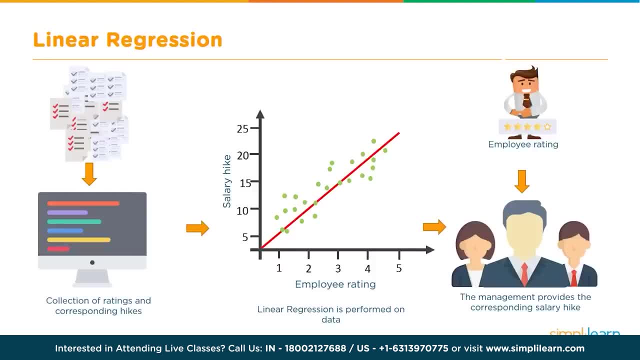 And a linear regression example. Now, salary is a continuous value. You can get 5000. 5500. 5600.. So it is not discrete like a cat or a dog Or an apple or a banana. These are discrete. 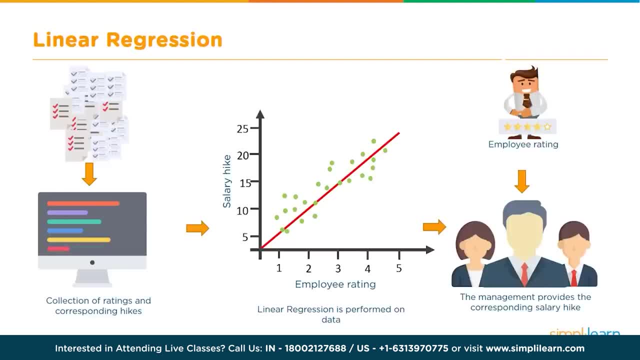 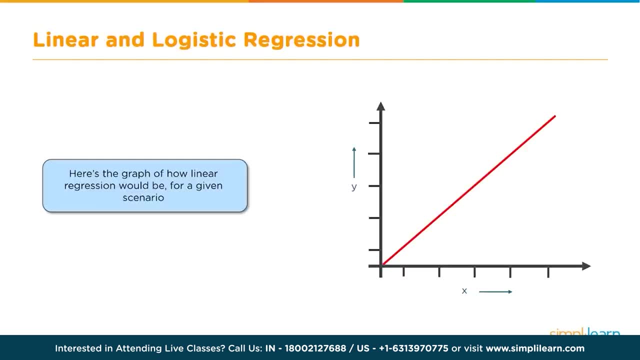 Or a yes or a no. These are discrete values. So this, where you are trying to find continuous values, Is where we use linear regression. So let's say, Just to extend on this scenario, We now want to find out Whether this employee is going to get a promotion. 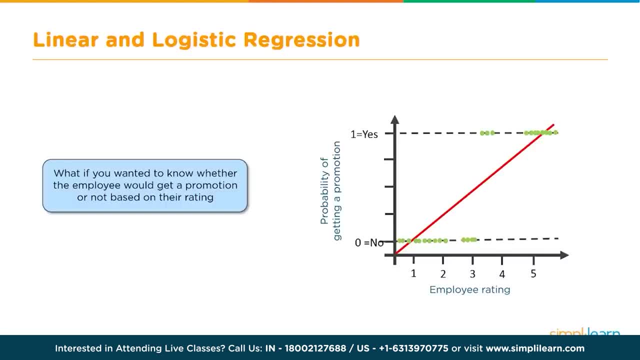 Or not. So we want to find out. That is a discrete problem, A yes or no kind of a problem. In this case, We actually cannot use linear regression, Even though we may have labeled data. So this is the labeled data. 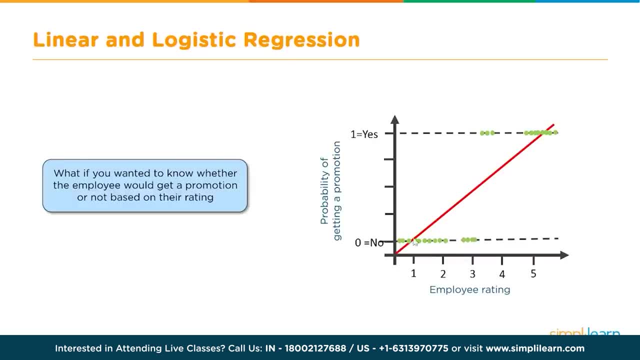 So, based on the employee rating, These are the ratings. And then some people got the promotion And this is the ratings For which people did not get promotion. That is a no, And this is the rating for which people got promotion. We just plotted the data about. 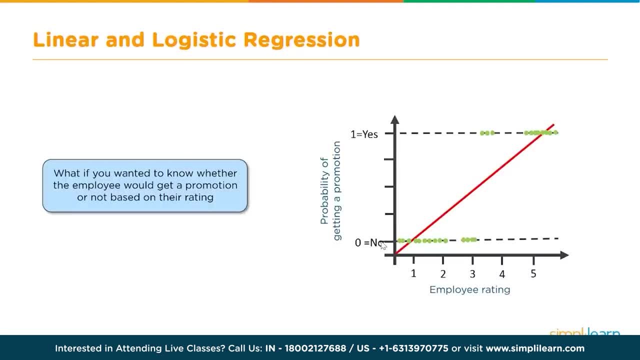 Whether a person has got An employee has got promotion or not, Yes or no, And what is the employee's rating, And ratings can be continuous, That is not an issue, But the output is discrete in this case, Whether employee got promotion. 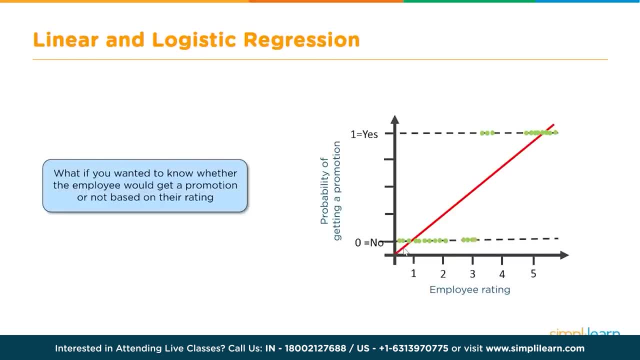 Yes or no. So if we try to plot that And we try to find a straight line, This is how it would look And, as you can see, Doesn't look very right Because looks like there will be lot of errors. This root mean square error. 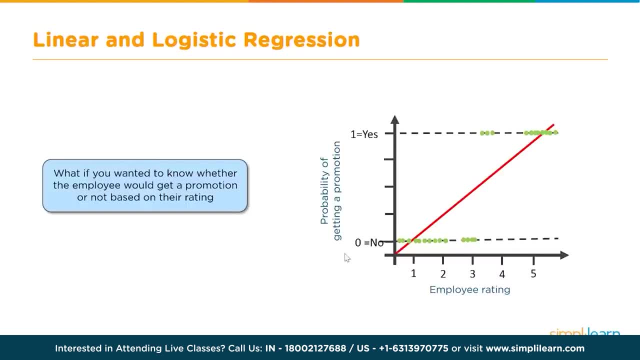 If you remember, for linear regression Would be very, very high. You cannot go beyond zero Or beyond one, So the graph should probably look somewhat like this: Clipped at zero and one, But still this straight line Doesn't look right. 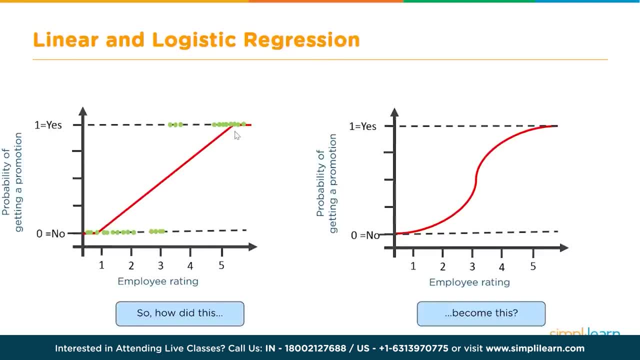 Therefore, instead of using A linear equation, We need to come up with something different, And therefore the logistic regression Model looks somewhat like this. So we calculate the probability And if we plot That probability- Not in the form of a straight line- 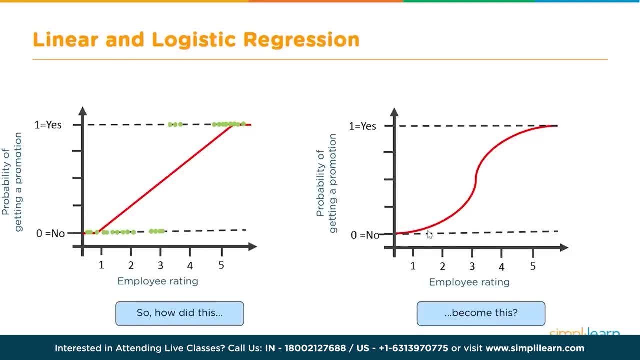 But some other equation. We will see very soon what that equation is. Then it is a gradual process. So you see here, People with some of these ratings Are not getting any promotions, And then slowly, at certain rating, They get promotion. 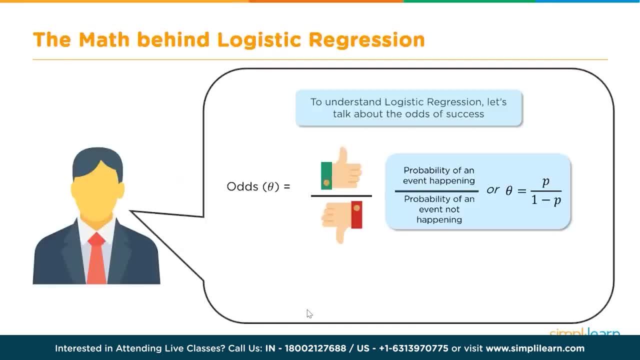 So it is a gradual process And this is how the math behind Logistic regression looks. So we are trying to find the odds For a particular event happening. And this is the formula For finding the odds: The probability of an event happening. 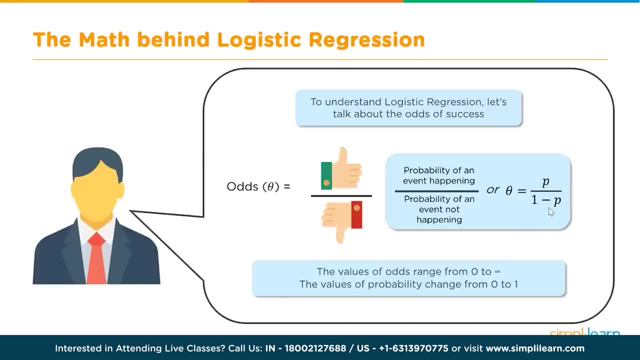 Divided by the probability Of the event not happening, So p if it is the probability Of the event happening, The probability of the person getting a promotion- And divided by the probability Of the person not getting a promotion, That is one minus p. 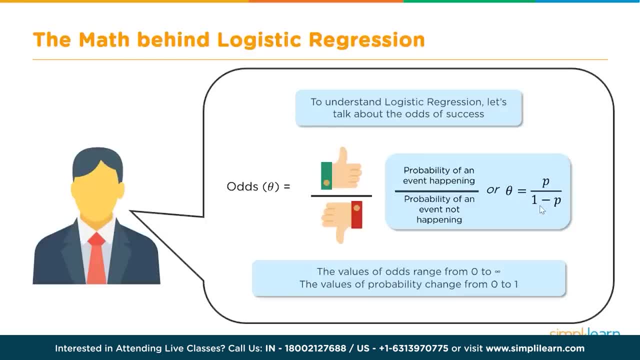 So this is how you measure the odds. Now. the values of the odds Range from zero to infinity. So when this probability Is zero, Then the odds Is equal to zero, And when the probability becomes one, Then the value of the odds is. 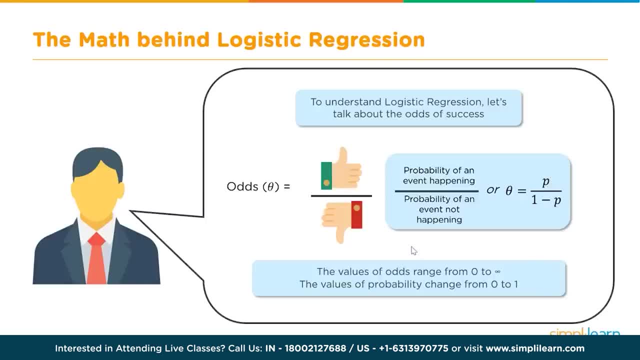 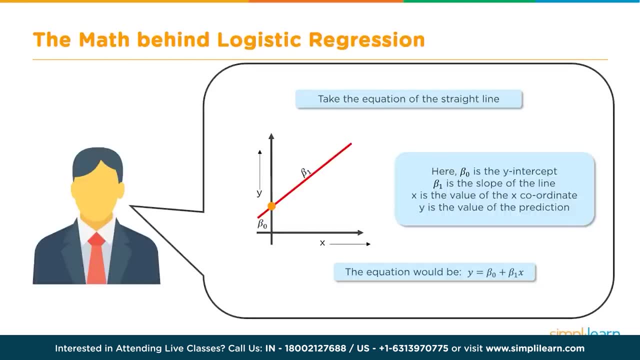 One by zero, that will be infinity, But the probability itself remains Between zero and one. Now this is how an equation Of a straight line looks. So y is equal to beta zero Plus beta one x, Where beta zero is the y intercept. 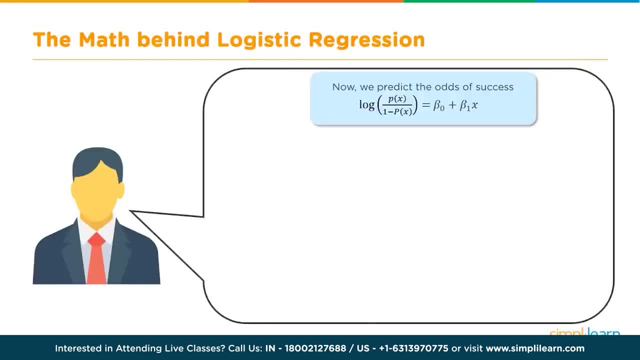 And beta one is the slope of the line. If we take the odds equation And take a log of both sides, Then this would look Like this, And the term logistic Is actually derived from the fact That we are doing this. 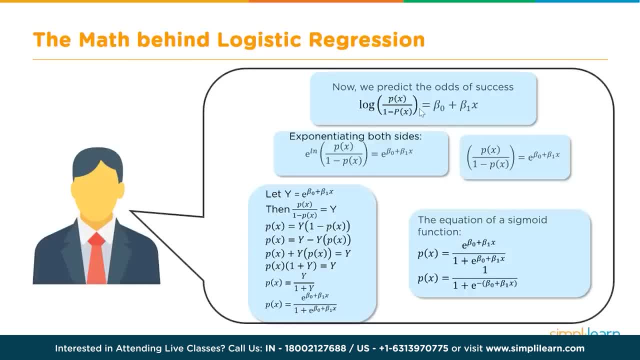 We take a log of p x by one minus p x. This is an extension of the calculation Of odds that we have seen And that is equal to beta zero Plus beta one x, Which is the equation of the straight line. And now, from here, 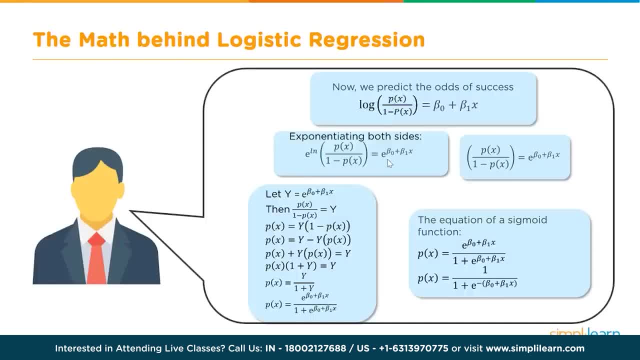 If you want to find out the value of p x, You will see. we can take The exponential on both sides. We will get the equation Of p x like this: p x is equal to one by one plus e to the power of minus. 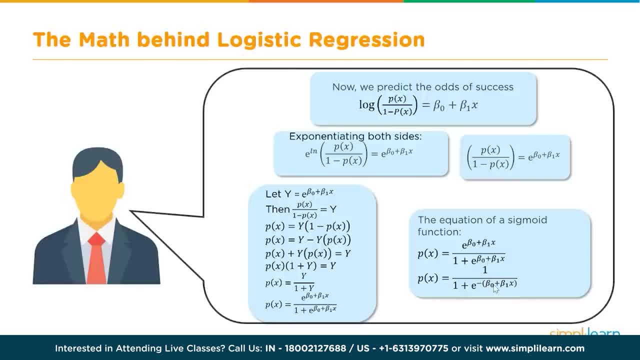 Beta zero plus beta one x. And recall this is nothing but The equation of the line Which is equal to y. y is equal to beta zero plus beta one x. So this is the equation Also known as the sigmoid function And this is the equation of the logistic regression. 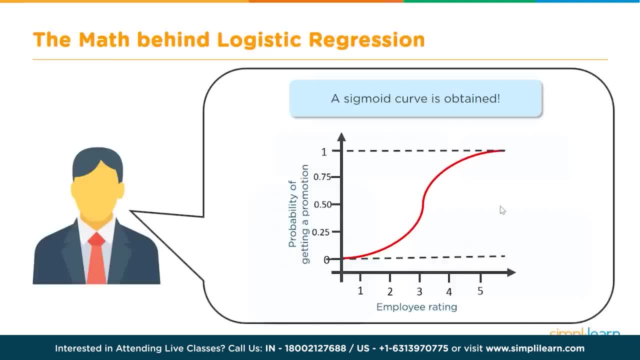 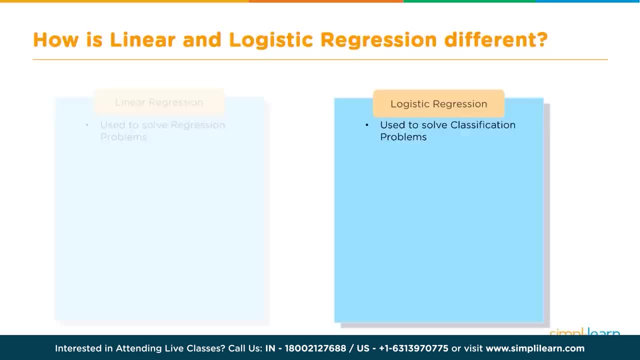 And if this is plotted, This is how the sigmoid curve Is obtained. So let's compare linear And logistic regression, How they are different from each other. Let's go back. So linear regression is solved Or used to solve regression problems. 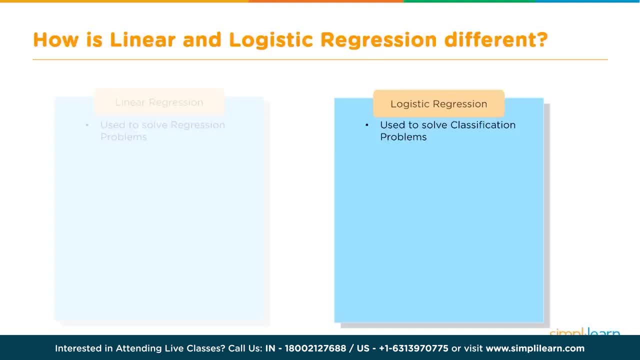 And logistic regression Is used to solve classification problems, So both are called regression. But linear regression Is used for solving regression problems Where we predict continuous values, Whereas logistic regression Is used for solving classification problems Where we have To predict discrete values. 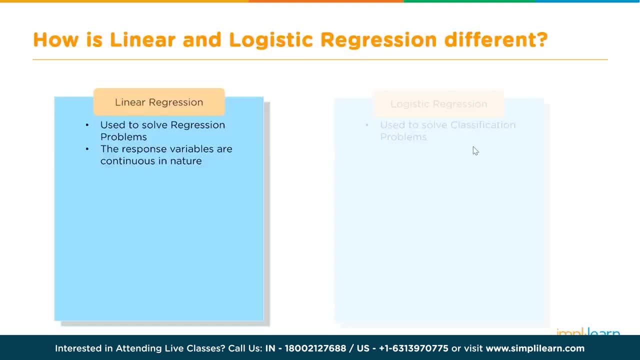 The response variables In case of linear regression Are continuous in nature, Whereas here they are categorical Or discrete in nature, And linear regression Helps to estimate the dependent variable When there is a change in the independent variable, Whereas here, in case of logistic regression. 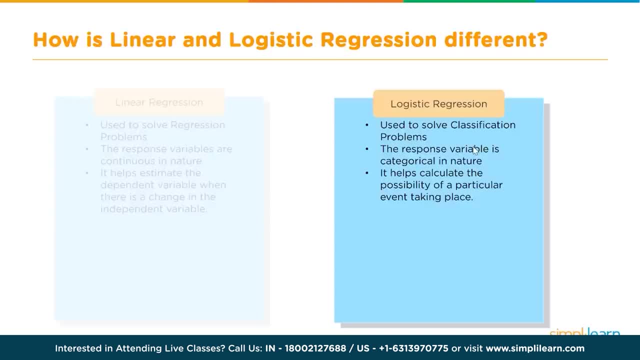 It helps to calculate the probability Or the possibility Of a particular event happening, And linear regression, as the name suggests, Is a straight line, Whereas logistic regression Is a sigmoid function And the curve is. The shape of the curve is S. 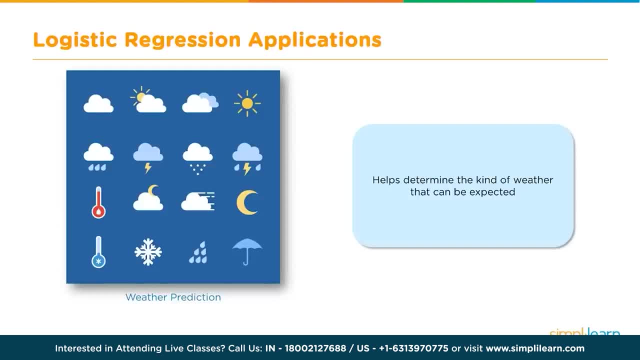 It's an S shaped curve. This is another example of Application of logistic regression In weather prediction- That it's going to rain or not rain. Now keep in mind Both are used in weather prediction. If we want to find the discrete values, 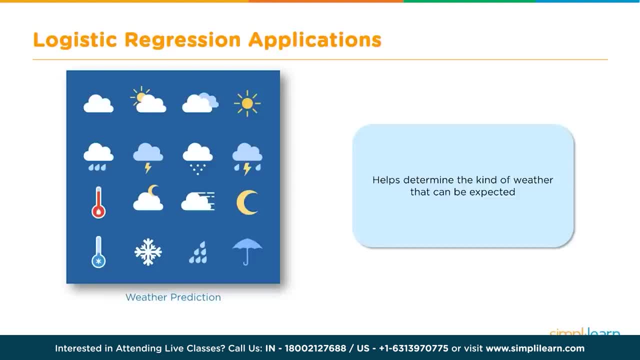 Like whether it's going to rain or not rain. That is a classification problem. We use logistic regression- What is going to be the temperature tomorrow? Then we use linear regression. So just keep in mind That in weather prediction we actually use both. 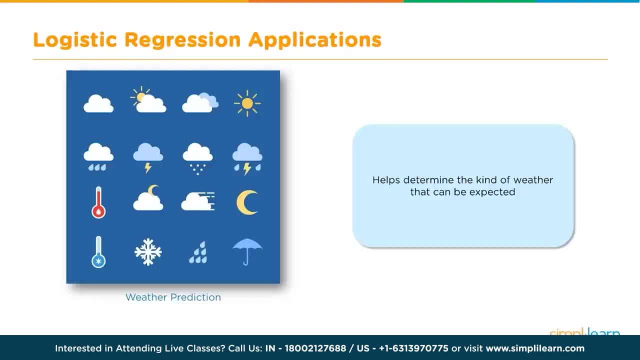 But these are some examples of logistic regression. So we want to find out Whether it's going to rain or not, Whether it's going to be sunny or not, Whether it's going to snow or not. These are all logistic regression examples. 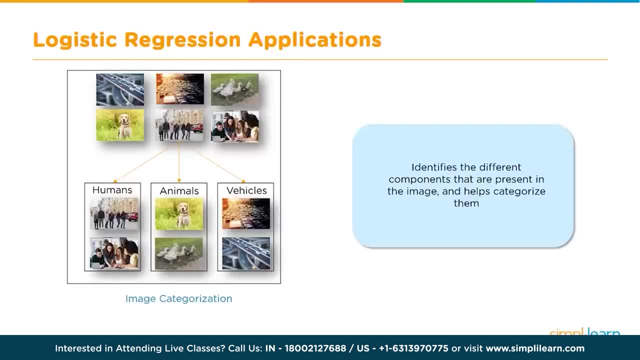 A few more examples. Classification of objects: This is again another example of logistic regression. Now here. of course These are multi class classification, So logistic regression Is not used In its original form, But it is used in a slightly different form. 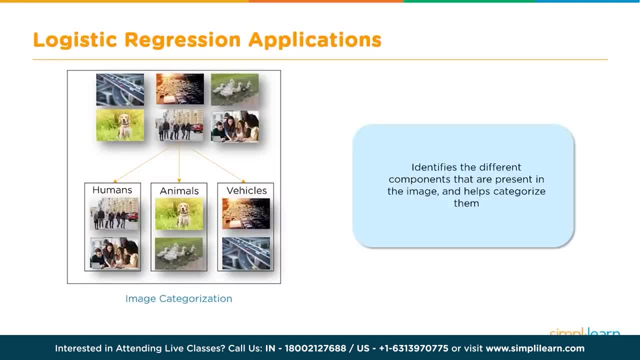 So we say Whether it is a dog or not a dog. I hope you understand. So instead of saying Is it a dog or a cat or an elephant, We convert this into saying Because we need to keep it to binary classification. 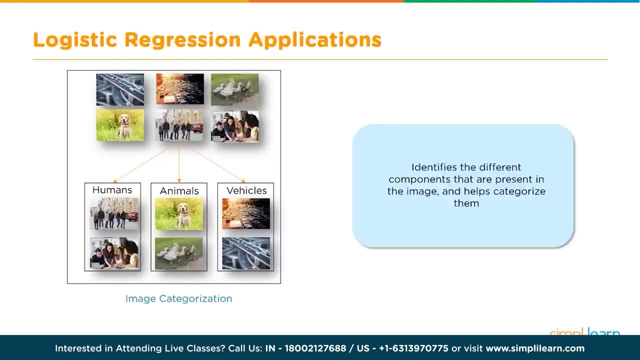 So we say: Is it a dog or not a dog, Is it a cat or not a cat? That's the way logistic regression can be used For classifying objects. Otherwise, there are other techniques Which can be used for performing multi class classification. 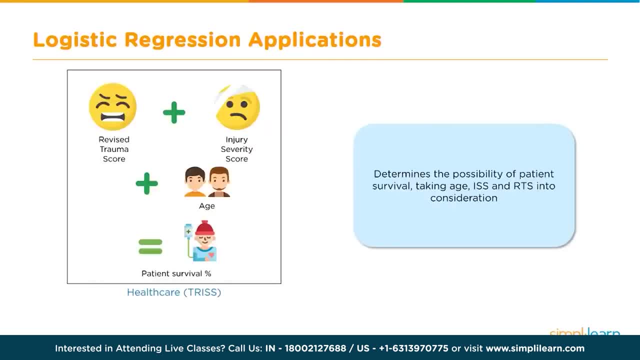 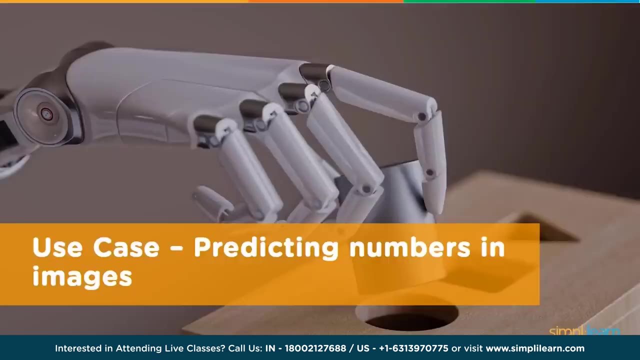 In healthcare, Logistic regression is used to find The survival rate of a patient. So they take multiple parameters Like trauma score, Age and so on and so forth, And they try to predict The rate of survival. Alright, now, finally, let's take an example. 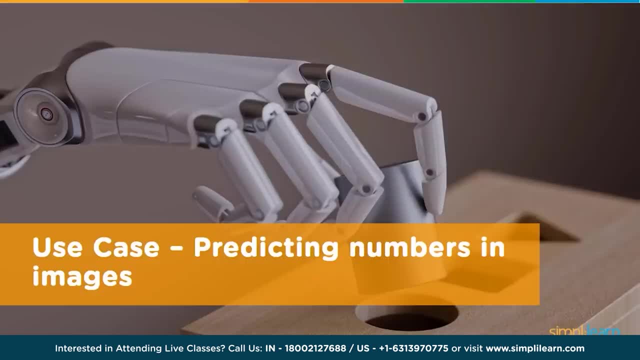 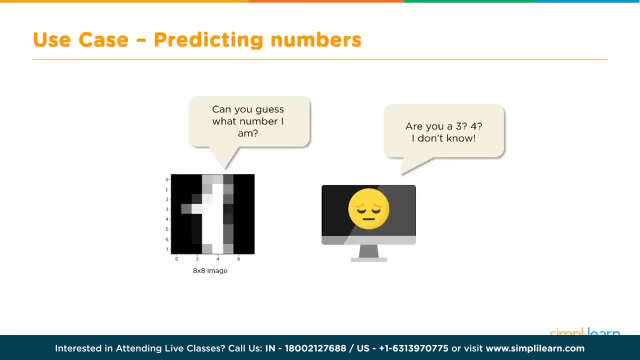 And see how we can apply Logistic regression To predict the number That is shown in the image. So this is actually a live demo. I will take you into jupiter notebook And show the code, But before that Let me take you through a couple of slides. 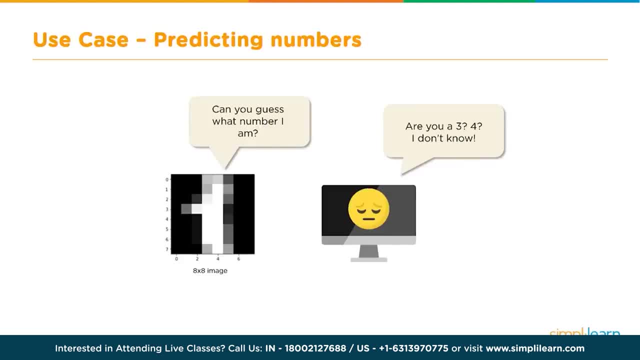 To explain what we are trying to do. So let's say you have an 8 by 8 image And there the image has a number: 1, 2, 3, 4.. And you need to train your model To predict what this number is. 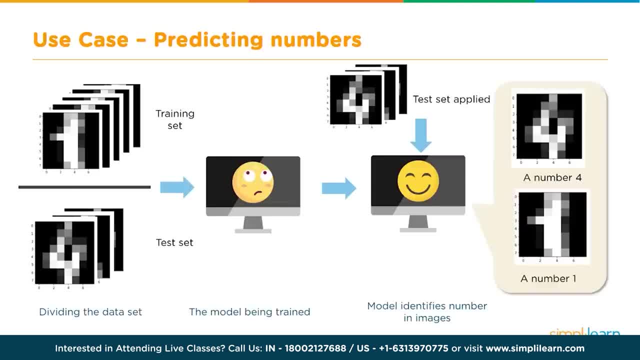 So how do we do this? So, the first thing is, obviously, We train the model. So, in this case, we are using logistic regression, So, and then we provide a training set To train the model, And then we test How accurate our model is. 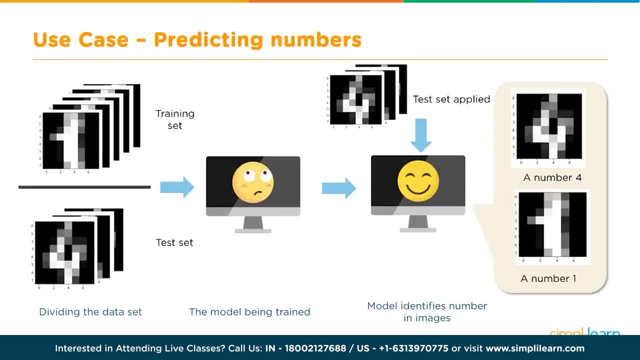 With the test data, Which means that, like any machine learning process, We split our initial data into two parts: Training set and test set. With the training set, we train our model And then, with the test set, we test the model Till we get good accuracy. 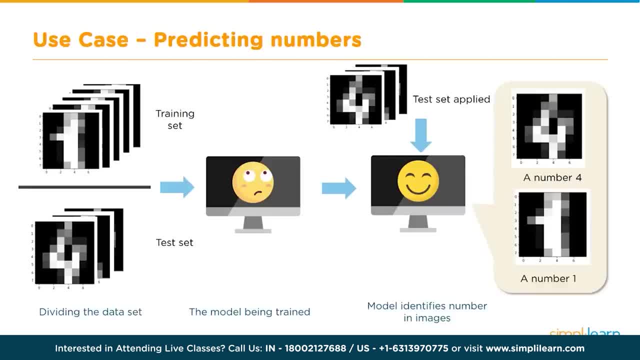 And then we use it for inference Right. So this is the typical methodology Of training, testing And then deploying of machine learning models. So let's take a look at the code And see what we are doing. So I will not go line by line. 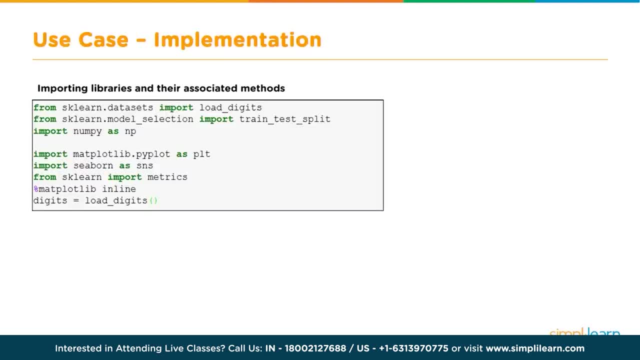 But just take you through some of the blocks. So first thing we do Is import all the libraries And then we basically take a look At the images And see what is the total number of images We can display using matplotlib. Some of the images: 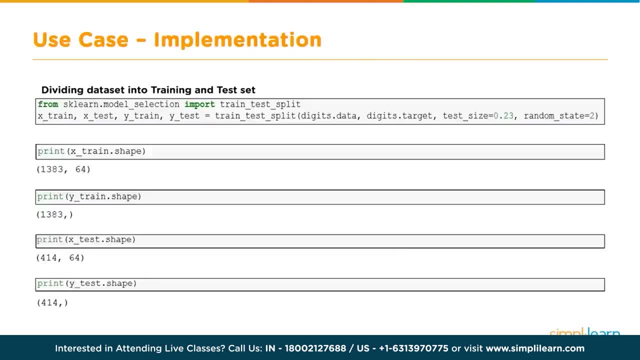 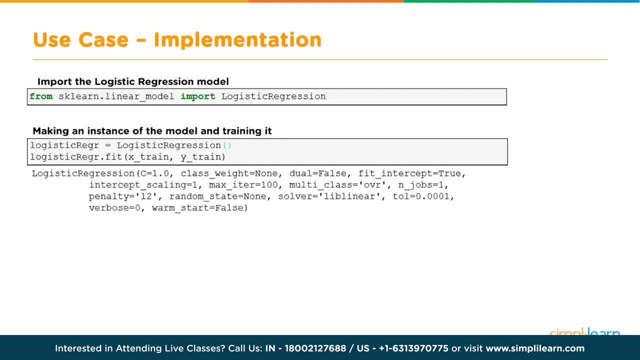 Or a sample of these images, And then we split the data into training and test, As I mentioned earlier, And we can do some exploratory analysis, And then we build our model, We train our model With the training set And then we test it with our test set. 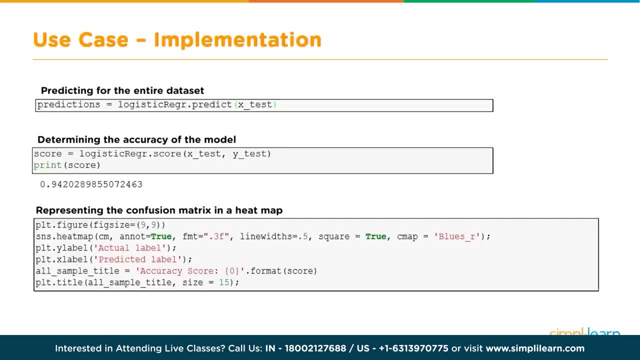 And find out how accurate our model is, Using the confusion matrix, The heat map, And use heat map for visualizing this, And I will show you in the code What exactly is the confusion matrix And how it can be used For finding the accuracy. 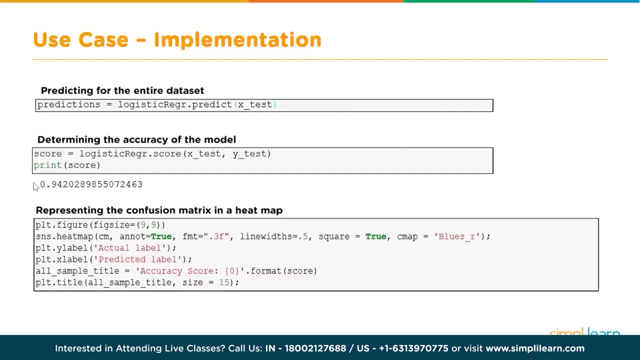 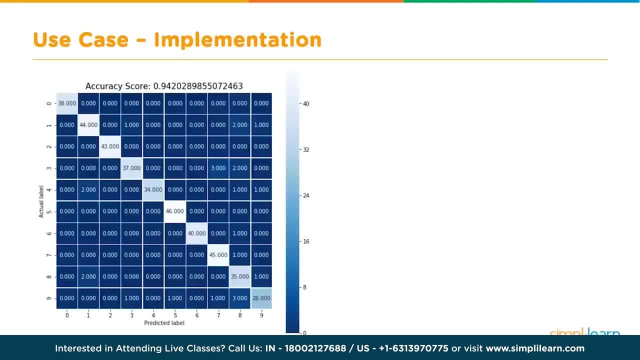 In our example We get an accuracy of about 0.94., Which is pretty good, Or 94%, which is pretty good. So what is a confusion matrix? This is an example of a confusion matrix And this is used for. 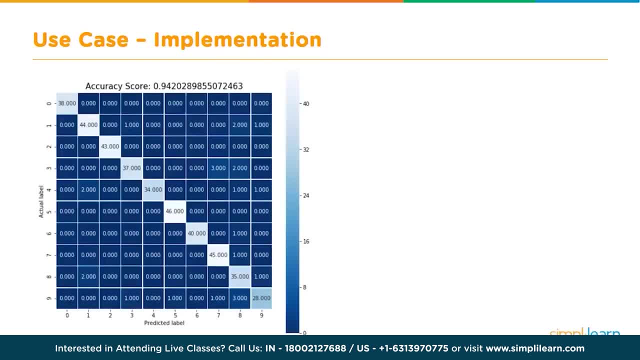 Identifying the accuracy Of a classification model Like a logistic regression model. So the most important part In a confusion matrix Is that first of all, As you can see, this is a matrix And the size of the matrix Is based on how many outputs. 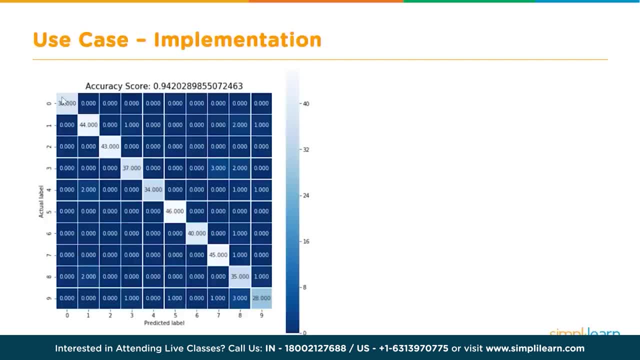 We are expecting. So the most important part here Is that the model will be Most accurate when we have The maximum numbers In its diagonal, Like in this case. That's why it has almost 93-94%, Because the diagonal should have. 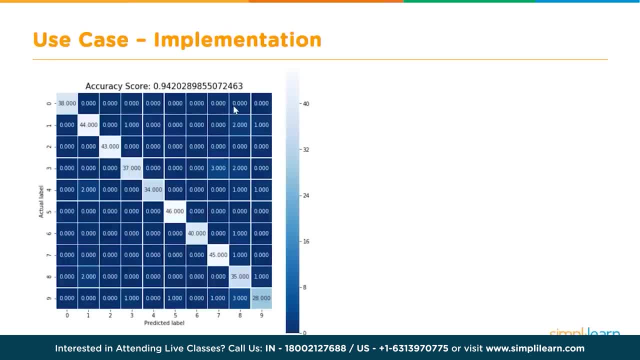 The maximum numbers And the others other than diagonal. The cells other than the diagonal Should have very few numbers. So here that's what is happening. There is a 1 here, But most of them Are along the diagonal. What does this mean? 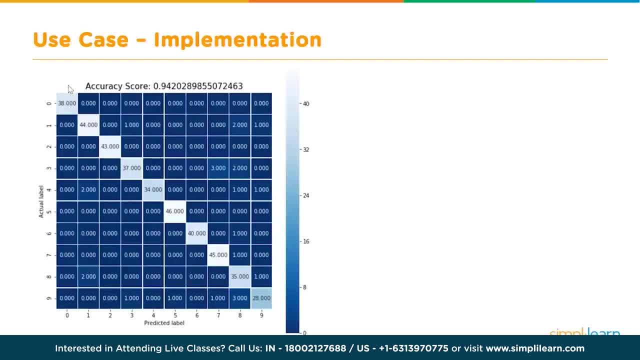 This means that the number that has been Fed is 0. And the number that has been detected Is also 0. So the predicted value and the actual value Are the same. So along the diagonals that is true, Which means that let's take this diagonal. 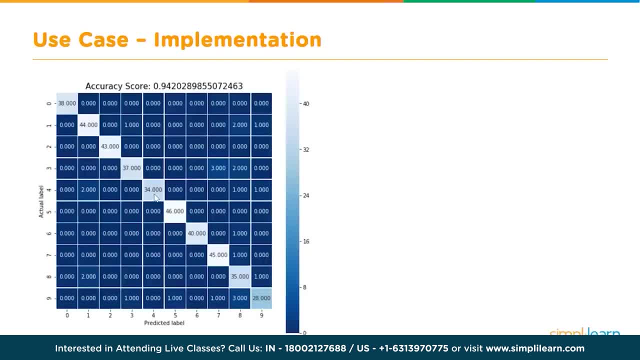 If the maximum number is here, That means that, Like here in this case, it is 34.. That means that 34 of the images That have been fed, or rather, actually There are two misclassifications in there, So 36 images. 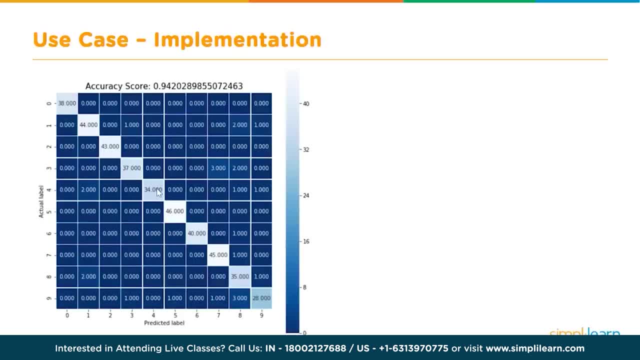 Have been fed, Which have number 4. And out of which 34 have been predicted Correctly as number 4. And one has been predicted as number 8. And another one has been predicted as Number 9.. So these are two misclassifications. 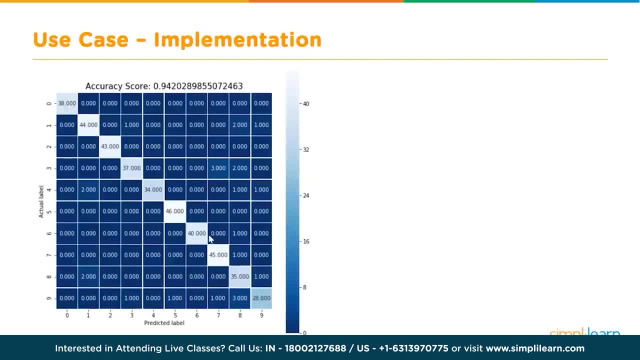 So that is the meaning of saying that The maximum number should be in the diagonal. So if you have all of them, Then the ideal model Which has, let's say, 100% accuracy, Everything will be only in the diagonal, There will be no numbers other than 0.. 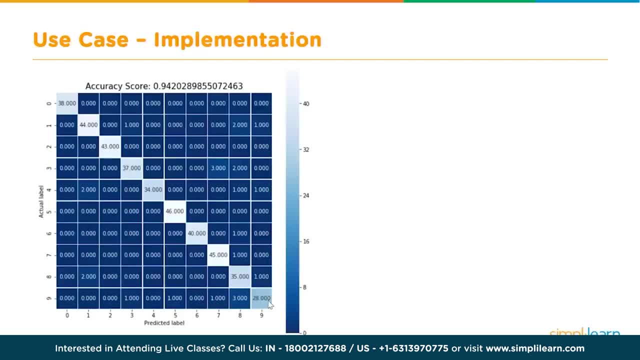 In all other cells, But that is like 100% accurate model. Okay, So that is the gist of how to use this matrix. How to use this confusion matrix- I know the name Is a little funny sounding: Confusion matrix. 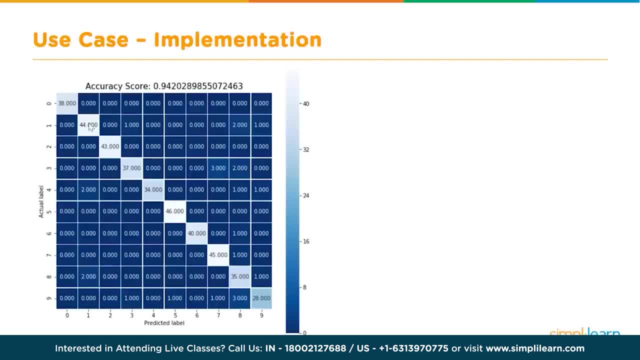 But actually it is not very confusing, It is very straight forward. So you are just plotting What is the labeled information Or what is the actual data That is also known as the ground truth. sometimes These are some fancy terms that are used. 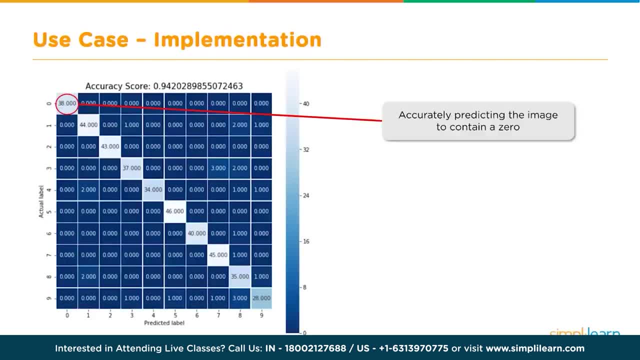 So predicted label and the actual label. That is all it is. So we are showing a little bit more information here. So 38 have been predicted And here you will see that All of them have been predicted correctly. There have been 38 zeros. 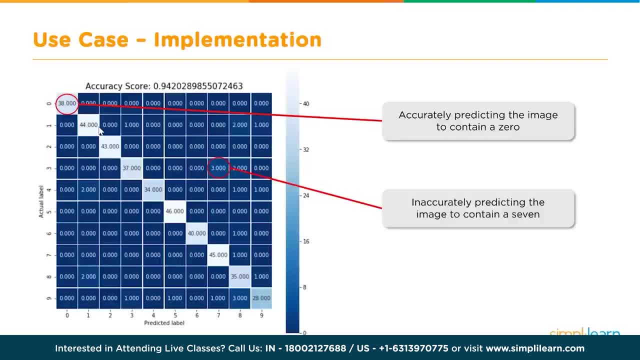 And the predicted value And the actual value is exactly the same, Whereas in this case It has 47 plus 5.. 42 have been fed the images. 42 images are Of digit 3. And the accuracy is: 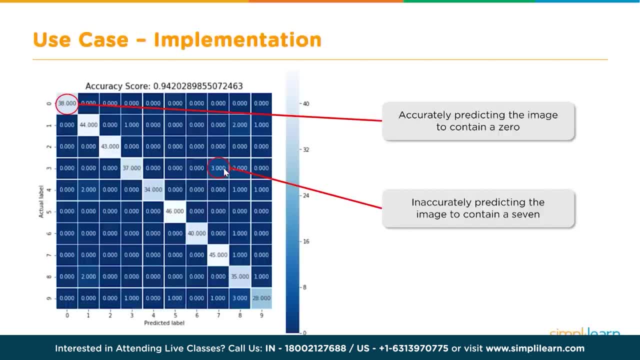 Only 37 of them have been accurately Predicted. 3 of them have been predicted as number 7. And 2 of them have been predicted as number 8. And so on and so forth. Okay, So with that, let us go into Jupyter Notebook. 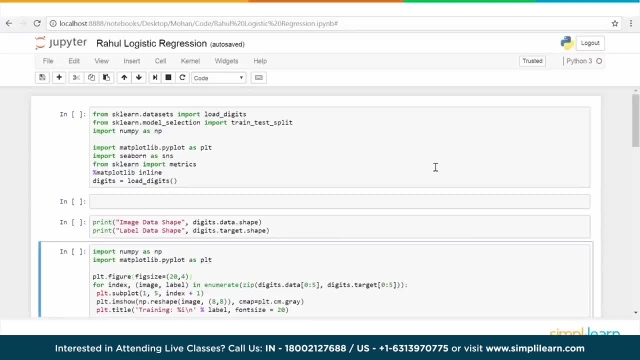 And see how the code looks. So this is the code In Jupyter Notebook For logistic regression. In this particular demo, What we are going to do is train our model To recognize digits, Which are the images Which have digits from. 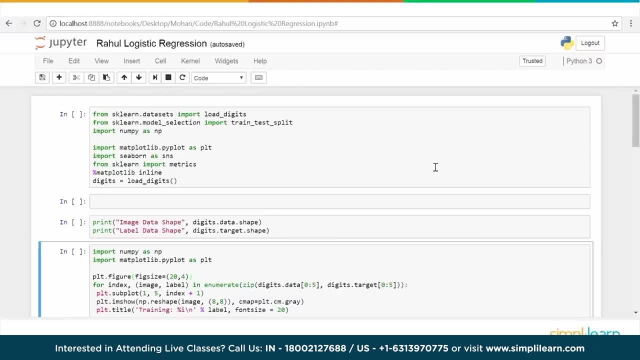 Let us say 0 to 5. Or 0 to 9. And then we will see How well it is trained And whether it is able to predict these numbers correctly Or not. So let us get started. So the first part is as usual. 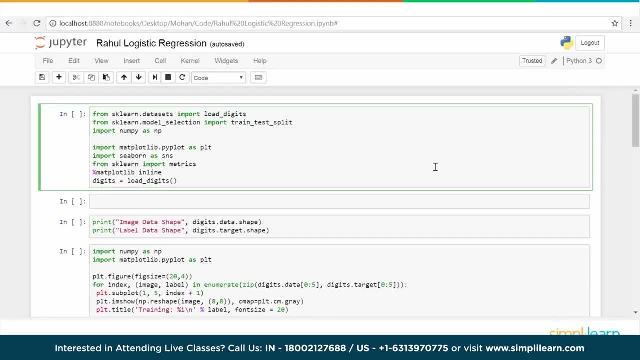 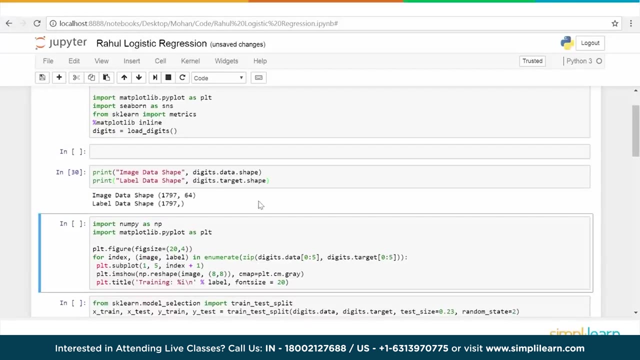 We are importing some libraries Which are required, And then the last line in this block Is to load the digits. So let us go ahead And run this code, Then here we will Visualize the shape of these digits So we can see here. 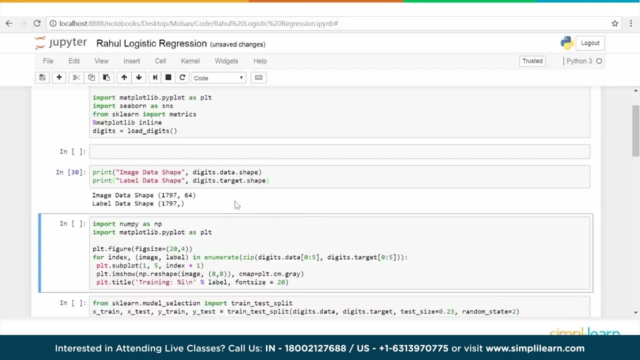 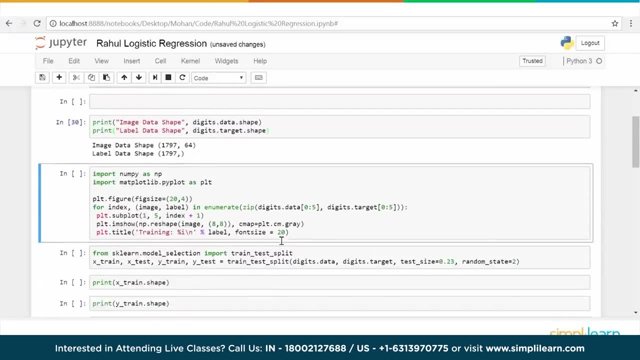 If we take a look, This is how the shape is: 1797 by 64.. These are like 8 by 8 images. So that is what is reflected in this shape. Now, from here onwards, We are basically Using some of the libraries that are required. 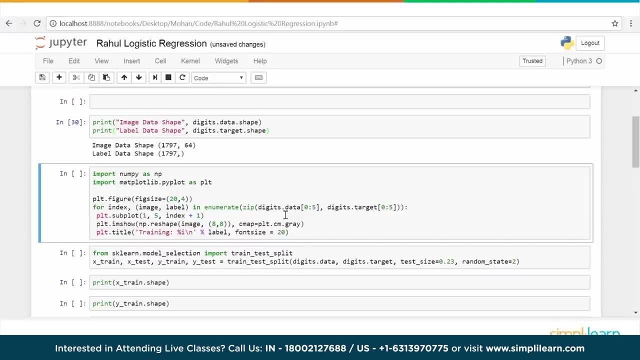 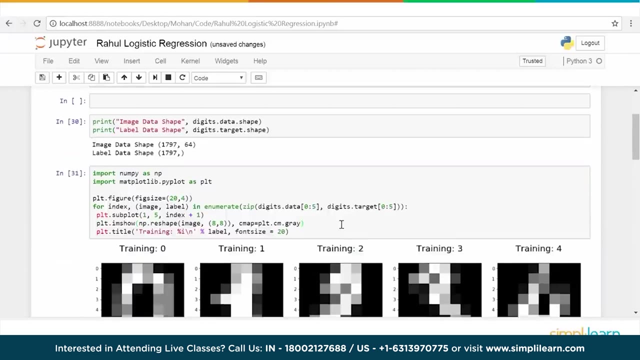 Like numpy and matplot, And we will take a look at Some of the sample images That we have loaded. So this one, for example, Creates a figure, And then we go ahead And take a few sample images To see how they look. 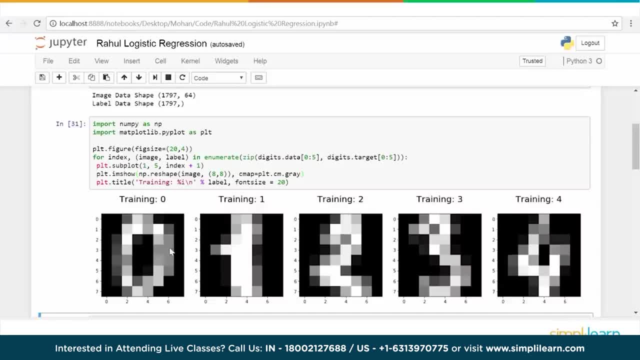 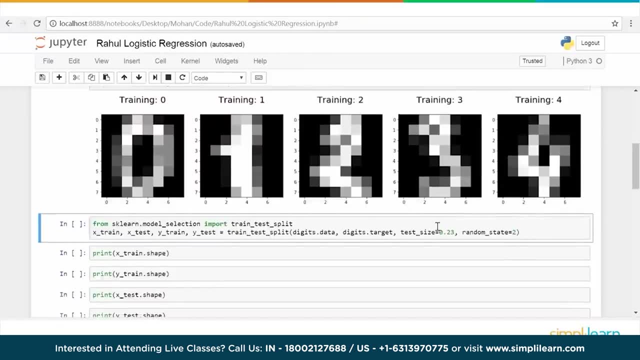 So let me run this code So that it becomes easy to understand. So these are about 5 images, Sample images, that we are looking at: 0,, 1,, 2,, 3,, 4.. This is how the data is. 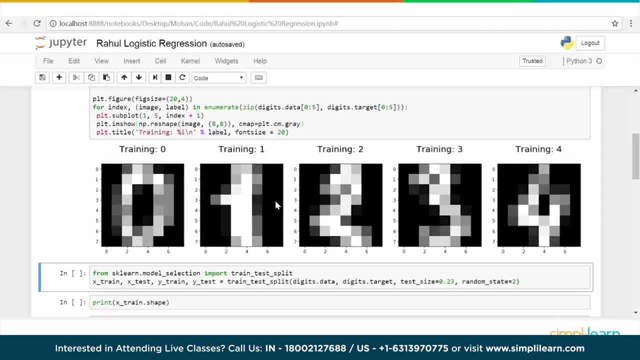 And based on this We will actually train Our logistic regression model And then we will test it And see how well it is able to recognize. So the way it works is The pixel information. So, as you can see here, This is an 8 by 8 pixel. 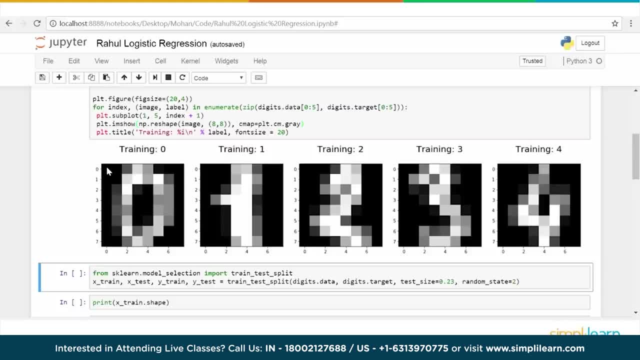 Kind of a image And each pixel, Whether it is activated or not activated, That is the information Available for each pixel. So, based on the pattern Of this activation and non activation Of the various pixels, This will be identified As a 0, for example. 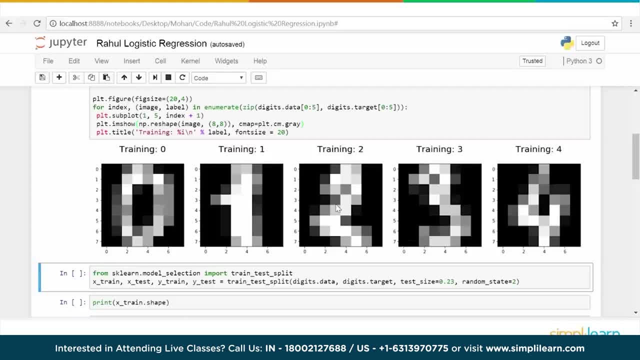 Similarly, as you can see. So overall, each of these numbers Actually has a different pattern Of the pixel activation, And that is pretty much That our model needs to learn. For which number? What is the pattern of the activation of the pixels? 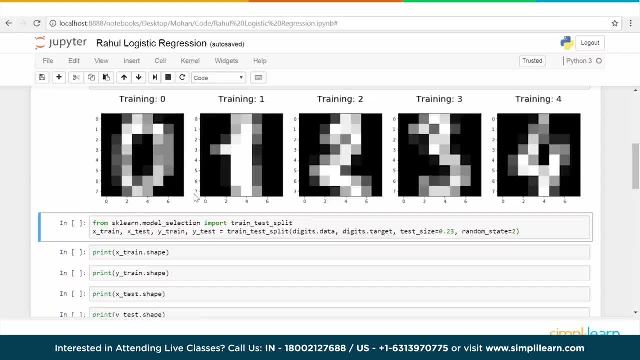 So that is what we are going to Train our model. So the first thing we need to do Is to split our data Into training and test. data set Right. So whenever we perform any training, We split the data into training and test. 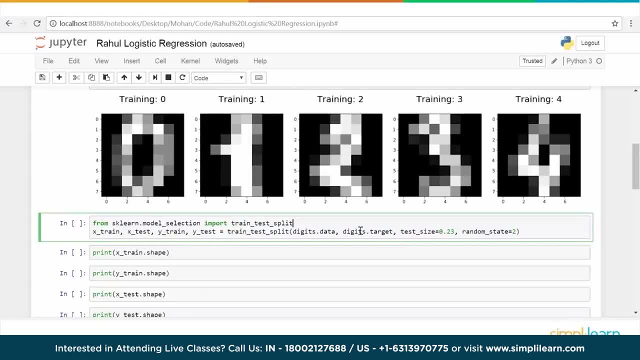 So that the training data set Is used to train the system. So we pass this probably Multiple times And then we test it with the test data set And the split is usually In the form of: And there are various ways in which you can split this data. 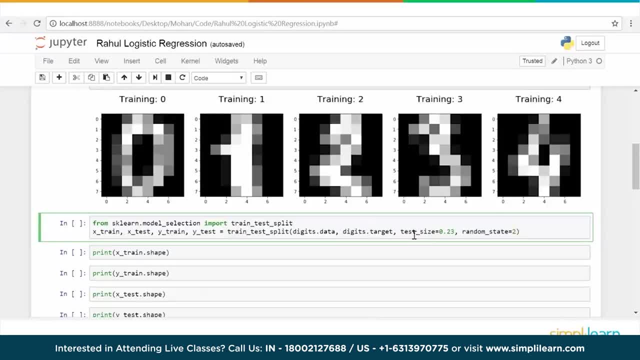 It is up to the individual preferences. In our case, here We are splitting in the form of 23 and 77. So when we say test size As 0.23. That means 23 percent Of the entire data. 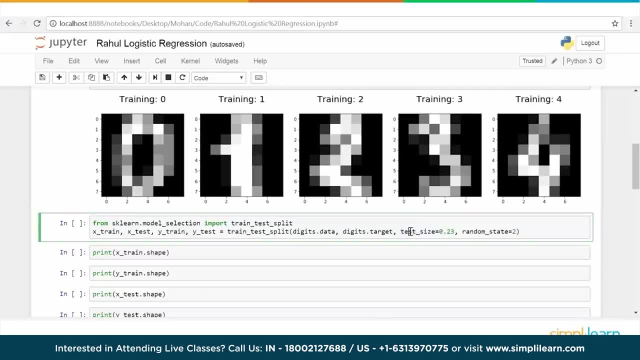 Is used for testing And the remaining 77 percent Is used for training. So there is a readily available function Which is called Train test split. So we don't have to write any special code For the splitting. It will automatically split the data. 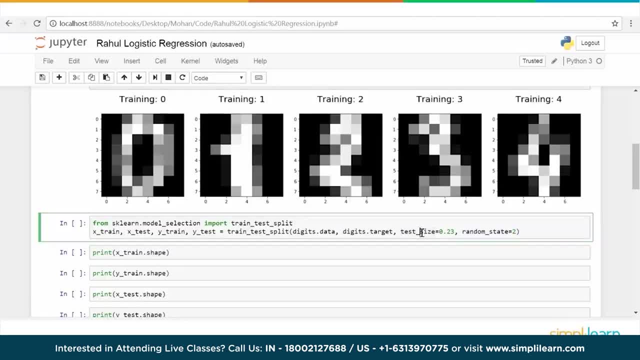 Based on the proportion that we give here, Which is test size. So we just give the test size, Automatically training size will be determined And we pass the data That we want to split And the results will be stored in X underscore train. 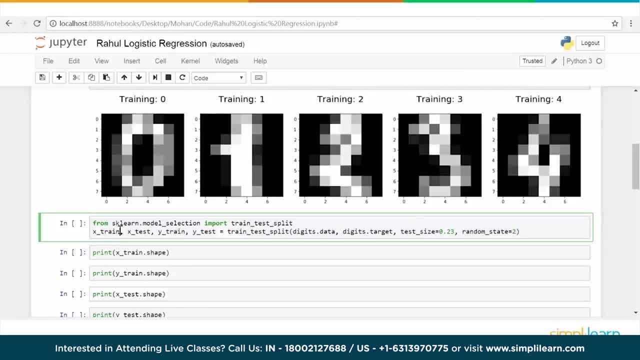 And Y underscore train For the training data set. And what is X underscore train? These are the features Right. X underscore train is the label Right. So in this case, what happens is We have the input value, Which is, or the features value. 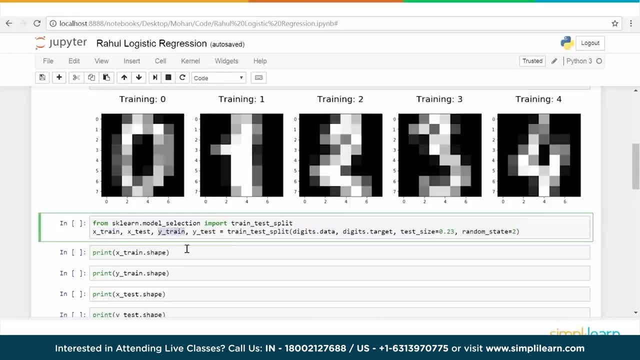 Which is in X underscore, train, And since this is labeled data For each of them, Each of the observations, We already have the label information Saying whether this digit is a 0. Or a 1. Or a 2., So that this is what will be used. 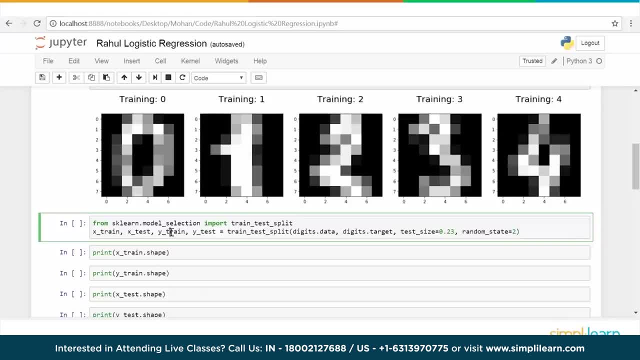 For comparison. For each observation It will compare with this, Right? So this is the label. So the same way, X underscore train- Y underscore train Is for the training data set. X underscore test- Y underscore test Is for the test data set. 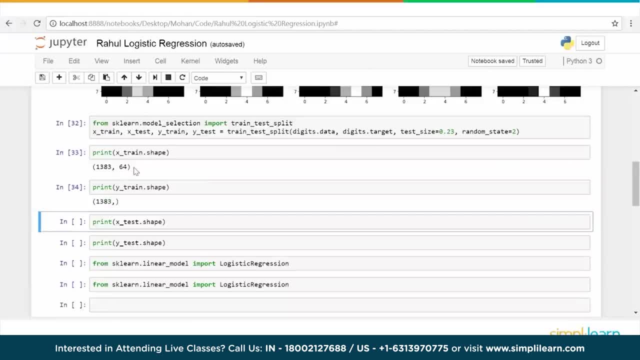 Okay, So let me go ahead and execute this code as well, And then we can go and check quickly: X underscore: train has 1383.. Because there is nothing like The second part is not required here. And then X underscore: test shape. 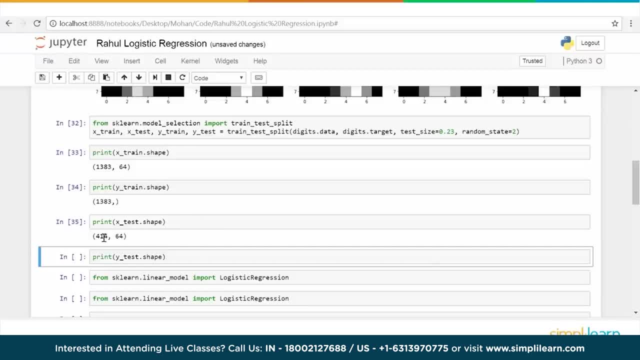 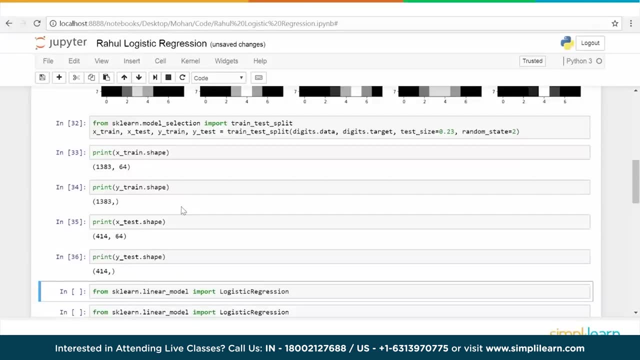 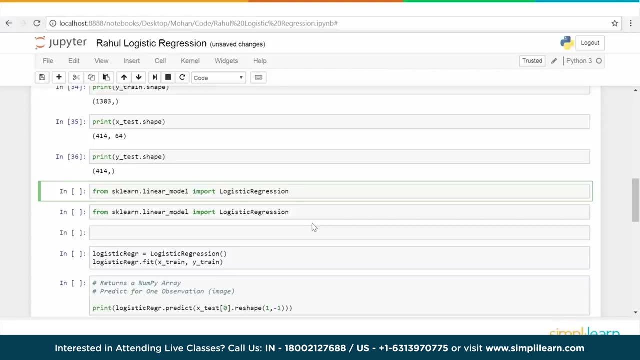 We see is 414.. So actually there are 414 observations In test And 1383 observations in train. So that's basically What these four lines of code are saying. Okay, Then we import the logistic regression library And which is a part of scikit learn. 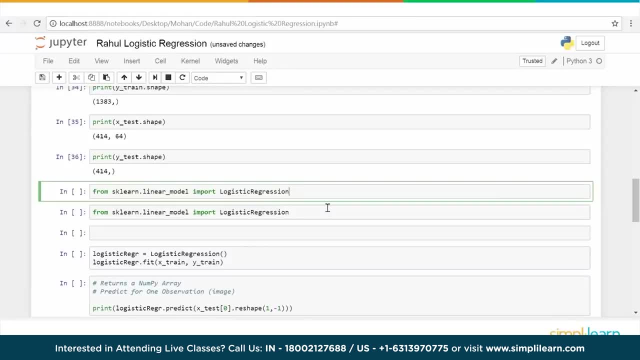 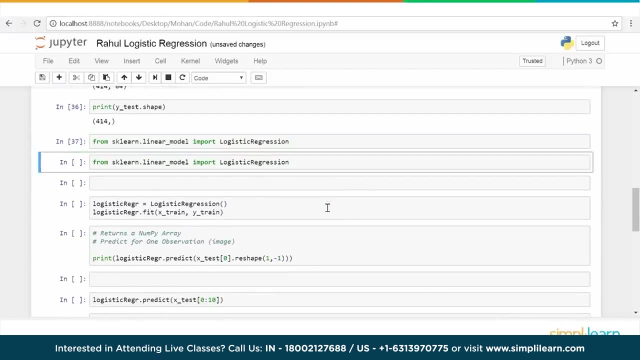 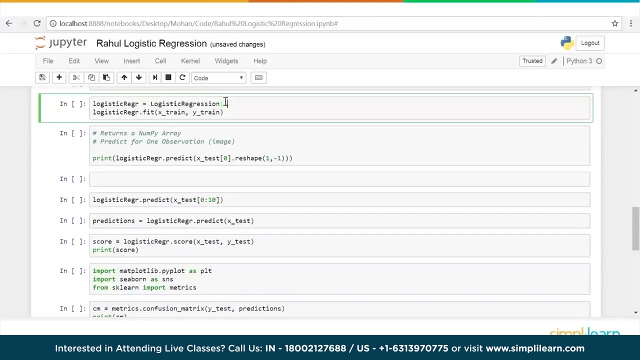 So We don't have to implement The logistic regression process itself. We just call these the function, And let me go ahead and execute that So that We have the logistic regression library imported. Now We create an instance of logistic regression. 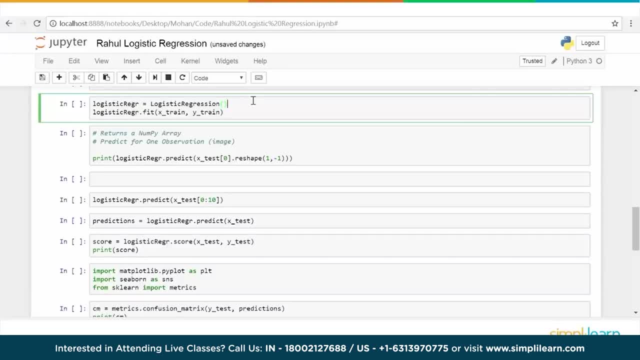 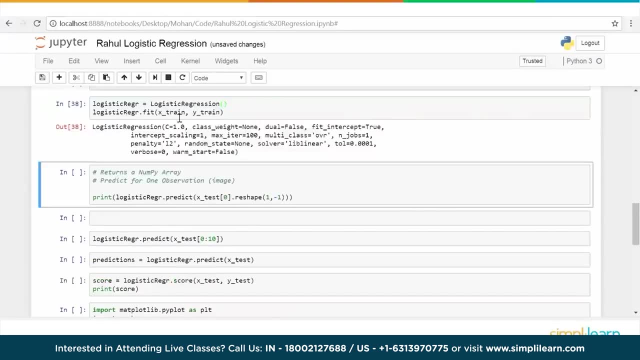 Right, So logistic regr Is an instance of logistic regression And then we use that For training our model. So let me first execute this code. So these two lines: This is the instance of logistic regression model, And then the second line. 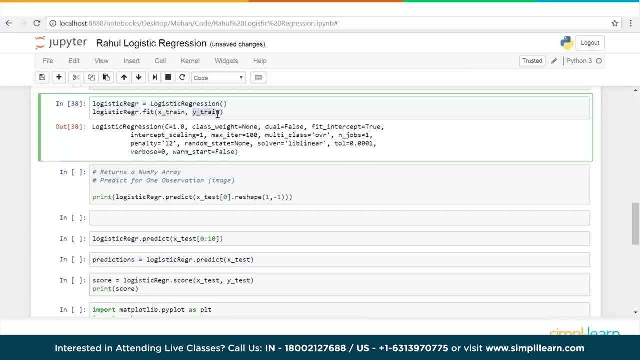 Is where we are passing our data, The training data set, And this is our- The predictors, And this is our target. We are passing this data set To train our model, Alright. So once we do this, In this case the data is not large. 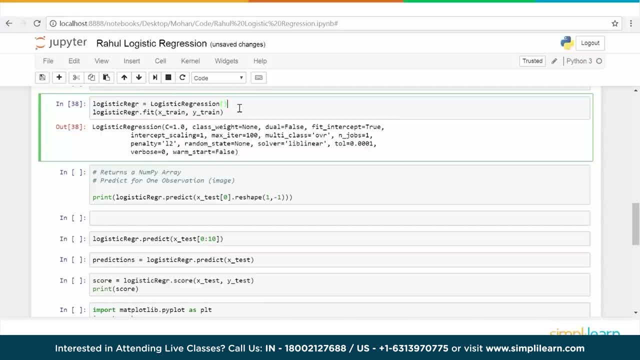 But by and large The training is what takes usually a lot of time. So we spend in machine learning, We spend a lot of time For the training part of it. So here the data set is relatively small, So it was pretty quick. 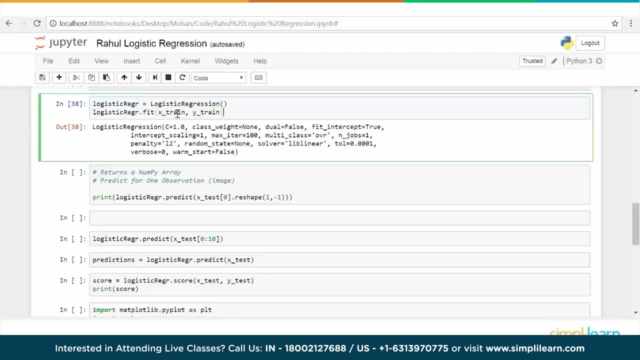 So now our model has been trained Using the training data set, And we want to see How accurate this is. So what we will do is We will test it out in probably phases, So let me first try out How well this is working for. 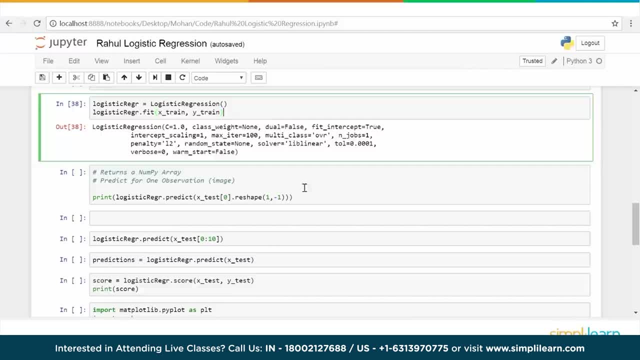 One image. I will just try it out with one image, The first entry in my test data set, And see whether it is Correctly predicting or not. And in order to test it, So for training purpose, We use the fit method. 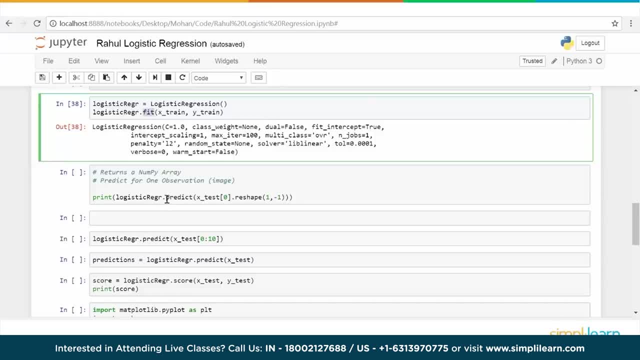 There is a method called fit, Which is for training the model And once the training is done, If you want to test for a particular value- New input- You use the predict method. So let's run the predict method And we pass this particular image. 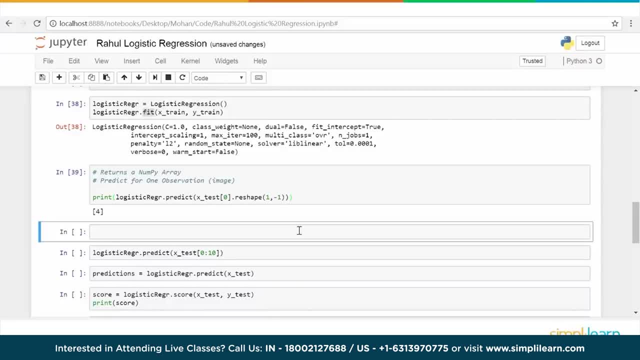 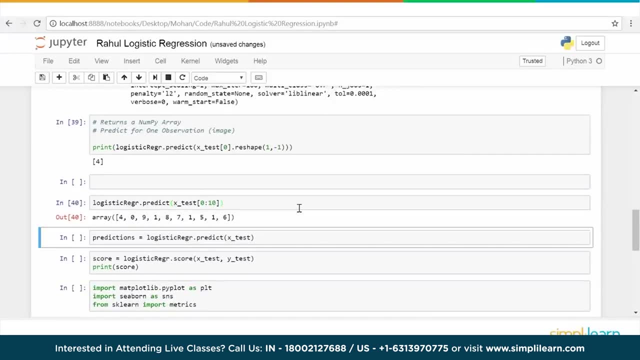 And we see that The shape is 4.. So let's try a few more. Let me see for the next 10.. Seems to be fine, So let me just go ahead And test the entire data set. That's basically what we will do. 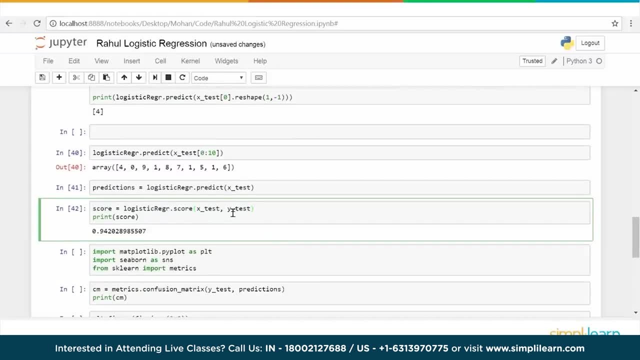 So now we want to find out How accurately this has performed. So we use the score method To find what is the percentage Of accuracy, And we see here that it has performed Up to 94% accurate. So that's on this part. 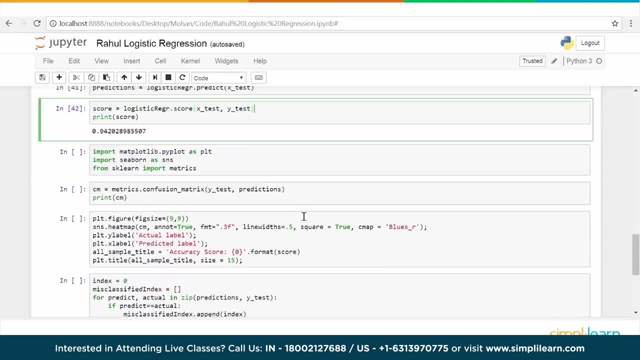 We can also see This accuracy Using what is known as confusion matrix. So let us go ahead And try that as well, So that we can also visualize How well this model Has done. So let me execute this piece of code. 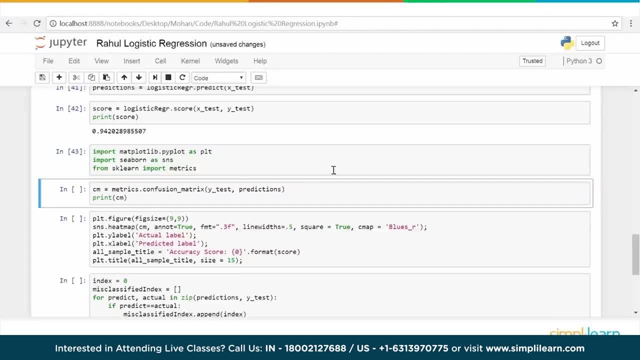 Which will basically import some of the libraries That are required, And we basically create A confusion matrix, An instance of confusion matrix, By running confusion matrix And passing these values. So we have. So this confusion underscore matrix Method takes two parameters. 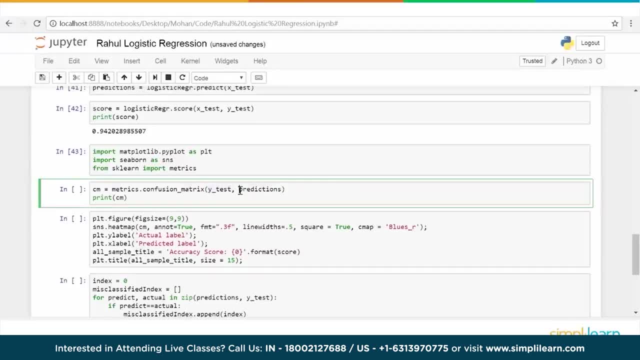 One is the y underscore test And the other is The prediction. So what is the y underscore test? These are the labeled values Which we already know For the test data set, And predictions are what the system has predicted For the test data set. 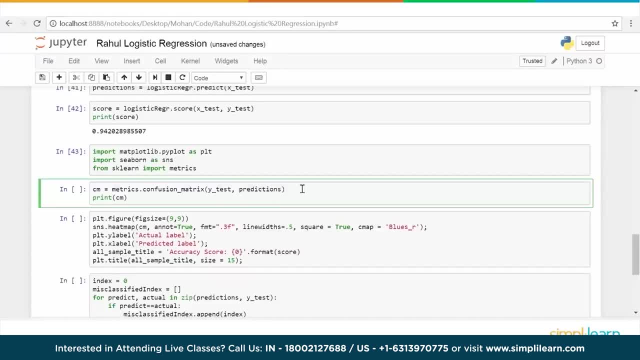 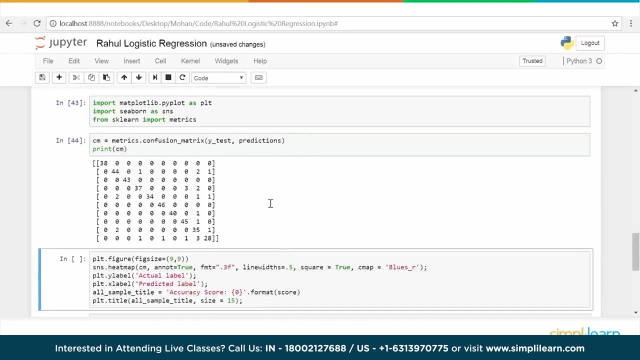 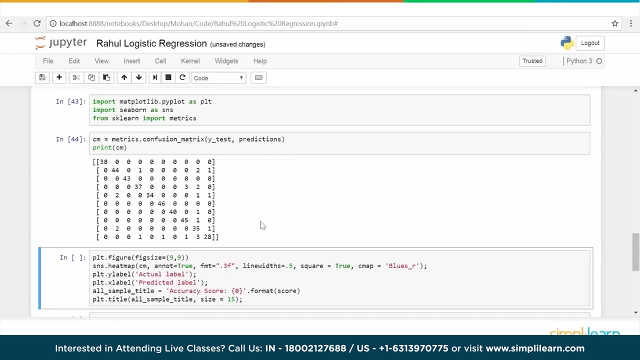 Okay, So this is known to us As the model has generated. So we kind of create the confusion matrix And we will print it And this is how the confusion matrix looks. As the name suggests, It is a matrix, And the key point out here is that 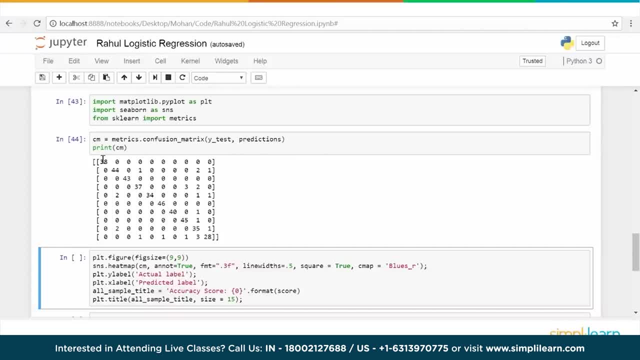 The accuracy of the model Is determined by How many numbers are there in the diagonal. The more the numbers In the diagonal, The better. the accuracy is Okay And, first of all, The accuracy of the matrix Is equal to the number of observations. 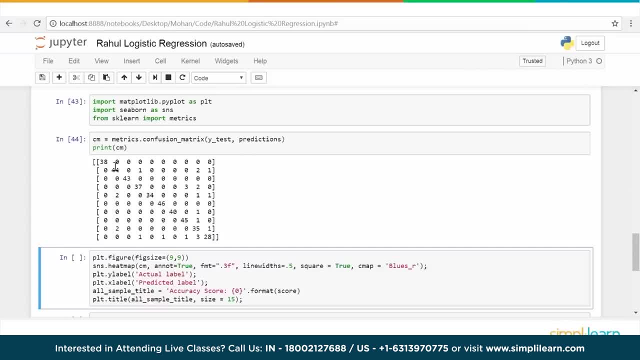 In the test data set. That is the first thing. So if you add up all these numbers, That will be equal to the number of observations In the test data set, And then out of that The maximum number of them should be in the diagonal. 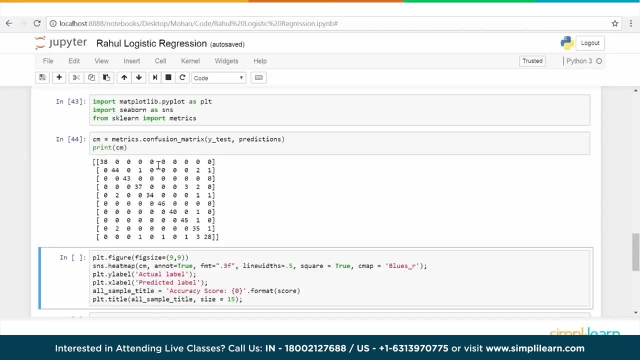 That means the accuracy is pretty good. If the numbers in the diagonal are less And in all other places There are a lot of numbers, Which means the accuracy is very low, That indicates a correct prediction. This means that the actual value 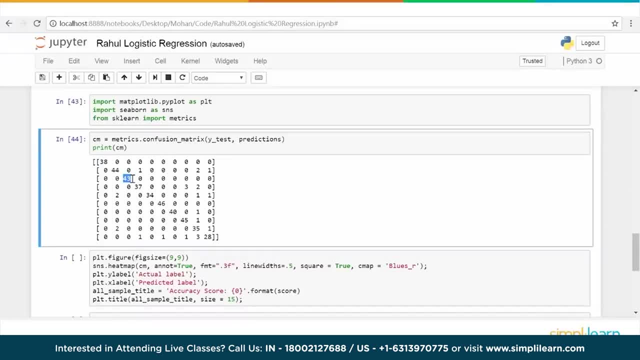 Is same as the predicted value. Here again, actual value is same as the predicted value, And so on. So the moment you see a number here, That means the actual value is something And the predicted value is something else. Similarly, here The actual value is something. 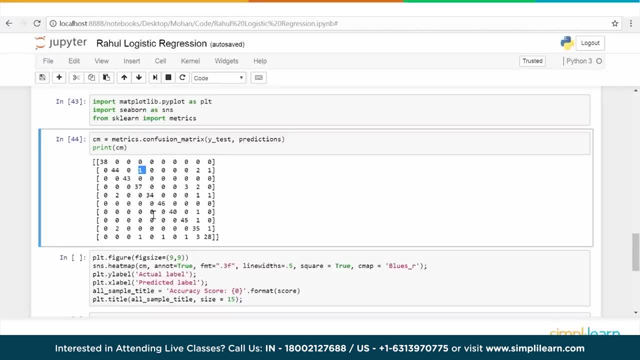 And the predicted value is something else. So that is basically How we read the confusion matrix. Now how do we find the accuracy? You can actually Divide the total values In the diagonal, So it is like 38 plus 44 plus 43.. 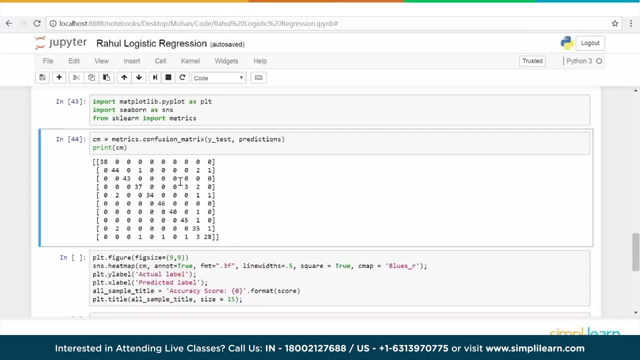 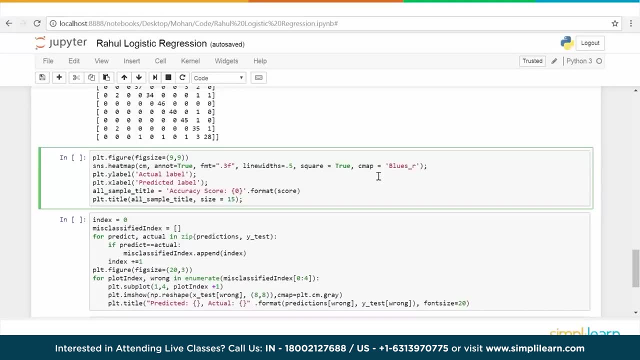 And so on, And divide that by the total number of Test observations. That will give you the percentage accuracy Using a confusion matrix. Now let us visualize this confusion matrix In a slightly more sophisticated way, Using a heat map. So we will create a heat map. 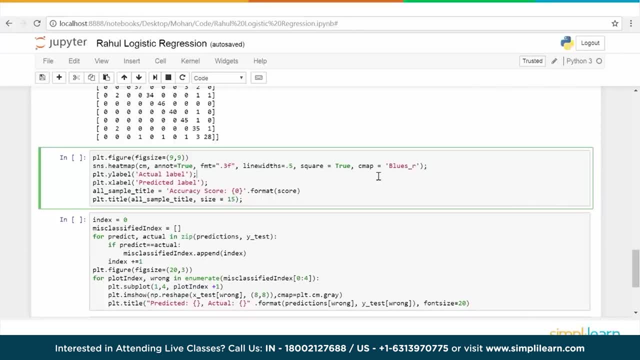 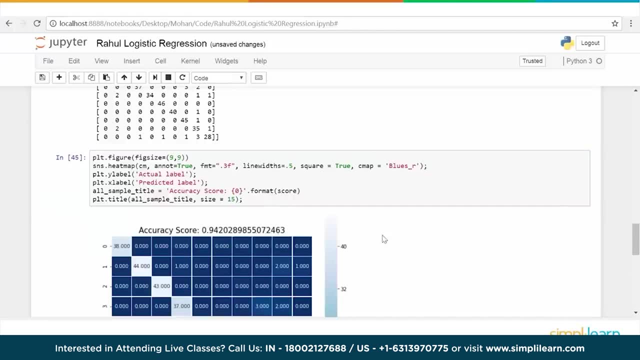 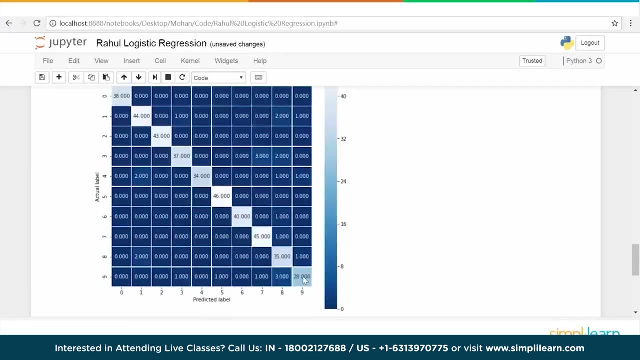 With some, We will add some colors as well. It is like a more visually Appealing. So that is the whole idea. So if we Let me run this piece of code And this is how the heat map looks And as you can see here, 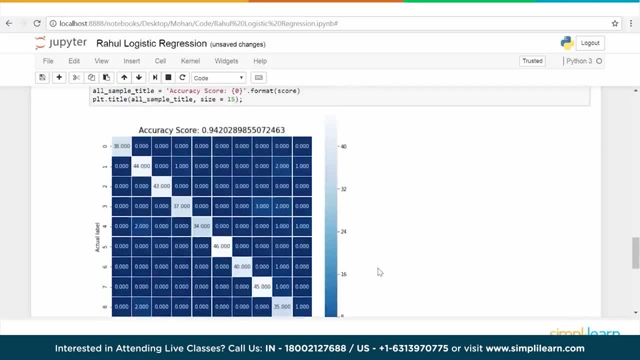 The diagonals again Are: all the values are here, Most of the values, So, which means reasonably, This seems to be reasonably accurate And, yeah, Basically the accuracy score is 94%. This is calculated, as I mentioned, By adding all these numbers. 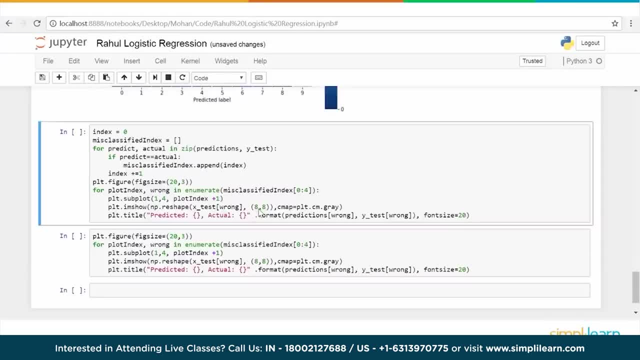 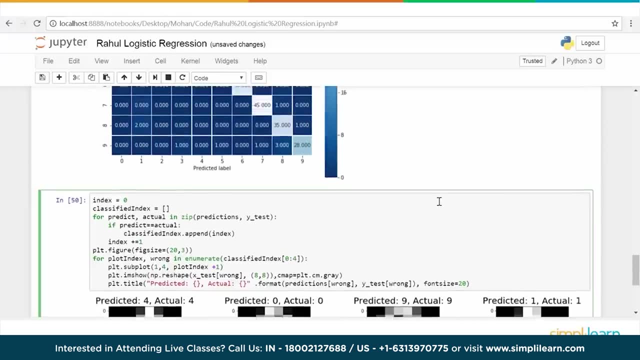 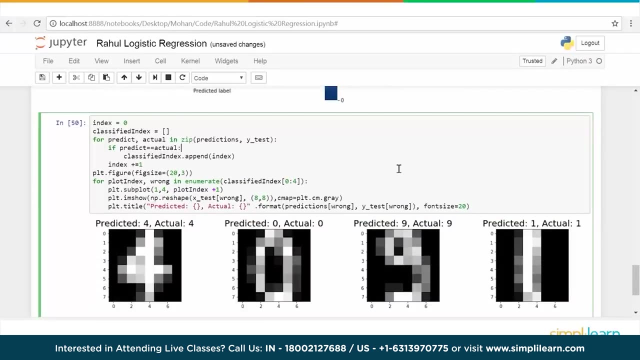 To the set. So this is the confusion matrix For logistic regression. Alright, So now that we have seen The confusion matrix, Let us take a quick sample And see how well The system has classified, And we will take a few examples. 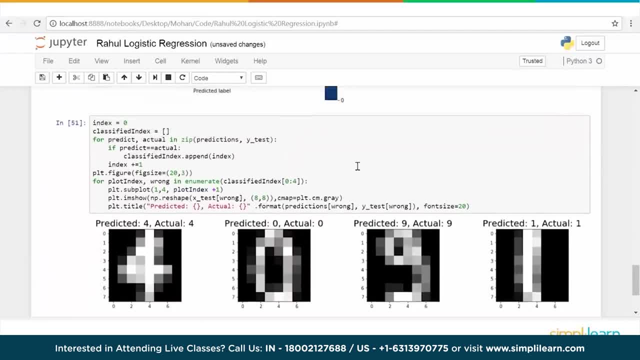 Of the data. So if we see here, We picked up randomly a few of them, So this is number 4.. Which is the actual value, Number 4.. This is an image of 0. So the predicted value is also 0.. 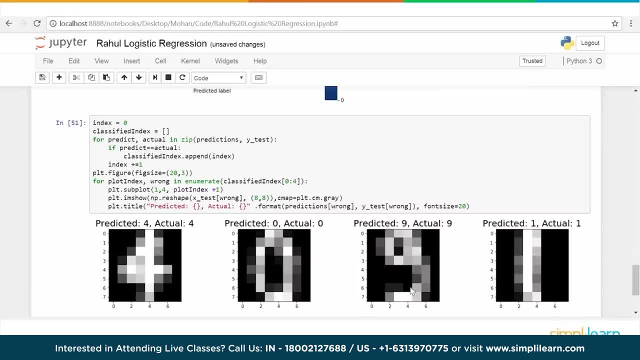 Actual value is, of course, 0.. Then this is the image of 9.. So this has also been predicted correctly: 9 and actual value is 9.. And this is the image of 1.. And again, This has been predicted correctly. 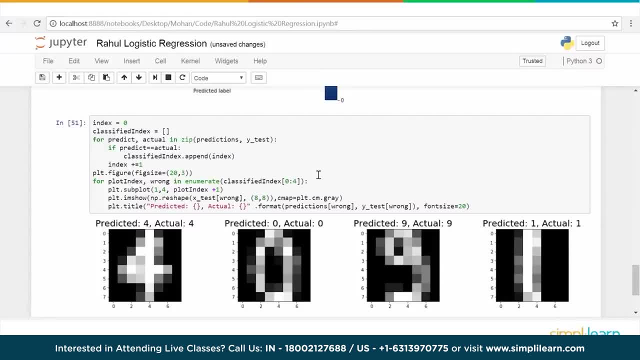 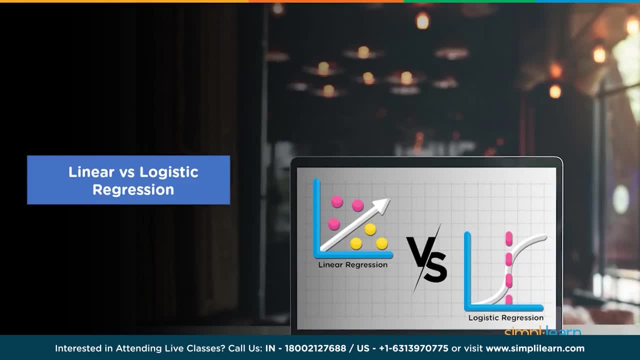 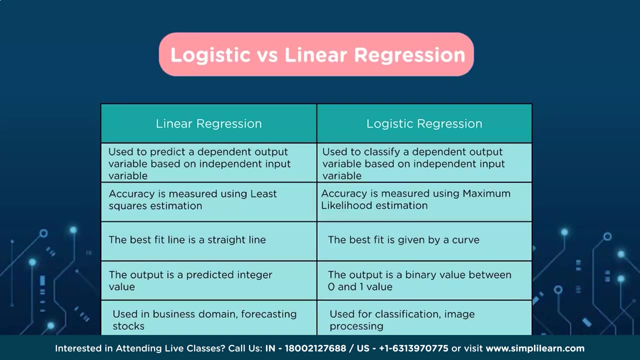 As like the actual value. So this was a quick demo Of logistic regression, How to use logistic regression To identify images And the regression models That come out of this. So we put them side to side. We have our linear regression. 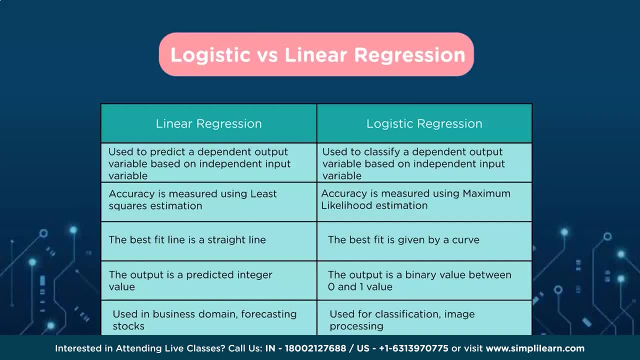 Which is a predictive number Used to predict a dependent output variable Based on independent input variable. Accuracy is measured Using least squares estimation. So that is where you take. You can also use absolute value. The least squares is more popular. There is reasons for that. 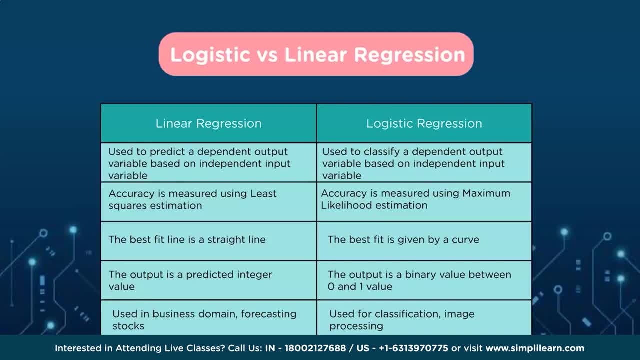 Mathematically And also for computer running. But it does give you an accuracy Based on the least squares estimation. The best fit line Is a straight line And clearly that is not always used In all the regression models. There is a lot of variations on that. 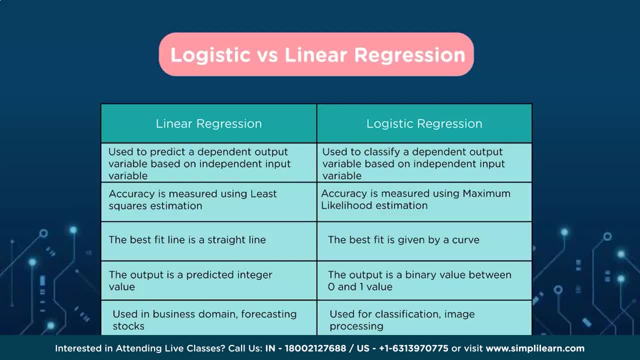 The output is a predicted integer value. Again, this is what we are talking about. We are talking about linear regression And we are talking about regression. It means the numbers coming out. Linear usually means we are looking for that line Versus a different model. 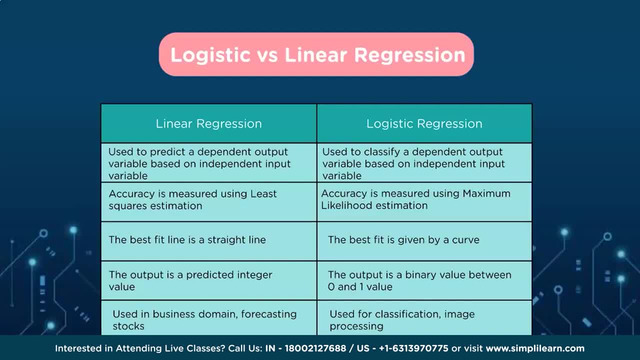 And it is used in business models. In the business domain- Forecasting stocks- It is used as a basis Of most predictions with numbers. So if you are looking at a lot of numbers, You are probably looking at A linear regression model. 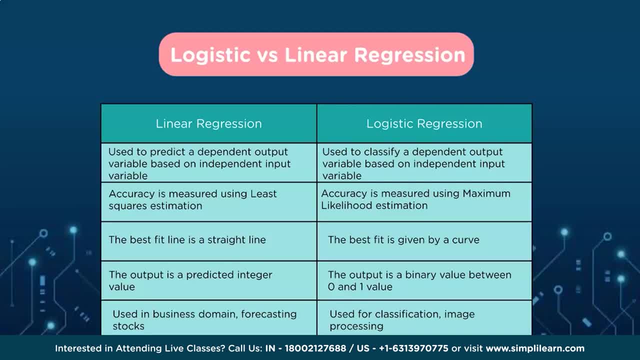 For instance, If you do just the high lows Of the stock exchange- And you are going to take a lot more of that If you want to make money off the stock, You will find that the linear regression model Fits probably better than. 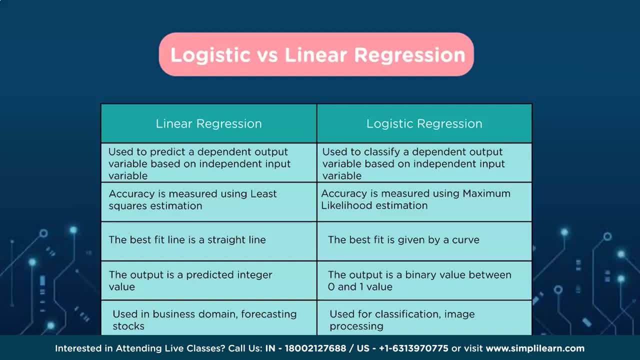 Almost any of the other models, Because they are numbers. They are just a straight set of numbers. You have a high value, A low value, Volume, That kind of thing. So when you are looking at something that is straight numbers And are connected in that way, 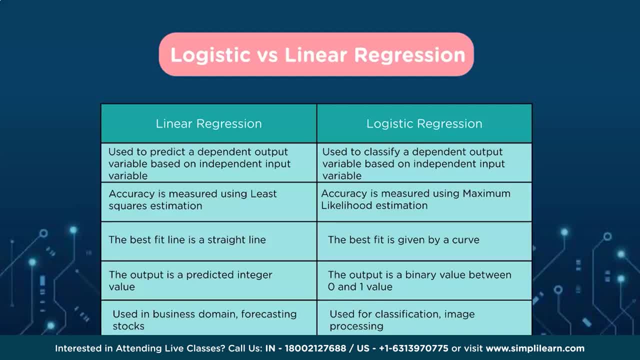 Usually you are talking about a linear regression model, And that is where you want to start: A logistic regression model Used to classify dependent output variable Based on independent input variable. So, just like the linear regression model And like all of our machine learning tools, 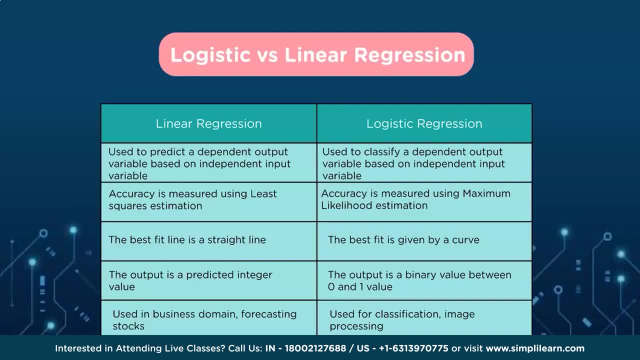 You have your features coming in, So in this case you might have An image or something like. that Is probably the very popular thing right now: Labeling broccoli and vegetables Or whatever. Accuracy is measured using Maximum likelihood estimation. The best fit is given by a curve. 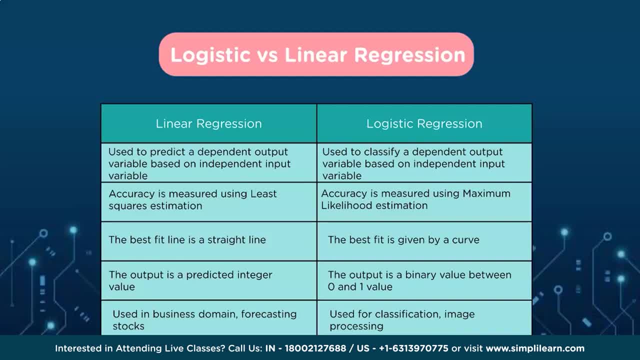 And we saw that When we are talking about linear regression, You are definitely talking about a straight line, Although there is other regression models That don't use straight lines, And usually when you are looking at Linear regression, The math, as you saw, 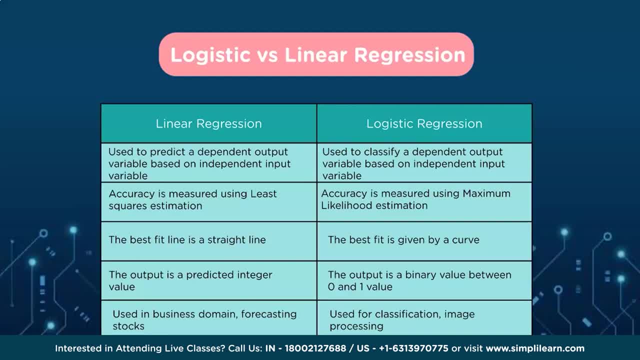 Was still kind of a Euclidean line, But it has now Got that sigmoid activation Which turns it into a heavily weighted curve, And the output Is a binary value between 0 and 1. And it is used for classification, Image processing, as I mentioned. 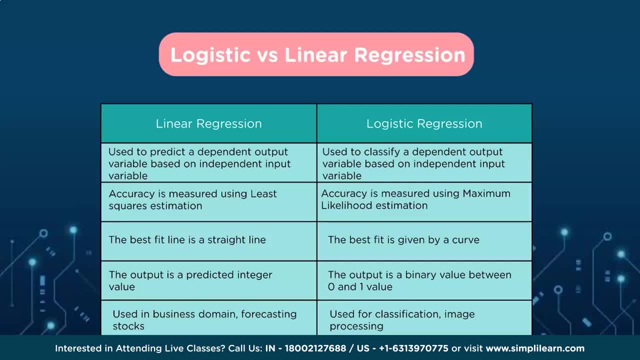 Is what people usually think of, Although They use it for classification Of Like a window of things. So you could take a window of stock history And you could Generate classifications based on that And separate the data that way, If it is going to be that this particular pattern occurs. 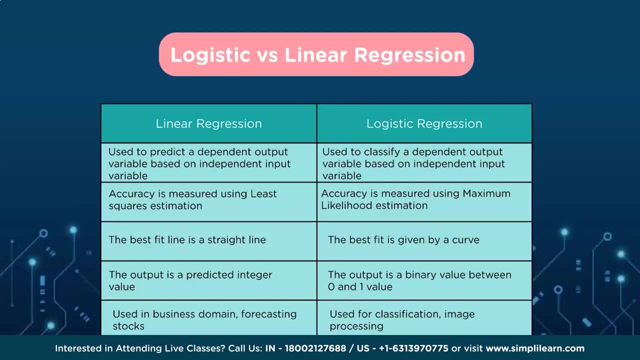 It is going to be upward trending Or downward trending. In fact, a number of stock Traders Use that Not to tell them how much to bid or what to bid, But they use it as to whether It is worth looking at the stock or not. 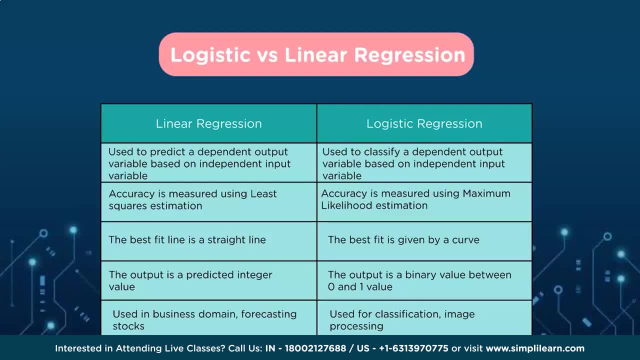 Whether the stock is going to go down or go up, And it is just a 0 or 1.. So let's do a demo So you can get a picture of what this looks like in Python code. Let's predict the price. 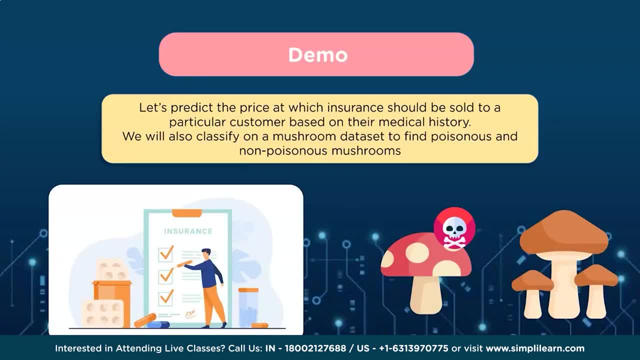 At which insurance should be sold To a particular customer Based on their medical history. We will also classify on a mushroom data set To find the poisonous And non-poisonous mushrooms. And when you look at these two data, The first one, 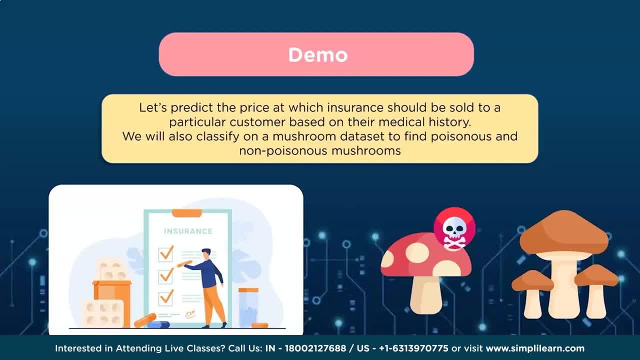 We are looking at the price. So the price is a number, So let's predict the price Which the insurance should be sold to. And the second one We are looking at: either it is poisonous or not poisonous. So first off, Before we begin the demo, 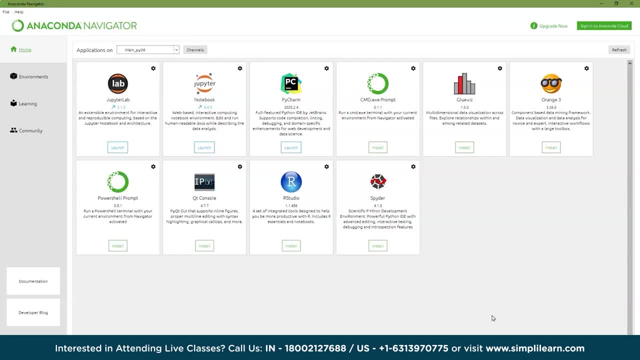 I am in the Anaconda Navigator. In this one I have loaded The Python 3.6.. And using the Jupyter Notebook- And you can use Jupyter Notebook by itself- You can use the Jupyter Lab, Which allows multiple tabs. 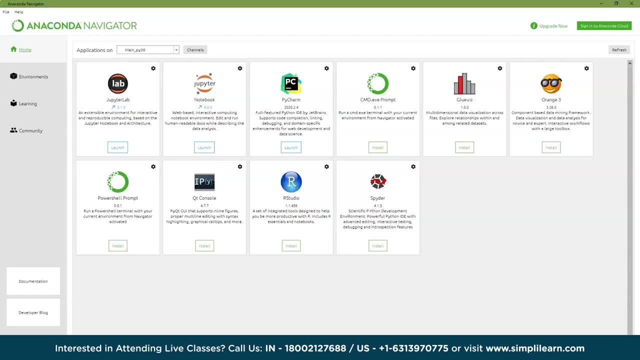 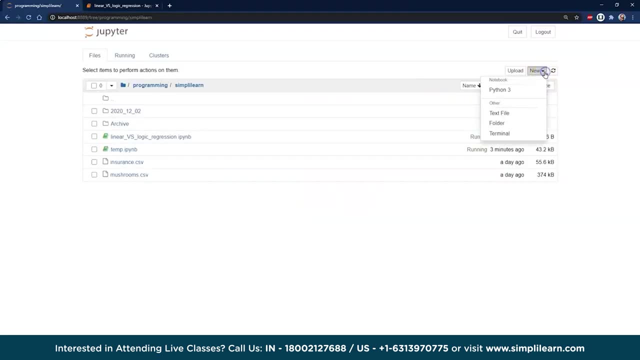 It is basically the notebook With tabs on it, But the Jupyter Notebook is just fine And it will go into Google Chrome For my Internet Explorer And from here we open up new And you will see Python 3.. And again, this is loaded with Python 3.6.. 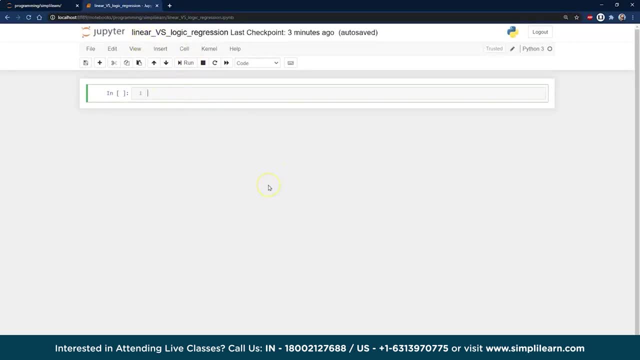 And we are doing the Linear versus logic, Regression or Logit. You will see, L-O-G-I-T Is one of the One of the names that kind of pops up When you do a search on here, But it is a logic. 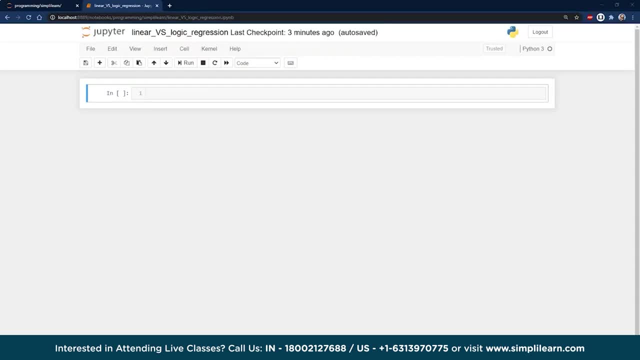 We are looking at the logistic regression models And we will start With the linear regression Because it is easy to understand: You draw a line through stuff And so in programming We got a lot of stuff to unfold here In our startup. 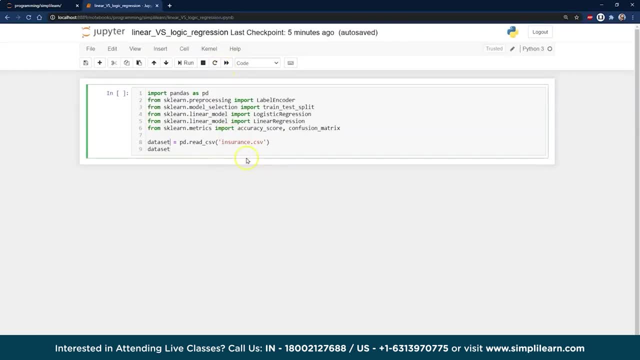 As we preload all of our different parts. Let's go ahead and break this up. We have, at the beginning, Import pandas, So this is our data frame. It is just a way of storing the data. Think of a When you talk about a data frame. 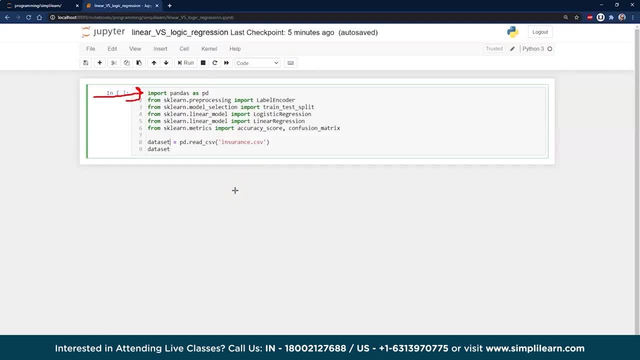 Think of a spreadsheet: Rows and columns. It is a nice way of viewing the data. And then we have: We are going to be bringing in our Pre-processing label encoder. I will show you what that is When we get down to it. 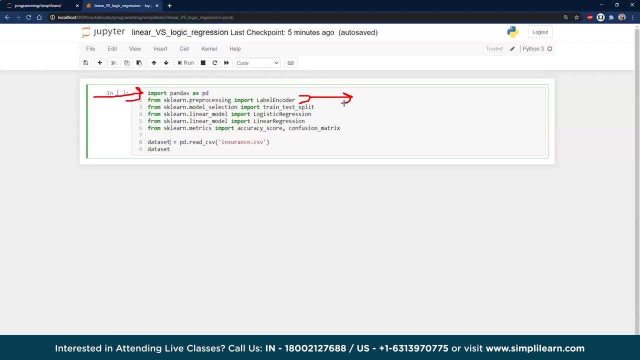 It is easier to see in the data. But there is some data in here Like sex. It is male or female, So it is not like an actual number. It is either one or the other. That kind of stuff ends up being encoded. 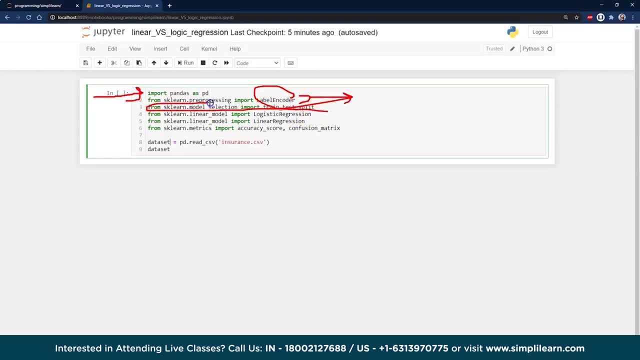 That is what this label encoder is. If you are going to build a model, You do not want to use all of the data. You want to use some of the data And then test it To see how good it is. It cannot have seen the data you are testing on. 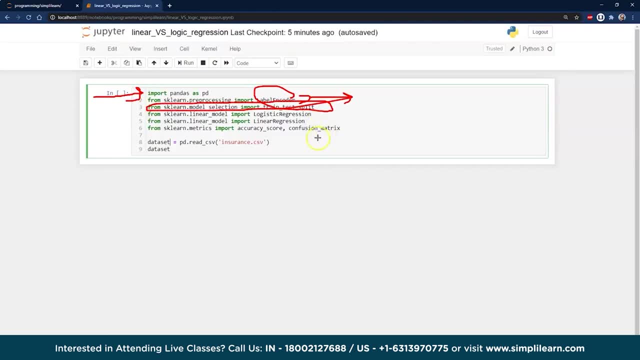 Until you are ready to test it on there And see how good it is. And then we have our logistic regression model, Our categorical one, And then we have our linear regression model. These are the two, These right here. Let me just clear all that. 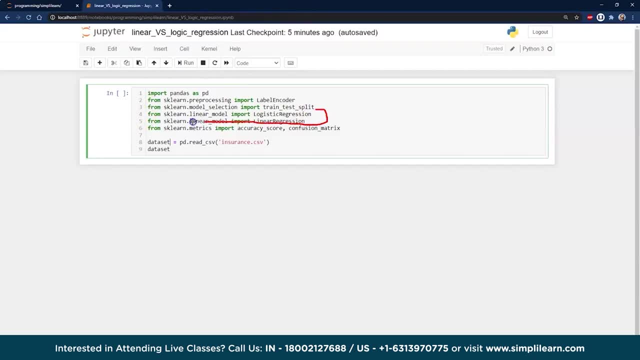 There we go. Here are what this is all about: Logistic versus linear. Is it categorical? Are we looking for a true or false, Or are we looking for a specific number? And then finally, Usually at the very end, We have to ask: 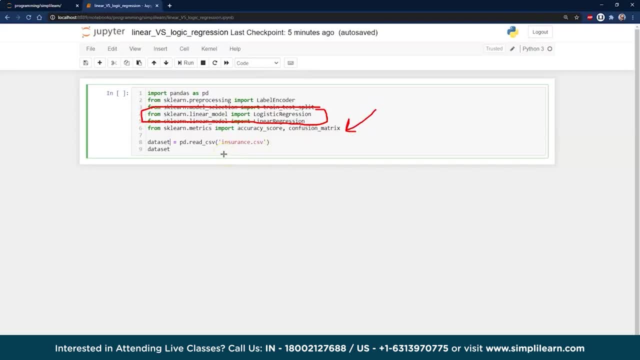 How accurate is our model? Did it work? If you are trying to predict something- In this case we are going to be doing Insurance costs- How close to the insurance cost Does it measure What you expect it to be If you are an insurance company? 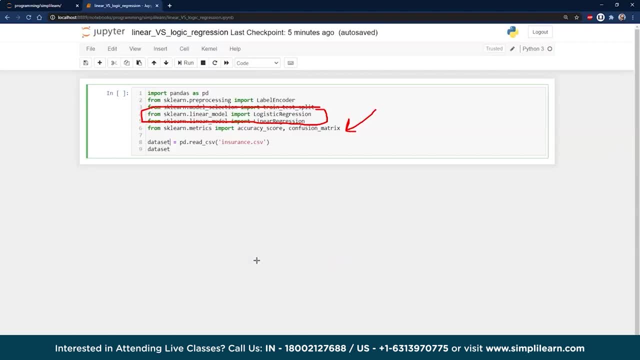 You don't want to promise to pay everybody's medical bill And not be able to, And, in the case of the mushrooms, You probably want to know Just how much at risk you are For following this model As to far as whether you are going to. 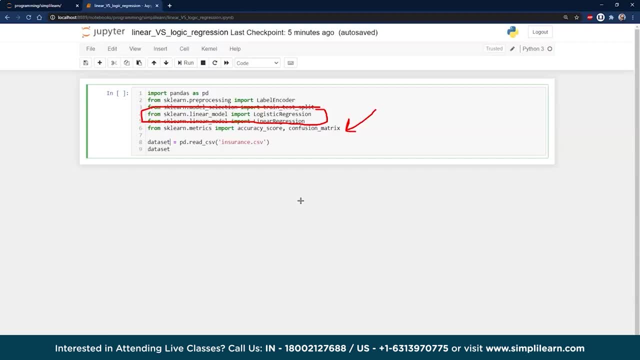 Eat a poisonous mushroom and die or not. So we will look at both of those And we will talk a little bit more About the shortcomings And the value Of these different processes. So let's go ahead and run this. This has loaded the data set on here. 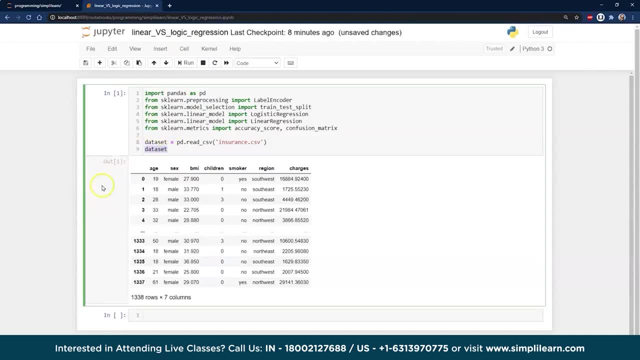 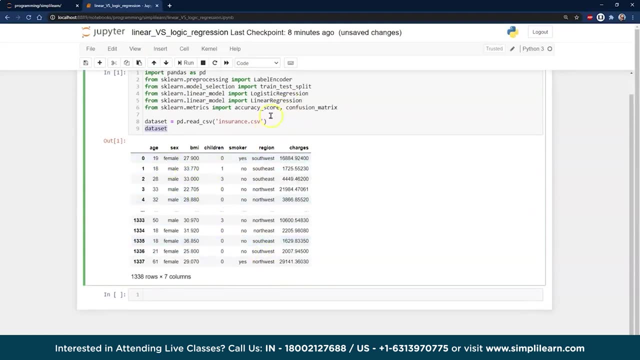 And then, because we are in Jupiter Notebook, I don't have to put the print on there, We just do data set And it prints out all the different data on here And you can see here for our insurance, Because that is what we are starting with. 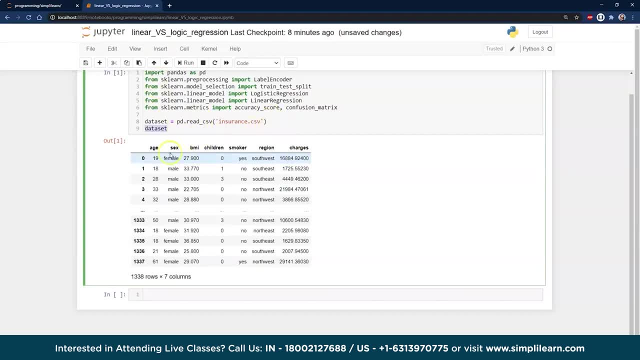 We are loading that with our pandas And it prints it in a nice format Where you can see the age, Sex, Body mass index, Number of children, Smoker. This is what we need to know. To give you a quote, 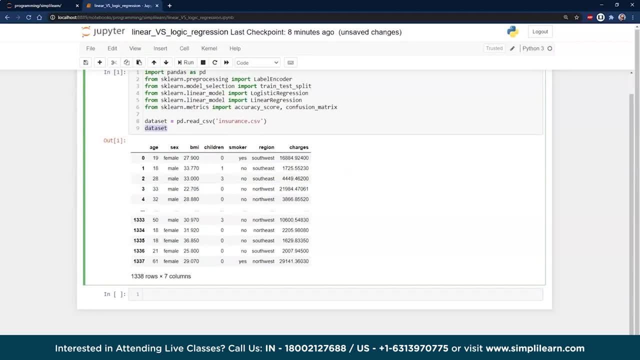 For what we are going to charge you for your insurance, And you can see that it has 1,338 rows And 7 columns. You can count the columns 1,2,3,4,5,6,7.. 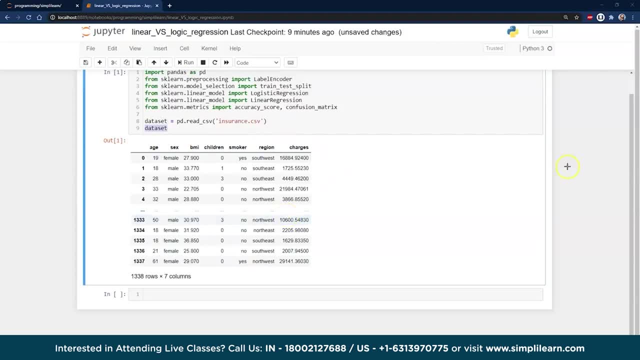 So there are 7 columns on here, And the column We are really interested in Is charges. I want to know what the charges are going to be. What can I expect? Not a very good arrow drawn What to expect Them to charge on there. 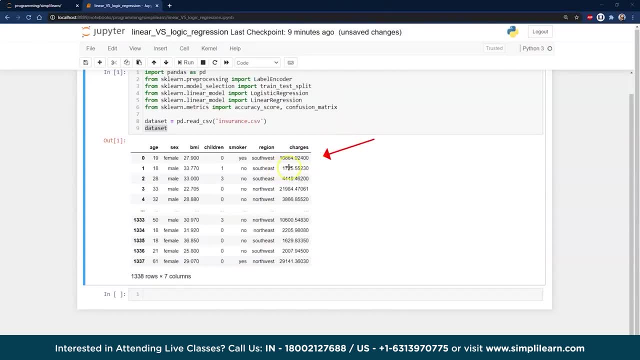 So is this going to be? Is this person going to cost me $16,884. Or is this person Only going to cost me $3,866.. How do we guess that, So that we can guess what the minimal? 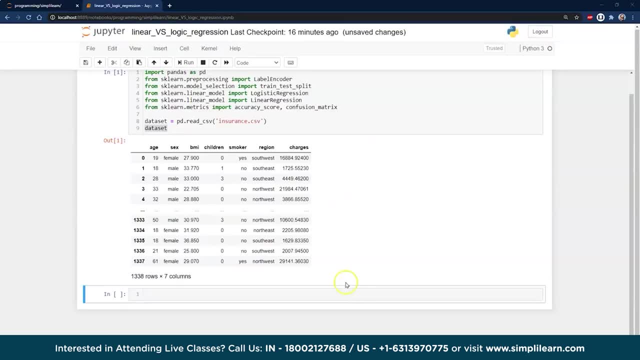 Charge is for their insurance. And then there is one other thing You really need to notice on this data, And I mentioned it before, But I am going to mention it again Because pre-processing data Is so much of the work in data science. 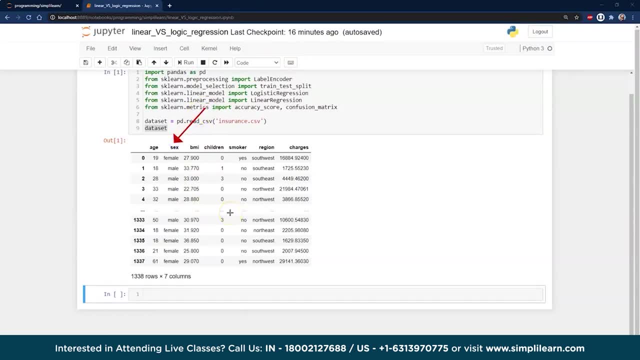 Sex. Well, how do you, How do you deal with female versus male? Are you a smoker, Yes or no? What does that mean? Region? How do you look at region? It is not a number. How do you draw a line? 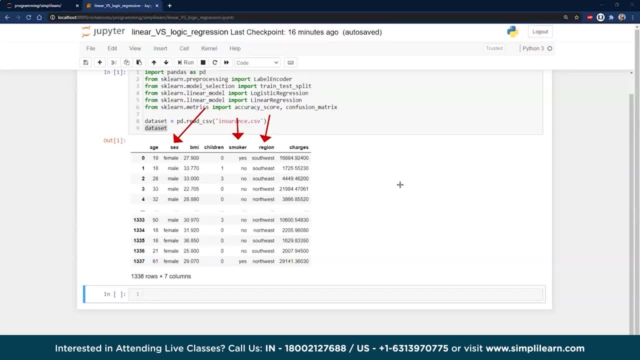 Between southwest and northwest. I guess you could do longitude and latitude, But the data doesn't come in like that. It comes in as true, false or whatever You know. it is either your southwest Or your northwest. So we need to do a little bit. 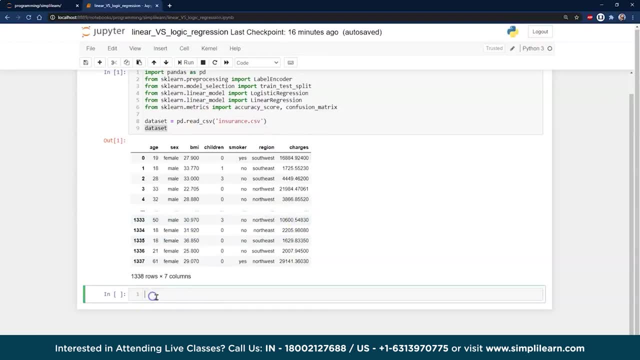 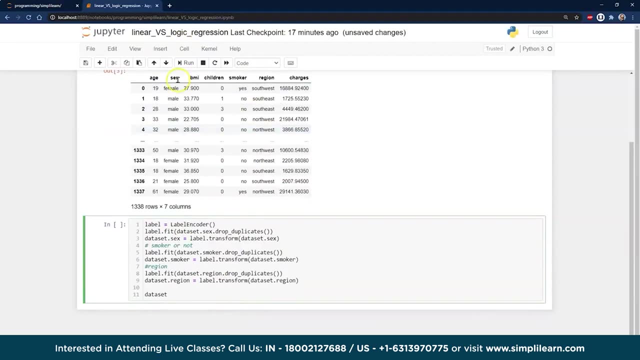 Of pre-processing of the data on here To make this work. Oops, there we go. Okay, so Let's take a look and see what we are doing With pre-processing. And again, this is really where you spend a lot of time. 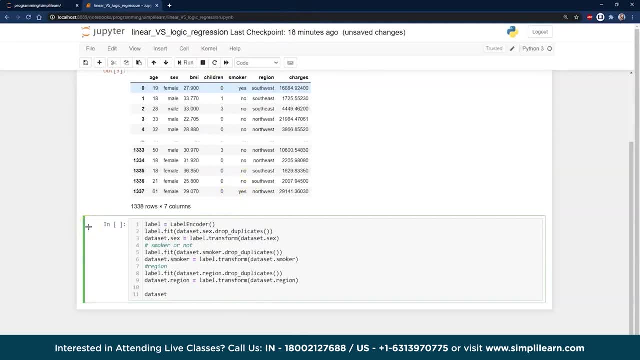 With data science, is trying to understand How and why, And so we are going to do- You will see right up here- Label, And then we are going to do a label encoder, One of the modules we brought in. So this is sklearns. 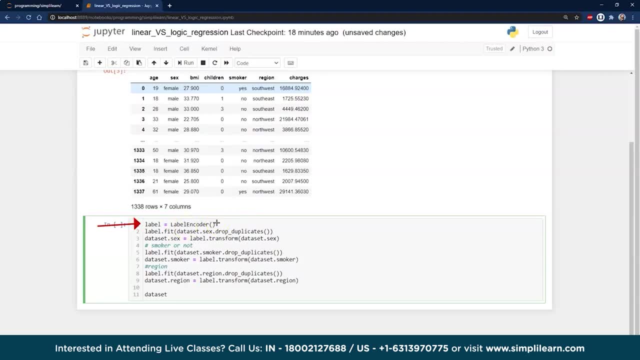 Label encoder. I like the fact that it is all pretty much Automated. But if you are doing a lot of work with label encoder, You should start to understand how that fits. And then we have Labelfit Right here. We are going to go ahead and do the data set. 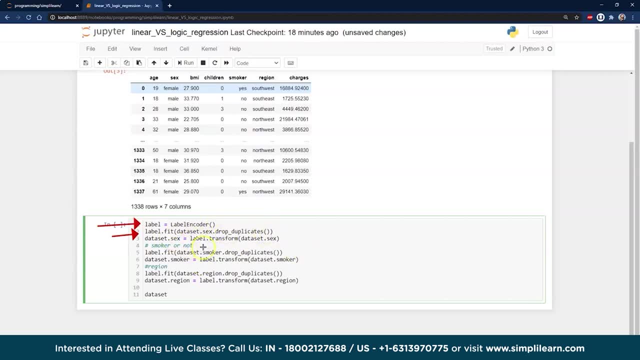 sexdrop duplicates And then for data set sex, We are going to do the label transform The data set sex, And so we are looking right here at Male or female, And so it usually just converts it to a 0 or 1.. 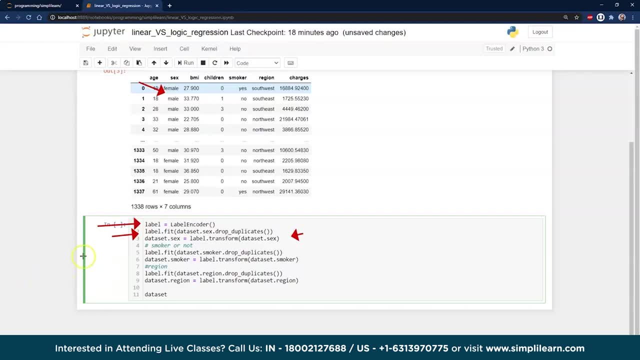 Because there is only two choices on here. Same thing with the smoker: It is 0 or 1.. So we are going to change the smoker- 0 or 1 on this. And then, Finally, we did region down here. Region does it a little bit different. 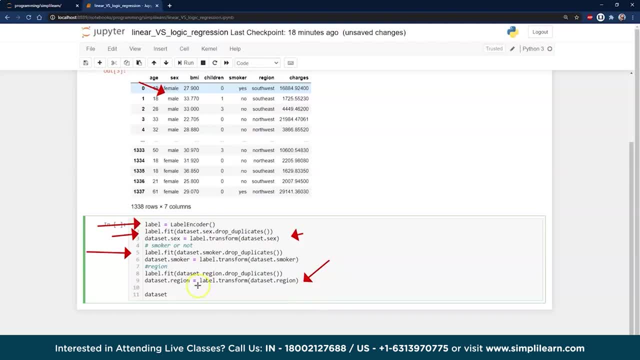 We will take a look at that. I think in this case It is probably going to do it, Because we did it on this label. transform With this particular set up. It gives each region a number Like 0,, 1,, 2,, 3.. 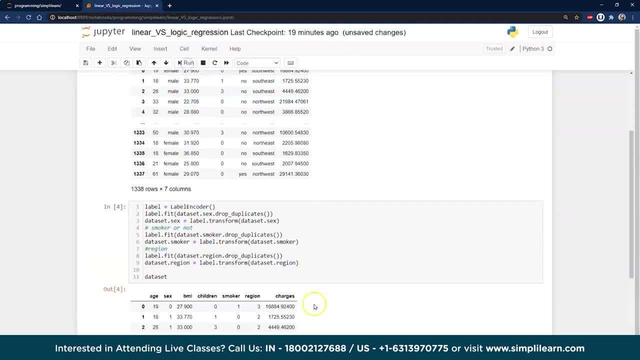 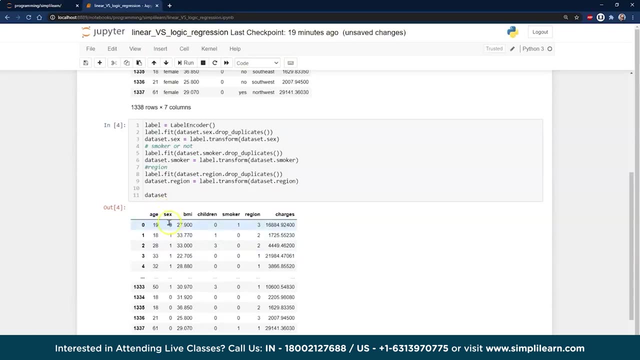 So let's go ahead and take a look and see what that looks like. Go ahead and run this And you can see that our new data set Has age. That is still a number. Sex is 0 or 1. So 0 is female. 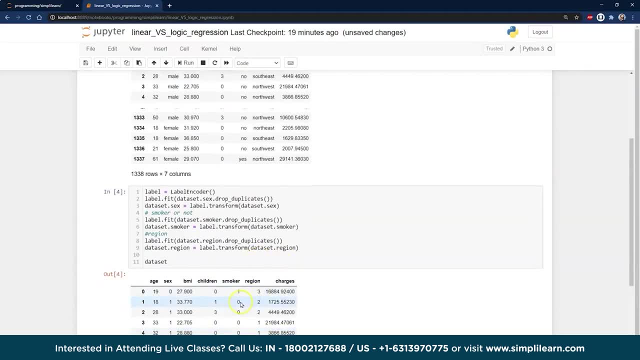 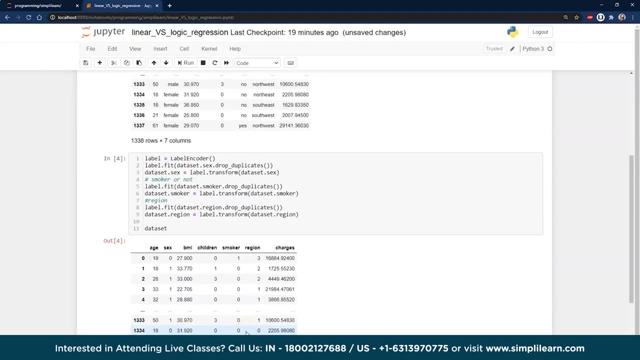 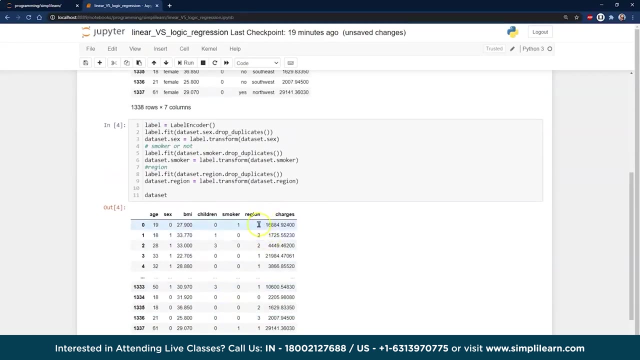 1 is male Number of children. We left that alone. Smoker 1 or 0. It says no or yes on there. We actually just do 1 for no, 0 or no, 1 for no. I am not sure how it organized them. 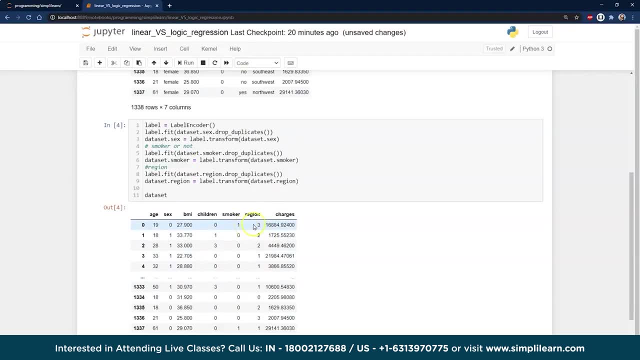 But it turns the smoker into 0 or 1.. Yes or no, And then region. It did this as 0,, 1,, 2,, 3.. When you are dealing with regions Or even word analysis, Instead of doing one column, 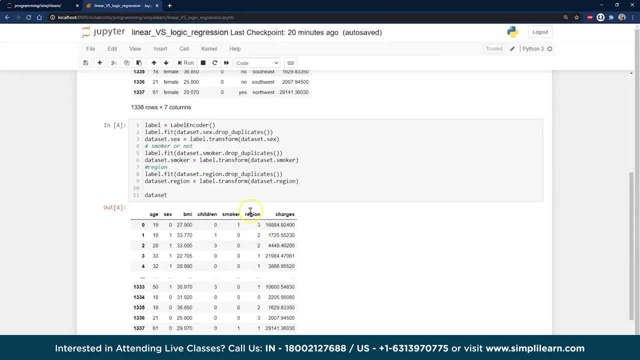 And labeling it 0,, 1,, 2,, 3.. A lot of times You increase your features, So you would have: region Northwest would be one column, Yes or no. Region southwest would be one column, Yes or no. 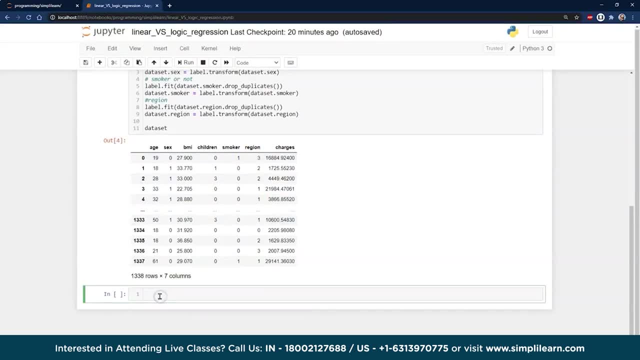 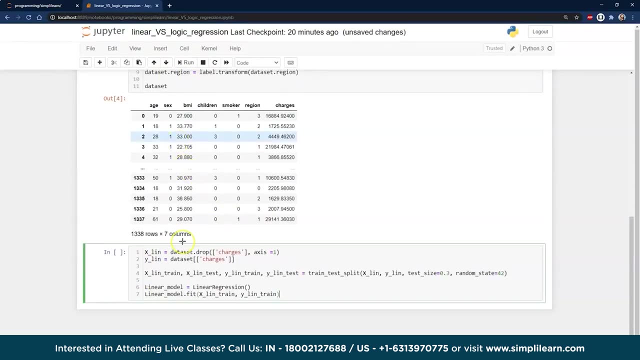 But for this particular set up, This will work just fine on here, Now that we spent all that time getting it set up. Here is the fun part. Here is the part where we are actually using Our set up on this And you will see right here. 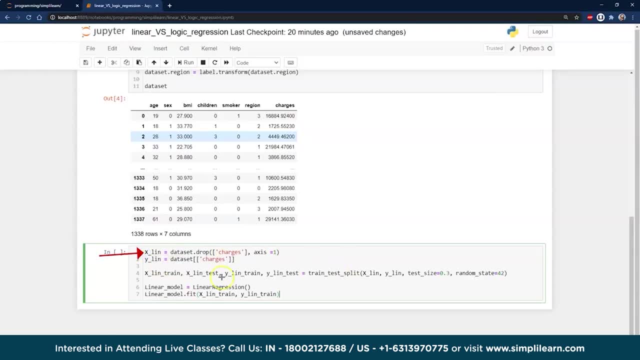 We have our Y linear regression Data set. drop the charges, Because that is what we want to predict. And so our X- I am sorry, Our X- linear data set. drop the charges, Because that is what we are going to predict. We are predicting charges right here. 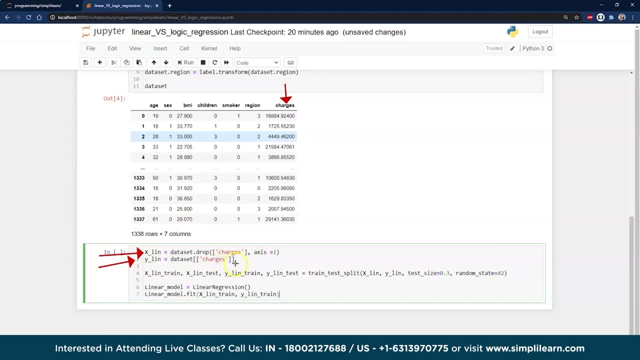 So we don't want that as our input for our features And our Y output is charges. That is what we want to guess. We want to guess what the charges are. And then what we talked about earlier Is we don't want to do all the data at once. 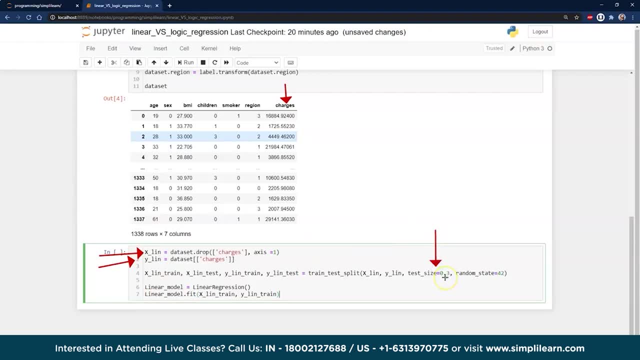 So we are going to take .3 Means 30%. We are going to take 30% of our data And it is going to be as the testing site. So here is our Y test And our X test down there, And so that part. 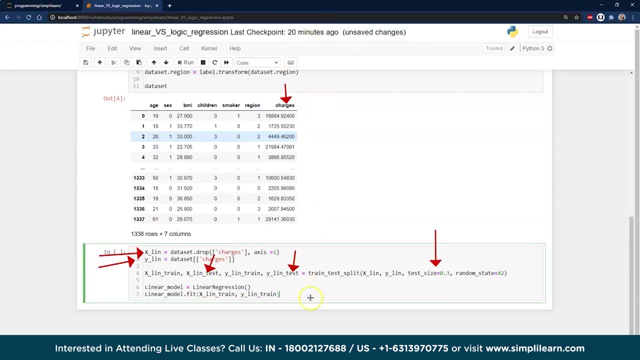 Our model will never see it Until we are ready to test To see how good it is. And then, of course, right here You will see our training set. This is what we are going to train it. We are going to train it on 70% of the data. 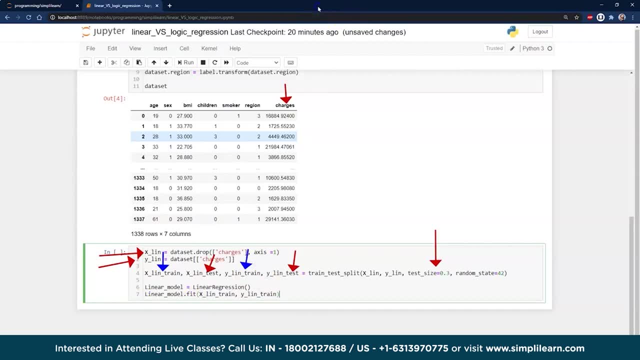 And then, finally, the big ones. This is where all the magic happens. This is where we are going to create Our magic, set up- And that is right here- Our linear model. We are going to set it equal to the linear regression model. 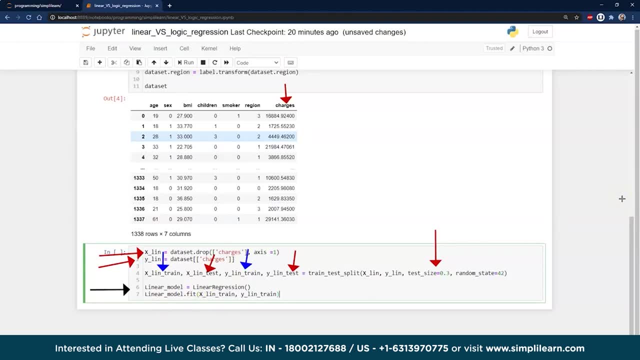 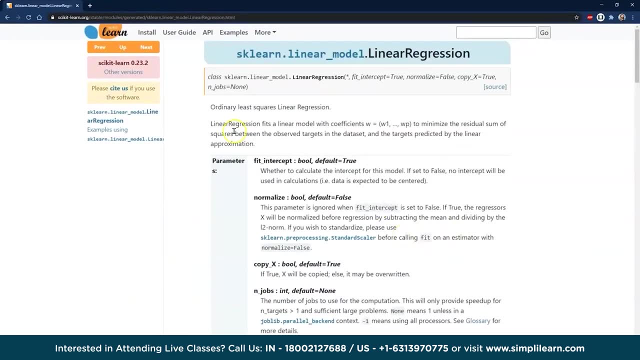 And then we are going to fit the data on here, And then at this point, I always like to pull up. If you are working with a new model, It is good to see where it comes from. This comes from the scikit learn. 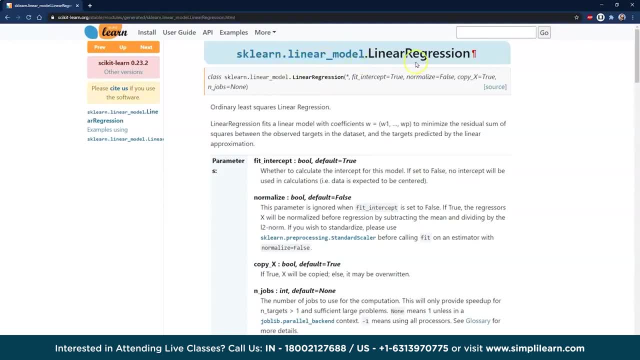 And this is the sklearn linear model, Linear regression that we imported earlier And you can see they have different parameters. The basic parameter works great If you are dealing with just numbers- I mentioned that earlier- with stock, High, lows, This model will do as good as any other model out there. 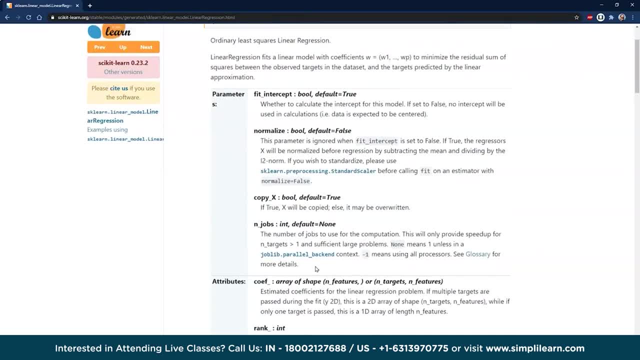 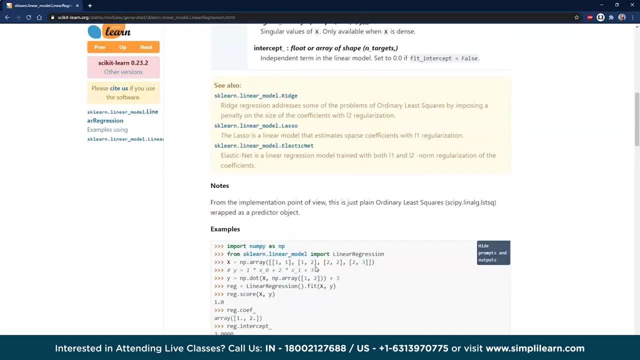 If you are doing just the very basic High lows And looking for a linear fit, A regression model fit. And one of the things When I am looking at this Is I look for methods And you will see, here is our fit. 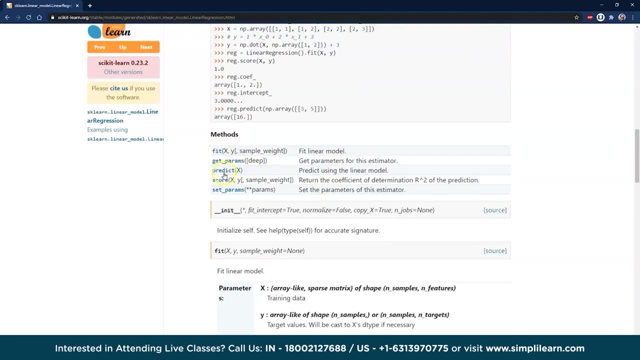 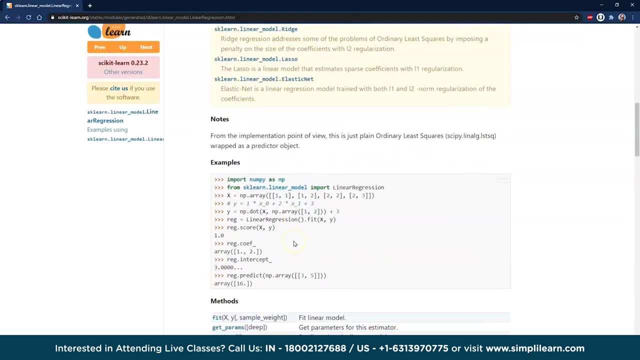 That we are using right now, And here is our predict, And we will actually do a little bit in the middle here As far as looking at some of the parameters Hidden behind it, The math that we talked about earlier, And so we go in this. 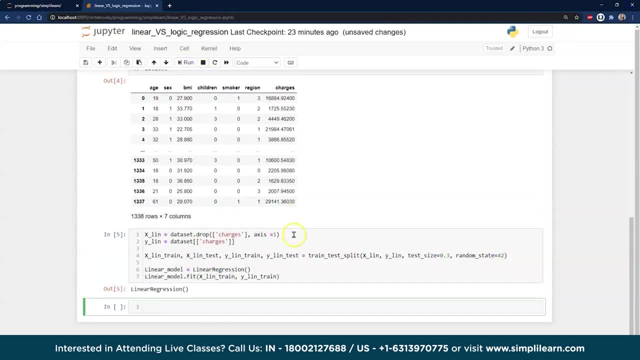 And we go ahead and run this. You will see it loads the linear regression model And it just has a nice output that says, Hey, I loaded the linear regression model. And then it loads the linear regression model And then the second part is: 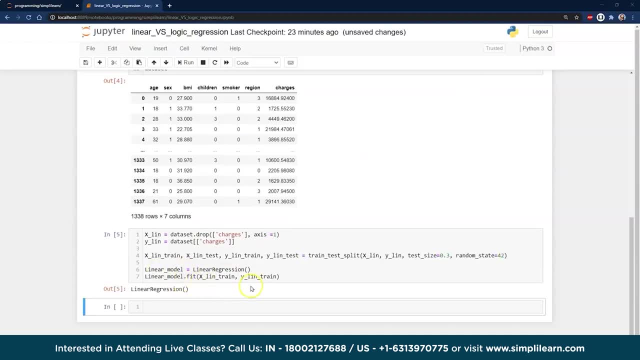 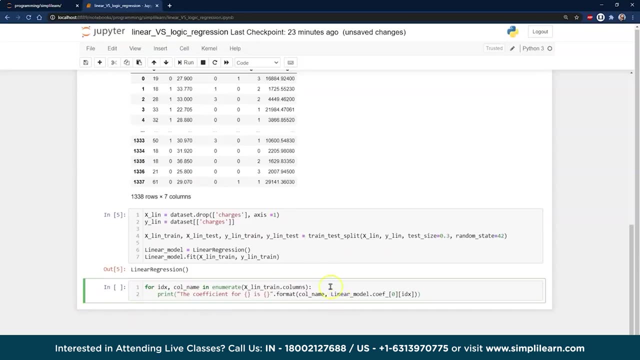 We did the fit, And so this model is now trained. Our linear model is now trained on the training data, And so one of the things we can look at Is the For IDX and column name And enumerate X linear trained columns. 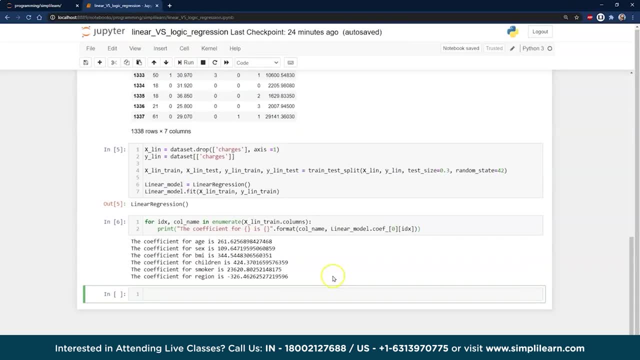 Kind of an interesting thing. This prints out the coefficients. So when you are looking at The back end of the data, You remember we had that formula: X1 plus BXX2.. Plus the intercept And so forth, These are the actual coefficients. 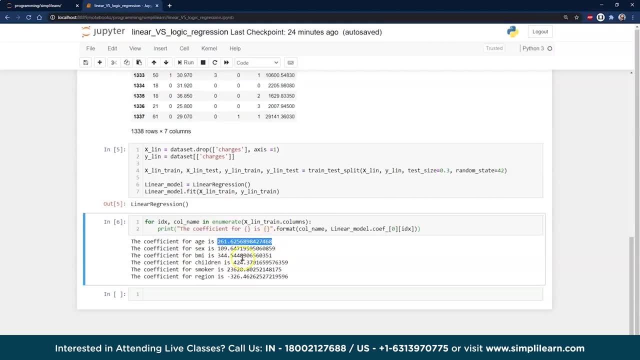 That are in here. This is what it is actually. multiplying these numbers by And you can see Like region gets a minus value. So when it adds it up, I guess region You can read a lot into these numbers. It gets very complicated. 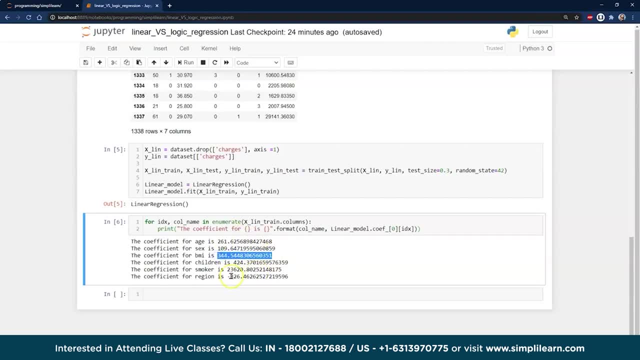 There is ways to mess with them. If you are doing a basic linear regression model, You might start looking in these And saying, hey, you know what Smoker. Look how smoker impacts the cost. It is just massive. So this is a flag that hey. 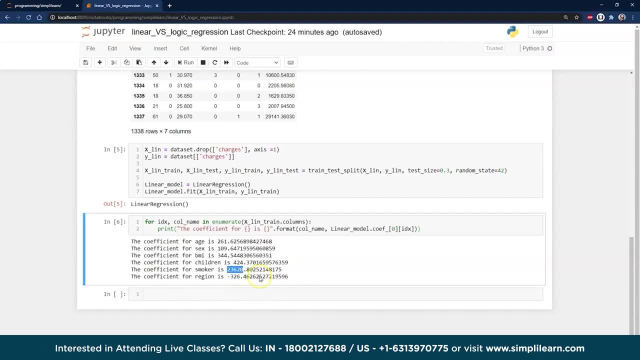 The value of the smoker Really affects this model. And then you can see here Where the body mass index- So somebody who is overweight Is probably less healthy And more likely to have cost money. And then of course, age is a factor. 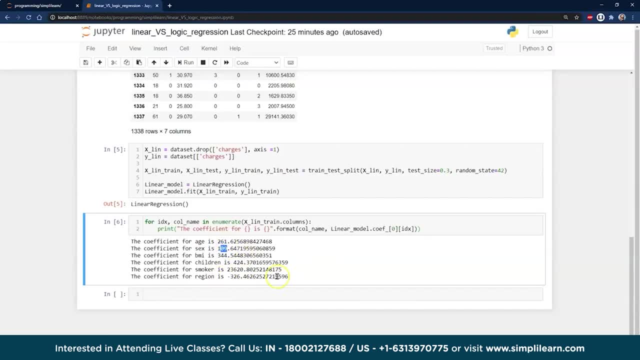 And then you can see down here: You have sex is then a factor also. It changes as you go in there. Negative number- It probably has its own meaning on there Again. it gets really complicated When you dig into the workings And how the linear model works on that. 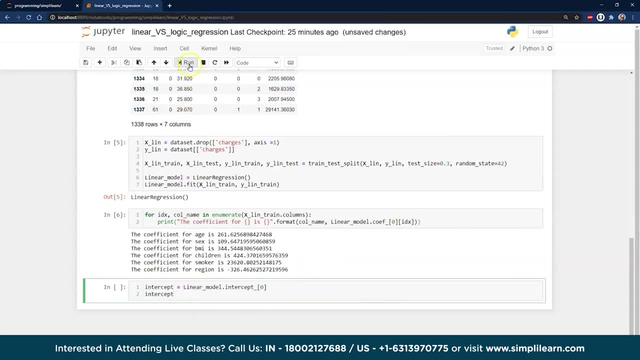 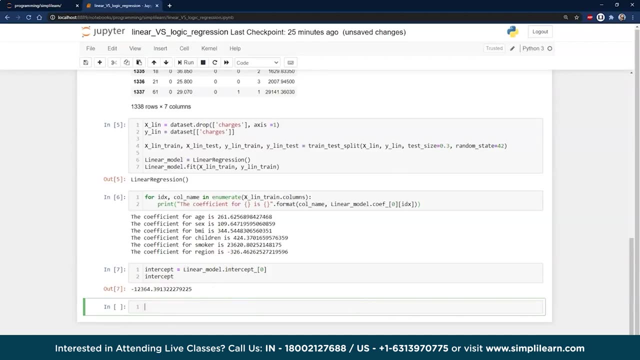 And so We can also look at the intercept. This is just kind of fun, So it starts at this negative number And then adds all these numbers to it. That is all that means. That is our intercept on there And that fits the data we have on that. 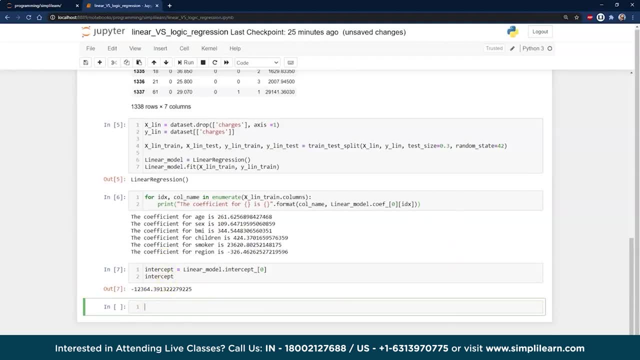 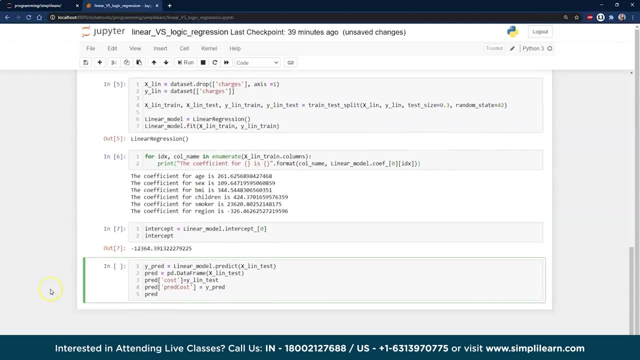 We can go back And Oops, give me just a second. There we go. We can go ahead and predict the unknown data And we can print that out. And if you are going to create a model To predict something, We will go ahead and predict it. 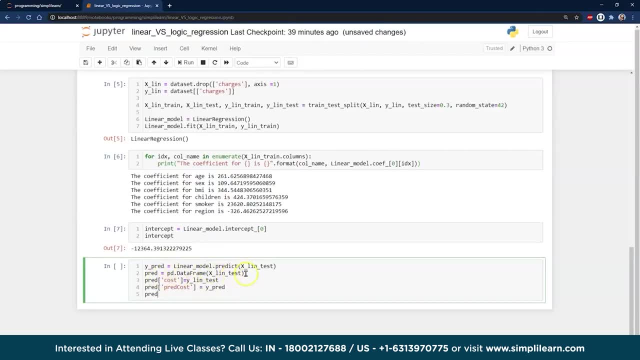 Here is our Y prediction value: Linear model predict. And then we will go ahead and create a new data frame, In this case from our X linear test group. We will go ahead and put the cost Back into this data frame And then we are going to put the predicted cost. 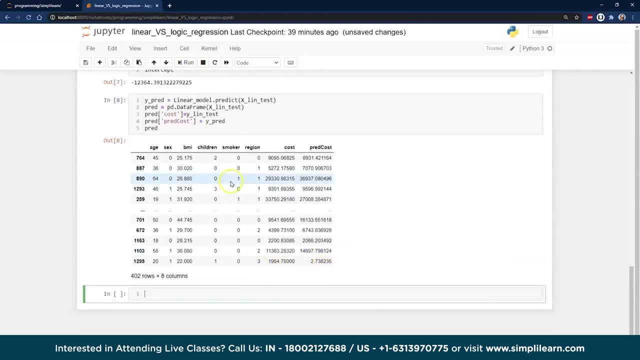 We are going to make that equal to our Y prediction And so when we pull this up, You can see here that we have The actual cost And what we predicted the cost is going to be. There is a lot of ways to measure the accuracy on there. 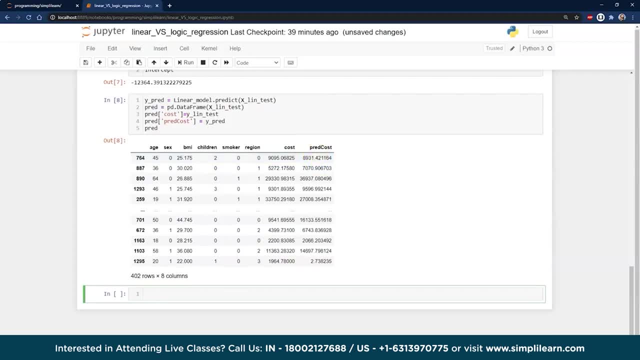 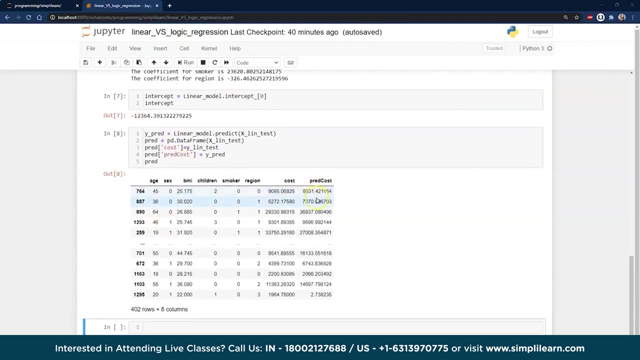 But we are going to go ahead and jump into Our mushroom data And so In this, You can see here, We have run our basic model, We have built our coefficients. You can see the intercept, You can see how we are generating a number here. 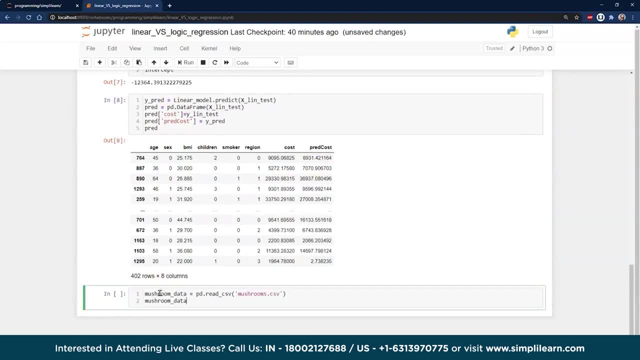 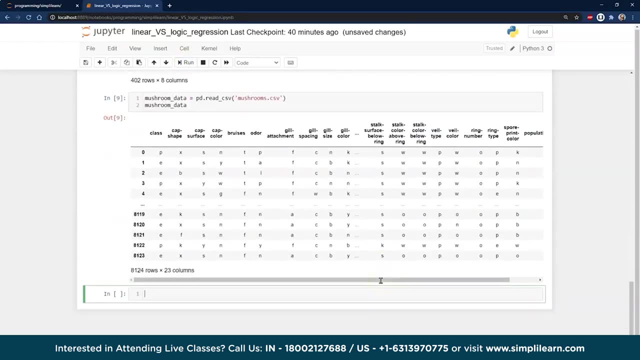 Now with mushrooms, We want a yes or no, We want to know whether we can eat them or not, And so here is our mushroom file. We are going to go ahead and run this, Take a look at the data And, again, you can ask for a copy of this file. 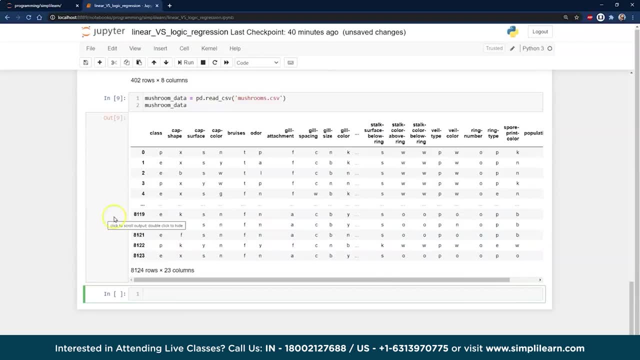 Send a note over to simplylearncom And you can see here That we have a class: The cap shape, Cap surface and so forth. So there is a lot of features, Different columns in here Going across, And when you look at this, 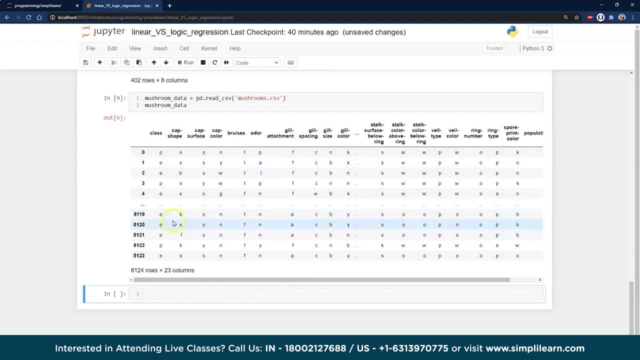 I am not even sure what these particular Like PEE, PE. I don't even know what the class is on this. I am going to guess by the notes That the class is Poisonous or edible. So if you remember before, 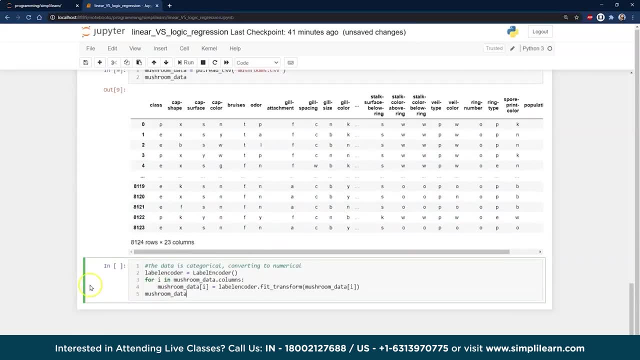 We had to do a little pre-coding On our data. Same thing with here. We have our cap shape, B or X or K. We have cap color. These really aren't numbers, So it is really hard to do anything. 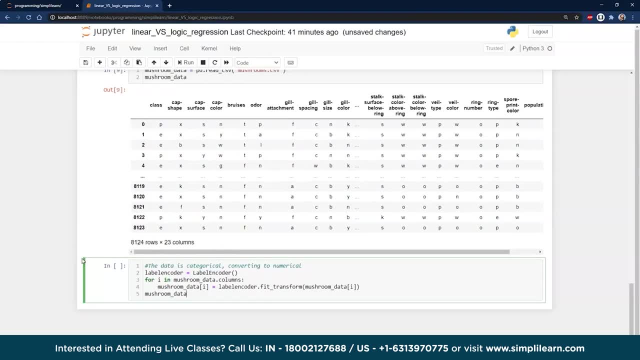 With just a single number, So we need to go ahead and turn those into a label encoder, Which, again, There is a lot of different encoders. With this particular label encoder It is just switching it to 0,, 1,, 2,, 3.. 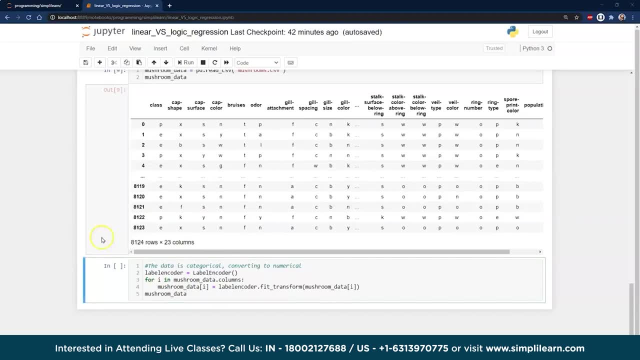 And giving it an integer value. In fact, If you look at all the columns, All of our columns are labels And so we are just going to Go ahead and loop through all the columns And the data And we are going to transform it into. 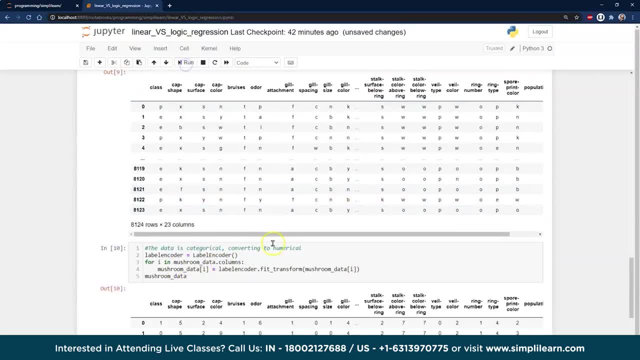 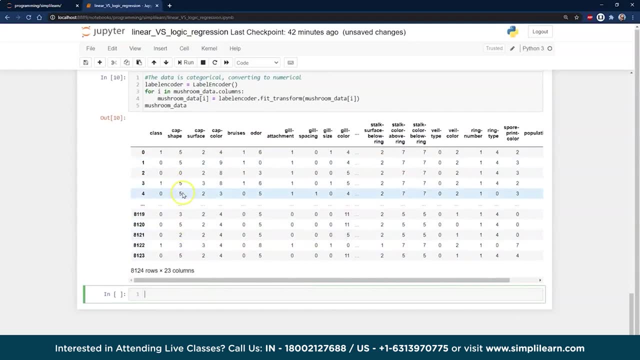 A label encoder, And so when we run this, You can see how this gets shifted from X B, X, X, K To 0,, 1,, 2,, 3,, 4,, 5. Or whatever it is. 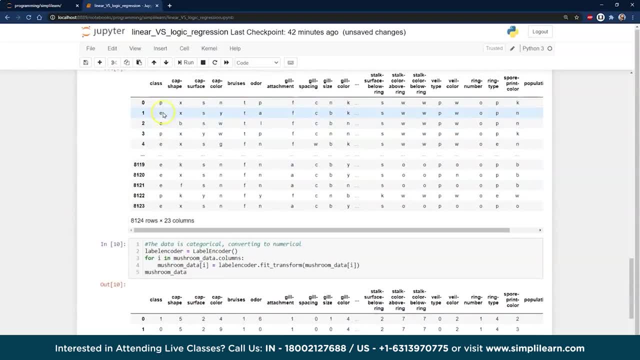 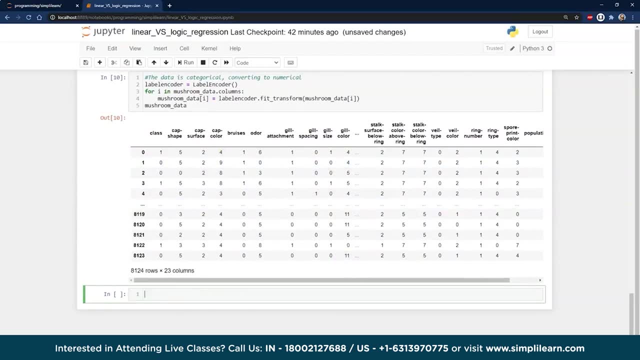 Class is 0, 1.. 1 being poisonous, 0 looks like it is edible, And so forth on here. So we are just encoding it. If you were doing this project On the results, You might encode it differently. 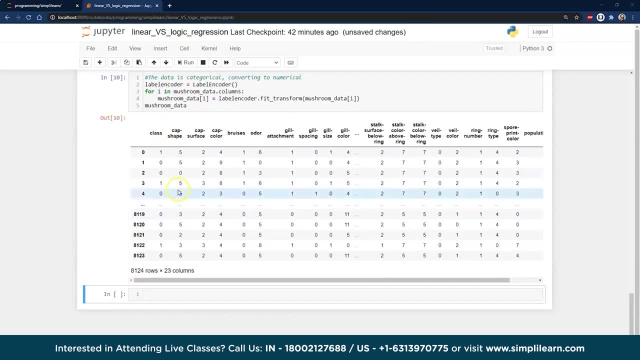 Like I mentioned earlier, You might actually increase the number of features, As opposed to laboring at 0,, 1,, 2,, 3,, 4, 5.. In this particular example, It is not going to make that big of a difference. 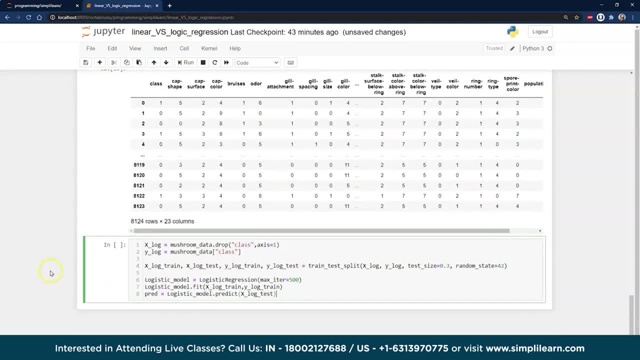 How we encode it. And then, of course, We are looking for the class Whether it is poisonous Or edible. So we are going to drop the class In our X logistics model And we are going to create our Y logistics model. 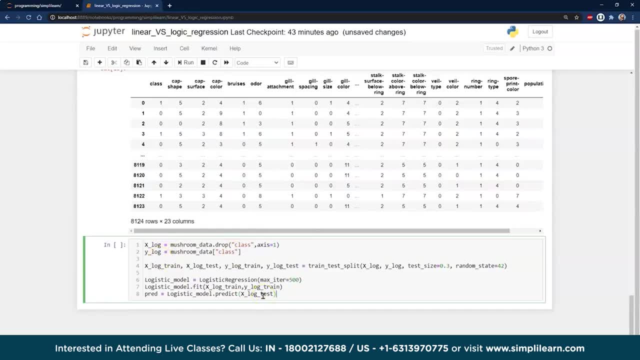 So here is our XY And, just like we did before, We are going to go ahead and split it, Using 30% for test, 70% to program the model on here. And that is right. here There we go. There is our train and test. 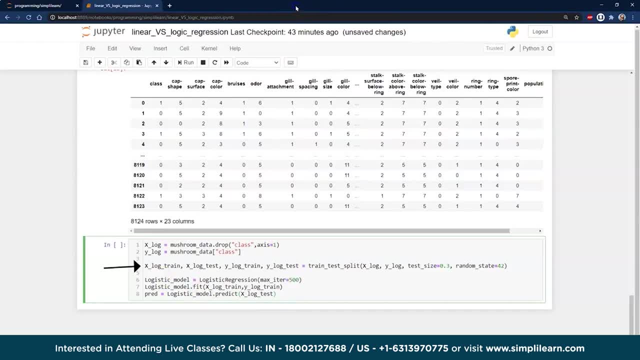 And then you will see here On this next setup. This is where we create our model, Which happens right here. We go ahead and Create a logistics model. I have up the max iterations If you don't Change this For this particular problem. 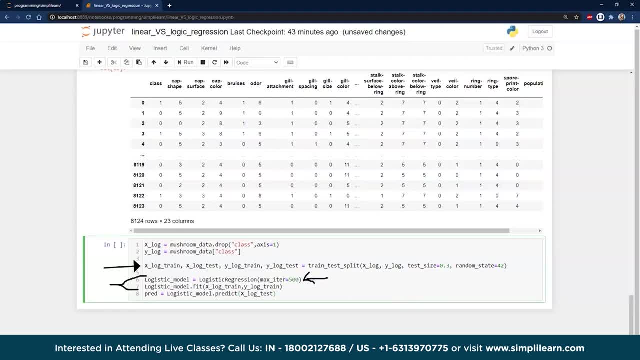 You will get a warning that says This has not converged. Because that is what it does. It goes through the math And it goes- hey, can we minimize the error? And it keeps finding a lower and lower error And it still is changing that number. 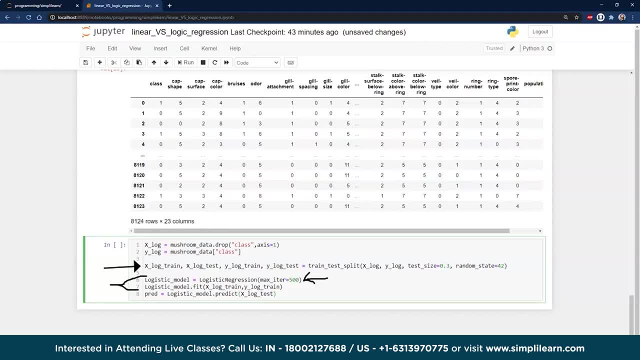 So that means it hasn't converged yet, And that is the lowest amount of error it can, And the default is 100.. There is a lot of settings in here, So when we go in here to Let me pull that up from the sklearn- 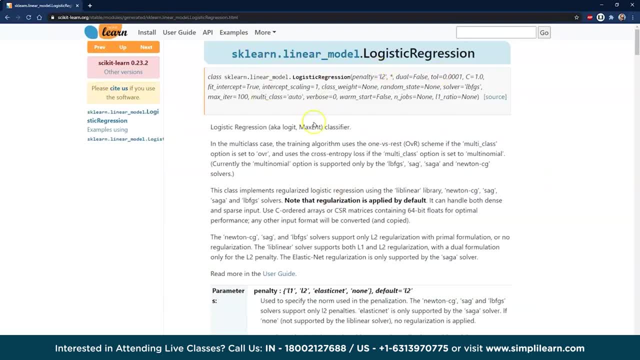 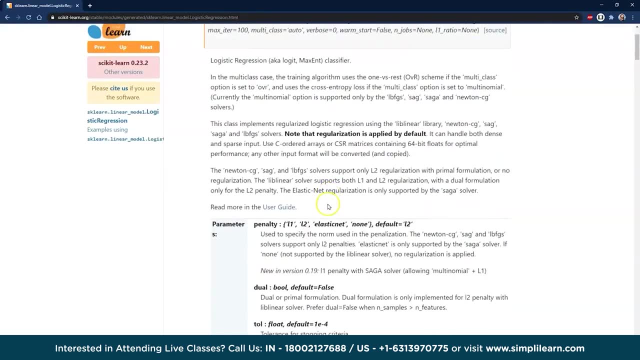 So we pull that up from the sklearn model. You can see here We have our logistics. It has our different settings on here That you can mess with. Most of these work pretty solid on this particular setup, So you don't usually mess a lot. 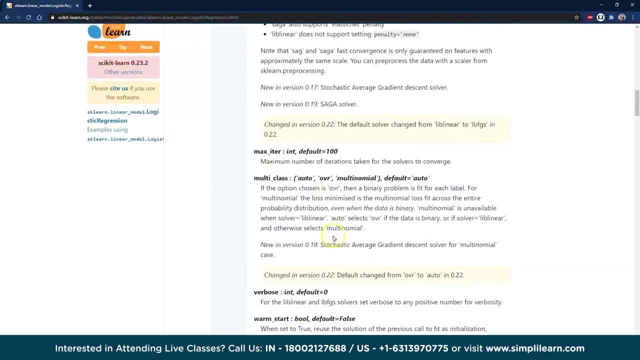 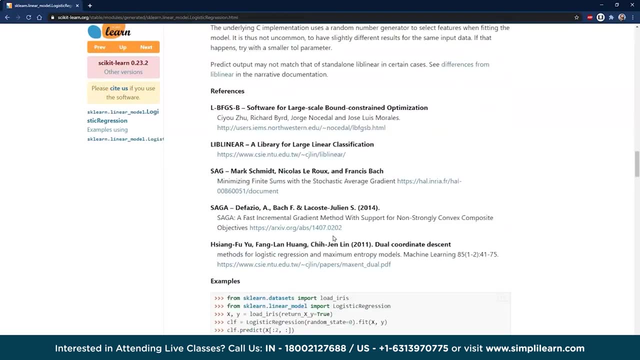 Usually I find myself adjusting the iteration And I will get that warning And then increase the iteration on there And, just like the other model, Just like you did with the other model, We can scroll down here and look for our methods And you can see there is a lot of methods. 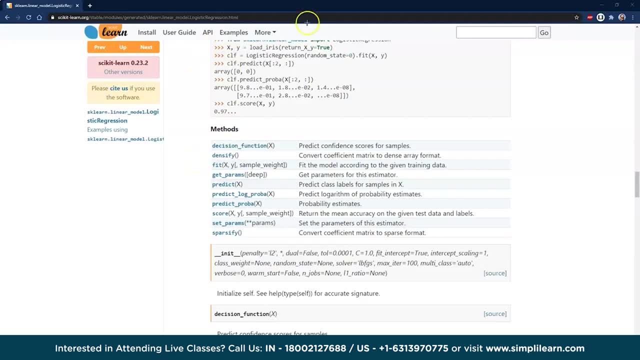 Available on here, And certainly there is a lot of different things You can do with it, But the most basic thing we do Is we fit our model, Make sure it is set right And then we actually predict something with it. So those are the two main things. 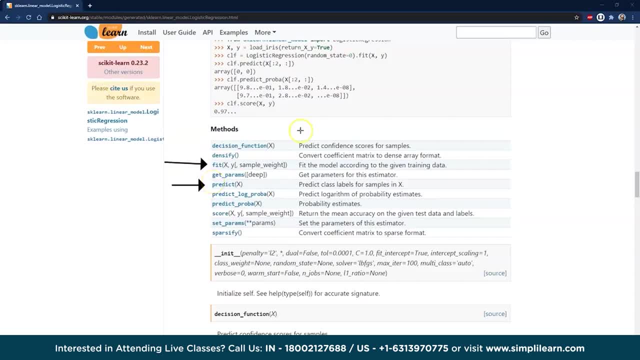 We are going to be looking at on this model Is fitting and predicting. There is a lot of cool things you can do, But for the most part These are the two which I use When I am going into one of these models. 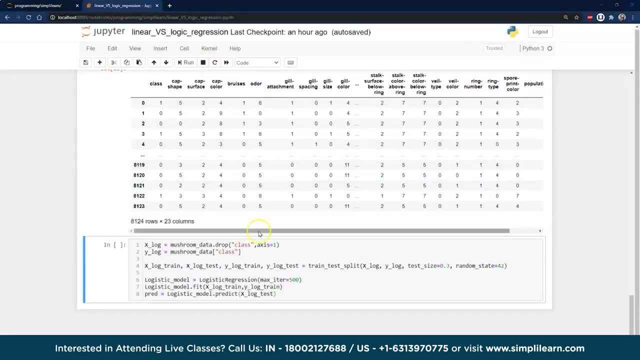 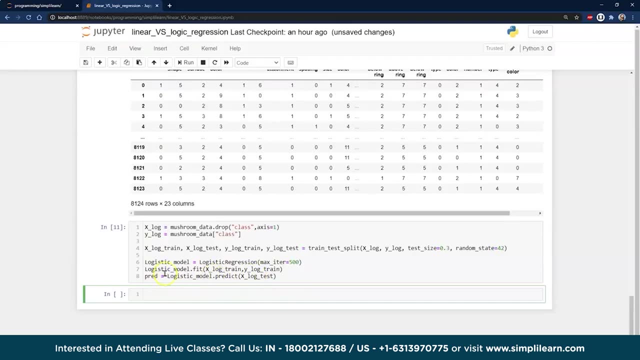 And setting them up. So let's go ahead and close out of our sklearn setup on there And we will go ahead and run this And you can see here It has now loaded this up there. We now have a logistic model And we have gone ahead. 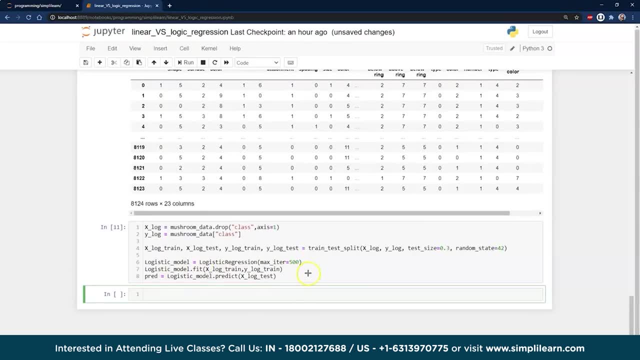 And done a predict here also, Just like I was showing you earlier. So here is where we are actually predicting the data. So we have done our first two lines of code. As we create the model, We fit the model to our training data. 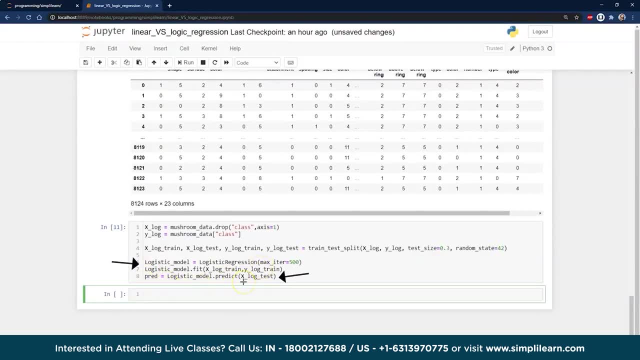 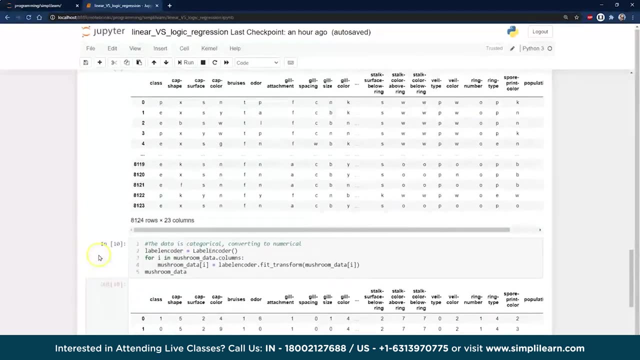 And then we go ahead And predict for our test data. Now, in the previous model, We didn't dive into the test score. I think I just showed you a graph And we can go in there, And there is a lot of tools to do this. 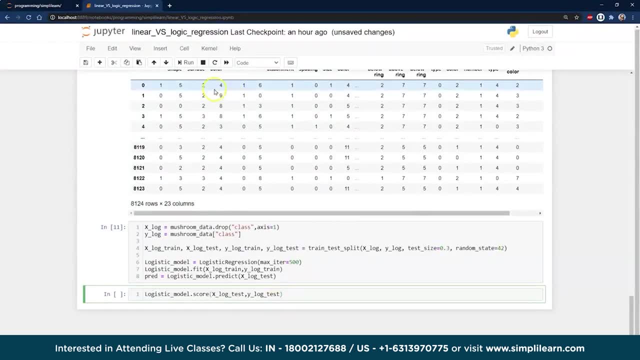 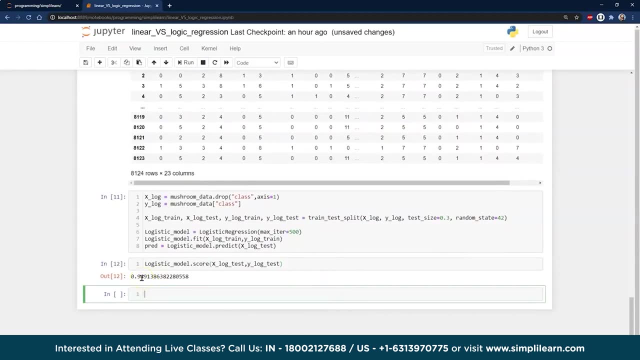 We are going to look at the model score On this one. Let me just go ahead and run the model score. And it says that it is pretty accurate. We are getting a roughly 95% accuracy. Wow, that is good, 95% accuracy. 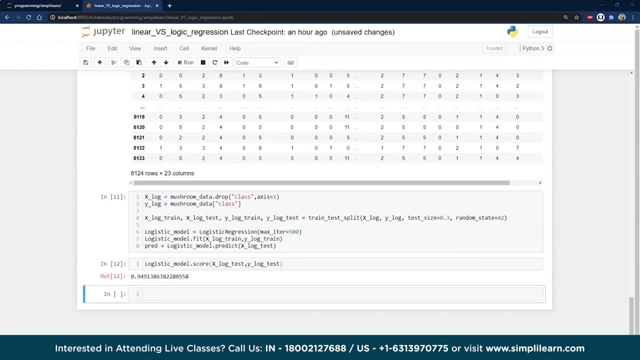 95% accuracy Might be good for a lot of things, But when you look at something As far as whether you are going to pick a mushroom On the side of the trail And eat it, We might want to look at the confusion matrix. 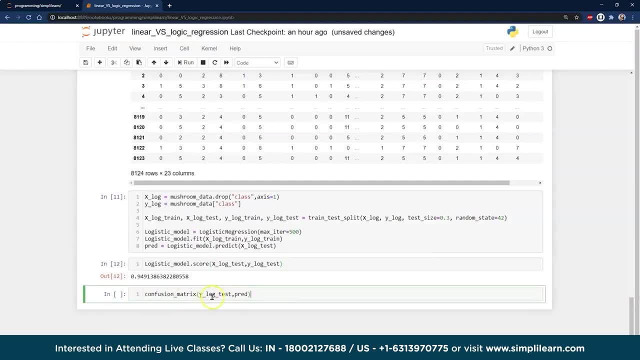 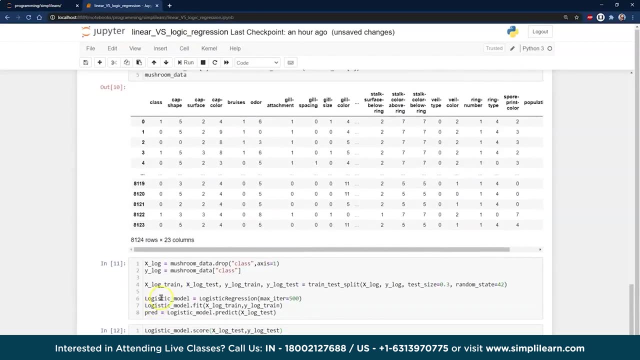 And for that We are going to put in our Y logistic test The actual values of edible and unedible And we are going to put in our prediction value And if you remember on here Let's see. I believe it is poisonous, was one. 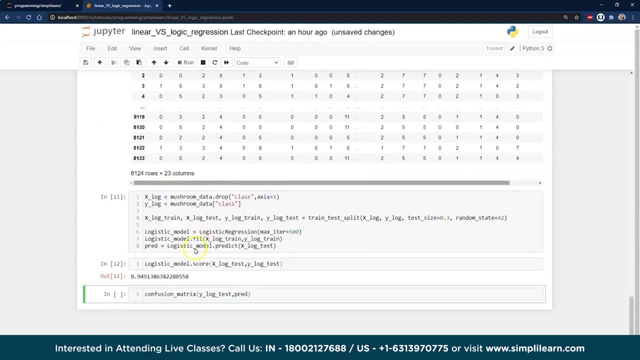 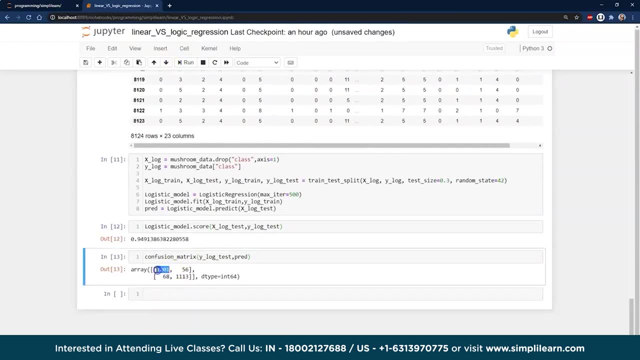 Poisonous was. two Zero is edible, So let's go ahead and run that Zero. one Zero is good. So here is a confusion matrix, And this is If you are not familiar with these. We have true, true, true, false. True, false, false, false. So it says: Out of the edible mushrooms, We correctly labeled 1201 mushrooms edible That were edible And we correctly measured 1113. Poisonous mushrooms As poisonous. But here is the kicker. I labeled 56 edible mushrooms As being Poisonous. Well, that is not too big of a deal- We just don't eat them. But I measured 68 mushrooms As being edible that were poisonous, So probably not the best choice. 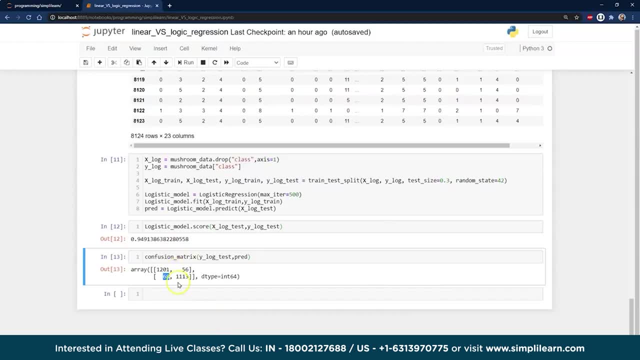 To use this model to predict Whether you are going to eat a mushroom or not, And you would want to dig a little deeper Before you start Picking mushrooms off the side of the trail. So a little warning there When you are looking at any of these data models. 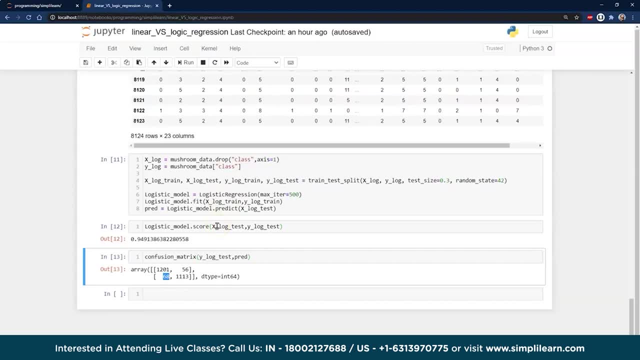 Looking at the error And how that error fits in with what domain you are in, Domain in this case being edible mushrooms. Be a little careful, Make sure that you are looking at them correctly. So we have looked at Edible or not edible. 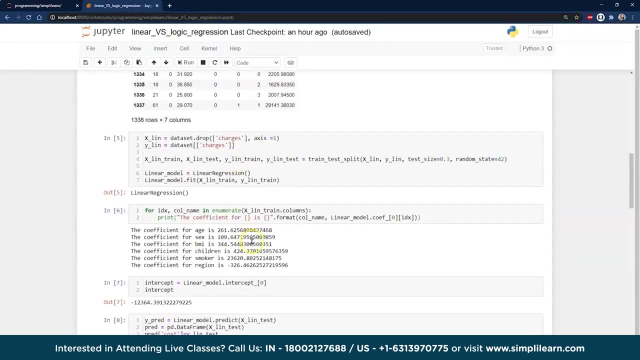 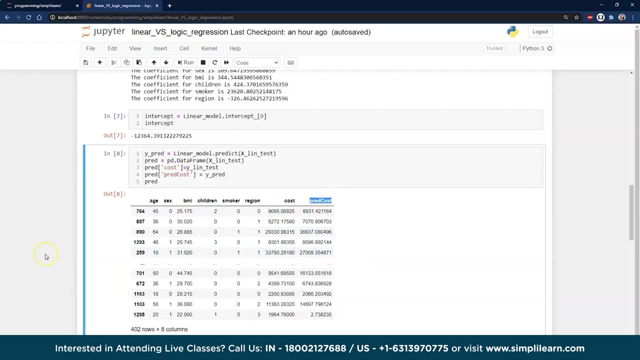 We have looked at Regression model as far as The end values- What is going to be the cost And what our predicted cost is- So we can start figuring out How much to charge these people for their insurance. And so these really are the fundamentals. 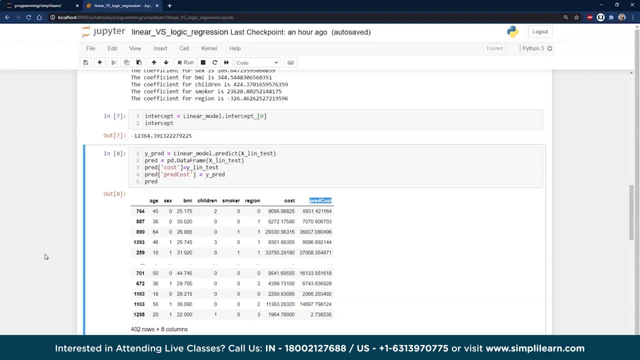 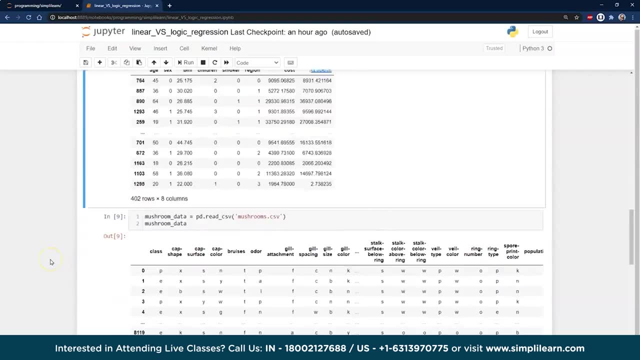 Of data science When you pull them together. When I say data science, I am talking about your machine learning code, And hopefully You got a little bit out of here. Again, you can contact our simply learn team And get a copy of these files. 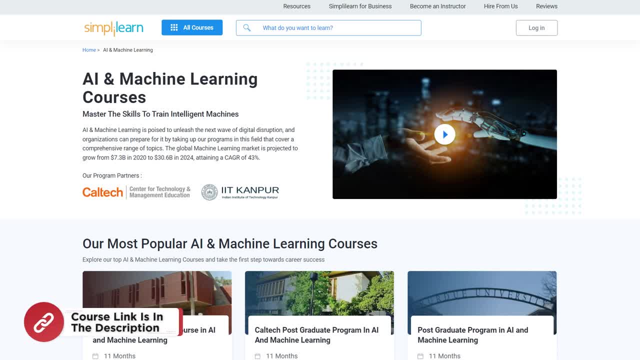 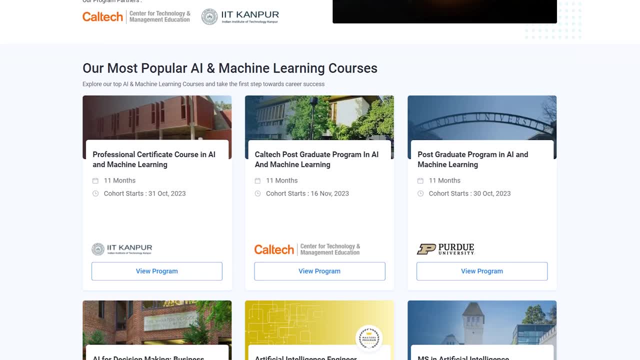 Or get more information on this. If you want to become an AI expert, You will need to look at The wide range of AI ML courses By simply learn In collaboration with top universities Across the globe, By enrolling in any of these certification programs. 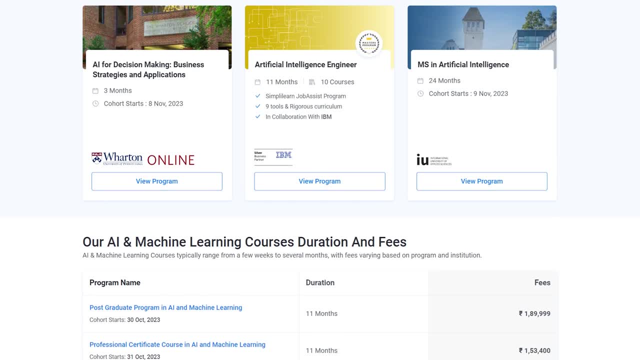 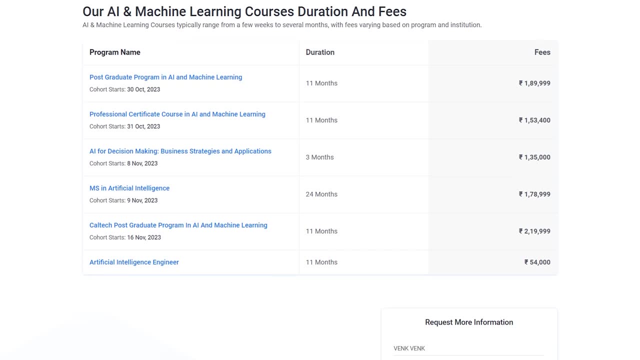 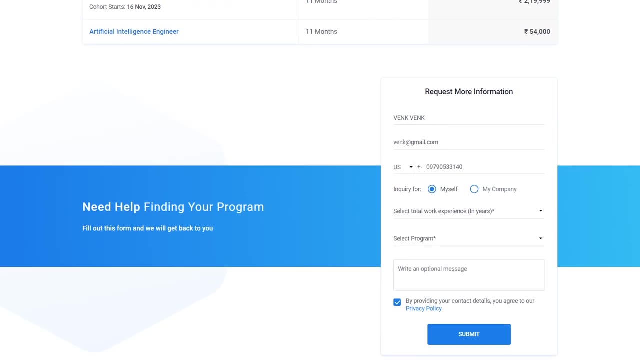 You will gain expertise in skills like Generative AI, Prompt engineering, Chat, GPT, Explainable AI, Machine learning algorithms, Supervised and unsupervised learning, Model training and optimization, If you have an experience in the tools like Chat, GPT, DALI, Python. 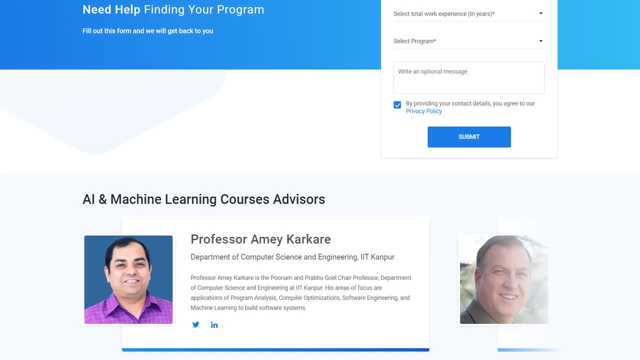 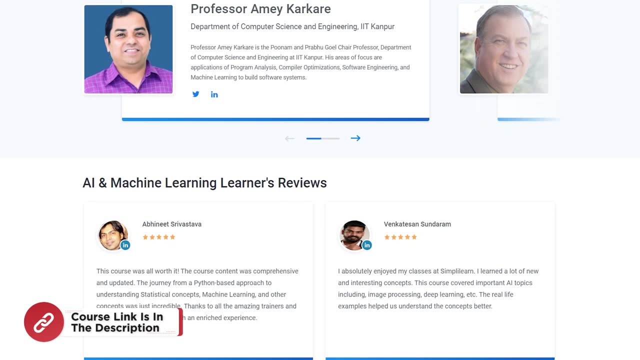 OpenCV and TensorFlow, You will catch the eyes of top recruiters. So what are you waiting for? Hurry up and enroll now. An year of experience is preferred To enroll in these courses. Find the course link in the description box. A confusion matrix. 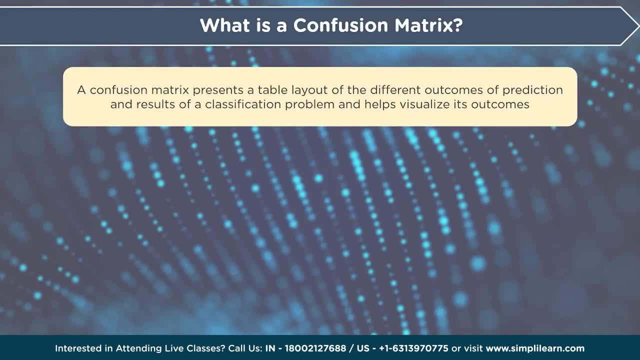 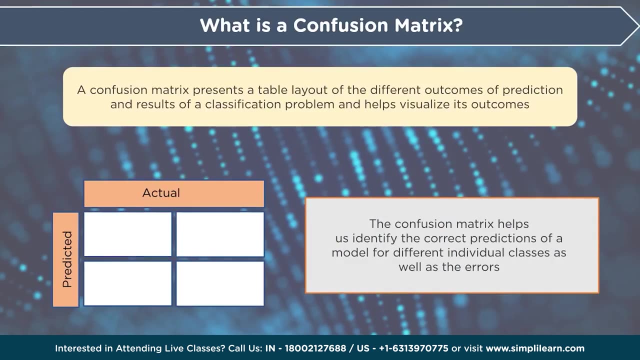 Represents a table layout Of the different outcomes of prediction And results of a classification problem And helps visualize its outcomes. And so you see, We have our simple chart, Predicted and actual. The confusion matrix Helps us identify the correct predictions. 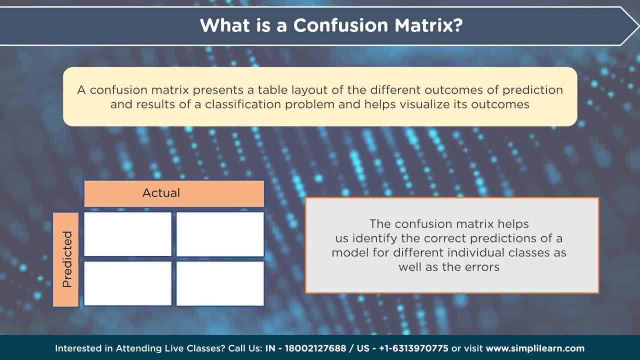 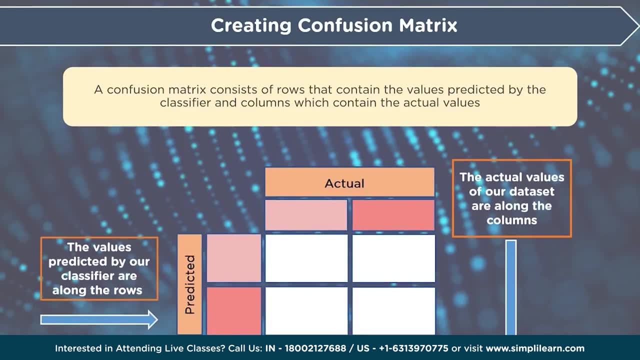 Of a model for different individual classes, As well as the errors. So you will see here That the values predicted by our classifier Are along the rows. This is what we are going to guess. it is Our model is guessing what this is. 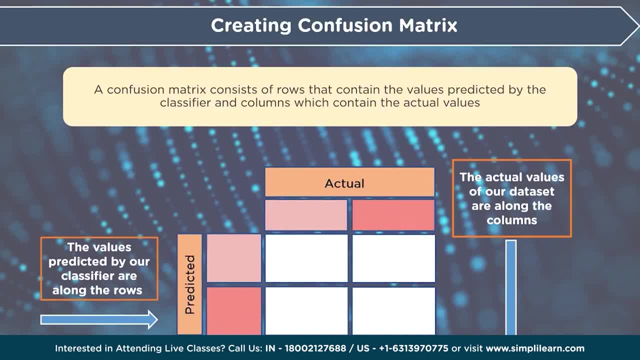 Based on its training. So we have already trained the model To guess whether it is spam or not spam Or whatever it is you are working on. So the values of our data set Are along the columns. So this is the actual value it is supposed to be. 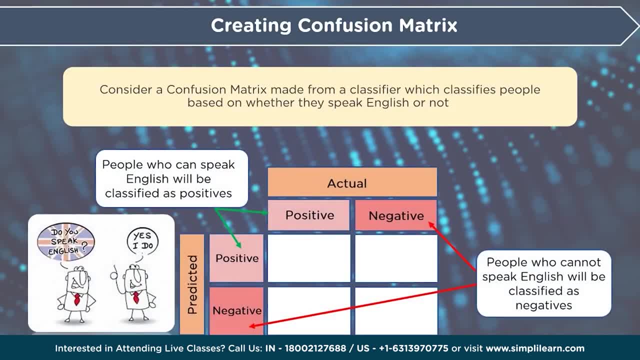 People who can speak English Will be classified as positives Because they have a number zero or one. Do you speak English, Yes or no? And you could extend this That they might have. Do you speak French? Do you speak whatever languages? 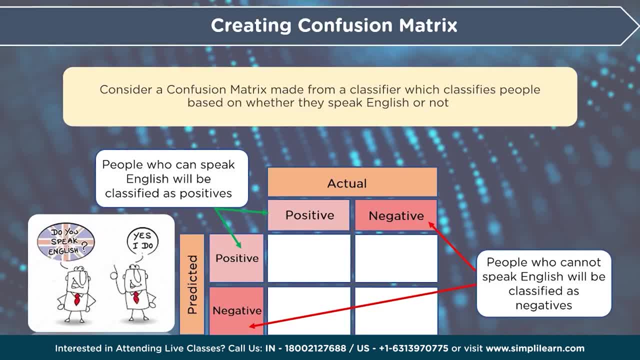 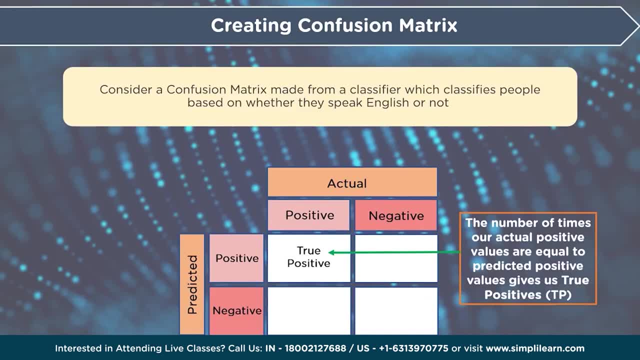 And so you might have a whole lot of classifiers That you would look at. each one of these People who cannot speak English Will be classified as negatives. The number of times our actual positive values Are equal to predicted positive values Gives us true positive. 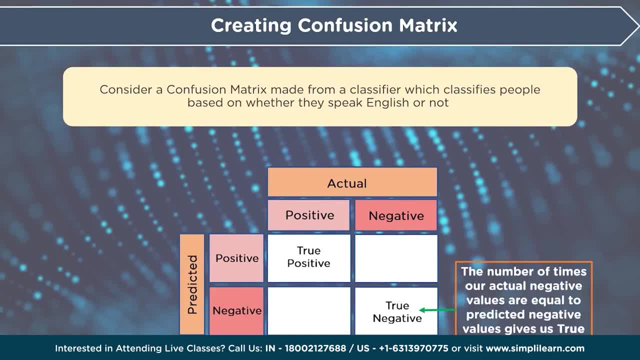 TP. The number of times our actual negative values Are equal to predictive negative values Gives us true negative TN. The number of times our model wrongly predicts Negative values as positives Gives us a false positive FP, And you will see. 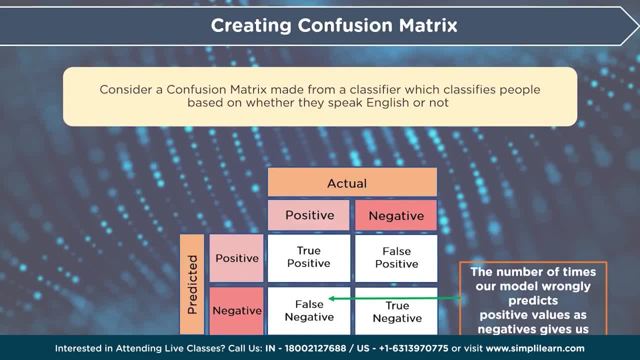 When you are working with these a lot, Memorizing that it is false positive. You can figure out what that is And pretty soon you are just looking at the FP Or the TP, Depending on what you are working on And the number of times our model wrongly predicts. 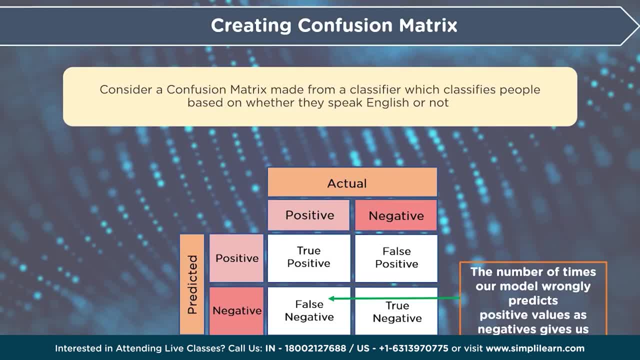 Positive values as negatives Gives us a false, negative FP. Now I am going to do a quick step out here. Let's say you are working in the medical And we are talking about cancer. Do you really want A bunch of false negatives? 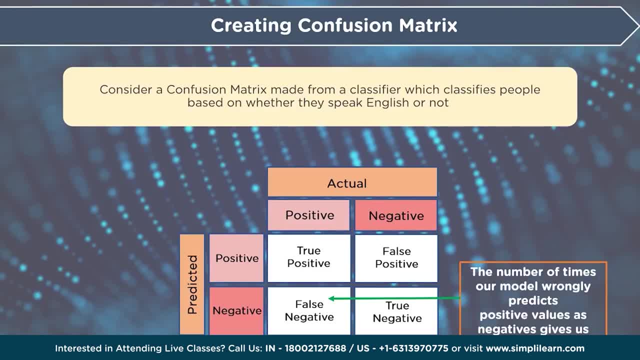 You want zero under false negative. So when you are working, When we look at this confusion matrix, If you have 5% false positives And 5% false negatives, It would be much better to even have 20% false positives. 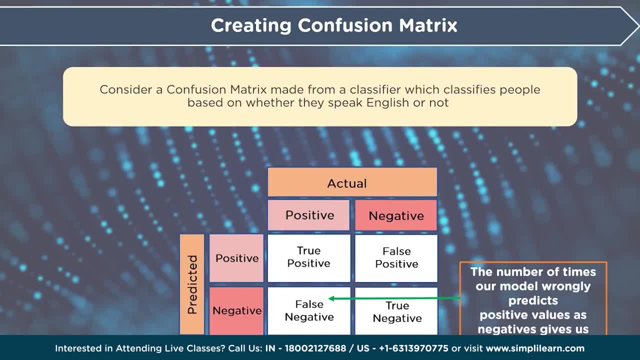 Because they go in and test it And zero false negatives. The same might be true If you are working on, Say, a car driving. Is this a safe place for the car to go? Well, you really don't want Any false positives. 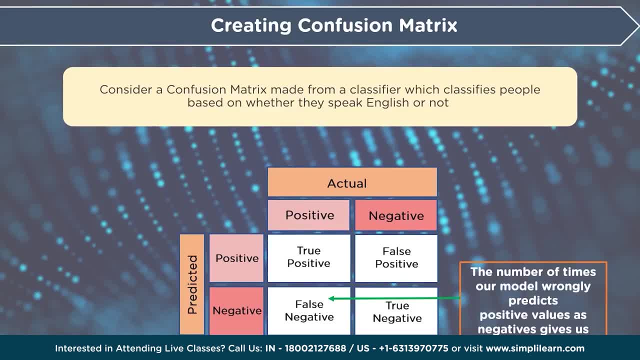 Yes, this is safe Right over the cliff In the project Or whatever it is you are working on. This chart suddenly has huge value. We were talking about spam email. How many important emails, Say, from your banking overdraft charge coming in? 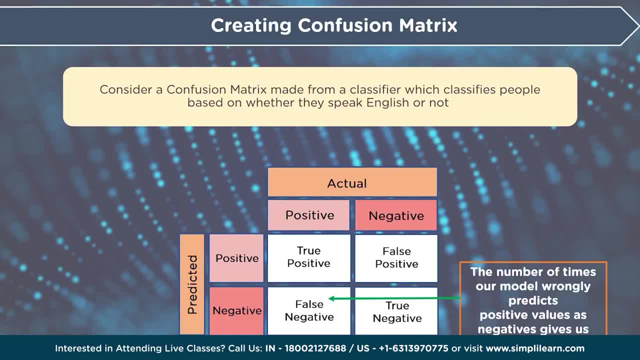 That you want to be A false negative. You don't want it to go in the spam folder. Likewise, you want to Get as much of the spam out of there, But you don't want to miss anything really important. Confusion matrix metrics. 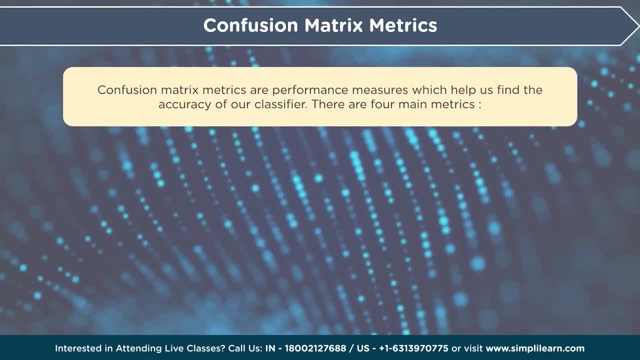 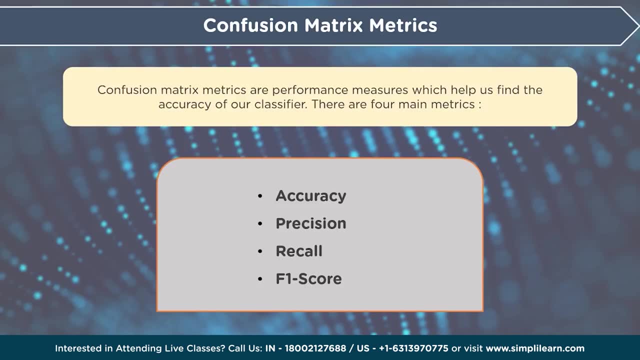 Are performance measures Which help us find The accuracy of our classifier. There are four main metrics: Accuracy, Precision, Recall And F1 score. The F1 score is the one I usually hear the most And accuracy is usually what you put on your chart. 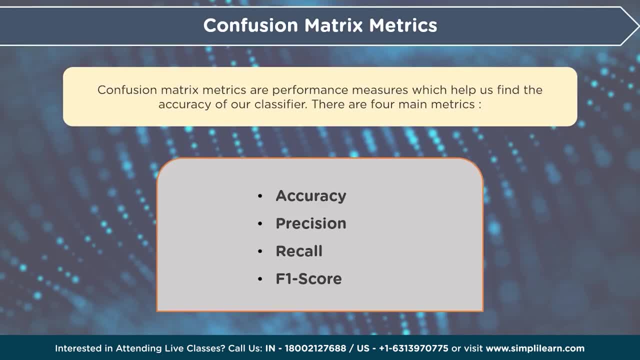 When you are standing in front of the shareholders. How accurate is it? People understand accuracy. F1 score is a little bit more on the math side And so you have to be a little careful When you are quoting F1 scores When you are sitting there with all the shareholders. 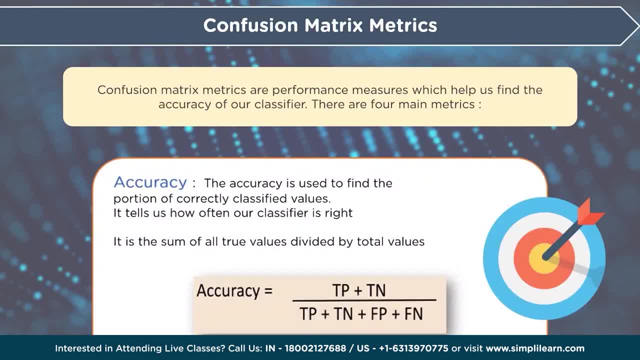 They will just glaze over So confusion. matrix metrics Are performance measures Which help us find the accuracy of our classifier. There are four main metrics: Accuracy: The accuracy is used to find the portion Of the correctly classified values. It tells us how often our classifier is right. 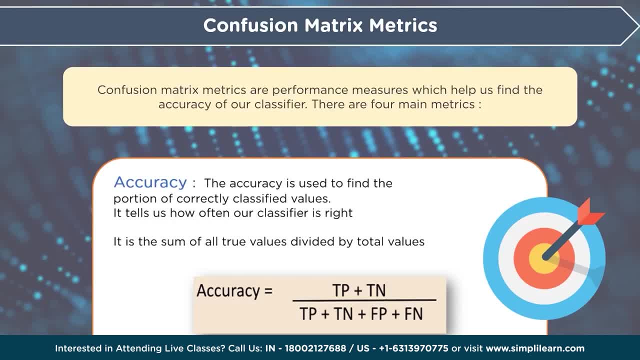 It is the sum of all true values Divided by the total values, And this makes sense. Again, it is one of those things I don't want to. You know, It depends on what you are looking for. Are you looking for? 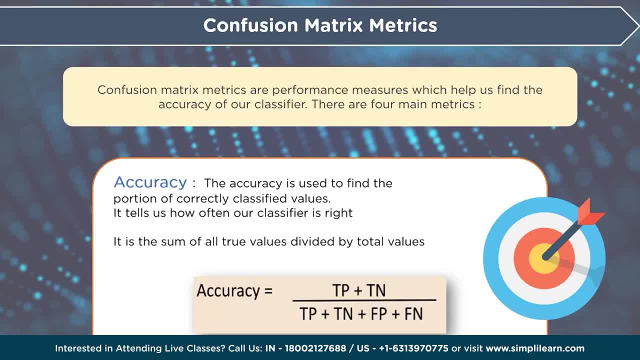 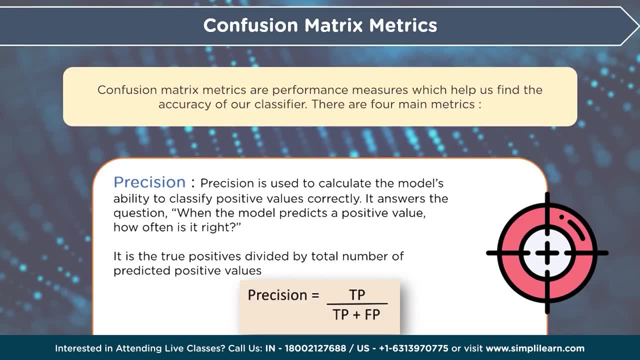 Not to miss any spam mails. Are you looking to drive down the road And not run anybody over? Precision Is used to calculate the models ability to classify Positive values correctly. It answers the question When the model predicts a positive value. 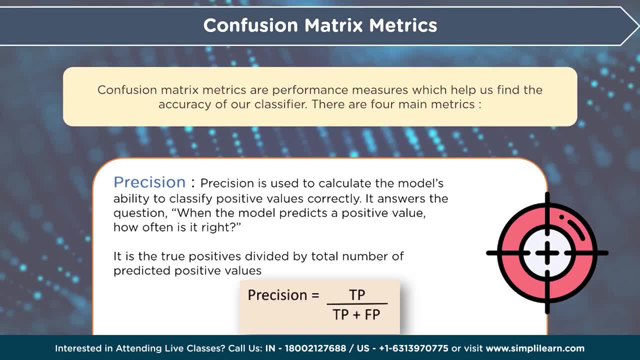 How often is it right? It is the true positive Divided by the total number of predicted positive values. Again, this one Depends on what project you are working on, Whether this is what you are going to be focusing on. So recall, 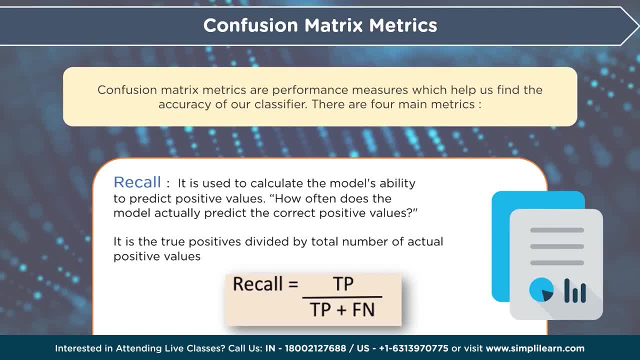 It is used to calculate the models ability To predict positive values. How often Does the model actually predict the correct Positive values? It is the true positive Divided by the total number of actual positive values, And then your F1 score. 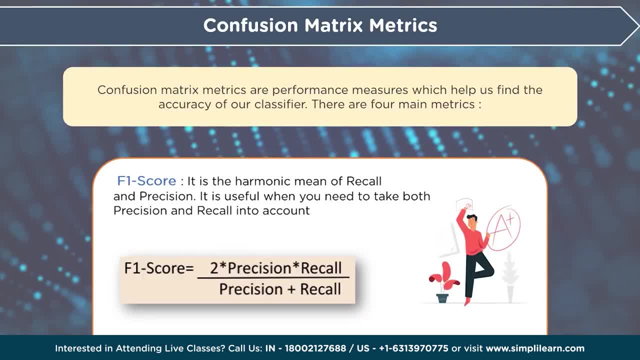 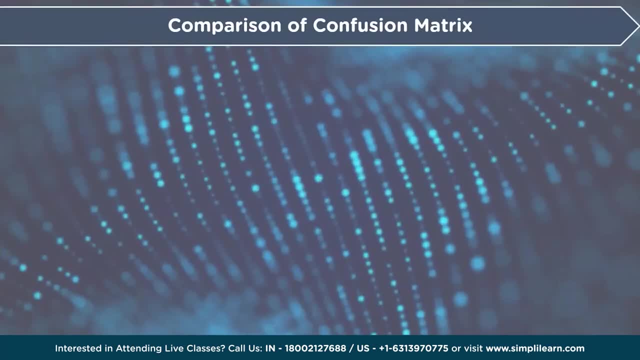 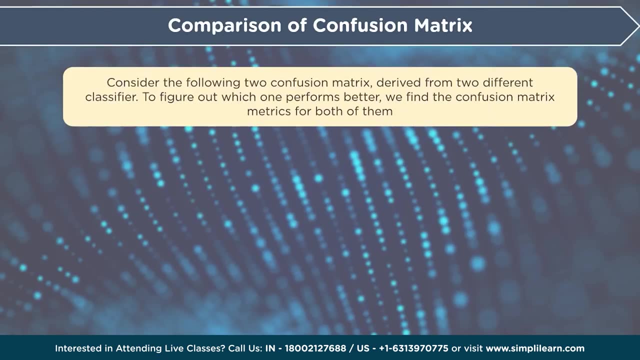 It is the harmonic Mean of recall and precision. It is useful when you need to take Both precision and recall Into account. Consider the following Two confusion matrix Derived from two different classifier To figure out Which one performs better. 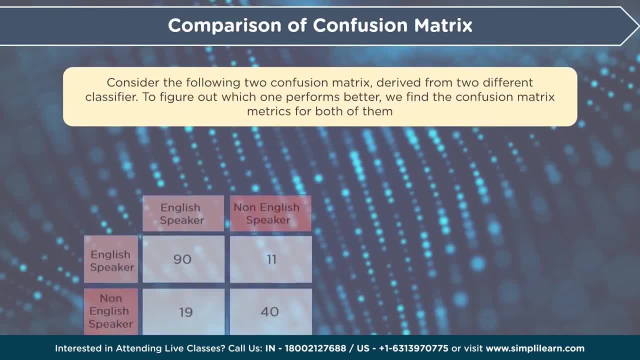 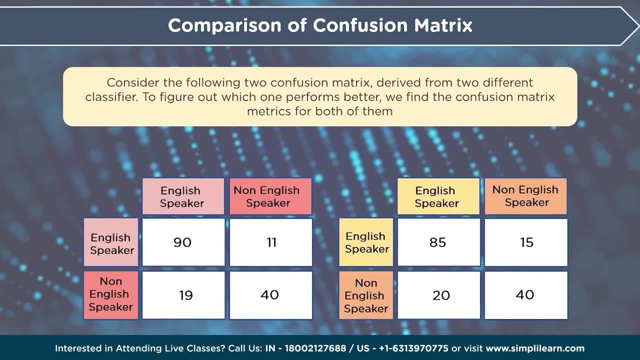 We can find the confusion matrix For both of them And you can see we are back to. Does it classify whether they can speak English or non speaker? They don't know the English language, And so we put these two Confusion matrixes out here. 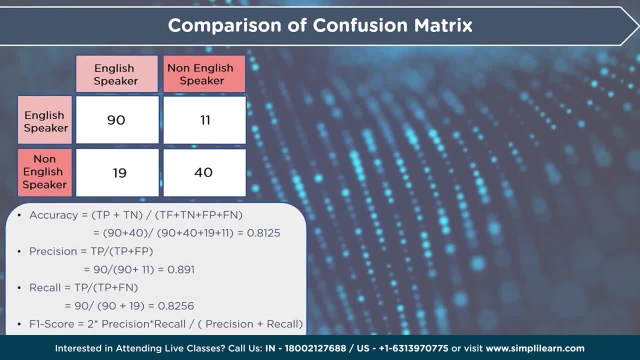 We can go ahead and do the math behind that. We can look up the accuracy Of TPN plus TN Over the TF plus TN plus FP Plus FN, And so we get an accuracy of .8125.. And we have a precision. 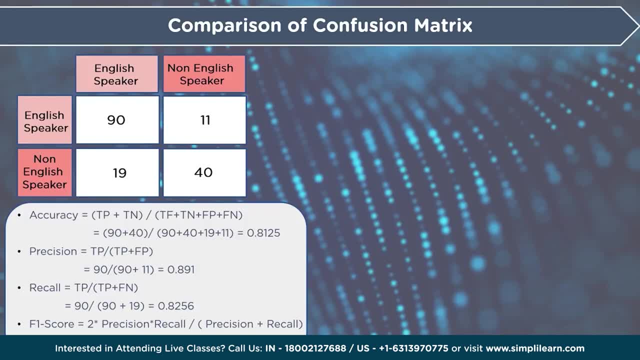 If you do the precision, Which is your TP Truth positive Over TP plus FP, We get .891.. And if we do the recall, We will end up with the .825.. That is your TP over TP plus FN. And then, of course, 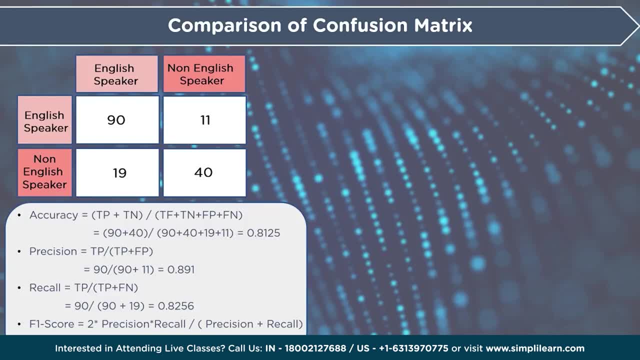 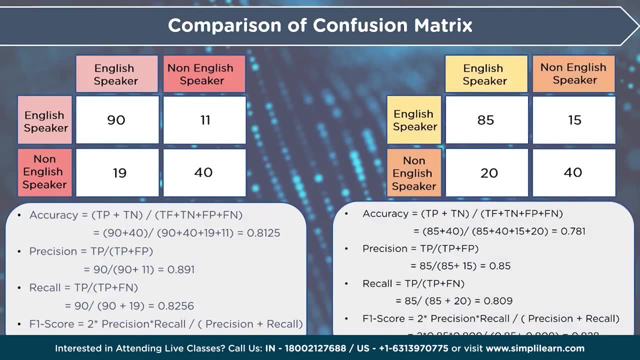 Your F1 score Times, precision times, recall Over precision plus recall And we get the .857.. And if we do that With another model, Let's say we had two different models And we are trying to see which one we want to use- 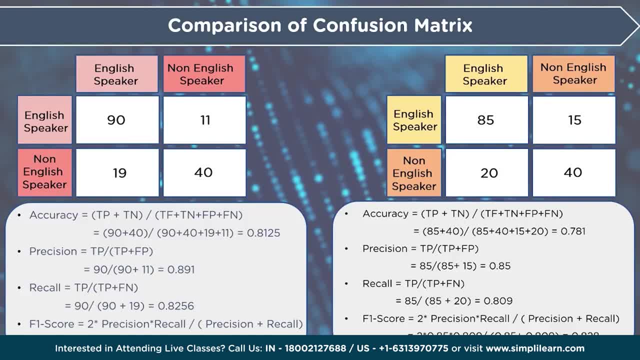 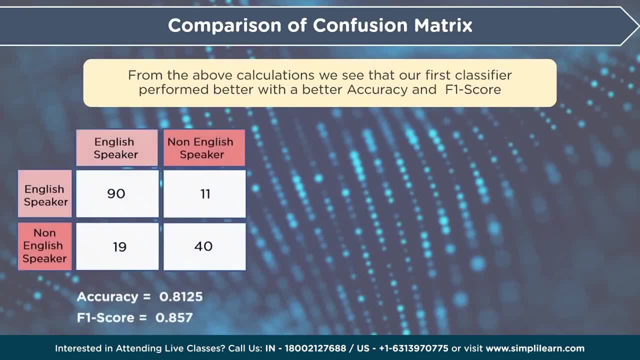 For whatever reason, We might go ahead and compute the same thing. We have our accuracy, Our precision and our recall And our F1 score And as we are looking at this, We might look at the accuracy And what we are interested in. 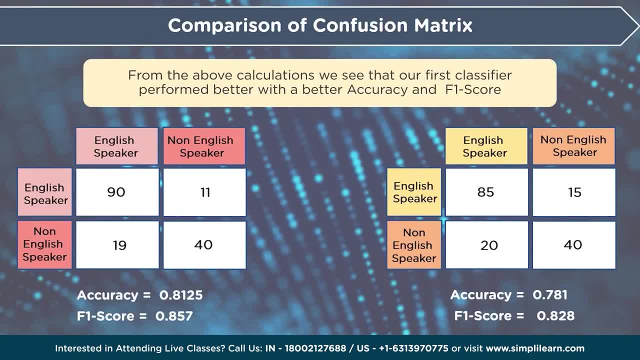 Is: how many people Are we able to classify As being able to speak English? I really don't want to know. I really don't want to know If they are non speakers. I would rather miss 10 people speaking English Instead of 15.. 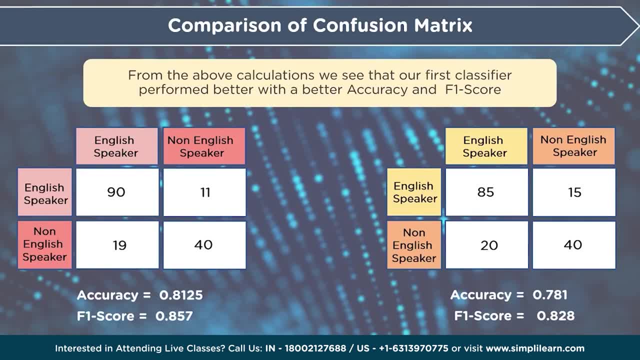 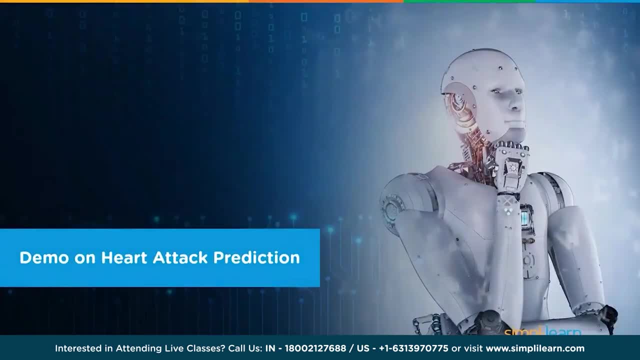 And so you can see from these charts We probably go with the first model Because it does a better job In guessing who speaks English And has a higher accuracy, Because in this case We have a demo, So you can see what this looks like. 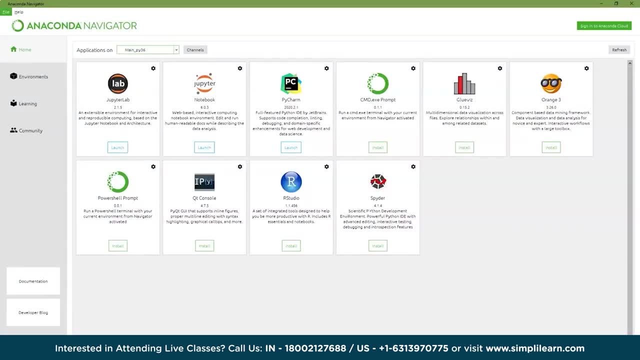 In the Python setup And in the actual coding, But this will go into Anaconda Navigator. If you are not familiar with Anaconda, It is a really good tool To use as far as doing display And demos And for quick development. 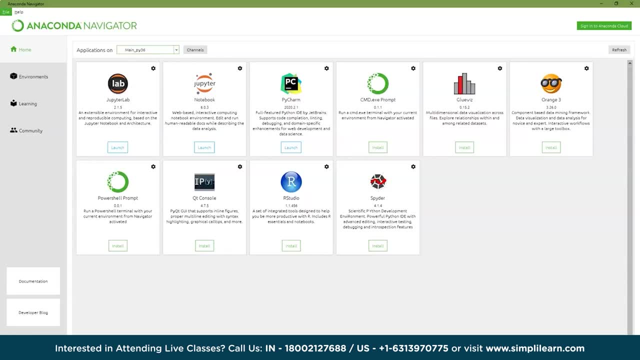 As a data scientist, I just love the package. Now, if you are going to do something heavier lifting, There are some limitations with Anaconda And with the setup. You can do just about anything in here With your Python, And for this we will go with Jupyter Notebook. 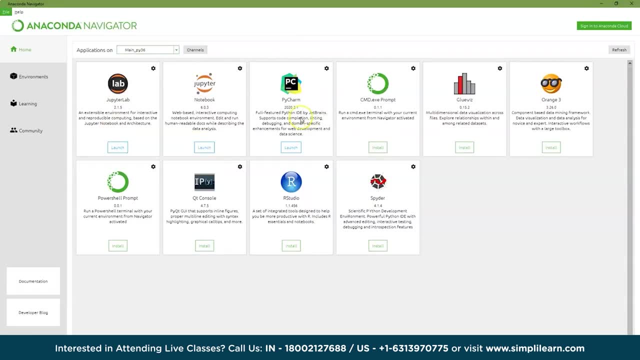 Jupyter Lab is the same as Jupyter Notebook, You will see they now have integration with PyCharm. If you work in PyCharm, Certainly there is a lot of other integrations That Anaconda has And we have opened up. 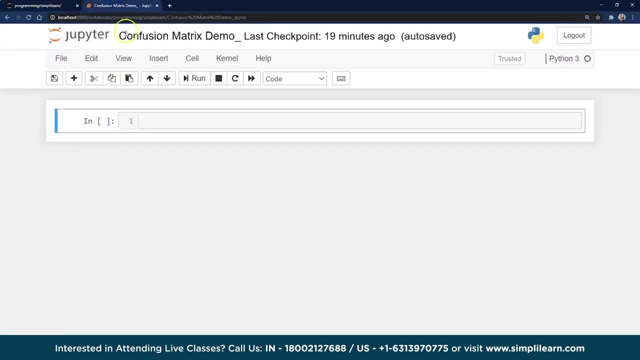 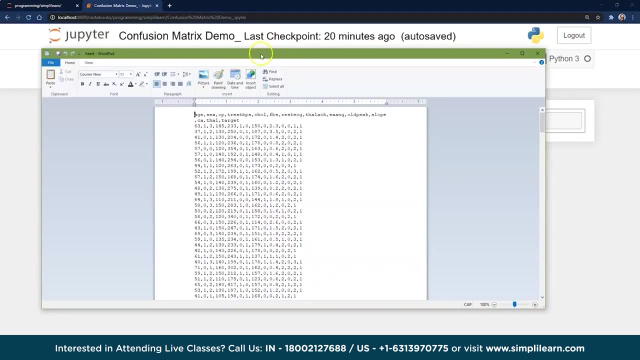 Simply learn files I work on And create a new file Called Confusion Matrix Demo, And the first thing we want to note Is the data we are working with Here. I have opened it up In a WordPad or Notepad or whatever. 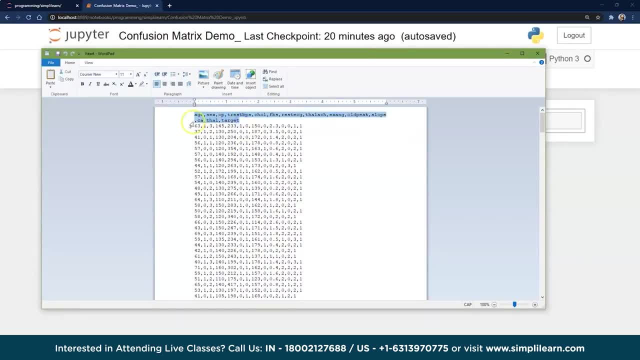 You can see it has a row of headers, Comma separated, And then all the data going down below, And then I saved this in the same file, So I don't have to remember what path I am working on. Of course, if you have your data separated, 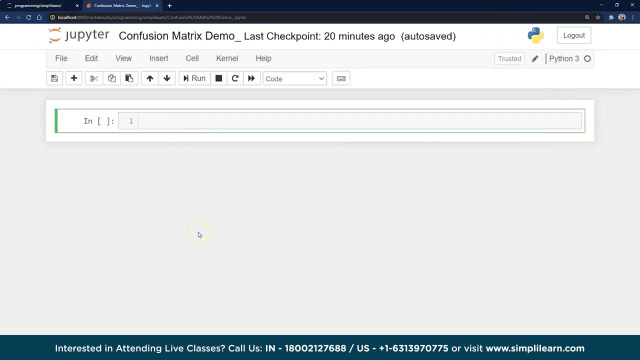 And you are working with a lot of data, You probably want to put it into a different folder Or file, Depending on what you are doing, And the first thing we want to do Is go ahead and import our tools. We are going to use the Pandas. 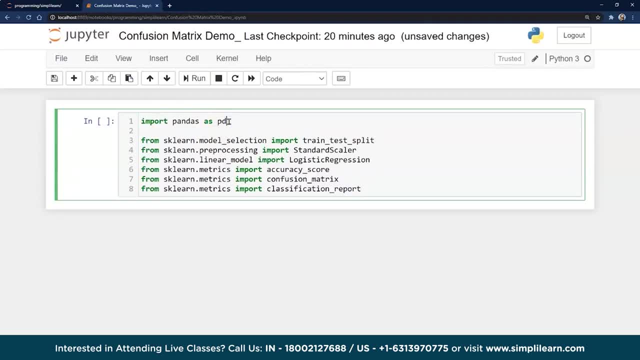 That is our data frame. If you haven't had a chance to work with the data frame, Please review. Pandas data frame. Go into simply learn. You can pull up the Pandas data frame Tutorial on there And then we are going to use. 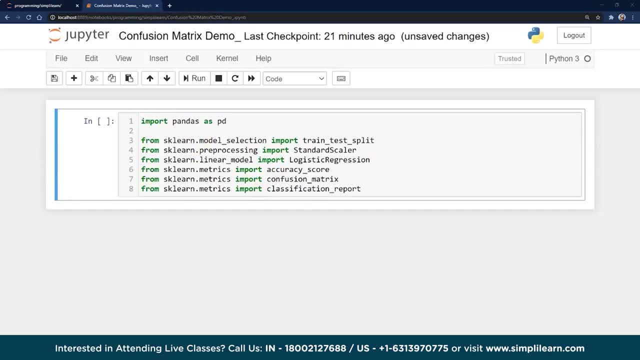 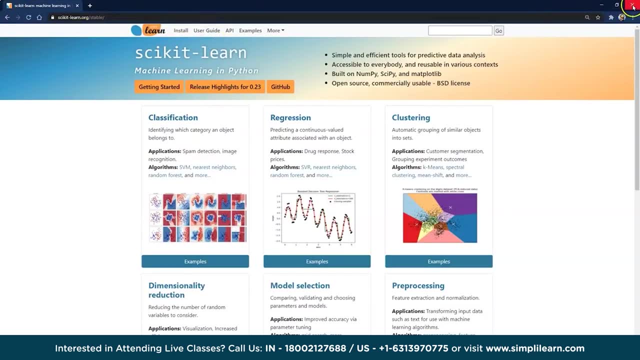 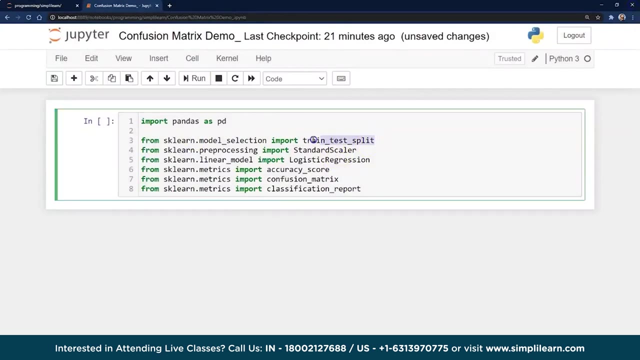 The Scikit framework, Which is all denoted as sklearn, And I can just pull this in. You can see, here is the Scikit-learnorg With the stable version That you can import into your Python And from here We are going to use the train test split. 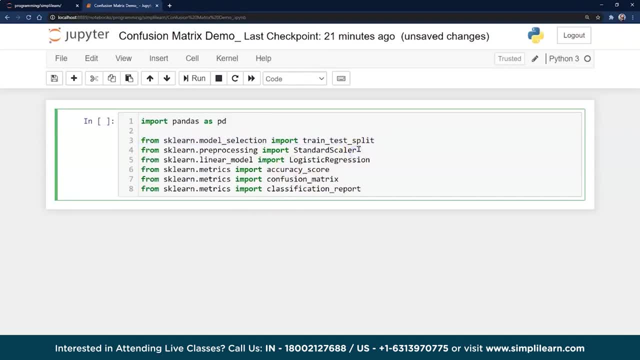 For splitting our data. We are going to do some pre-processing, We are going to do Use the logistic regression model. That is our actual Machine learning model we are using, And then, with this particular Setup, is about, We are going to do the accuracy score. 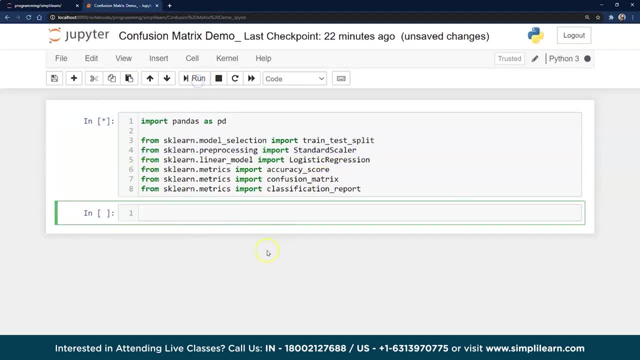 The confusion matrix And the classifier report. So let me go ahead and run that And bring all that information in And, just like we always do, Once we open the file, We need to go ahead and load our data in here. So we are going to go ahead and do our. 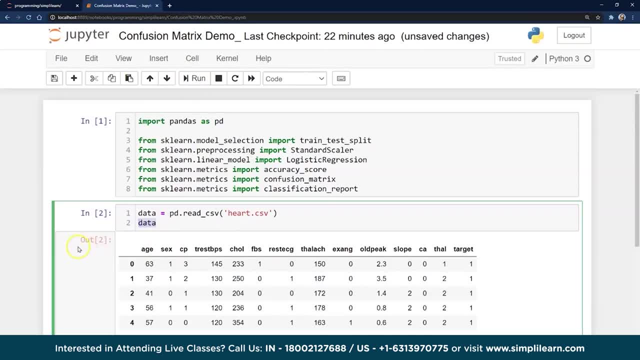 Pandas read CSV And then, just because we are in Jupyter Notebook, We can just put data to read the data in here. A lot of times we will actually Let me just do this. I prefer to do just the head of the data. 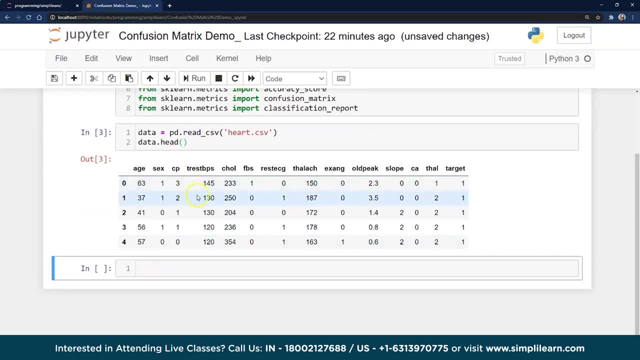 Or the top part And you can see we have age 6.. I am not sure what CP stands for: Test BPS cholesterol. So a lot of different measurements. If you were in this domain, You would know what all these different 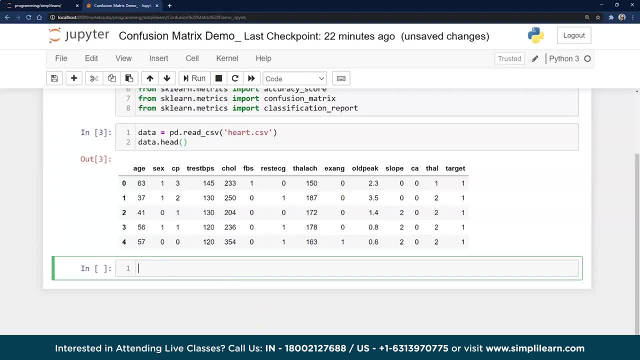 Measurements mean. I don't want to focus on that too much, Because when we are talking about data science, A lot of times you have no idea What the data means. If you have ever looked up the breast cancer measurement, It is just a bunch of measurements. 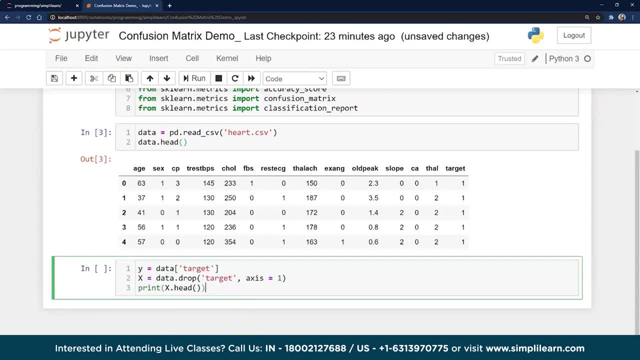 And numbers. Unless you are a doctor, You are going to have no idea what those measurements mean. But if it is your specialty in your domain, You better know them. So we are going to go ahead and create Y And we are going to set it equal to the target. 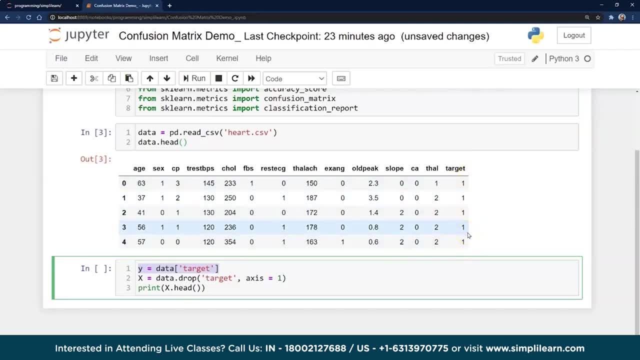 Our target value here, And it is either 1 or 0. So we have a classifier. If you are dealing with 1, 0. True, false, What do you have? You have a classifier And then our X is going to be. 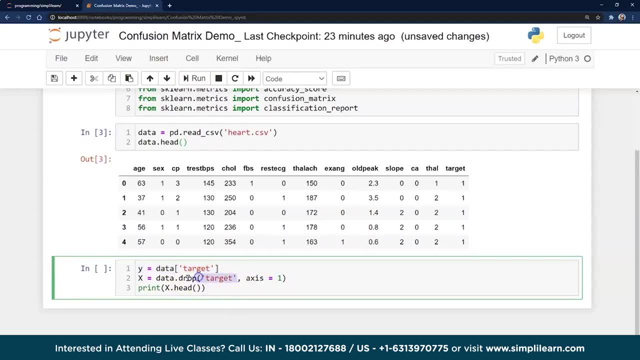 Everything except for the target. So we are going to go ahead and drop the target. Axis equals 1.. Remember that is columns Versus the index or rows. Axis equals 0. Would give you an error, So we are going to drop like row 2.. 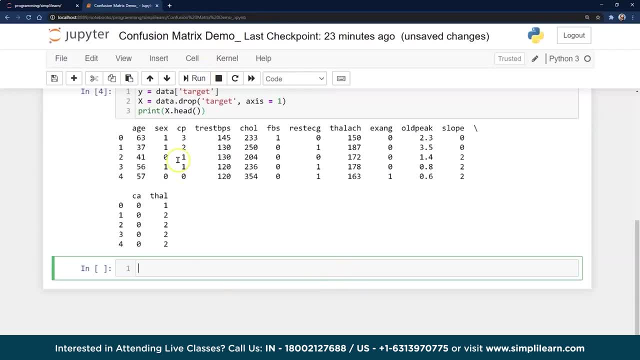 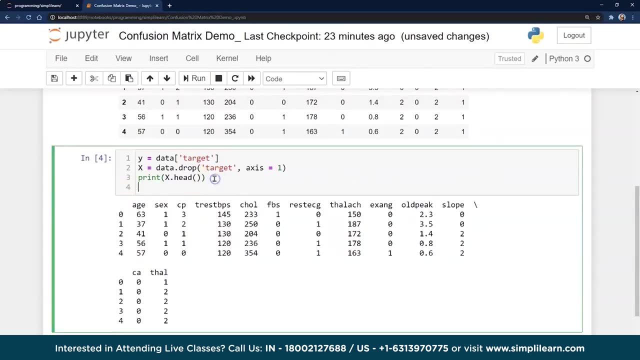 And then we will go ahead and just print that out. So you can see what we are looking at. And here we have Y data, X data. You can see from the X data We have the X head And we can go ahead and just do print. 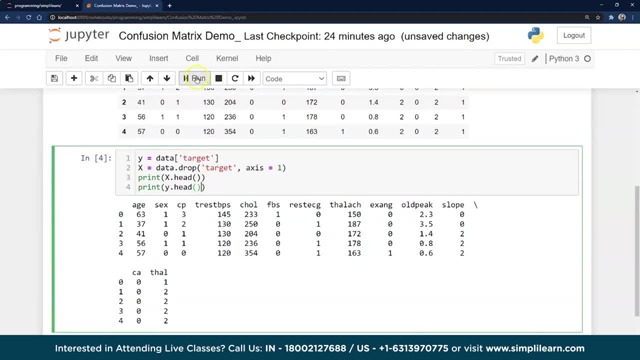 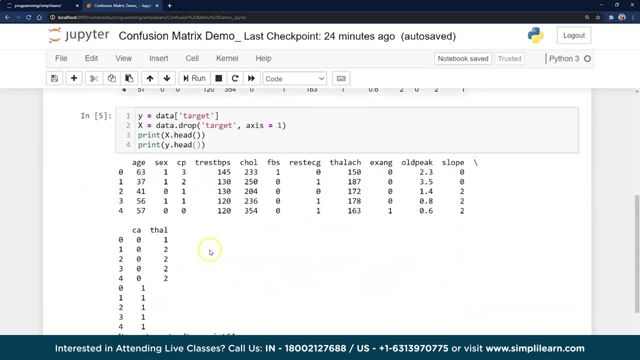 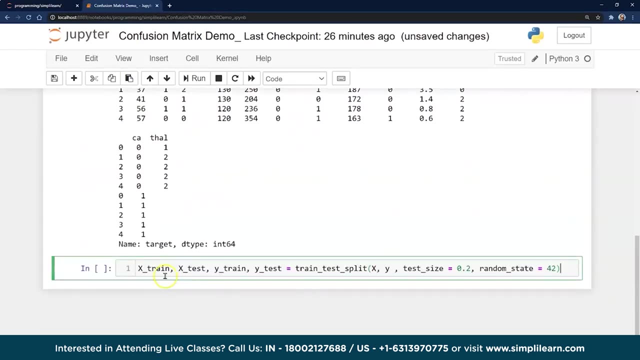 The Y head data And run that. So this is all loading the data That we have done so far. If there is a confusion in there, You can just tape and review it, And then we need to go ahead and split our data. 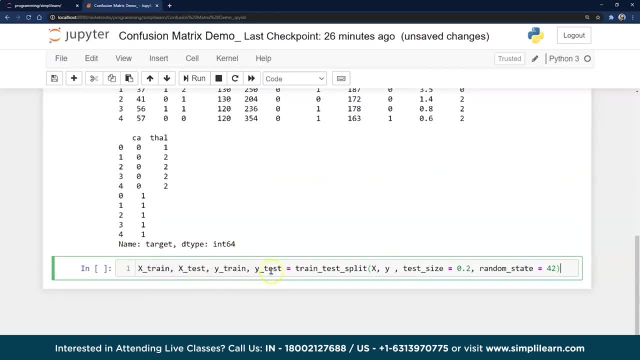 Into our X train, X test, Y train, Y test. And keep in mind you always want to split the data Before we do the scalar And the reason is that You want the scalar on the training data To be set on the training data. 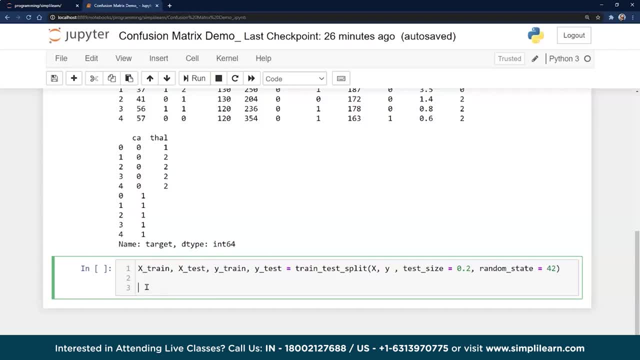 Or fit to it, But not on the test data. Think of this as being out in the field. You are, not Your results, So it is always important to do Make sure whatever you do to the training data Or whatever fit you are doing. 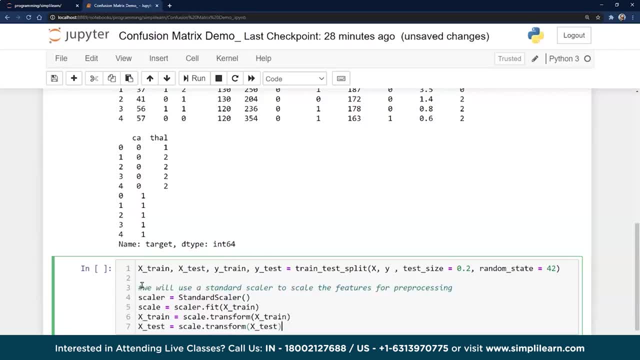 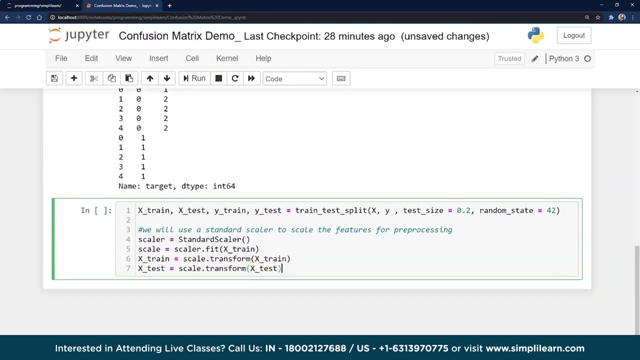 Is always done on the training, Not on the test. And then we want to go ahead and scale the data. Now We are working with Linear regression model. I will mention this here in a minute, When we get to the actual model. 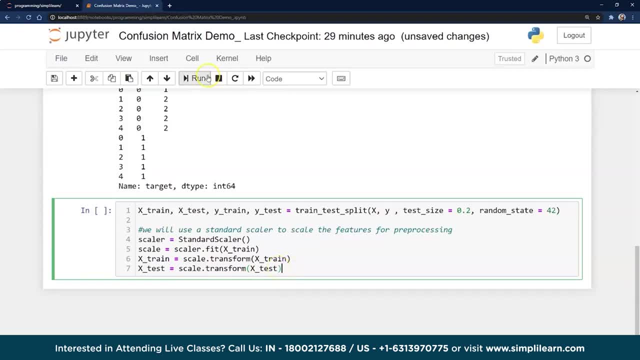 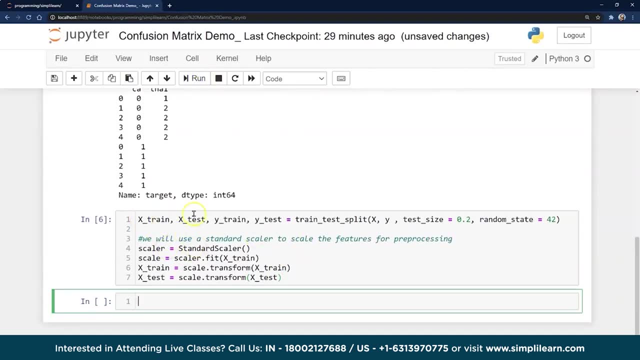 So sometimes you don't need to scale it When you are working with linear regression models. It is not going to change your result as much. It has a huge impact. But we are going to go ahead and take. Here is our X train. 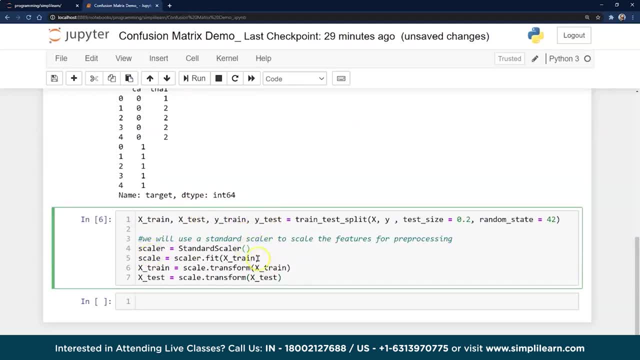 X test, Y train, Y test. We create our scalar. We go ahead and scale. The scale is going to fit the X train. And then we are going to go ahead and take our X train And transform it, And then we also need to take our X test. 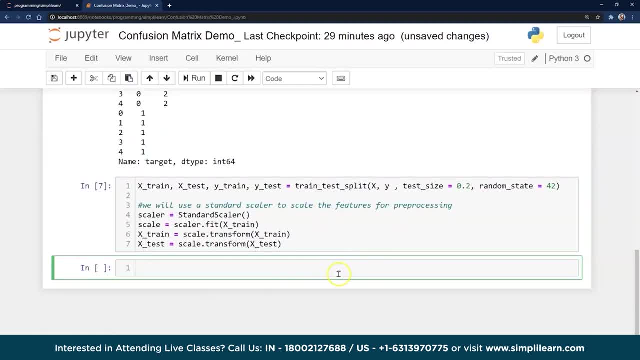 And transform it based on the scale on here, So that our X is now Between that nice minus one to one And that is our data setup And hopefully All of that looks fairly familiar to you If you have done a number of our other classes. 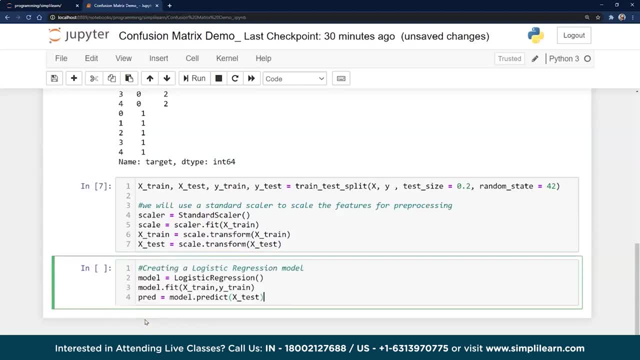 And you are up to the setup on here, And then what we want to go ahead and do Is create our model And we are going to use the logistic regression model And from the logistic regression model, We are going to go ahead and fit. 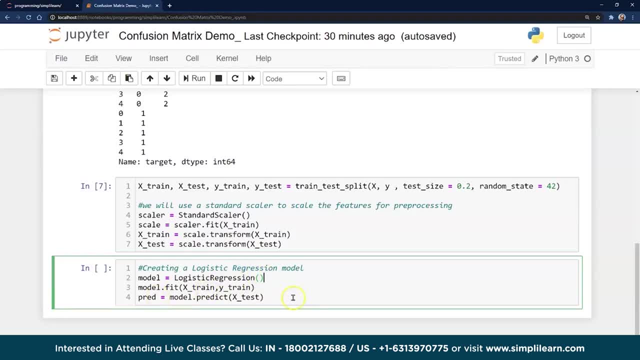 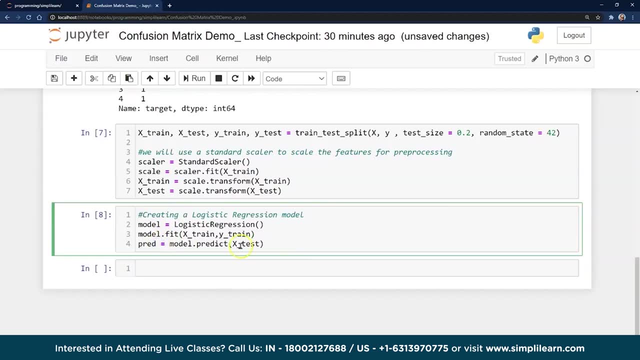 Our X train and Y train, And then we will run our predicted value on here, And so let's go ahead and run that. And so now We are, We actually have, like our X test And our prediction. So, if you remember from 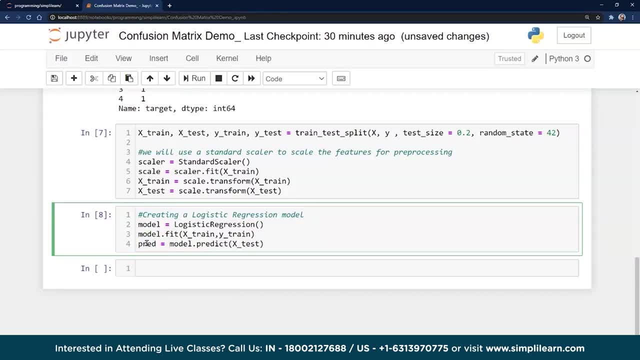 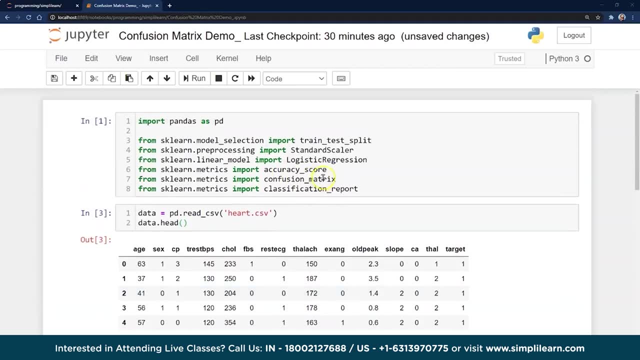 Our matrix. We are looking for the actual Versus, the prediction And how those compare. And if I take us back up here, You are going to notice that we imported The accuracy score, The confusion matrix And the classification report. 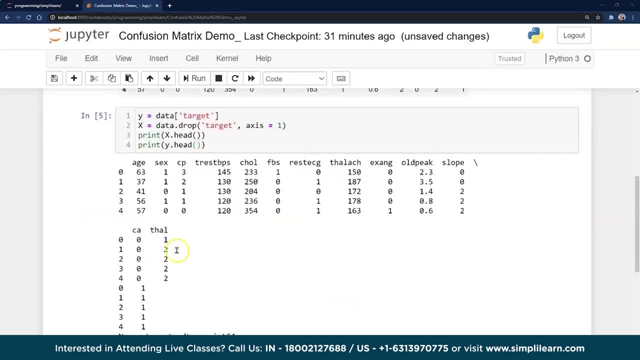 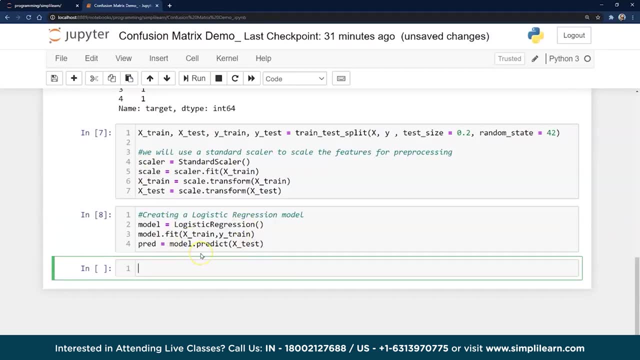 And there is, of course, our logistic regression, The model we are using for this, And I did mention I was going to talk a little bit about scalar And the regression model, The scalar On a lot of your regression models, Your basic mass standard regression models. 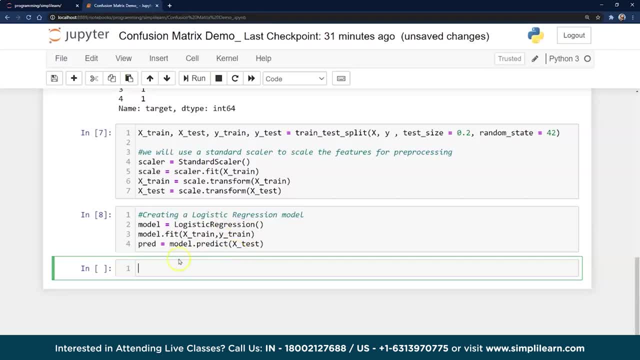 And I would have to look it up for the logistic regression model. When you are using a standard regression model, You don't need to scale the data, It is already just built in. by the way, the model works In most cases, But if you are in a neural network, 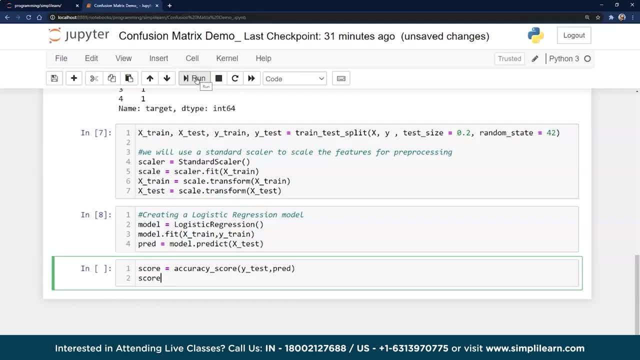 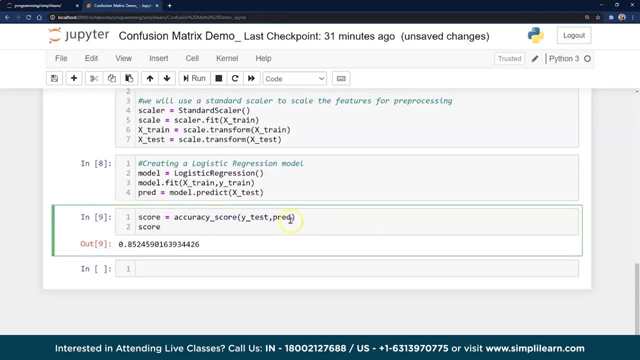 And there is a lot of other different setups, Then you really want to take this And fit that on there, And so we can go in And do the accuracy. And this is, if you remember correctly, We were looking at the accuracy. 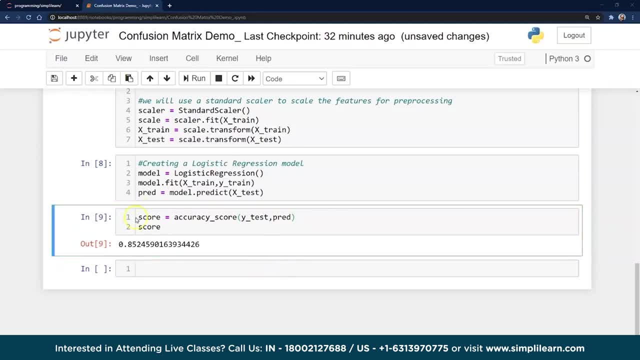 With the English speaking. So this is saying Our accuracy As to whether this person is. I believe this is the heart data set. It is going to be accurate About 85% of the time As far as whether it is going to predict. 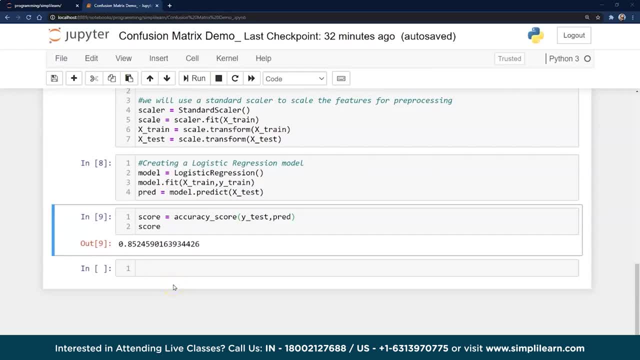 The person is going to have a heart condition Or the one As it comes up with the 01 on there, Which would mean at this point That you have an 85% being correct On telling someone they are extremely high risk. 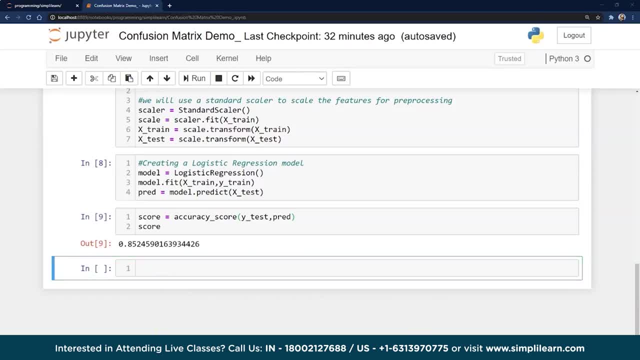 For a heart attack kind of thing, And so we want to go ahead And create our confusion matrix, And let me just do that. Of course, the software does everything for us, So we will go ahead and run this And you can see right here. 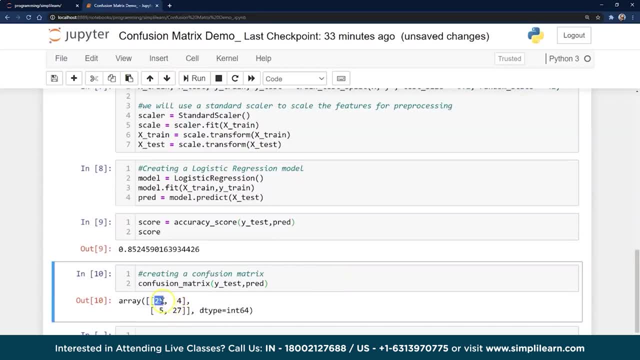 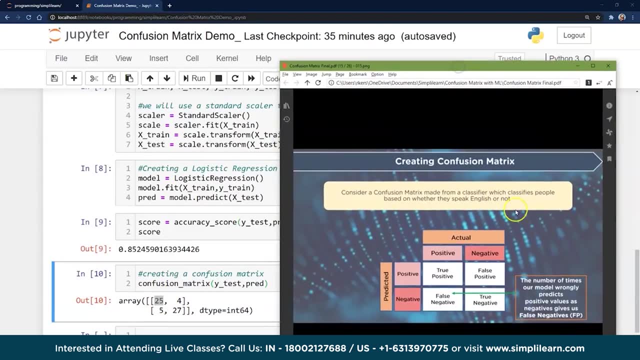 Here is our 25. Prediction- Correct predictions right here, And if you remember From our slide, I will just bring this over. so it is a nice visual. We have our true positive, False positive. So we had 25 which were true. 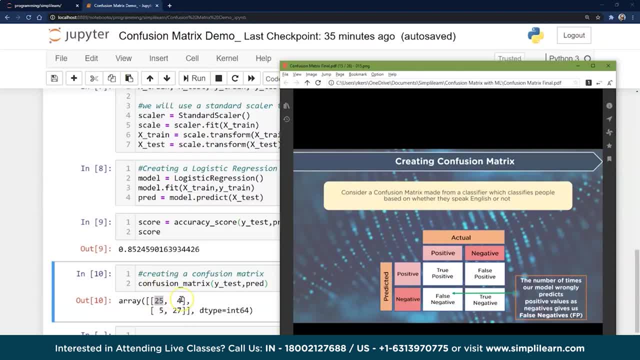 That it said: hey, this person is going to be high risk At heart And we had 4 that were still high risk- That it said were false. So out of these 25 people, Or out of these 29 people- And that makes sense because you have .85.. 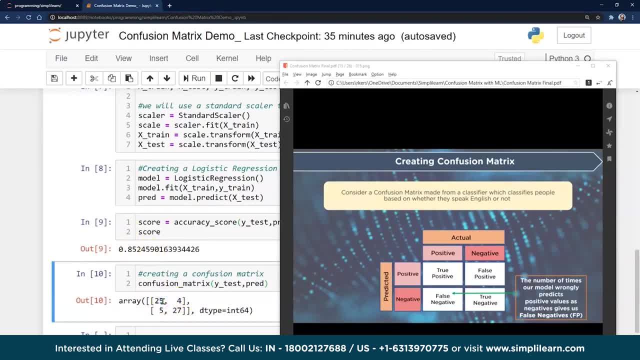 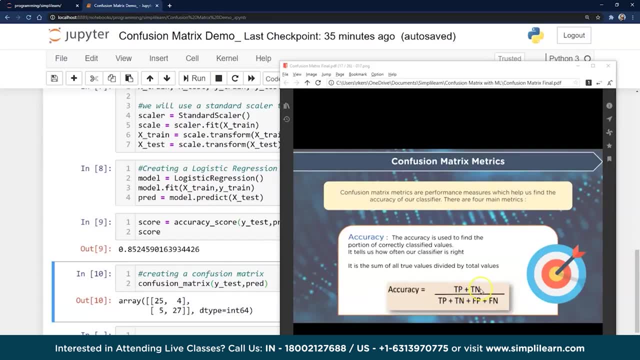 Out of 29 people. It was correct on 25 of them, And so here is our accuracy score. We were just looking at that. Our accuracy is your true positive And your true negative over all of them. So how true is it? 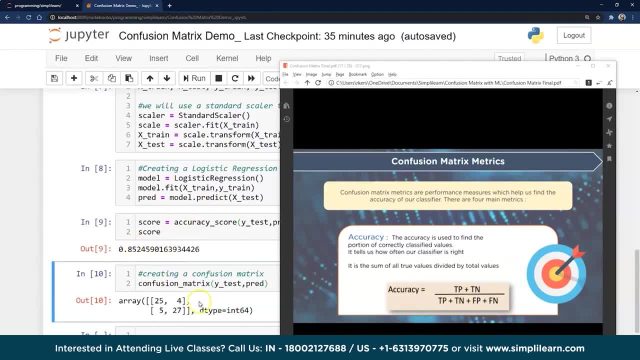 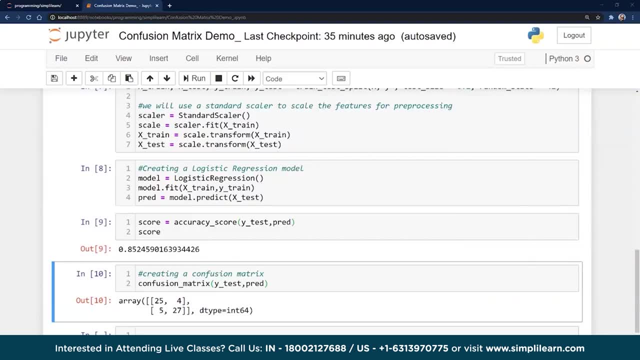 And there is our accuracy coming up here- .85. And then we have our nice matrix generated from that And you can see right here Is a similar matrix we had going from the slide And this starts to This. should start asking questions at this point. 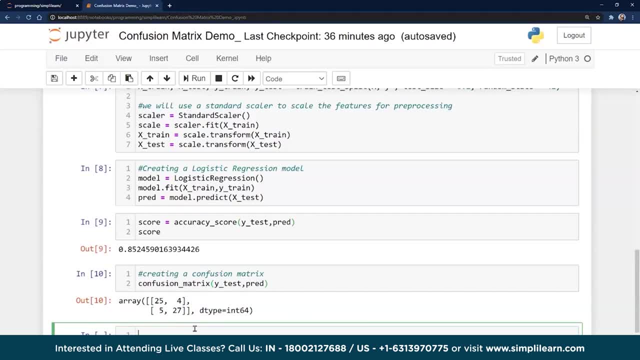 So if you are in a board meeting Or you are working with us, You want to start looking at this data here And saying, well, Is this good enough? Is this number of people? And hopefully you would have a much larger data set. 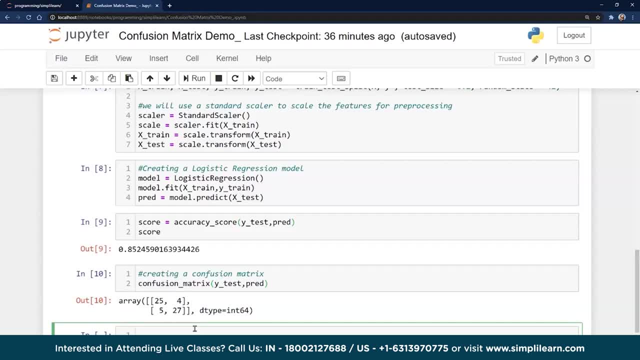 Is my confusion matrix showing for the True positive And false positive? Is that acceptable for what we are doing? And, of course, if you are going to put together Whatever data you are putting out, You might want to separate the True negative. 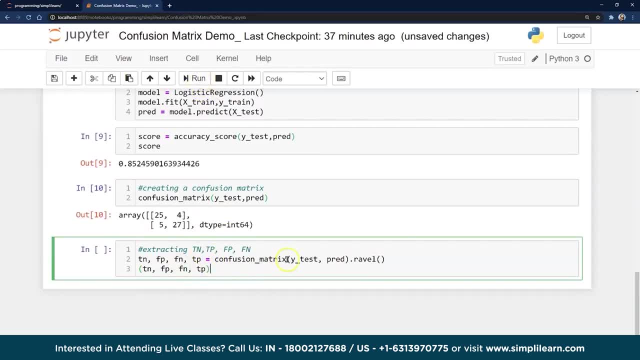 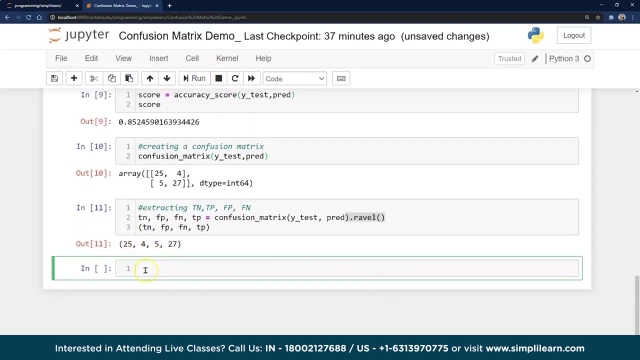 False positive, False negative, False positive. And then of course the ravel part Lets you set that up, So you can just split that right up into a nice tuple. And the final thing we want to show you here In the coding: 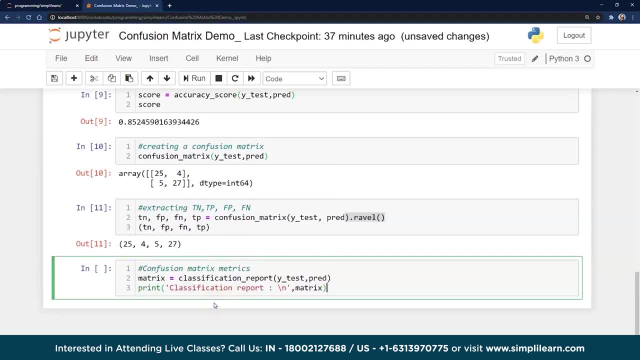 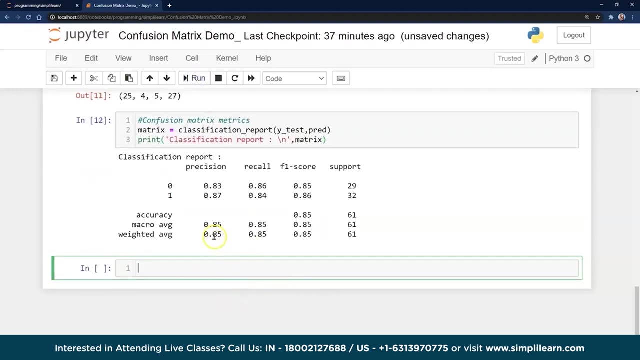 On this part Is the confusion: matrix metrics, And so We can come in here And just use the matrix equals classification report, The y test And the predict, And then we are going to take that classification report And go ahead and print that out. 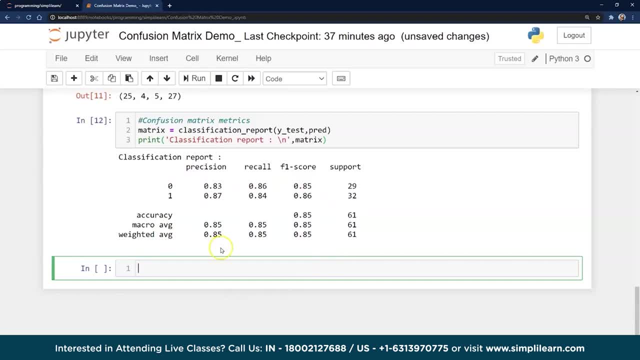 And you can see here It does a nice job, Giving you your accuracy, Your micro average, Your weighted average. You have your precision, Your recall, Your F1 score And your support All in one window, So you can start looking at this data. 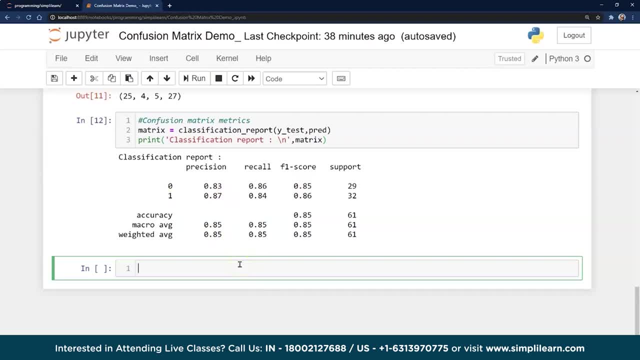 And saying: oh okay, Our precision is at .83.. .87 for getting a positive And .83 for the negative side. Which is a valid information or not to use? And when we are looking at a heart attack prediction, We are only looking at one aspect. 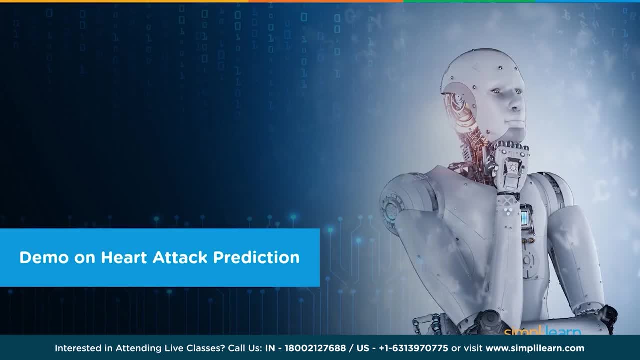 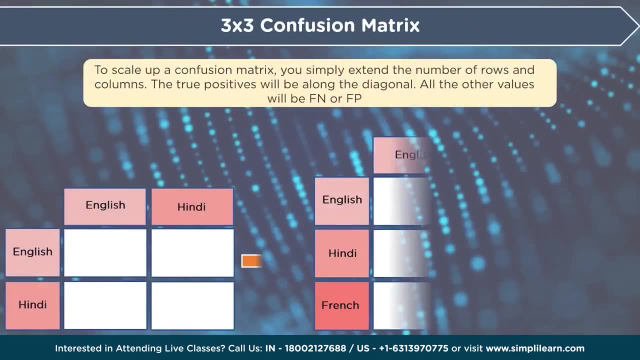 What's the chances of this person having a heart attack or not? You might have something. where We went back to the languages, Maybe you also want to know Whether they speak English Or Hindi Or French And you can see right here. 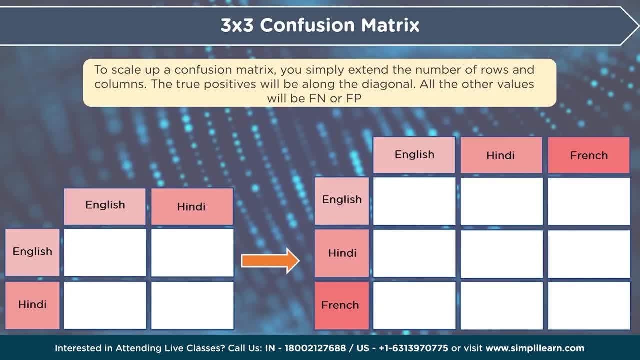 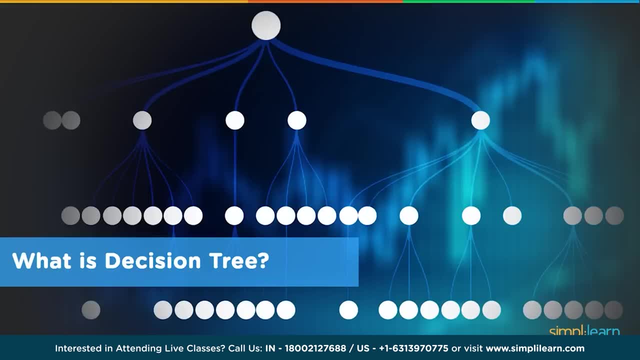 That we can now take our confusion matrix And just expand it as big as we need to, Depending on how many different classifiers We are working on. What is a decision tree? Let's go through a very simple example Before we dig in deep. 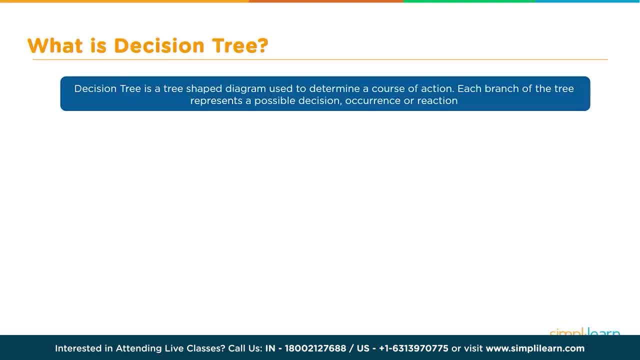 Decision tree is a tree shaped diagram Used to determine a course of action. Each branch of the tree represents a possible decision, Occurrence or reaction. Let's start with a simple question: How to identify a random vegetable from a shopping bag? So we have this group of vegetables in here. 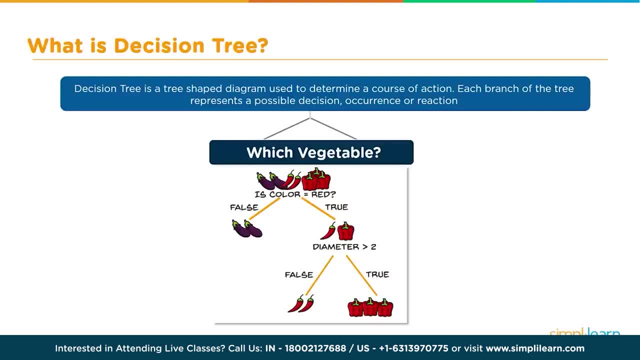 And we can start off by asking a simple question: Is it red? And if it's not, Then it's going to be the purple fruit to the left. Probably an eggplant Is the diameter greater than two. If false, It's going to be a red chili. 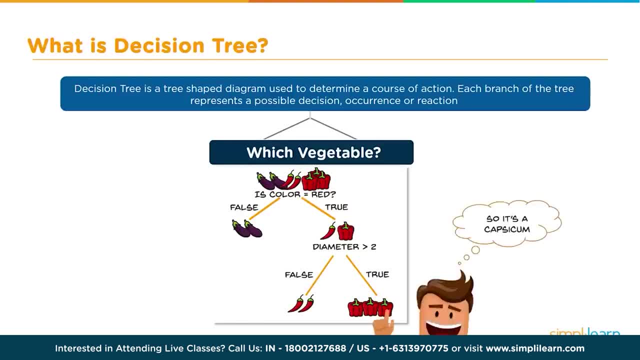 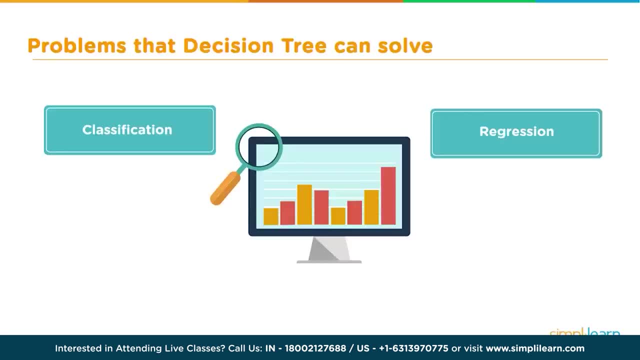 And if it's true, It's going to be a bell pepper from the capsicum family, So it's a capsicum Problems that decision tree can solve. So let's look at the two different categories The decision tree can be used on. 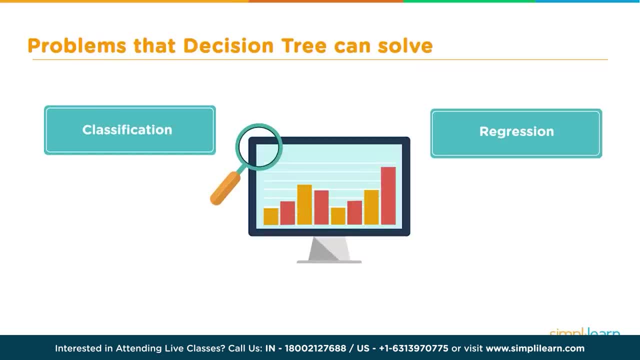 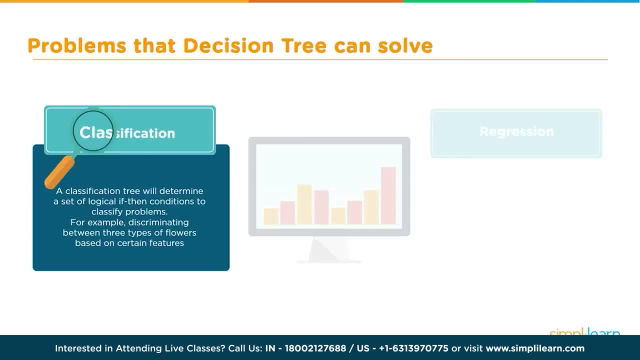 It can be used on the classification- The true, false, yes, no- And it can be used on regression, Where we figure out what the next value is in a series of numbers Or a group of data. In classification, We'll determine a set of logical 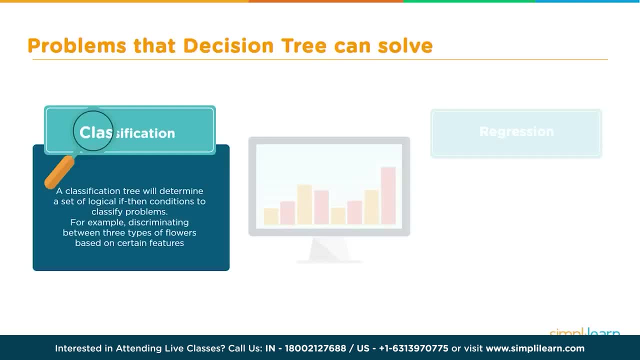 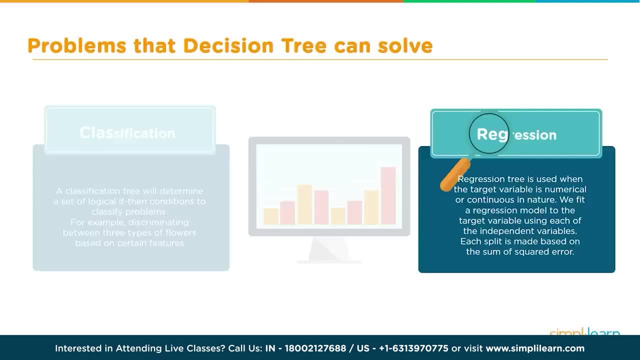 If, then conditions to classify problems, For example Discriminating between three types of flowers Based on certain features. In regression, A regression tree is used when the target variable Is numerical or continuous in nature. We fit the regression model to the target variable. 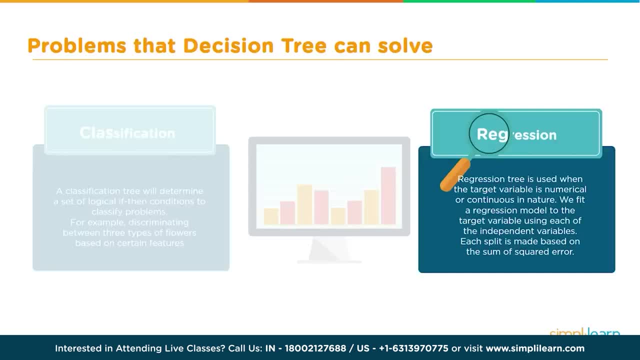 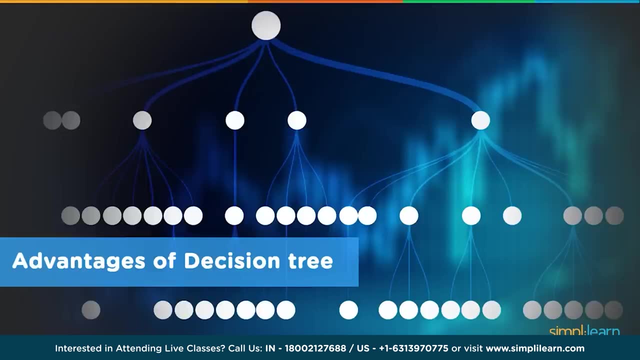 Using each of the independent variables. Each split is made based On the sum of squared error. Before we dig deeper Into the mechanics Of the decision tree, We'll look at the advantages of using a decision tree And we'll also take a glimpse at the disadvantages. 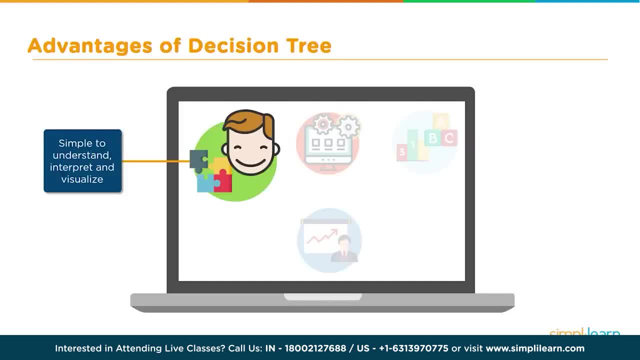 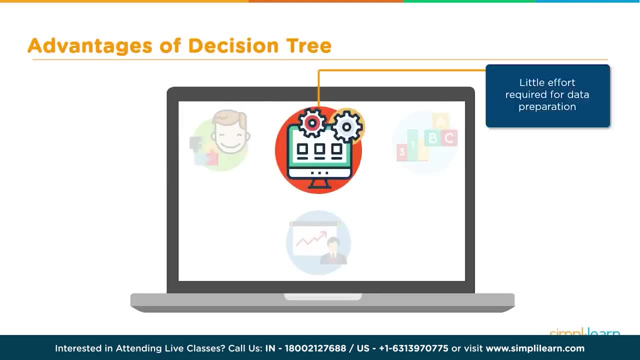 The first thing you'll notice Is that it's simple to understand, Interpret and visualize. It really shines here, Because you can see exactly what's going on In a decision tree. Little effort is required for data preparation, So you don't have to do special scaling. 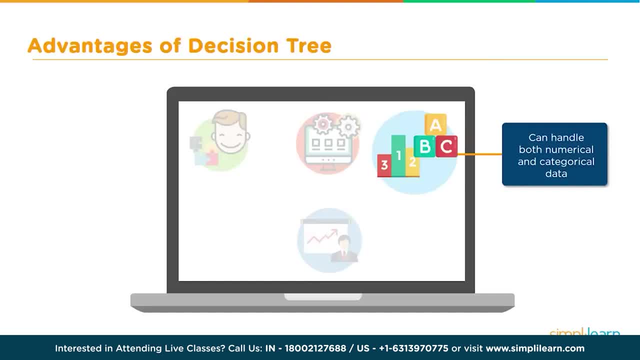 There's a lot of things you don't have to worry about When using a decision tree. It can handle both numerical and categorical data. As we discovered earlier, The parameters don't affect its performance, So even if the data doesn't fit, 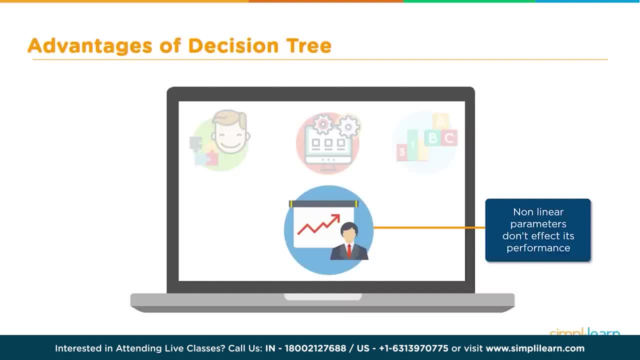 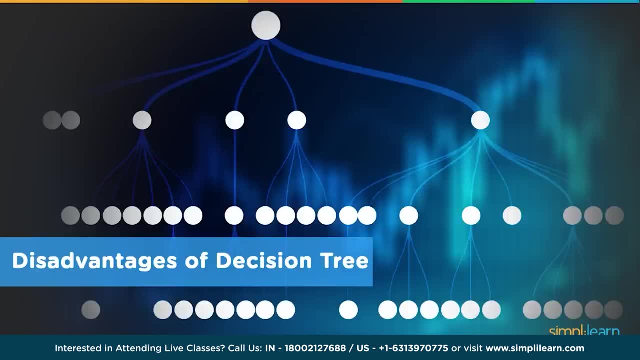 An easy curved graph. You can still use it to create An effective decision Or prediction. If we're going to look at the advantages of a decision tree, We also need to understand The disadvantages of a decision tree. The first disadvantage is overfitting. 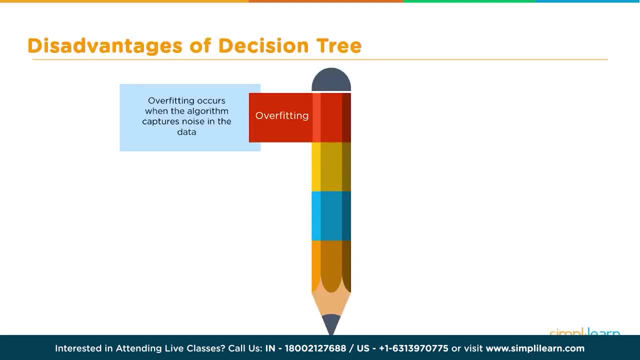 Overfitting occurs when the algorithm Captures noise in the data. That means you're solving for one specific instance Instead of a general solution For all the data. The model can get unstable Due to small variation in data. Low bias tree. 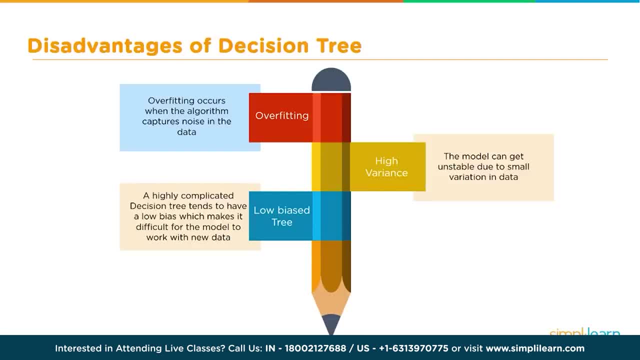 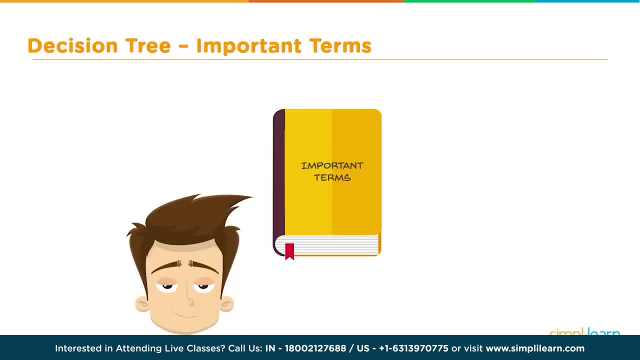 A highly complicated decision tree Tends to have a low bias, Which makes it difficult for the model to work with new data Decision tree Important terms. Before we dive in further, We need to look at some basic terms. We need to have some definitions. 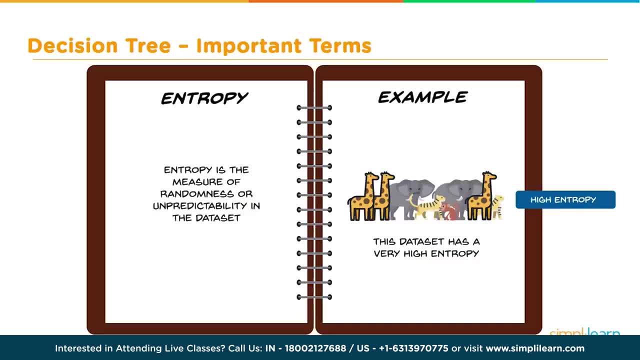 To go with our decision tree And the different parts we're going to be using. We'll start with entropy. Entropy is a measure of randomness In a data set. For example, We have a group of animals In this picture. 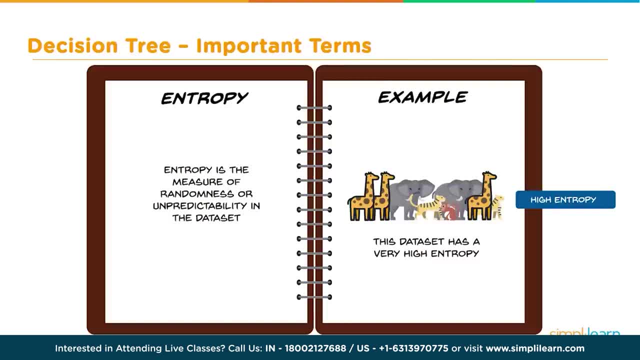 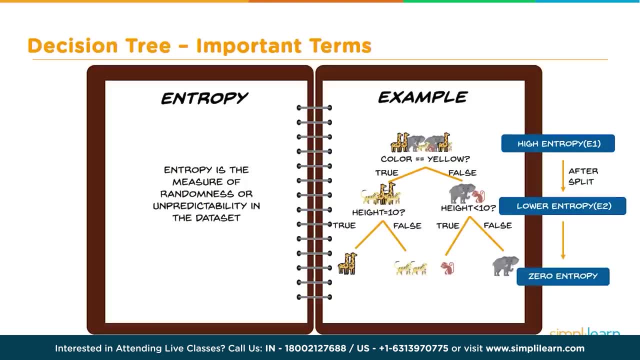 There's four different kinds of animals And this data set is considered to have a high entropy. You really can't pick out what kind of animal it is Based on looking at just the four animals As a big clump of entities. So as we start splitting it into subgroups, 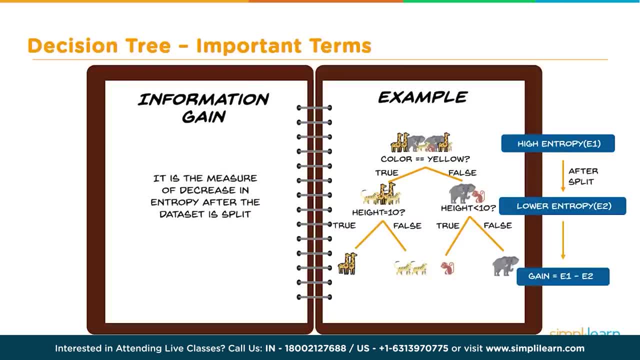 We come up with our second definition, Which is information gain. Information gain: It is a measure of decrease in entropy After the data set is split Based on the color yellow. We've split one group of animals on one side As true, and those who aren't yellow as false. 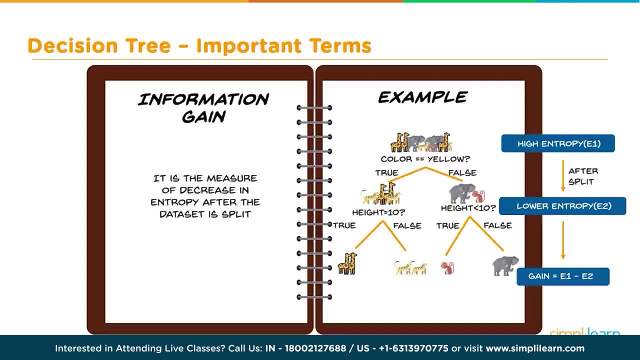 As we continue down the yellow side, We split based on the height. True or false equals 10.. And on the other side, height is less than 10.. True or false. And as you see, as we split it, The entropy continues to be less and less and less. 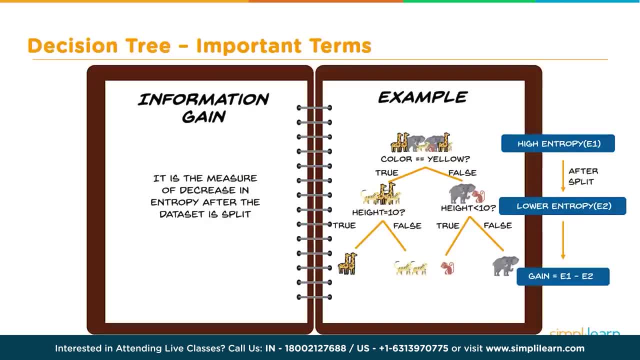 And so our information gain is simply the entropy E1 from the top And how it's changed to E2 in the bottom, And we'll look at the deeper math, Although you really don't need to know When you actually do the programming in Python. 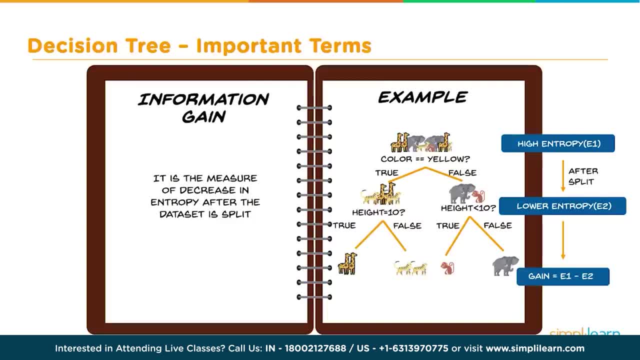 Because it'll do it for you, But we'll look on the actual math At how they compute entropy. Finally, we want to know the different parts of our tree And they call the leaf node. Leaf node carries the classification or the decision. 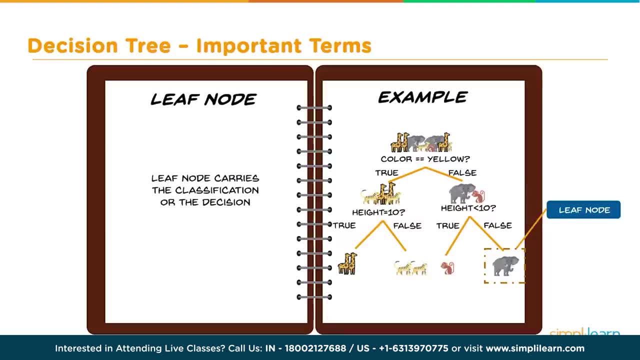 So it's the final end. at the bottom, The decision node has two or more branches. This is where we're breaking the group up Into different parts And finally you have the root node. The top most decision node is known as the root node. 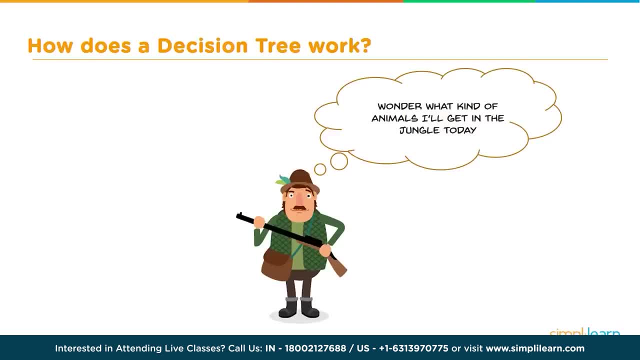 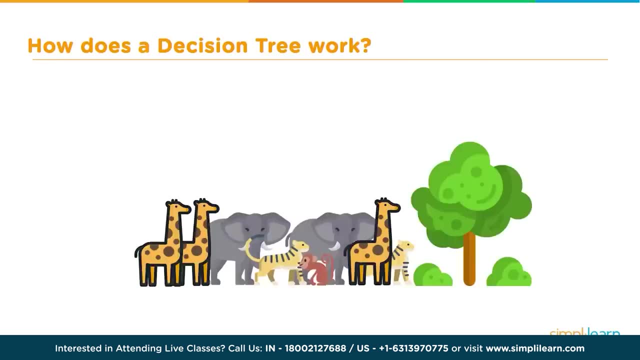 How does a decision tree work? If you're a group of animals, I'll get the jungle today. Maybe you're the hunter with the gun. Or if you're more into photography, You're a photographer with a camera. So let's look at this group of animals. 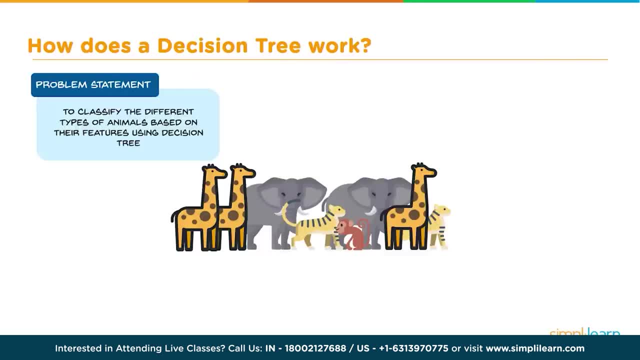 And let's try to classify different types of animals Based on their features using a decision tree. So the problem statement is To classify the different types of animals Based on their features using a decision tree. The data set is looking quite messy. 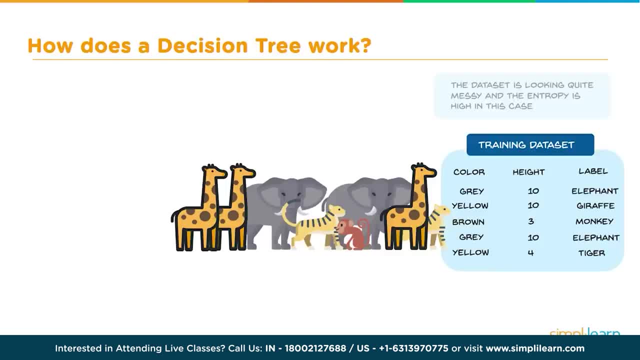 And the entropy is high in this case. So let's look at a training set Or a training data set, And then we have our different animals. We have our elephants, our giraffes, Our monkeys and our tigers, And they're of different colors and shapes. 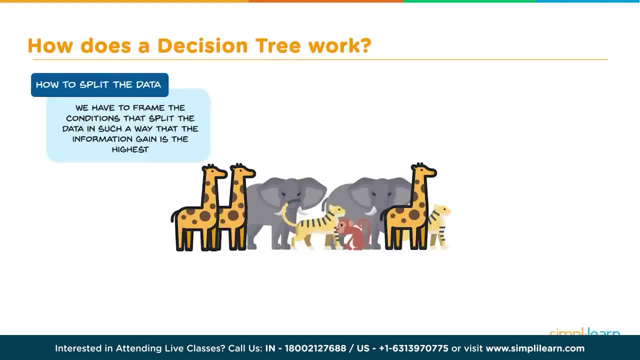 Let's see what that looks like And how do we split the data. We have to frame the conditions that split the data In such a way that the information gain is the highest. Note Gain is the measure of decrease in entropy After splitting. 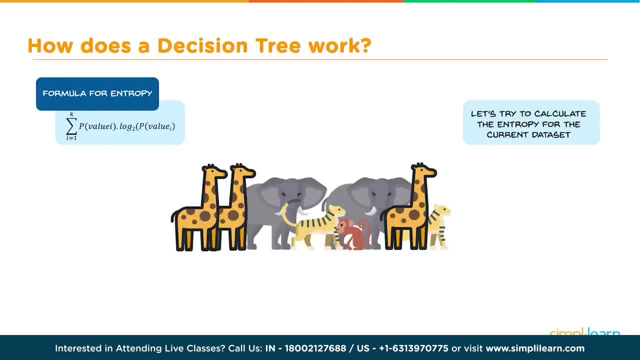 So the formula for entropy is the sum- That's what this symbol looks like, Kind of like a funky E- Of K. K would represent the number of animals, The different animals in there, Where value or P Value of I Would be the percentage of that animal. 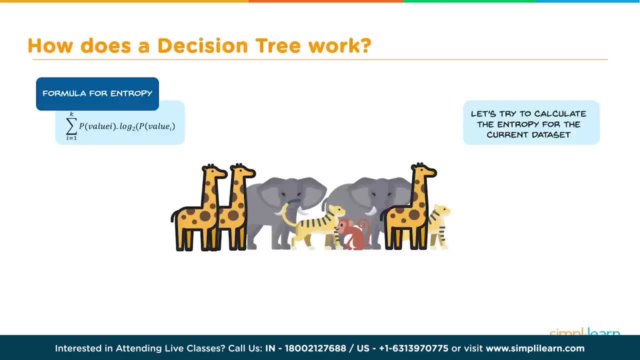 Times the log base: 2. Of the same, The percentage of that animal. Let's try to calculate the entropy for the current data set And take a look at what that looks like, And don't be afraid of the math. You don't really have to memorize this math. 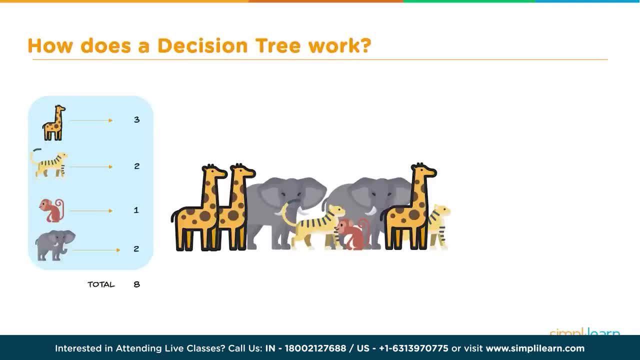 Just be aware that it's there. And this is what's going on in the background. We have two tigers, One monkey, Two elephants- A total of eight animals gathered, And if we plug that into the formula, We get an entropy. 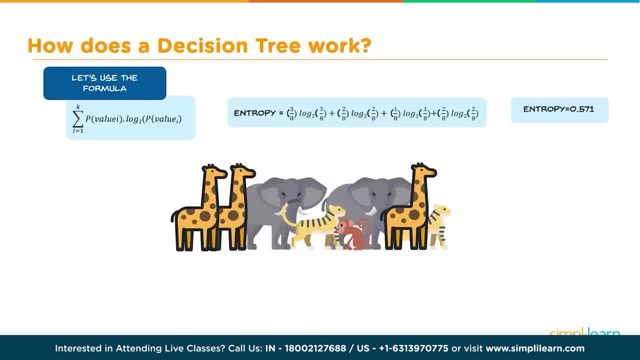 That equals 3 over 8. So we have three giraffes, A total of 8. Times the log. Usually they use base 2 on the log, So log base 2. Of 3 over 8. Plus. 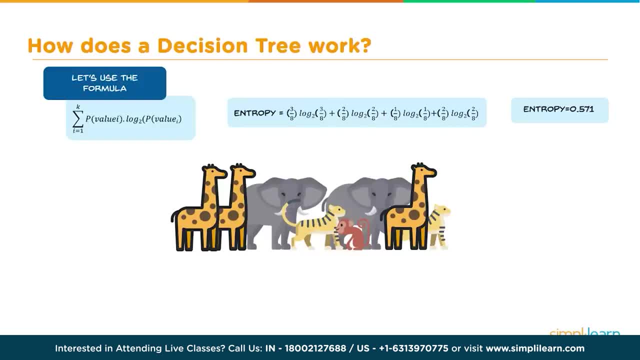 2 over 8 of the tigers Log base, 2. Over 8.. And if we plug that into our computer or calculator I obviously can't do logs in my head. We get an entropy equal to .571.. The program: 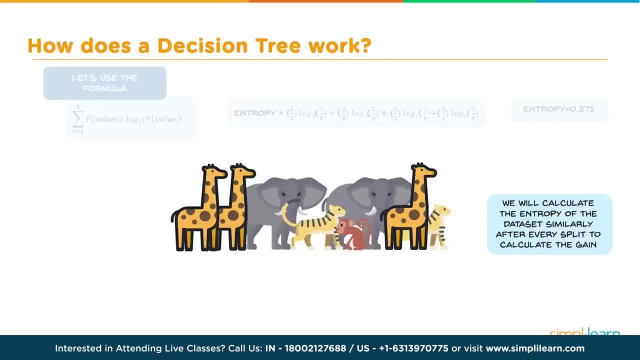 Will actually calculate the entropy of the data set. Similarly, after every split, To calculate the gain. Now, we're not going to go through each set One at a time To see what those numbers are. We just want you to be aware that this is a formula. 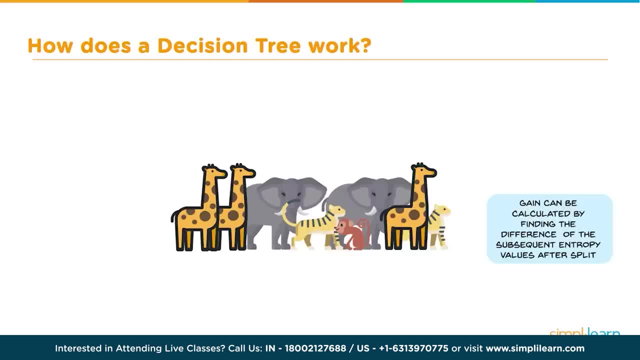 Or the mathematics behind it. We're going to look at the subsequent entropy values After a split. Now we will try to choose a condition That gives us the highest gain. We will do that by splitting the data, Using each condition And checking that the gain we get out of them. 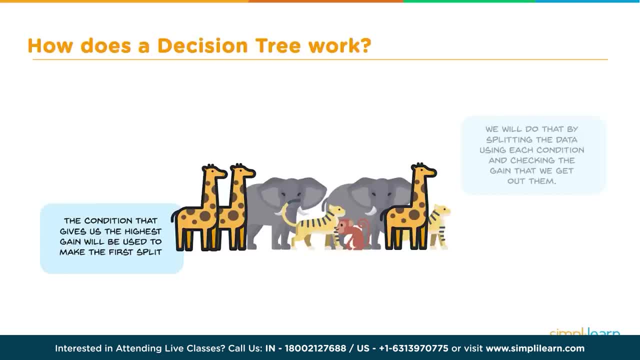 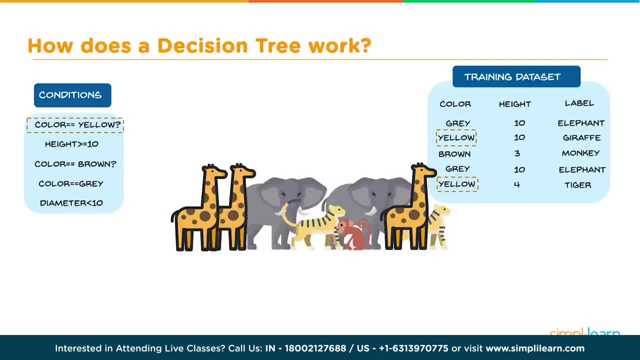 The condition that gives us the highest gain Will be used to make the first split. Can you guess what that first split will be? Just by looking at this image, As a human, it's probably pretty easy to split it. Let's see if you're right. 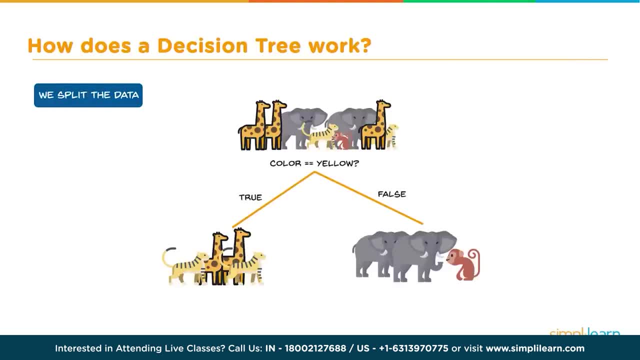 If you guessed the color yellow, You're correct. If it's true, That group of animals goes to the left. If it's false, It goes to the right. The entropy after the splitting has decreased considerably. However, We still need some splitting at both the branches. 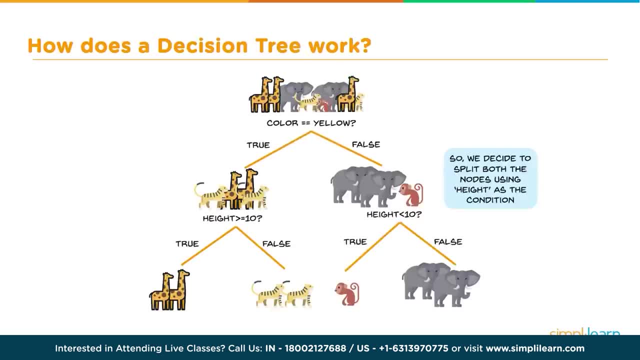 To attain an entropy value equal to zero. So we decide to split both the nodes, Using height as a condition. Since every branch now contains single label type, We can say that entropy in this case Has reached the least value. And here you see, we have the giraffes. 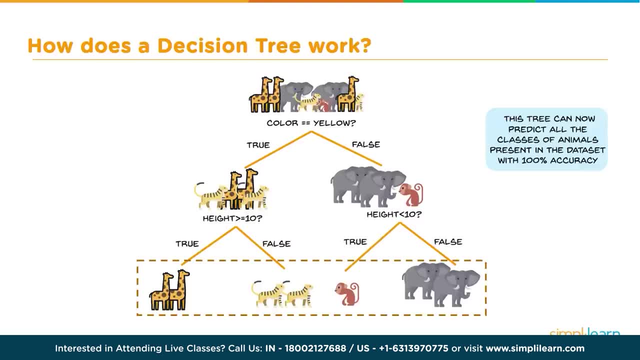 The tigers, All separated into their own groups. This tree can now predict all the classes of animals Present in the data set with 100% accuracy. That was easy Use case: Loan repayment prediction. Let's get into my favorite part. 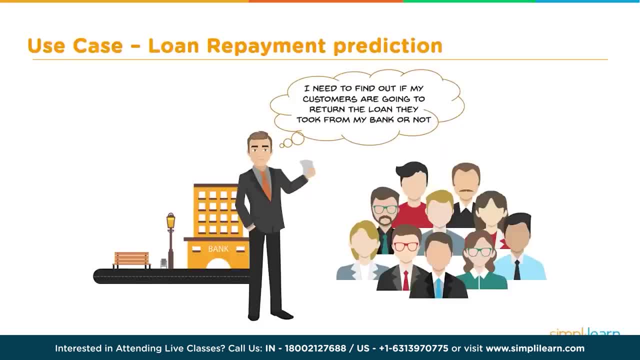 And open up some Python And see what the programming code and the scripting looks like. In here we're going to want to do a prediction And we start with this individual here Who's requesting to find out how good his customers are going to be. 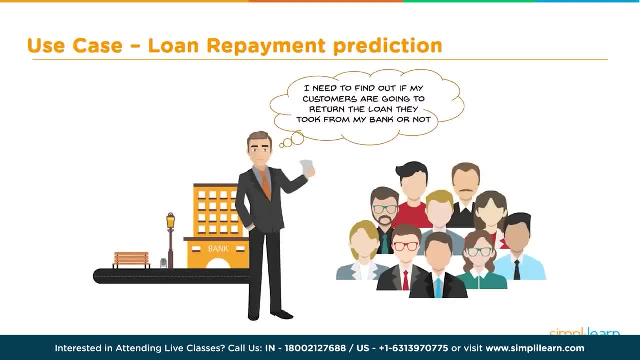 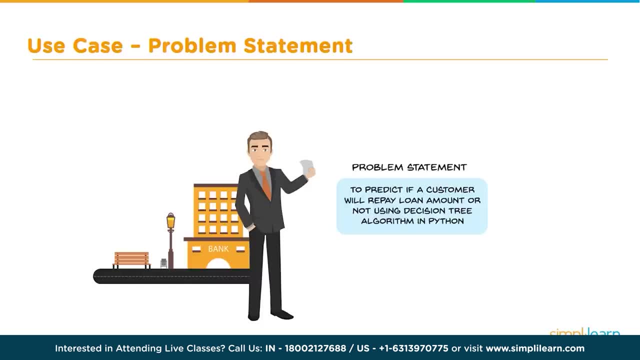 Whether they're going to repay their loan or not For his bank. We're going to generate a problem statement To predict if a customer will repay a loan amount Or not, And then we're going to be using the decision tree algorithm in Python. 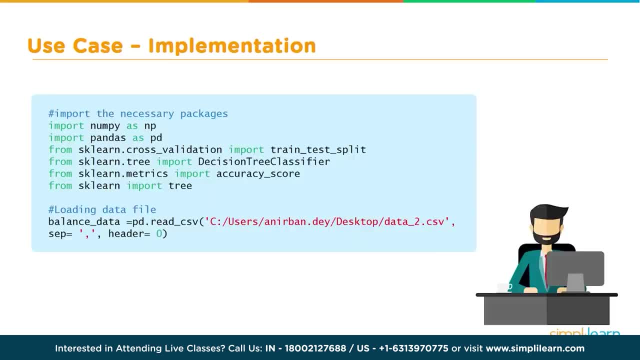 Let's see what that looks like And let's dive into the code. In our first few steps of implementation, We're going to start by importing the necessary packages That we need from Python And we're going to load up our data. 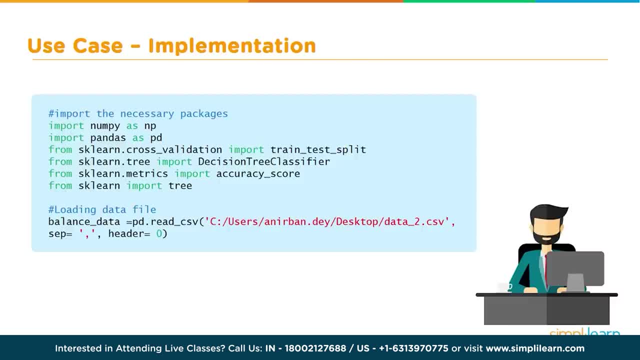 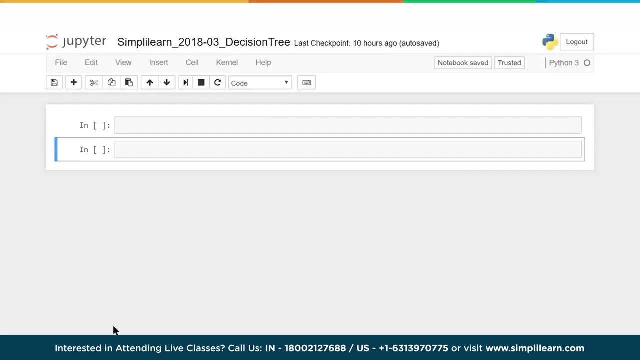 And take a look at what the data looks like. So the first thing I need Is I need something to edit my Python and run it in. So let's flip on over, And here I'm using the Anaconda Notebook. Now you can use any Python IDE you like to run it in. 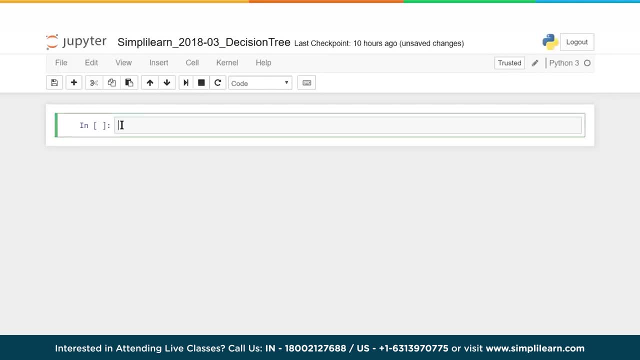 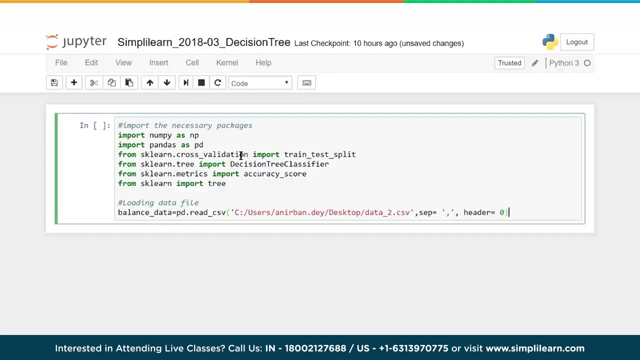 But I find the Jupyter Notebook's really nice For doing things on the fly, And let's go ahead and just paste that code in the beginning, And before we start Let's talk a little bit about what we're bringing in And then we're going to do a couple things in here. 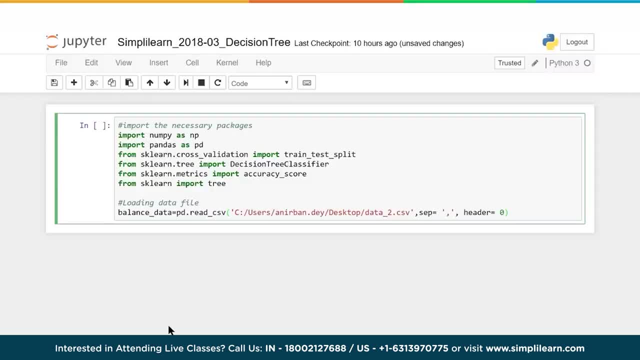 We have to make a couple changes As we go through this first part of the import. The first thing we bring in is numpy As np. That's very standard When we're dealing with mathematics, Especially with very complicated machine learning tools. 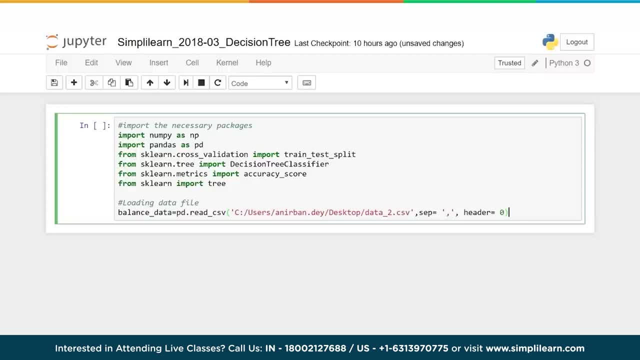 For your numbers. It's called number Python. It has your mathematics in there. In this case we actually could take it out, But generally you'll need it for most of your different things you work with, And then we're going to use pandas as pd. 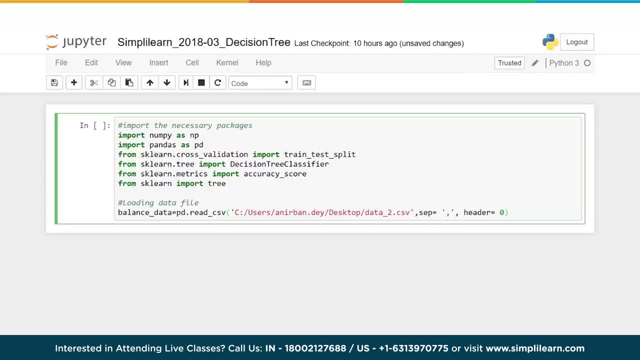 That's also a standard. The pandas is a data frame setup And you can liken this to taking your basic data And storing it in a way that looks like an Excel spreadsheet. So, as we come back to this, When you see np or pd, 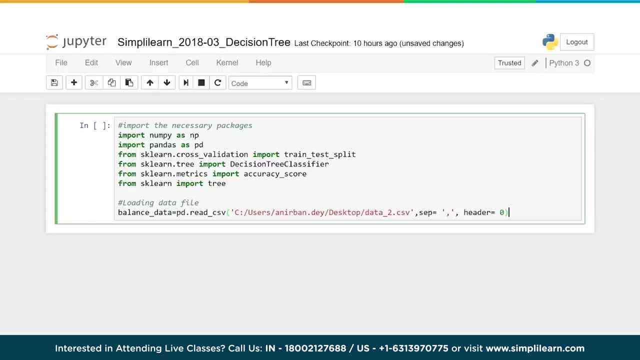 Those are very standard uses. You'll know that that's the pandas And I'll show you a little bit more. When we explore the data in just a minute, Then we're going to need to split the data. So I'm going to bring in our train, test and split. 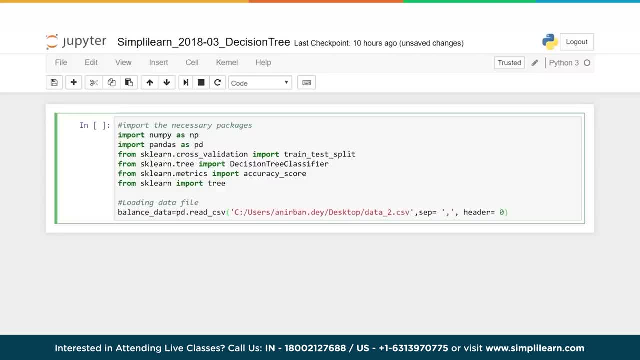 And this is coming from the sklearn Package: cross validation. In just a minute we're going to change that And we'll go over that too. And then there's also the sktree Import decision tree classifier. That's the actual tool we're using. 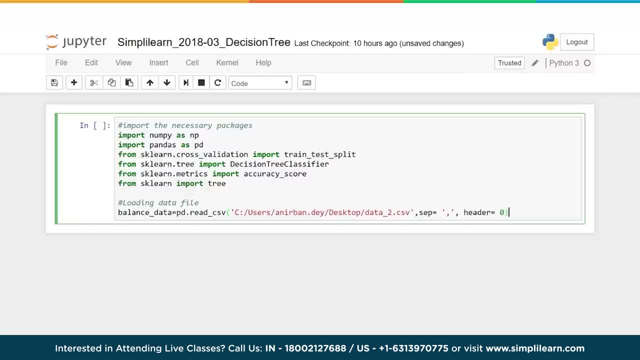 Remember, I told you don't be afraid of the mathematics, It's going to be done for you. Well, the decision tree classifier has all that mathematics in there for you, So you don't have to figure it back out again. And then we have sklearnmetrics. 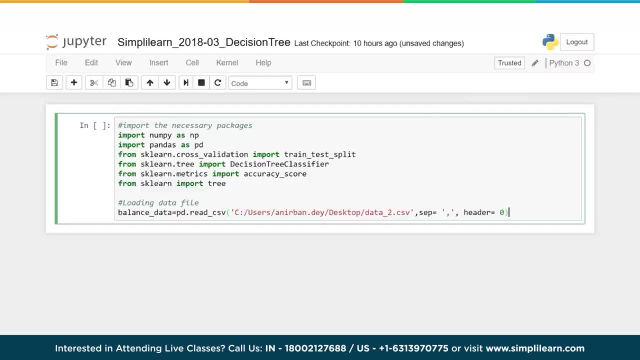 For accuracy score. We need to score our setup. That's the whole reason we're splitting it between the training and testing data. And finally, we still need the sklearnimporttree, And that's just the basic tree function That's needed for the decision tree classifier. 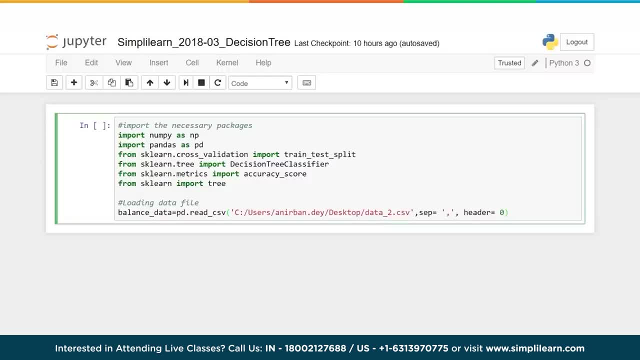 And finally, we're going to load our data down here And I'm going to run this And we're going to get two things on here: One, we're going to get an error And two, we're going to get a warning. Let's see what that looks like. 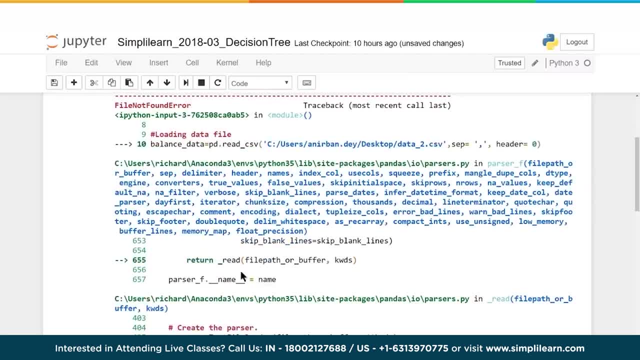 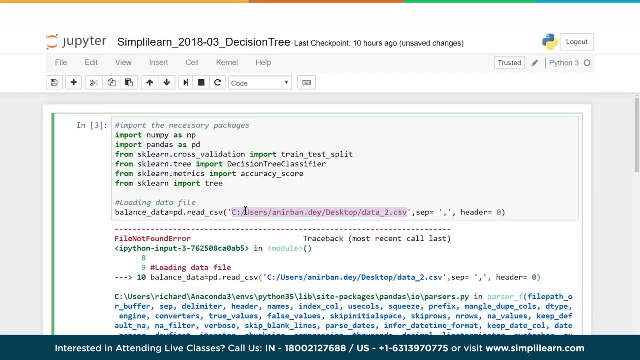 So the first thing we had is: we have an error. Why is this error here? Well, it's looking at this and says: I need to read a file, And when this was written, The person who wrote it. This is their path where they stored the file. 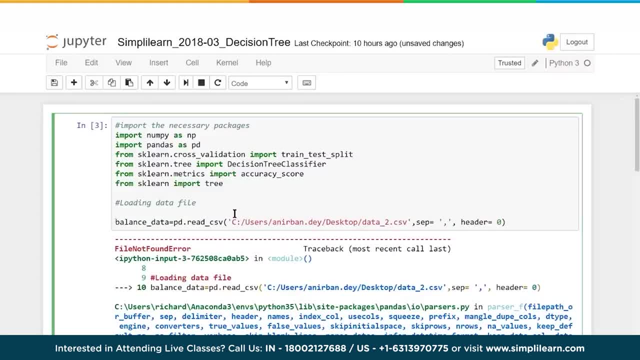 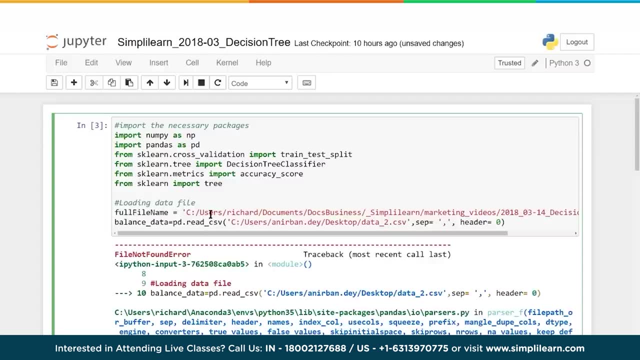 So let's go ahead and fix that, And I'm going to put in here My file path. I'm just going to call it full file name And you'll see. it's on my C drive And there's this very lengthy setup on here. 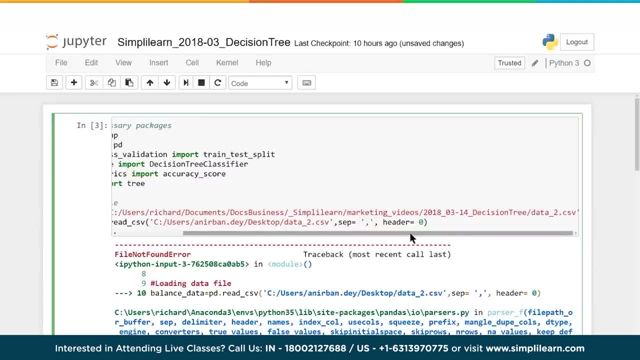 Where I stored the data2.csv file. Don't worry too much about the full path, Because on your computer it will be different. The data.2.csv file was generated And it's going to be the same- Generated by simply learn. 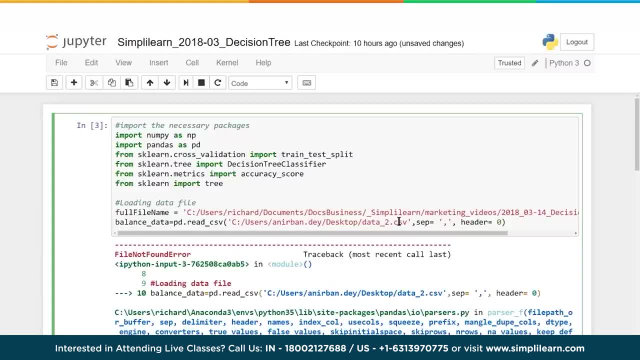 If you want a copy of that, You can comment down below And request it here in the YouTube, And then, if I'm going to give it a name- Full file name- I'm going to go ahead and change it here To full. 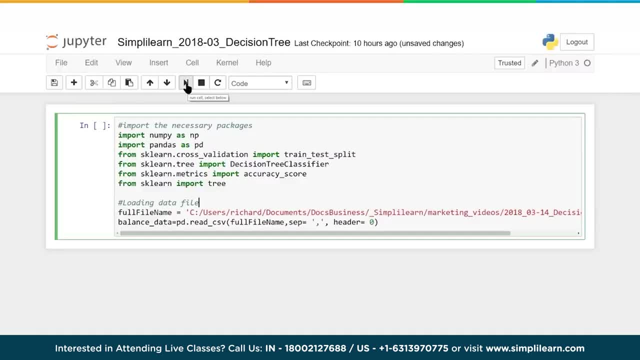 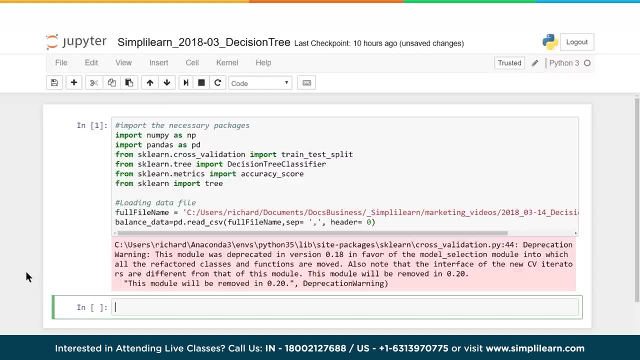 File name. So let's go ahead and run it now And see what happens. And we get a warning. When you're coding, Understanding these different warnings And these different errors that come up Is probably the hardest lesson to learn. So let's just go ahead and take a look at this. 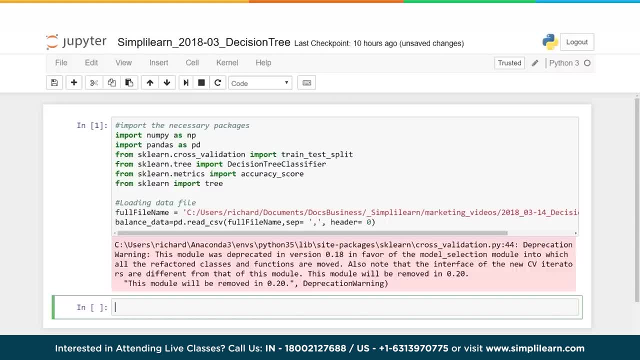 And use this as an opportunity To understand what's going on here. If you read the warning, It says the cross validation Is depreciated. So it's a warning on it's being removed And it's going to be moved in favor. 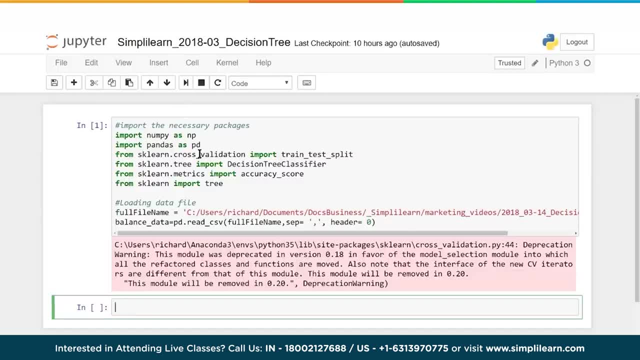 Of the model selection. So if we go up here To sklearn dot cross validation And if you research this And go to the sklearn site, You'll find out that you can actually just swap it right in there With model selection. And so when I come in here, 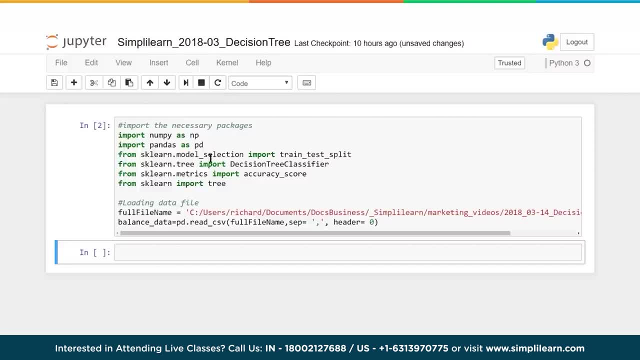 And I run it again: That removes a warning. What they've done Is they've had two different developers Develop it in two different branches And then they decided to keep one of those And eventually get rid of the other one. That's all that is. 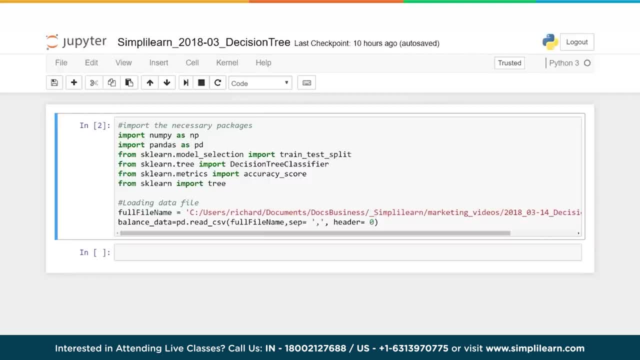 And very easy and quick to fix. Before we go any further, I went ahead and opened up the data From this file. Remember the data file we just loaded on here, The data underscore two dot csv. Let's talk a little bit more about that. 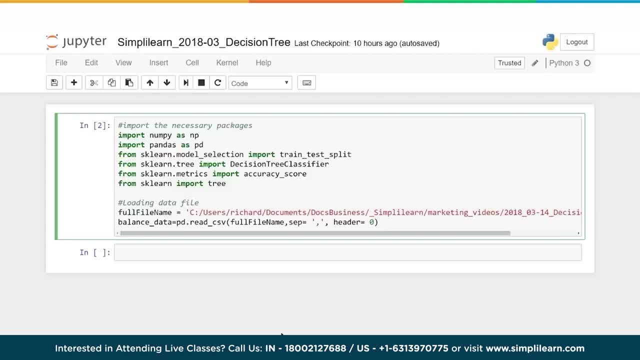 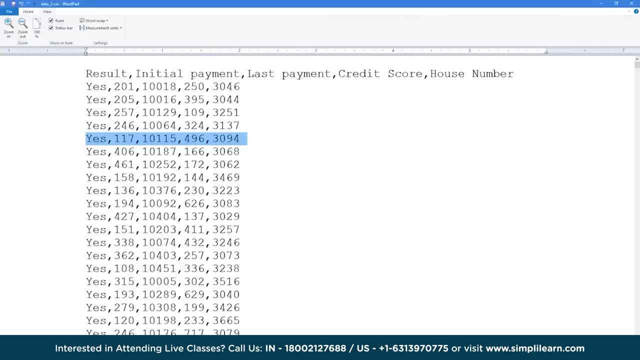 And see what that looks like Both as a text file- Because it's a comma separated variable file- And in a spreadsheet. This is what it looks like as a basic text file. You can see at the top they've created a header. 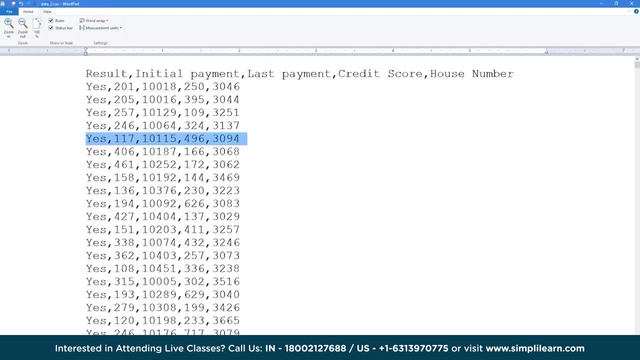 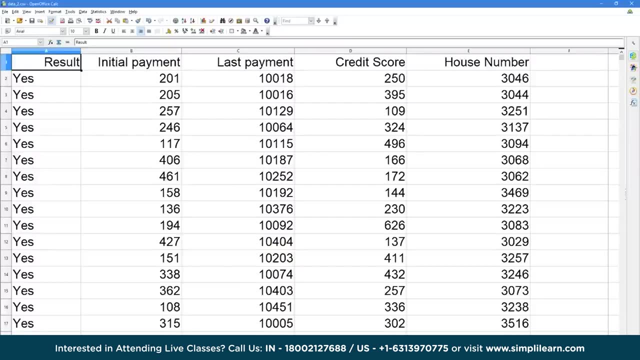 And it's got one, two, three, four, five columns And each column has data in it. And let me flip this over. Let's look at this in an actual spreadsheet So you can see what that looks like. And here I've opened it up in the open office: calc. 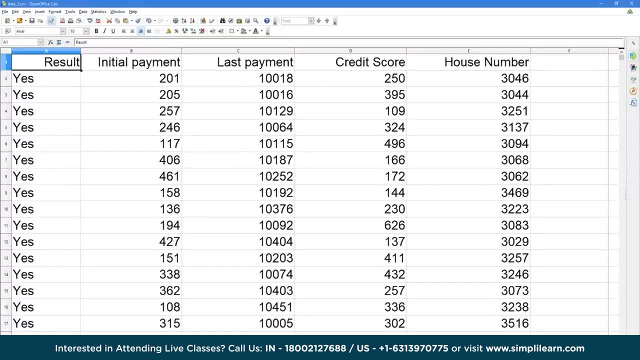 Which is pretty much the same as excel, And zoomed in And you can see we've got our columns And our rows of data A little easier to read. in here We have a result. Yes, yes, no, We have initial payment. 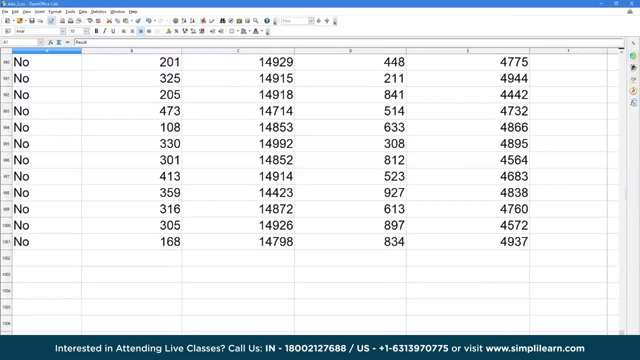 Last payment Credit score House number If we scroll way down, The first one being a column And then one thousand lines of data. Now, as a programmer, If you're looking at a small amount of data, I usually start by pulling it up in different sources. 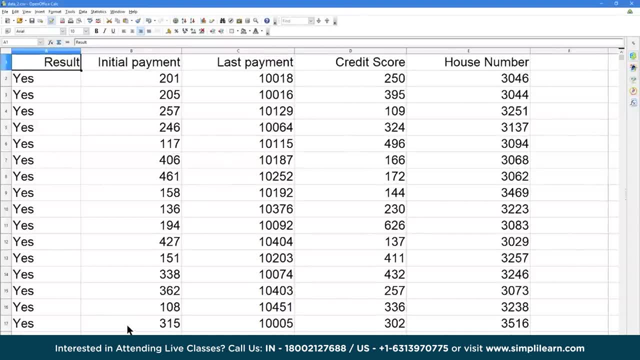 So I can see what I'm working with, But in larger data you won't have that option. It would just be too large. So you need to either bring in a small amount That you can look at it like we're doing right now. 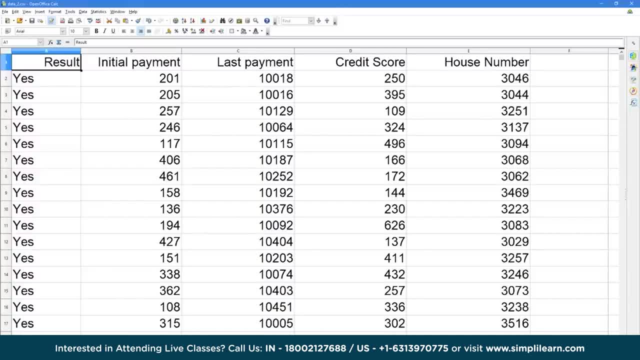 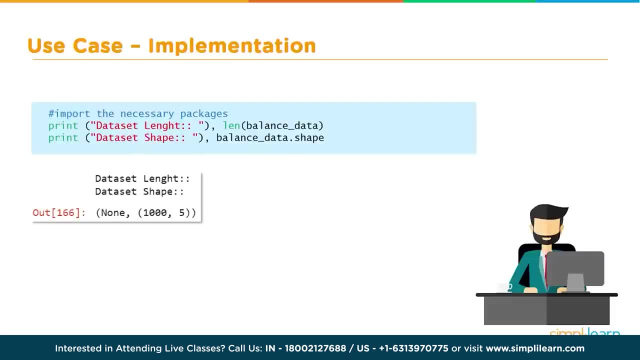 Or we can start looking at it through the python code. So let's go ahead and move on And take the next couple of steps To explore the data using python. Let's go ahead And see what it looks like in python To print the length and the shape of the data. 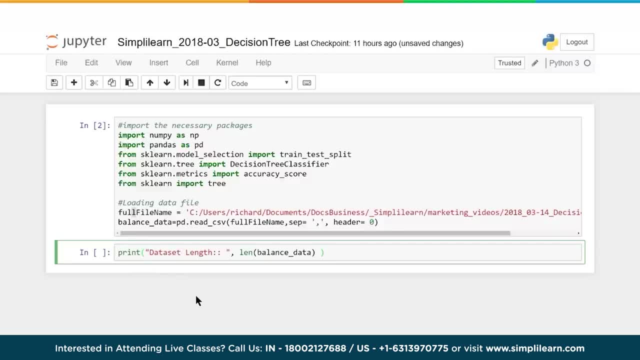 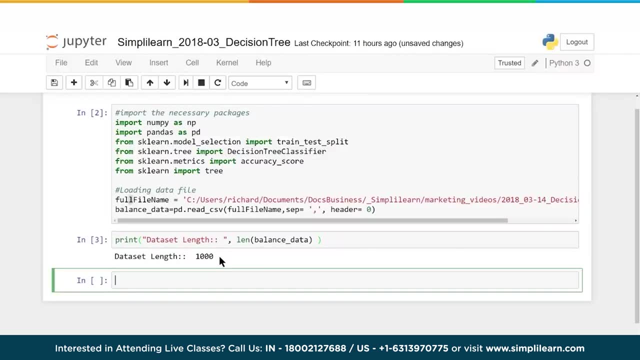 So let's start By printing the length of the database. We can use a simple lin function from python, And when I run this, You'll see that it's a thousand long, And that's what we expected. There's a thousand lines of data in there. 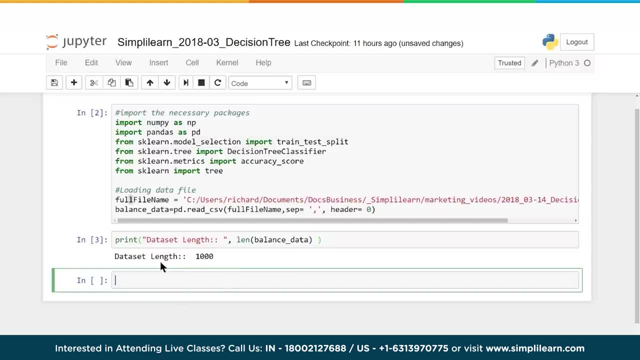 If you subtract the column head- This is one of the nice things When we did the balance data From the panda, read You'll see that the header is row zero, So it automatically removes a row And then shows the data separate. 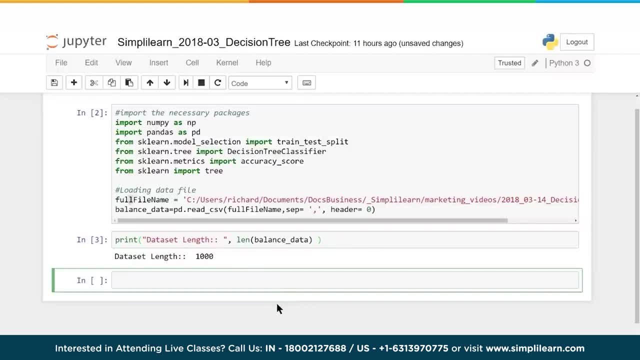 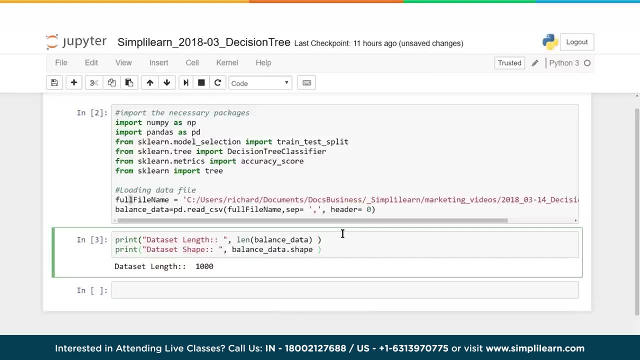 It does a good job sorting that data out for us, And then we can use a different function. Let's take a look at that And again, we're going to utilize the tools in panda And since the balance underscore data Was loaded as a panda data frame, 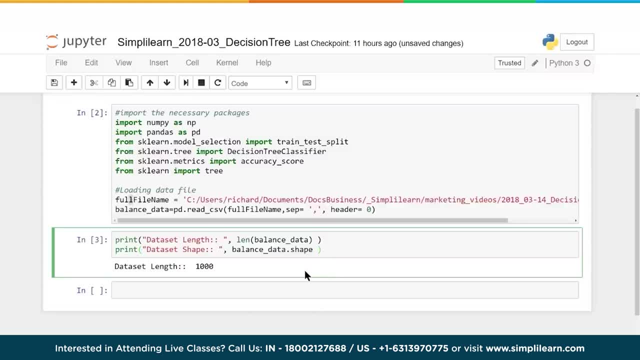 We can do a shape on it. And let's go ahead and run the shape And see what that looks like. And since the balance underscore data Was loaded as a panda data frame, We can do a shape on it. What's nice about the shape? 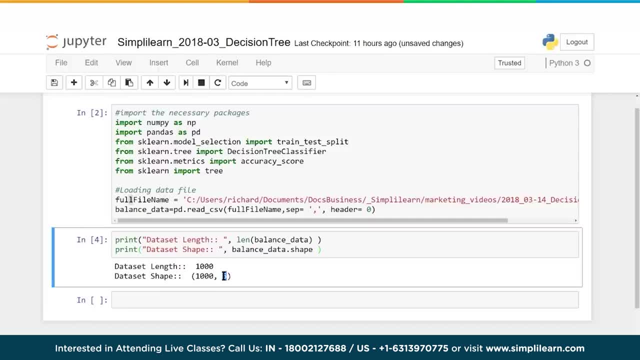 Is not only does it give me the length of the data- We have a thousand lines- It also tells me there's five columns. So when we were looking at the data, We had five columns of data. And then let's take one more step. 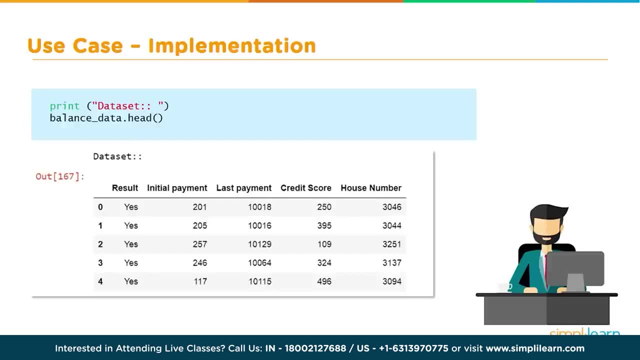 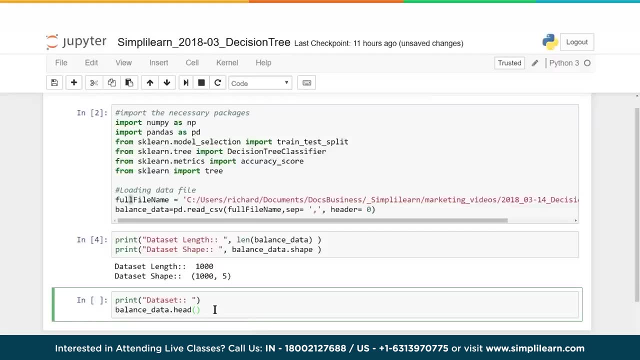 To explore the data using python, And now that we've taken a look at the length And the shape, Let's go ahead and use the pandas module for head- Another beautiful thing in the data set That we can utilize. So let's put that on our sheet here. 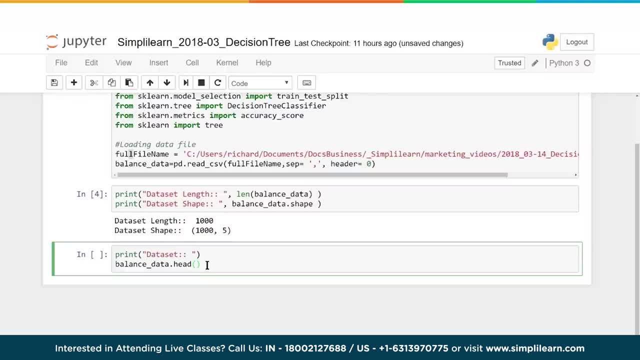 And we have print data set Head And this is a pandas print statement of its own, So it has its own print feature in there. And then we went ahead and gave a label For our print job here of data set, Just a simple print statement. 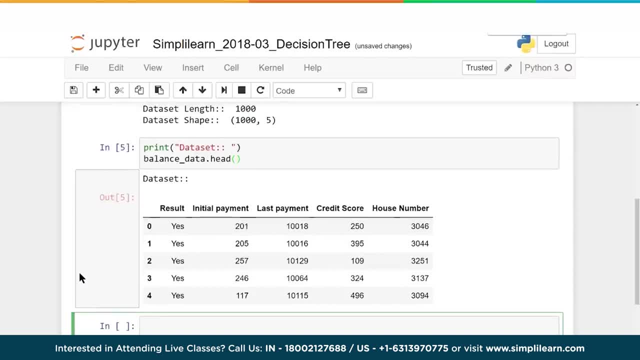 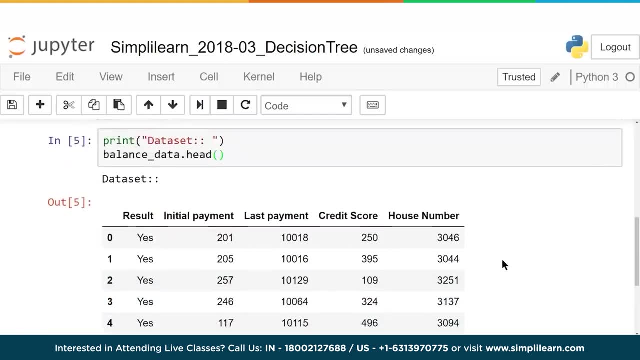 And when we run that, Let's just take a closer look at that. Let me zoom in here. There we go. Pandas does such a wonderful job Of making this a very clean, Readable data set. So you can look at the data. 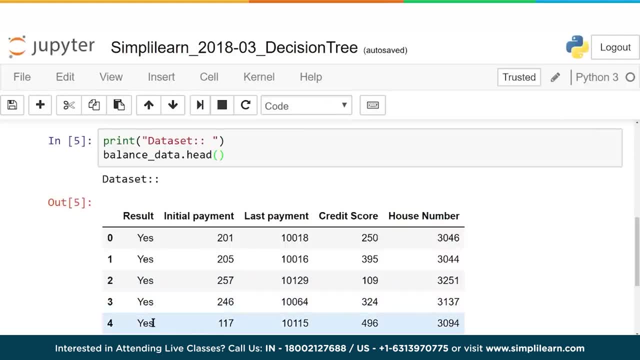 So you can have it. When you put it as the head, It prints the first five lines of the data And we always start with zero. So we have five lines. We have zero. one, two, three, four Instead of one, two, three, four, five. 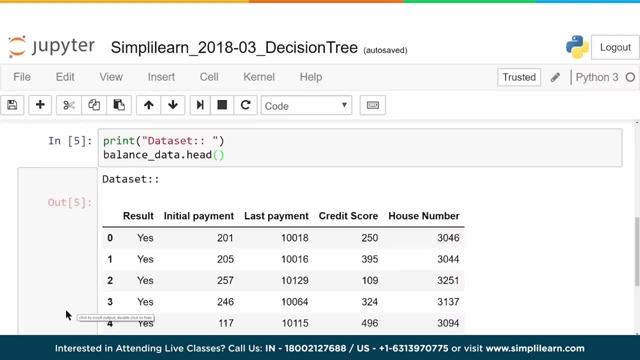 That's a standard scripting and programming set As you want to start with the zero position, And that is what the data head does. It pulls the first five rows of data, Puts it in a nice format that you can look at And view. 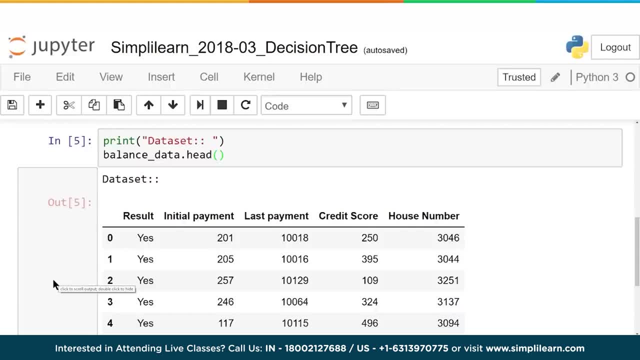 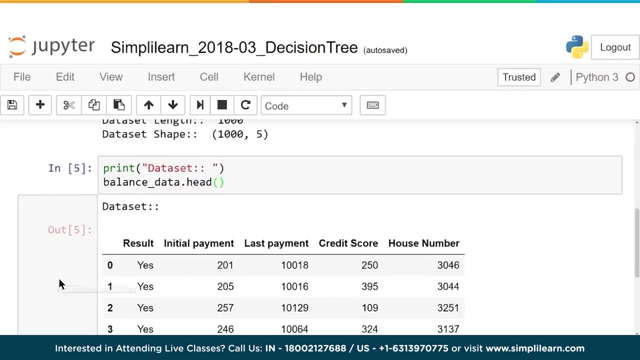 Very powerful tool to view the data. So instead of having to flip and open up an excel spreadsheet Or trying to look at a word doc Where it's all scrunched together And hard to read, You can now get a nice open view of what you're working with. 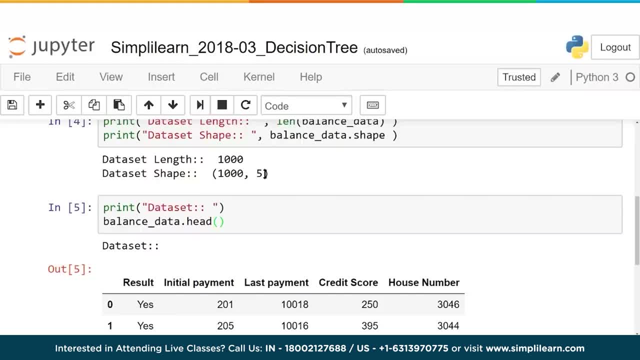 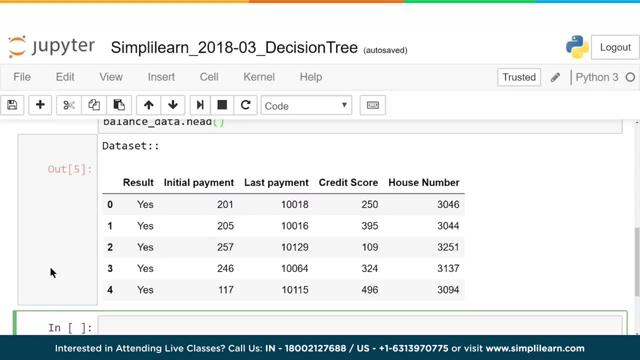 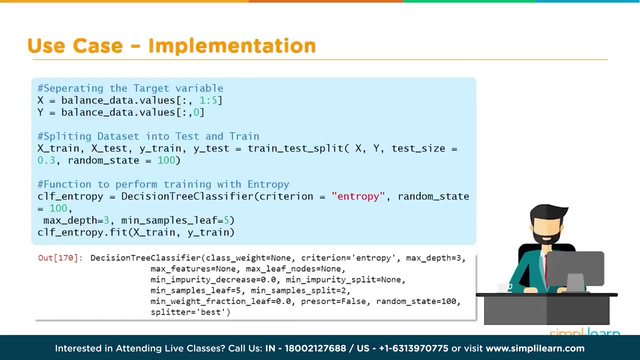 We're working with a shape of a thousand long, Five wide, So we have five columns And we do the full data head. You can actually see what this data looks like: The initial payment, Last payment, Credit scores, House number. 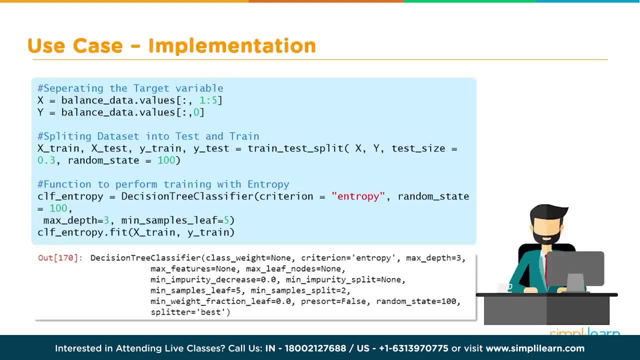 So let's take this, Now that we've explored the data- And to do that We need to first Separate the data out- We're going to separate it into two groups So that we have something to actually train the data with. 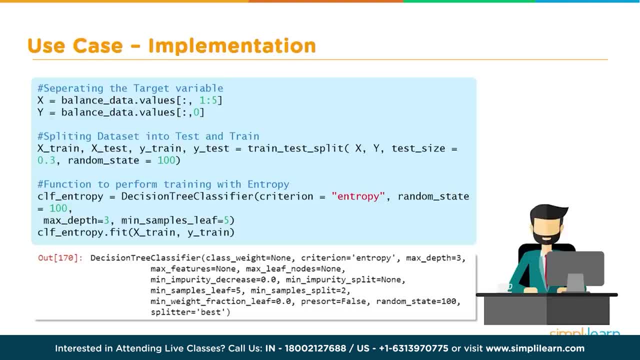 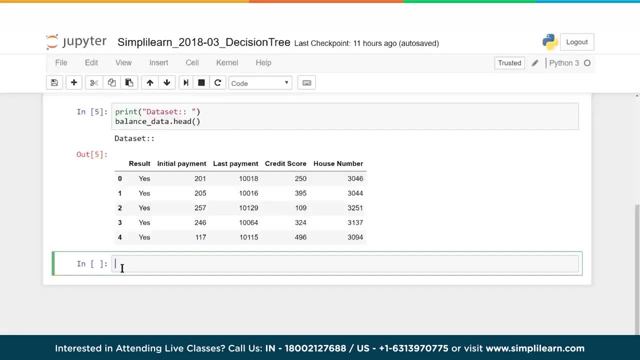 And then we have some data on the side to test it, To see how good our model is. Remember, with any of the machine learning, You always want to have some kind of test set To weigh it against. So you know how good your model is. 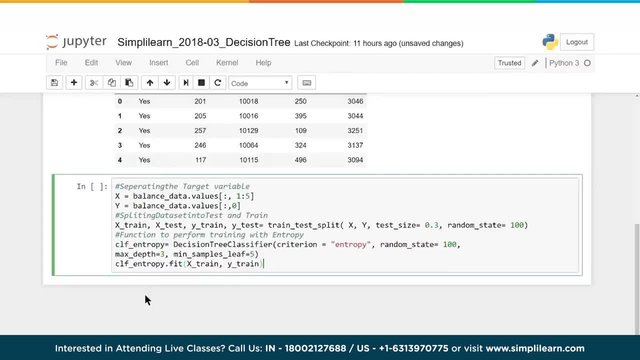 When you distribute it. Let's go ahead and break this code down And look at it in pieces. So first we have our X and Y. X is going to be our data And Y is going to be the answer Or the target. 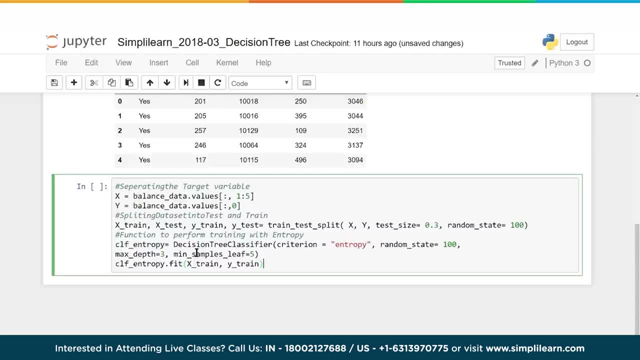 You can look at it as source and target. In this case, we're using X and Y to denote the data in And the data that we're actually trying to guess what the answer is going to be, And so to separate it, We can simply put in: 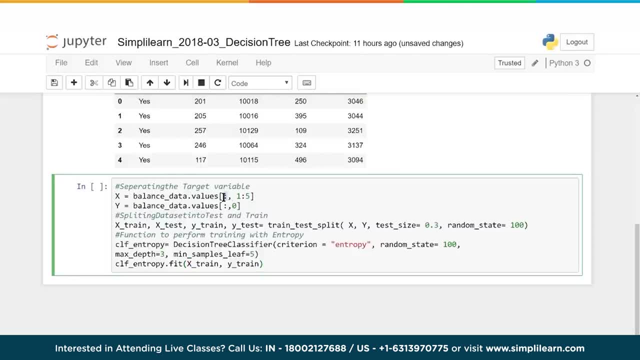 X equals the balance of the data. dot values. The first brackets Means that we're going to select all the lines In the database, So it's all the data, And the second one says We're only going to look at columns one through five. 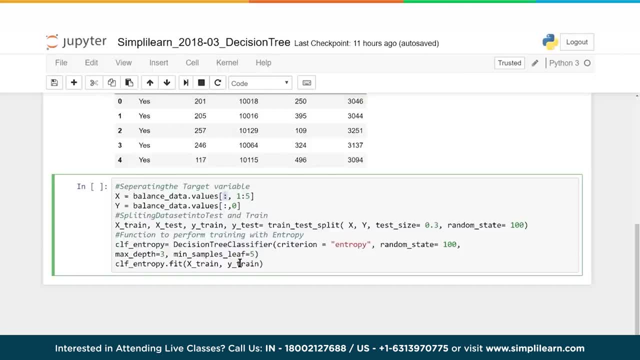 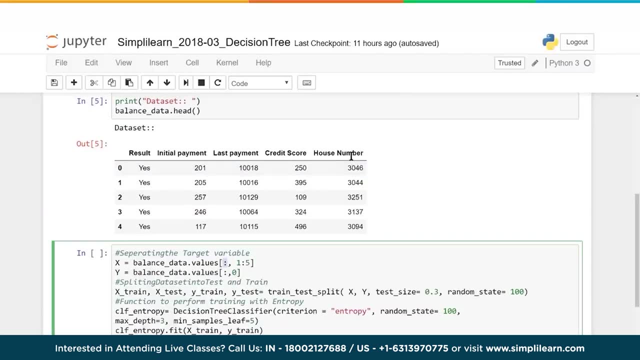 Remember, we always start with zero. Zero is a yes or no And that's whether the loan went default or not. So we want to start with one. If we go back up here, That's the initial payment And it goes all the way through the house number. 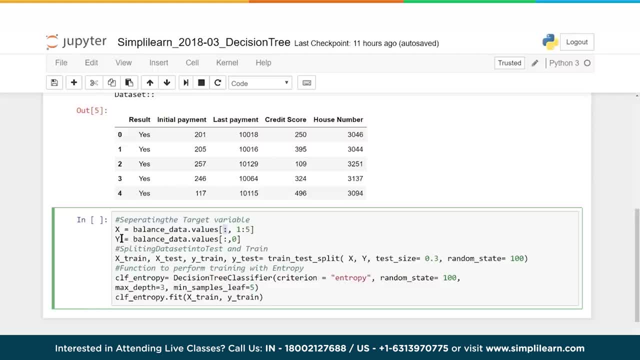 Well, if we want to look at one through five, We can do the same thing for Y, Which is the answers, And we're going to set that just equal to the zero row. So it's just the zero row, And then it's all rows going in there. 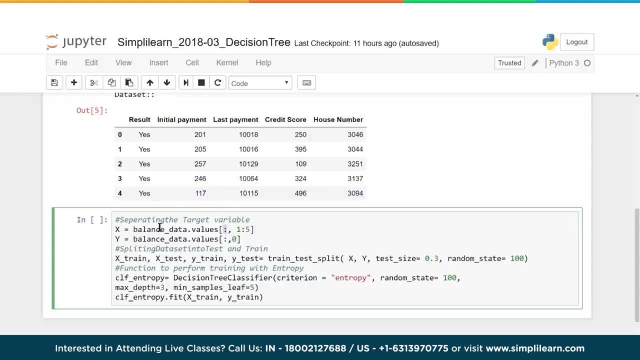 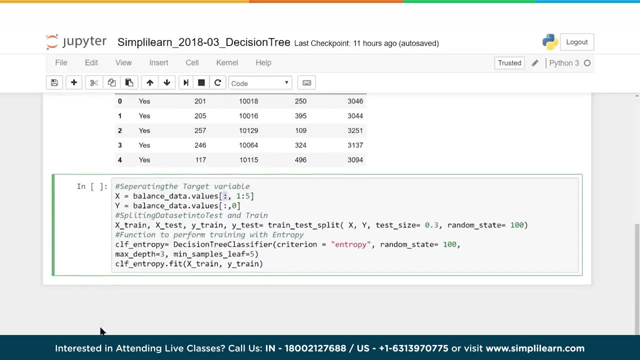 So now we've divided this into Two different data sets, One of them with the Data going in And one with the answers. Next We need to split the data, And here You'll see that we have it split into. 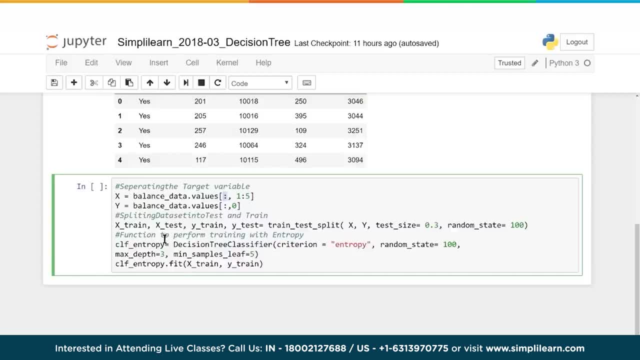 Four different parts. The first one is your X training, Your X test. Your Y train, Your Y test. Simply put, We have X going in Where we're going to train it, And then we have X test Where we're going to test that data. 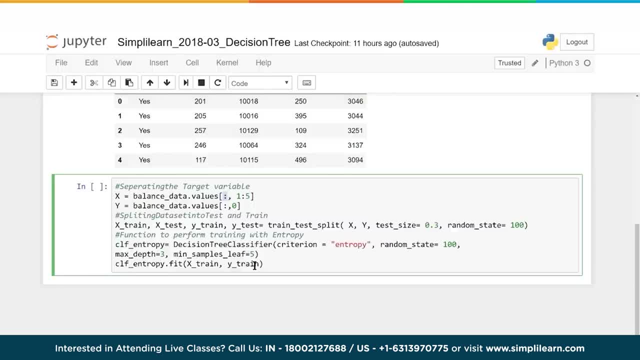 And we have to know in the end What the Y was supposed to be. And that's where this train test split comes in. That we loaded earlier in the modules. This does it all for us And you can see. they set the test size equal to point three. 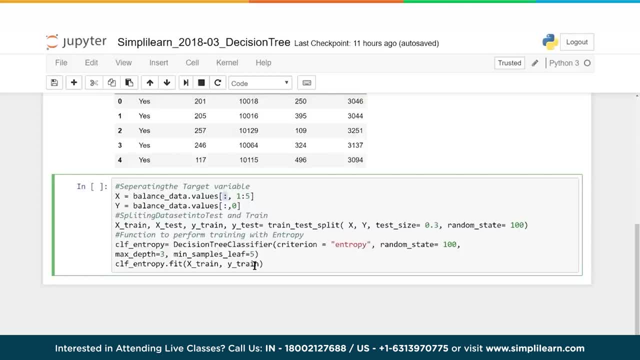 So that's roughly thirty percent Will be used in the test. And then we use a random state, So it's completely random which rows it takes out of there, And then finally we get to actually build our decision tree, And they've called it here. 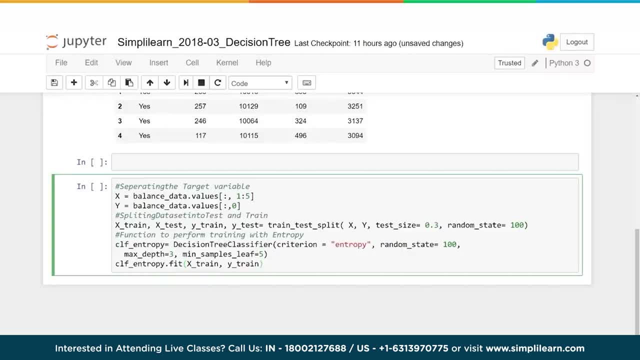 CLF underscore entropy. That's the actual decision tree Or decision tree classifier, And in here they've added a couple variables Which we'll explore in just a minute, And then, finally, We need to fit the data to that. So we take our CLF entropy. 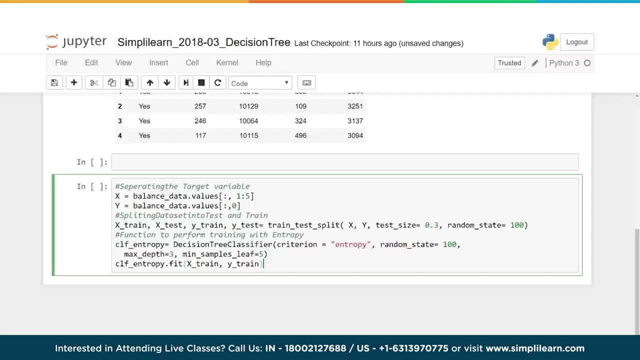 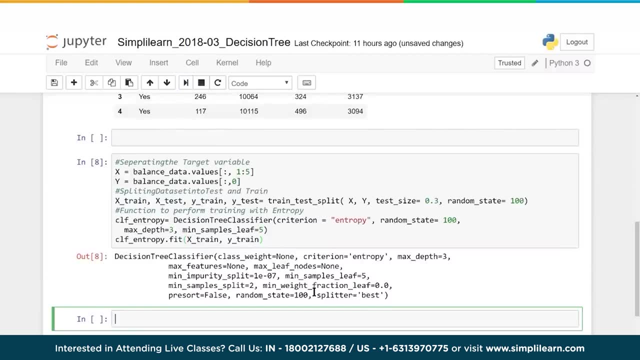 That we created And we fit the X train And since we know the answers for X train are the Y train, We go ahead and put those in And let's go ahead and run this And what most of these sklearn modules do. 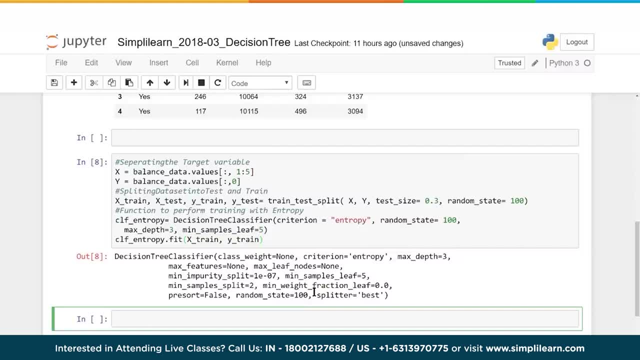 Is when you set up the variable- In this case we set the CLF entropy- It automatically prints out what's in that decision tree. There's a lot of variables you can play with in here And it's quite beyond the scope of this tutorial. 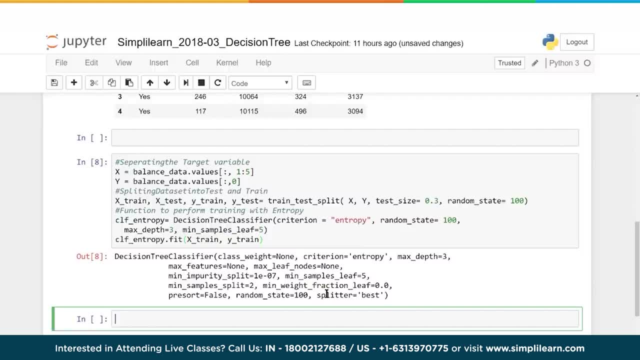 To go through all of these and how they work. But we're working on entropy. That's one of the options. We've added that it's completely a random state Of 100.. So 100 percent And we have a max depth of 3.. 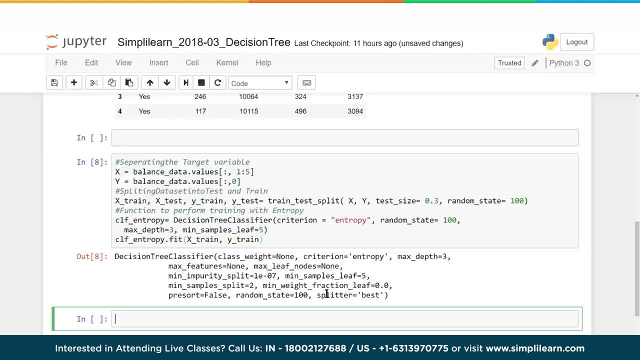 Now the max depth. if you remember above When we were doing the different graphs of animals, Means, it's only going to go down 3 layers Before it stops And then we have minimal samples of leaves, So it's going to have at least 5 leaves at the end. 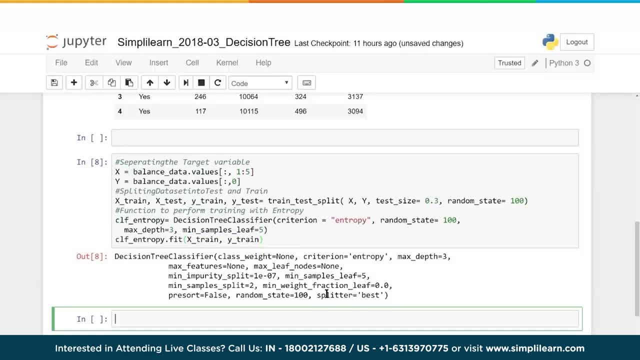 So we'll have at least 3 splits, We'll have no more than 3 layers And at least 5 end leaves, With the final result at the bottom, Now that we've created Our decision tree Classifier, Not only created it, but trained it. 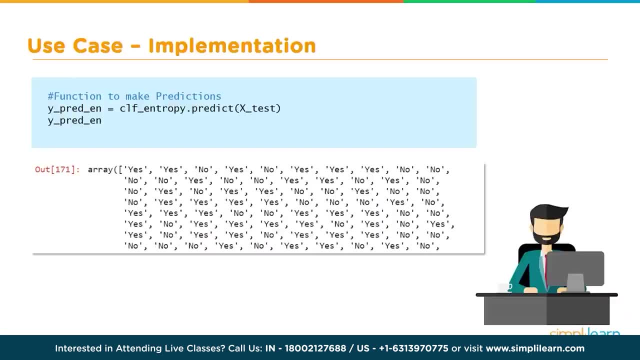 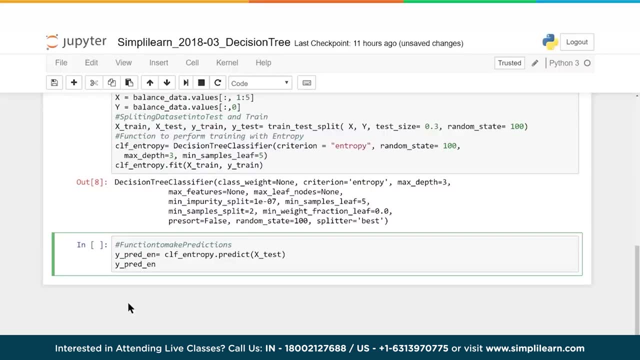 Let's go ahead and apply it and see what that looks like. So let's go ahead and make a prediction And see what that looks like. We're going to paste our predict code in here And before we run it, Let's just take a quick look at what it's doing here. 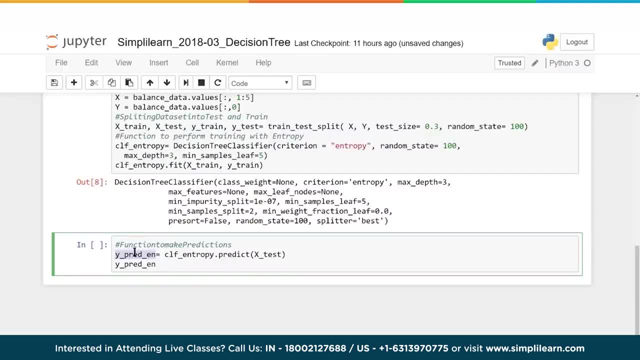 We have a variable ypredict That we're going to do And we're going to use our Variable clfentropy that we created And then you'll see predict And it's very common in the sklearn modules That their different tools 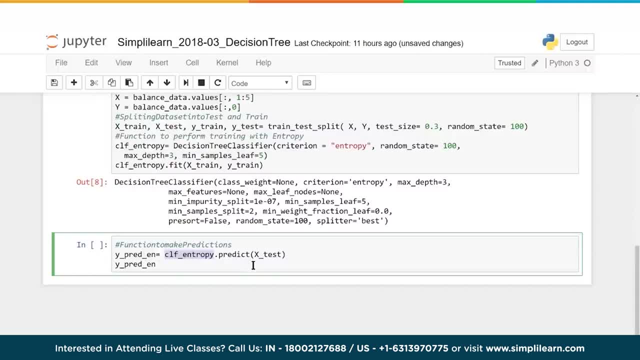 Have the predict When you're actually running a prediction. In this case, we're going to put our xtestdata in here. Now, if you delivered this for use- An actual commercial use- And distributed it, You'll see the new loans you're putting in here to guess. 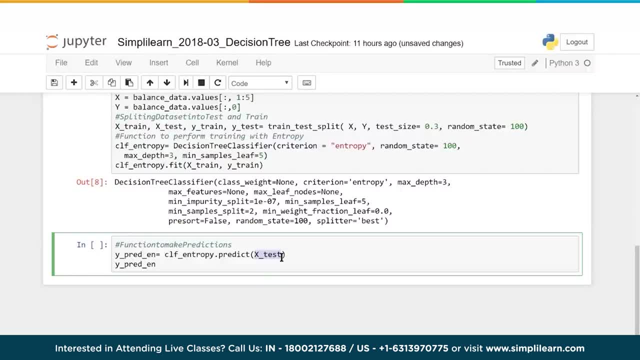 Whether the person's going to be Pay them back or not. In this case, though, We need to test out the data And just see how good our sample is, How good of our tree does at predicting the loan payments And, finally, since anaconda. 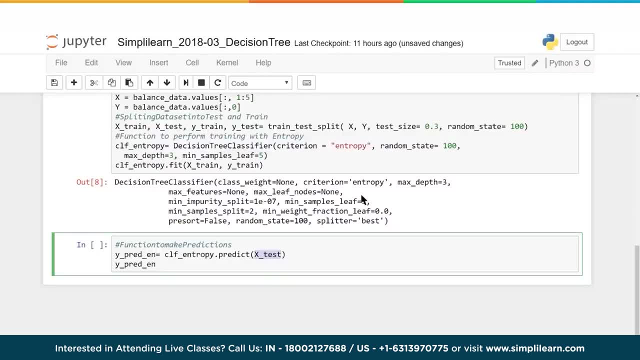 Jupyter notebook Works as a command line for python. We can simply put the ypredicten to print it. I could just as easily Have put the print And put brackets around ypredicten to print it out And do that. 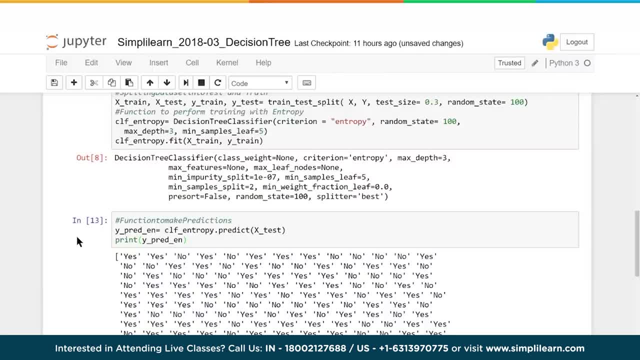 It doesn't matter which way you do it And you'll see right here that it runs a prediction. This is roughly 300 in here. Remember it's 30% of 1000.. So you should have about 300 answers in here. 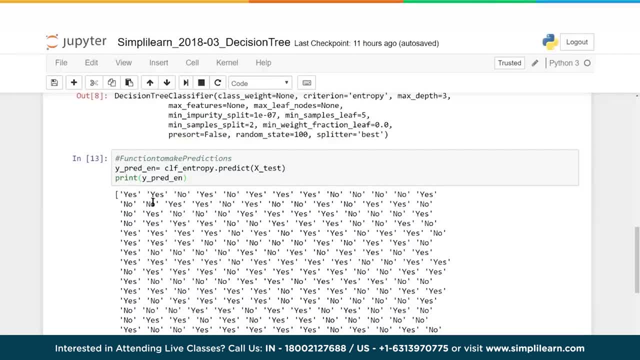 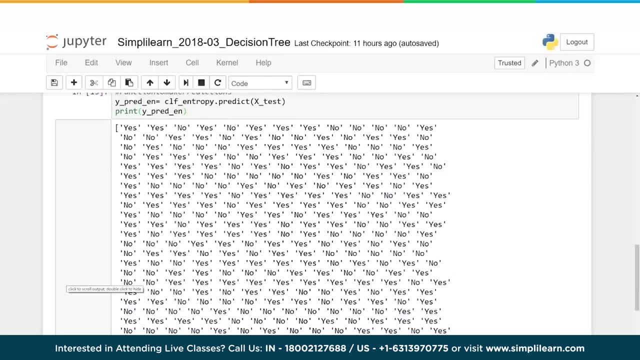 And this tells you Which each one of those lines of our Test went in there, And this is what our ypredict came out. So let's move on to the next step. We're going to take this data And try to figure out just how good a model we have. 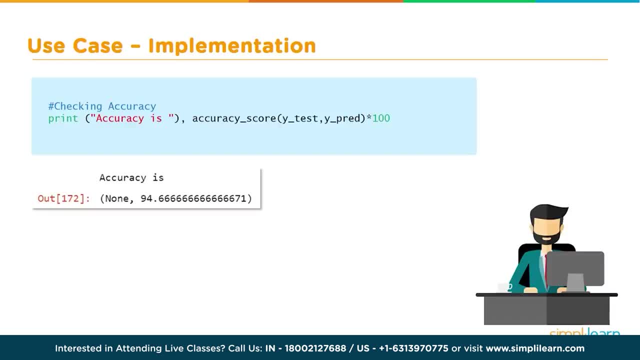 So here we go. since sklearn Does all the heavy lifting for you And all the math, We have a simple line of code To let us know what the accuracy is, And let's go ahead and go through that And see what that means and what that looks like. 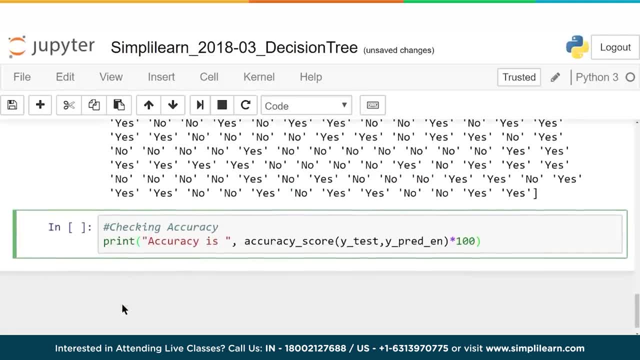 Let's go ahead and paste this in And let me zoom in a little bit. There we go, See, we have a nice full picture And we'll see. here we're just going to do a print. accuracy is, And then we do the accuracy score. 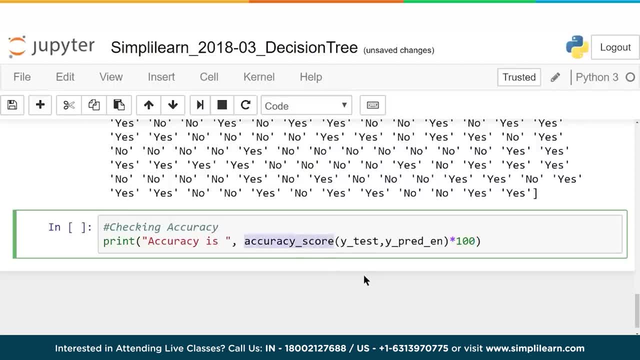 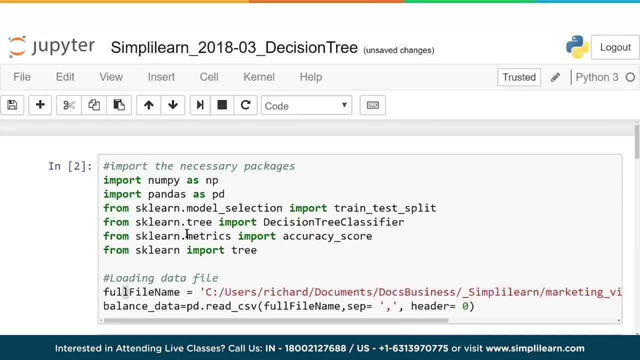 And this was something we imported earlier, If you remember, at the very beginning. Let me just scroll up there real quick So you can see where that's coming from. That's coming from here, down here, From sklearnmetrics Import accuracy score. 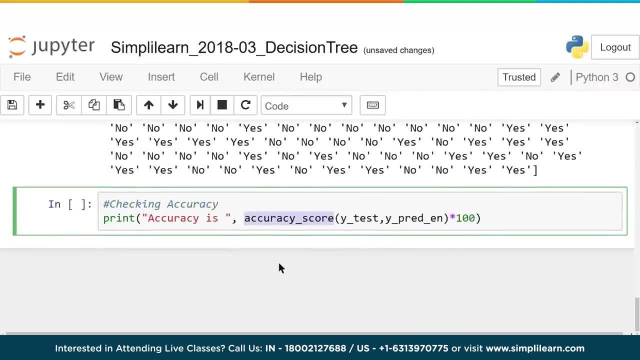 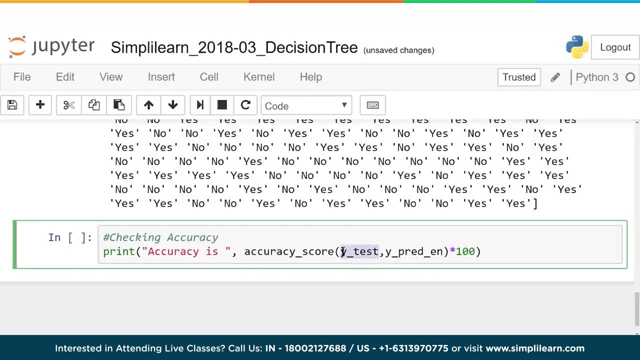 And you could probably run a script, Make your own script to do this very easily. How accurate is it? How many out of 300 do we get right? And so we put in our y test. That's the one we ran the predict on. 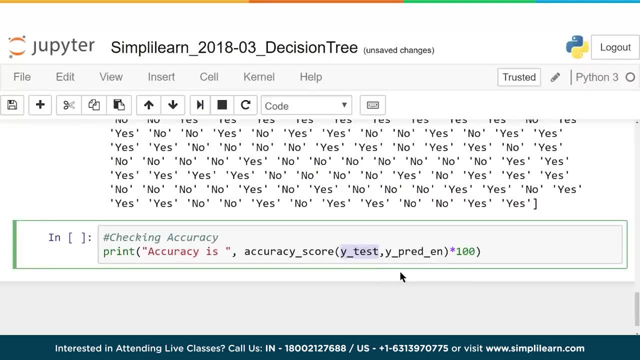 And then we put in our y predict en. That's the answers we got, And we're just going to multiply that by 100. Because this is just going to give us an answer as a decimal And we want to see it as a percentage. 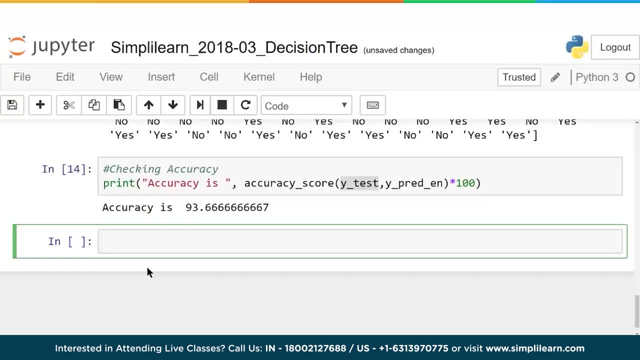 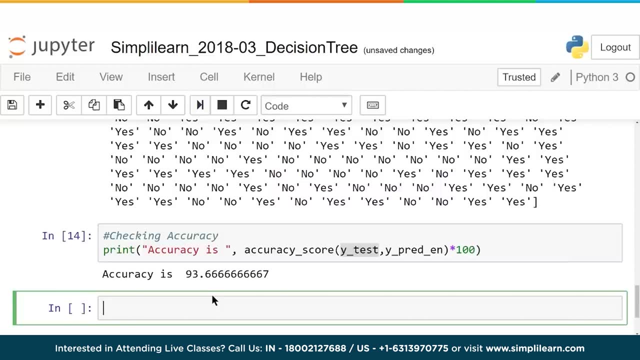 And let's run that, Let's see what it looks like And if you see, here We got an accuracy of 93.66667.. So when we look at the number of loans And we look at how good our model fit, 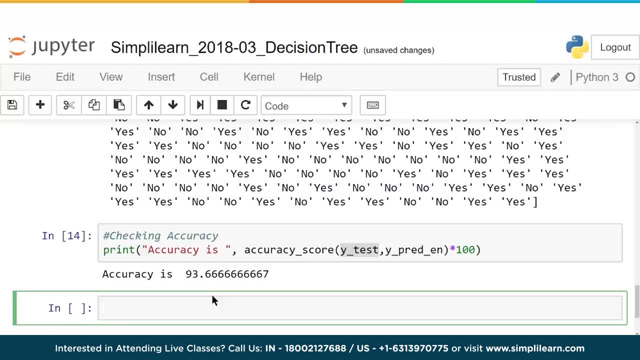 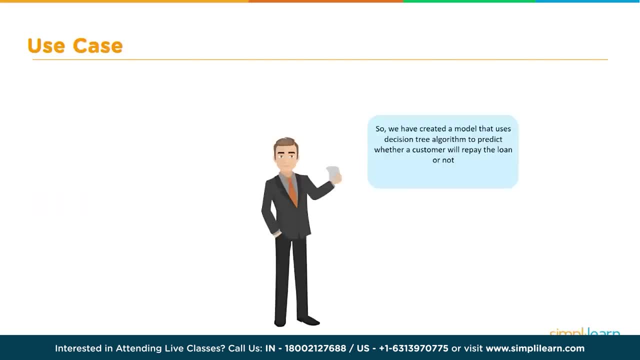 We can tell people It has about a 93.6 fitting to it. So just a quick recap on that. We now have accuracy set up on here, And so we have created a model That uses the decision tree algorithm To predict whether a customer will repay the loan or not. 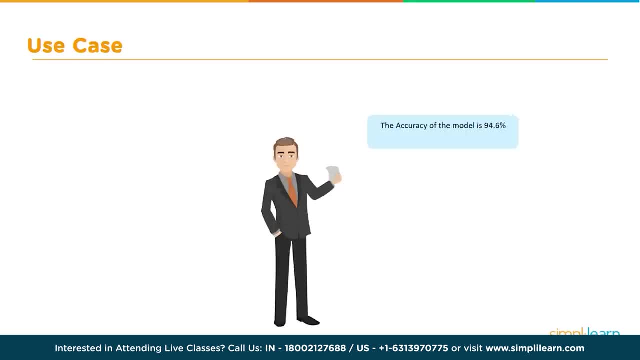 The accuracy of the model is about 94.6%. The best way to do that Is to use the decision tree, And the bank can now use this model To decide whether it should approve the loan request From a particular customer or not. 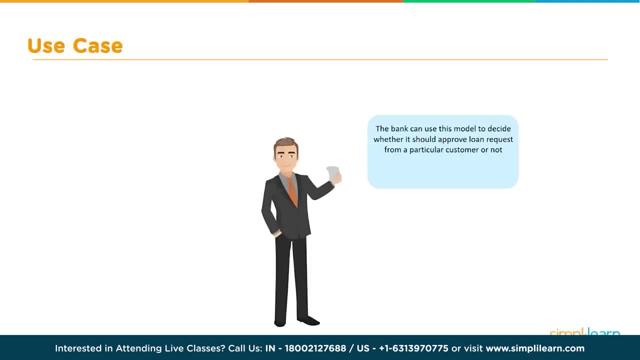 And so this information is really powerful. We may not be able to, as individuals, Understand all these numbers, Because they have thousands of numbers that come in, But you can see that this is a smart decision for the bank To use a tool like this. 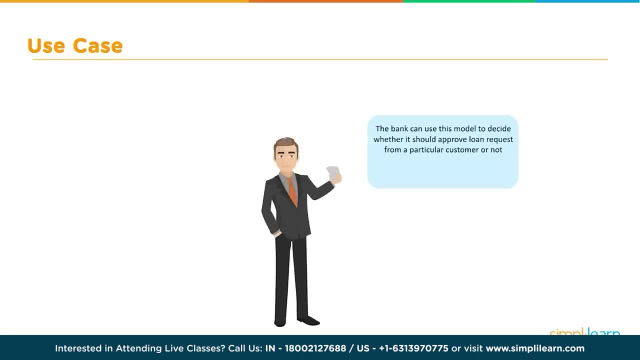 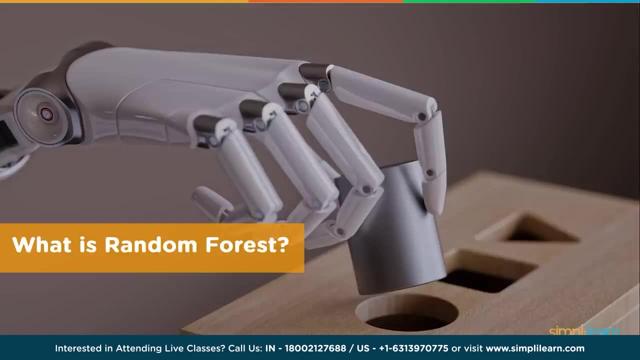 To help them to predict how good their profit is going to be Off of the loan balances And how many are going to default or not. Let us dig deep into the theory Of exactly how it works And let's look at What is random: forest. 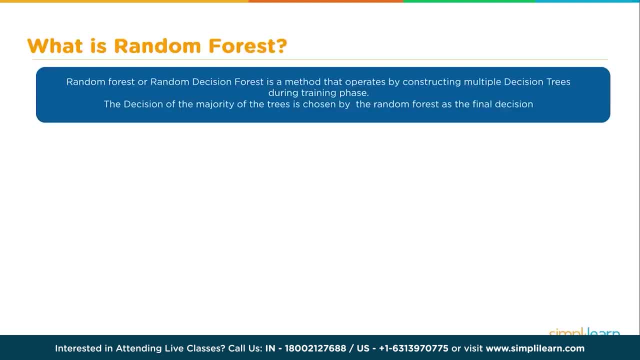 Random forest Or random decision forest Is a method that operates By constructing multiple decision trees. The decision of the majority of the trees Is chosen by the random forest As the final decision- And we have some nice graphics here- We have a decision tree. 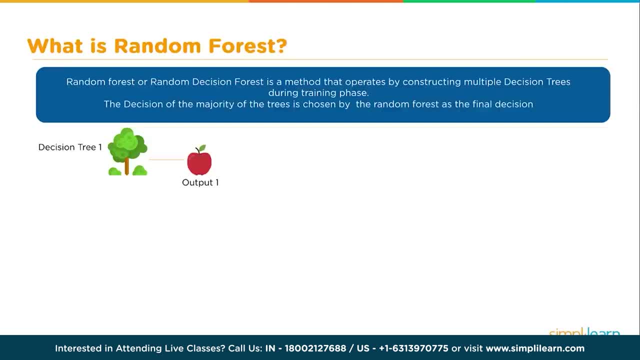 And they actually use a real tree to denote the decision tree, Which I love, And, given a random, some kind of picture of a fruit, This decision tree decides that the output is an apple. And we have a decision tree too, Where we have that picture of the fruit goes in. 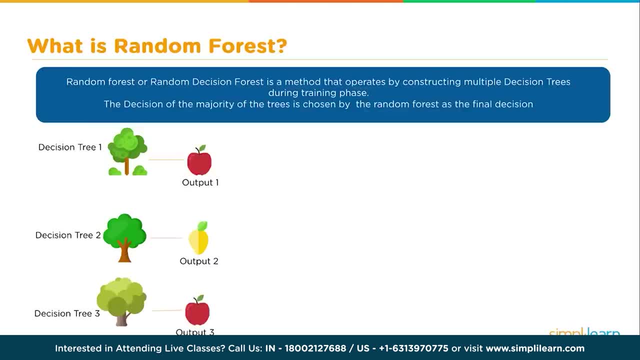 And this one decides that it is a lemon, And the decision tree gets another image And it decides it is an apple, And then this all comes together in what they call the random forest. And this random forest Then looks at it and says: 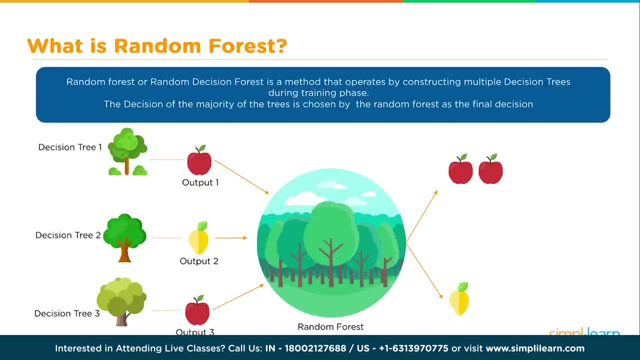 Okay, I got two votes for apple, One vote for lemon. The majority is apples, So the final decision is apples. To understand how the random forest works, We first need to dig a little deeper And take a look at the random forest. 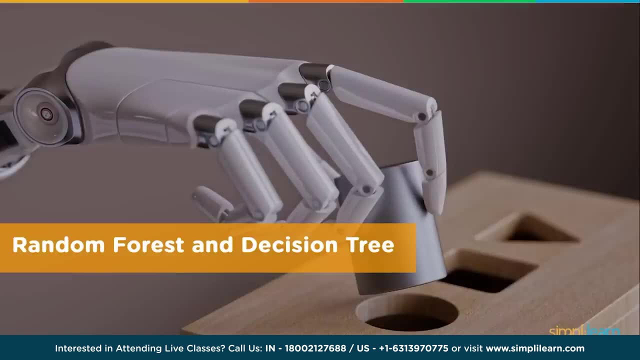 And the actual decision tree And see how it builds that decision tree. In looking closer at how the individual decision trees work, We will go ahead and continue to use the fruit example, Since we are talking about trees and forests. A decision tree is a tree shaped diagram. 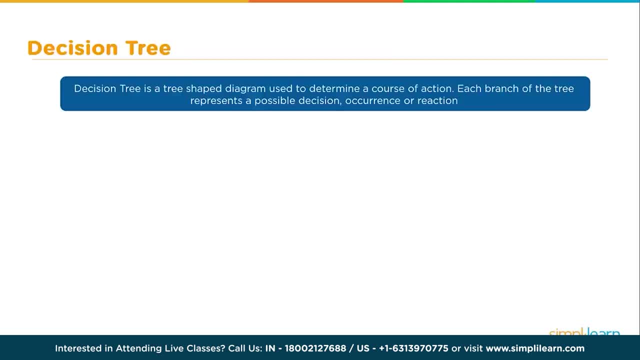 Used to determine a course of action. Each branch of the tree represents a possible decision, Occurrence or reaction. So in here we have a bowl of fruit And if you look at that, It looks like they switched from lemons to oranges. 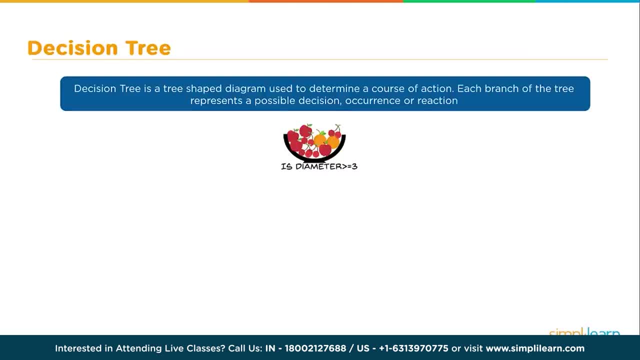 So we have oranges, cherries and apples, And the first decision of the decision tree Might be a decision tree Which is a tree Is a diameter greater than or equal to three, And if it says false, It knows that they are cherries. 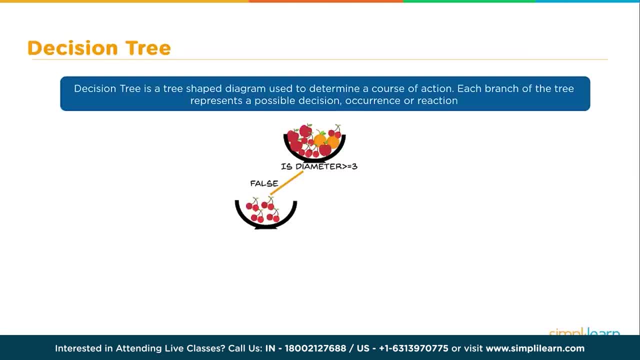 Because everything else is bigger than that. So all the cherries fall into that decision. So we have all that data we are training, We can look at that. We know that is what is going to come up. Is the color orange? Well, it goes. hmmm, orange or red? 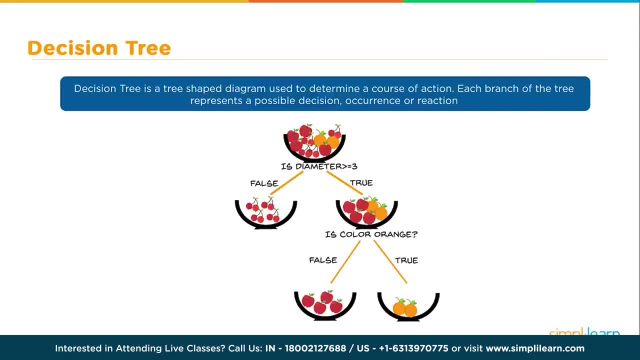 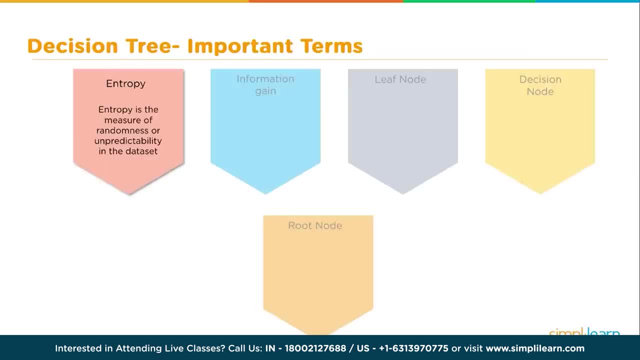 Well, if it is true, Then it comes out as the orange, And if it is false, That leaves apples. So in this example, These are very important terms to know, Because these are very central to understanding the decision tree When working with them. 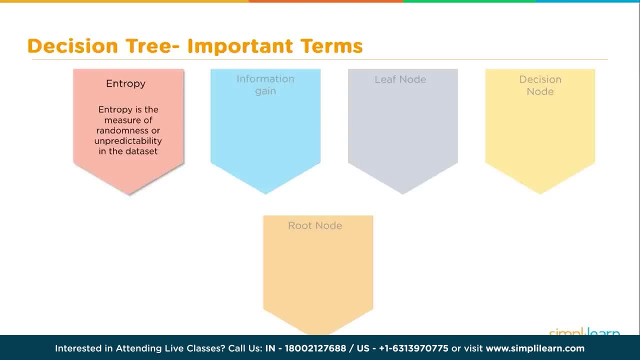 The first is entropy. Everything on the decision tree And how it makes a decision is based on entropy. Entropy is a measure of randomness Or unpredictability in the data set. Then they also have information gain, The leaf node, The decision node. 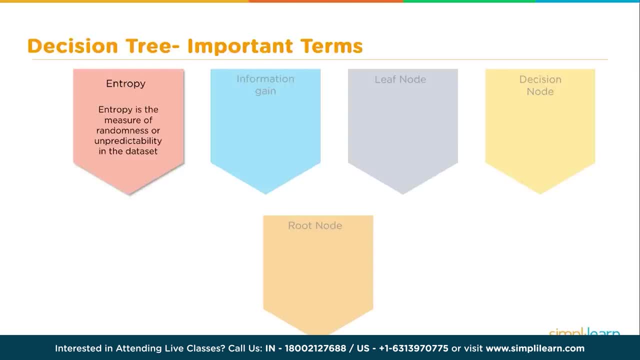 And the root node. We will cover these other four terms As we go down the tree, But let's start with entropy. So, starting with entropy, We have here a high amount of randomness. What that means is that Whatever is coming out of this decision, 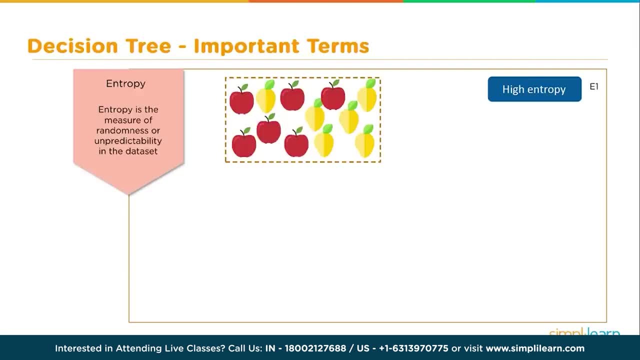 If it was going to guess based on this data, It wouldn't be able to tell you Whether it is a lemon or an apple. It would just say it is a fruit. So the first thing we want to do Is we want to split this apart. 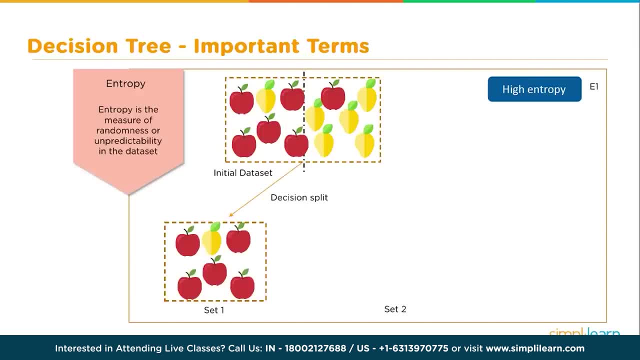 We take the initial data set. We are going to create a data set one And a data set two. We just split it in two And if you look at these new data sets, The entropy of each of those sets Is much less. 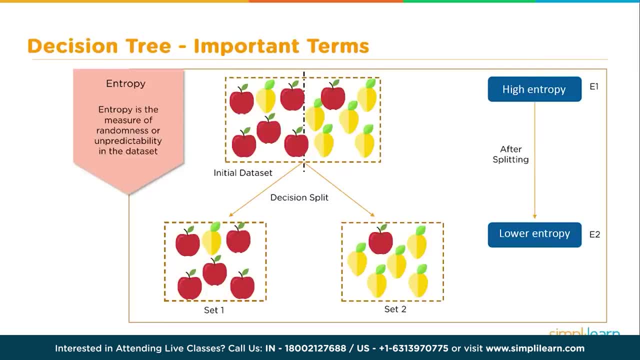 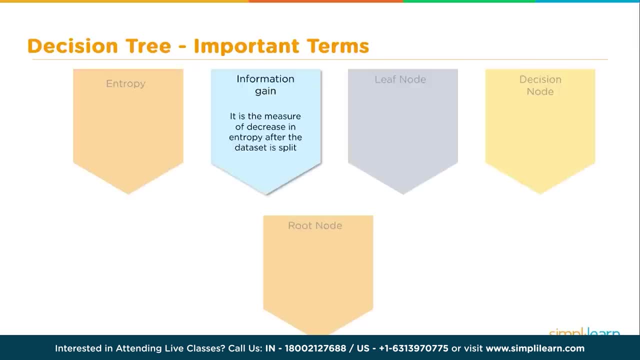 So for the first one, Whatever comes in there, It is going to sort that data And say if this data goes this direction It is probably an apple, And if it goes into the other direction It is probably a lemon. So that brings us up to information gain. 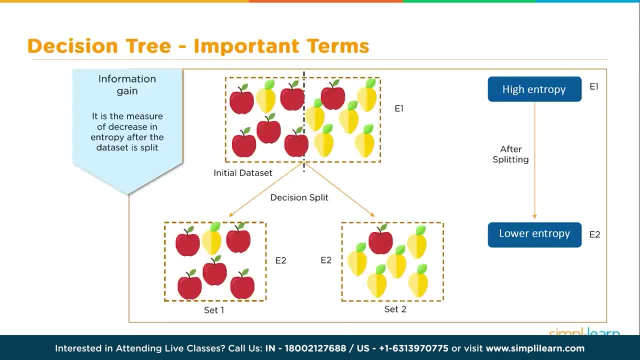 It is the measure of decrease in the entropy After the data set is split. What that means in here Is that we have gone from one set Which has a very high entropy. We have added in the values of E1 for the first one. 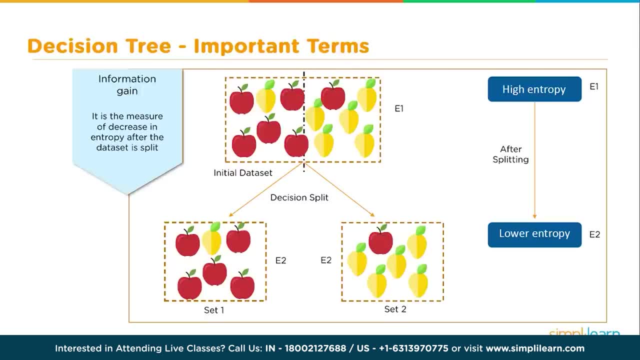 And E2 for the second two, Which are much lower, And so that information gain Is increased greatly in this example, And so you can find that the information gain Simply equals Decision E1. Minus E2.. As we are going down our list of definitions, 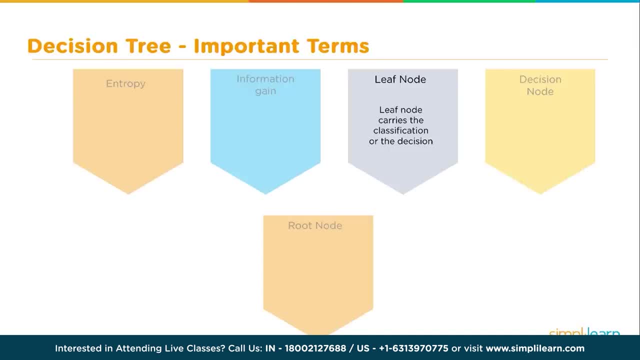 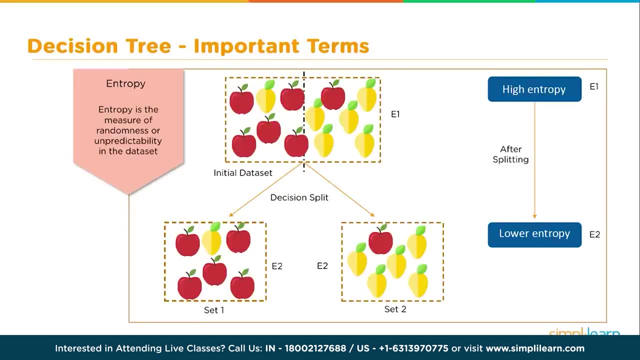 We will look at the leaf node And the leaf node Carries the classification or the decision. So we look down here To the leaf node, To our set 1 or our set 2.. When it comes down there And it says this object has gone into set 1.. 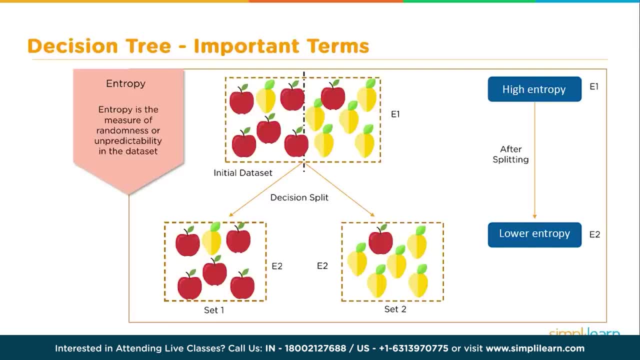 If it has gone into set 1.. It is going to be split By some means And we will either end up with apples On the leaf node Or a lemon on the leaf node, And on the right it will either be an apple or lemons. 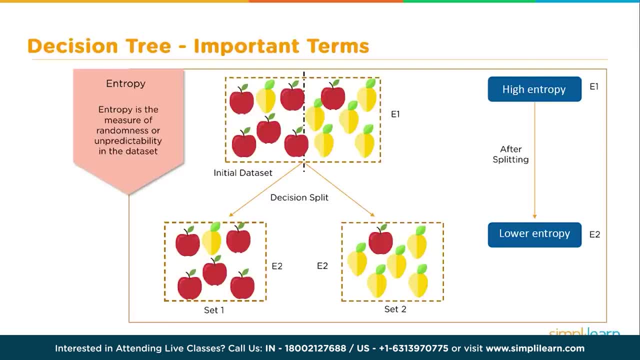 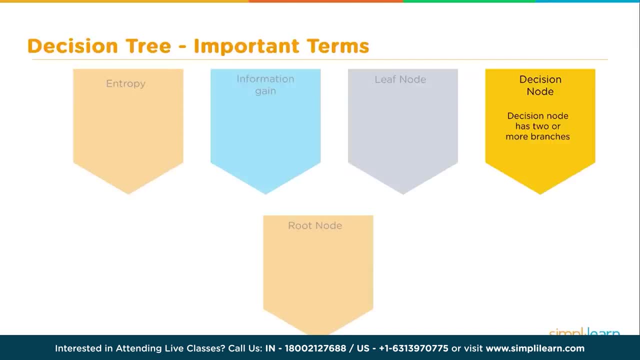 Those leaf nodes are those final decisions Or classifications. That is the definition of leaf node in here. If we are going to have a final leaf Where we make the decision, We will look for the nodes above it And they call those decision nodes. 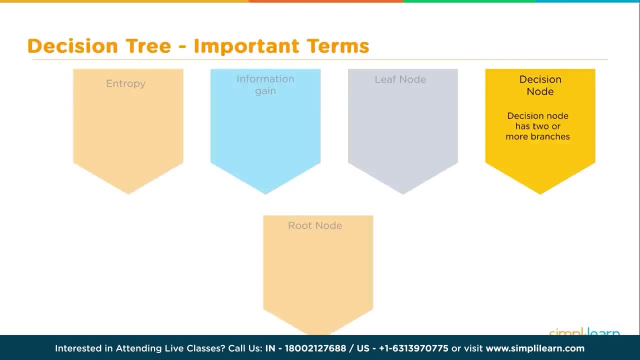 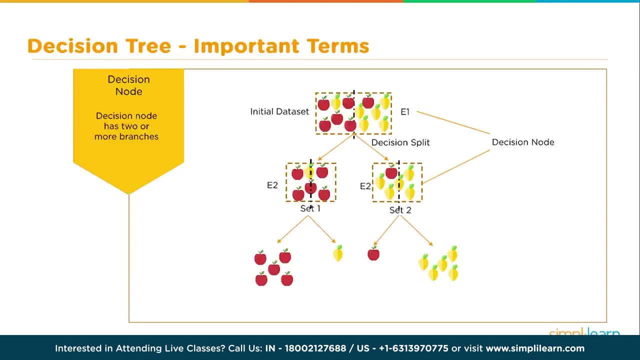 A decision node. Decision node has two or more branches And you can see here where we have the Five apples and one lemon And in the other case, the five lemons and one apple. They have to make a choice Of which tree it goes down. 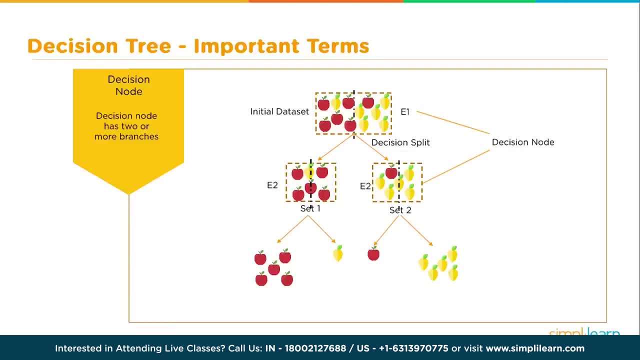 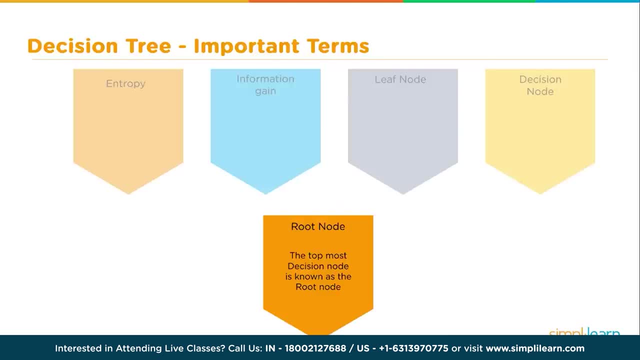 Based on some kind of measurement Or information given to the tree. And that brings us to our last definition: The root node. The top, most decision node Is known as the root node, And this is where you have All of your data. 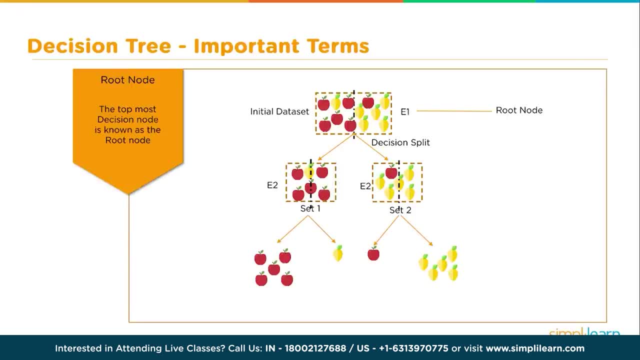 And you have your first decision it has to make Or the first split in information. So far, we have looked at a very general image With the fruit being split. Let's look and see exactly What that means to split the data And how do we make those decisions on there. 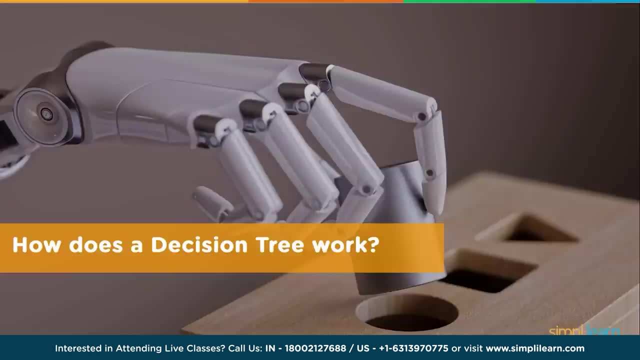 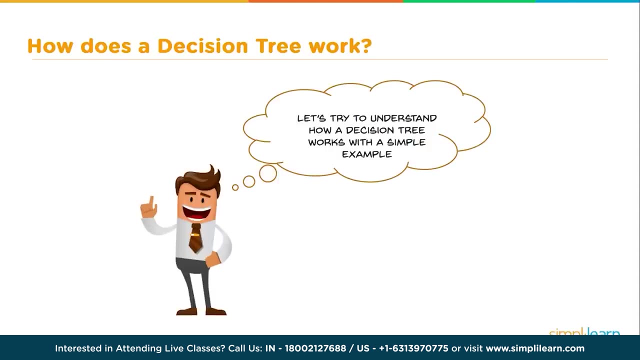 Let's go in there And find out how does A decision tree work. So let's try to understand this And let's use a simple example And we will stay with the fruit. We have a bowl of fruit And so let's create a problem statement. 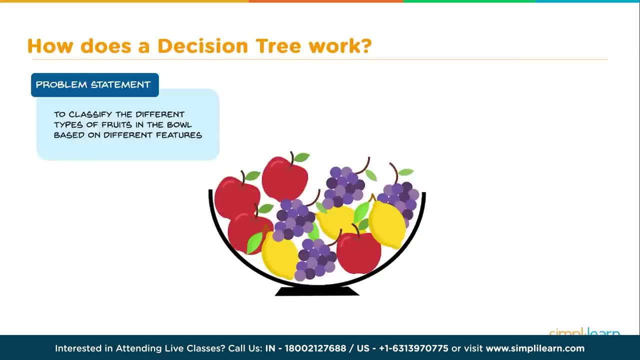 And the problem is we want to classify The different types of fruits In the bowl based on different features. The data set in the bowl Is looking quite messy And the entropy is high in this case. So if this bowl was our decision maker? 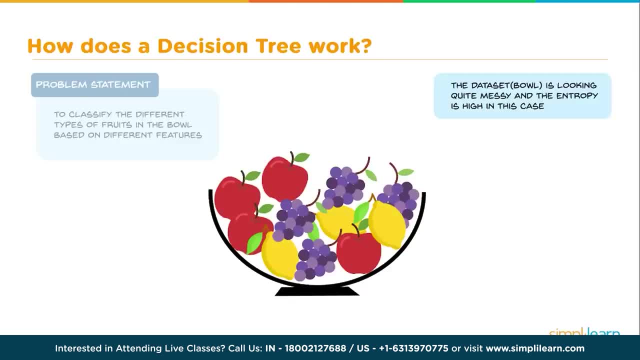 It wouldn't know what choice to make. It has so many choices. Which one do you pick? Apple, grapes or lemons? And so we look in here And we have the data set. So this is our data that we are training, our data with. 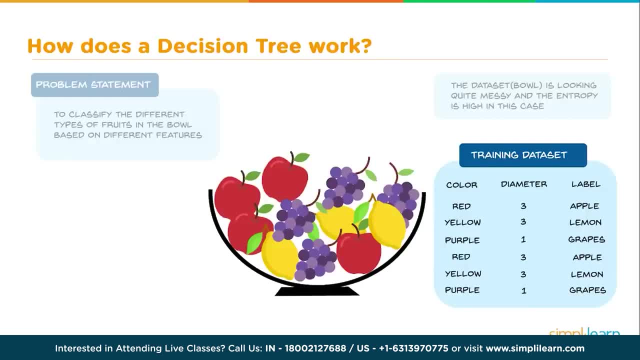 And we have a number of options here. We have the color And under the color we have red, yellow, purple. We have a diameter: 3, 3, 1, 3, 3, 1.. And we have a label. 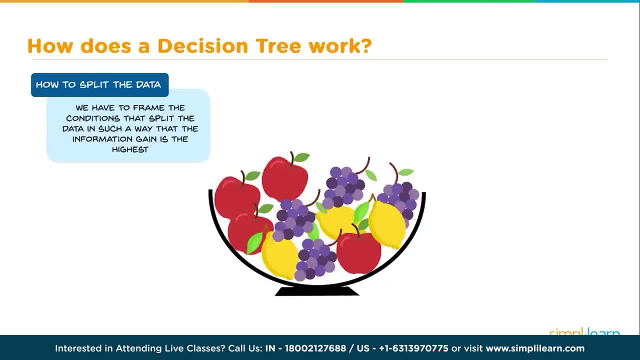 Apple lemon grapes. apple lemon grapes. And how do we split the data? We have to frame the conditions to split the data In such a way that the information gain is the highest, And it is very key to note. 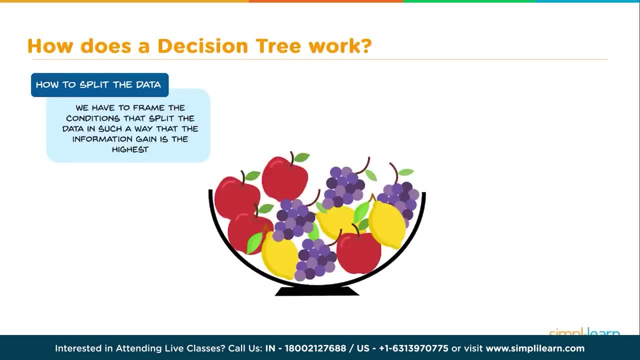 That we are looking for the best gain. We don't want to just start sorting out the smallest piece in there. We want to split it the biggest way we can, And so we measure this decrease in entropy. That is what they call it: entropy. 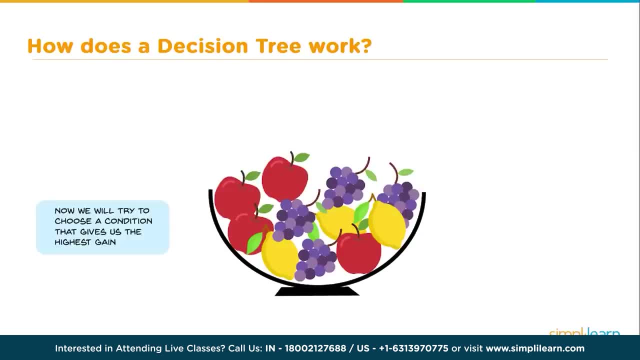 There is our entropy After splitting, And now we will try to choose a condition that gives us the highest gain. We will do that by splitting the data, using each condition And checking the gain that we get out of them. The conditions that give us the highest gain will be used to make the first split. 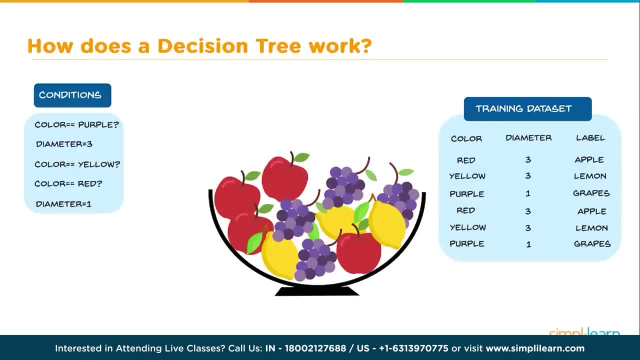 So let's take a look at these different conditions. We have color, We have diameter And if we look underneath that, we have a couple of different values. We have: diameter equals 3.. Color equals yellow. red. Diameter equals 1.. 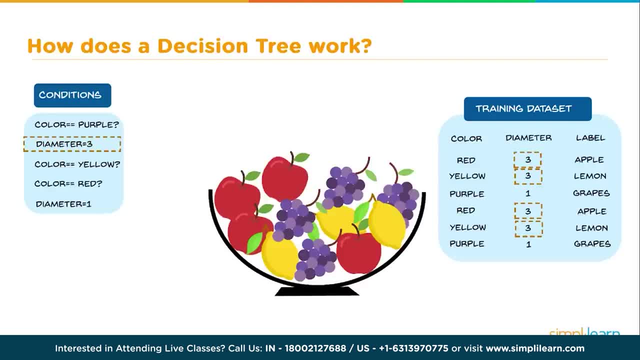 And when we look at that You will see over here we have 1,, 2,, 3, 4 threes. That is a pretty hard selection. So let's say the condition gives us the maximum gain of 3.. So we have the most pieces fall into that range. 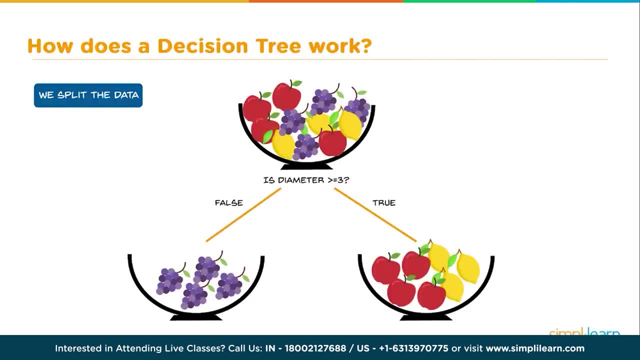 So our first split from our decision node Is we split the data based on the diameter. Is it greater than or equal to 3?? If it is not- that is false- It goes into the great bowl. If it is true, It goes into a bowl full of lemon and apples. 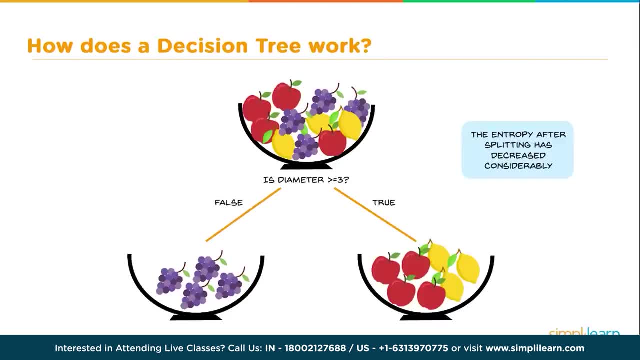 The entropy after splitting has decreased considerably, So now we can make two decisions. If you look at it, There is very much less chaos going on there. This node has already attained an entropy value of 0.. As you can see, There is only one kind of label left for this branch. 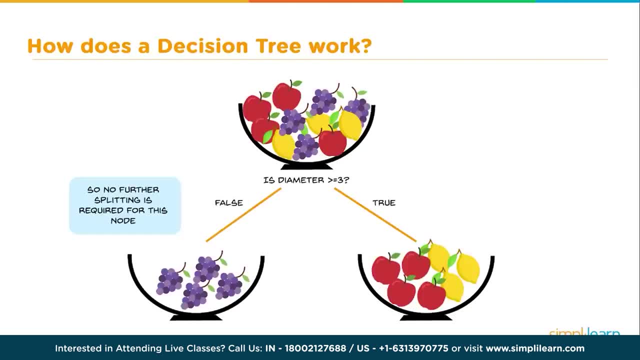 So no further splitting is required for this node. However, This node on the right Is still requires a split to decrease the entropy further. So we split the right node Further based on color. If you look at this, If I split it on color, 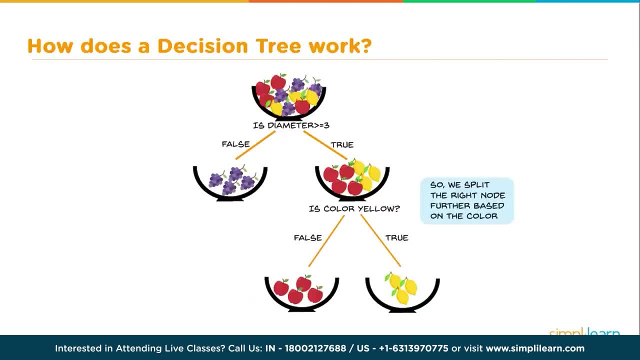 That pretty much cuts it right down the middle. That is the only thing we have left in our choices Of color and diameter too, And if the color is yellow, It is going to go to the right bowl, And if it is false, 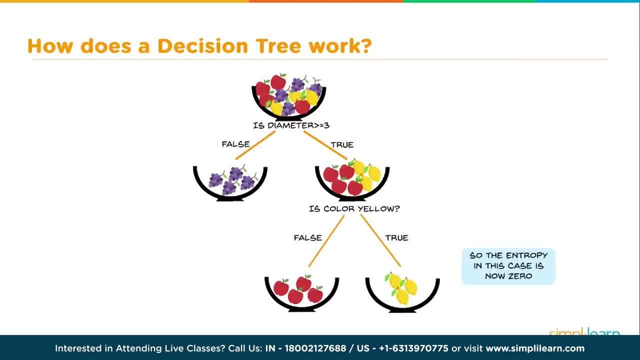 It is going to go to the left bowl, So the entropy in this case is now 0.. So now we have 3 bowls with 0 entropy. There is only one type of data in each one of those bowls, So we can predict a lemon with 100% accuracy. 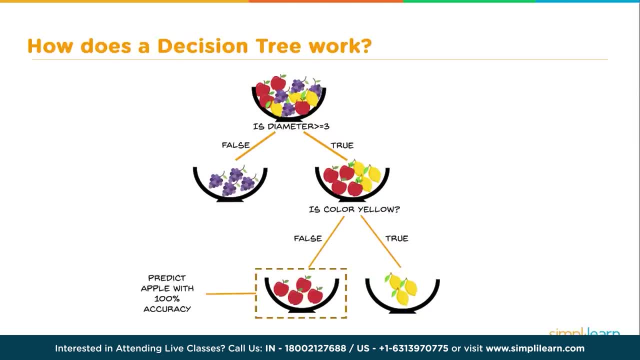 And we can predict a lemon with 100% accuracy And we can predict the apple also with 100% accuracy, Along with our grapes up there. So we have looked at kind of a basic tree In our forest. But what we really want to know is: 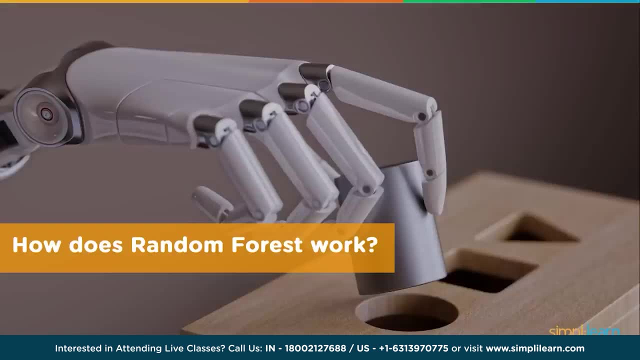 How does a random forest work as a whole? So to begin our random forest classifier, Let's say we already have built 3 trees And we are going to start with the first tree. That looks like this, Just like we did in the example. 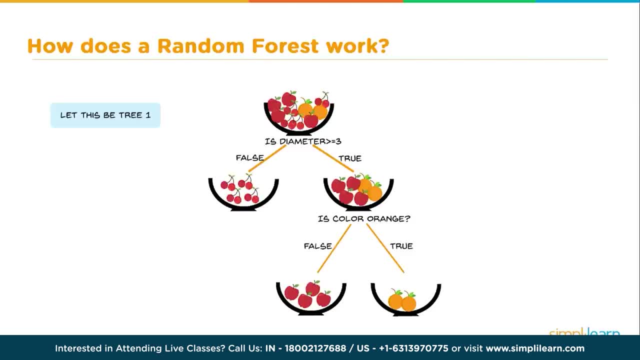 This tree looks at the diameter If it is greater than or equal to 3. It is true. Otherwise it is false. So one side goes to the smaller diameter, One side goes to the larger diameter. And if the color is orange, 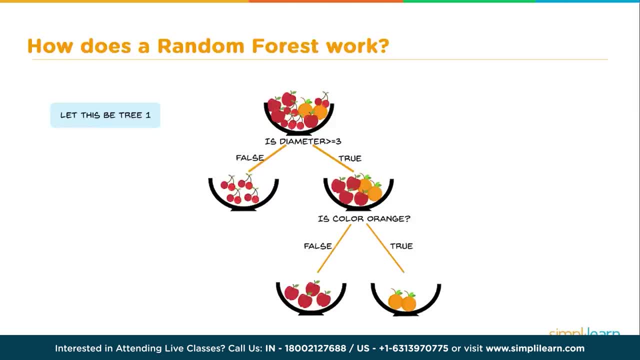 It is going to go to the right. True, We are using oranges now instead of lemons, And if it is red, it is going to go to the left. False, We build a second tree, very similar, But it is split differently. 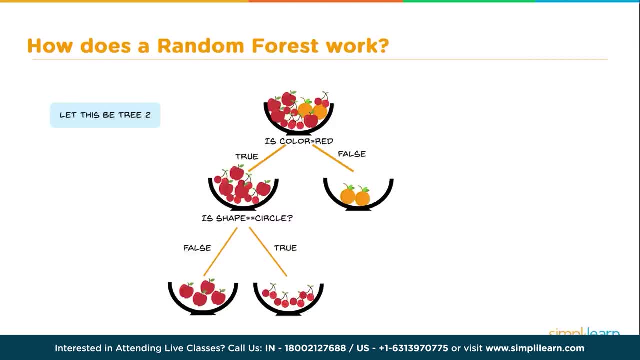 Instead of the first one being split by diameter, This one when they created it. If you look at that first bowl, It has a lot of red objects. So it says, is the color red, Then the fastest. And so of course, if it is true, it goes to the left. 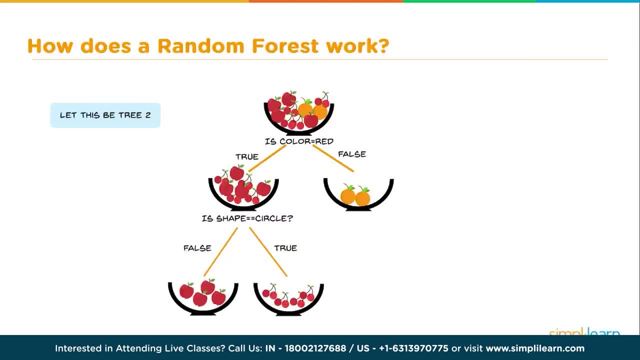 If it is false, it goes to the right And then it looks at the shape: False or true, and so on and so on. And tree 3. Is the diameter equal to 1?? And it came up with this because there is a lot of cherries in this bowl. 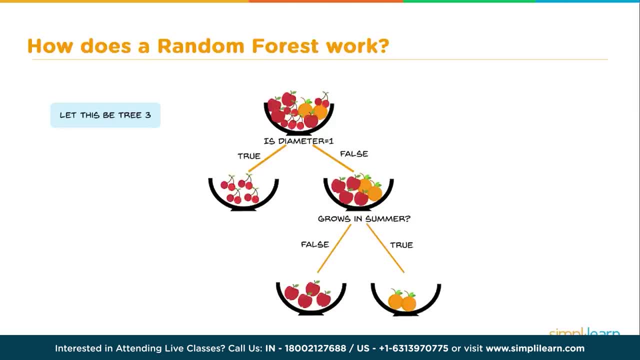 So that would be the biggest split on there. Is the diameter equal to 1?? That is going to drop the entropy the quickest And, as you can see, it splits it into true, If it goes false. and they have added another category: Does it grow in the summer? 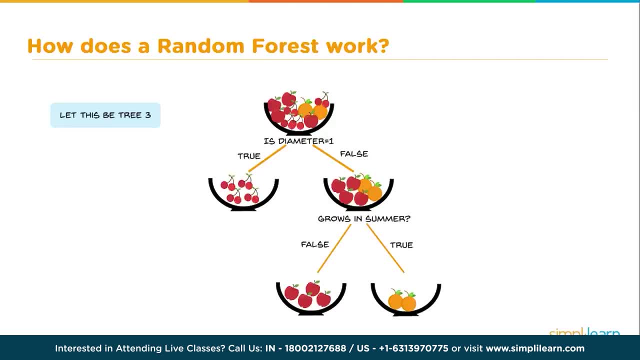 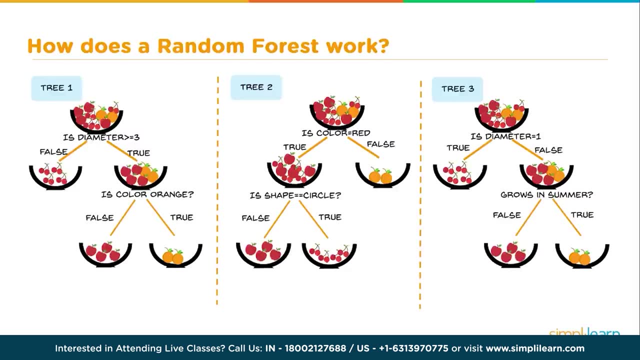 And if it is false, It goes off to the left. If it is true, it goes off to the right. Let's go ahead and bring these 3 trees. You can see them all in one image. So this would be 3 completely different trees. 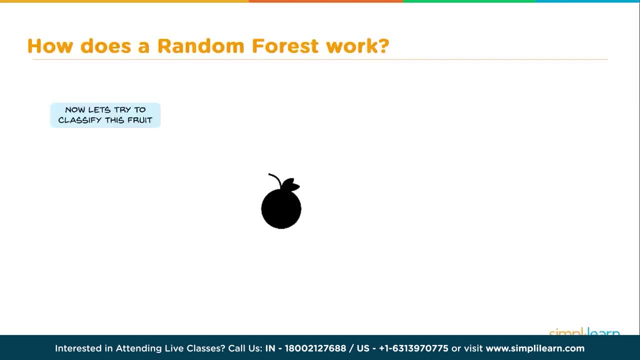 Categorizing a fruit. And let's take a fruit Now. let's try this And this fruit. if you look at it, we have blackened it out. You can't see the color on it, So it is missing data. Remember one of the things we talked about earlier? 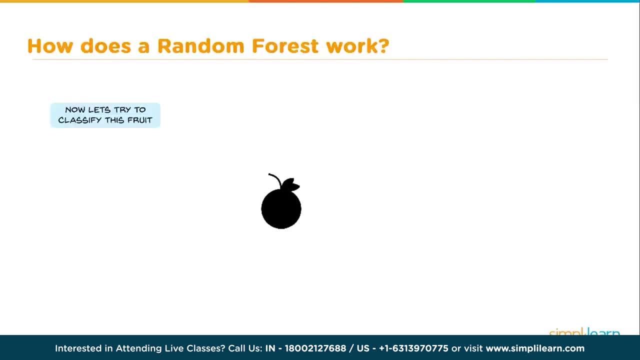 Is that? a random forest works really good if you are missing data, If you are missing pieces. So this fruit has an image. You can see it in the right camera when they took the picture And we are going to take a look at this. 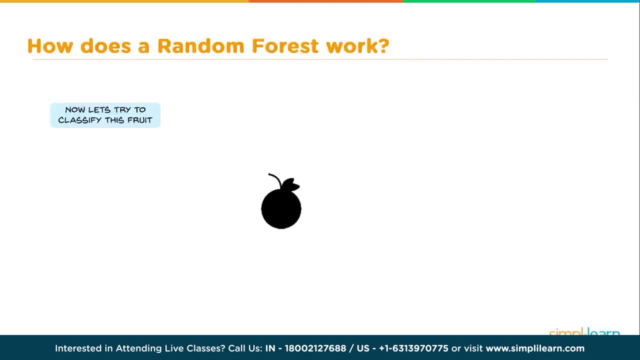 And it is going to have. They put the color in there, So ignore the color down there, But the diameter equals 3. We find out it grows in the summer. equals yes, And the shape is a circle. And if you go to the right, 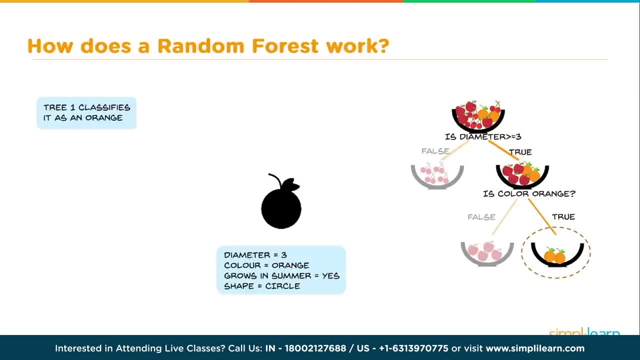 You can look at what one of the decision trees did. This is the third one. Is the diameter greater than or equal to 3?? Is the color orange? Well, it doesn't really know on this one, But if you look at the value it would say true. 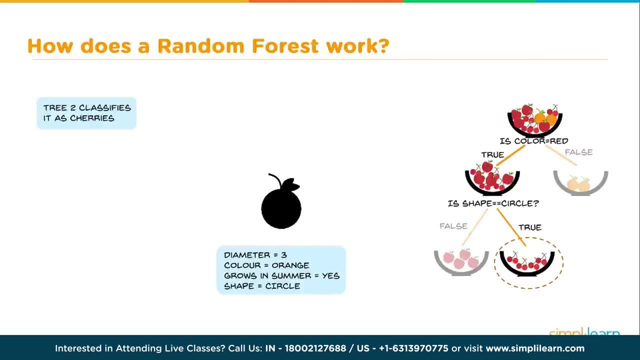 Is the color equal red. Is the shape a circle? True, it is a circle. So this would look at it and say, oh, that is a cherry. And then we go to the other classifier And it says: is the diameter equal 1?? 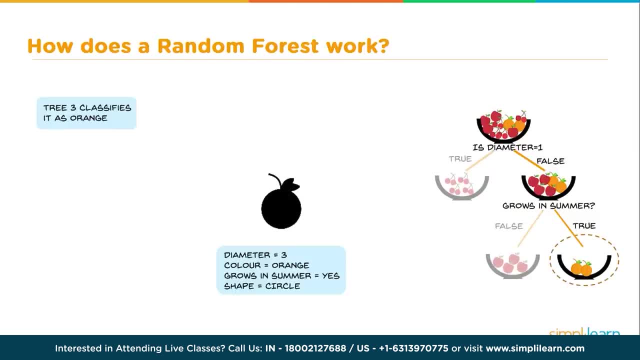 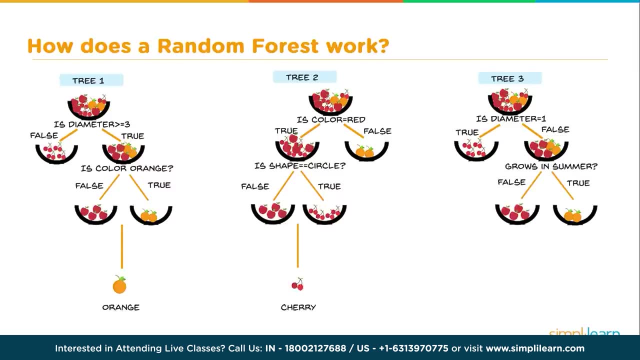 Well, that is false. Does it grow in the summer? True, So it goes down and looks at it as oranges. So how does this random forest work? The first one says it is an orange, The second one said it was a cherry. 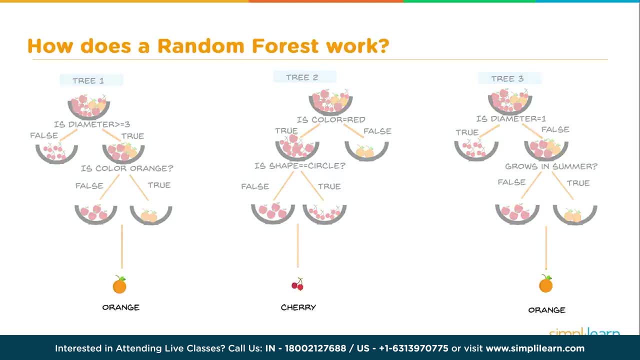 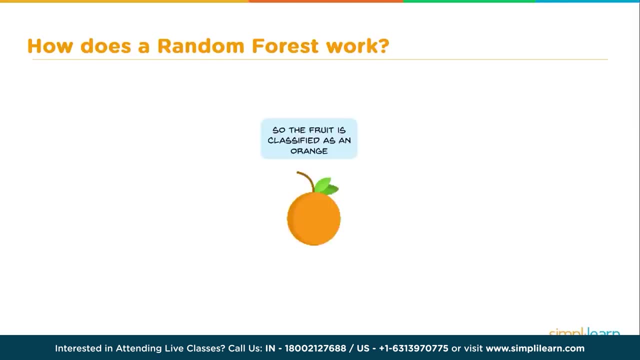 And the third one says it is an orange, And you can guess if you have two oranges. When you add that all together, The majority of the vote says orange. So the answer is It is classified as an orange, Even though we didn't know the color and we are missing data on it. 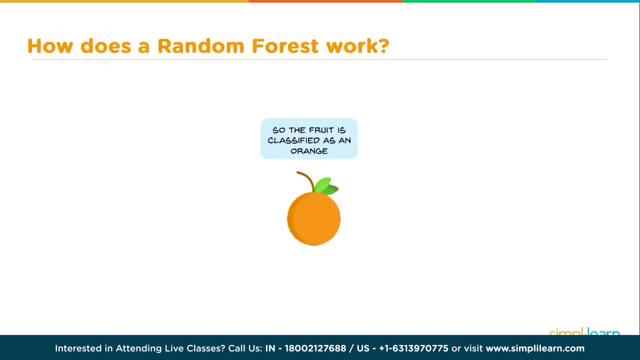 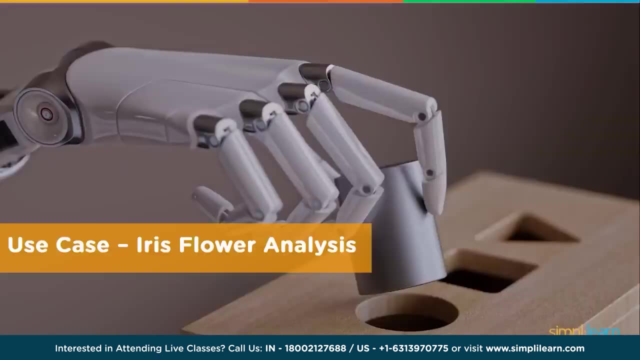 I don't know about you, But I am getting tired of fruit, So let's switch. and I did promise you We would start looking at a case example And get into some python coding. Today we are going to use the case The iris flower analysis. 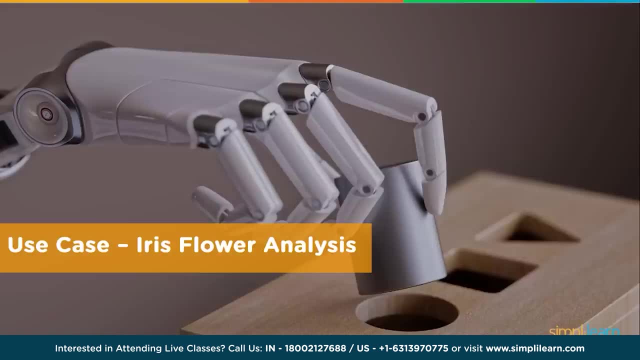 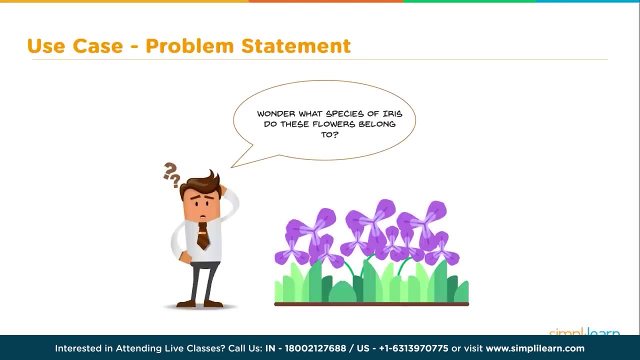 This is the exciting part, As we roll up our sleeves And actually look at some python coding, We need to go ahead And create a problem statement: Wonder: what species of iris do these flowers belong to? Let's try to predict the species of the flowers. 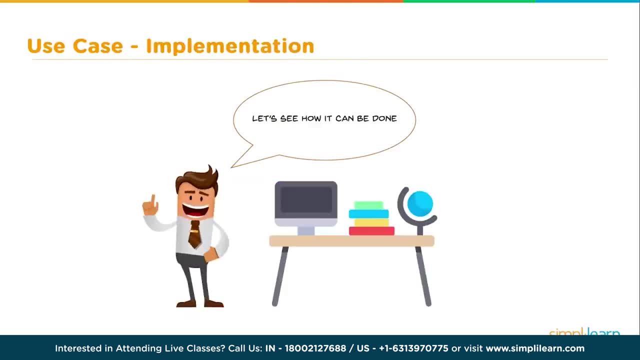 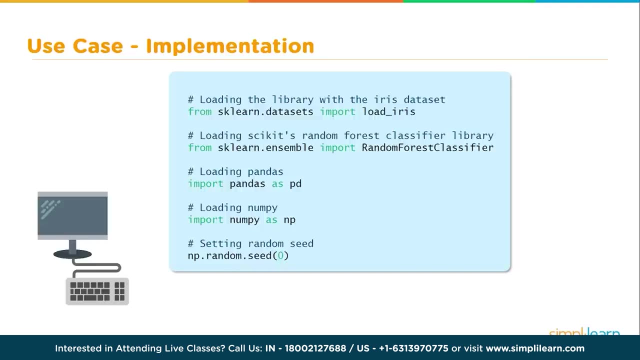 Using machine learning in python. Let's see how it can be done. So here we begin to go ahead And implement our python code, And you will find That the first half of our implementation Is all about organizing And exploring the data coming in. 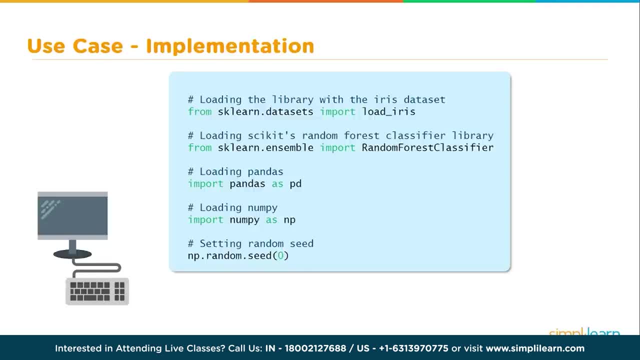 Let's go ahead and take this first step, Which is loading the different modules Into python. Let's put that in our favorite editor. Whatever your favorite editor is- In this case, I am going to be using The anaconda jupiter notebook. 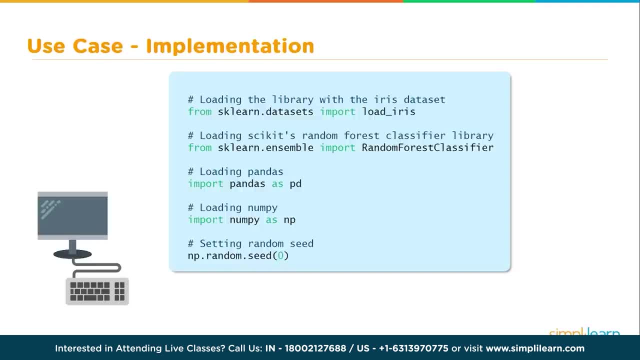 Which is one of my favorites. Certainly, there is notepad plus plus And eclipse and dozens of others, Or just even using the python terminal window- Any of those will work just fine To go ahead and explore this python coding. So here we go. 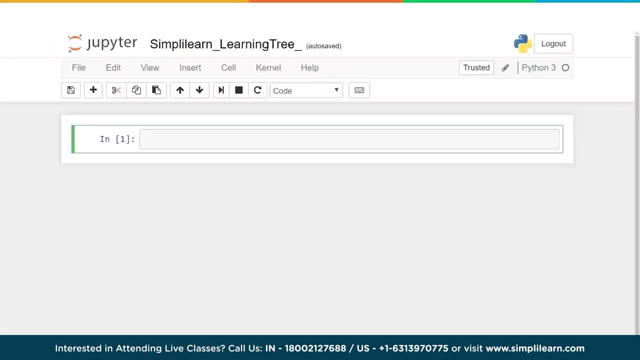 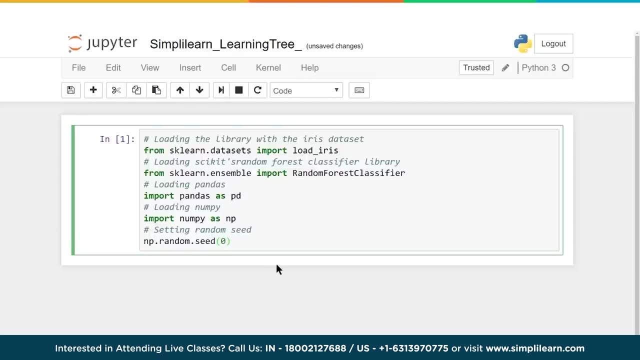 Let's go ahead and flip over to our jupiter notebook, And I have already opened up a new page For python 3 code And I am just going to paste this In there and let's take a look And see what we are bringing into our python. 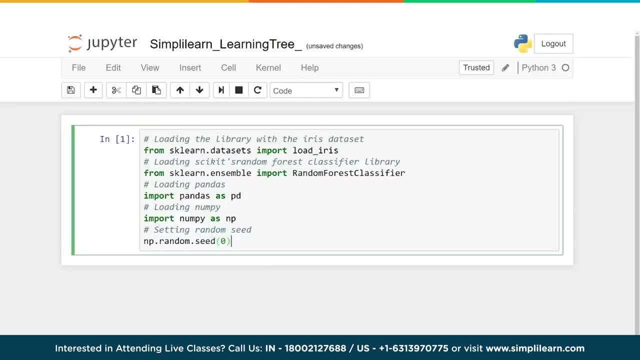 The first thing we are going to do Is, from the sklearndatasets, Import load iris. Now, this isn't the actual data. This is just the module That allows us to bring in the data, The load iris, And the iris is so popular. 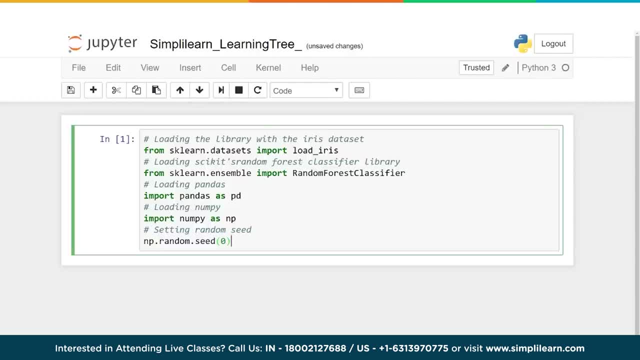 It has been around since 1936. When Ronald Fisher published a paper on it, And they are measuring the different parts of the flower And, based on those measurements, Predicting what kind of flower it is, We need to go ahead and import a random forest classifier. 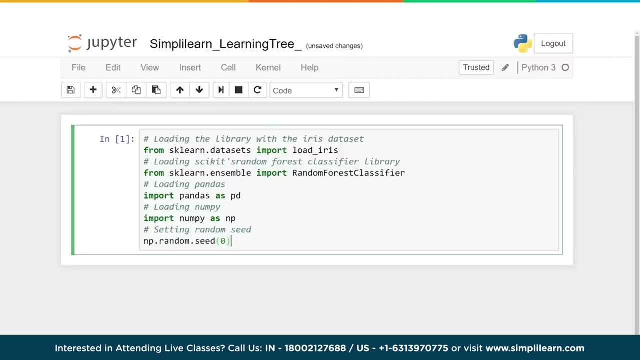 From the sklearn module, So sklearnensemble Import random forest classifier. And then we want to bring in two more modules And these are Probably the most commonly used modules In python and data science. With any of the other modules That we bring in. 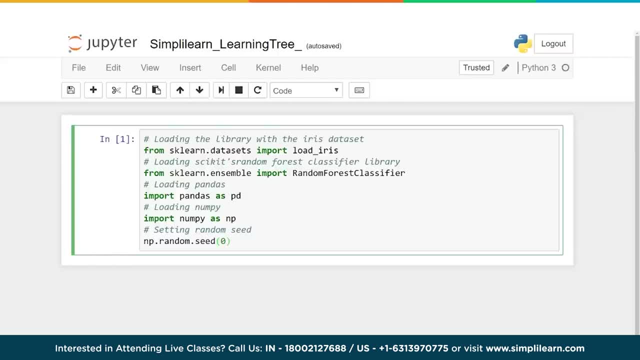 And one is going to be pandas. We are going to import pandas as pd- Pd is the common term used for pandas, And pandas is basically Creates a data format for us, Where, when you create a pandas data frame, It looks like an x scale spreadsheet. 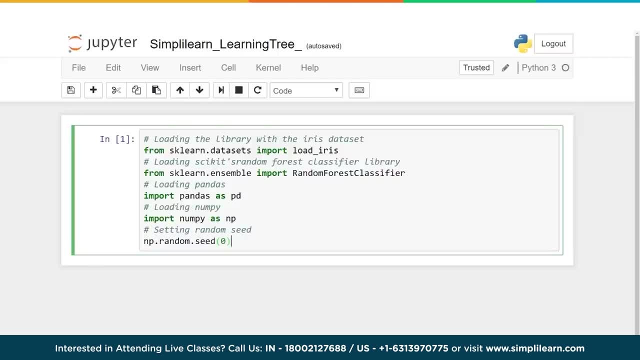 And you will see that in a minute When we start digging deeper into the code. Panda is just wonderful Because it plays nice with all the other modules in there. And then we have numpy, Which is our numbers python And the numbers python allows us to. 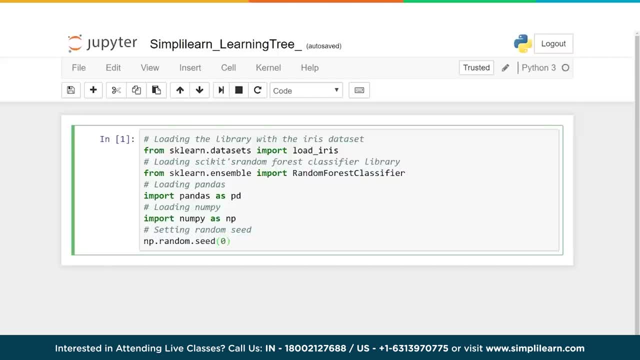 Do different mathematical sets on here. We will see right off the bat. We are going to take our np And we are going to go ahead and seed the randomness with it With zero. So, nprandomseed, This code doesn't actually show anything. 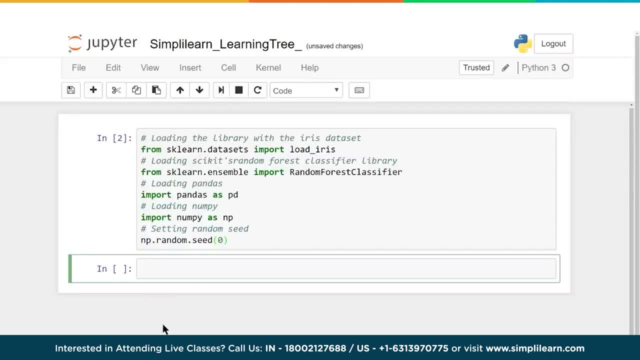 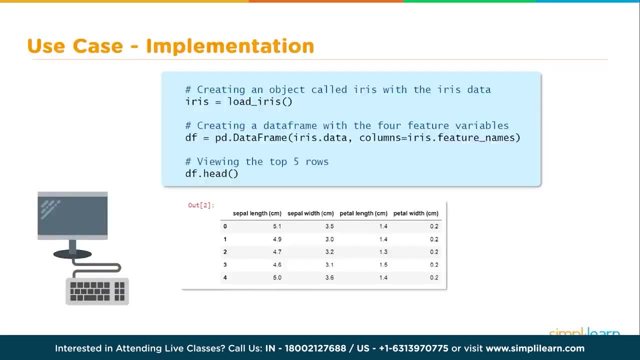 We are going to go ahead and run it, Because I need to make sure I have all those loaded, And then let's take a look at the next module on here. The next six slides, Including this one, Are all about exploring the data. 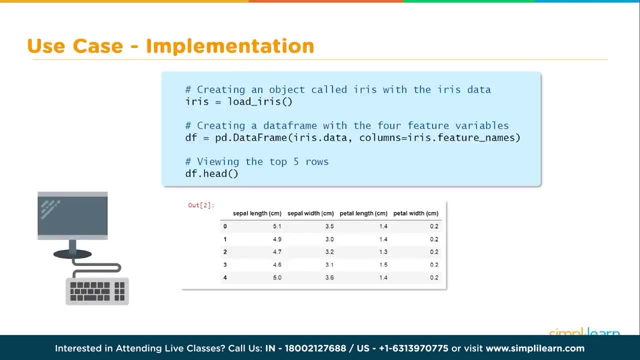 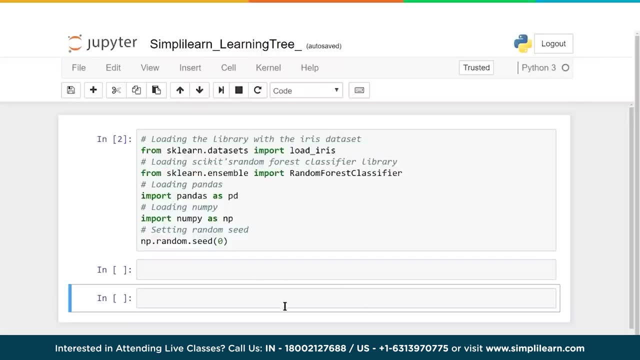 Remember I told you half of this is about looking at the data And getting it all set. So let's go ahead and take this code right here, The script, And let's get that over into our Jupyter notebook. And here we go. 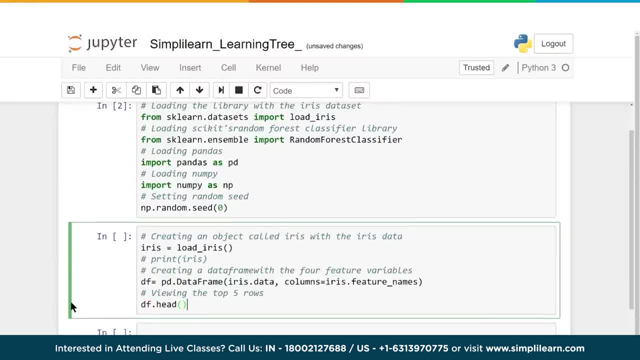 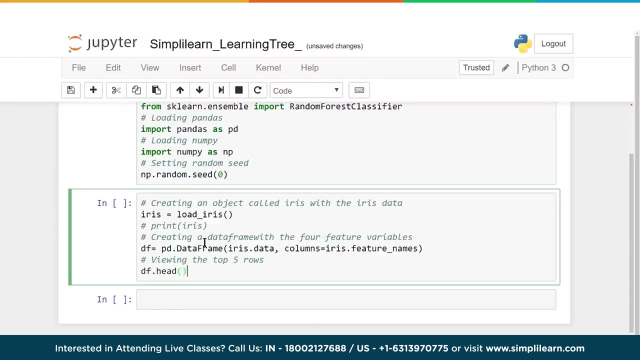 We have gone ahead and run the imports And I am going to paste the code down here And let's take a look and see what is going on. The first thing we are doing Is we are actually loading the iris data And, if you remember, up here 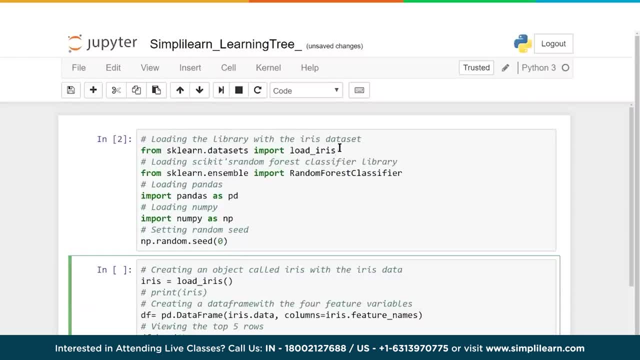 We loaded the module That tells it how to get the iris data. Now we are actually assigning that data To the variable iris And then we are going to go ahead and use the df To define data frame, And that is going to equal pd. 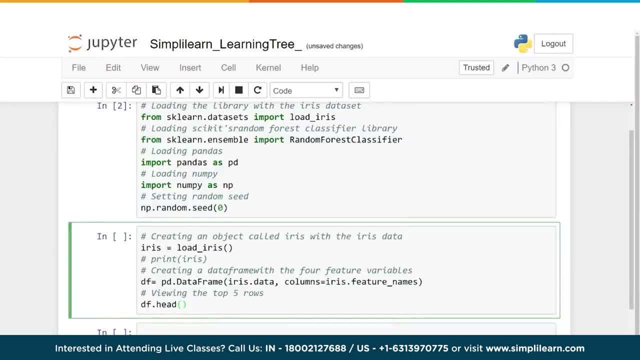 And, if you remember, that is pandas as pd. So that is our pandas And panda data frame. And then we are looking at iris data Columns- equals iris feature names- And we are going to do the df head And let's run this. 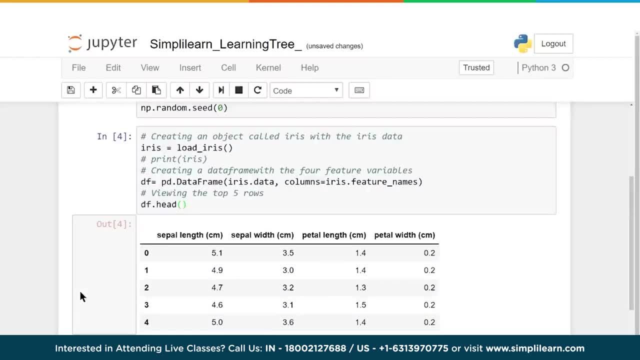 So you can understand what is going on here. The first thing you want to notice Is that our df has created What looks like an excel spreadsheet And in this excel spreadsheet We have set the columns. So up on the top you can see the four different columns. 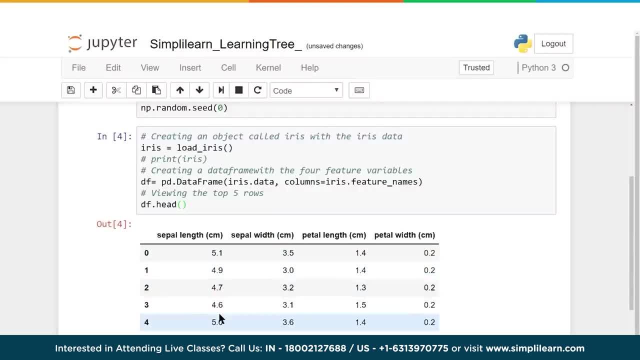 And then we have the data- Irisdata- down below. It is a little confusing Without knowing where this data is coming from. So let's look at the bigger picture And I am going to go print. I am just going to change this for a moment. 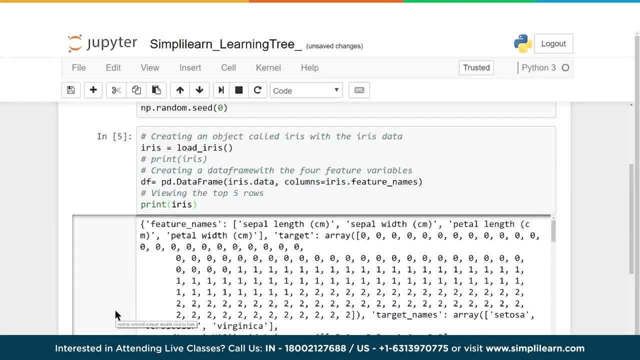 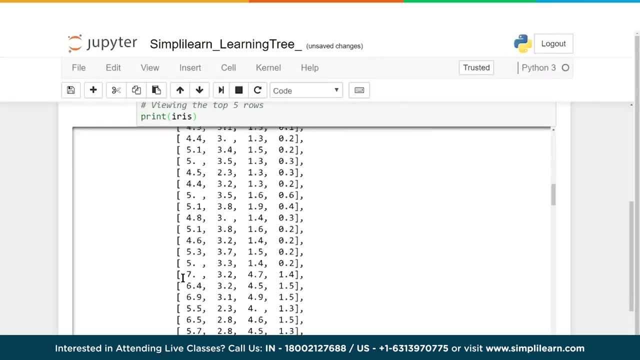 And we are going to print all of iris And see what that looks like. So when I print all of iris I get this long list of information And you can scroll through here And see all the different titles on there. What is important to notice? 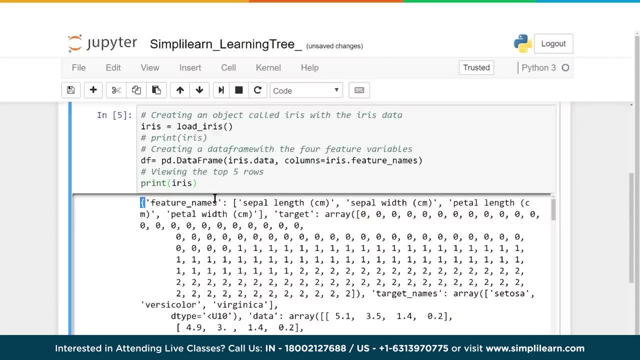 Is that? first off, there is brackets at the beginning. So this is a python dictionary, And in a python dictionary You will have a key Or a label And this label pulls up And all of that information comes after it. So feature names. 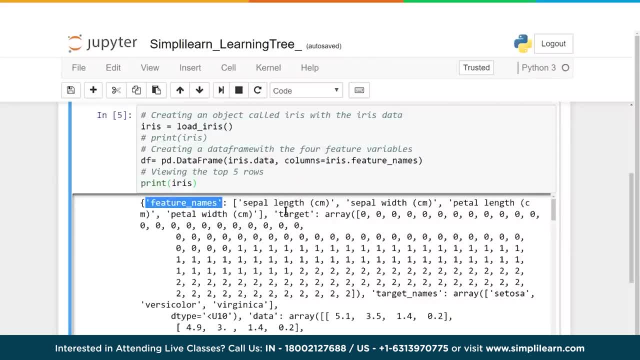 Which we actually used over here under columns Is equal to an array of sepal length, Sepal width, Petal length, Petal width. These are the different names they have for the four different columns And if you scroll down far enough, 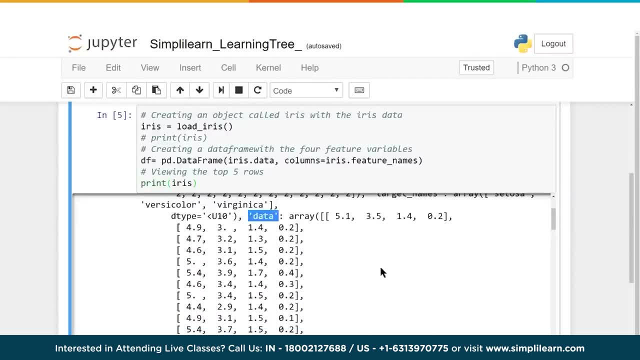 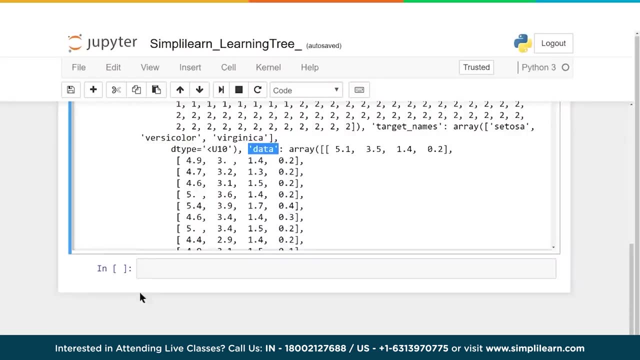 You will also see data down here. Oh goodness, it came up right towards the top And data is equal to the different data we are looking at Now. there is a lot of other things in here, Like target. We are going to be pulling that up in a minute. 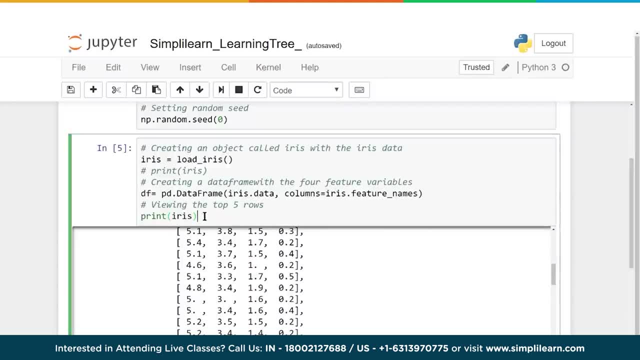 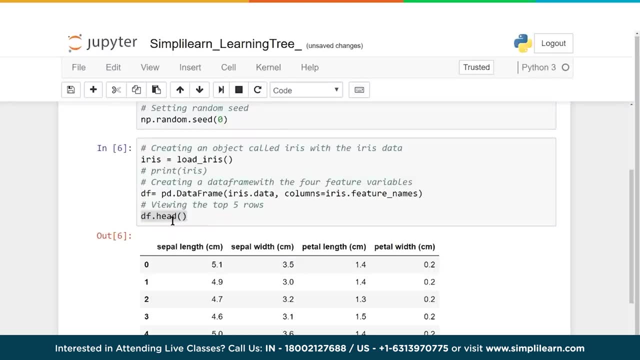 Target names, which is further down, And we will show you that also in a minute. Let's go ahead and set that back To the head, And this is one of the neat features of pandas And panda data frames Is when you do dfhead. 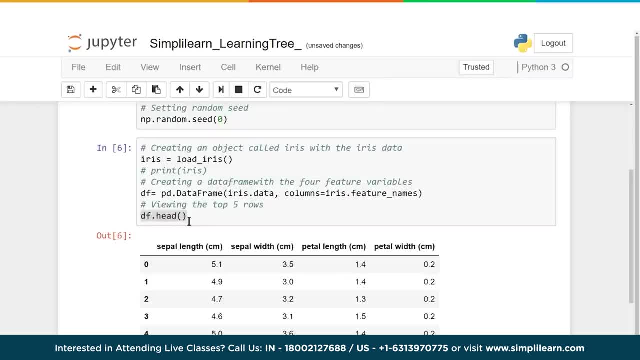 Or the panda data framehead. It will print the first five lines Of the data set in there, Along with the headers, If you have it. In this case we have the column headers set to iris features And in here you will see that we have. 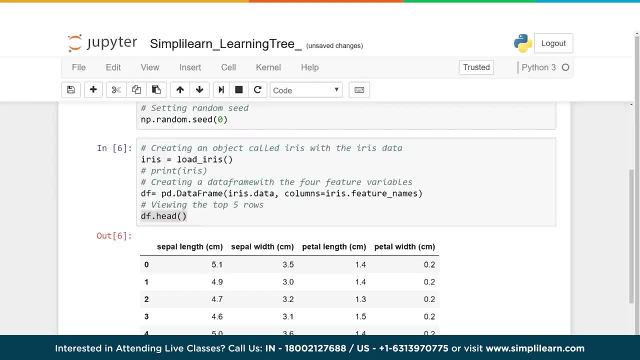 0,, 1,, 2,, 3, 4.. In python, Most arrays always start at 0. So when you look at the first five, It is going to be 0,, 1,, 2,, 3, 4.. 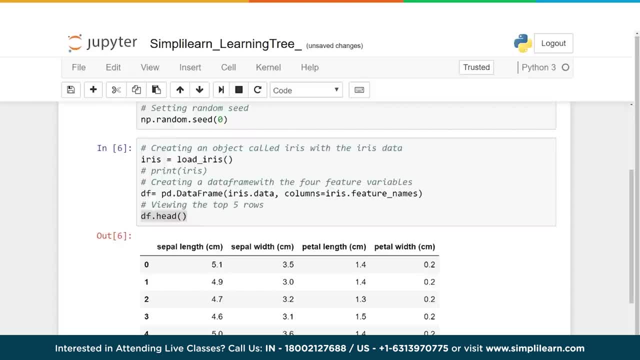 Not 1,, 2,, 3,, 4,, 5.. So now we have got our iris data imported into a data frame. Let's take a look at the next piece of code in here, And so in this section here. 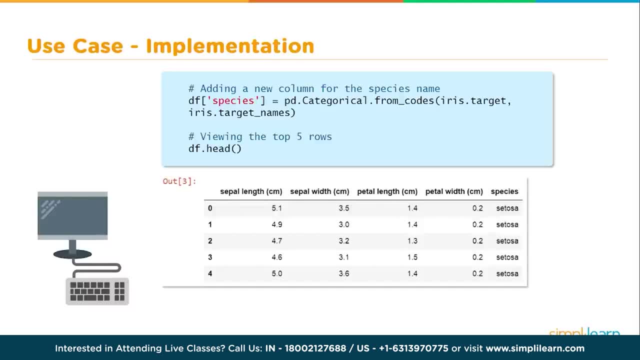 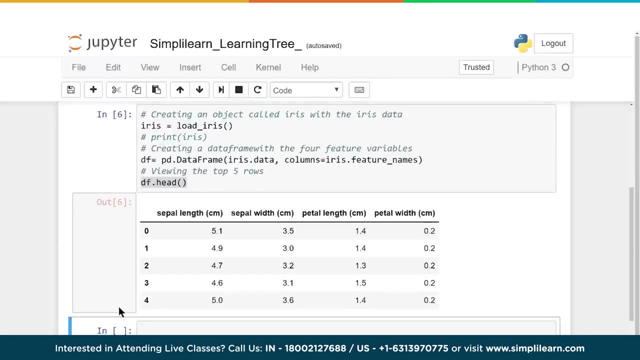 Of the code. We are going to take a look at the target And let's go ahead and get this into our notebook, This piece of code, So we can discuss it a little bit more in detail. So here we are in our Jupyter notebook. 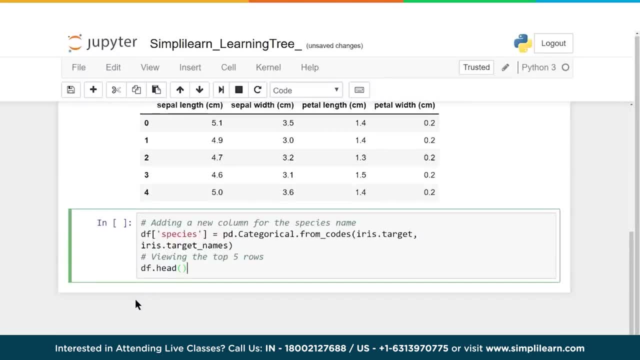 I am going to put the code in here And before I run it I want to look at a couple of things going on. So we have DF species And this is interesting Because right here you will see where I have DF species in brackets. 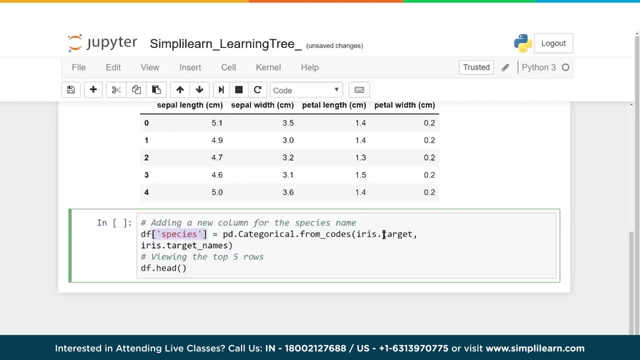 Which is the key code For creating another column. And here we have iris dot target. Now these are both in the pandas setup on here, So in pandas We can do either one- I could have just as easily done iris- And then in brackets target. 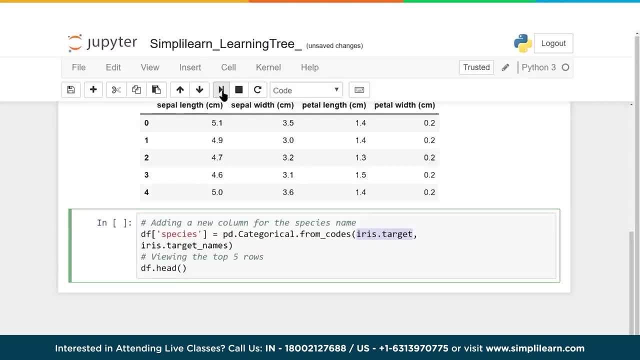 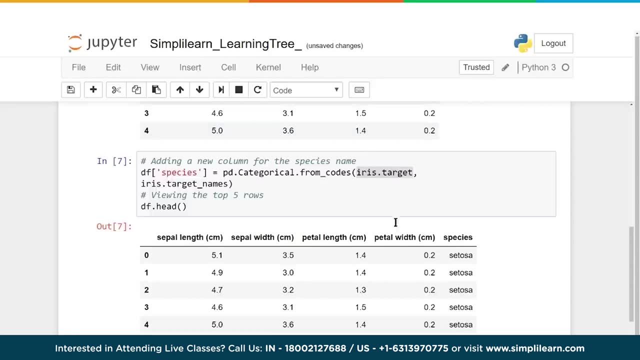 Depending on what I am working on, Both are acceptable. Let's go ahead and run this code And see how this changes, And what we have done is we have added the target From the iris data set As another column on the end. 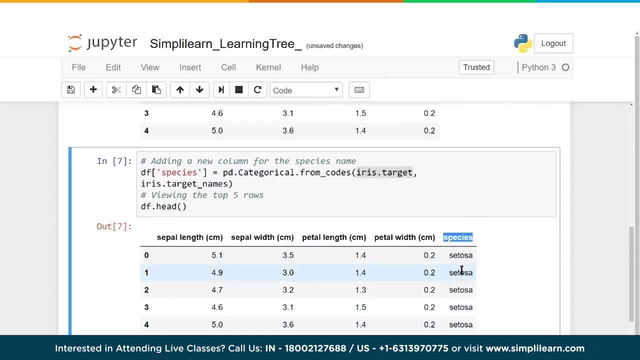 Now, what species is? This is what we are trying to predict. So we have our data, Which tells us the answer For all these different pieces, And then we have added a column with the answer. That way, when we do our final setup. 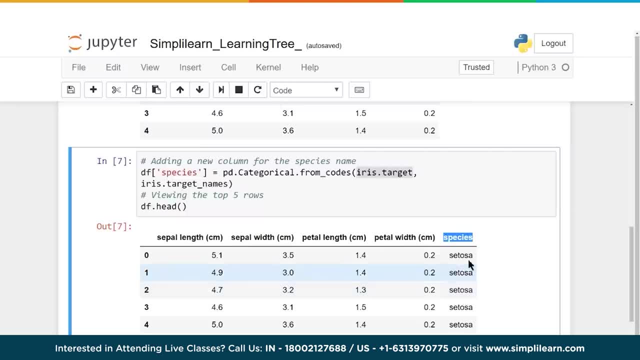 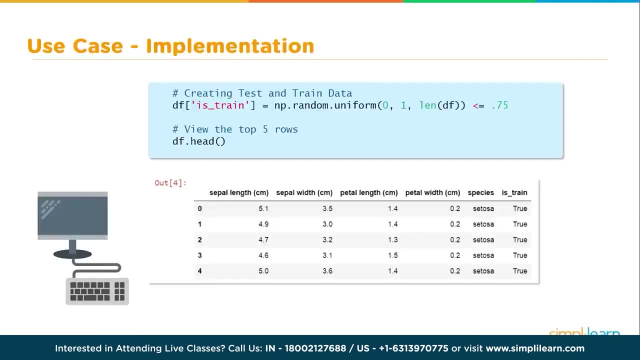 We will have the ability to program our neural network To look for this different data, To see what a setosa is, Or a vericolor, which we will see in just a minute, Or a virginica. Those are the three that are in there. 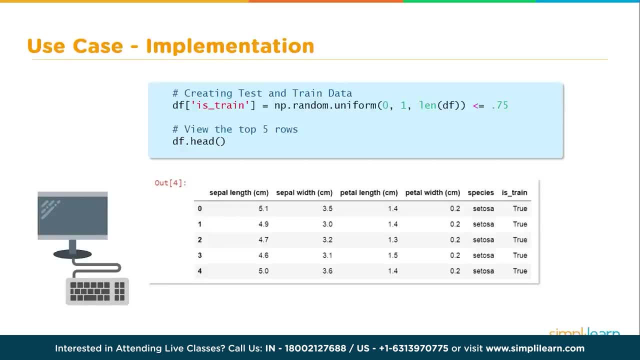 And now we are going to add one more column. I know we are organizing all this data over and over again. It is kind of fun. There is a lot of ways to organize it. What is nice about putting everything onto one data frame? 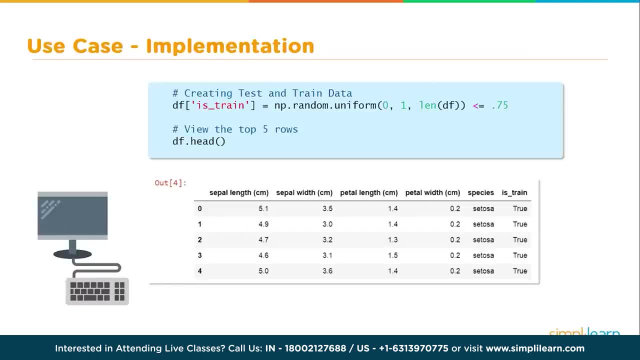 Is. I can then do a printout And it shows me exactly what I am looking at, And I will show you where that is different, Where you can alter that And do it slightly differently, But let's go ahead and put this into our. 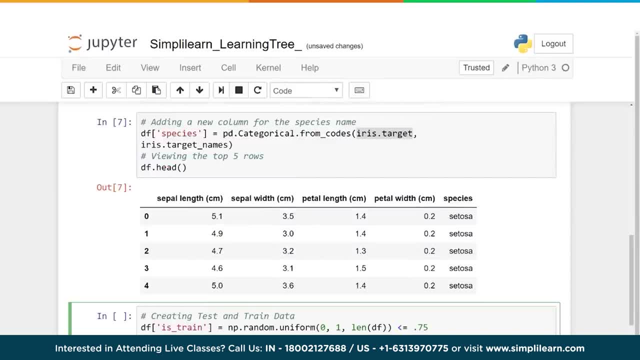 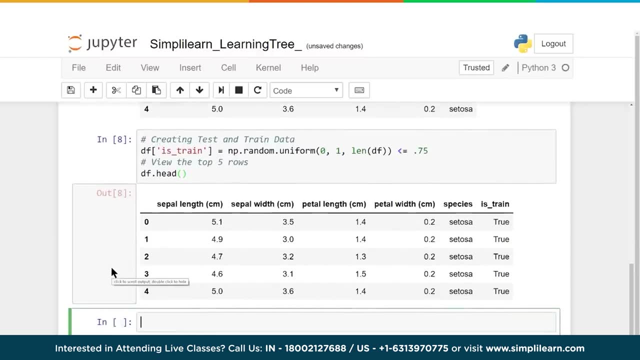 Script up to that now. And here we go. We are going to put that down here And we are going to run that, And let's talk a little bit about what we are doing Now. we are exploring data And one of the challenges is knowing. 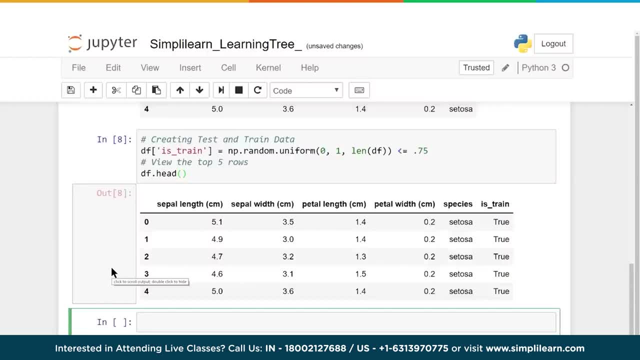 How good your model is. Did your model work? And to do this, we need to split the data, And we split it into two different parts. They usually call it the training And the testing, And so in here we are going to go ahead and put that in our database. 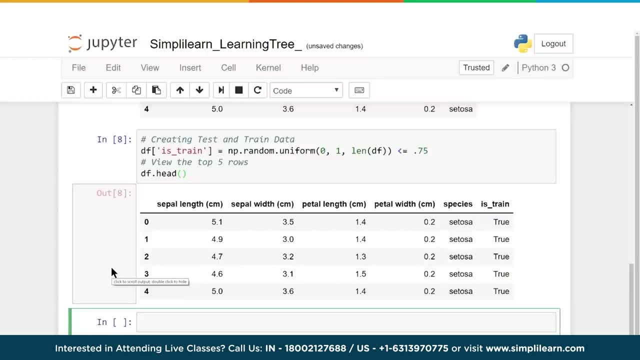 So you can see it clearly. We have set it df And remember you can put brackets. This is creating another column Is train, So we are going to use part of it for training And this equals np. Remember that stands for numpy. 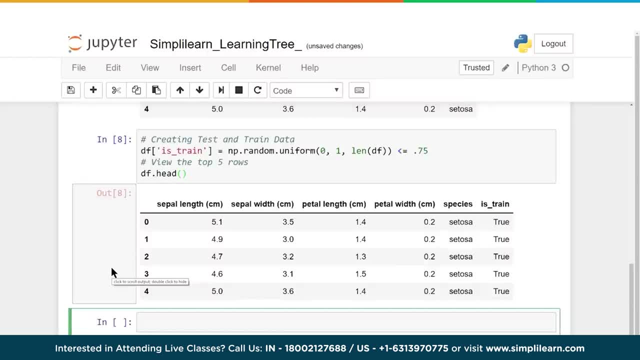 randomuniform. So we are generating a random number Between 0 and 1.. And we are going to do it for each of the rows. That is where the length df comes from. So each row gets a generated number And if it is less than .75, it is true. 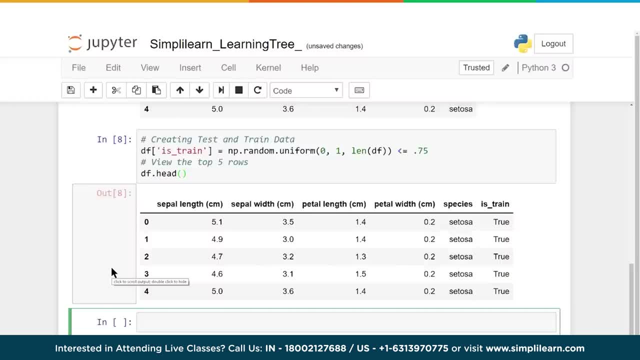 And if it is greater than .75 it is false. So we are going to take 75% of the data Roughly, Because there is a randomness involved And we are going to use that to train it, And then the other 25% we are going to hold off to the side. 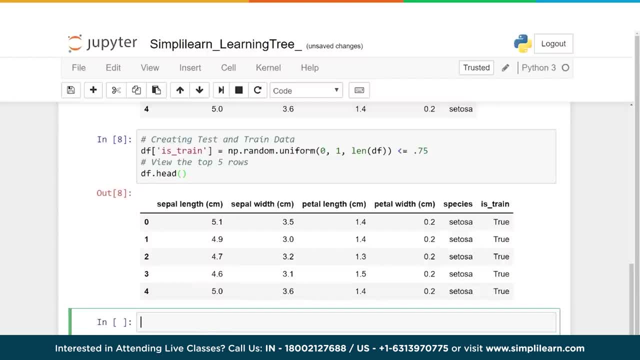 And use that to test it later on. So let's flip back over and see what the next step is. So, now that we have labeled our database For which is training and which is testing, Let's go ahead and sort that into two different variables. 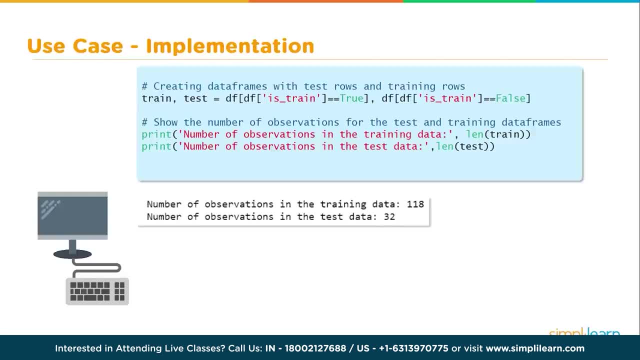 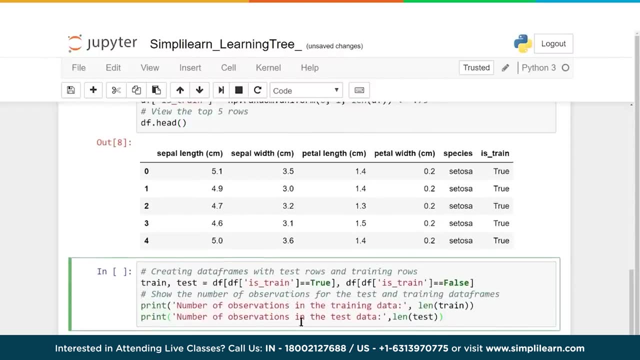 Train and test, And let's take this code And let's bring it into our project, And here we go, Let's paste it on down here. And before I run this, Let's just take a quick look at what is going on here. 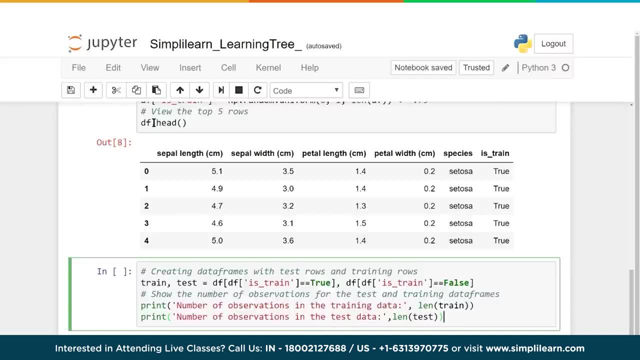 Is we have up above, We created- Remember, there is our defhead which prints the first five rows, And we have added a column: is train at the end, And so we are going to take that And we are going to create two variables. 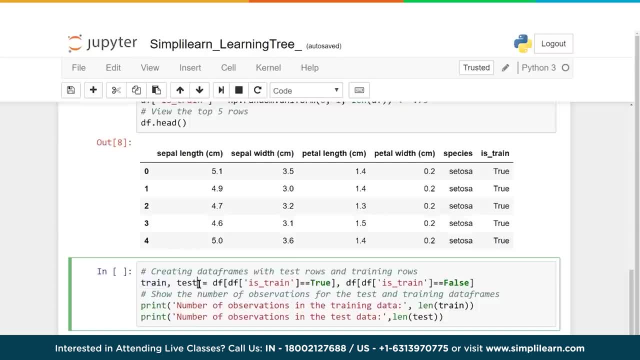 We are going to create two new data frames. One is called train, One is called test- 75% in train, 25% in test- And then to sort that out, We are going to do that by doing df, Our original data frame, with the iris data in it. 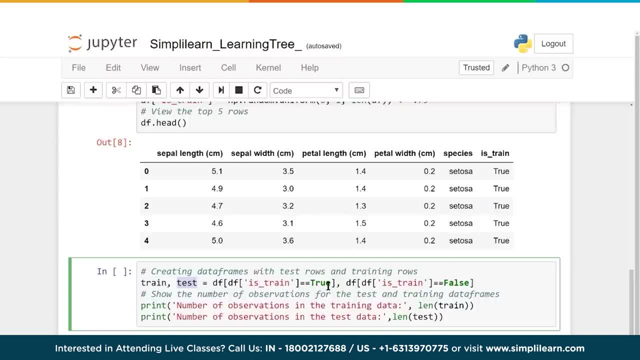 And if df is train equals true, That is going to go in the train, And if df is train equals false, It goes in the test, And so when I run this, We are going to print out the number in each one. Let's see what that looks like. 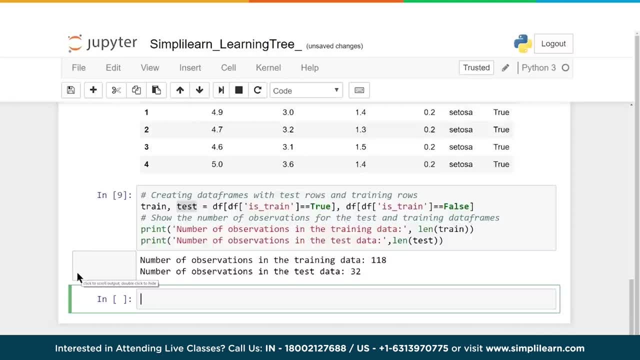 And you will see that it puts 118 in the training module And it puts 32 in the testing module, Which lets us know that there was 150 lines of data in here. So if you went and looked at the original data, You can see that there is 150 lines. 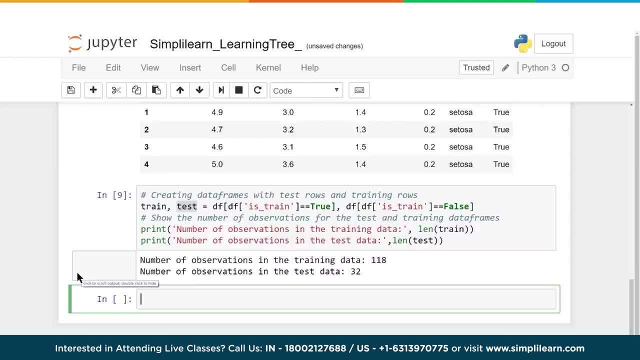 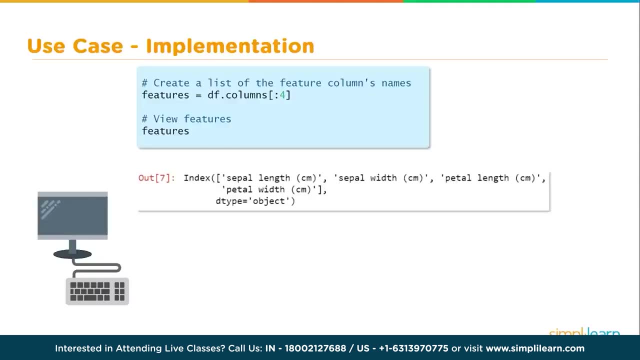 And that is roughly 75% in one And 25% for us to test our model on afterward. So let's jump back to our code And see where this goes. In the next two steps, We want to do one more thing with our data. 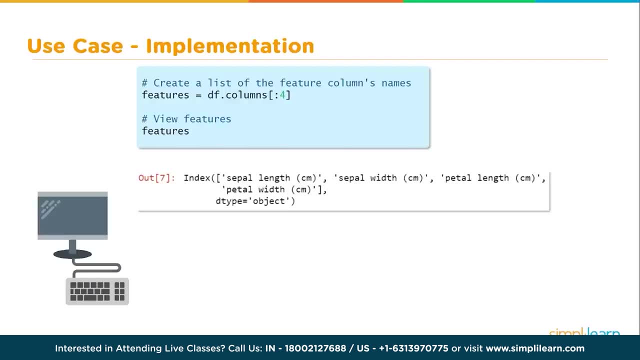 And that is, make it readable to humans. I don't know about you, But I hate looking at 0s and 1s, So let's start with the features And let's go ahead and take those And make those readable to humans. 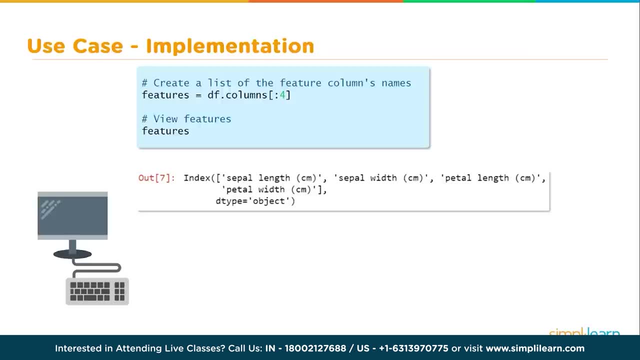 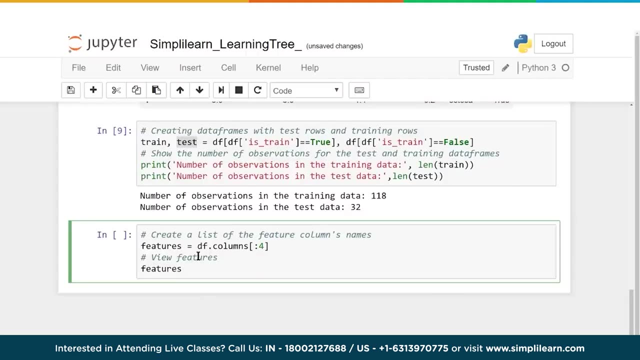 And let's put that in our code, And that is our model, And paste it in And you will see, here We have done a couple very basic things. We know that the columns in our data frame- Again, this is a panda thing. 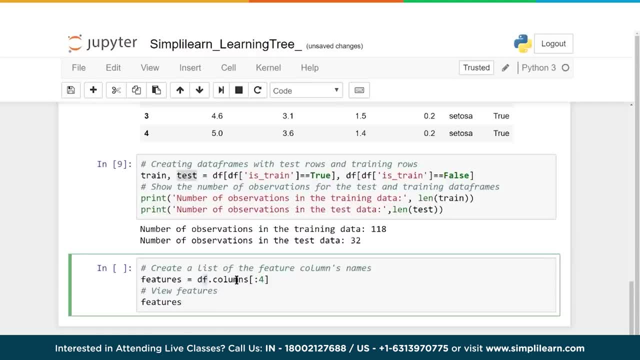 The DF columns And we know the first four of them: 0,, 1,, 2, 3.. That would be the first four- Are going to be the features Or the titles of those columns. So when I run this, 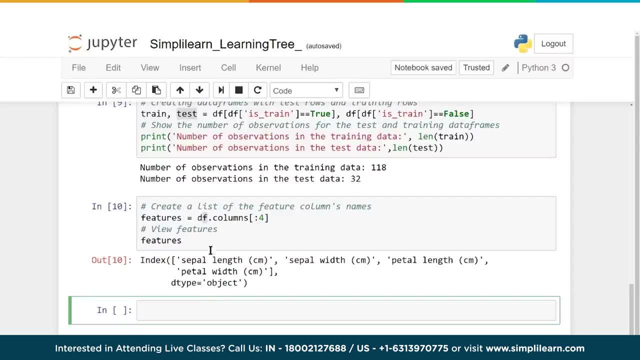 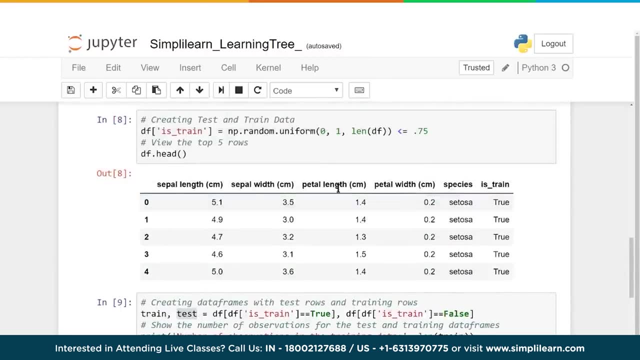 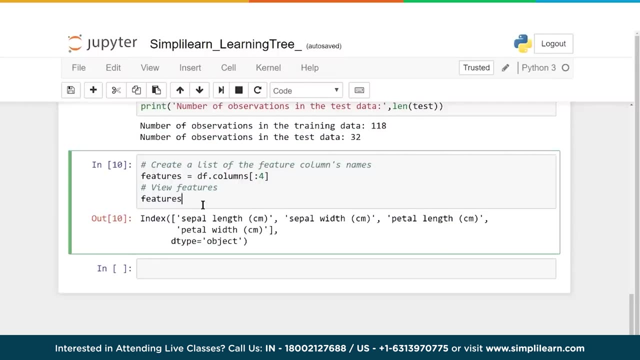 You will see down here That it creates an index- SEPA length And petal width- And this should be familiar Because if you look up here, Here is our column titles going across, And here is the first four. One thing I want you to notice here: 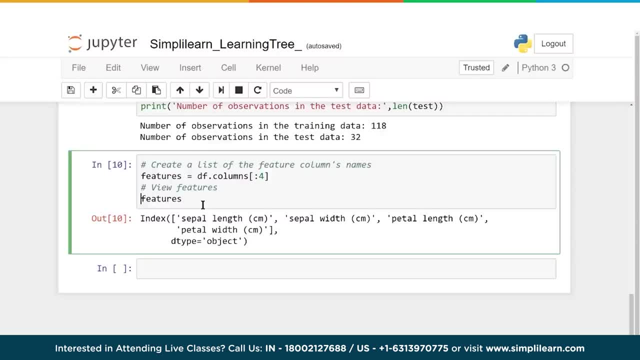 Is that when you are in a command line, Whether it is Jupyter Notebook Or you are running command line in the terminal window- If you just put the name of it It will print it out. This is the same as doing print features. 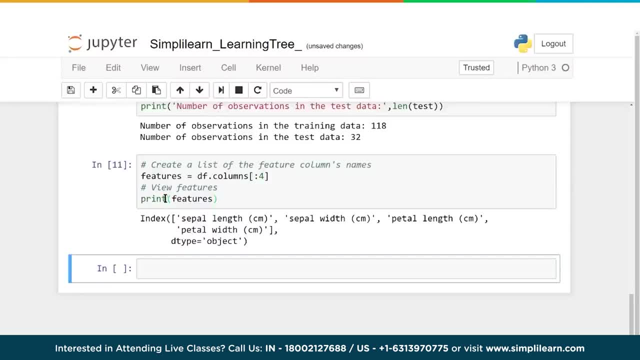 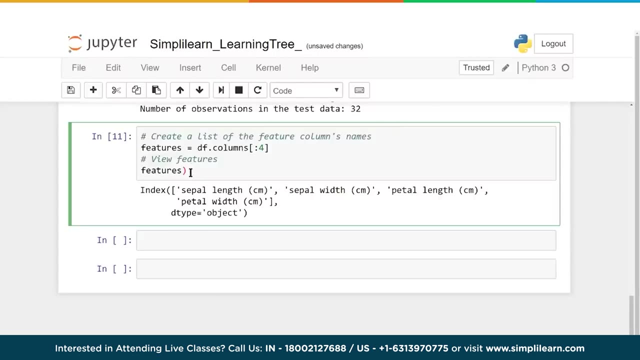 And the shorthand is You just put features in here. If you are actually writing a code And saving the script And running it by remote, You really need to put the print in there. But for this, When I run it, You will see it gives me the same thing. 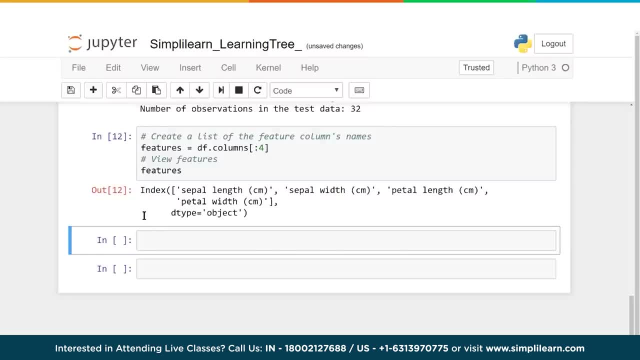 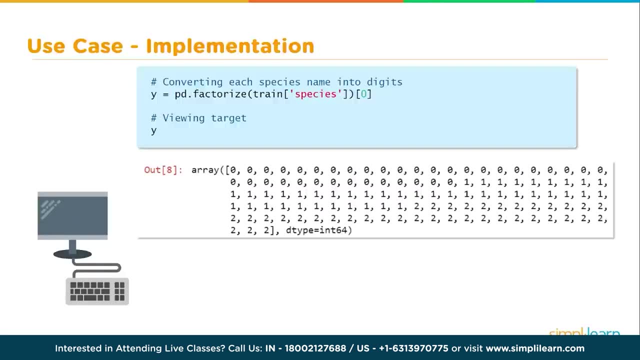 But for this We want to go ahead And we will just leave it as features Because it doesn't really matter, And this is one of the fun things about Jupyter Notebooks: I am just building the code as we go, And then we need to go ahead. 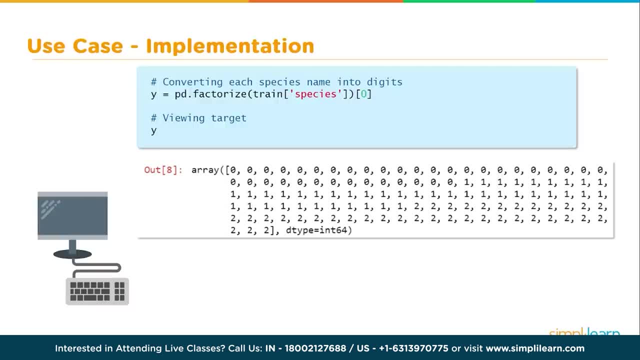 And create the labels for the other part, And then we are going to go ahead And convert the species on here Into something the computer understands. So let's put this code into our script And see where that takes us. Alright, Here we go. 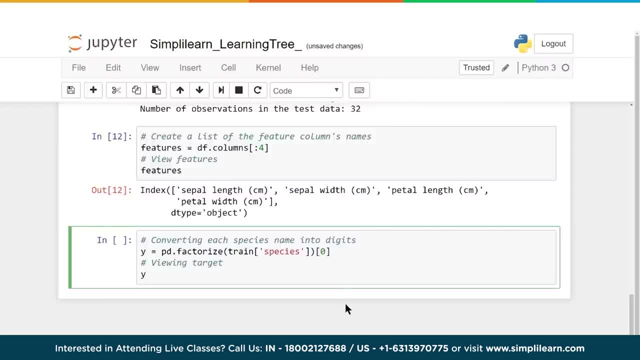 We have set y equal to pd. dot factorize- Train species of zero. So let's break this down just a little bit. We have our pandas Right here. PD Factorize: What is factorize doing? We are going to look at what train species is. 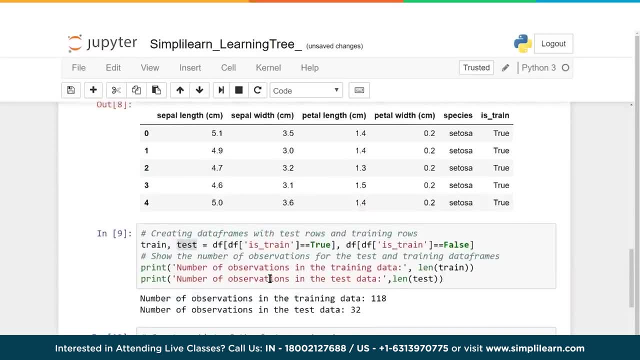 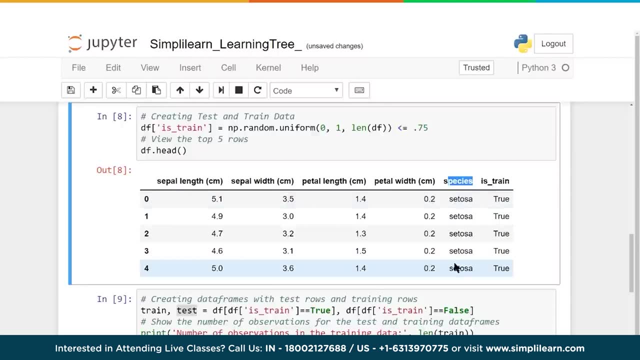 And why we are looking at the group zero on there And let's go up here And here is our species. Remember this: We created this whole column here For species And then it has setosa, setosa, setosa, setosa. 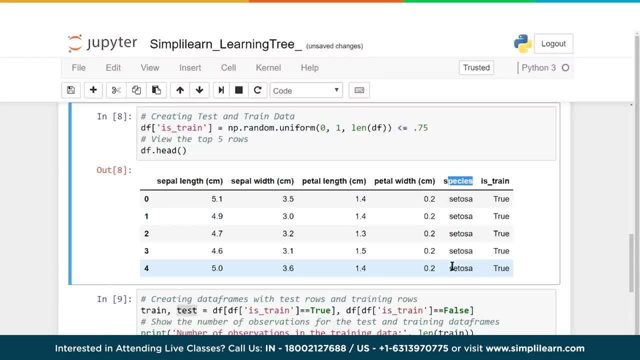 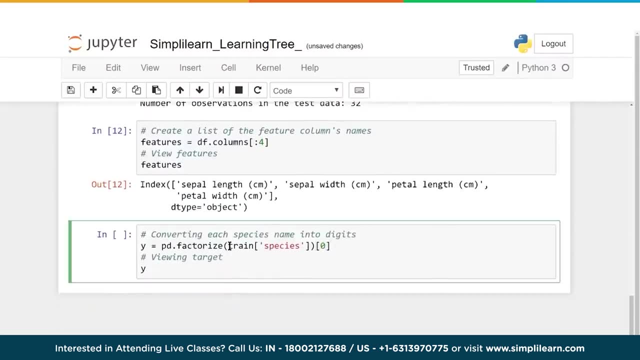 And if you scroll down enough, You would also see virginica And vericolor. We need to convert that into something the computer understands: Zeros and ones, So the train species Of zero. This is in the format of an array of arrays. 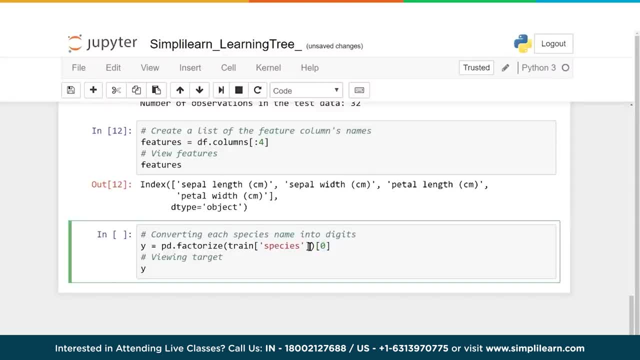 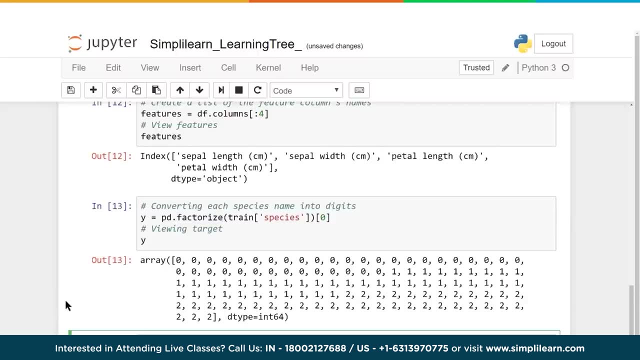 So you have to have the zero on the end And then species is just that column. Factorize Goes in there and looks at the fact That there is only three of them. So when I run this, You will see that y generates an array. 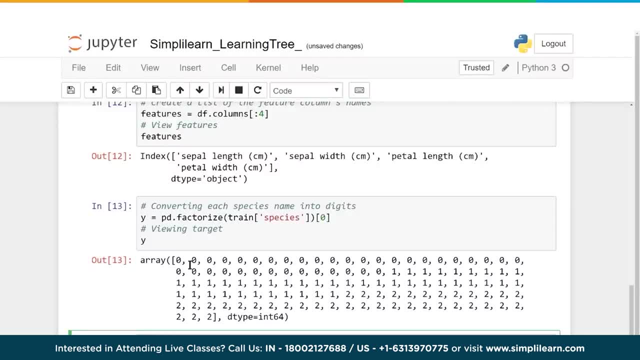 That is equal to. In this case it is the training set And it is zeros, ones and twos Representing the three different kinds of flowers we have. So now we have something the computer understands And we have a nice table That we can read and understand. 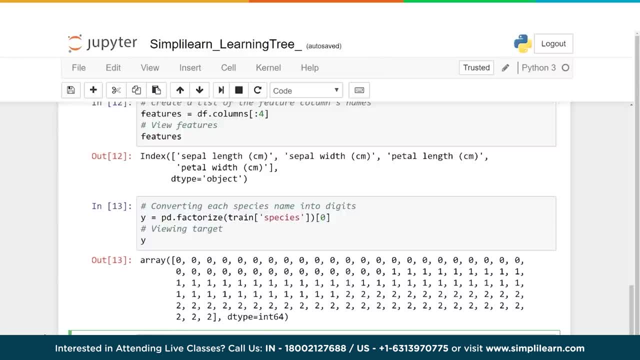 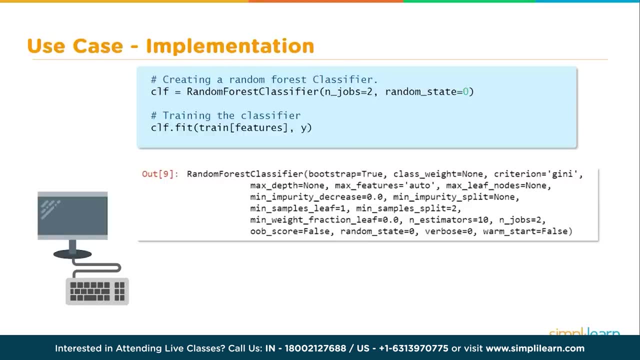 And now, finally, We get to actually start doing the predicting. So here we go. We have two lines of code. Oh, my goodness, that was a lot of work To get to two lines of code, But there is a lot in these two lines of code. 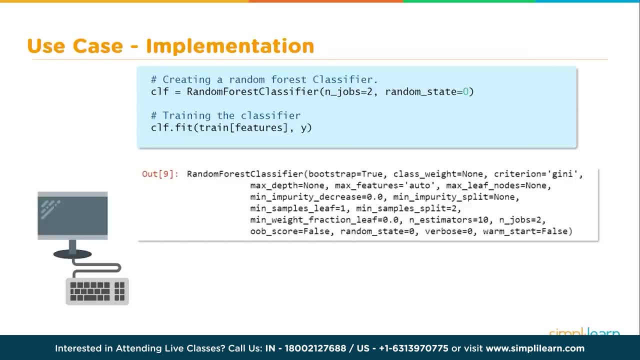 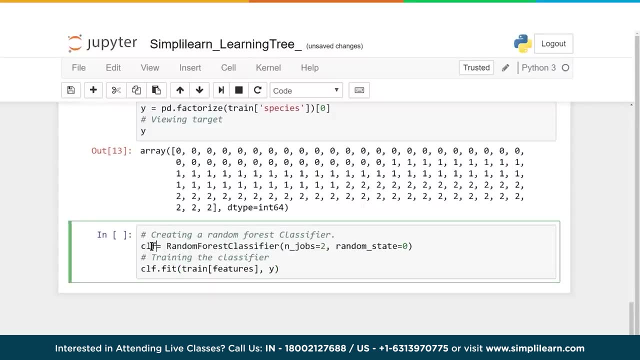 So let's take a look and see what is going on here And put this into our Full script that we are running. Let's paste this in here And let's take a look and see what this is. We are creating a variable clf. 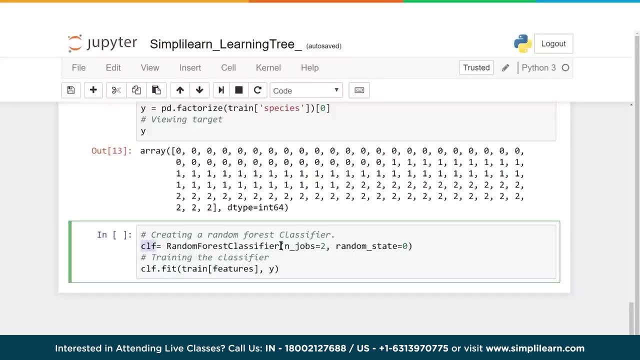 And we are going to set this Equal to the random forest class And we are passing two variables in here And there is a lot of variables You can play with. As far as these two are concerned, They are very standard In jobs. all that does is to prioritize it. 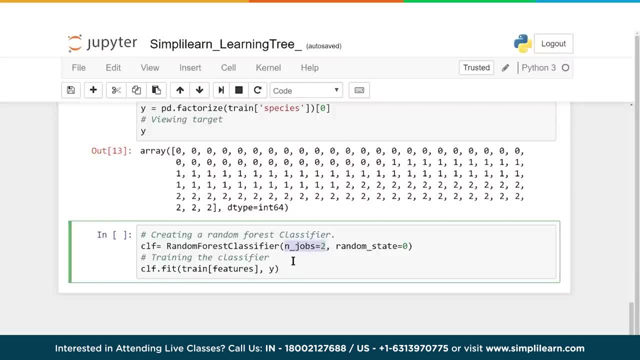 Not something to really worry about. Usually, when you are doing this on your own computer, You do in jobs equals two. If you are working in a larger or big data And you need to prioritize it differently, This is what that number does. 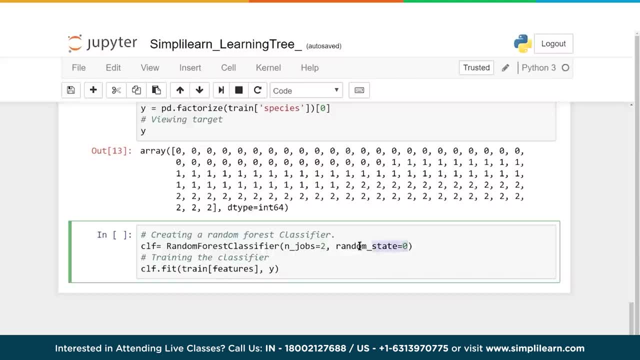 It changes your priorities And how it is going to run across the system And things like that. So that is fine for here, But let's go ahead and run this. We also have clffit train features comma y, And before we run it, 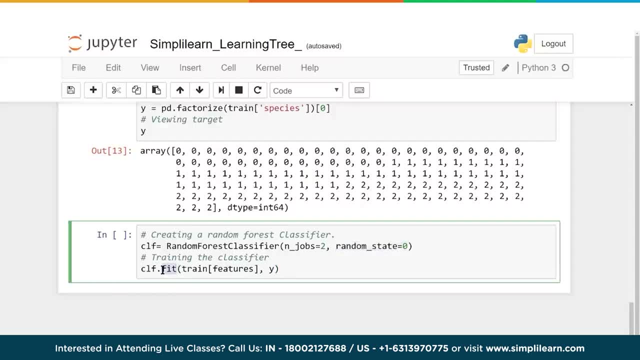 Let's talk about this a little bit more clffit. So we are fitting, We are training it. We are actually creating our random forest classifier right here. This is the code that does everything, And we are going to take our training set. 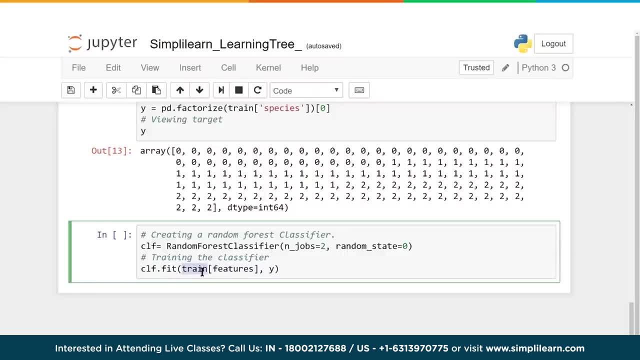 Remember, we kept our test off to the side And we are going to take our training set With the features, And then we are going to go ahead and put that in, And here is our target, The y. So the y is zero, one and two. 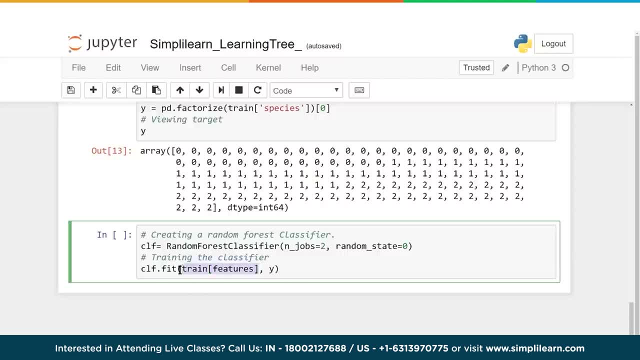 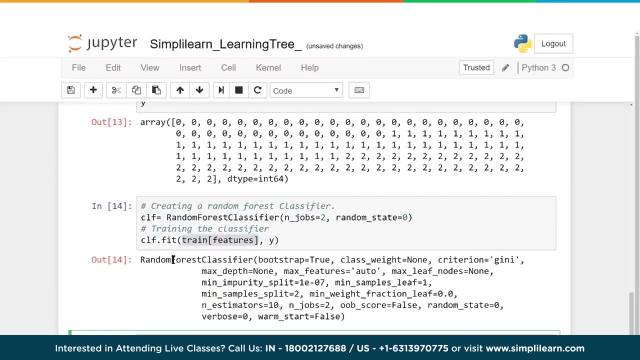 That we just created And the features. is the actual data going in That we put into the training set. Let's go ahead and run that. And this is kind of an interesting thing Because it printed out the random forest classifier And everything around it. 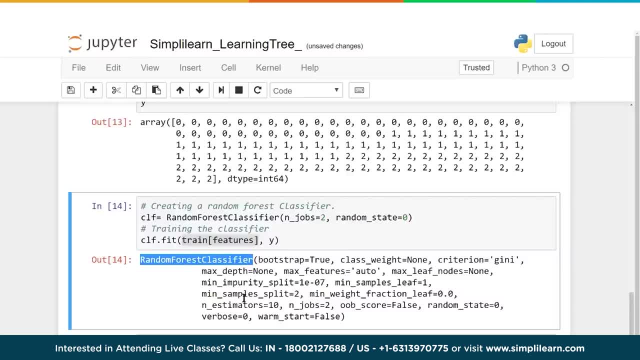 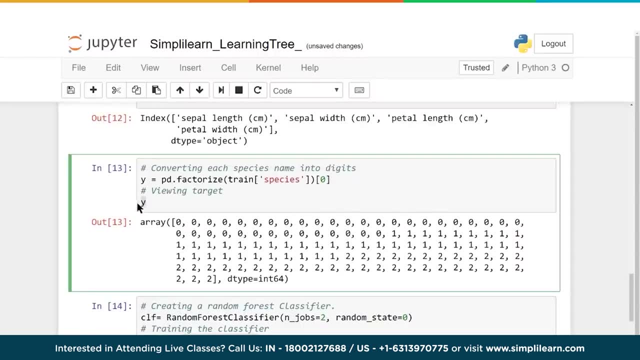 And so when you are running this In your terminal window Or in a script like this, This automatically treats this, Just like when we were up here And I typed in y And it printed out y instead of print y. This does the same thing. 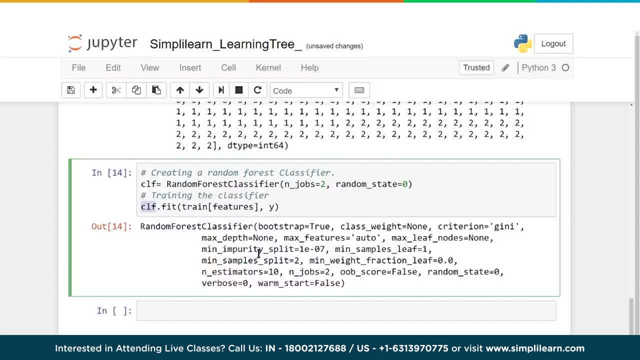 It treats this as a variable and prints it out. But if you were actually running your code, That wouldn't be the case. And what it has printed out Is: it shows us all the different variables we can change. And if we go down here, 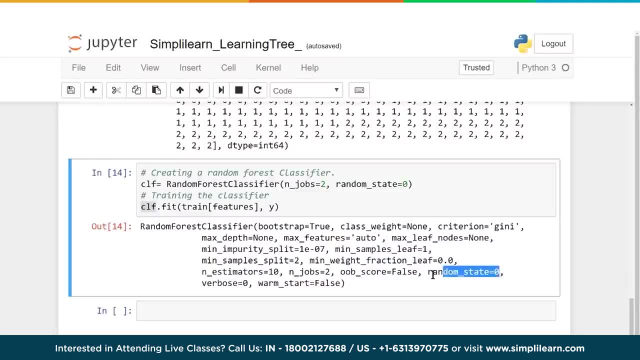 You can actually see in jobs equals two. You can see the random state equals zero. Those are the two that we sent in there. You would really have to dig deep And find out all these different meanings Of all these different settings on here. 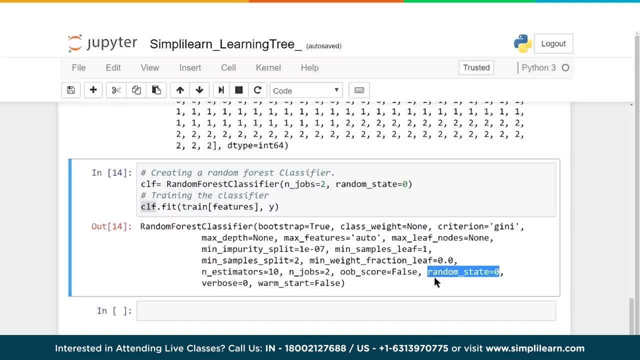 Some of them are self explanatory If you kind of think about it a little bit. Like max features is auto, So all the features that we are putting in there Is just going to automatically take all four of them. Whatever we send it, it will take. 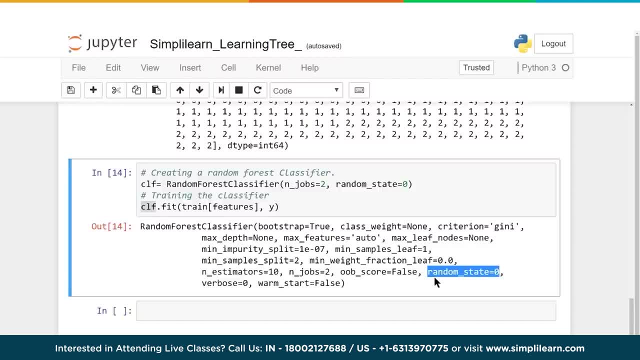 Some of them might have so many features Because you are processing words. There might be like 1.4 million features in there Because you are doing legal documents, And that is how many different words are in there. At that point you probably want to limit the maximum features. 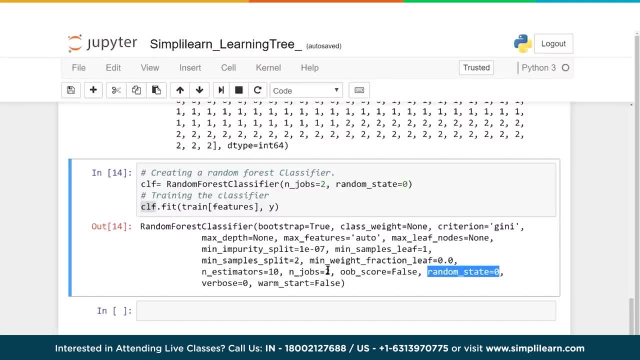 That you are going to process. Remember we had the fruit And we are talking about the leaf nodes. Like I said, there is a lot in this. We are looking at a lot of stuff here, So you might have- in this case There is probably only, I think- three leaf nodes. 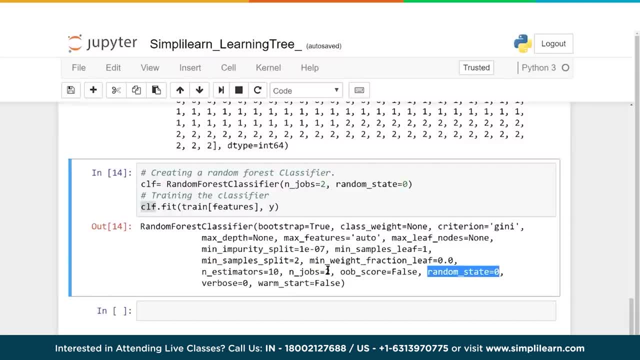 Maybe four. You might have thousands of leaf nodes, At which point you do need to put a cap on that And say, okay, you can only go so far, And then we are going to use all of our resources on processing this, And that really is what most of these are about. 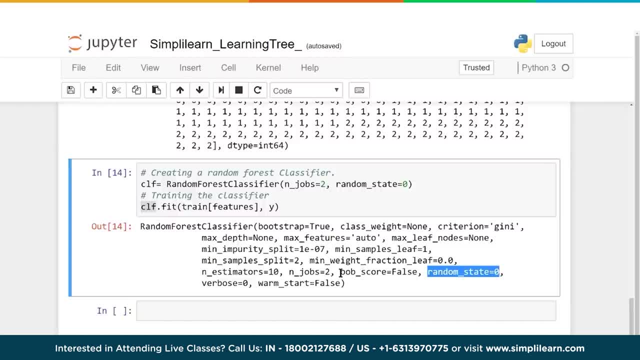 Is limiting the process And making sure we don't overwhelm a system, And there are some other settings in here. Warm start equals false, Warm start is if you are programming it one piece at a time Externally, Since we are not 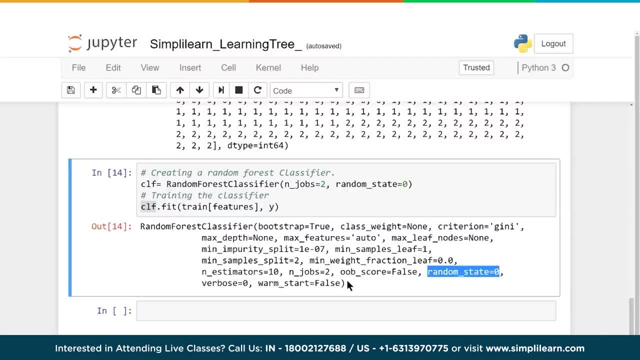 We are not going to continually train this particular learning tree And again, like I said, There is a lot of things in here That you will want to look up more detail from the sklearn And if you are digging in deep And running a major project on here. 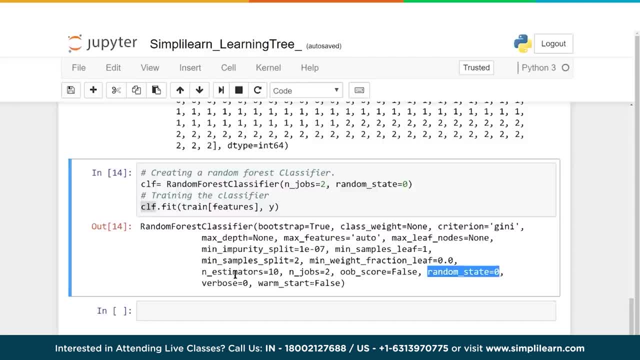 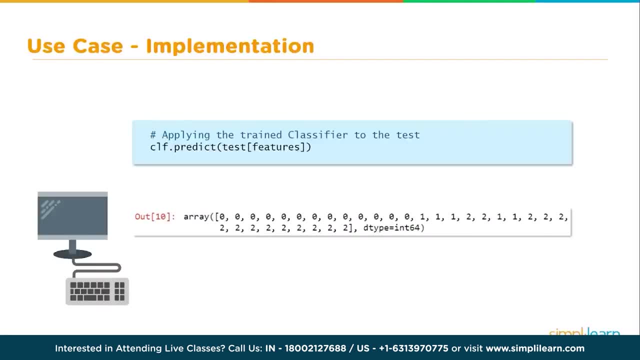 For today, though, All we need to do is fit or train our features And our target Y, So now we have our training model. What is next? We now need to test it. Remember, we set aside the test feature Test group. 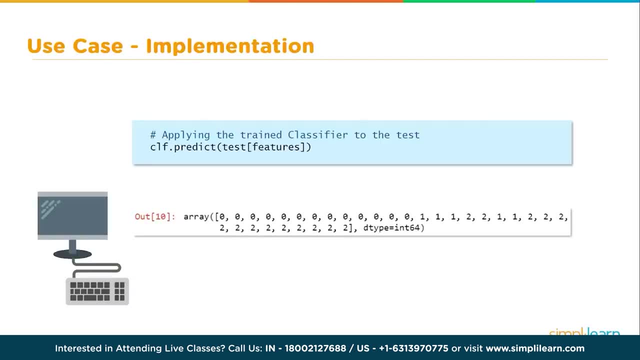 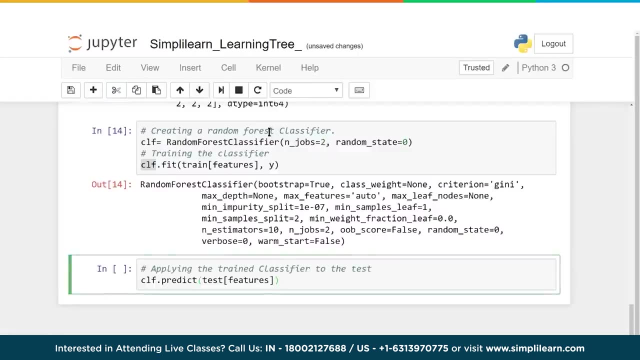 25% of the data. So let's go ahead and take this code And let's put it into our script And see what that looks like. Okay, here we go And we are going to run this And it is going to come out. 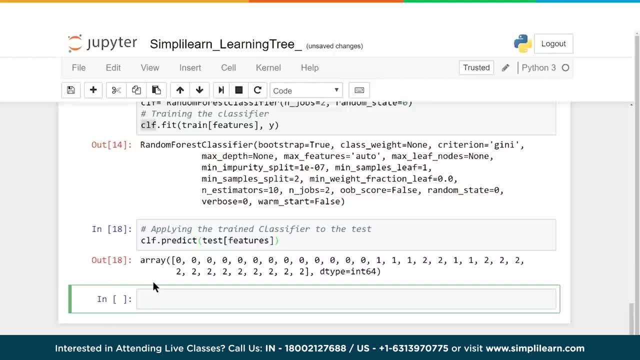 With a bunch of zeros, ones and twos, Which represents the three types of flowers: The setosa, the virginica and the versicolor. And what we are putting into our predict Is the test group. So we are going to test features. 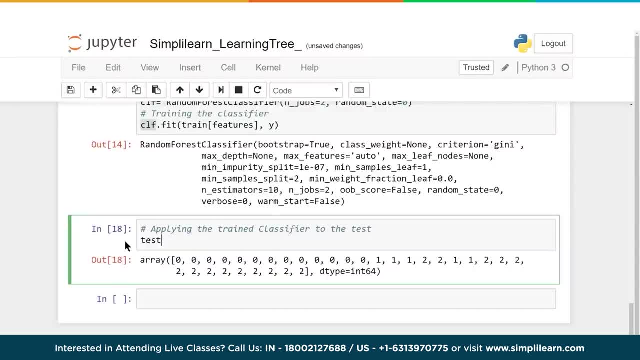 And I always like to know what it is. I am looking at. So real quick, We are going to do test features And remember features is an array Of sepal length, sepal width. Petal length- petal width. 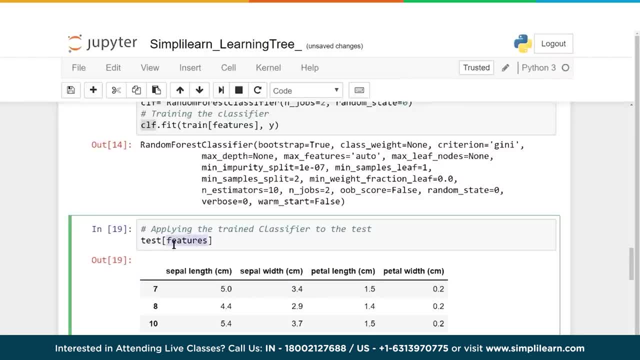 So when we put it in this way, It actually loads all these different columns That we loaded into features. So if we did just features, Let me just do features in here. See what features looks like With pandas data frames. You will see that it is an index. 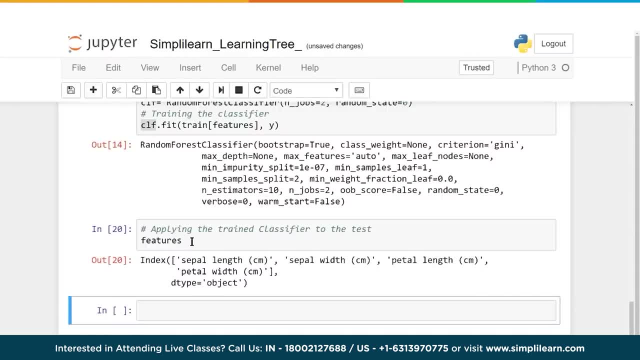 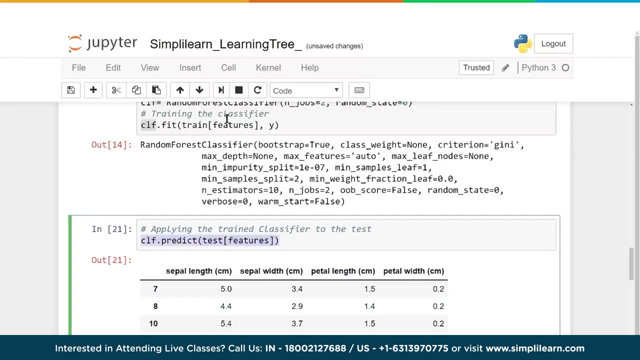 So when you put an index in like this- Into test features Into test- It then takes those columns And creates a panda data frames from those columns And in this case We are going to go ahead And put those into our predict. 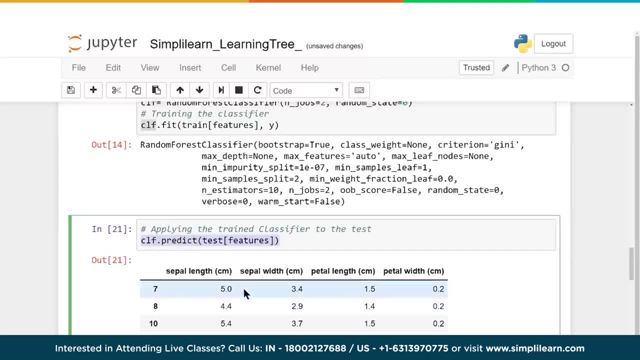 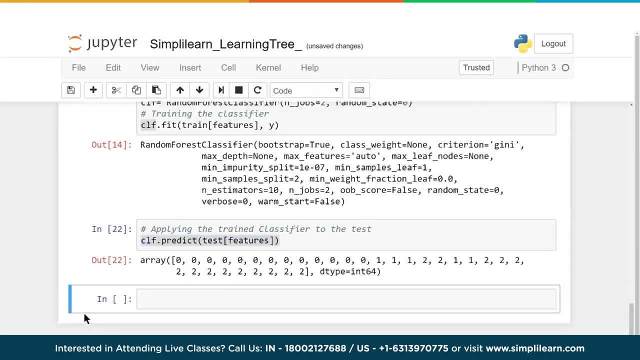 So we are going to put each one of these lines Of data- The 5.0,, 3.4,, 1.5, .2.. And we are going to put those in And we are going to predict What our new forest classifier. 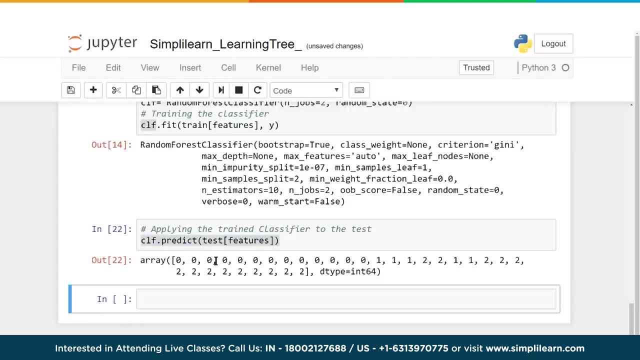 Is going to come up with, And this is what it predicts. It predicts 0, 0,, 0, 1, 2, 1, 1,, 2,, 2, 2.. And again, This is the flower type. 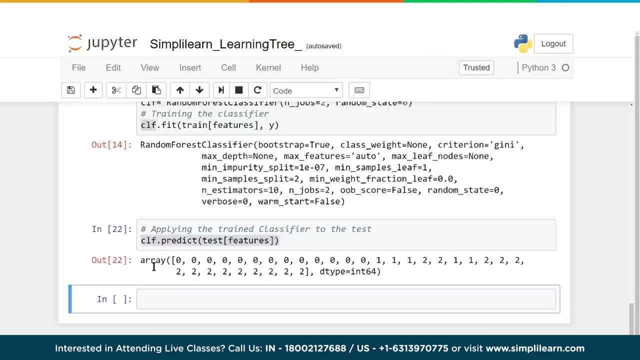 Satosa, virginica and versicolor. So now that we have taken our test features, Let's explore that. Let's see exactly What that data means to us. So the first thing we can do with our predicts Is we can actually generate. 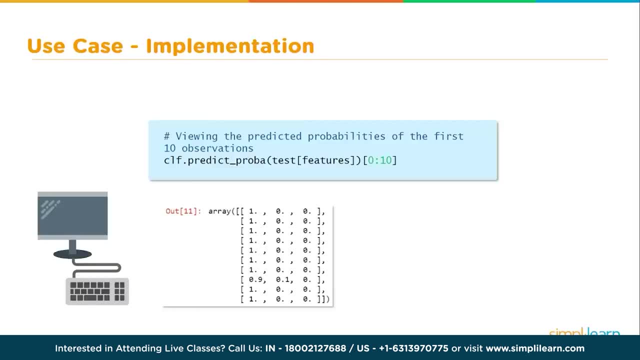 A different, predict, A prediction model. When I say different, We are going to view it differently. It is not that the data itself is different. So let's take this next piece of code And put it into our script. So we are pasting it in here. 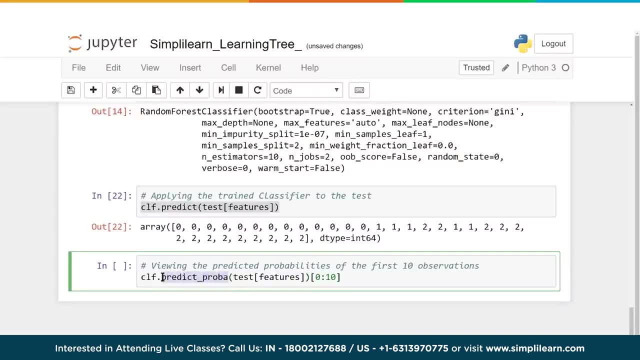 And you will see that we are doing predict And we have added underscore proba For probability. So there is our clfpredict probability. So we are running it Just like we ran it up here, But this time, With this, we are going to get a slightly different result. 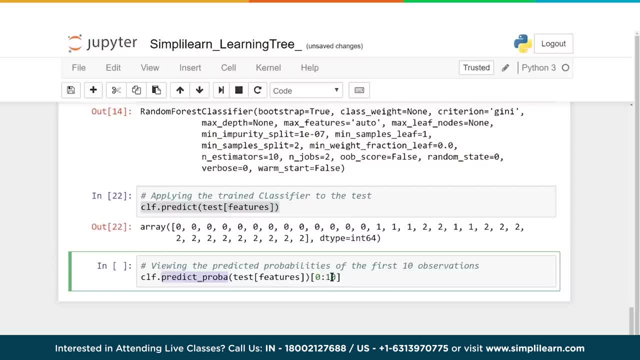 So you will see down here, Instead of looking at all of them, Which was what? 27.. You will see right down here That this generates a much larger field on the probability, And let's take a look and see what that looks like. 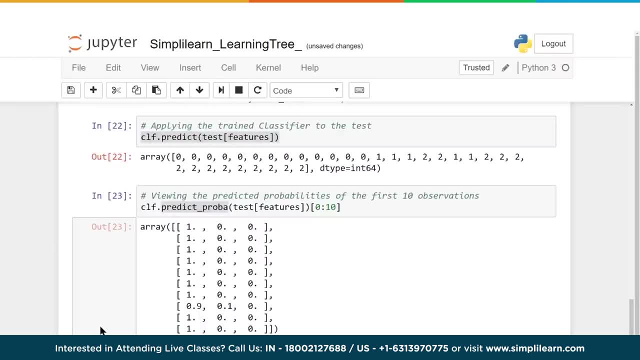 And what that means. So when we do the predict, Underscore, proba For probability, It generates three numbers. So we had three leaf nodes at the end And if you remember from all the theory we did, This is the predictors. 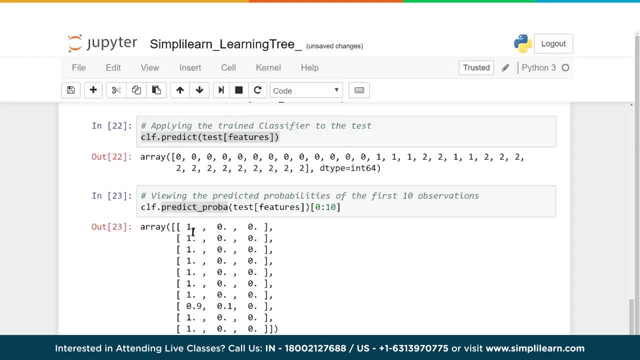 The first one is predicting For satosa. It predicts a zero for virginica, And it predicts a zero for versicolor, And so on, and so on, and so on. And let's You know what? I am going to change this just a little bit. 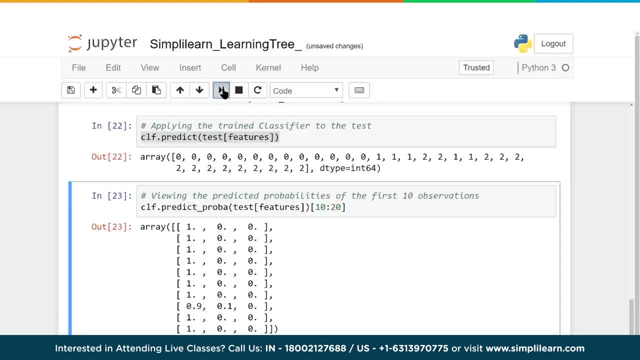 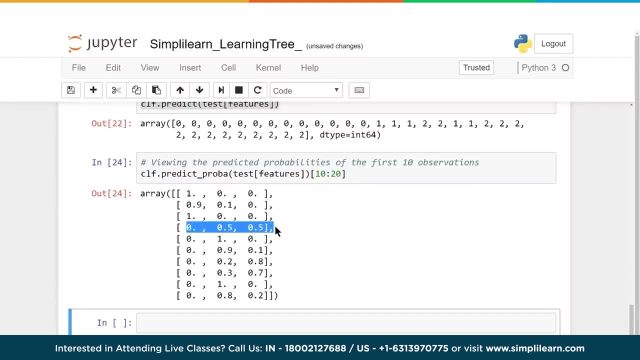 Let's look at 10 to 20.. Just because we can And we start to get a little different of data And you will see right down here It gets to this one, This line right here, And this line has 0,, 0.5,, 0.5. 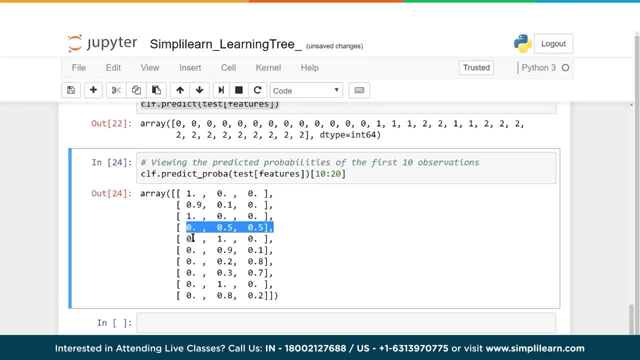 And so if we are going to vote And we have two equal votes, It is going to go with the first one. So it says satosa gets 0 votes, Virginica gets 0.5 votes, Versicolor gets 0.5 votes. 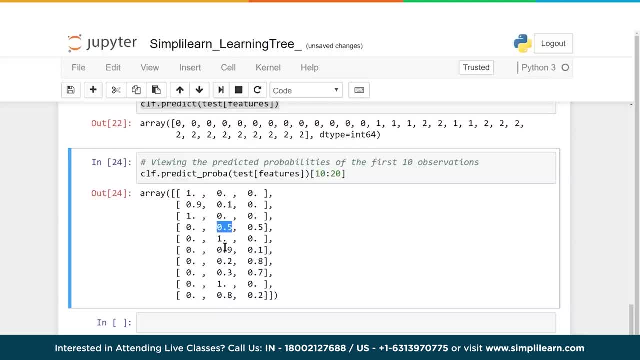 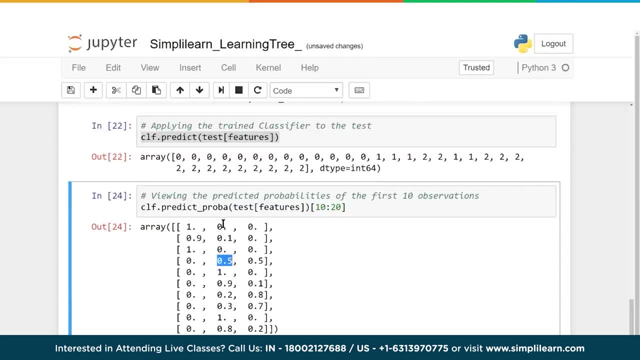 But let's just go with the virginica, Since these two are equal, And so on and so on. down the list You can see how they vary on here. So now we have looked at both. How to do a basic predict of the features. 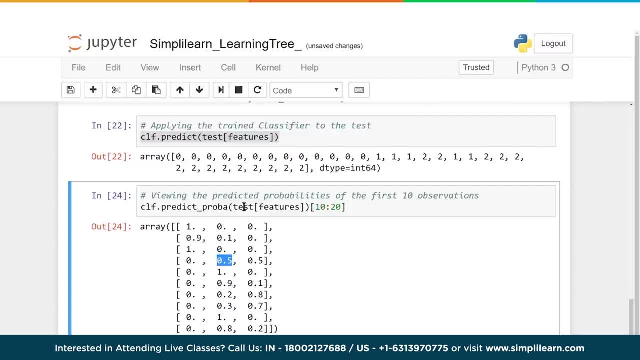 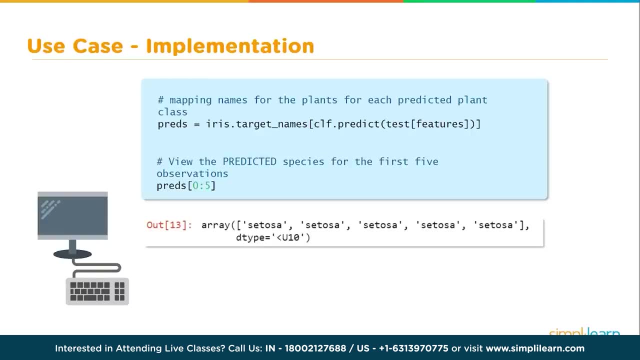 And we have looked at the predict probability. Let's see what is next on here. So now we want to go ahead And start mapping names for the plants. We want to attach names So that it makes a little more sense for us. 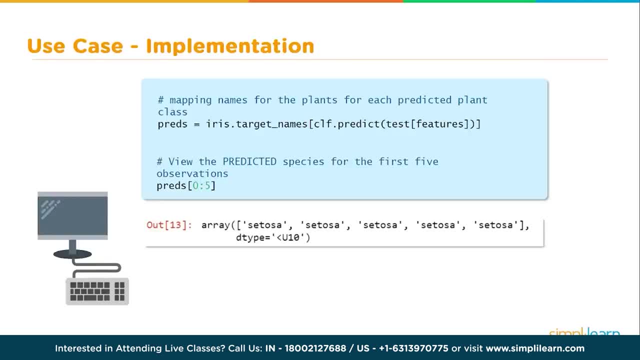 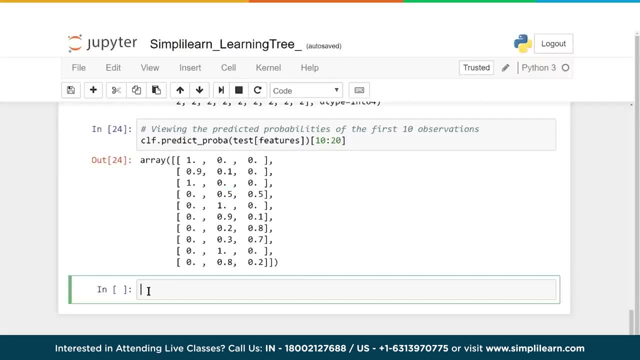 And this is what we are going to do in these next two steps. We are going to start by Setting up our predictions And mapping them to the names, So let's see what that looks like And let's go ahead and paste that code in here. 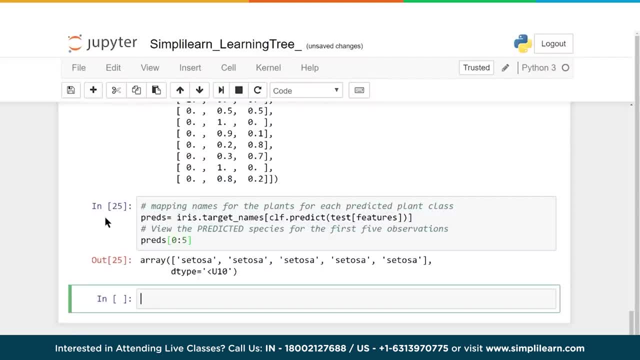 And run it, And this goes along with the next piece of code, So we will skip through this quickly And then come back to it a little bit. So here is iristargetnames, And if you remember correctly, This was the names. 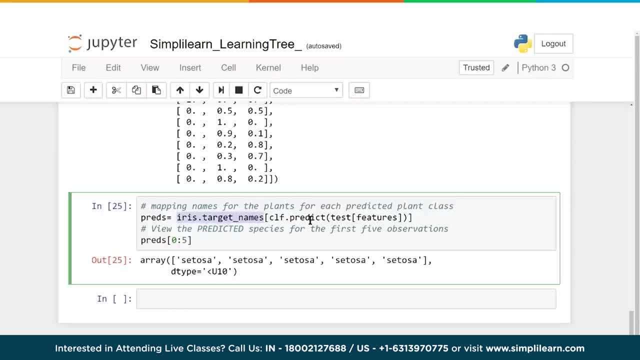 That we have been talking about this whole time, The setosa virginica versicolor. And then we are going to go ahead and do the prediction again. We could have just set a variable equal to this Instead of re-running it each time. 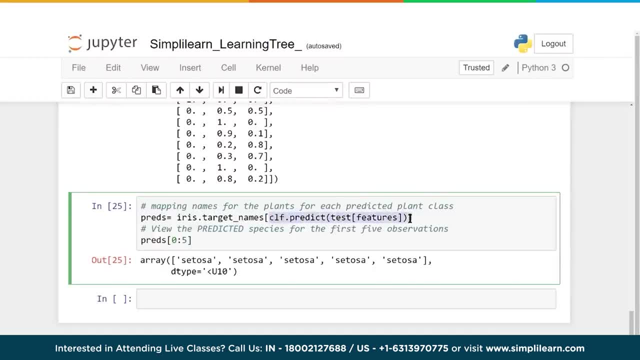 But we are going to go ahead and run it again: clfpredictTestFeatures- Remember that returns the 0s, the 1s and the 2s, And then we are going to set that equal to predictions. So this time we are actually putting it in a variable. 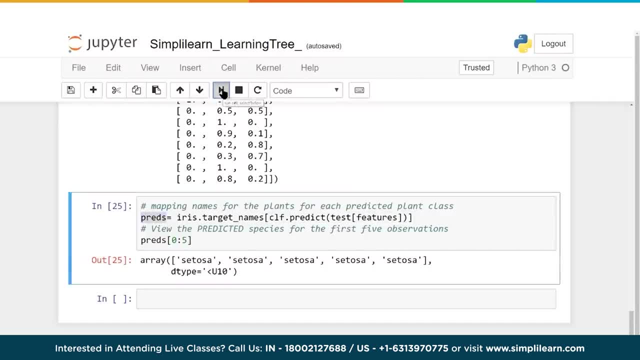 And when I run this, It distributes, It comes out as an array And then it returns as a variable And the array is: setosa, setosa, setosa, setosa, setosa. We are only looking at the first 5.. 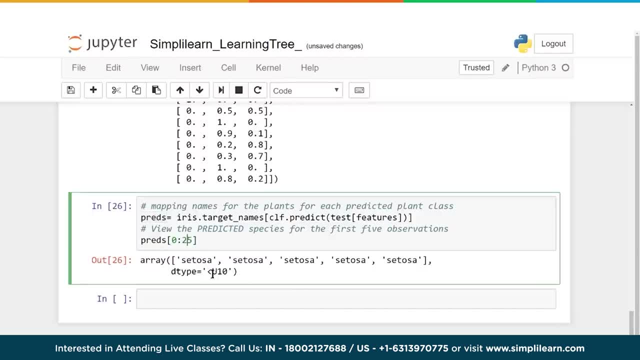 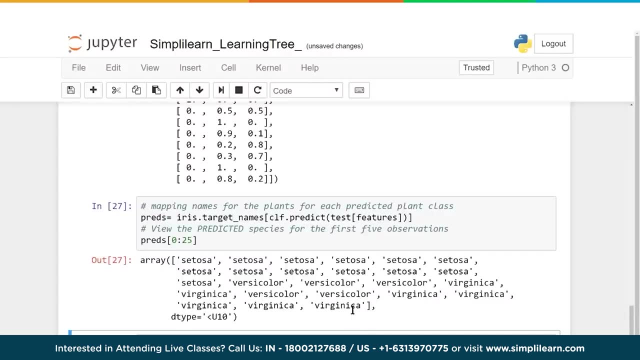 We could actually do. Let's do the first 25.. Just so we can see a little bit more on there, And you will see that it starts mapping it To all the different flower types: The versicolor and the virginica in there. 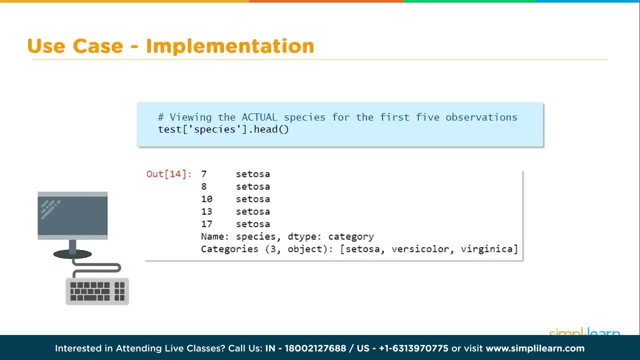 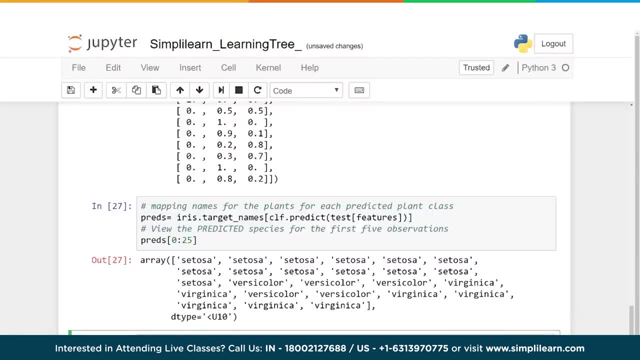 And let's see how this goes with the next one. So let's take a look at the top part of our species in here And we will take this code and put it in our script. And let's put that down here and paste it. 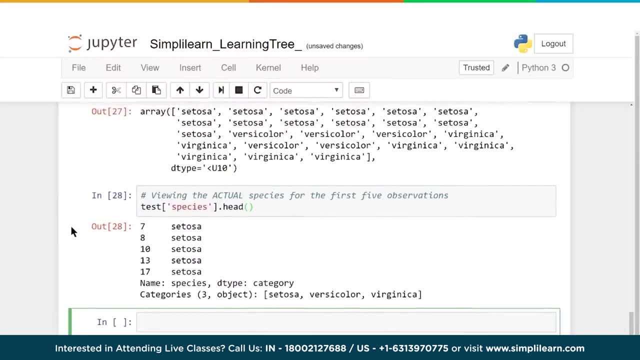 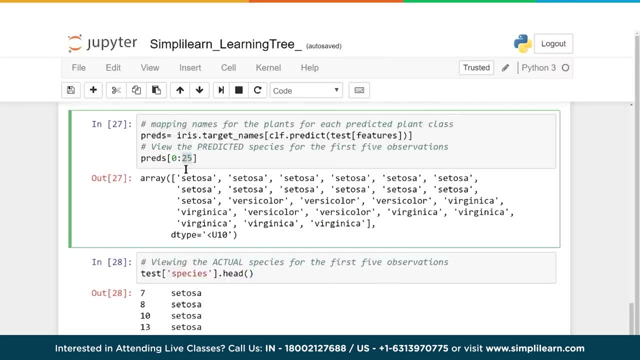 There we go, And let's talk about both these sections of code here And how they go together. The first one Is our predictions, And I went ahead and did predictions through 25.. Let's just do 5. And so we have setosa, setosa, setosa, setosa. 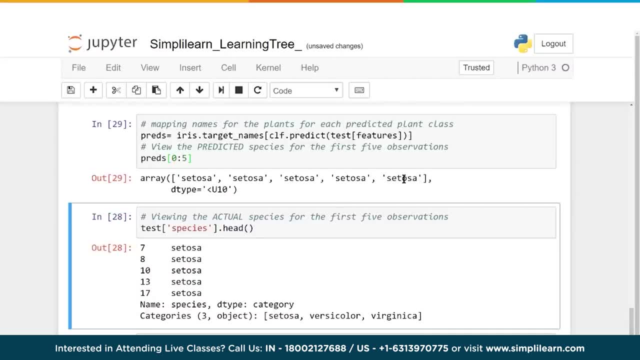 That is what we are predicting from our test model. And then we come down here And we look at test species And remember I could have just done testspecieshead And you will see it says setosa, setosa, setosa, setosa. 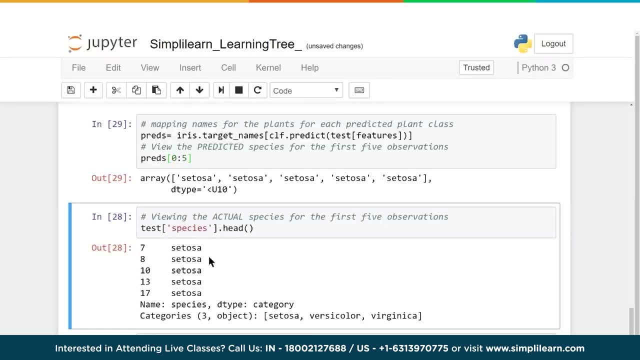 And they match, And they match, And they match. So the first one is what our forest is doing. So the first one is what our forest is doing, And the second one is what the actual data is. And the second one is what the actual data is. 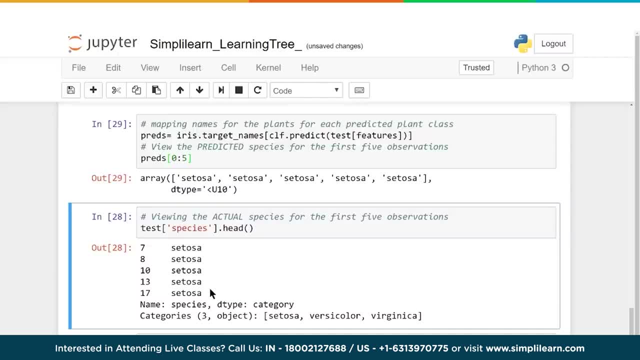 Now we need to combine these so that we can understand what that means. Now we need to combine these so that we can understand what that means. We need to know how good our forest is, How good it is at predicting the features. So that is where we come up to the next step. 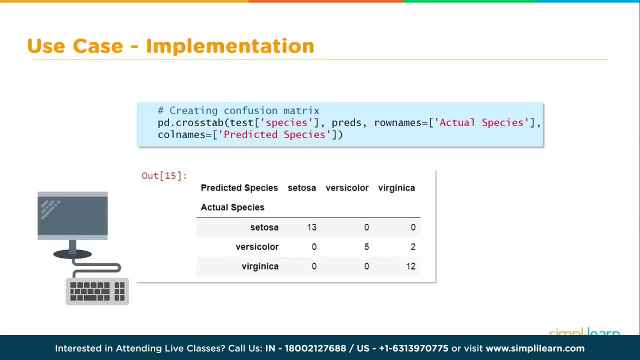 Which is lots of fun. We are going to use a single line of code To combine our predictions and our actuals, So we have a nice chart to look at And let's go ahead and put that in our script In our Jupyter notebook here. 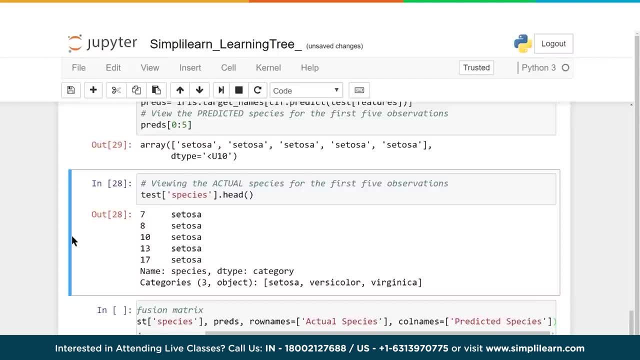 Let's see, Let's go ahead and paste that in. Because I am on the Jupyter notebook, I can do a control minus. Because I am on the Jupyter notebook, I can do a control minus. You can see the whole line there. 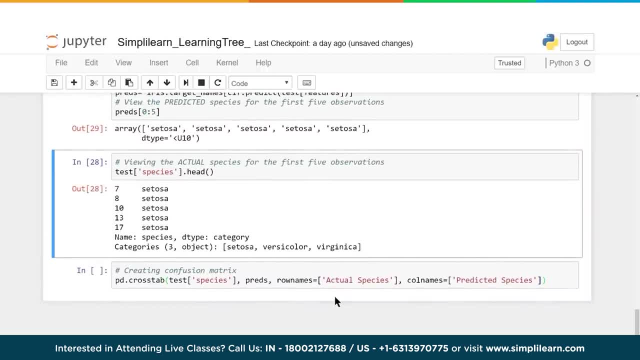 There we go, Resize it And let's take a look and see what is going on here. We are going to create in pandas- Remember, PD stands for pandas- And we are doing a cross tab. This function takes two sets of data. 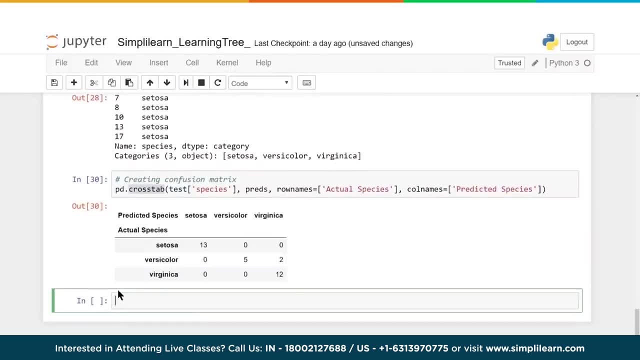 And creates a chart out of them. So when I run it you will get a nice chart down here And we have the predicted species. And we have the predicted species. So across the top you will see the Cetosa versicolor virginica. 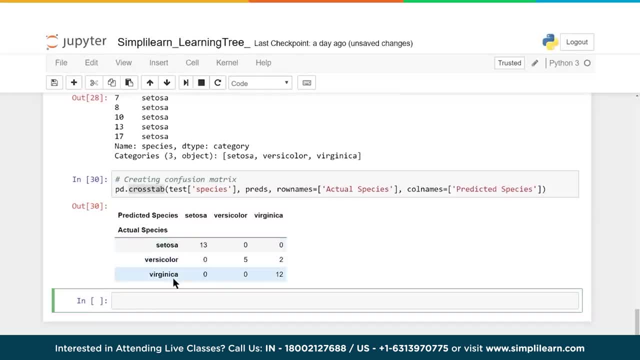 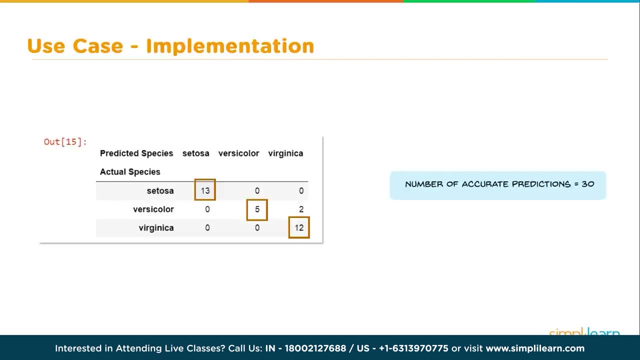 And the actual species, Cetosa versicolor virginica. And so the way to read this chart. Let's go ahead and take a look at how to read this chart here. When you read this chart, You have Cetosa where they meet. 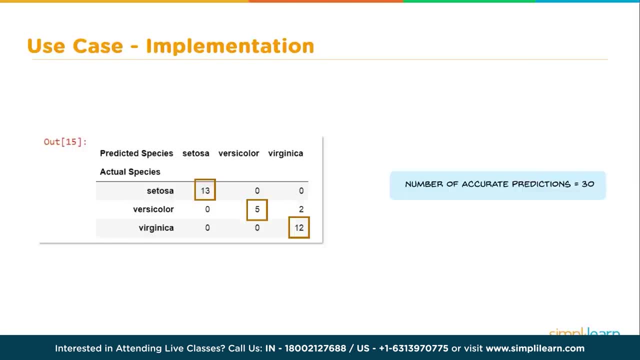 You have versicolor where they meet, And you have virginica where they meet, And they are meeting where the actual and the predicted agree. So this is the number of accurate predictions. So in this case it equals 30.. If you add 13 plus 40.. 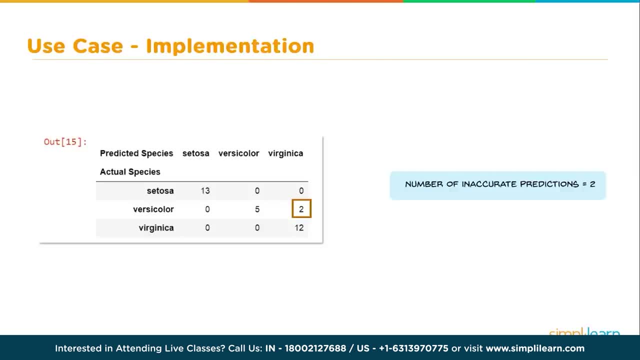 35 plus 12, you get 30. And then we notice here where it says virginica, but it was supposed to be versicolor. This is inaccurate. So now we have 2. 2 inaccurate predictions And 30 accurate predictions. 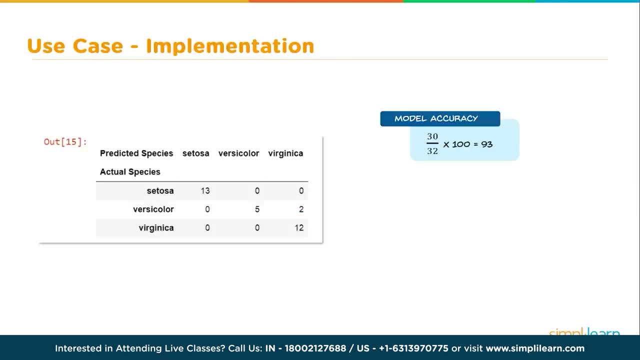 So we will say that the model accuracy is 93. That's just 30 divided by 32. And if we multiply it by 100. We can say that it is 93% accurate. So we have a 93% accuracy with our model. 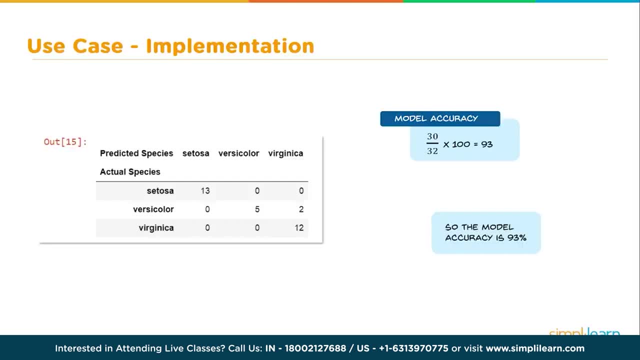 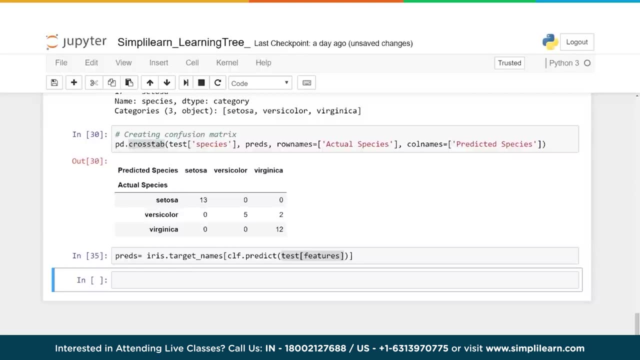 I did want to add one more quick thing in here on our scripting Before we wrap it up. So let's flip back on over to my script In here. we are going to take this line of code from up above. I don't know if you remember it. 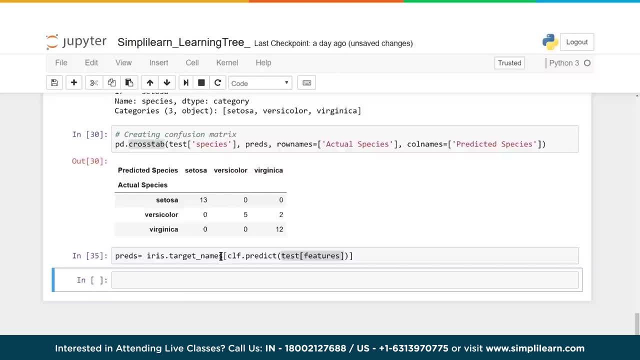 But predicts equals the iris dot target underscore names. So we are going to map it to the names And we are going to run the prediction And we read it on test features. But you know, we are not just testing it, We want to actually deploy it. 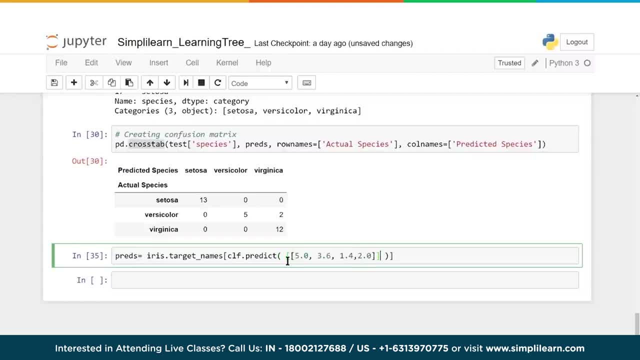 So at this point I would go ahead and change this, And this is an array of arrays. This is really important When you are running these to know that. So you need the double brackets And I could actually create data. Let's just do two flowers. 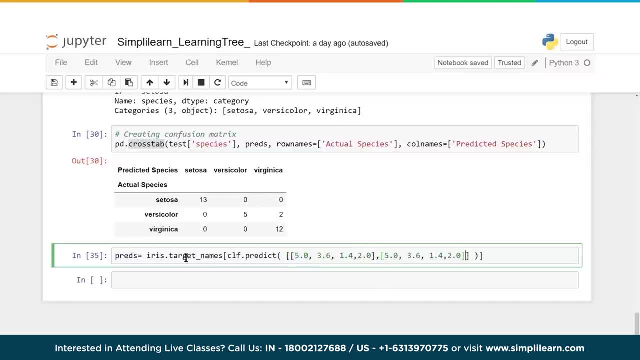 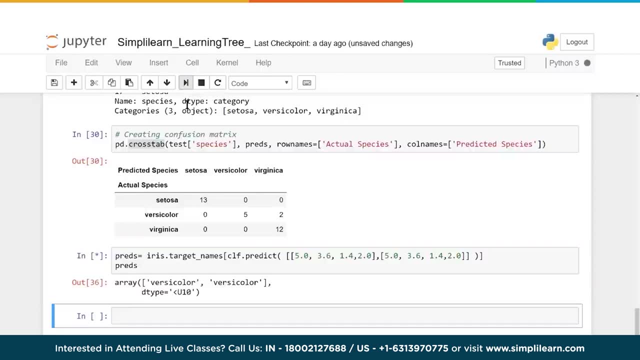 So maybe I am processing more data coming in And we will put two flowers in here, And then I actually want to see what the answer is. So let's go ahead and type in Preds and print that out. And when I run this, 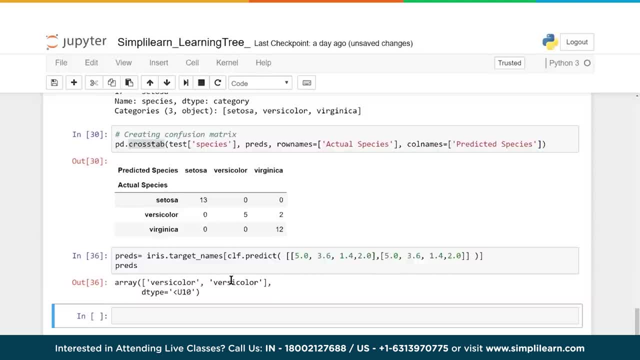 You will see that I have now predicted two flowers That maybe I measured in my front yard As Versicolor and Versicolor Not surprising, So let's put the same data in for each one. This would be the actual end product going out. 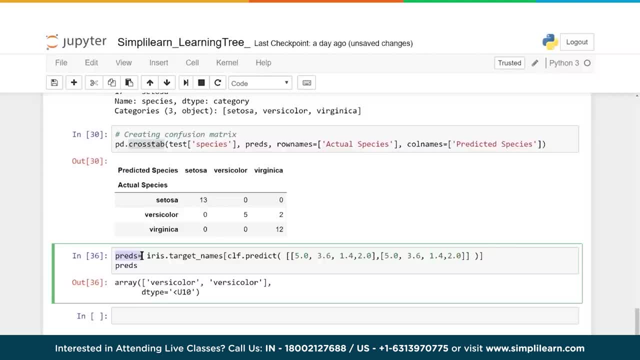 to be used on data that you don't know the answer for. So that is going to conclude our scripting part of this, And let's just go ahead and take a look at the key takeaways with today's tutorial, If you want to become an AI expert, 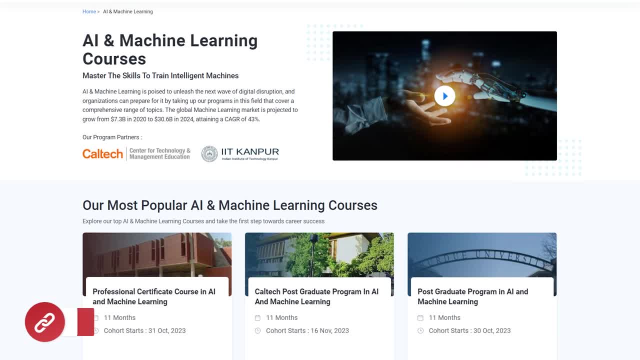 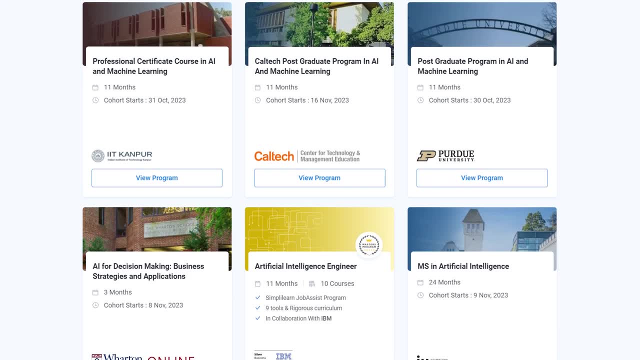 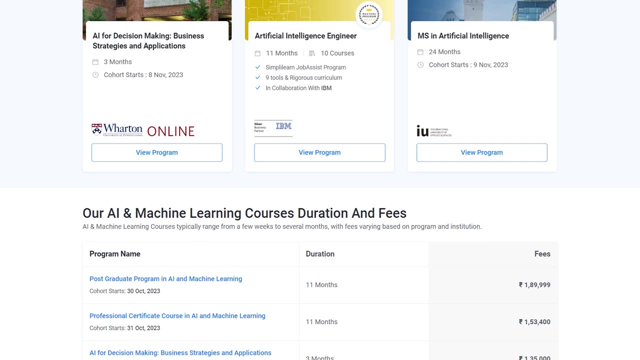 and get handsome salary packages. Look at the wide range of AI ML courses by Simdela in collaboration with top universities across the globe, And even in any of these certification programs, You will gain expertise in skills like Generative AI, Prompt Engineering, ChatGPT. 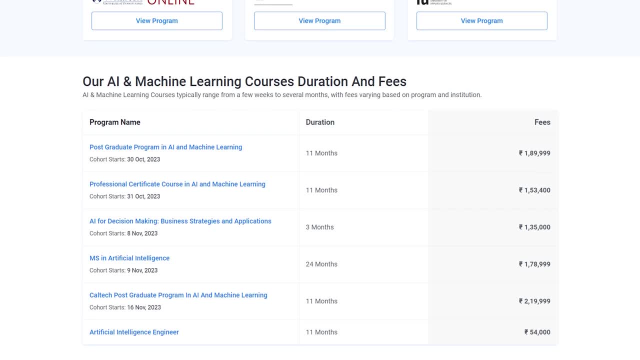 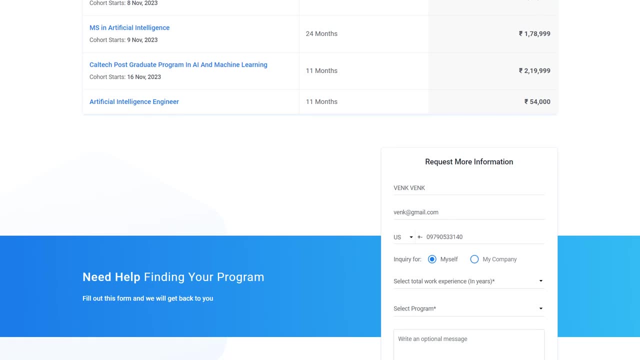 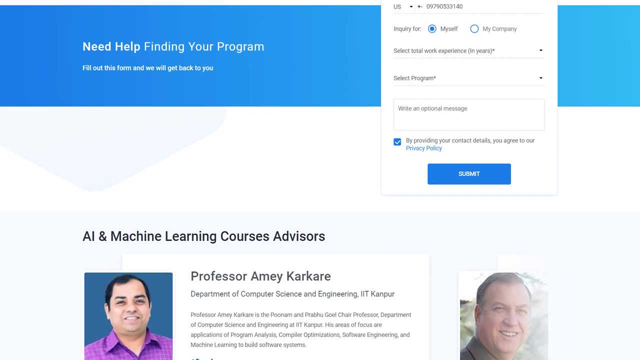 Explainable AI, Machine Learning Algorithms, Supervised and Unsupervised Learning, Model Training and Optimization, And there is much more on the list With hands on experience in the tools like ChatGPT, DALI, Python, OpenCV and TensorFlow. 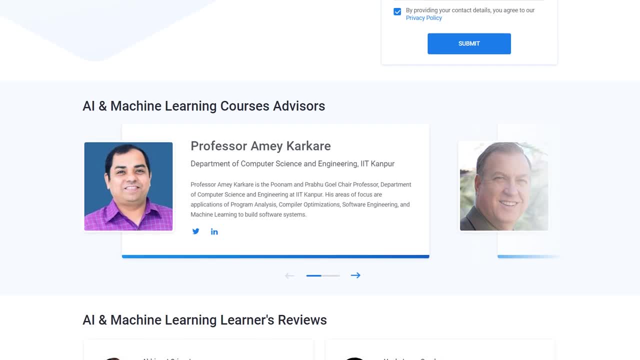 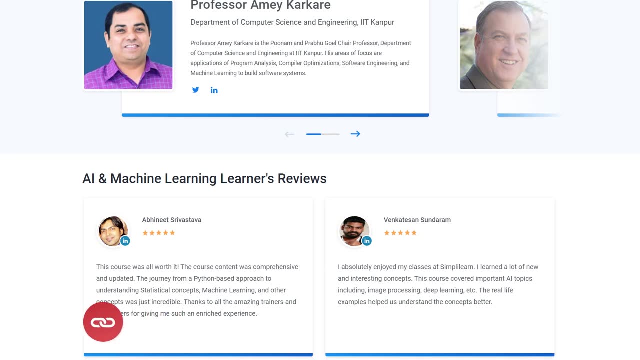 You will catch the eyes of top recruiters. So what are you waiting for Then? enroll now. An year of experience is preferred to enroll in these courses. Find the course link in the description box By now. we all know machine learning models make predictions by learning from the 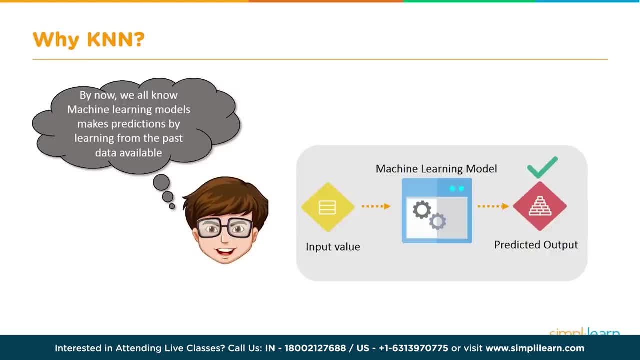 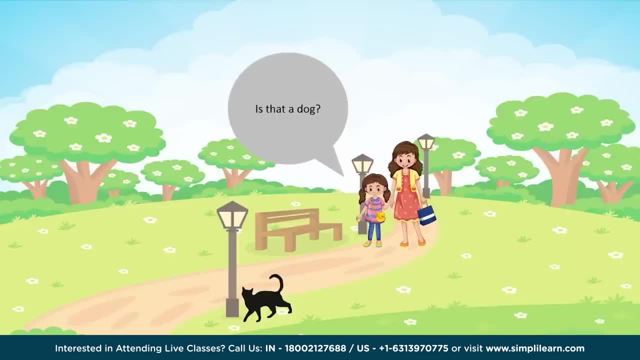 past data available. So we have our input values. our machine learning model builds on those inputs of what we already know and then we use that to create a predicted output. Is that a dog, Little kid, looking over there watching the black cat cross their path? 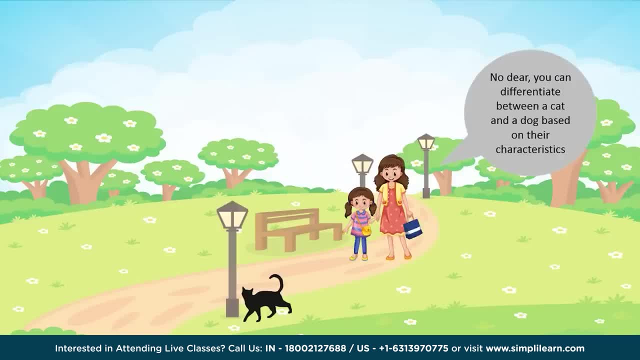 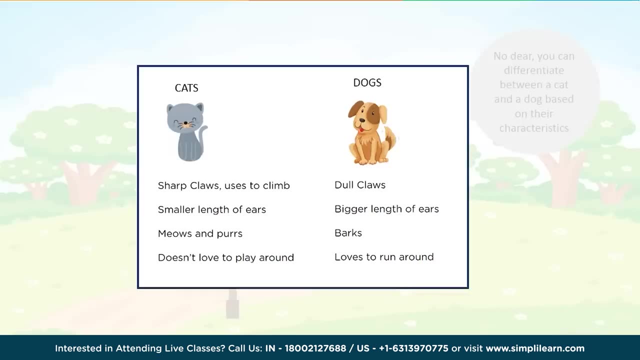 No dear, you can differentiate between a cat and a dog based on their characteristics. Cats: Cats have sharp claws, uses to climb, smaller length of ears, meows and purrs. doesn't love to play around. Dogs have dull claws. 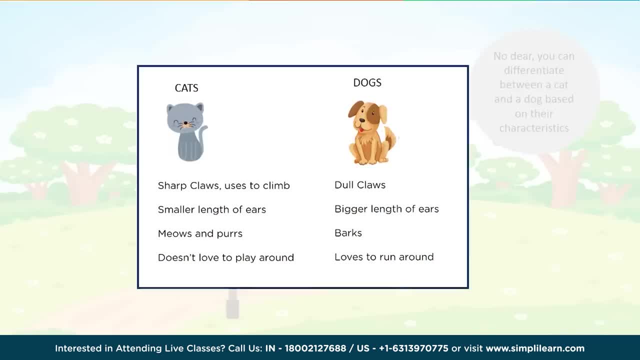 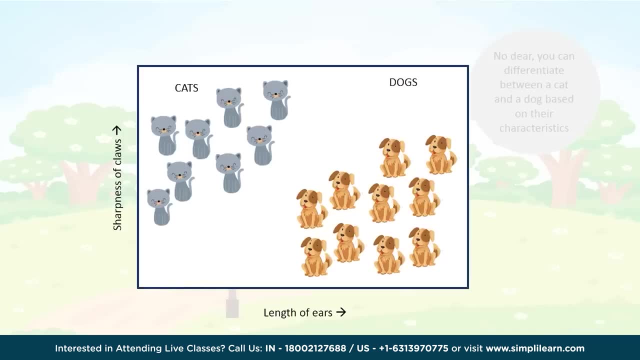 bigger length of ears. barks, loves to run around. You usually don't see a cat running around people, although I do have a cat that does that where dogs do, And we can look at these. we can evaluate the sharpness of the claws. 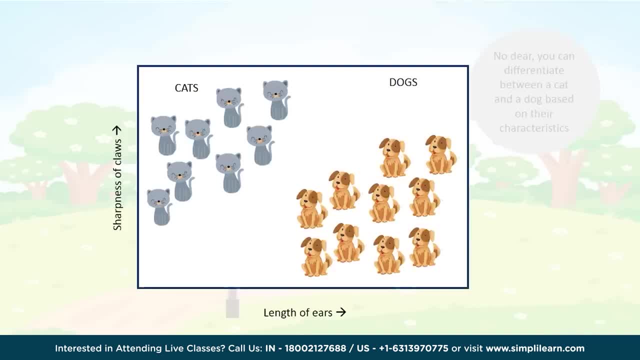 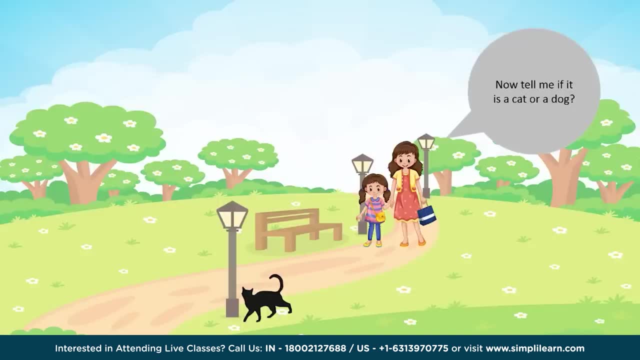 and we can usually sort out cats from dogs based on even those two characteristics. Now tell me if it is a cat or a dog. Now I'd question. usually little kids know cats and dogs by now, Unless they live in a place where there's not many cats or dogs. 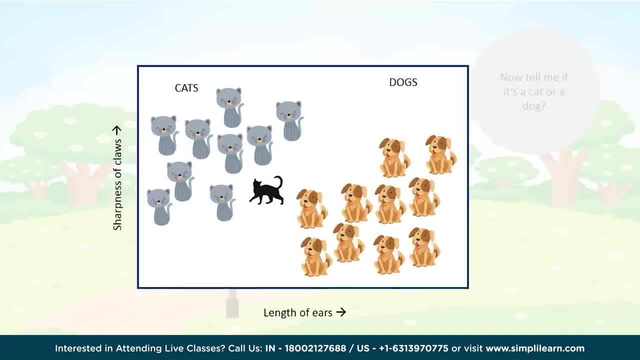 So if we look at the sharpness of the claws, the length of the ears, and we can see that the cat has smaller ears and sharper claws than the other animals, Its features are more like cats. it must be a cat: Sharp claws, length of ears. 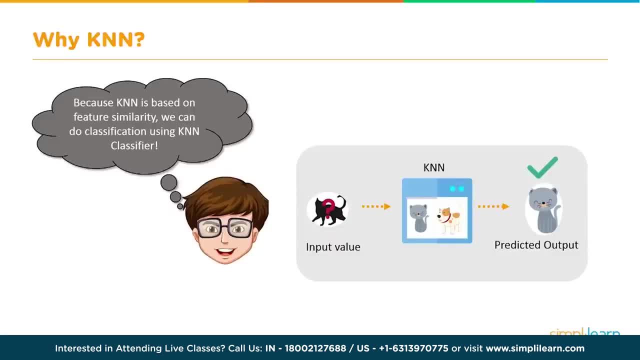 and it goes in the cat group. If KNN is based on feature similarity, we can do classification using KNN classifier. So we have our input value, the picture of the black cat. it goes into our trained model and it predicts that this is a cat coming out. 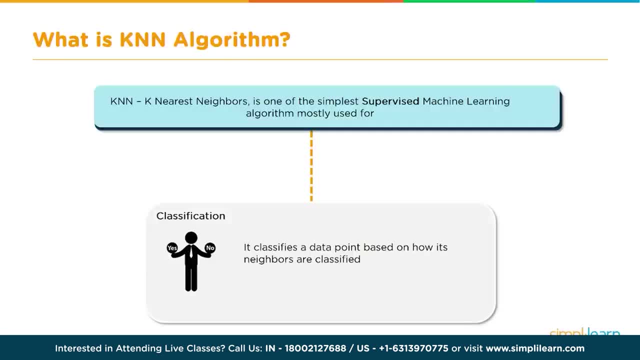 So what is KNN? What is the KNN algorithm? K nearest neighbors is what that stands for. It's one of the simplest supervised machine learning algorithms mostly used for classification. So we want to know: is this a dog or it's not a dog? 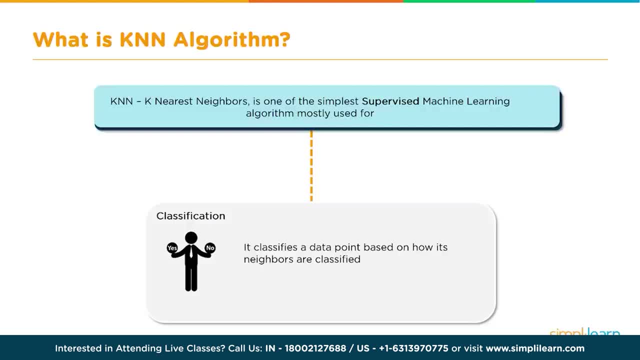 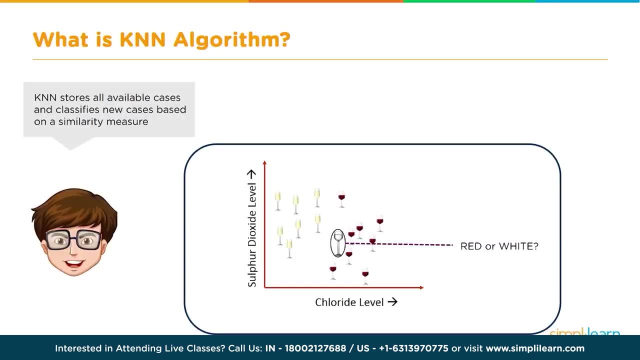 Is this a cat or not a cat? It classifies a data point based on how its neighbors are classified. KNN stores all available cases and classifies new cases based on a similarity measure. And here we've gone from cats and dogs right into wine, another favorite of mine. 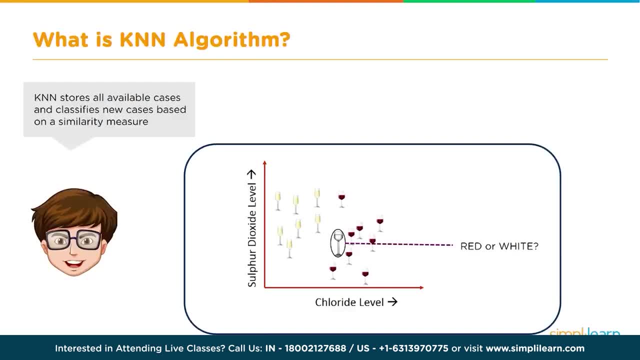 KNN stores all available cases and classifies new cases based on a similarity measure. And here you see, we have a measurement of sulfur dioxide versus the chloride level and then the different wines they've tested and where they fall on that graph for sulfur dioxide and how much chloride. 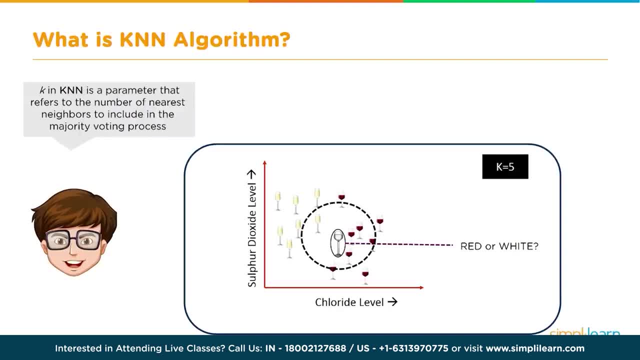 K, and KNN is a perimeter that refers to the number of nearest neighbors to include in the majority of the voting process, And so if we add a new glass of wine there- red or white- we want to know what the neighbors are. In this case, we're going to put K equals 5.. 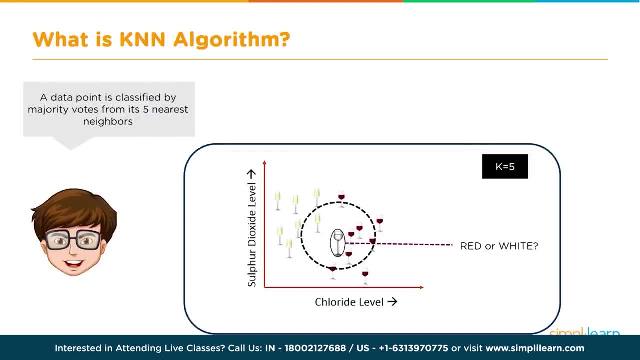 We'll talk about K in just a minute. A data point is classified by the majority of votes from its 5 nearest neighbors. Here, the unknown point would be classified as red, since 4 out of 5 neighbors are red. So how do we choose K? 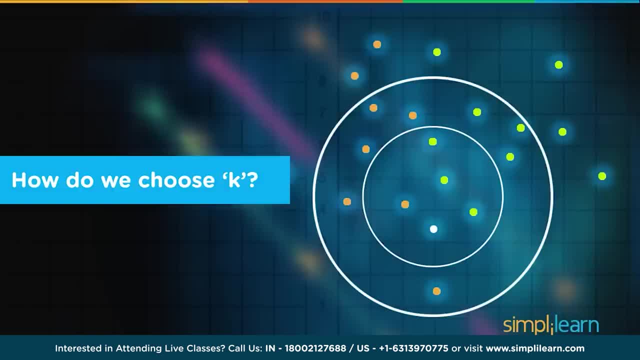 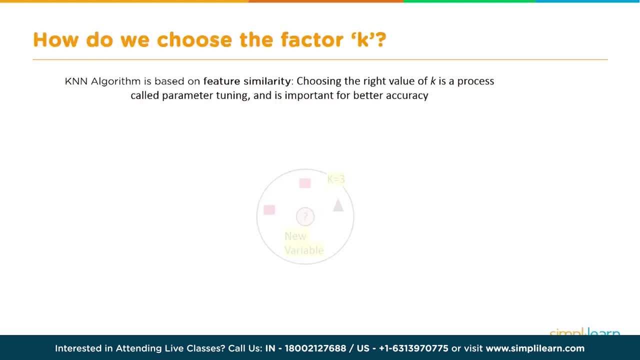 How do we know K equals 5? I mean, that was the value we put in there, and so we're going to talk about it. How do we choose the factor K? KNN algorithm is based on feature similarity. Choosing the right value of K. 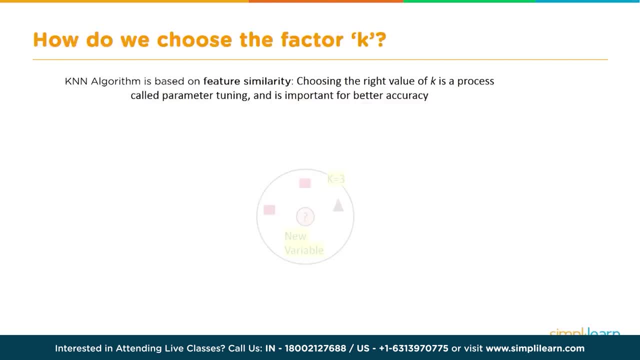 is a process called parameter tuning and is important for better accuracy. So at K equals 3, we can classify- we have a question mark in the middle- as either a square or not. Is it a square or is it, in this case, a triangle? And so if we set K equals to 3, 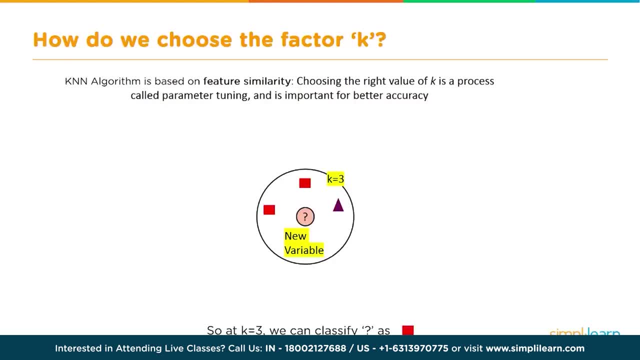 we're going to look at the 3 nearest neighbors. we're going to say this is a square And if we put a question mark in the middle and put K equals to 7, we classify as a triangle, depending on what the other data is around it. 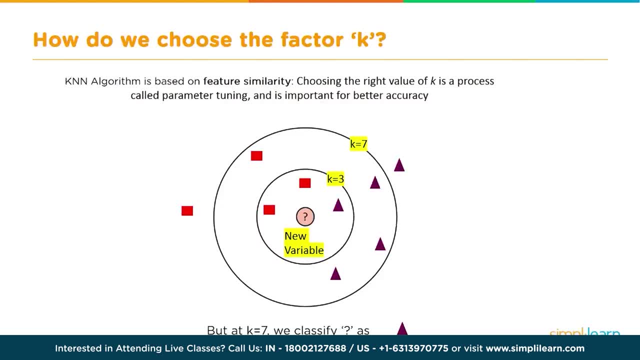 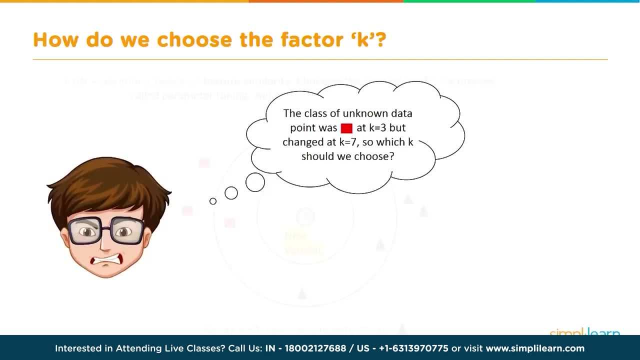 And you can see as the K changes, depending on where that point is. that drastically changes your answer And we jump here and we go. how do we choose the factor of K? You'll find this in all machine learning. choosing these factors, that's the face you get. 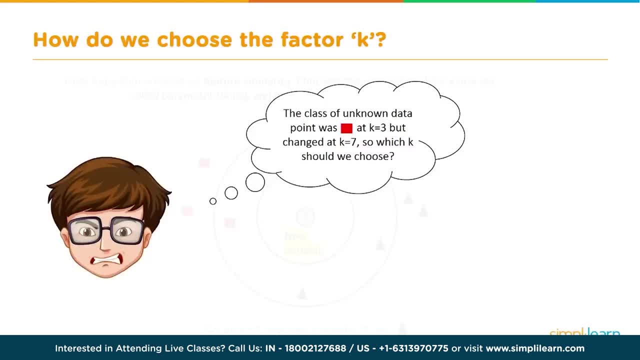 It's like, oh my gosh, did I choose the right K? Did I set it right- my values- in whatever machine learning tool you're looking at, so that you don't have a huge bias in terms of KNN, the number of K, if you choose it too low? 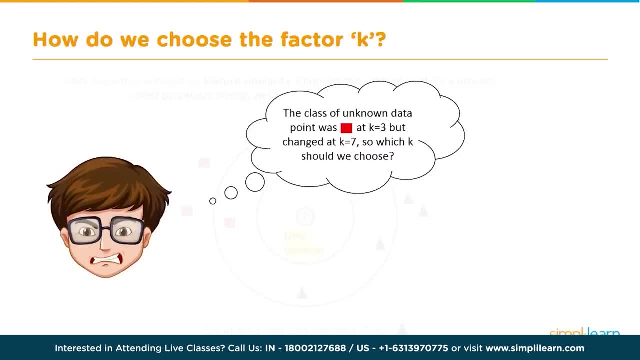 the bias is based on. it's just too noisy, it's right next to a couple things and it's going to pick those things and you might get a skewed answer And if your K is too big then it's going to take forever to process, so you're going to run into processing issues. 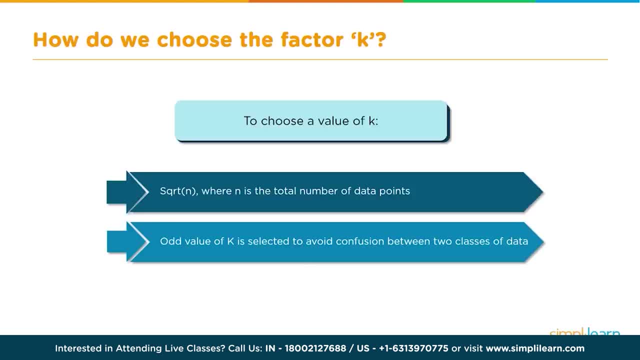 and resource issues. So what we do, the most common use- and there's other options for choosing K- is to use the square root of N. so N is the total number of values you have. in most cases you also if it's an even number. so if you're using squares and triangles, 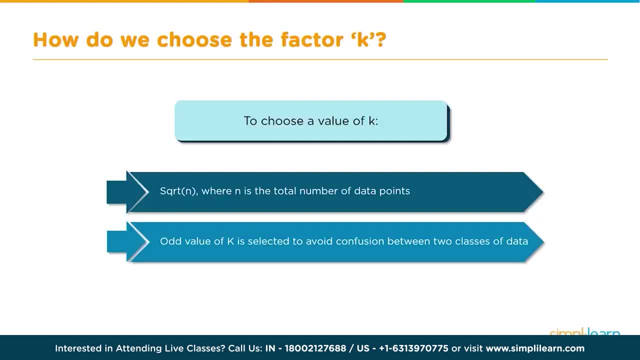 if it's even you want to make your K value odd. that helps it select better. so in other words, you're not going to have a balance between two different factors that are equal. so usually take the square root of N and if it's even you, add one to it. 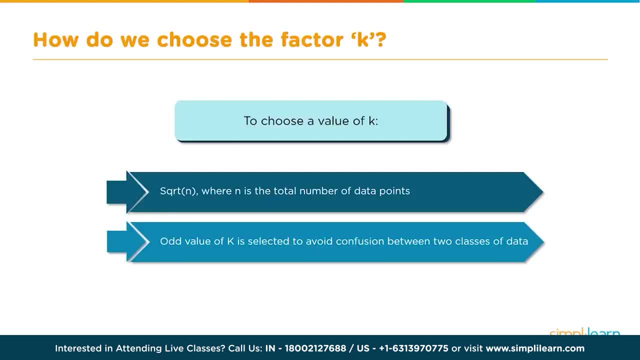 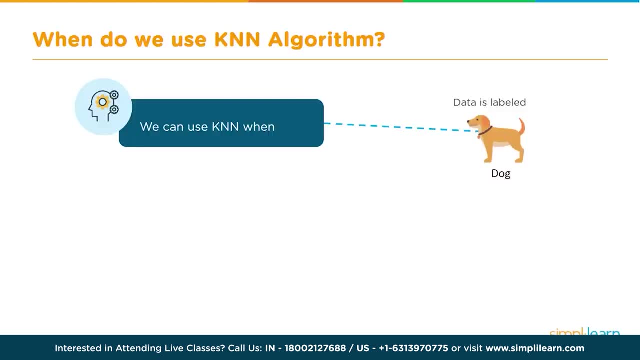 or subtract one from it, and that's where you get the K value from. that is the most common use and it's pretty solid. it works very well. When do we use KNN? So you need a label on it. we know we have a group of pictures. 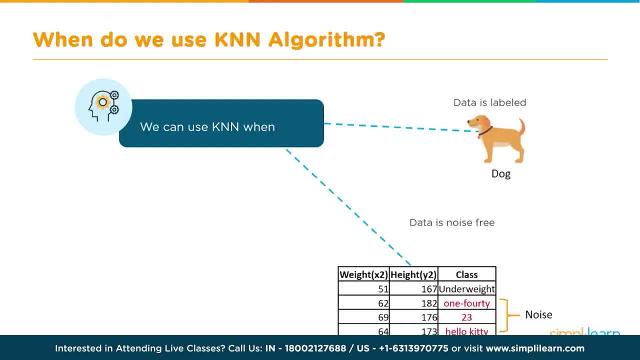 with dogs, dogs, cats, cats. data is noise free and so you can see here when we have a class and we have, like, underweight 140,, 23,, hello kitty, normal. that's pretty confusing. we have a high variety of data coming in. 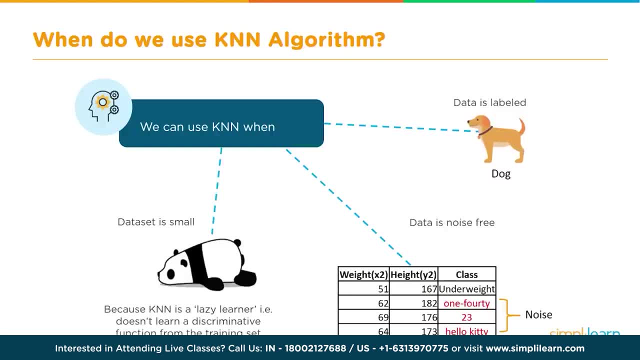 so it's very noisy and that would cause an issue. data set is small, so we're usually working with smaller data sets where you might get into a gig of data. if it's really clean, doesn't have a lot of noise. it's a lazy learner. 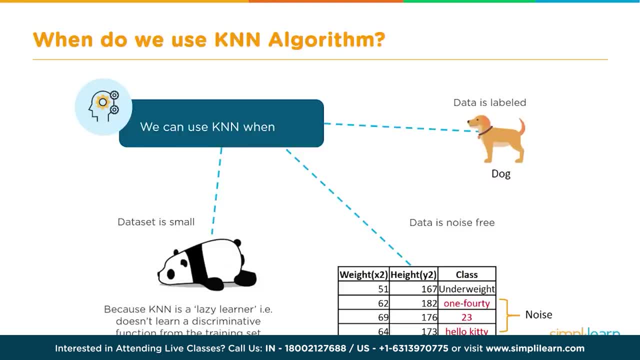 ie. it doesn't learn a discriminative function from the training set, so it's very lazy. so if you have very complicated data and you have a large amount of it, you're not going to use the KNN, but it's really great to get a place to start. 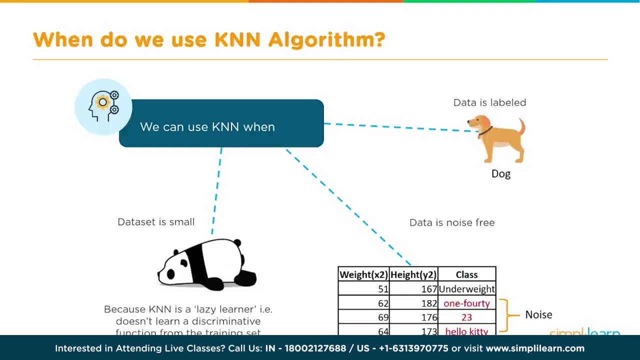 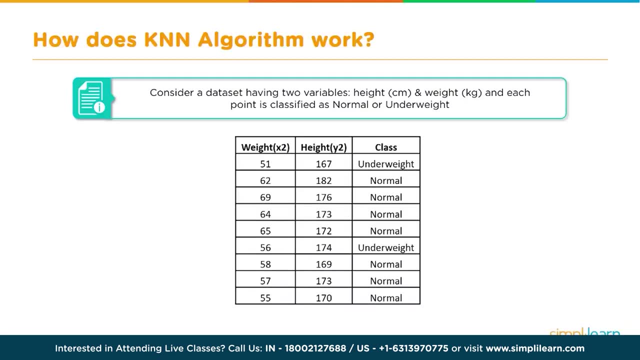 even with large data. you can sort out a small sample and get an idea of what that looks like. using the KNN and also just using for smaller data sets, KNN works really good. How does the KNN algorithm work? The KNN algorithm works by: 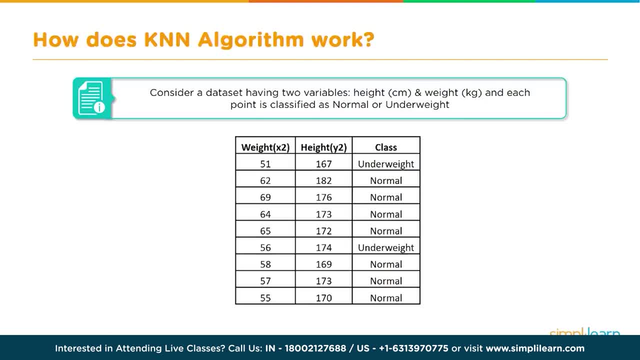 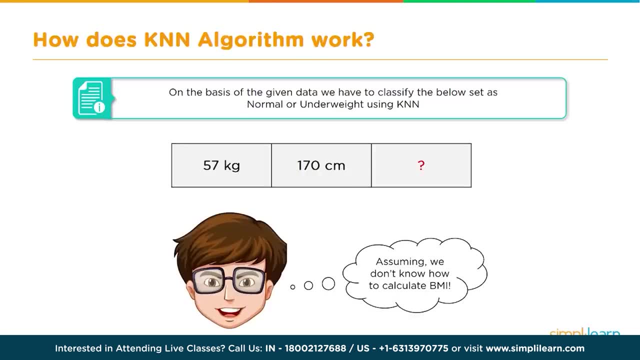 using a set of variables and each point is classified as normal or underweight. so we can see right here we have two variables: true, false. they're either normal or they're not. they're underweight. on the basis of the given data, we have to classify the below set. 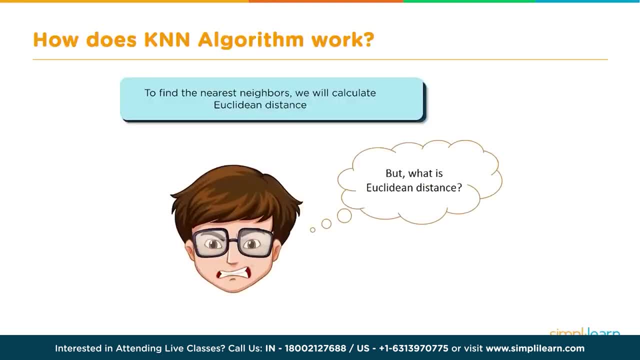 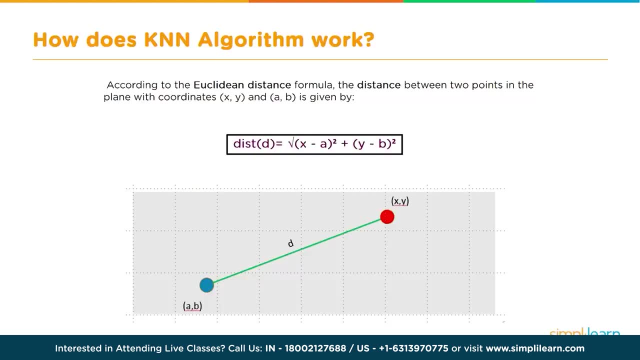 as normal or underweight using KNN. so if we have new data coming in that says 57 kilograms, we have to calculate the distance between two points in the plane with. the coordinates is given by distance. D equals the square root of plus and you can remember that. 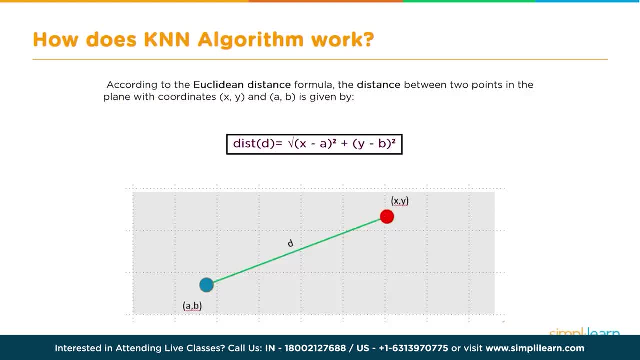 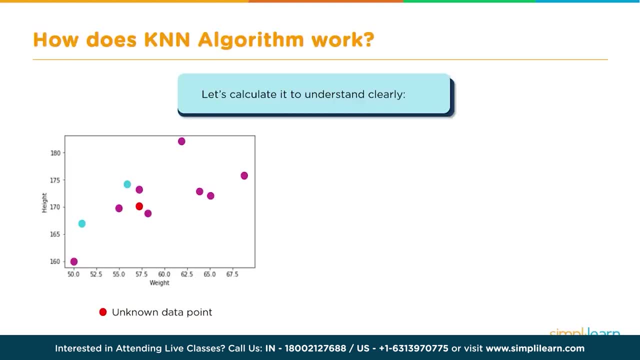 from the two edges of a triangle. we're computing the third edge. since we know the x side and the y side, let's calculate it to understand clearly. so we have our unknown point, we placed it there in red, and we have our other points where the data is scattered around. 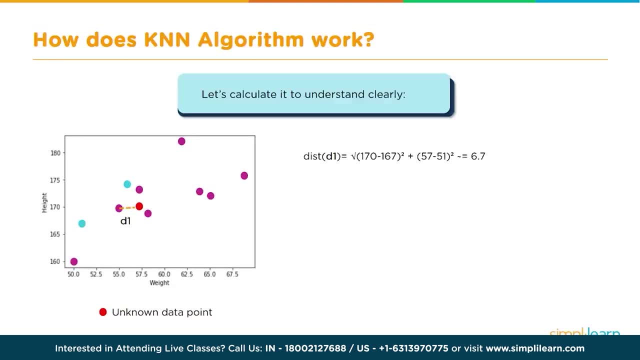 D1 is the square root of 170 minus 167 squared, plus 57 minus 51 squared, which is about 6.7, and distance 2 is about 13 and distance 3 is about 13.4. similarly, we will calculate the Euclidean distance of: 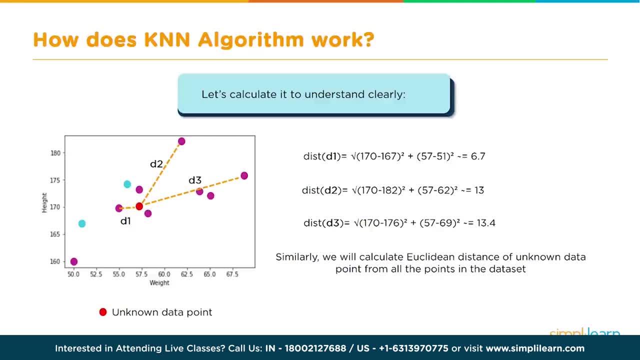 unknown data point from all the points in the data set and because we're dealing with small amount of data, that's not that hard to do. it's actually pretty quick for a computer and it's not really complicated math on the Euclidean distance. hence we have calculated the Euclidean distance. 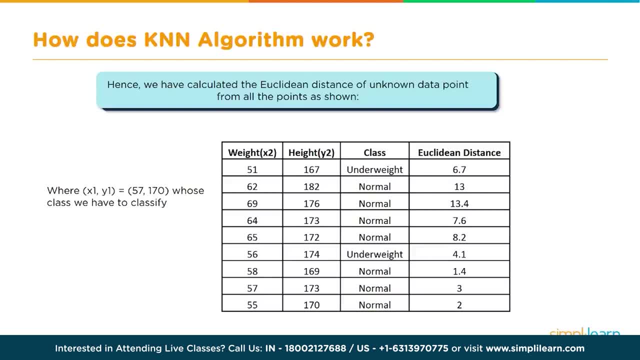 of unknown data point, from all the points as shown, where x1 and y1 equal 57 and 170, whose class we have to classify. so now we're looking at that, we're saying, well, here's the Euclidean distance. who's going to be their closest neighbors? 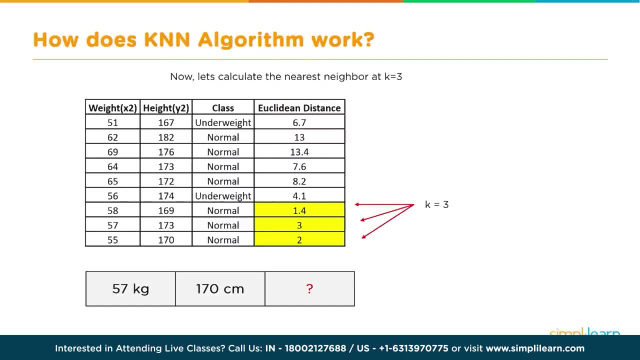 now let's calculate the nearest neighbor at k equals 3 and we can see the three closest neighbors. puts them at normal and that's pretty self evident. when you look at this graph it's pretty easy to say: normal, normal, normal, three votes for normal. this is going to be a normal weight. 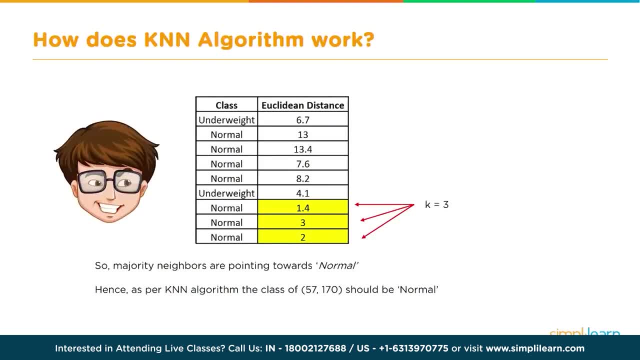 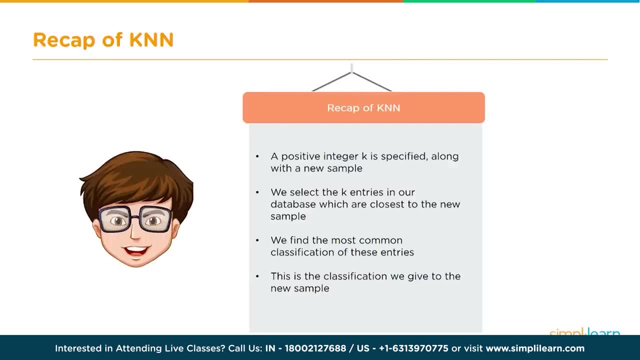 so majority of neighbors are pointing towards normal. hence, as per KNN algorithm, the class of 57 and 170 should be normal. so a recap of KNN positive integer k is specified along with a new sample. we select the k entries in our database which are closest to the new sample. 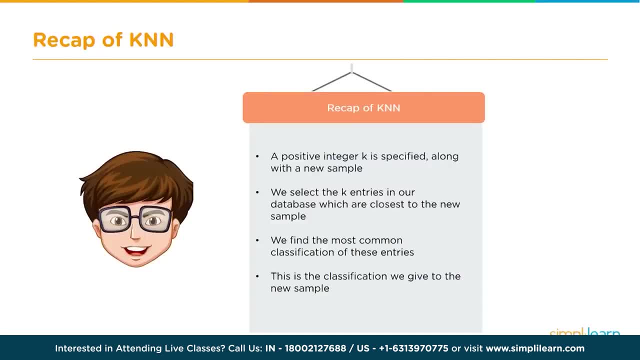 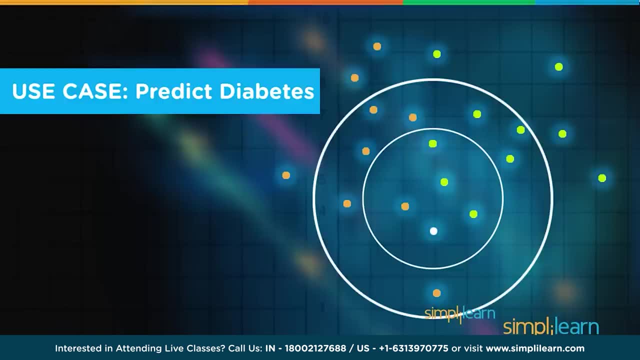 we find the most common classification of these entries. this is the classification we give to the new sample. so, as you can see, it's pretty straight forward. we're just looking for the closest thing that match what we got. so let's take a look and see what that looks like. 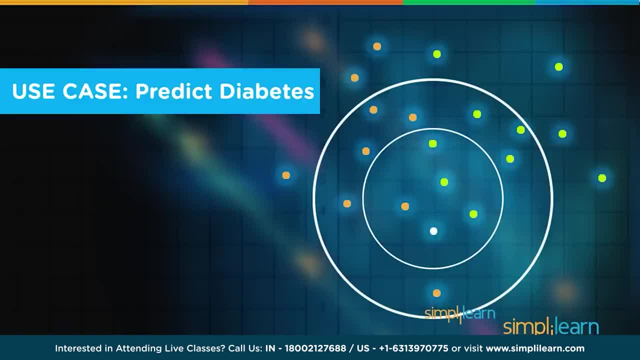 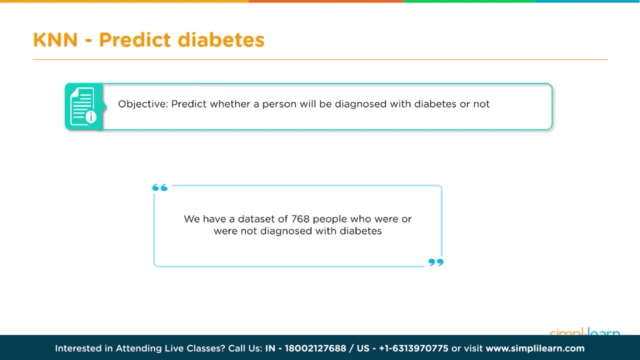 in a use case in python. so let's dive into the predict diabetes use case. so use case: predict diabetes. the objective: predict whether a person will be diagnosed with diabetes or not. we have a data set of 768 people who were or were not diagnosed with diabetes. 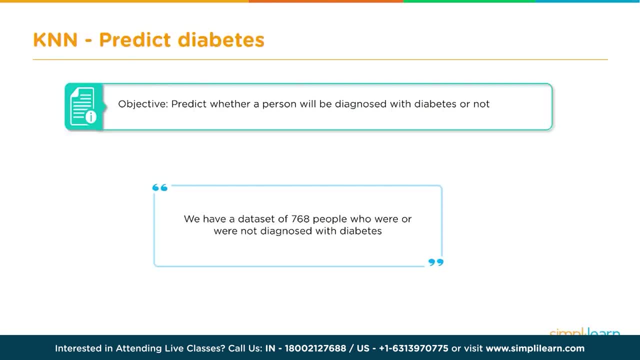 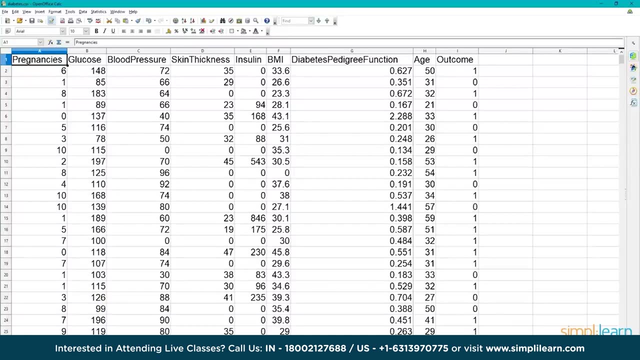 and let's go ahead and open that file and just take a look at that data. and this is in a simple spreadsheet format. the data itself is comma separated- very common set of data and it's also a very common way to get the data and you can see here we have columns A through I. 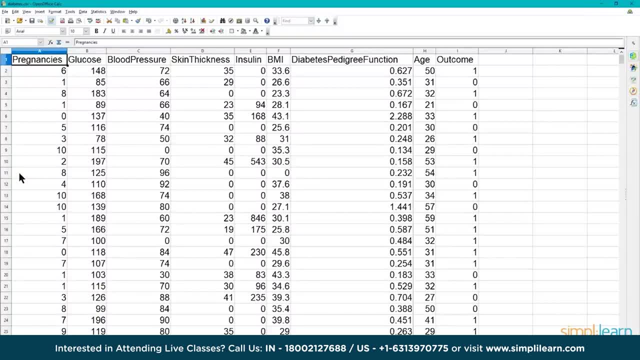 that's what. 1,, 2,, 3,, 4,, 5,, 6,, 7,, 8, 8 columns with a particular attribute, and then the 9th column, which is the outcome, is whether they have diabetes. as a data scientist, the first thing you should be looking at 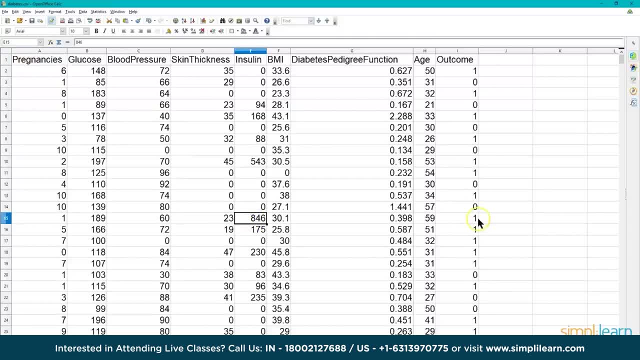 is insulin. well, you know, if someone has insulin, they have diabetes because that's why they're taking it and that could cause issue in some of the machine learning packages. the basic setup. this works fine for doing the KNN and the next thing you notice is it didn't take very much. 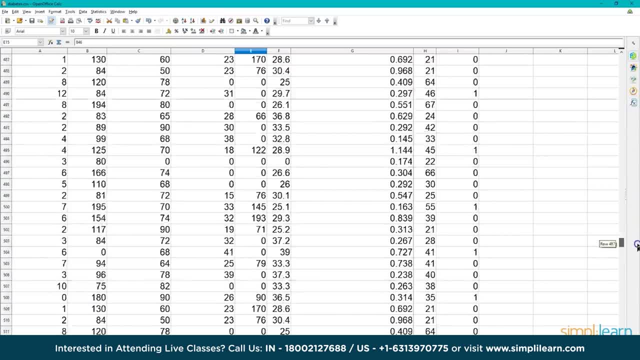 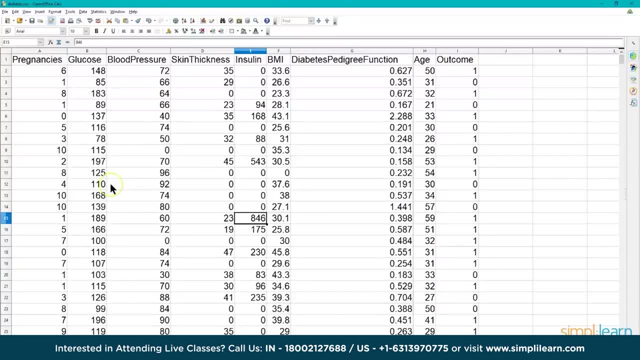 to open it up, I can scroll down to the bottom of the data. there's 768. it's pretty much a small data set, you know, at 769. I can easily fit this into my RAM on my computer. I can look at it, I can manipulate it. 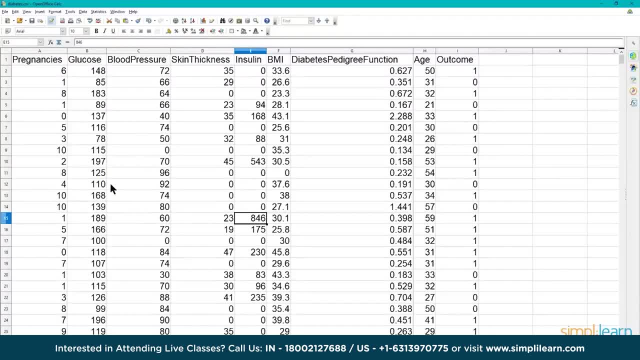 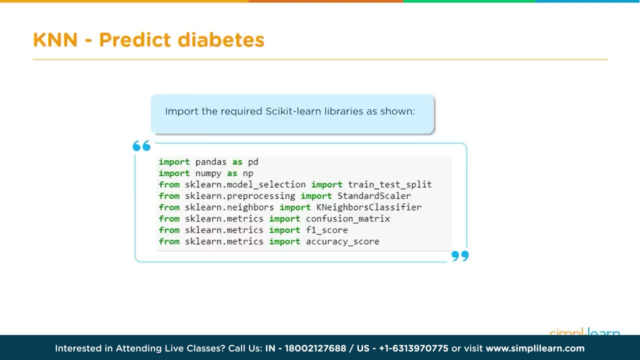 and it's not going to really tax, just a regular desktop computer. you don't even need an enterprise version to run a lot of this. so let's start with importing all the tools we need, and before that, of course, I need to discuss what IDE I'm using. certainly you can use any. 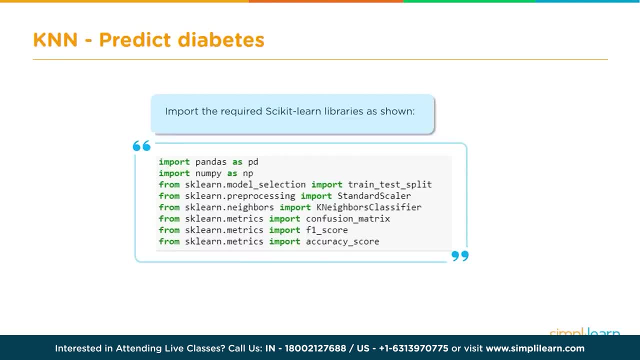 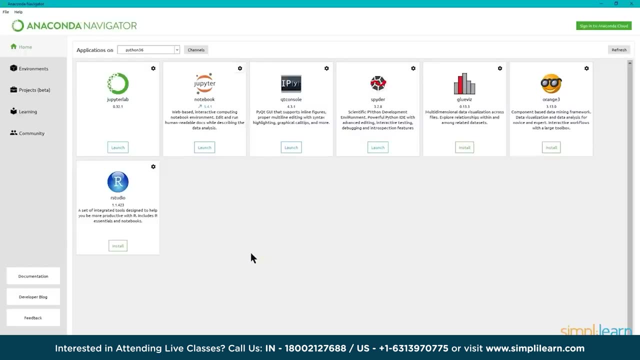 particular editor for Python but I like to use for doing very basic visual stuff, the Anaconda, which is great for doing demos with the Jupyter notebook, and just a quick view of the Anaconda Navigator, which is the new release out there, which is really nice you can see under home. I can choose. 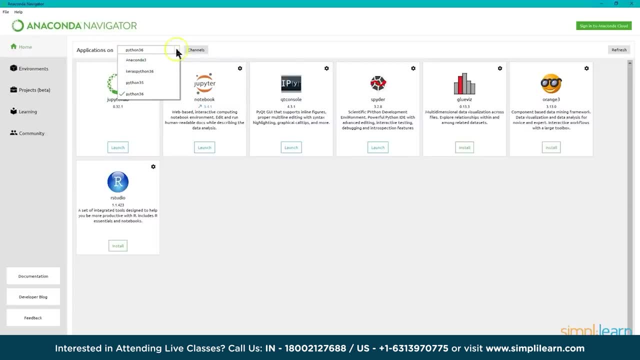 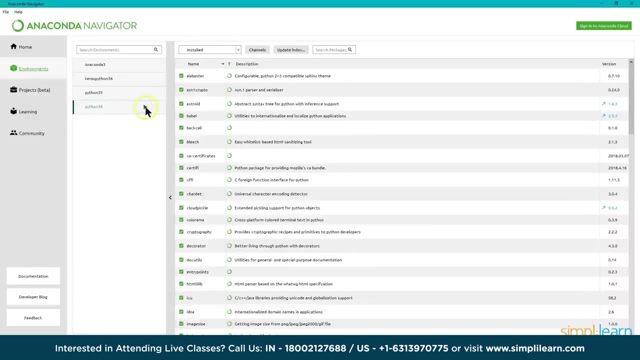 my application. we're going to be using Python 3.6. I have a couple different versions on this particular machine. if I go under environments, I can create a unique environment for each one, which is nice, and there's even a little button there where I can install different. 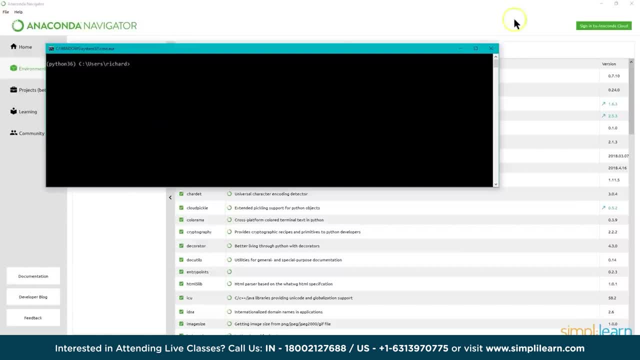 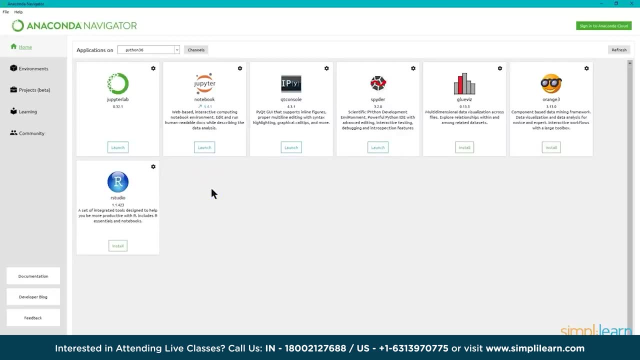 packages. so if I click on that button and open the terminal, I can then use a simple pip install to install different packages I'm working with. let's go ahead and go back under home and we're going to launch our notebook, and I've already, you know. 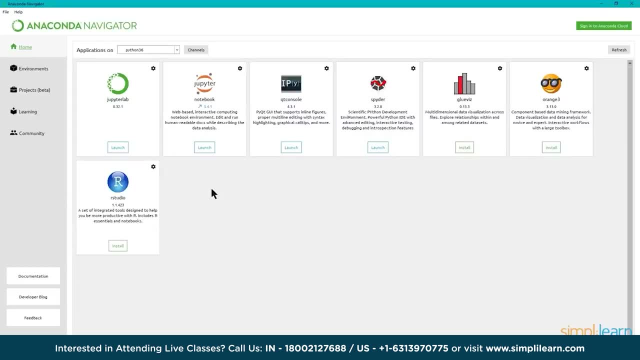 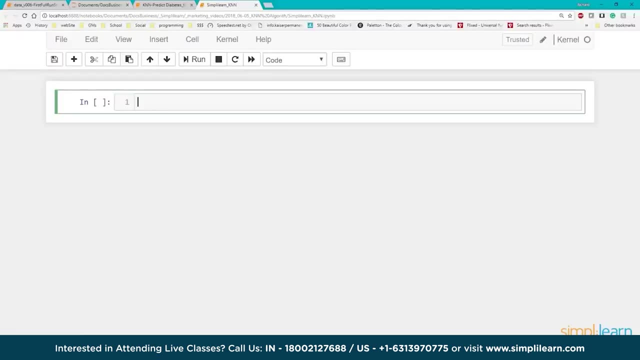 kind of like the old cooking shows. I've already prepared a lot of my stuff, so we don't have to wait for it to launch, because it takes a few minutes for it to open up a browser window. in this case, I'm going to. it's going to open up Chrome. 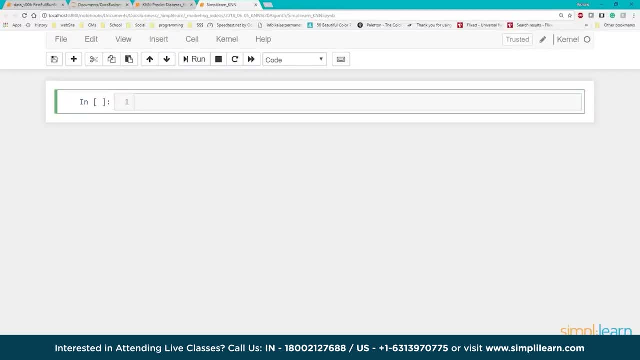 so you have a number of windows open up at the top, the one we're working in, and since we're working on the knn predict whether a person will have diabetes or not, let's go and put that title in there, and I'm also going to go. 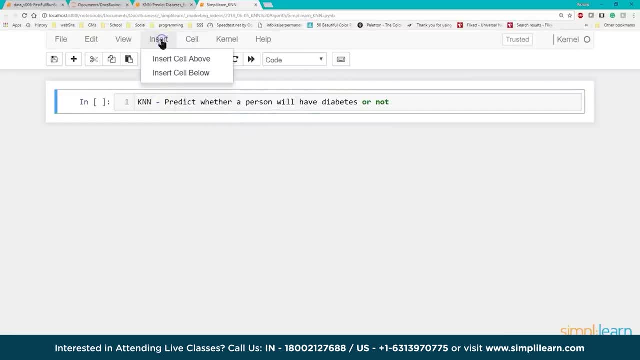 up here and click on cell. actually, we want to go ahead and first insert a cell below and then I'm going to go back up to the top cell and I'm going to change the cell type to markdown. that means this is not going to run as Python it's. 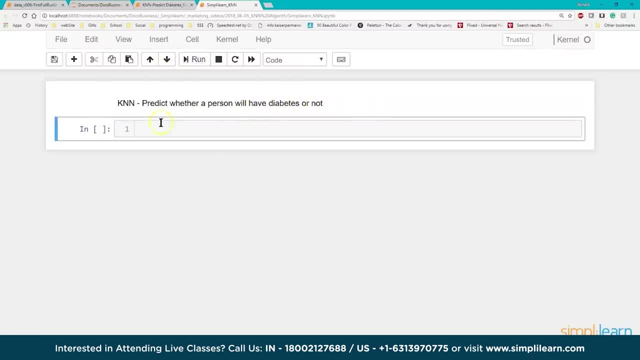 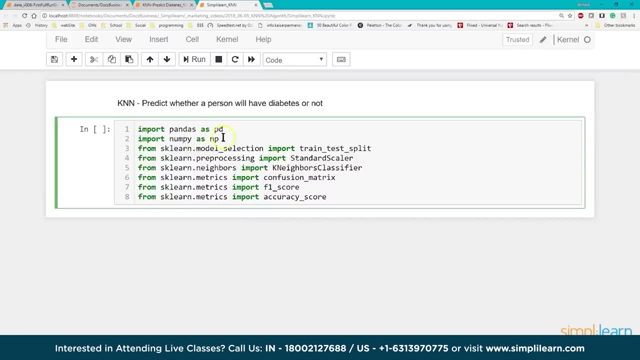 a markdown language. so if I run this first one it comes up in nice big letters, which is kind of nice. remind us of Python and by now you should be familiar with doing all of our imports. we're going to import the pandas as PD import numpy is. 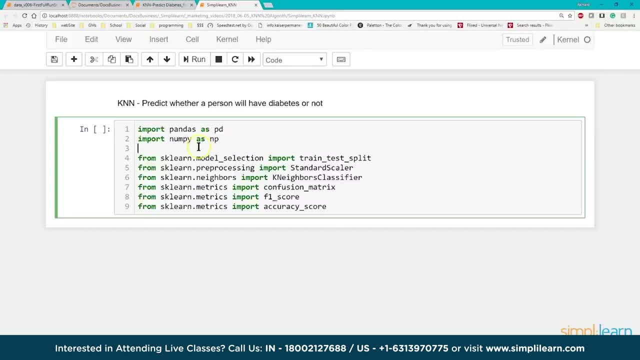 NP. pandas is the pandas data frame and numpy is a number array, very powerful tools to use in here. so we have our imports. so we've brought in our pandas, our numpy, our two general Python tools, and then you can see over here we have our train test. 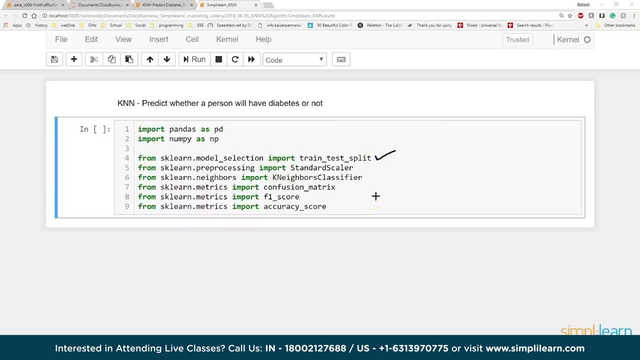 split. by now you should be familiar with splitting the data. we want to split part of it for training our thing, and then we want to go ahead and test the remaining data to see how good it is pre-processing a standard scalar pre-processor, so we don't have a bias. 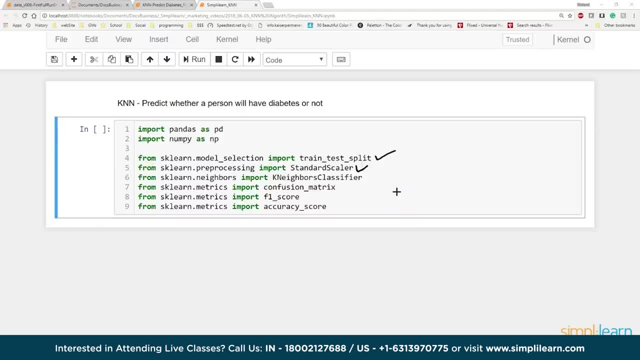 of really large numbers. remember in the data we had like number pregnancies isn't going to get very large where the amount of insulin they take and get up to 256. so 256 versus 6, that will skew results. so we want to go ahead and change that so that they're all uniform. 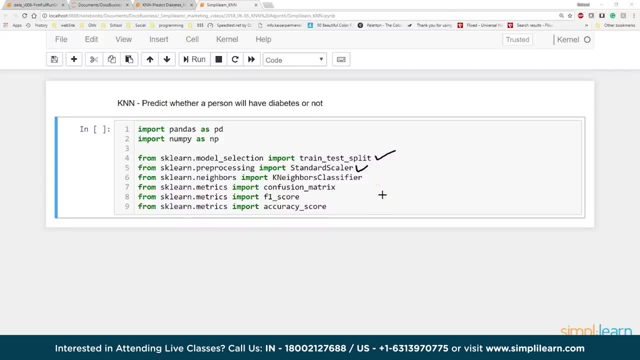 between minus one and one. and then the actual tool. this is the K neighbors classifier resource, so we're going to go ahead and change that so that they're going to use. and finally, the last three are three tools to test. all about testing our model. how good is it? we just 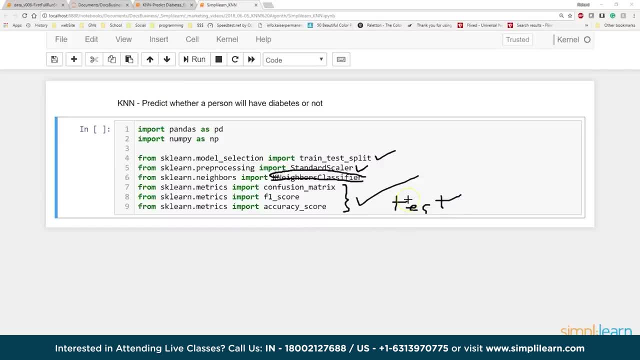 put down test on there and we have our confusion matrix, our f1 score and our accuracy. so we have our two general Python modules we're importing and then we have our six modules specific from the sklearn setup and then we do need to go ahead and run this. so these are. 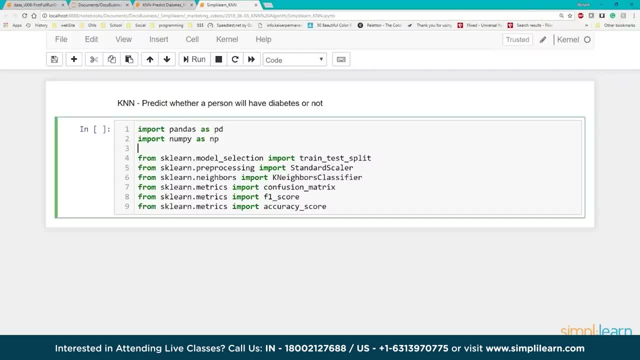 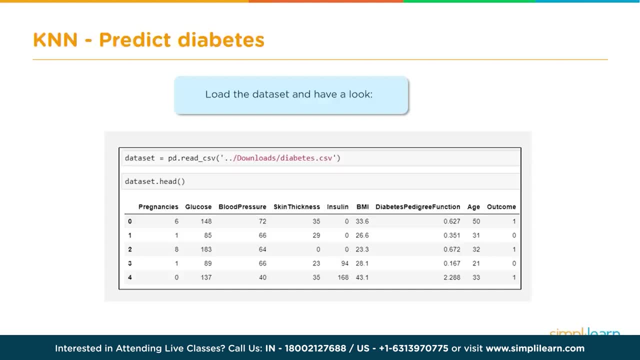 actually imported. there we go and then move on to the next step, and so in this set, we're going to go ahead and import this, and then we're going to import this, and then we're going to go ahead and load the database. we're going to use pandas- remember, pandas is PD and 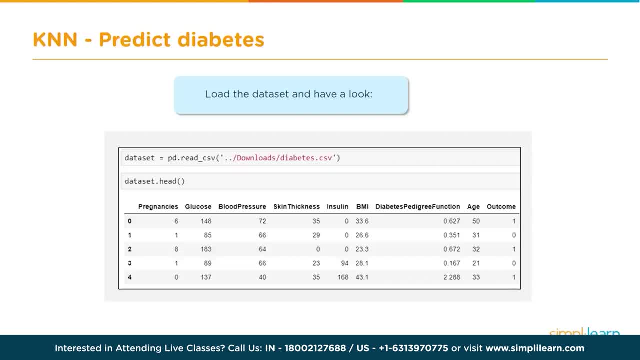 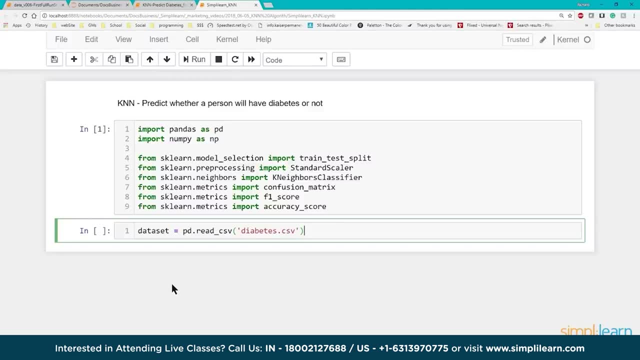 we'll take a look at the data in Python. we looked at it in a simple spreadsheet, but usually I like to also pull it up so that we can see what we're doing. so here's our data set: equals PD, dot. read CSV. that's a pandas command and the 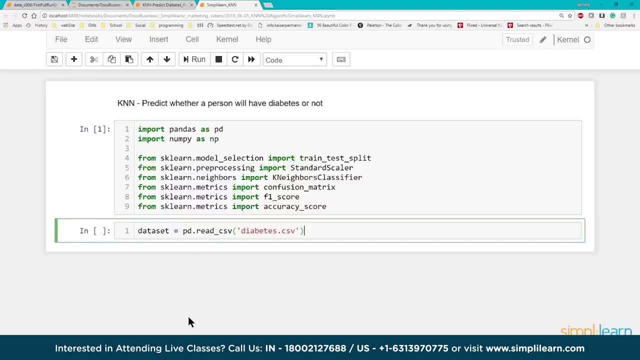 diabetes folder. I just put in the same folder where my ipython script is. if you put in a different folder you'd need the full length on there. we can also do a quick length of the data set and then the data set. that is a simple Python. 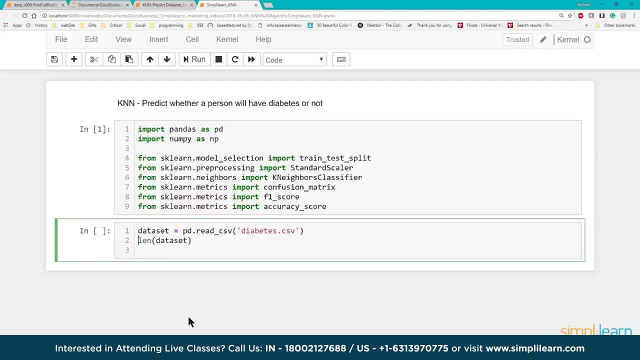 command LEN for length. we might even let's go ahead and print that. we'll go print and if you do it on its own line, link that data set in the Jupyter notebook. it'll automatically print it. but when you're in most of your different setups you want to do the 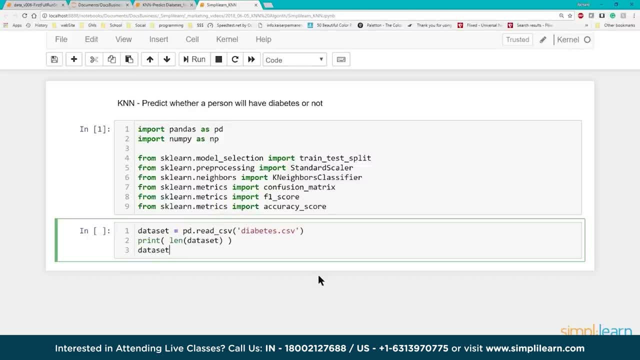 print in front of there and then we want to take a look at the actual data set and since we're in pandas, we can simply do data set head and again. let's go ahead and add the print in there. if you put a bunch of these in a row, you know. 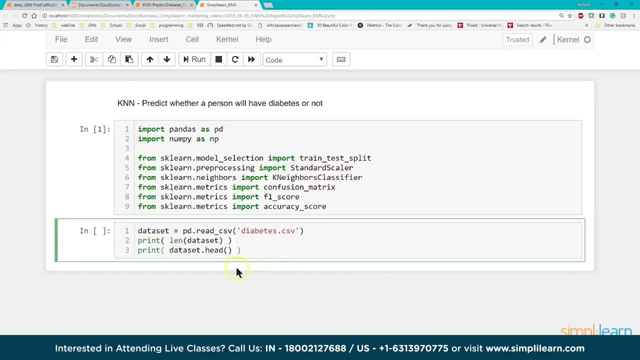 the data set one head, data set two head. it only prints out the last one. so I usually always like to keep the print statement in there. but because most projects only use one data frame- pandas data frame- doing it this way doesn't really matter, the other way works just. 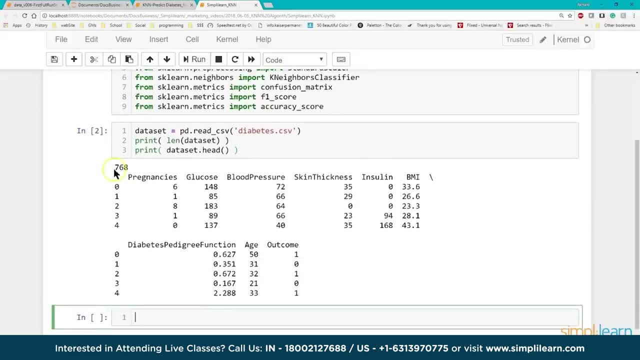 fine and you can see. when we hit the run button we have the 768 lines which we knew, and we have our pregnancies. it's automatically given a label on the left. remember, the head only shows the first five lines, so we have zero through four. and just a quick look at the data. you 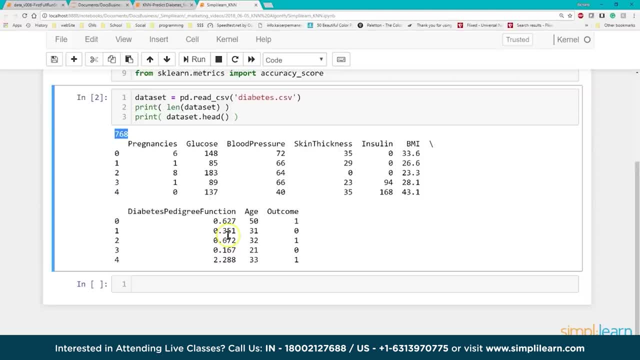 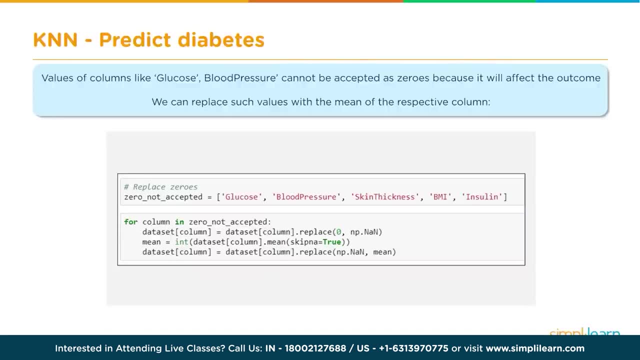 can see. it matches what we looked at in that before we have pregnancy, glucose blood pressure, all the way to age, and then the outcome on the end. and we're going to do a couple things in this next step. we're going to create a list of columns where we can't have zero. there's. 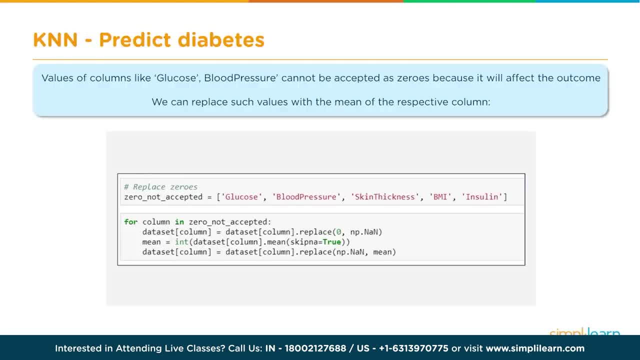 no such thing as zero skin thickness or zero blood pressure, zero glucose- any of those, you'd be dead. so not a really good factor if they don't, if they have a zero in there, because they didn't have the data and we'll take a look at that. 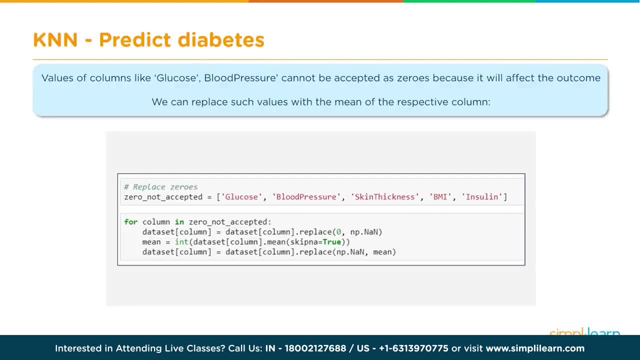 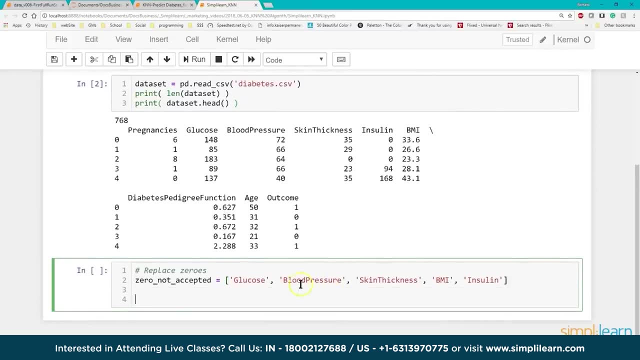 because we're going to start replacing that information with a couple of different things. let's see what that looks like. so first we create a nice list. as you can see, we have the values talked about: glucose, blood pressure, skin thickness, and this is a nice way when 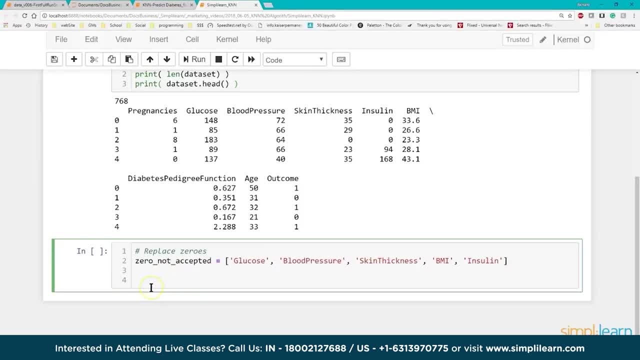 you're working with columns is to list the columns. you need to do some kind of transformation on a very common thing to do and then, for this particular setup, we certainly could use the. there's some panda tools that will do a lot of this, where we can replace the na, but we're 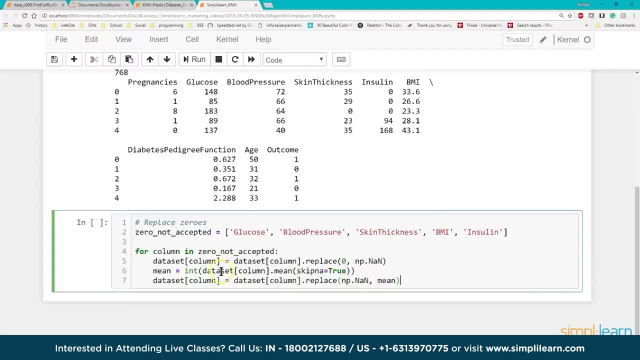 going to go ahead and do it as a data set column equals data set column, dot. replace this is: this is still pandas. you can do a direct. there's also one that you look for your na? n. a lot of different options in here, but the na? n. 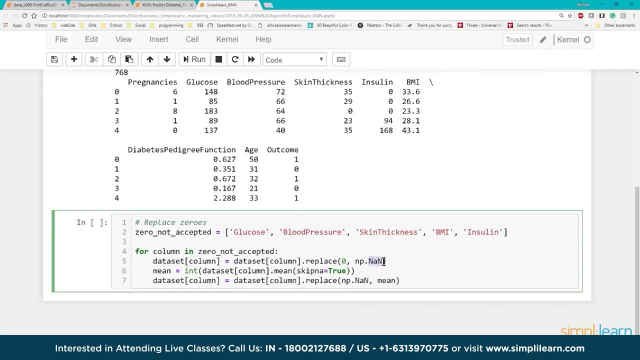 numpy na n is what that stands for. is is none. it doesn't exist. so the first thing we're doing here is we're replacing the zero with a numpy none. there's no data there. that's what that says. that's what this is saying right here. so put the zero in and we're going. 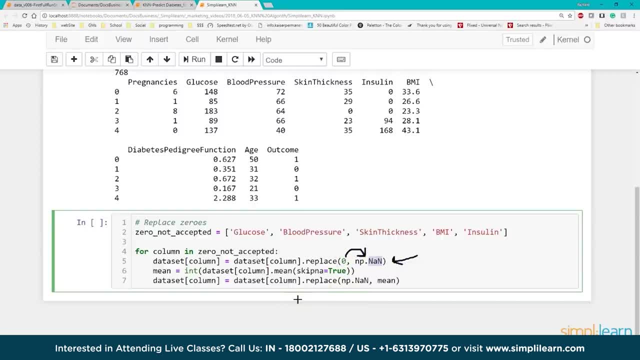 to play zeros with no data. so if it's a zero, that means a person's well, hopefully not dead. oh, they just didn't get the data. the next thing we want to do is we're going to create the mean, which is the integer from the data set, from the 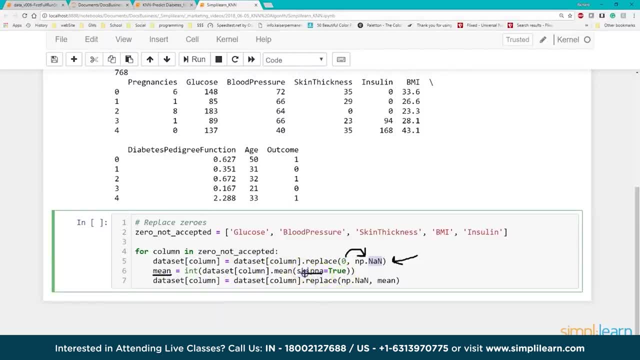 column dot mean where we skip na's. we can do that. that is a pandas command there the skip na. so we're going to figure out the mean of that data set and then we're going to take that data set column and we're going to replace all 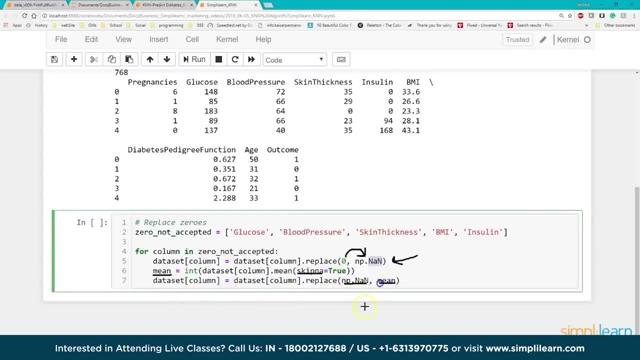 the NP na n with the means: why did we do that? and we could have actually just taken this step and gone right down here and just replace zero and skip anything were, except you can actually there's a way to skip zeros and then just replace all the zeros, but in this case we want. 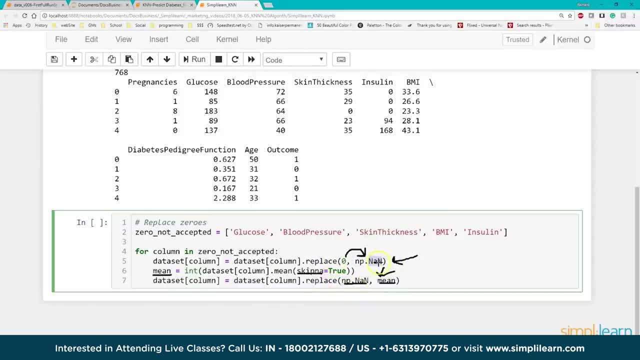 to go ahead and do it this way, so you can see that we're switching this to a non-existent value. then we're going to create the mean. well, this is the average person. so if we don't know what it is, if they did not get the data, the data is. 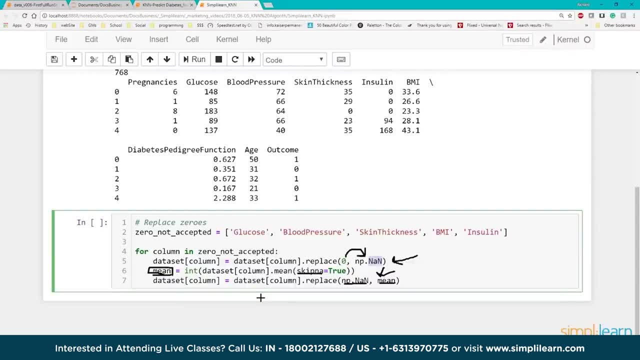 missing. one of the tricks is you replace it with the average, what is the most common data for that. this way you can still use the rest of those values to do your computation and it kind of just brings that particular value of those missing values out of the equation. let's 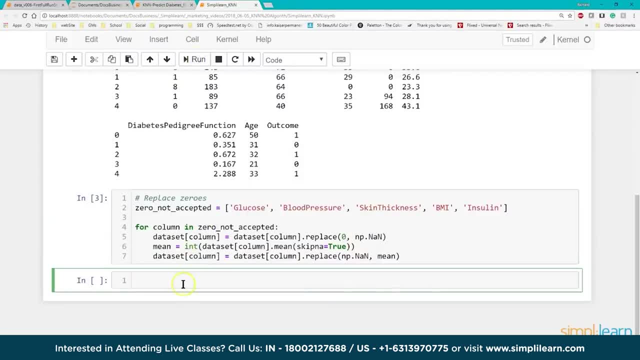 go ahead and take this and we'll go ahead and run. it doesn't actually do anything, so we're still preparing our data. if you want to see what that looks like, it we don't have anything in the first few lines, just not going to show up. 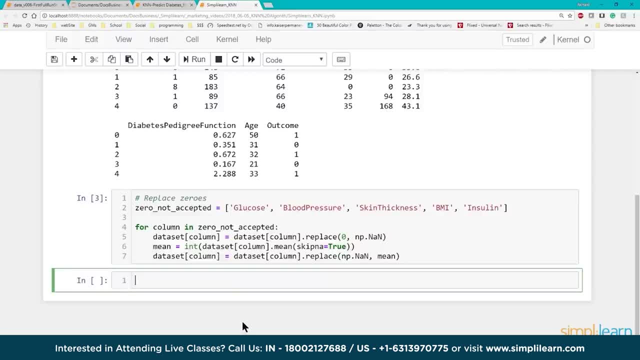 but we certainly could look at a row. let's do that. let's go into our data set was printed data set and let's pick. in this case, let's just do glucose and if I run this, this is going to print all the different glucose levels. I'm going to. 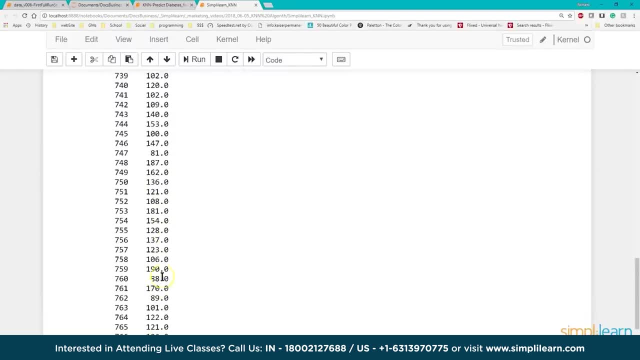 bring it down here and it's going down and we thankfully don't see anything in here that looks like missing data. at least on the ones that shows you can see it skipped a bunch in the middle. that's what it does if you have too many lines. 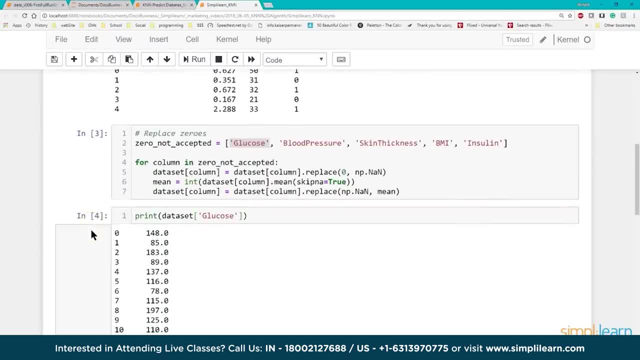 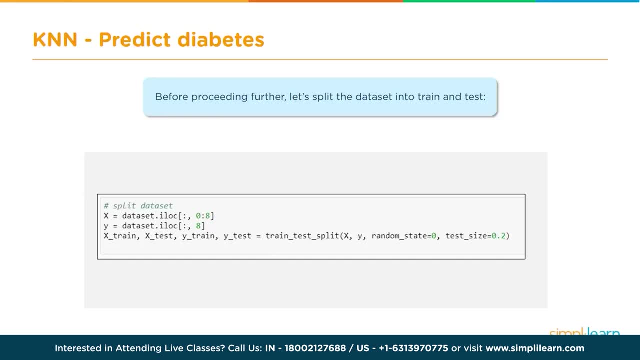 in jupiter notebook. it'll skip a few and go on to the next in a data set. let me go and remove this and we'll just zero out that. and, of course, before we do any processing, before proceeding any further, we need to split the data set into our 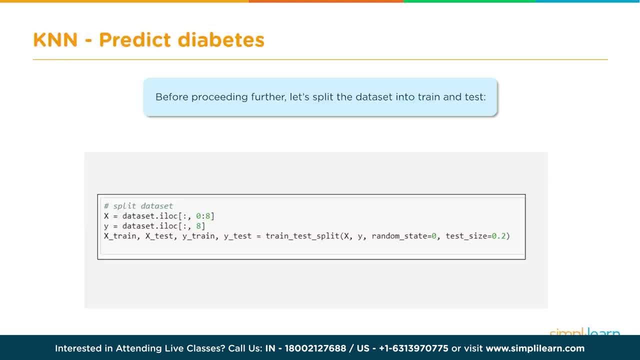 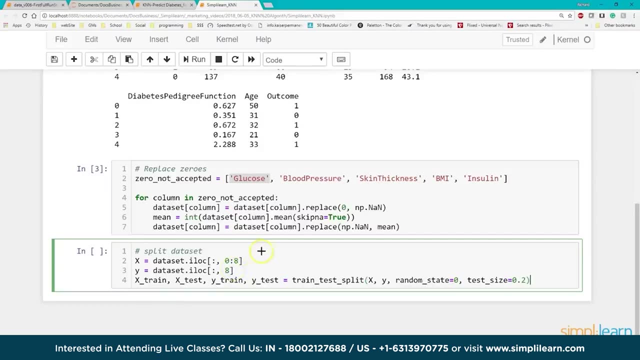 train and testing data. that way we have something to train it with and something to test it on. and you're going to notice, we did a little something here with the Pandas database code. There we go my drawing tool. We've added in this right here off the data set, And what this says is that the first one in Pandas- this is from the PD Pandas- it's going to say, within the data set, we want to look at the I location and it is all rows. That's what that says. So we're going to keep all the rows, But we're only looking at zero, column zero to eight. Remember column nine? here it is right up here, we printed it in here. is outcome? Well, that's not part of the training data, that's part of the answer. Yes, column nine. 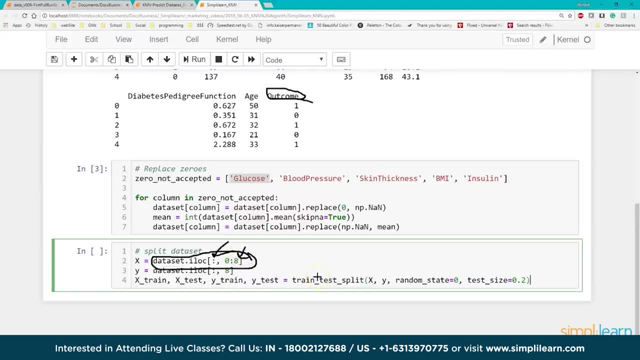 but it's listed as eight number eight. So zero to eight is nine columns. So eight is the value And when you see it in here, zero. this is actually zero to seven, it doesn't include the last one. And then we go down here to Y, which is our answer, And we want just the last one, just column eight. And you can do it this way with this particular notation. And then, if you remember, we imported the train test split. that's part of the SK learn right there. And we simply put in our X and our Y. we're going to do. 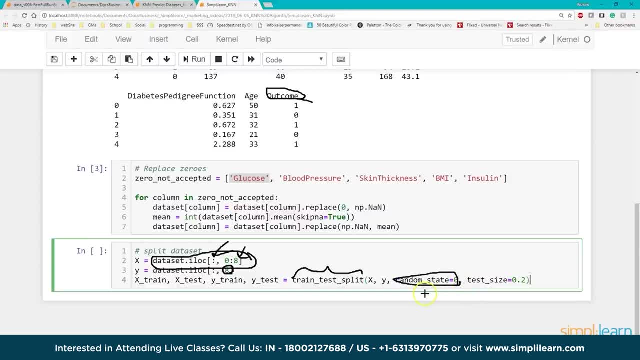 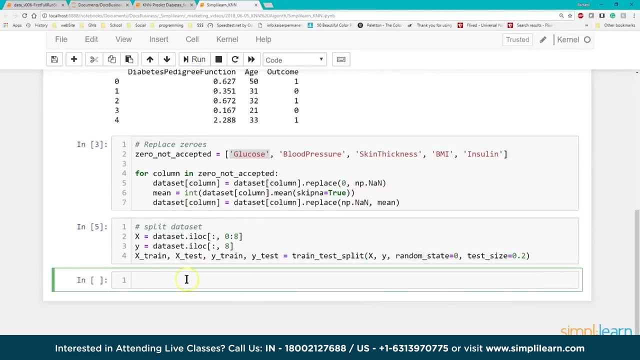 random state equals zero. you don't have to necessarily seed it. that's a seed number. I think the default is one when you seed it. I'd have to look that up. And then the test size. test size is point two. that simply means we're going to take 20% of the data and put it aside so that we can test it later. That's all that is, And again, we're going to run it. not very exciting. So far we haven't had any printout other than to look at the data. But that is a lot of. this is prepping this data. Once you prep it, the actual lines of code are quick and easy And we're almost there. But the actual running of our KNN. 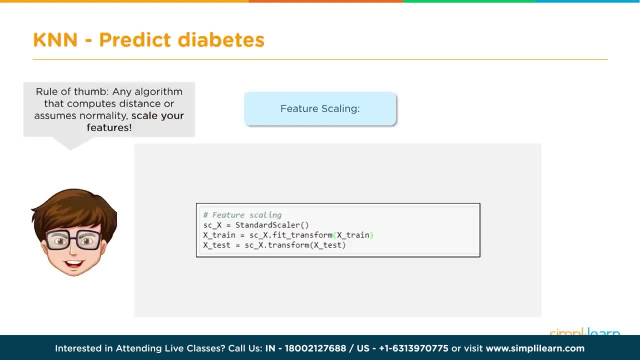 we need to go ahead and do a scale the data. If you remember correctly, we're fitting the data and a standard scaler, which means, instead of the data being, from, you know, five to 303 in one column and the next column is one to six. we're going to set that all so that all the data is between minus one and one. That's what that standard scaler does, keeps it standardized, And we only want to fit the scaler with the training set, But we want to make sure the testing set is the X test. going in is also. 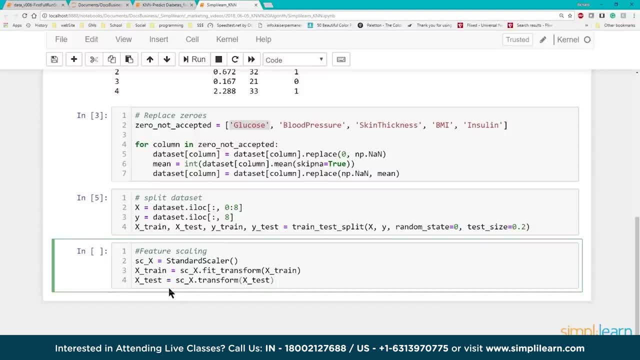 transformed. So it's processing it the same. So here we go with our standard scaler. we're going to call it SC underscore x for the scaler And we're going to import the standard scaler into this variable And then our X train equals SC underscore x, dot, fit, transform. So we're creating the scaler on the X train variable And then our X test we're also going to transform it. So we've trained and transformed the X train And then the X test isn't part of that training. it isn't part of that training. the transformer. 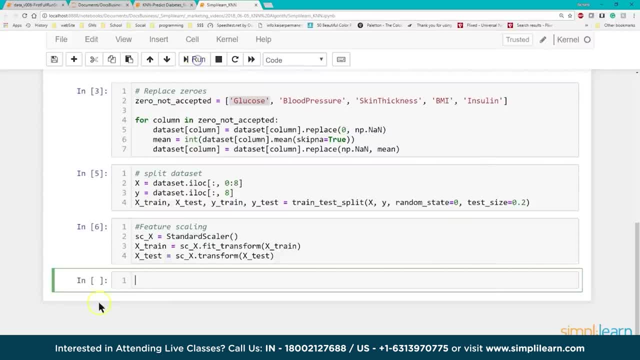 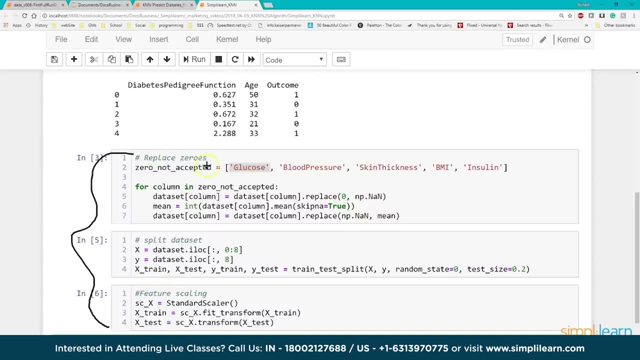 it just gets transformed. That's all it does. And again we're going to go and run this And if you look at this, we've now gone through these steps, all three of them. we've taken care of replacing our zeros for key columns that shouldn't be zero And we replace that with the means of those columns that way that they fit right in with our data models. We've come down here. we split the data, So now we have our test data and our training data, And then we've taken and we scaled the data. 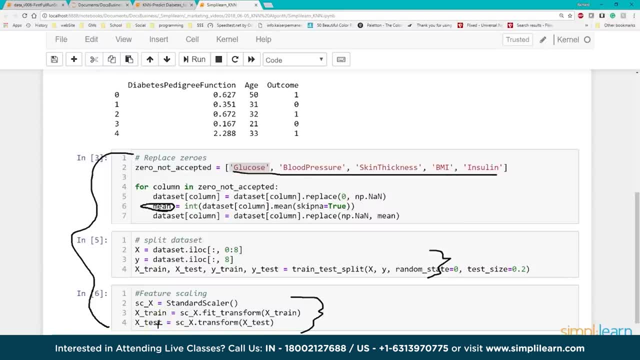 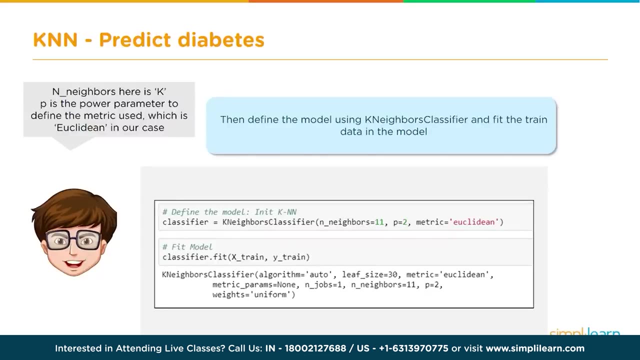 So all of our data going in? no, no, we don't. we don't train the Y part, the Y train and Y test. that never has to be trained, It's only the data going in. That's what we want to train in there, then define the model using k, neighbors classifier and fit the train data in the model. So we do all that data prep And you can see down here we're only going to have a couple lines of code where we're actually building our model and training it. That's one of the cool things about Python and how far we've come. It's such an exciting time to be in the world. 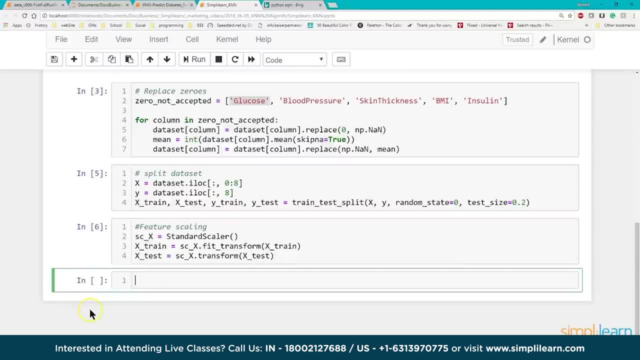 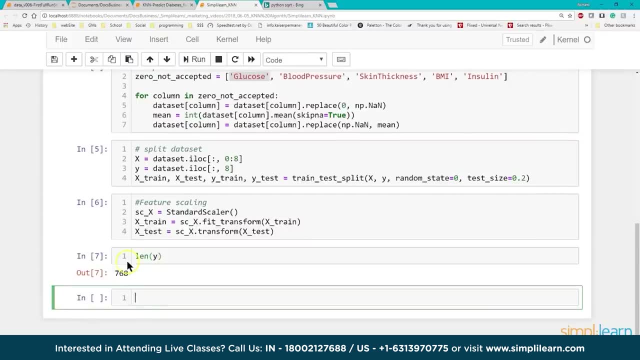 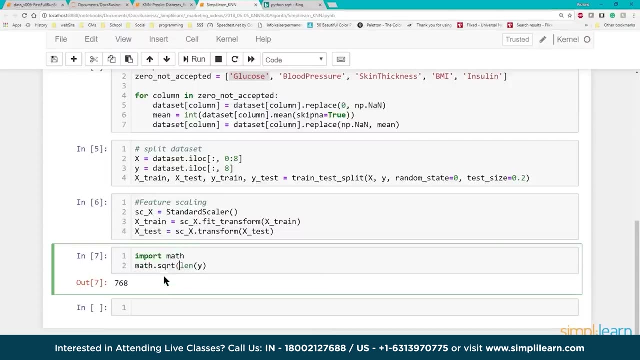 And machine learning, because there's so many automated tools. Let's see, before we do this, let's do a quick length of and let's do Y we want. let's just do length of Y And we get 768.. And if we import math, we do math dot square root. Let's do Y train, There we go. It's actually supposed to be X train. Before we do this, let's go ahead and do import math and do math square root, length of Y test. And when I 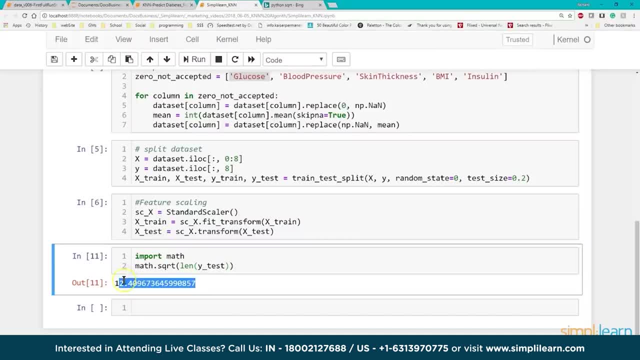 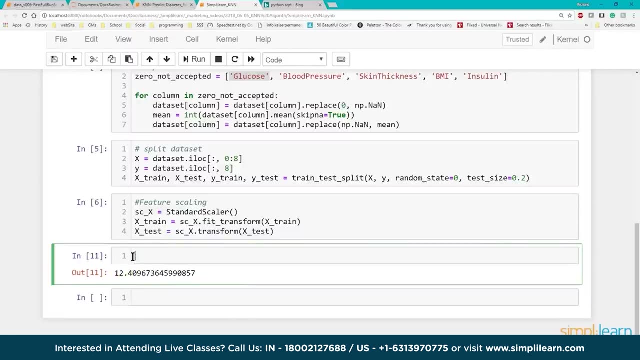 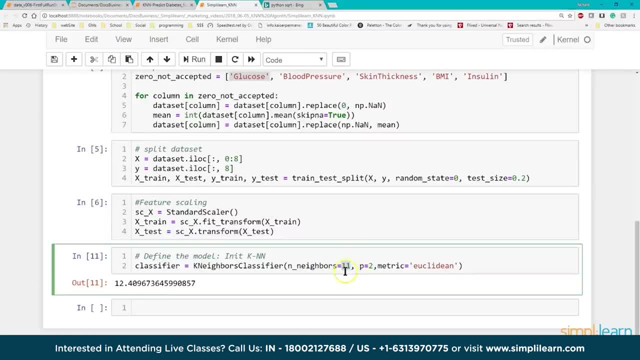 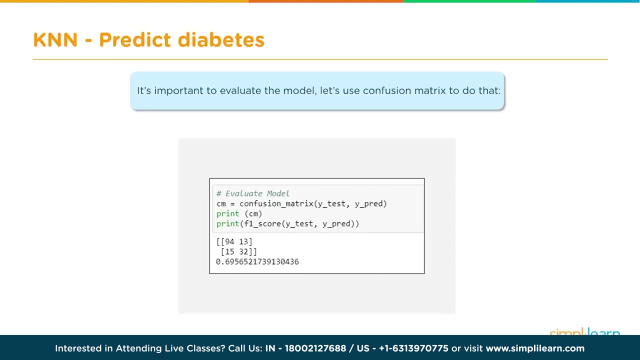 remember we did 12 minus one for 11.. So we have an odd number of neighbors. P equals two, because we're looking for is it? are they diabetic or not? And we're using the Euclidean metric. There are other means of measuring the distance. You could do like square. square means values, all kinds of measure this- But the Euclidean is the most common one and it works quite well. It's important to evaluate the model. Let's use the confusion matrix to do that, And we're going to use the confusion matrix, Wonderful tool, And then we'll jump into the 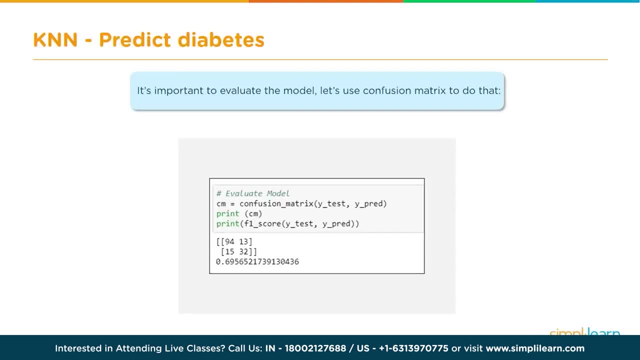 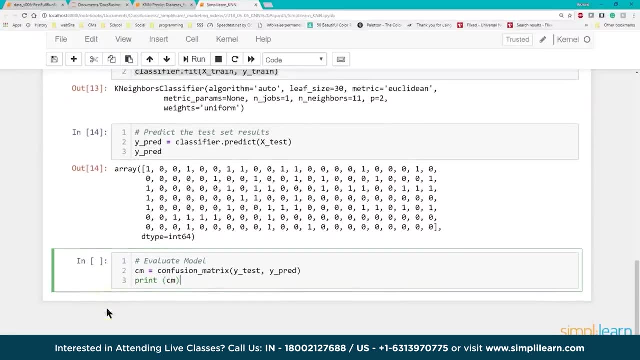 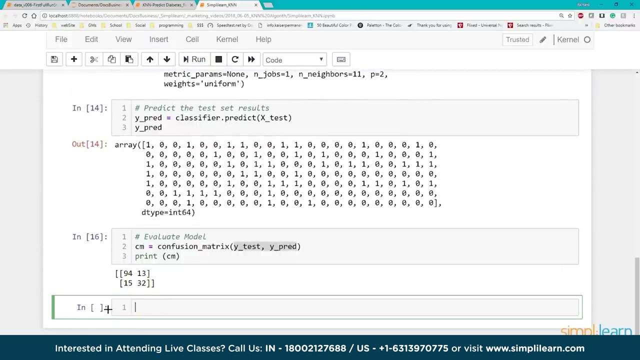 F1 score And finally, accuracy score, which is probably the most commonly used quoted number when you go into a meeting or something like that. So let's go ahead and paste that in there And we'll set the CM equal to confusion. matrix Y test, Y predict. So those are the two values we're going to put in there And let me go ahead and run that and print it out. And the way you interpret this is: you have the Y predicted, which would be your title up here. Let's just do P-R-E-D. 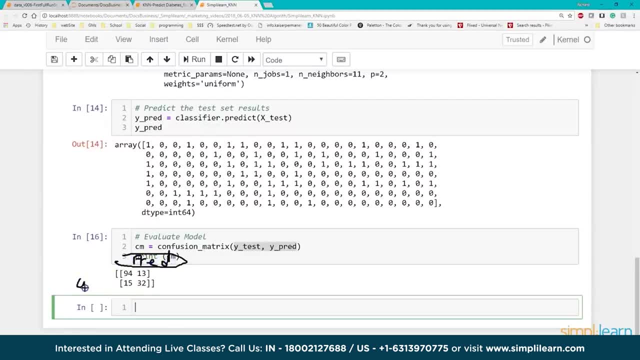 Predicted across the top and actual going down. Actual. It's always hard to write in here. actual That means that this column here down the middle that's the important column And it means that our prediction said 94 and prediction and the actual agreed on 94 and 32.. This number here, the 13 and the 15, those are what was wrong, So you could have like three different if you're looking at this across three different. 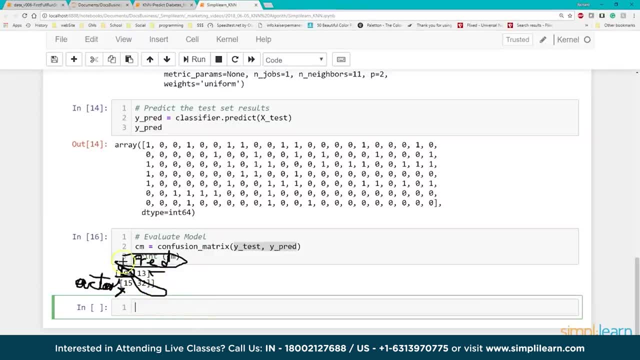 variables instead of just two. you'd end up with the third row down here and the column going down the middle. So in the first case we have the- and I believe the zero is a- 94, people who don't have diabetes. The prediction said that 13 of those people did have diabetes and were at high risk And the 32 that had diabetes it had correct, But our prediction said another 15 out of that 15 it classified as incorrect. So you can see where that classification comes in and how that works. 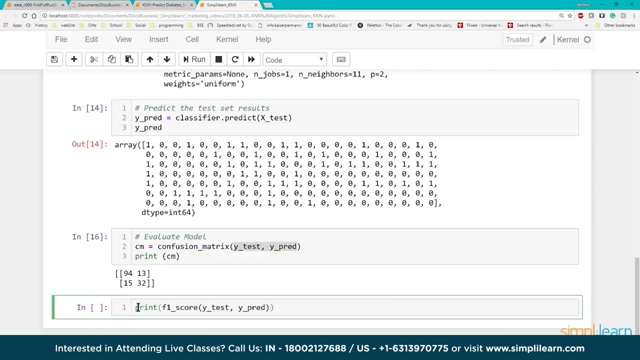 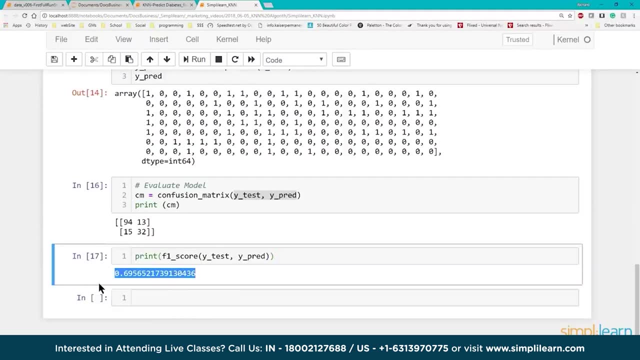 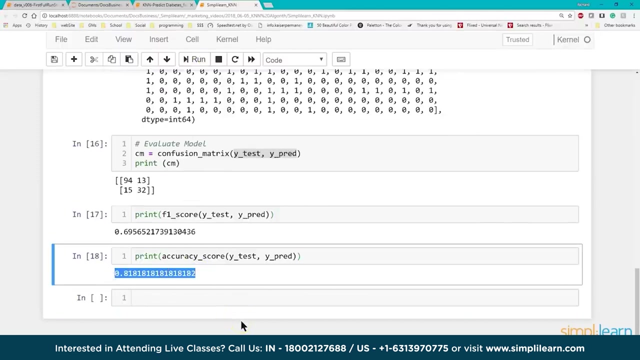 On the confusion matrix, Then we're going to go ahead and print the F1 score. You just run that And you see we get a .69 in our F1 score. The F1 takes into account both sides of the balance of false positives, Where, if we go ahead and just do the accuracy account- and that's what most people think of- is it looks at just how many we got right out of how many we got wrong. So a lot of people. when you're a data scientist and you're talking to other data scientists. 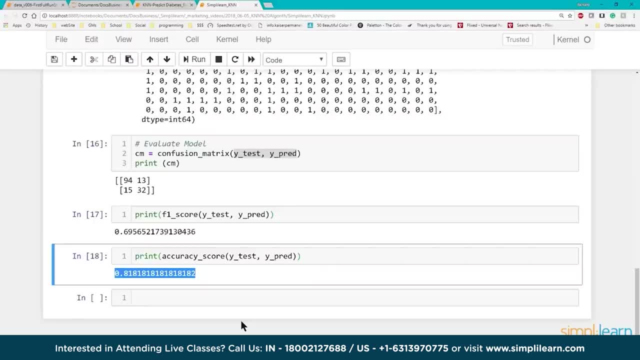 they're going to ask you what the F1 score, the F score, is. If you're talking to the general public or the decision makers in the business, they're going to ask what the accuracy is. And the accuracy is always better than the F1 score. But the F1 score is more telling. It lets us know that there's more false positives than we would like on here. But 82%- not too bad for a quick flash. look at people's different statistics. and running an SK Learn and running the KNN- the K nearest neighbor on it. 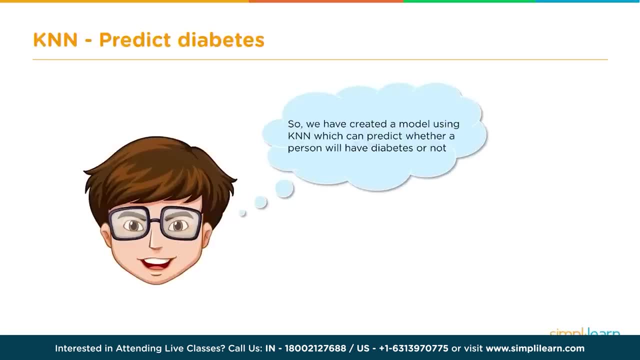 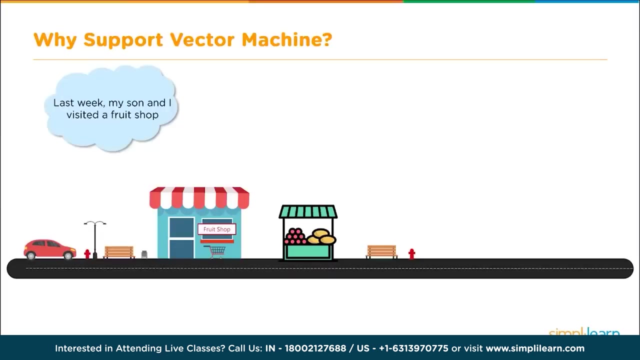 So we have a question here. I've created a model using KNN which can predict whether a person will have diabetes or not, or at the very least whether they should go get a checkup and have their glucose checked regularly or not. The print accuracy score we got the .818, was pretty close to what we got- and find out why support vector machine. So in this example, last week my son and I visited a fruit shop. Dad, is that an apple or a strawberry? So the question comes up: what fruit did I just pick up from the fruit stand? After a couple of seconds you can figure out. 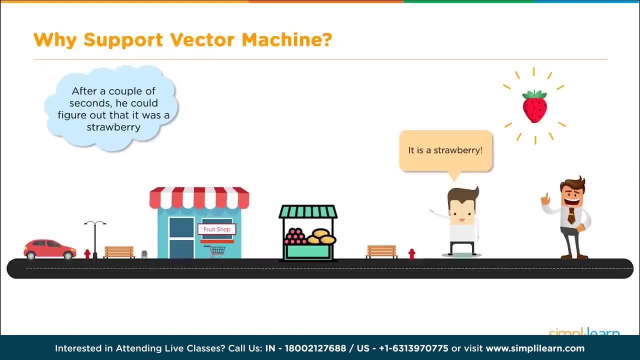 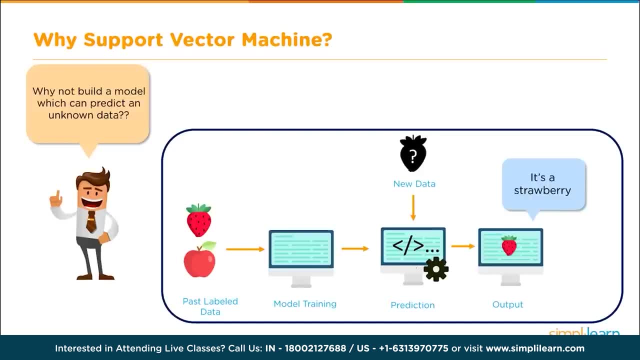 that it was a strawberry. So let's take this model a step further and let's- why not? build a model which can predict an unknown data. And then this: we're going to be looking at some sweet strawberries or crispy apples. We want it to be able to label those two and decide what. 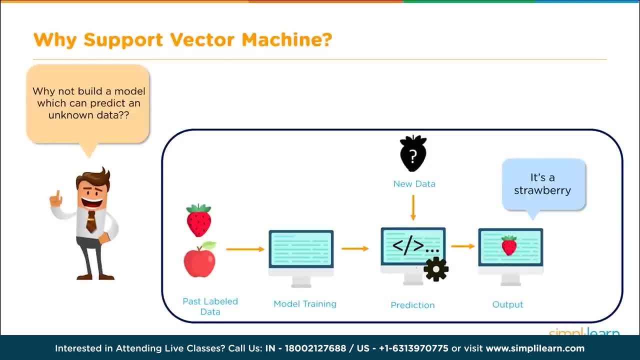 the fruit is, And we do that by having data already put in. So we already have a bunch of strawberries. We know our strawberries and they're already labeled as such. We already have a bunch of apples. We know our apples and are labeled as such. 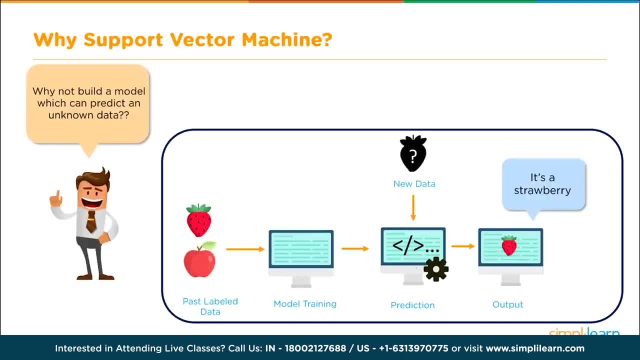 Then once we train our model, that model then can be given the new data. And the new data is this image: In this case, you can see a question mark on it and it comes through and goes: it's a strawberry. In this case we're using the support vector machine model. 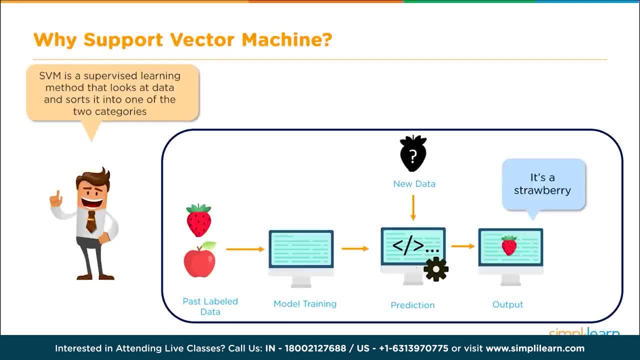 SVM is a supervised learning method that looks at data and sorts it into one of two categories, And in this case we're sorting the strawberry into the strawberry side. At this point, you should be asking the question: how does the prediction work? 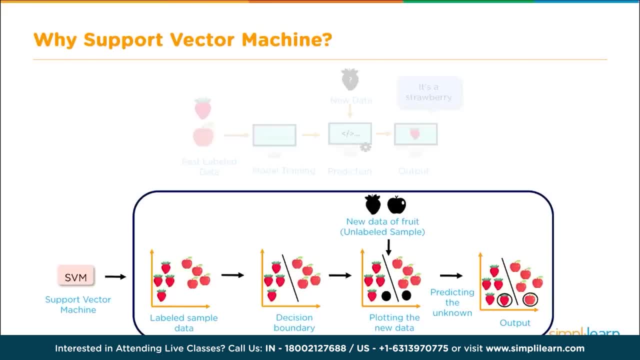 Before we dig into an example with numbers, let's apply this to our fruit scenario. We have our support vector machine. We've taken it and we've taken a labeled sample of data- strawberries and apples- and we've drawn a line down the middle between the two groups. 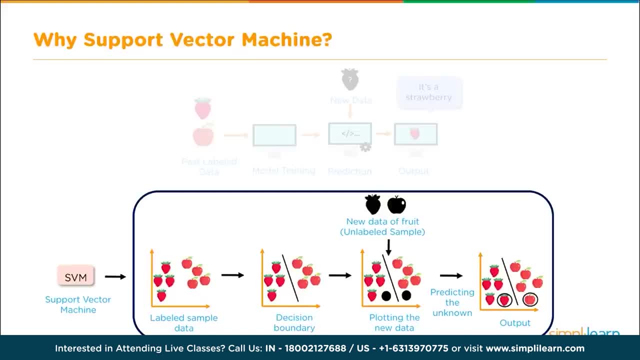 This split now allows us to take new data, in this case an apple and a strawberry, and place them in the appropriate group based on which side of the line they fall in, And that way we can predict the unknown. As colorful and tasty as the fruit example is, let's take a look at another example, with some numbers involved. 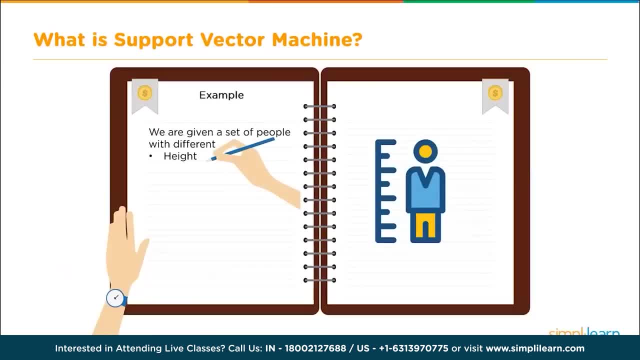 And we can take a closer look at how the math works In this example. we're going to be classifying men and women And we're going to start with a set of people with a different height and a different weight And to make this work, we'll have to have a sample data set of female 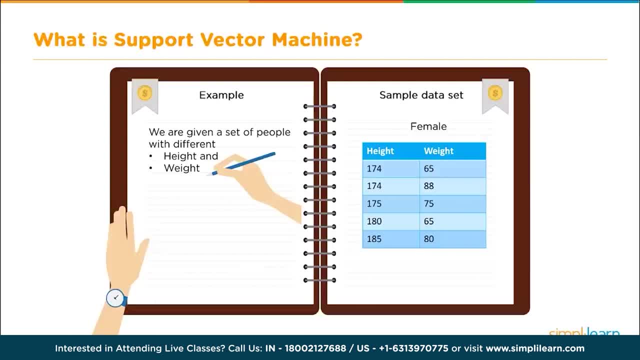 where you have their height and weight: 174,, 65,, 174,, 88, and so on- And we'll need a sample data set of the male. They have a height 179,, 90,, 180 to 80, and so on. 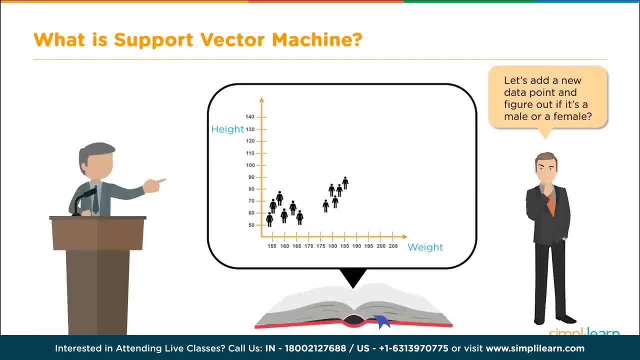 Let's go ahead and put this on a graph so we have a nice visual. So you can see, here we have two groups, based on the height versus the weight, And on the left side we're going to have the women, On the right side we're going to have the men. 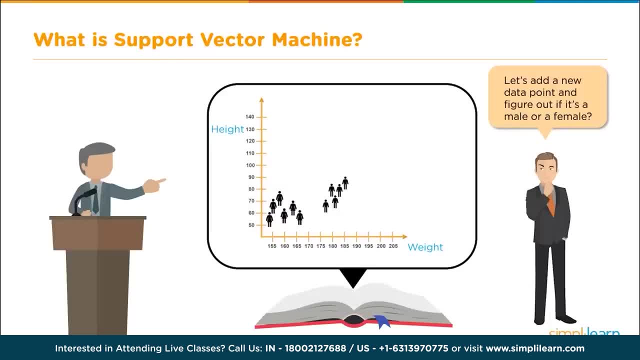 Now, if we're going to create a classifier, let's add a new data point and figure out if it's male or female. So before we can do that, we need to split our data first. We can split our data by choosing any of these lines: 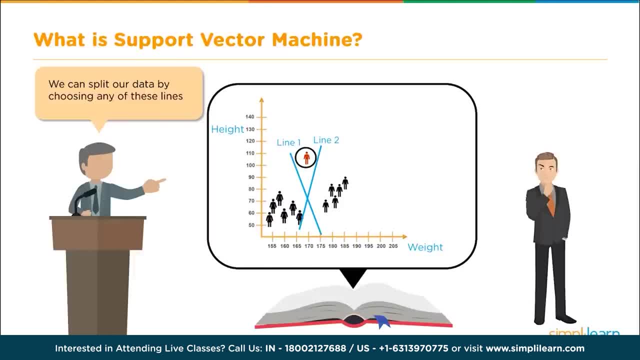 In this case we've drawn two lines through the data in the middle that separates the men from the women. But to predict the gender of a new data point, we should split the data in the best possible way. And we say the best possible way because this line has a maximum space that separates the two groups. 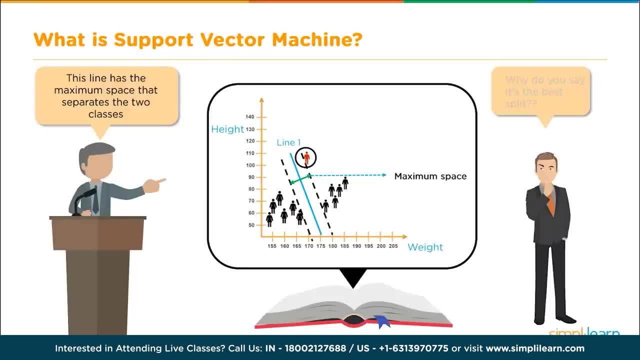 So we can say the best possible way, because this line has a maximum space that separates the two classes. Here you can see there's a clear split between the two different classes and in this one there's not so much a clear split. This doesn't have the maximum space that separates the two. 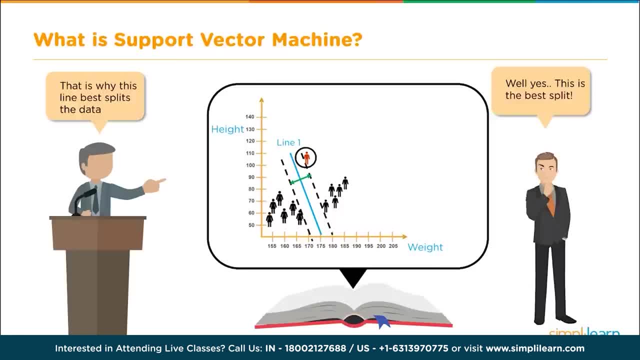 That is why this line best splits the data. We don't want to just do this by eyeballing it, And before we go further, we need to add some technical terms to this. We can also say that the distance between the points in the line should be as far as possible. 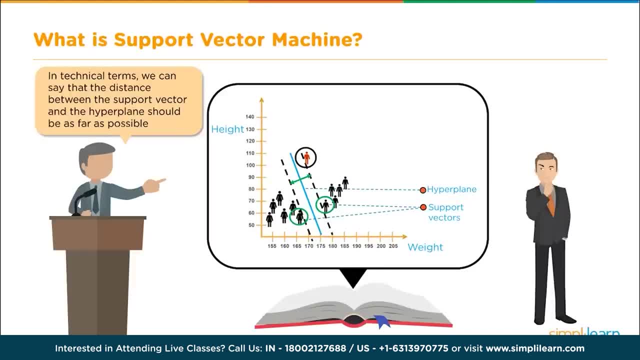 In technical terms we can say the distance between the support vector and the hyperplane is equal to the distance between the support vector and the hyperplane. And we can also say that the distance between the points and the line should be as far as possible. 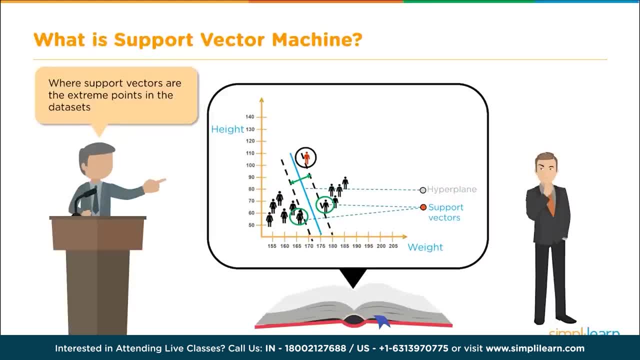 And we can also say that the distance between the points and the line should be as far as possible, And this is where the support vectors are the extreme points in the data set, And this is where the support vectors are the extreme points in the data set. 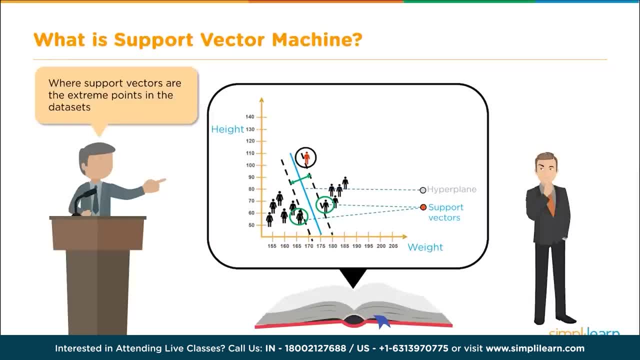 And if you look at this data set, they have circled two points which seem to be right on the outskirts of the women and one on the outskirts of the men. And if you look at this data set, they have circled two points which seem to be right on the outskirts of the women and one on the outskirts of the men. 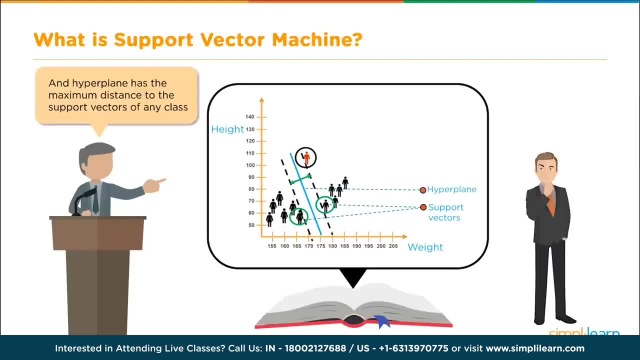 And if you look at this data set, they have circled two points which seem to be right on the outskirts of the women and one on the outskirts of the men, And hyperplane has the maximum distance to the support vectors of any class. 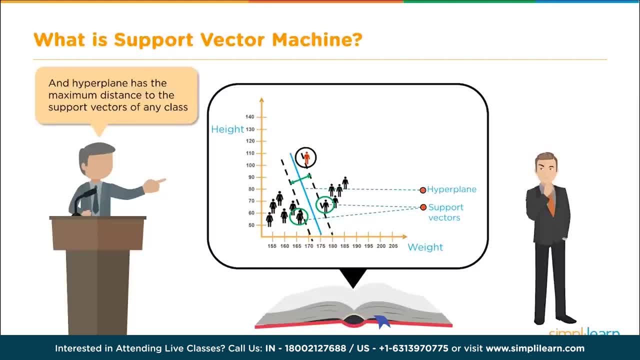 And hyperplane has the maximum distance to the support vectors of any class. And hyperplane has the maximum distance to the support vectors of any class. Now you'll see the line down the middle, and we call this the hyperplane because when you're dealing with multiple dimensions, it's really not just a line but a plane of intersections. 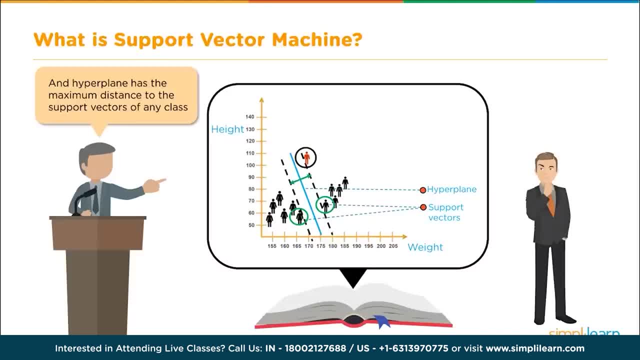 Now you'll see the line down the middle, and we call this the hyperplane, because when you're dealing with multiple dimensions, it's really not just a line but a plane of intersections. Now you'll see the line down the middle, and we call this the hyperplane, because when you're dealing with multiple dimensions, it's really not just a line but a plane of intersections. 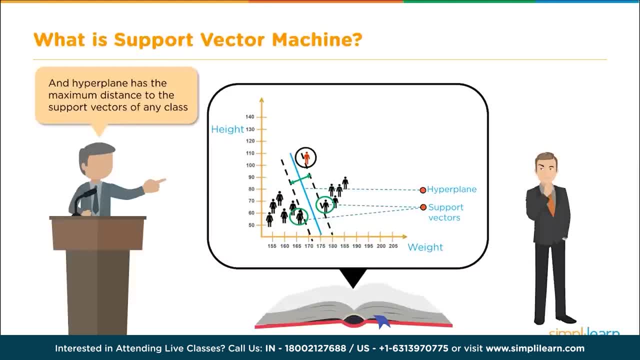 Now you'll see the line down the middle, and we call this the hyperplane, because when you're dealing with multiple dimensions, it's really not just a line but a plane of intersections, And you can see here where the support vectors have been drawn in dashed lines. 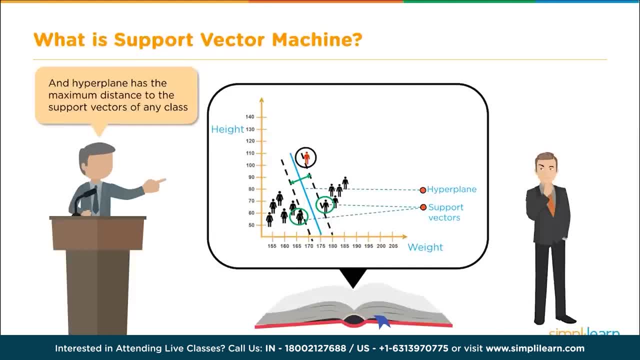 And you can see here where the support vectors have been drawn in dashed lines. And you can see here where the support vectors have been drawn in dashed lines. The math behind this is very simple. We take D plus the shortest distance to the closest positive point, which would be on the men's side. 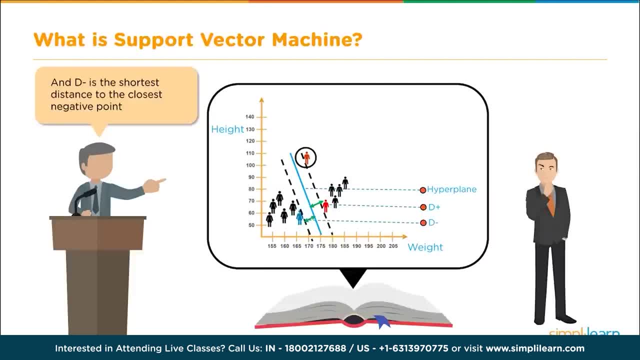 We take D plus the shortest distance to the closest positive point, which would be on the men's side. We take D plus the shortest distance to the closest positive point, which would be on the men's side, And D minus is the shortest distance to the closest negative point, which is on the women's side. 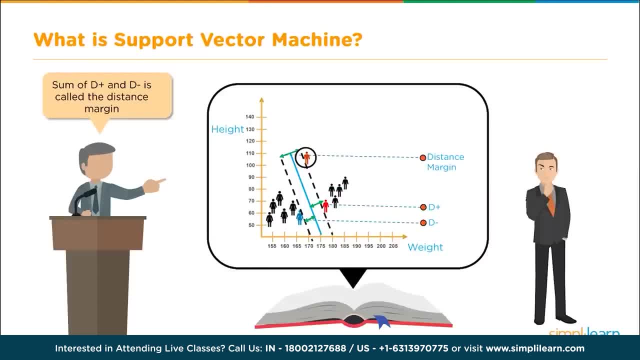 And D minus is the shortest distance to the closest negative point, which is on the women's side. The sum of D plus and D minus is called the distance margin, or the distance between the two support vectors that are shown in the dashed lines. 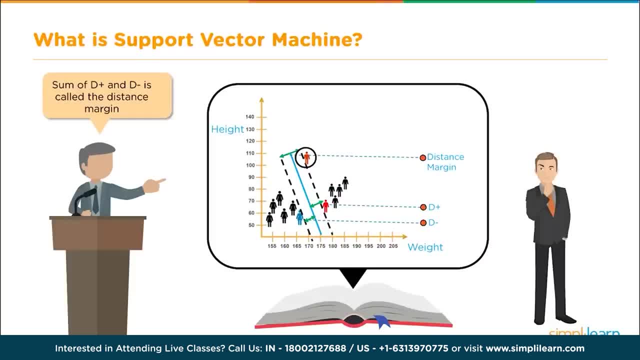 The sum of D plus and D minus is called the distance margin, or the distance between the two support vectors that are shown in the dashed lines. The sum of D plus and D minus is called the distance margin, or the distance between the two support vectors that are shown in the dashed lines. 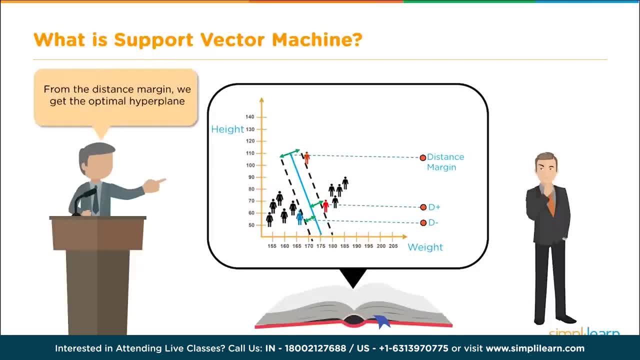 The sum of D plus and D minus is called the distance margin, or the distance between the two support vectors that are shown in the dashed lines, And then, by finding the largest distance margin, we can get the optimal hyperplane. And then, by finding the largest distance margin, we can get the optimal hyperplane. 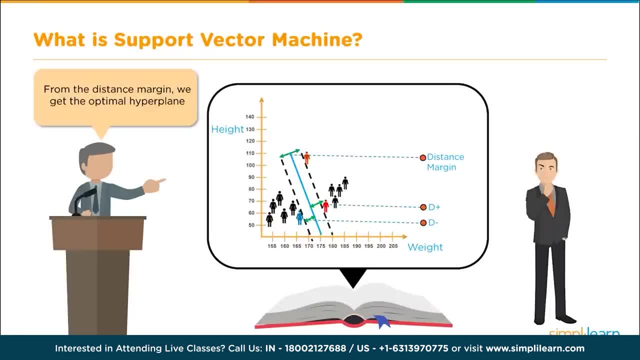 And then, by finding the largest distance margin, we can get the optimal hyperplane. Once we've created an optimal hyperplane, we can easily see which side the new data fits in. Once we've created an optimal hyperplane, we can easily see which side the new data fits in. 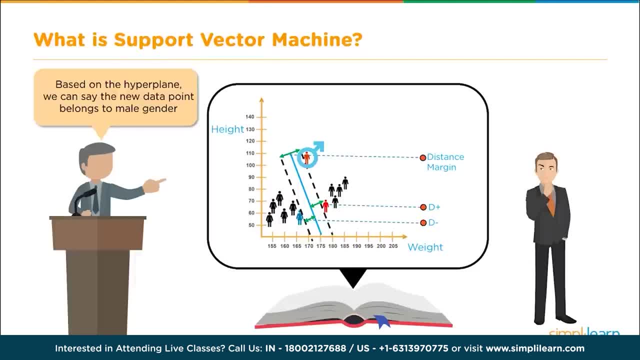 And, based on the hyperplane, we can say the new data point belongs to the male gender And, based on the hyperplane, we can say the new data point belongs to the male gender And, based on the hyperplane, we can say the new data point belongs to the male gender. 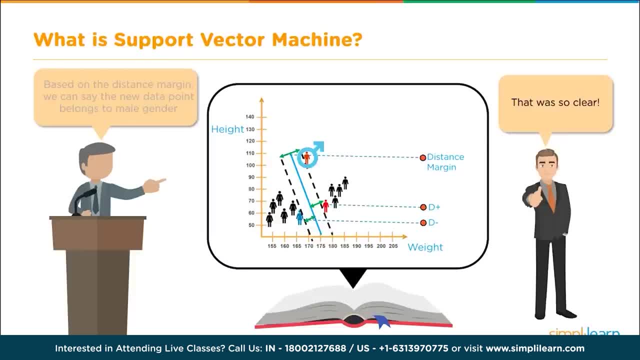 Hopefully that's clear how that works on a visual level. As a data scientist, you should also be asking what happens if the hyperplane is not optimal. As a data scientist, you should also be asking what happens if the hyperplane is not optimal. 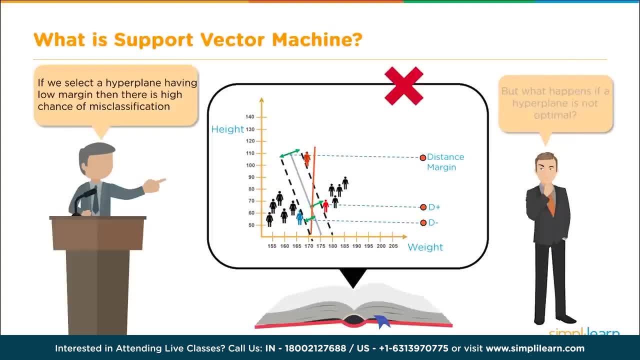 As a data scientist, you should also be asking what happens if the hyperplane is not optimal. If we select a hyperplane having low margin, then there is a high chance of misclassification. If we select a hyperplane having low margin, then there is a high chance of misclassification. 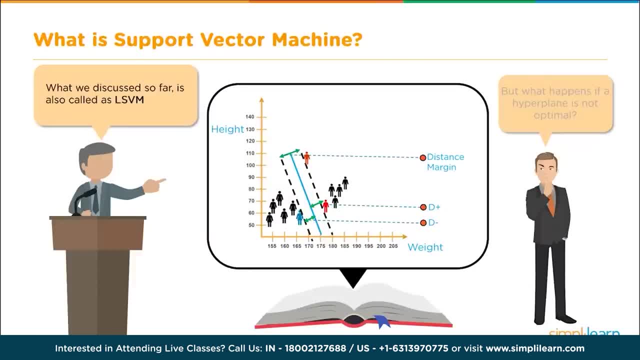 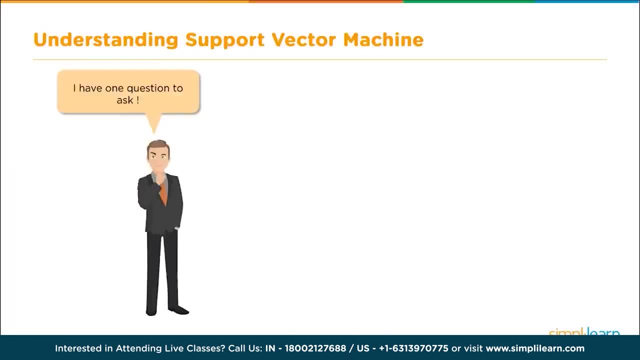 This particular SVM model, the one we discussed so far, is also called or referred to as the LSVM. So far, so clear, but a question should be coming up. So far, so clear, but a question should be coming up. We have our sample data set, but instead of looking like this, what if it looked like this? 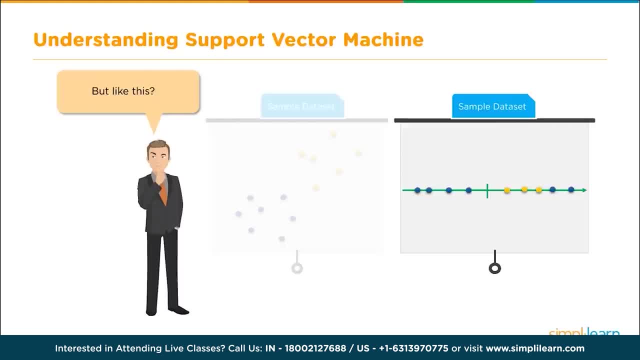 We have our sample data set, but instead of looking like this, what if it looked like this? We have our sample data set, but instead of looking like this, what if it looked like this: Where we have two sets of data, but one of them occurs in the middle of another set? 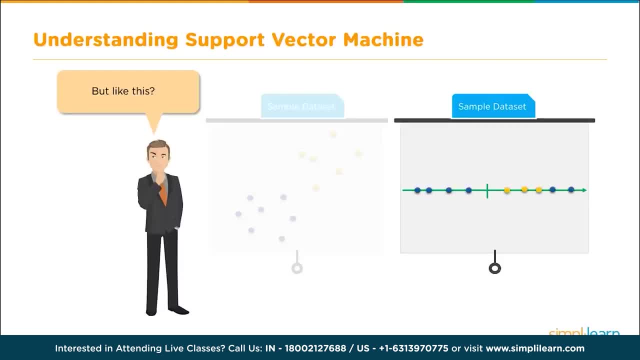 Where we have two sets of data but one of them occurs in the middle of another set. You can see here where we have the blue and the yellow and then blue again on the other side of our data line. You can see here where we have the blue and the yellow and then blue again on the other side of our data line. 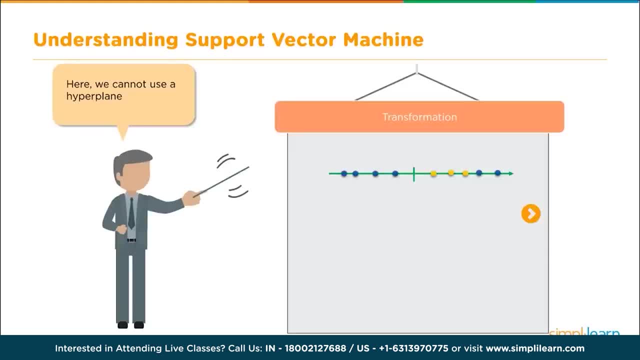 In this data set, we can't use a hyperplane. In this data set, we can't use a hyperplane. So when you see data like this, it's necessary to move away from a 1D view of the data to a two-dimensional view of the data. 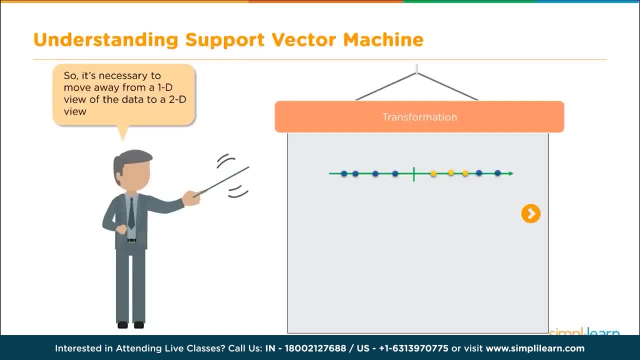 So, when you see data like this, it's necessary to move away from a 1D view of the data to a two-dimensional view of the data. So, when you see data like this, it's necessary to move away from a 1D view of the data to a two-dimensional view of the data. 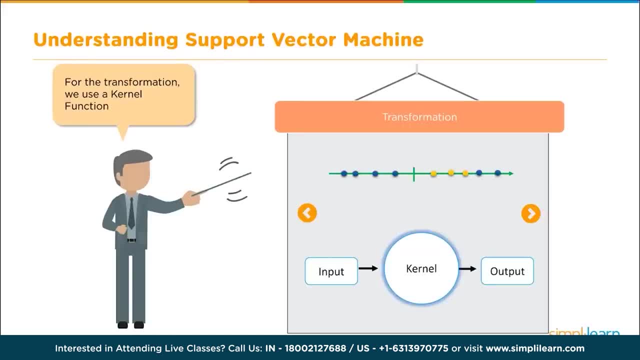 So, when you see data like this, it's necessary to move away from a 1D view of the data to a two-dimensional view of the data. So, when you see data like this, it's necessary to move away from a 1D view of the data to a two-dimensional view of the data. 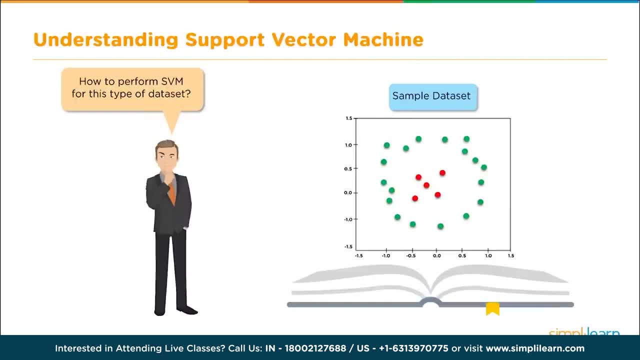 So, when you see data like this, it's necessary to move away from a 1D view of the data to a two-dimensional view of the data. So, when you see data like this, it's necessary to move away from a 1D view of the data to a two-dimensional view of the data. 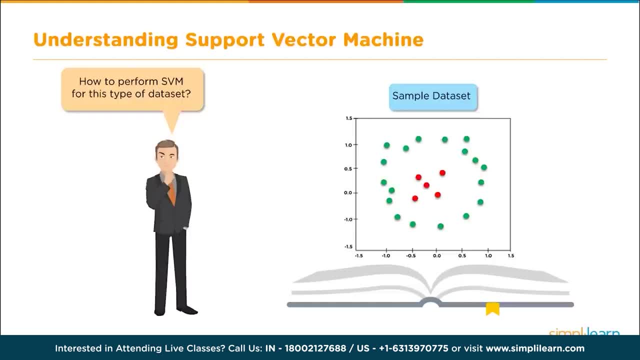 So, when you see data like this, it's necessary to move away from a 1D view of the data to a two-dimensional view of the data. So, when you see data like this, it's necessary to move away from a 1D view of the data to a two-dimensional view of the data. 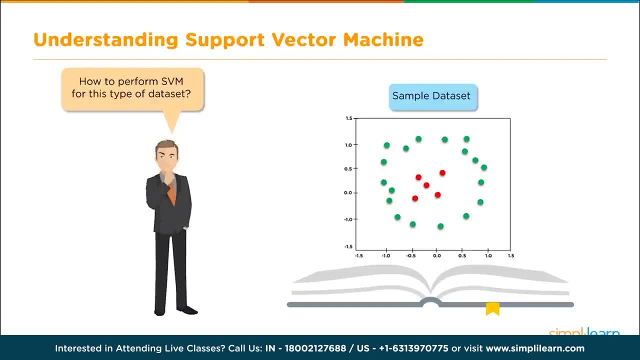 So, when you see data like this, it's necessary to move away from a 1D view of the data to a two-dimensional view of the data. So, when you see data like this, it's necessary to move away from a 1D view of the data to a two-dimensional view of the data. 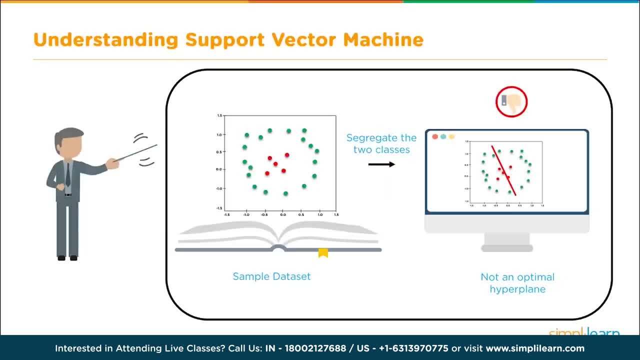 So, when you see data like this, it's necessary to move away from a 1D view of the data to a two-dimensional view of the data. So, when you see data like this, it's necessary to move away from a 1D view of the data to a two-dimensional view of the data. 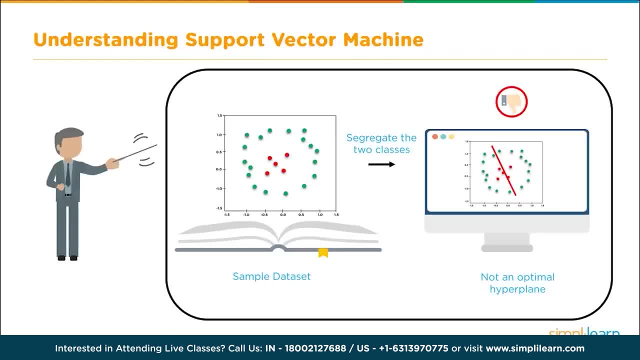 So, when you see data like this, it's necessary to move away from a 1D view of the data to a two-dimensional view of the data. So, when you see data like this, it's necessary to move away from a 1D view of the data to a two-dimensional view of the data. 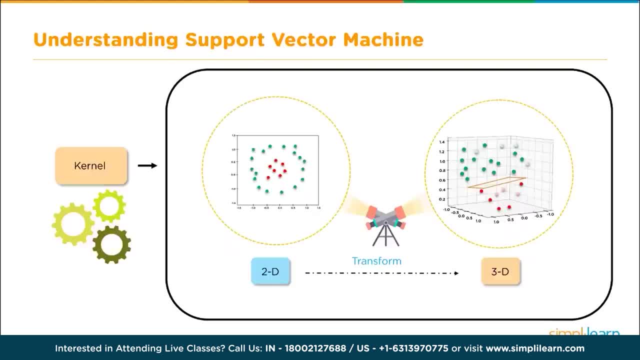 So, when you see data like this, it's necessary to move away from a 1D view of the data to a two-dimensional view of the data. So, when you see data like this, it's necessary to move away from a 1D view of the data to a two-dimensional view of the data. 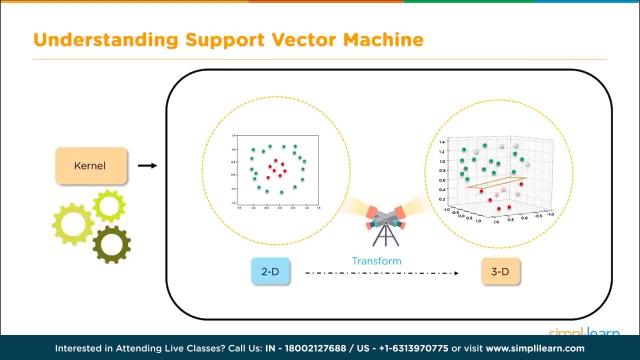 So, when you see data like this, it's necessary to move away from a 1D view of the data to a two-dimensional view of the data. So, when you see data like this, it's necessary to move away from a 1D view of the data to a two-dimensional view of the data. 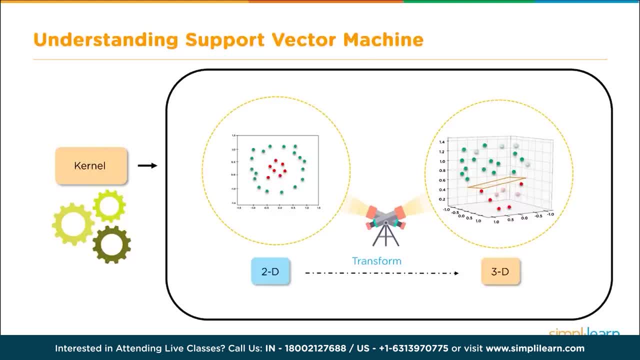 So, when you see data like this, it's necessary to move away from a 1D view of the data to a two-dimensional view of the data. So, when you see data like this, it's necessary to move away from a 1D view of the data to a two-dimensional view of the data. 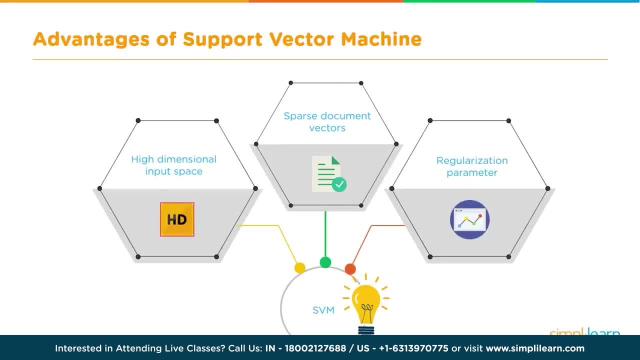 So, when you see data like this, it's necessary to move away from a 1D view of the data to a two-dimensional view of the data. So, when you see data like this, it's necessary to move away from a 1D view of the data to a two-dimensional view of the data. 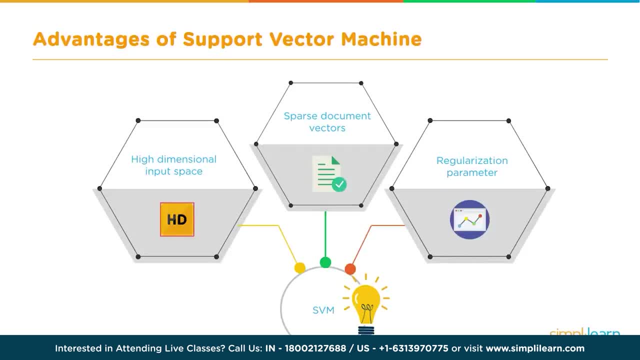 So, when you see data like this, it's necessary to move away from a 1D view of the data to a two-dimensional view of the data. So, when you see data like this, it's necessary to move away from a 1D view of the data to a two-dimensional view of the data. 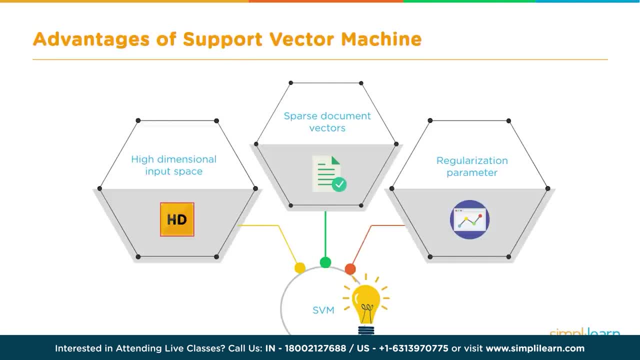 So, when you see data like this, it's necessary to move away from a 1D view of the data to a two-dimensional view of the data. So, when you see data like this, it's necessary to move away from a 1D view of the data to a two-dimensional view of the data. 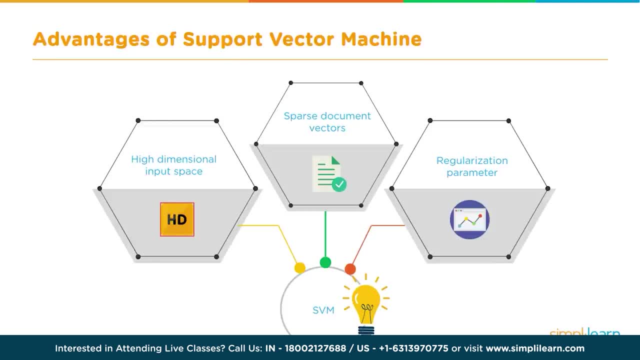 So, when you see data like this, it's necessary to move away from a 1D view of the data to a two-dimensional view of the data. So, when you see data like this, it's necessary to move away from a 1D view of the data to a two-dimensional view of the data. 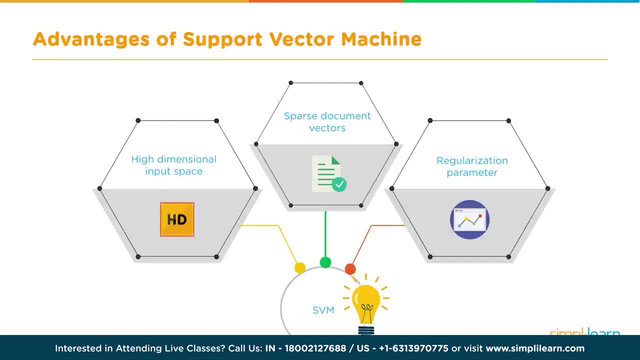 So, when you see data like this, it's necessary to move away from a 1D view of the data to a two-dimensional view of the data. So, when you see data like this, it's necessary to move away from a 1D view of the data to a two-dimensional view of the data. 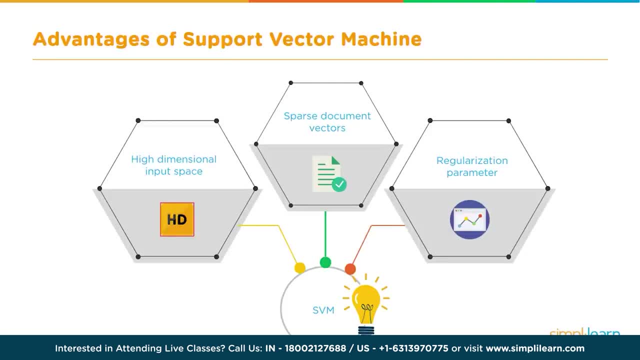 So, when you see data like this, it's necessary to move away from a 1D view of the data to a two-dimensional view of the data. So, when you see data like this, it's necessary to move away from a 1D view of the data to a two-dimensional view of the data. 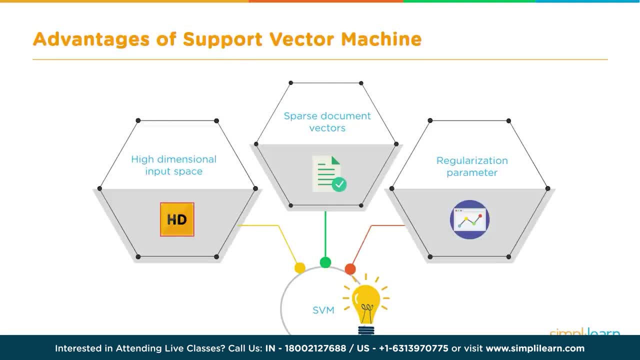 So, when you see data like this, it's necessary to move away from a 1D view of the data to a two-dimensional view of the data. So, when you see data like this, it's necessary to move away from a 1D view of the data to a two-dimensional view of the data. 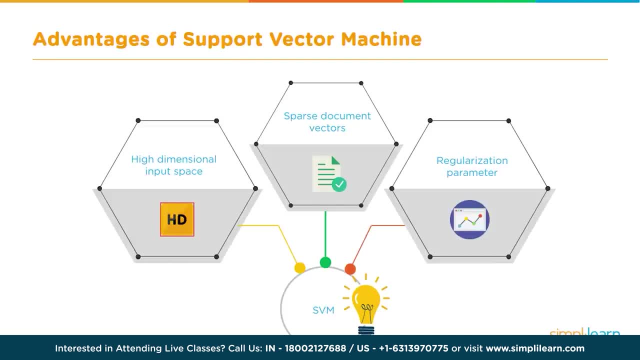 So, when you see data like this, it's necessary to move away from a 1D view of the data to a two-dimensional view of the data. So, when you see data like this, it's necessary to move away from a 1D view of the data to a two-dimensional view of the data. 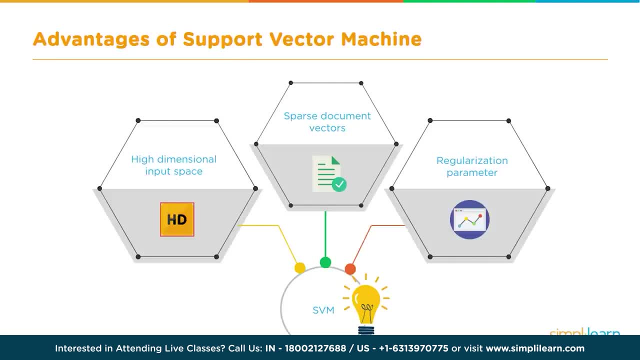 So, when you see data like this, it's necessary to move away from a 1D view of the data to a two-dimensional view of the data. So, when you see data like this, it's necessary to move away from a 1D view of the data to a two-dimensional view of the data. 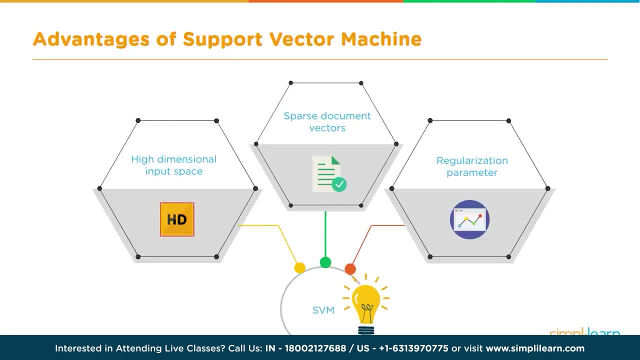 So, when you see data like this, it's necessary to move away from a 1D view of the data to a two-dimensional view of the data. So, when you see data like this, it's necessary to move away from a 1D view of the data to a two-dimensional view of the data. 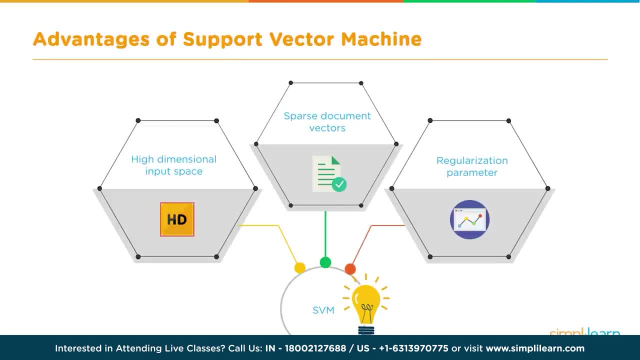 So, when you see data like this, it's necessary to move away from a 1D view of the data to a two-dimensional view of the data. So, when you see data like this, it's necessary to move away from a 1D view of the data to a two-dimensional view of the data. 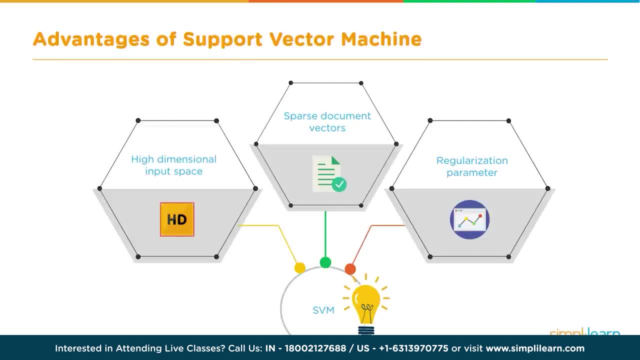 So, when you see data like this, it's necessary to move away from a 1D view of the data to a two-dimensional view of the data. So, when you see data like this, it's necessary to move away from a 1D view of the data to a two-dimensional view of the data. 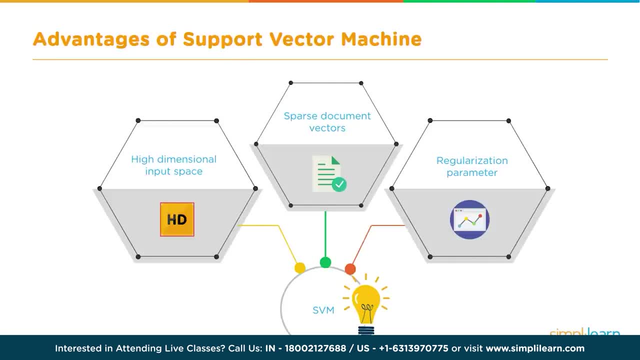 So, when you see data like this, it's necessary to move away from a 1D view of the data to a two-dimensional view of the data. So, when you see data like this, it's necessary to move away from a 1D view of the data to a two-dimensional view of the data. 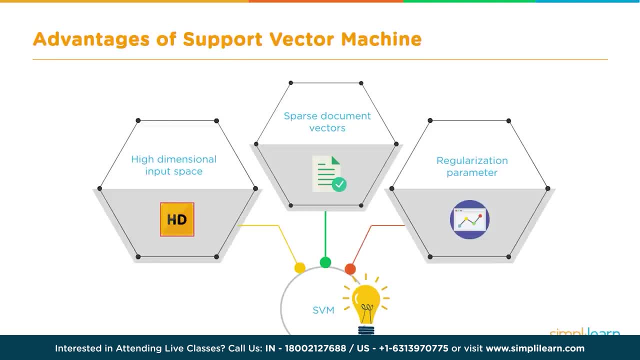 So, when you see data like this, it's necessary to move away from a 1D view of the data to a two-dimensional view of the data. So, when you see data like this, it's necessary to move away from a 1D view of the data to a two-dimensional view of the data. 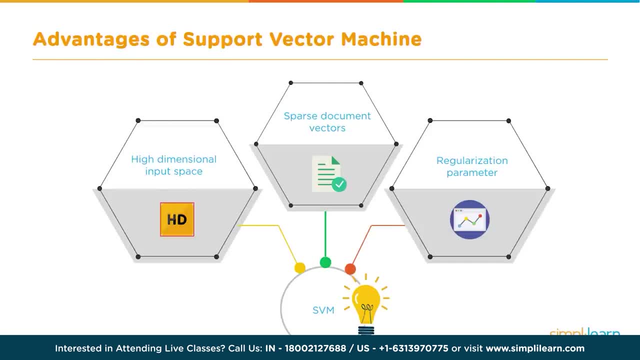 So, when you see data like this, it's necessary to move away from a 1D view of the data to a two-dimensional view of the data. So, when you see data like this, it's necessary to move away from a 1D view of the data to a two-dimensional view of the data. 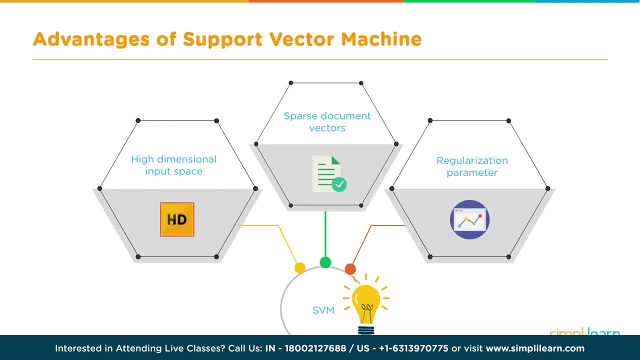 So, when you see data like this, it's necessary to move away from a 1D view of the data to a two-dimensional view of the data. So, when you see data like this, it's necessary to move away from a 1D view of the data to a two-dimensional view of the data. 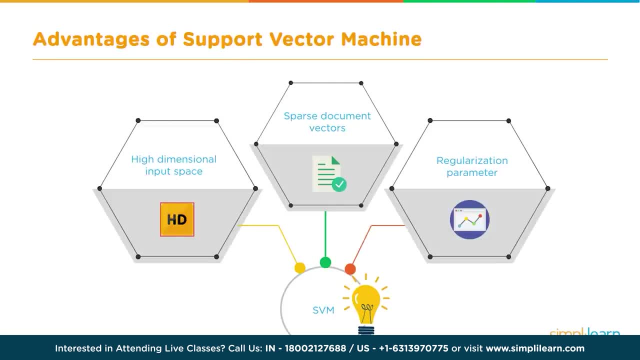 So, when you see data like this, it's necessary to move away from a 1D view of the data to a two-dimensional view of the data. So, when you see data like this, it's necessary to move away from a 1D view of the data to a two-dimensional view of the data. 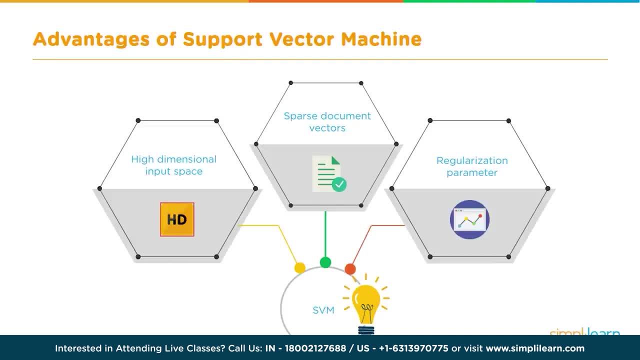 So, when you see data like this, it's necessary to move away from a 1D view of the data to a two-dimensional view of the data. So, when you see data like this, it's necessary to move away from a 1D view of the data to a two-dimensional view of the data. 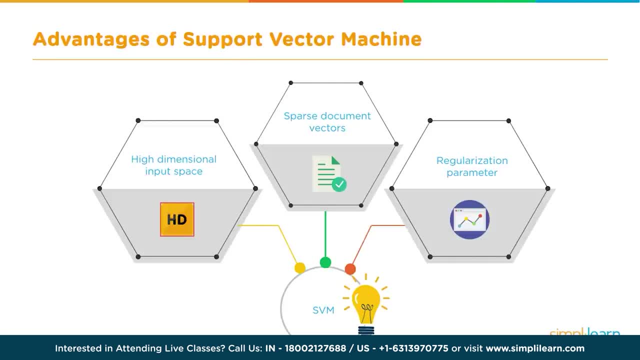 So, when you see data like this, it's necessary to move away from a 1D view of the data to a two-dimensional view of the data. So, when you see data like this, it's necessary to move away from a 1D view of the data to a two-dimensional view of the data. 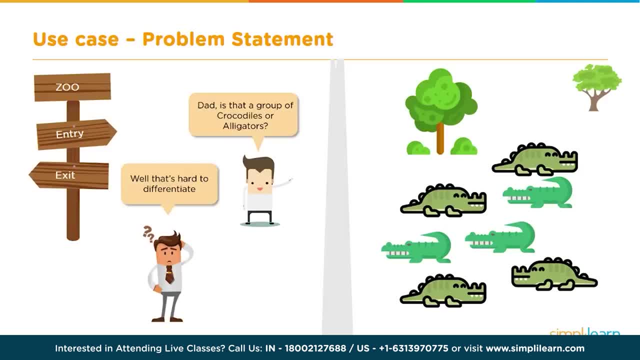 So, when you see data like this, it's necessary to move away from a 1D view of the data to a two-dimensional view of the data. So, when you see data like this, it's necessary to move away from a 1D view of the data to a two-dimensional view of the data. 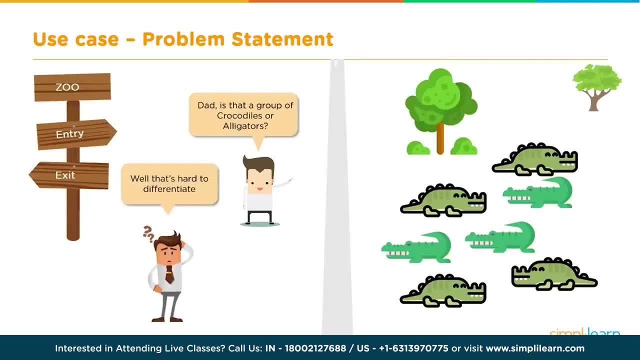 So, when you see data like this, it's necessary to move away from a 1D view of the data to a two-dimensional view of the data. So, when you see data like this, it's necessary to move away from a 1D view of the data to a two-dimensional view of the data. 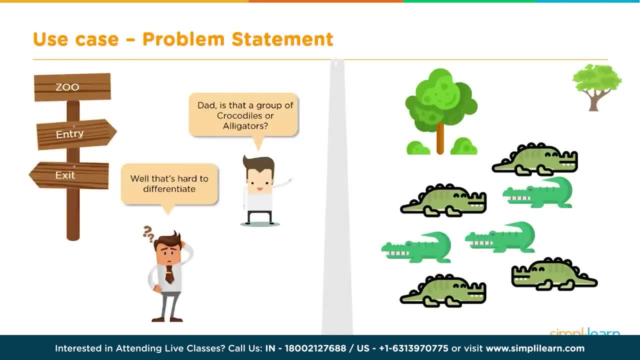 So, when you see data like this, it's necessary to move away from a 1D view of the data to a two-dimensional view of the data. So, when you see data like this, it's necessary to move away from a 1D view of the data to a two-dimensional view of the data. 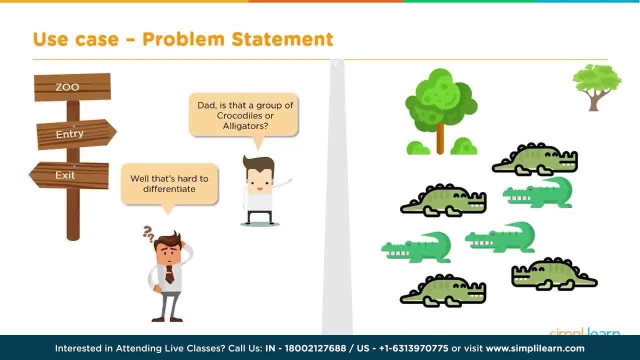 So, when you see data like this, it's necessary to move away from a 1D view of the data to a two-dimensional view of the data. So, when you see data like this, it's necessary to move away from a 1D view of the data to a two-dimensional view of the data. 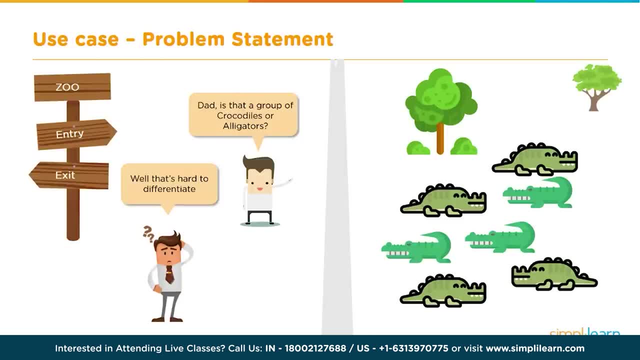 So, when you see data like this, it's necessary to move away from a 1D view of the data to a two-dimensional view of the data. So, when you see data like this, it's necessary to move away from a 1D view of the data to a two-dimensional view of the data. 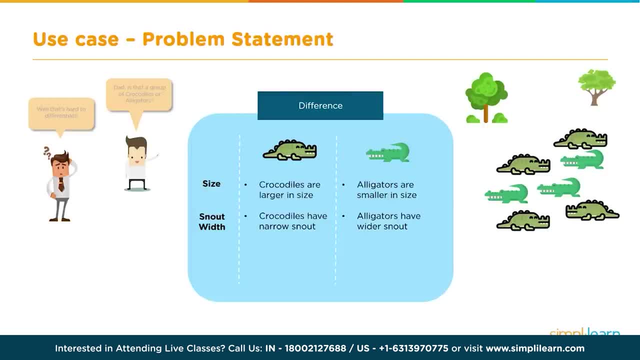 So, when you see data like this, it's necessary to move away from a 1D view of the data to a two-dimensional view of the data. So, when you see data like this, it's necessary to move away from a 1D view of the data to a two-dimensional view of the data. 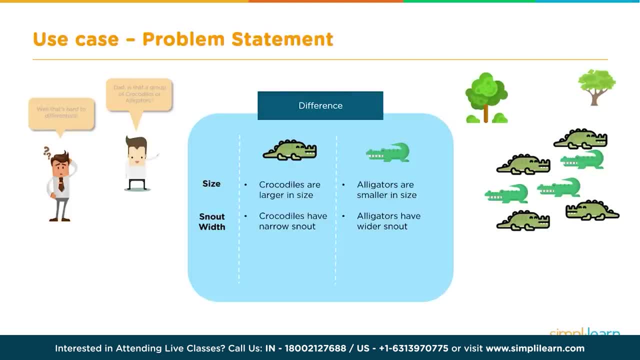 So, when you see data like this, it's necessary to move away from a 1D view of the data to a two-dimensional view of the data. So, when you see data like this, it's necessary to move away from a 1D view of the data to a two-dimensional view of the data. 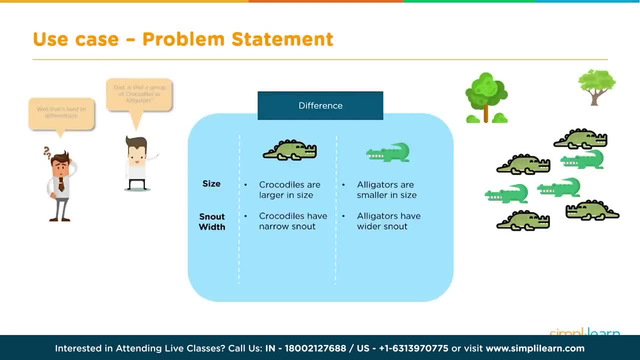 So, when you see data like this, it's necessary to move away from a 1D view of the data to a two-dimensional view of the data. So, when you see data like this, it's necessary to move away from a 1D view of the data to a two-dimensional view of the data. 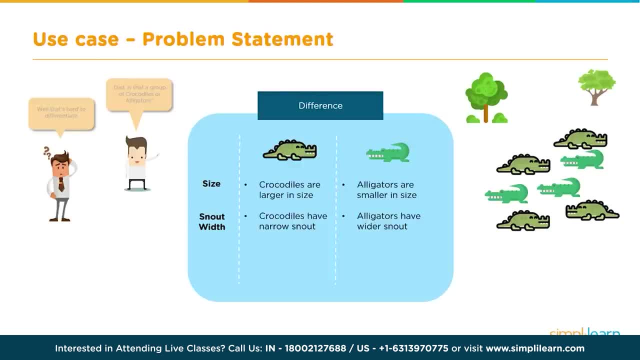 So, when you see data like this, it's necessary to move away from a 1D view of the data to a two-dimensional view of the data. So, when you see data like this, it's necessary to move away from a 1D view of the data to a two-dimensional view of the data. 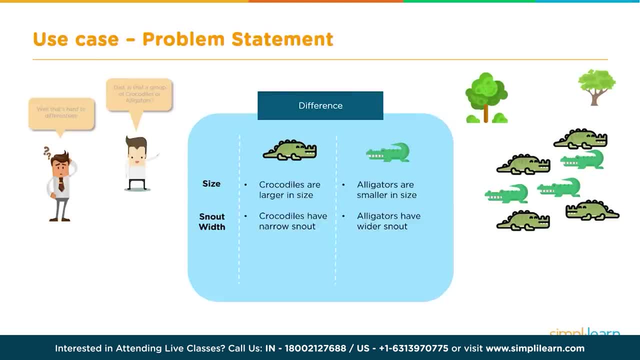 So, when you see data like this, it's necessary to move away from a 1D view of the data to a two-dimensional view of the data. So, when you see data like this, it's necessary to move away from a 1D view of the data to a two-dimensional view of the data. 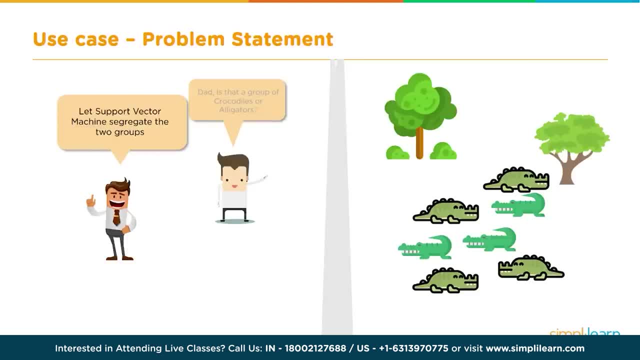 So, when you see data like this, it's necessary to move away from a 1D view of the data to a two-dimensional view of the data. So, when you see data like this, it's necessary to move away from a 1D view of the data to a two-dimensional view of the data. 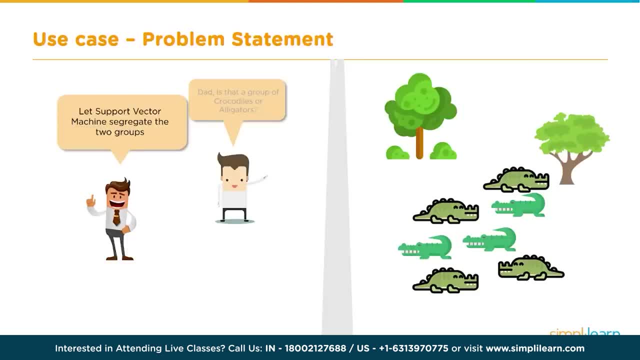 So, when you see data like this, it's necessary to move away from a 1D view of the data to a two-dimensional view of the data. So, when you see data like this, it's necessary to move away from a 1D view of the data to a two-dimensional view of the data. 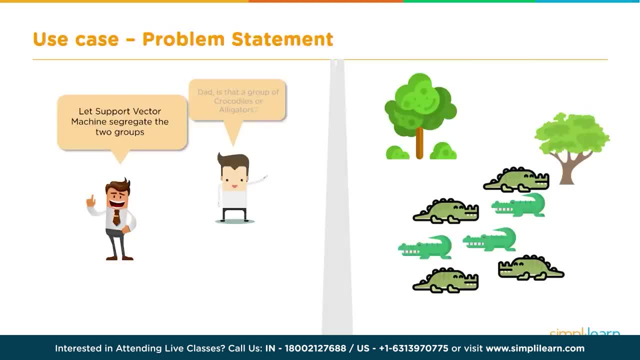 So, when you see data like this, it's necessary to move away from a 1D view of the data to a two-dimensional view of the data. So, when you see data like this, it's necessary to move away from a 1D view of the data to a two-dimensional view of the data. 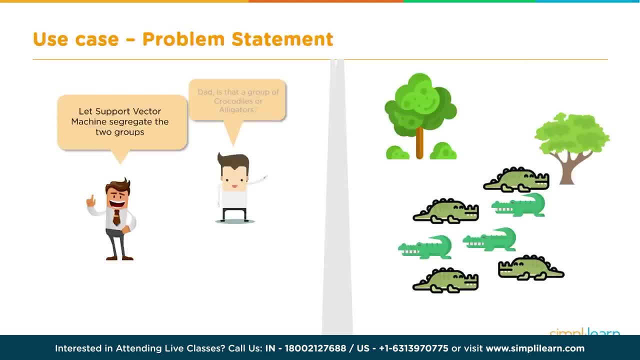 So, when you see data like this, it's necessary to move away from a 1D view of the data to a two-dimensional view of the data. So, when you see data like this, it's necessary to move away from a 1D view of the data to a two-dimensional view of the data. 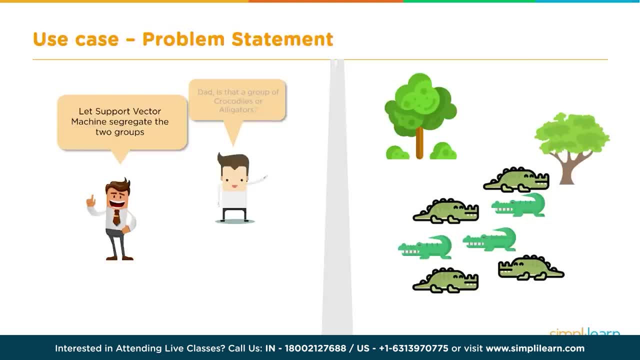 So, when you see data like this, it's necessary to move away from a 1D view of the data to a two-dimensional view of the data. So, when you see data like this, it's necessary to move away from a 1D view of the data to a two-dimensional view of the data. 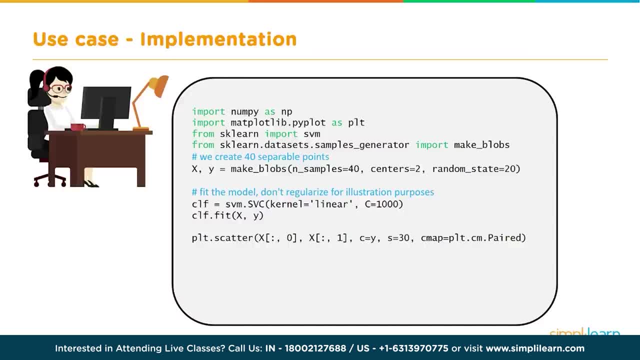 So, when you see data like this, it's necessary to move away from a 1D view of the data to a two-dimensional view of the data. So, when you see data like this, it's necessary to move away from a 1D view of the data to a two-dimensional view of the data. 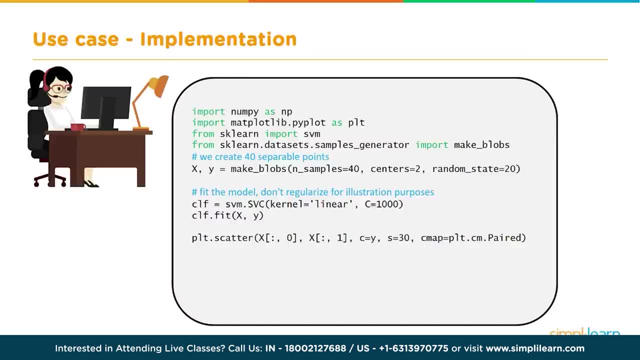 So, when you see data like this, it's necessary to move away from a 1D view of the data to a two-dimensional view of the data. So, when you see data like this, it's necessary to move away from a 1D view of the data to a two-dimensional view of the data. 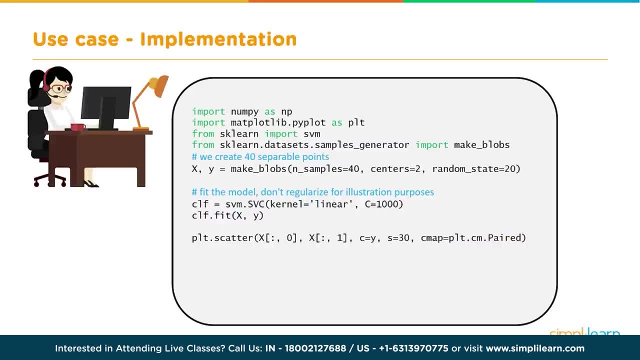 So, when you see data like this, it's necessary to move away from a 1D view of the data to a two-dimensional view of the data. So, when you see data like this, it's necessary to move away from a 1D view of the data to a two-dimensional view of the data. 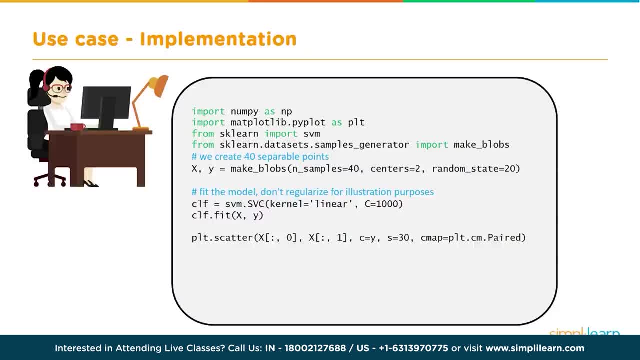 So, when you see data like this, it's necessary to move away from a 1D view of the data to a two-dimensional view of the data. So, when you see data like this, it's necessary to move away from a 1D view of the data to a two-dimensional view of the data. 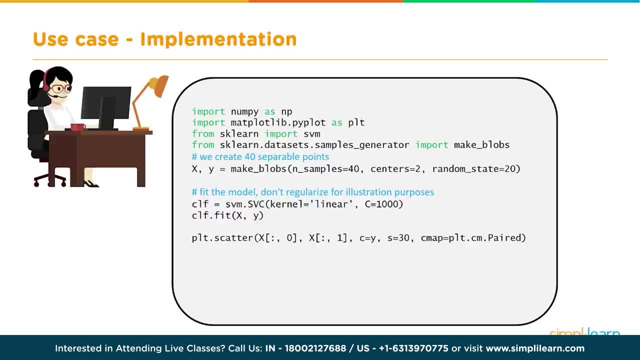 So, when you see data like this, it's necessary to move away from a 1D view of the data to a two-dimensional view of the data. So, when you see data like this, it's necessary to move away from a 1D view of the data to a two-dimensional view of the data. 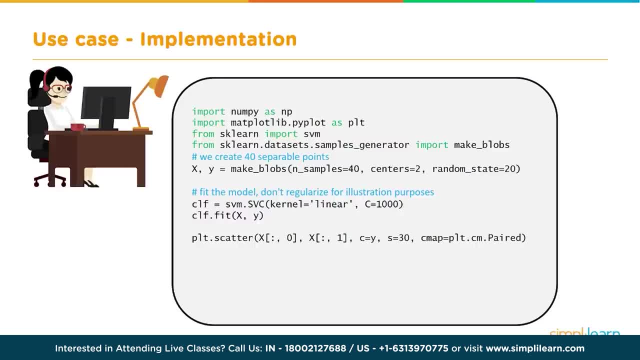 So, when you see data like this, it's necessary to move away from a 1D view of the data to a two-dimensional view of the data. So, when you see data like this, it's necessary to move away from a 1D view of the data to a two-dimensional view of the data. 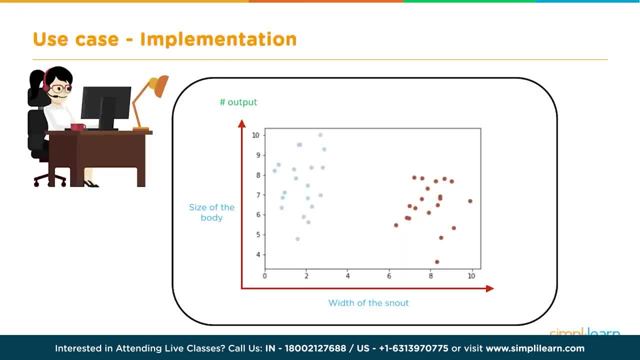 So, when you see data like this, it's necessary to move away from a 1D view of the data to a two-dimensional view of the data. So, when you see data like this, it's necessary to move away from a 1D view of the data to a two-dimensional view of the data. 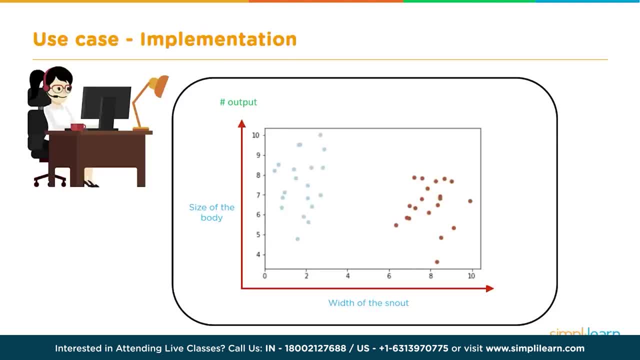 So, when you see data like this, it's necessary to move away from a 1D view of the data to a two-dimensional view of the data. So, when you see data like this, it's necessary to move away from a 1D view of the data to a two-dimensional view of the data. 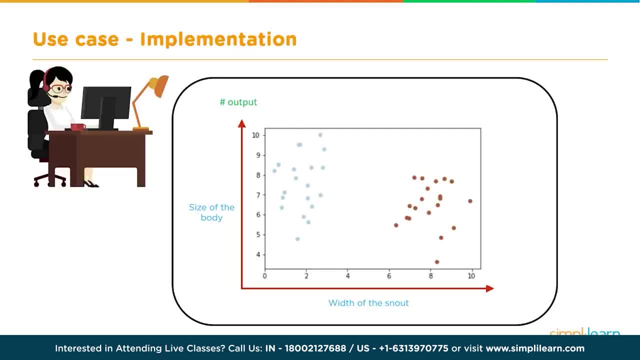 So, when you see data like this, it's necessary to move away from a 1D view of the data to a two-dimensional view of the data. So, when you see data like this, it's necessary to move away from a 1D view of the data to a two-dimensional view of the data. 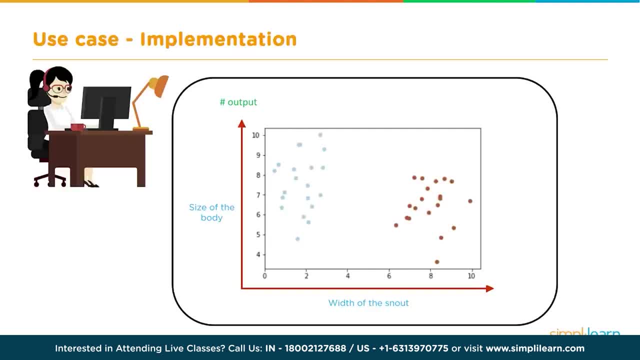 So, when you see data like this, it's necessary to move away from a 1D view of the data to a two-dimensional view of the data. So, when you see data like this, it's necessary to move away from a 1D view of the data to a two-dimensional view of the data. 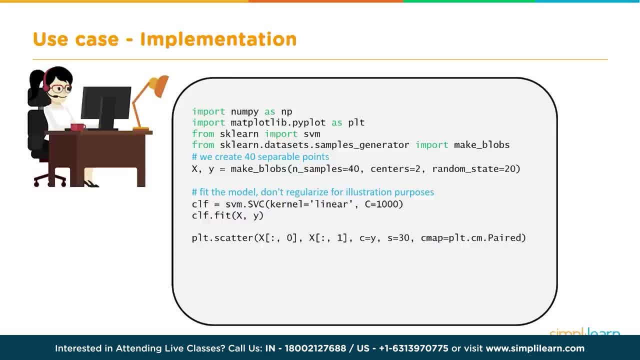 So, when you see data like this, it's necessary to move away from a 1D view of the data to a two-dimensional view of the data. So, when you see data like this, it's necessary to move away from a 1D view of the data to a two-dimensional view of the data. 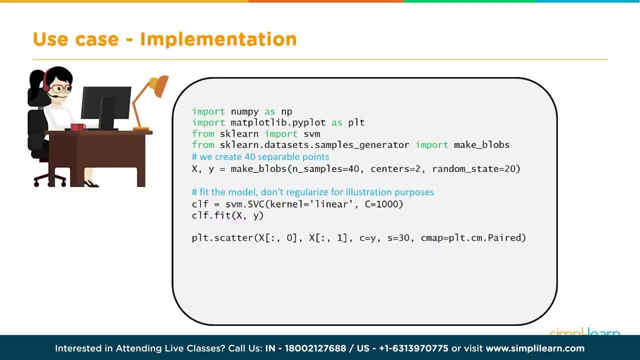 So, when you see data like this, it's necessary to move away from a 1D view of the data to a two-dimensional view of the data. So, when you see data like this, it's necessary to move away from a 1D view of the data to a two-dimensional view of the data. 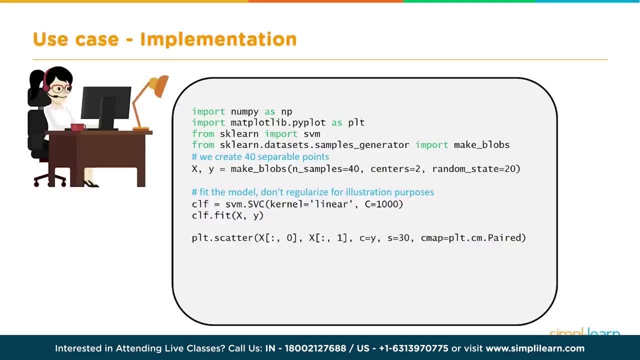 So, when you see data like this, it's necessary to move away from a 1D view of the data to a two-dimensional view of the data. So, when you see data like this, it's necessary to move away from a 1D view of the data to a two-dimensional view of the data. 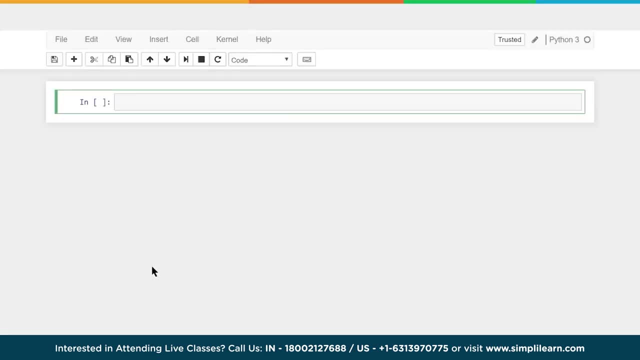 So, when you see data like this, it's necessary to move away from a 1D view of the data to a two-dimensional view of the data. So, when you see data like this, it's necessary to move away from a 1D view of the data to a two-dimensional view of the data. 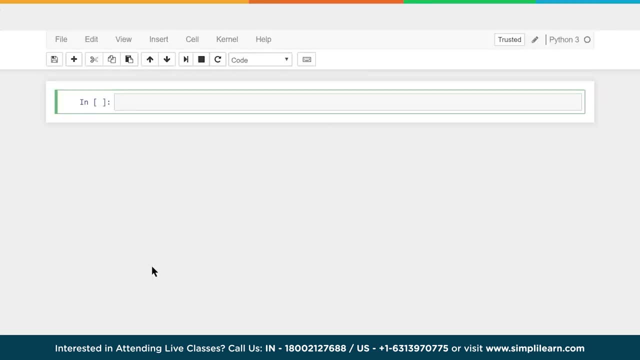 So, when you see data like this, it's necessary to move away from a 1D view of the data to a two-dimensional view of the data. So, when you see data like this, it's necessary to move away from a 1D view of the data to a two-dimensional view of the data. 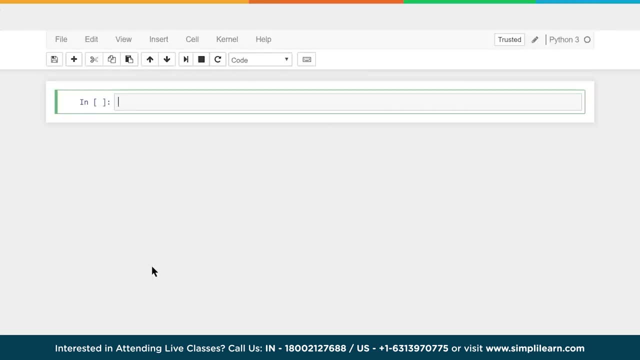 So, when you see data like this, it's necessary to move away from a 1D view of the data to a two-dimensional view of the data. So, when you see data like this, it's necessary to move away from a 1D view of the data to a two-dimensional view of the data. 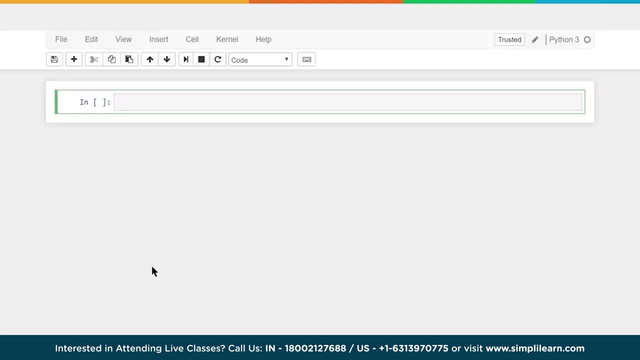 So, when you see data like this, it's necessary to move away from a 1D view of the data to a two-dimensional view of the data. So, when you see data like this, it's necessary to move away from a 1D view of the data to a two-dimensional view of the data. 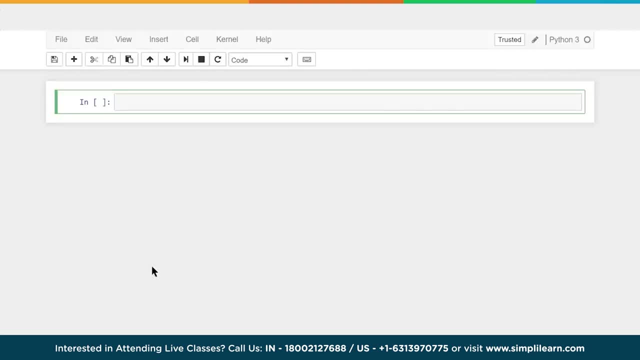 So, when you see data like this, it's necessary to move away from a 1D view of the data to a two-dimensional view of the data. So, when you see data like this, it's necessary to move away from a 1D view of the data to a two-dimensional view of the data. 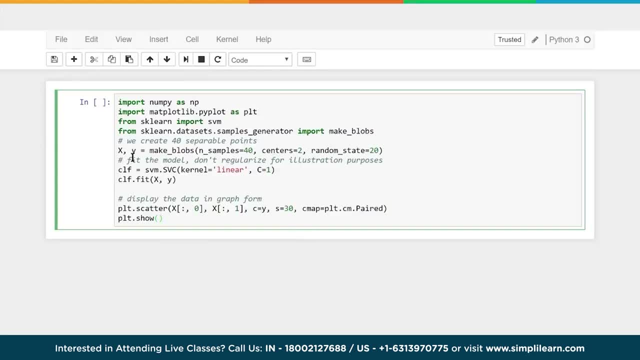 So, when you see data like this, it's necessary to move away from a 1D view of the data to a two-dimensional view of the data. So, when you see data like this, it's necessary to move away from a 1D view of the data to a two-dimensional view of the data. 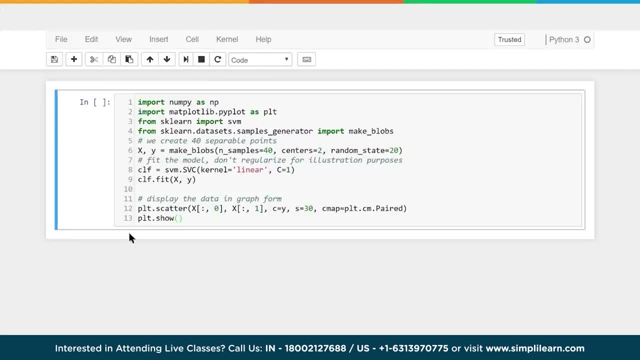 So, when you see data like this, it's necessary to move away from a 1D view of the data to a two-dimensional view of the data. So, when you see data like this, it's necessary to move away from a 1D view of the data to a two-dimensional view of the data. 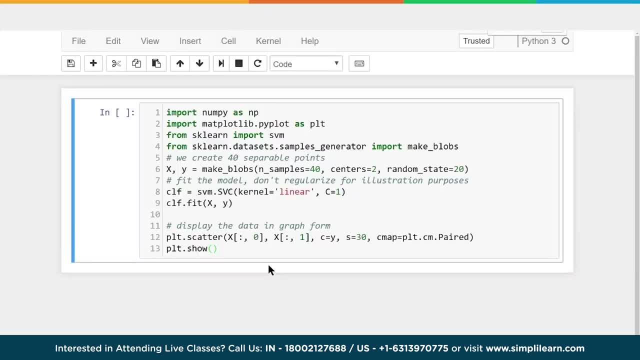 So, when you see data like this, it's necessary to move away from a 1D view of the data to a two-dimensional view of the data. So, when you see data like this, it's necessary to move away from a 1D view of the data to a two-dimensional view of the data. 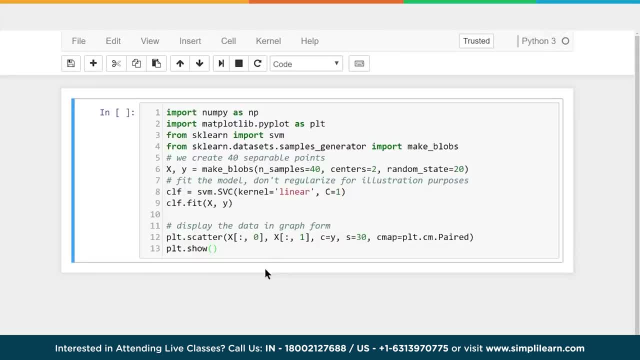 So, when you see data like this, it's necessary to move away from a 1D view of the data to a two-dimensional view of the data. So, when you see data like this, it's necessary to move away from a 1D view of the data to a two-dimensional view of the data. 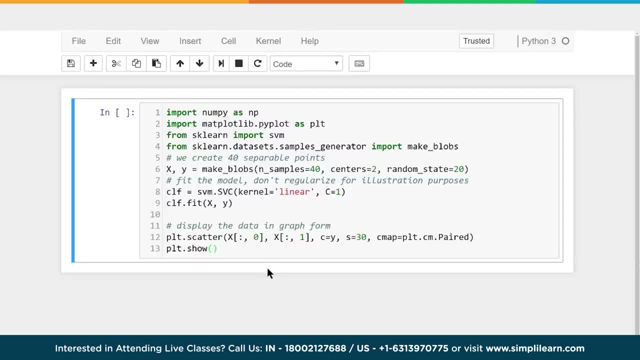 So, when you see data like this, it's necessary to move away from a 1D view of the data to a two-dimensional view of the data. So, when you see data like this, it's necessary to move away from a 1D view of the data to a two-dimensional view of the data. 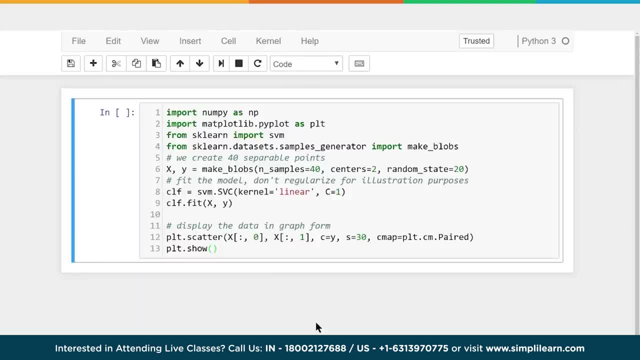 So, when you see data like this, it's necessary to move away from a 1D view of the data to a two-dimensional view of the data. So, when you see data like this, it's necessary to move away from a 1D view of the data to a two-dimensional view of the data. 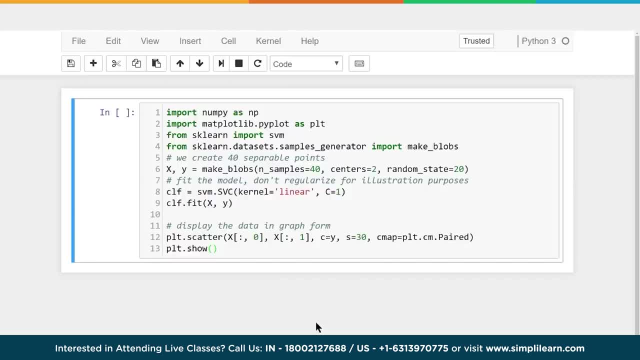 So, when you see data like this, it's necessary to move away from a 1D view of the data to a two-dimensional view of the data. So, when you see data like this, it's necessary to move away from a 1D view of the data to a two-dimensional view of the data. 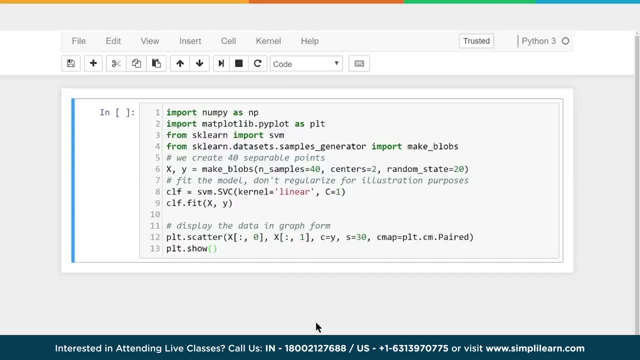 So, when you see data like this, it's necessary to move away from a 1D view of the data to a two-dimensional view of the data. So, when you see data like this, it's necessary to move away from a 1D view of the data to a two-dimensional view of the data. 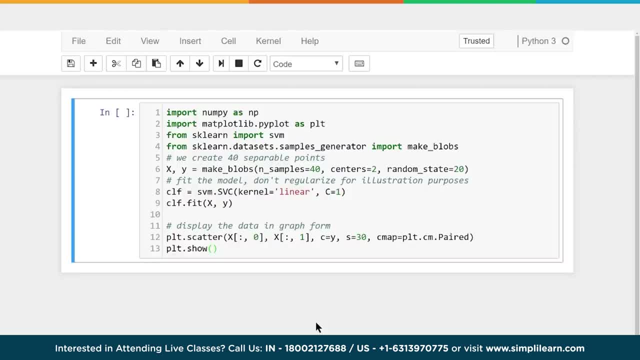 So, when you see data like this, it's necessary to move away from a 1D view of the data to a two-dimensional view of the data. So, when you see data like this, it's necessary to move away from a 1D view of the data to a two-dimensional view of the data. 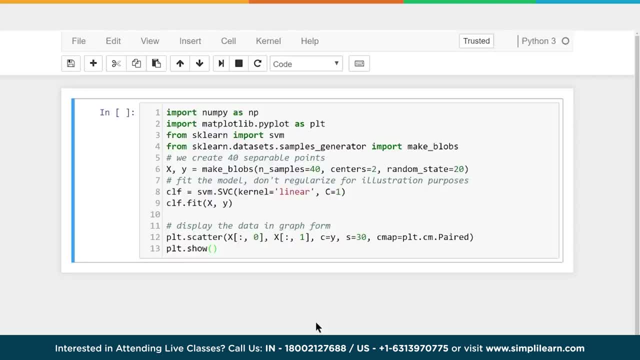 So, when you see data like this, it's necessary to move away from a 1D view of the data to a two-dimensional view of the data. So, when you see data like this, it's necessary to move away from a 1D view of the data to a two-dimensional view of the data. 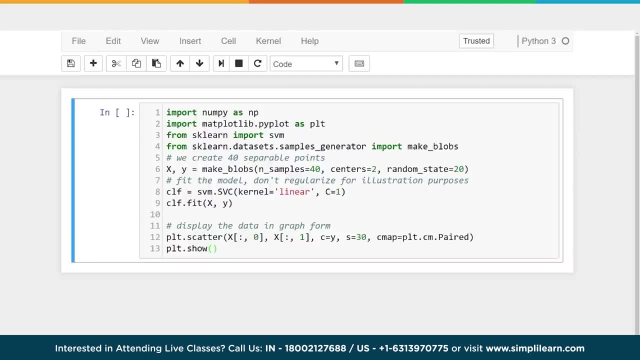 So, when you see data like this, it's necessary to move away from a 1D view of the data to a two-dimensional view of the data. So, when you see data like this, it's necessary to move away from a 1D view of the data to a two-dimensional view of the data. 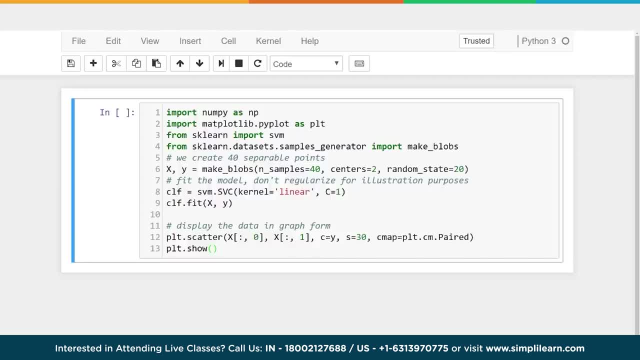 So, when you see data like this, it's necessary to move away from a 1D view of the data to a two-dimensional view of the data. So, when you see data like this, it's necessary to move away from a 1D view of the data to a two-dimensional view of the data. 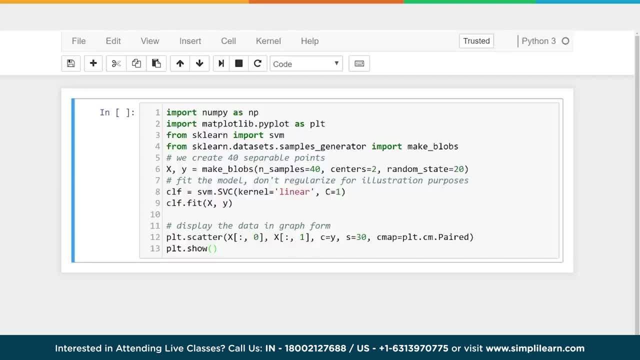 So, when you see data like this, it's necessary to move away from a 1D view of the data to a two-dimensional view of the data. So, when you see data like this, it's necessary to move away from a 1D view of the data to a two-dimensional view of the data. 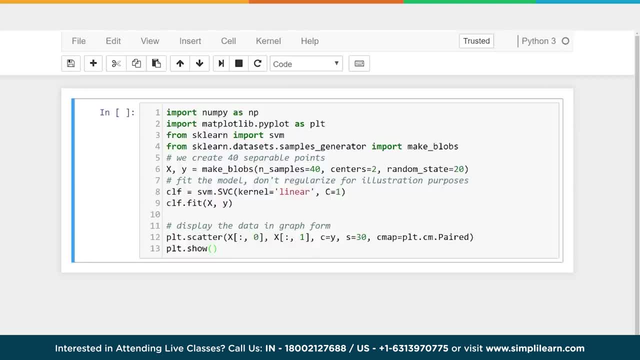 So, when you see data like this, it's necessary to move away from a 1D view of the data to a two-dimensional view of the data. So, when you see data like this, it's necessary to move away from a 1D view of the data to a two-dimensional view of the data. 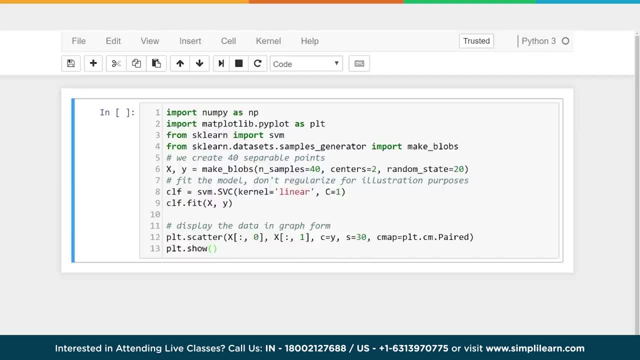 So, when you see data like this, it's necessary to move away from a 1D view of the data to a two-dimensional view of the data. So, when you see data like this, it's necessary to move away from a 1D view of the data to a two-dimensional view of the data. 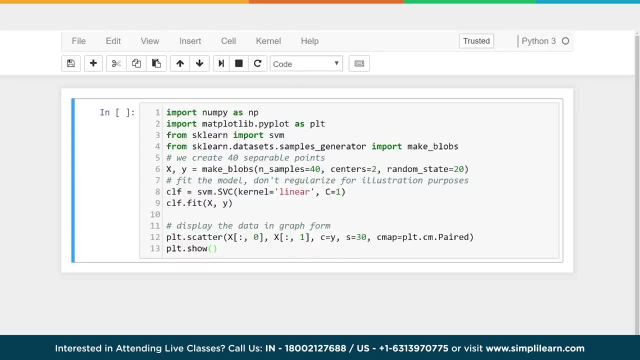 So, when you see data like this, it's necessary to move away from a 1D view of the data to a two-dimensional view of the data. So, when you see data like this, it's necessary to move away from a 1D view of the data to a two-dimensional view of the data. 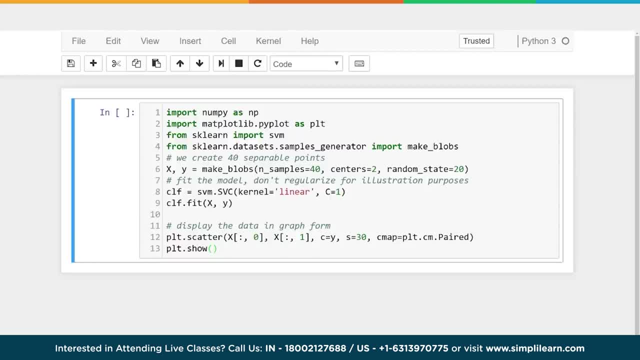 So, when you see data like this, it's necessary to move away from a 1D view of the data to a two-dimensional view of the data. So, when you see data like this, it's necessary to move away from a 1D view of the data to a two-dimensional view of the data. 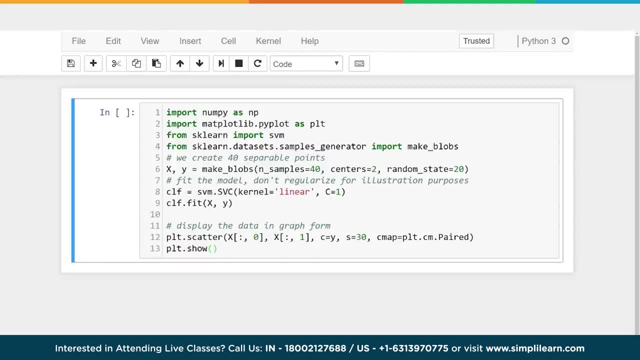 So, when you see data like this, it's necessary to move away from a 1D view of the data to a two-dimensional view of the data. So, when you see data like this, it's necessary to move away from a 1D view of the data to a two-dimensional view of the data. 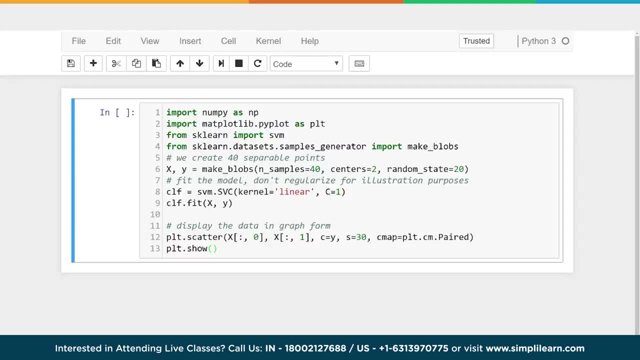 So, when you see data like this, it's necessary to move away from a 1D view of the data to a two-dimensional view of the data. So, when you see data like this, it's necessary to move away from a 1D view of the data to a two-dimensional view of the data. 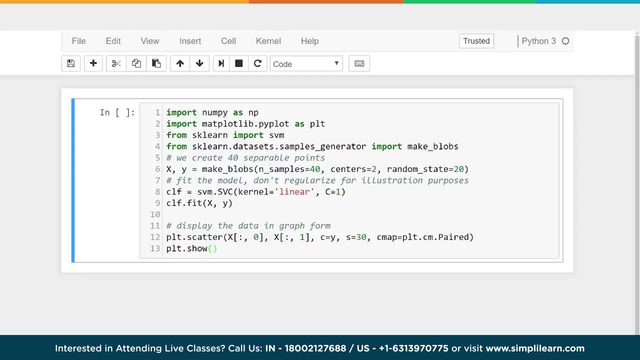 So, when you see data like this, it's necessary to move away from a 1D view of the data to a two-dimensional view of the data. So, when you see data like this, it's necessary to move away from a 1D view of the data to a two-dimensional view of the data. 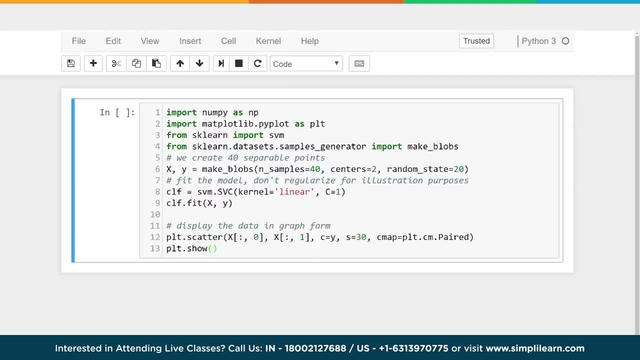 So, when you see data like this, it's necessary to move away from a 1D view of the data to a two-dimensional view of the data. So, when you see data like this, it's necessary to move away from a 1D view of the data to a two-dimensional view of the data. 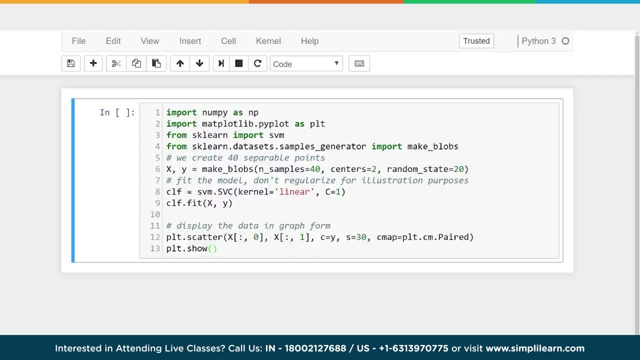 So, when you see data like this, it's necessary to move away from a 1D view of the data to a two-dimensional view of the data. So, when you see data like this, it's necessary to move away from a 1D view of the data to a two-dimensional view of the data. 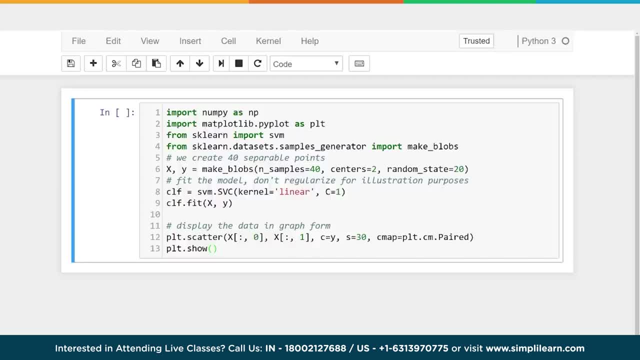 So, when you see data like this, it's necessary to move away from a 1D view of the data to a two-dimensional view of the data. So, when you see data like this, it's necessary to move away from a 1D view of the data to a two-dimensional view of the data. 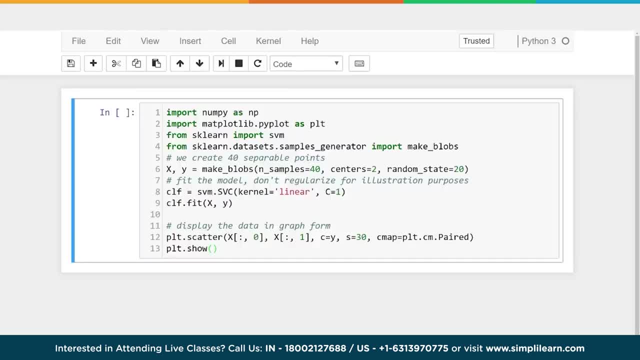 So, when you see data like this, it's necessary to move away from a 1D view of the data to a two-dimensional view of the data. So, when you see data like this, it's necessary to move away from a 1D view of the data to a two-dimensional view of the data. 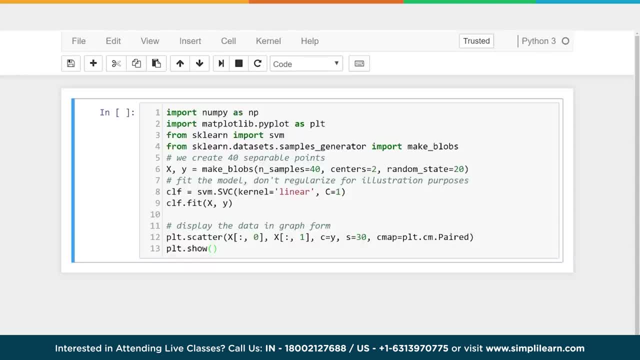 So, when you see data like this, it's necessary to move away from a 1D view of the data to a two-dimensional view of the data. So, when you see data like this, it's necessary to move away from a 1D view of the data to a two-dimensional view of the data. 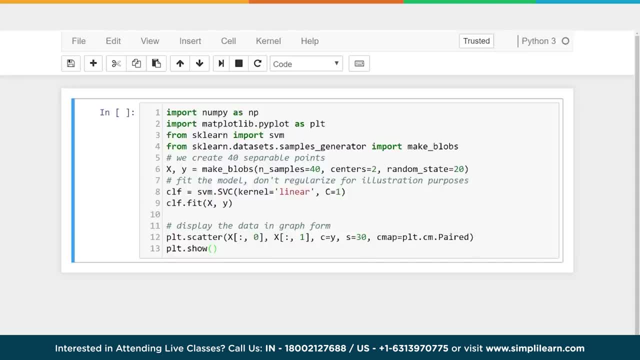 So, when you see data like this, it's necessary to move away from a 1D view of the data to a two-dimensional view of the data. So, when you see data like this, it's necessary to move away from a 1D view of the data to a two-dimensional view of the data. 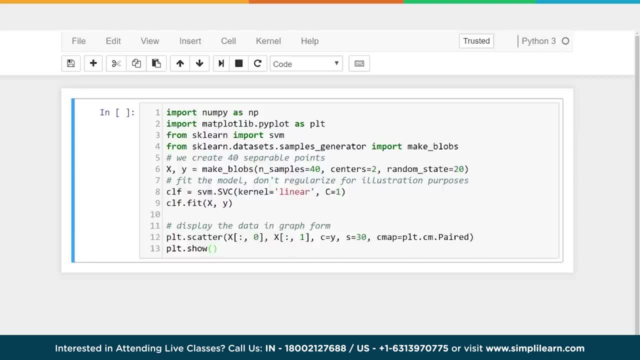 So, when you see data like this, it's necessary to move away from a 1D view of the data to a two-dimensional view of the data. So, when you see data like this, it's necessary to move away from a 1D view of the data to a two-dimensional view of the data. 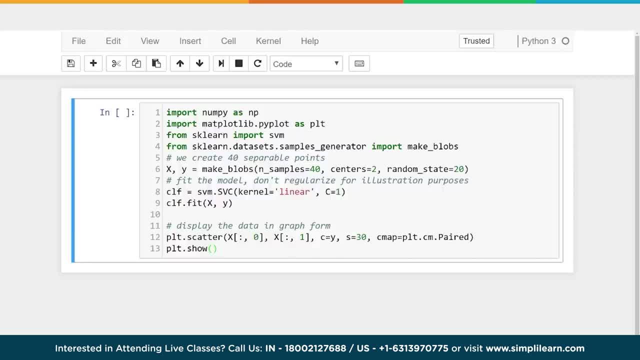 So, when you see data like this, it's necessary to move away from a 1D view of the data to a two-dimensional view of the data. So, when you see data like this, it's necessary to move away from a 1D view of the data to a two-dimensional view of the data. 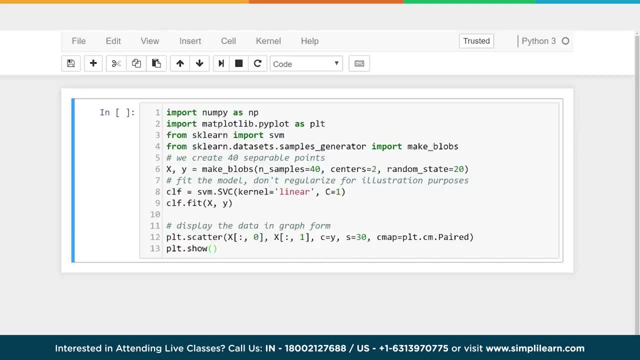 So, when you see data like this, it's necessary to move away from a 1D view of the data to a two-dimensional view of the data. So, when you see data like this, it's necessary to move away from a 1D view of the data to a two-dimensional view of the data. 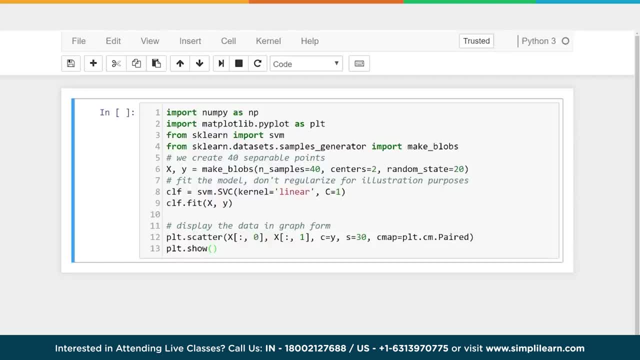 So, when you see data like this, it's necessary to move away from a 1D view of the data to a two-dimensional view of the data. So, when you see data like this, it's necessary to move away from a 1D view of the data to a two-dimensional view of the data. 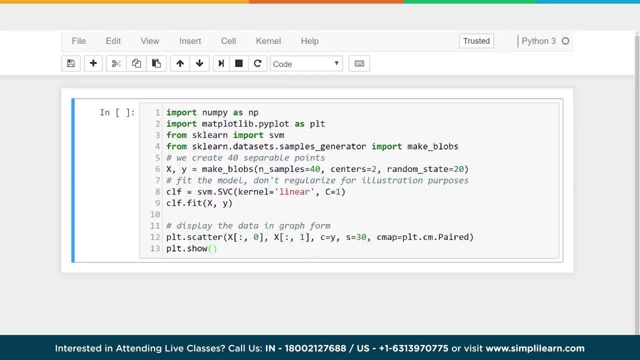 So, when you see data like this, it's necessary to move away from a 1D view of the data to a two-dimensional view of the data. So, when you see data like this, it's necessary to move away from a 1D view of the data to a two-dimensional view of the data. 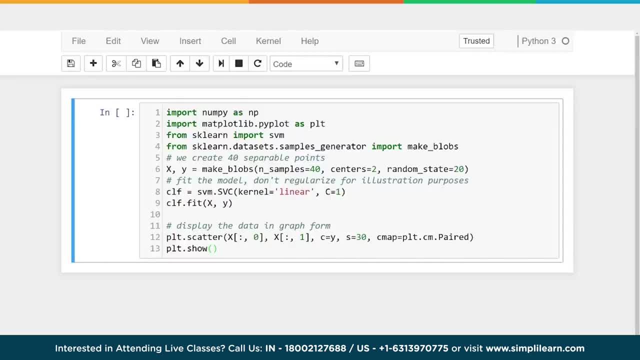 So, when you see data like this, it's necessary to move away from a 1D view of the data to a two-dimensional view of the data. So, when you see data like this, it's necessary to move away from a 1D view of the data to a two-dimensional view of the data. 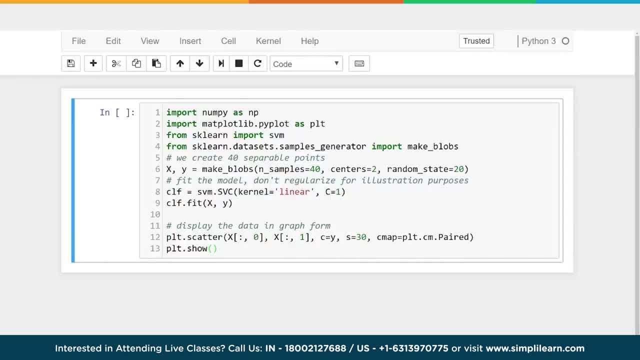 So, when you see data like this, it's necessary to move away from a 1D view of the data to a two-dimensional view of the data. So, when you see data like this, it's necessary to move away from a 1D view of the data to a two-dimensional view of the data. 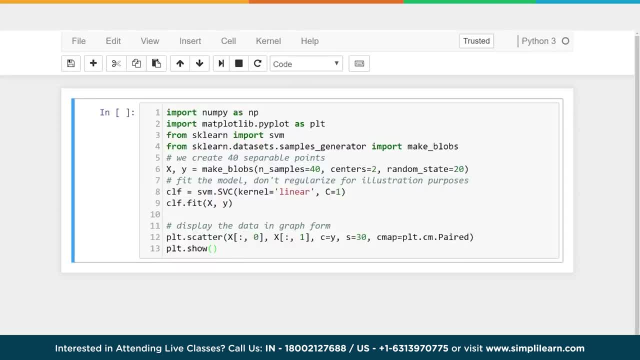 So, when you see data like this, it's necessary to move away from a 1D view of the data to a two-dimensional view of the data. So, when you see data like this, it's necessary to move away from a 1D view of the data to a two-dimensional view of the data. 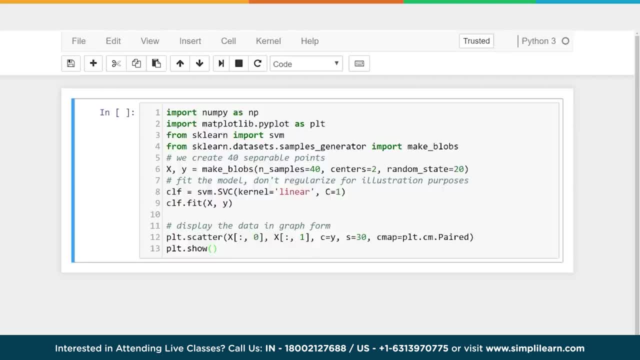 So, when you see data like this, it's necessary to move away from a 1D view of the data to a two-dimensional view of the data. So, when you see data like this, it's necessary to move away from a 1D view of the data to a two-dimensional view of the data. 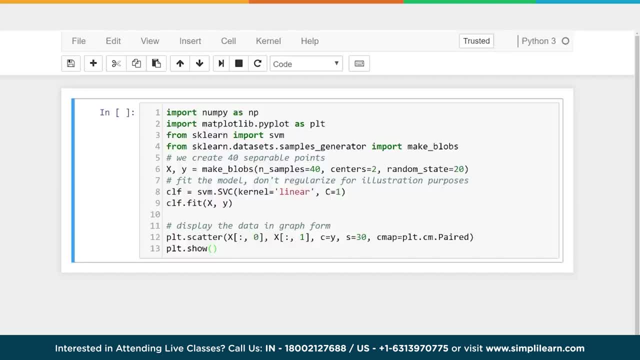 So, when you see data like this, it's necessary to move away from a 1D view of the data to a two-dimensional view of the data. So, when you see data like this, it's necessary to move away from a 1D view of the data to a two-dimensional view of the data. 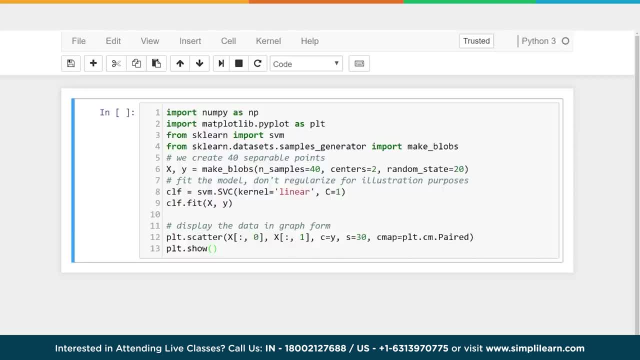 So, when you see data like this, it's necessary to move away from a 1D view of the data to a two-dimensional view of the data. So, when you see data like this, it's necessary to move away from a 1D view of the data to a two-dimensional view of the data. 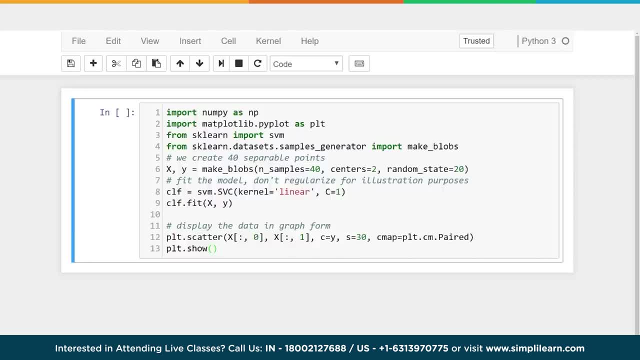 So, when you see data like this, it's necessary to move away from a 1D view of the data to a two-dimensional view of the data. So, when you see data like this, it's necessary to move away from a 1D view of the data to a two-dimensional view of the data. 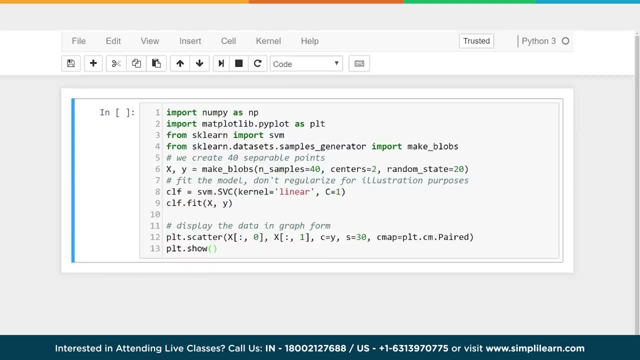 So, when you see data like this, it's necessary to move away from a 1D view of the data to a two-dimensional view of the data. So, when you see data like this, it's necessary to move away from a 1D view of the data to a two-dimensional view of the data. 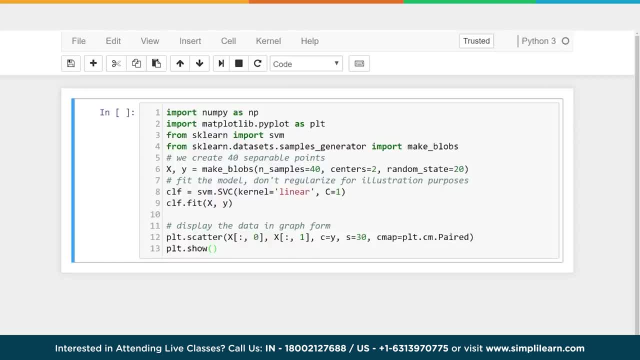 So, when you see data like this, it's necessary to move away from a 1D view of the data to a two-dimensional view of the data. So, when you see data like this, it's necessary to move away from a 1D view of the data to a two-dimensional view of the data. 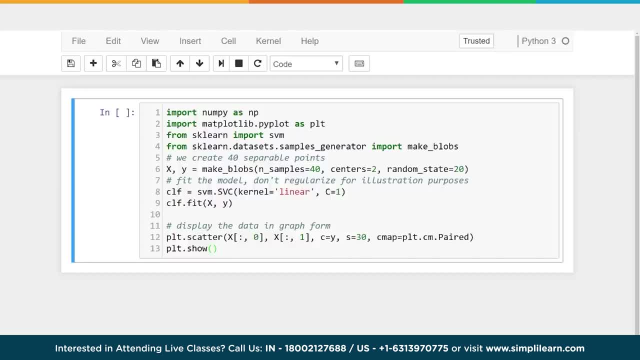 So, when you see data like this, it's necessary to move away from a 1D view of the data to a two-dimensional view of the data. So, when you see data like this, it's necessary to move away from a 1D view of the data to a two-dimensional view of the data. 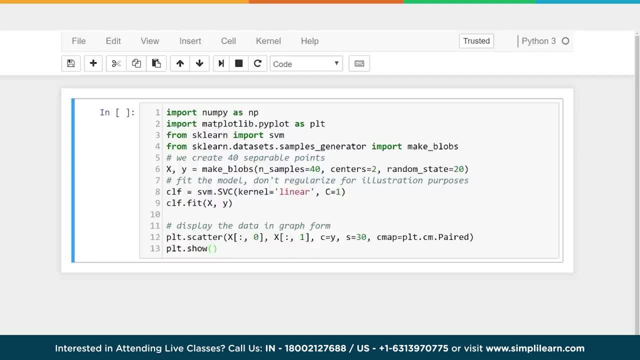 So, when you see data like this, it's necessary to move away from a 1D view of the data to a two-dimensional view of the data. So, when you see data like this, it's necessary to move away from a 1D view of the data to a two-dimensional view of the data. 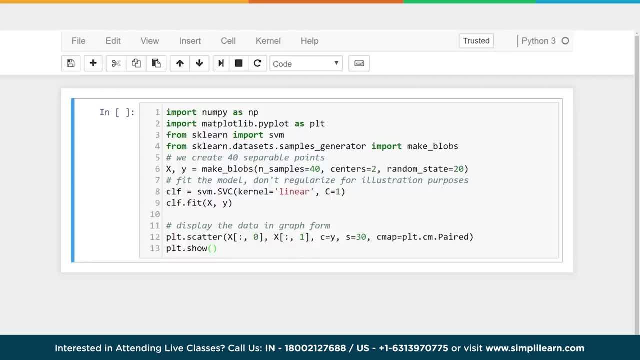 So, when you see data like this, it's necessary to move away from a 1D view of the data to a two-dimensional view of the data. So, when you see data like this, it's necessary to move away from a 1D view of the data to a two-dimensional view of the data. 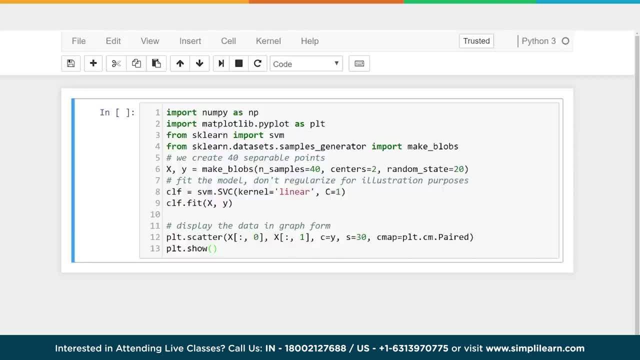 So, when you see data like this, it's necessary to move away from a 1D view of the data to a two-dimensional view of the data. So, when you see data like this, it's necessary to move away from a 1D view of the data to a two-dimensional view of the data. 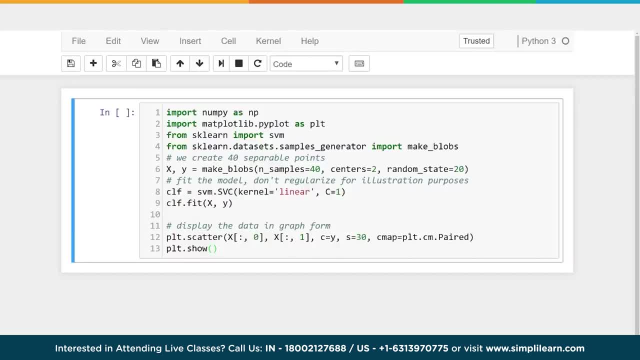 So, when you see data like this, it's necessary to move away from a 1D view of the data to a two-dimensional view of the data. So, when you see data like this, it's necessary to move away from a 1D view of the data to a two-dimensional view of the data. 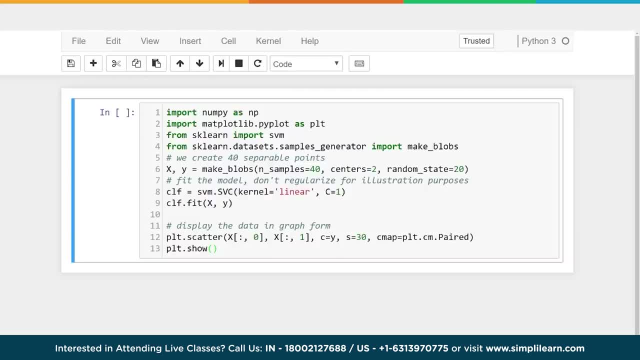 So, when you see data like this, it's necessary to move away from a 1D view of the data to a two-dimensional view of the data. So, when you see data like this, it's necessary to move away from a 1D view of the data to a two-dimensional view of the data. 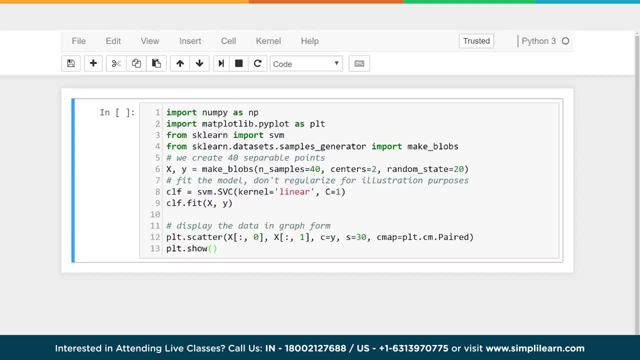 So, when you see data like this, it's necessary to move away from a 1D view of the data to a two-dimensional view of the data. So, when you see data like this, it's necessary to move away from a 1D view of the data to a two-dimensional view of the data. 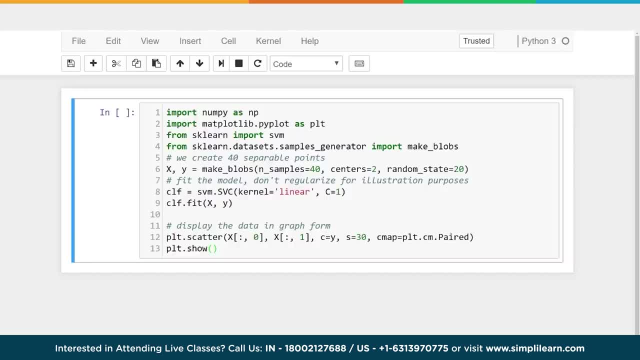 So, when you see data like this, it's necessary to move away from a 1D view of the data to a two-dimensional view of the data. So, when you see data like this, it's necessary to move away from a 1D view of the data to a two-dimensional view of the data. 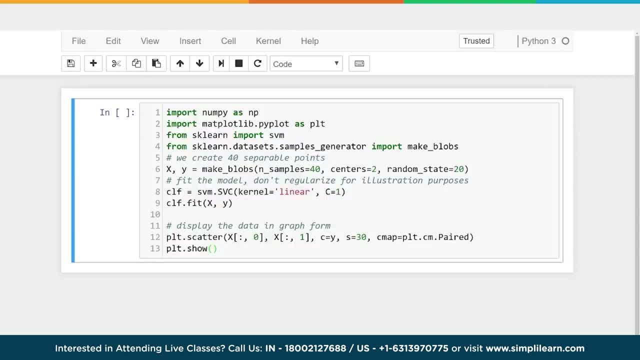 So, when you see data like this, it's necessary to move away from a 1D view of the data to a two-dimensional view of the data. So, when you see data like this, it's necessary to move away from a 1D view of the data to a two-dimensional view of the data. 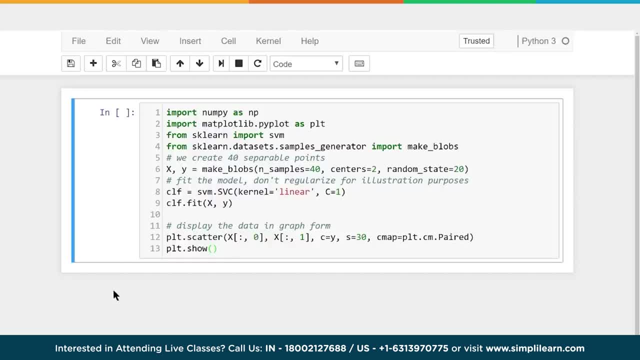 So, when you see data like this, it's necessary to move away from a 1D view of the data to a two-dimensional view of the data. So, when you see data like this, it's necessary to move away from a 1D view of the data to a two-dimensional view of the data. 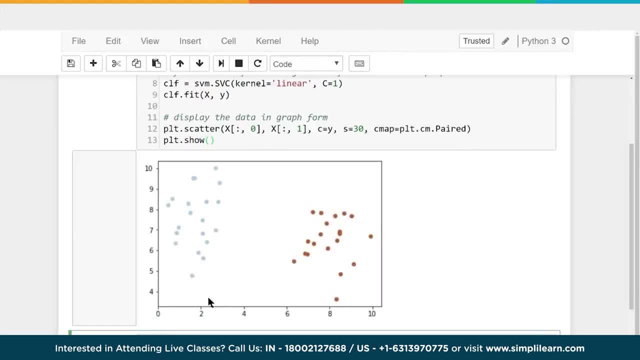 So, when you see data like this, it's necessary to move away from a 1D view of the data to a two-dimensional view of the data. So, when you see data like this, it's necessary to move away from a 1D view of the data to a two-dimensional view of the data. 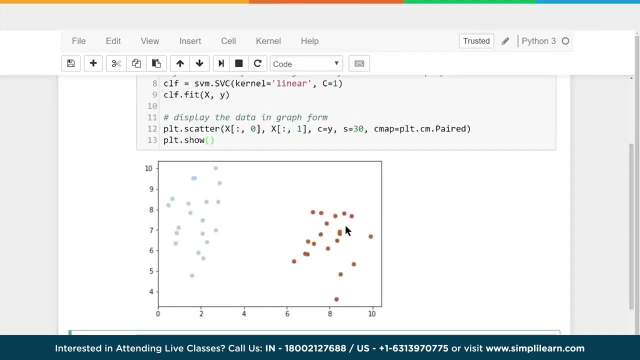 So, when you see data like this, it's necessary to move away from a 1D view of the data to a two-dimensional view of the data. So, when you see data like this, it's necessary to move away from a 1D view of the data to a two-dimensional view of the data. 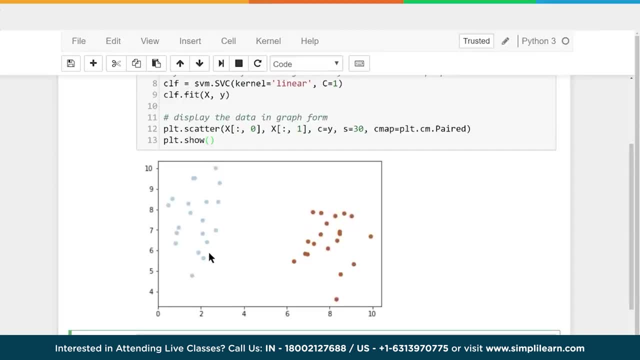 So, when you see data like this, it's necessary to move away from a 1D view of the data to a two-dimensional view of the data. So, when you see data like this, it's necessary to move away from a 1D view of the data to a two-dimensional view of the data. 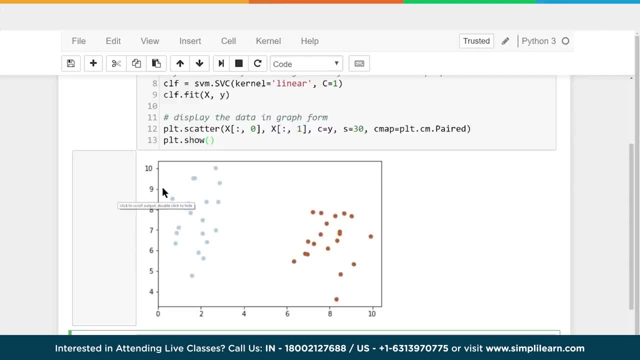 So, when you see data like this, it's necessary to move away from a 1D view of the data to a two-dimensional view of the data. So, when you see data like this, it's necessary to move away from a 1D view of the data to a two-dimensional view of the data. 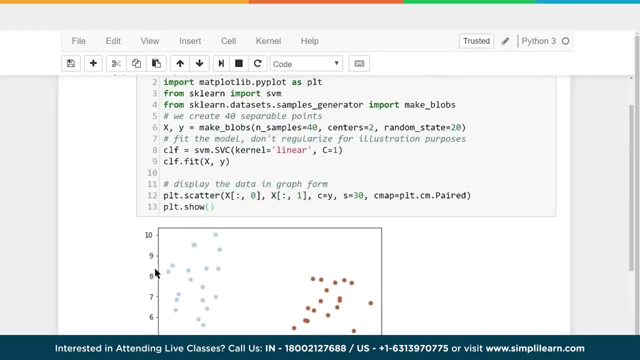 So, when you see data like this, it's necessary to move away from a 1D view of the data to a two-dimensional view of the data. So, when you see data like this, it's necessary to move away from a 1D view of the data to a two-dimensional view of the data. 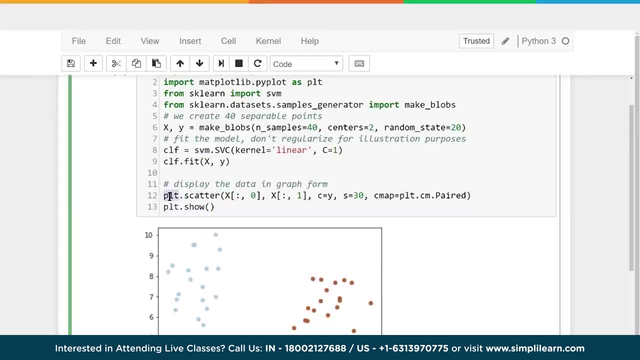 So, when you see data like this, it's necessary to move away from a 1D view of the data to a two-dimensional view of the data. So, when you see data like this, it's necessary to move away from a 1D view of the data to a two-dimensional view of the data. 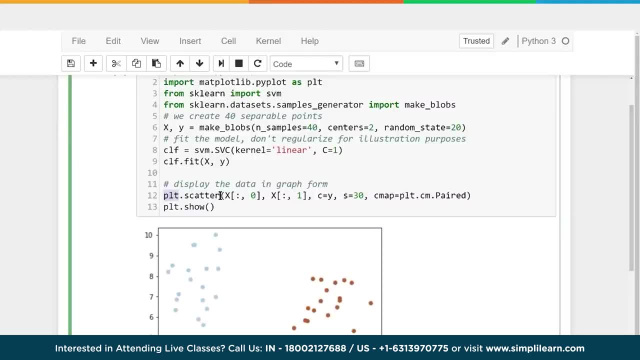 So, when you see data like this, it's necessary to move away from a 1D view of the data to a two-dimensional view of the data. So, when you see data like this, it's necessary to move away from a 1D view of the data to a two-dimensional view of the data. 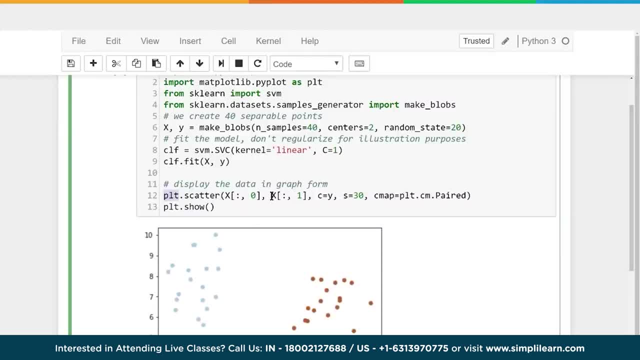 So, when you see data like this, it's necessary to move away from a 1D view of the data to a two-dimensional view of the data. So, when you see data like this, it's necessary to move away from a 1D view of the data to a two-dimensional view of the data. 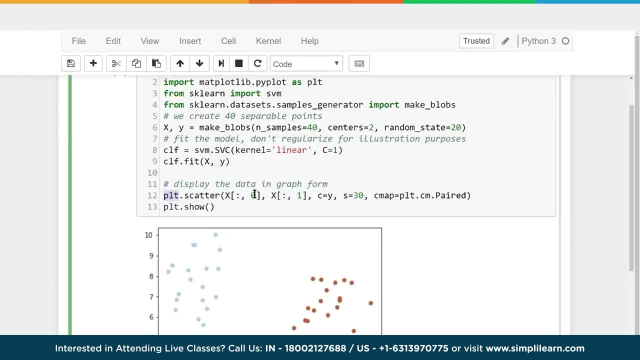 So, when you see data like this, it's necessary to move away from a 1D view of the data to a two-dimensional view of the data. So, when you see data like this, it's necessary to move away from a 1D view of the data to a two-dimensional view of the data. 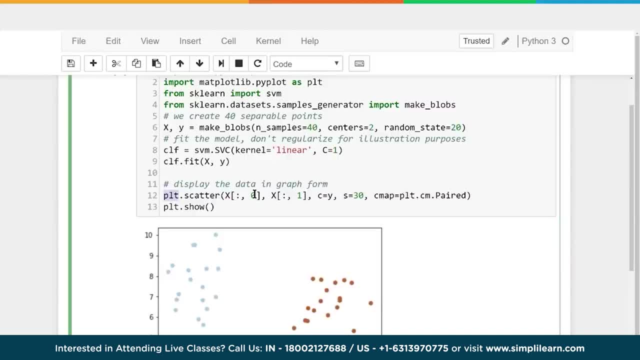 So, when you see data like this, it's necessary to move away from a 1D view of the data to a two-dimensional view of the data. So, when you see data like this, it's necessary to move away from a 1D view of the data to a two-dimensional view of the data. 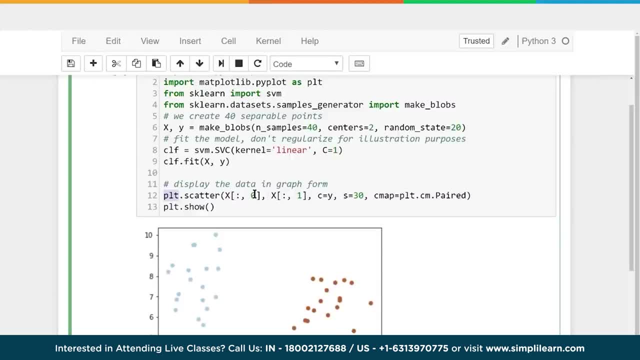 So, when you see data like this, it's necessary to move away from a 1D view of the data to a two-dimensional view of the data. So, when you see data like this, it's necessary to move away from a 1D view of the data to a two-dimensional view of the data. 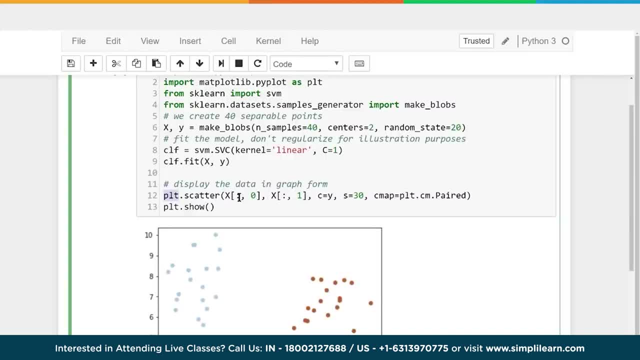 So, when you see data like this, it's necessary to move away from a 1D view of the data to a two-dimensional view of the data. So, when you see data like this, it's necessary to move away from a 1D view of the data to a two-dimensional view of the data. 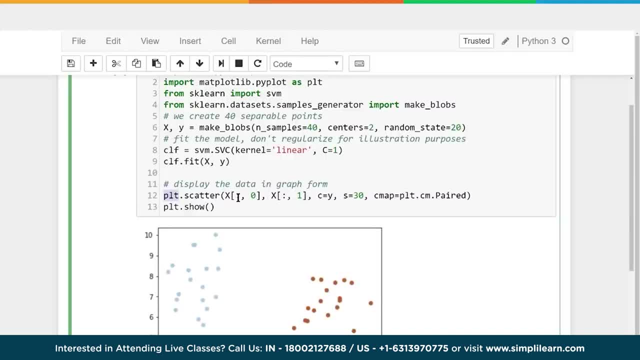 So, when you see data like this, it's necessary to move away from a 1D view of the data to a two-dimensional view of the data. So, when you see data like this, it's necessary to move away from a 1D view of the data to a two-dimensional view of the data. 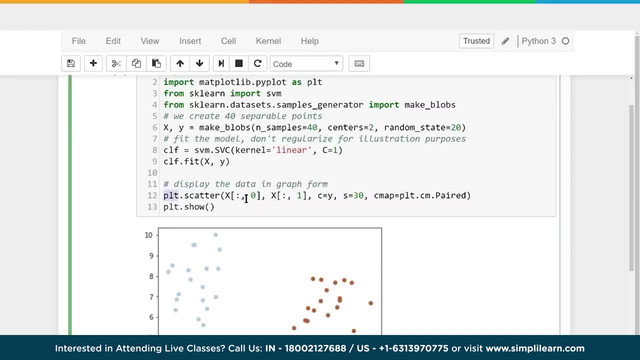 So, when you see data like this, it's necessary to move away from a 1D view of the data to a two-dimensional view of the data. So, when you see data like this, it's necessary to move away from a 1D view of the data to a two-dimensional view of the data. 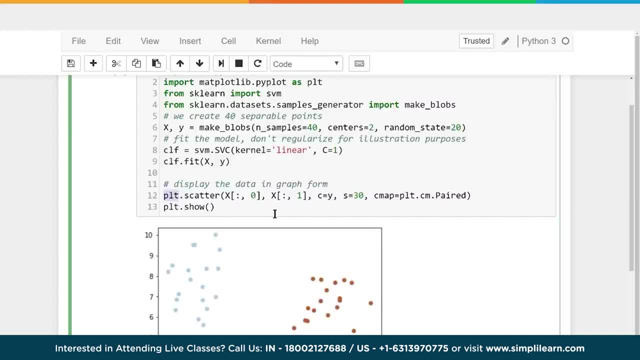 So, when you see data like this, it's necessary to move away from a 1D view of the data to a two-dimensional view of the data. So, when you see data like this, it's necessary to move away from a 1D view of the data to a two-dimensional view of the data. 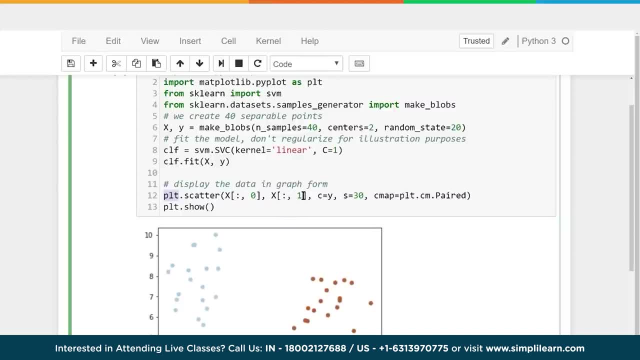 So, when you see data like this, it's necessary to move away from a 1D view of the data to a two-dimensional view of the data. So, when you see data like this, it's necessary to move away from a 1D view of the data to a two-dimensional view of the data. 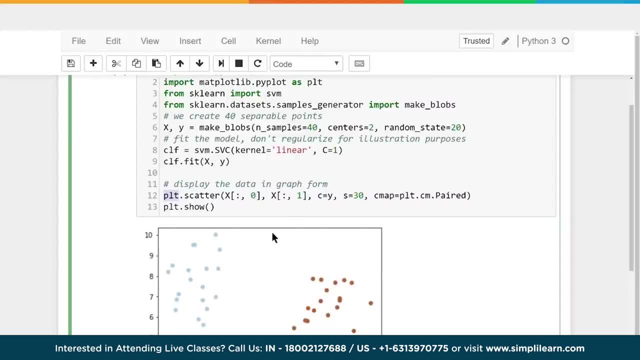 So, when you see data like this, it's necessary to move away from a 1D view of the data to a two-dimensional view of the data. So, when you see data like this, it's necessary to move away from a 1D view of the data to a two-dimensional view of the data. 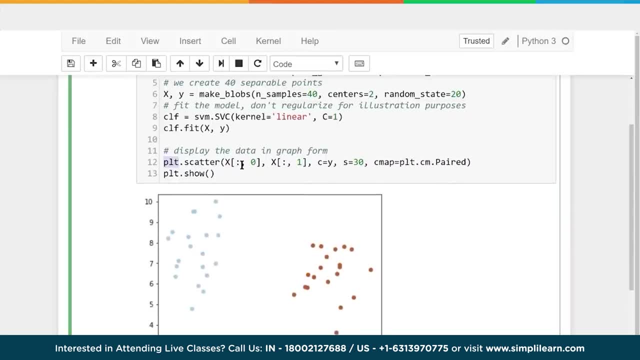 So, when you see data like this, it's necessary to move away from a 1D view of the data to a two-dimensional view of the data. So, when you see data like this, it's necessary to move away from a 1D view of the data to a two-dimensional view of the data. 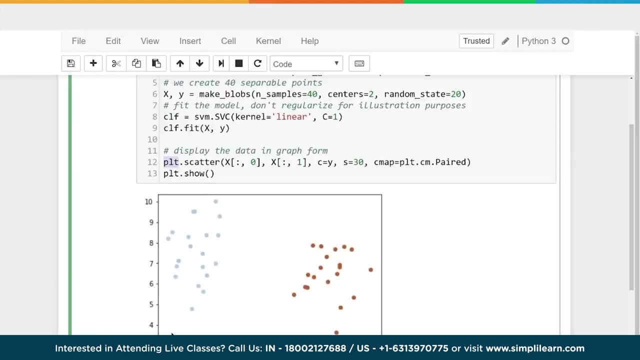 So, when you see data like this, it's necessary to move away from a 1D view of the data to a two-dimensional view of the data. So, when you see data like this, it's necessary to move away from a 1D view of the data to a two-dimensional view of the data. 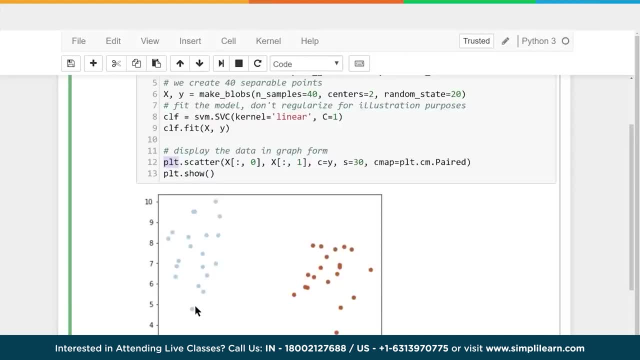 So, when you see data like this, it's necessary to move away from a 1D view of the data to a two-dimensional view of the data. So, when you see data like this, it's necessary to move away from a 1D view of the data to a two-dimensional view of the data. 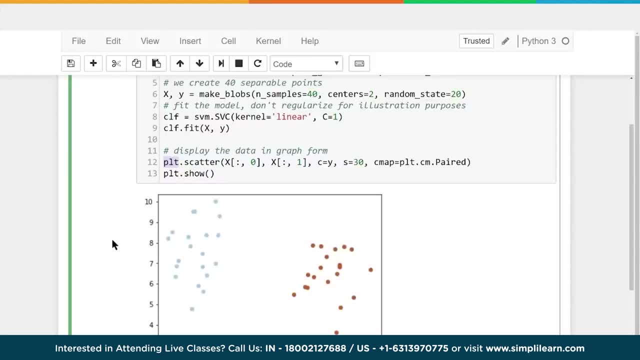 So, when you see data like this, it's necessary to move away from a 1D view of the data to a two-dimensional view of the data. So, when you see data like this, it's necessary to move away from a 1D view of the data to a two-dimensional view of the data. 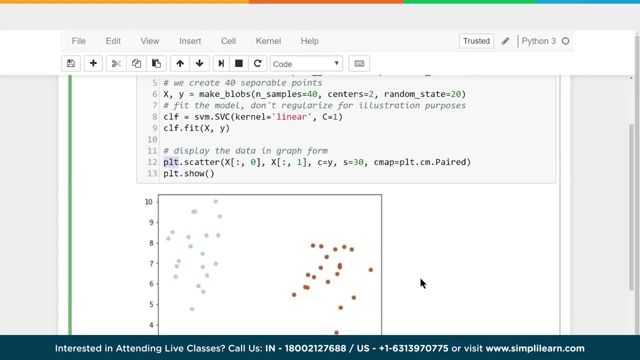 So, when you see data like this, it's necessary to move away from a 1D view of the data to a two-dimensional view of the data. So, when you see data like this, it's necessary to move away from a 1D view of the data to a two-dimensional view of the data. 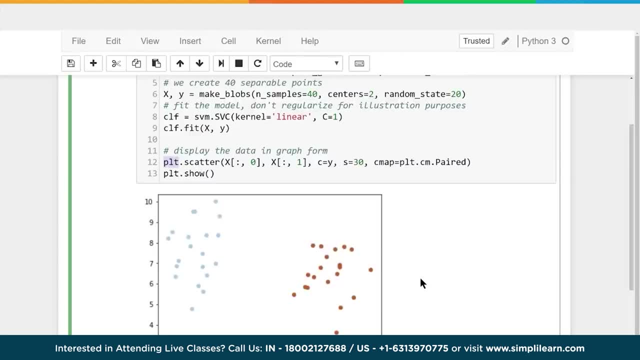 So, when you see data like this, it's necessary to move away from a 1D view of the data to a two-dimensional view of the data. So, when you see data like this, it's necessary to move away from a 1D view of the data to a two-dimensional view of the data. 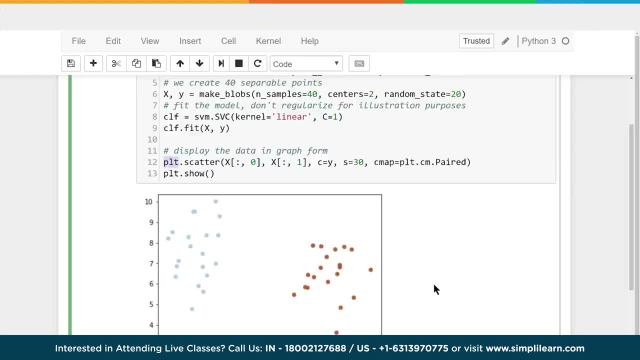 So, when you see data like this, it's necessary to move away from a 1D view of the data to a two-dimensional view of the data. So, when you see data like this, it's necessary to move away from a 1D view of the data to a two-dimensional view of the data. 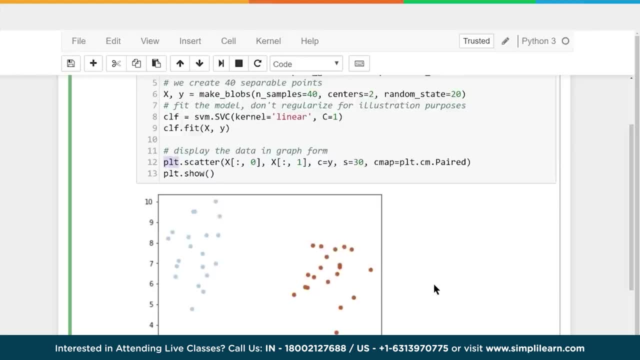 So, when you see data like this, it's necessary to move away from a 1D view of the data to a two-dimensional view of the data. So, when you see data like this, it's necessary to move away from a 1D view of the data to a two-dimensional view of the data. 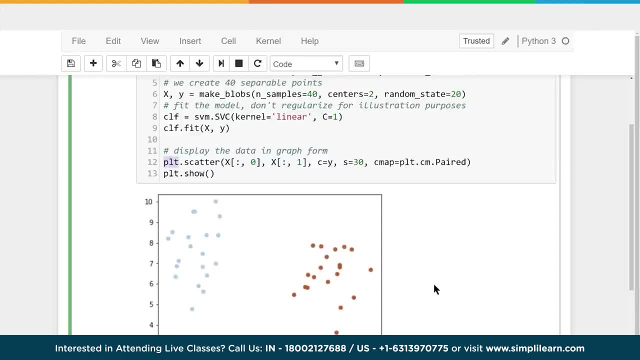 So, when you see data like this, it's necessary to move away from a 1D view of the data to a two-dimensional view of the data. So, when you see data like this, it's necessary to move away from a 1D view of the data to a two-dimensional view of the data. 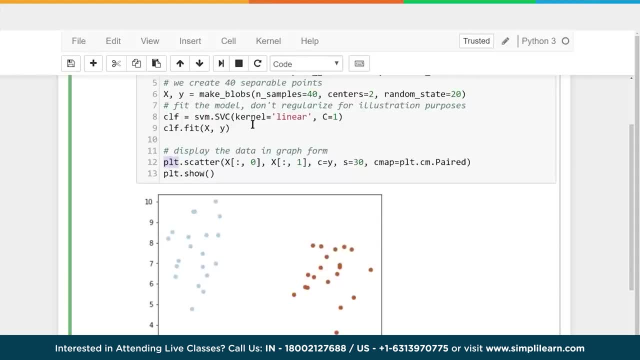 So, when you see data like this, it's necessary to move away from a 1D view of the data to a two-dimensional view of the data. So, when you see data like this, it's necessary to move away from a 1D view of the data to a two-dimensional view of the data. 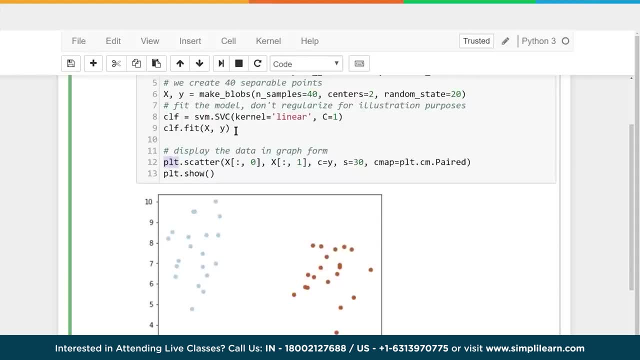 So, when you see data like this, it's necessary to move away from a 1D view of the data to a two-dimensional view of the data. So, when you see data like this, it's necessary to move away from a 1D view of the data to a two-dimensional view of the data. 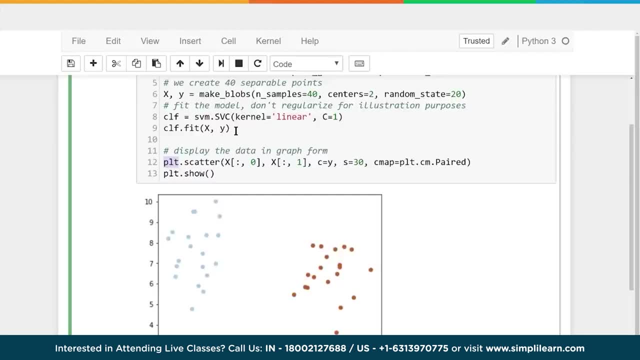 So, when you see data like this, it's necessary to move away from a 1D view of the data to a two-dimensional view of the data. So, when you see data like this, it's necessary to move away from a 1D view of the data to a two-dimensional view of the data. 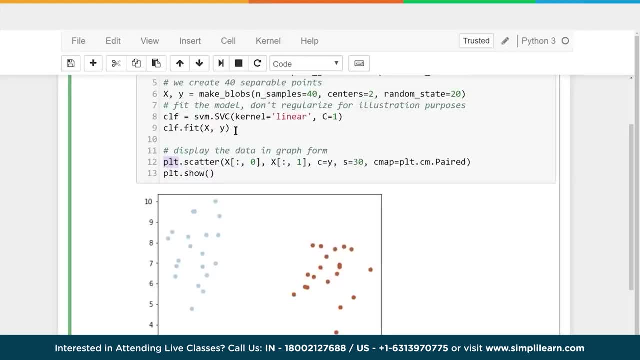 So, when you see data like this, it's necessary to move away from a 1D view of the data to a two-dimensional view of the data. So, when you see data like this, it's necessary to move away from a 1D view of the data to a two-dimensional view of the data. 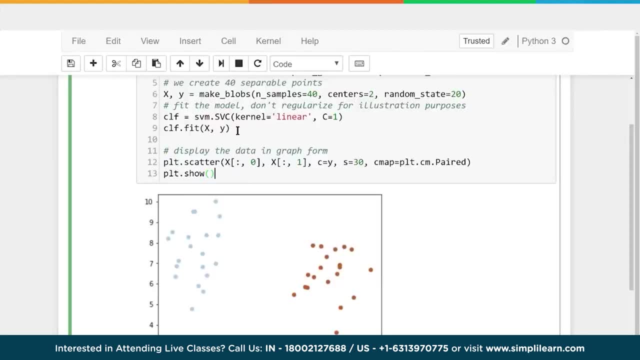 So, when you see data like this, it's necessary to move away from a 1D view of the data to a two-dimensional view of the data. So, when you see data like this, it's necessary to move away from a 1D view of the data to a two-dimensional view of the data. 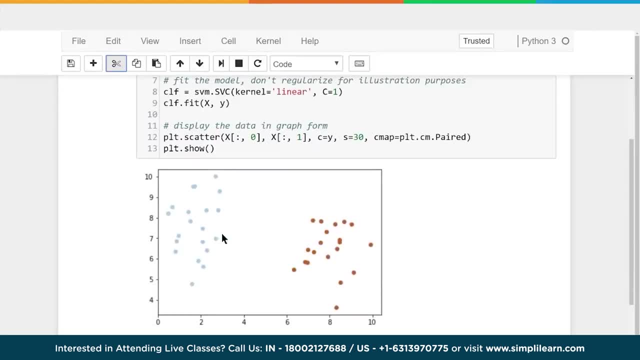 So, when you see data like this, it's necessary to move away from a 1D view of the data to a two-dimensional view of the data. So, when you see data like this, it's necessary to move away from a 1D view of the data to a two-dimensional view of the data. 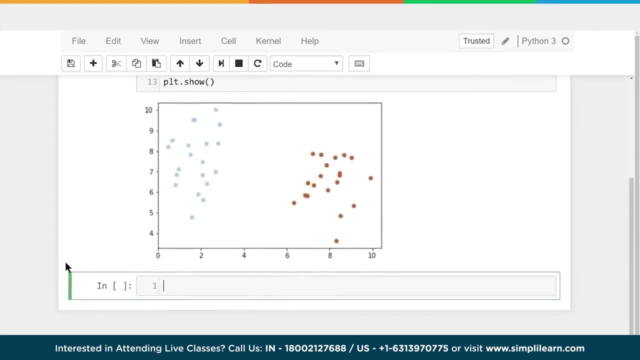 So, when you see data like this, it's necessary to move away from a 1D view of the data to a two-dimensional view of the data. So, when you see data like this, it's necessary to move away from a 1D view of the data to a two-dimensional view of the data. 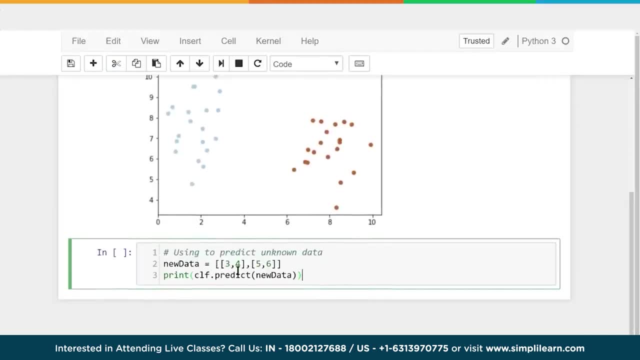 So, when you see data like this, it's necessary to move away from a 1D view of the data to a two-dimensional view of the data. So, when you see data like this, it's necessary to move away from a 1D view of the data to a two-dimensional view of the data. 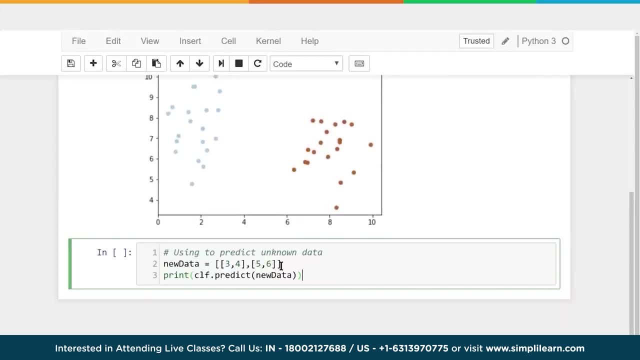 So, when you see data like this, it's necessary to move away from a 1D view of the data to a two-dimensional view of the data. So, when you see data like this, it's necessary to move away from a 1D view of the data to a two-dimensional view of the data. 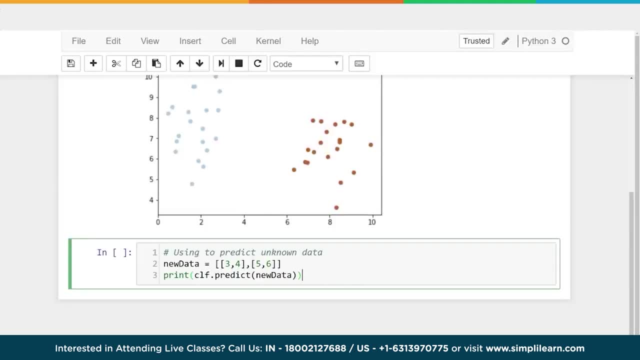 So, when you see data like this, it's necessary to move away from a 1D view of the data to a two-dimensional view of the data. So, when you see data like this, it's necessary to move away from a 1D view of the data to a two-dimensional view of the data. 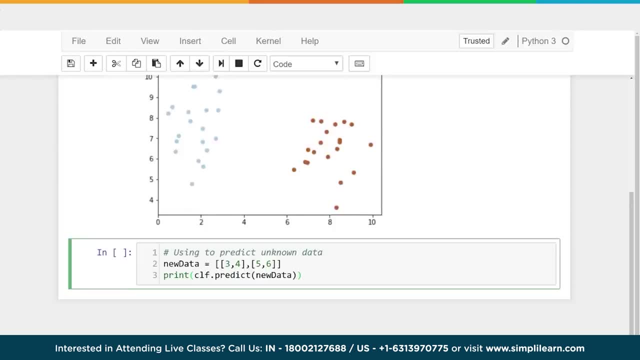 So, when you see data like this, it's necessary to move away from a 1D view of the data to a two-dimensional view of the data. So, when you see data like this, it's necessary to move away from a 1D view of the data to a two-dimensional view of the data. 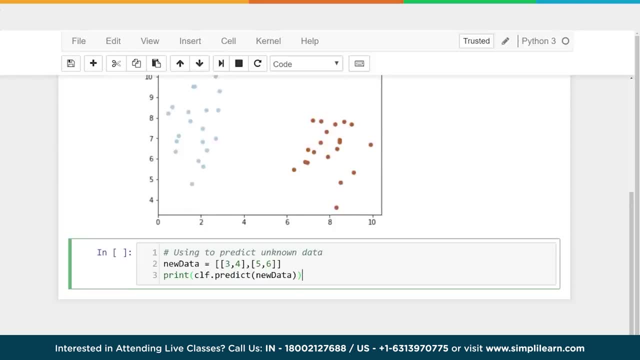 So, when you see data like this, it's necessary to move away from a 1D view of the data to a two-dimensional view of the data. So, when you see data like this, it's necessary to move away from a 1D view of the data to a two-dimensional view of the data. 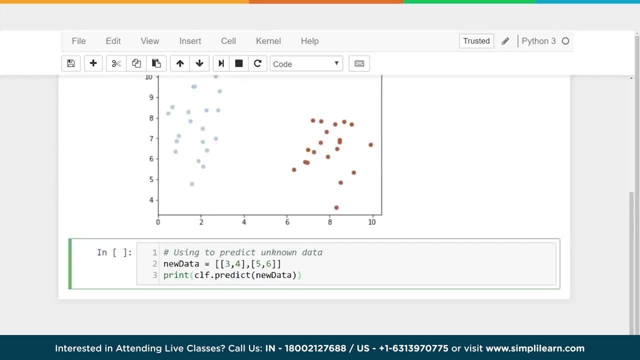 So, when you see data like this, it's necessary to move away from a 1D view of the data to a two-dimensional view of the data. So, when you see data like this, it's necessary to move away from a 1D view of the data to a two-dimensional view of the data. 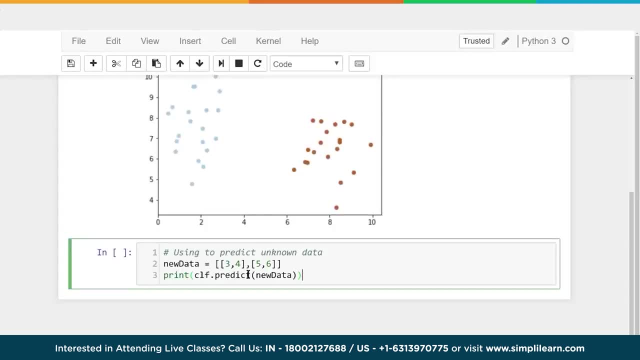 So, when you see data like this, it's necessary to move away from a 1D view of the data to a two-dimensional view of the data. So, when you see data like this, it's necessary to move away from a 1D view of the data to a two-dimensional view of the data. 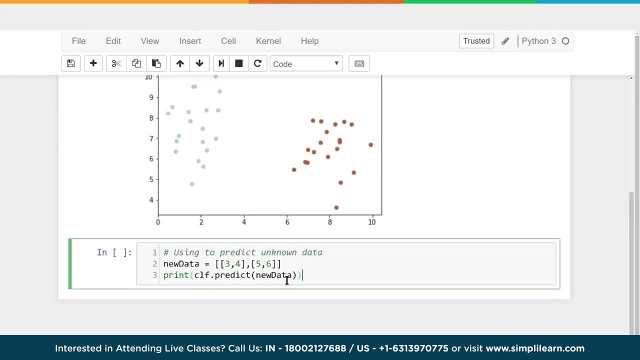 So, when you see data like this, it's necessary to move away from a 1D view of the data to a two-dimensional view of the data. So, when you see data like this, it's necessary to move away from a 1D view of the data to a two-dimensional view of the data. 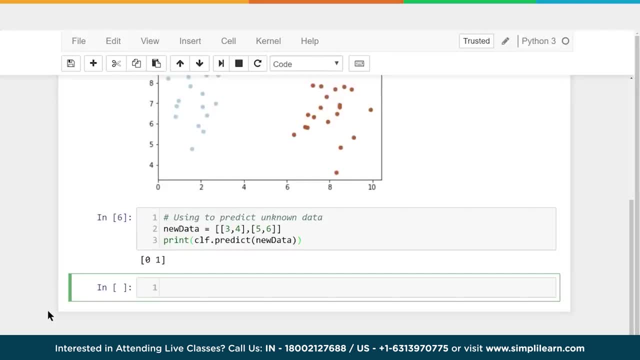 So, when you see data like this, it's necessary to move away from a 1D view of the data to a two-dimensional view of the data. So, when you see data like this, it's necessary to move away from a 1D view of the data to a two-dimensional view of the data. 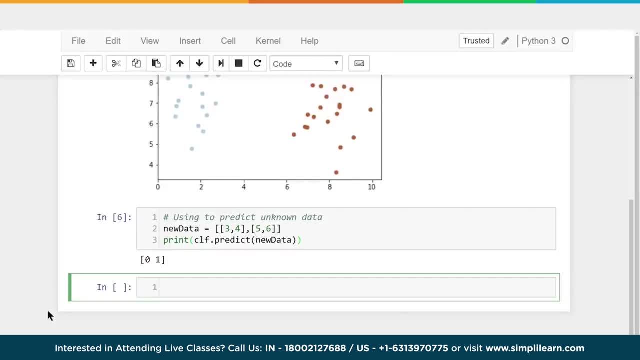 So, when you see data like this, it's necessary to move away from a 1D view of the data to a two-dimensional view of the data. So, when you see data like this, it's necessary to move away from a 1D view of the data to a two-dimensional view of the data. 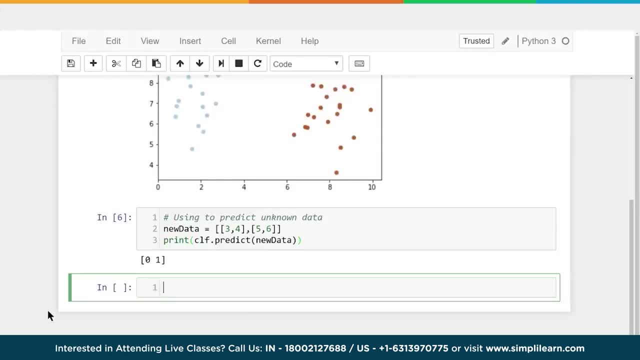 So, when you see data like this, it's necessary to move away from a 1D view of the data to a two-dimensional view of the data. So, when you see data like this, it's necessary to move away from a 1D view of the data to a two-dimensional view of the data. 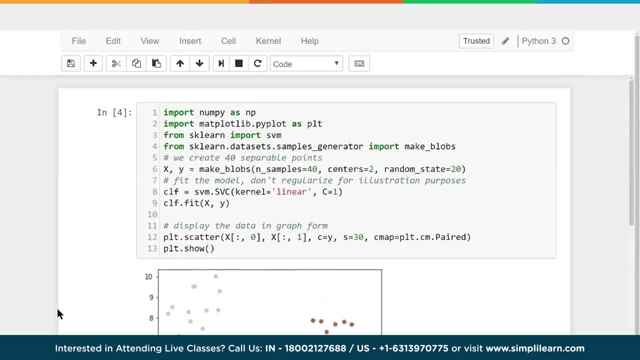 So, when you see data like this, it's necessary to move away from a 1D view of the data to a two-dimensional view of the data. So, when you see data like this, it's necessary to move away from a 1D view of the data to a two-dimensional view of the data. 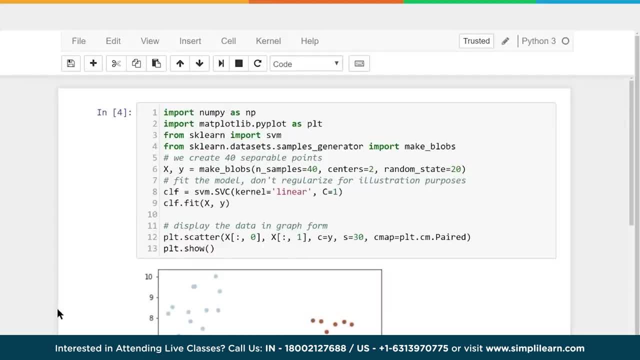 So, when you see data like this, it's necessary to move away from a 1D view of the data to a two-dimensional view of the data. So, when you see data like this, it's necessary to move away from a 1D view of the data to a two-dimensional view of the data. 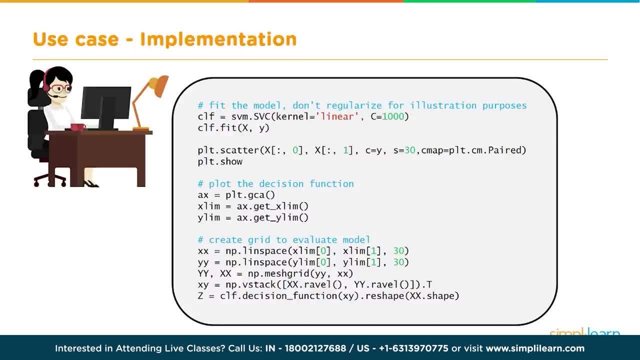 So, when you see data like this, it's necessary to move away from a 1D view of the data to a two-dimensional view of the data. So, when you see data like this, it's necessary to move away from a 1D view of the data to a two-dimensional view of the data. 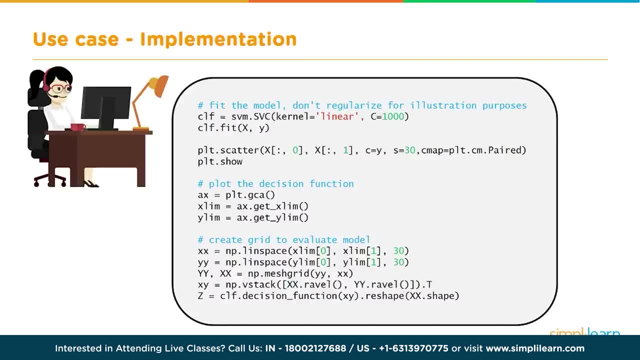 So, when you see data like this, it's necessary to move away from a 1D view of the data to a two-dimensional view of the data. So, when you see data like this, it's necessary to move away from a 1D view of the data to a two-dimensional view of the data. 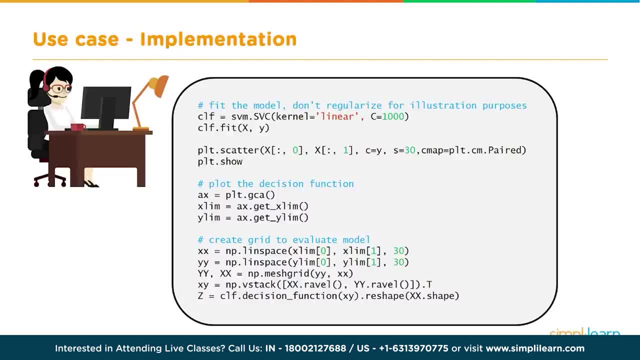 So, when you see data like this, it's necessary to move away from a 1D view of the data to a two-dimensional view of the data. So, when you see data like this, it's necessary to move away from a 1D view of the data to a two-dimensional view of the data. 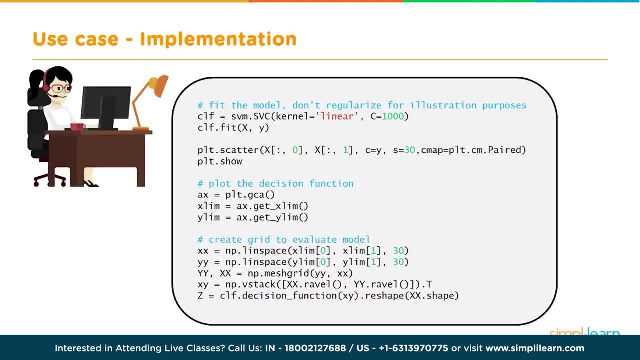 So, when you see data like this, it's necessary to move away from a 1D view of the data to a two-dimensional view of the data. So, when you see data like this, it's necessary to move away from a 1D view of the data to a two-dimensional view of the data. 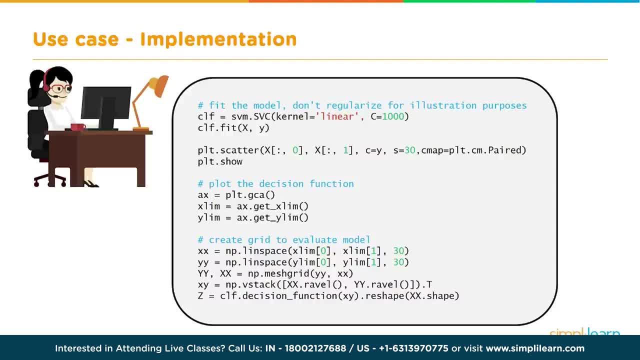 So, when you see data like this, it's necessary to move away from a 1D view of the data to a two-dimensional view of the data. So, when you see data like this, it's necessary to move away from a 1D view of the data to a two-dimensional view of the data. 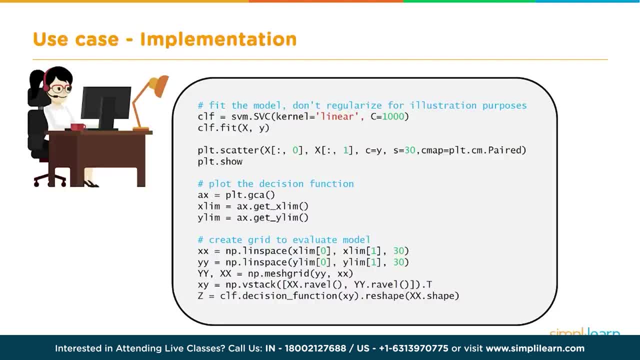 So, when you see data like this, it's necessary to move away from a 1D view of the data to a two-dimensional view of the data. So, when you see data like this, it's necessary to move away from a 1D view of the data to a two-dimensional view of the data. 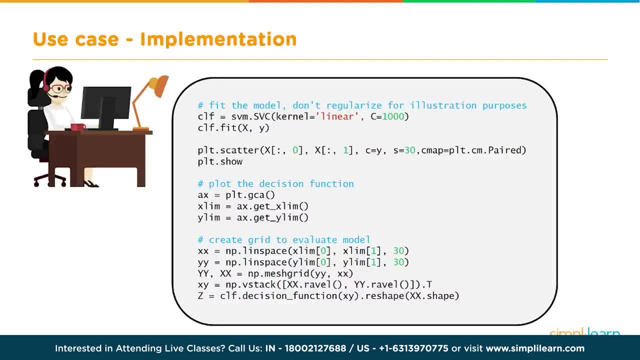 So, when you see data like this, it's necessary to move away from a 1D view of the data to a two-dimensional view of the data. So, when you see data like this, it's necessary to move away from a 1D view of the data to a two-dimensional view of the data. 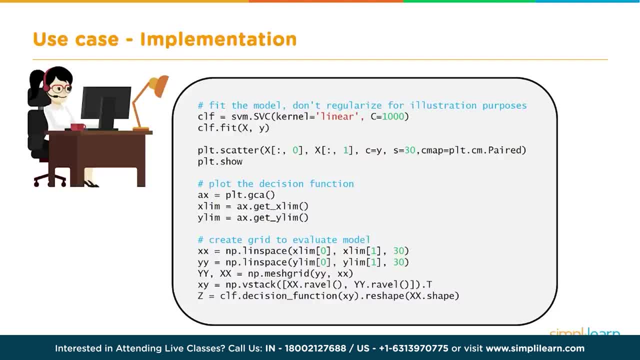 So, when you see data like this, it's necessary to move away from a 1D view of the data to a two-dimensional view of the data. So, when you see data like this, it's necessary to move away from a 1D view of the data to a two-dimensional view of the data. 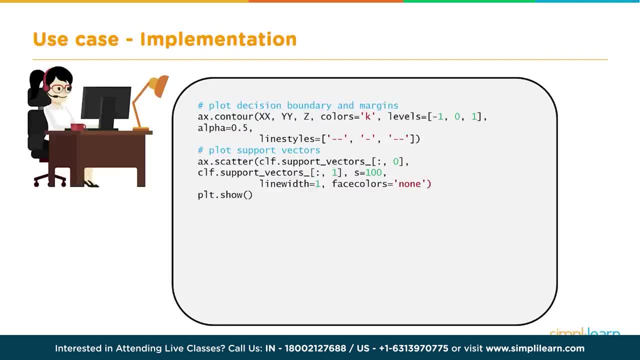 So, when you see data like this, it's necessary to move away from a 1D view of the data to a two-dimensional view of the data. So, when you see data like this, it's necessary to move away from a 1D view of the data to a two-dimensional view of the data. 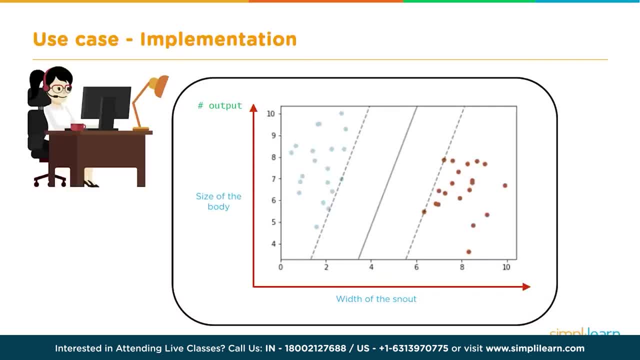 So, when you see data like this, it's necessary to move away from a 1D view of the data to a two-dimensional view of the data. So, when you see data like this, it's necessary to move away from a 1D view of the data to a two-dimensional view of the data. 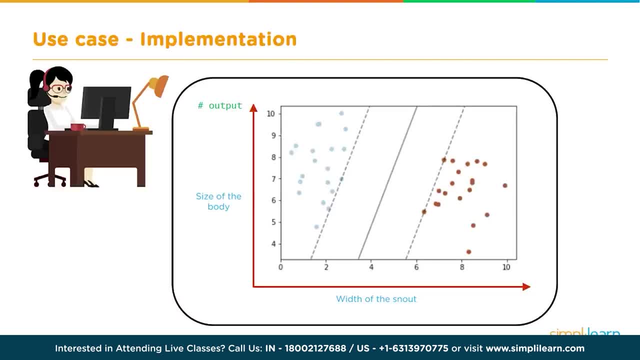 So, when you see data like this, it's necessary to move away from a 1D view of the data to a two-dimensional view of the data. So, when you see data like this, it's necessary to move away from a 1D view of the data to a two-dimensional view of the data. 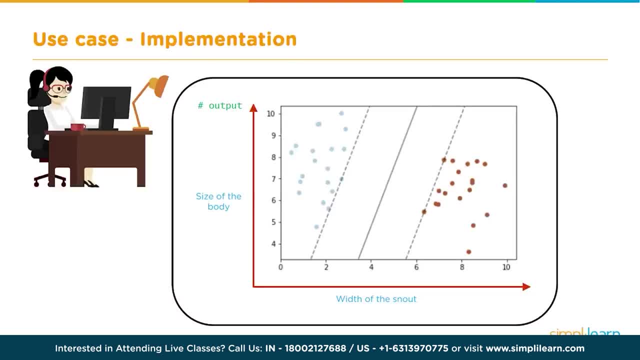 So, when you see data like this, it's necessary to move away from a 1D view of the data to a two-dimensional view of the data. So, when you see data like this, it's necessary to move away from a 1D view of the data to a two-dimensional view of the data. 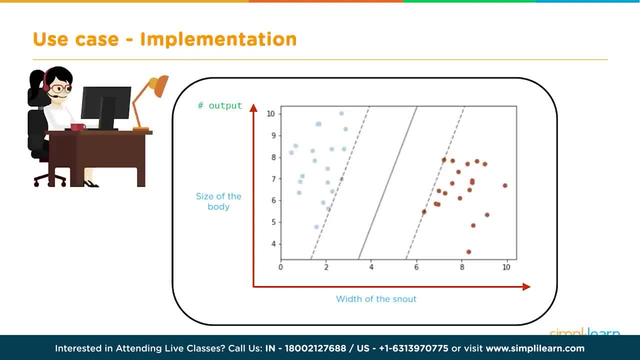 So, when you see data like this, it's necessary to move away from a 1D view of the data to a two-dimensional view of the data. So, when you see data like this, it's necessary to move away from a 1D view of the data to a two-dimensional view of the data. 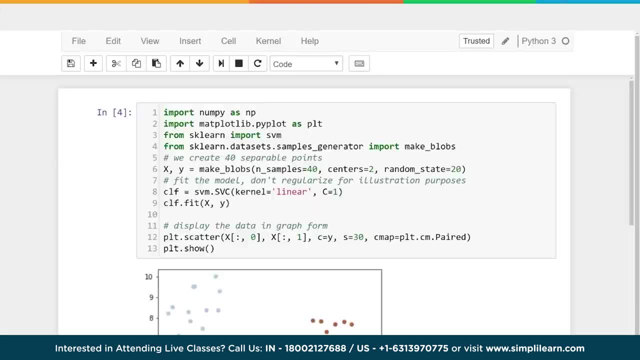 So, when you see data like this, it's necessary to move away from a 1D view of the data to a two-dimensional view of the data. So, when you see data like this, it's necessary to move away from a 1D view of the data to a two-dimensional view of the data. 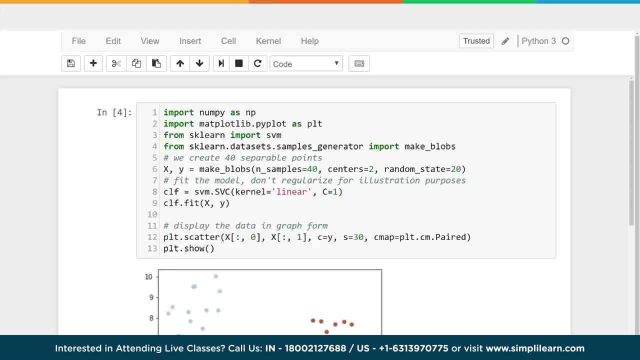 So, when you see data like this, it's necessary to move away from a 1D view of the data to a two-dimensional view of the data. So, when you see data like this, it's necessary to move away from a 1D view of the data to a two-dimensional view of the data. 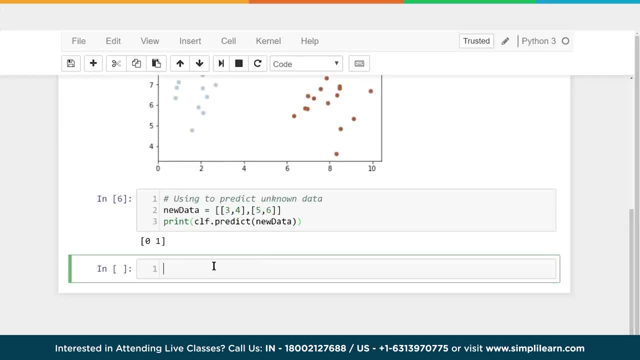 So, when you see data like this, it's necessary to move away from a 1D view of the data to a two-dimensional view of the data. So, when you see data like this, it's necessary to move away from a 1D view of the data to a two-dimensional view of the data. 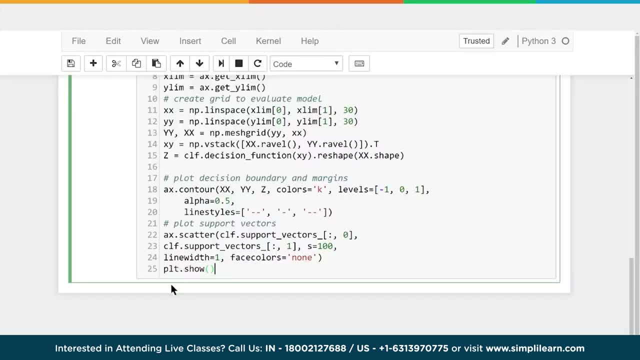 So, when you see data like this, it's necessary to move away from a 1D view of the data to a two-dimensional view of the data. So, when you see data like this, it's necessary to move away from a 1D view of the data to a two-dimensional view of the data. 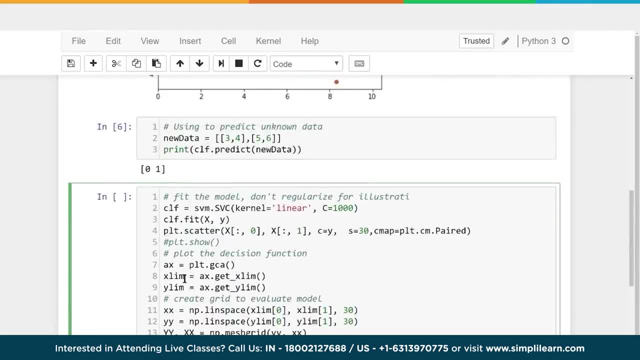 So, when you see data like this, it's necessary to move away from a 1D view of the data to a two-dimensional view of the data. So, when you see data like this, it's necessary to move away from a 1D view of the data to a two-dimensional view of the data. 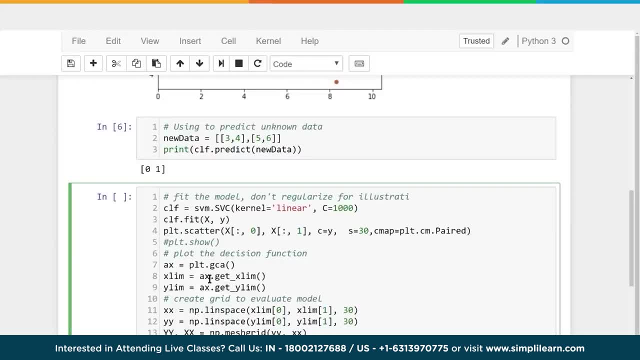 So, when you see data like this, it's necessary to move away from a 1D view of the data to a two-dimensional view of the data. So, when you see data like this, it's necessary to move away from a 1D view of the data to a two-dimensional view of the data. 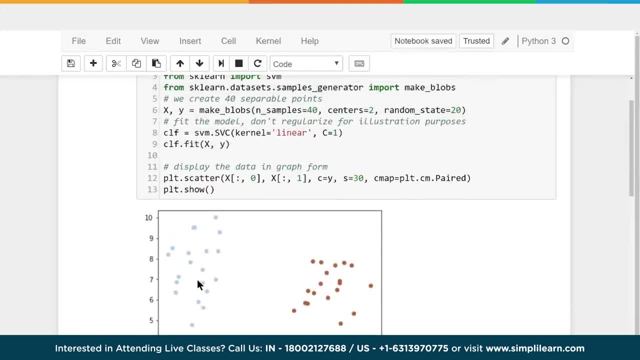 So, when you see data like this, it's necessary to move away from a 1D view of the data to a two-dimensional view of the data. So, when you see data like this, it's necessary to move away from a 1D view of the data to a two-dimensional view of the data. 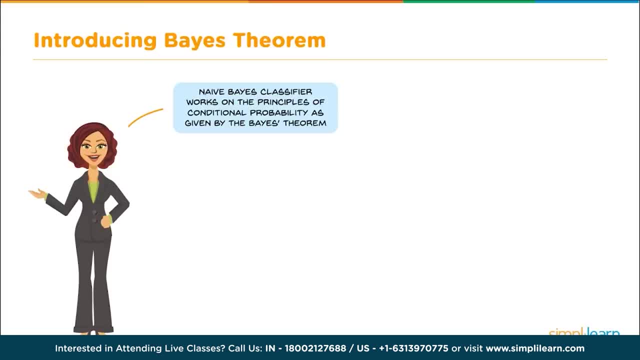 So, when you see data like this, it's necessary to move away from a 1D view of the data to a two-dimensional view of the data. So, when you see data like this, it's necessary to move away from a 1D view of the data to a two-dimensional view of the data. 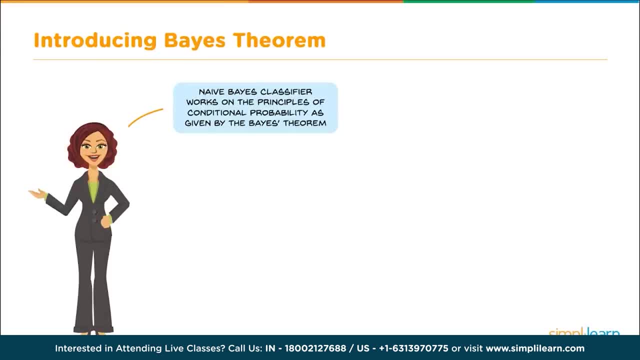 So, when you see data like this, it's necessary to move away from a 1D view of the data to a two-dimensional view of the data. So, when you see data like this, it's necessary to move away from a 1D view of the data to a two-dimensional view of the data. 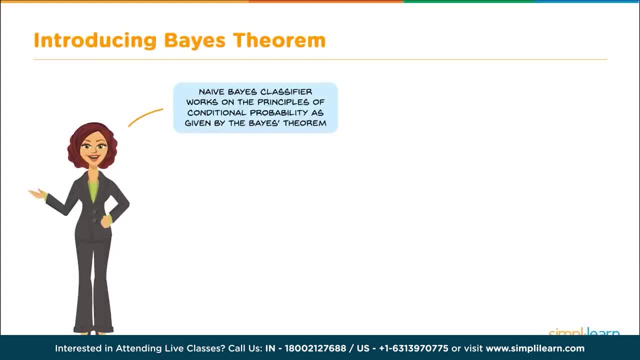 So, when you see data like this, it's necessary to move away from a 1D view of the data to a two-dimensional view of the data. So, when you see data like this, it's necessary to move away from a 1D view of the data to a two-dimensional view of the data. 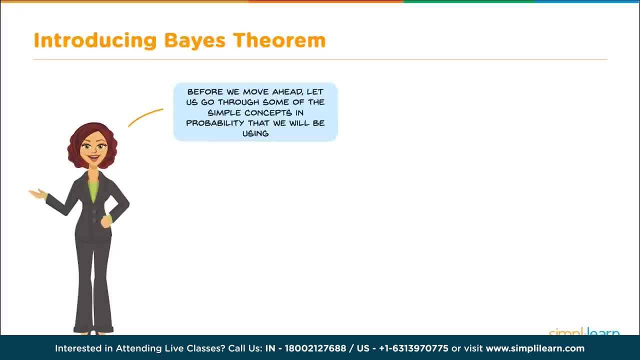 So, when you see data like this, it's necessary to move away from a 1D view of the data to a two-dimensional view of the data. So, when you see data like this, it's necessary to move away from a 1D view of the data to a two-dimensional view of the data. 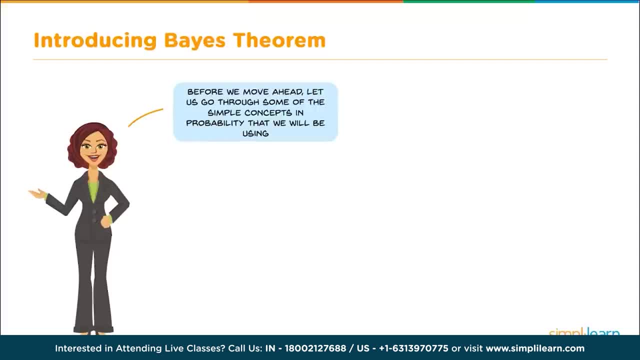 So, when you see data like this, it's necessary to move away from a 1D view of the data to a two-dimensional view of the data. So, when you see data like this, it's necessary to move away from a 1D view of the data to a two-dimensional view of the data. 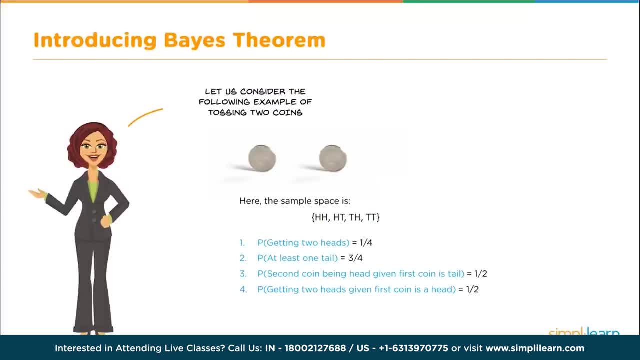 So, when you see data like this, it's necessary to move away from a 1D view of the data to a two-dimensional view of the data. So, when you see data like this, it's necessary to move away from a 1D view of the data to a two-dimensional view of the data. 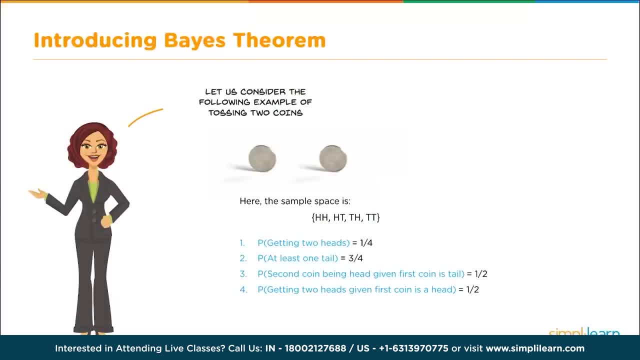 So, when you see data like this, it's necessary to move away from a 1D view of the data to a two-dimensional view of the data. So, when you see data like this, it's necessary to move away from a 1D view of the data to a two-dimensional view of the data. 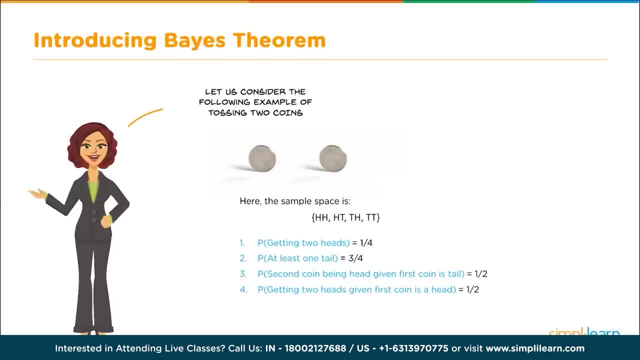 So, when you see data like this, it's necessary to move away from a 1D view of the data to a two-dimensional view of the data. So, when you see data like this, it's necessary to move away from a 1D view of the data to a two-dimensional view of the data. 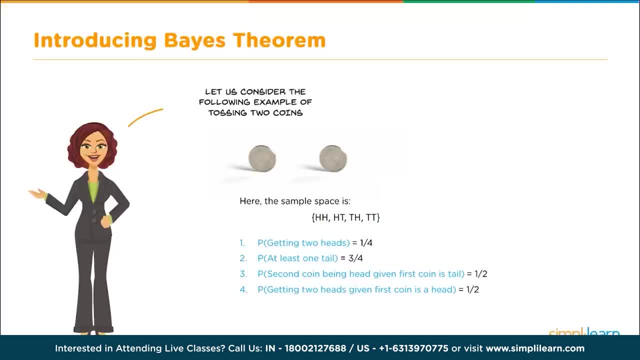 So, when you see data like this, it's necessary to move away from a 1D view of the data to a two-dimensional view of the data. So, when you see data like this, it's necessary to move away from a 1D view of the data to a two-dimensional view of the data. 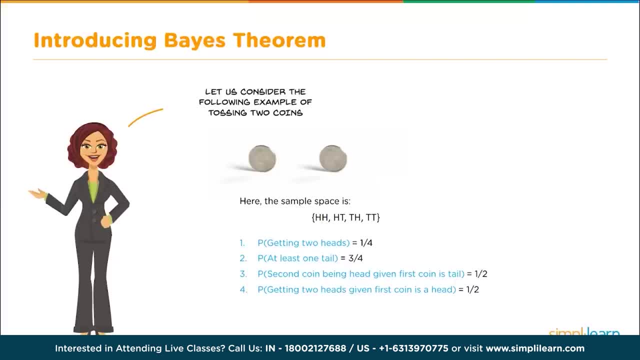 So, when you see data like this, it's necessary to move away from a 1D view of the data to a two-dimensional view of the data. So, when you see data like this, it's necessary to move away from a 1D view of the data to a two-dimensional view of the data. 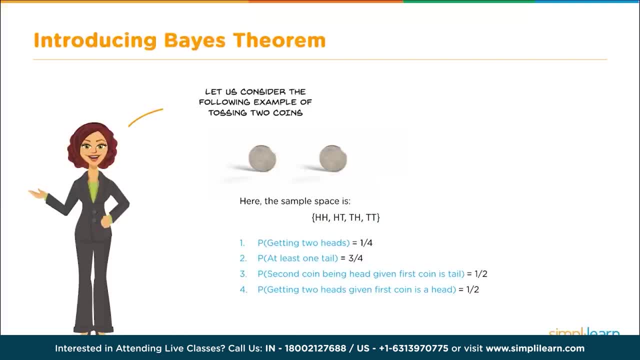 So, when you see data like this, it's necessary to move away from a 1D view of the data to a two-dimensional view of the data. So, when you see data like this, it's necessary to move away from a 1D view of the data to a two-dimensional view of the data. 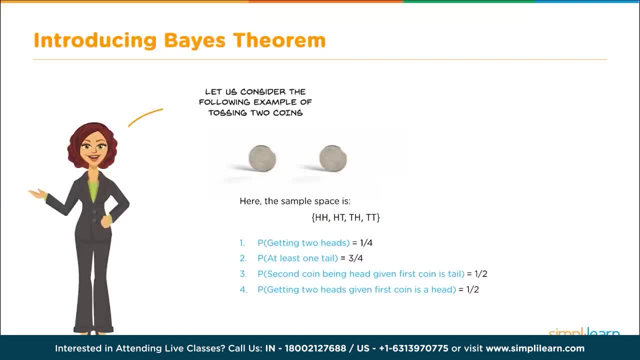 So, when you see data like this, it's necessary to move away from a 1D view of the data to a two-dimensional view of the data. So, when you see data like this, it's necessary to move away from a 1D view of the data to a two-dimensional view of the data. 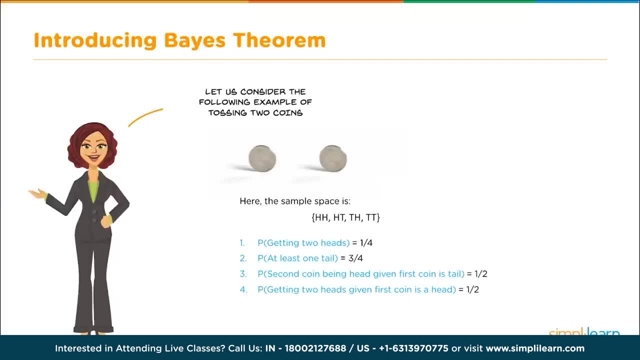 So, when you see data like this, it's necessary to move away from a 1D view of the data to a two-dimensional view of the data. So, when you see data like this, it's necessary to move away from a 1D view of the data to a two-dimensional view of the data. 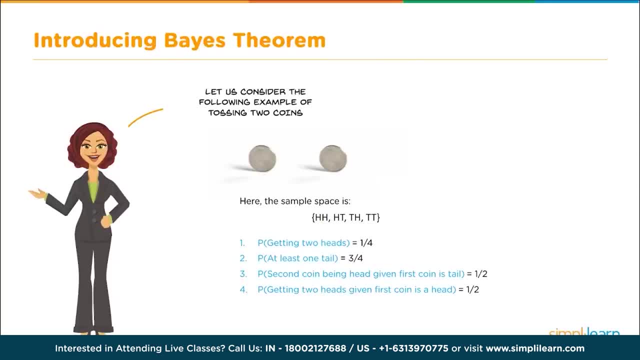 So, when you see data like this, it's necessary to move away from a 1D view of the data to a two-dimensional view of the data. So, when you see data like this, it's necessary to move away from a 1D view of the data to a two-dimensional view of the data. 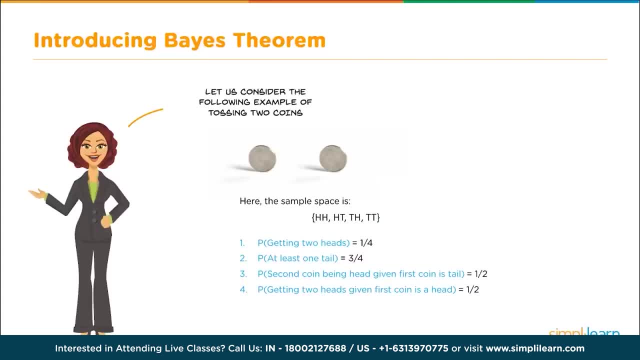 So, when you see data like this, it's necessary to move away from a 1D view of the data to a two-dimensional view of the data. So, when you see data like this, it's necessary to move away from a 1D view of the data to a two-dimensional view of the data. 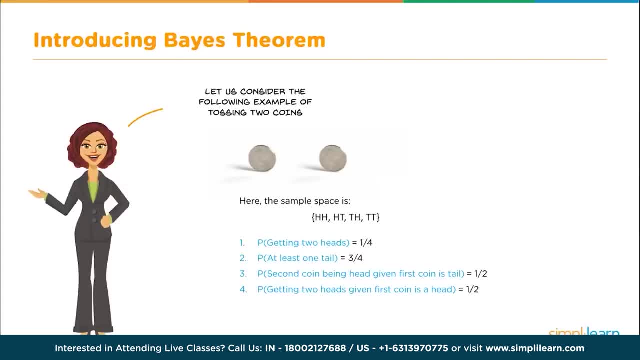 So, when you see data like this, it's necessary to move away from a 1D view of the data to a two-dimensional view of the data. So, when you see data like this, it's necessary to move away from a 1D view of the data to a two-dimensional view of the data. 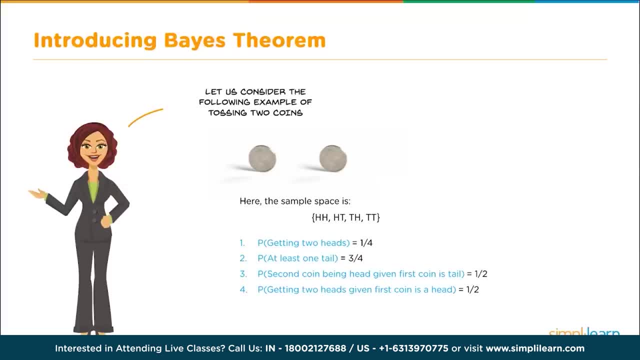 So, when you see data like this, it's necessary to move away from a 1D view of the data to a two-dimensional view of the data. So, when you see data like this, it's necessary to move away from a 1D view of the data to a two-dimensional view of the data. 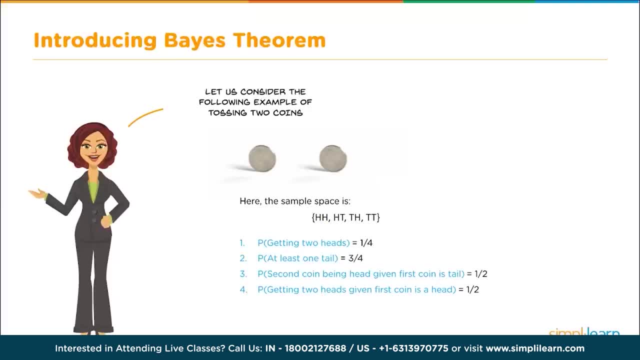 So, when you see data like this, it's necessary to move away from a 1D view of the data to a two-dimensional view of the data. So, when you see data like this, it's necessary to move away from a 1D view of the data to a two-dimensional view of the data. 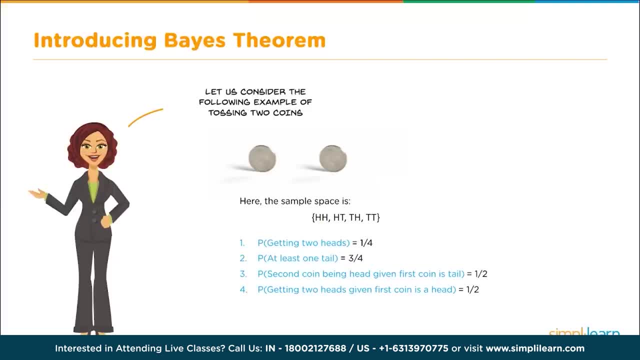 So, when you see data like this, it's necessary to move away from a 1D view of the data to a two-dimensional view of the data. So, when you see data like this, it's necessary to move away from a 1D view of the data to a two-dimensional view of the data. 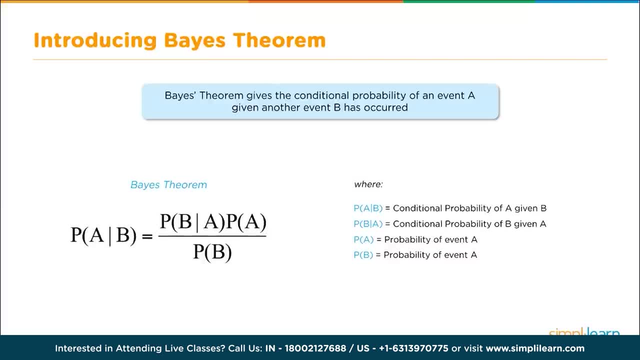 So, when you see data like this, it's necessary to move away from a 1D view of the data to a two-dimensional view of the data. So, when you see data like this, it's necessary to move away from a 1D view of the data to a two-dimensional view of the data. 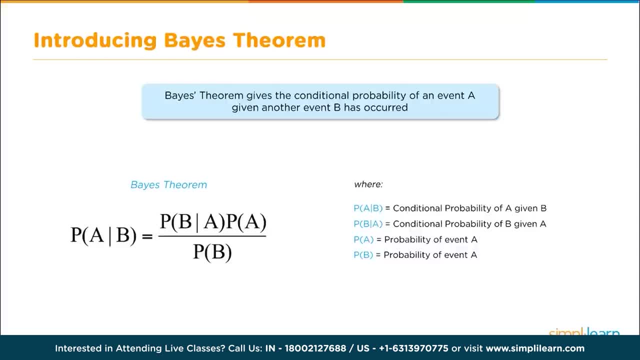 So, when you see data like this, it's necessary to move away from a 1D view of the data to a two-dimensional view of the data. So, when you see data like this, it's necessary to move away from a 1D view of the data to a two-dimensional view of the data. 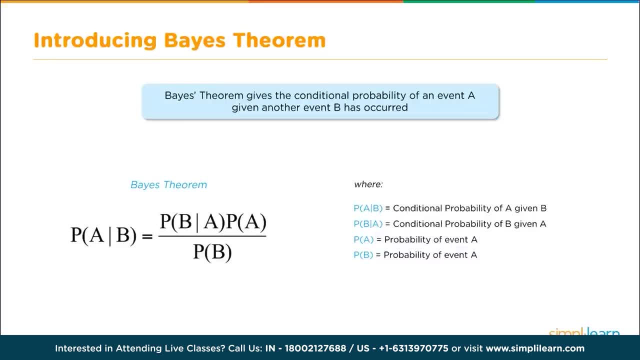 So, when you see data like this, it's necessary to move away from a 1D view of the data to a two-dimensional view of the data. So, when you see data like this, it's necessary to move away from a 1D view of the data to a two-dimensional view of the data. 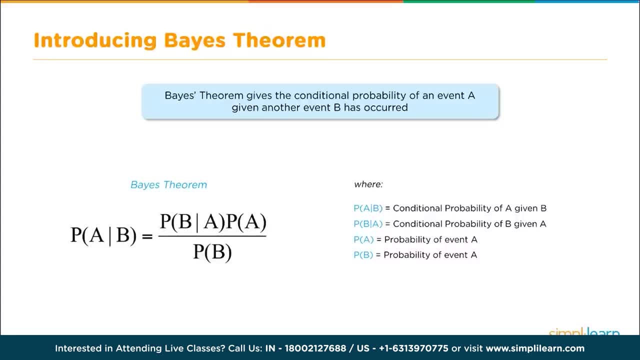 So, when you see data like this, it's necessary to move away from a 1D view of the data to a two-dimensional view of the data. So, when you see data like this, it's necessary to move away from a 1D view of the data to a two-dimensional view of the data. 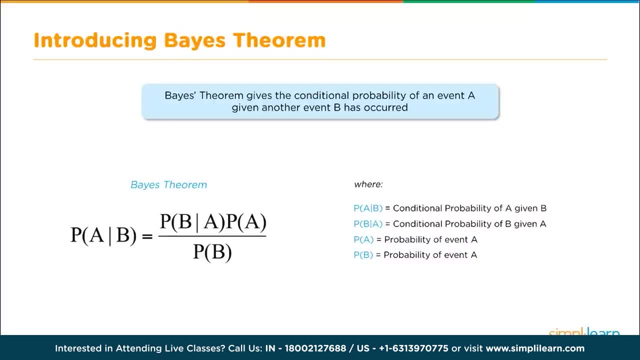 So, when you see data like this, it's necessary to move away from a 1D view of the data to a two-dimensional view of the data. So, when you see data like this, it's necessary to move away from a 1D view of the data to a two-dimensional view of the data. 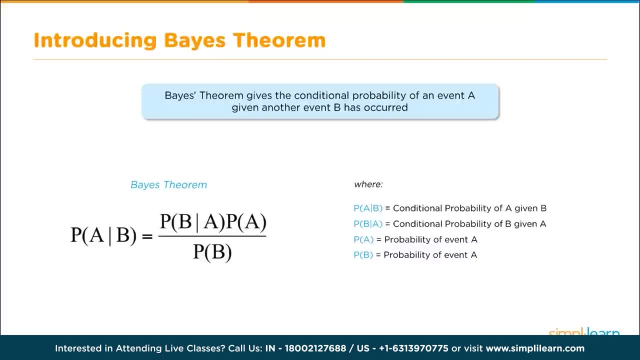 So, when you see data like this, it's necessary to move away from a 1D view of the data to a two-dimensional view of the data. So, when you see data like this, it's necessary to move away from a 1D view of the data to a two-dimensional view of the data. 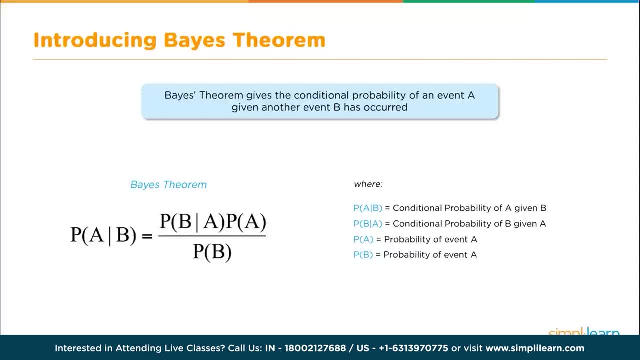 So, when you see data like this, it's necessary to move away from a 1D view of the data to a two-dimensional view of the data. So, when you see data like this, it's necessary to move away from a 1D view of the data to a two-dimensional view of the data. 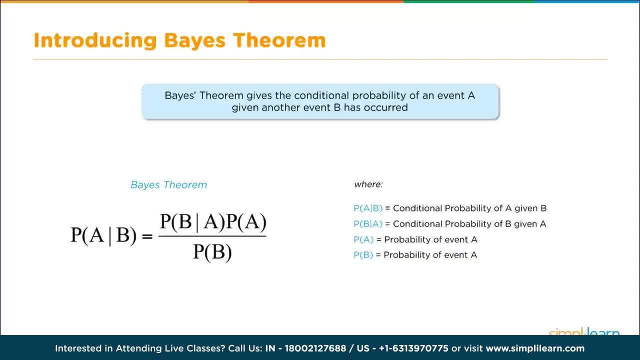 So, when you see data like this, it's necessary to move away from a 1D view of the data to a two-dimensional view of the data. So, when you see data like this, it's necessary to move away from a 1D view of the data to a two-dimensional view of the data. 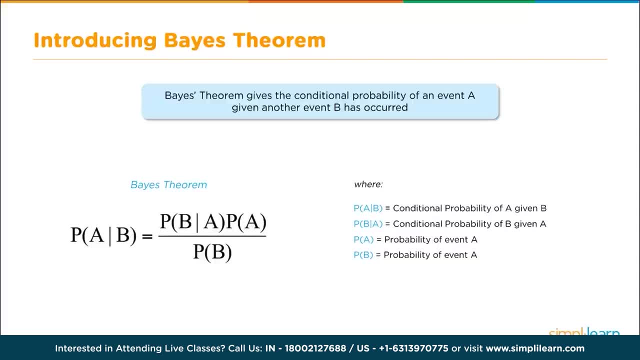 So, when you see data like this, it's necessary to move away from a 1D view of the data to a two-dimensional view of the data. So, when you see data like this, it's necessary to move away from a 1D view of the data to a two-dimensional view of the data. 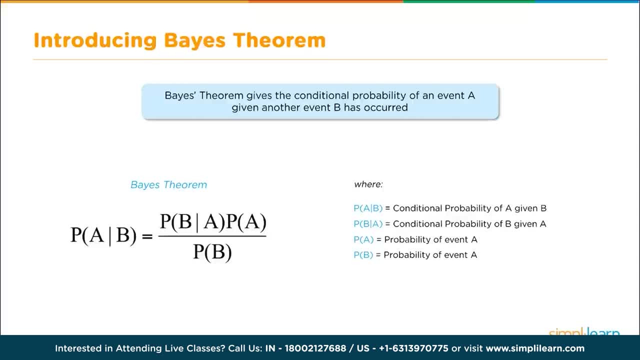 So, when you see data like this, it's necessary to move away from a 1D view of the data to a two-dimensional view of the data. So, when you see data like this, it's necessary to move away from a 1D view of the data to a two-dimensional view of the data. 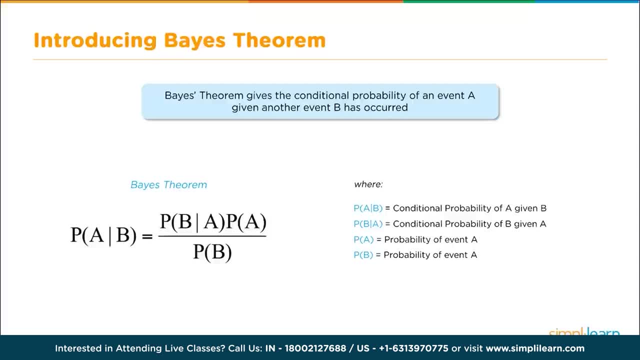 So, when you see data like this, it's necessary to move away from a 1D view of the data to a two-dimensional view of the data. So, when you see data like this, it's necessary to move away from a 1D view of the data to a two-dimensional view of the data. 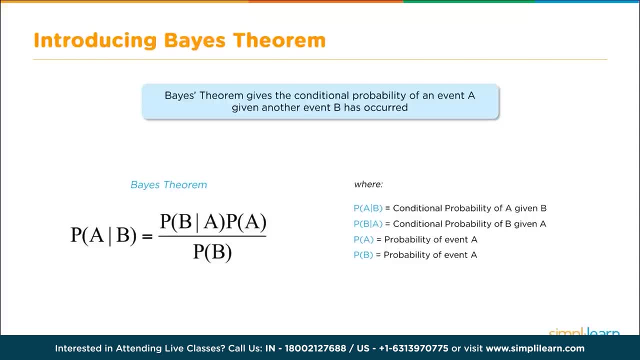 So, when you see data like this, it's necessary to move away from a 1D view of the data to a two-dimensional view of the data. So, when you see data like this, it's necessary to move away from a 1D view of the data to a two-dimensional view of the data. 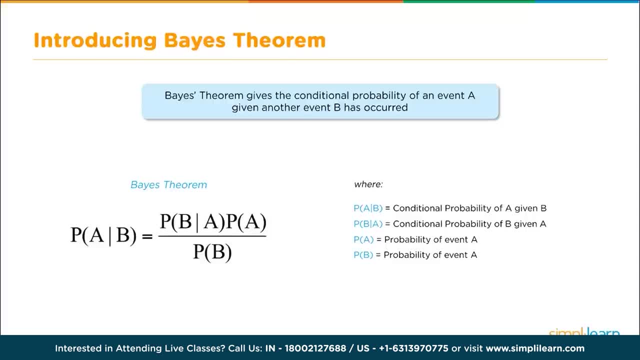 So, when you see data like this, it's necessary to move away from a 1D view of the data to a two-dimensional view of the data. So, when you see data like this, it's necessary to move away from a 1D view of the data to a two-dimensional view of the data. 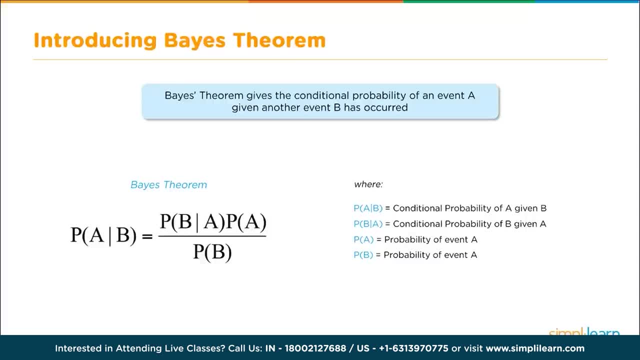 So, when you see data like this, it's necessary to move away from a 1D view of the data to a two-dimensional view of the data. So, when you see data like this, it's necessary to move away from a 1D view of the data to a two-dimensional view of the data. 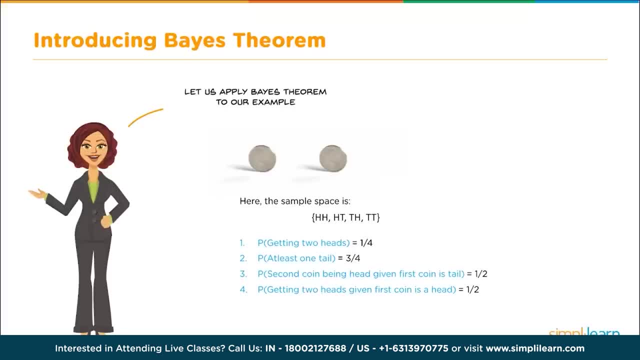 So, when you see data like this, it's necessary to move away from a 1D view of the data to a two-dimensional view of the data. So, when you see data like this, it's necessary to move away from a 1D view of the data to a two-dimensional view of the data. 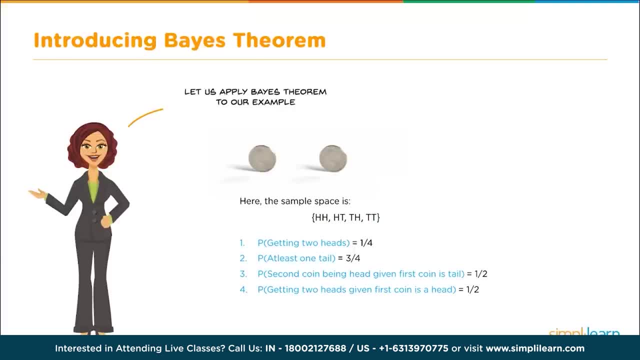 So, when you see data like this, it's necessary to move away from a 1D view of the data to a two-dimensional view of the data. So, when you see data like this, it's necessary to move away from a 1D view of the data to a two-dimensional view of the data. 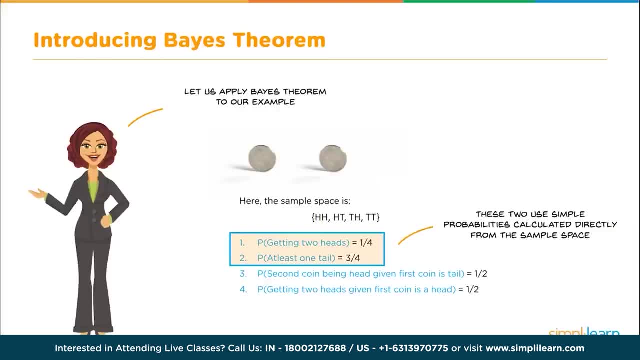 So, when you see data like this, it's necessary to move away from a 1D view of the data to a two-dimensional view of the data. So, when you see data like this, it's necessary to move away from a 1D view of the data to a two-dimensional view of the data. 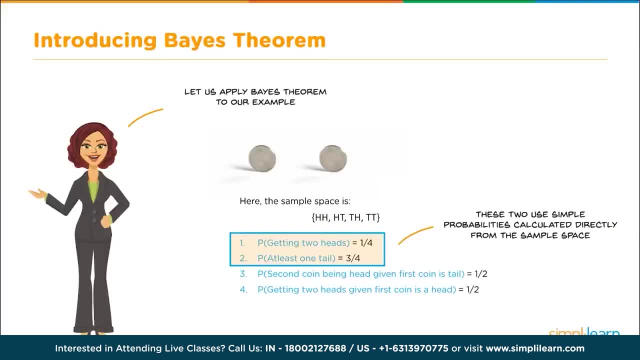 So, when you see data like this, it's necessary to move away from a 1D view of the data to a two-dimensional view of the data. So, when you see data like this, it's necessary to move away from a 1D view of the data to a two-dimensional view of the data. 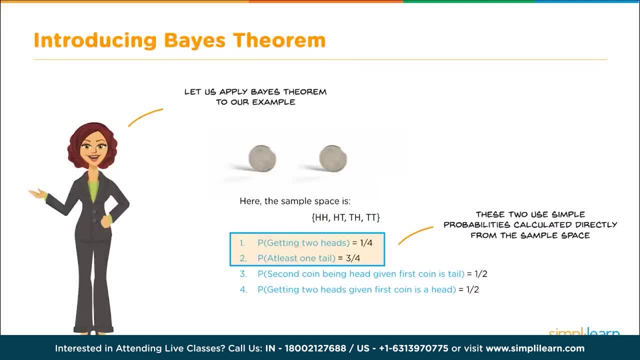 So, when you see data like this, it's necessary to move away from a 1D view of the data to a two-dimensional view of the data. So, when you see data like this, it's necessary to move away from a 1D view of the data to a two-dimensional view of the data. 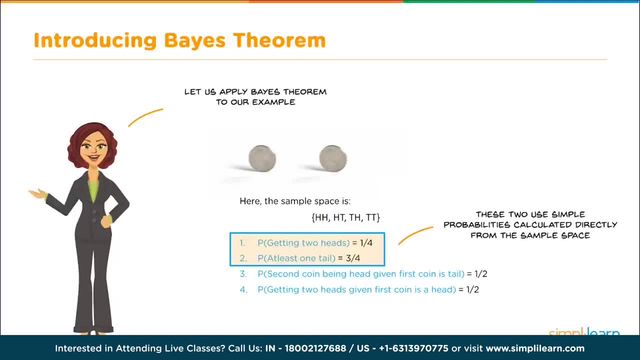 So, when you see data like this, it's necessary to move away from a 1D view of the data to a two-dimensional view of the data. So, when you see data like this, it's necessary to move away from a 1D view of the data to a two-dimensional view of the data. 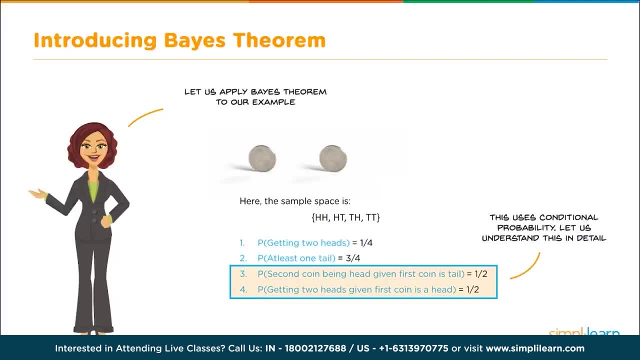 So, when you see data like this, it's necessary to move away from a 1D view of the data to a two-dimensional view of the data. So, when you see data like this, it's necessary to move away from a 1D view of the data to a two-dimensional view of the data. 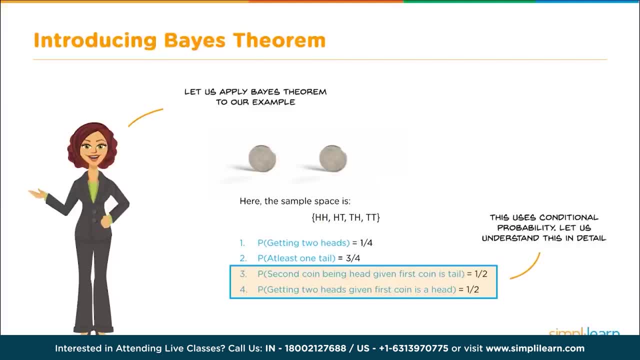 So, when you see data like this, it's necessary to move away from a 1D view of the data to a two-dimensional view of the data. So, when you see data like this, it's necessary to move away from a 1D view of the data to a two-dimensional view of the data. 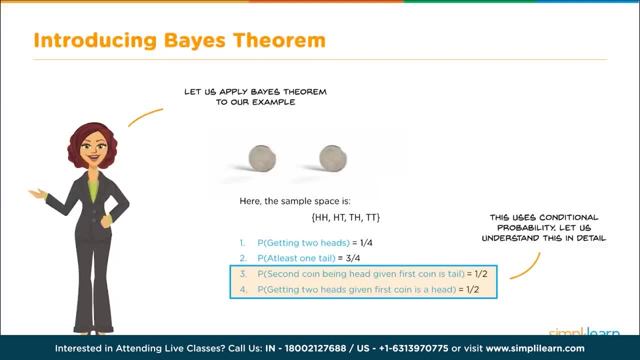 So, when you see data like this, it's necessary to move away from a 1D view of the data to a two-dimensional view of the data. So, when you see data like this, it's necessary to move away from a 1D view of the data to a two-dimensional view of the data. 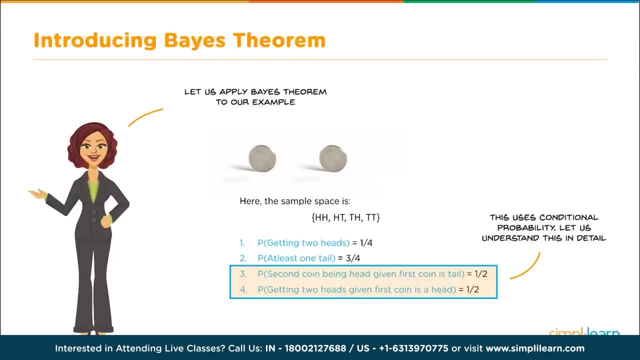 So, when you see data like this, it's necessary to move away from a 1D view of the data to a two-dimensional view of the data. So, when you see data like this, it's necessary to move away from a 1D view of the data to a two-dimensional view of the data. 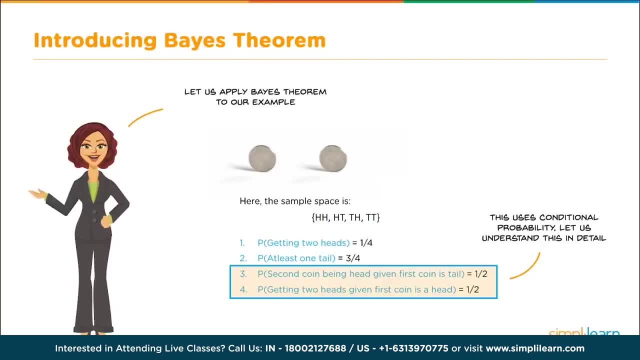 So, when you see data like this, it's necessary to move away from a 1D view of the data to a two-dimensional view of the data. So, when you see data like this, it's necessary to move away from a 1D view of the data to a two-dimensional view of the data. 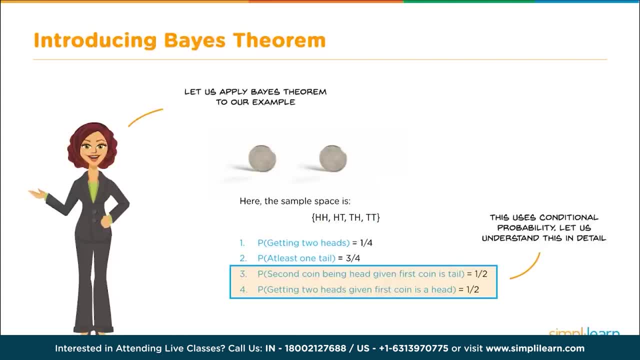 So, when you see data like this, it's necessary to move away from a 1D view of the data to a two-dimensional view of the data. So, when you see data like this, it's necessary to move away from a 1D view of the data to a two-dimensional view of the data. 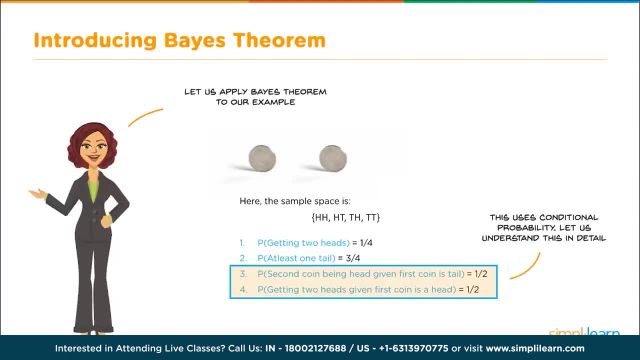 So, when you see data like this, it's necessary to move away from a 1D view of the data to a two-dimensional view of the data. So, when you see data like this, it's necessary to move away from a 1D view of the data to a two-dimensional view of the data. 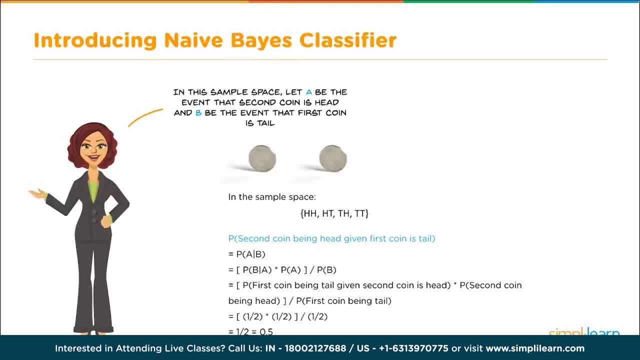 So, when you see data like this, it's necessary to move away from a 1D view of the data to a two-dimensional view of the data. So, when you see data like this, it's necessary to move away from a 1D view of the data to a two-dimensional view of the data. 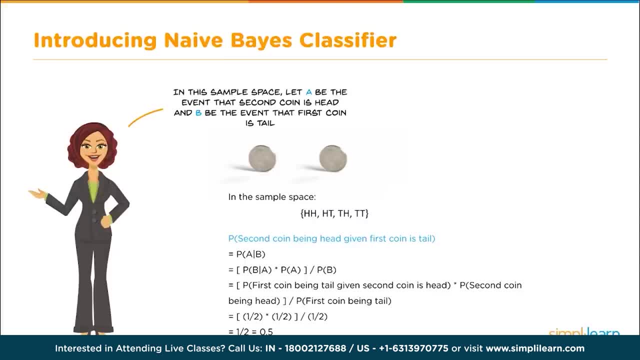 So, when you see data like this, it's necessary to move away from a 1D view of the data to a two-dimensional view of the data. So, when you see data like this, it's necessary to move away from a 1D view of the data to a two-dimensional view of the data. 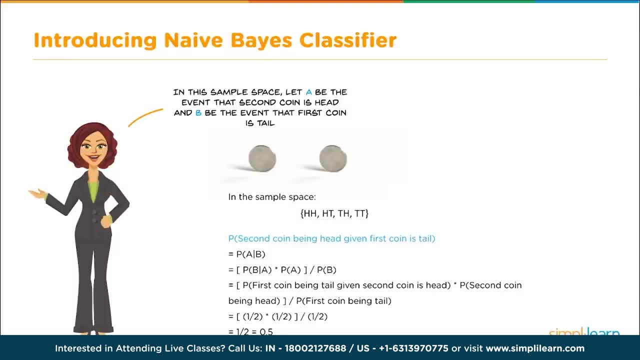 So, when you see data like this, it's necessary to move away from a 1D view of the data to a two-dimensional view of the data. So, when you see data like this, it's necessary to move away from a 1D view of the data to a two-dimensional view of the data. 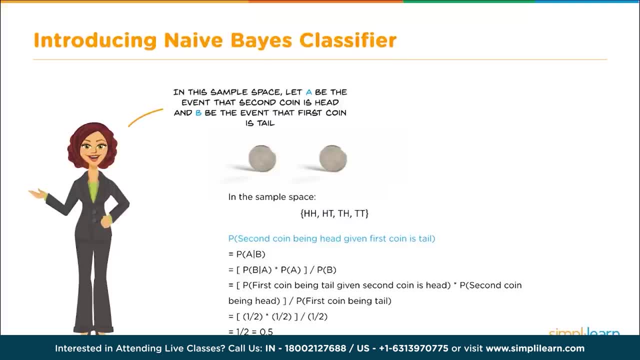 So, when you see data like this, it's necessary to move away from a 1D view of the data to a two-dimensional view of the data. So, when you see data like this, it's necessary to move away from a 1D view of the data to a two-dimensional view of the data. 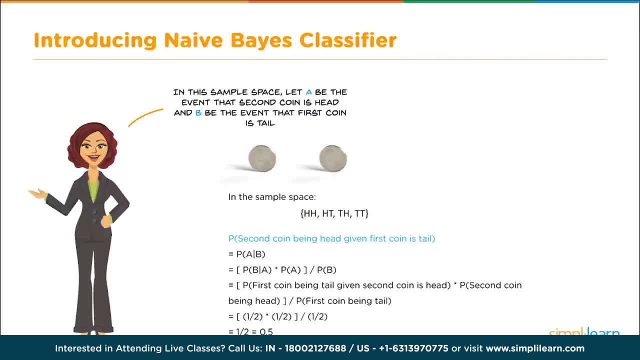 So, when you see data like this, it's necessary to move away from a 1D view of the data to a two-dimensional view of the data. So, when you see data like this, it's necessary to move away from a 1D view of the data to a two-dimensional view of the data. 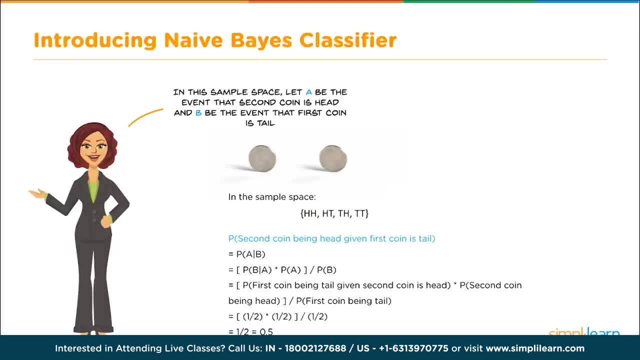 So, when you see data like this, it's necessary to move away from a 1D view of the data to a two-dimensional view of the data. So, when you see data like this, it's necessary to move away from a 1D view of the data to a two-dimensional view of the data. 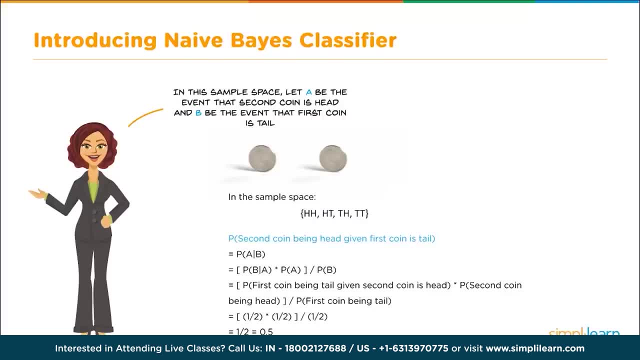 So, when you see data like this, it's necessary to move away from a 1D view of the data to a two-dimensional view of the data. So, when you see data like this, it's necessary to move away from a 1D view of the data to a two-dimensional view of the data. 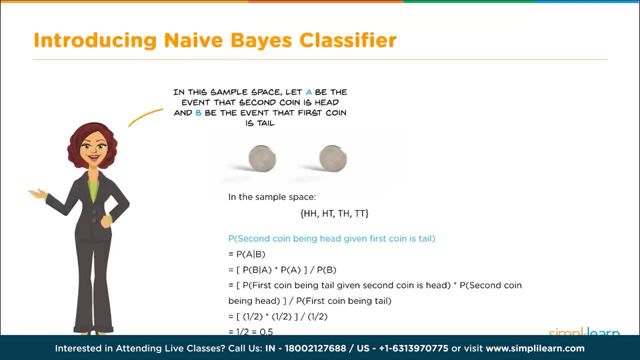 So, when you see data like this, it's necessary to move away from a 1D view of the data to a two-dimensional view of the data. So, when you see data like this, it's necessary to move away from a 1D view of the data to a two-dimensional view of the data. 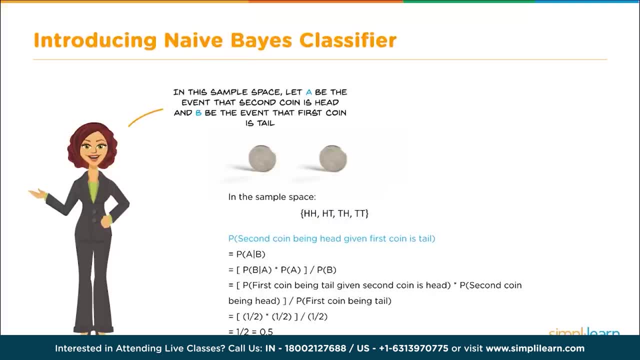 So, when you see data like this, it's necessary to move away from a 1D view of the data to a two-dimensional view of the data. So, when you see data like this, it's necessary to move away from a 1D view of the data to a two-dimensional view of the data. 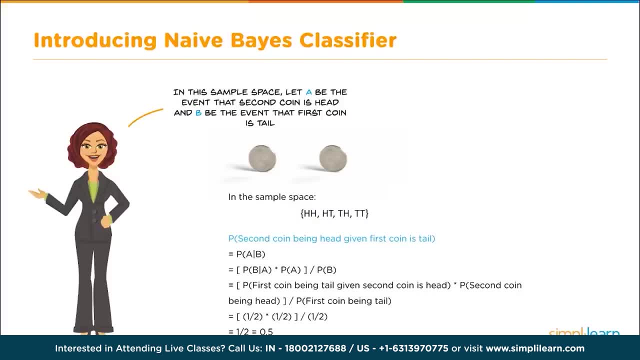 So, when you see data like this, it's necessary to move away from a 1D view of the data to a two-dimensional view of the data. So, when you see data like this, it's necessary to move away from a 1D view of the data to a two-dimensional view of the data. 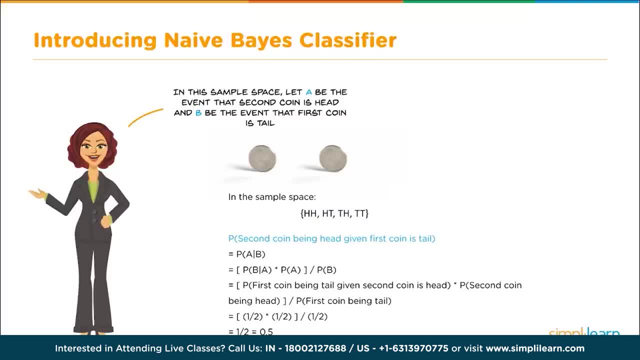 So, when you see data like this, it's necessary to move away from a 1D view of the data to a two-dimensional view of the data. So, when you see data like this, it's necessary to move away from a 1D view of the data to a two-dimensional view of the data. 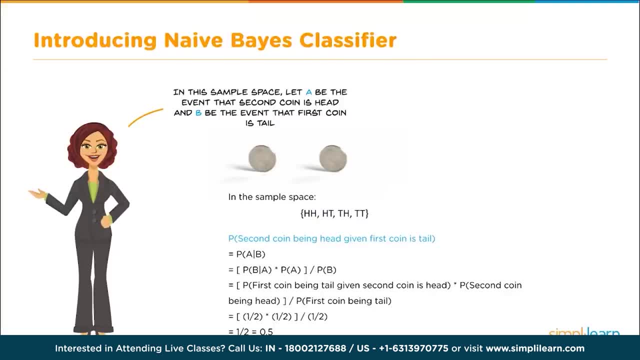 So, when you see data like this, it's necessary to move away from a 1D view of the data to a two-dimensional view of the data. So, when you see data like this, it's necessary to move away from a 1D view of the data to a two-dimensional view of the data. 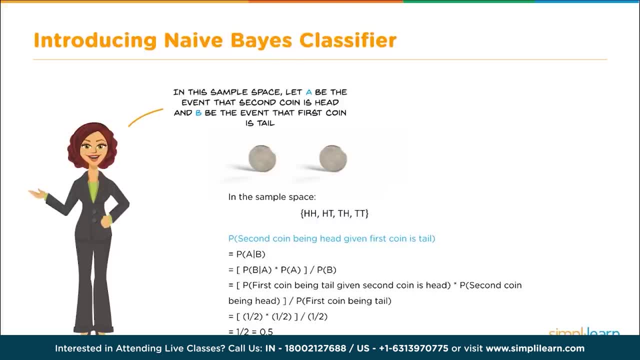 So, when you see data like this, it's necessary to move away from a 1D view of the data to a two-dimensional view of the data. So, when you see data like this, it's necessary to move away from a 1D view of the data to a two-dimensional view of the data. 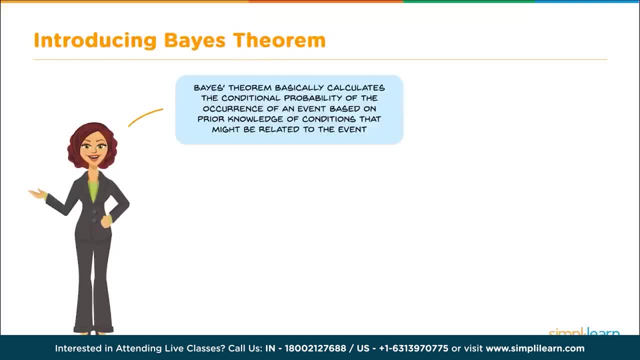 So, when you see data like this, it's necessary to move away from a 1D view of the data to a two-dimensional view of the data. So, when you see data like this, it's necessary to move away from a 1D view of the data to a two-dimensional view of the data. 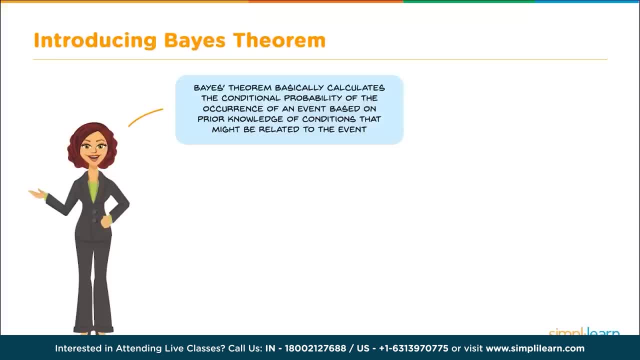 So, when you see data like this, it's necessary to move away from a 1D view of the data to a two-dimensional view of the data. So, when you see data like this, it's necessary to move away from a 1D view of the data to a two-dimensional view of the data. 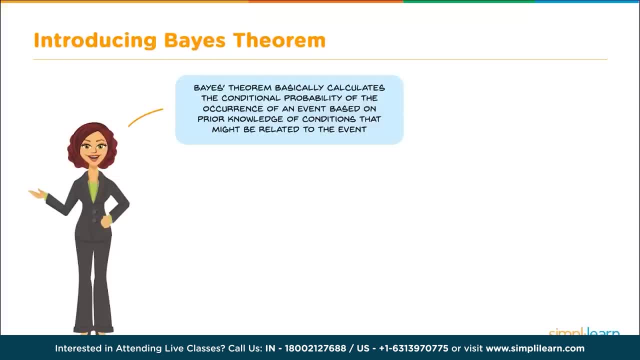 So, when you see data like this, it's necessary to move away from a 1D view of the data to a two-dimensional view of the data. So, when you see data like this, it's necessary to move away from a 1D view of the data to a two-dimensional view of the data. 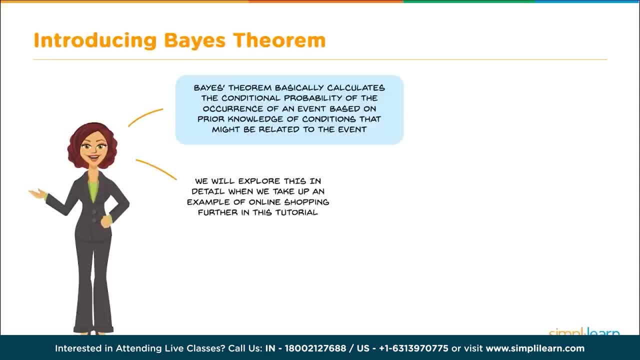 So, when you see data like this, it's necessary to move away from a 1D view of the data to a two-dimensional view of the data. So, when you see data like this, it's necessary to move away from a 1D view of the data to a two-dimensional view of the data. 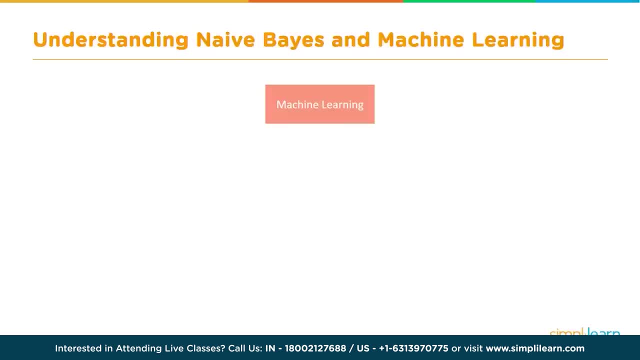 So, when you see data like this, it's necessary to move away from a 1D view of the data to a two-dimensional view of the data. So, when you see data like this, it's necessary to move away from a 1D view of the data to a two-dimensional view of the data. 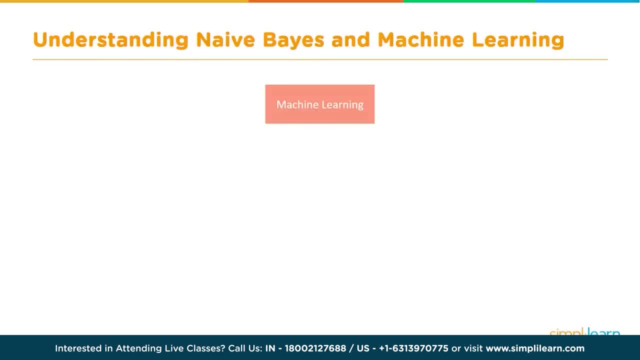 So, when you see data like this, it's necessary to move away from a 1D view of the data to a two-dimensional view of the data. So, when you see data like this, it's necessary to move away from a 1D view of the data to a two-dimensional view of the data. 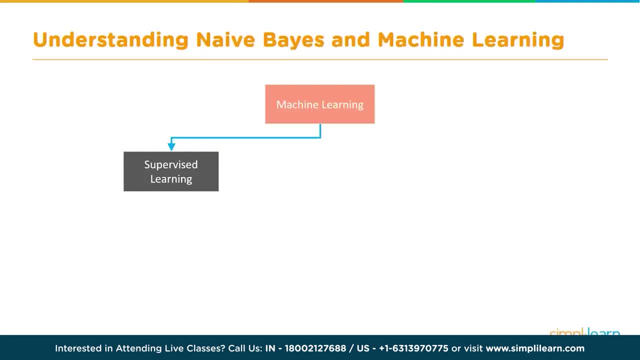 So, when you see data like this, it's necessary to move away from a 1D view of the data to a two-dimensional view of the data. So, when you see data like this, it's necessary to move away from a 1D view of the data to a two-dimensional view of the data. 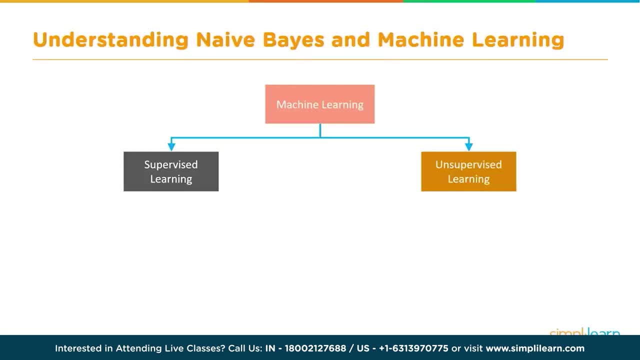 So, when you see data like this, it's necessary to move away from a 1D view of the data to a two-dimensional view of the data. So, when you see data like this, it's necessary to move away from a 1D view of the data to a two-dimensional view of the data. 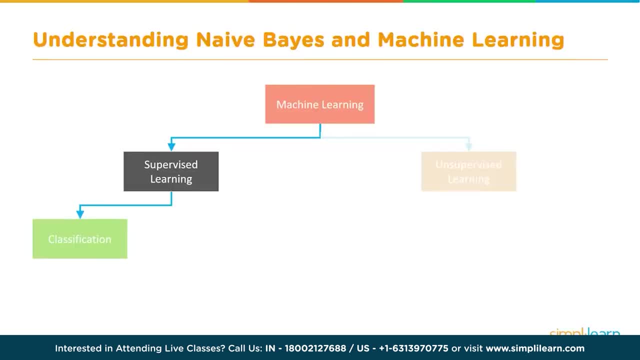 So, when you see data like this, it's necessary to move away from a 1D view of the data to a two-dimensional view of the data. So, when you see data like this, it's necessary to move away from a 1D view of the data to a two-dimensional view of the data. 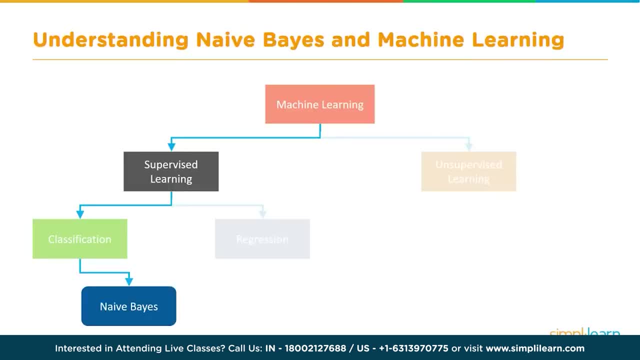 So, when you see data like this, it's necessary to move away from a 1D view of the data to a two-dimensional view of the data. So, when you see data like this, it's necessary to move away from a 1D view of the data to a two-dimensional view of the data. 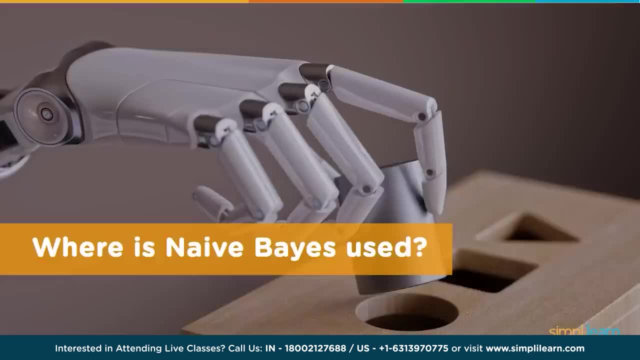 So, when you see data like this, it's necessary to move away from a 1D view of the data to a two-dimensional view of the data. So, when you see data like this, it's necessary to move away from a 1D view of the data to a two-dimensional view of the data. 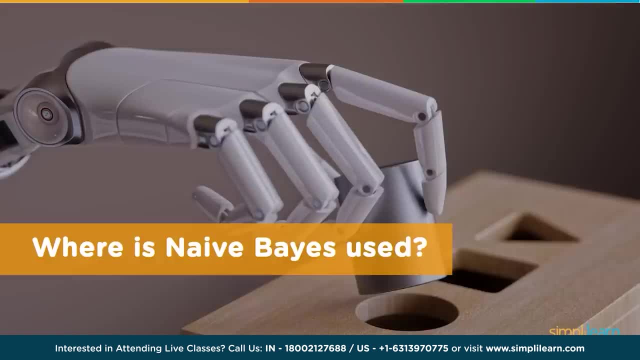 So, when you see data like this, it's necessary to move away from a 1D view of the data to a two-dimensional view of the data. So, when you see data like this, it's necessary to move away from a 1D view of the data to a two-dimensional view of the data. 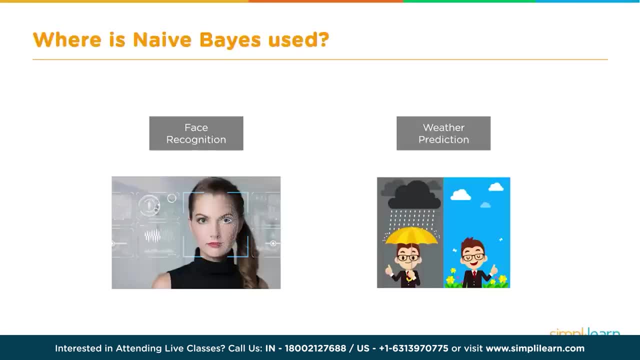 So, when you see data like this, it's necessary to move away from a 1D view of the data to a two-dimensional view of the data. So, when you see data like this, it's necessary to move away from a 1D view of the data to a two-dimensional view of the data. 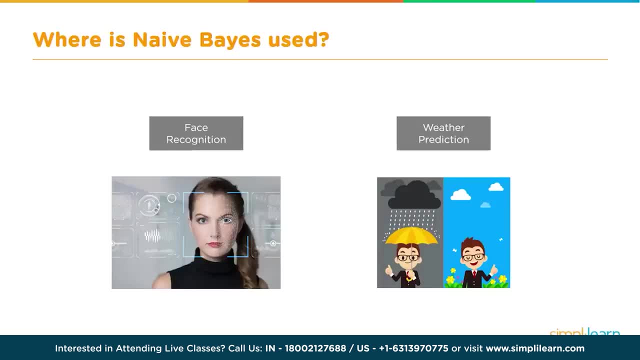 So, when you see data like this, it's necessary to move away from a 1D view of the data to a two-dimensional view of the data. So, when you see data like this, it's necessary to move away from a 1D view of the data to a two-dimensional view of the data. 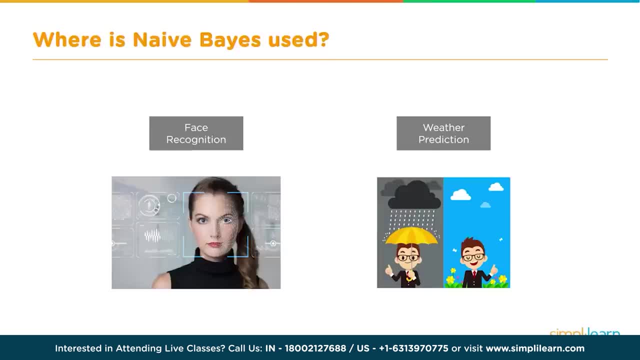 So, when you see data like this, it's necessary to move away from a 1D view of the data to a two-dimensional view of the data. So, when you see data like this, it's necessary to move away from a 1D view of the data to a two-dimensional view of the data. 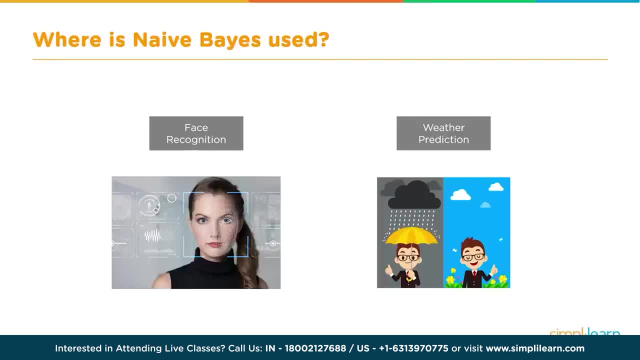 So, when you see data like this, it's necessary to move away from a 1D view of the data to a two-dimensional view of the data. So, when you see data like this, it's necessary to move away from a 1D view of the data to a two-dimensional view of the data. 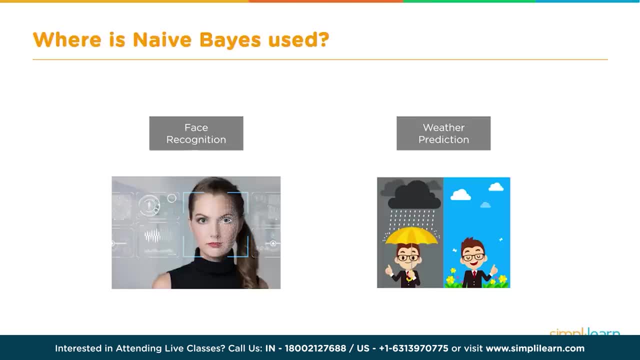 So, when you see data like this, it's necessary to move away from a 1D view of the data to a two-dimensional view of the data. So, when you see data like this, it's necessary to move away from a 1D view of the data to a two-dimensional view of the data. 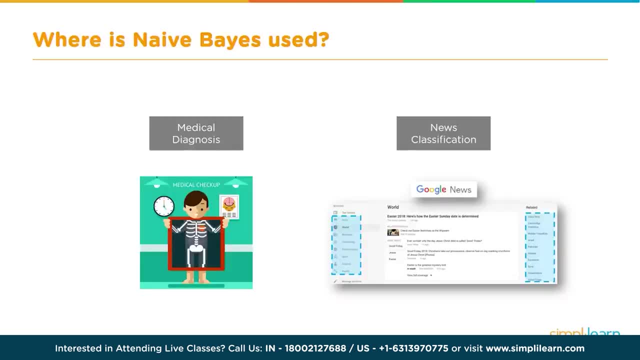 So, when you see data like this, it's necessary to move away from a 1D view of the data to a two-dimensional view of the data. So, when you see data like this, it's necessary to move away from a 1D view of the data to a two-dimensional view of the data. 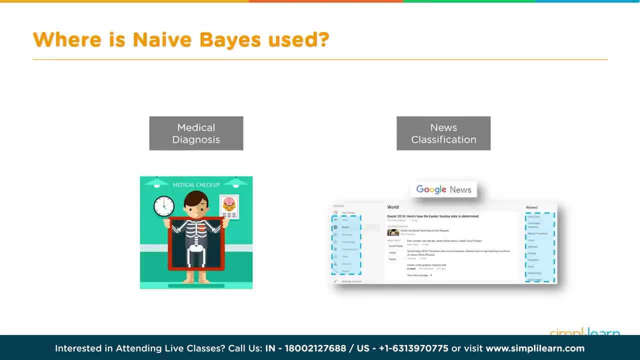 So, when you see data like this, it's necessary to move away from a 1D view of the data to a two-dimensional view of the data. So, when you see data like this, it's necessary to move away from a 1D view of the data to a two-dimensional view of the data. 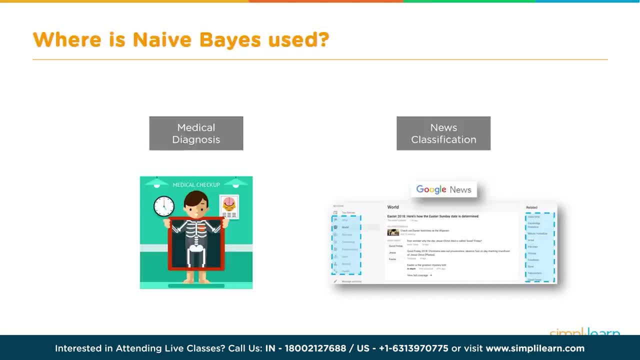 So, when you see data like this, it's necessary to move away from a 1D view of the data to a two-dimensional view of the data. So, when you see data like this, it's necessary to move away from a 1D view of the data to a two-dimensional view of the data. 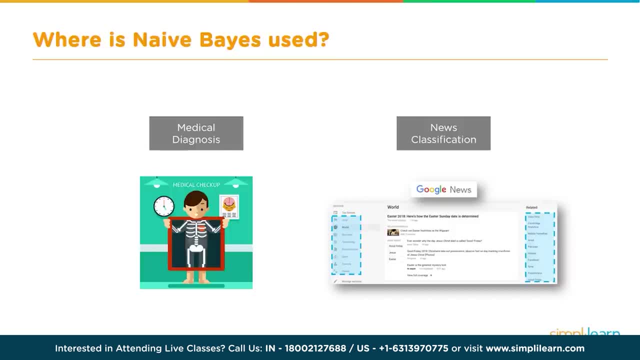 So, when you see data like this, it's necessary to move away from a 1D view of the data to a two-dimensional view of the data. So, when you see data like this, it's necessary to move away from a 1D view of the data to a two-dimensional view of the data. 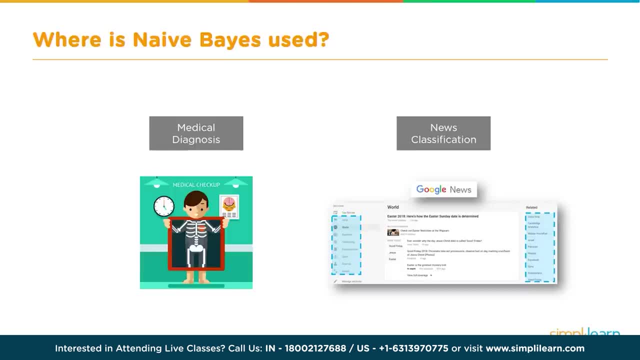 So, when you see data like this, it's necessary to move away from a 1D view of the data to a two-dimensional view of the data. So, when you see data like this, it's necessary to move away from a 1D view of the data to a two-dimensional view of the data. 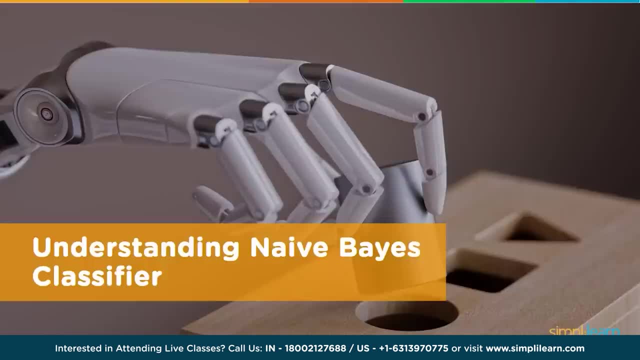 So, when you see data like this, it's necessary to move away from a 1D view of the data to a two-dimensional view of the data. So, when you see data like this, it's necessary to move away from a 1D view of the data to a two-dimensional view of the data. 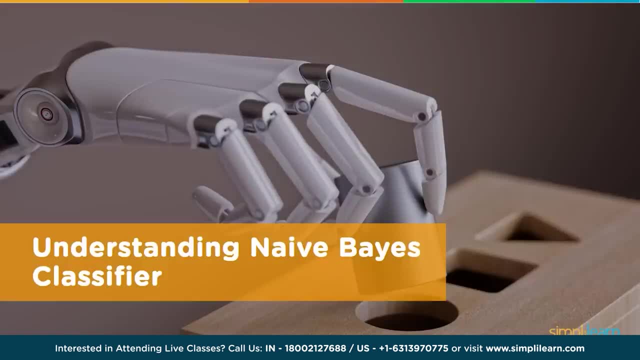 So, when you see data like this, it's necessary to move away from a 1D view of the data to a two-dimensional view of the data. So, when you see data like this, it's necessary to move away from a 1D view of the data to a two-dimensional view of the data. 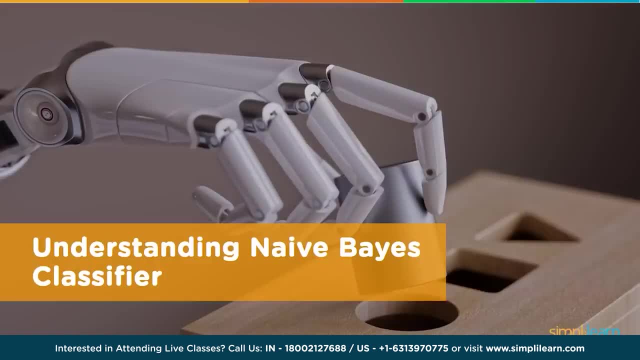 So, when you see data like this, it's necessary to move away from a 1D view of the data to a two-dimensional view of the data. So, when you see data like this, it's necessary to move away from a 1D view of the data to a two-dimensional view of the data. 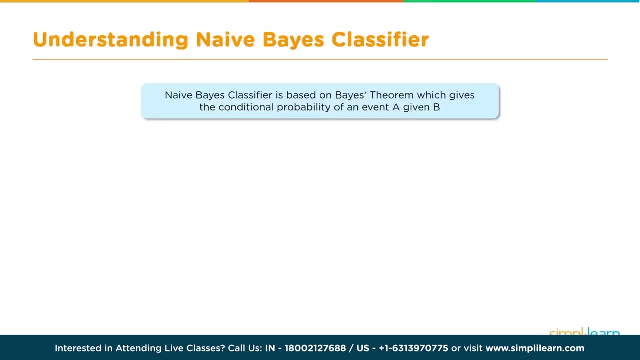 So, when you see data like this, it's necessary to move away from a 1D view of the data to a two-dimensional view of the data. So, when you see data like this, it's necessary to move away from a 1D view of the data to a two-dimensional view of the data. 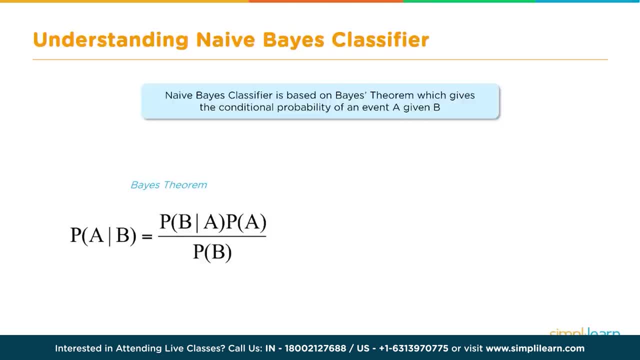 So, when you see data like this, it's necessary to move away from a 1D view of the data to a two-dimensional view of the data. So, when you see data like this, it's necessary to move away from a 1D view of the data to a two-dimensional view of the data. 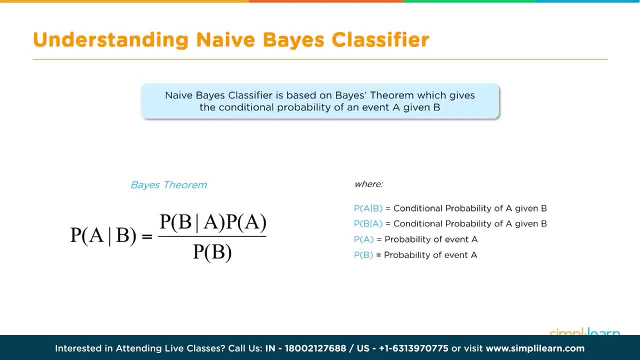 So, when you see data like this, it's necessary to move away from a 1D view of the data to a two-dimensional view of the data. So, when you see data like this, it's necessary to move away from a 1D view of the data to a two-dimensional view of the data. 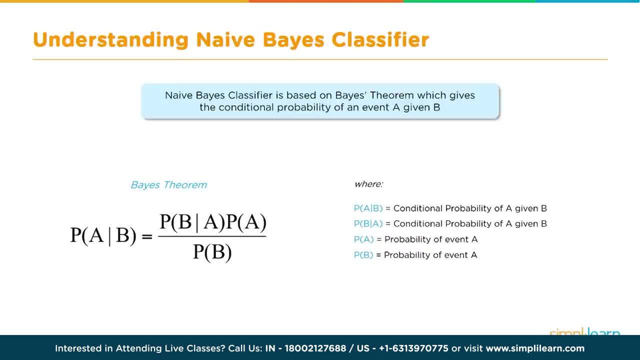 So, when you see data like this, it's necessary to move away from a 1D view of the data to a two-dimensional view of the data. So, when you see data like this, it's necessary to move away from a 1D view of the data to a two-dimensional view of the data. 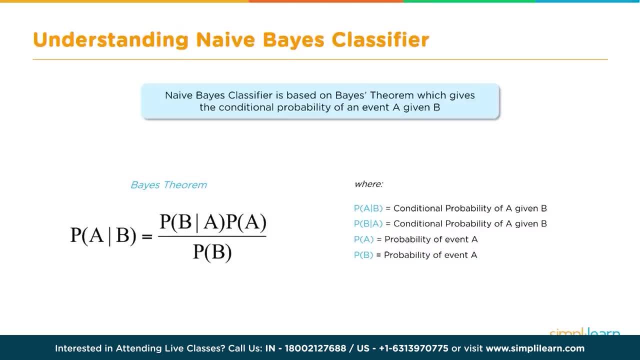 So, when you see data like this, it's necessary to move away from a 1D view of the data to a two-dimensional view of the data. So, when you see data like this, it's necessary to move away from a 1D view of the data to a two-dimensional view of the data. 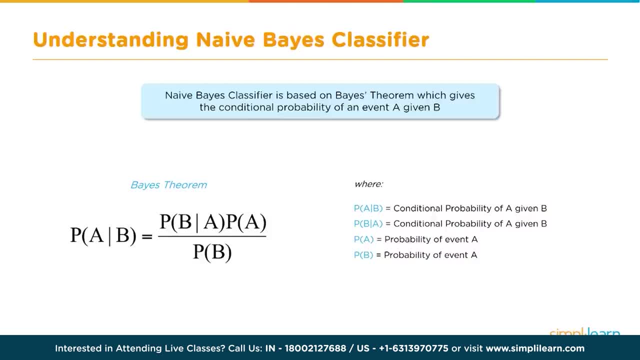 So, when you see data like this, it's necessary to move away from a 1D view of the data to a two-dimensional view of the data. So, when you see data like this, it's necessary to move away from a 1D view of the data to a two-dimensional view of the data. 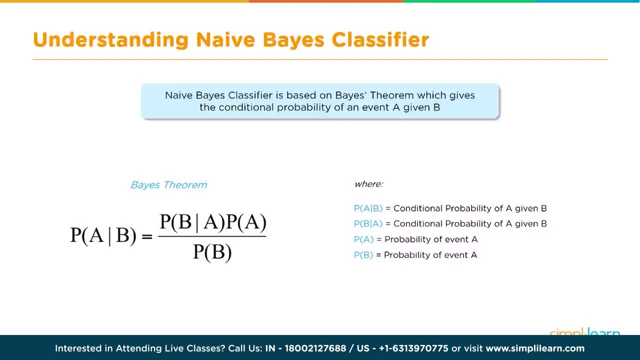 So, when you see data like this, it's necessary to move away from a 1D view of the data to a two-dimensional view of the data. So, when you see data like this, it's necessary to move away from a 1D view of the data to a two-dimensional view of the data. 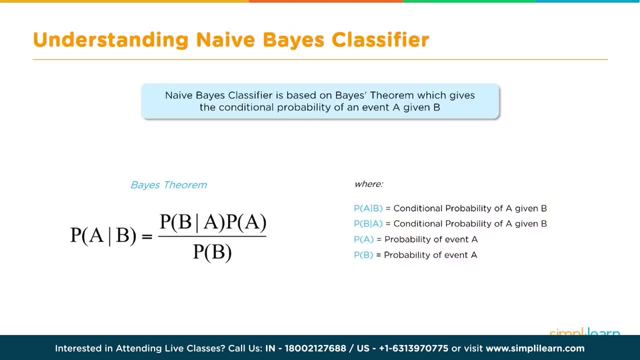 So, when you see data like this, it's necessary to move away from a 1D view of the data to a two-dimensional view of the data. So, when you see data like this, it's necessary to move away from a 1D view of the data to a two-dimensional view of the data. 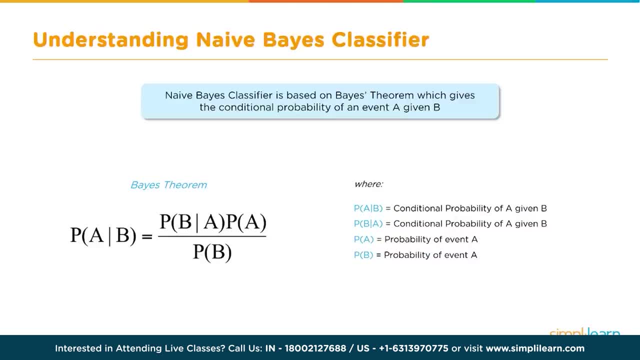 So, when you see data like this, it's necessary to move away from a 1D view of the data to a two-dimensional view of the data. So, when you see data like this, it's necessary to move away from a 1D view of the data to a two-dimensional view of the data. 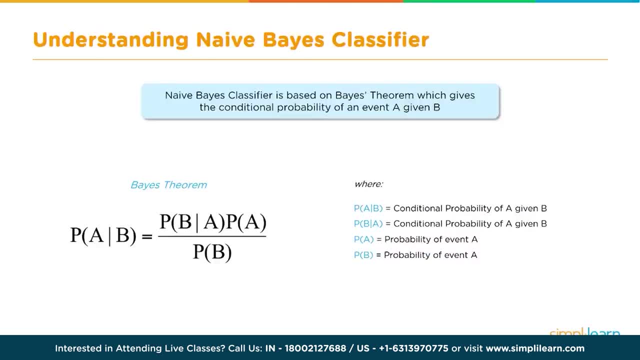 So, when you see data like this, it's necessary to move away from a 1D view of the data to a two-dimensional view of the data. So, when you see data like this, it's necessary to move away from a 1D view of the data to a two-dimensional view of the data. 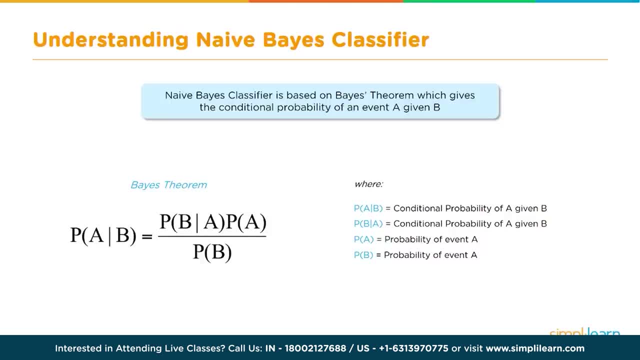 So, when you see data like this, it's necessary to move away from a 1D view of the data to a two-dimensional view of the data. So, when you see data like this, it's necessary to move away from a 1D view of the data to a two-dimensional view of the data. 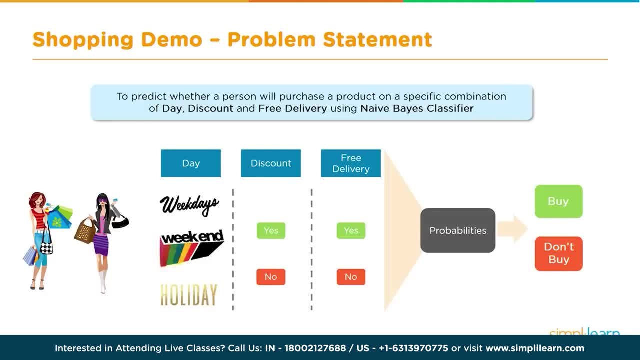 So, when you see data like this, it's necessary to move away from a 1D view of the data to a two-dimensional view of the data. So, when you see data like this, it's necessary to move away from a 1D view of the data to a two-dimensional view of the data. 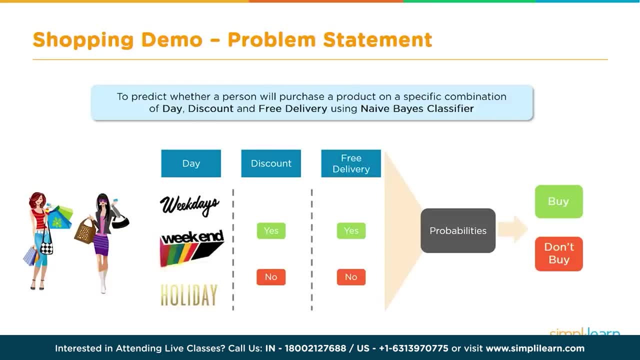 So, when you see data like this, it's necessary to move away from a 1D view of the data to a two-dimensional view of the data. So, when you see data like this, it's necessary to move away from a 1D view of the data to a two-dimensional view of the data. 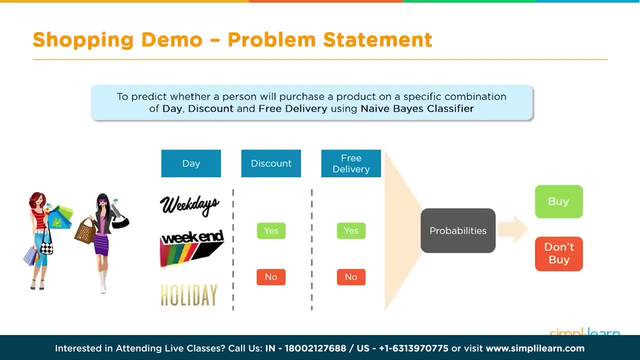 So, when you see data like this, it's necessary to move away from a 1D view of the data to a two-dimensional view of the data. So, when you see data like this, it's necessary to move away from a 1D view of the data to a two-dimensional view of the data. 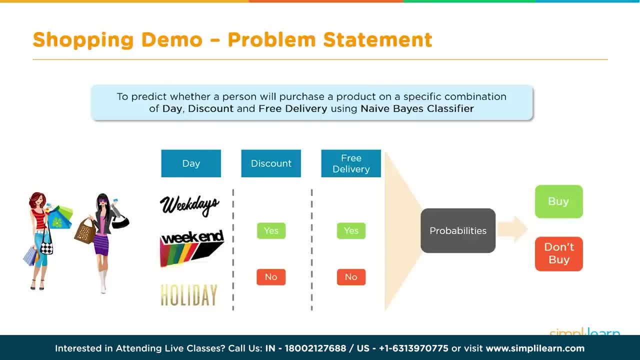 So, when you see data like this, it's necessary to move away from a 1D view of the data to a two-dimensional view of the data. So, when you see data like this, it's necessary to move away from a 1D view of the data to a two-dimensional view of the data. 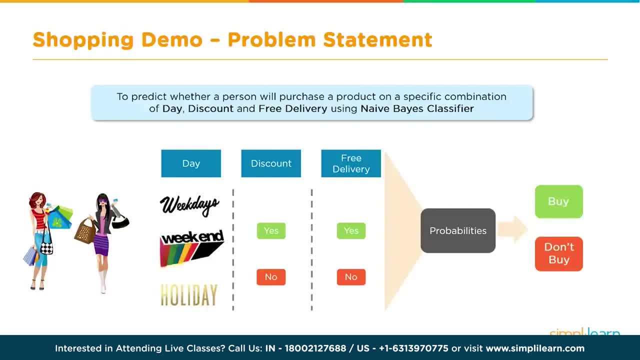 So, when you see data like this, it's necessary to move away from a 1D view of the data to a two-dimensional view of the data. So, when you see data like this, it's necessary to move away from a 1D view of the data to a two-dimensional view of the data. 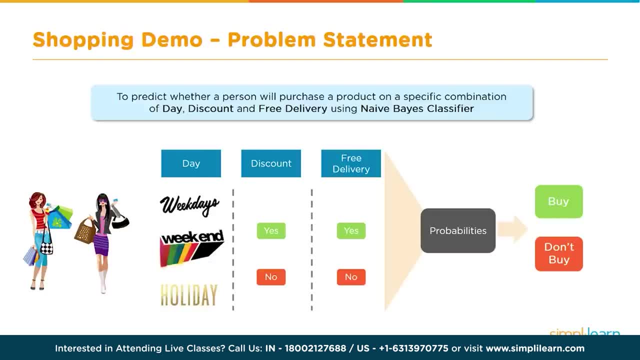 So, when you see data like this, it's necessary to move away from a 1D view of the data to a two-dimensional view of the data. So, when you see data like this, it's necessary to move away from a 1D view of the data to a two-dimensional view of the data. 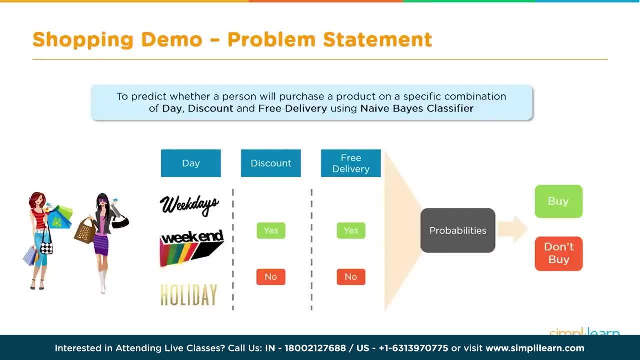 So, when you see data like this, it's necessary to move away from a 1D view of the data to a two-dimensional view of the data. So, when you see data like this, it's necessary to move away from a 1D view of the data to a two-dimensional view of the data. 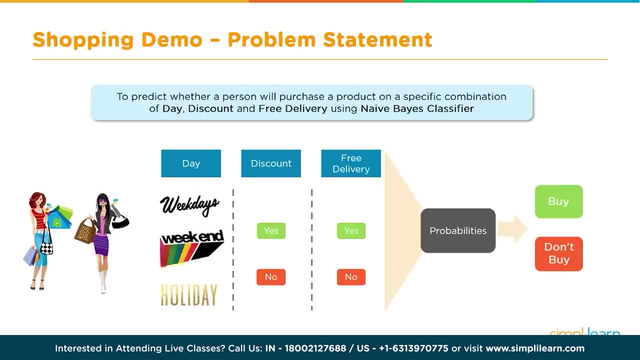 So, when you see data like this, it's necessary to move away from a 1D view of the data to a two-dimensional view of the data. So, when you see data like this, it's necessary to move away from a 1D view of the data to a two-dimensional view of the data. 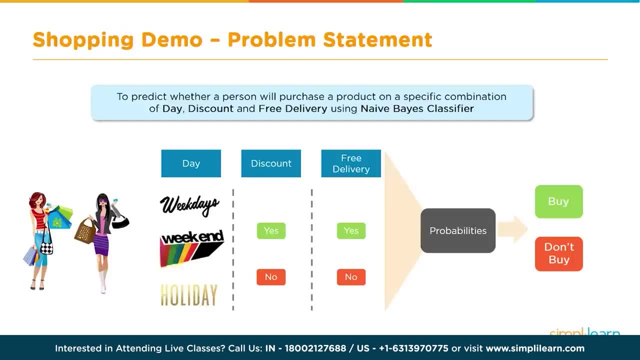 So, when you see data like this, it's necessary to move away from a 1D view of the data to a two-dimensional view of the data. So, when you see data like this, it's necessary to move away from a 1D view of the data to a two-dimensional view of the data. 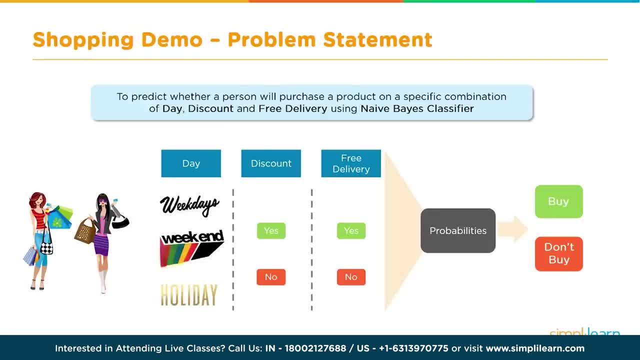 So, when you see data like this, it's necessary to move away from a 1D view of the data to a two-dimensional view of the data. So, when you see data like this, it's necessary to move away from a 1D view of the data to a two-dimensional view of the data. 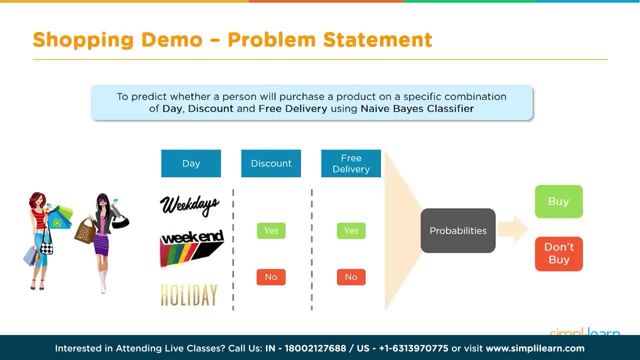 So, when you see data like this, it's necessary to move away from a 1D view of the data to a two-dimensional view of the data. So, when you see data like this, it's necessary to move away from a 1D view of the data to a two-dimensional view of the data. 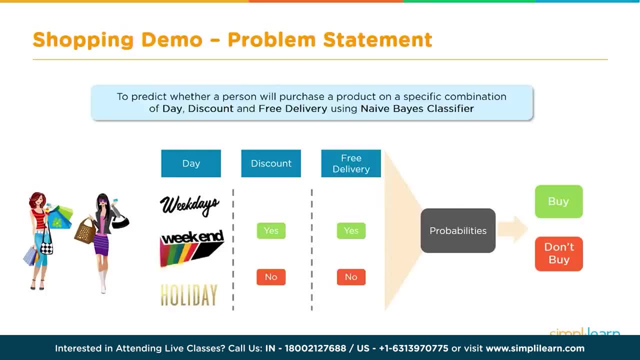 So, when you see data like this, it's necessary to move away from a 1D view of the data to a two-dimensional view of the data. So, when you see data like this, it's necessary to move away from a 1D view of the data to a two-dimensional view of the data. 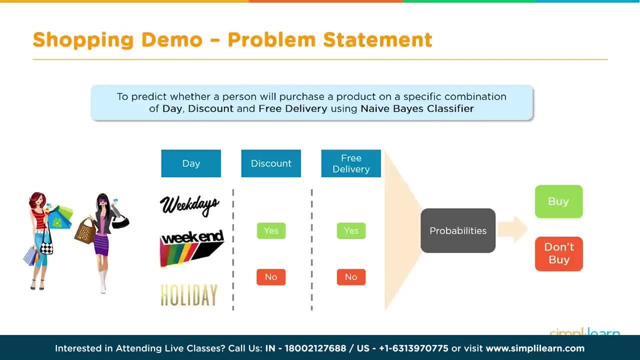 So, when you see data like this, it's necessary to move away from a 1D view of the data to a two-dimensional view of the data. So, when you see data like this, it's necessary to move away from a 1D view of the data to a two-dimensional view of the data. 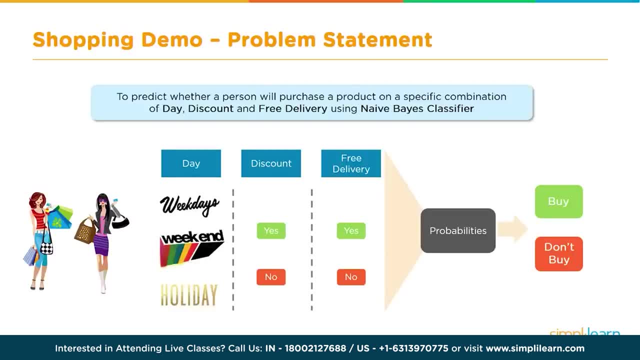 So, when you see data like this, it's necessary to move away from a 1D view of the data to a two-dimensional view of the data. So, when you see data like this, it's necessary to move away from a 1D view of the data to a two-dimensional view of the data. 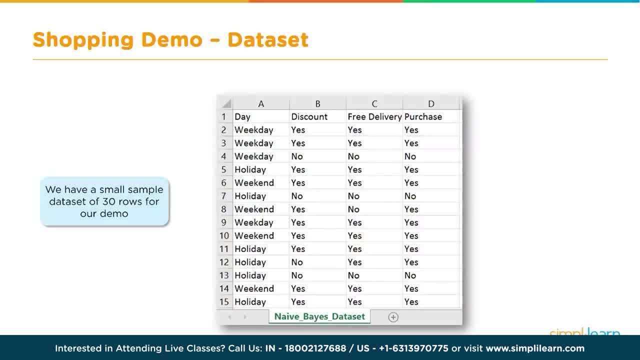 So, when you see data like this, it's necessary to move away from a 1D view of the data to a two-dimensional view of the data. So, when you see data like this, it's necessary to move away from a 1D view of the data to a two-dimensional view of the data. 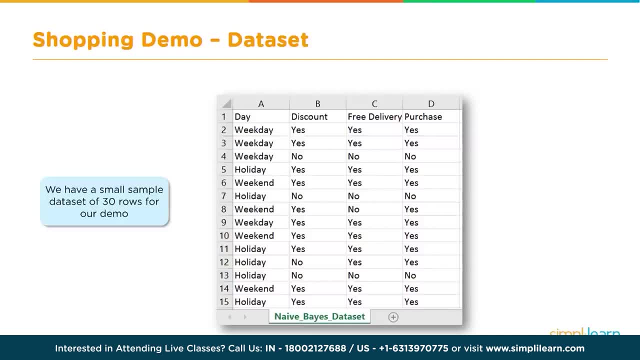 So, when you see data like this, it's necessary to move away from a 1D view of the data to a two-dimensional view of the data. So, when you see data like this, it's necessary to move away from a 1D view of the data to a two-dimensional view of the data. 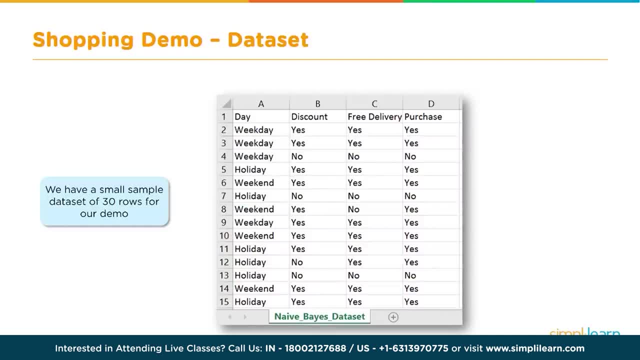 So, when you see data like this, it's necessary to move away from a 1D view of the data to a two-dimensional view of the data. So, when you see data like this, it's necessary to move away from a 1D view of the data to a two-dimensional view of the data. 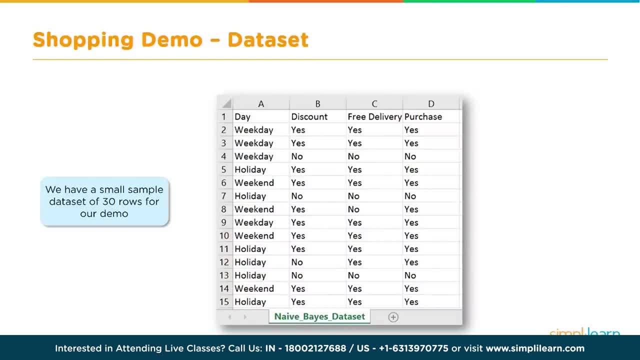 So, when you see data like this, it's necessary to move away from a 1D view of the data to a two-dimensional view of the data. So, when you see data like this, it's necessary to move away from a 1D view of the data to a two-dimensional view of the data. 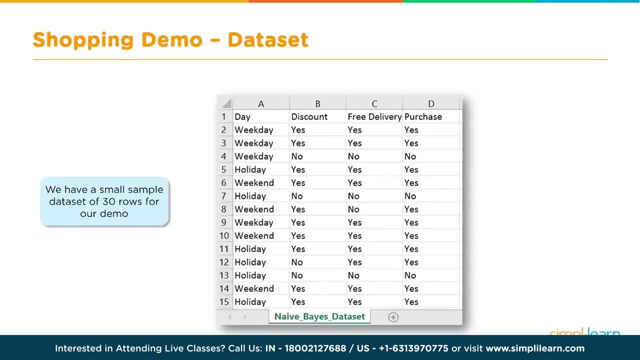 So, when you see data like this, it's necessary to move away from a 1D view of the data to a two-dimensional view of the data. So, when you see data like this, it's necessary to move away from a 1D view of the data to a two-dimensional view of the data. 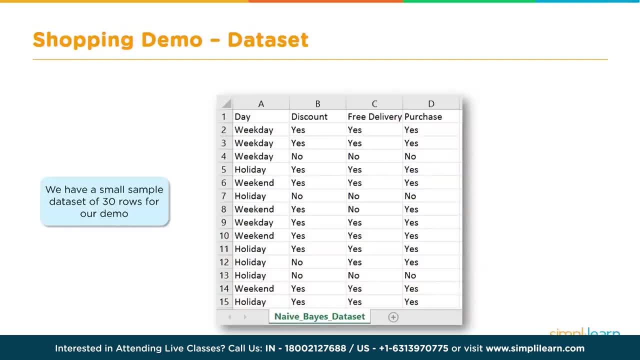 So, when you see data like this, it's necessary to move away from a 1D view of the data to a two-dimensional view of the data. So, when you see data like this, it's necessary to move away from a 1D view of the data to a two-dimensional view of the data. 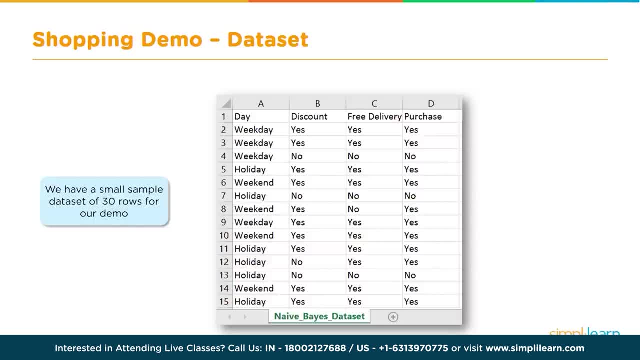 So, when you see data like this, it's necessary to move away from a 1D view of the data to a two-dimensional view of the data. So, when you see data like this, it's necessary to move away from a 1D view of the data to a two-dimensional view of the data. 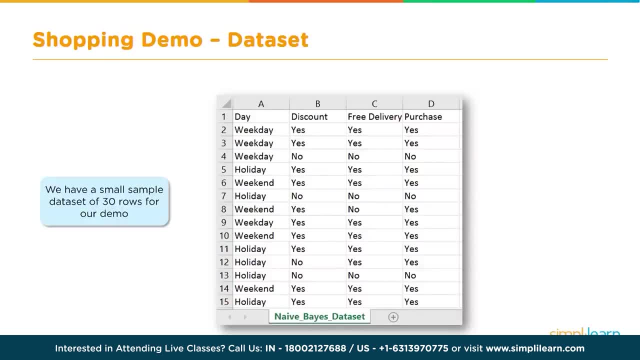 So, when you see data like this, it's necessary to move away from a 1D view of the data to a two-dimensional view of the data. So, when you see data like this, it's necessary to move away from a 1D view of the data to a two-dimensional view of the data. 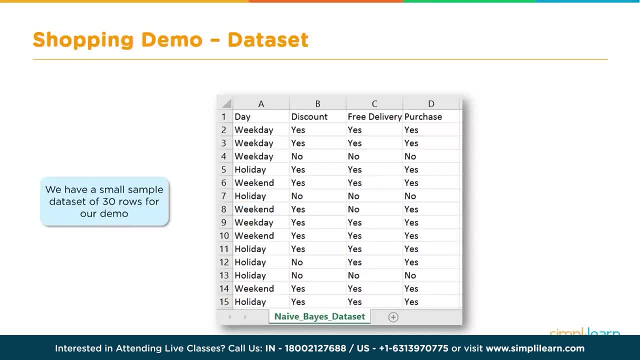 So, when you see data like this, it's necessary to move away from a 1D view of the data to a two-dimensional view of the data. So, when you see data like this, it's necessary to move away from a 1D view of the data to a two-dimensional view of the data. 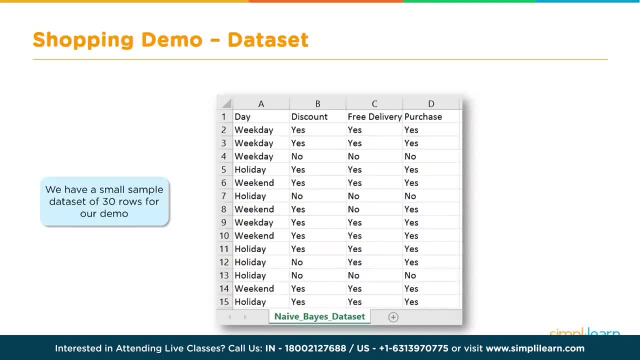 So, when you see data like this, it's necessary to move away from a 1D view of the data to a two-dimensional view of the data. So, when you see data like this, it's necessary to move away from a 1D view of the data to a two-dimensional view of the data. 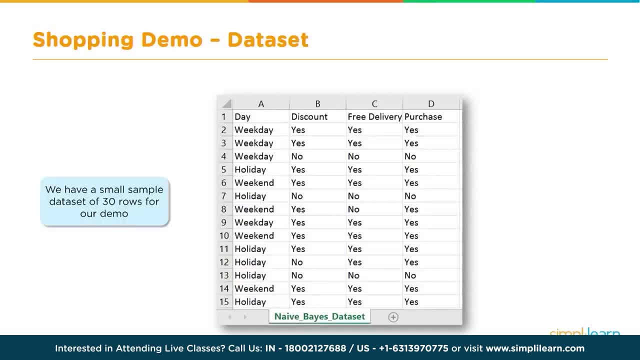 So, when you see data like this, it's necessary to move away from a 1D view of the data to a two-dimensional view of the data. So, when you see data like this, it's necessary to move away from a 1D view of the data to a two-dimensional view of the data. 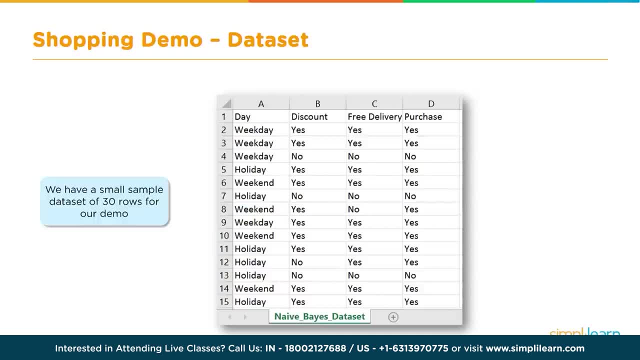 So, when you see data like this, it's necessary to move away from a 1D view of the data to a two-dimensional view of the data. So, when you see data like this, it's necessary to move away from a 1D view of the data to a two-dimensional view of the data. 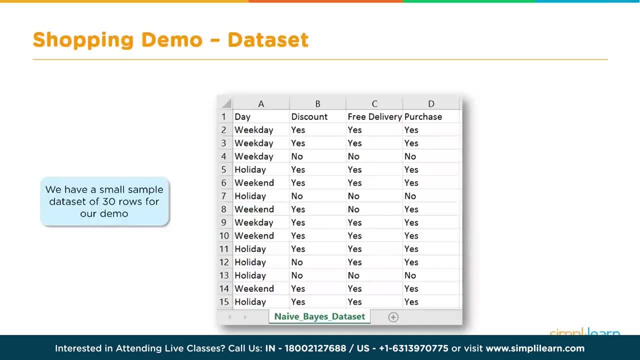 So, when you see data like this, it's necessary to move away from a 1D view of the data to a two-dimensional view of the data. So, when you see data like this, it's necessary to move away from a 1D view of the data to a two-dimensional view of the data. 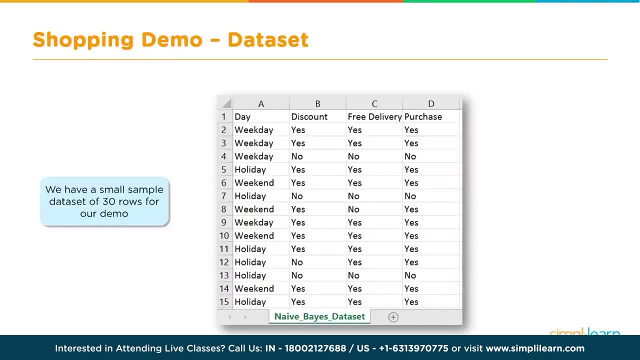 So, when you see data like this, it's necessary to move away from a 1D view of the data to a two-dimensional view of the data. So, when you see data like this, it's necessary to move away from a 1D view of the data to a two-dimensional view of the data. 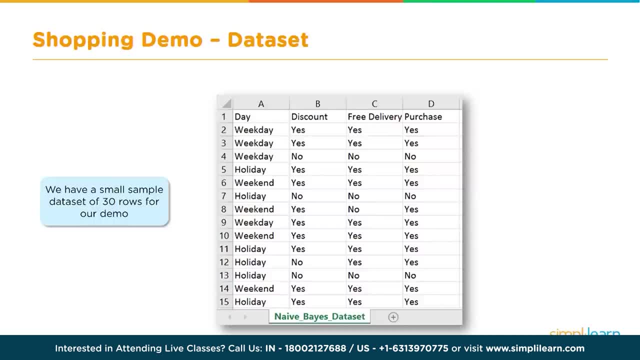 So, when you see data like this, it's necessary to move away from a 1D view of the data to a two-dimensional view of the data. So, when you see data like this, it's necessary to move away from a 1D view of the data to a two-dimensional view of the data. 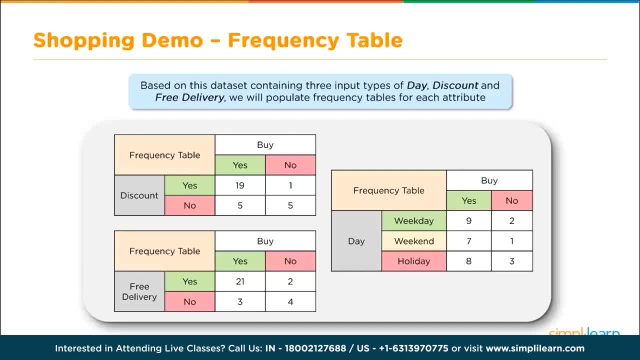 So, when you see data like this, it's necessary to move away from a 1D view of the data to a two-dimensional view of the data. So, when you see data like this, it's necessary to move away from a 1D view of the data to a two-dimensional view of the data. 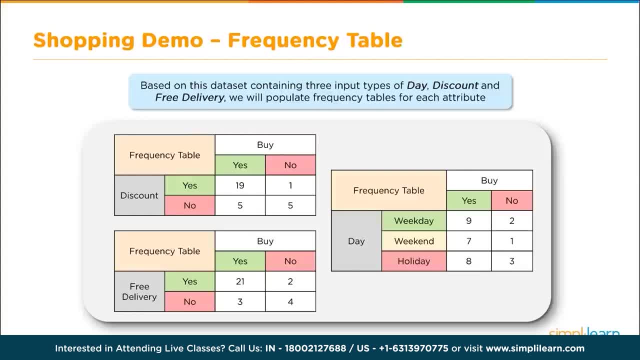 So, when you see data like this, it's necessary to move away from a 1D view of the data to a two-dimensional view of the data. So, when you see data like this, it's necessary to move away from a 1D view of the data to a two-dimensional view of the data. 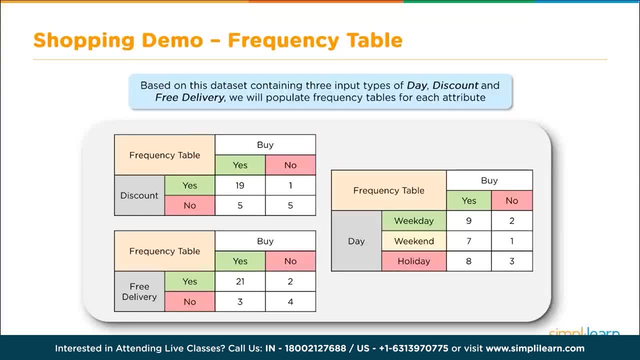 So, when you see data like this, it's necessary to move away from a 1D view of the data to a two-dimensional view of the data. So, when you see data like this, it's necessary to move away from a 1D view of the data to a two-dimensional view of the data. 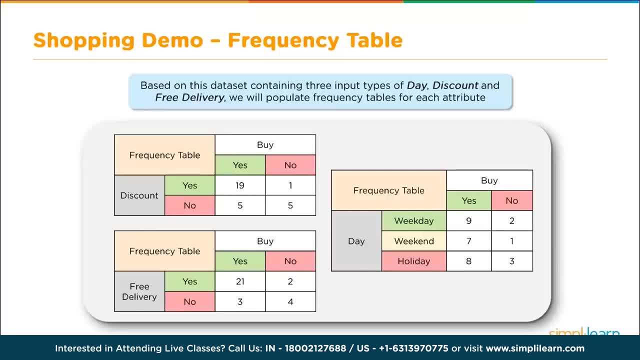 So, when you see data like this, it's necessary to move away from a 1D view of the data to a two-dimensional view of the data. So, when you see data like this, it's necessary to move away from a 1D view of the data to a two-dimensional view of the data. 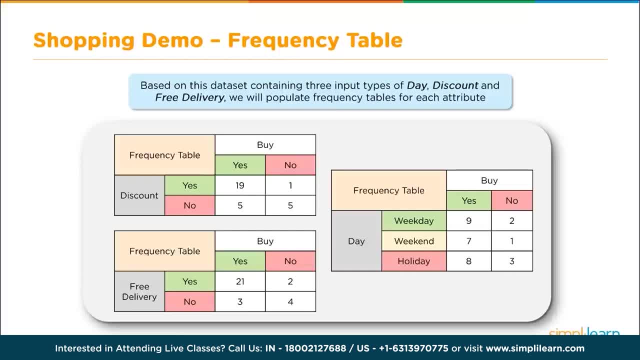 So, when you see data like this, it's necessary to move away from a 1D view of the data to a two-dimensional view of the data. So, when you see data like this, it's necessary to move away from a 1D view of the data to a two-dimensional view of the data. 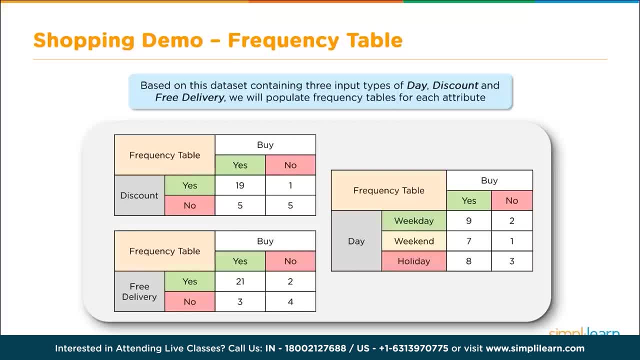 So, when you see data like this, it's necessary to move away from a 1D view of the data to a two-dimensional view of the data. So, when you see data like this, it's necessary to move away from a 1D view of the data to a two-dimensional view of the data. 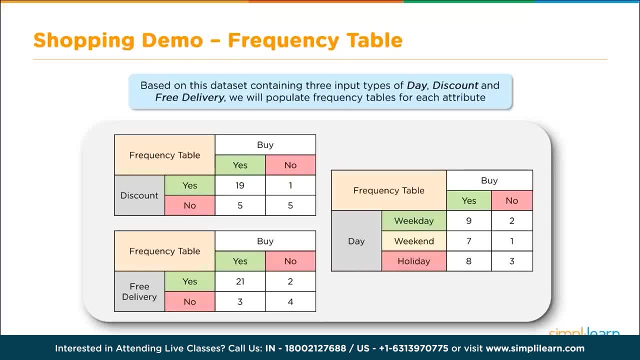 So, when you see data like this, it's necessary to move away from a 1D view of the data to a two-dimensional view of the data. So, when you see data like this, it's necessary to move away from a 1D view of the data to a two-dimensional view of the data. 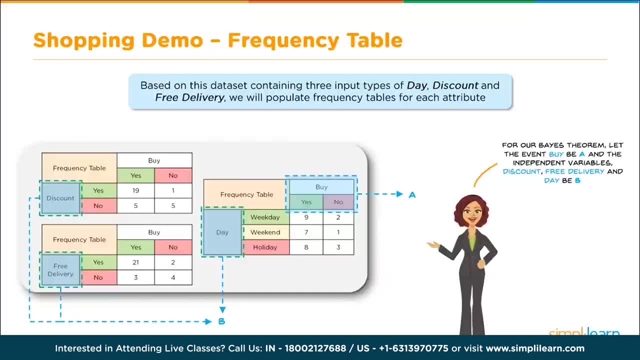 So, when you see data like this, it's necessary to move away from a 1D view of the data to a two-dimensional view of the data. So, when you see data like this, it's necessary to move away from a 1D view of the data to a two-dimensional view of the data. 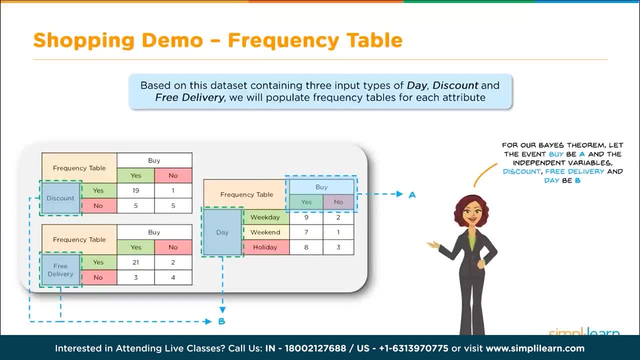 So, when you see data like this, it's necessary to move away from a 1D view of the data to a two-dimensional view of the data. So, when you see data like this, it's necessary to move away from a 1D view of the data to a two-dimensional view of the data. 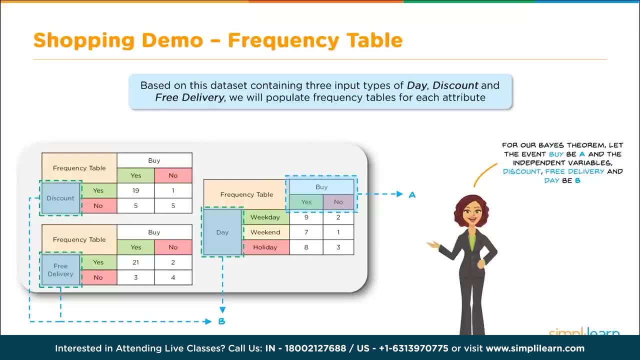 So, when you see data like this, it's necessary to move away from a 1D view of the data to a two-dimensional view of the data. So, when you see data like this, it's necessary to move away from a 1D view of the data to a two-dimensional view of the data. 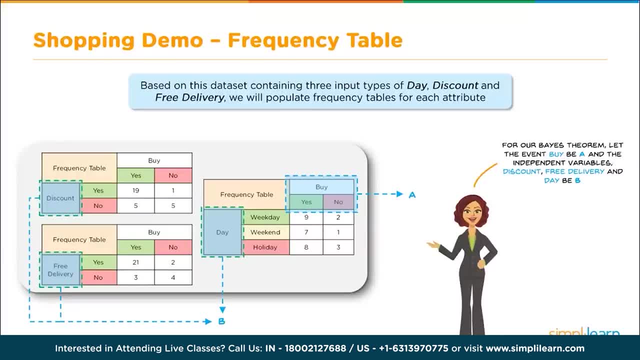 So, when you see data like this, it's necessary to move away from a 1D view of the data to a two-dimensional view of the data. So, when you see data like this, it's necessary to move away from a 1D view of the data to a two-dimensional view of the data. 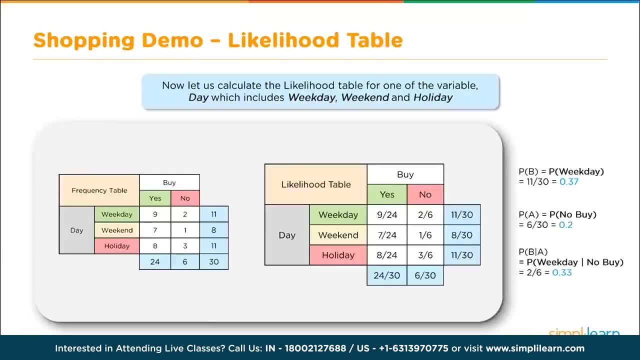 So, when you see data like this, it's necessary to move away from a 1D view of the data to a two-dimensional view of the data. So, when you see data like this, it's necessary to move away from a 1D view of the data to a two-dimensional view of the data. 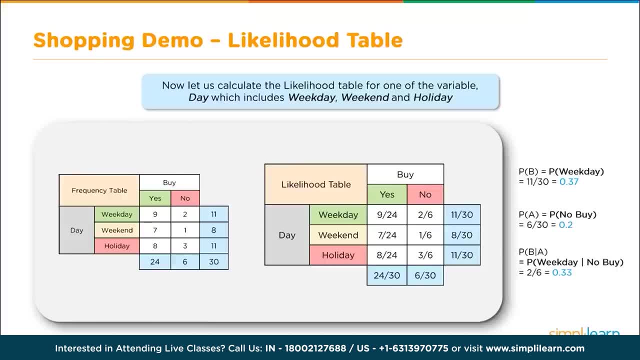 So, when you see data like this, it's necessary to move away from a 1D view of the data to a two-dimensional view of the data. So, when you see data like this, it's necessary to move away from a 1D view of the data to a two-dimensional view of the data. 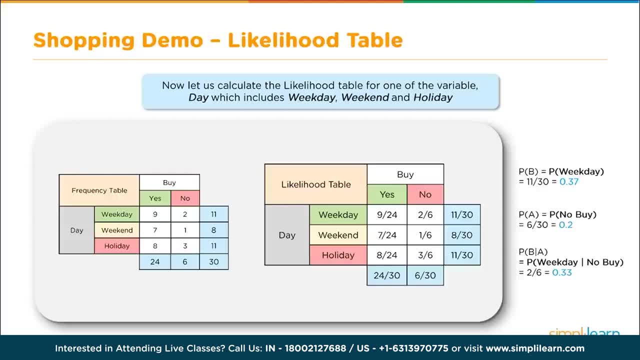 So, when you see data like this, it's necessary to move away from a 1D view of the data to a two-dimensional view of the data. So, when you see data like this, it's necessary to move away from a 1D view of the data to a two-dimensional view of the data. 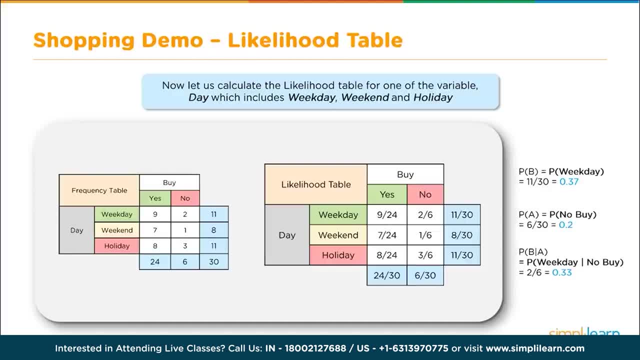 So, when you see data like this, it's necessary to move away from a 1D view of the data to a two-dimensional view of the data. So, when you see data like this, it's necessary to move away from a 1D view of the data to a two-dimensional view of the data. 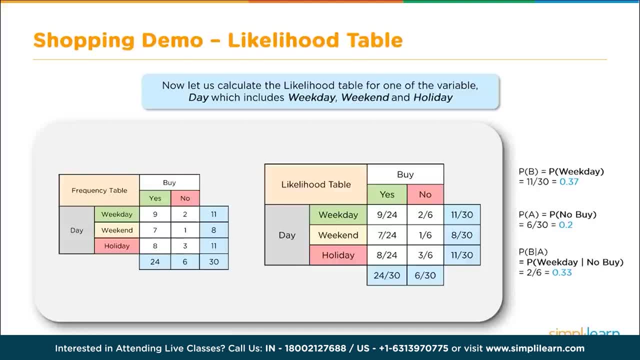 So, when you see data like this, it's necessary to move away from a 1D view of the data to a two-dimensional view of the data. So, when you see data like this, it's necessary to move away from a 1D view of the data to a two-dimensional view of the data. 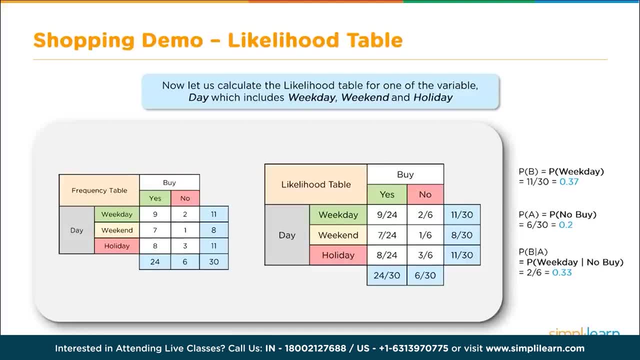 So, when you see data like this, it's necessary to move away from a 1D view of the data to a two-dimensional view of the data. So, when you see data like this, it's necessary to move away from a 1D view of the data to a two-dimensional view of the data. 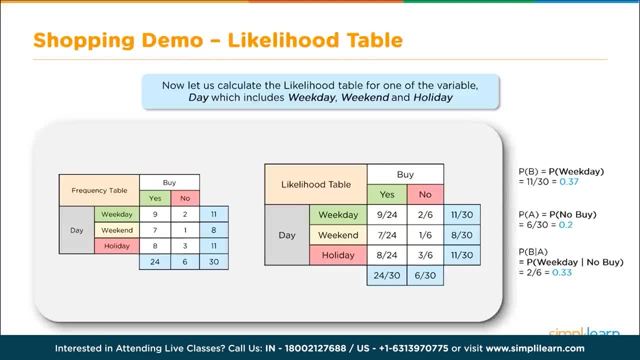 So, when you see data like this, it's necessary to move away from a 1D view of the data to a two-dimensional view of the data. So, when you see data like this, it's necessary to move away from a 1D view of the data to a two-dimensional view of the data. 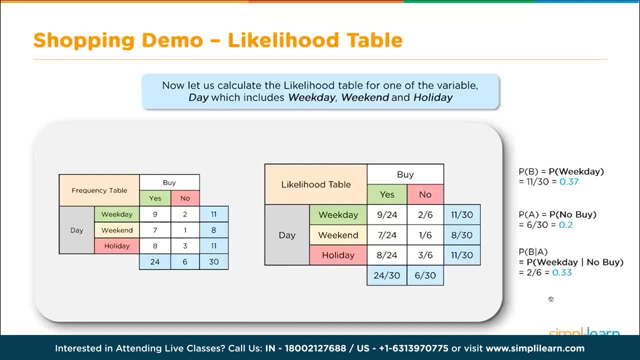 So, when you see data like this, it's necessary to move away from a 1D view of the data to a two-dimensional view of the data. So, when you see data like this, it's necessary to move away from a 1D view of the data to a two-dimensional view of the data. 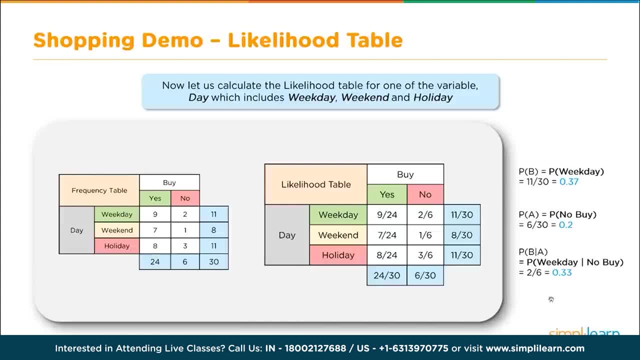 So, when you see data like this, it's necessary to move away from a 1D view of the data to a two-dimensional view of the data. So, when you see data like this, it's necessary to move away from a 1D view of the data to a two-dimensional view of the data. 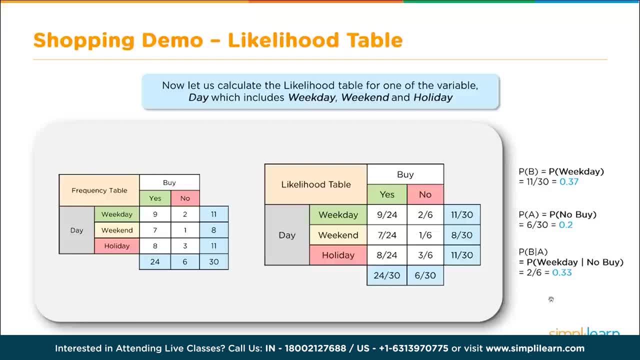 So, when you see data like this, it's necessary to move away from a 1D view of the data to a two-dimensional view of the data. So, when you see data like this, it's necessary to move away from a 1D view of the data to a two-dimensional view of the data. 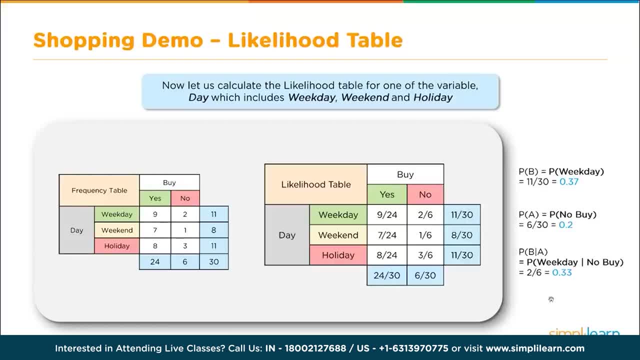 So, when you see data like this, it's necessary to move away from a 1D view of the data to a two-dimensional view of the data. So, when you see data like this, it's necessary to move away from a 1D view of the data to a two-dimensional view of the data. 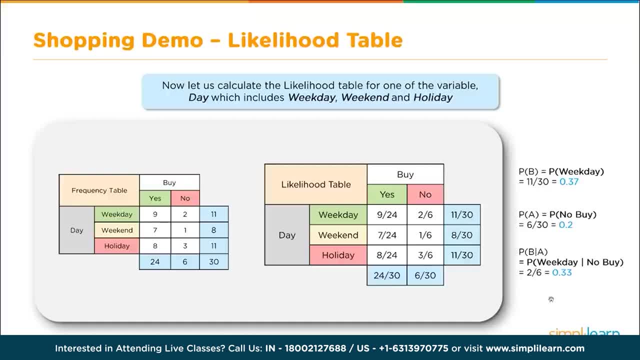 So, when you see data like this, it's necessary to move away from a 1D view of the data to a two-dimensional view of the data. So, when you see data like this, it's necessary to move away from a 1D view of the data to a two-dimensional view of the data. 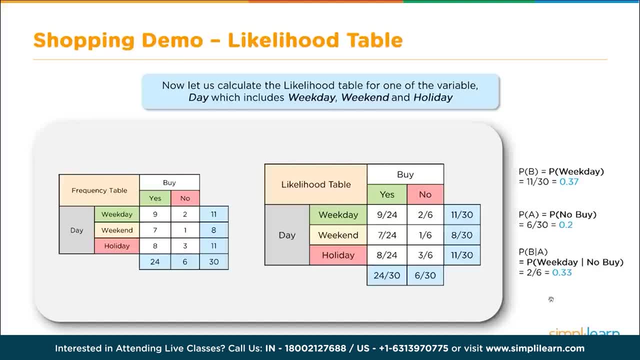 So, when you see data like this, it's necessary to move away from a 1D view of the data to a two-dimensional view of the data. So, when you see data like this, it's necessary to move away from a 1D view of the data to a two-dimensional view of the data. 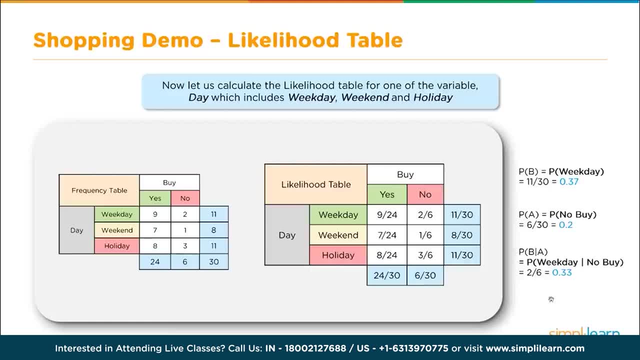 So, when you see data like this, it's necessary to move away from a 1D view of the data to a two-dimensional view of the data. So, when you see data like this, it's necessary to move away from a 1D view of the data to a two-dimensional view of the data. 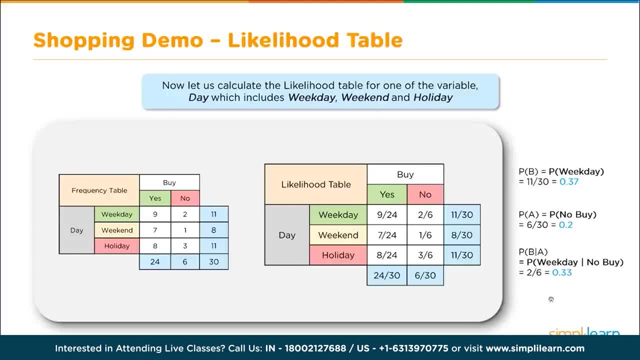 So, when you see data like this, it's necessary to move away from a 1D view of the data to a two-dimensional view of the data. So, when you see data like this, it's necessary to move away from a 1D view of the data to a two-dimensional view of the data. 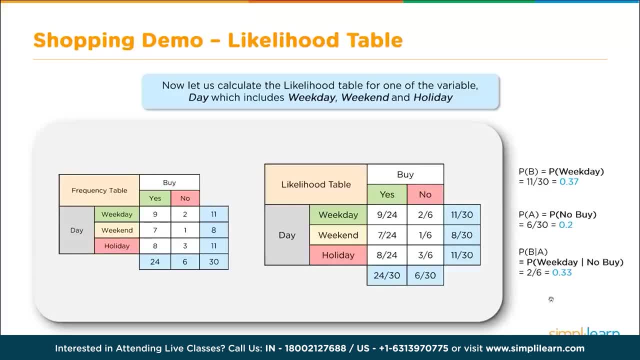 So, when you see data like this, it's necessary to move away from a 1D view of the data to a two-dimensional view of the data. So, when you see data like this, it's necessary to move away from a 1D view of the data to a two-dimensional view of the data. 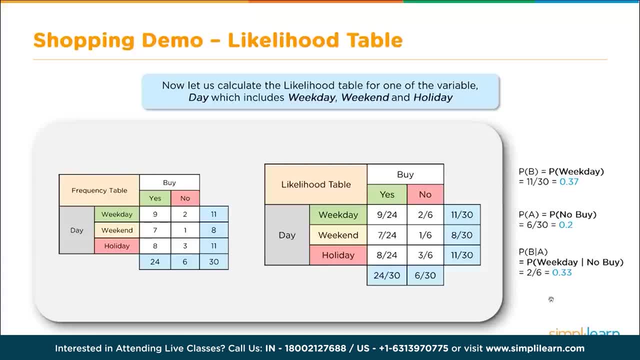 So, when you see data like this, it's necessary to move away from a 1D view of the data to a two-dimensional view of the data. So, when you see data like this, it's necessary to move away from a 1D view of the data to a two-dimensional view of the data. 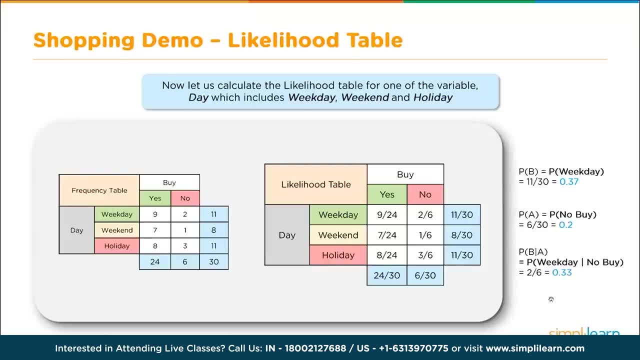 So, when you see data like this, it's necessary to move away from a 1D view of the data to a two-dimensional view of the data. So, when you see data like this, it's necessary to move away from a 1D view of the data to a two-dimensional view of the data. 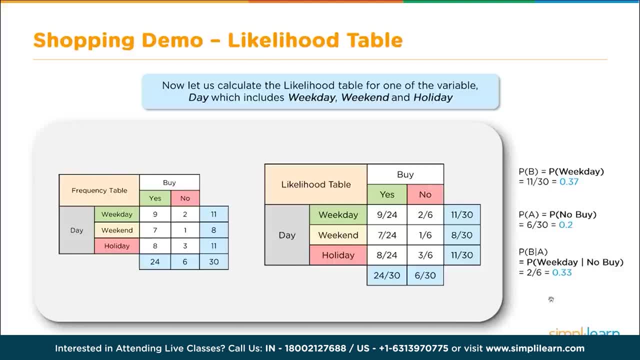 So, when you see data like this, it's necessary to move away from a 1D view of the data to a two-dimensional view of the data. So, when you see data like this, it's necessary to move away from a 1D view of the data to a two-dimensional view of the data. 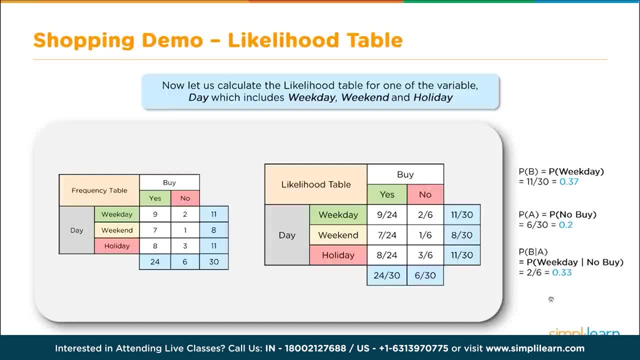 So, when you see data like this, it's necessary to move away from a 1D view of the data to a two-dimensional view of the data. So, when you see data like this, it's necessary to move away from a 1D view of the data to a two-dimensional view of the data. 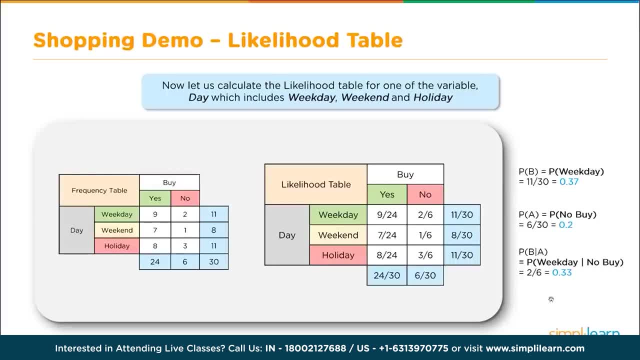 So, when you see data like this, it's necessary to move away from a 1D view of the data to a two-dimensional view of the data. So, when you see data like this, it's necessary to move away from a 1D view of the data to a two-dimensional view of the data. 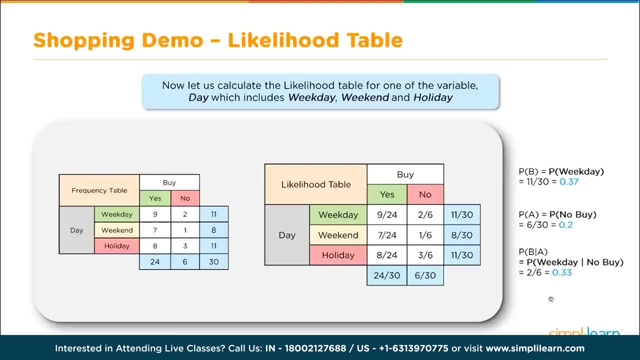 So, when you see data like this, it's necessary to move away from a 1D view of the data to a two-dimensional view of the data. So, when you see data like this, it's necessary to move away from a 1D view of the data to a two-dimensional view of the data. 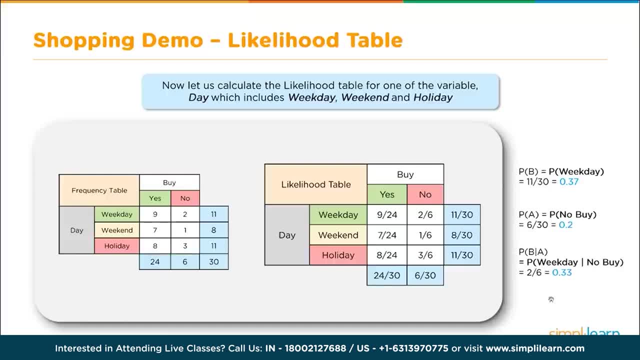 So, when you see data like this, it's necessary to move away from a 1D view of the data to a two-dimensional view of the data. So, when you see data like this, it's necessary to move away from a 1D view of the data to a two-dimensional view of the data. 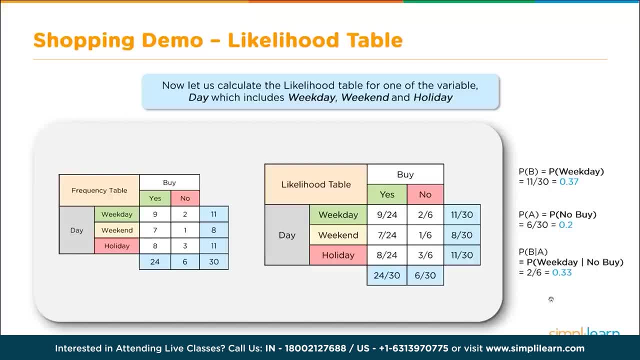 So, when you see data like this, it's necessary to move away from a 1D view of the data to a two-dimensional view of the data. So, when you see data like this, it's necessary to move away from a 1D view of the data to a two-dimensional view of the data. 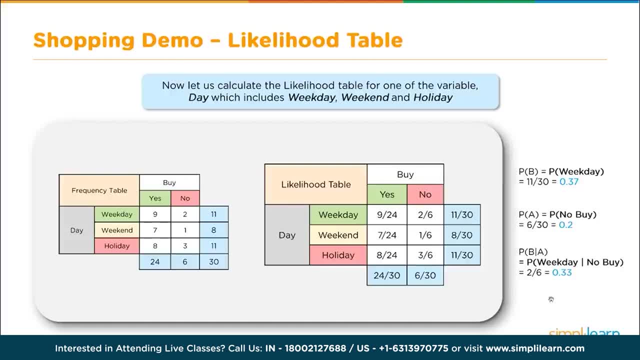 So, when you see data like this, it's necessary to move away from a 1D view of the data to a two-dimensional view of the data. So, when you see data like this, it's necessary to move away from a 1D view of the data to a two-dimensional view of the data. 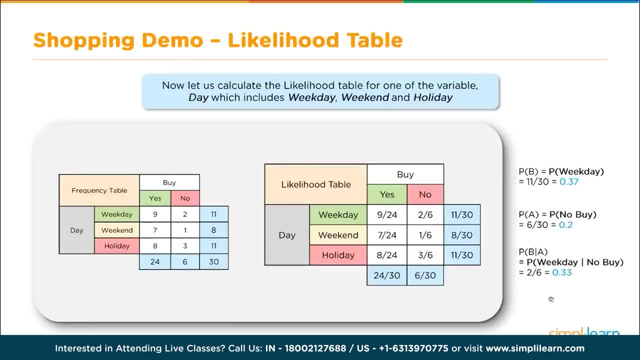 So, when you see data like this, it's necessary to move away from a 1D view of the data to a two-dimensional view of the data. So, when you see data like this, it's necessary to move away from a 1D view of the data to a two-dimensional view of the data. 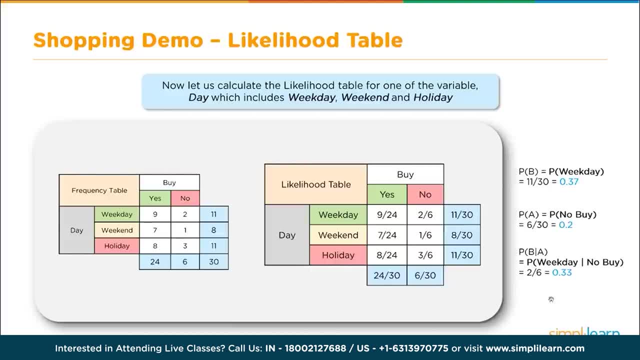 So, when you see data like this, it's necessary to move away from a 1D view of the data to a two-dimensional view of the data. So, when you see data like this, it's necessary to move away from a 1D view of the data to a two-dimensional view of the data. 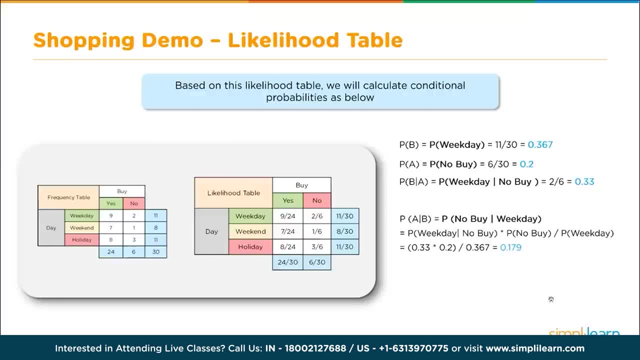 So, when you see data like this, it's necessary to move away from a 1D view of the data to a two-dimensional view of the data. So, when you see data like this, it's necessary to move away from a 1D view of the data to a two-dimensional view of the data. 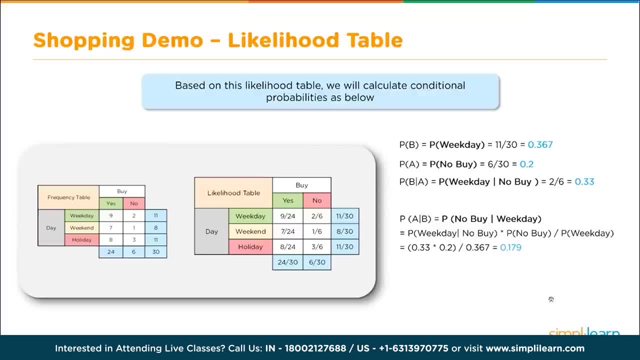 So, when you see data like this, it's necessary to move away from a 1D view of the data to a two-dimensional view of the data. So, when you see data like this, it's necessary to move away from a 1D view of the data to a two-dimensional view of the data. 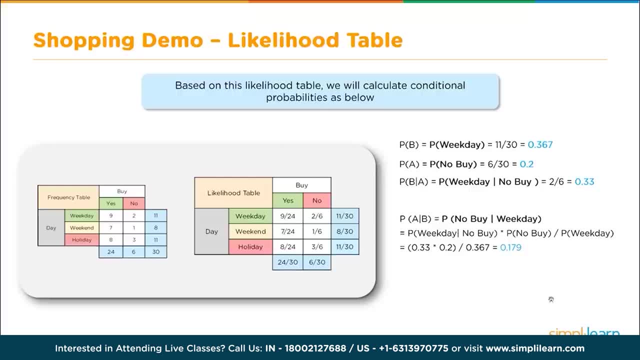 So, when you see data like this, it's necessary to move away from a 1D view of the data to a two-dimensional view of the data. So, when you see data like this, it's necessary to move away from a 1D view of the data to a two-dimensional view of the data. 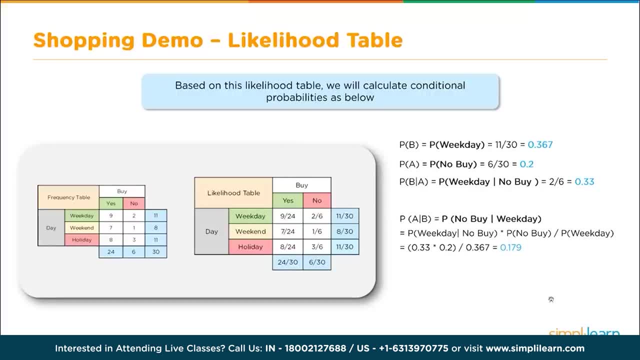 So, when you see data like this, it's necessary to move away from a 1D view of the data to a two-dimensional view of the data. So, when you see data like this, it's necessary to move away from a 1D view of the data to a two-dimensional view of the data. 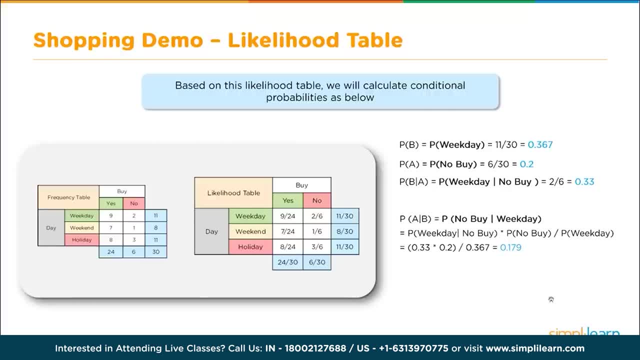 So, when you see data like this, it's necessary to move away from a 1D view of the data to a two-dimensional view of the data. So, when you see data like this, it's necessary to move away from a 1D view of the data to a two-dimensional view of the data. 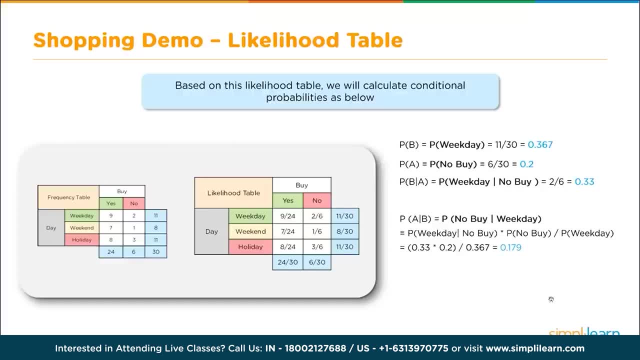 So, when you see data like this, it's necessary to move away from a 1D view of the data to a two-dimensional view of the data. So, when you see data like this, it's necessary to move away from a 1D view of the data to a two-dimensional view of the data. 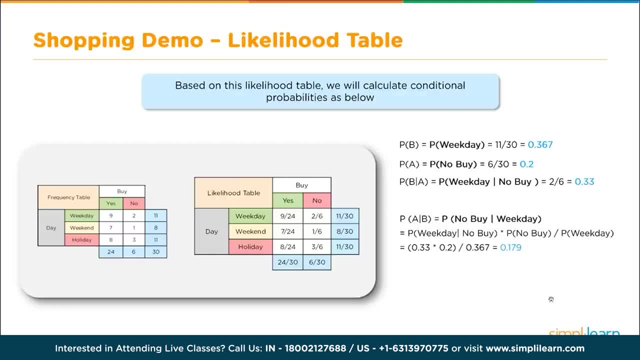 So, when you see data like this, it's necessary to move away from a 1D view of the data to a two-dimensional view of the data. So, when you see data like this, it's necessary to move away from a 1D view of the data to a two-dimensional view of the data. 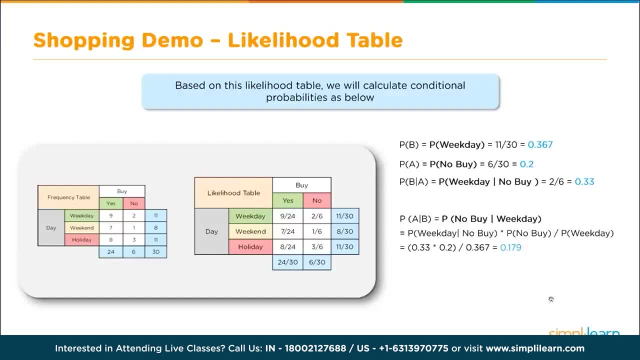 So, when you see data like this, it's necessary to move away from a 1D view of the data to a two-dimensional view of the data. So, when you see data like this, it's necessary to move away from a 1D view of the data to a two-dimensional view of the data. 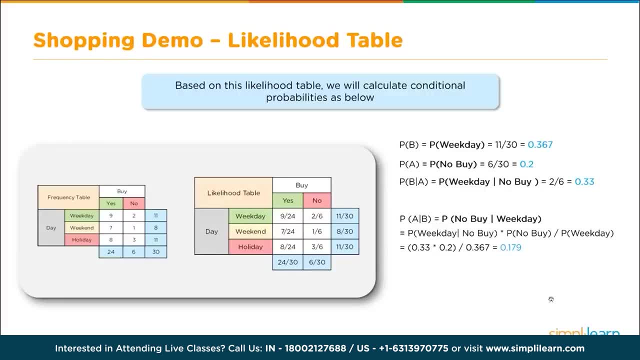 So, when you see data like this, it's necessary to move away from a 1D view of the data to a two-dimensional view of the data. So, when you see data like this, it's necessary to move away from a 1D view of the data to a two-dimensional view of the data. 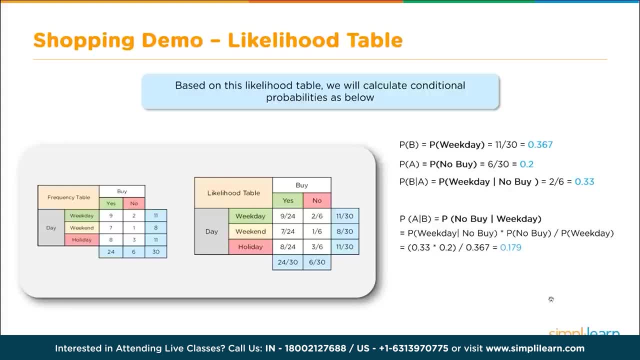 So, when you see data like this, it's necessary to move away from a 1D view of the data to a two-dimensional view of the data. So, when you see data like this, it's necessary to move away from a 1D view of the data to a two-dimensional view of the data. 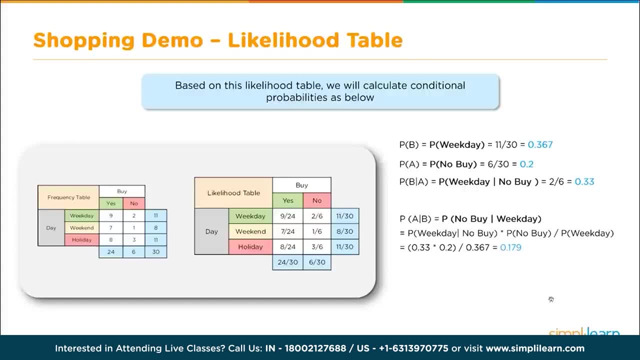 So, when you see data like this, it's necessary to move away from a 1D view of the data to a two-dimensional view of the data. So, when you see data like this, it's necessary to move away from a 1D view of the data to a two-dimensional view of the data. 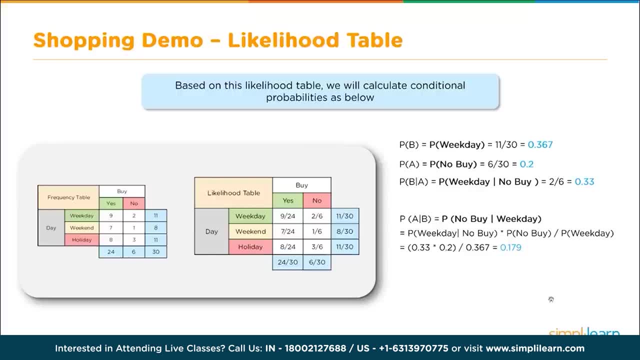 So, when you see data like this, it's necessary to move away from a 1D view of the data to a two-dimensional view of the data. So, when you see data like this, it's necessary to move away from a 1D view of the data to a two-dimensional view of the data. 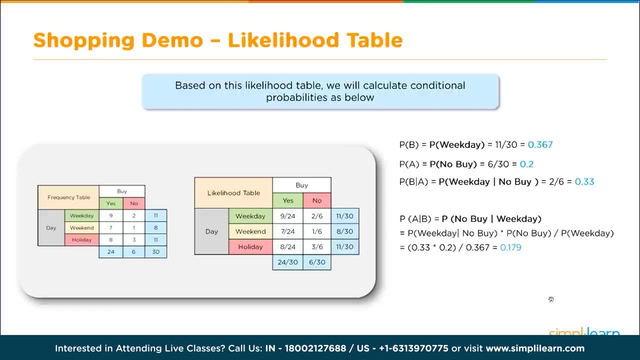 So, when you see data like this, it's necessary to move away from a 1D view of the data to a two-dimensional view of the data. So, when you see data like this, it's necessary to move away from a 1D view of the data to a two-dimensional view of the data. 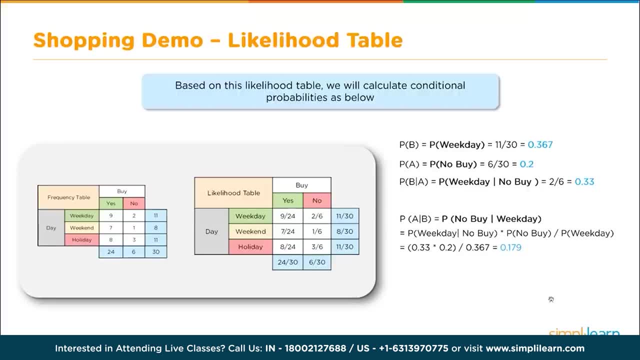 So, when you see data like this, it's necessary to move away from a 1D view of the data to a two-dimensional view of the data. So, when you see data like this, it's necessary to move away from a 1D view of the data to a two-dimensional view of the data. 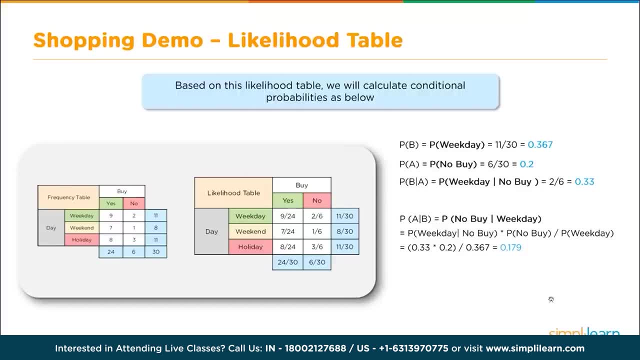 So, when you see data like this, it's necessary to move away from a 1D view of the data to a two-dimensional view of the data. So, when you see data like this, it's necessary to move away from a 1D view of the data to a two-dimensional view of the data. 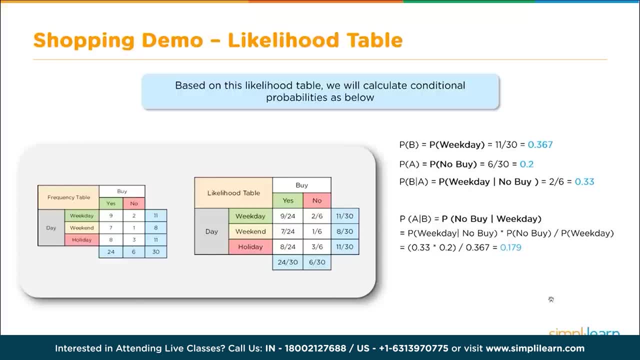 So, when you see data like this, it's necessary to move away from a 1D view of the data to a two-dimensional view of the data. So, when you see data like this, it's necessary to move away from a 1D view of the data to a two-dimensional view of the data. 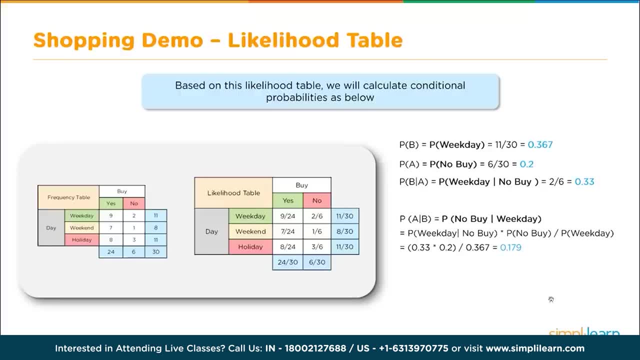 So, when you see data like this, it's necessary to move away from a 1D view of the data to a two-dimensional view of the data. So, when you see data like this, it's necessary to move away from a 1D view of the data to a two-dimensional view of the data. 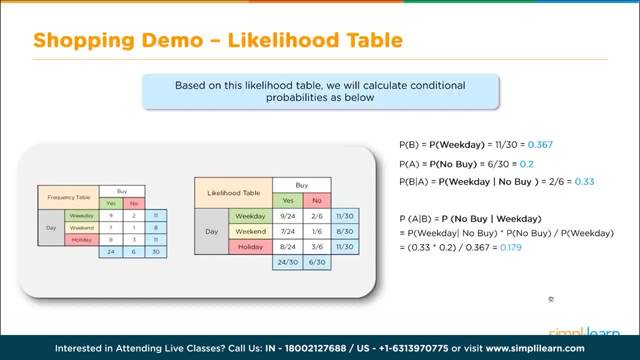 So, when you see data like this, it's necessary to move away from a 1D view of the data to a two-dimensional view of the data. So, when you see data like this, it's necessary to move away from a 1D view of the data to a two-dimensional view of the data. 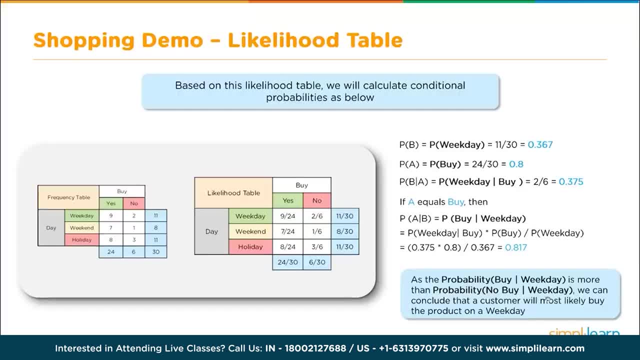 So, when you see data like this, it's necessary to move away from a 1D view of the data to a two-dimensional view of the data. So, when you see data like this, it's necessary to move away from a 1D view of the data to a two-dimensional view of the data. 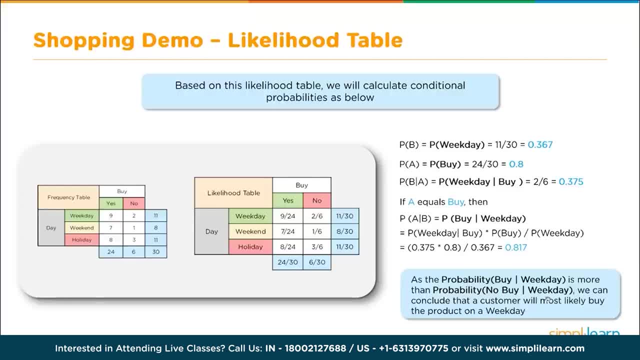 So, when you see data like this, it's necessary to move away from a 1D view of the data to a two-dimensional view of the data. So, when you see data like this, it's necessary to move away from a 1D view of the data to a two-dimensional view of the data. 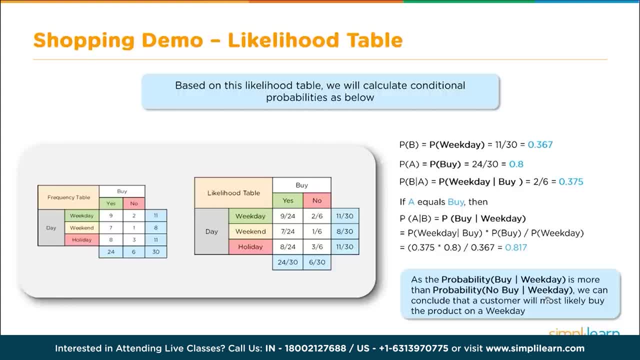 So, when you see data like this, it's necessary to move away from a 1D view of the data to a two-dimensional view of the data. So, when you see data like this, it's necessary to move away from a 1D view of the data to a two-dimensional view of the data. 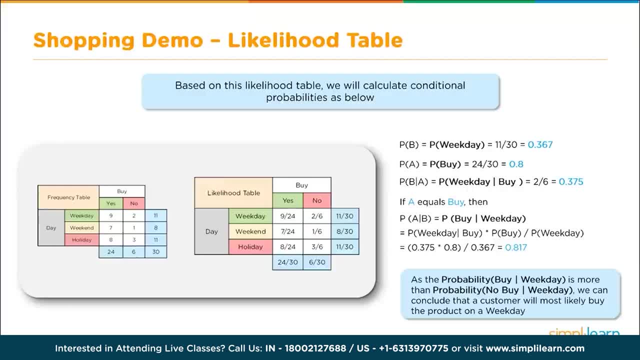 So, when you see data like this, it's necessary to move away from a 1D view of the data to a two-dimensional view of the data. So, when you see data like this, it's necessary to move away from a 1D view of the data to a two-dimensional view of the data. 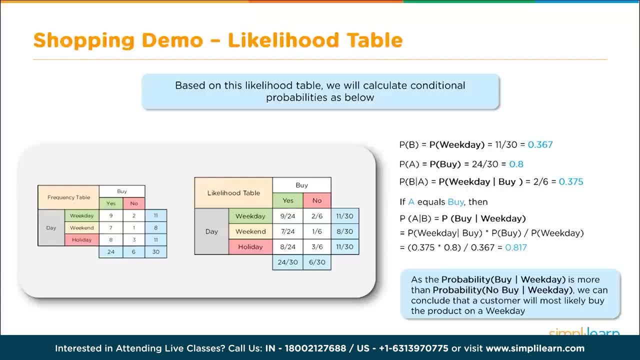 So, when you see data like this, it's necessary to move away from a 1D view of the data to a two-dimensional view of the data. So, when you see data like this, it's necessary to move away from a 1D view of the data to a two-dimensional view of the data. 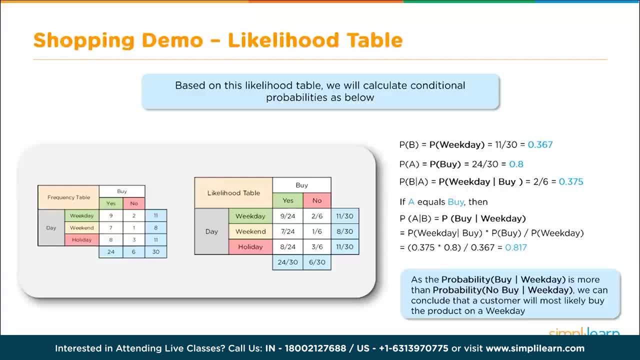 So, when you see data like this, it's necessary to move away from a 1D view of the data to a two-dimensional view of the data. So, when you see data like this, it's necessary to move away from a 1D view of the data to a two-dimensional view of the data. 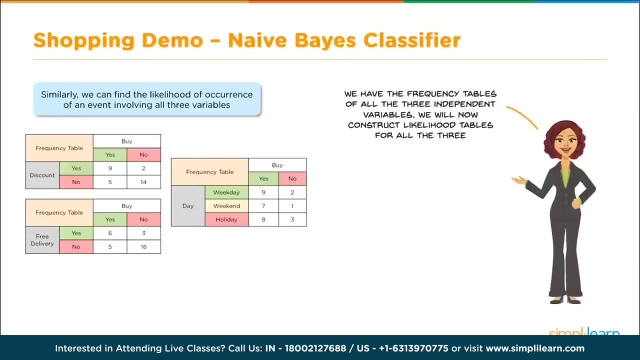 So, when you see data like this, it's necessary to move away from a 1D view of the data to a two-dimensional view of the data. So, when you see data like this, it's necessary to move away from a 1D view of the data to a two-dimensional view of the data. 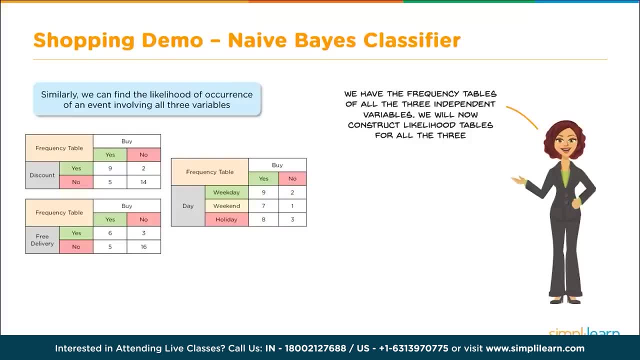 So, when you see data like this, it's necessary to move away from a 1D view of the data to a two-dimensional view of the data. So, when you see data like this, it's necessary to move away from a 1D view of the data to a two-dimensional view of the data. 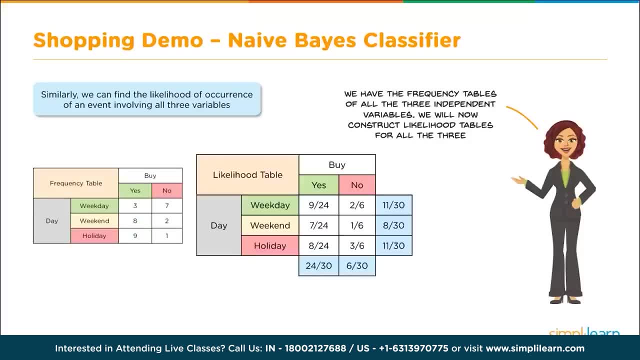 So, when you see data like this, it's necessary to move away from a 1D view of the data to a two-dimensional view of the data. So, when you see data like this, it's necessary to move away from a 1D view of the data to a two-dimensional view of the data. 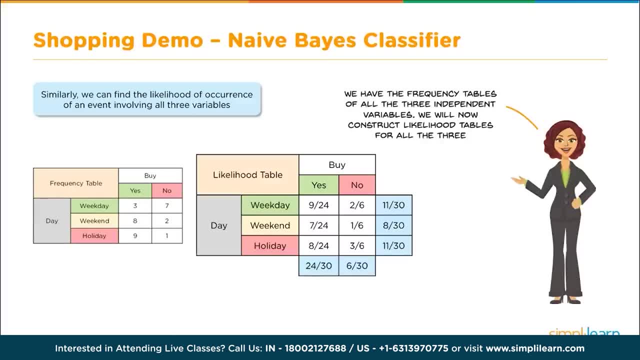 So, when you see data like this, it's necessary to move away from a 1D view of the data to a two-dimensional view of the data. So, when you see data like this, it's necessary to move away from a 1D view of the data to a two-dimensional view of the data. 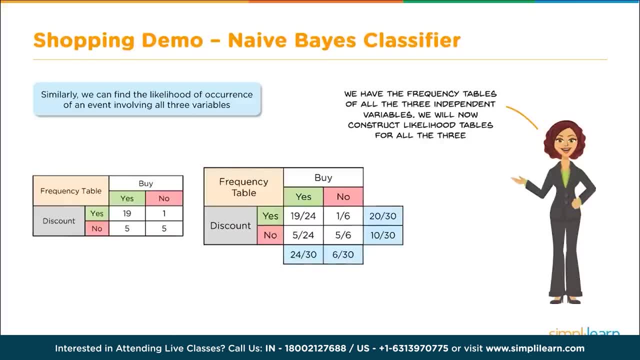 So, when you see data like this, it's necessary to move away from a 1D view of the data to a two-dimensional view of the data. So, when you see data like this, it's necessary to move away from a 1D view of the data to a two-dimensional view of the data. 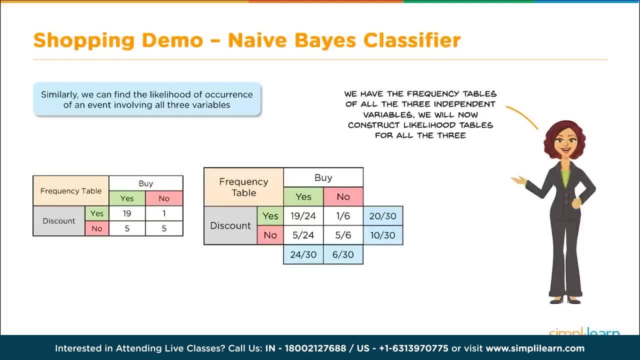 So, when you see data like this, it's necessary to move away from a 1D view of the data to a two-dimensional view of the data. So, when you see data like this, it's necessary to move away from a 1D view of the data to a two-dimensional view of the data. 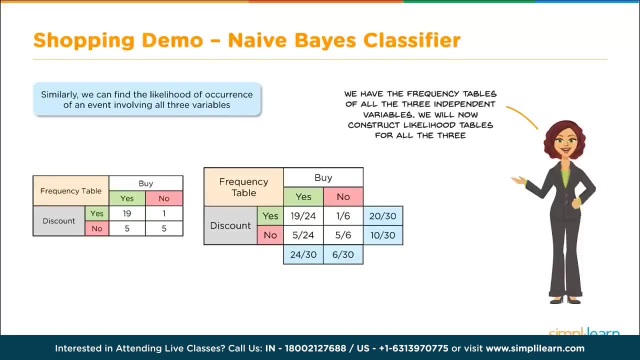 So, when you see data like this, it's necessary to move away from a 1D view of the data to a two-dimensional view of the data. So, when you see data like this, it's necessary to move away from a 1D view of the data to a two-dimensional view of the data. 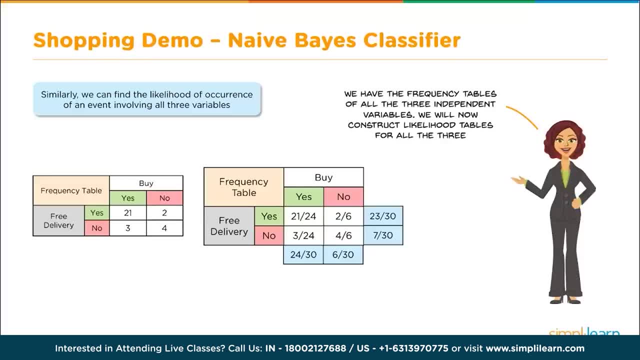 So, when you see data like this, it's necessary to move away from a 1D view of the data to a two-dimensional view of the data. So, when you see data like this, it's necessary to move away from a 1D view of the data to a two-dimensional view of the data. 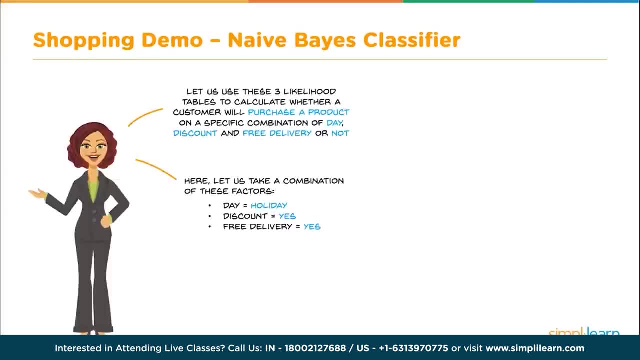 So, when you see data like this, it's necessary to move away from a 1D view of the data to a two-dimensional view of the data. So, when you see data like this, it's necessary to move away from a 1D view of the data to a two-dimensional view of the data. 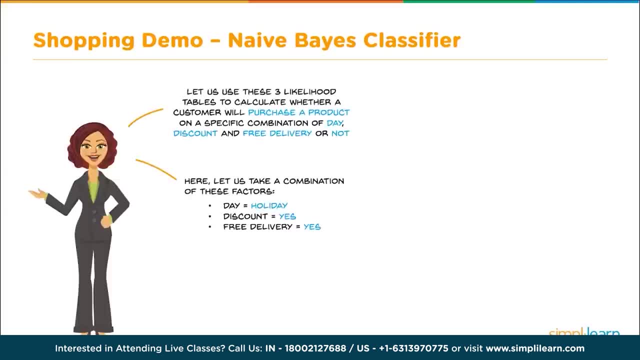 So, when you see data like this, it's necessary to move away from a 1D view of the data to a two-dimensional view of the data. So, when you see data like this, it's necessary to move away from a 1D view of the data to a two-dimensional view of the data. 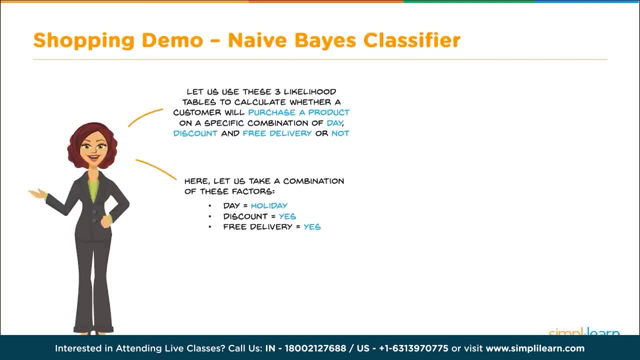 So, when you see data like this, it's necessary to move away from a 1D view of the data to a two-dimensional view of the data. So, when you see data like this, it's necessary to move away from a 1D view of the data to a two-dimensional view of the data. 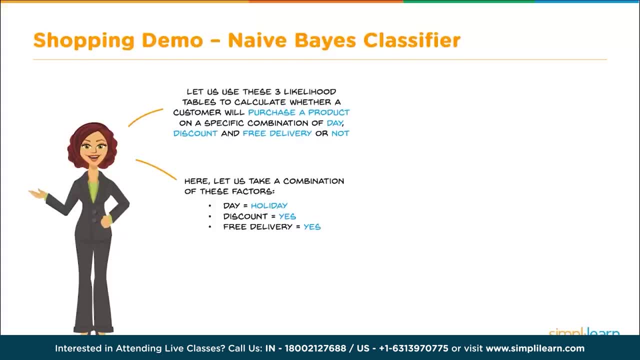 So, when you see data like this, it's necessary to move away from a 1D view of the data to a two-dimensional view of the data. So, when you see data like this, it's necessary to move away from a 1D view of the data to a two-dimensional view of the data. 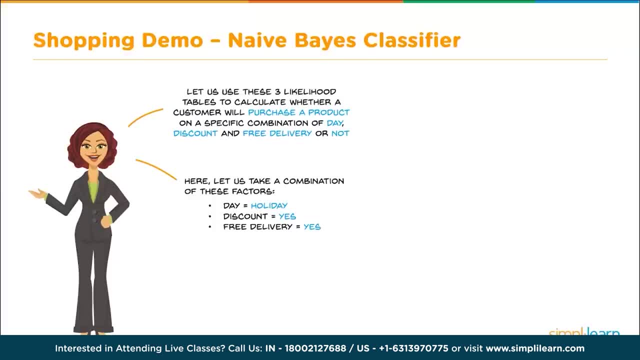 So, when you see data like this, it's necessary to move away from a 1D view of the data to a two-dimensional view of the data. So, when you see data like this, it's necessary to move away from a 1D view of the data to a two-dimensional view of the data. 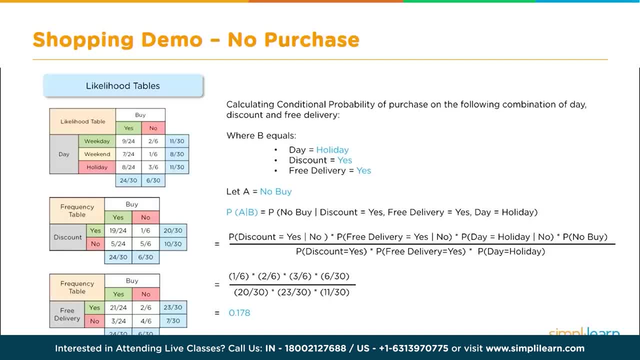 So, when you see data like this, it's necessary to move away from a 1D view of the data to a two-dimensional view of the data. So, when you see data like this, it's necessary to move away from a 1D view of the data to a two-dimensional view of the data. 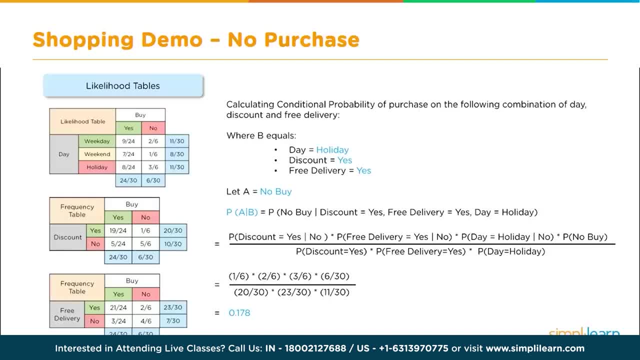 So, when you see data like this, it's necessary to move away from a 1D view of the data to a two-dimensional view of the data. So, when you see data like this, it's necessary to move away from a 1D view of the data to a two-dimensional view of the data. 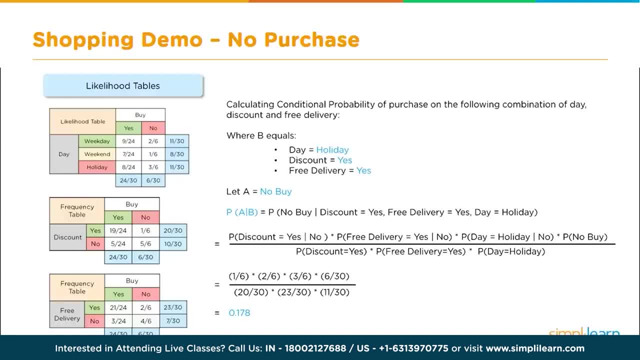 So, when you see data like this, it's necessary to move away from a 1D view of the data to a two-dimensional view of the data. So, when you see data like this, it's necessary to move away from a 1D view of the data to a two-dimensional view of the data. 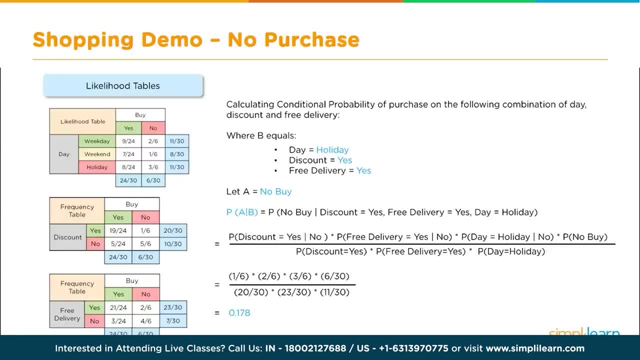 So, when you see data like this, it's necessary to move away from a 1D view of the data to a two-dimensional view of the data. So, when you see data like this, it's necessary to move away from a 1D view of the data to a two-dimensional view of the data. 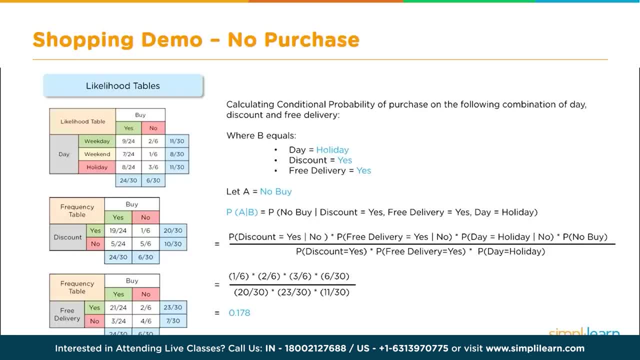 So, when you see data like this, it's necessary to move away from a 1D view of the data to a two-dimensional view of the data. So, when you see data like this, it's necessary to move away from a 1D view of the data to a two-dimensional view of the data. 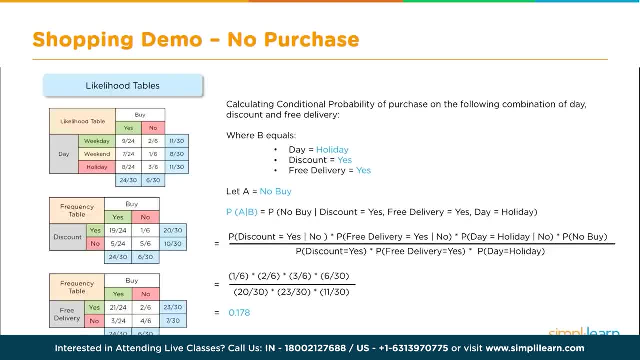 So, when you see data like this, it's necessary to move away from a 1D view of the data to a two-dimensional view of the data. So, when you see data like this, it's necessary to move away from a 1D view of the data to a two-dimensional view of the data. 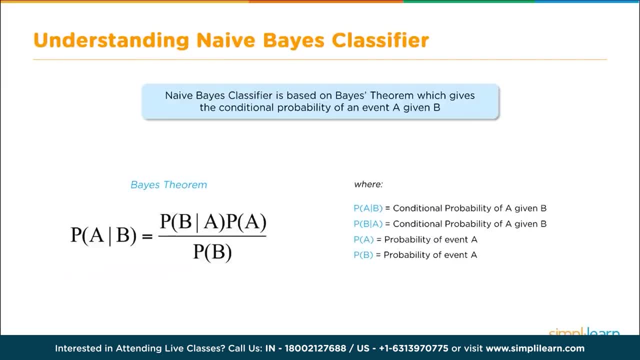 So, when you see data like this, it's necessary to move away from a 1D view of the data to a two-dimensional view of the data. So, when you see data like this, it's necessary to move away from a 1D view of the data to a two-dimensional view of the data. 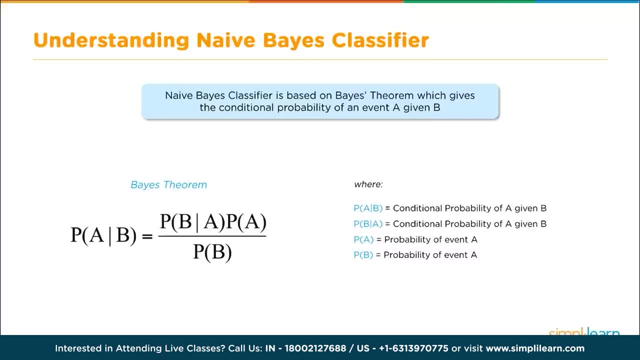 So, when you see data like this, it's necessary to move away from a 1D view of the data to a two-dimensional view of the data. So, when you see data like this, it's necessary to move away from a 1D view of the data to a two-dimensional view of the data. 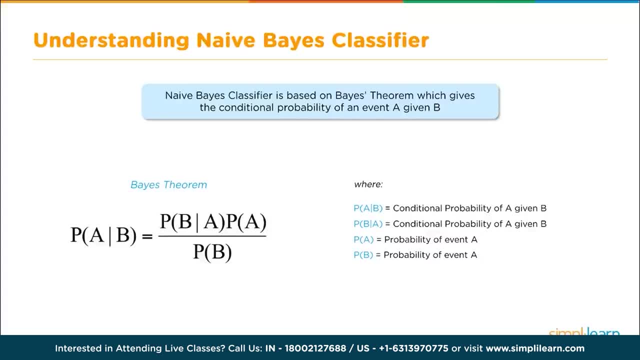 So, when you see data like this, it's necessary to move away from a 1D view of the data to a two-dimensional view of the data. So, when you see data like this, it's necessary to move away from a 1D view of the data to a two-dimensional view of the data. 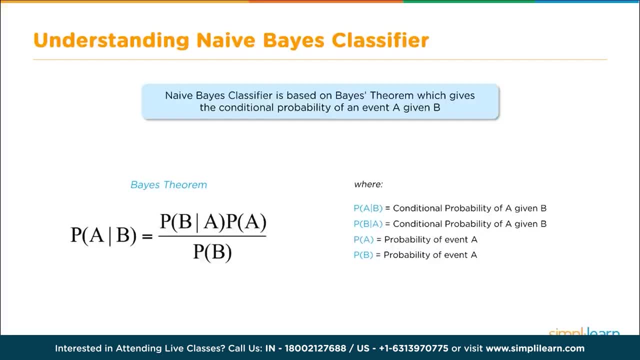 So, when you see data like this, it's necessary to move away from a 1D view of the data to a two-dimensional view of the data. So, when you see data like this, it's necessary to move away from a 1D view of the data to a two-dimensional view of the data. 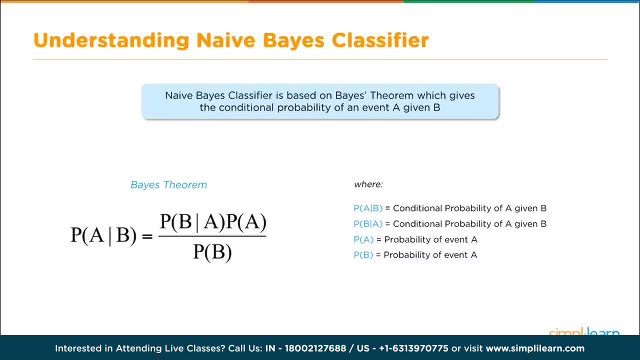 So, when you see data like this, it's necessary to move away from a 1D view of the data to a two-dimensional view of the data. So, when you see data like this, it's necessary to move away from a 1D view of the data to a two-dimensional view of the data. 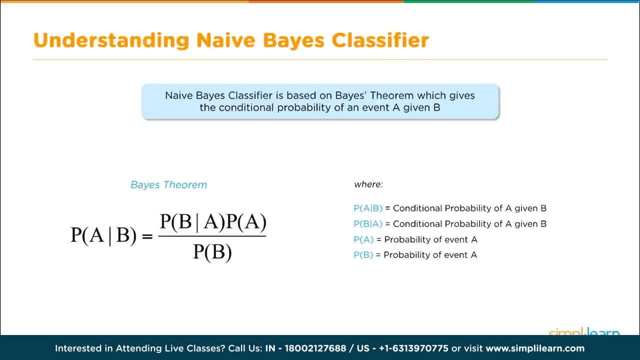 So, when you see data like this, it's necessary to move away from a 1D view of the data to a two-dimensional view of the data. So, when you see data like this, it's necessary to move away from a 1D view of the data to a two-dimensional view of the data. 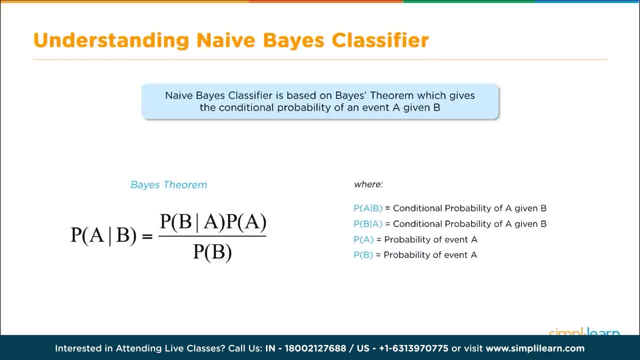 So, when you see data like this, it's necessary to move away from a 1D view of the data to a two-dimensional view of the data. So, when you see data like this, it's necessary to move away from a 1D view of the data to a two-dimensional view of the data. 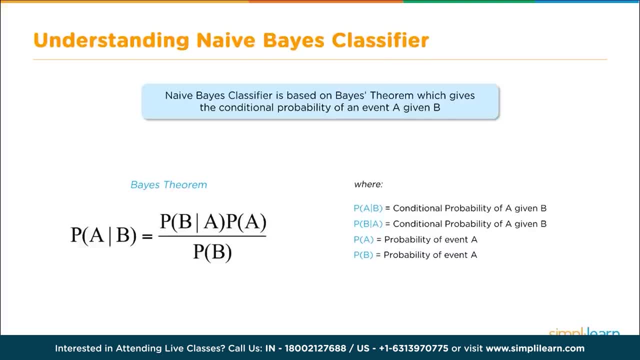 So, when you see data like this, it's necessary to move away from a 1D view of the data to a two-dimensional view of the data. So, when you see data like this, it's necessary to move away from a 1D view of the data to a two-dimensional view of the data. 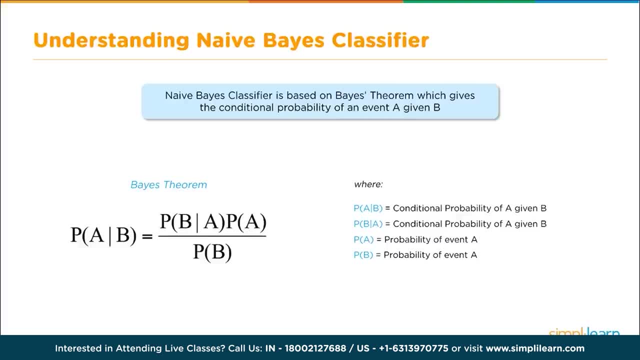 So, when you see data like this, it's necessary to move away from a 1D view of the data to a two-dimensional view of the data. So, when you see data like this, it's necessary to move away from a 1D view of the data to a two-dimensional view of the data. 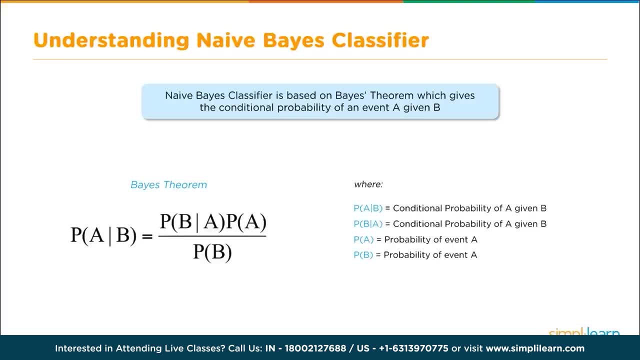 So, when you see data like this, it's necessary to move away from a 1D view of the data to a two-dimensional view of the data. So, when you see data like this, it's necessary to move away from a 1D view of the data to a two-dimensional view of the data. 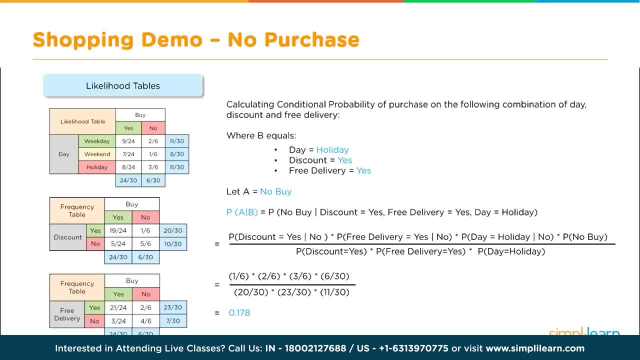 So, when you see data like this, it's necessary to move away from a 1D view of the data to a two-dimensional view of the data. So, when you see data like this, it's necessary to move away from a 1D view of the data to a two-dimensional view of the data. 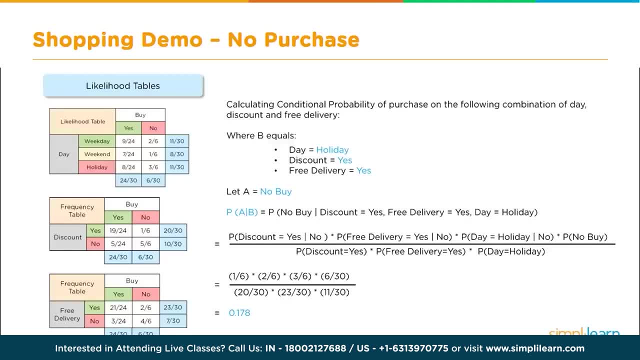 So, when you see data like this, it's necessary to move away from a 1D view of the data to a two-dimensional view of the data. So, when you see data like this, it's necessary to move away from a 1D view of the data to a two-dimensional view of the data. 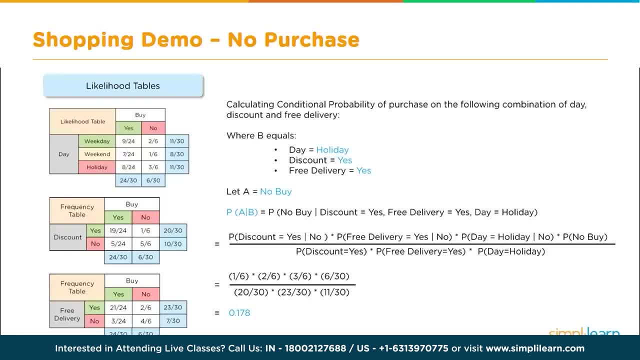 So, when you see data like this, it's necessary to move away from a 1D view of the data to a two-dimensional view of the data. So, when you see data like this, it's necessary to move away from a 1D view of the data to a two-dimensional view of the data. 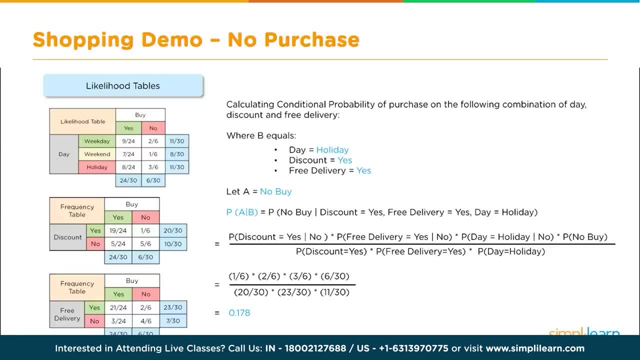 So, when you see data like this, it's necessary to move away from a 1D view of the data to a two-dimensional view of the data. So, when you see data like this, it's necessary to move away from a 1D view of the data to a two-dimensional view of the data. 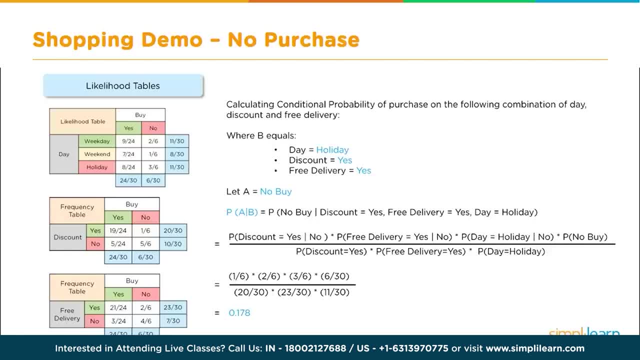 So, when you see data like this, it's necessary to move away from a 1D view of the data to a two-dimensional view of the data. So, when you see data like this, it's necessary to move away from a 1D view of the data to a two-dimensional view of the data. 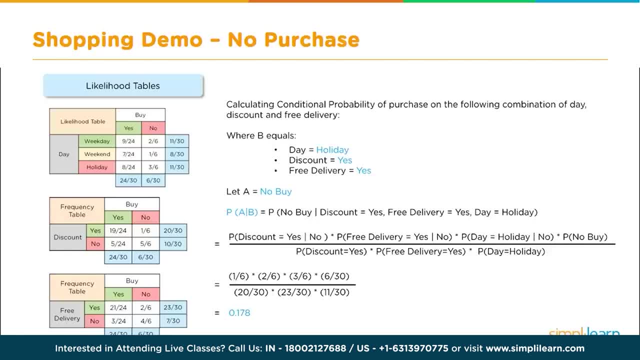 So, when you see data like this, it's necessary to move away from a 1D view of the data to a two-dimensional view of the data. So, when you see data like this, it's necessary to move away from a 1D view of the data to a two-dimensional view of the data. 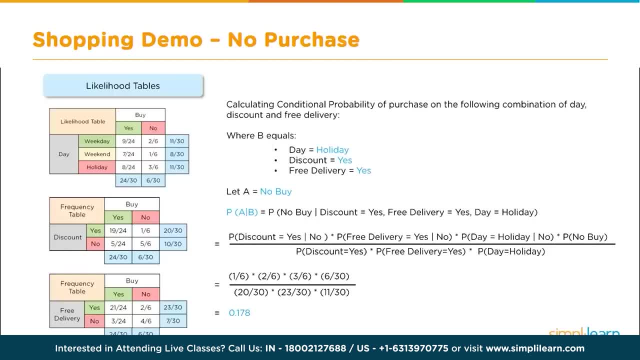 So, when you see data like this, it's necessary to move away from a 1D view of the data to a two-dimensional view of the data. So, when you see data like this, it's necessary to move away from a 1D view of the data to a two-dimensional view of the data. 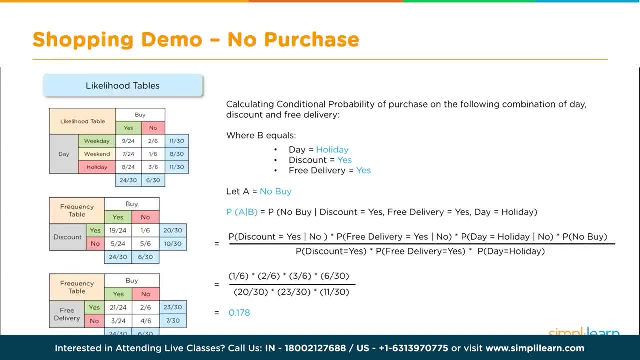 So, when you see data like this, it's necessary to move away from a 1D view of the data to a two-dimensional view of the data. So, when you see data like this, it's necessary to move away from a 1D view of the data to a two-dimensional view of the data. 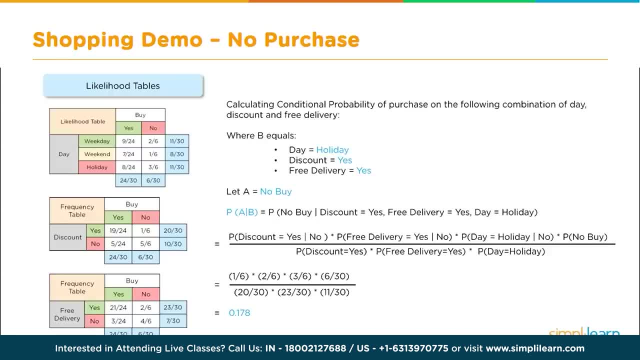 So, when you see data like this, it's necessary to move away from a 1D view of the data to a two-dimensional view of the data. So, when you see data like this, it's necessary to move away from a 1D view of the data to a two-dimensional view of the data. 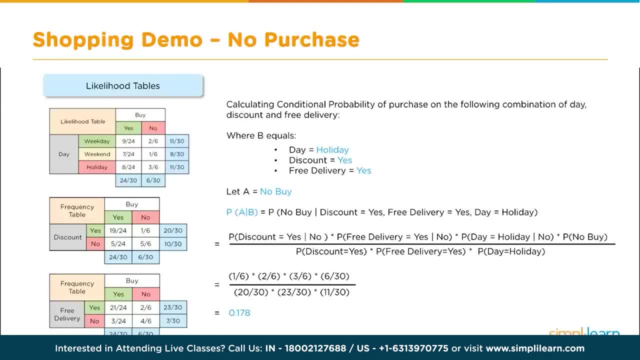 So, when you see data like this, it's necessary to move away from a 1D view of the data to a two-dimensional view of the data. So, when you see data like this, it's necessary to move away from a 1D view of the data to a two-dimensional view of the data. 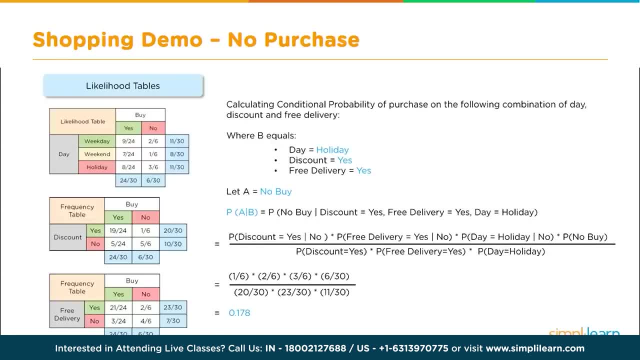 So, when you see data like this, it's necessary to move away from a 1D view of the data to a two-dimensional view of the data. So, when you see data like this, it's necessary to move away from a 1D view of the data to a two-dimensional view of the data. 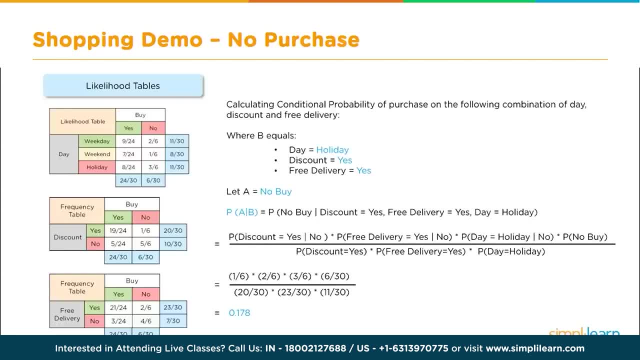 So, when you see data like this, it's necessary to move away from a 1D view of the data to a two-dimensional view of the data. So, when you see data like this, it's necessary to move away from a 1D view of the data to a two-dimensional view of the data. 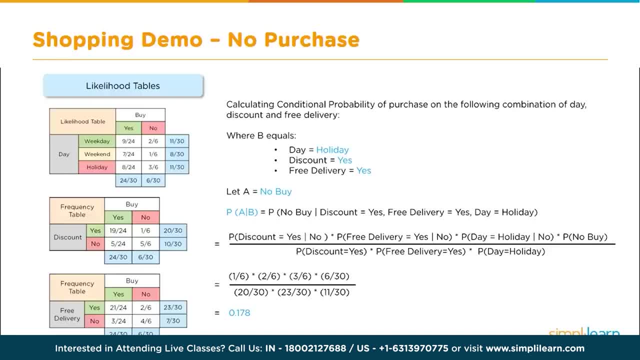 So, when you see data like this, it's necessary to move away from a 1D view of the data to a two-dimensional view of the data. So, when you see data like this, it's necessary to move away from a 1D view of the data to a two-dimensional view of the data. 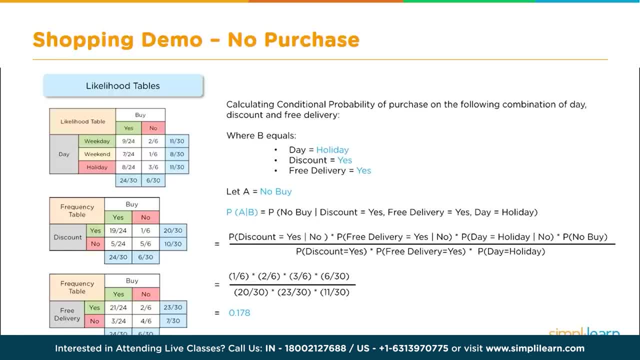 So, when you see data like this, it's necessary to move away from a 1D view of the data to a two-dimensional view of the data. So, when you see data like this, it's necessary to move away from a 1D view of the data to a two-dimensional view of the data. 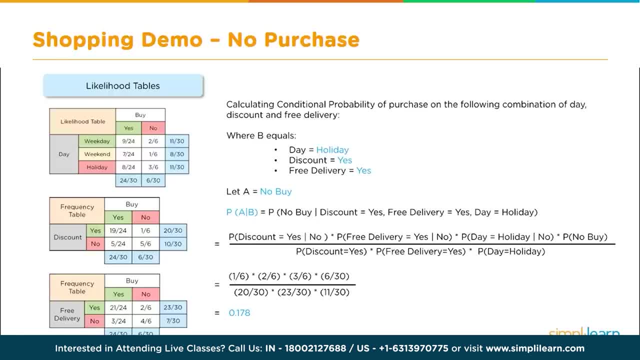 So, when you see data like this, it's necessary to move away from a 1D view of the data to a two-dimensional view of the data. So, when you see data like this, it's necessary to move away from a 1D view of the data to a two-dimensional view of the data. 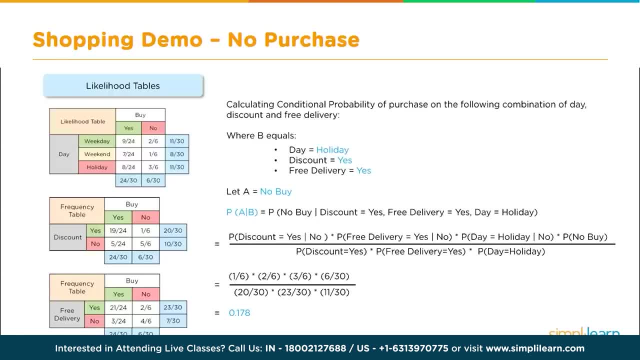 So, when you see data like this, it's necessary to move away from a 1D view of the data to a two-dimensional view of the data. So, when you see data like this, it's necessary to move away from a 1D view of the data to a two-dimensional view of the data. 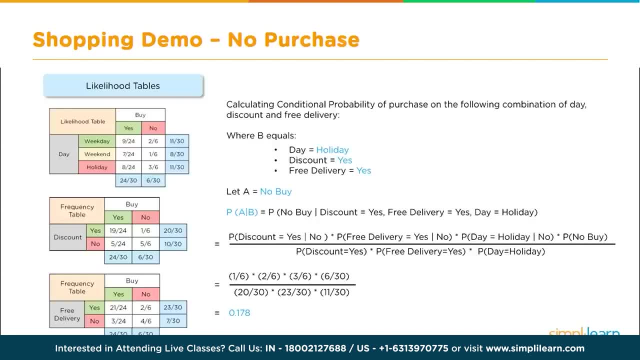 So, when you see data like this, it's necessary to move away from a 1D view of the data to a two-dimensional view of the data. So, when you see data like this, it's necessary to move away from a 1D view of the data to a two-dimensional view of the data. 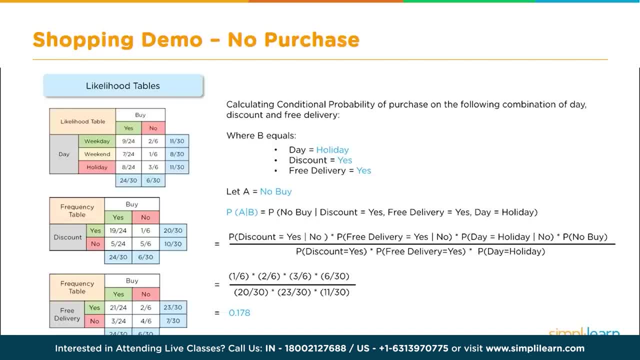 So, when you see data like this, it's necessary to move away from a 1D view of the data to a two-dimensional view of the data. So, when you see data like this, it's necessary to move away from a 1D view of the data to a two-dimensional view of the data. 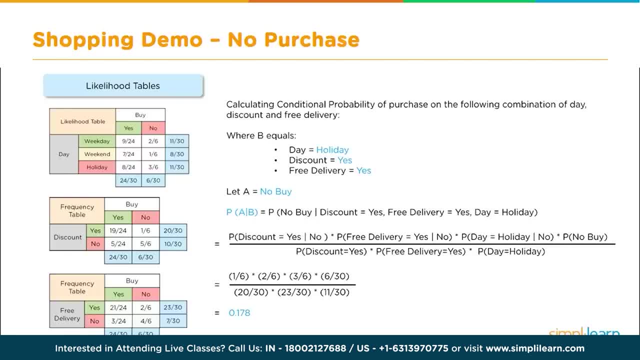 So, when you see data like this, it's necessary to move away from a 1D view of the data to a two-dimensional view of the data. So, when you see data like this, it's necessary to move away from a 1D view of the data to a two-dimensional view of the data. 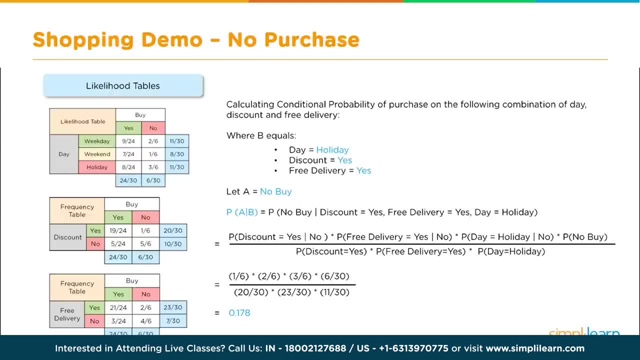 So, when you see data like this, it's necessary to move away from a 1D view of the data to a two-dimensional view of the data. So, when you see data like this, it's necessary to move away from a 1D view of the data to a two-dimensional view of the data. 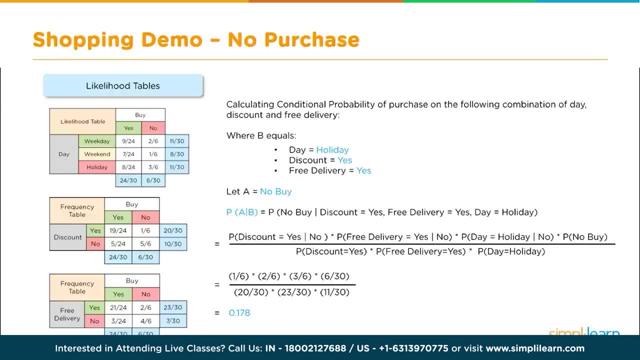 So, when you see data like this, it's necessary to move away from a 1D view of the data to a two-dimensional view of the data. So, when you see data like this, it's necessary to move away from a 1D view of the data to a two-dimensional view of the data. 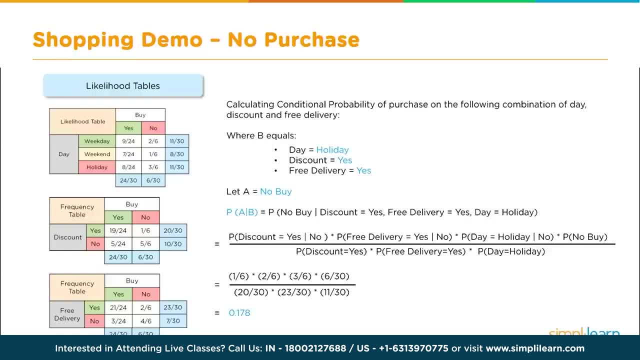 So, when you see data like this, it's necessary to move away from a 1D view of the data to a two-dimensional view of the data. So, when you see data like this, it's necessary to move away from a 1D view of the data to a two-dimensional view of the data. 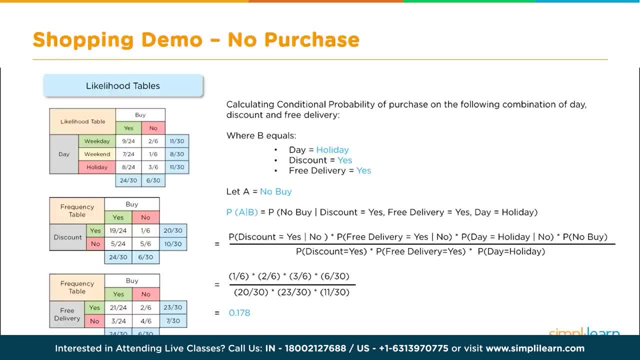 So, when you see data like this, it's necessary to move away from a 1D view of the data to a two-dimensional view of the data. So, when you see data like this, it's necessary to move away from a 1D view of the data to a two-dimensional view of the data. 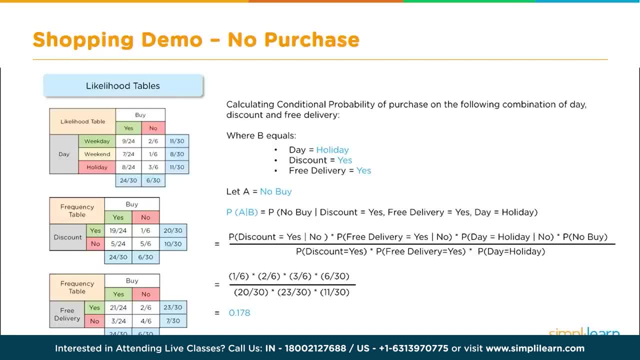 So, when you see data like this, it's necessary to move away from a 1D view of the data to a two-dimensional view of the data. So, when you see data like this, it's necessary to move away from a 1D view of the data to a two-dimensional view of the data. 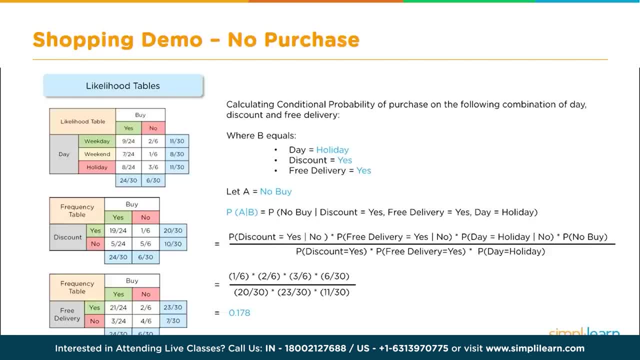 So, when you see data like this, it's necessary to move away from a 1D view of the data to a two-dimensional view of the data. So, when you see data like this, it's necessary to move away from a 1D view of the data to a two-dimensional view of the data. 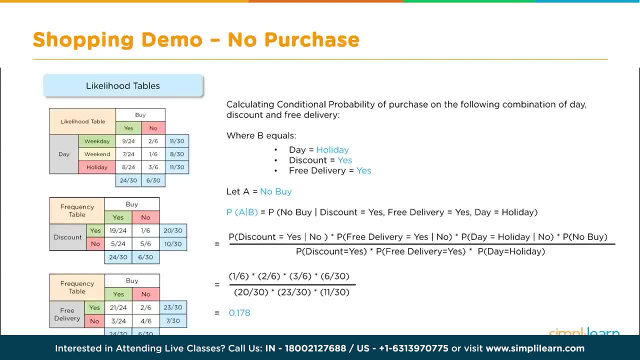 So, when you see data like this, it's necessary to move away from a 1D view of the data to a two-dimensional view of the data. So, when you see data like this, it's necessary to move away from a 1D view of the data to a two-dimensional view of the data. 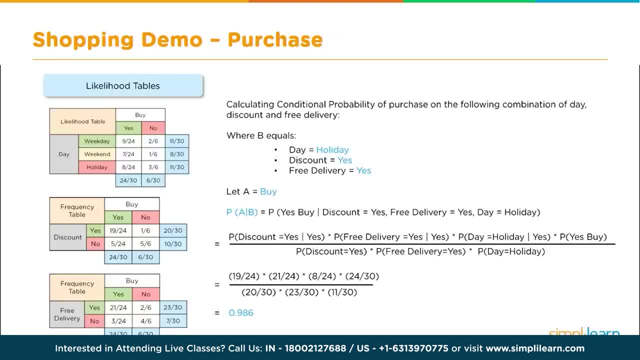 So, when you see data like this, it's necessary to move away from a 1D view of the data to a two-dimensional view of the data. So, when you see data like this, it's necessary to move away from a 1D view of the data to a two-dimensional view of the data. 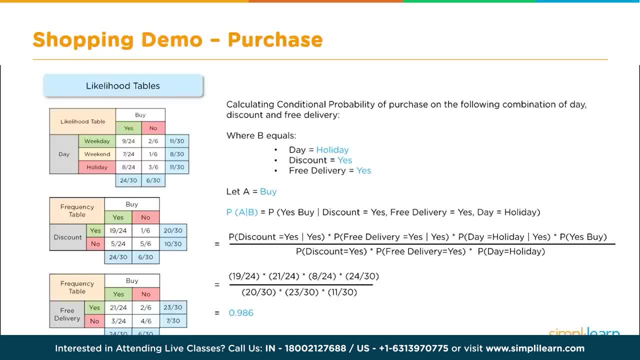 So, when you see data like this, it's necessary to move away from a 1D view of the data to a two-dimensional view of the data. So, when you see data like this, it's necessary to move away from a 1D view of the data to a two-dimensional view of the data. 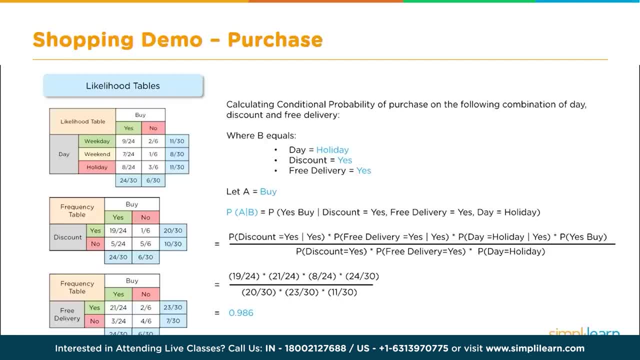 So, when you see data like this, it's necessary to move away from a 1D view of the data to a two-dimensional view of the data. So, when you see data like this, it's necessary to move away from a 1D view of the data to a two-dimensional view of the data. 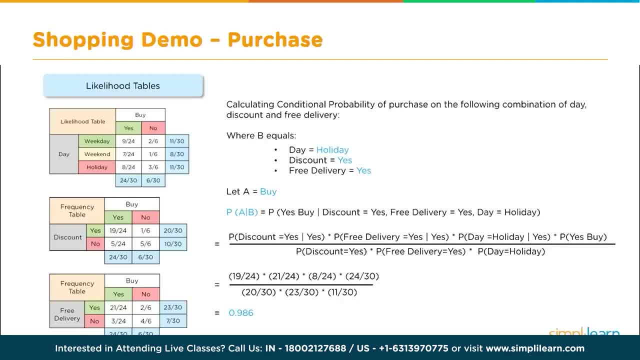 So, when you see data like this, it's necessary to move away from a 1D view of the data to a two-dimensional view of the data. So, when you see data like this, it's necessary to move away from a 1D view of the data to a two-dimensional view of the data. 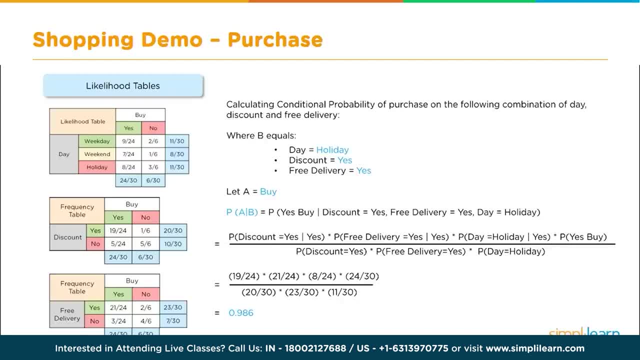 So, when you see data like this, it's necessary to move away from a 1D view of the data to a two-dimensional view of the data. So, when you see data like this, it's necessary to move away from a 1D view of the data to a two-dimensional view of the data. 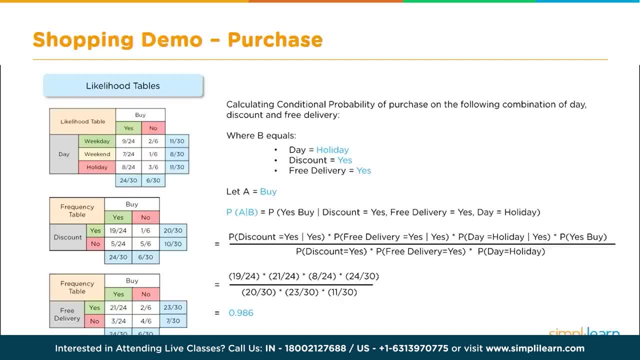 So, when you see data like this, it's necessary to move away from a 1D view of the data to a two-dimensional view of the data. So, when you see data like this, it's necessary to move away from a 1D view of the data to a two-dimensional view of the data. 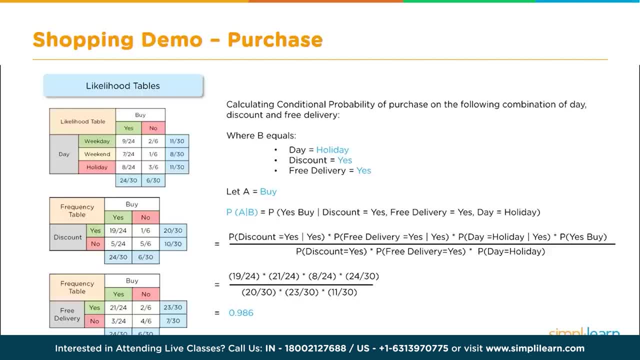 So, when you see data like this, it's necessary to move away from a 1D view of the data to a two-dimensional view of the data. So, when you see data like this, it's necessary to move away from a 1D view of the data to a two-dimensional view of the data. 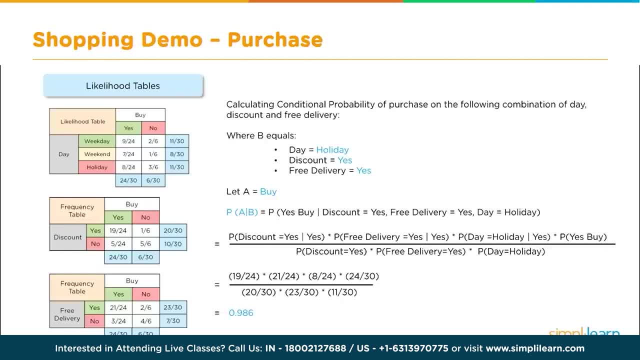 So, when you see data like this, it's necessary to move away from a 1D view of the data to a two-dimensional view of the data. So, when you see data like this, it's necessary to move away from a 1D view of the data to a two-dimensional view of the data. 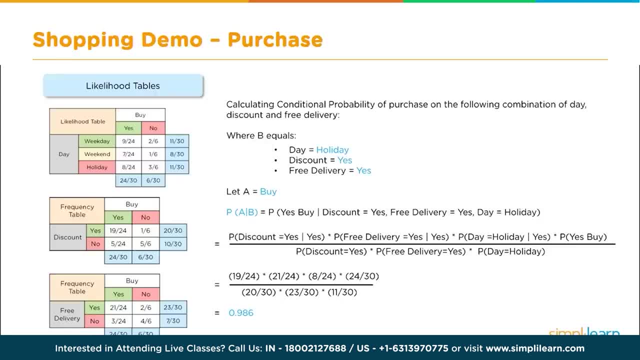 So, when you see data like this, it's necessary to move away from a 1D view of the data to a two-dimensional view of the data. So, when you see data like this, it's necessary to move away from a 1D view of the data to a two-dimensional view of the data. 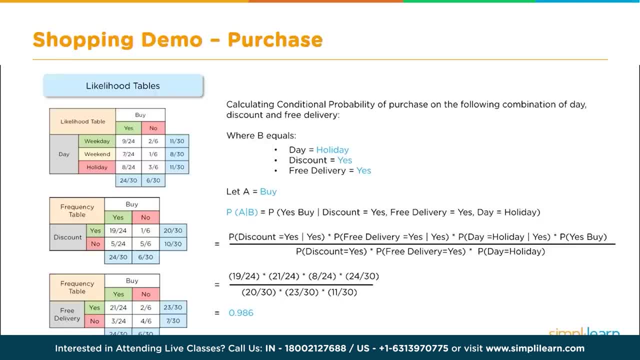 So, when you see data like this, it's necessary to move away from a 1D view of the data to a two-dimensional view of the data. So, when you see data like this, it's necessary to move away from a 1D view of the data to a two-dimensional view of the data. 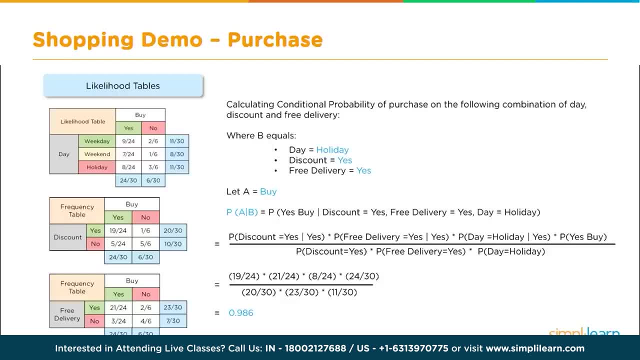 So, when you see data like this, it's necessary to move away from a 1D view of the data to a two-dimensional view of the data. So, when you see data like this, it's necessary to move away from a 1D view of the data to a two-dimensional view of the data. 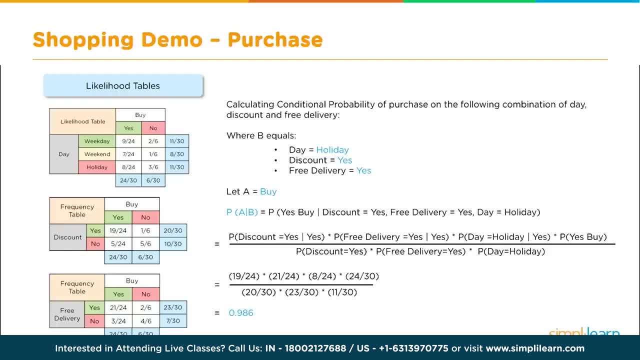 So, when you see data like this, it's necessary to move away from a 1D view of the data to a two-dimensional view of the data. So, when you see data like this, it's necessary to move away from a 1D view of the data to a two-dimensional view of the data. 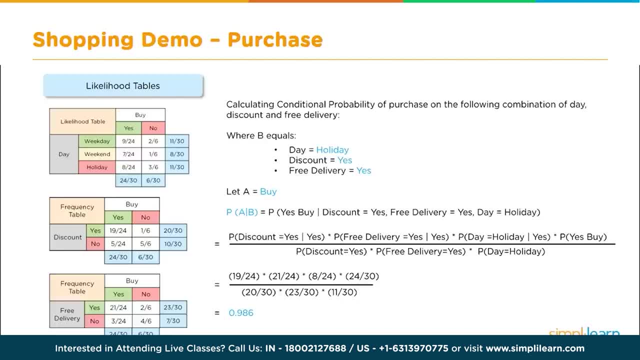 So, when you see data like this, it's necessary to move away from a 1D view of the data to a two-dimensional view of the data. So, when you see data like this, it's necessary to move away from a 1D view of the data to a two-dimensional view of the data. 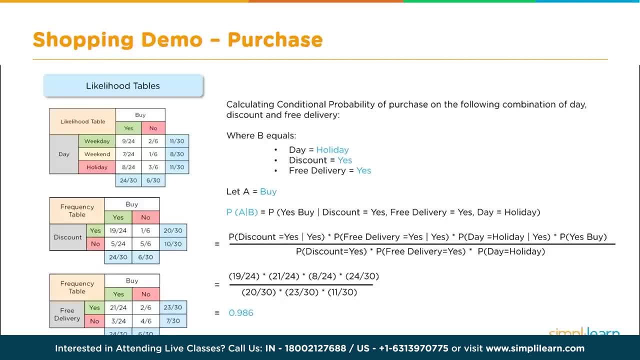 So, when you see data like this, it's necessary to move away from a 1D view of the data to a two-dimensional view of the data. So, when you see data like this, it's necessary to move away from a 1D view of the data to a two-dimensional view of the data. 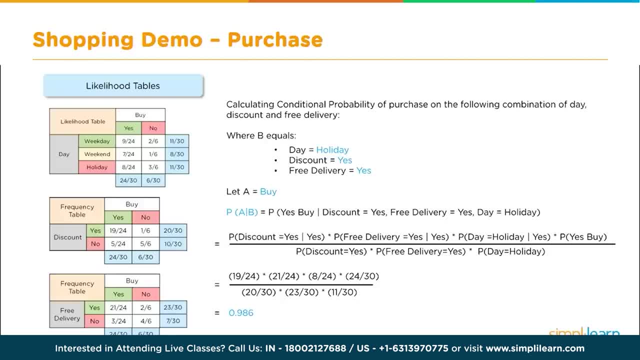 So, when you see data like this, it's necessary to move away from a 1D view of the data to a two-dimensional view of the data. So, when you see data like this, it's necessary to move away from a 1D view of the data to a two-dimensional view of the data. 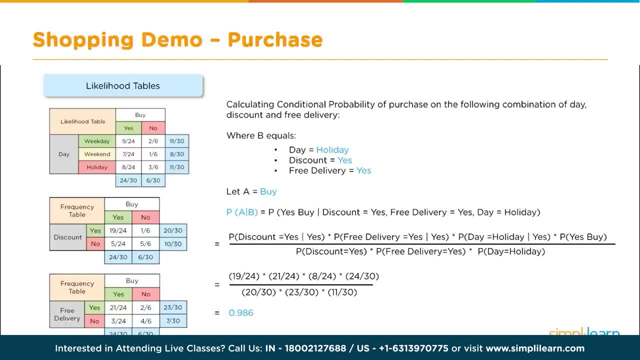 So, when you see data like this, it's necessary to move away from a 1D view of the data to a two-dimensional view of the data. So, when you see data like this, it's necessary to move away from a 1D view of the data to a two-dimensional view of the data. 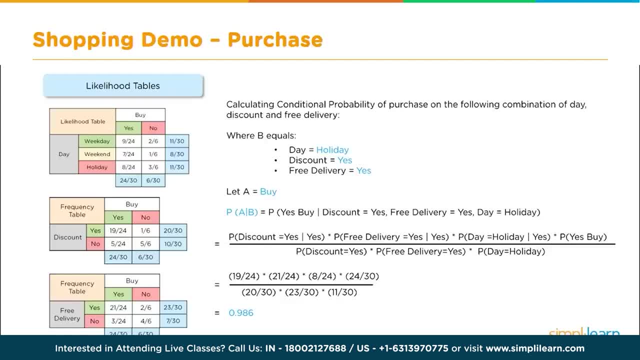 So, when you see data like this, it's necessary to move away from a 1D view of the data to a two-dimensional view of the data. So, when you see data like this, it's necessary to move away from a 1D view of the data to a two-dimensional view of the data. 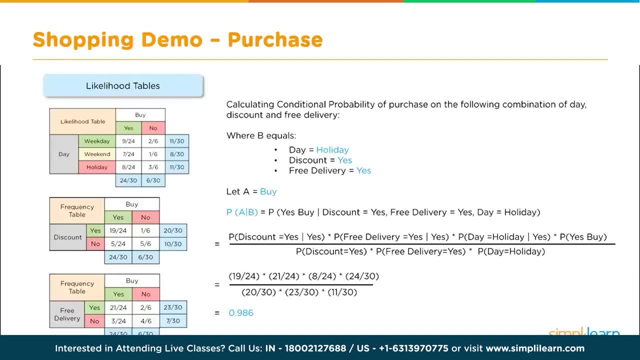 So, when you see data like this, it's necessary to move away from a 1D view of the data to a two-dimensional view of the data. So, when you see data like this, it's necessary to move away from a 1D view of the data to a two-dimensional view of the data. 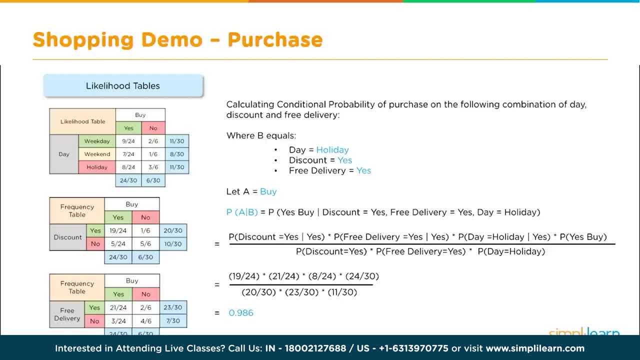 So, when you see data like this, it's necessary to move away from a 1D view of the data to a two-dimensional view of the data. So, when you see data like this, it's necessary to move away from a 1D view of the data to a two-dimensional view of the data. 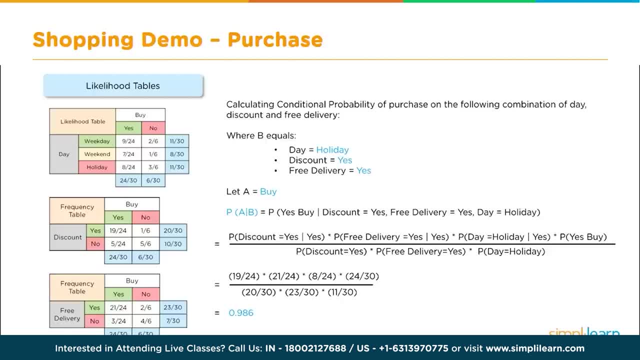 So, when you see data like this, it's necessary to move away from a 1D view of the data to a two-dimensional view of the data. So, when you see data like this, it's necessary to move away from a 1D view of the data to a two-dimensional view of the data. 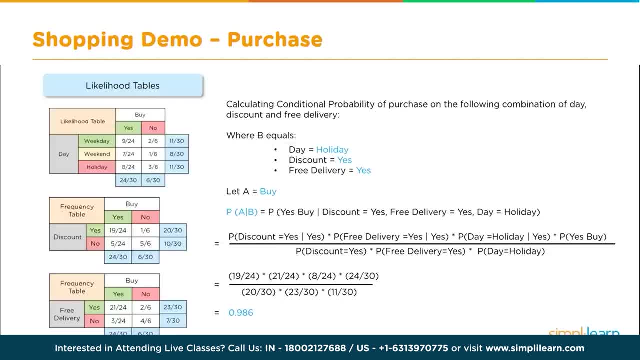 So, when you see data like this, it's necessary to move away from a 1D view of the data to a two-dimensional view of the data. So, when you see data like this, it's necessary to move away from a 1D view of the data to a two-dimensional view of the data. 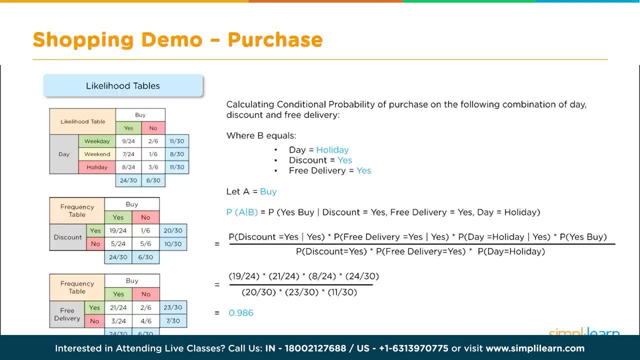 So, when you see data like this, it's necessary to move away from a 1D view of the data to a two-dimensional view of the data. So, when you see data like this, it's necessary to move away from a 1D view of the data to a two-dimensional view of the data. 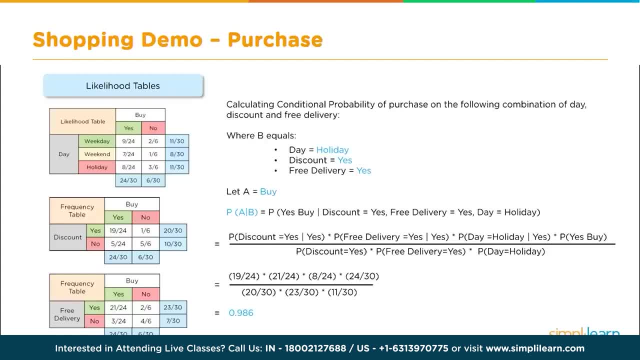 So, when you see data like this, it's necessary to move away from a 1D view of the data to a two-dimensional view of the data. So, when you see data like this, it's necessary to move away from a 1D view of the data to a two-dimensional view of the data. 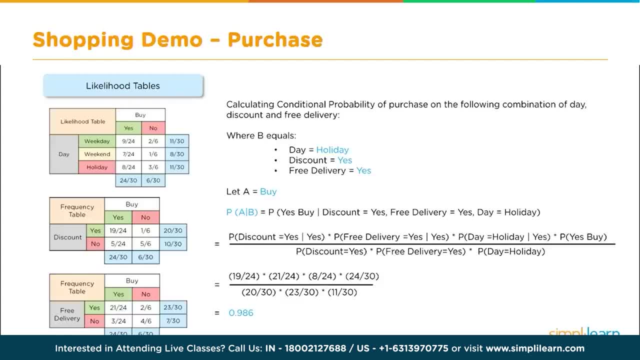 So, when you see data like this, it's necessary to move away from a 1D view of the data to a two-dimensional view of the data. So, when you see data like this, it's necessary to move away from a 1D view of the data to a two-dimensional view of the data. 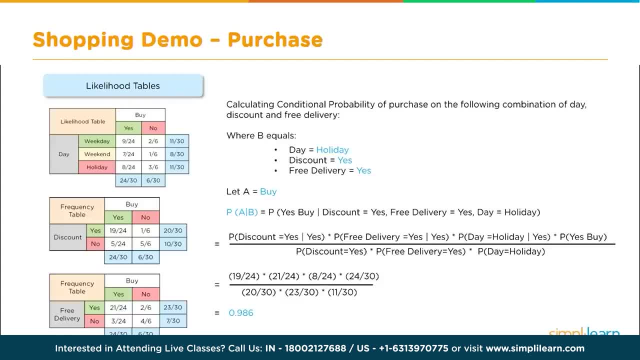 So, when you see data like this, it's necessary to move away from a 1D view of the data to a two-dimensional view of the data. So, when you see data like this, it's necessary to move away from a 1D view of the data to a two-dimensional view of the data. 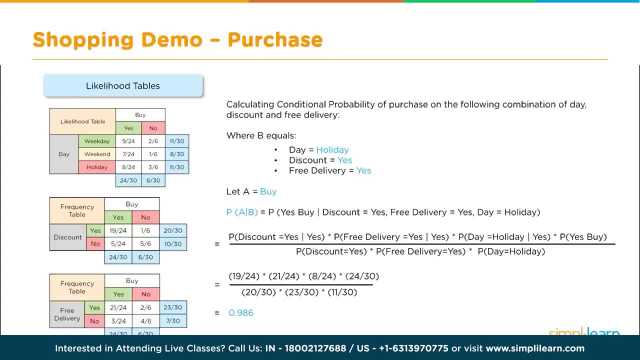 So, when you see data like this, it's necessary to move away from a 1D view of the data to a two-dimensional view of the data. So, when you see data like this, it's necessary to move away from a 1D view of the data to a two-dimensional view of the data. 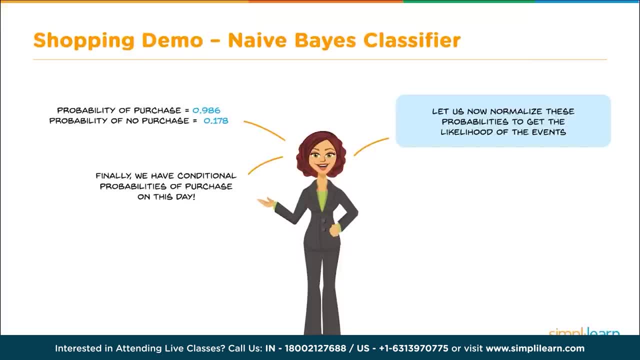 So, when you see data like this, it's necessary to move away from a 1D view of the data to a two-dimensional view of the data. So, when you see data like this, it's necessary to move away from a 1D view of the data to a two-dimensional view of the data. 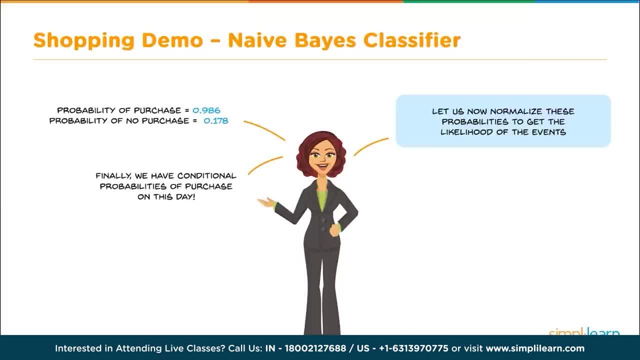 So, when you see data like this, it's necessary to move away from a 1D view of the data to a two-dimensional view of the data. So, when you see data like this, it's necessary to move away from a 1D view of the data to a two-dimensional view of the data. 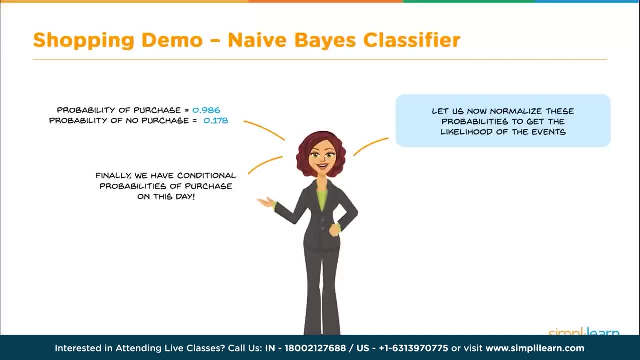 So, when you see data like this, it's necessary to move away from a 1D view of the data to a two-dimensional view of the data. So, when you see data like this, it's necessary to move away from a 1D view of the data to a two-dimensional view of the data. 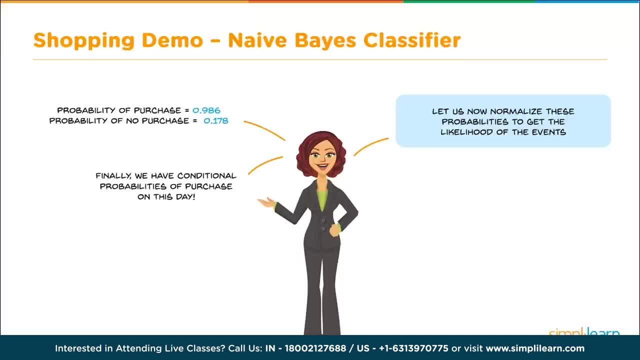 So, when you see data like this, it's necessary to move away from a 1D view of the data to a two-dimensional view of the data. So, when you see data like this, it's necessary to move away from a 1D view of the data to a two-dimensional view of the data. 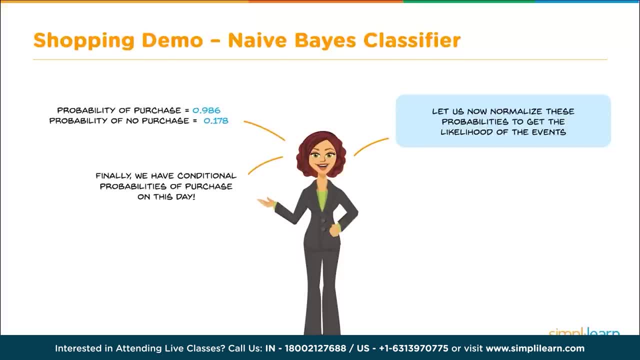 So, when you see data like this, it's necessary to move away from a 1D view of the data to a two-dimensional view of the data. So, when you see data like this, it's necessary to move away from a 1D view of the data to a two-dimensional view of the data. 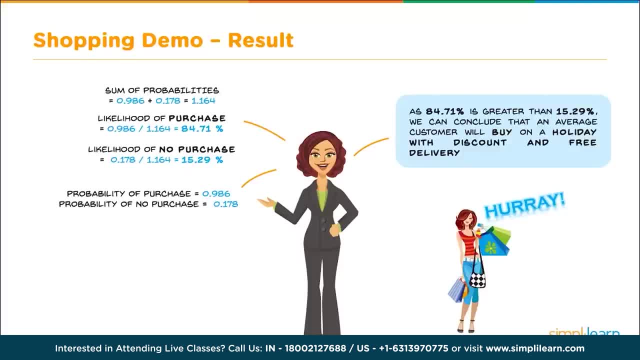 So, when you see data like this, it's necessary to move away from a 1D view of the data to a two-dimensional view of the data. So, when you see data like this, it's necessary to move away from a 1D view of the data to a two-dimensional view of the data. 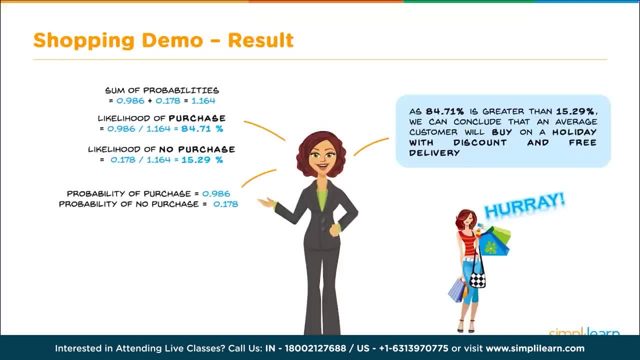 So, when you see data like this, it's necessary to move away from a 1D view of the data to a two-dimensional view of the data. So, when you see data like this, it's necessary to move away from a 1D view of the data to a two-dimensional view of the data. 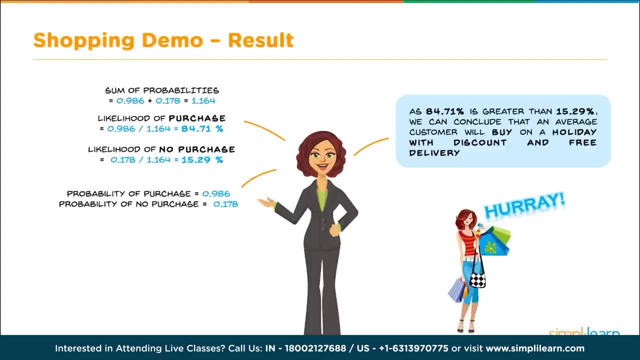 So, when you see data like this, it's necessary to move away from a 1D view of the data to a two-dimensional view of the data. So, when you see data like this, it's necessary to move away from a 1D view of the data to a two-dimensional view of the data. 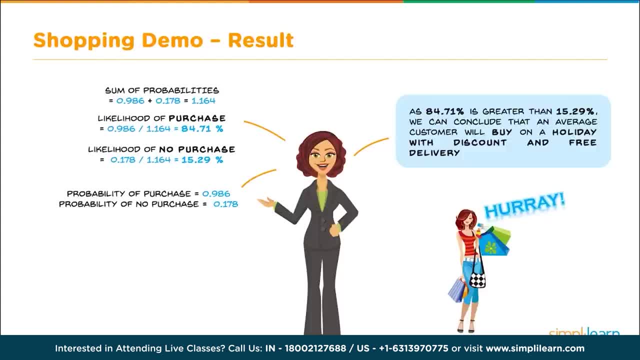 So, when you see data like this, it's necessary to move away from a 1D view of the data to a two-dimensional view of the data. So, when you see data like this, it's necessary to move away from a 1D view of the data to a two-dimensional view of the data. 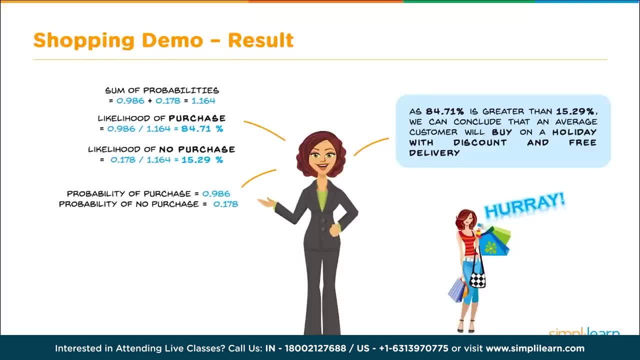 So, when you see data like this, it's necessary to move away from a 1D view of the data to a two-dimensional view of the data. So, when you see data like this, it's necessary to move away from a 1D view of the data to a two-dimensional view of the data. 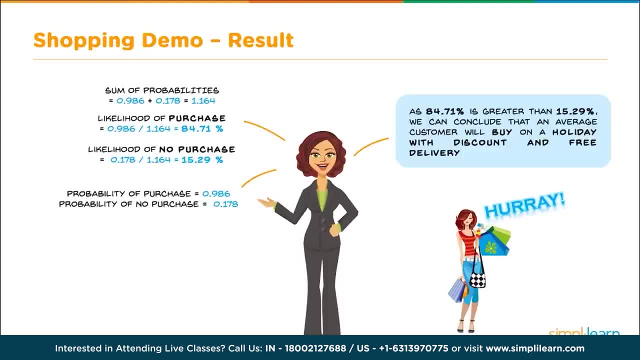 So, when you see data like this, it's necessary to move away from a 1D view of the data to a two-dimensional view of the data. So, when you see data like this, it's necessary to move away from a 1D view of the data to a two-dimensional view of the data. 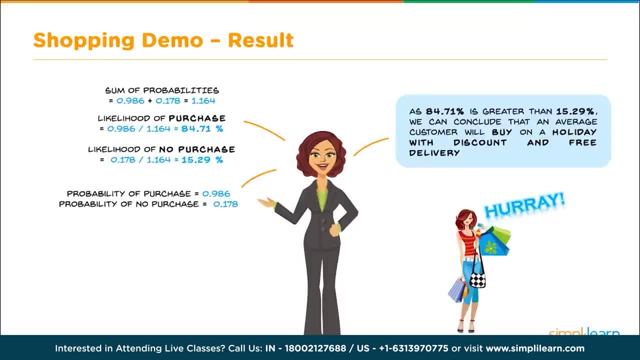 So, when you see data like this, it's necessary to move away from a 1D view of the data to a two-dimensional view of the data. So, when you see data like this, it's necessary to move away from a 1D view of the data to a two-dimensional view of the data. 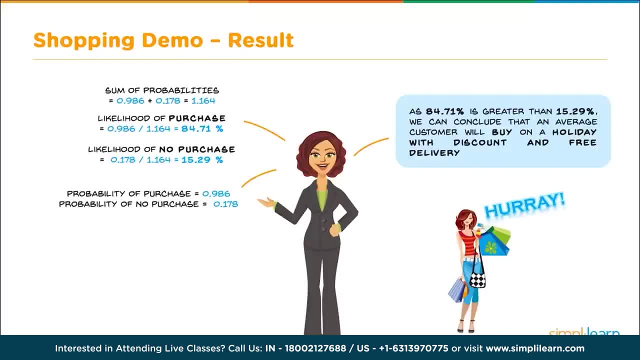 So, when you see data like this, it's necessary to move away from a 1D view of the data to a two-dimensional view of the data. So, when you see data like this, it's necessary to move away from a 1D view of the data to a two-dimensional view of the data. 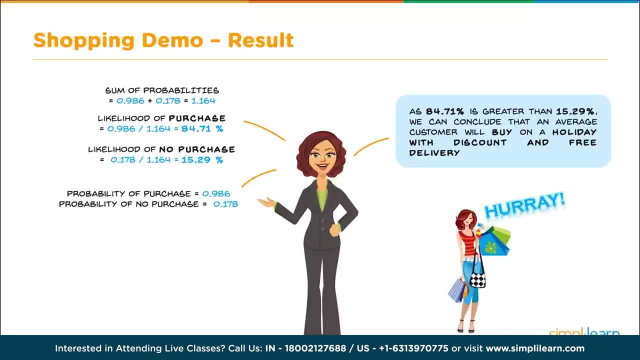 So, when you see data like this, it's necessary to move away from a 1D view of the data to a two-dimensional view of the data. So, when you see data like this, it's necessary to move away from a 1D view of the data to a two-dimensional view of the data. 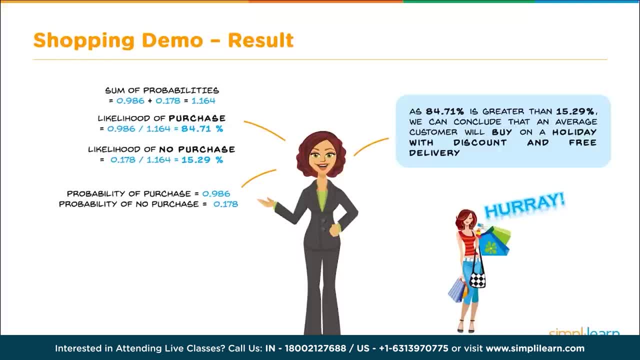 So, when you see data like this, it's necessary to move away from a 1D view of the data to a two-dimensional view of the data. So, when you see data like this, it's necessary to move away from a 1D view of the data to a two-dimensional view of the data. 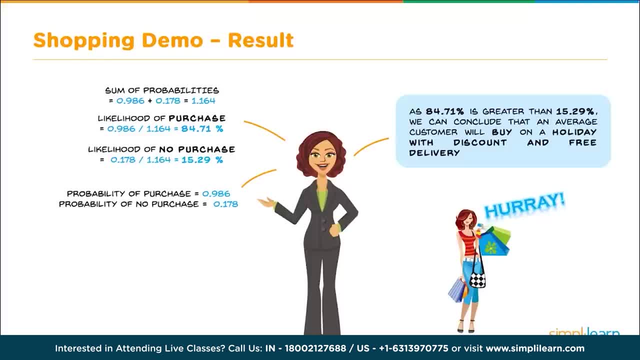 So, when you see data like this, it's necessary to move away from a 1D view of the data to a two-dimensional view of the data. So, when you see data like this, it's necessary to move away from a 1D view of the data to a two-dimensional view of the data. 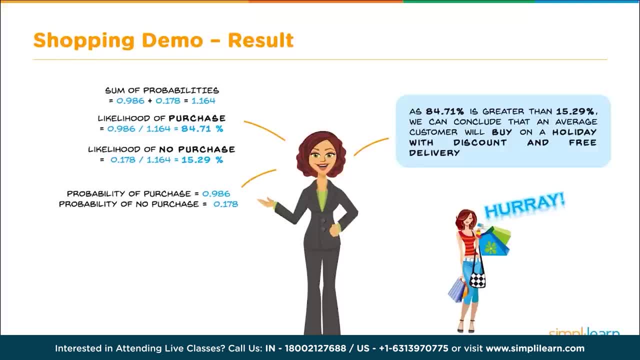 So, when you see data like this, it's necessary to move away from a 1D view of the data to a two-dimensional view of the data. So, when you see data like this, it's necessary to move away from a 1D view of the data to a two-dimensional view of the data. 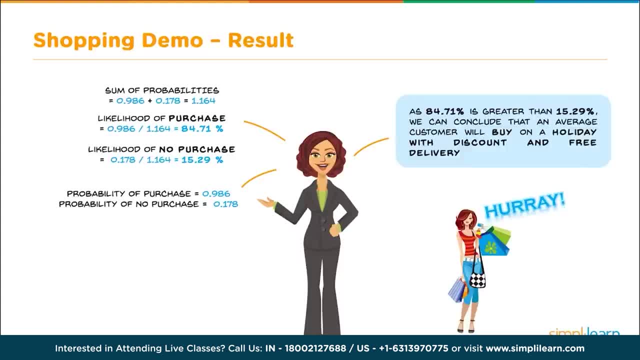 So, when you see data like this, it's necessary to move away from a 1D view of the data to a two-dimensional view of the data. So, when you see data like this, it's necessary to move away from a 1D view of the data to a two-dimensional view of the data. 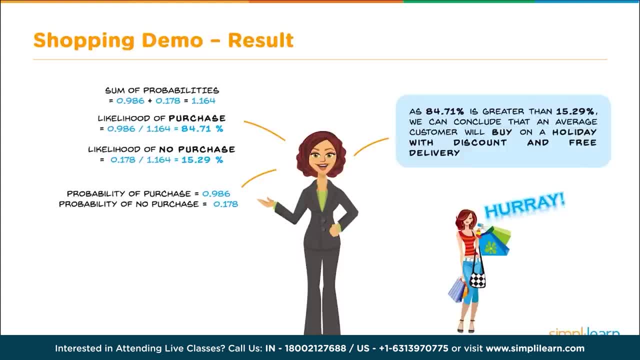 So, when you see data like this, it's necessary to move away from a 1D view of the data to a two-dimensional view of the data. So, when you see data like this, it's necessary to move away from a 1D view of the data to a two-dimensional view of the data. 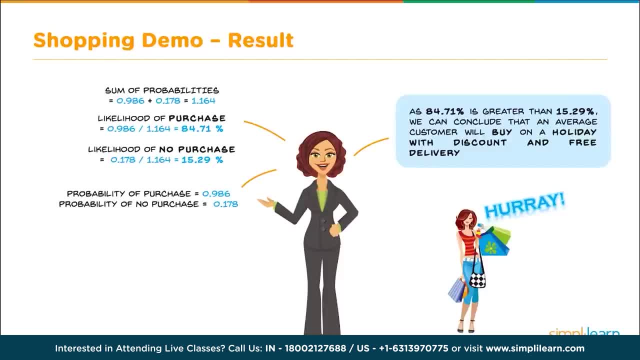 So, when you see data like this, it's necessary to move away from a 1D view of the data to a two-dimensional view of the data. So, when you see data like this, it's necessary to move away from a 1D view of the data to a two-dimensional view of the data. 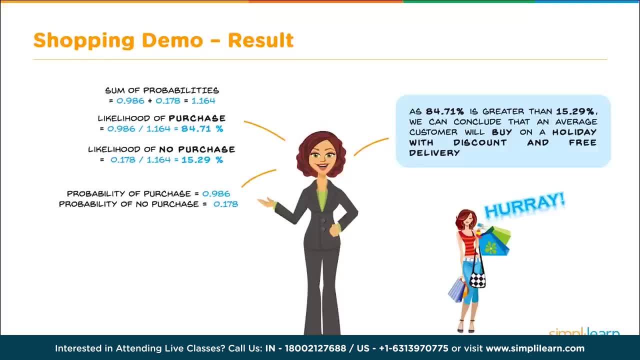 So, when you see data like this, it's necessary to move away from a 1D view of the data to a two-dimensional view of the data. So, when you see data like this, it's necessary to move away from a 1D view of the data to a two-dimensional view of the data. 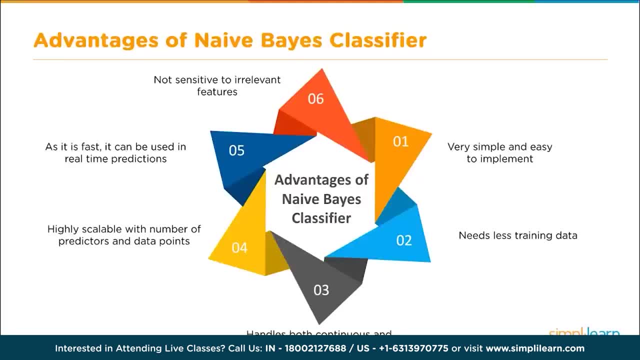 So, when you see data like this, it's necessary to move away from a 1D view of the data to a two-dimensional view of the data. So, when you see data like this, it's necessary to move away from a 1D view of the data to a two-dimensional view of the data. 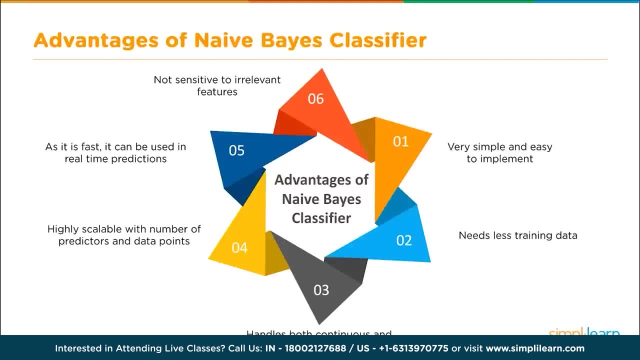 So, when you see data like this, it's necessary to move away from a 1D view of the data to a two-dimensional view of the data. So, when you see data like this, it's necessary to move away from a 1D view of the data to a two-dimensional view of the data. 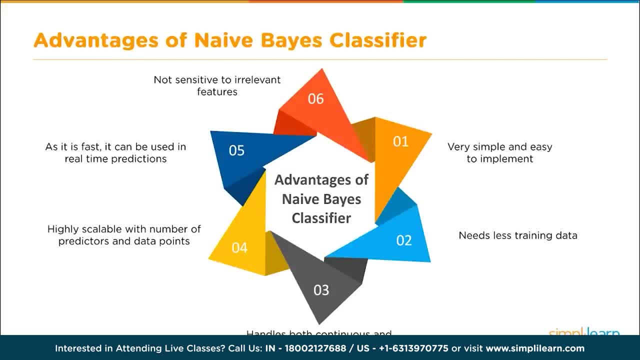 So, when you see data like this, it's necessary to move away from a 1D view of the data to a two-dimensional view of the data. So, when you see data like this, it's necessary to move away from a 1D view of the data to a two-dimensional view of the data. 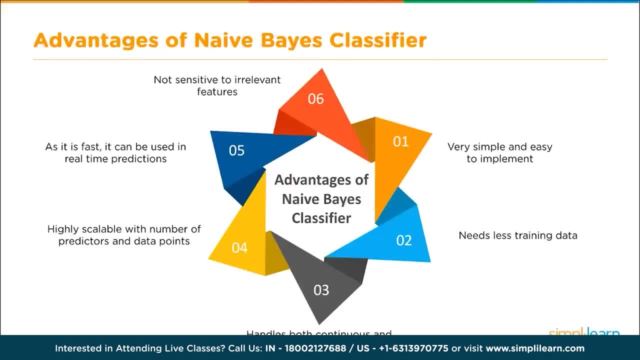 So, when you see data like this, it's necessary to move away from a 1D view of the data to a two-dimensional view of the data. So, when you see data like this, it's necessary to move away from a 1D view of the data to a two-dimensional view of the data. 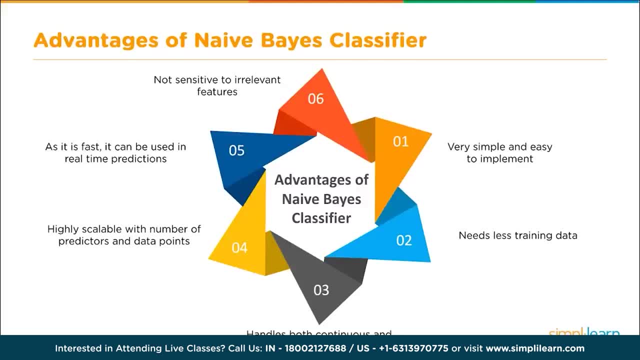 So, when you see data like this, it's necessary to move away from a 1D view of the data to a two-dimensional view of the data. So, when you see data like this, it's necessary to move away from a 1D view of the data to a two-dimensional view of the data. 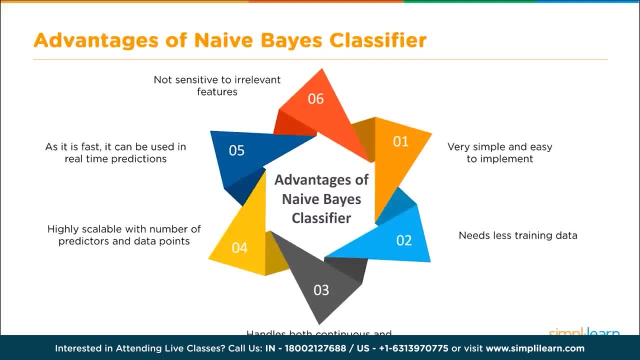 So, when you see data like this, it's necessary to move away from a 1D view of the data to a two-dimensional view of the data. So, when you see data like this, it's necessary to move away from a 1D view of the data to a two-dimensional view of the data. 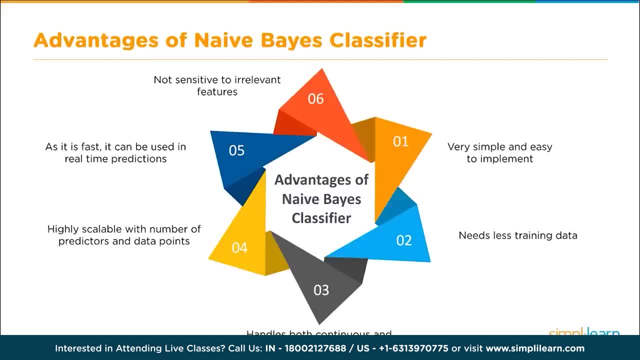 So, when you see data like this, it's necessary to move away from a 1D view of the data to a two-dimensional view of the data. So, when you see data like this, it's necessary to move away from a 1D view of the data to a two-dimensional view of the data. 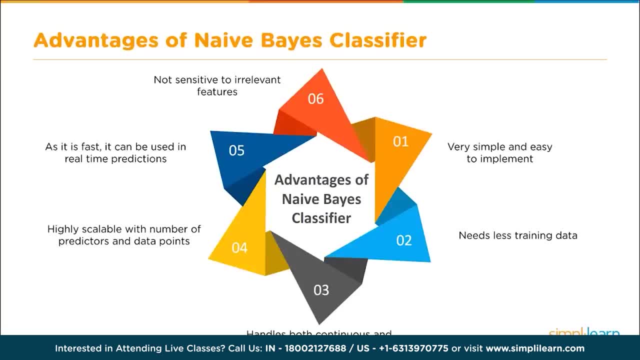 So, when you see data like this, it's necessary to move away from a 1D view of the data to a two-dimensional view of the data. So, when you see data like this, it's necessary to move away from a 1D view of the data to a two-dimensional view of the data. 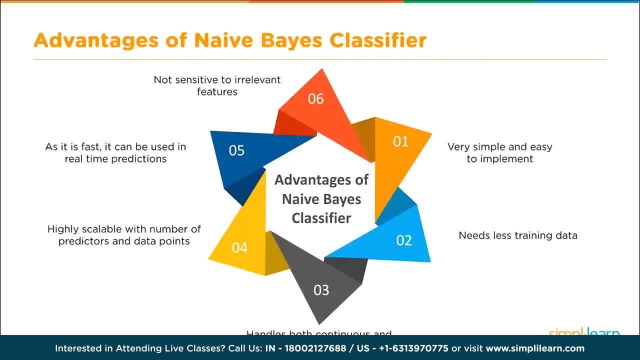 So, when you see data like this, it's necessary to move away from a 1D view of the data to a two-dimensional view of the data. So, when you see data like this, it's necessary to move away from a 1D view of the data to a two-dimensional view of the data. 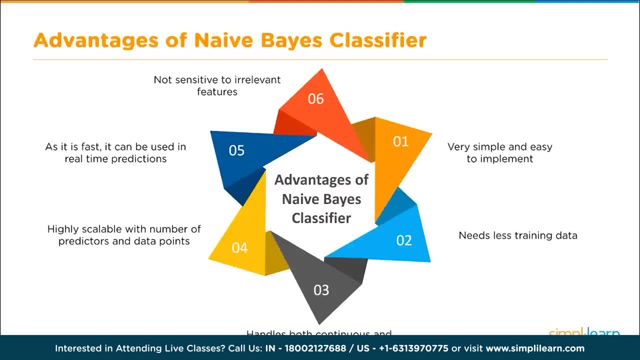 So, when you see data like this, it's necessary to move away from a 1D view of the data to a two-dimensional view of the data. So, when you see data like this, it's necessary to move away from a 1D view of the data to a two-dimensional view of the data. 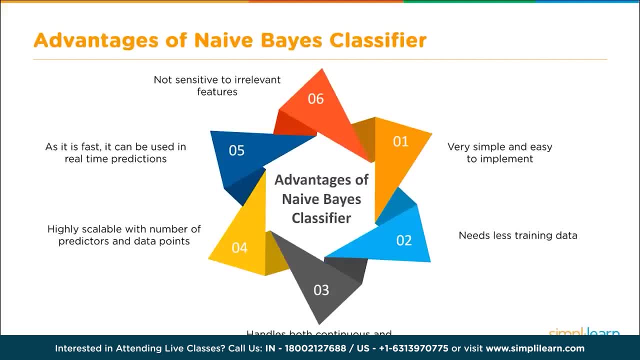 So, when you see data like this, it's necessary to move away from a 1D view of the data to a two-dimensional view of the data. So, when you see data like this, it's necessary to move away from a 1D view of the data to a two-dimensional view of the data. 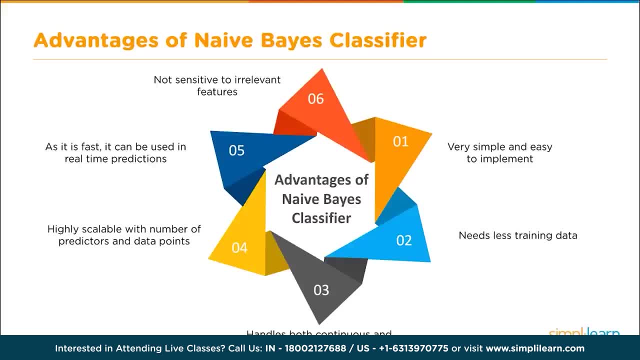 So, when you see data like this, it's necessary to move away from a 1D view of the data to a two-dimensional view of the data. So, when you see data like this, it's necessary to move away from a 1D view of the data to a two-dimensional view of the data. 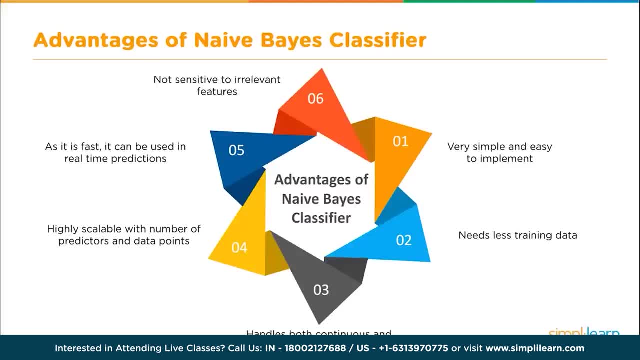 So, when you see data like this, it's necessary to move away from a 1D view of the data to a two-dimensional view of the data. So, when you see data like this, it's necessary to move away from a 1D view of the data to a two-dimensional view of the data. 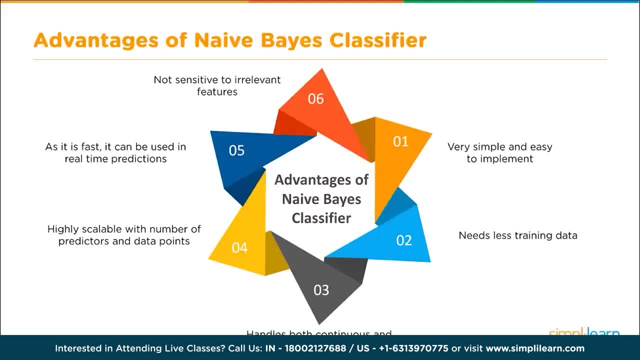 So, when you see data like this, it's necessary to move away from a 1D view of the data to a two-dimensional view of the data. So, when you see data like this, it's necessary to move away from a 1D view of the data to a two-dimensional view of the data. 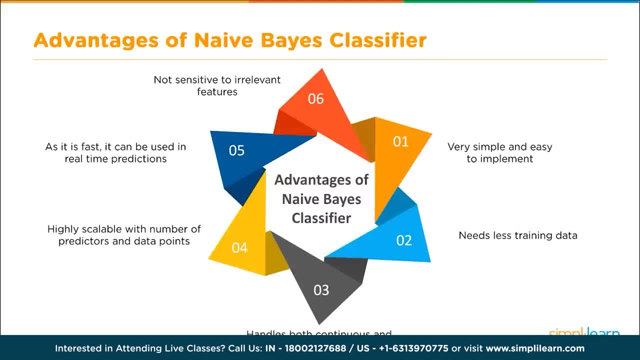 So, when you see data like this, it's necessary to move away from a 1D view of the data to a two-dimensional view of the data. So, when you see data like this, it's necessary to move away from a 1D view of the data to a two-dimensional view of the data. 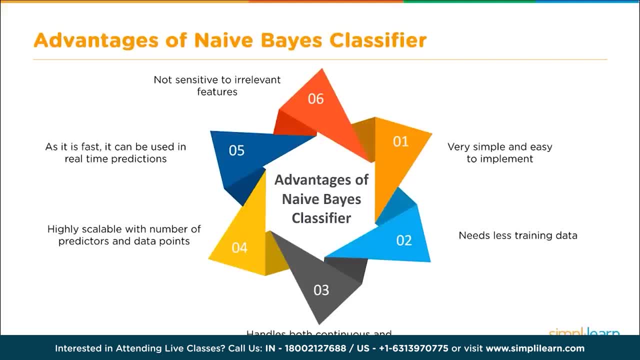 So, when you see data like this, it's necessary to move away from a 1D view of the data to a two-dimensional view of the data. So, when you see data like this, it's necessary to move away from a 1D view of the data to a two-dimensional view of the data. 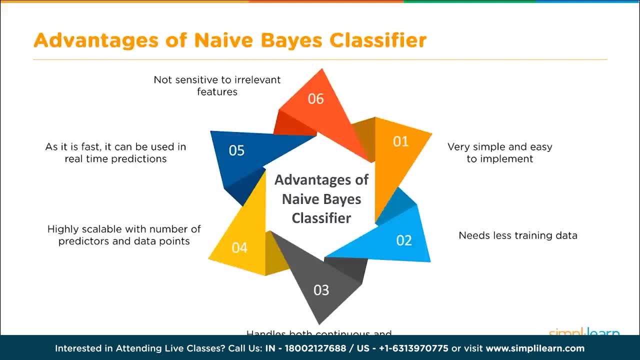 So, when you see data like this, it's necessary to move away from a 1D view of the data to a two-dimensional view of the data. So, when you see data like this, it's necessary to move away from a 1D view of the data to a two-dimensional view of the data. 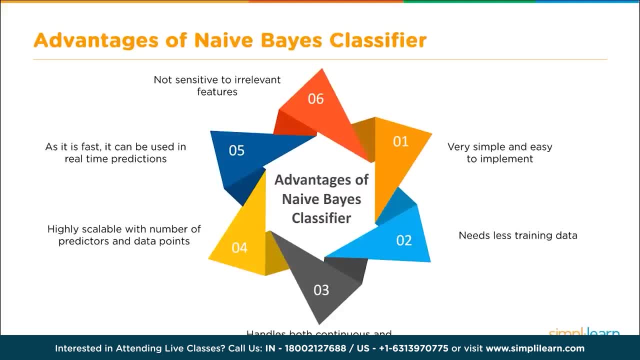 So, when you see data like this, it's necessary to move away from a 1D view of the data to a two-dimensional view of the data. So, when you see data like this, it's necessary to move away from a 1D view of the data to a two-dimensional view of the data. 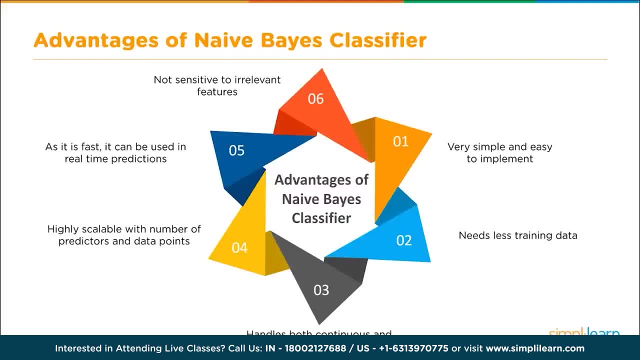 So, when you see data like this, it's necessary to move away from a 1D view of the data to a two-dimensional view of the data. So, when you see data like this, it's necessary to move away from a 1D view of the data to a two-dimensional view of the data. 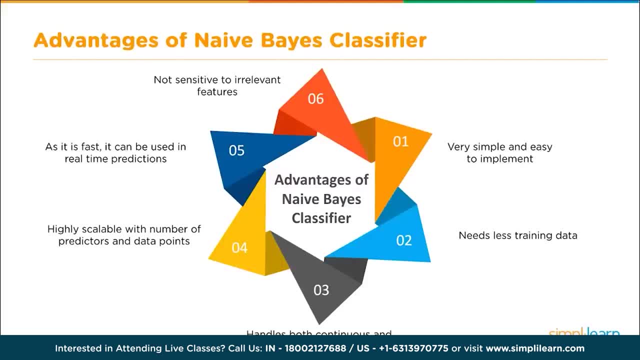 So, when you see data like this, it's necessary to move away from a 1D view of the data to a two-dimensional view of the data. So, when you see data like this, it's necessary to move away from a 1D view of the data to a two-dimensional view of the data. 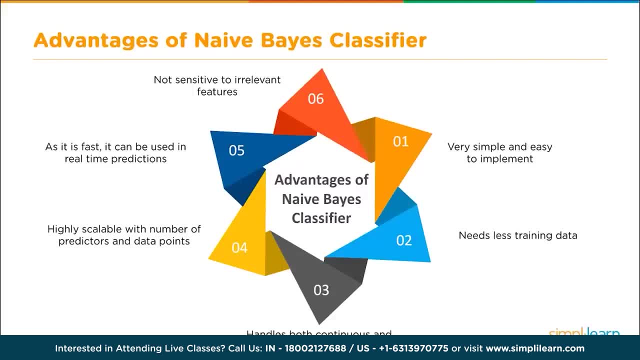 So, when you see data like this, it's necessary to move away from a 1D view of the data to a two-dimensional view of the data. So, when you see data like this, it's necessary to move away from a 1D view of the data to a two-dimensional view of the data. 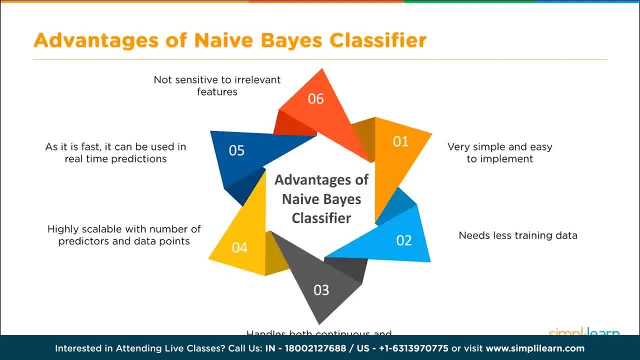 So, when you see data like this, it's necessary to move away from a 1D view of the data to a two-dimensional view of the data. So, when you see data like this, it's necessary to move away from a 1D view of the data to a two-dimensional view of the data. 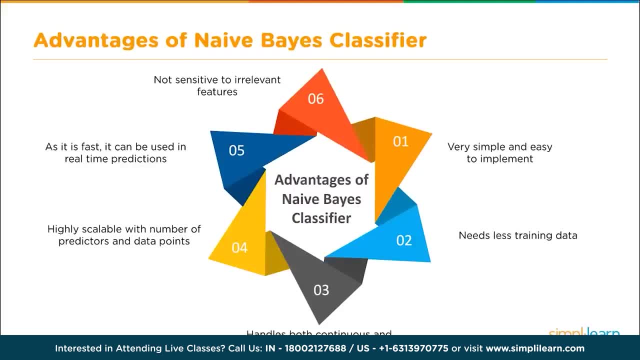 So, when you see data like this, it's necessary to move away from a 1D view of the data to a two-dimensional view of the data. So, when you see data like this, it's necessary to move away from a 1D view of the data to a two-dimensional view of the data. 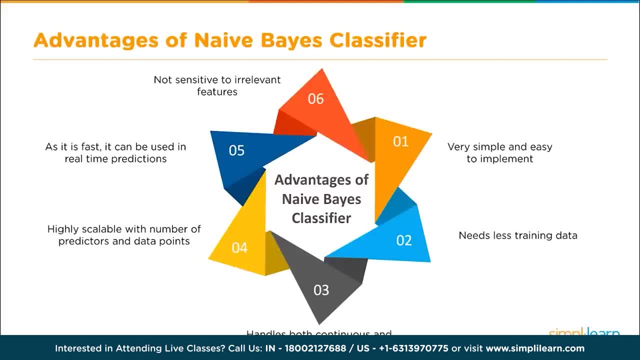 So, when you see data like this, it's necessary to move away from a 1D view of the data to a two-dimensional view of the data. So, when you see data like this, it's necessary to move away from a 1D view of the data to a two-dimensional view of the data. 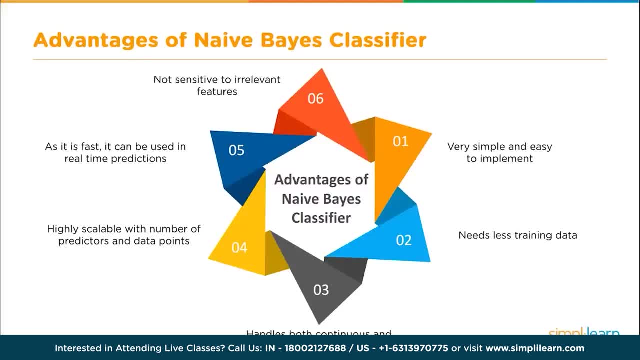 So, when you see data like this, it's necessary to move away from a 1D view of the data to a two-dimensional view of the data. So, when you see data like this, it's necessary to move away from a 1D view of the data to a two-dimensional view of the data. 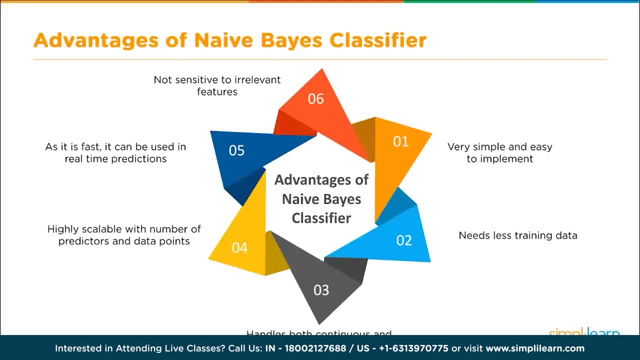 So, when you see data like this, it's necessary to move away from a 1D view of the data to a two-dimensional view of the data. So, when you see data like this, it's necessary to move away from a 1D view of the data to a two-dimensional view of the data. 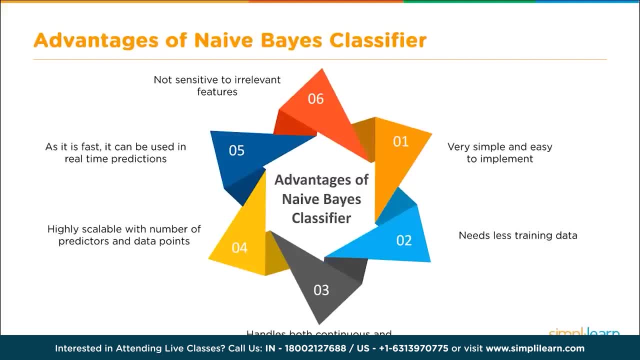 So, when you see data like this, it's necessary to move away from a 1D view of the data to a two-dimensional view of the data. So, when you see data like this, it's necessary to move away from a 1D view of the data to a two-dimensional view of the data. 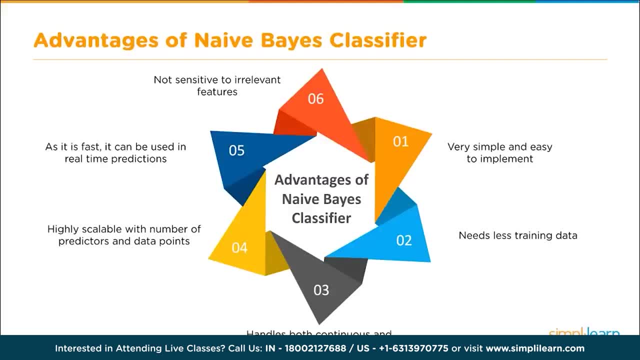 So, when you see data like this, it's necessary to move away from a 1D view of the data to a two-dimensional view of the data. So, when you see data like this, it's necessary to move away from a 1D view of the data to a two-dimensional view of the data. 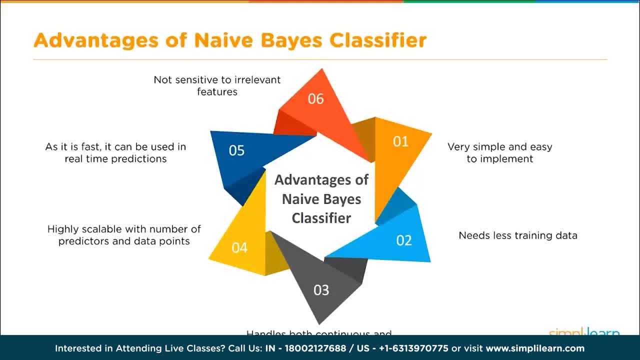 So, when you see data like this, it's necessary to move away from a 1D view of the data to a two-dimensional view of the data. So, when you see data like this, it's necessary to move away from a 1D view of the data to a two-dimensional view of the data. 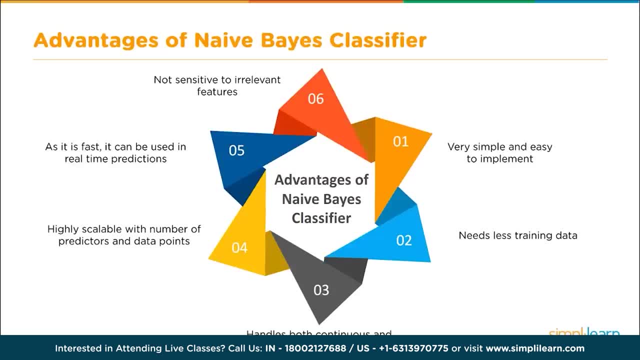 So, when you see data like this, it's necessary to move away from a 1D view of the data to a two-dimensional view of the data. So, when you see data like this, it's necessary to move away from a 1D view of the data to a two-dimensional view of the data. 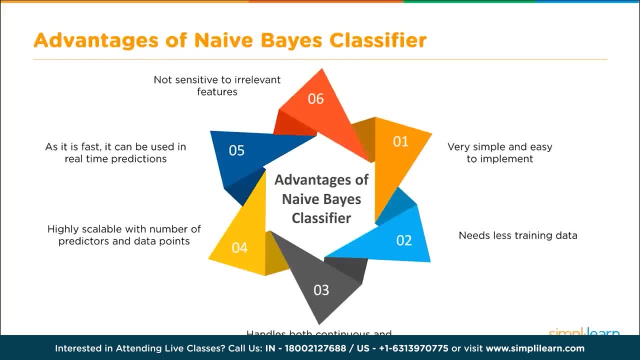 So, when you see data like this, it's necessary to move away from a 1D view of the data to a two-dimensional view of the data. So, when you see data like this, it's necessary to move away from a 1D view of the data to a two-dimensional view of the data. 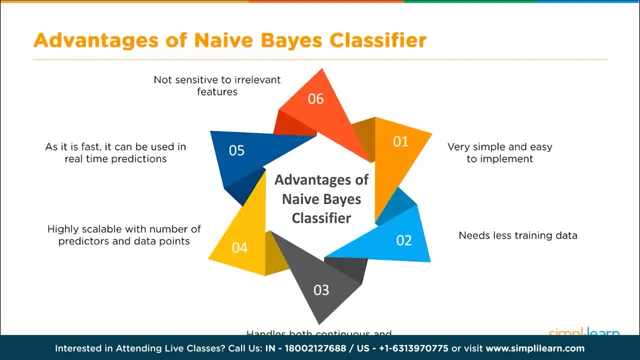 So, when you see data like this, it's necessary to move away from a 1D view of the data to a two-dimensional view of the data. So, when you see data like this, it's necessary to move away from a 1D view of the data to a two-dimensional view of the data. 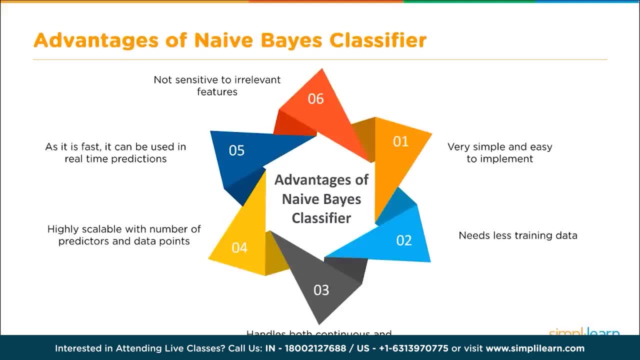 So, when you see data like this, it's necessary to move away from a 1D view of the data to a two-dimensional view of the data. So, when you see data like this, it's necessary to move away from a 1D view of the data to a two-dimensional view of the data. 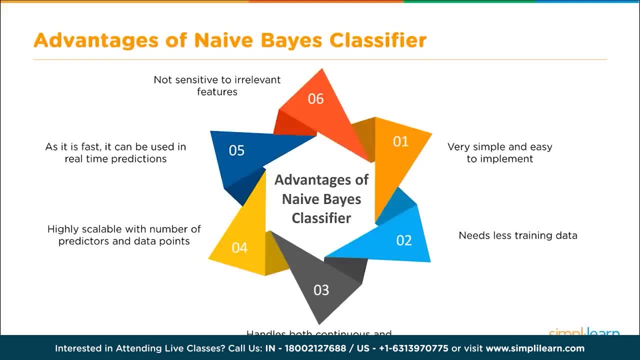 So, when you see data like this, it's necessary to move away from a 1D view of the data to a two-dimensional view of the data. So, when you see data like this, it's necessary to move away from a 1D view of the data to a two-dimensional view of the data. 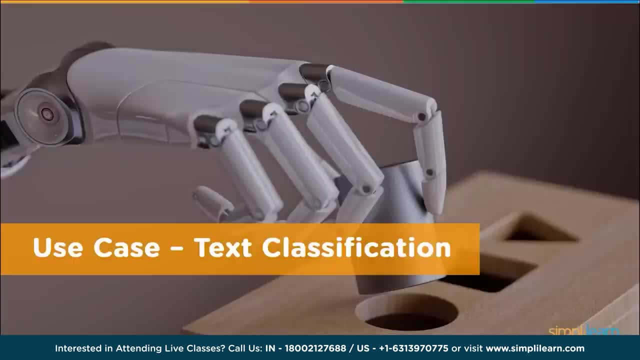 So, when you see data like this, it's necessary to move away from a 1D view of the data to a two-dimensional view of the data. So, when you see data like this, it's necessary to move away from a 1D view of the data to a two-dimensional view of the data. 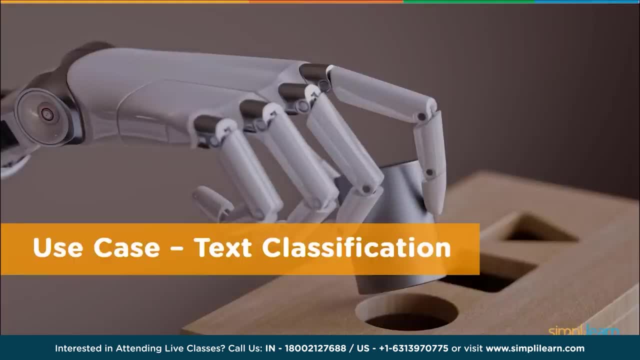 So, when you see data like this, it's necessary to move away from a 1D view of the data to a two-dimensional view of the data. So, when you see data like this, it's necessary to move away from a 1D view of the data to a two-dimensional view of the data. 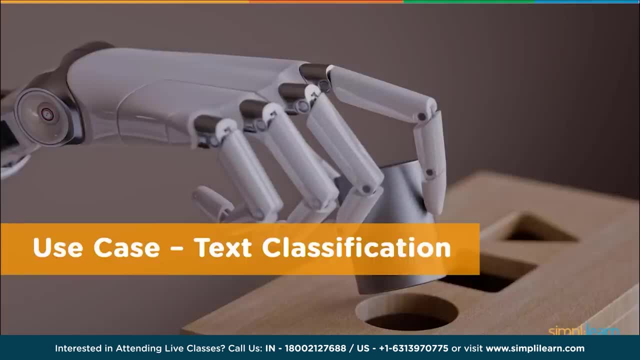 So, when you see data like this, it's necessary to move away from a 1D view of the data to a two-dimensional view of the data. So, when you see data like this, it's necessary to move away from a 1D view of the data to a two-dimensional view of the data. 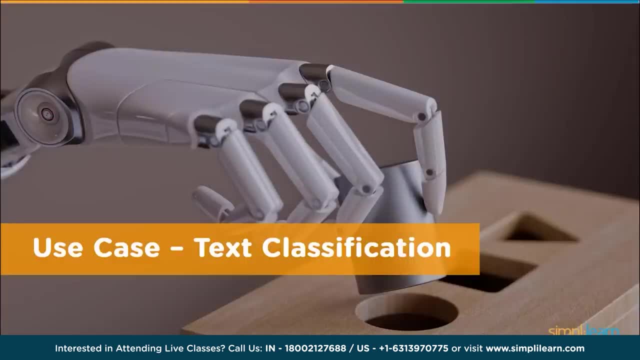 So, when you see data like this, it's necessary to move away from a 1D view of the data to a two-dimensional view of the data. So, when you see data like this, it's necessary to move away from a 1D view of the data to a two-dimensional view of the data. 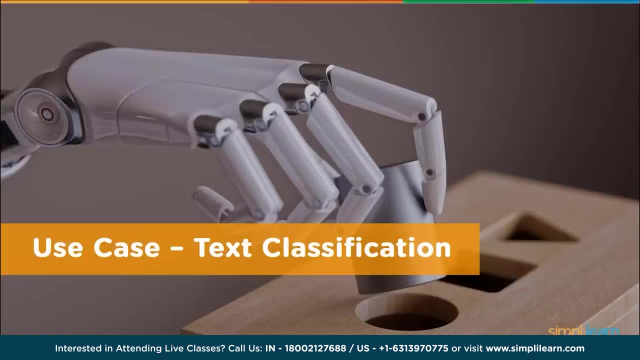 So, when you see data like this, it's necessary to move away from a 1D view of the data to a two-dimensional view of the data. So, when you see data like this, it's necessary to move away from a 1D view of the data to a two-dimensional view of the data. 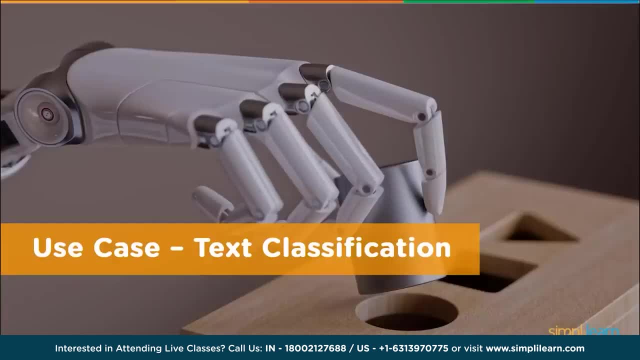 So, when you see data like this, it's necessary to move away from a 1D view of the data to a two-dimensional view of the data. So, when you see data like this, it's necessary to move away from a 1D view of the data to a two-dimensional view of the data. 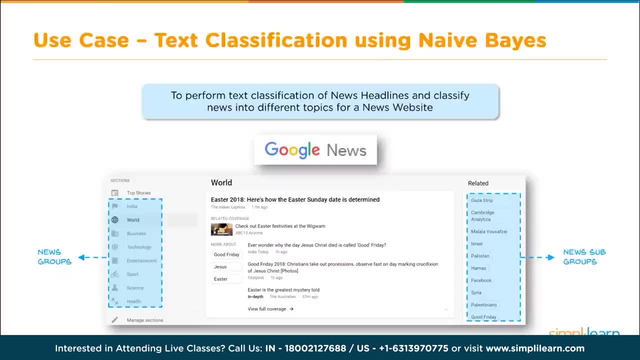 So, when you see data like this, it's necessary to move away from a 1D view of the data to a two-dimensional view of the data. So, when you see data like this, it's necessary to move away from a 1D view of the data to a two-dimensional view of the data. 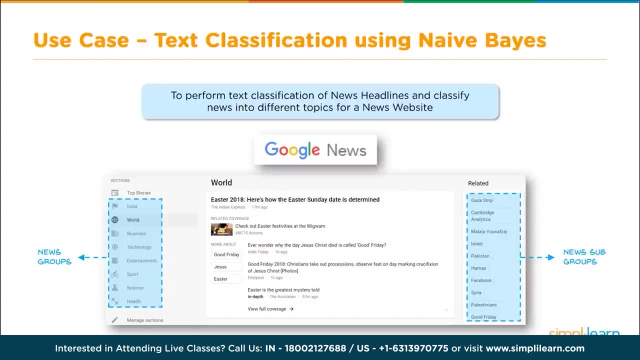 So, when you see data like this, it's necessary to move away from a 1D view of the data to a two-dimensional view of the data. So, when you see data like this, it's necessary to move away from a 1D view of the data to a two-dimensional view of the data. 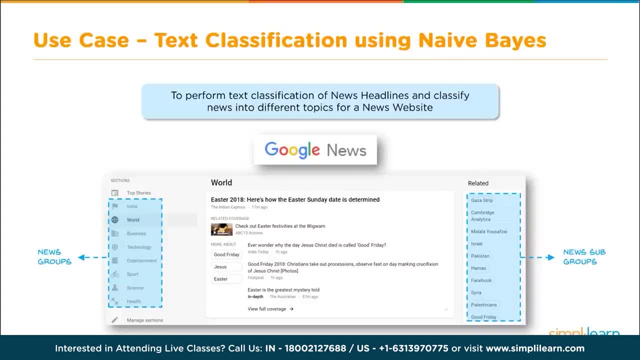 So, when you see data like this, it's necessary to move away from a 1D view of the data to a two-dimensional view of the data. So, when you see data like this, it's necessary to move away from a 1D view of the data to a two-dimensional view of the data. 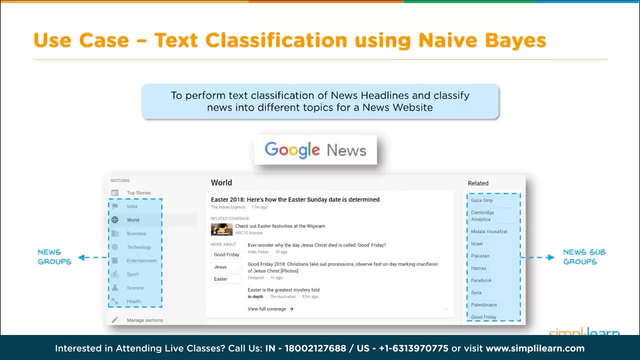 So, when you see data like this, it's necessary to move away from a 1D view of the data to a two-dimensional view of the data. So, when you see data like this, it's necessary to move away from a 1D view of the data to a two-dimensional view of the data. 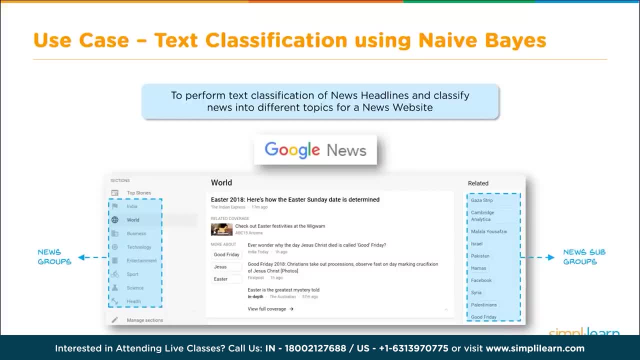 So, when you see data like this, it's necessary to move away from a 1D view of the data to a two-dimensional view of the data. So, when you see data like this, it's necessary to move away from a 1D view of the data to a two-dimensional view of the data. 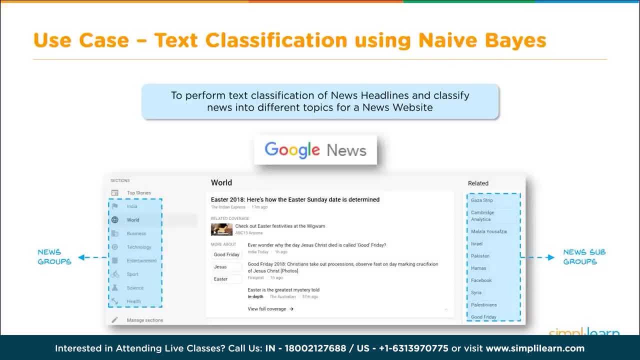 So, when you see data like this, it's necessary to move away from a 1D view of the data to a two-dimensional view of the data. So, when you see data like this, it's necessary to move away from a 1D view of the data to a two-dimensional view of the data. 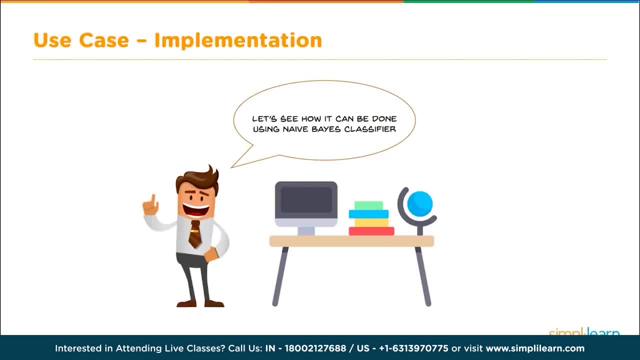 So, when you see data like this, it's necessary to move away from a 1D view of the data to a two-dimensional view of the data. So, when you see data like this, it's necessary to move away from a 1D view of the data to a two-dimensional view of the data. 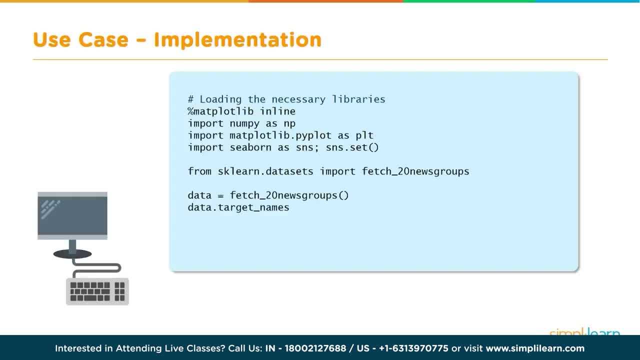 So, when you see data like this, it's necessary to move away from a 1D view of the data to a two-dimensional view of the data. So, when you see data like this, it's necessary to move away from a 1D view of the data to a two-dimensional view of the data. 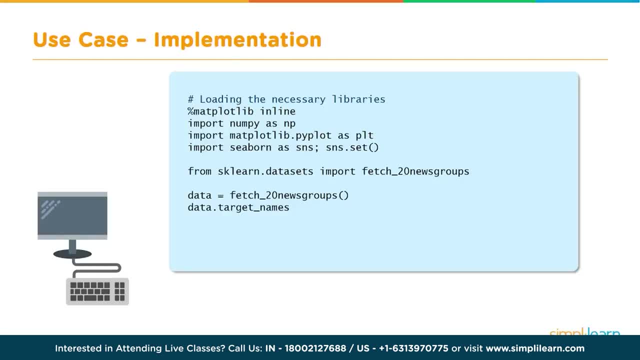 So, when you see data like this, it's necessary to move away from a 1D view of the data to a two-dimensional view of the data. So, when you see data like this, it's necessary to move away from a 1D view of the data to a two-dimensional view of the data. 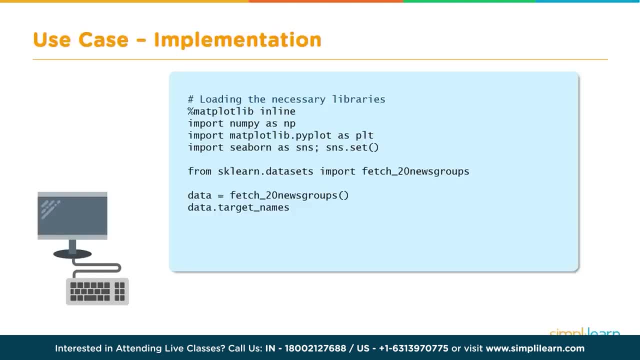 So, when you see data like this, it's necessary to move away from a 1D view of the data to a two-dimensional view of the data. So, when you see data like this, it's necessary to move away from a 1D view of the data to a two-dimensional view of the data. 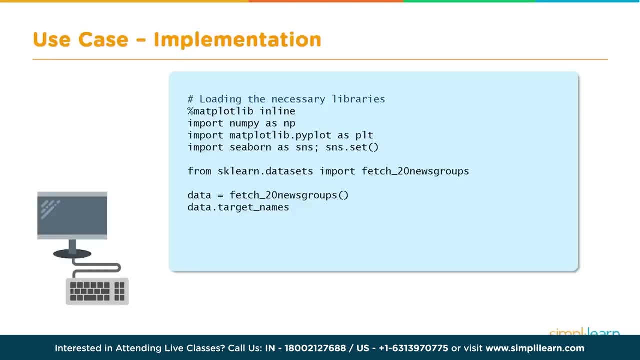 So, when you see data like this, it's necessary to move away from a 1D view of the data to a two-dimensional view of the data. So, when you see data like this, it's necessary to move away from a 1D view of the data to a two-dimensional view of the data. 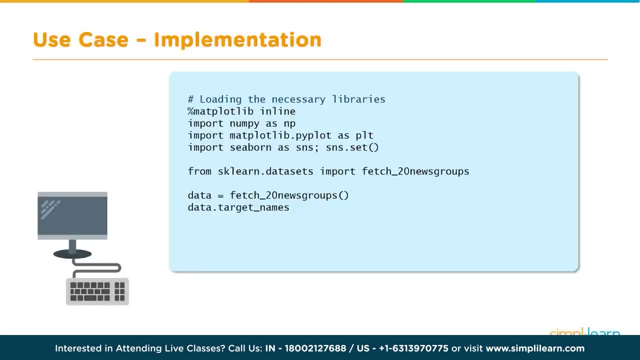 So, when you see data like this, it's necessary to move away from a 1D view of the data to a two-dimensional view of the data. So, when you see data like this, it's necessary to move away from a 1D view of the data to a two-dimensional view of the data. 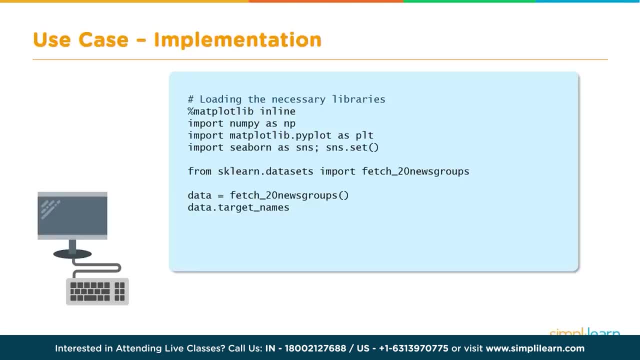 So, when you see data like this, it's necessary to move away from a 1D view of the data to a two-dimensional view of the data. So, when you see data like this, it's necessary to move away from a 1D view of the data to a two-dimensional view of the data. 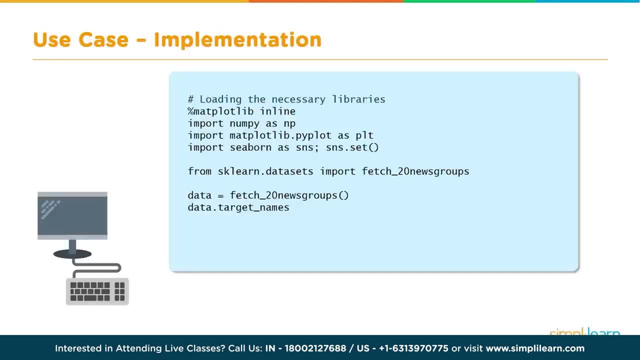 So, when you see data like this, it's necessary to move away from a 1D view of the data to a two-dimensional view of the data. So, when you see data like this, it's necessary to move away from a 1D view of the data to a two-dimensional view of the data. 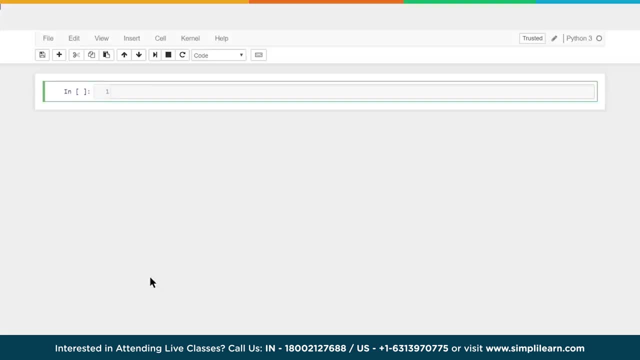 So, when you see data like this, it's necessary to move away from a 1D view of the data to a two-dimensional view of the data. So, when you see data like this, it's necessary to move away from a 1D view of the data to a two-dimensional view of the data. 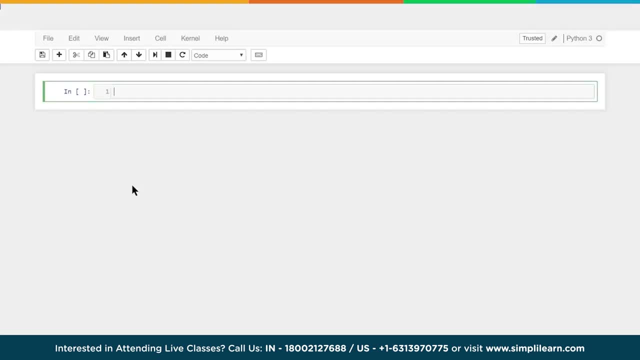 So, when you see data like this, it's necessary to move away from a 1D view of the data to a two-dimensional view of the data. So, when you see data like this, it's necessary to move away from a 1D view of the data to a two-dimensional view of the data. 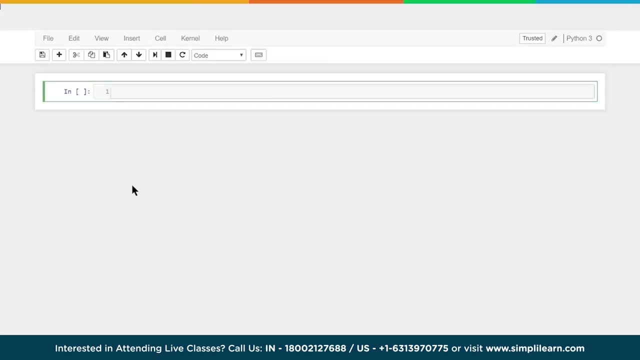 So, when you see data like this, it's necessary to move away from a 1D view of the data to a two-dimensional view of the data. So, when you see data like this, it's necessary to move away from a 1D view of the data to a two-dimensional view of the data. 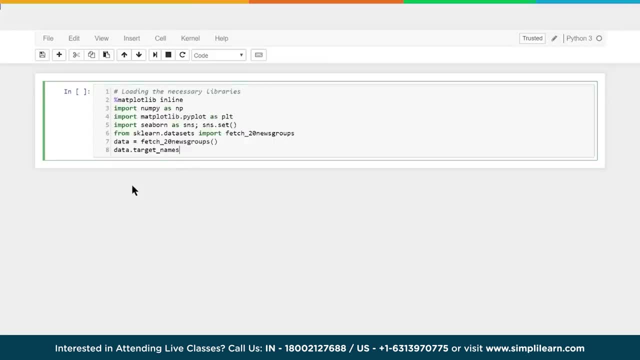 So, when you see data like this, it's necessary to move away from a 1D view of the data to a two-dimensional view of the data. So, when you see data like this, it's necessary to move away from a 1D view of the data to a two-dimensional view of the data. 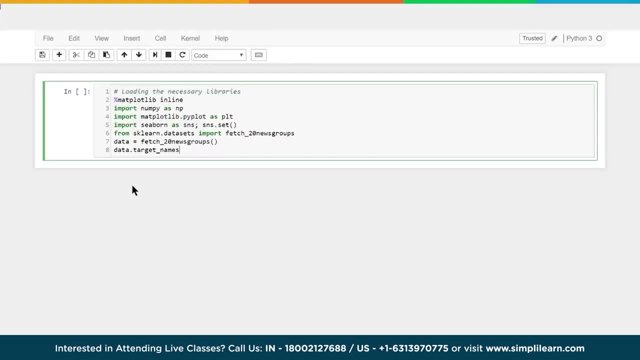 So, when you see data like this, it's necessary to move away from a 1D view of the data to a two-dimensional view of the data. So, when you see data like this, it's necessary to move away from a 1D view of the data to a two-dimensional view of the data. 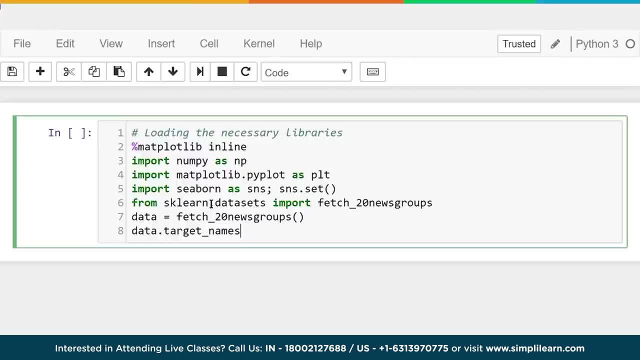 So, when you see data like this, it's necessary to move away from a 1D view of the data to a two-dimensional view of the data. So, when you see data like this, it's necessary to move away from a 1D view of the data to a two-dimensional view of the data. 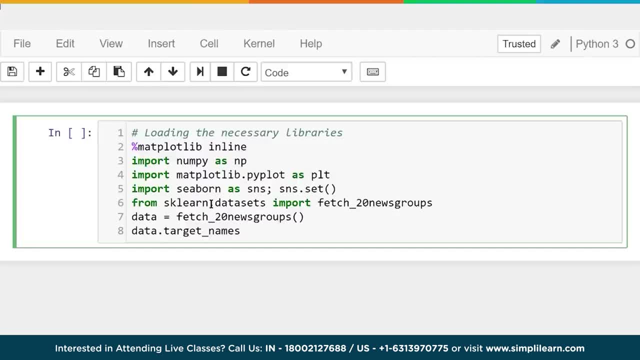 So, when you see data like this, it's necessary to move away from a 1D view of the data to a two-dimensional view of the data. So, when you see data like this, it's necessary to move away from a 1D view of the data to a two-dimensional view of the data. 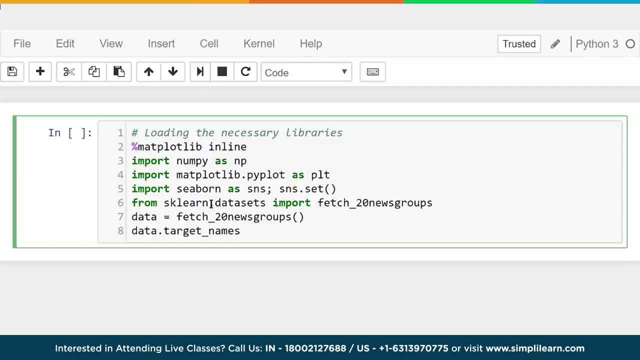 So, when you see data like this, it's necessary to move away from a 1D view of the data to a two-dimensional view of the data. So, when you see data like this, it's necessary to move away from a 1D view of the data to a two-dimensional view of the data. 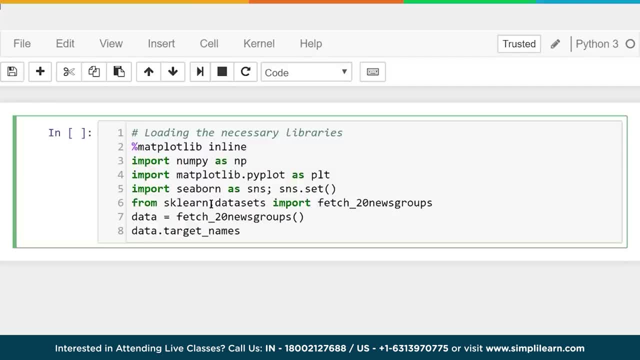 So, when you see data like this, it's necessary to move away from a 1D view of the data to a two-dimensional view of the data. So, when you see data like this, it's necessary to move away from a 1D view of the data to a two-dimensional view of the data. 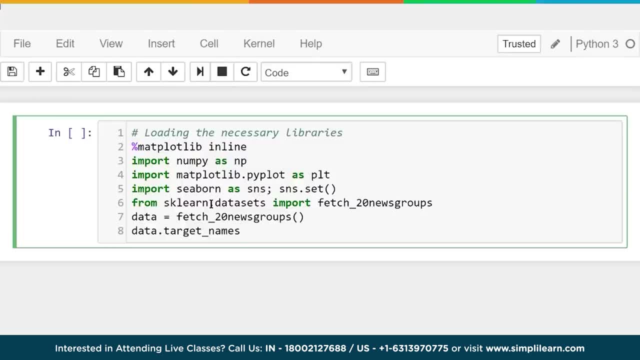 So, when you see data like this, it's necessary to move away from a 1D view of the data to a two-dimensional view of the data. So, when you see data like this, it's necessary to move away from a 1D view of the data to a two-dimensional view of the data. 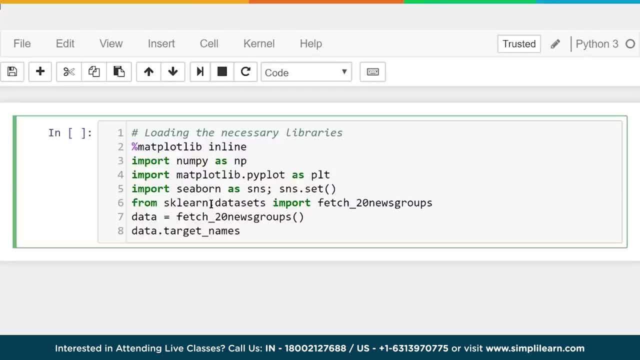 So, when you see data like this, it's necessary to move away from a 1D view of the data to a two-dimensional view of the data. So, when you see data like this, it's necessary to move away from a 1D view of the data to a two-dimensional view of the data. 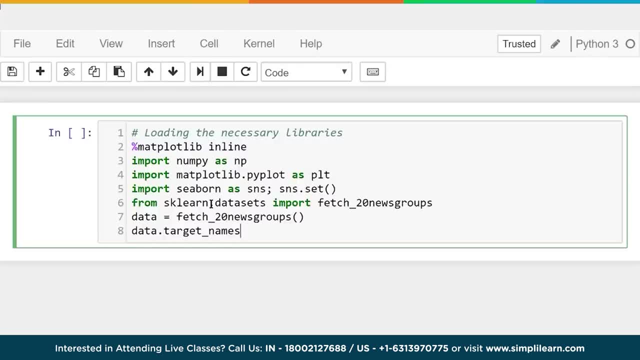 So, when you see data like this, it's necessary to move away from a 1D view of the data to a two-dimensional view of the data. So, when you see data like this, it's necessary to move away from a 1D view of the data to a two-dimensional view of the data. 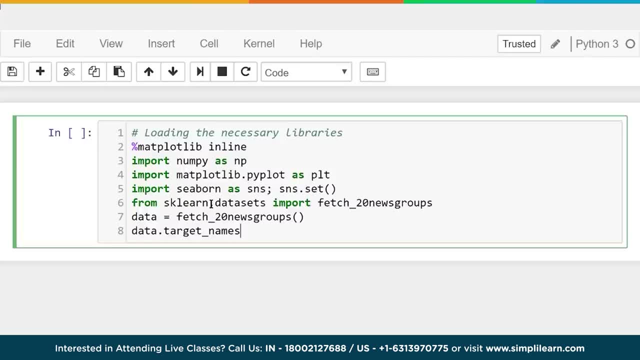 So, when you see data like this, it's necessary to move away from a 1D view of the data to a two-dimensional view of the data. So, when you see data like this, it's necessary to move away from a 1D view of the data to a two-dimensional view of the data. 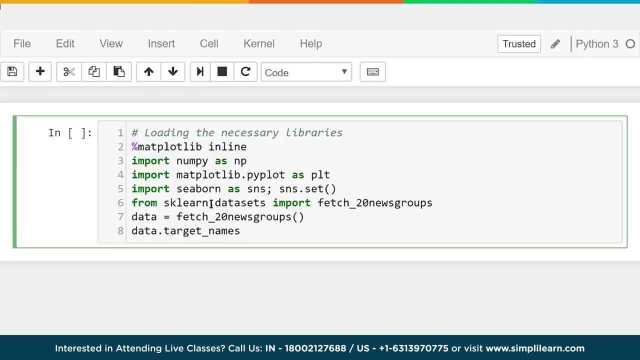 So, when you see data like this, it's necessary to move away from a 1D view of the data to a two-dimensional view of the data. So, when you see data like this, it's necessary to move away from a 1D view of the data to a two-dimensional view of the data. 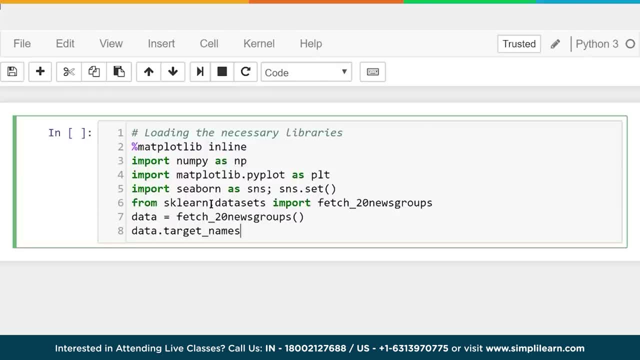 So, when you see data like this, it's necessary to move away from a 1D view of the data to a two-dimensional view of the data. So, when you see data like this, it's necessary to move away from a 1D view of the data to a two-dimensional view of the data. 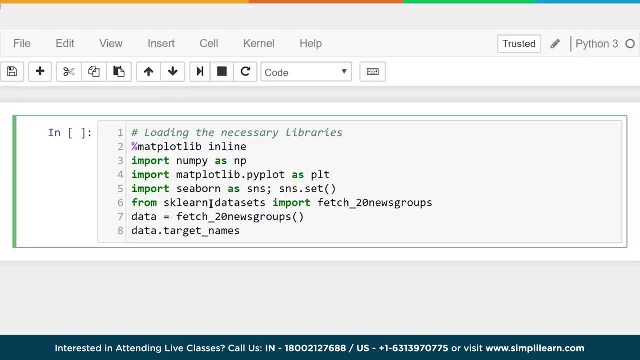 So, when you see data like this, it's necessary to move away from a 1D view of the data to a two-dimensional view of the data. So, when you see data like this, it's necessary to move away from a 1D view of the data to a two-dimensional view of the data. 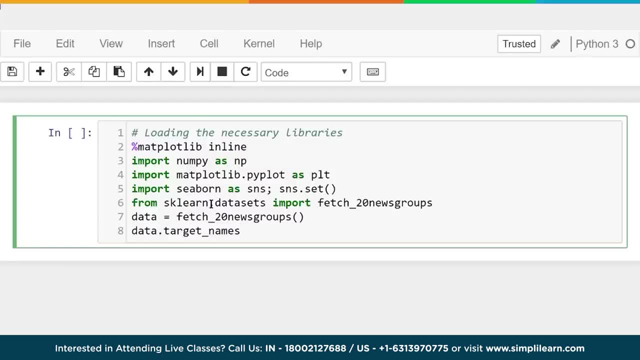 So, when you see data like this, it's necessary to move away from a 1D view of the data to a two-dimensional view of the data. So, when you see data like this, it's necessary to move away from a 1D view of the data to a two-dimensional view of the data. 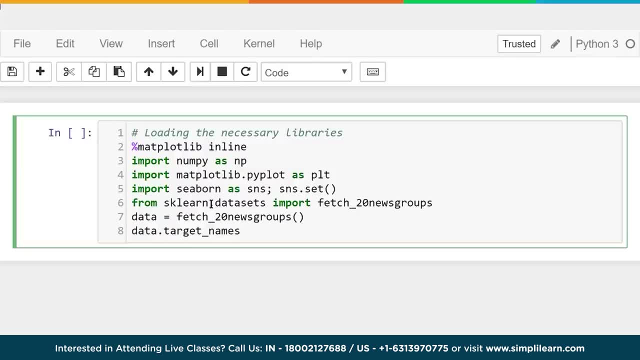 So, when you see data like this, it's necessary to move away from a 1D view of the data to a two-dimensional view of the data. So, when you see data like this, it's necessary to move away from a 1D view of the data to a two-dimensional view of the data. 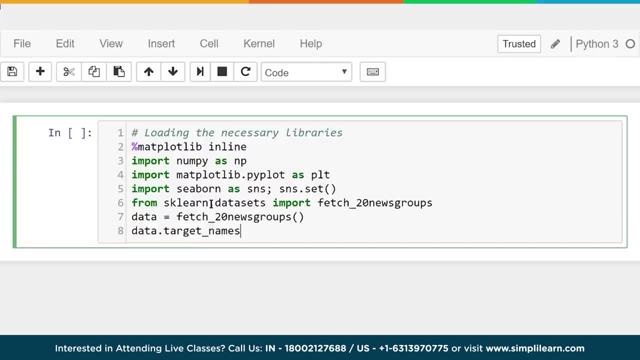 So, when you see data like this, it's necessary to move away from a 1D view of the data to a two-dimensional view of the data. So, when you see data like this, it's necessary to move away from a 1D view of the data to a two-dimensional view of the data. 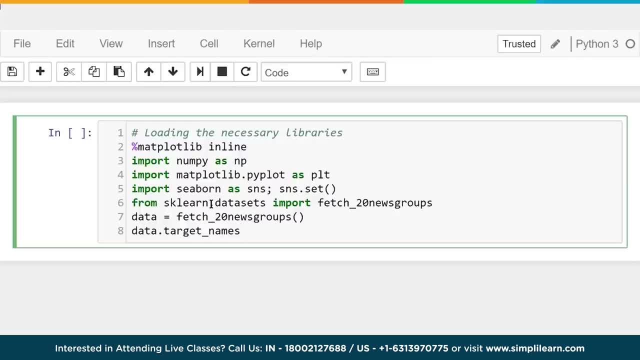 So, when you see data like this, it's necessary to move away from a 1D view of the data to a two-dimensional view of the data. So, when you see data like this, it's necessary to move away from a 1D view of the data to a two-dimensional view of the data. 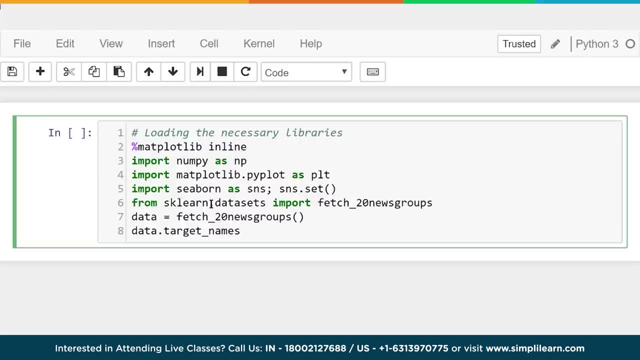 So, when you see data like this, it's necessary to move away from a 1D view of the data to a two-dimensional view of the data. So, when you see data like this, it's necessary to move away from a 1D view of the data to a two-dimensional view of the data. 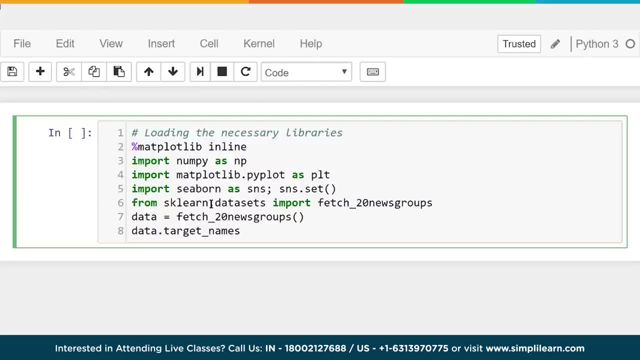 So, when you see data like this, it's necessary to move away from a 1D view of the data to a two-dimensional view of the data. So, when you see data like this, it's necessary to move away from a 1D view of the data to a two-dimensional view of the data. 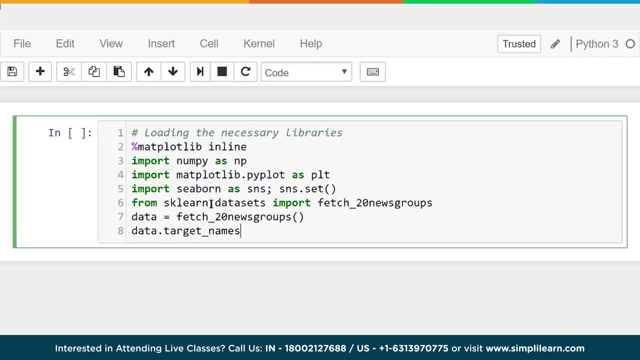 So, when you see data like this, it's necessary to move away from a 1D view of the data to a two-dimensional view of the data. So, when you see data like this, it's necessary to move away from a 1D view of the data to a two-dimensional view of the data. 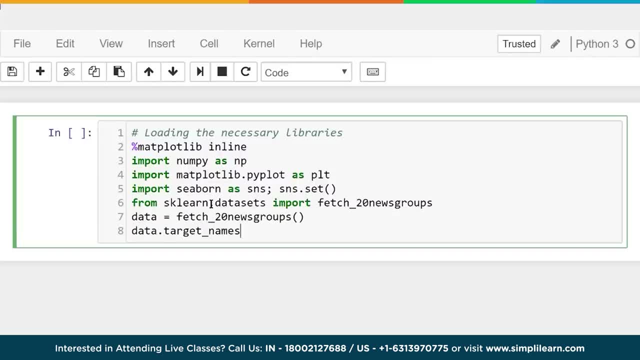 So, when you see data like this, it's necessary to move away from a 1D view of the data to a two-dimensional view of the data. So, when you see data like this, it's necessary to move away from a 1D view of the data to a two-dimensional view of the data. 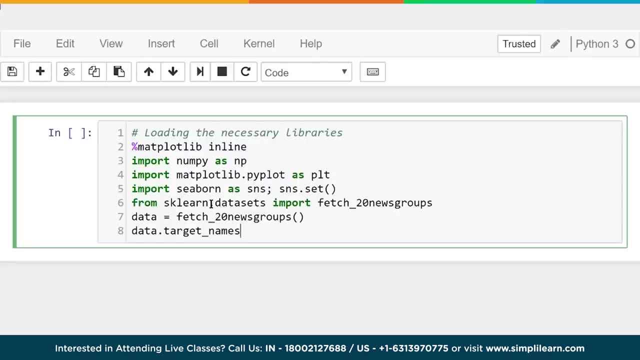 So, when you see data like this, it's necessary to move away from a 1D view of the data to a two-dimensional view of the data. So, when you see data like this, it's necessary to move away from a 1D view of the data to a two-dimensional view of the data. 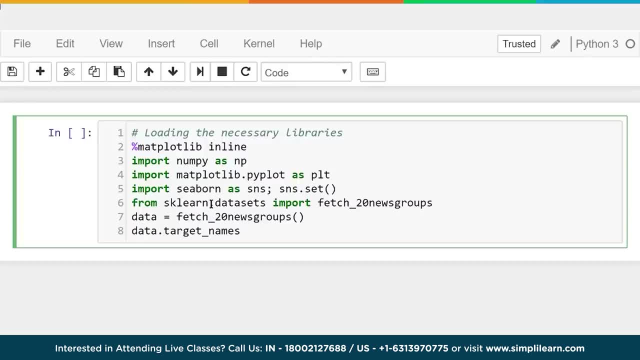 So, when you see data like this, it's necessary to move away from a 1D view of the data to a two-dimensional view of the data. So, when you see data like this, it's necessary to move away from a 1D view of the data to a two-dimensional view of the data. 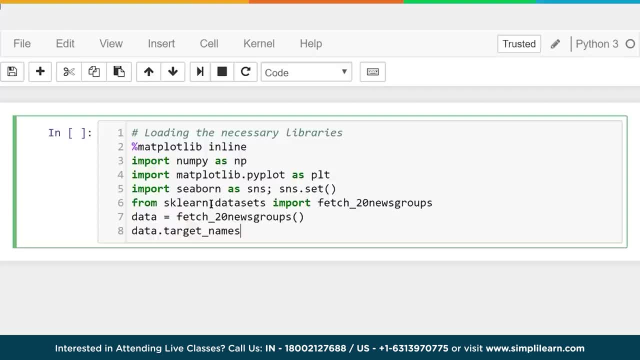 So, when you see data like this, it's necessary to move away from a 1D view of the data to a two-dimensional view of the data. So, when you see data like this, it's necessary to move away from a 1D view of the data to a two-dimensional view of the data. 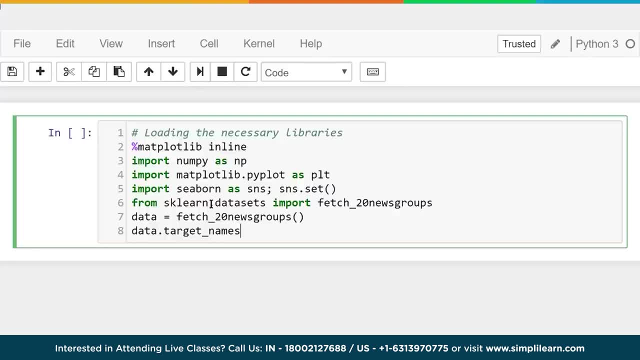 So, when you see data like this, it's necessary to move away from a 1D view of the data to a two-dimensional view of the data. So, when you see data like this, it's necessary to move away from a 1D view of the data to a two-dimensional view of the data. 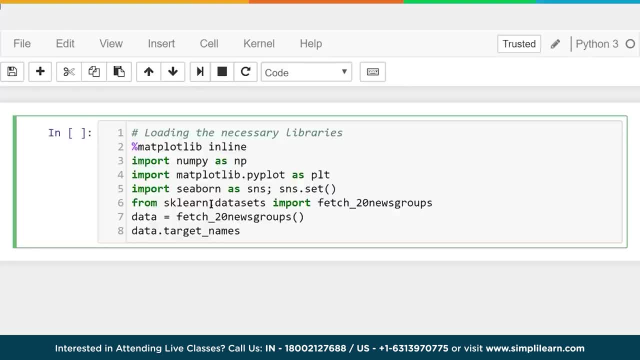 So, when you see data like this, it's necessary to move away from a 1D view of the data to a two-dimensional view of the data. So, when you see data like this, it's necessary to move away from a 1D view of the data to a two-dimensional view of the data. 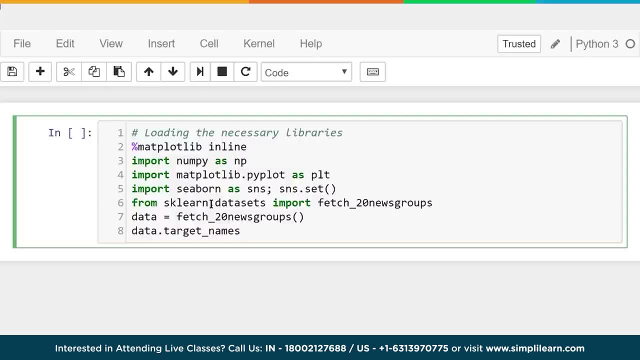 So, when you see data like this, it's necessary to move away from a 1D view of the data to a two-dimensional view of the data. So, when you see data like this, it's necessary to move away from a 1D view of the data to a two-dimensional view of the data. 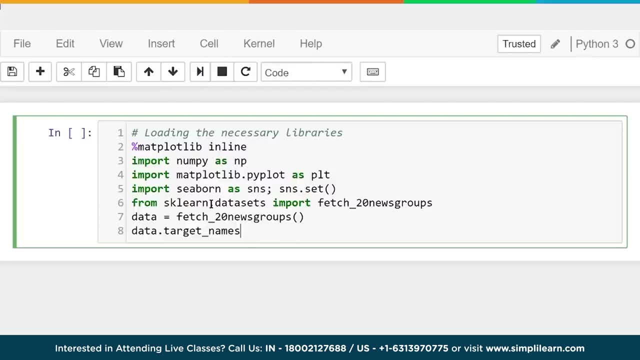 So, when you see data like this, it's necessary to move away from a 1D view of the data to a two-dimensional view of the data. So, when you see data like this, it's necessary to move away from a 1D view of the data to a two-dimensional view of the data. 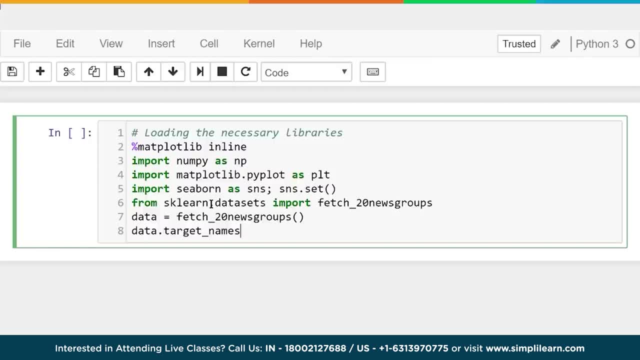 So, when you see data like this, it's necessary to move away from a 1D view of the data to a two-dimensional view of the data. So, when you see data like this, it's necessary to move away from a 1D view of the data to a two-dimensional view of the data. 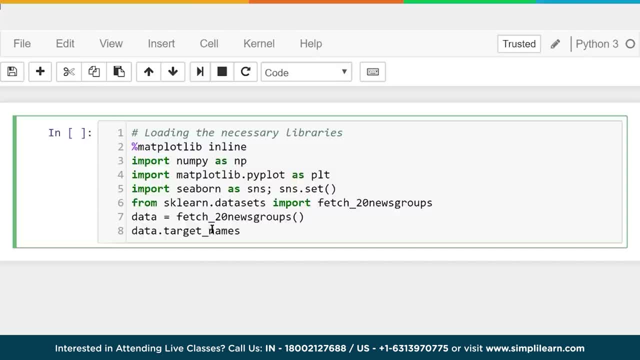 So, when you see data like this, it's necessary to move away from a 1D view of the data to a two-dimensional view of the data. So, when you see data like this, it's necessary to move away from a 1D view of the data to a two-dimensional view of the data. 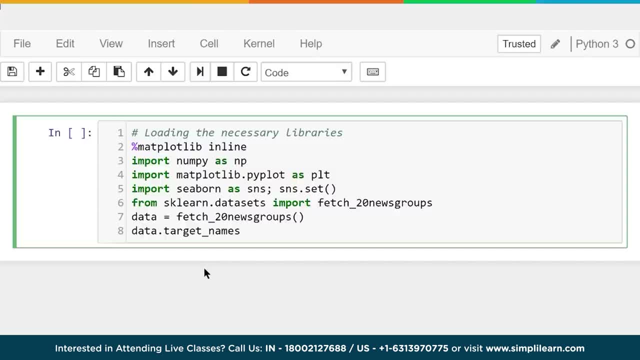 So, when you see data like this, it's necessary to move away from a 1D view of the data to a two-dimensional view of the data. So, when you see data like this, it's necessary to move away from a 1D view of the data to a two-dimensional view of the data. 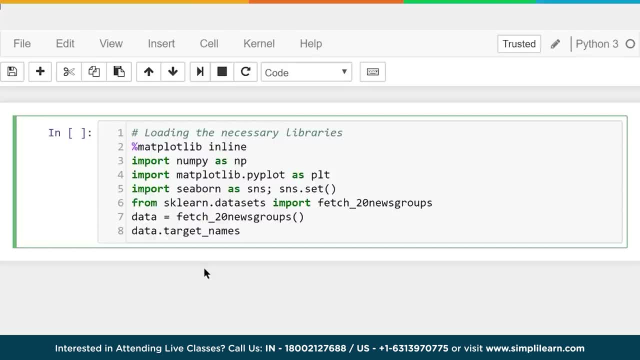 So, when you see data like this, it's necessary to move away from a 1D view of the data to a two-dimensional view of the data. So, when you see data like this, it's necessary to move away from a 1D view of the data to a two-dimensional view of the data. 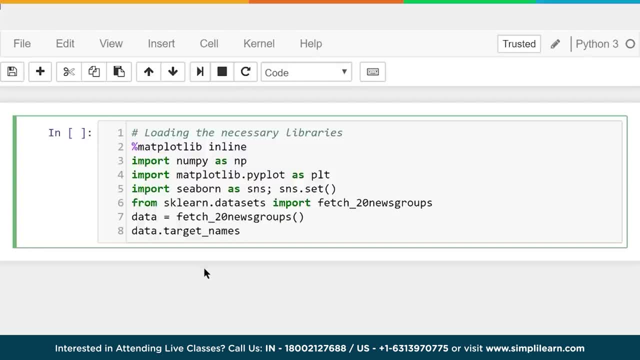 So, when you see data like this, it's necessary to move away from a 1D view of the data to a two-dimensional view of the data. So, when you see data like this, it's necessary to move away from a 1D view of the data to a two-dimensional view of the data. 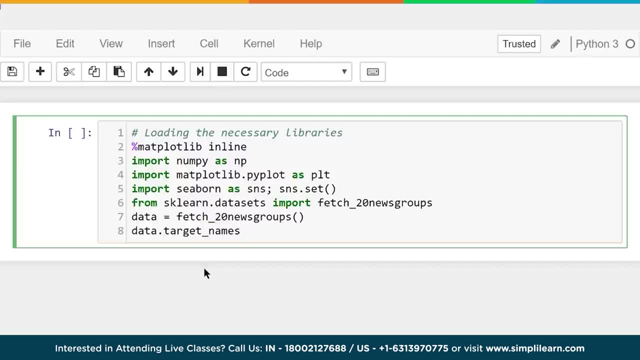 So, when you see data like this, it's necessary to move away from a 1D view of the data to a two-dimensional view of the data. So, when you see data like this, it's necessary to move away from a 1D view of the data to a two-dimensional view of the data. 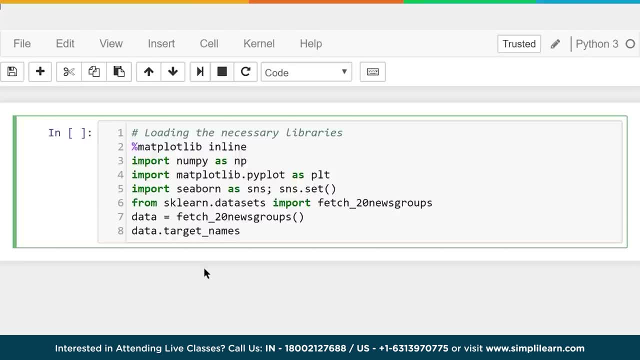 So, when you see data like this, it's necessary to move away from a 1D view of the data to a two-dimensional view of the data. So, when you see data like this, it's necessary to move away from a 1D view of the data to a two-dimensional view of the data. 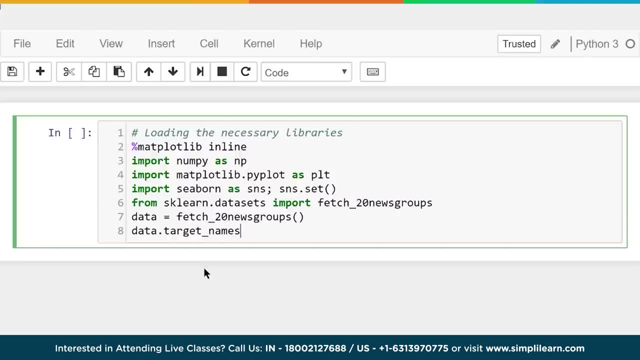 So, when you see data like this, it's necessary to move away from a 1D view of the data to a two-dimensional view of the data. So, when you see data like this, it's necessary to move away from a 1D view of the data to a two-dimensional view of the data. 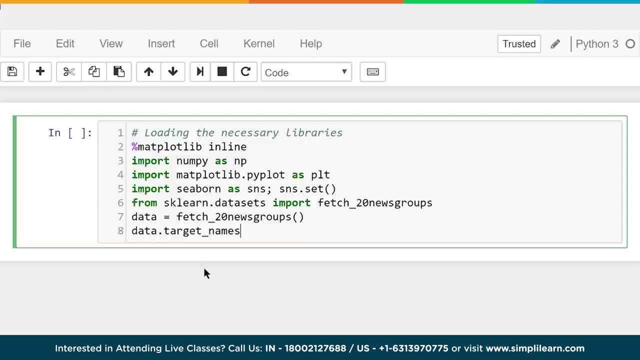 So, when you see data like this, it's necessary to move away from a 1D view of the data to a two-dimensional view of the data. So, when you see data like this, it's necessary to move away from a 1D view of the data to a two-dimensional view of the data. 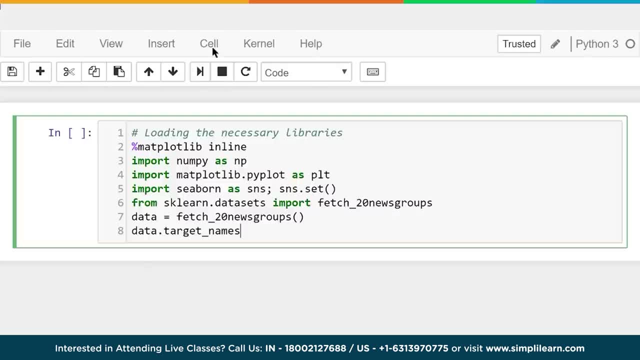 So, when you see data like this, it's necessary to move away from a 1D view of the data to a two-dimensional view of the data. So, when you see data like this, it's necessary to move away from a 1D view of the data to a two-dimensional view of the data. 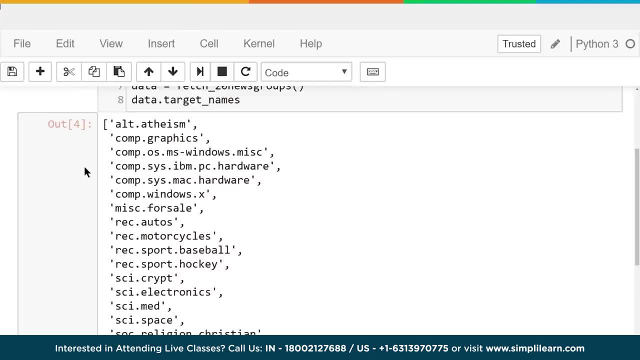 So, when you see data like this, it's necessary to move away from a 1D view of the data to a two-dimensional view of the data. So, when you see data like this, it's necessary to move away from a 1D view of the data to a two-dimensional view of the data. 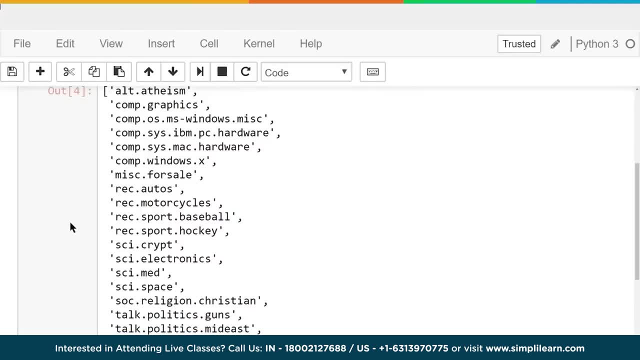 So, when you see data like this, it's necessary to move away from a 1D view of the data to a two-dimensional view of the data. So, when you see data like this, it's necessary to move away from a 1D view of the data to a two-dimensional view of the data. 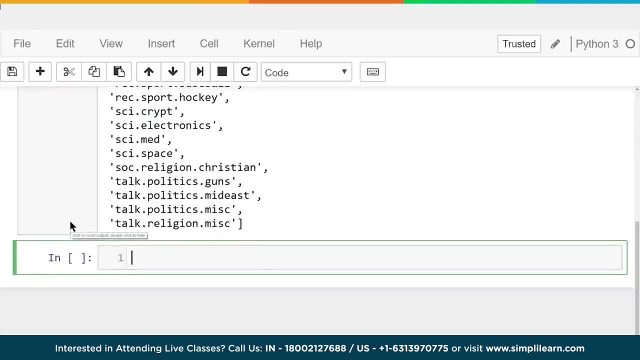 So, when you see data like this, it's necessary to move away from a 1D view of the data to a two-dimensional view of the data. So, when you see data like this, it's necessary to move away from a 1D view of the data to a two-dimensional view of the data. 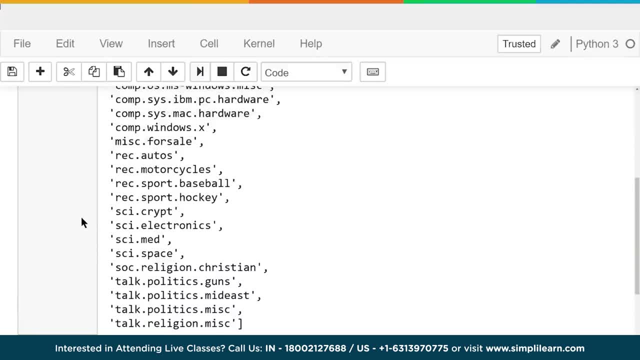 So, when you see data like this, it's necessary to move away from a 1D view of the data to a two-dimensional view of the data. So, when you see data like this, it's necessary to move away from a 1D view of the data to a two-dimensional view of the data. 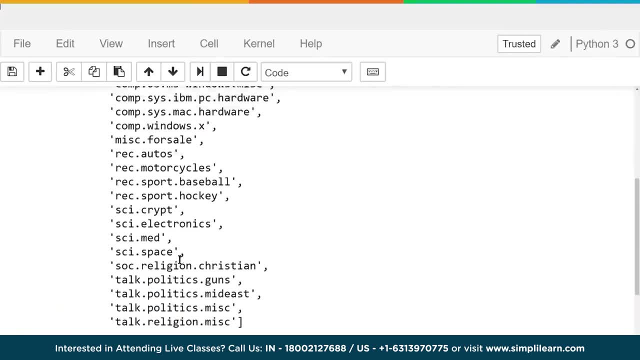 So when you see data like this, it's necessary to move away from a 1D view of the data to a two-dimensional view of the data, And it's called Fetch 20 because you'll see, there's- I believe there's 20 different topics in here, or 20 different categories as we scroll down. 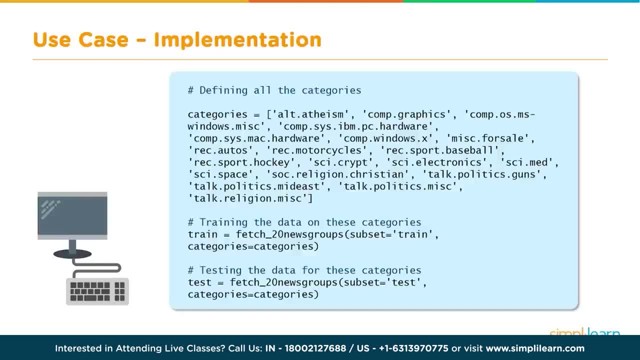 Now we've gone through the 20 different categories and we're going to go ahead and start defining all the categories and set up our data. So we're actually going to go ahead and get the data all set up and take a look at our data. 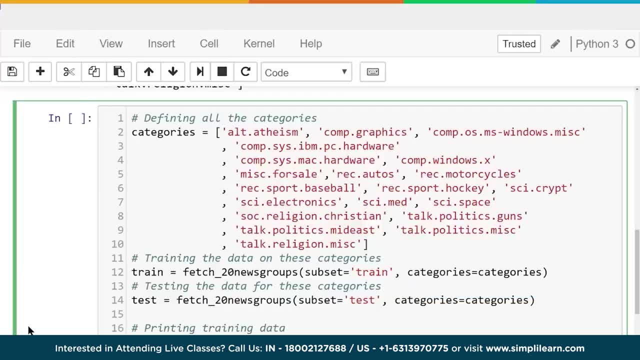 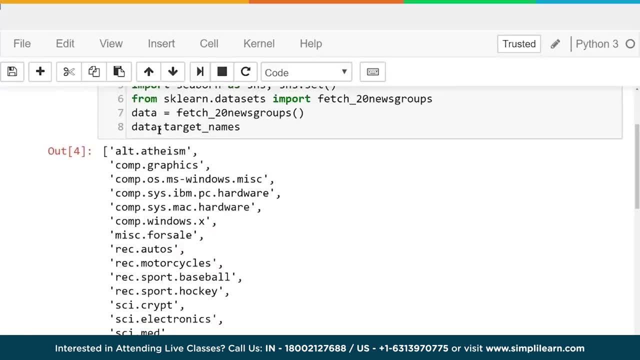 And let's move this over to our Jupyter notebook and let's see what this code does. First, we're going to set our categories. Now, if you noticed up here, I could have just as easily set this equal to datatarget underscore names, because it's the same thing. 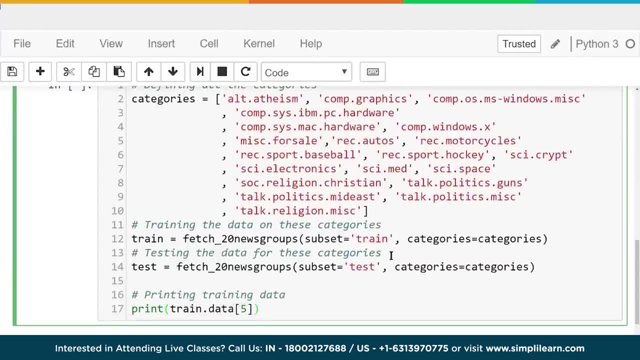 But we want to kind of spell it out for you so you can see the different categories. It kind of makes it more visual so you can see what your data is looking like in the background. Once we've created the categories, we're going to open up a train set. 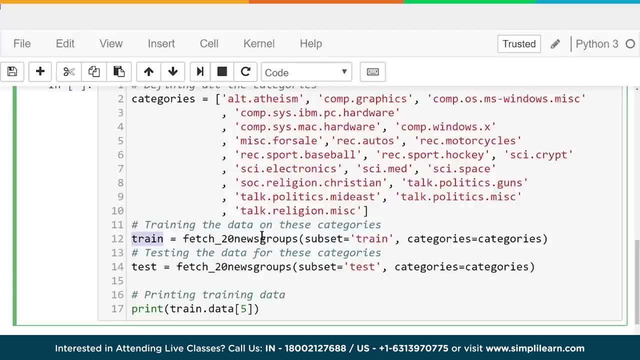 So this training set of data is going to go into Fetch 20 news groups and it's a subset in there called train, And categories equals categories. So we're pulling out those categories And then if you have a train set, you should also have the testing set. 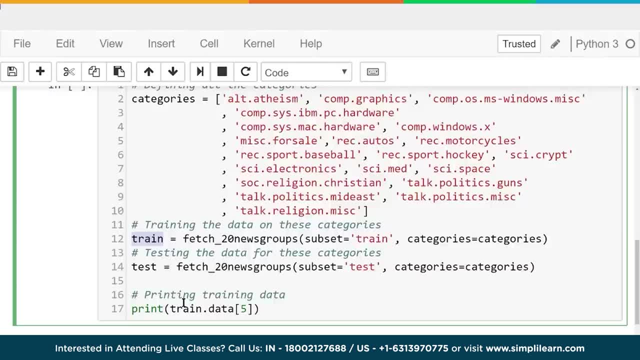 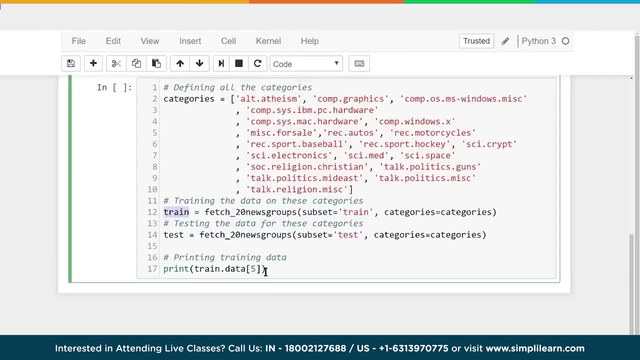 We have test equals Fetch, 20 news groups. subset equals test and categories equals categories. Let's go down one size so it all fits on my screen. There we go, And just so we can really see what's going on. let's see what happens when we print out one part of that data. 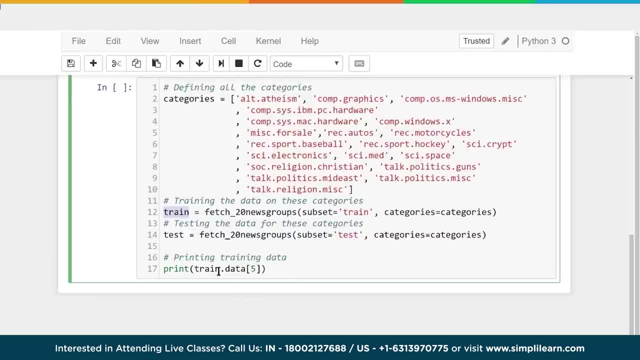 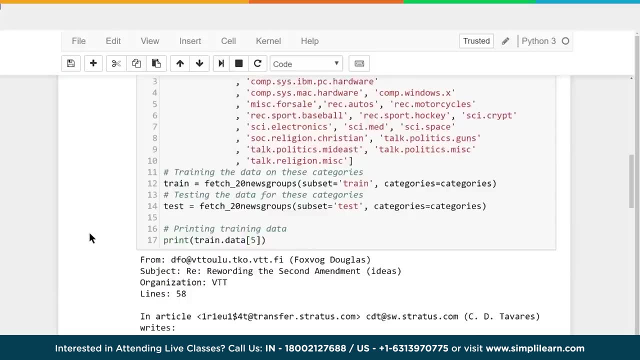 So it creates train and under train it creates traindata. And we're just going to look at data piece number five And let's go ahead and run that and see what that looks like. And you can see When I print traindata number five under train it prints out one of the articles. 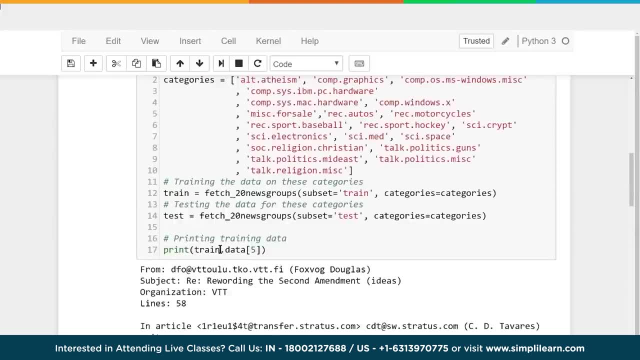 This is article number five. You can go through and read it on there And we can also go in here and change this to test, which should look identical because it's splitting the data up into different groups. train and test And we'll see test. number five is a different article, but it's another article in here. 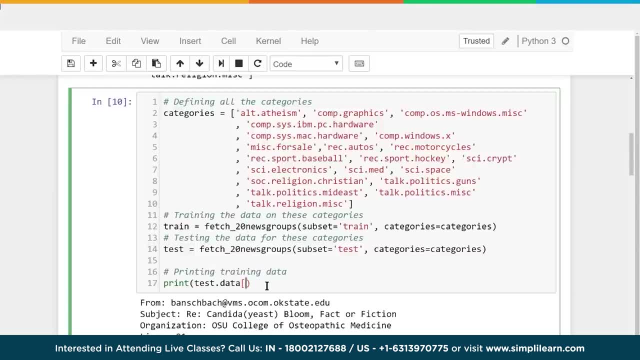 And maybe you're curious and you want to see just how many articles are in here. We could do length of traindata And we'll see. And if we run that, you'll see that the training data has 11,314 articles. 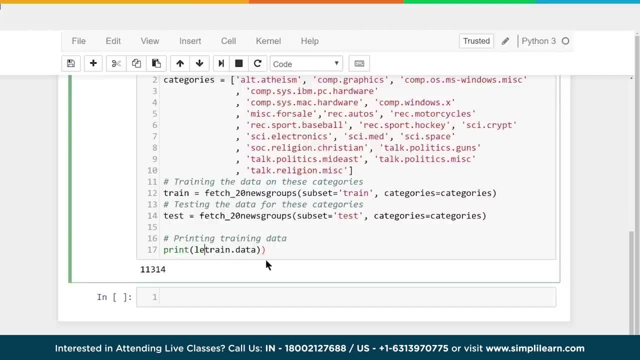 So we're not going to go through all those articles. That's a lot of articles- But we can look at one of them just so you can see what kind of information is coming out of it and what we're looking at. And we'll just look at number five for today. 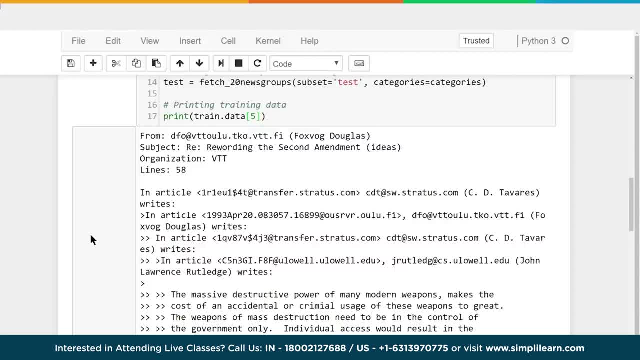 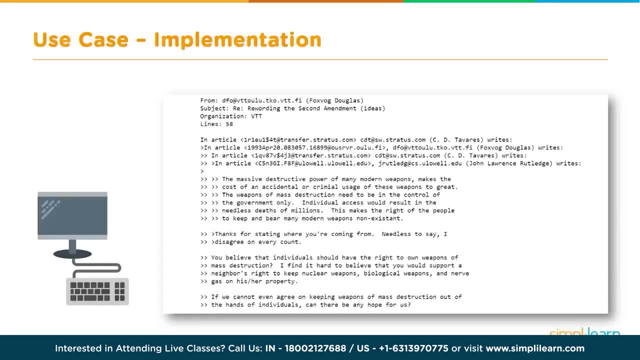 And here we have it, rewording the Second Amendment: IDs VTT, line 58, lines 58 in article et cetera, And you can scroll all the way down and see all the different parts to there. Now we've looked at it and that's pretty complicated. 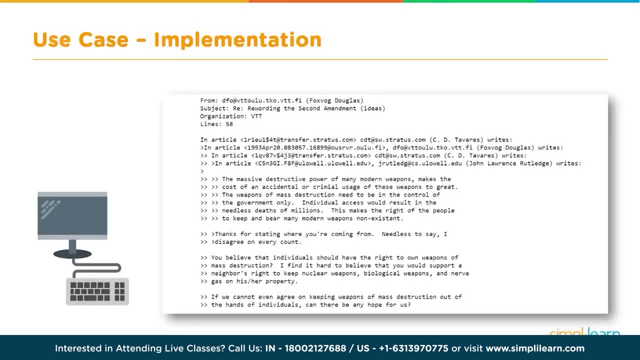 When you look at one of these articles to try to figure out how do you weight this. If you look down here, we have different words and maybe the word from- Well from- is probably in all the articles, So it's not going to have a lot of meaning. as far as trying to figure out whether this article fits one of the categories or not, 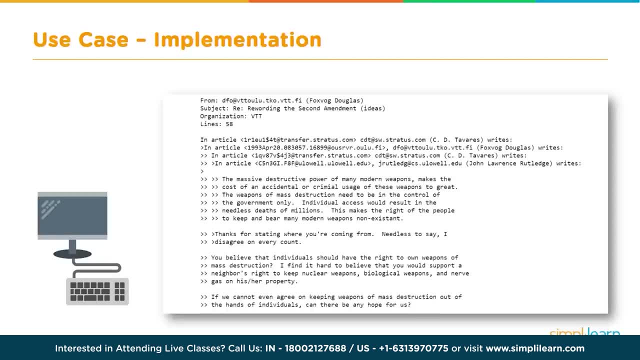 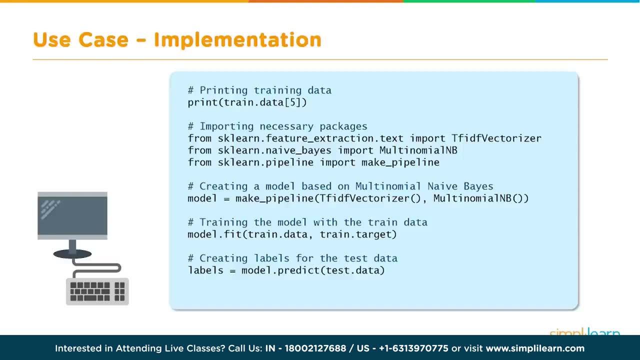 So trying to figure out which category it fits in based on these words is where the challenge comes in. Now that we've viewed our data, we're going to dive in and do the actual predictions. This is the actual naive base, And we're going to throw another model at you or another module at you here in just a second. 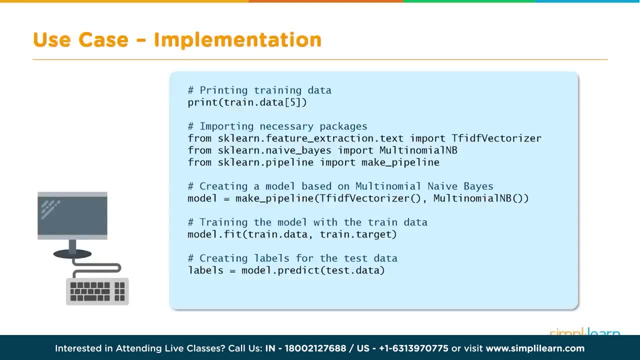 We can't go into too much detail, but it deals specifically working with words and text and what they call tokenizing those words. So let's take this code and let's skip on over to our Jupyter notebook and walk through it, And here we are in our Jupyter notebook. 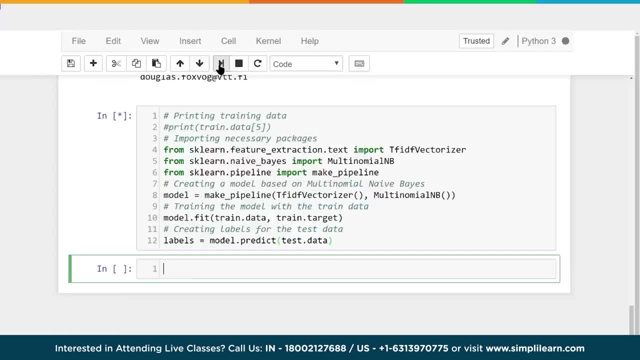 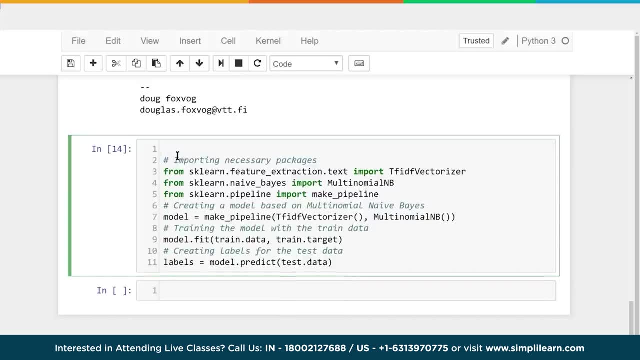 Let's paste that in there And I can run this code right off the bat. It's not actually going to display anything yet, but it has a lot going on in here. So the top: we had the print module from the earlier one. 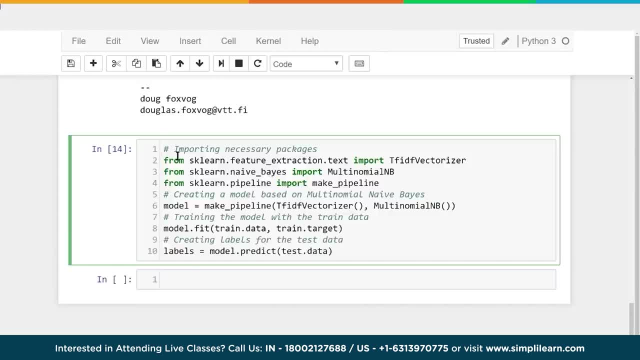 I didn't know why that was in there. So we're going to start by importing our necessary packages And from the sklearnfeaturesextractiontxt, we're going to import tfidfvectorizer. I told you we're going to throw a module at you. 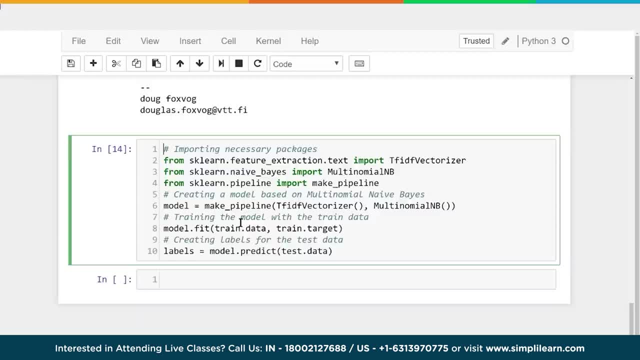 We can't go too much into the math behind this or how it works. You can look it up. The notation for the math is usually tfidf And that's just a way of weighing the words, And it weighs the words based on how many times they're used in a document. how many times or how many documents they're used in. 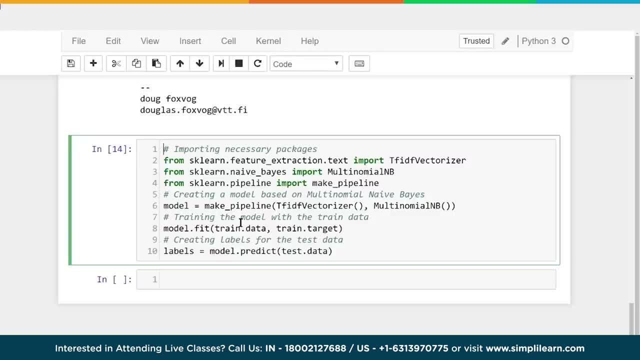 And it's a well-used formula. It's been around forever. It's been around for a while. It's a little confusing to put this in here, But let's let her know that it just goes in there and weights the different words in the document for us. 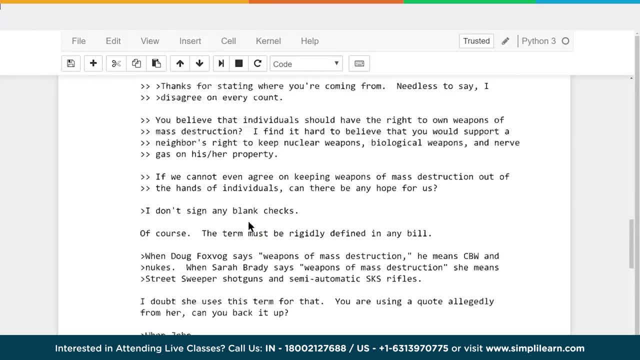 That way we don't have to wait. And if you put a weight on it- if you remember I was talking about that up here earlier- if these are all emails, they probably all have the word from in them. From probably has a very low weight. 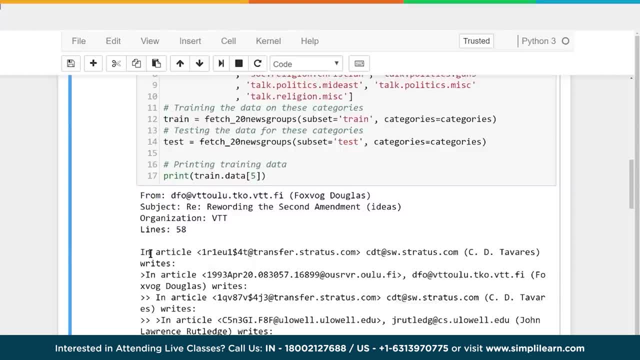 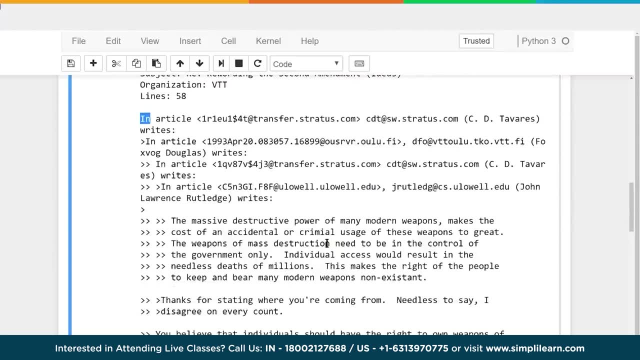 It has very little value in telling you what this document's about. Same with words like in, in, article, in, articles, in, cost of, on, maybe, cost might, or Or words like criminal, Criminal weapons destruction. these might have a heavier weight because you describe a little bit more what the article's doing. 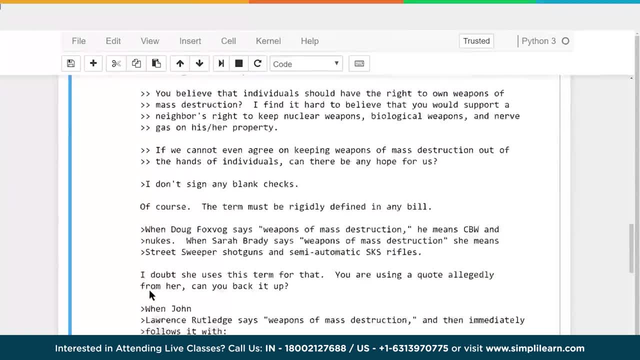 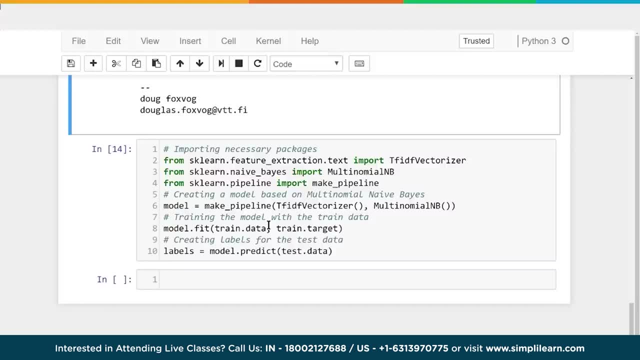 Well, how do you figure out all those weights in the different articles? That's what this module does, That's what the TF-IDF vectorizer is going to do for us. And then we're going to import our sklearnnaivebase and that's our multinomial NB, multinomial naive base. 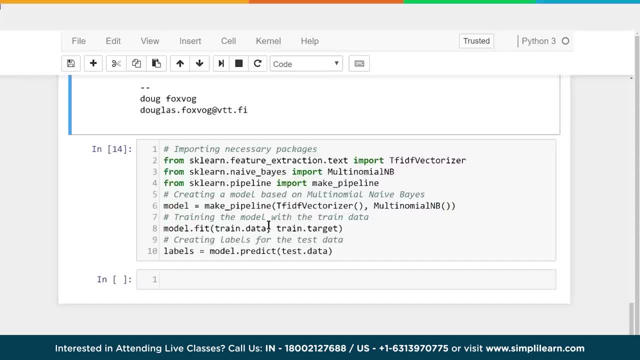 Pretty easy to understand that where that comes from. And then finally we have the sklearn pipeline, import Make pipeline. Now, the make pipeline is just a cool piece of code because we're going to take the information we get from the TF-IDF vectorizer and we're going to pump that into the multinomial NB. 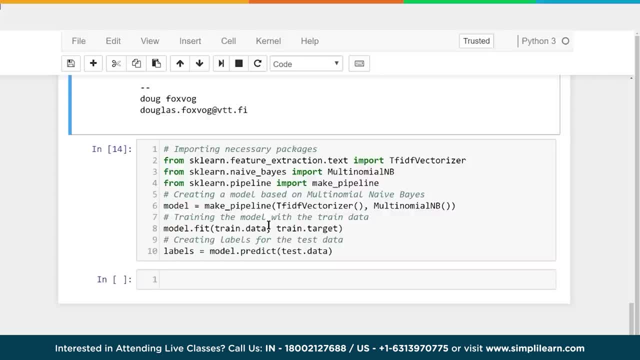 So a pipeline is just a way of organizing how things flow. It's used commonly. You probably already guessed what it is. If you've done any businesses, they talk about the sales pipeline. If you're on a work crew or project manager, you have your pipeline of information that's going through or your projects. 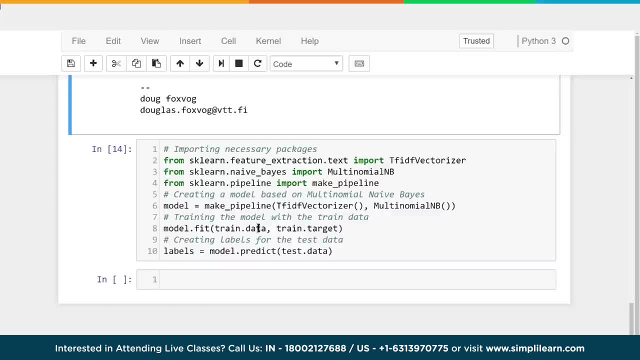 And what has to be done, in what order That's all this pipeline is. We're going to take the TF-ID vectorizer and then we're going to push that into the multinomial NB. Now we've designated that as the variable model. 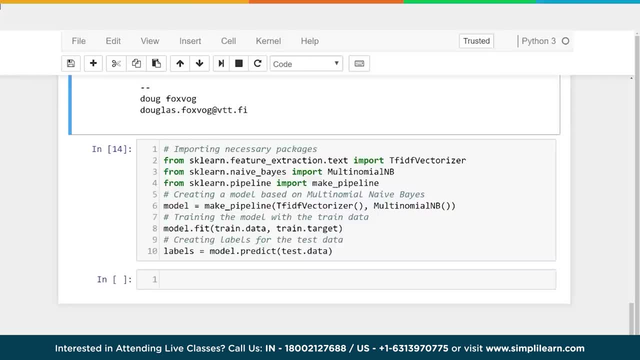 We have our pipeline model and we're going to take that model And this is just so elegant. This is done in just a couple of lines of code, Modelfit, And we're going to fit the data, and first the train data and then the train target. 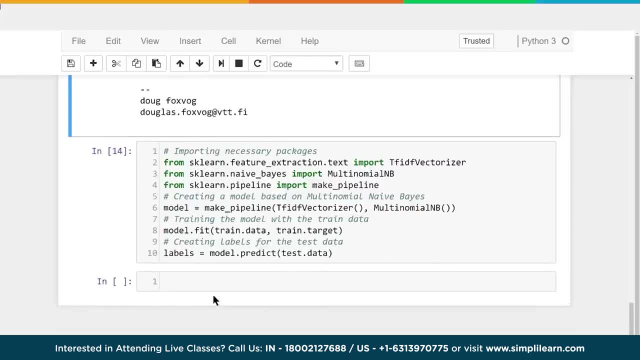 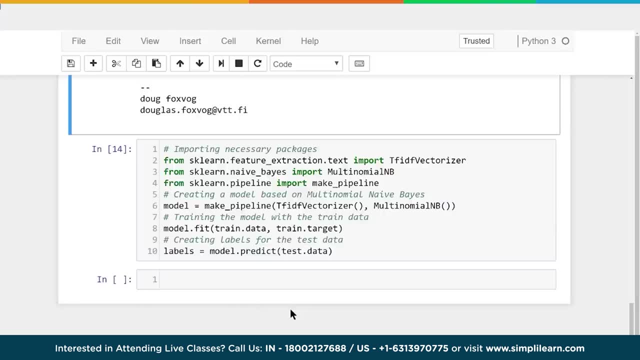 Now the train data. It has the different articles in it. You can see the one we were just looking at And the traintarget is what category they already categorized that particular article as, And what's happening here is the train data is going into the TF-ID vectorizer. 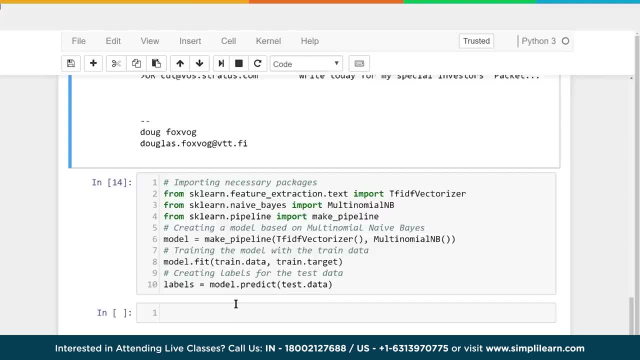 So when you have one of these articles that goes in there, it weights all the words in there. So there's thousands of words with different weights on them. I remember once running a model on this and I literally had 2.4 million tokens go into this. 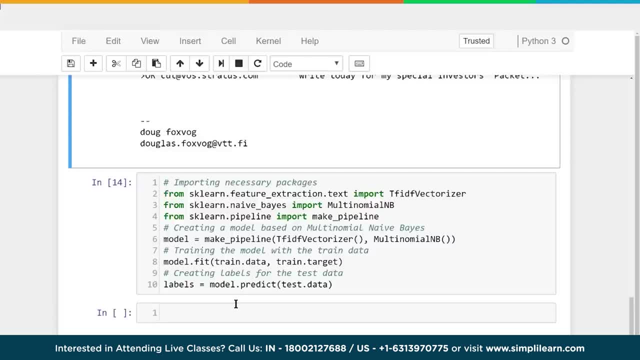 So when you're dealing Like large document bases, you can have a huge number of different words. It then takes those words, gives them a weight And then, based on that weight, based on the words and the weights, it then puts that into the multinomial NB. 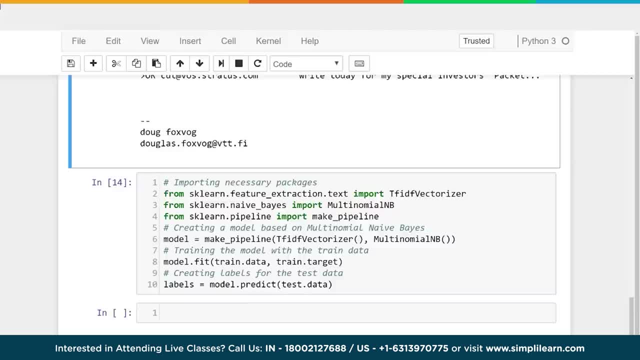 And once we go into our naive bays, we want to put the train target in there. So the train data that's been mapped to the TF-ID vectorizer is now going through the multinomial NB, And then we're telling it: well, these are the answers. 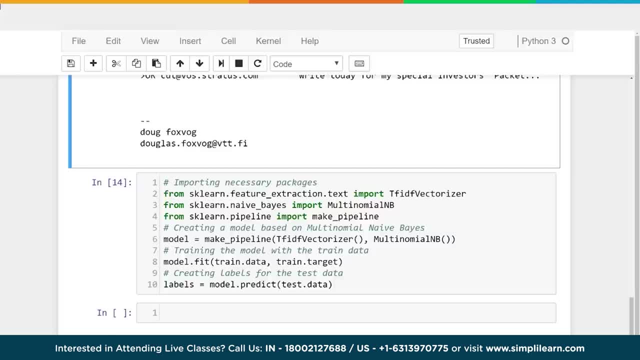 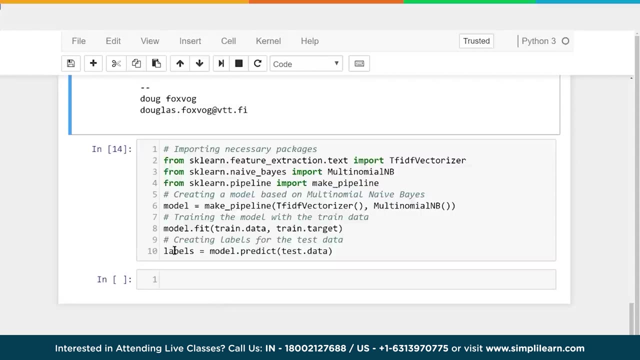 These are the answers to the different documents. So this document that has all these words, with these different weights from the first part is going to be, whatever category it comes out of- Maybe it's the talk show or the article on religion- miscellaneous. Once we fit that model, we can then take labels and we're going to set that equal to modelpredict. 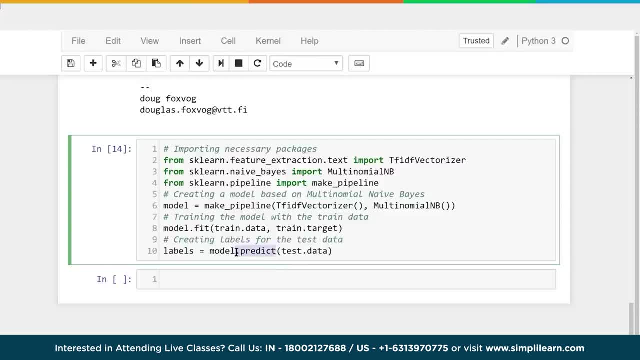 Most of the SKLearn use the term predict to let us know that we've now trained the model and now we want to get some answers And we're going to put our test data in there, because our test data Is the stuff we held off to the side. 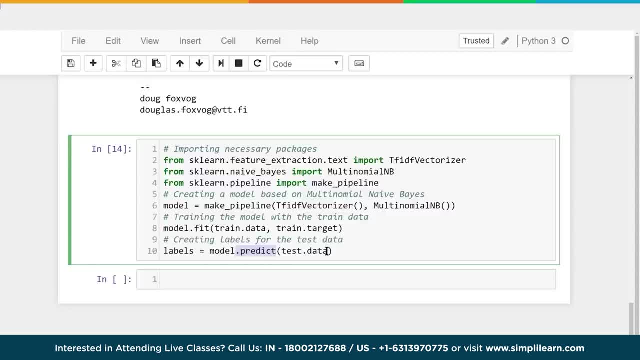 We didn't train it on there and we don't know what's going to come up out of it. And we just want to find out how good our labels are. Do they match what they should be? Now, I've already run this through. 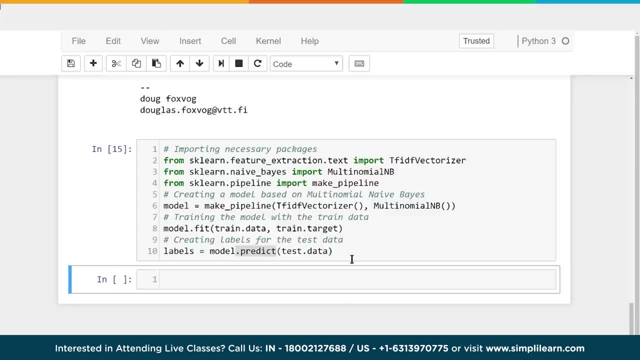 There's no actual output to it to show. This is just setting it all up. This is just training our model, creating the labels so we can see how good it is, And then we move on to the next step, to find out what happened. 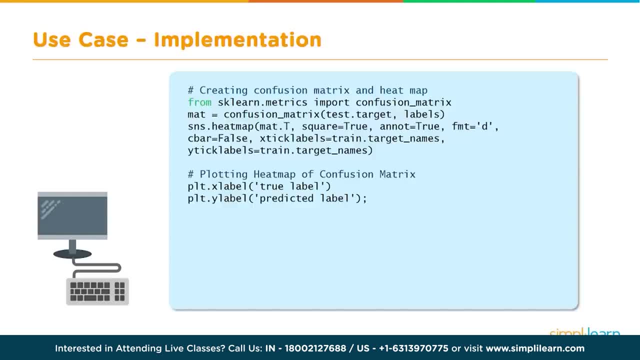 To do this, we're going to go ahead and create a confusion matrix and a heat map. So the confusion matrix, Which is confusing just by its very name, It's basically going to ask how confused is our answer? Did it get it correct or did it miss some things in there or have some missed labels? 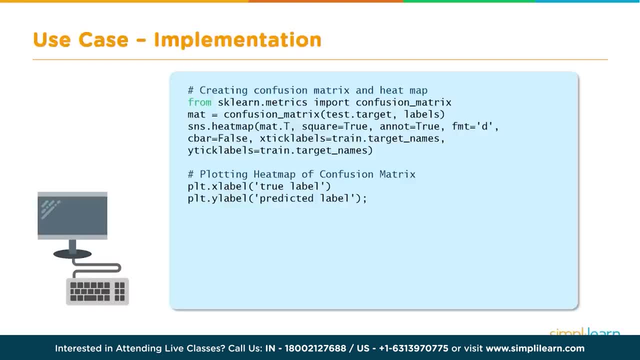 And then we're going to put that on a heat map, So we'll have some nice colors to look at to see how that plots out. Let's go ahead and take this code and see how that. take a walk through it and see what that looks like. 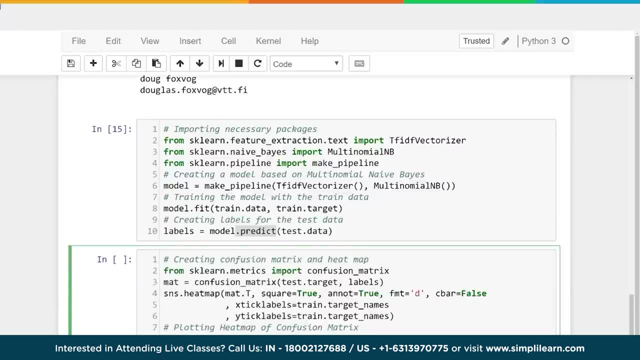 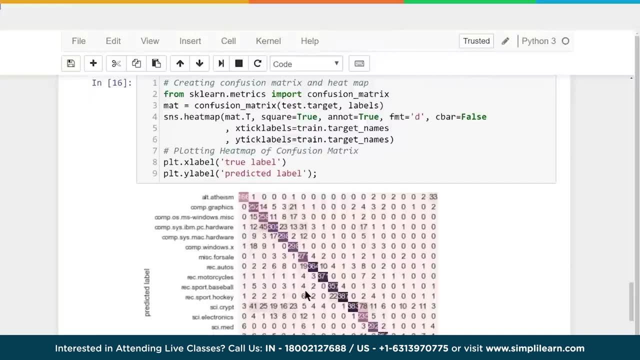 So back to our Jupyter notebook. I'm going to put the code in there and let's go ahead and run that code. Take it just a moment And remember we had the inline. That way my graph shows up on the inline here. 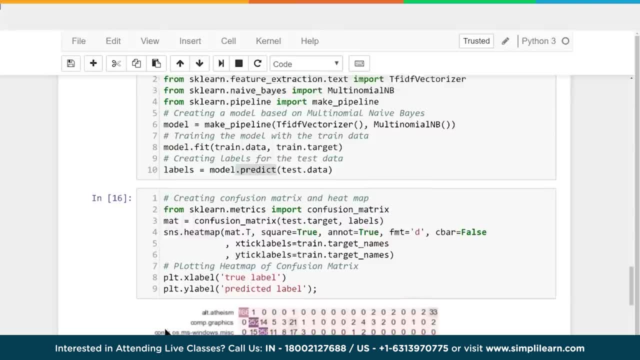 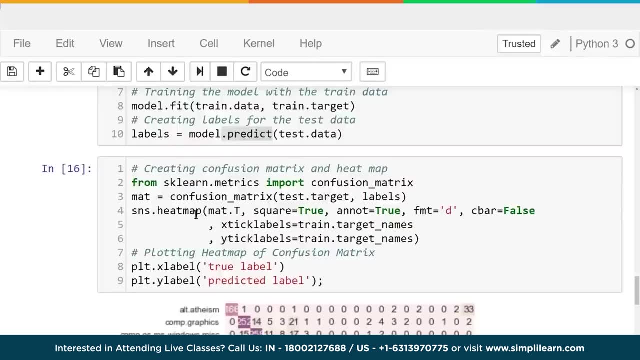 And let's walk through the code and then we'll look at this and see what that means. So let me get a little bit bigger. There we go, No reason not to use a whole screen Too big. So we have here from SKLearnMetrics import confusion matrix. 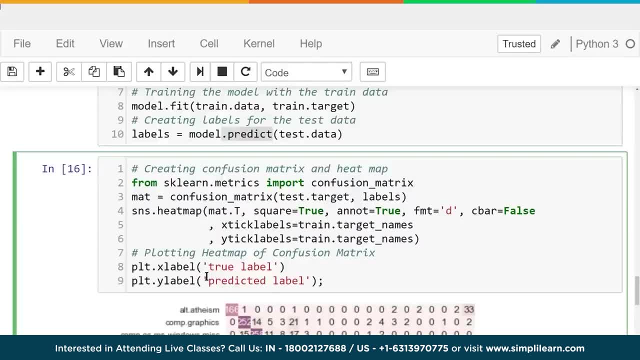 And that's just going to generate a set of data that says the prediction was such. the actual truth was either agreed with it or is something different, And it's going to add up those numbers so we can take a look and just see how well it works. 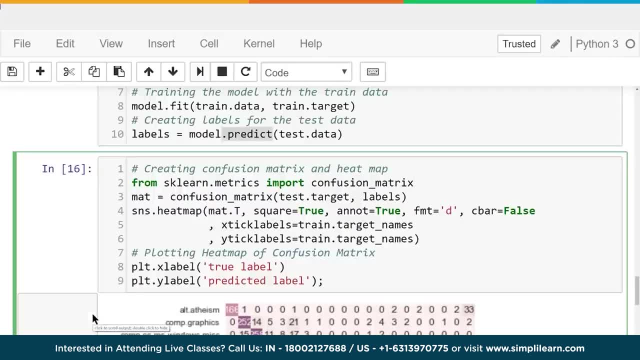 And we're going to set a variable mat equal to confusion matrix. We have our test target, our test data. that was not part of the training- Very important in data science. We always keep our test data separate, Otherwise it's not a valid model if we can't properly test it with new data. 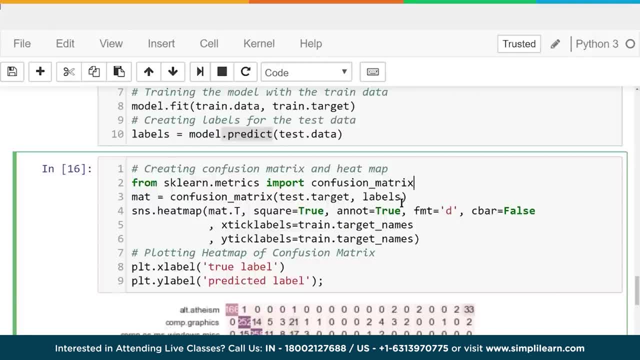 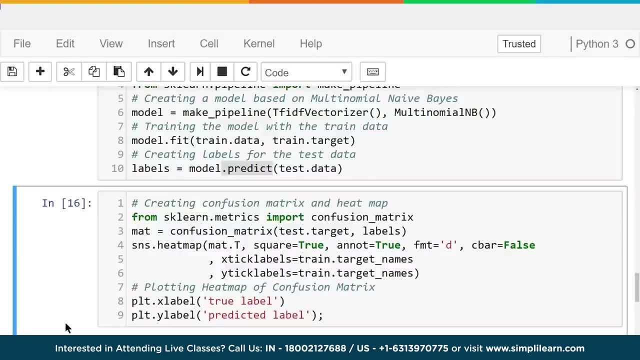 And this is the labels we created from that test data. These are the ones that we predict it's going to be. So we go in and we create our SN heat map. The SNS is our seaborne, which sits on top of the pi plot. 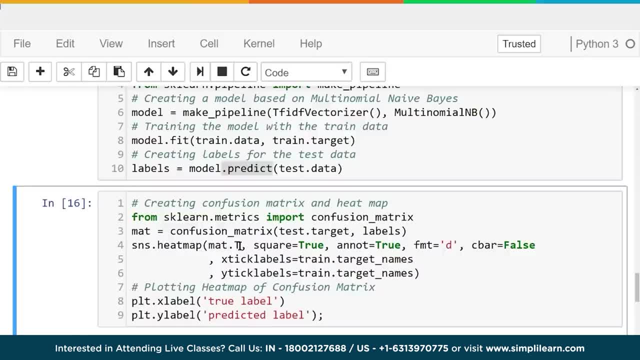 So when we create a SNSheatmap we take our confusion matrix and it's going to be matt, And then we have other variables that go into the SNSheatmap. We're not going to go into detail what all the variables mean. 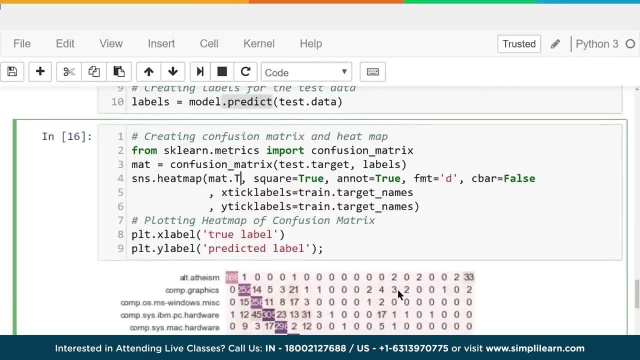 The annotation equals true. That's what tells it to put the numbers here. So you have the 166, the 1, the 0001.. Format D and C bar equals false. have to do with the format. If you take those out, you'll see that some things disappear. 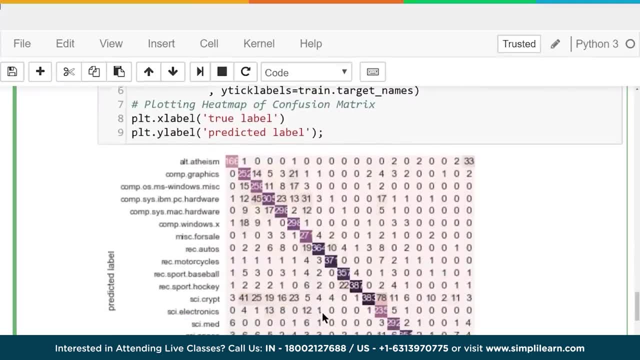 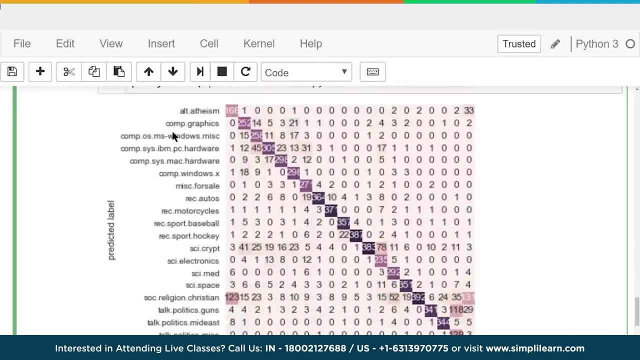 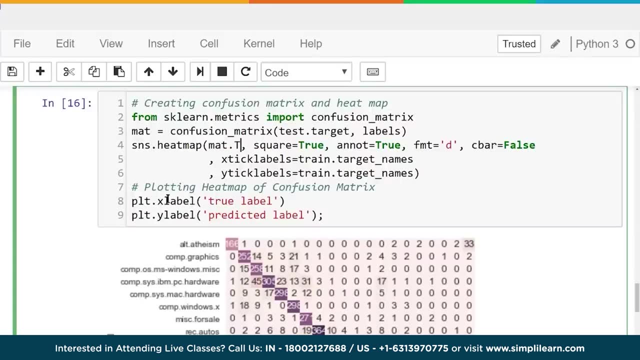 And you can see right here: that's the alt atheism, comp, graphics, comp, osms, windowsmiscellaneous. And then, finally, we have our pltxlabel. Remember the SNS or the seaborne sits on top of our matplot library. our plt. 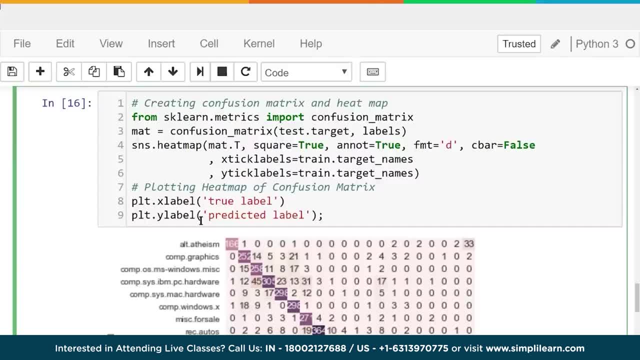 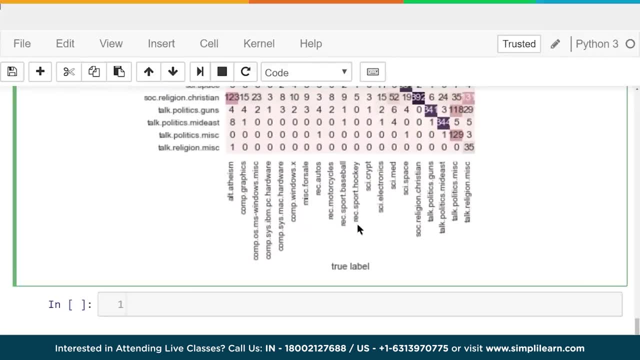 And so we want to just tell it: xlabel equals a true is true, The labels are true. And then the Y label is prediction label. So when we say a true, this is what it actually is And the prediction is what we predicted. 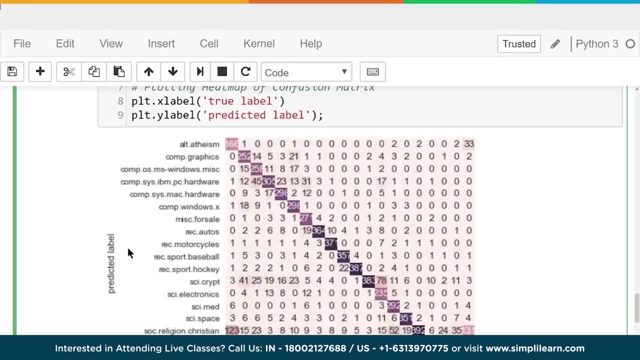 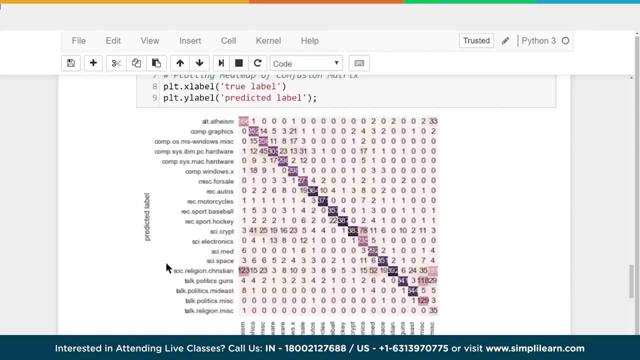 And let's look at this graph, because that's probably a little confusing the way we rattled through it, And what I'm going to do is I'm going to go ahead and flip back to the slides Because they have a black background they put in there. that helps it shine a little bit better. 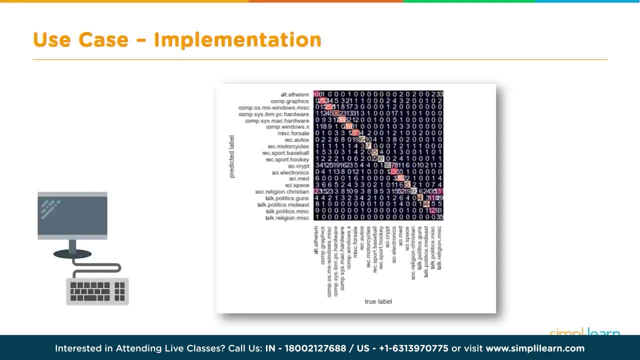 So you can see the graph a little bit easier. So in reading this graph, what we want to look at is how the color scheme has come out, And you'll see a line right down the middle diagonally from upper left to bottom right. 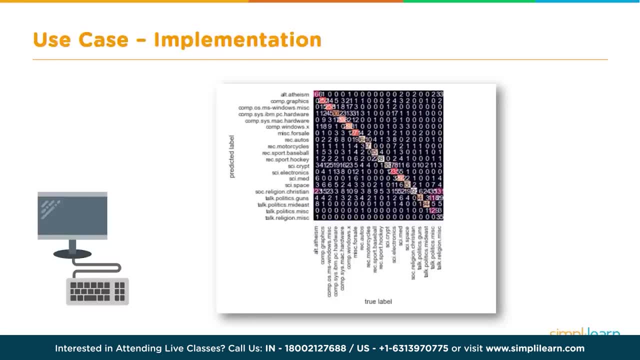 What that is is if you look at the labels, we have our prediction label, We have our predicted label on the left and our true label on the right. Those are the numbers where the prediction and the true come together, And this is what we want to see, is we want to see those lit up. 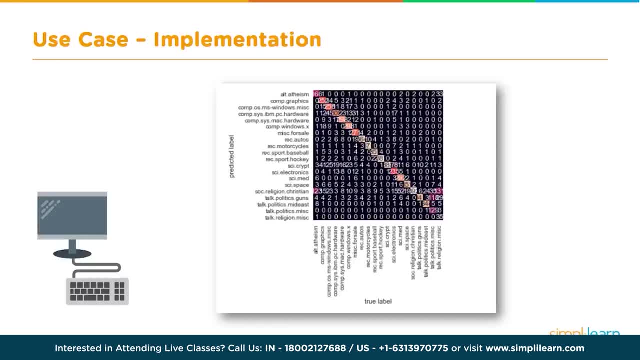 That's what that heat map does, As you can see that it did a good job of finding those data And you'll notice that there's a couple of red spots on there where it missed. You know it's a little confused when we talk about talk religion- miscellaneous- versus talk politics- miscellaneous. 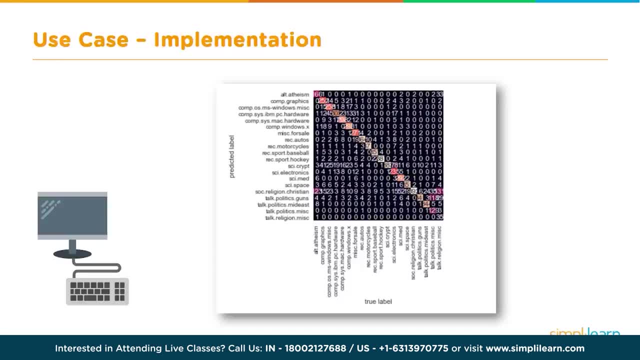 Social religion, Christian versus alt atheism. It mislabeled. It mislabeled some of those, And those are very similar topics, so you could understand why it might mislabel them, But overall it did a pretty good job. If we're going to create these models, we want to go ahead and be able to use them. 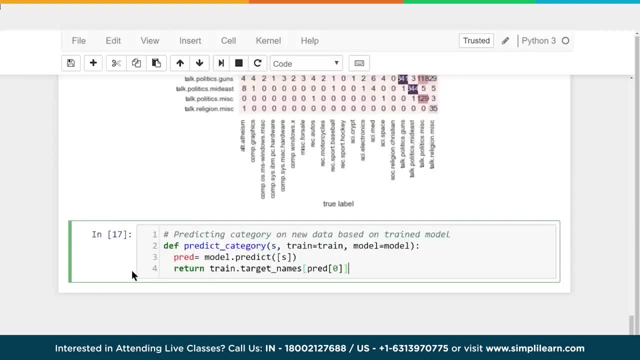 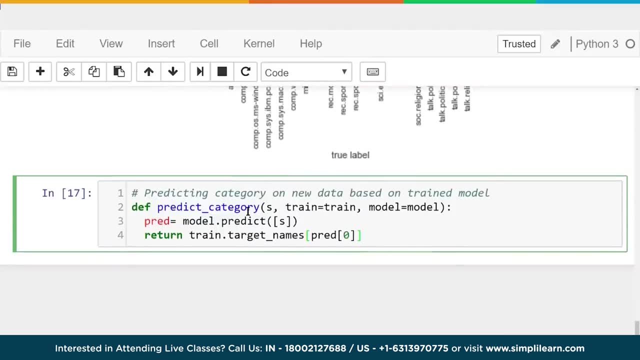 So let's see what that looks like. To do this, let's go ahead and create a definition, a function to run, And we're going to call this function. Let me just expand that just a notch here. There we go. I like mine in big letters. 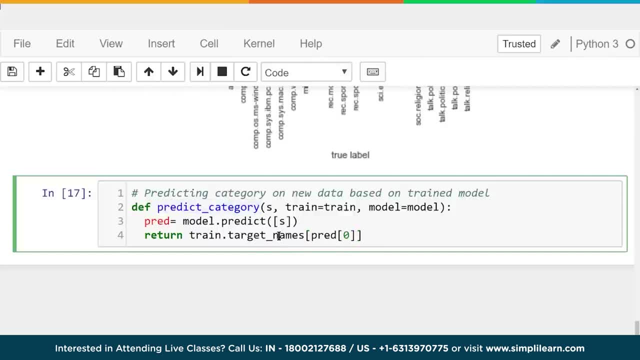 Predict categories. We want to predict the category. We're going to send it S a string. We're sending it train equals train. We have our training model And then we had our pipeline model equals model. This way, we don't have to resend these variables each time. 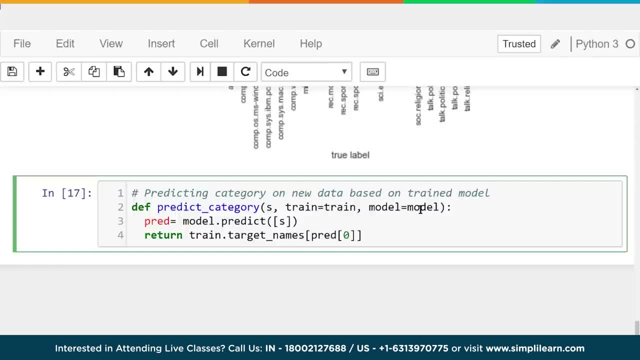 The definition knows that, because I said train equals train and I put the equal for model And then we're going to set the prediction equal to the model dot predict S. So it's going to send whatever string we send to it. It's going to push that string through the pipeline, the model pipeline. 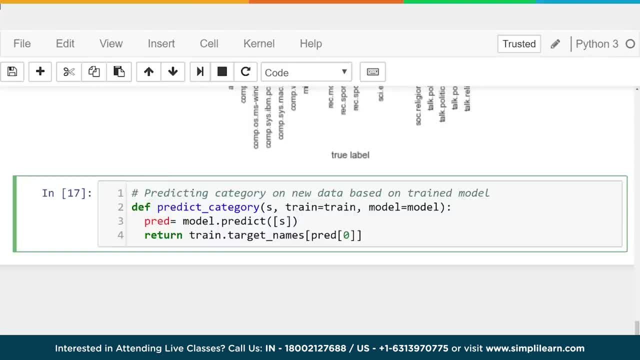 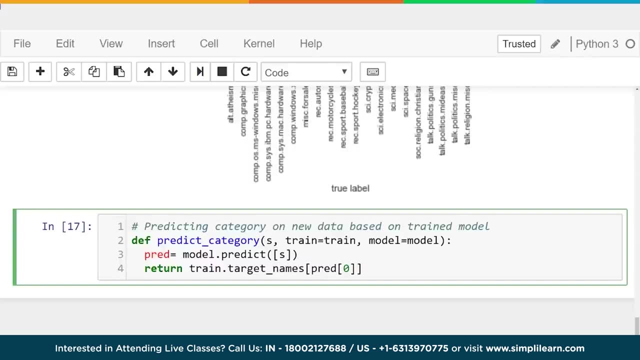 It's going to go through and tokenize it and put it through the TF, IDF, Convert that into numbers and weights for all the different documents and words, And then it'll put that through our naive bays And from it we'll go ahead and get our prediction. 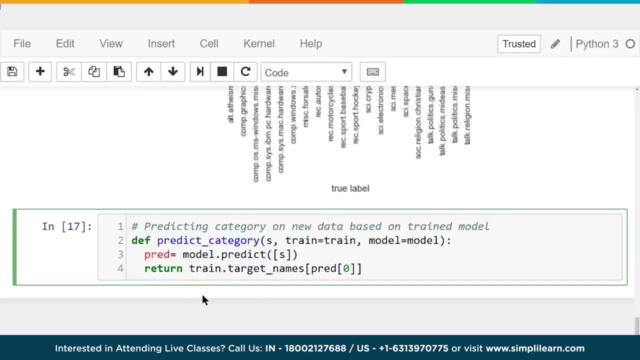 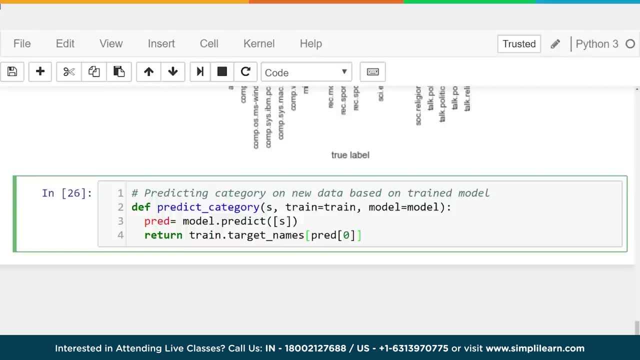 We're going to predict what value it is And so we're going to return train dot target names- predict of zero. And remember that the train dot target names, that's just categories. I could have just as easily put categories in there. dot: predict of zero. 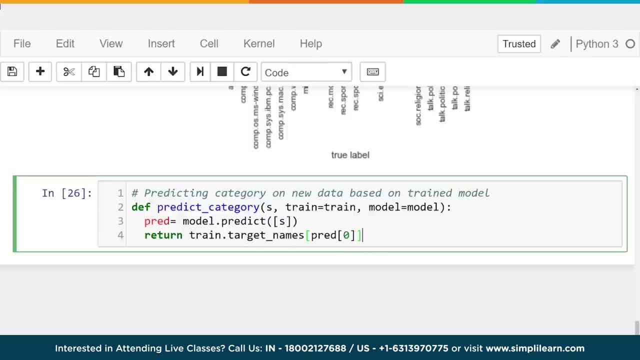 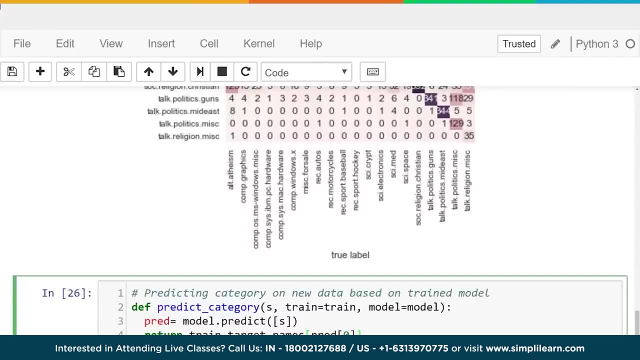 So we're taking the prediction, which is a number, and we're converting it to an actual category. We're converting it from. I don't know what the actual numbers are, but let's say, zero equals alt atheism. So we're going to convert that zero to the word. 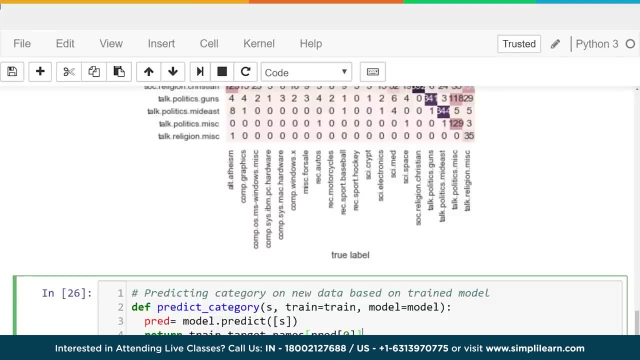 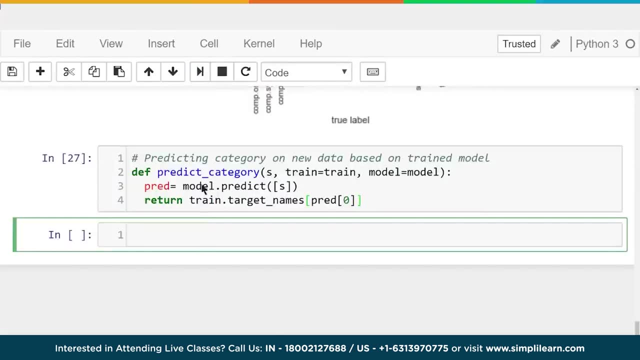 Or one. maybe it equals comp graphics. So we're going to convert number one into comp graphics, That's all that is. And then we need to go ahead and run this. So I load that up And then, once I run that, we can start doing some predictions. 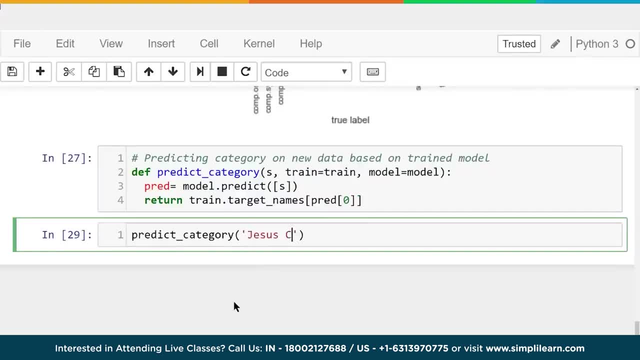 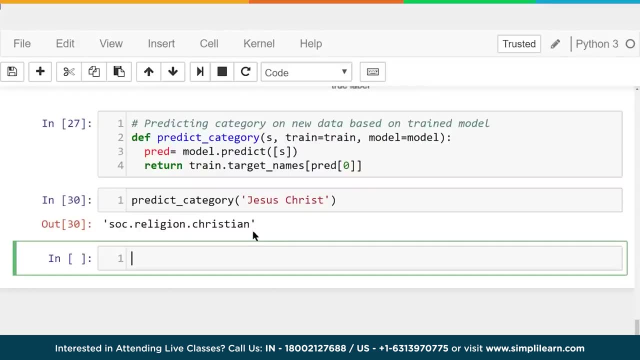 I'm going to go ahead and type in predict category And let's just do predict category Jesus Christ And it comes back and says it's social religion Christian. That's pretty good. Now note I didn't put print on this, One of the nice things about the Jupyter notebook editor and a lot of inline editors. 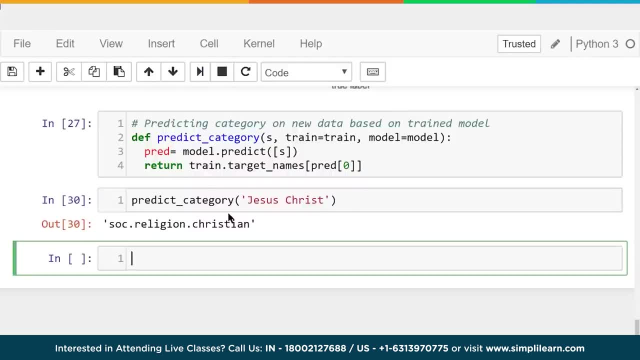 is if you just put the name of the variable out, it's returning the variable train dot target underscore names. it'll automatically print that for you In your own ID. you might have to put in print. Let's see where else we can take this. 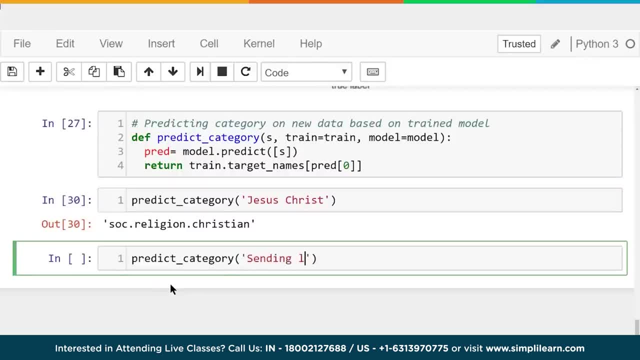 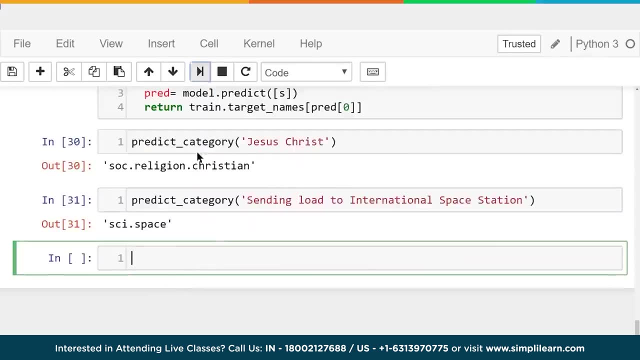 And maybe you're a space science buff, Sending load to international space station And if we run that, we get science space. Or maybe you're a automobile buff, And let's do. they were going to tell me Audi is better than BMW. 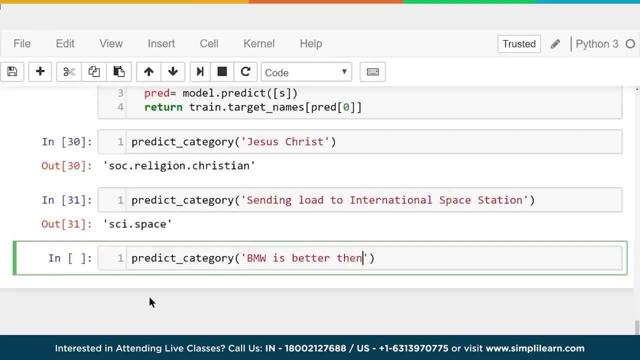 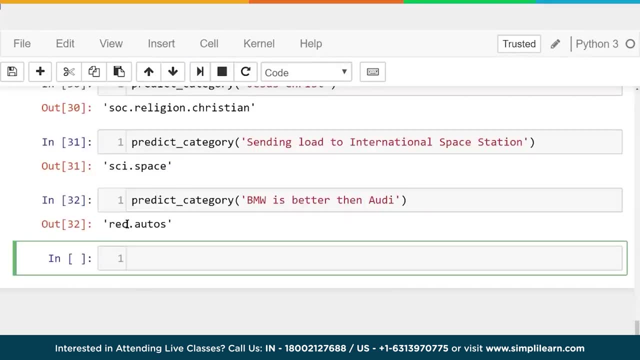 But I'm going to do. BMW is better than an Audi, So maybe you're a car buff And we run that And you'll see. it says recreational. I'm assuming that's what REC stands for. So I did a pretty good job labeling that one. 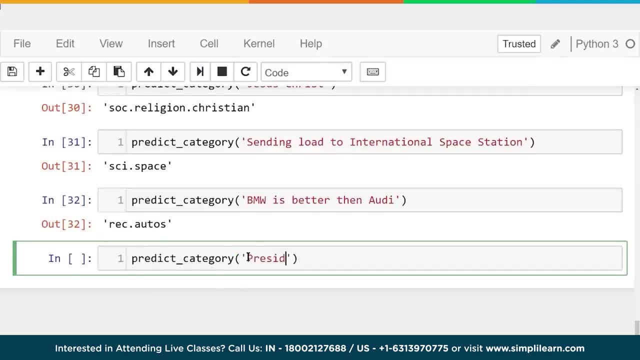 How about if we have something like a caption running through there, President of India, And if we run that it comes up and says: talk politics miscellaneous. So when we take our definition or our function and we run all these things through, kudos, we made it. 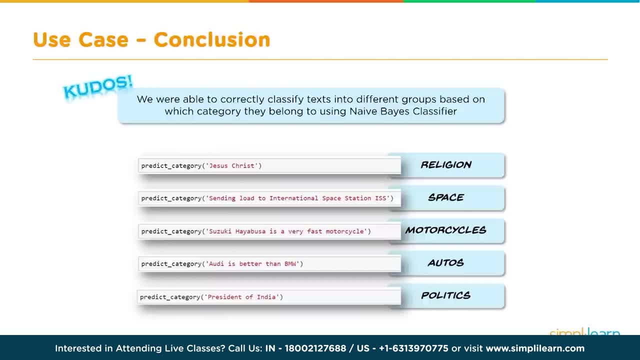 We were able to correctly classify texts into different groups, based on which category they belong to, using the Naive Bayes classifier. Now we did throw in the pipeline the TF-IDF vectorizer, We threw in the graphs. Those are all things that you don't necessarily have to know. 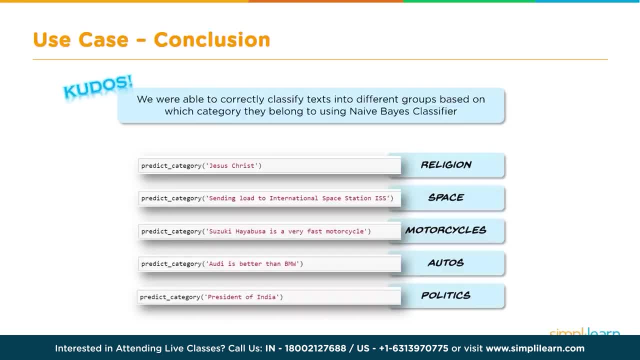 to understand the Naive Bayes setup or classifier, But they're important to know. One of the main uses for the Naive Bayes is with the TF-IDF tokenizer or vectorizer, where it tokenizes a word and has labels And we use the pipeline because you need to push all that data through. 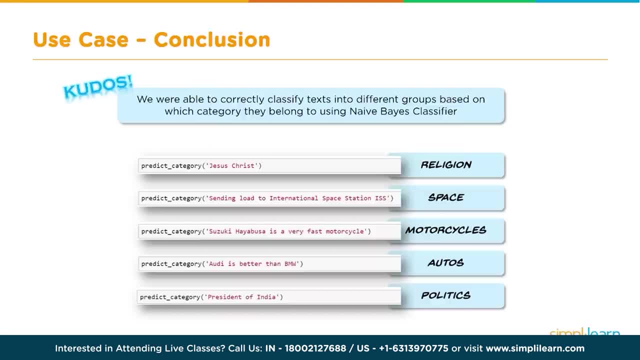 and it makes it really easy and fast. You don't have to know those to understand Naive Bayes, But they certainly help for understanding the industry and data science. And we can see our categorizer, our Naive Bayes classifier. We were able to predict the category: religion, space, motorcycles, autos, politics. 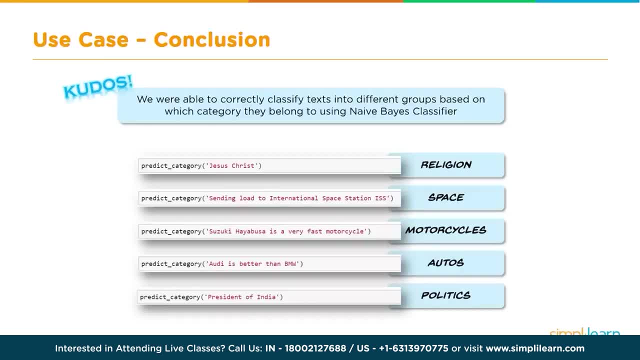 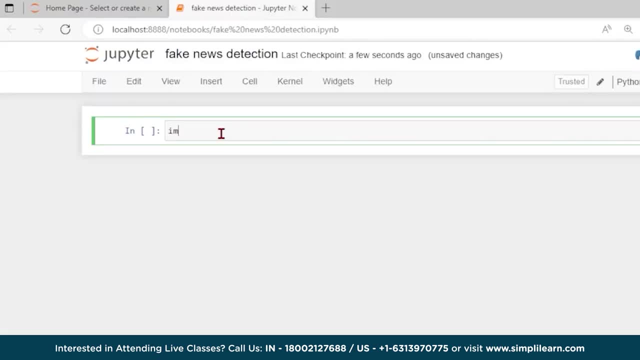 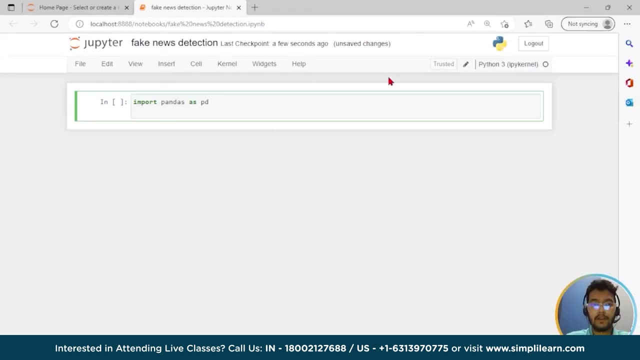 and properly classify all these different things we pushed into our prediction and our trained model. So first we will import some major libraries of Python. So here I will write: import pandas as pd, Then import numpy as np, Then import cborn as sns. 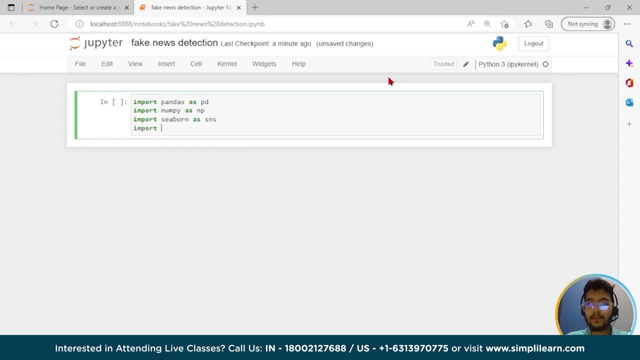 Then import sklearnmodelselection, Then import train test split. Next I will import matplotlib pyplot as plt. Okay, so now you already know what pplot is. Then I will write here from sklearnmetrics. import accuracy score, then from sklearnmetrics. 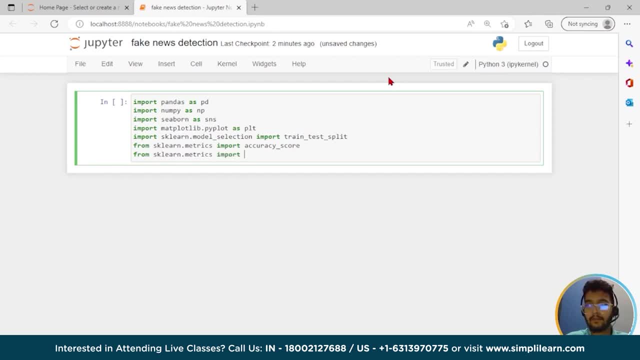 import classification to report, then import re, then import string. ok, then press enter. so it is saying: here I have to write from sklearnmetricsmetrics. everything seems good loading, let's see. ok, till then. numpy is a python library used for working with arrays. it also has function for working with domain of linear algebra and 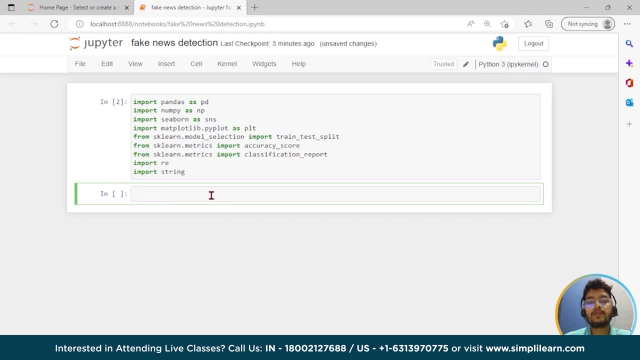 matrices. it is an open source project and you can use it freely. numpy stand for numerical python pandas, so panda is a software library written for python programming language for data manipulation and analysis. in particular, it offers data structure and operation for manipulating numerical tables and time series. then seaborn, an open source python library based on matplotlib. 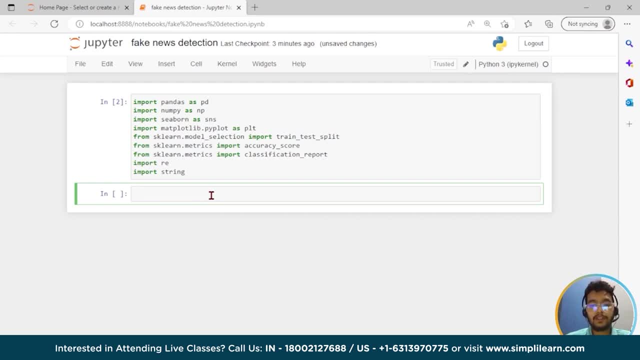 is called seaborn. it is utilized for data exploration and data visualization. with data frames and the pandas library, seaborn functions with ease. then matplotlib for python and its numerical extension numpy. matplotlib is a cross platform for the data visualization and graphical charting package. as a result, it presents a strong open. 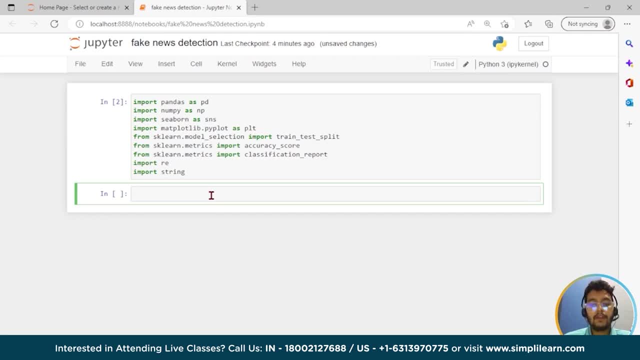 source suitable for matlab. the apis for matplotlib allow programmers to incorporate graphs into gi applications. then this train test split. we may build our training data and the test data with the aid of sklearn train test split function. This is so simple because the original dataset often serves as both the training data and the test data. 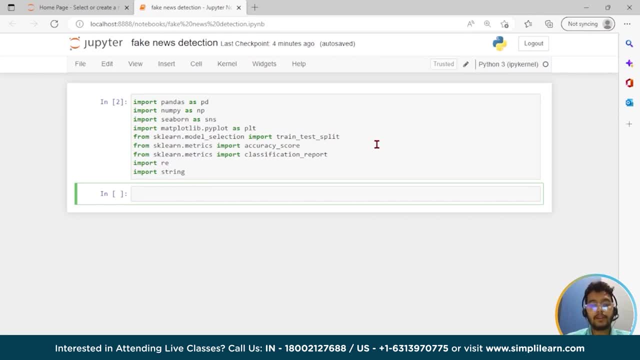 Starting with a single dataset, we divide it into two datasets to obtain the information needed to create a model like hone and test Accuracy Score. The accuracy score is used to gauge the model's effectiveness by calculating the ratio of total true positive to total true negative. 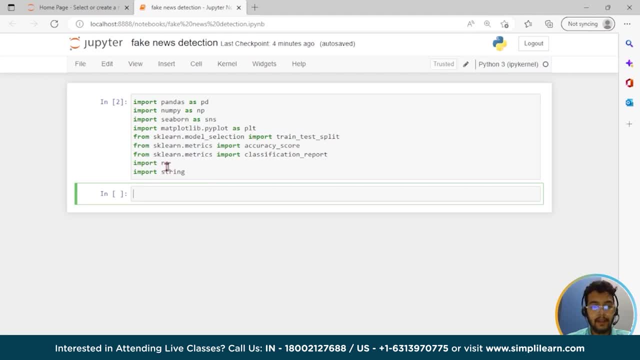 across all the model predictions, Use RE Regular Expression. The functions in the model allow you to determine whether a given text fits a given regular expression or not, which is known as RE String. A collection of letters, words or other characters is called a string. 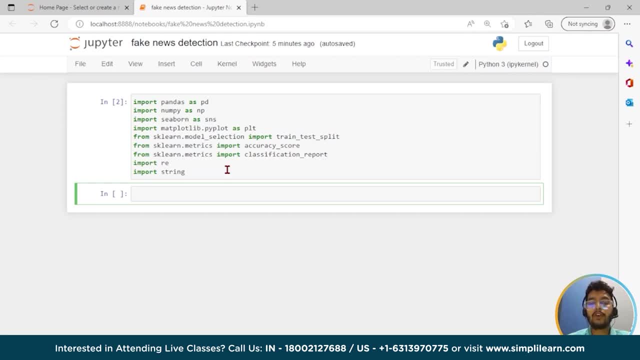 It is one of the basic data structures that serves as the foundation of manipulating data. The str class is a built-in string class in Python, because Python strings are immutable: They cannot be modified after they have been formed. So now let's import the dataset. we will be going to import two datasets, one for the. 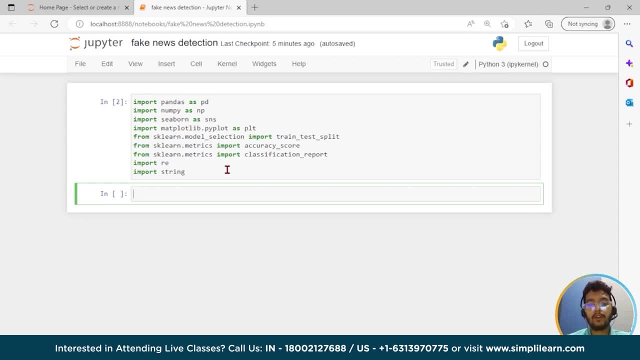 fake news and one for the true news. or you can say: not fake news. So I will write here: pf. underscore. fake equals to pd dot. read underscore csv. Then search the details: Detective information, Ordinary type. What I said, df. fake, Then fake csv. You can download this dataset from the description. 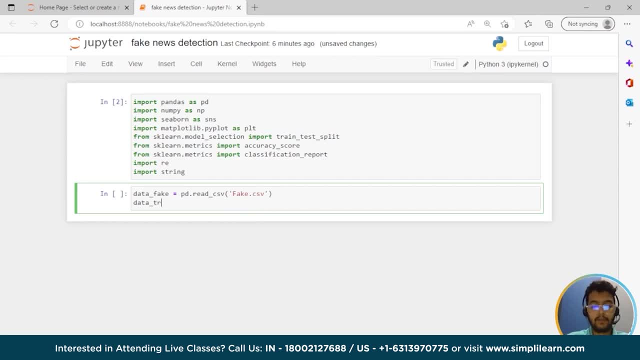 box below. Then data: wahoo, unicorn true 0.4, available user and return awesome を to readPHCage underscore: csv: sorry csv. and fake news: sorry, true, true dot csv. okay, then press enter. so these are the two data set. you can download these data set from the description box below. 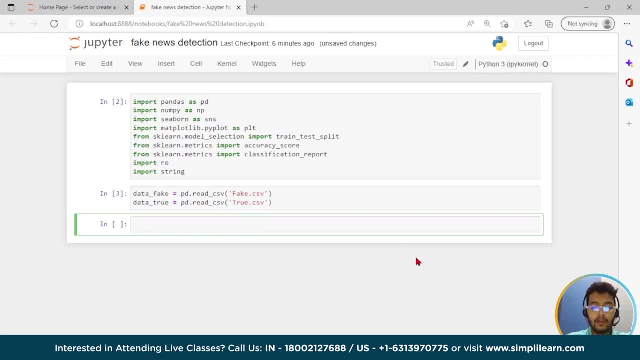 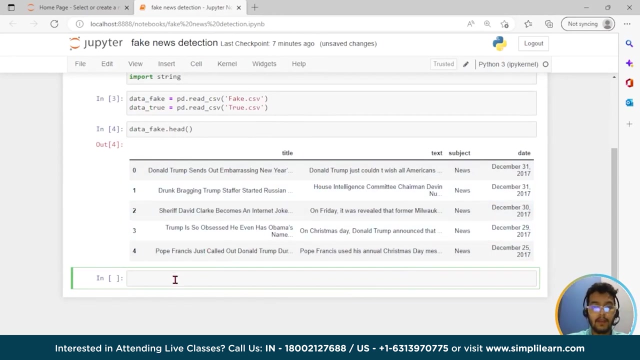 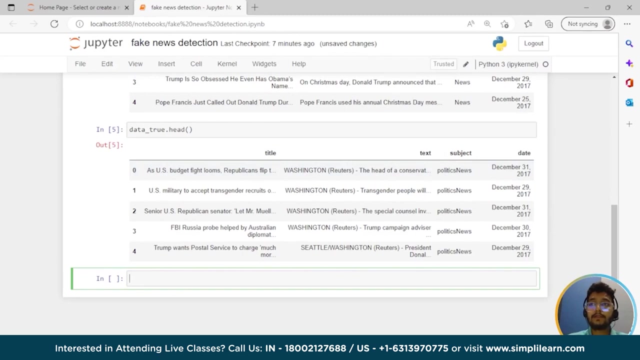 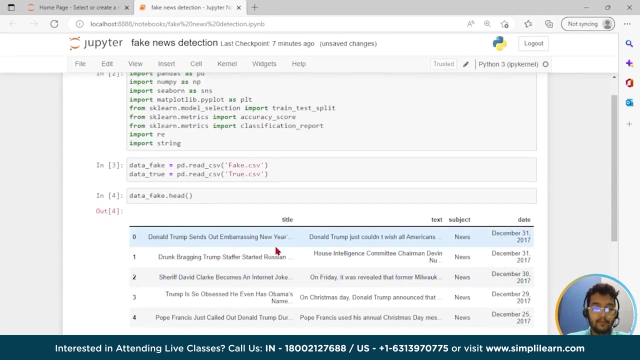 so let's see the board data set. okay, then i will write here: data underscore: fake dot head. so this is the fake data. okay, then data underscore: true dot. and this is the true data. okay, this is not fake. so if you want to see your top five rows, 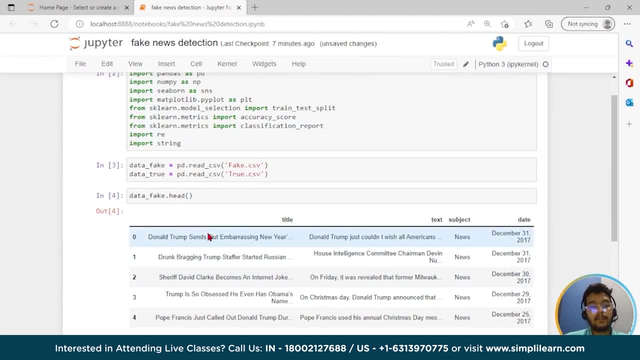 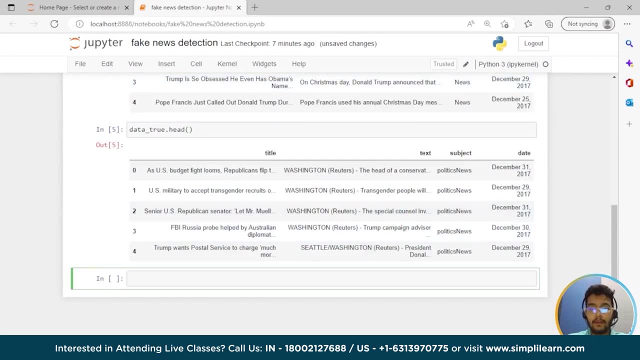 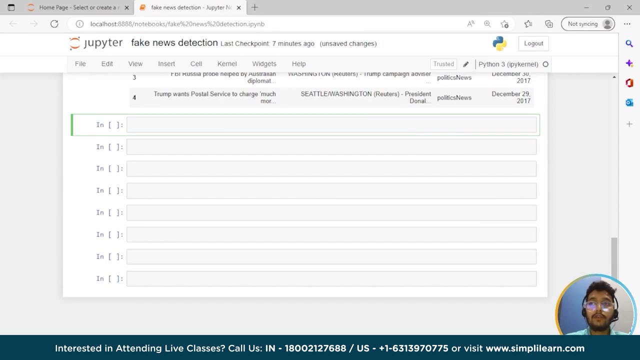 of the particular data set, you can use head, and if you want to see the last five rows of the data set, you can use tail instead of head. okay, so let me give some space for the better visual. so now we will insert column class as a target feature. 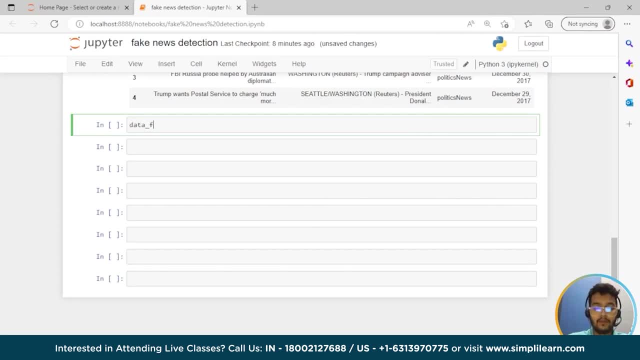 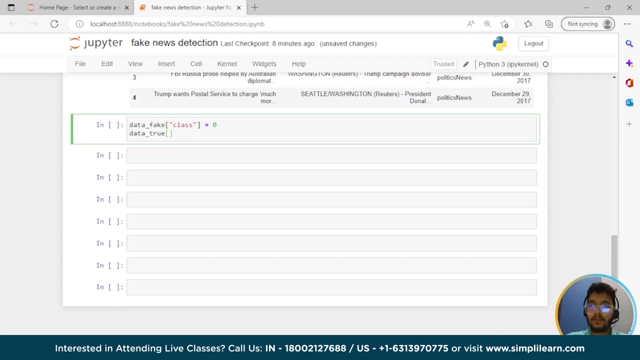 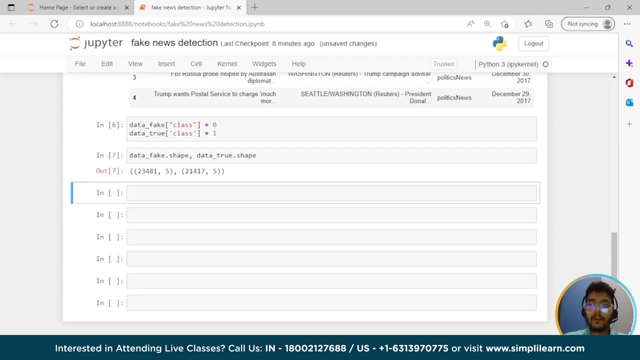 okay, then i will write here: data underscore fake: plus equals to zero, then data underscore true and plus equals to one. okay, then i will write here: data underscore fake dot shape and data underscore true dot shape. okay, then press enter so the shape method return the shape of an array. 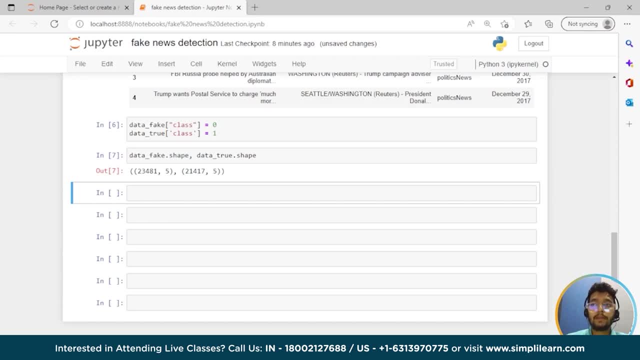 the shape is a tuple of integers. these number represent the length of the corresponding array dimension. in other words, a tuple containing the quantities of entries on each axis is a array shape dimension and it shouldn't be dropped으로 array shape dimension. so what's the meaning of shape in the fake world? in this data set we have? 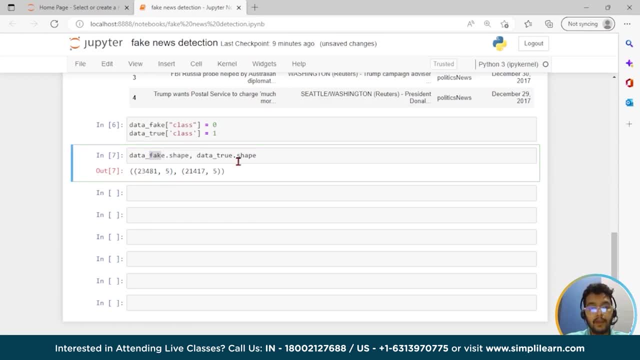 two, three, four, eight, one rows and five columns. and in this data set, true, we have two, one, four, one, seven rows and five column. okay, so these are the rows, column, rows, column for the particular data set. so now let's move and let's remove the last 10 rows for the manual testing. okay. 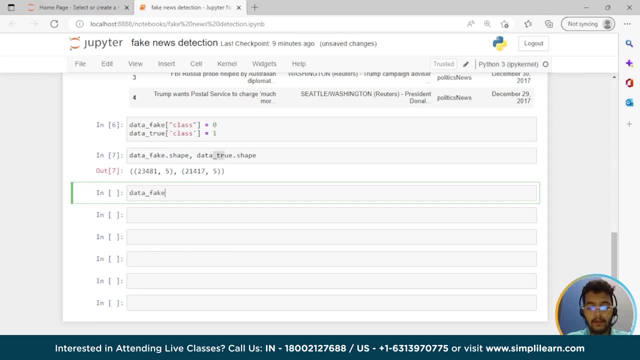 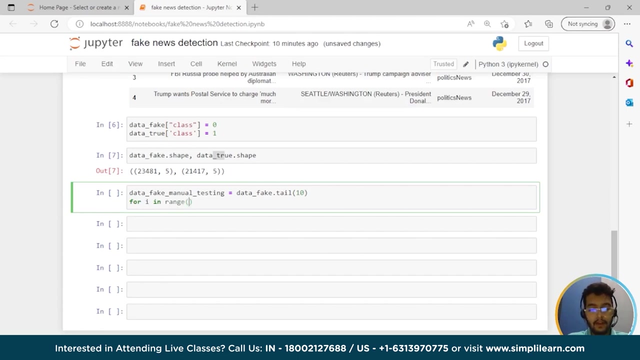 then I will write here data and let's go fake, let's go manual testing was to data and let's go fake. dot tail, or the last 10 rows, I have to write here 10. okay, so for I, in range of two, three, four, eight, one, seven, zero comma. two, three, four, seven, zero comma minus one. 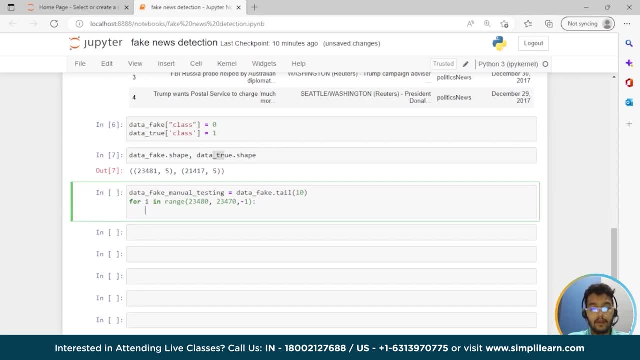 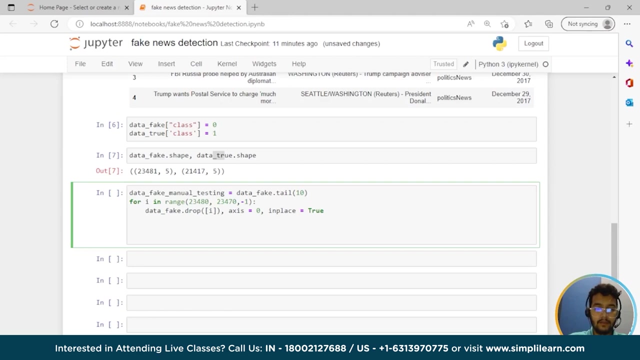 and df underscore, not df data underscore, fake dot. drop one instead of one. I can write here: I comma. this equals to zero place. oh, we were then data right it it underscore. I will copy from here and I will make any particular changes. so here I can write: true dosing 아드. 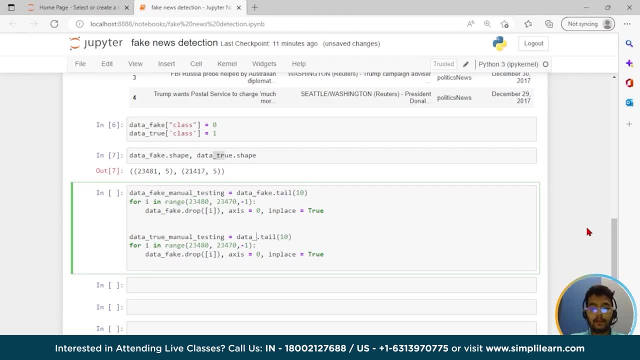 and I will copy it from here and I will paste it here and I will make a particular changes here. so here I can write true, and then I can write true. then I have to change the number 21416, 21406 minus 1, same. so press enter. 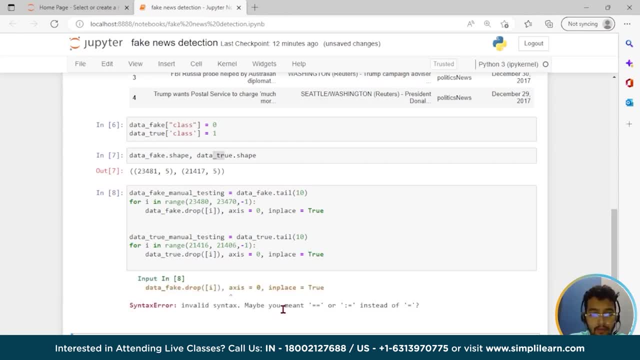 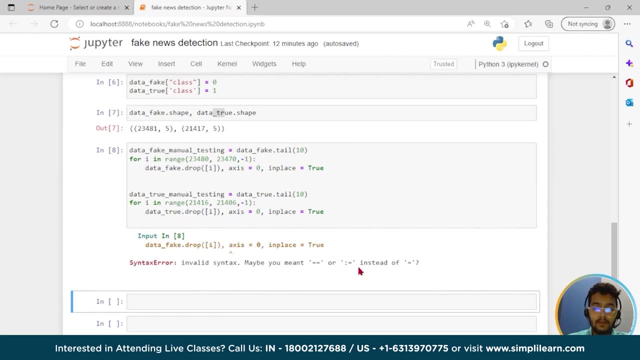 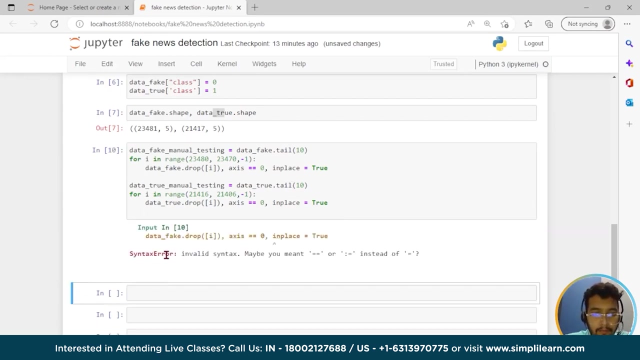 x is equal to 0, x is equal to 0. let's change x. maybe you need double 0 or we will put here double and I am putting this takedrop: x is equal to 0 in place. ok, let's write yeah, so axis is not defined. 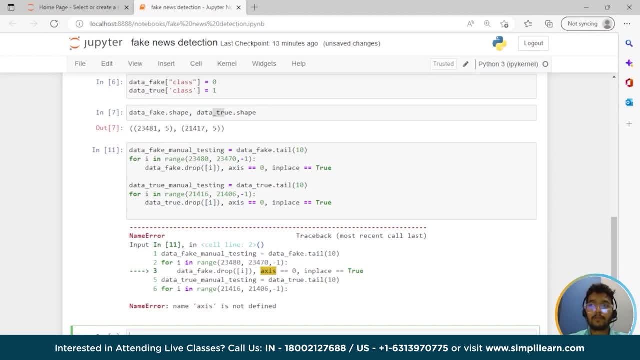 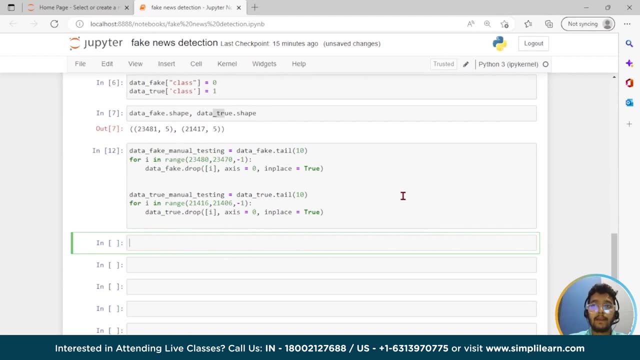 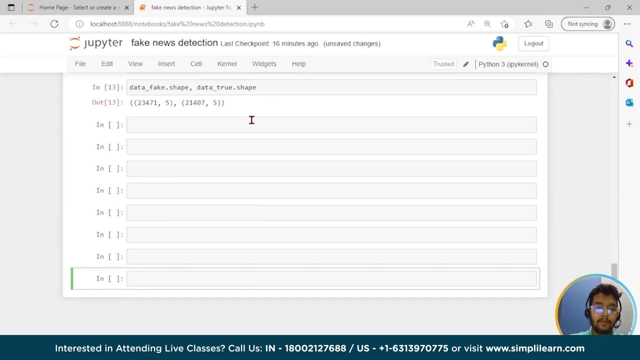 now it's working, so ok. so ok, ok, ok, ok, ok. let me see now data underscore: fake dot shape: ok, and data dot: true. data underscore: true dot shape. as you can see, 10 rows are deleted from each data set, so I will write here: data underscore. 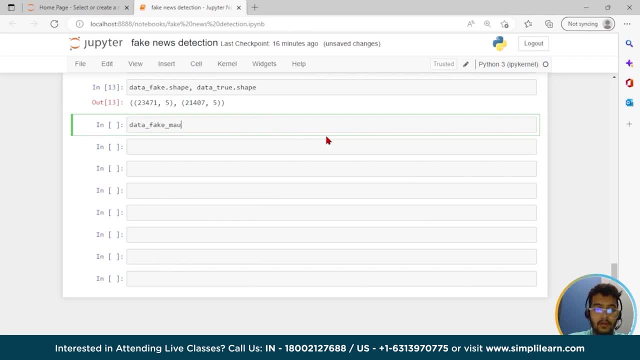 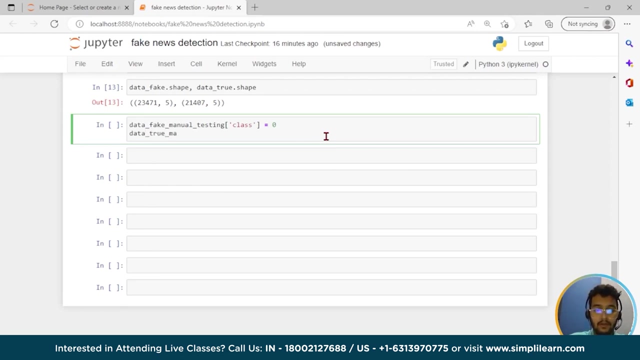 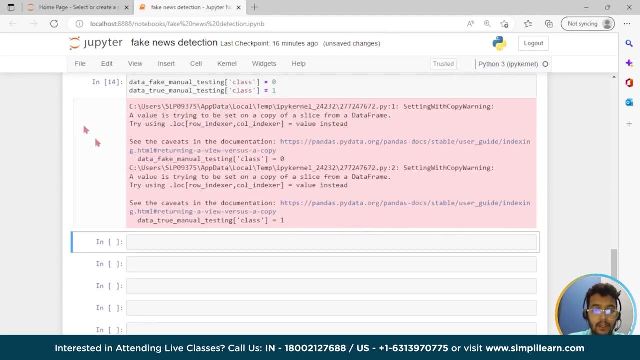 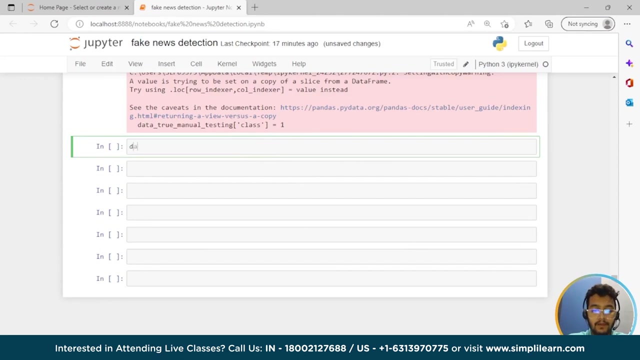 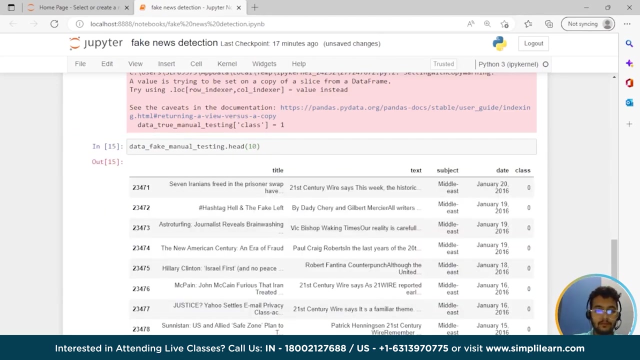 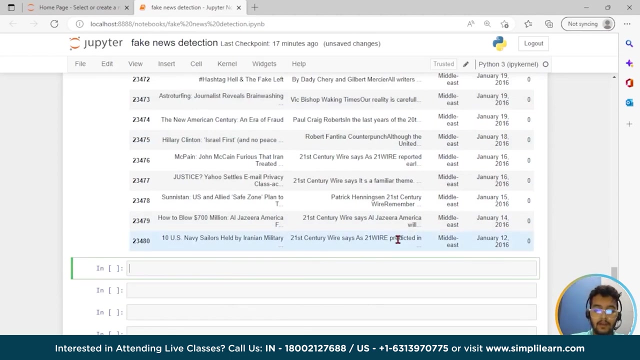 fake underscore manual testing class equals to 0 and data under school through underscore manual underscore testing x equals to 1. ok, just ignore this warning and let's see data underscore: fake data. as you can see, we have this and then data dot. sorry underscore, true underscore. 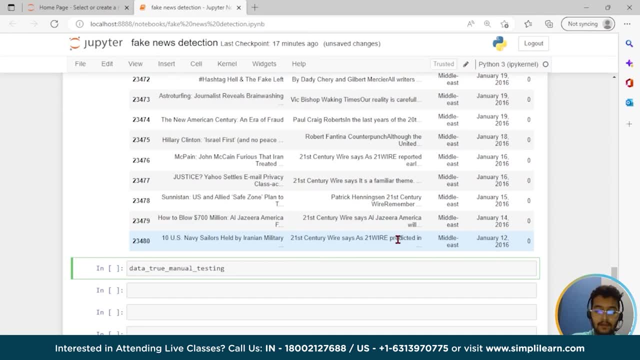 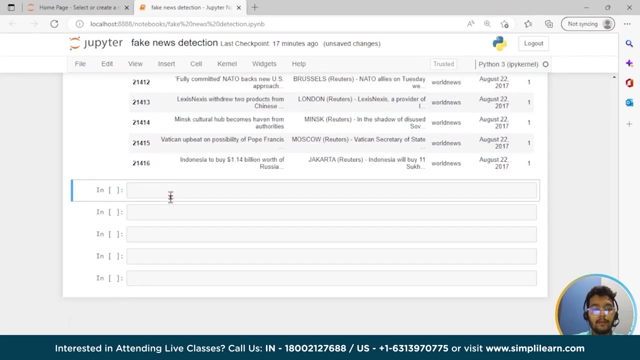 manual testing dot. ok. ok, so this is the true data set, so here I will merge data underscore: merge goes to pd dot- concat. concat is used for the concatenation, so we will use this for the concatenation here. data underscore- fake data underscore- proof comma. 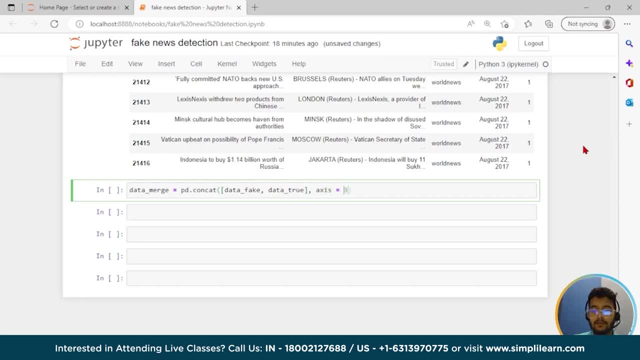 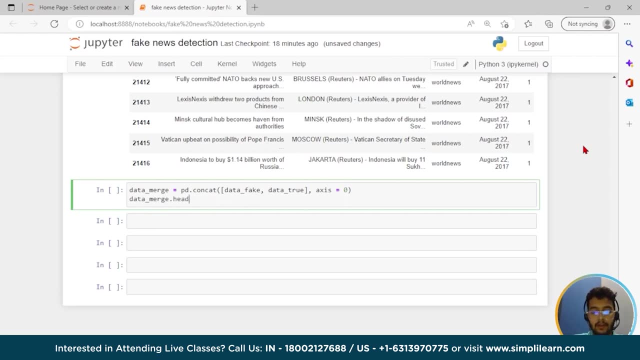 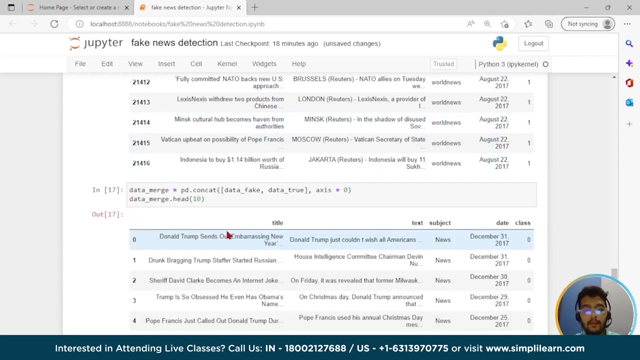 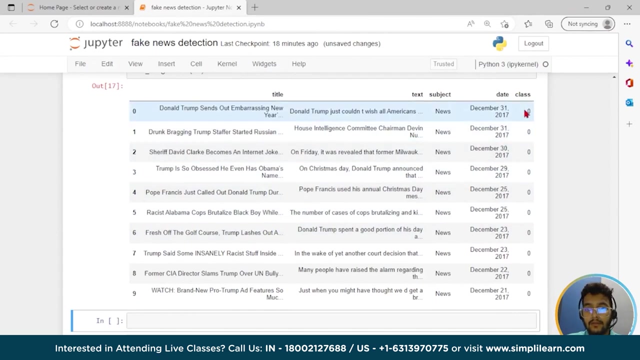 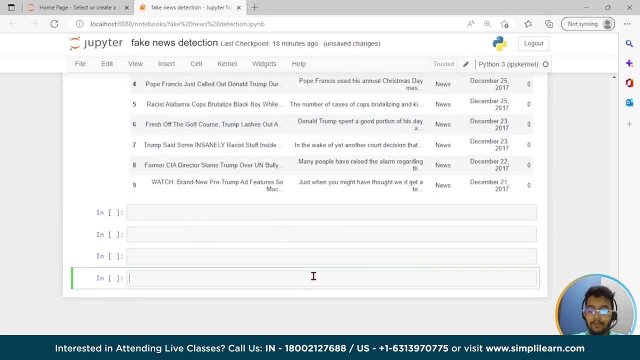 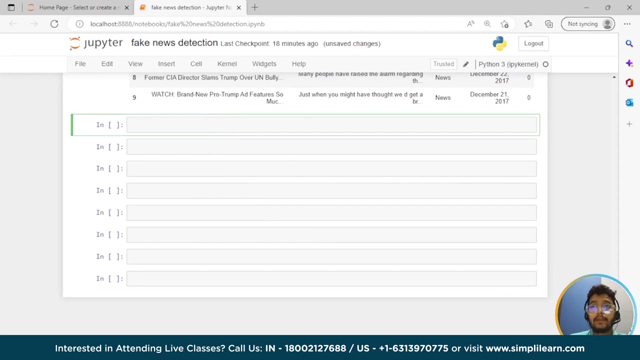 axis equals to 0, then data underscore: merge dot head the top 10 rows. yeah, right, As you can see, the data is merged here. First it will come for the fake news and then, with that, for the true news, And let's merge true and fake data frames. 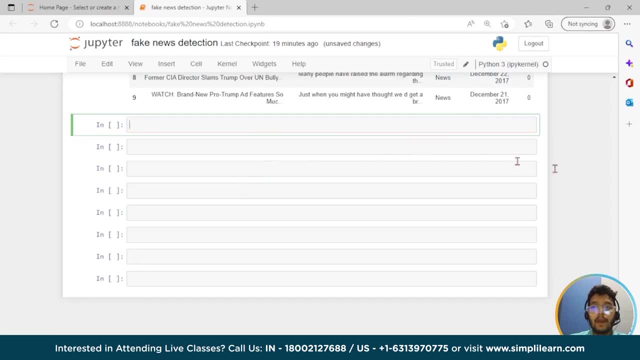 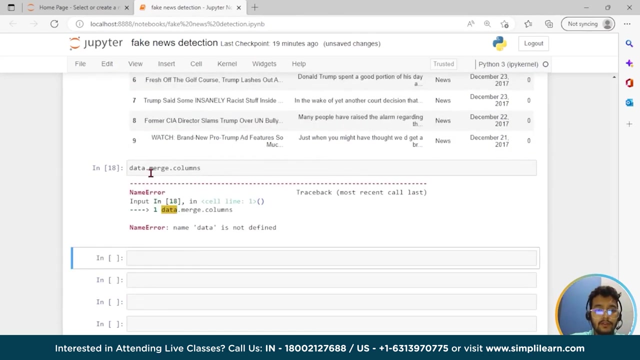 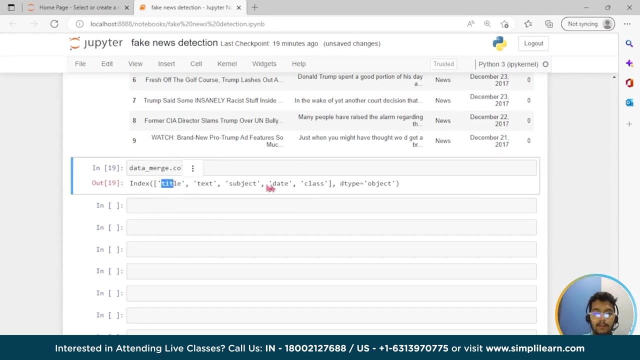 Okay, We did this and let's merge the column, then datamergecolumns, or let's see the columns. It is not defined, but I wrote data underscore merge. These are the columns. Same type of columns: Title, text, subject, date, class. 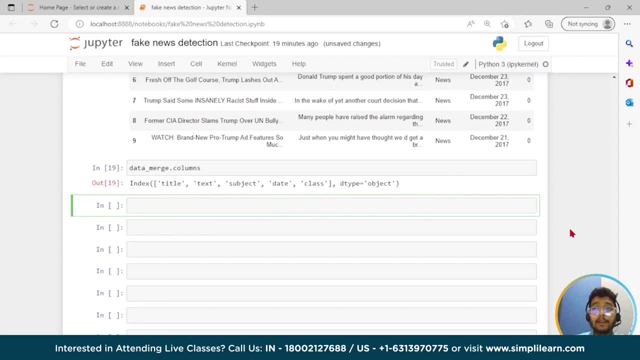 Okay, Now let's remove those columns which are not required for the further process. So here I will write: data underscore, all equals to data underscore. merge Prop Title: I don't need Then. Subject: We don't need Then. 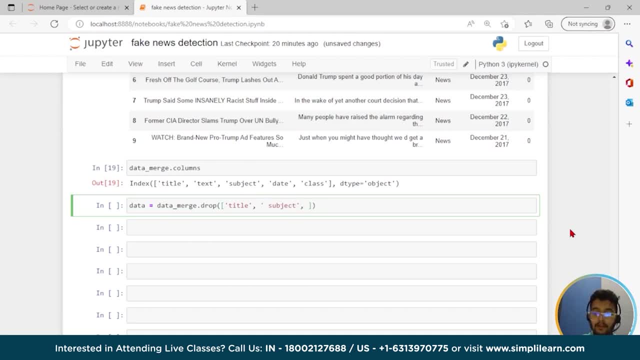 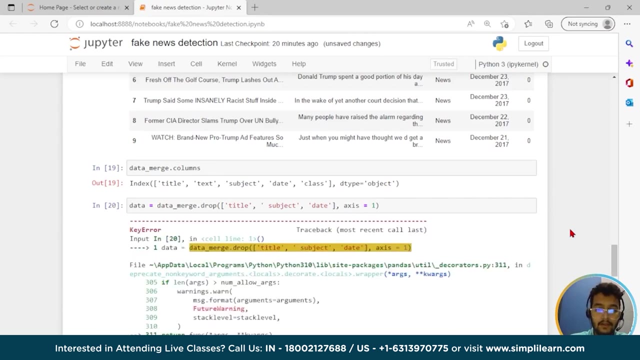 So 1.. So let's check some null values. It is giving error, Yeah, One of this, One of this. So let's check some null values. It is giving error. One of this, And then it will give error. 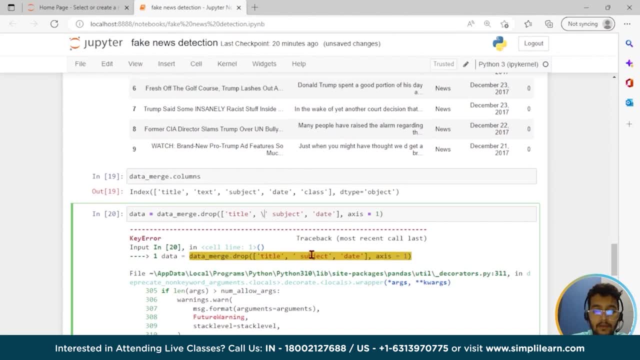 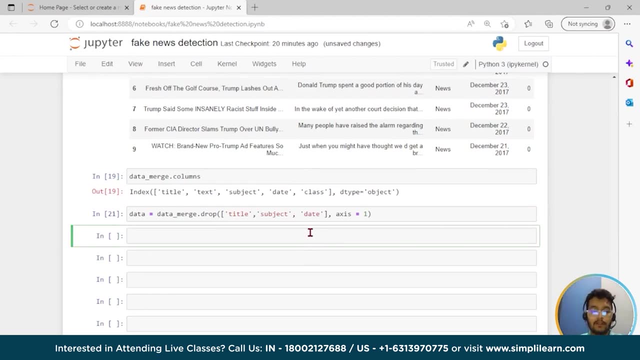 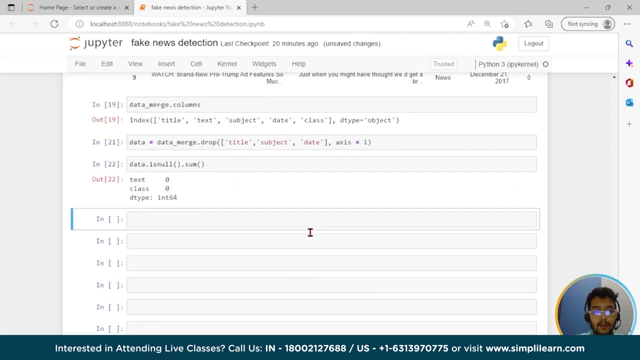 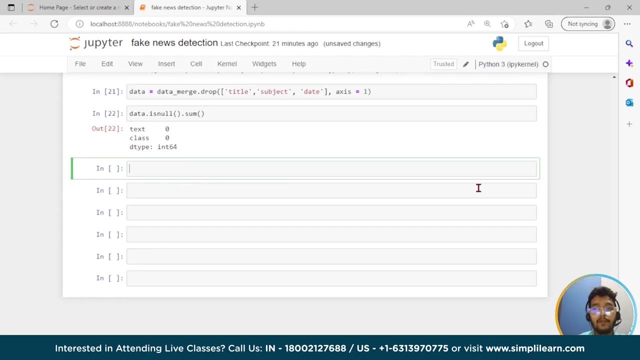 So let's check some null values. And then it is giving error. So let's check some null values, that's good. then data dot is null dot sum center, so no null values. okay, then let's do the random shuffling of the data frames. 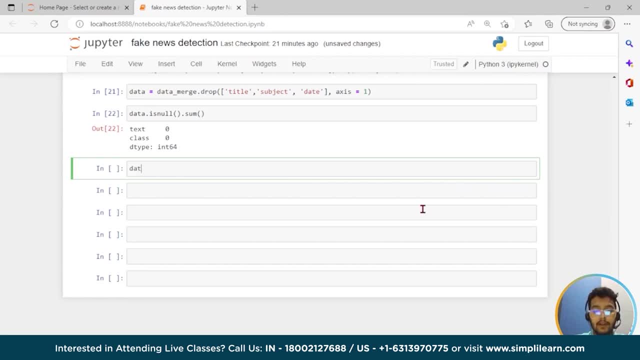 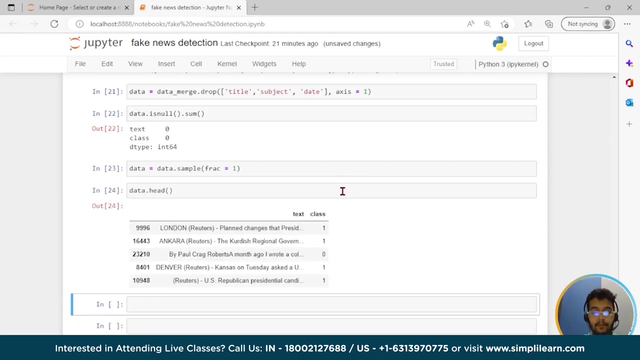 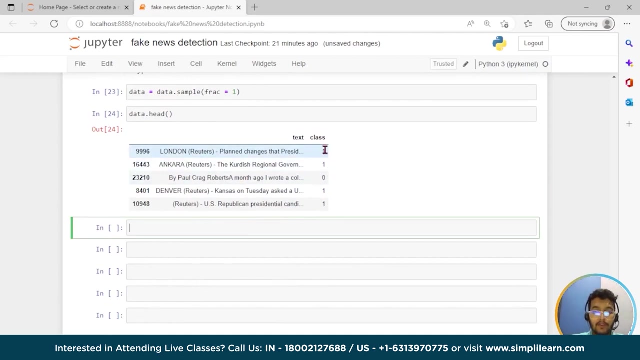 okay, for that we have to write here: data question: data dot. sample one and data data dot. now you can see here the random shuffling is done, and one for the true data reset and zero for the fake news one. okay, then let me write here data dot. 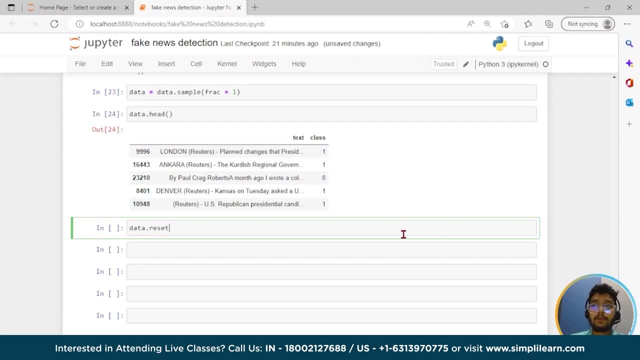 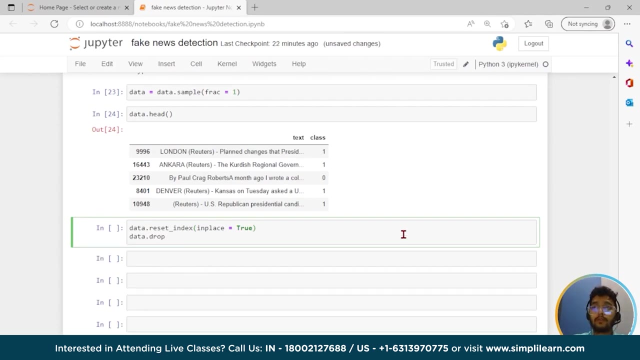 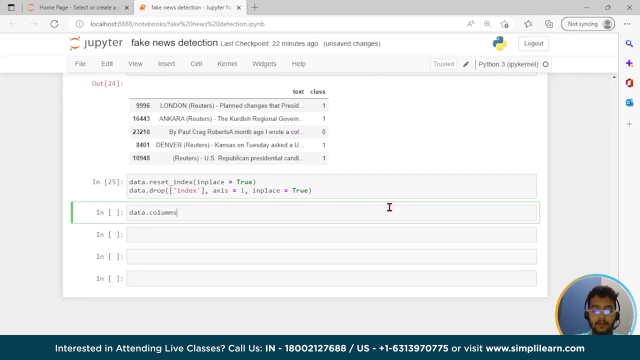 reset underscore index. this because you through data dot drop comma axis was to one comma in place. equation true. ok, then let me see columns now, yeter dot columns. so here we have two columns now and then we can write a column, because the data is even side and that educator is only one line. 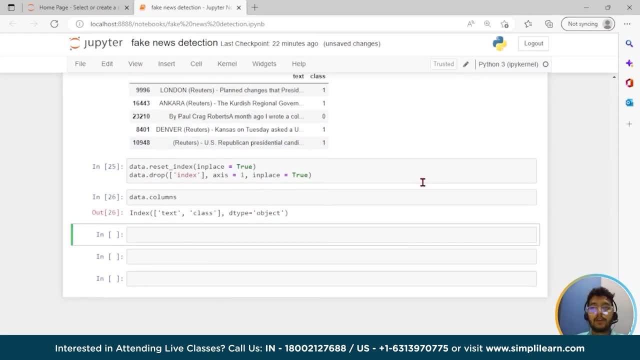 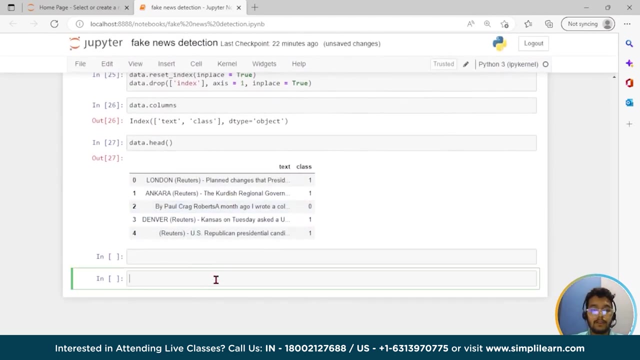 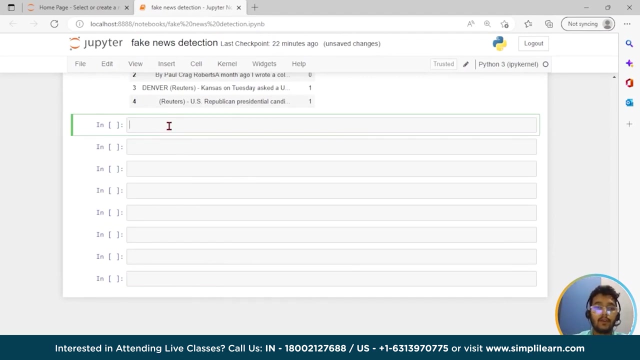 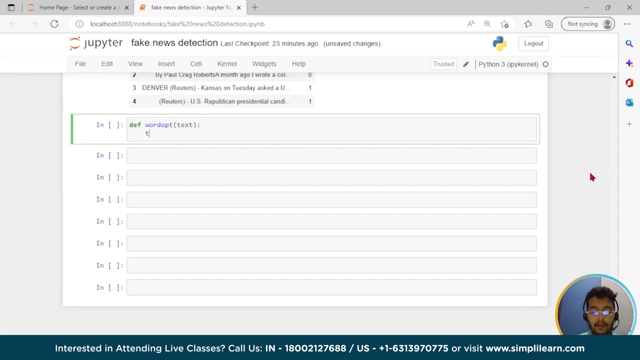 two columns only rest. we have deleted. okay, let's see data dot add. everything seems good. let's proceed further and let's create a function to process the text. okay, okay, for that i will write here. but okay, you can use any name, text and text equal to text dot. lower. okay, and 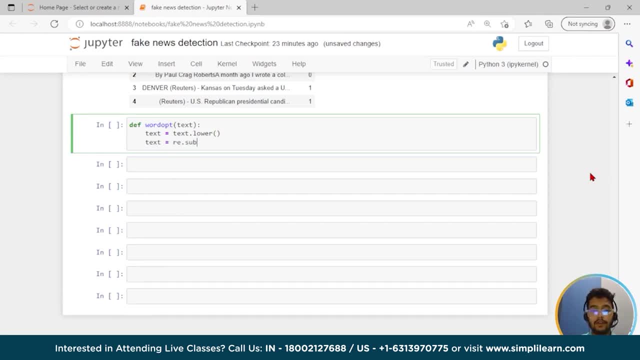 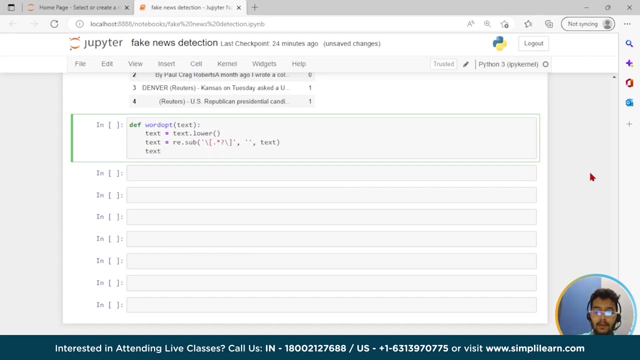 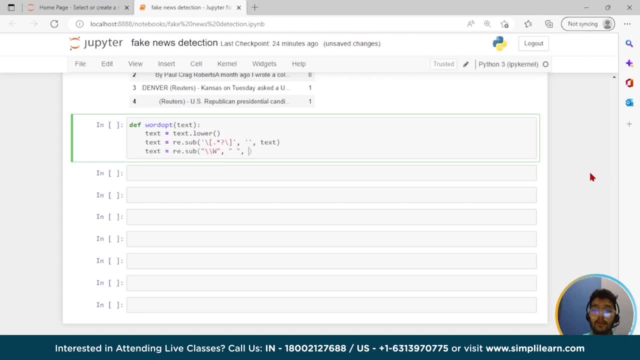 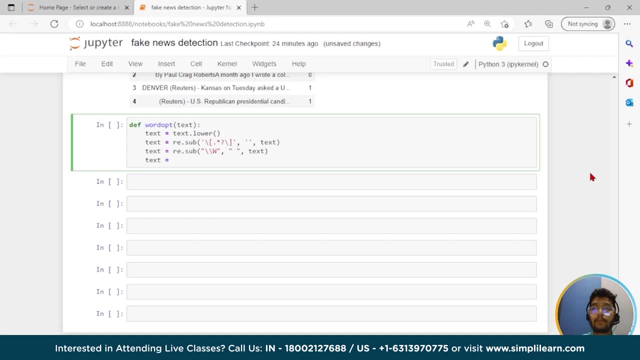 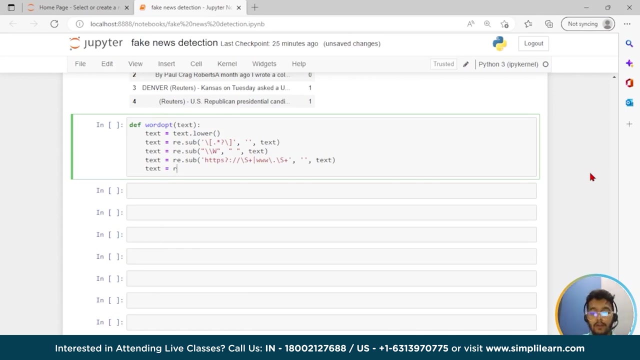 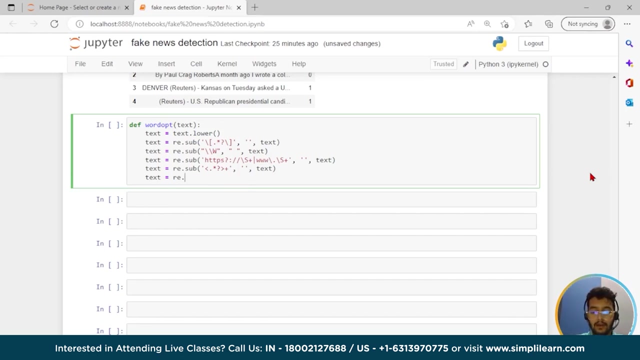 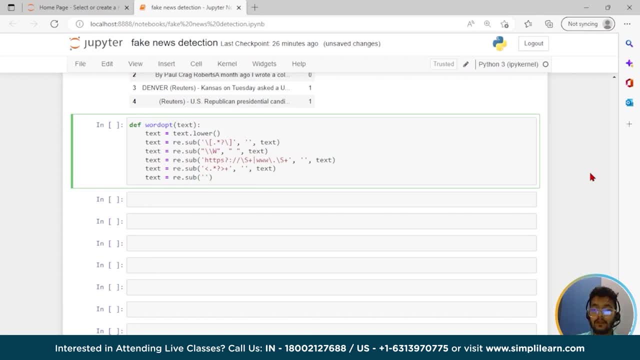 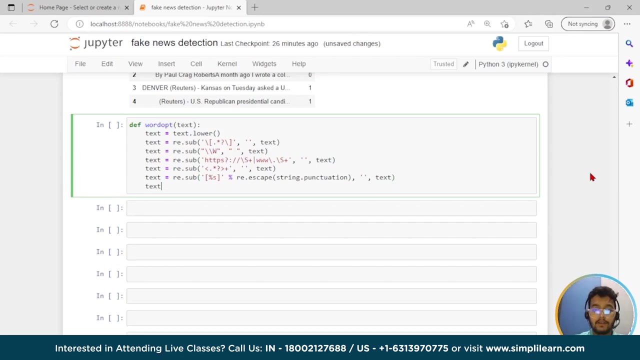 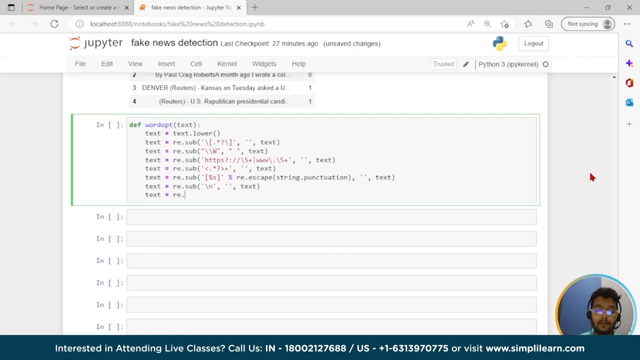 then percentage, as again percentage for re dot escape function. right here string dot punctuation, comma, then comma, then text. right, then text equals to re dot substring and n comma text equals to re dot substring. right here and again t and again ok, so then comma, then again text. 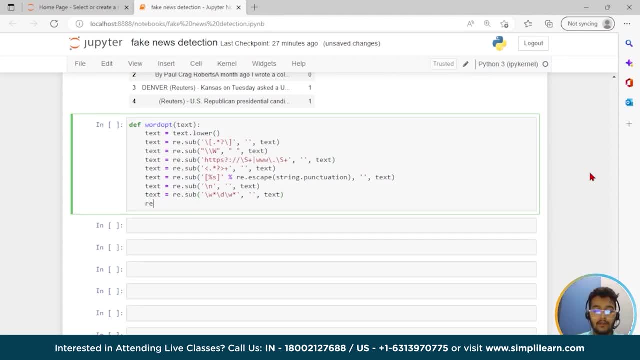 then at the end I have to write here: return text. so everything like this type of special character will be removed from the data set. ok, let's run this. yeah, so here I will write df- sorry, not df- data data. then text pursue data dot apply to the function in wordport. 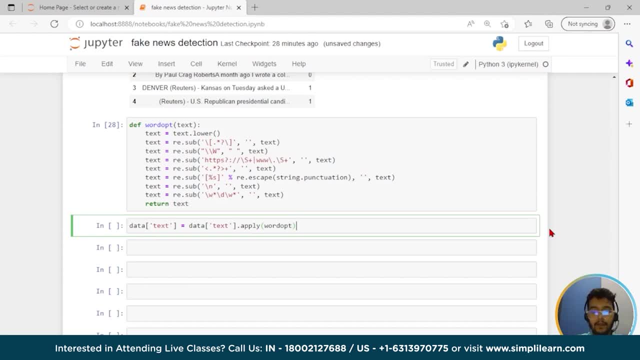 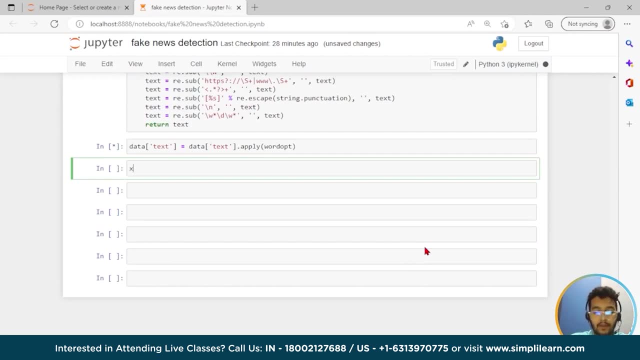 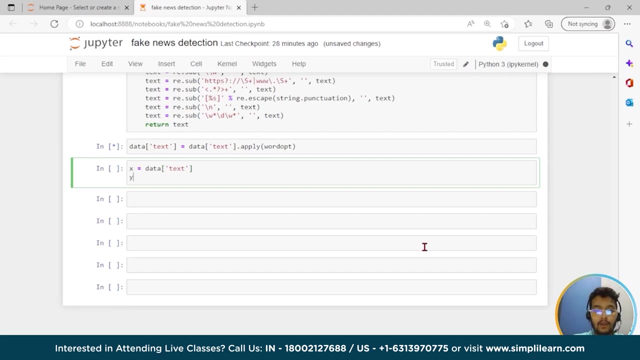 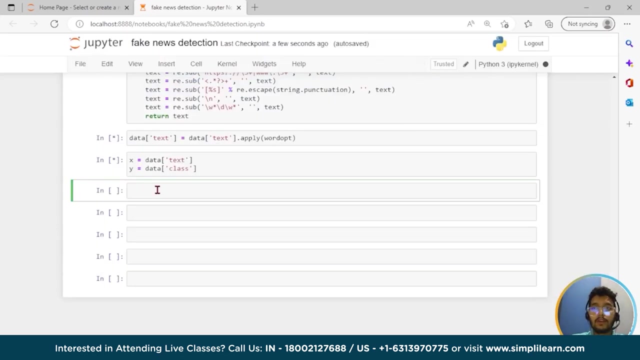 word opt. ok, press enter. yeah. so now let's define the dependent and independent variables. ok, x equal to 2, yquassu data text and yquassu data class. okay, then splitting training and testing data: okay, sorry, so here i will write x underscore train comma, x underscore test. 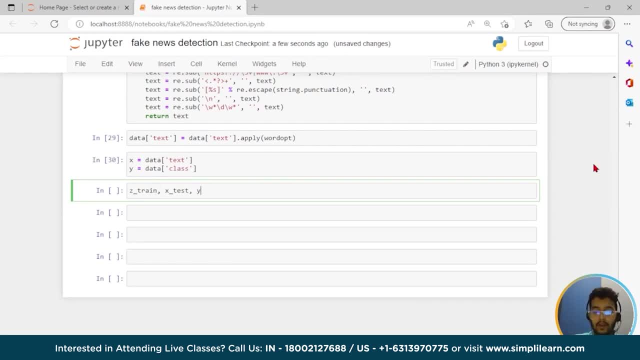 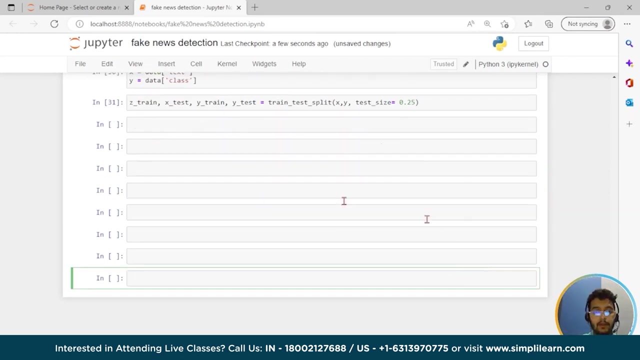 uh, then y underscore train comma. y underscore test goes to train underscore test, underscore split. then x comma, y comma test. let's go. size goes to 0.25. okay, press enter. so now let's convert text to vectors. for that i have to write here: that is x. 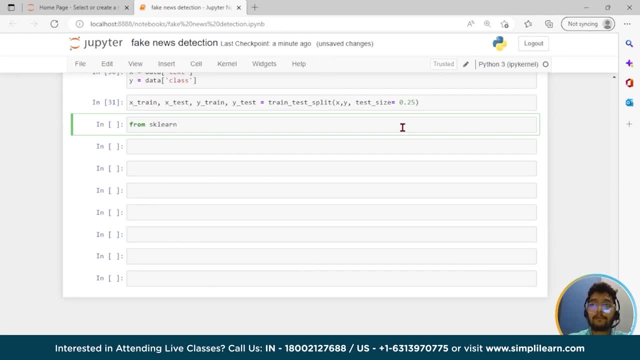 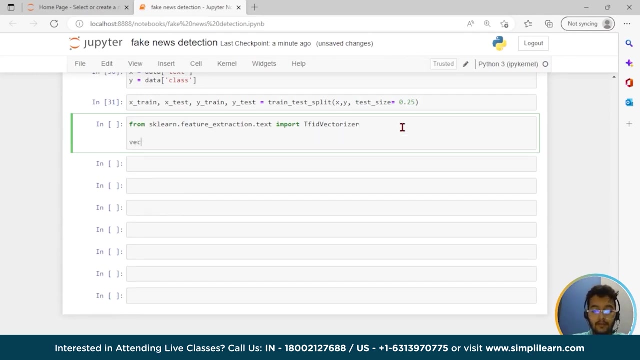 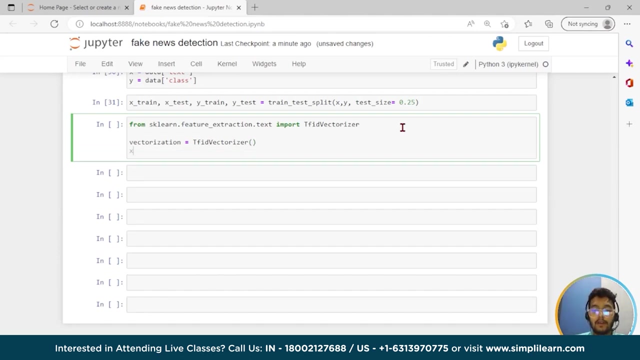 so here i will write from escalon: dot feature: extraction dot text: import e vectorizer. okay, then vectorization equals to g, f, i, d vectorizer. okay, then three underscore train equals to vectorization, or is that it? yeah, vectorization: dot fit, then transform x underscore train. 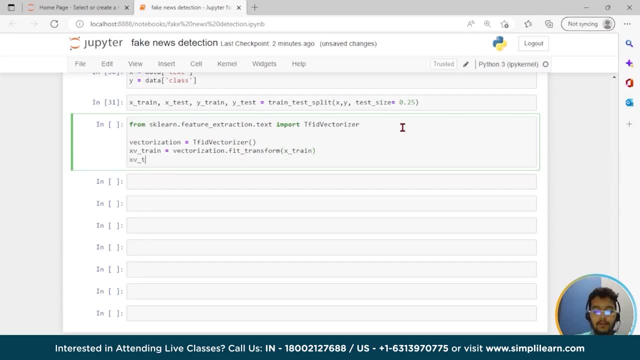 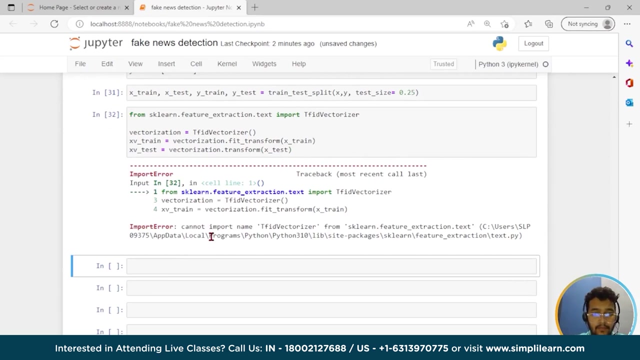 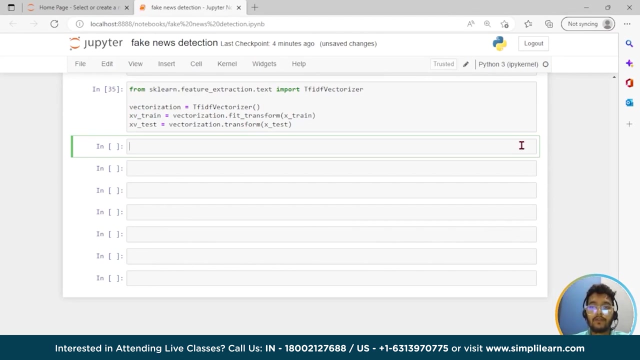 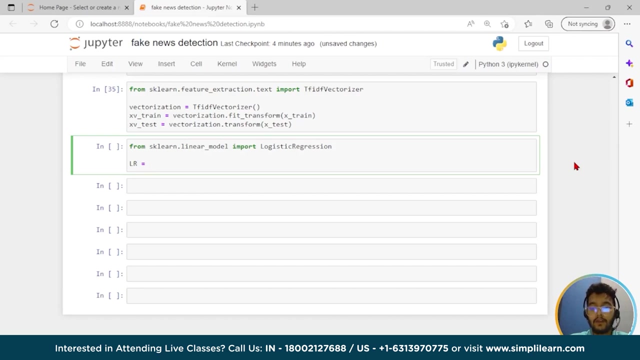 okay, then xv underscore test equals to characterization equation dot. transform x underscore test. okay and press enter. so now let's see our first model, logistic regression. so here i will write from escalon dot: linear underscore model: okay, import logistic creation. okay, then lr goes to logistic regression. 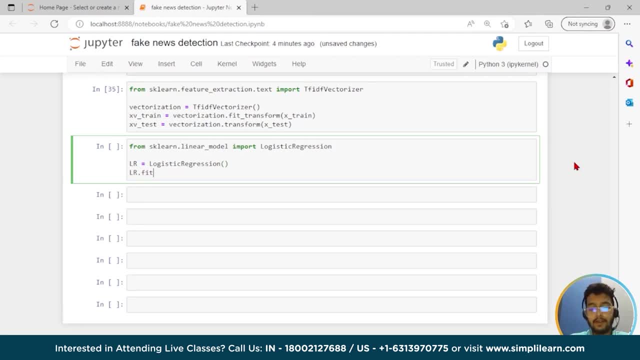 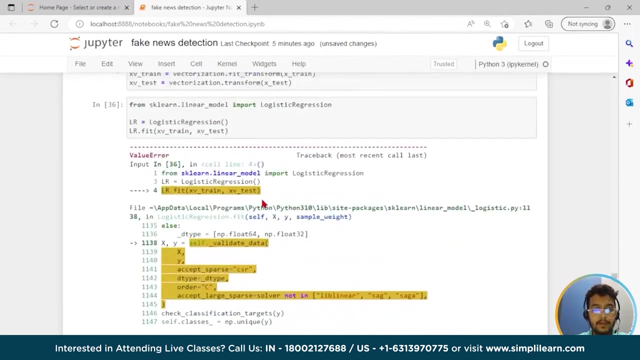 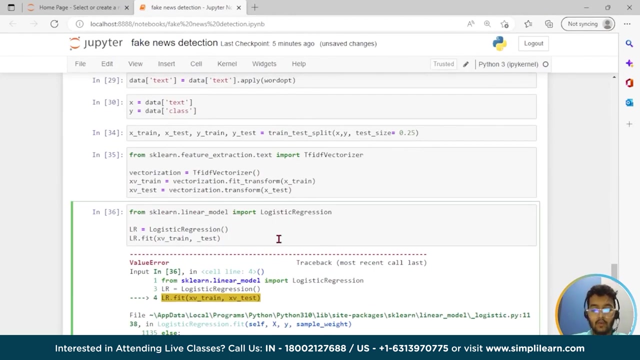 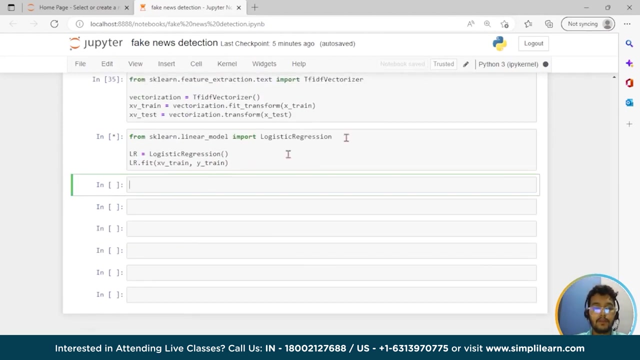 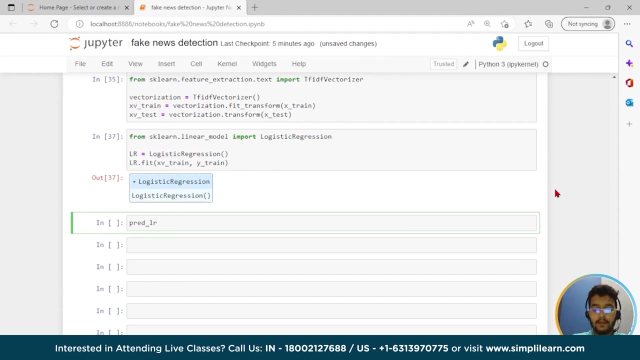 i have to write here lr dot fit, then xv dot dot train, comma xv underscore test. okay and press enter here: l dot xv dot train. okay. here i have to write y train, okay, and press enter will work. so here i will write: prediction underscore- linear regression question. 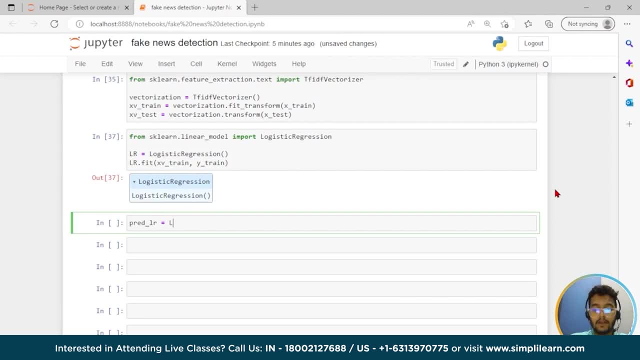 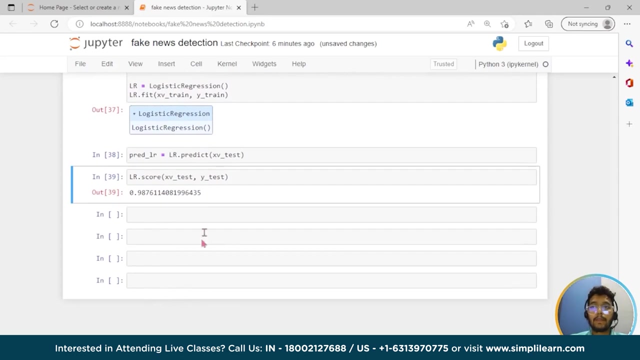 so here i will write prediction: underscore linear regression matrix: l r dot predict. let's go test. okay, let's see the accuracy score. for that i have to write lr dot score. then xv underscore test, comma y underscore test. okay, let's see the accuracy. So here, as you can see, accuracy is quite good, 98 percent. now let's print the classification. 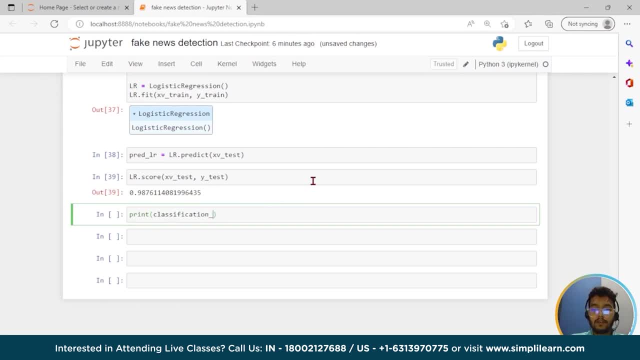 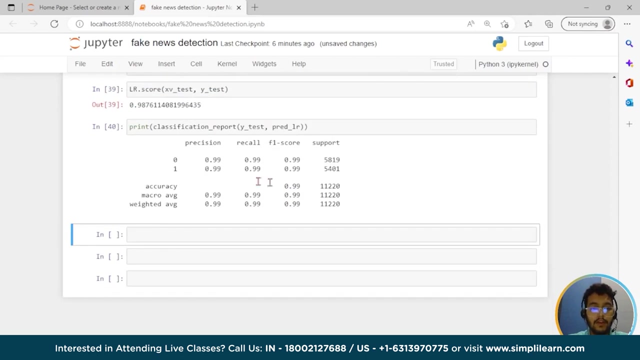 So this is: you can see precision score, then F1 score, then support value, accuracy. okay, so now we will do this same for the decision tree gradient boosting. So now we will do this same for the decision tree gradient boosting classifier, random forest classifier: okay, then we will do model testing, then we will predict this. 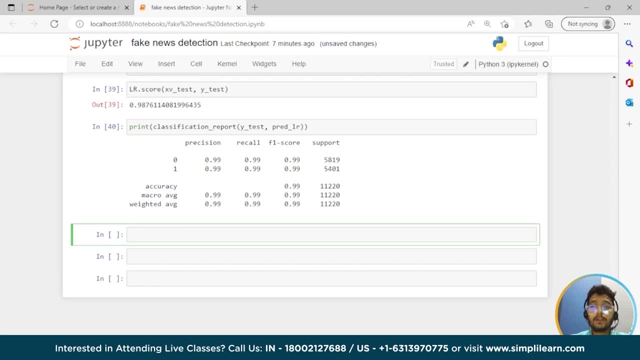 classifier: random forest classifier. okay, then we will do model testing, then we will predict this. so now for the decision tree classification. so for that I have to import from sk learn dot free import decision re classifier: okay, then at the short form i will write here, copy it from here then. 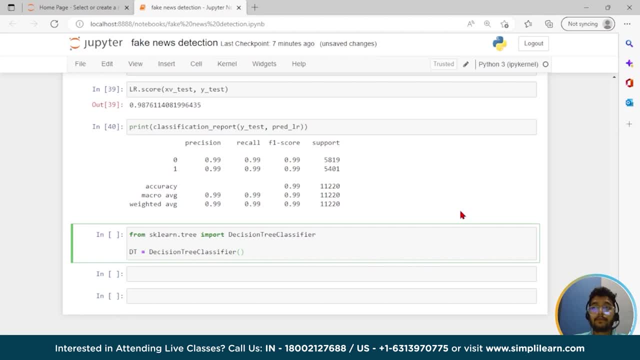 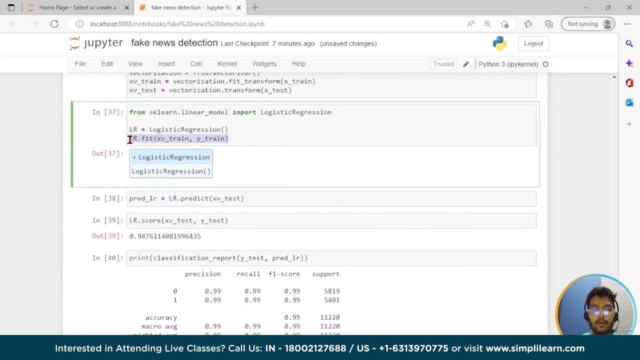 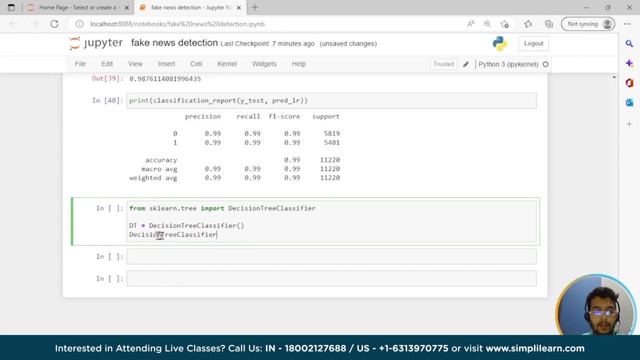 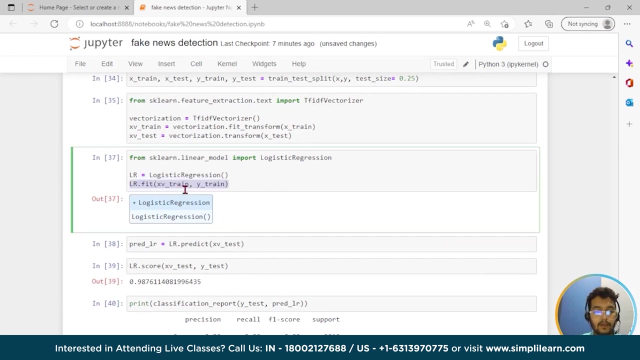 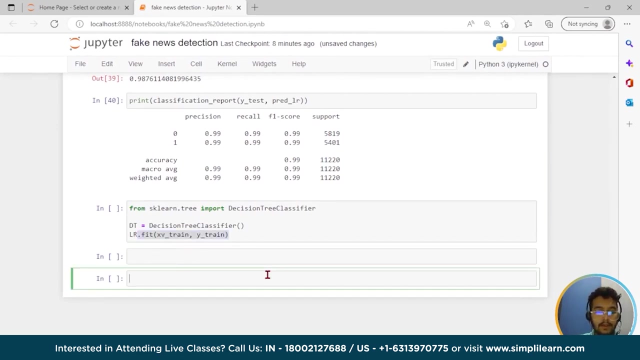 okay, then i have to write the same as this, so i will copy it from here. and let's change linear regression to season three classifier. okay, then i will write here same dt question, okay, okay. okay, then let's just write g t dot, predict three. let's go things. 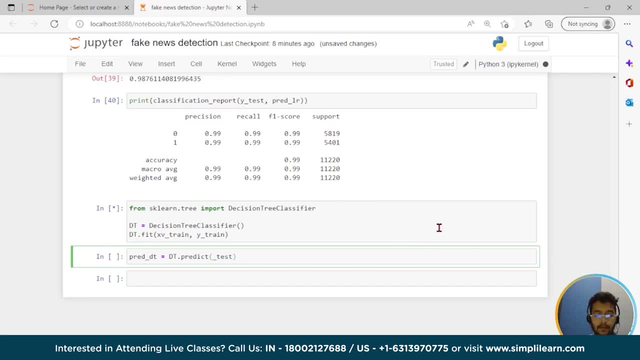 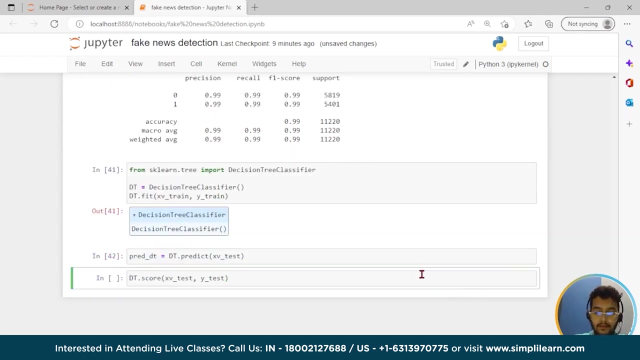 3010 gt, dot predict three. let's go test. still loading. it will take time. okay, till then, let me write here for the accuracy: 3 underscore test, comma y. let's wait. okay, the accuracy. so, as you can see, accuracy. 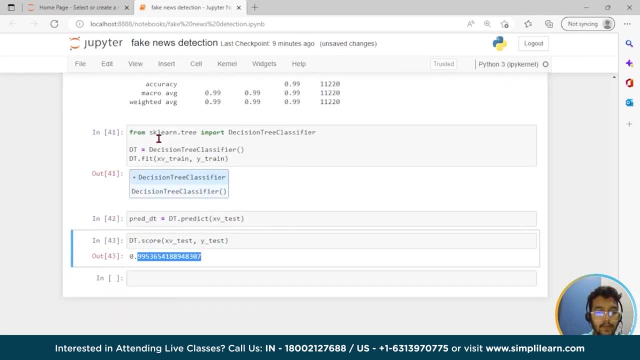 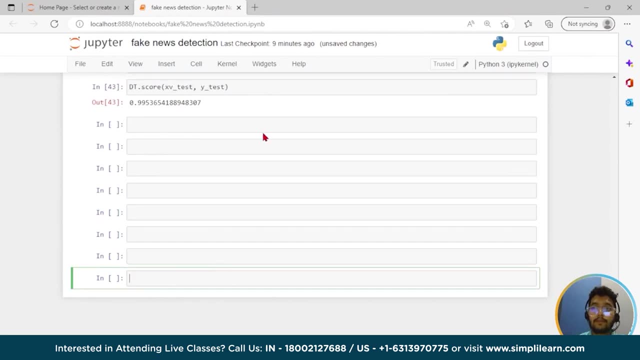 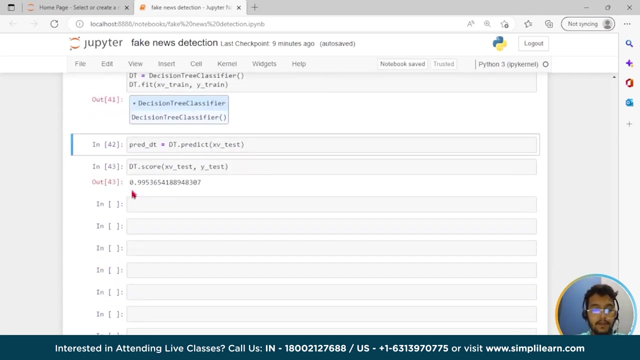 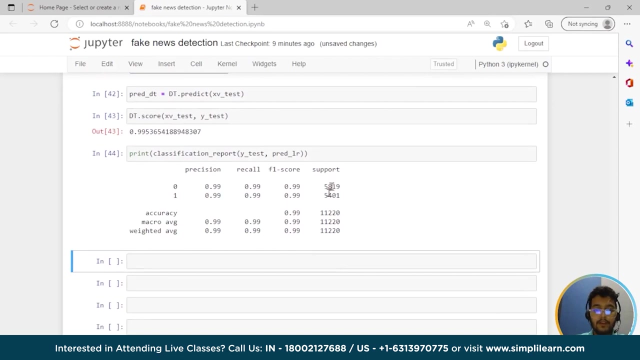 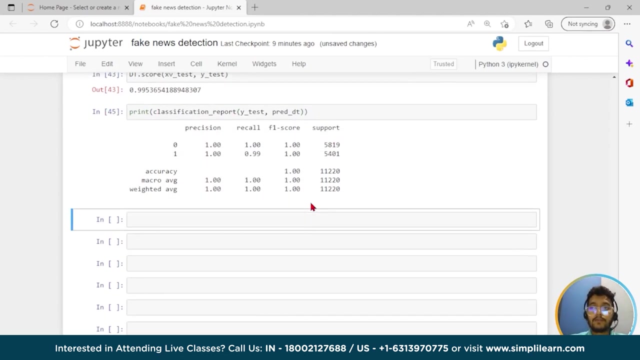 is good than this. linear regression okay. logistic regression okay. so let me, let me predict print. okay, so this is the accuracy score. this is all the report. okay, so this is the accuracy score. yeah, now let's move for the gradient boosting classifier. okay, 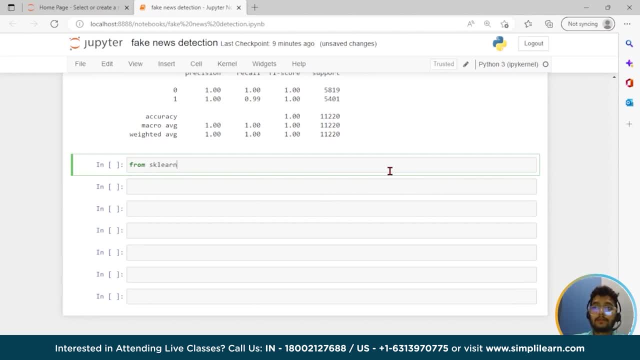 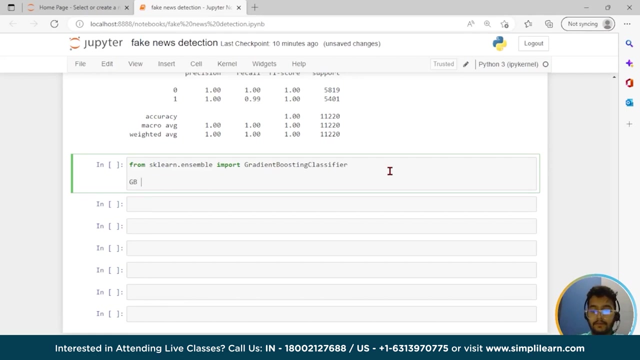 for that. I've read from sql dot ensemble: fourth gradient, boosting classifier- classifier. I will write here: gb equals to. let me copy it from here. okay, I will give here random underscore state: 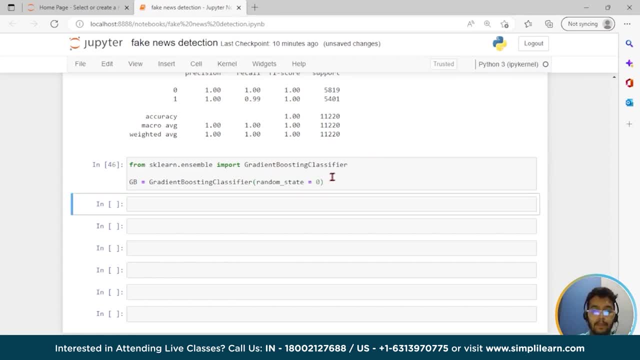 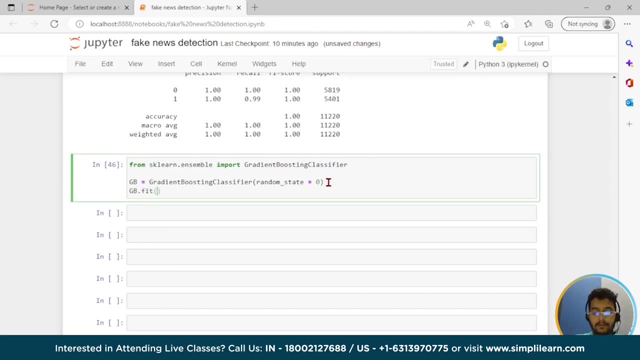 equals to zero. wait, wait, wait, wait. so I will write here: gb dot state xv underscore train. comma y underscore train. okay, then press enter here I will write: predict underscore. 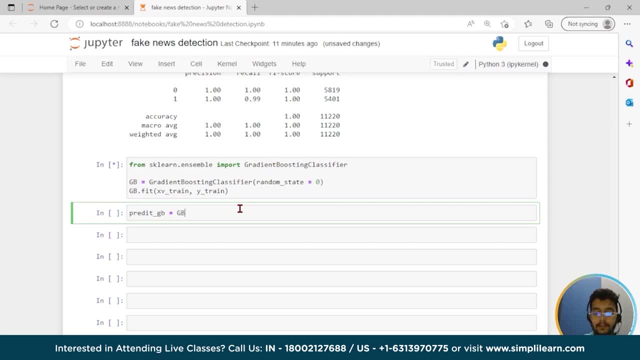 gb equals to gb dot weight. sorry, predict three: dot test or dot underscore test. okay, till then it's loading, so I will write here for the score and I will write gb dot. 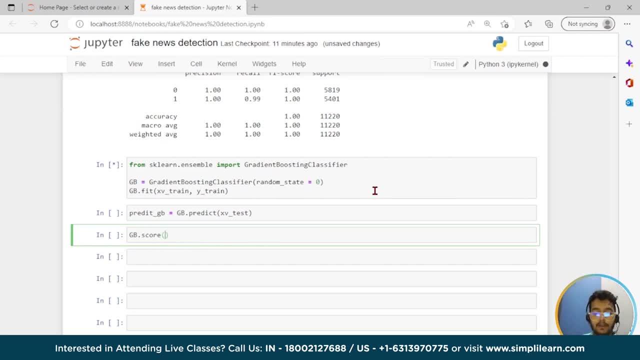 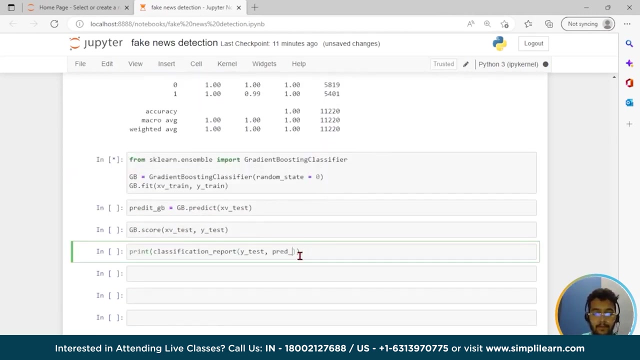 score, then three underscore test, comma y underscore test. okay, so let's wait. it is running this part. till then let me write for the printing this here. it's taking time. 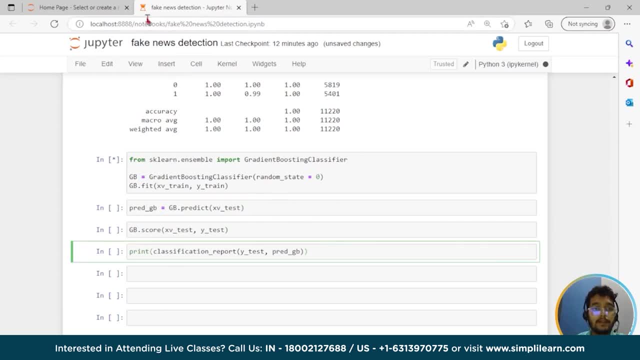 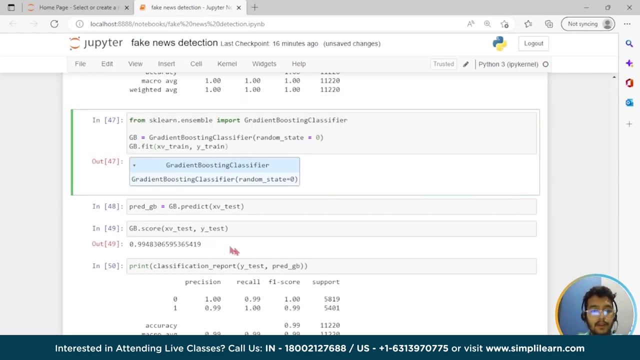 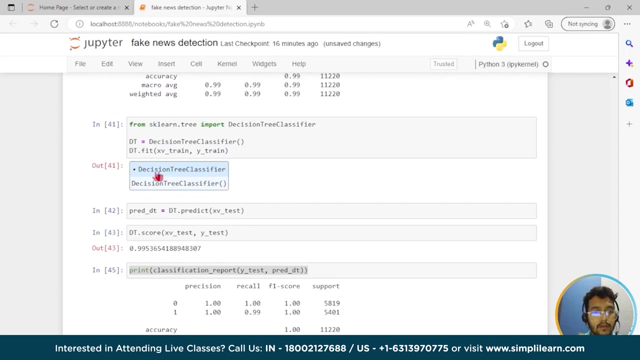 taking time, still taking time, but if I will run this, it's not coming because of this. yeah, it's done now, so you can see the accuracy is not good then decision tree, but yeah, it is also good. 99.4, something. 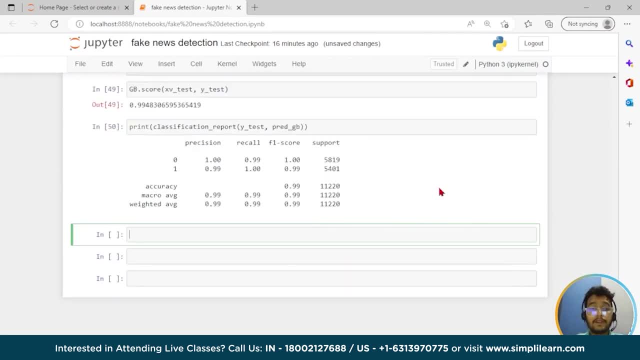 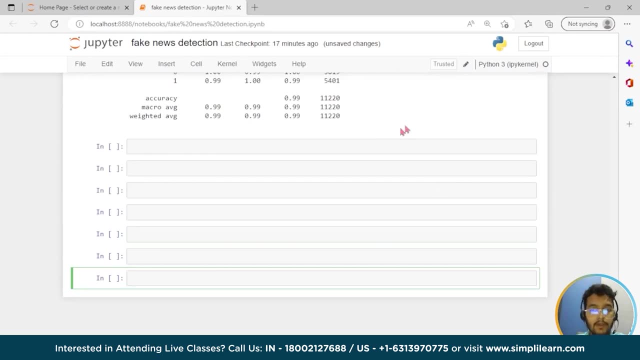 I just got the now. if it's on zero, it's my trade. if it's too low, it's too low. right, that's not good. think what if it's minus 13, okay, it's good. I don't know something not good. but if I 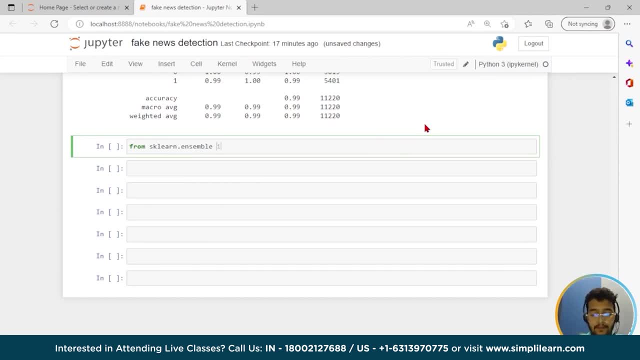 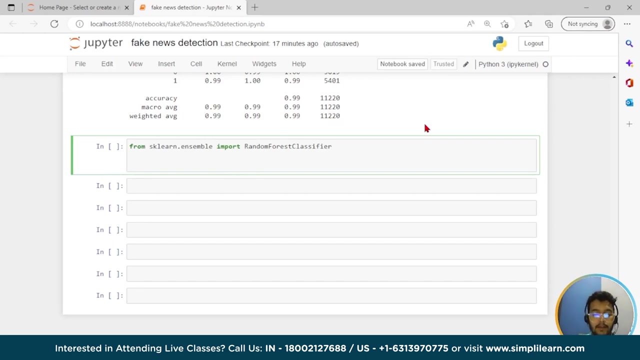 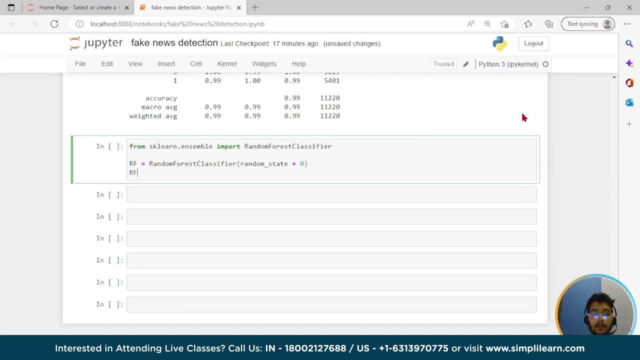 want toのm and the assembly is load, then these and on however long. so classifier okay, and here i will write: rf was to write, i will copy it from here, then random state: first, here we go, then r dot fit. 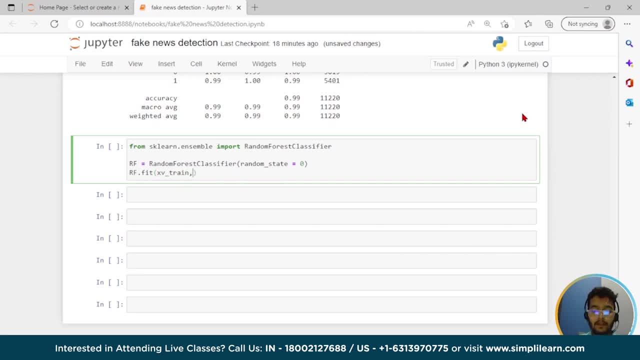 three underscore train: comma y underscore train. okay, then press enter and predict underscore rc or f. let's go us to rf dot. predict c underscore test. okay, till then i will write here. it's still loading, it will take time, so till then i will write for the score. score: accuracy score xv underscore test. comma y underscore test. okay, then i will. 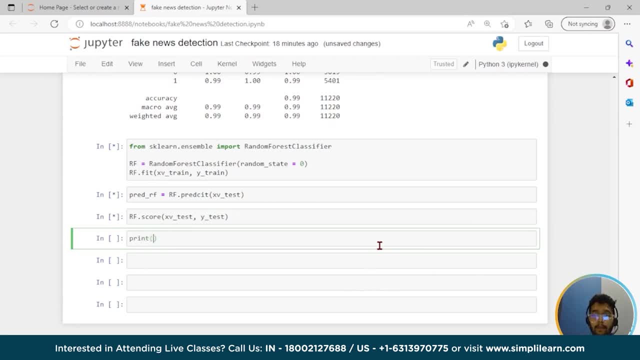 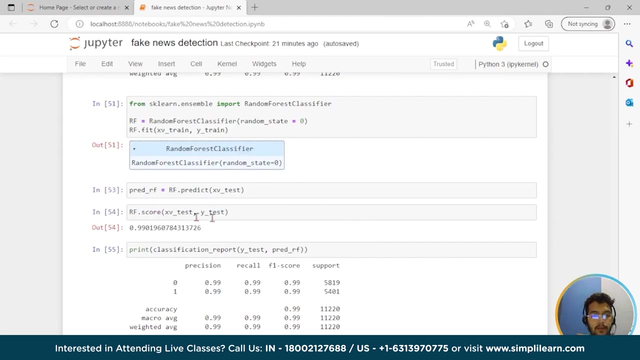 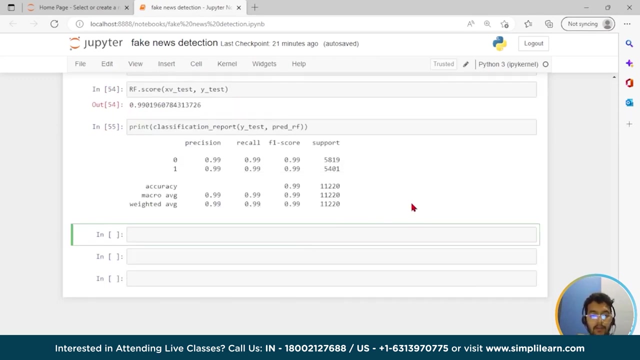 write here till then. print classification quote. and y underscore test comma. it will take time little bit. so uh, it run. the accuracy score is 99. it is also good. so now i will write the code for the model testing. so i will get back to you by after writing the code. so 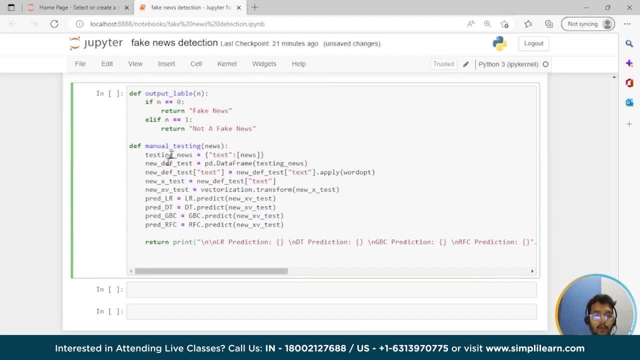 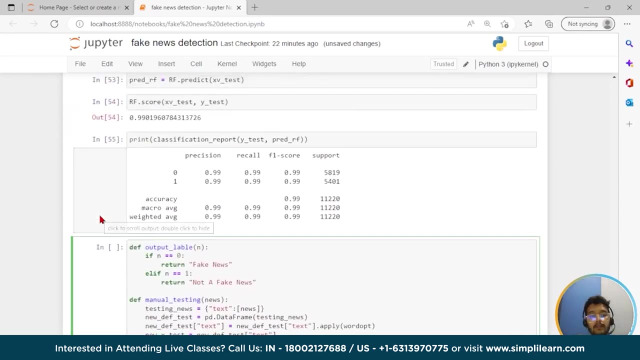 so i have made two functions: one for the output label and one for the manual testing. okay, so it will predict the all the from the all models from the it. so it will predict the it- the news is fake or not- from all the models. okay, so for that let me write. 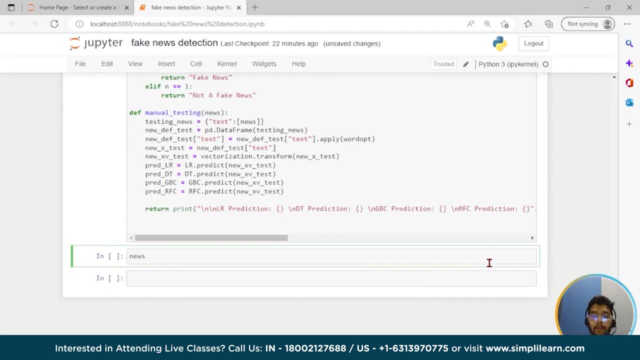 here news was to string what. okay, then i will write here manual underscore testing. okay, so here i will. you can add any news from the. you can copy it from the internet or whatever, from wherever you want. so i'm just copying from the internet. okay, from the google. 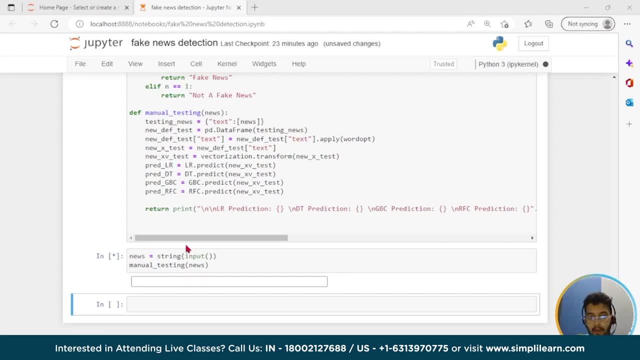 the news which is not fake. okay, i'm just copying from the internet. okay, from the google, the news which is not fake. okay, i'm just copying from the internet. okay, from the google, the news which is not fake. okay, i'm adding: which is not fake, because i already know. i searched on google, so i'm entering. 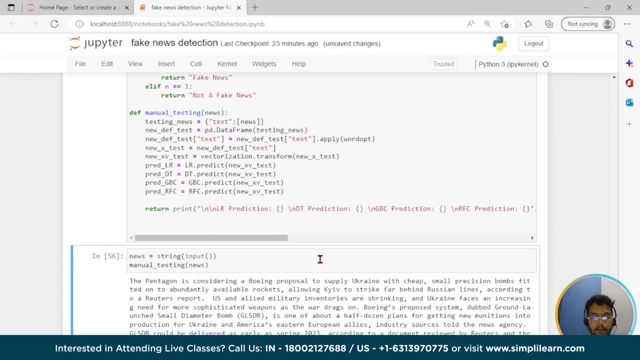 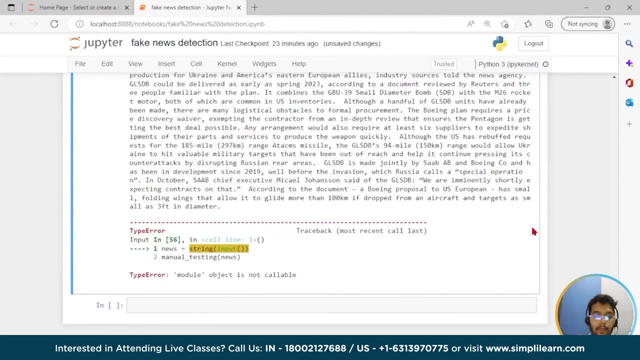 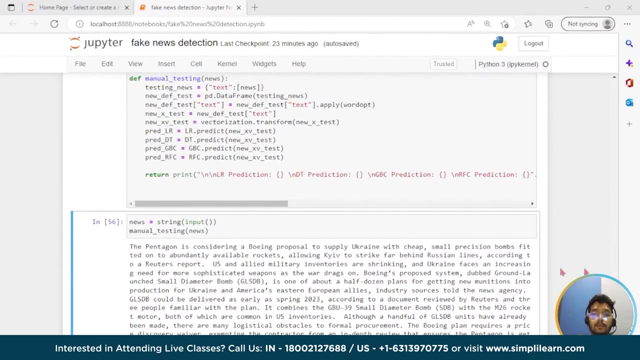 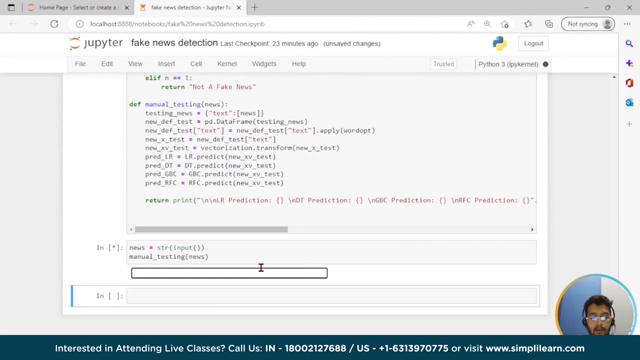 this. so just run it, let's see what is showing. okay, string. okay, object is not callable. okay, let me check this first. okay, i have to give here str only. yeah, let's check. okay, i have to add here again the script. yeah, manual testing is not defined. 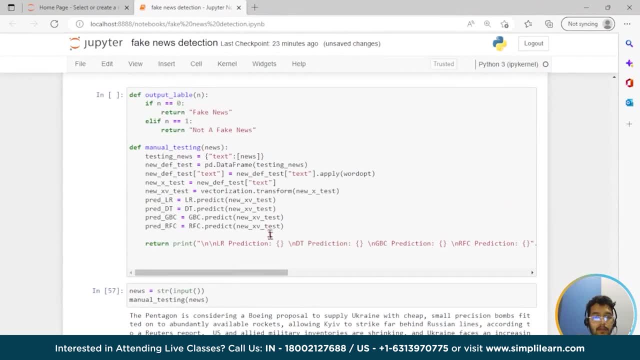 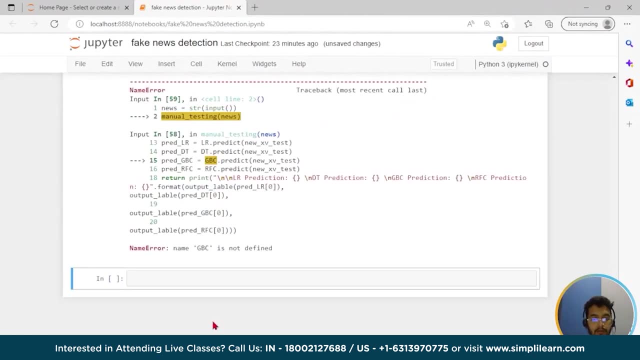 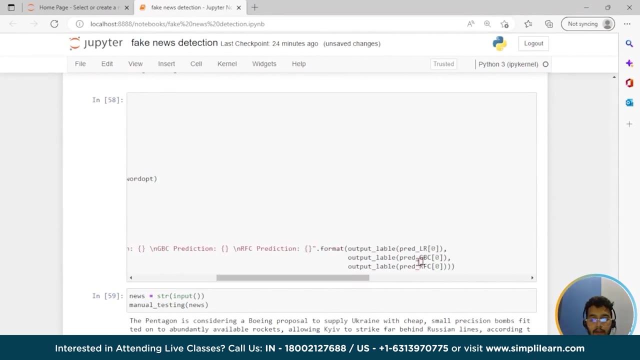 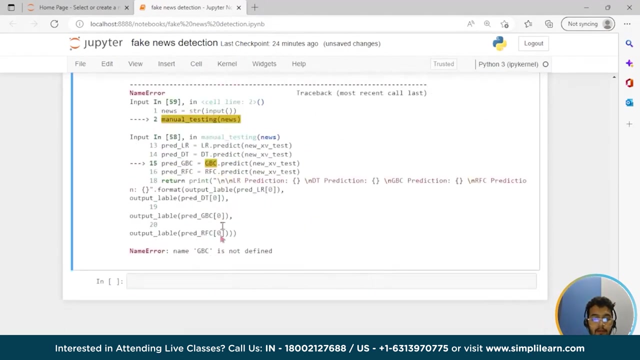 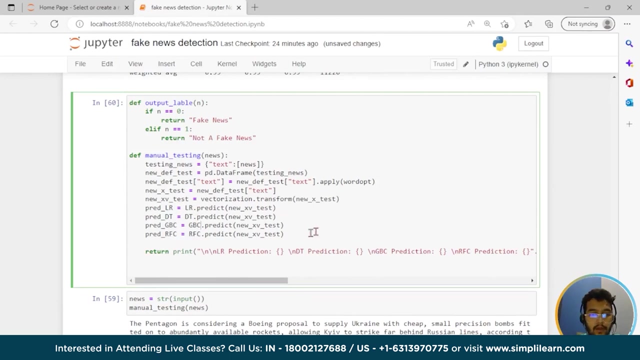 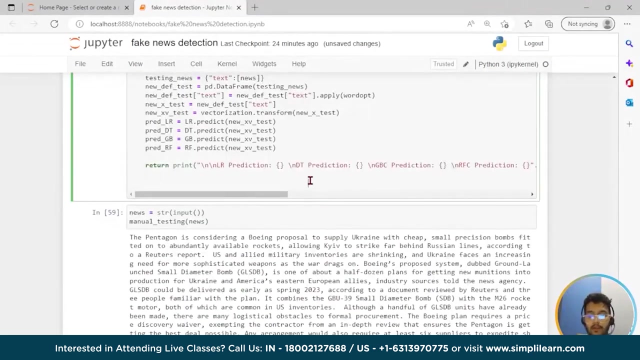 let me see manual testing. okay, i have to edit something. it is just gb and it is just rf. gbc is not defined, okay, okay, so what i have to do? i have to remove this, this. everything seems sorted. now, give me a year. first, I don't need blogs. 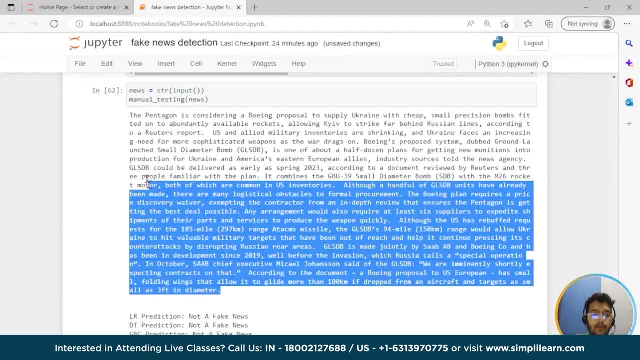 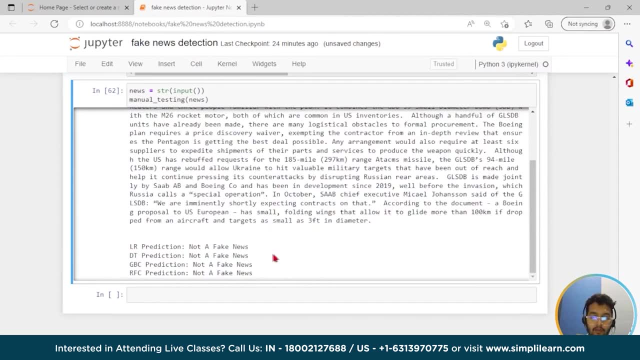 as I said to you, I just copied this news from the internet. i already know the news is not fake, so it is showing not a fake news. okay, so now what I will do. I will copy one fake news from the internet and let's see it is detecting it or not. 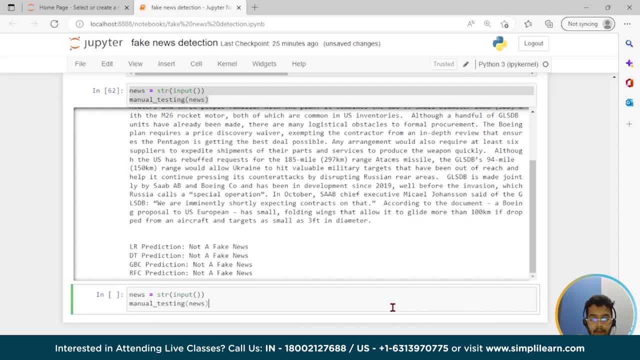 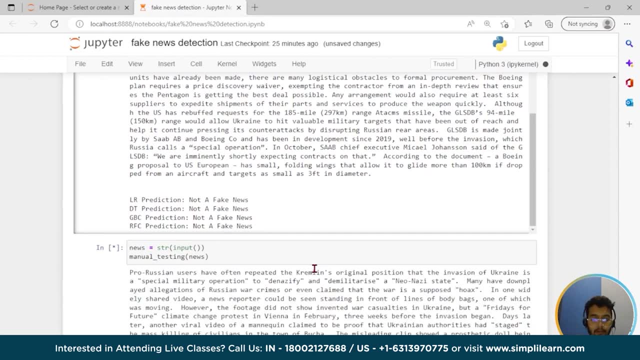 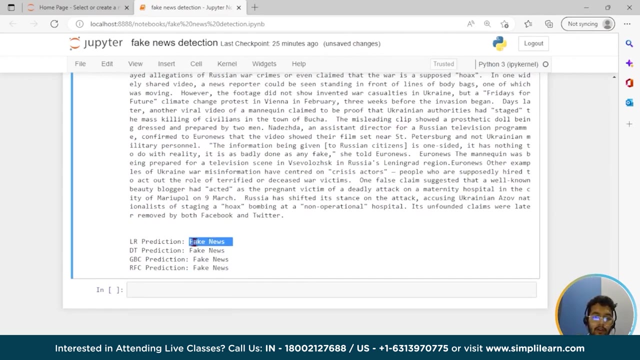 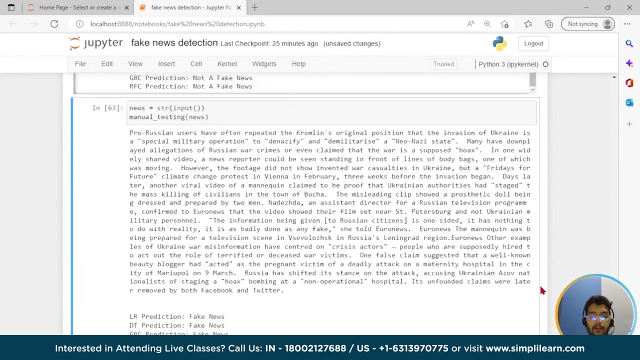 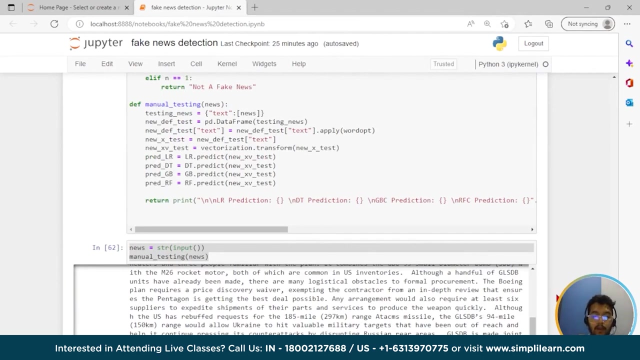 okay, So let me please run this and let me add the news for this, so all the models are predicting: right, it is a fake news. or you can add your own script like: this is the fake news. okay, i hope you guys understand till here. so i hope you guys must have understand how to detect a. 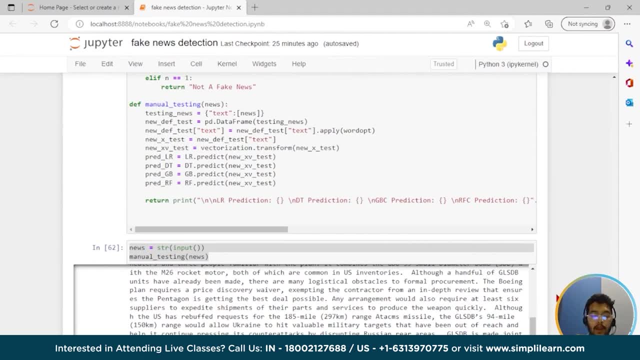 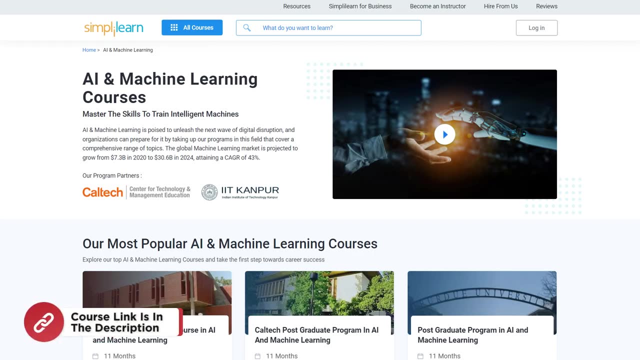 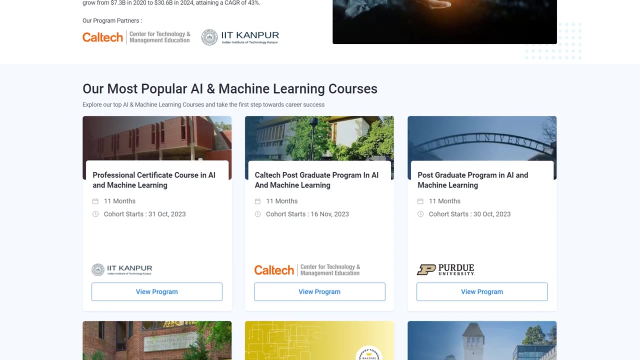 fake news. using machine learning, you can. you can copy any news from the internet and you can check it is fake or not. if you want to become an ai expert and gain handsome salary packages, look at the wide range of ai ml courses by simplela, in collaboration with top universities. 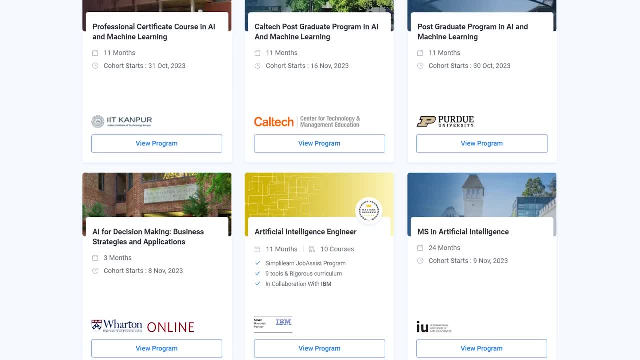 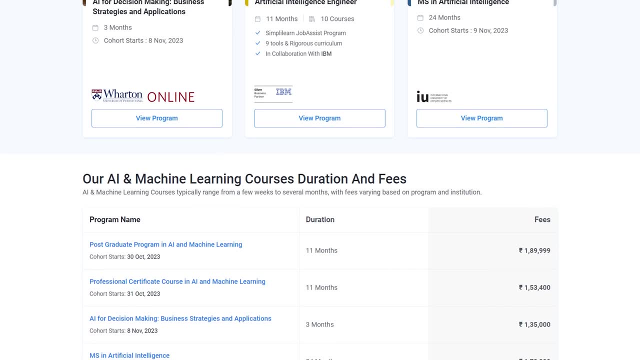 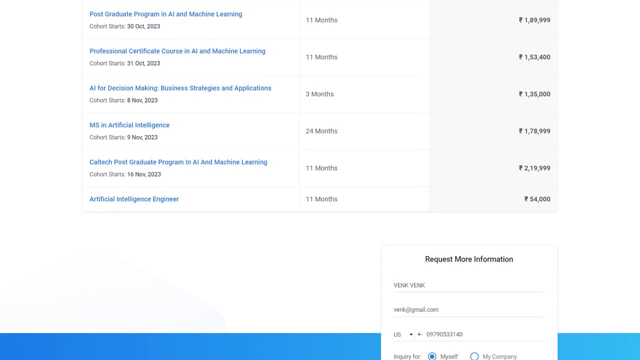 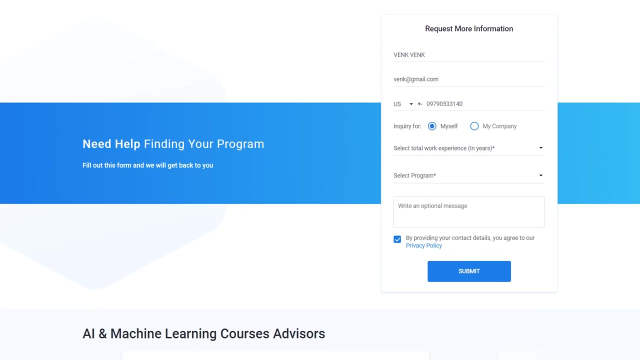 across the globe. by enrolling in any of these certification programs, you will gain expertise in skills like generative ai, prompt engineering, chat, gpt, explainable ai and machine learning algorithms, supervised and unsupervised learning, model training and optimization, and there is much more on the list, with hands-on experience in the tools like chat, gpt, dali, python, open. 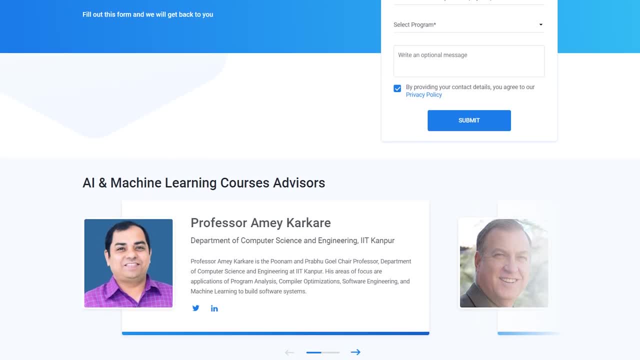 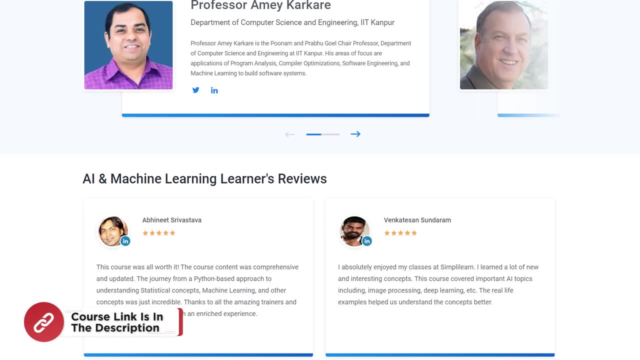 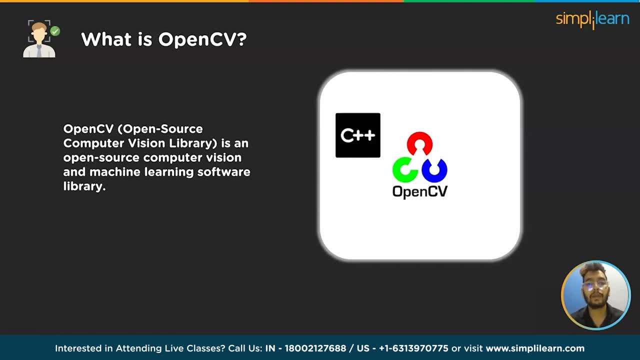 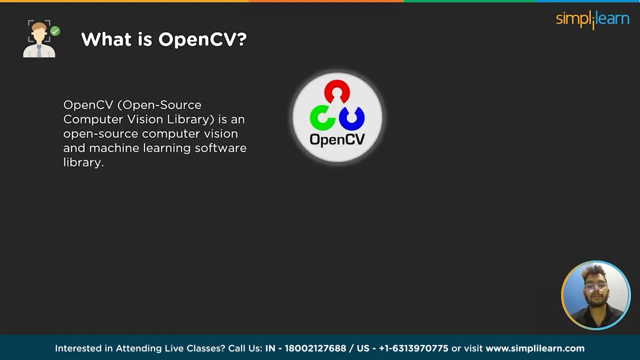 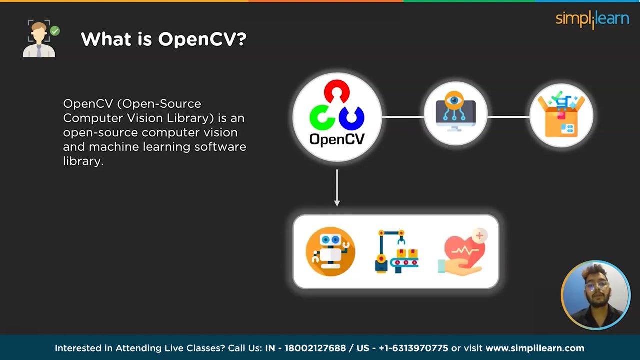 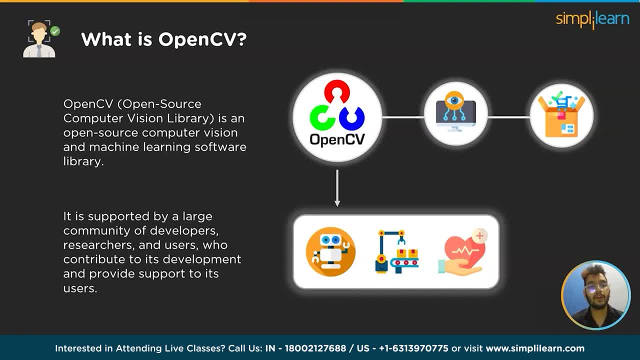 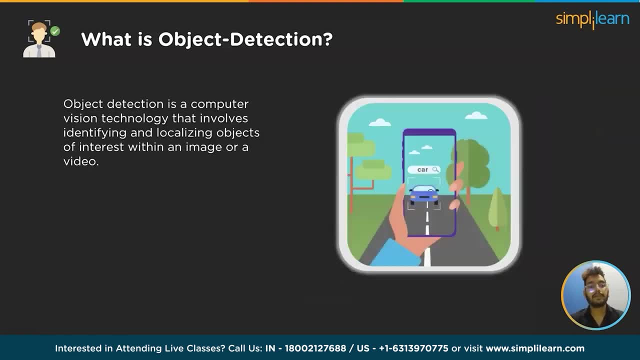 It is supported by a large community of developers, researchers and users who contribute to its development and provide support to its users. so now let's see what is object detection. object detection is a computer vision technology that involves Identifying and localizing the object of interest within an image or a video. 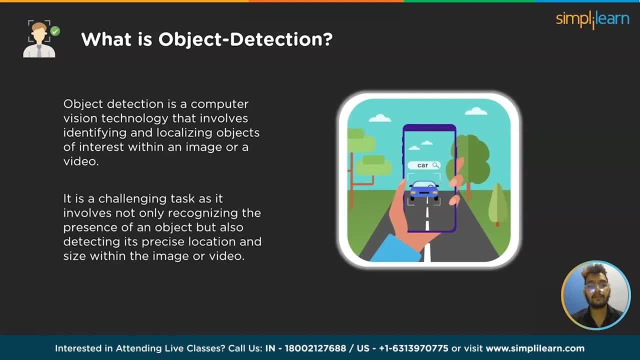 It is a challenging task, as it involves not only recognizing the presence of an object, But also detecting its precise location and size within the image or video. Object detection algorithm typically used deep learning techniques, such as CNN, to analyze the image or video for identifying the objects. 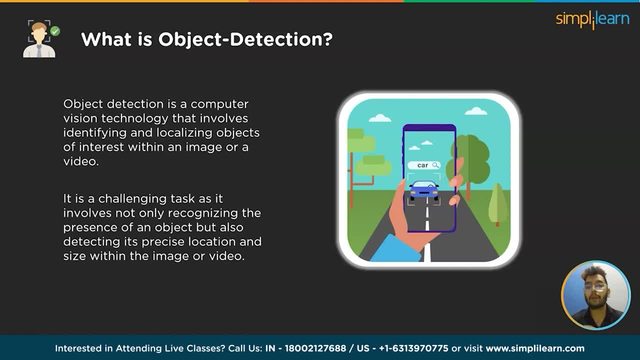 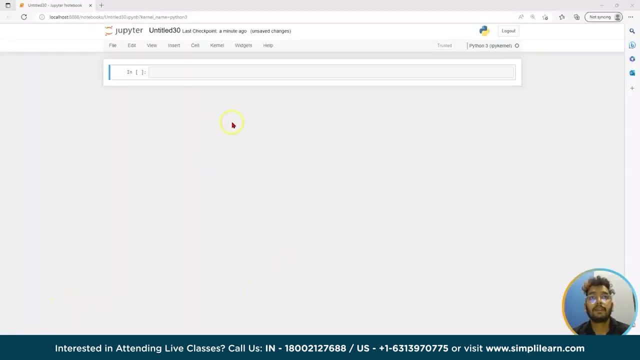 These algorithms can also determine the boundaries of the object by drawing a bounding box around them. So after understanding what is object detection, now let's move on to the programming part. So this is a kernel, Python kernel. Here we will change this name. 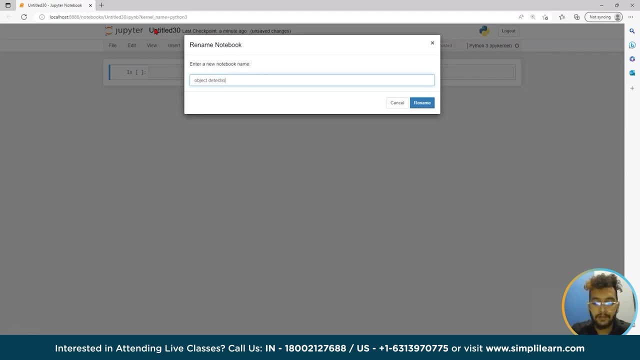 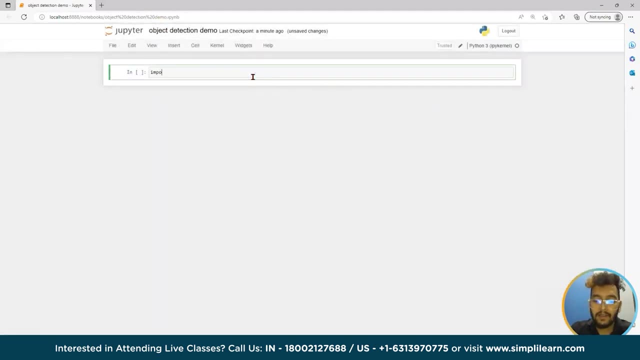 So here I will write object detection demo. Okay, so first we will import some major library like OpenCV, So for that we will write import cv2, and the next one is import matplotlibpyplot as plt. So why we are writing plt? Because we can't write again and again matplotlibpyplot. 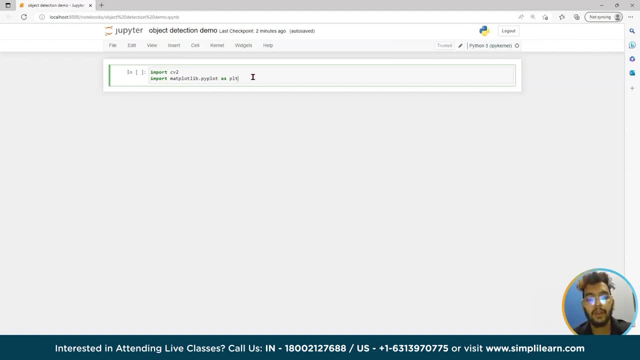 Okay, it's a long one, so we can write a short form plt. So yeah, let's run this. So what is OpenCV? OpenCV is an open source software library for computer vision and machine learning. The OpenCV full form is open source computer vision library. 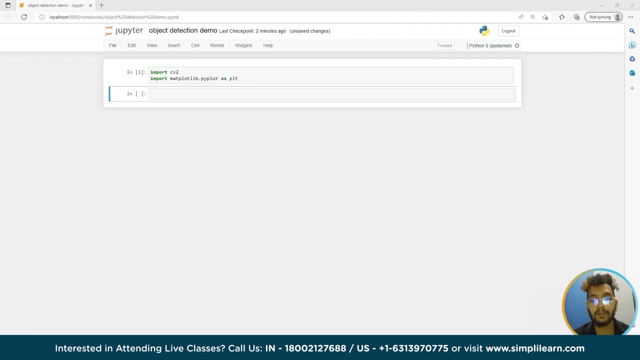 It was created to provide a shared infrastructure for application for computer vision and to speed up the use of machine learning perception in consumer products. OpenCV as a BSD license software make it simple for companies to use and chase the goal. Okay, So there are some. 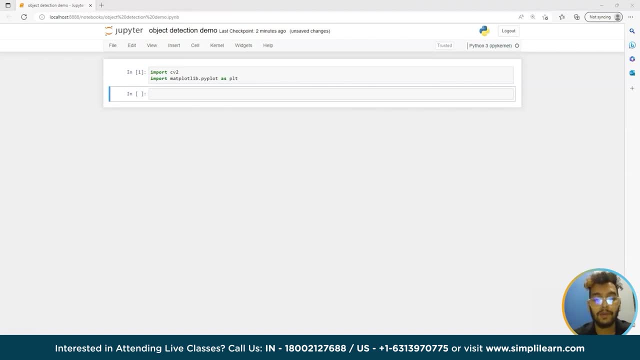 predefined packages and libraries that make our life simple, and OpenCV is one of them. Second one is matplotlib. Matplotlib is a easy to use and an amazing visualize library in Python. It is built on numpy array and designed to work with broader scipy stack, and consists of several plots like line bar, scatter, histogram and many others. 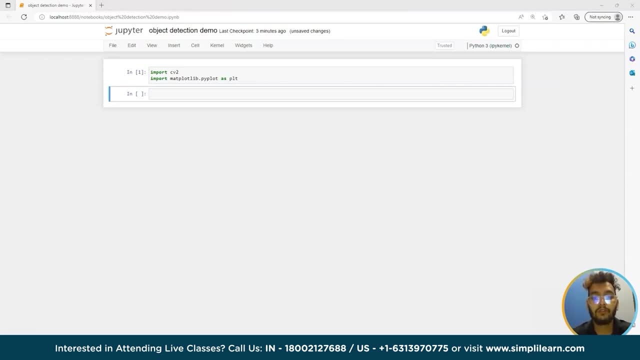 Okay, so, moving forward, we will import our file. Okay, so here I will write config. file goes to: this is our filename: SSD, ssd. underscore, mobilenet b3, large coco- 20, 20, 22, 22, 22, 30, 27. 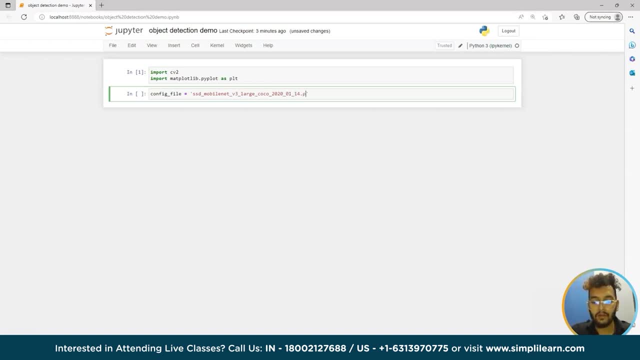 30, 14, 14, 14.. find this file on the description box below: frozen model question. explain you. 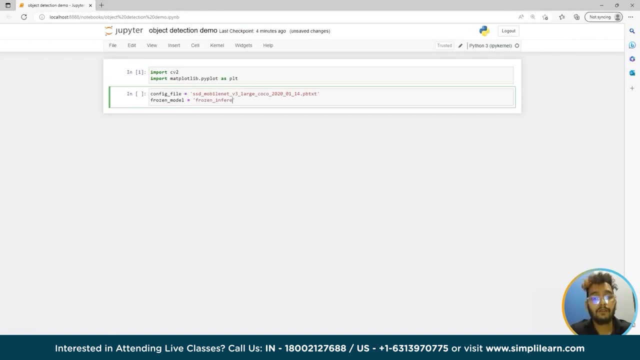 every single thing. inference graph- dot PV. okay, so let me run it first. mobile net as a name applied. the mobile net model is designed to use in mobile application and it's tensorflow first. mobile computer vision model. mobile net use depth-wise separable convolutions. it significantly reduces the numbers of 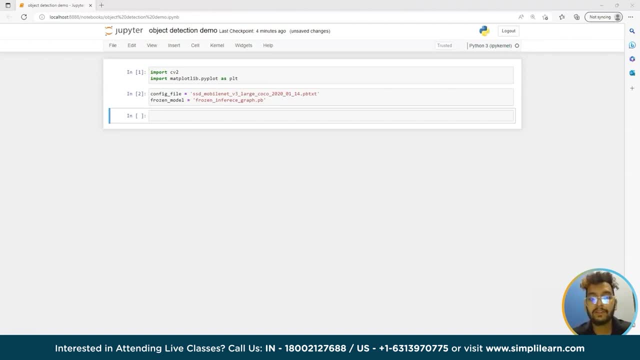 parameter when compared to the network with regular convolutions with the same depth in the Nets. this is that in the lightweight of the deep neural network. so mobile net is a class of CNN that was open source by Google and therefore this gives us an excellent starting point for training our classifiers that are 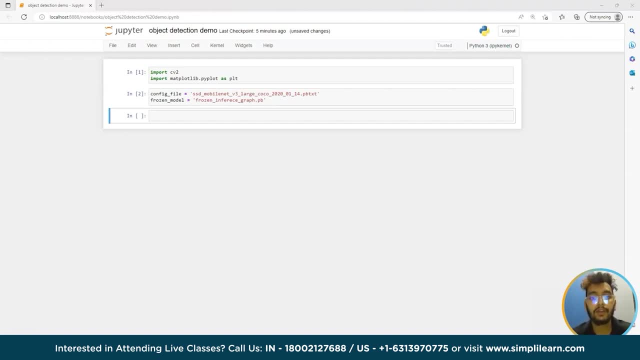 insanely small and insanely fast. okay, so what is this large coco? this is a data set- coco data set. like with applications such as object detection, segmentation and captioning, the coco data set is widely understood by the state-of-the-art of neural network. its versatility and the multi-purpose scene variation serve best to train a computer. 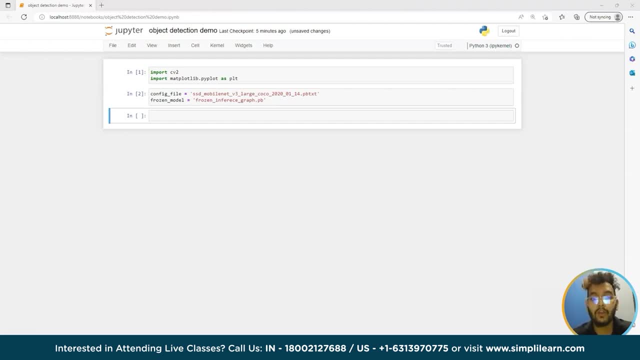 vision model and benchmark its performance. okay, so what is coco? the common object in context is one of the most popular large-scale label images data set available for public use. it represent a handful of object we encounter in the data set on a daily basis and contains image annotations in 80 categories I will show. 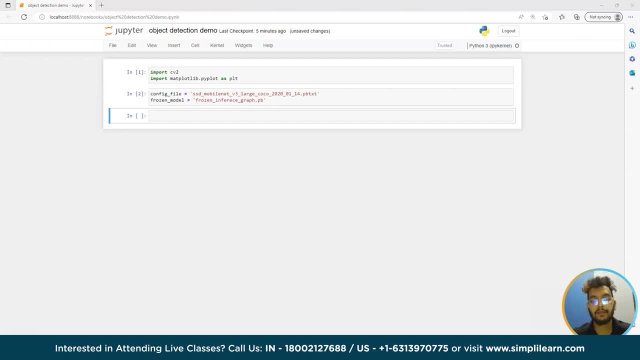 you the categories I have with over 1.5 million object instances. okay, so modern day AI driven solution are still not capable of producing absolute accuracy and result, which comes down to the fact that coco data set is a major benchmark for CV to train, test and polish refined models for faster scaling of the 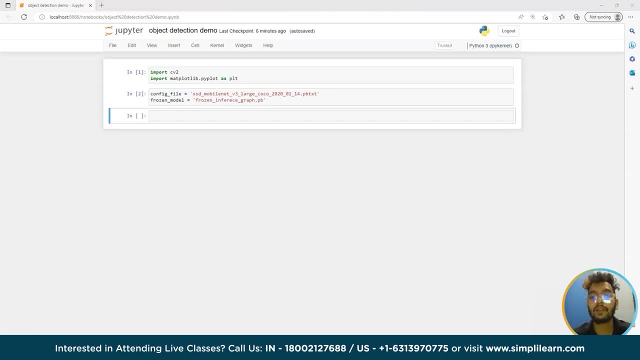 annotation pipeline. on the top of that, the coco data set is a supplement to transfer learning, where the data used for one model serves as a starting point for the another. so what is frozen insurance graph like? freezing is the process to identify and save all the required graphs, like weights and many others, in a 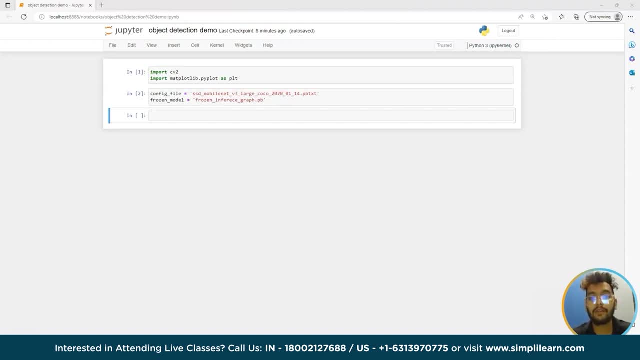 single file that you can usually use. a typical transfer flow model contains four files and this contains a complete graph. okay, so forward, let's create one model here. I will write model first to cv2.dnm model- who's done? and then config file. hey, I am giving the parameters two. 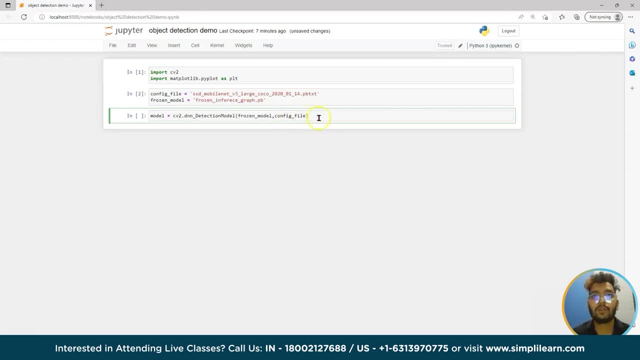 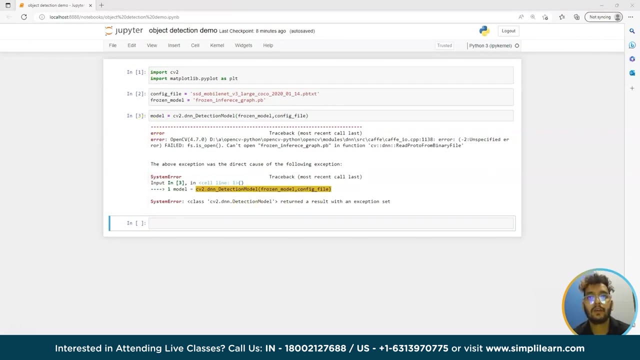 parameters like for the model and config file go here. yeah, we run it first. okay, this okay. so I've had a CV to dot DNM detection model. return on the data set is an exception set. the question comes: what is the meaning of detection model or DNN detection model? oh, this class represent a high level API for object. 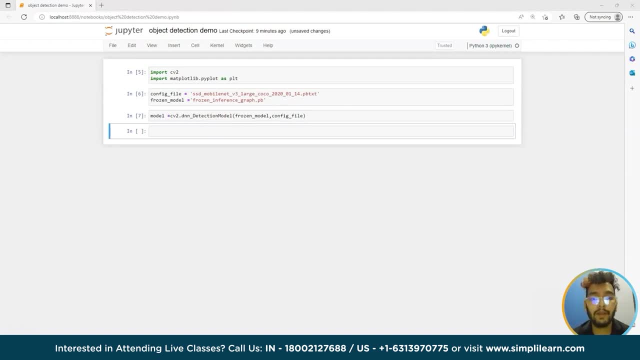 detection networks. detection models allows to set parameters for pre processing input. image detection model creates net from file and with trained weights and config sets it. processing input runs forward, pass and return the result: detection. okay, moving forward, let's set the class labels. okay, class labels. I name. 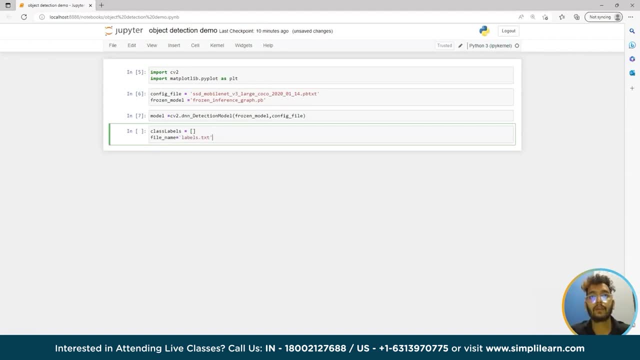 so labels dot txt. I will put this file on the description box below. you can download from there. open file name you as labels. this trip. and so here I created one array of name, class labels. so this is the file name. what I'm doing, I am putting this label file into this class label. okay, so here, if I will, 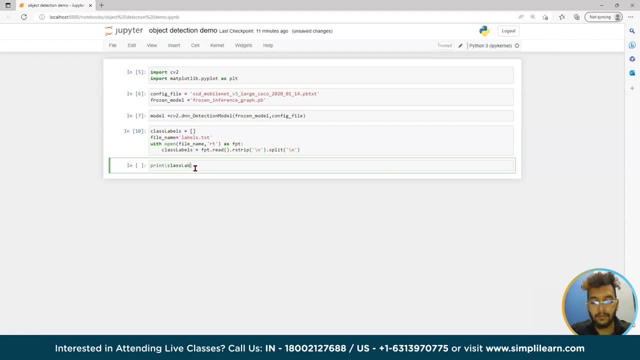 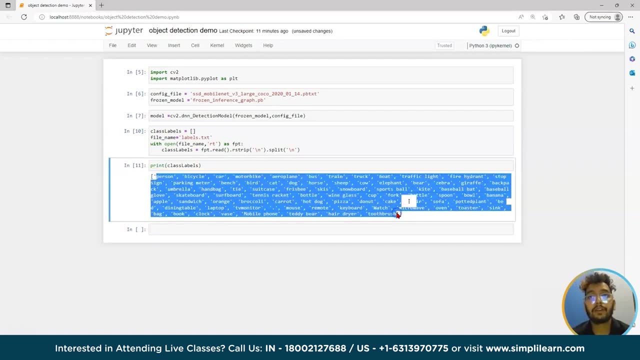 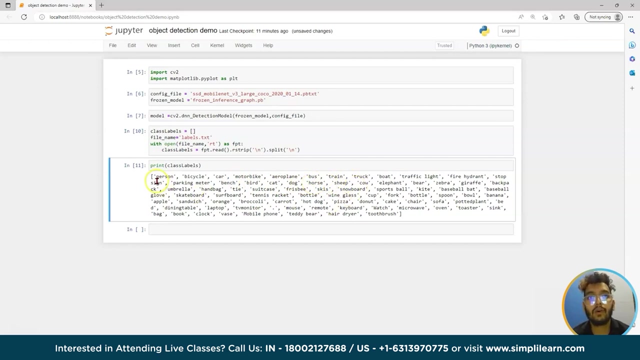 print class labels are the 80 categories in the cocoa data set. okay, this person, bicycle, car, motor bike, airplane, bus, train. these all are the 80 categories. I will put this file label dot T X in the description box below. you can find download from there. I. 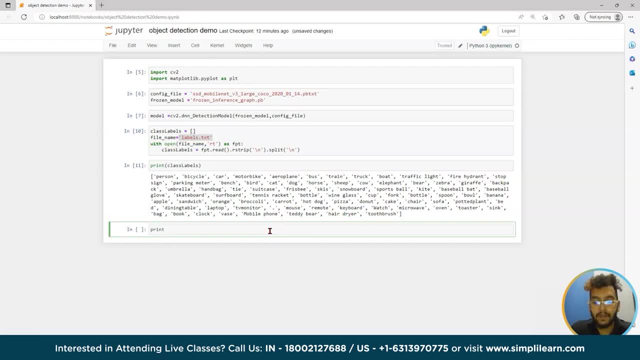 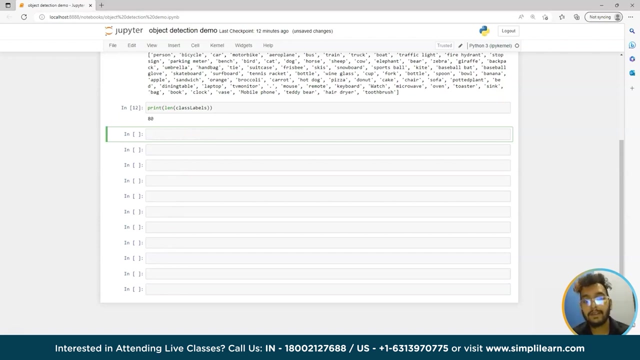 okay, fine, let's print the length of the Cocoa data set, or you can see class labels- is 80, as you can see. I have already told you the length will be 80, so here let's set this. some model input size is scaling, mean and all I will write here. 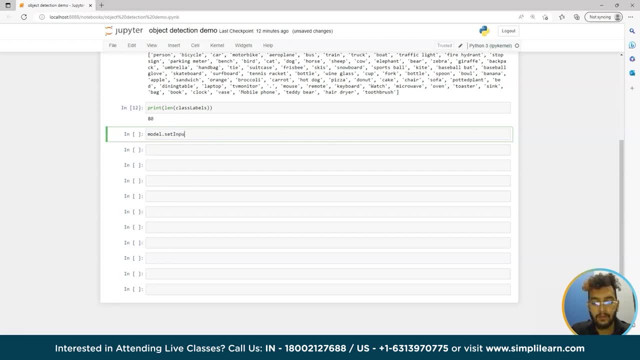 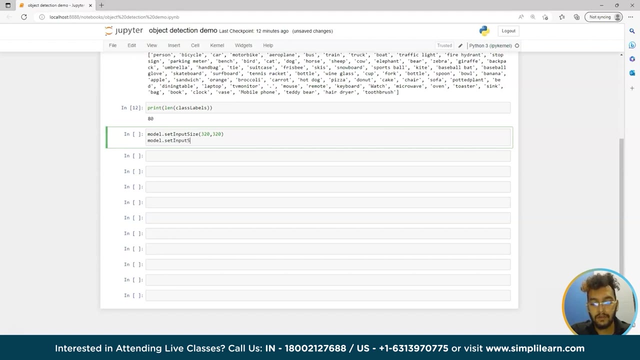 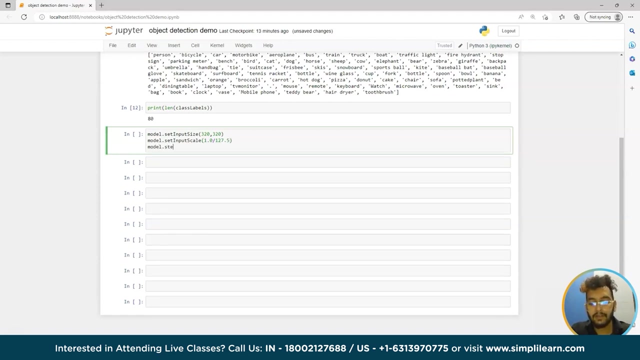 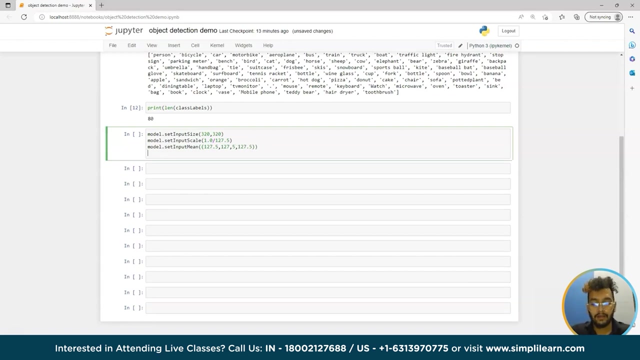 model dot set is t20. well, dot set input scale: 1.0- 1.0- 27.5. okay, I will explain, you don't worry. model dot set: input me 127.5 comma, 127.5, 127.5, okay, and then model. 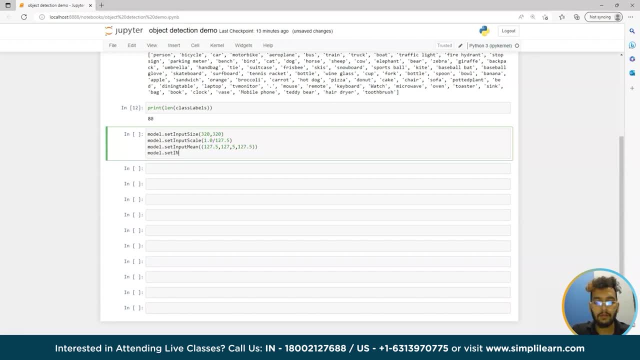 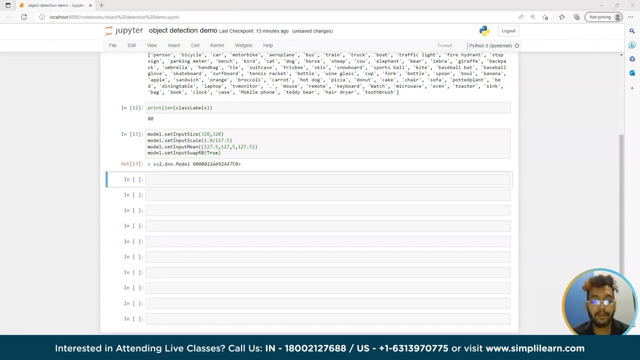 dot set will be what is set input size. okay, so set input size is a size of new frame. data shape of the new blob: less than 0. okay, so this is the size of the new frame. second one is set input scale. the set input scale is a scale factor of the value for the frame, or you can say the: 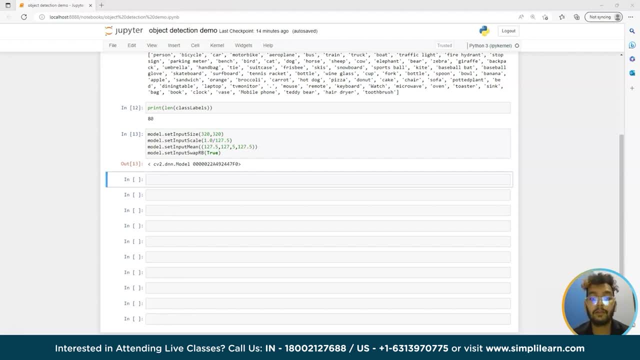 perimeter will be the multiplier of the frame values, or you can say multiplier for the frame values. so input mean. so it set the mean value for the frame, the frame in which the photo will come, the video will come or my webcam will come. so it set the mean value for the frame or the for parameters. mean is killer. 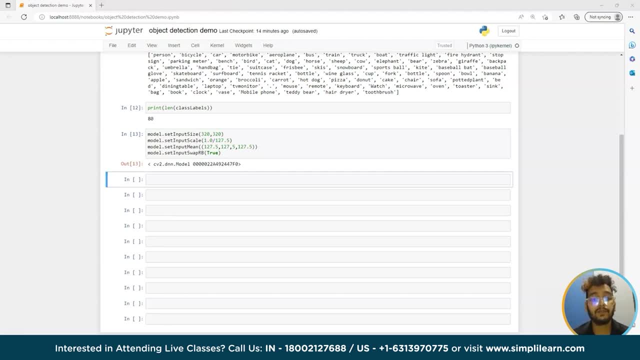 with the mean values which are subtracted from the channels. you can say: and the last one is set input. swap RB, so it set the flag. swap RB for the every frame. we don't have to put every time a single frame for a particular image. it will be set the true for the all the images. okay, so parameters will be swap. 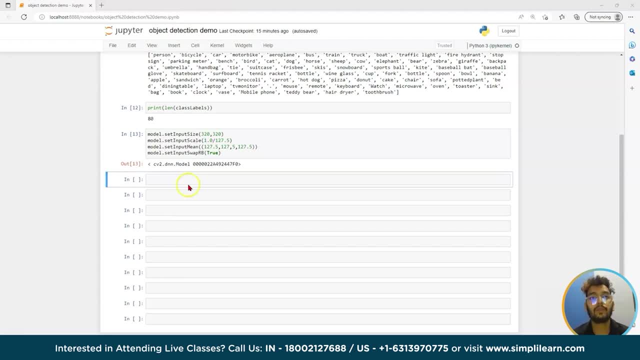 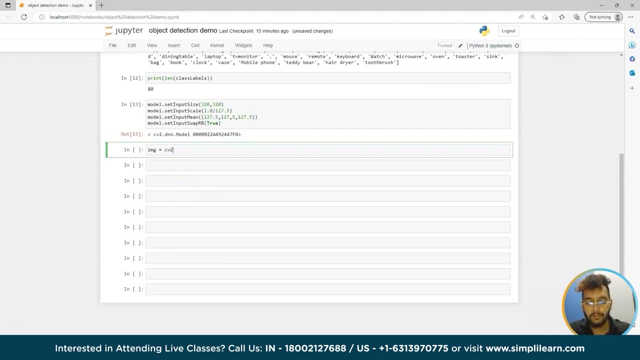 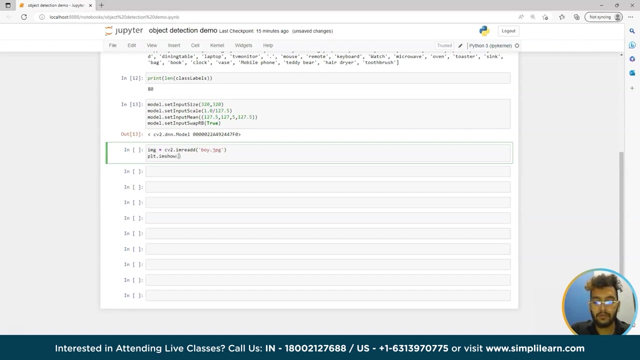 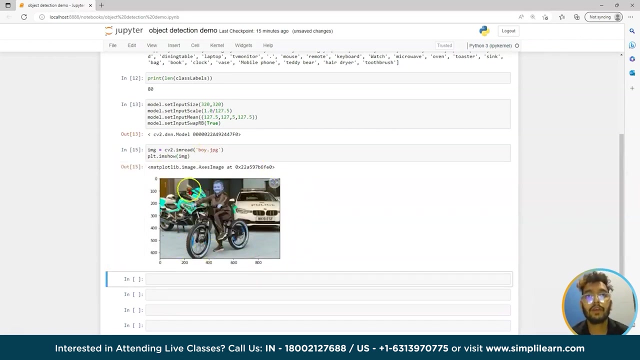 RB flag, which indicates a swap, first and the last channels. so, moving forward, we will put one image. you, I am read, boy, don't give it, D, don't, I am sure. so this is the size of 320 by 320. okay, so first thing is you can download this. 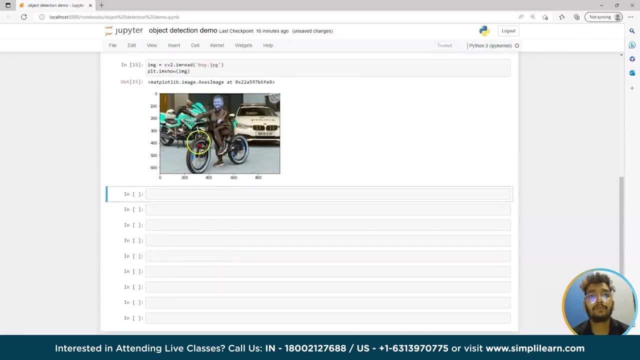 the random image of from the Google I took from Google itself. so now what we will do. we will set the class index, the confidence value, in B box. B box is the boundary box which I will create for that particular person: cycle, motorbike and the car. okay, because to model of. 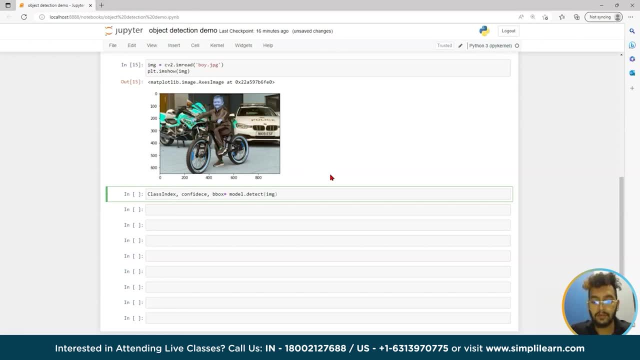 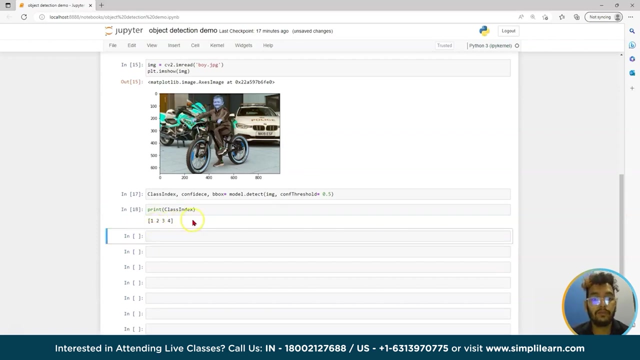 that the confidence threshold is useful. if my model II will confirm its, the particular image, which is the taxing, is correct, it will bring the name. okay, you, you, let me print and class: class index is coming: 1,, 2,, 3,, 4.. 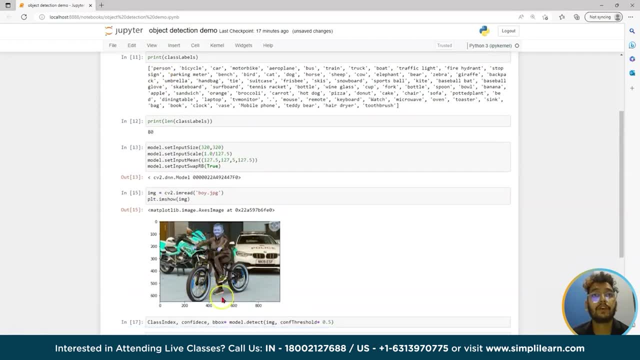 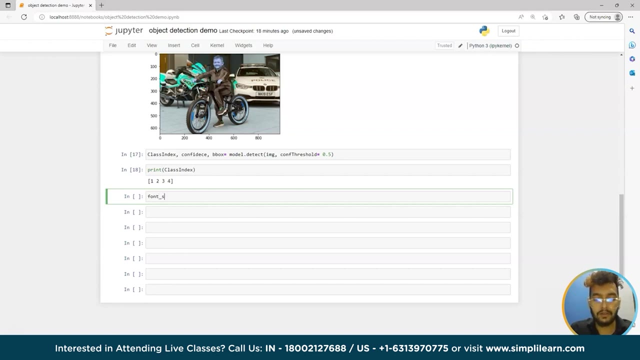 Okay, So 1 means person, 2 means bicycle, 3 means car and 4 means motorbike. This is the class index: Index for particular label. What I will do, I will print the boxes. font scale equals to 3 and the font equals to. 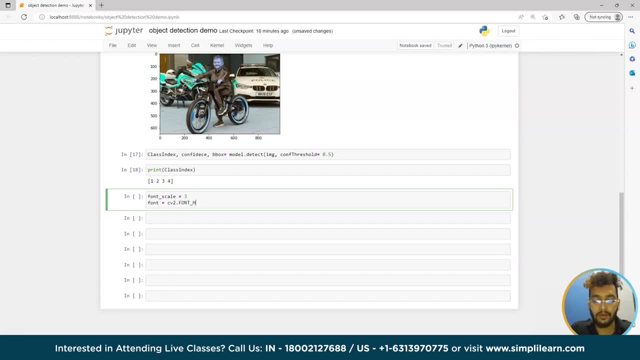 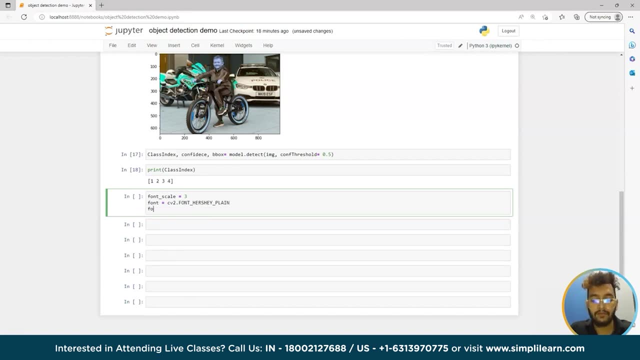 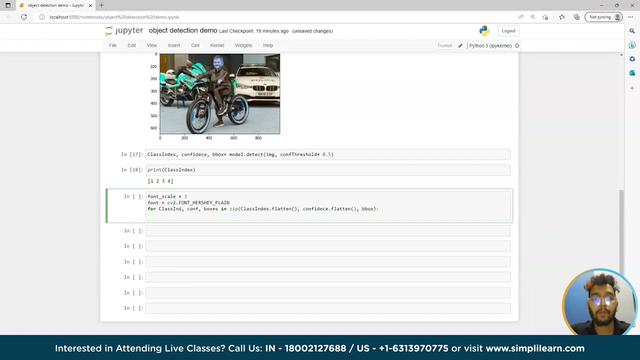 cv2.font- hershey plain font- class index and the confidence and the boxes and next dot pattern: confidence pattern box, the boundary box. okay, And I will write here: cv2.font- cv2.rectangle- make the rectangle set the image and the box is 5, 0, 0. 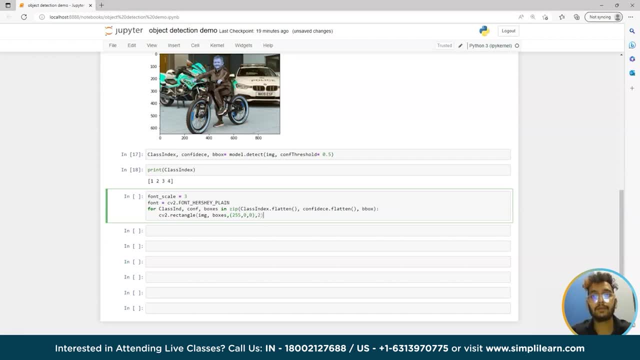 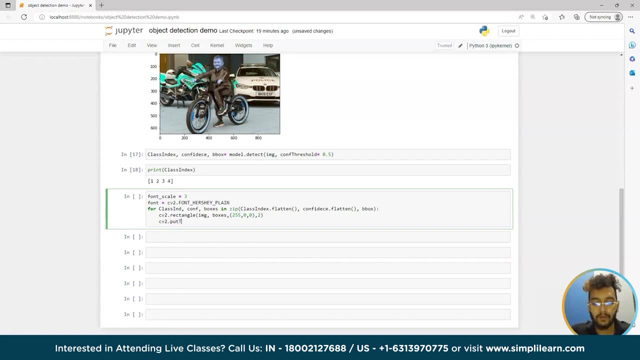 is the color of the box and this will be the thickness. Okay, Then I will write cv2.put text, cv2.put image and cv2.put image. then class labels have a light glass index, because always index starts with zero. That's fine. 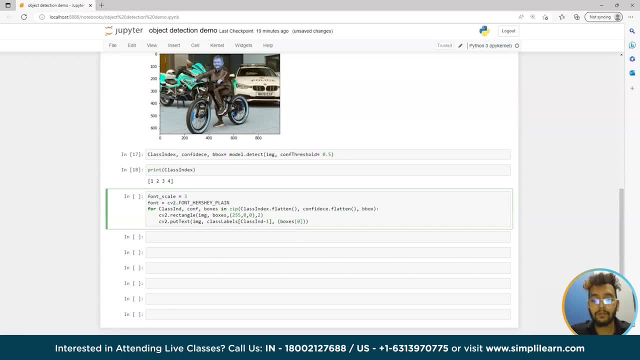 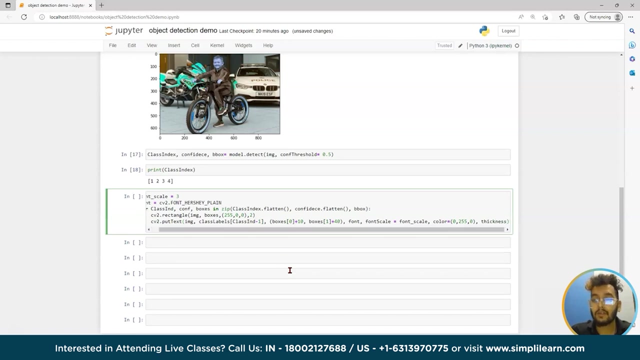 And the boxes are in this black box and comma color. this will be the text color: 0,255, 0 and the thickness 3. let me run it no error. ok, now plt, dot, I am sure. then cv2 dot, cvt color, then cvt. 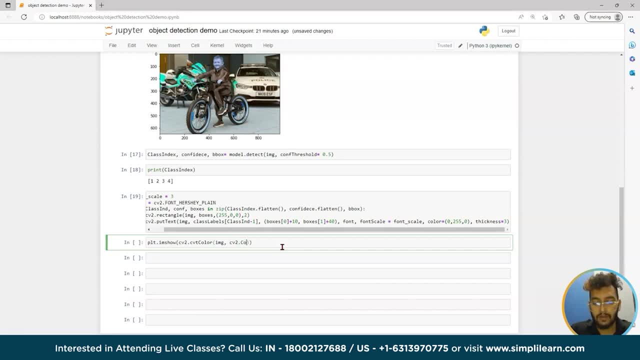 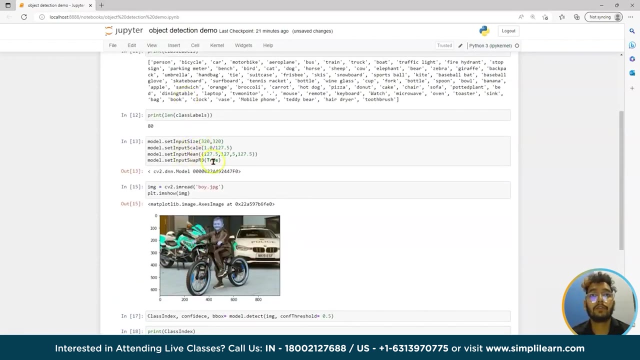 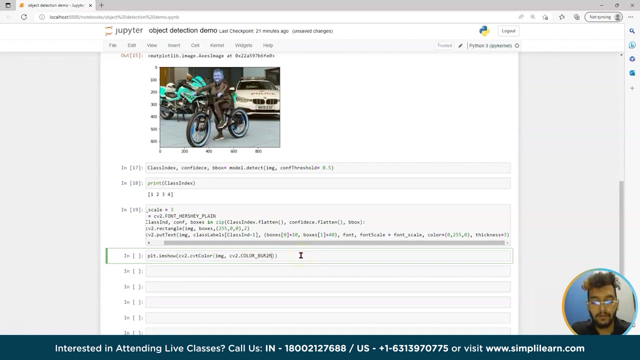 2 dot color color, then bgr to brg. that is why we wrote swap rb equals to true, because every time we will convert bgr to brg- sorry rgb, so we don't have to write again and again. it will convert all the files into. 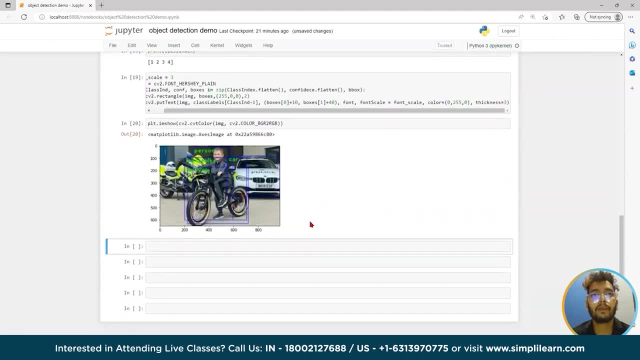 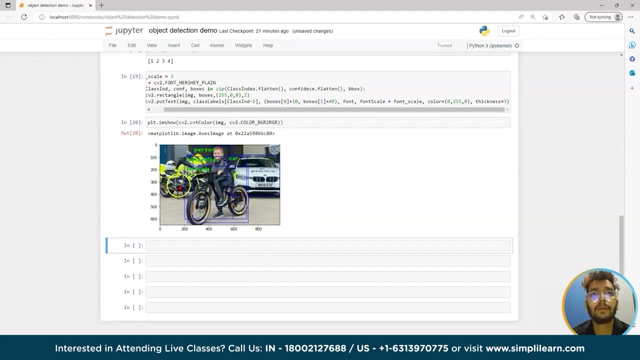 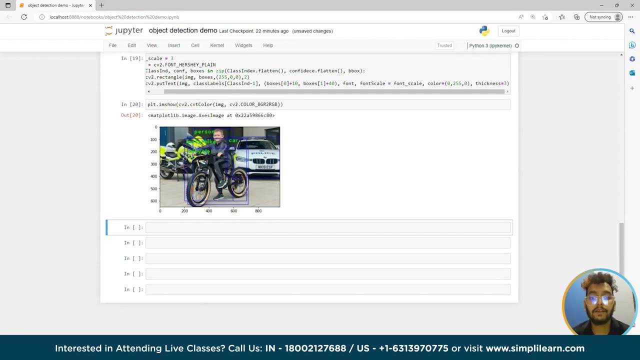 rgb. ok, run it. ok, as you can see, the motorbike is coming, bicycle is coming, the person is coming, the car will come. ok, so it is detecting the ride for the image. now. we will do this for the video and for the webcam. we are done with this image one. 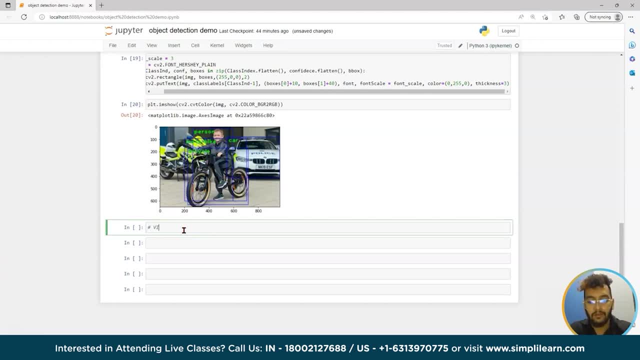 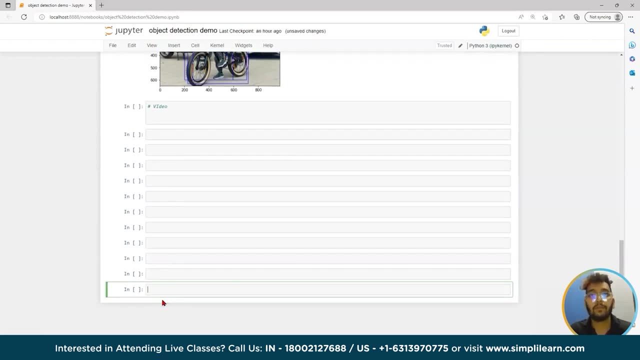 and then I will write here: ok, so this is we will do for the video. for the video I will write here: cap equals to capture. you can write any name, so cv2 dot video capture, so you can take any random video. I took this pexels, george. 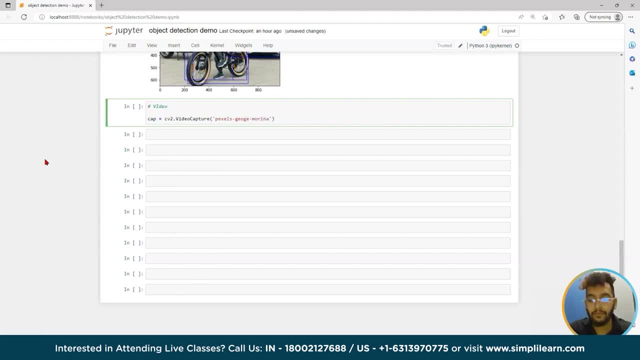 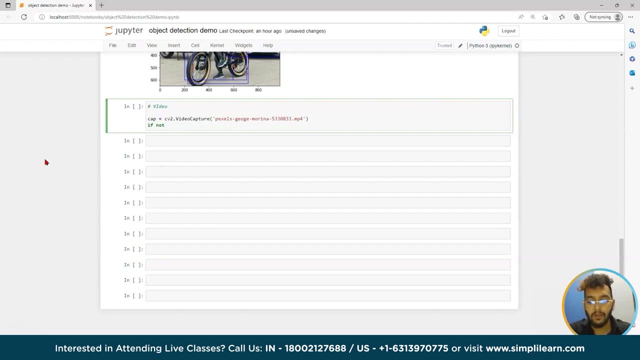 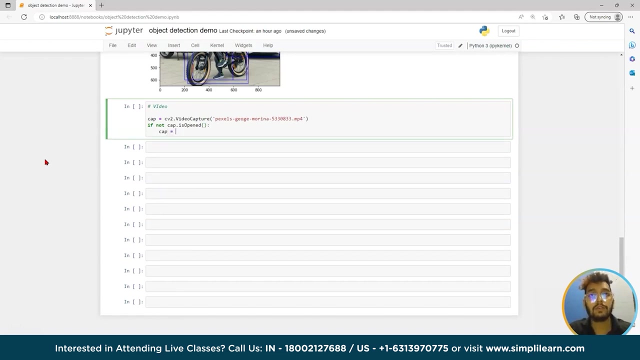 you can comment down, share the link for so for a file. ok, we will change the name of the clip. so if we want to know, do you can change any name for the clip? so I will write here. app dot is open, so here I will write: cap. 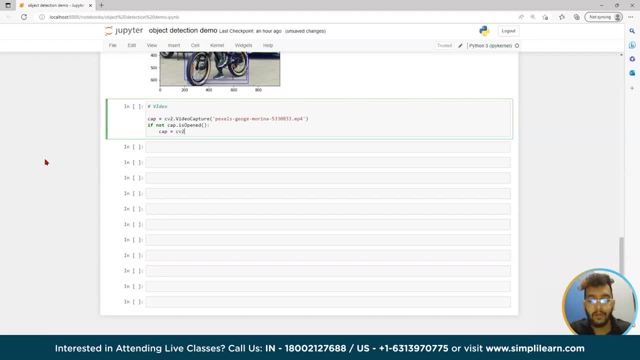 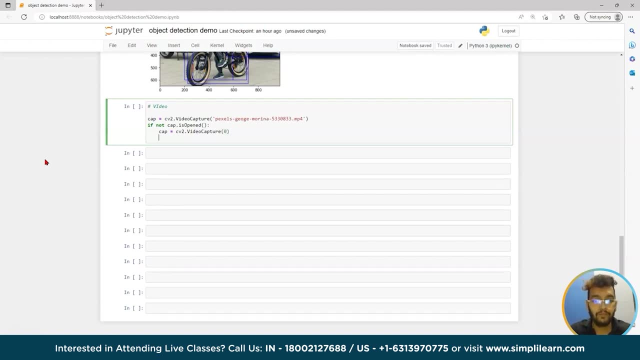 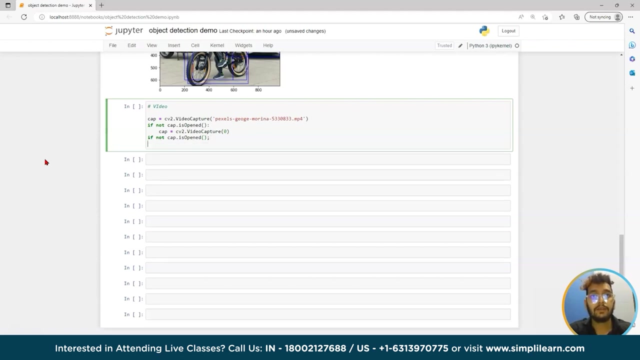 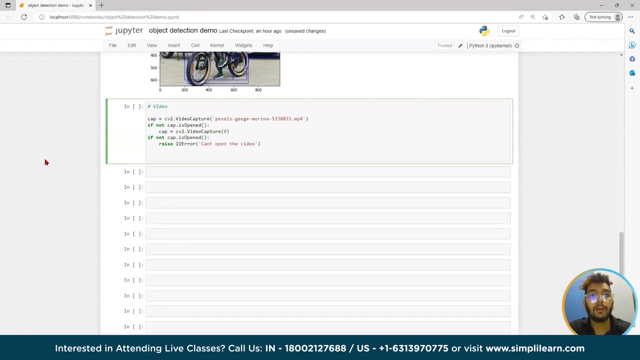 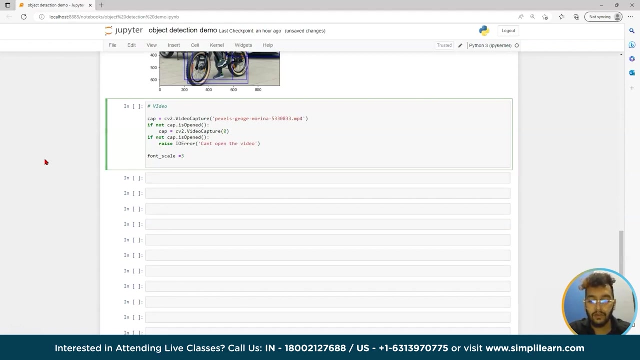 equals to cv2. sorry, cv2 dot capture view. and if not, cap dot is open, then and raise output error: can't open the video. can't open the video here. everything will be the same. font scale equals to 3. ok, font equals to cv2 dot. 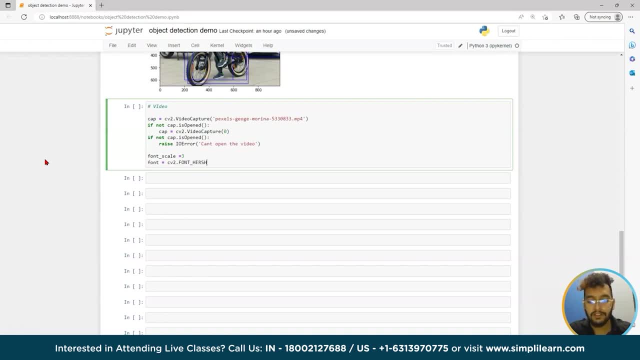 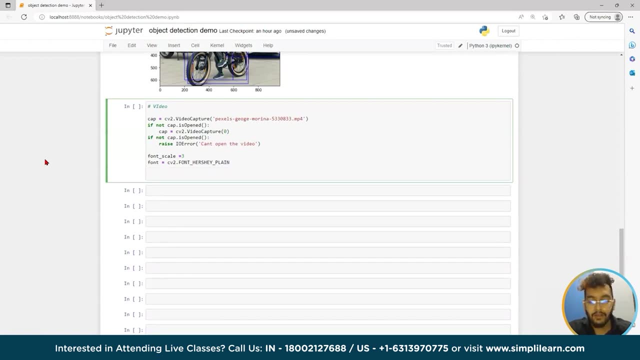 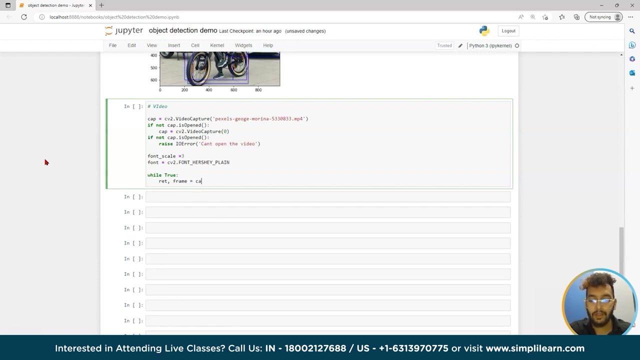 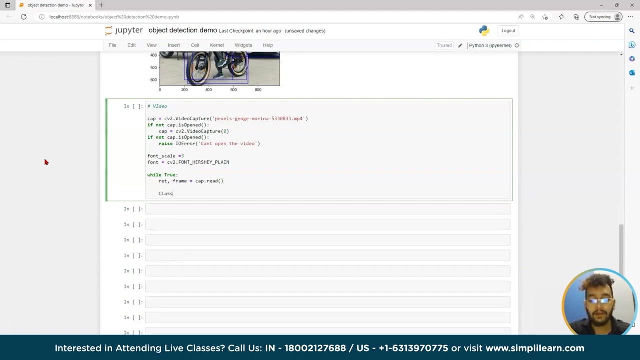 font harshe in. ok, so here I will write: while true form of frame equals to, equals to cap dot sheet. this is for the reading of the file, the same I will write: class, index comma. confidence comma. boundary box equals to model dot detect frame and the confidence. 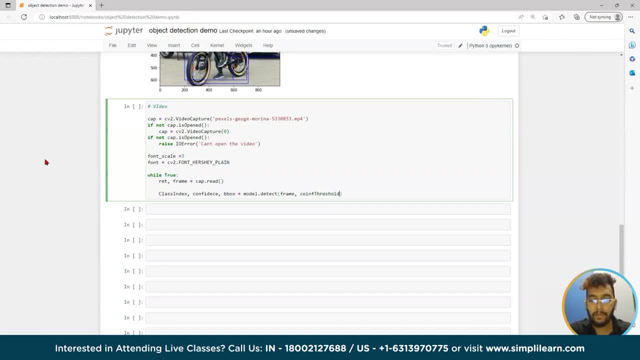 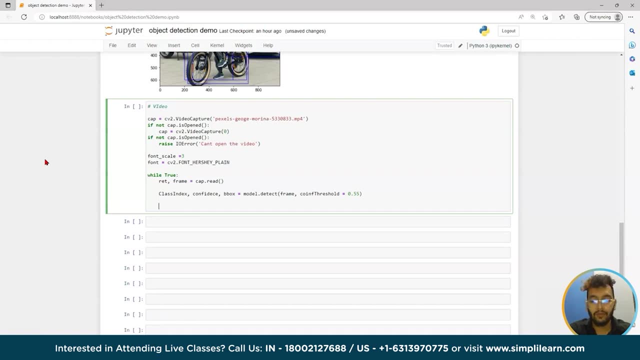 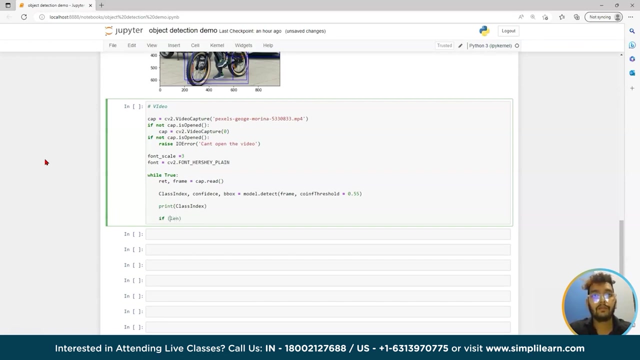 threshold equals to 0.55. ok, everything is the same we did before, so here I will print class index. ok, so here I will write if and the class index and does not equals to 0. and what to perform is here I have to write for. 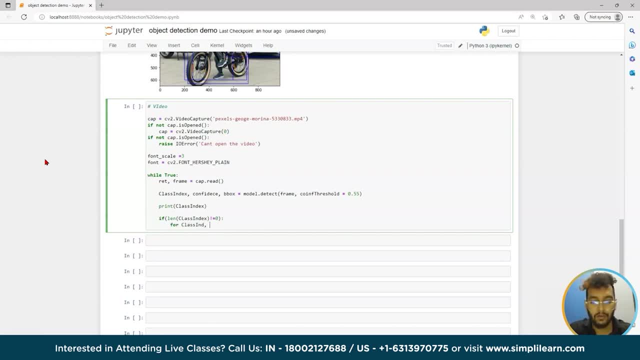 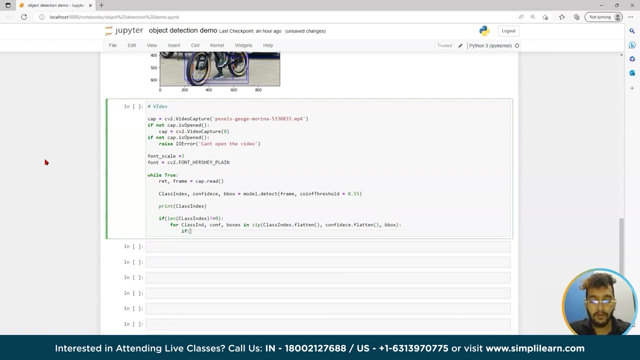 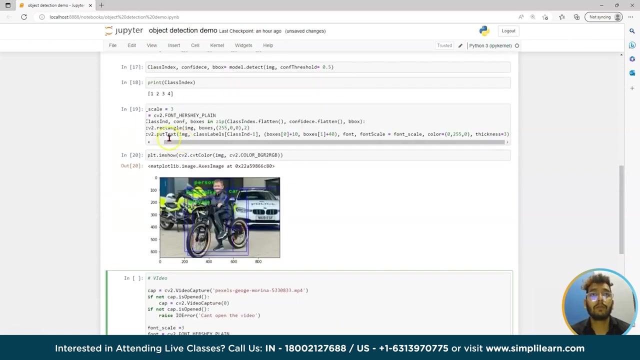 class index comma, confidence comma. boxes in zip class index dot flatten. flatten is a layers ok, confidence, confidence flatten. and if class class index is greater than equals to 80? and if class index is greater than equals to 80, and what to do then I will copy from here: 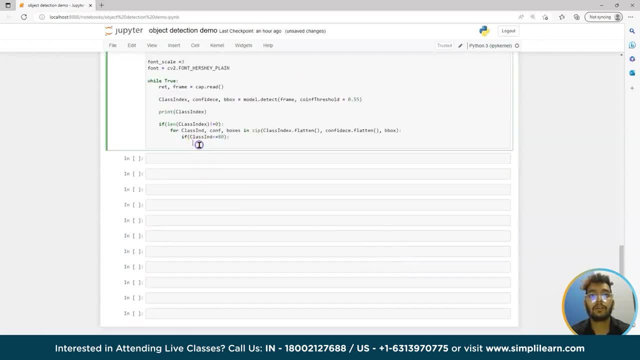 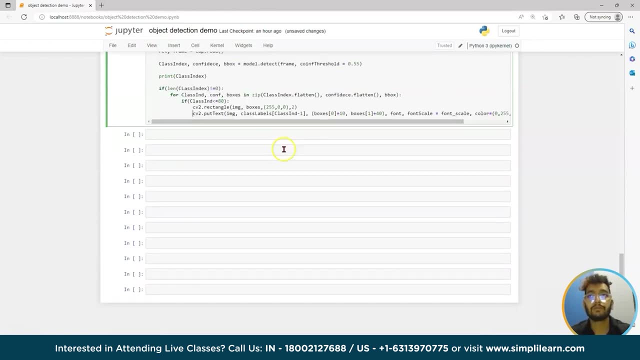 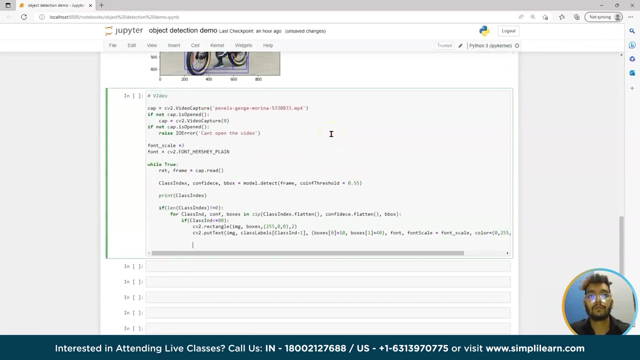 okay, the same thing I have to write here, you here. I will write cv2 dot. I am sure this will be the return in the frame: object detection by simply learn and frame. or if cv2 dot- red key, cv2 dot, red key and 0 ffx. 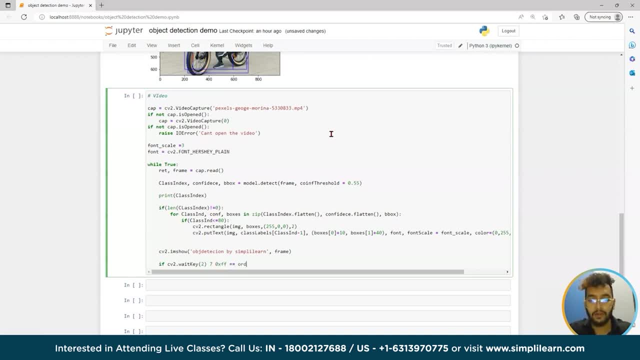 equals to ordq. okay, then here I will write: break. will you break when get into 2? the wait key will be 2. okay, I will write. I will tell you what is the wait key. here I will write: cap dot release and cv2 dot destroy. 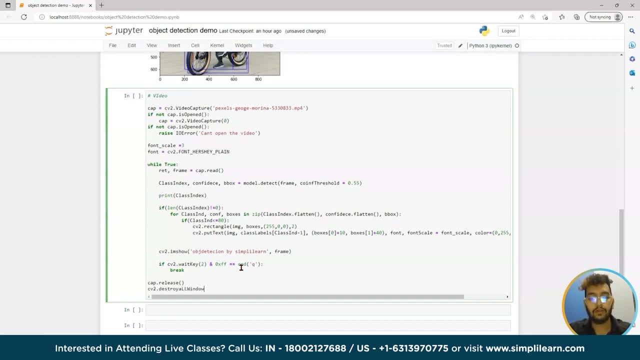 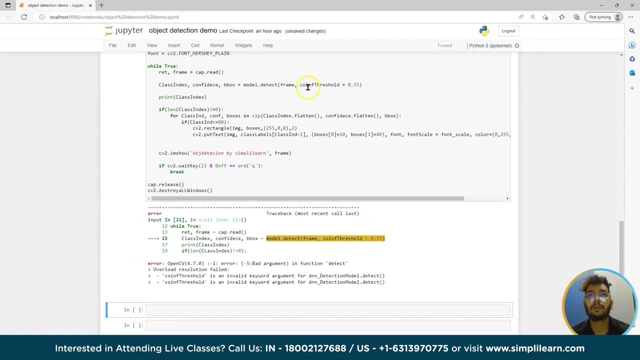 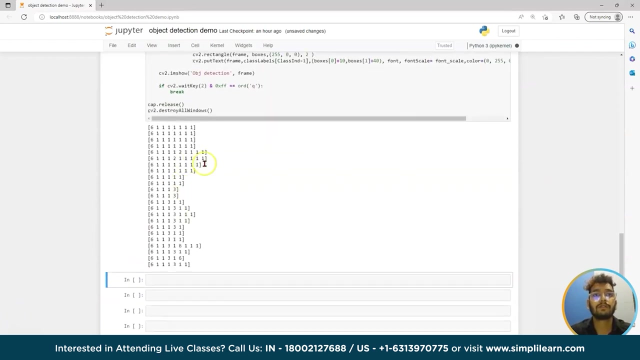 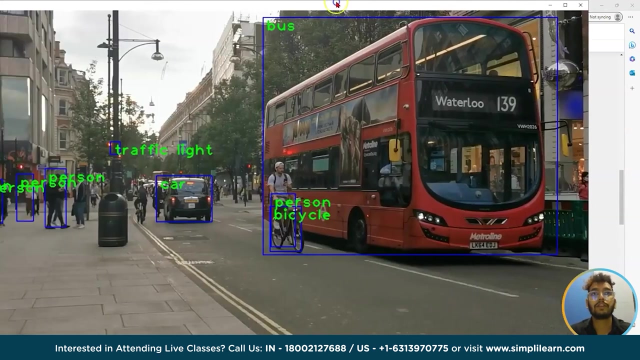 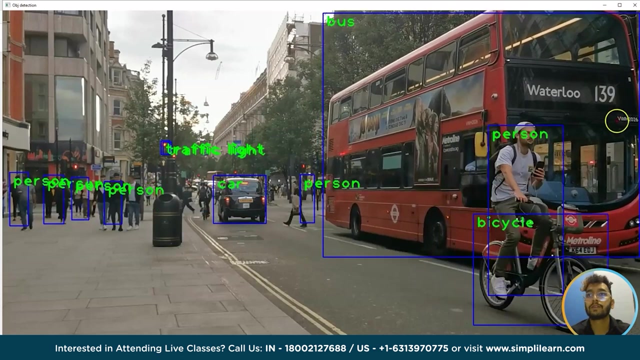 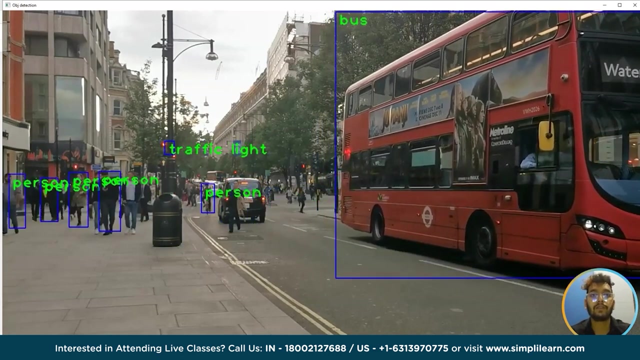 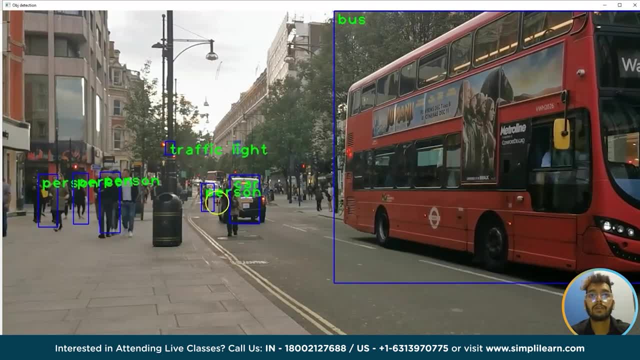 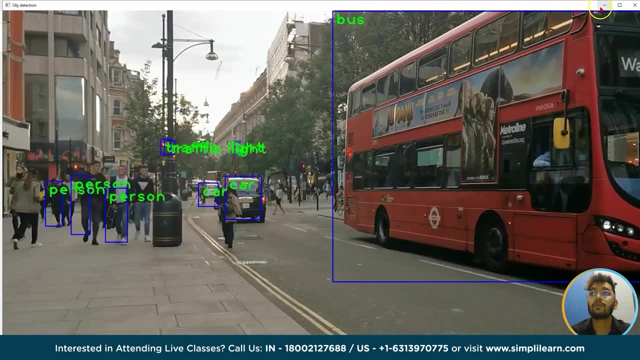 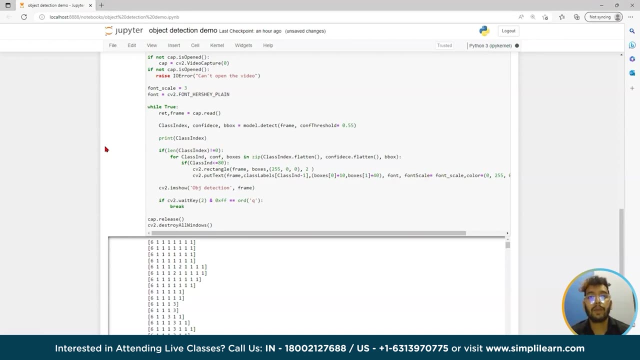 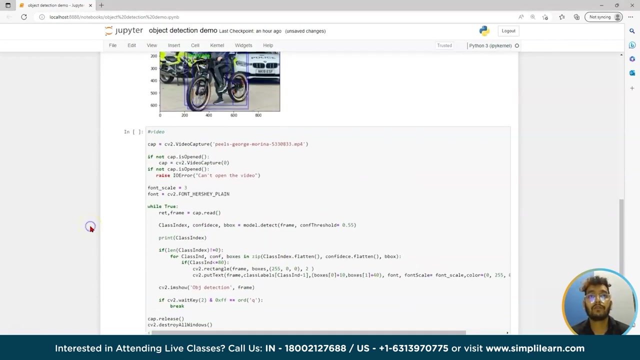 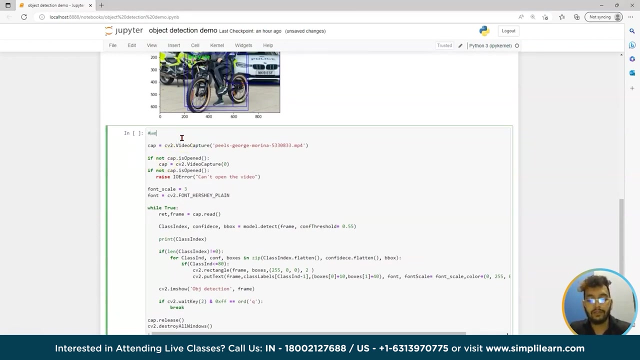 for the video is coming right, okay, person, okay, person, traffic, light, bus. this is how you can do for the video, okay, so now, let's, we will do for the webcam live. so this is for the video. so if we want to do for the webcam, okay, so we need to just change. 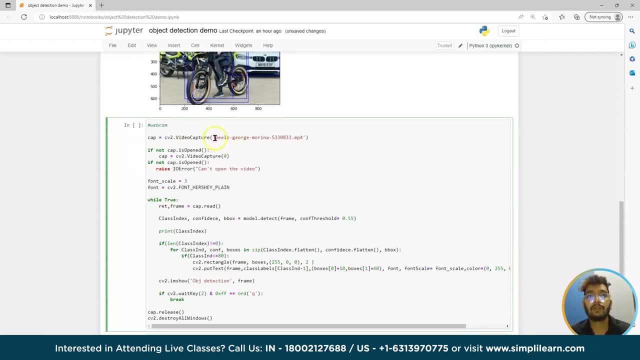 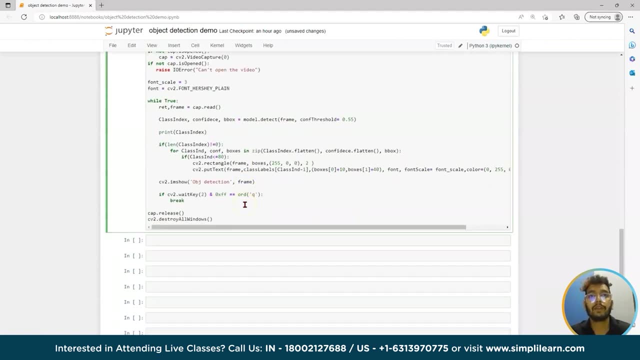 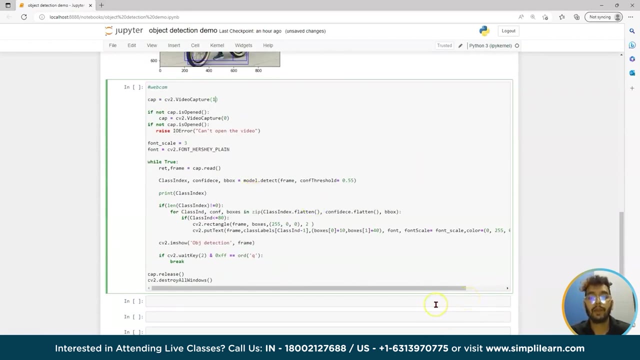 one, one thing only we have to change. instead of giving the file, we have to write one here. okay, the rest will be the same. got it. so I have to just shut down my webcam. so let me shut down the webcam and get back to you. 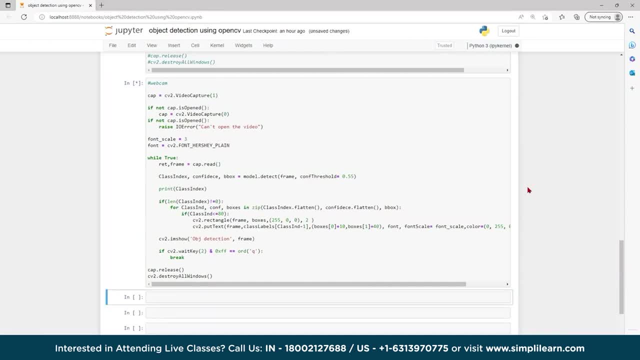 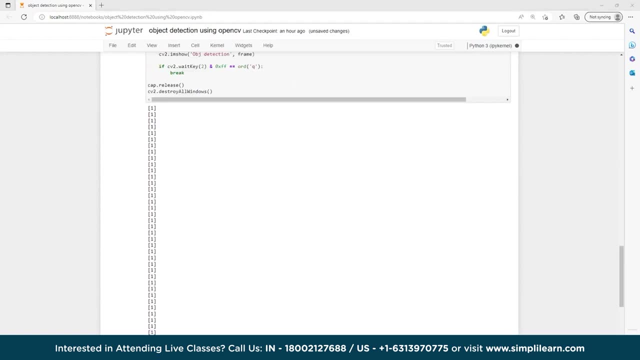 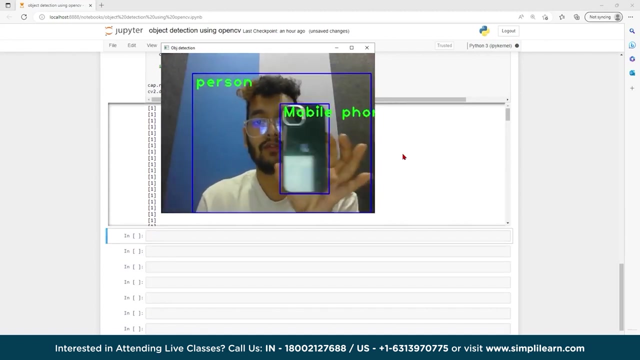 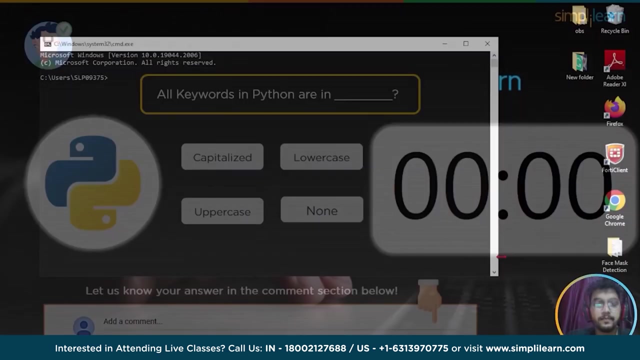 so, as you can see, this is a 320 by 320 box, so this is coming right, okay. so if I will show this, the mobile phone is coming right now, okay, so this is how you can do the correct object detection, okay, so first we will. 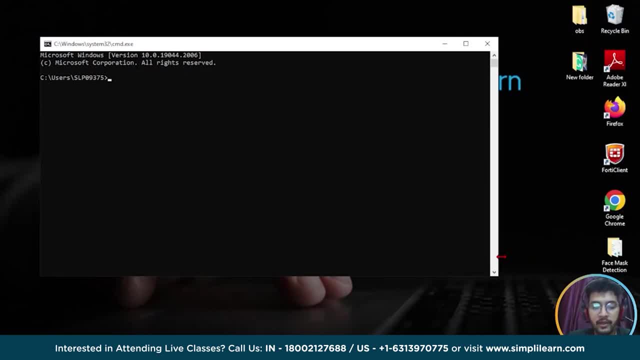 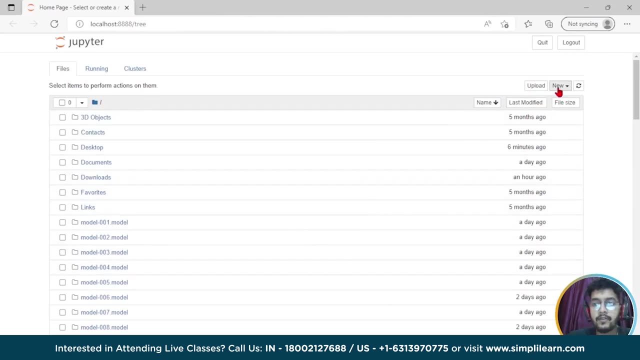 open command prompt to write a command to open Jupyter notebook. so here we will write Jupyter notebook, then press enter. so it will take some time. yeah, so this is the landing page of Jupyter notebook and here we have to new. then python 3, so this is how the Jupyter 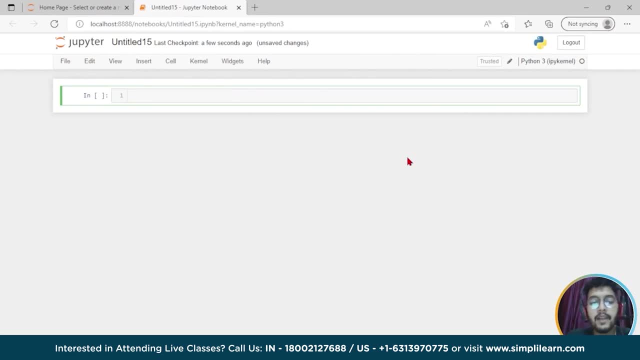 notebook looks like. so at first we will import some major libraries of python which help in creating a mass detection system. so here I will write: import cv2, comma, os and press enter. then I will give the path. then data path equals to c. 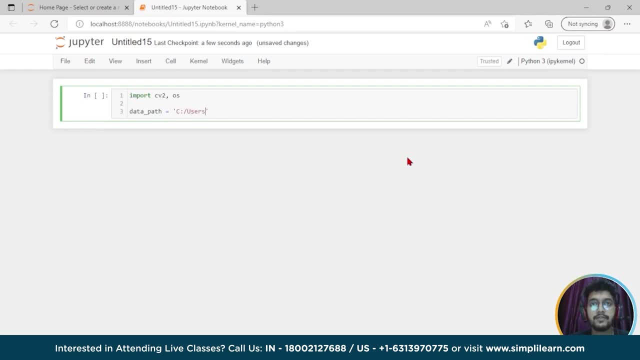 then slash users, then slash SLP 09375 and slash desktop and slash and face mask. get action and slash dataset. okay, it will be slash- my bad sorry. and slash- okay, it's look fine. so here I will write categories equals to OS dot list, directory list, dir, then I will assign data underscore path. 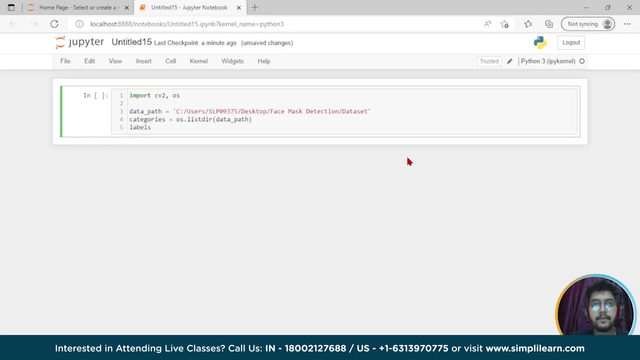 then I will create some labels equals to here I will write: I will write here I for I in range. then here I will give labels equals to I for that name and I in range is pass, and then I will account length of categories. yeah, then press enter. then here i will write label. 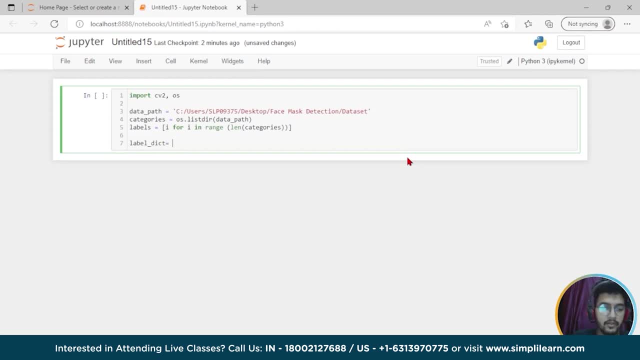 then ticked directory, pursue directory, then zip, then categories, labels. so here i will write print, then label directory. okay, then i will print categories, then i will print labels. okay, then press enter. yeah, so here cv means capturing video. the cv2 function in opencv can read video. 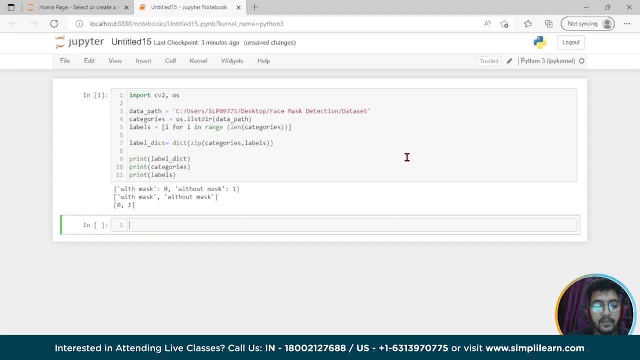 video capture. by using pass zero as a function parameter we can access of our webcam. we may pass rtsp URL in the function parameter to capture cctv footage, which is quite helpful for video analysis. then os, The OS module in Python, has function for adding and deleting folders, retrieving their contents. 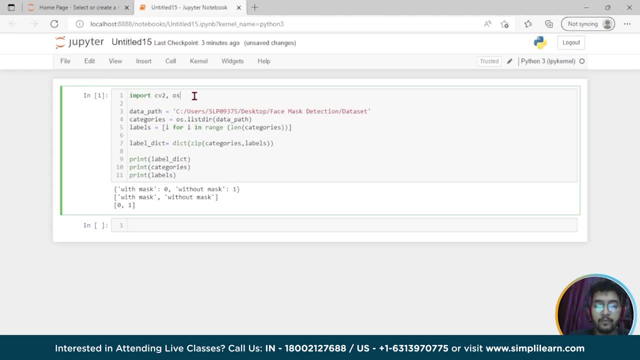 changing the directory, locating the current directory and more. Before you can communicate with the underlying operating system, you must import the OS module and this oslist directory. to retrieve a list of all files and folders in the given directory, Use python oslist directory method. 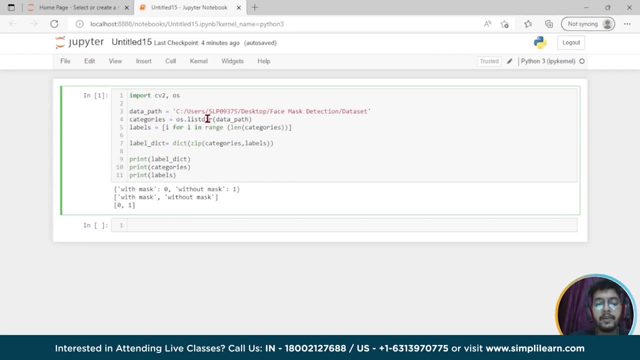 The list of files or directory in the current working directory will be returned. if no directory is specified, Then Label. The TkInterWidget class, called a label, is used to show text or an image. The user views the label. they can not be interact with it. 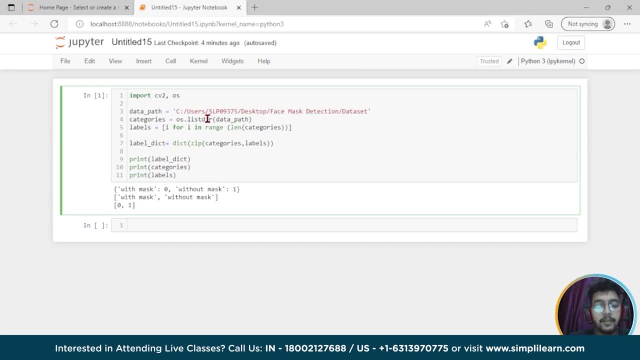 So, moving forward, I will write code, so just stay with me. after that I will explain you line wise. So here I will write That image: underscore size equals to 100.. Then I will create two classes: data, Then target: Okay, erase. 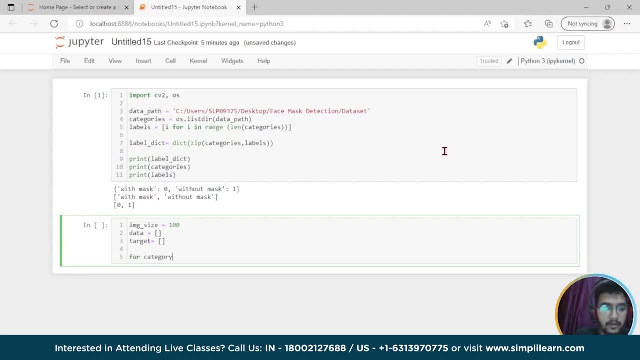 Then I will write here for category in categories: folder sigue path, Then folder underscore spot. And now I am setting historia to folder underscore path: folder underscore path equal to os trial path, Then join, Then data underscore мел of call a array. 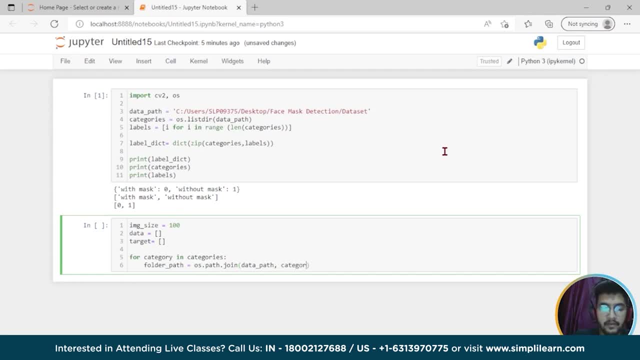 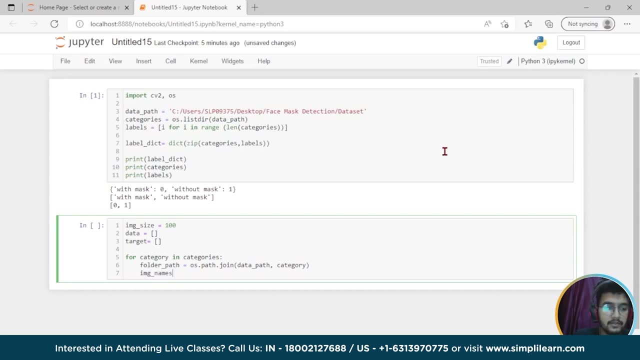 Charc category. okay, then img image names equals to os dot list directory, then folder path. just stay with me. i will explain you linewise. okay, so here i will write for img name in img names: img underscore path equals to os dot path. dot join img. 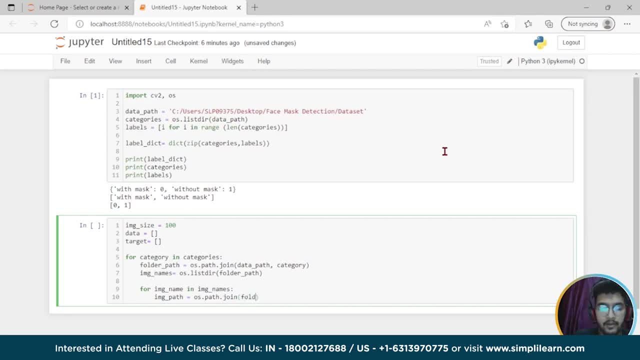 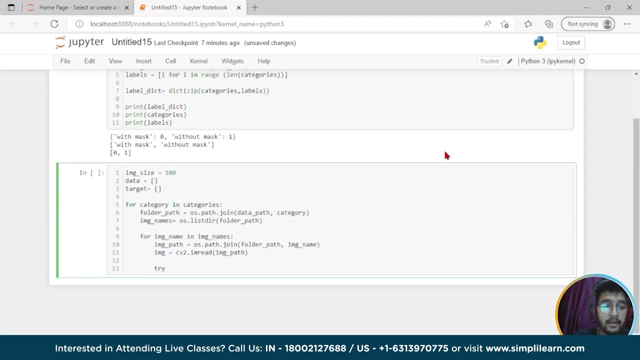 then i will write here folder, i repeat, i repeat. so here we write folder underscore path, then img underscore name. so img equals to cv2 dot imread, then img underscore path. so here i will write: try that gray equals to cv2 dot cvt, then capital c color. 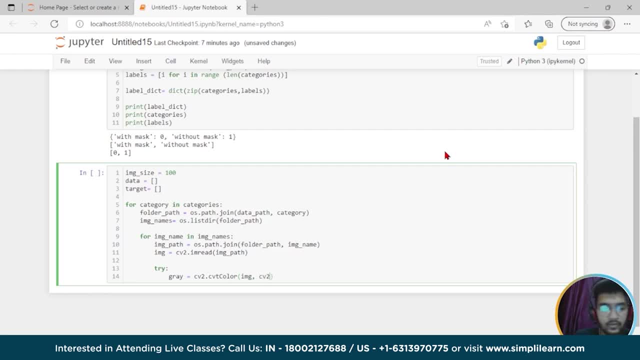 then img comma cv2, dot cvt. then img comma cv2, dot cvt. then color, then underscore b, g, r to RGB. okay, so i will go for the gray one cvt color: bgr to rgb, yeah, right, right. so now im going to go to the color whom i need to Hearing- Dark blue to be playing. 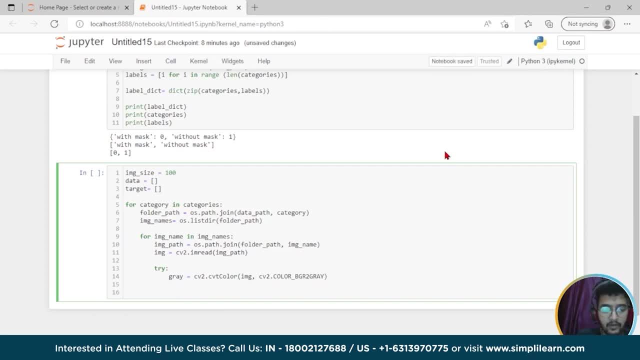 so i will write here resize. okay, not in capital letter. resize equals to cv2 dot resize than gray comma img size. comma, img size. why this two img size? because like length and like width and breadth would be shame like 100. so press enter, so i will write data dot. append, then resized. 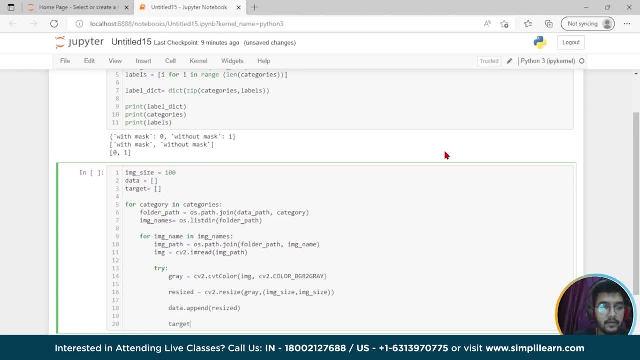 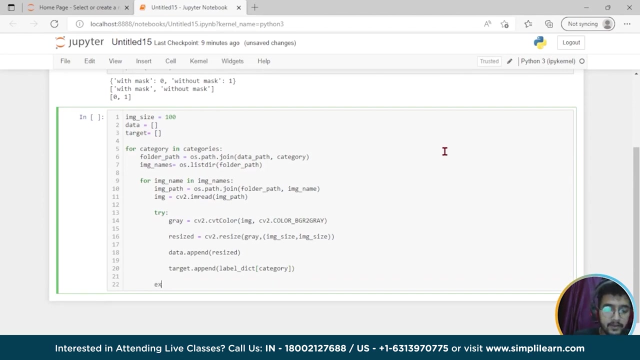 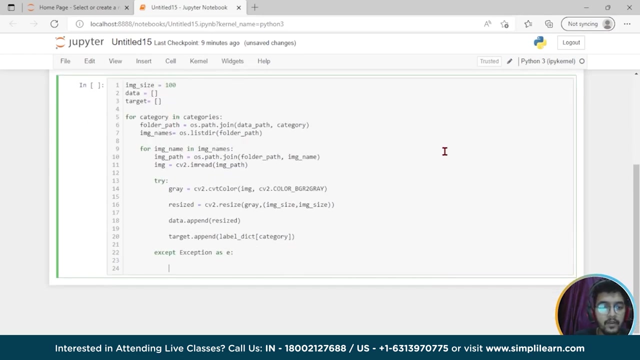 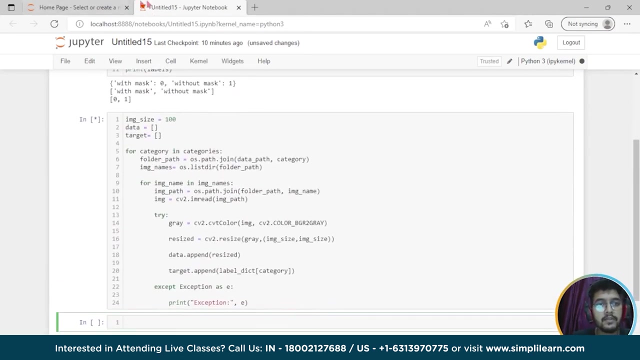 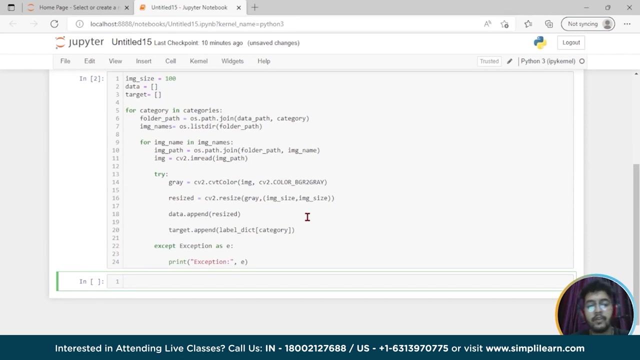 then target dot, append, then label, then directory of category. okay, so i will write here: accept exception as e. so here i will print then exception, comma, e okay, then press enter. let's see, there should be no error. so it is loading. let's wait, no error. okay, no error. so image size should be like 100 by 100. so that is why i wrote here 100. 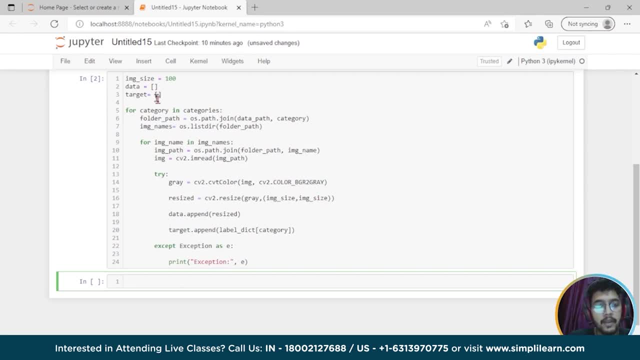 then image size: 100 by 100, and i made two arrays like for one for data, then one for target. so this for this gray cost to cbt, dot, cvt color image. so converting the image into grayscale. okay, then this line resize equals to gray scale. okay then to gray scale. okay, then this line resize equals. 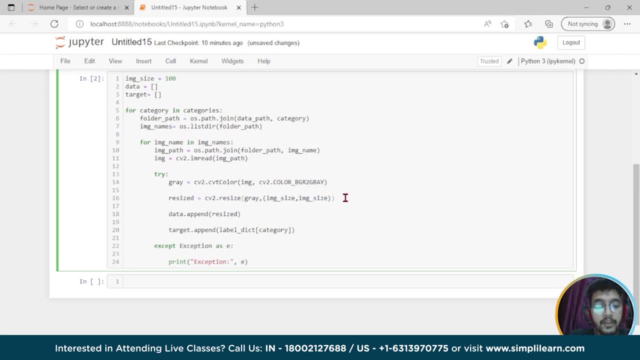 to cvt dot resize gray img, so resizing the gray scale into like 100 by 100, since we need a fixed common size for all the images in the data set. okay, then this target dot append label directly, so appending the image like and the label categories into the list list. what is list data? 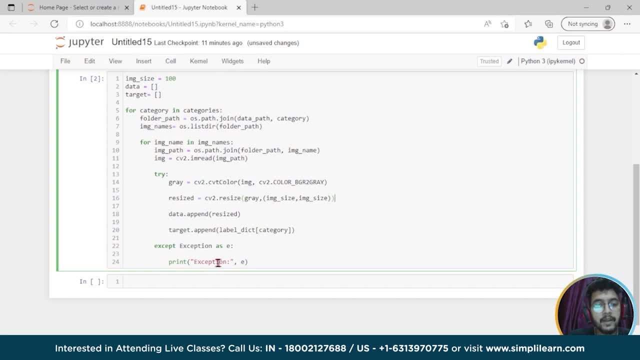 set. so, like for the last print exception e. so if any exception raised, the exception will be printed here and the pass to the next image. okay, so moving forward, let's import numpy and save this data and the target. okay, so i will write here import numpy as np. 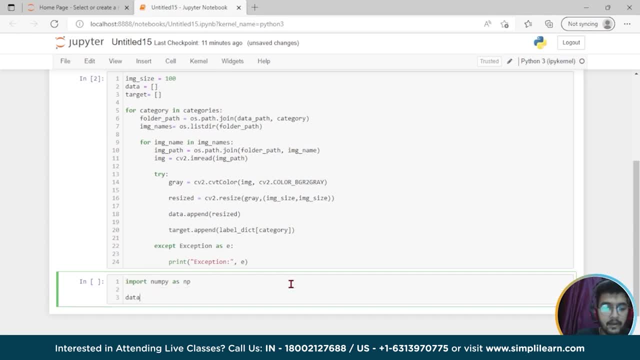 right, then i will write here: data equals to np dot array, then again data by 255.0. okay, then again data equals to np dot reshape, then data comma, data dot shape, then zero comma, img size comma. img size comma one. okay, then press enter. then for target: 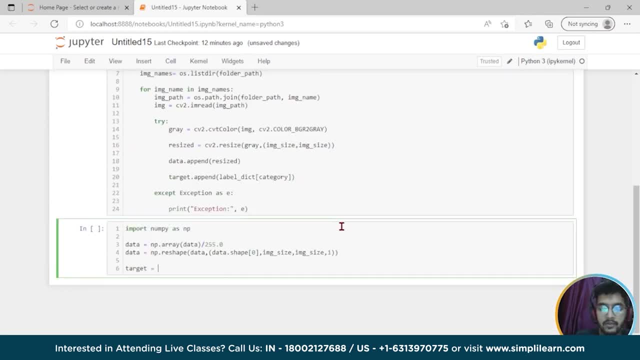 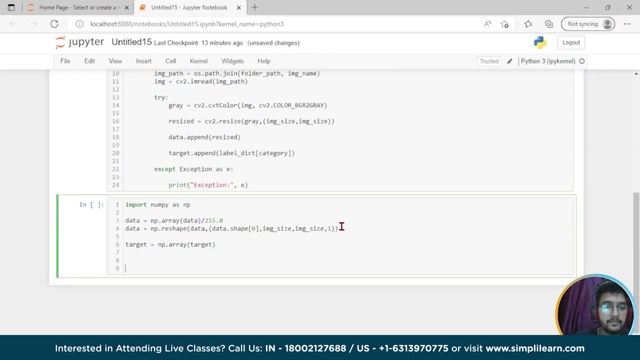 let me put those just like this: then target equals to np dot array, then target: okay, okay, so here i will write from keras: dot utils, import and p utils. okay, so here i will add new underscore: target equals to np underscore, utils, dot. two underscore categories: categorical, i guess. categorical, then target. 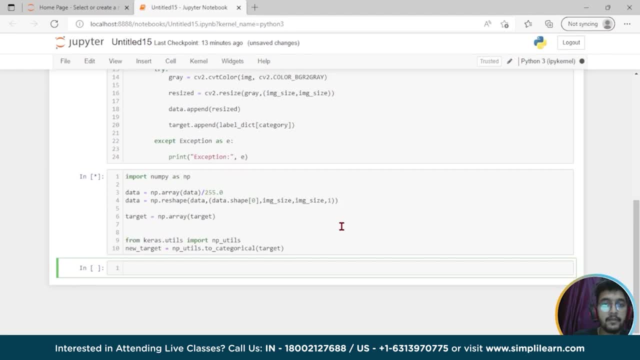 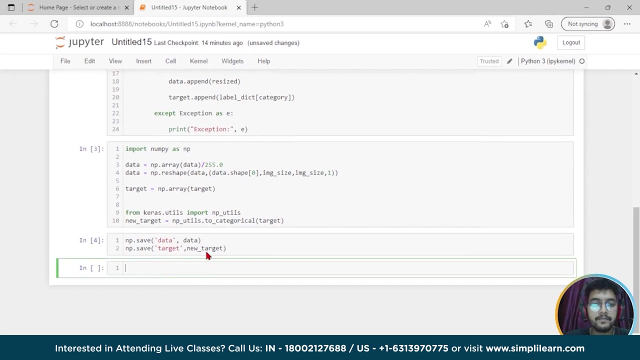 okay, then press enter. so here i will save: np dot: save this data comma- data. okay, and np dot- save this target comma- new target. okay, so press enter here. so numpy. numpy is a python library used for working with there is. it also has a function for working with in the domain of linear algebra and matrices. it is an open source project and you. 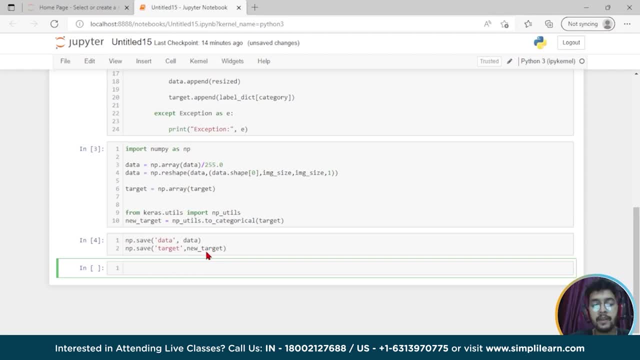 can use it freely. numpy stand for numerical python and this, keras, a python interface for artificial neutral network, is provided by the open source software package known as keras. the tensorflow library interface is provided by the keras. a number of backends were supported by keras up until version 2.3, including tensorflow microsoft. 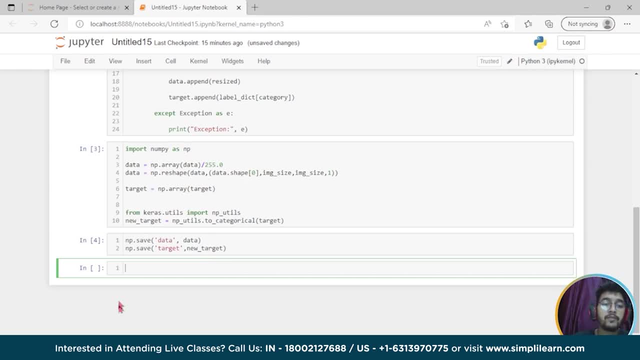 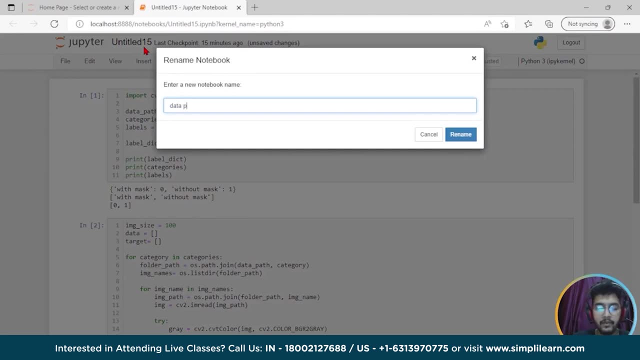 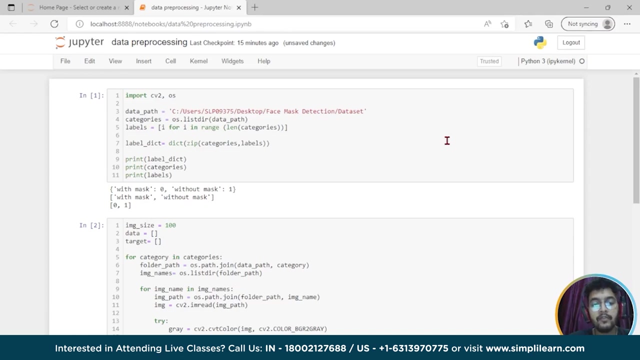 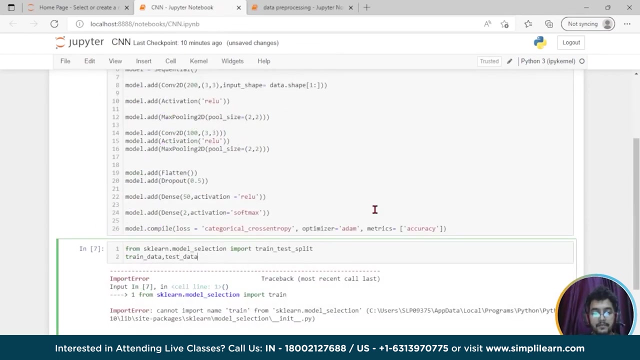 cognitive. so this is the part of the data processing, this all this part of the data processing. so let me write here: data pre-processing, pre-processing. so the data pre-processing part is done. now we will create the another file of this python for the training cnn. cnn means convocational neural network. okay, test data comma train underscore. 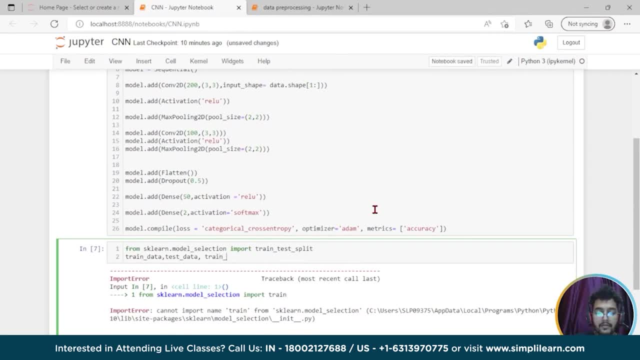 target test underscore target equals to train underscore target test. underscore target test. underscore target test underscore target goes to train underscore split. then we will split on data and target comma. yes, size should be 0.1. okay, so now i will give presenter okay train split. train split is not defined. 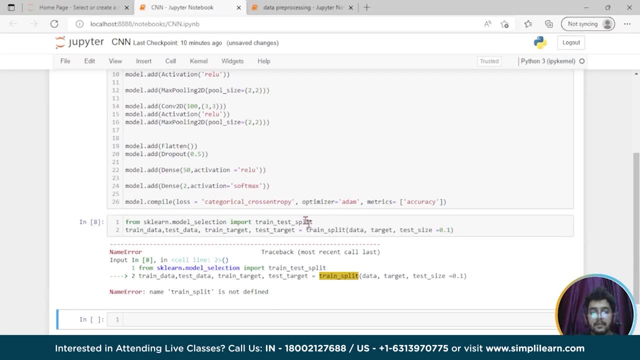 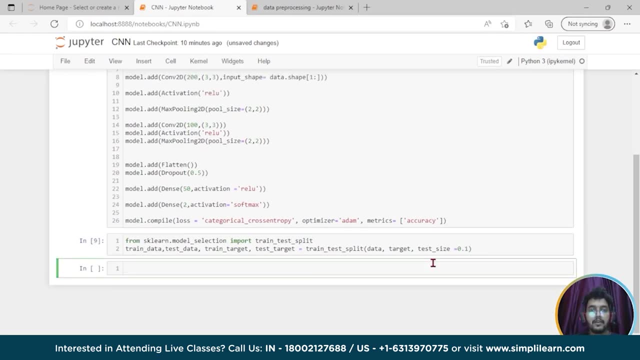 okay, it is train test split. yeah, so now i will write: checkpoint equals to model checkpoint. then again model checkpoint, checkpoint, checkpoint teng. do checkpoint checkpoint 28, 28, 28, i repeat. so here i will write: model comma epoch than 0. 3d comma epoch than 0, 3d dot model. 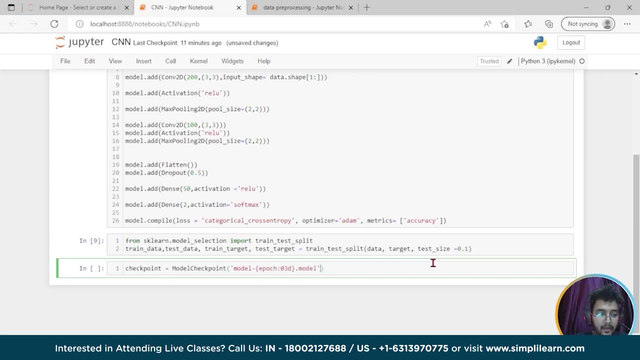 comma epoch than 0 3d dot model. okay, So here I have to write: monitor equals to value loss, underscore loss, comma verbose equals to zero comma, save best Only equals to true comma mode. equals to mode should be auto. Okay, then I will press enter. 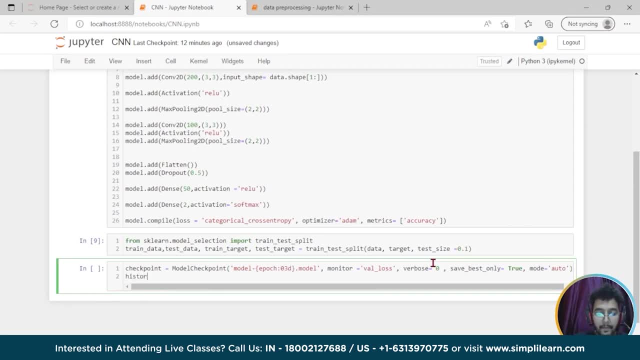 Then here I will write history. It goes to model dot fit to train underscore data comma. train underscore target comma. APOCHS equals to 20 comma. callbacks equals to checkpoint comma. validation validation underscore split equals to 0.2,. the best ratio. 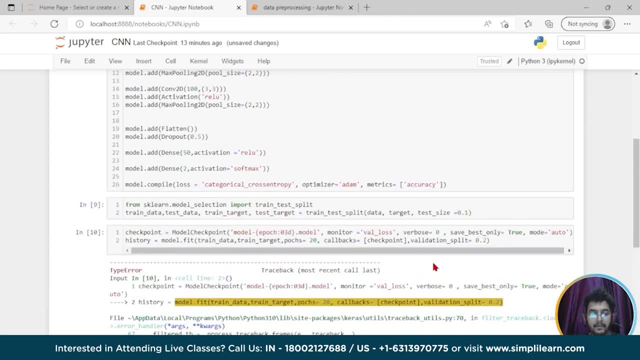 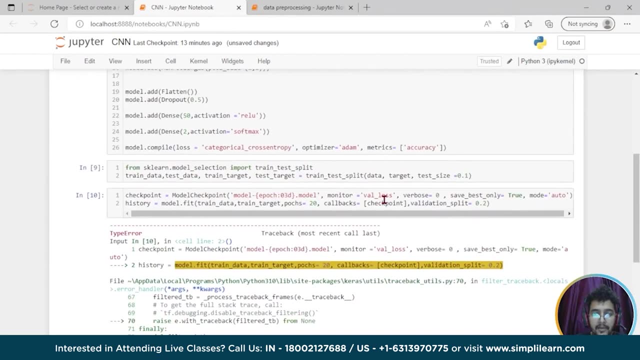 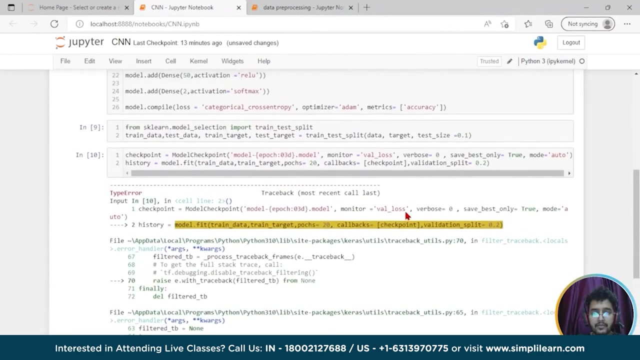 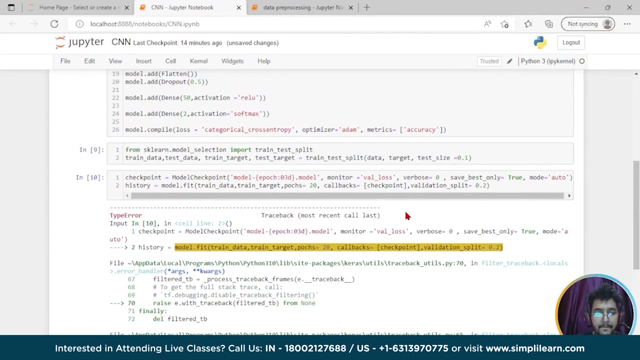 Okay, so let me press enter. Okay, there is one error. model dot fit got an x. Okay, there should be a spelling mistake. Cool, I think I already posted it. Oh yeah, no problem. No problem, I don't think we need that. 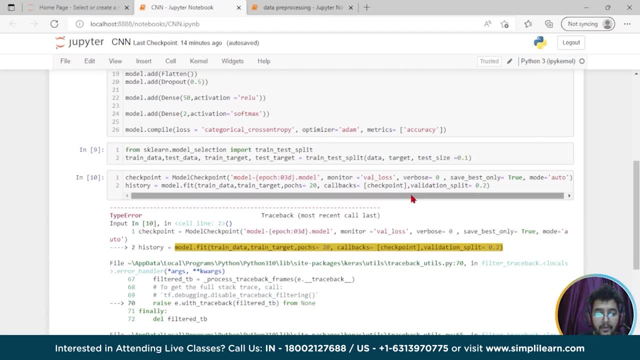 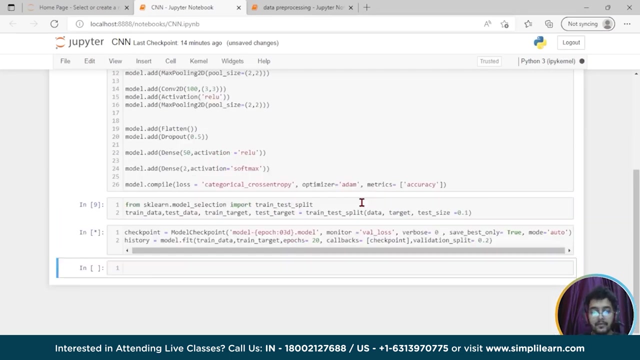 dot model. it is fine. then monitor goes to value loss, verbose equals to zero, save best only because it through, then more. okay, so here I have to write, maybe it will. so it will take some time to go till 20. okay, so it will download one by. 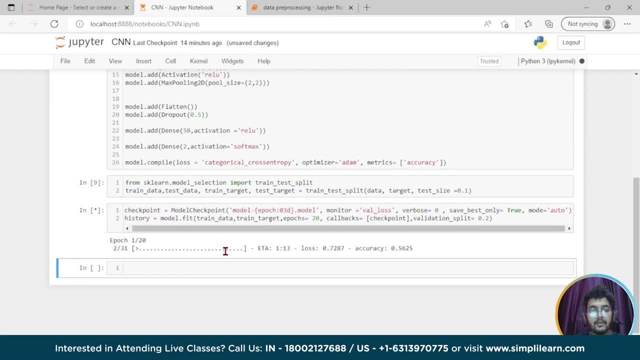 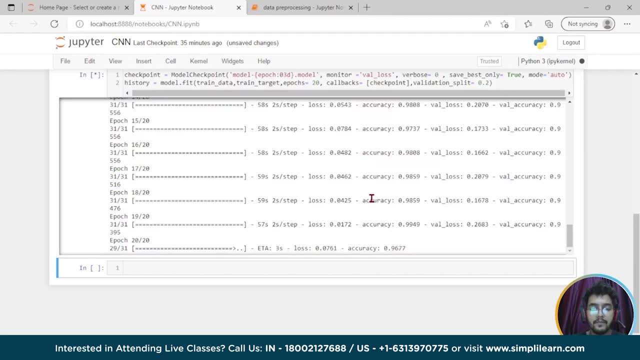 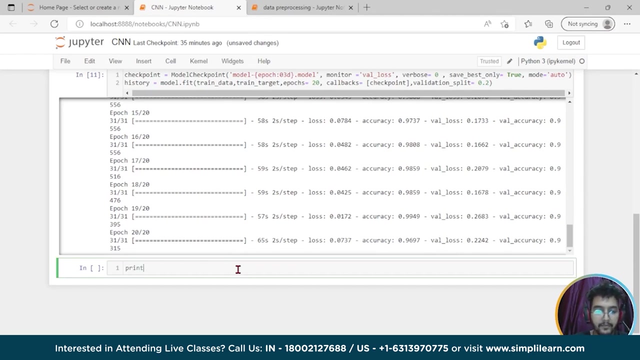 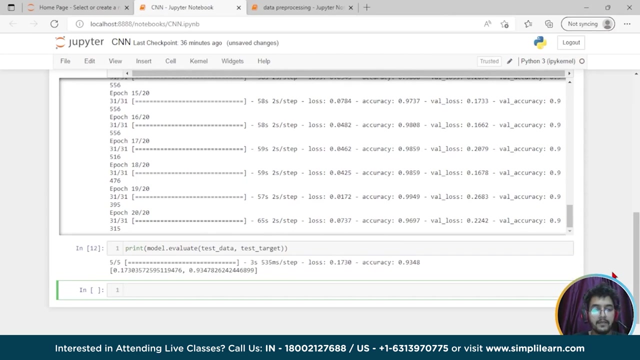 one. so we will wait for a while. so the model checkpoints are completed. so here I will write print, then model dot: evaluate: okay. here I will write test underscore data comma, test underscore target, then press enter, okay, okay, so I hope you guys understand till here. if you have any question or any query regarding 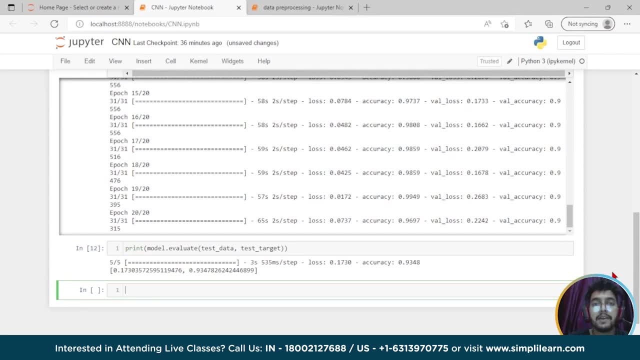 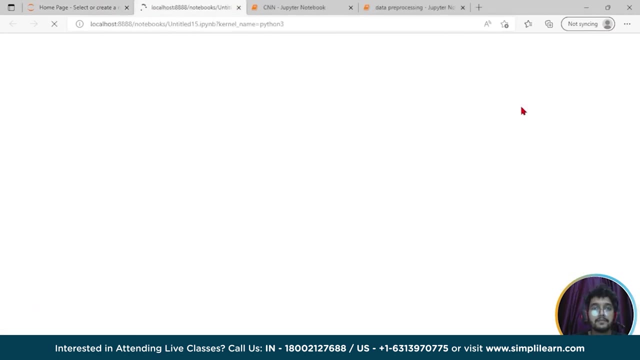 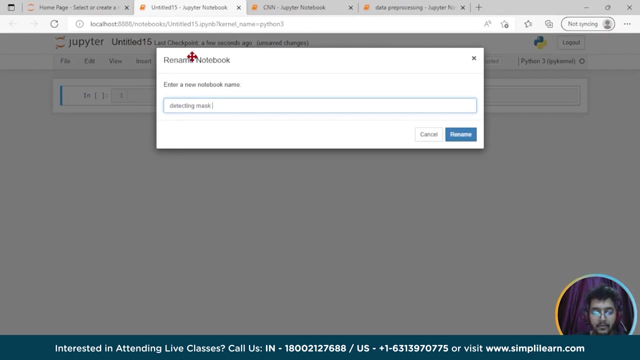 any code, just put as in comments. our team will shortly provide you the correct solution. okay, so moving forward, we will do. we will create another file for detecting mask. okay, so I will go here and then new file, python. so I will write here: detecting mask file. okay. 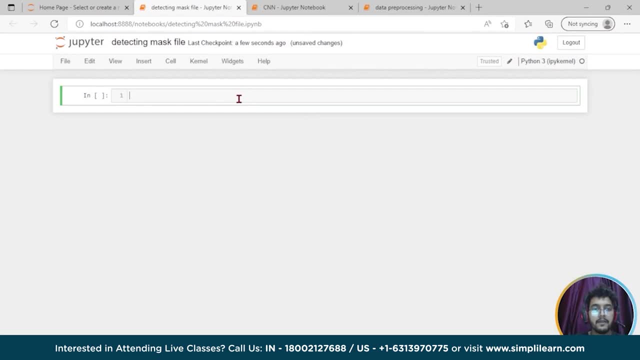 okay, yeah, so I will import some libraries here here as thought models. condom, okay, да, we will import cv2 and we will import numpy as np. Trans дiction, remember the name. ok, okay, numpy as np. okay, so presenter. so what i will do, i will write here: model. 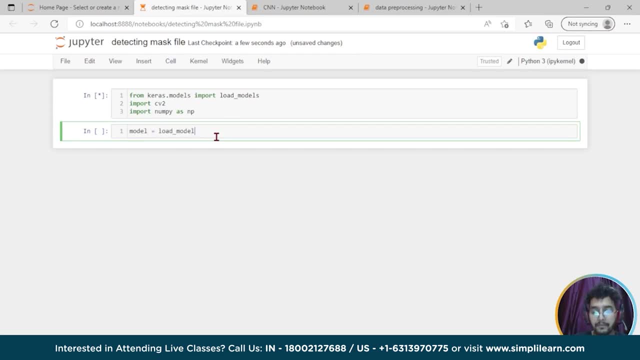 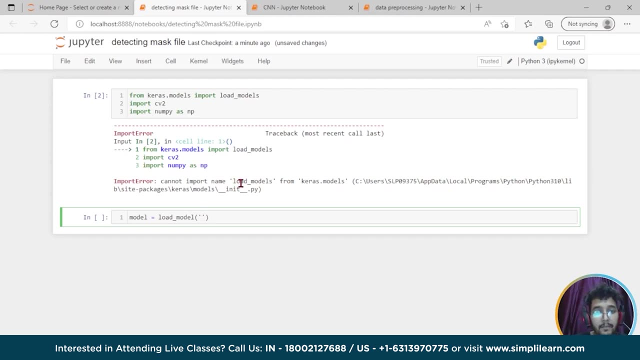 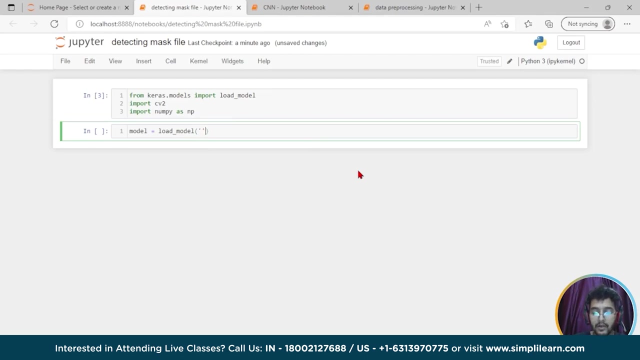 equals to load underscore model, then okay, keras model from chaos cannot import name. okay, so so it is model only. yeah, so here i will add model equal to load model. so i will write here: model 017, dot model. okay, so here i will write face underscore classifier. 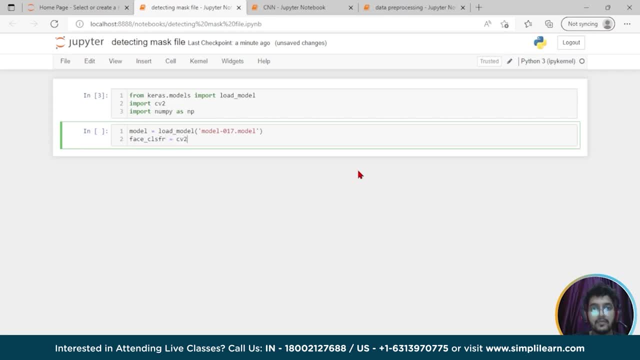 equals to cv2 dot cascade- cascade classifier. so this is one file for frontal phase default. so you can find this file on the description box below, so i will write here our cascade underscore: parental phase underscore: default dot. xml. okay, so source equals to cv2 dot- video. 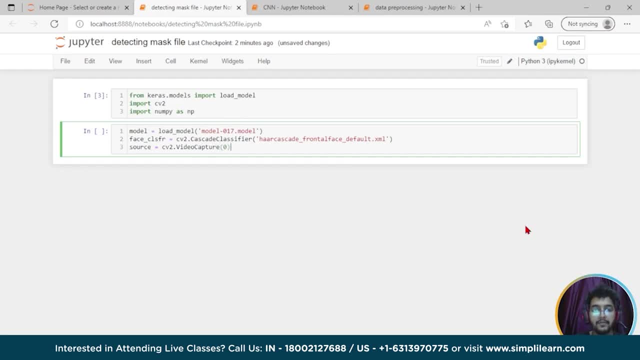 capture 0.. it will open our camera. so labels: underscore: directory: kosu- zero mask and one for no mask. okay so, color directory kosu like: no mask for red and mask for green. okay so here at zero, then zero, comma two. fifty five, comma zero, then again comma for one. there should be zero comma, zero, comma 257. okay so. 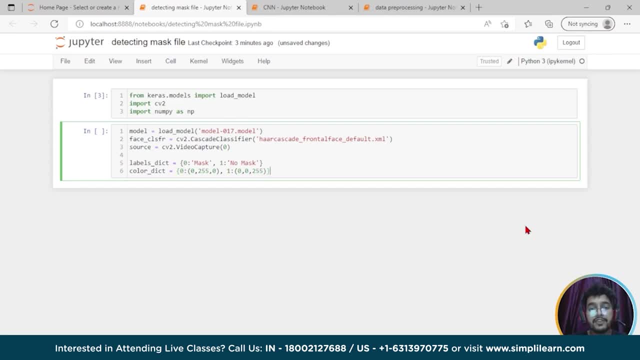 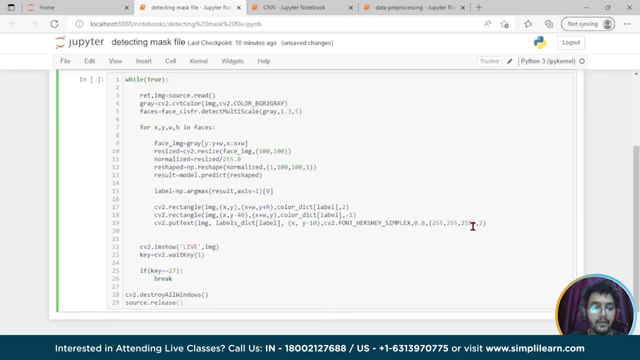 i hope you guys understand till here. so if you have any question or any query regarding any code, so just put as in comments. our team will surely provide you the correct solution. so the code is written. so let me run this for this. first i have to like, so first i have. 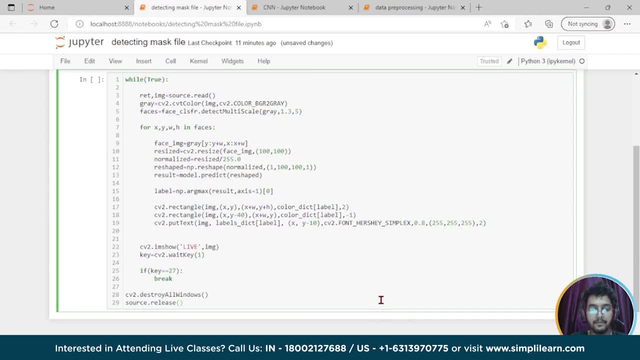 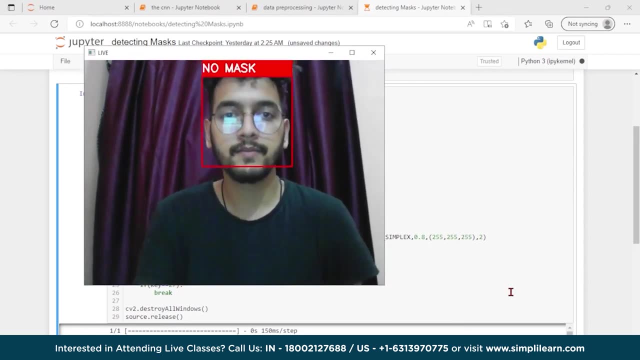 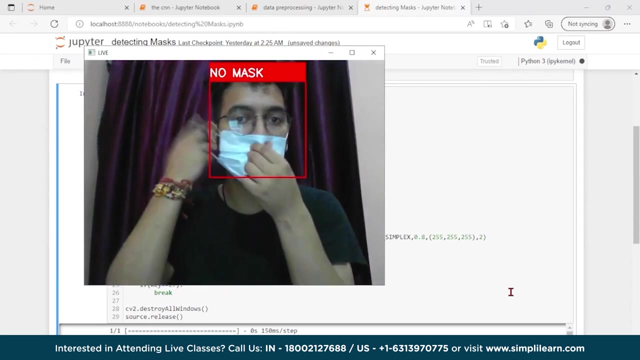 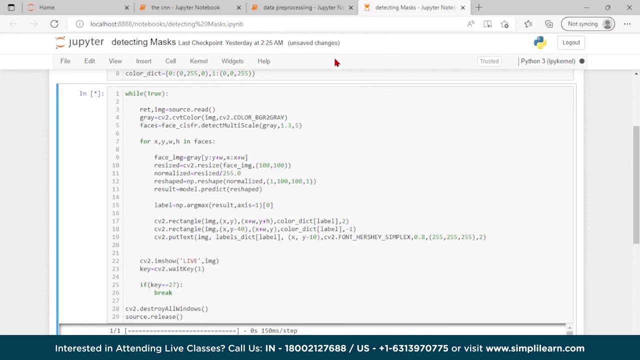 to close my this person on a screen camera. so the code is running fine. now it is showing no mask. now it is showing mask. so i hope you guys understand till here. if you have any queries, any question regarding any code, just put as its comment. our team will shortly provide the correct solution. 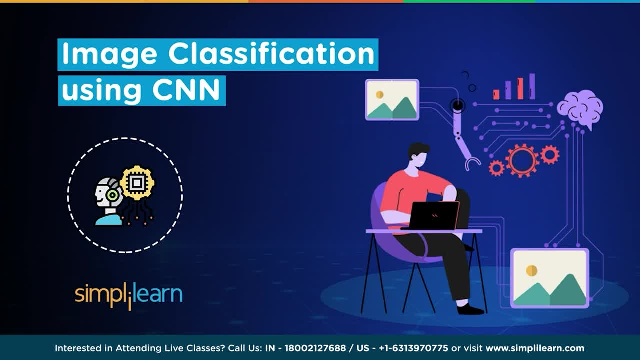 in today's session we will discuss what image classification is and, moving ahead, we will discuss what cnn is and at the end we will do a hands-off lab demo of image classification- what اینEtS using CNN. so before we move on to the programming part, let's discuss what 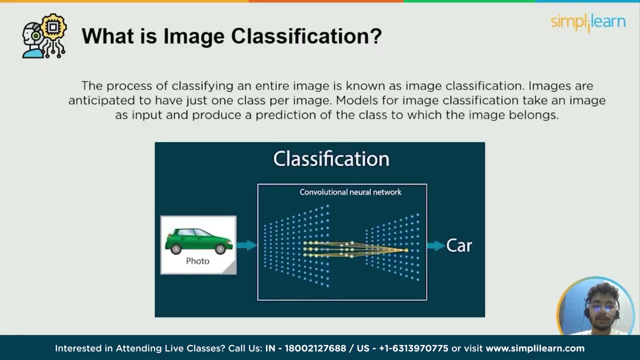 image classification is and proceed further for the same. what is image classification? the process of classifying an entire image is known as image classification. images are anticipated to have just one class per image. models for image classification taken an image as input and produce a prediction of the class to which the image belongs. we can utilize image. 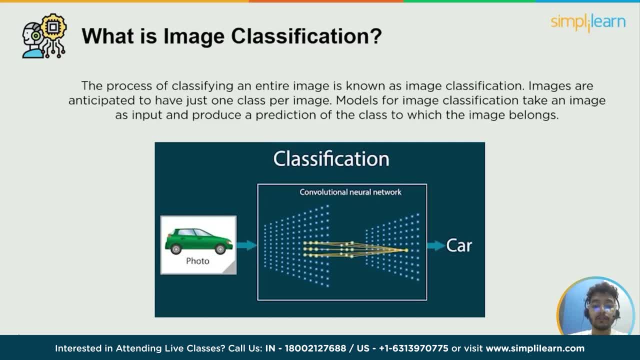 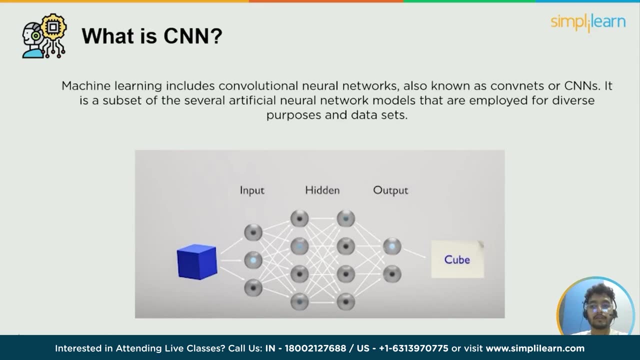 classification models when we are not interested in individual instance of items with position information or their shape. so let's see what is CNN. machine learning includes convolutional neural networks, also known as convents or CNNs. it is a subset of the several artificial neural network models that are employed. 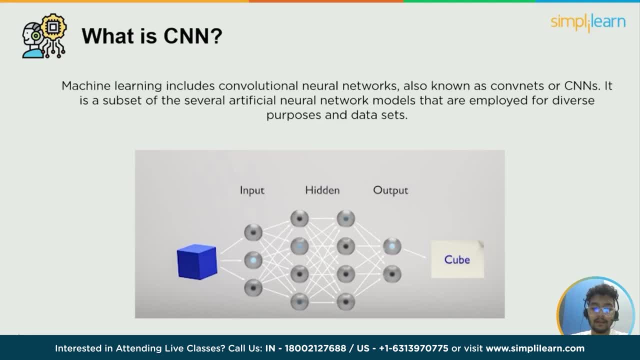 for diverse purpose and data science. a CNN is a particular type of network design for deep learning algorithm that is utilized for tasks like image recognition and pixel data processing and so more. okay, although there are different kinds of neural network in deep learning, CNNs are preferred neural architect for identify and recognizing. 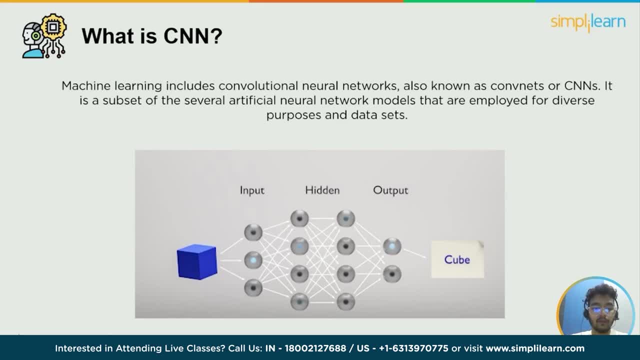 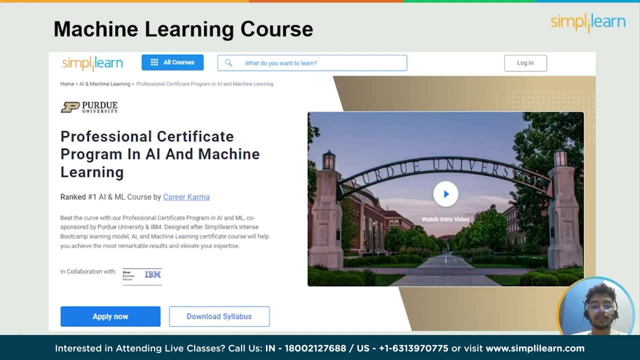 object. therefore, they are really suited for computer vision activities and application where accurate object recognition is crucial, such as facial and self-driving automobile system. so moving ahead. so, dear learners, if you want to upskill your AI and machine learning skill, so give yourself a chance to simply and professional certificate program in AI. 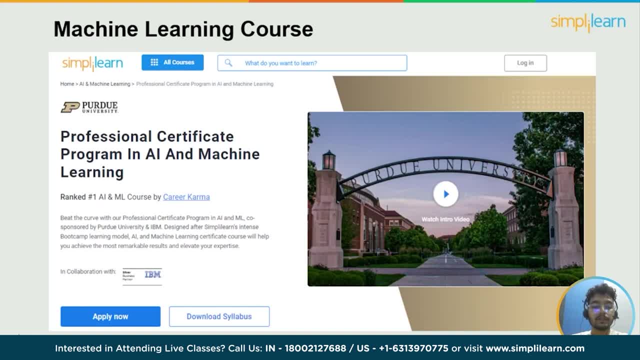 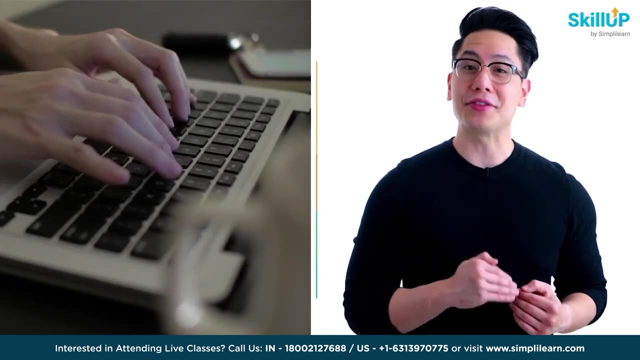 and machine learning, which comes with the completion certificate and in-depth knowledge of AI and machine learning. check this course out. details from the description box below. so now let's move to a programming part of how to do image classification using CNN. if getting your learning method is half the battle, what if you could do that for free visit scale up by: 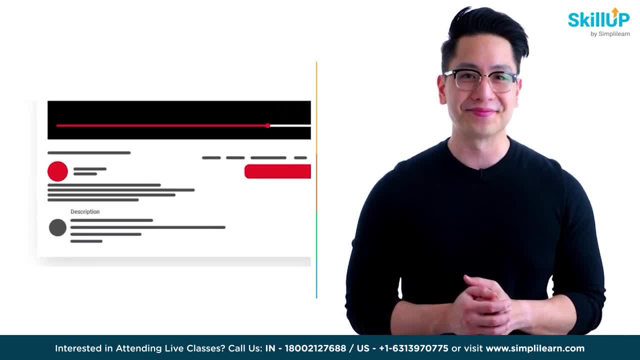 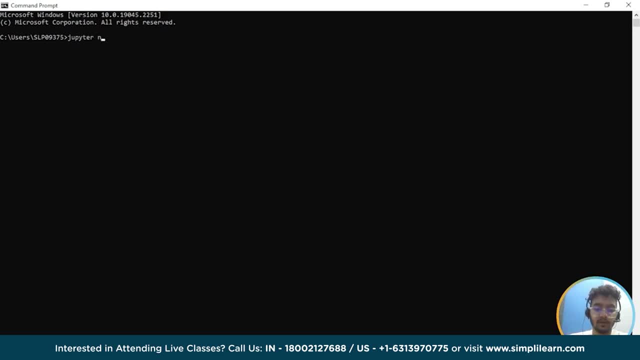 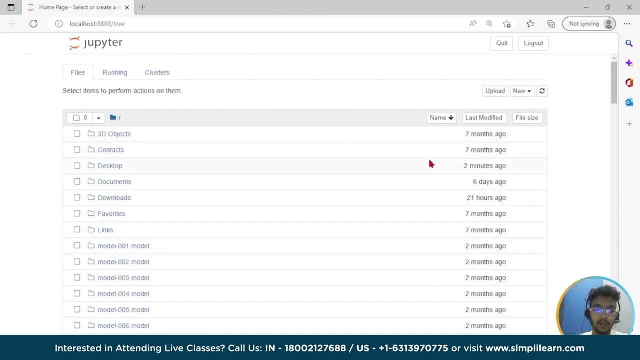 simply learn. click on the link in the description to know more. so first we we will open a command prompt to write a command to open Jupyter notebook. so here we will write Jupyter notebook, press enter. so this is the landing page of Jupyter notebook. so here you can select new python file. 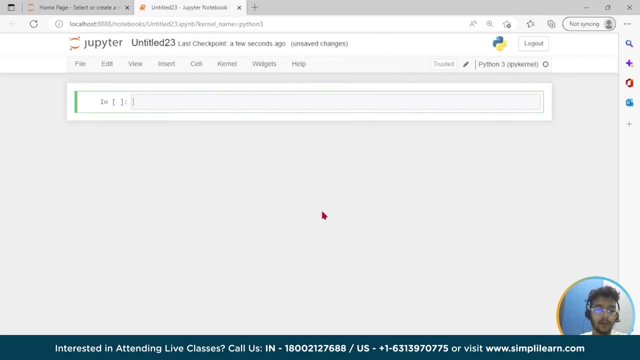 so this is how the kernels look like. okay, Jupyter notebook kernels look like so: first we will import some major libraries of python which will help us in like analyzing the data. okay, so in this file we will classify small images of cifar 10 dataset from tensorflow Keras. 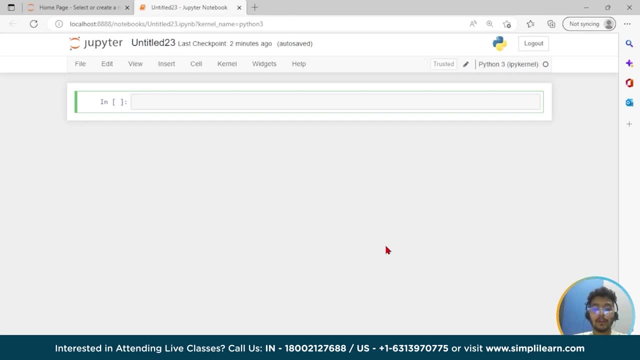 dataset. there are total 10 classes as shown below. so we will use cnn for the classification purpose. okay, so here I will write: import: insert flow as tf- okay, so from tensorflow dot Keras. import data sets from our layers models: okay, so we will import numpy as np right and import matplotlib as plt. 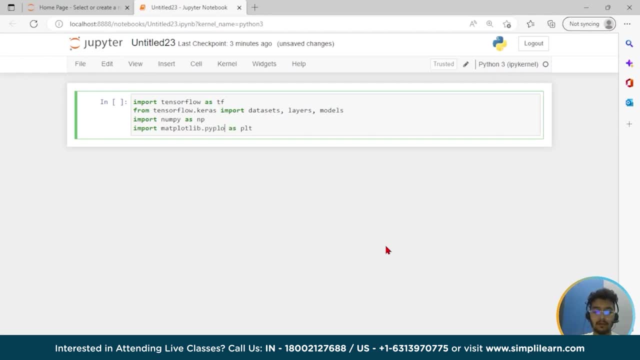 right. okay, so here I will like by plot as plt: right, so tensorflow one this. so tensorflow is a free and open source machine learning and artificial intelligence software library. it can be used for variety of applications, but it focuses on mainly deep neural network training and the inference purpose. okay, got it. and this numpy numpy is a python library. 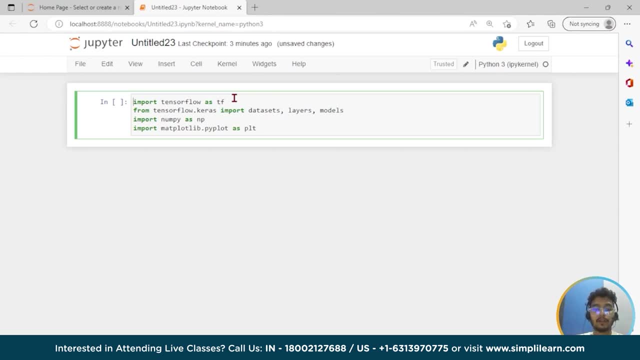 used for working with the arrays. it also has a function for working with the domain of linear algebra and matrices. it is an open source project and you can use it freely. numpy stand for numerical python and this third one, matplotlib for python and its numerical extension. numpy matplotlib is: 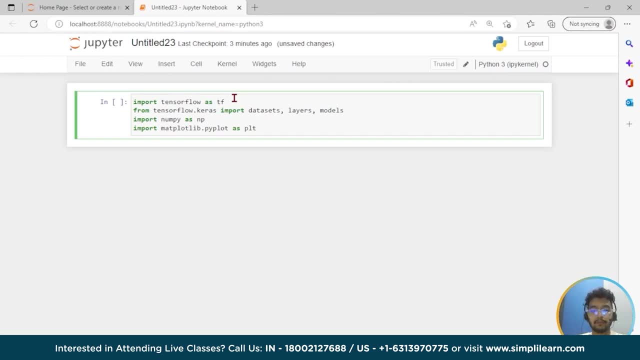 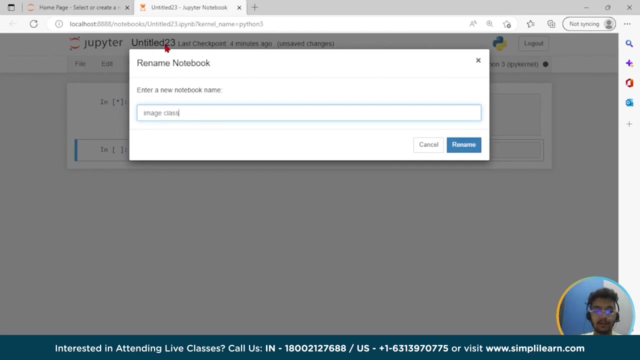 a cross-platform data visualization and graphical charting package. as a result, it present a strong open-source substitute for matlab. the apis application programming interfaces for matplotlib allow programmers to incorporate graphs into java. ui applications got it, so let's run this. let me change image classification using 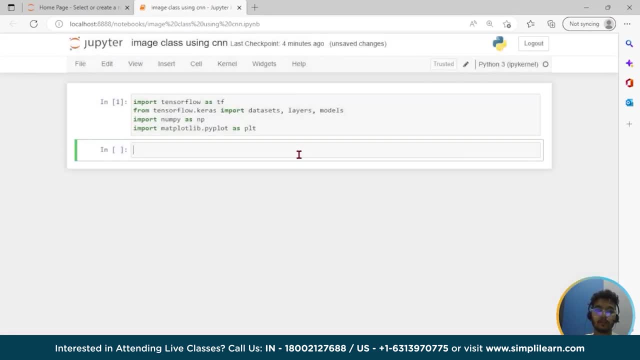 the annan. okay, so let's load the data set. okay, we will load the data set from the uh load data a function. so here i will write x underscore train, comma y underscore train: okay. and one for test: x underscore test. comma y underscore test: okay. then 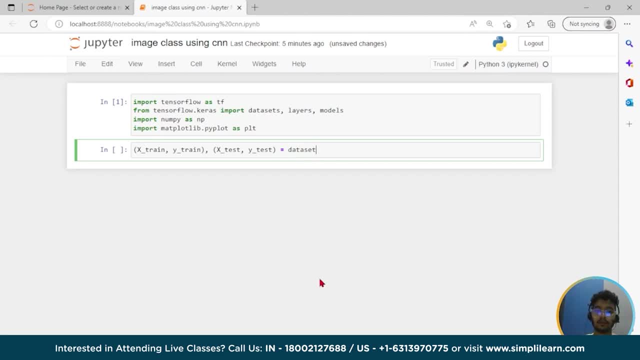 equals to data set. data sets dot. we are using cipher 10 c for 10 for 10 dot. load dot underscore data. okay, so it will load our data. so let's load the data. oh, data is loaded. let's see x test dot shape. okay, yeah, so, as you can see, 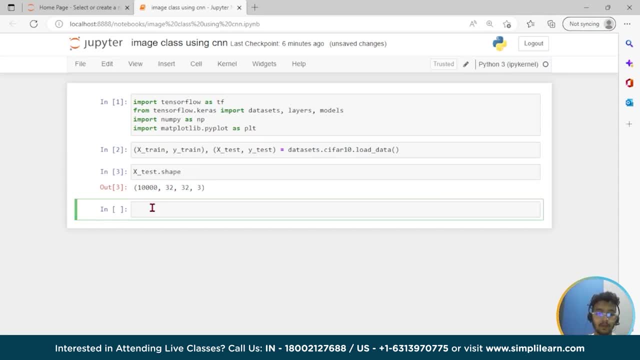 so we have thousand rows and one more x underscore train dot shape. yeah, so, as you can see. so we have thousand rows and one more x underscore during dot underscore during dot shape shape. Let me run this So here you can see Like we see the training data. 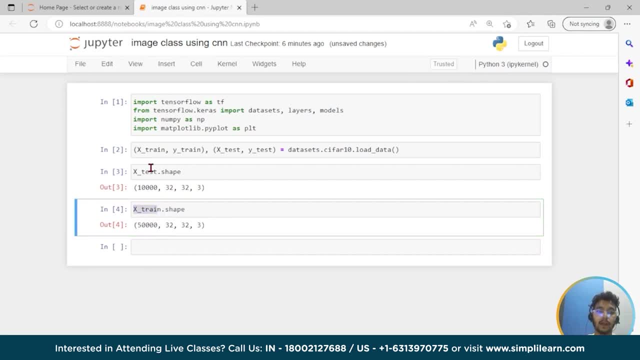 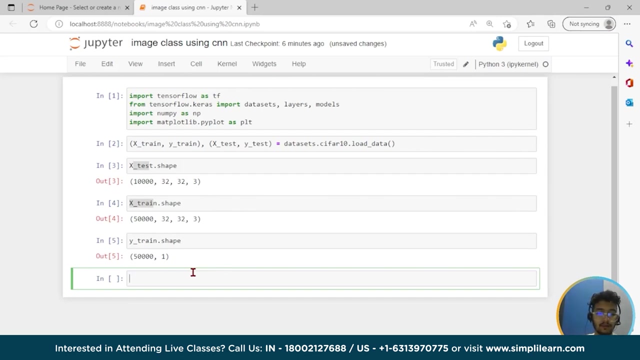 like training images are 50,000 and the test images are 10,000. okay, So this is for testing, this is for training, and, And so, moving ahead, we will see, for the Y Rain dot shape Thousand, and here we will see the array. so why underscore train? 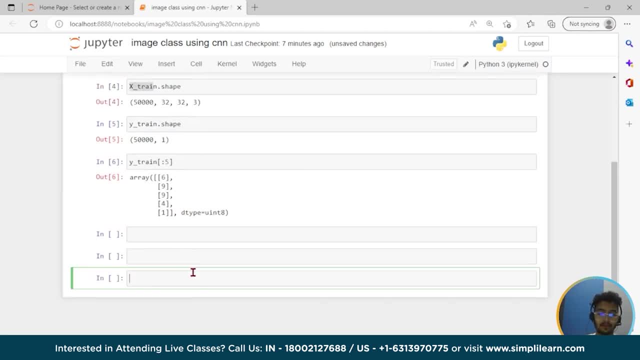 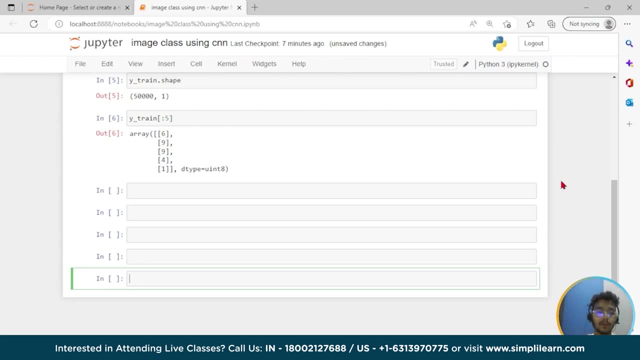 Five. okay, let's run this first. Let me give some space, Yeah. So here, why underscore? train is a 2d array, Like for our classification. having one day is a good knee, you know. So what we will do. we will convert this to now 1d error. This is 2d array. We will convert into 1d array. 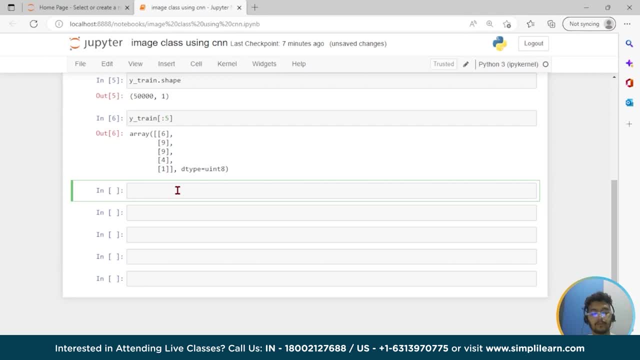 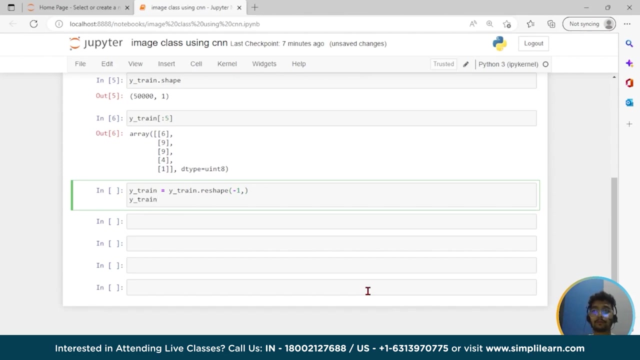 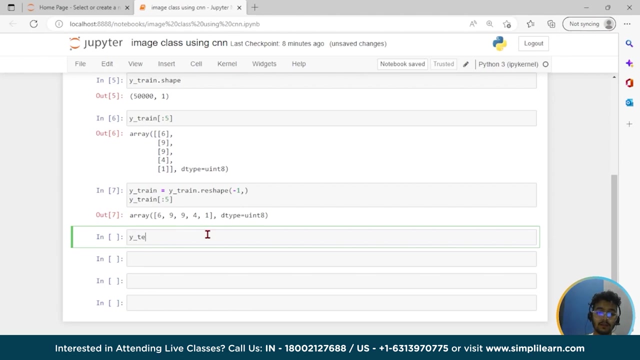 Okay, for that You Will write here: why underscore train Was to why underscore train. dot reshape Minus one, Then why underscore train? And again semicolon 5. Let's run this Okay. So now this is 1d array, so Why underscore test Goes to why underscore test. 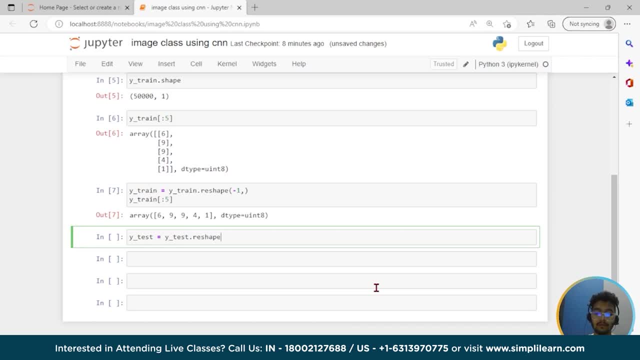 Dot the shape In minus 1. Here I will write Classes. Of course you. there are some classes Okay in the data set, like airplane, Comma, automobile, But Cat, Yeah, Dog, Okay, So let's find your, me, Ours, You Try To Get. These are the same classes. 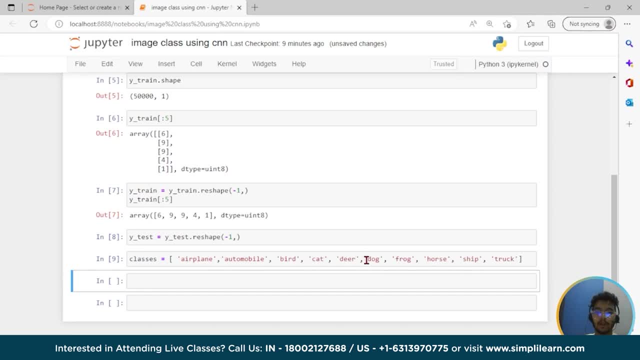 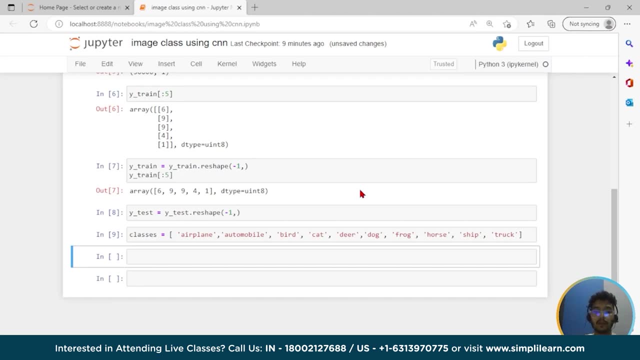 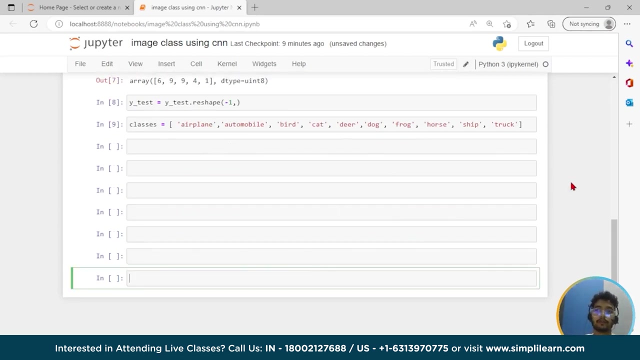 In like airplane, automobile, bird, cat, deer. so it will be helping classifying the images. so let's plot some images to see like what they, what they exactly are. okay, so we will, what we will do. we will create one function for that. let me write here: def plot underscore sample. 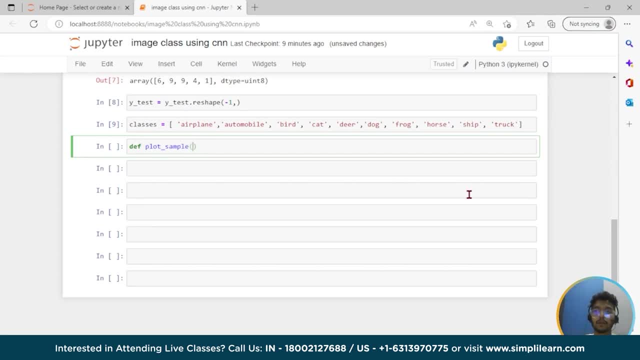 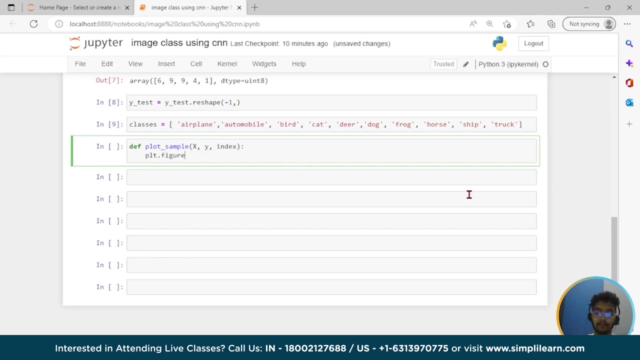 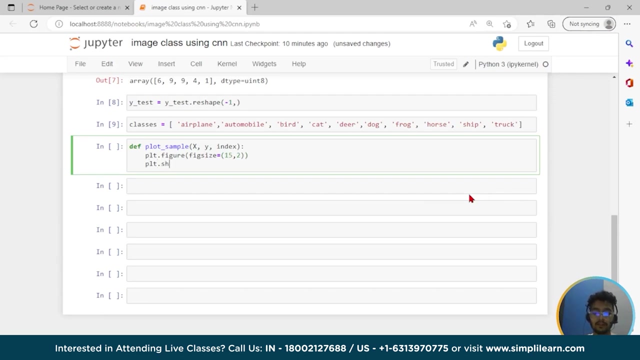 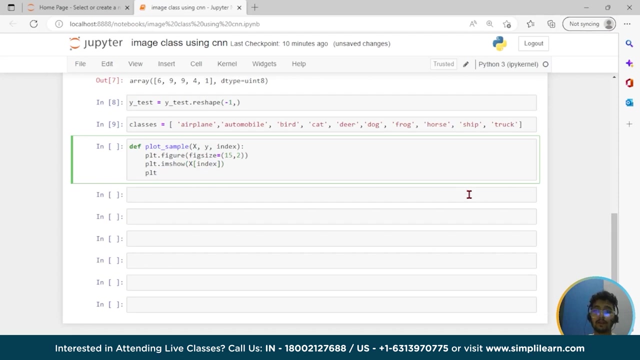 okay then x comma, y comma index. okay, then i will write here plot dot figure, plt, dot figure. then figure size should be comma two equals to plt, dot show. image show to, i am sure, x index, plt, dot, x, label classes, y index. okay, so let's see some samples of the images, so i will write a plot. 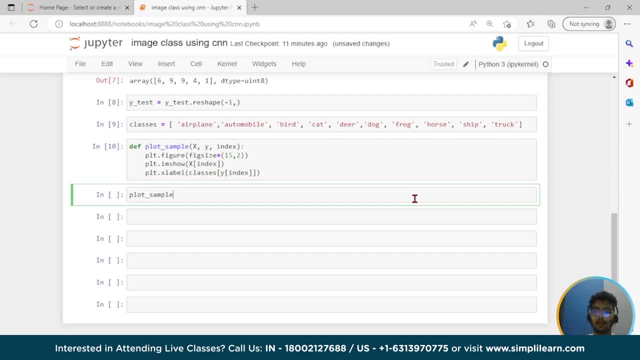 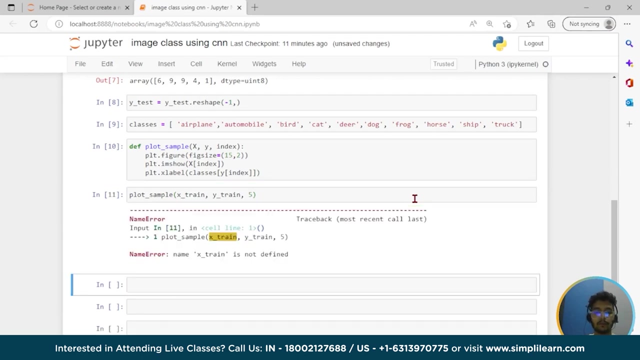 underscore sample: x. underscore train comma. y underscore train: okay, comma. let's see the fifth image. okay, then enter should be capital. so, as you can see, this is a car, so it should be capital. so, as you can see, this is a car, so it should be capital. 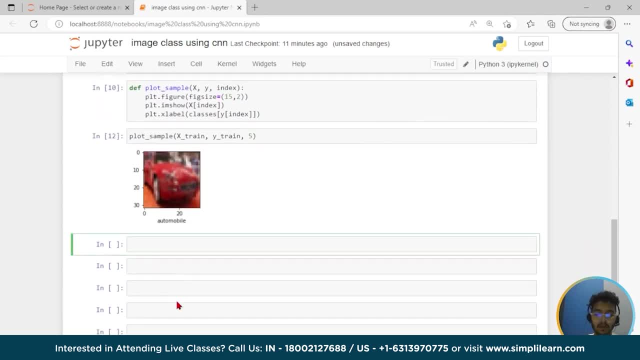 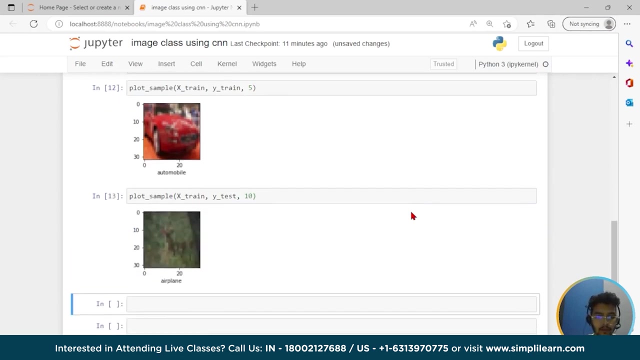 is showing autumn oil, okay, so let's see once more: like: plot underscore sample x underscore train comma. y underscore test comma. we'll see the tenth one. okay, it is not quite visible, so we'll go for the lemon, okay. okay, i am why it is showing wrong: because i use a test. 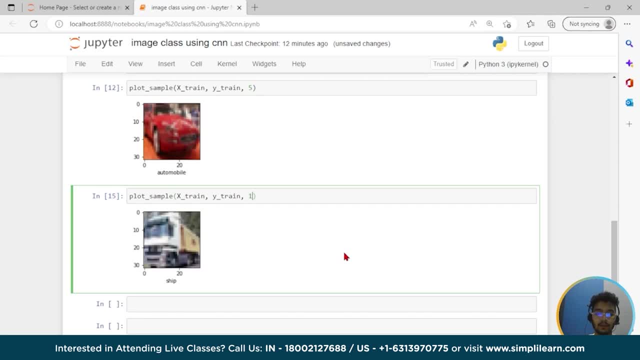 i have to use here train instead of test, then it will show. i think, correct, yeah, you can see horse, then odds. then what about 201 image? see, you can see. so we will see once more 500 fancy frog. okay, it's not quite visible. yeah, so you can see. 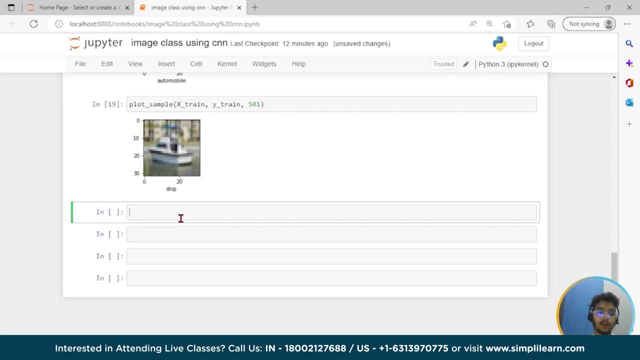 here the proper shape. okay, so what we will do now. we will normalize the images to a number from zero to one image has three channels, like rgb colors so, and each value in the channel can range from 0 to 255. hence, to normalize in 0 to 1 range, we need to divide it by 255. okay, so now what we will do. we 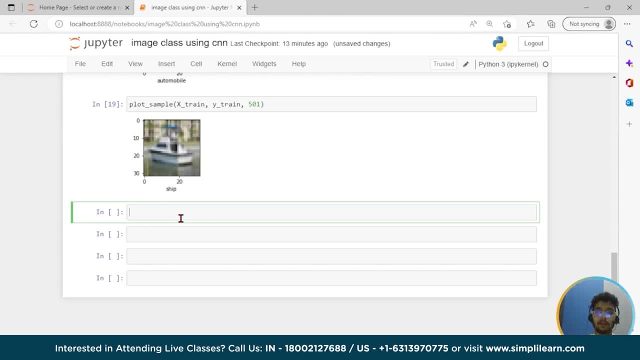 will normalize the data. we will normalize the data. so now what we will do. we will normalize the data. stuff massage. okay, test test part of 0.05' isear to range between 0 to 1. we will build simple artificial neural network for image classification. first, 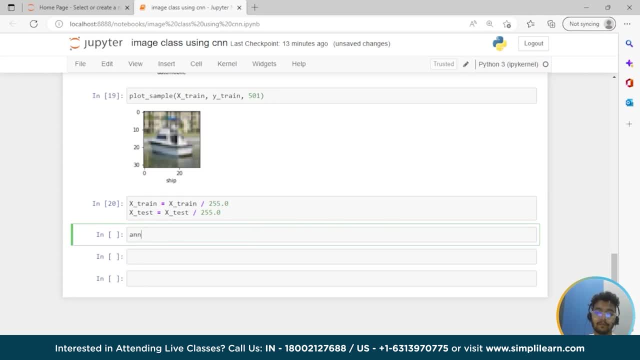 ok, so we will write here: ANN opposed to modelsSequential. ok, then I will write here: layersplatten report, underscore shape equals to 32 comma 32 comma 3. ok, then again layerstens. ok, then again layerstens. ok, then again layerstens. 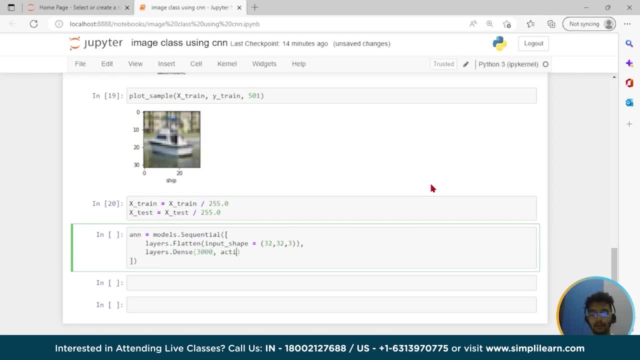 3000 comma activation, also real, you got it. and again for the thousand. so i will what i will do, i will copy it and paste it here. okay, so thousand. so uh, let's let me at one more, one more layer, layer, dot, tens. layer, dot, tens. 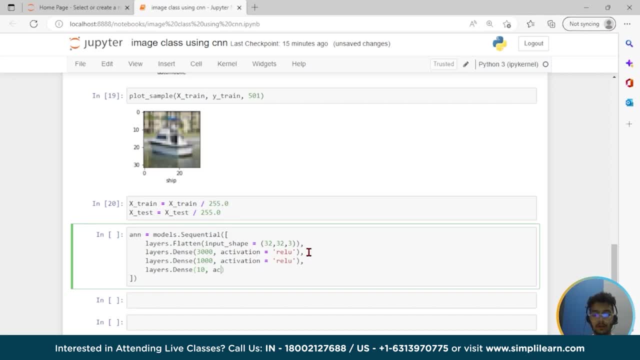 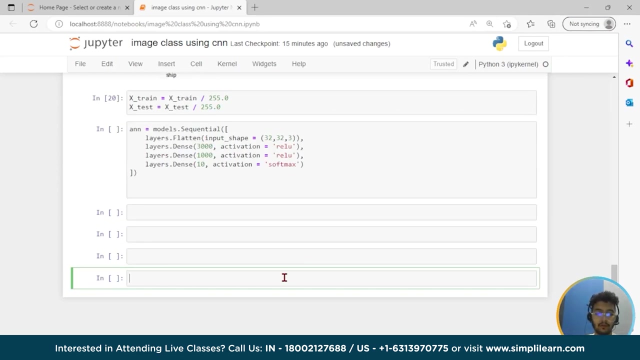 layer dot tens, Vie. One more layer to make a zero, one more layer to make a zero with 10 connection, with 10 connection, with 10 connection, comma activation, softmax. okay, then i will, then i will, then i will. okay, let me give, then i will. okay, let me give. 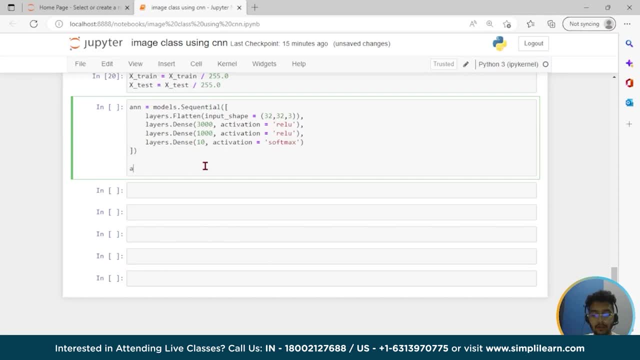 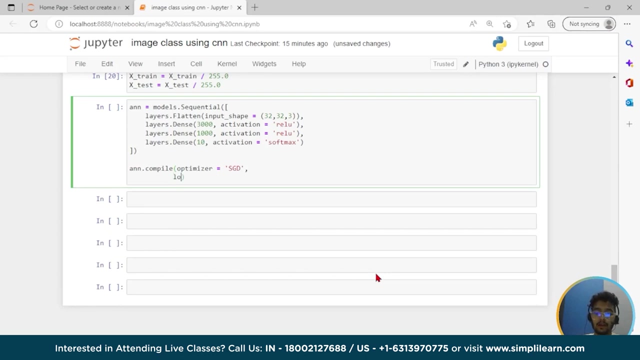 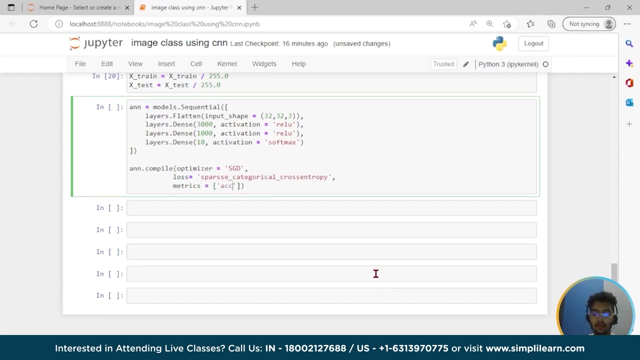 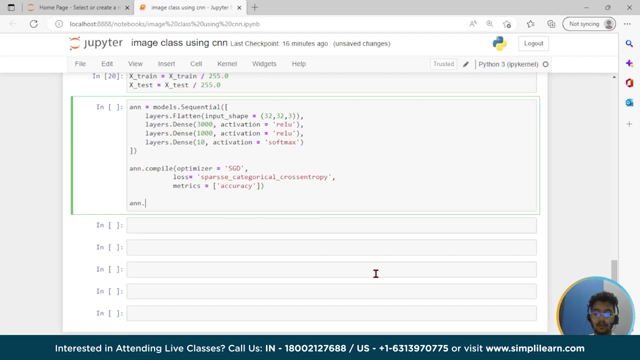 better pessoas, better examples. go ANN and dot. compile optimizer: okay, go to sgd and comma. i will write here: loss equals to sparse categorical cross entropy, okay. so here i will write comma. then matrix equals to accuracy. ann. dot fit underscore train underscore train comma, epochs, okay. so number i will give you box equals to: 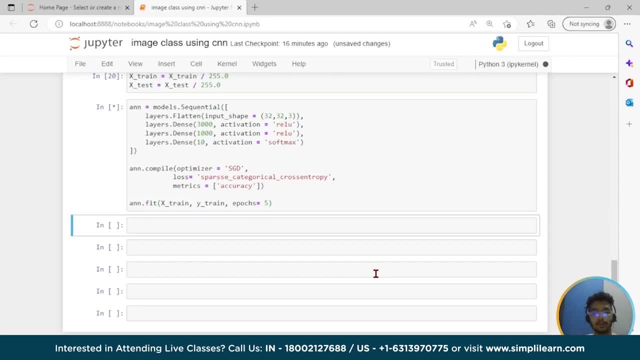 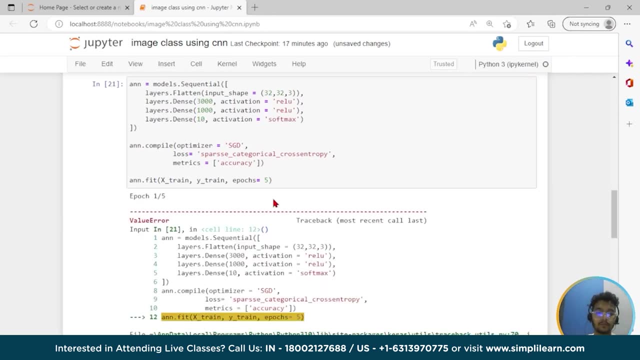 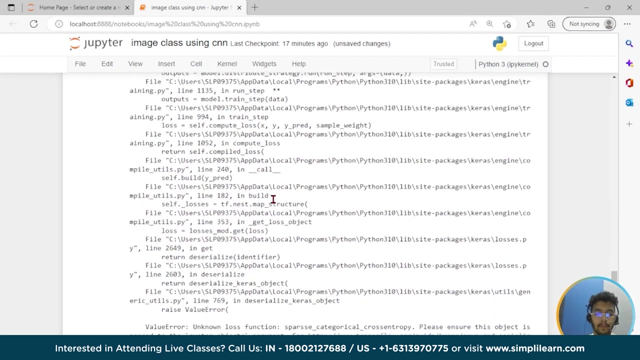 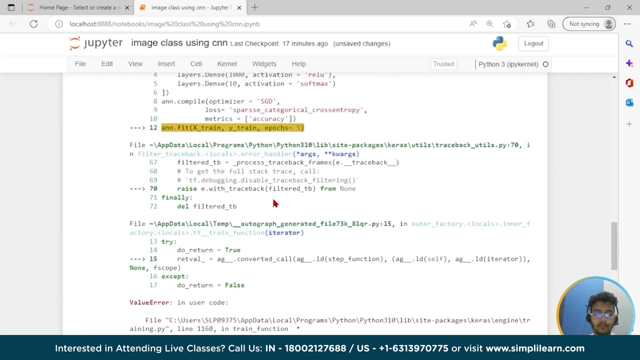 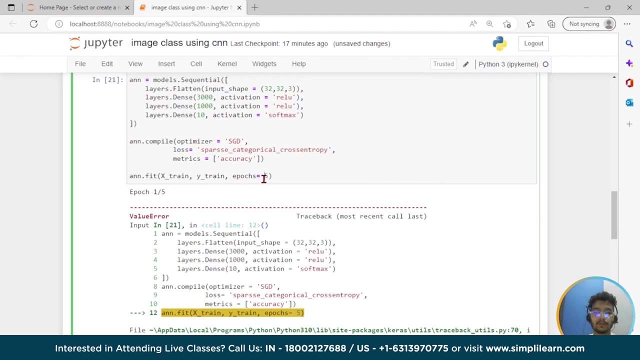 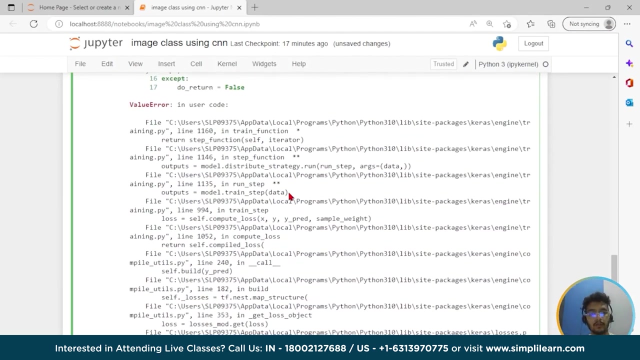 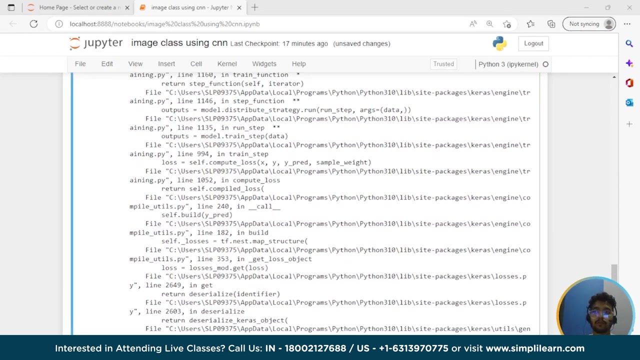 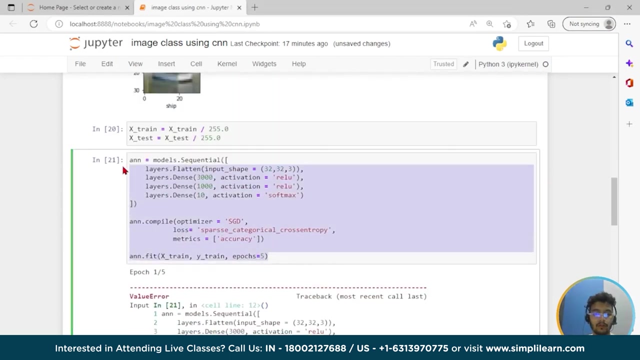 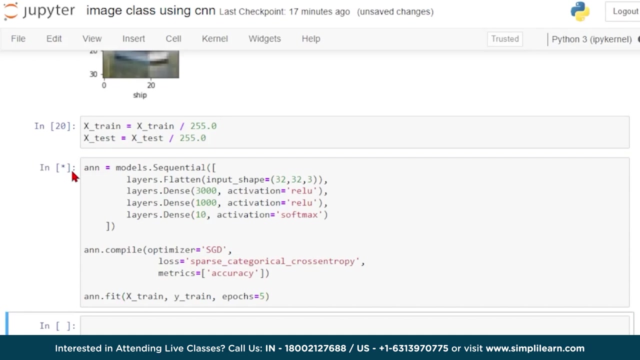 five. right, so it will take time to run. it's running here. there is some issue, so underscore train epochs equals to five what it is saying when user go the file program c and then okay, so i'll copy it and push it again. run it again. okay, now it's working okay. 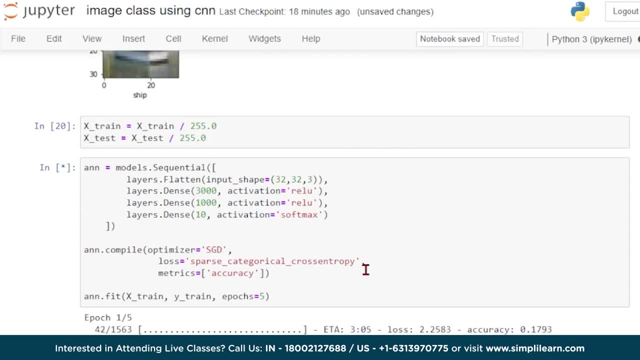 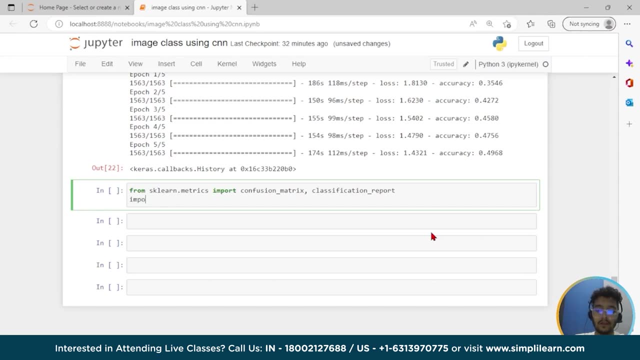 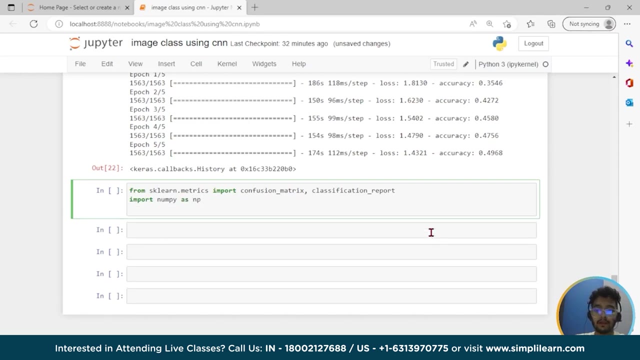 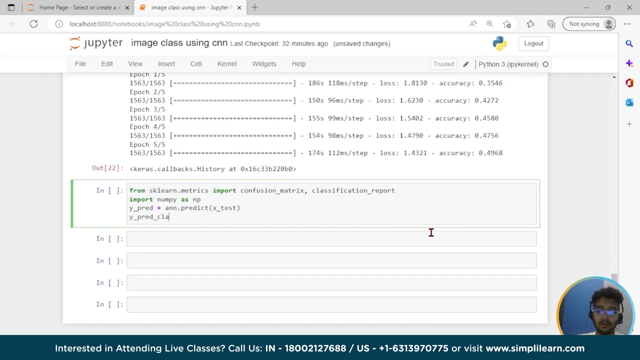 so it will take time and then i will get back to you. okay, then import numpy. you guys already know what numpy is: np. y underscore prediction versus ann dot predict, predict, predict, predict, predict, predict x underscore test. okay, then y underscore prediction, underscore classes goes to np dot. 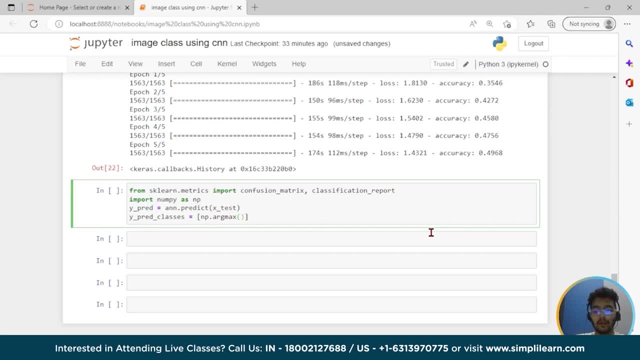 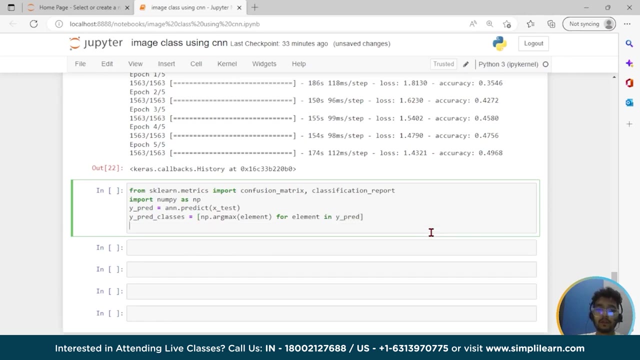 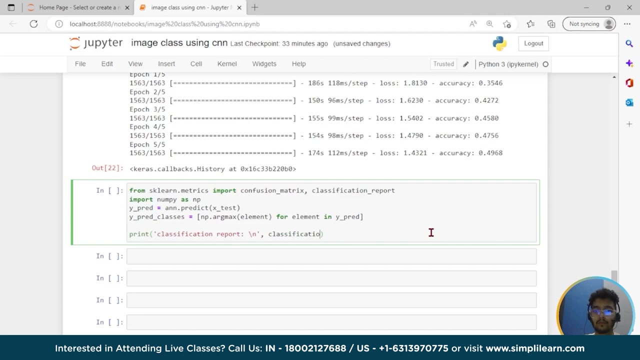 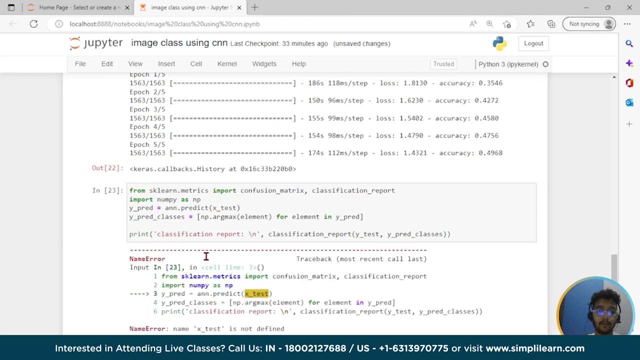 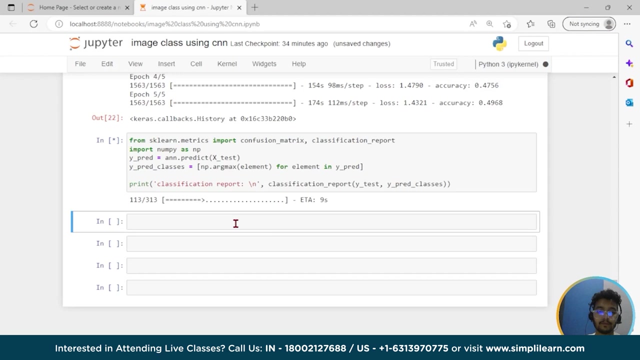 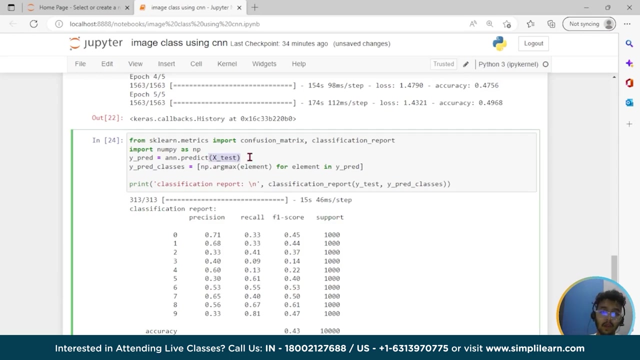 argument: max element or element in: y underscore prediction print classification, port comma classification underscore report. then y underscore test comma. y underscore prediction underscore classes. okay, so let me run this. this is capital. yeah, it will take less time. now we will create a graph. okay, like x text is like we have thousand images, so 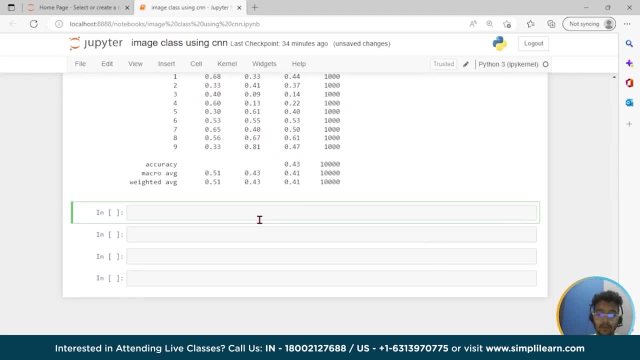 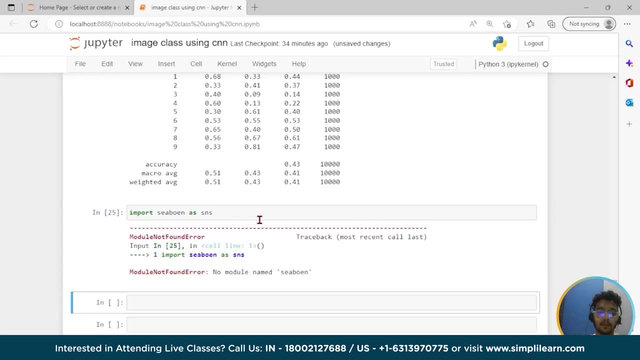 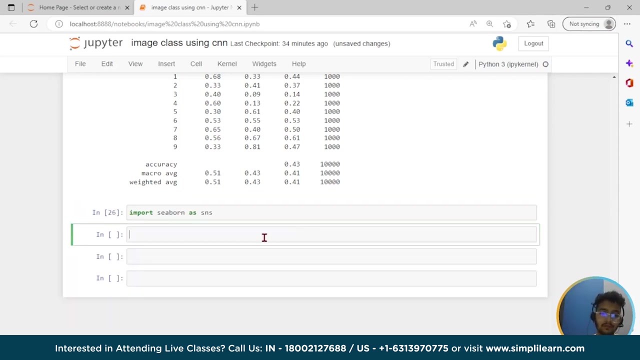 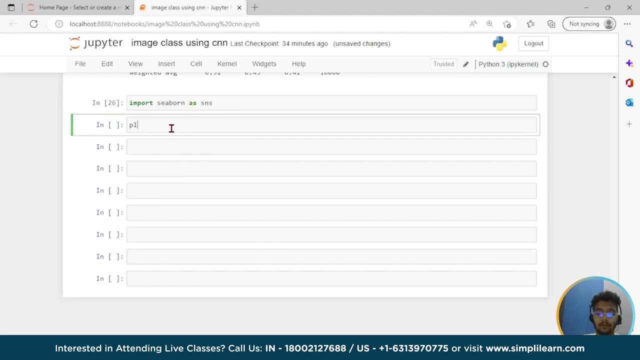 graph will be like messed up still, let's see. so i like import c bond as sns. okay, let's see, bond. yeah, let me give some space here. i will write plt dot bigger, because i should be thirteen comma seven. okay, then, sns, we will create a heat map. 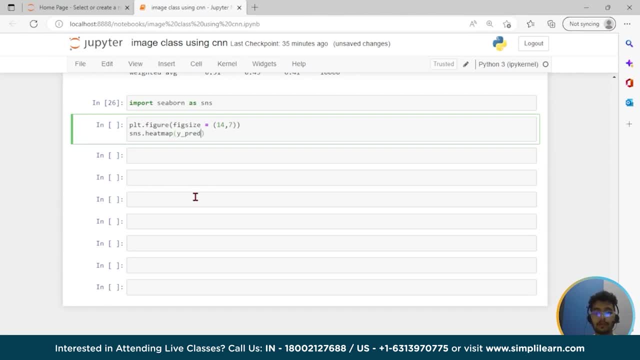 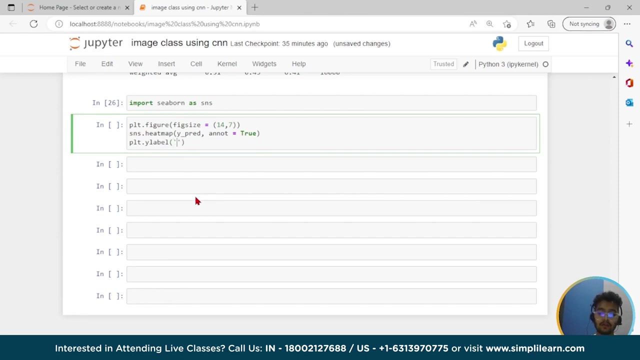 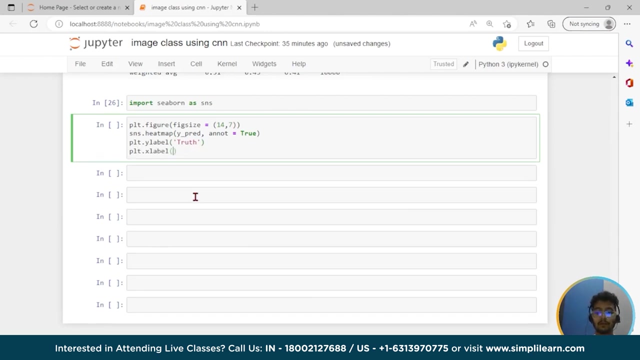 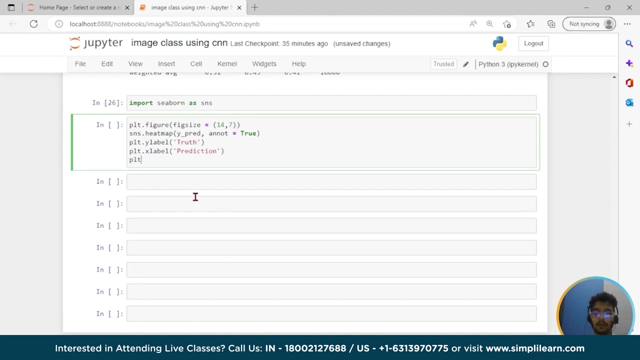 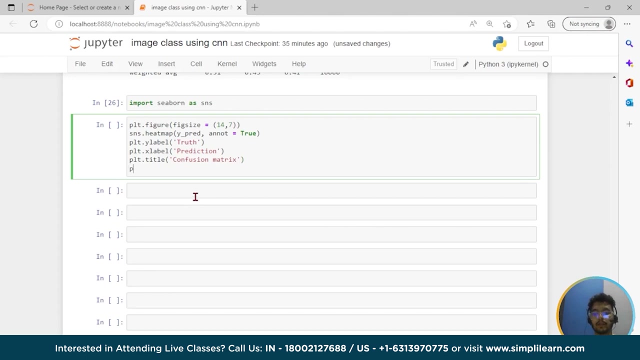 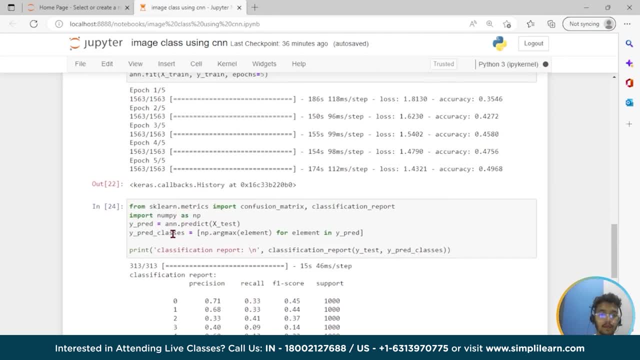 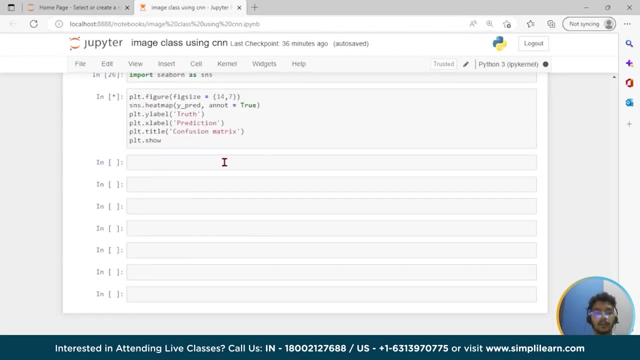 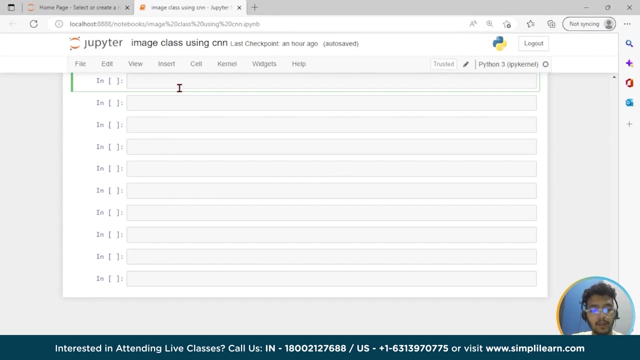 let me run this. okay, the y prediction has x text. it's still running. let's wait, let's wait, let's wait. so now let's make cnn model. okay, to train our images. so for that i will add cnn equals to models, dot: sequential. okay, right, yeah. so let me run this. 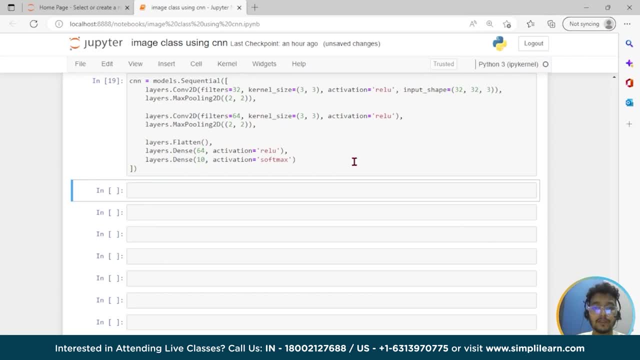 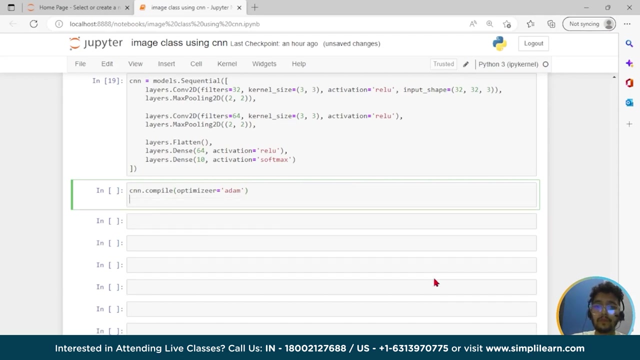 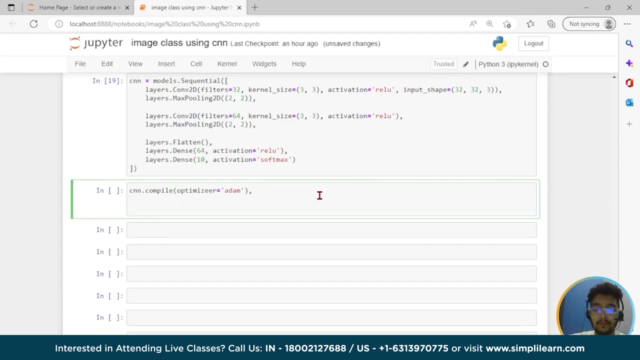 so this is our cnn model from which we will train our images, and cnn like compile, then optimize. optimizer equals to adam, okay, okay, comma, right here, then loss, ok, spars, spars, categorical, categorical, okay, then cross, ok, and comma and comma. i will write here matrix. okay, i will write here matrix. 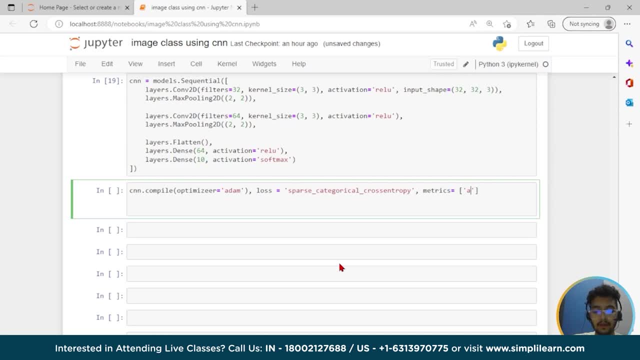 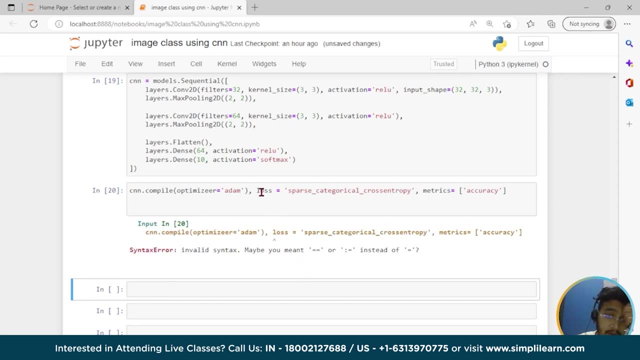 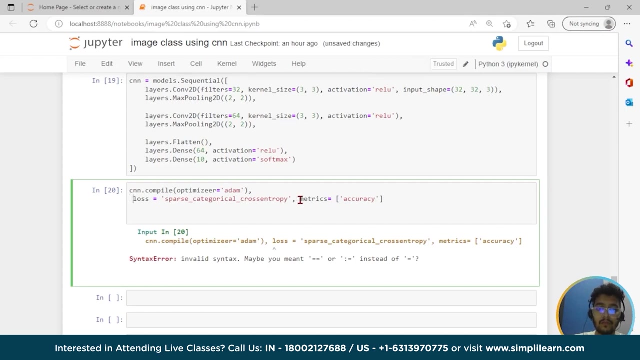 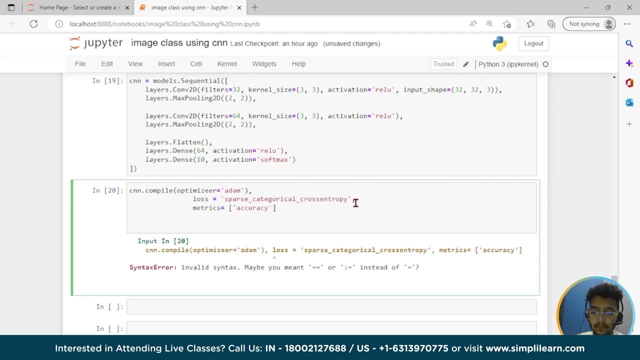 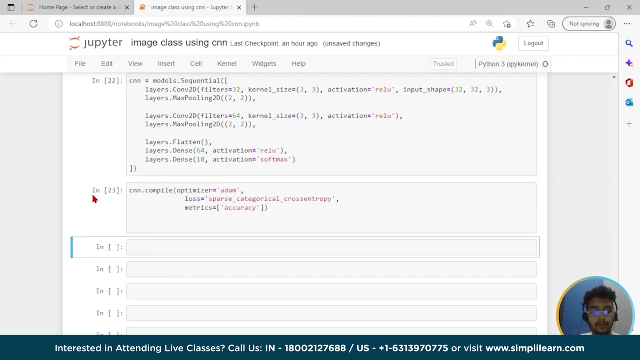 and comma. i will write here: matrix equals to Qresy. run this, okay here. same goes for you. okay, loss. what can i do? i will rewrite this. okay, now let's check cnn model for the 10 epochs. okay, let's see, the accuracy is increasing or not? 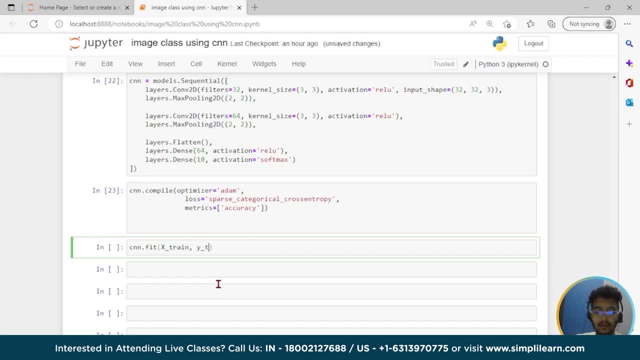 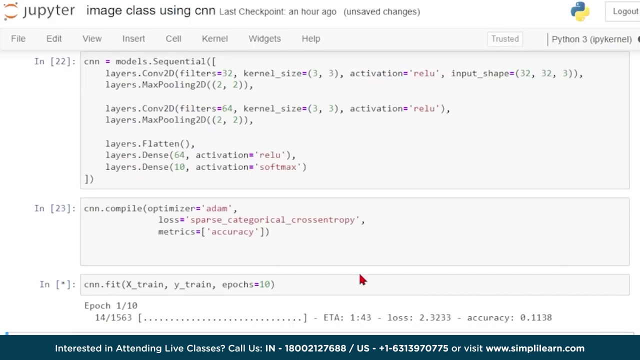 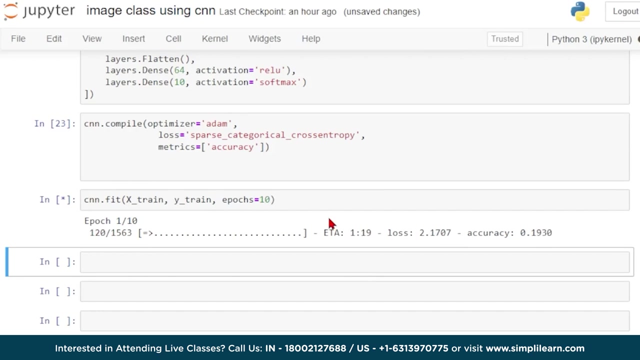 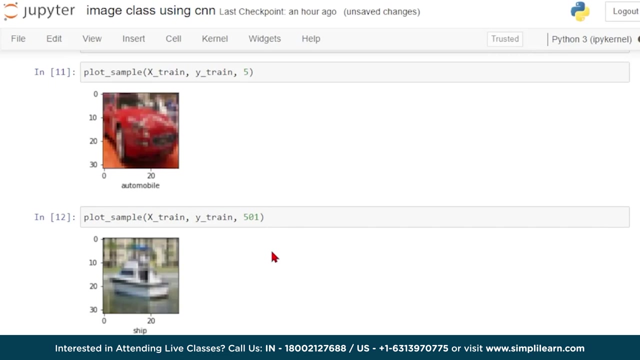 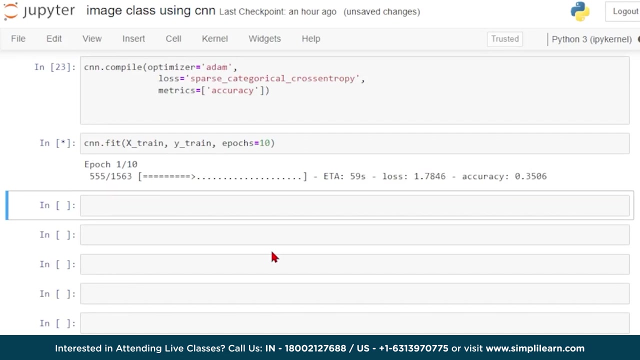 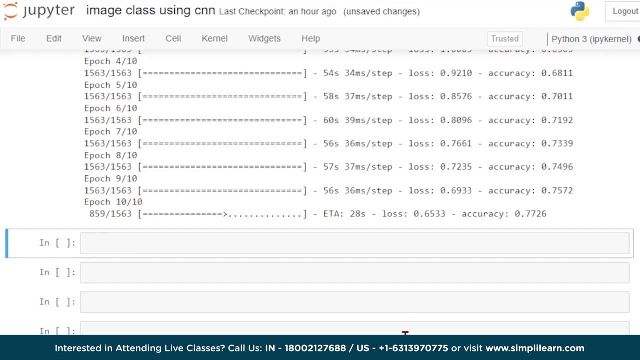 let's go. train comma y, underscore train box. also, it is started. it will take less time than the previous one. okay, see, if you want this whole code, you can comment down the same. okay, so after completing this i will get back to you. so it is almost done. 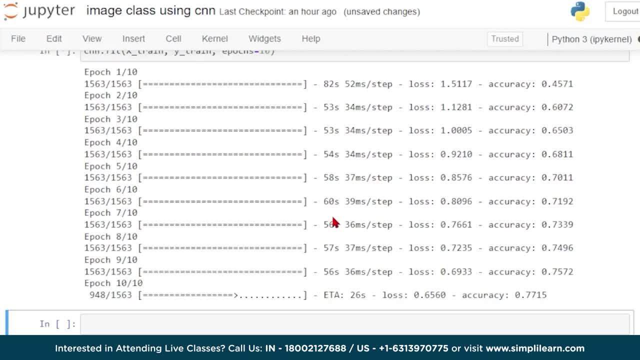 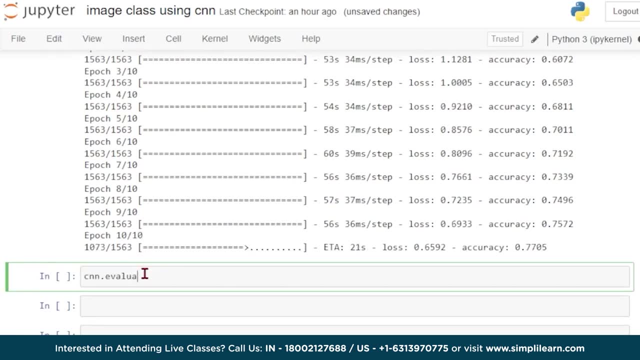 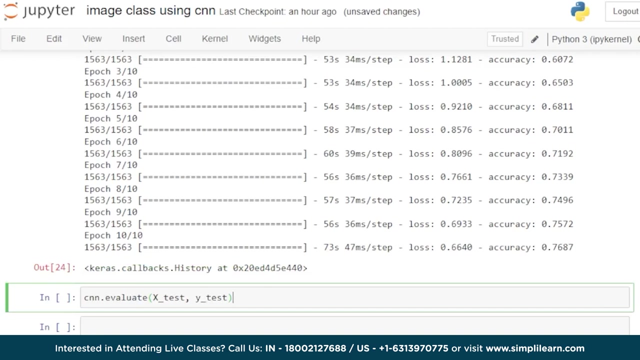 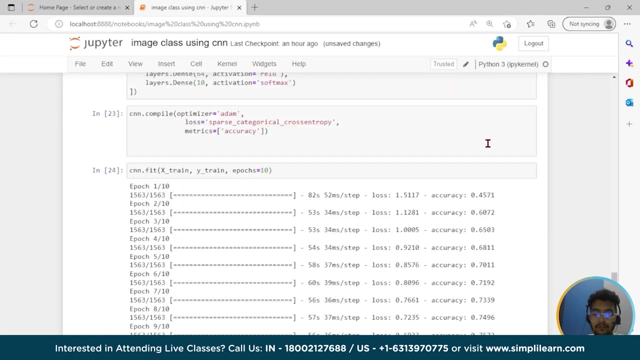 like 27 seconds for the 10 epochs. till then let me write cnn dot: evaluate x underscore test. comma y underscore test. okay, so with cnn the end five epoch security was around like 70 percent and which is a significant improvement over ann. okay, and then we have like just 49. 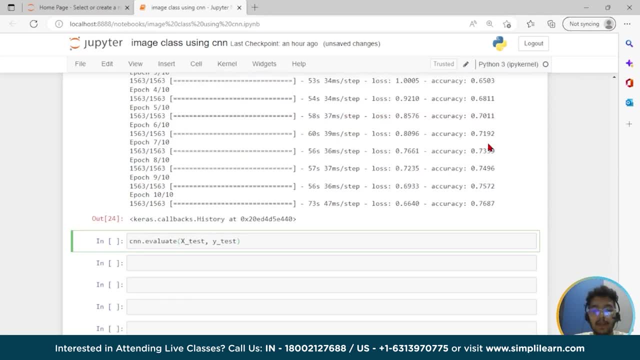 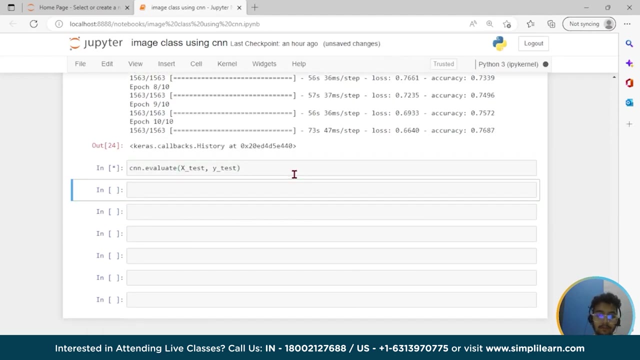 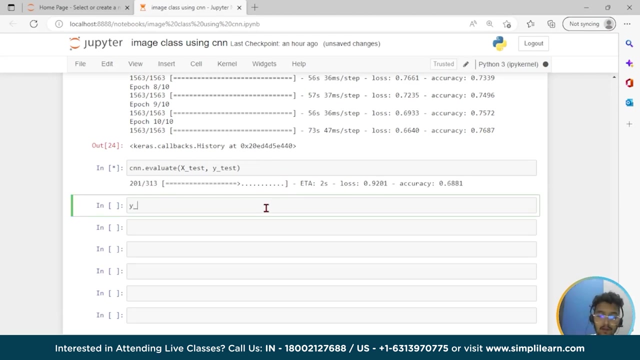 okay, and cnn's are the best for image classification and gives the superb accuracy. also, computation is the much less compared to simple ann, as max pooling reduces the image dimension while still preserving these features. okay, so let me run this. take some time till. then i will write y underscore. 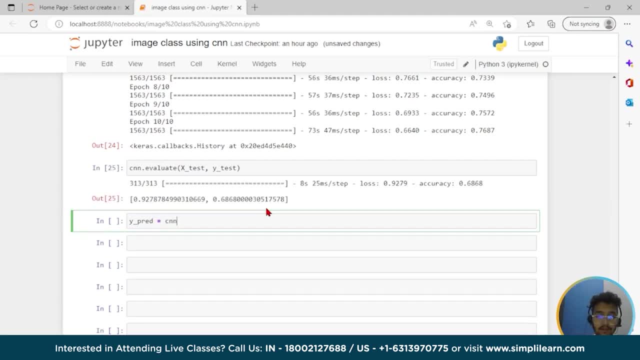 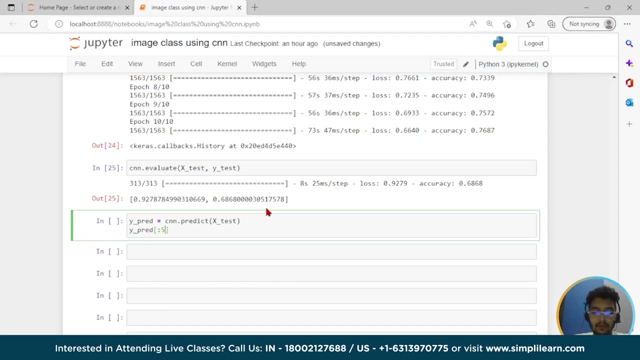 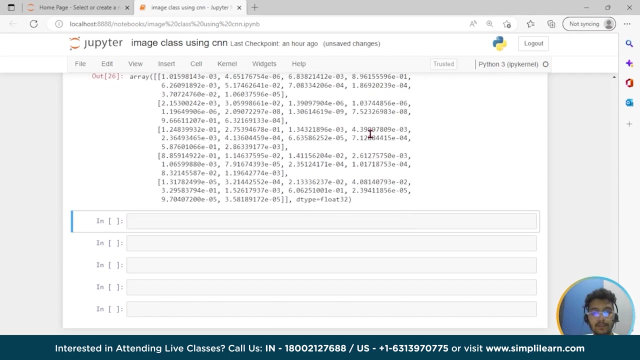 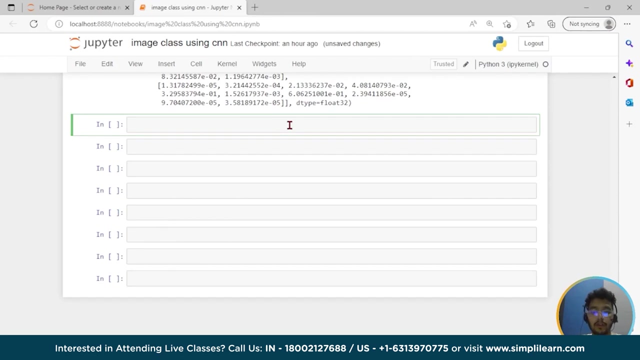 prediction equals to cnn, dot predict and x underscore test. okay, then i will write a y underscore prediction, then column five. let me run this so you can see the accuracy and all the array. okay, yeah, so let's. classes goes to np, dot, arg, max element or element. 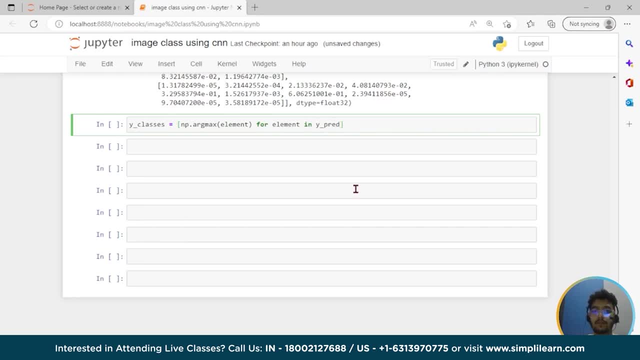 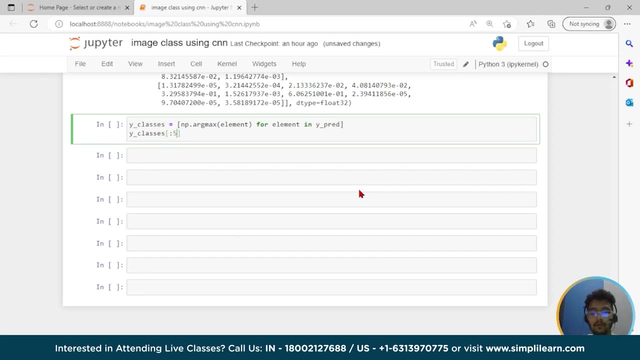 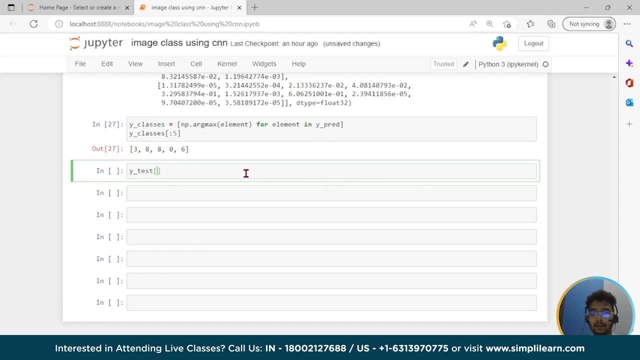 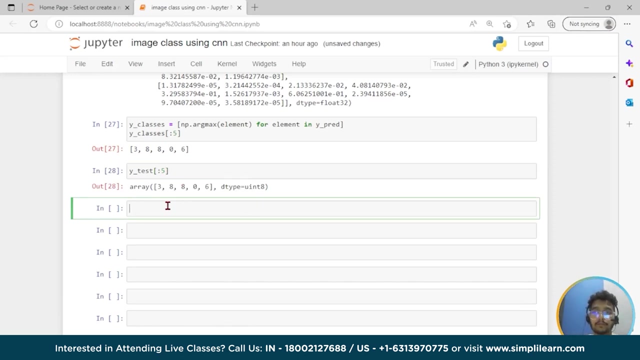 in y prediction. okay, then y underscore classes. then these are the number of classes. then y underscore test is column five. these are the array, so it's converted into area. then now let's see the. it is predicting right image or wrong image. okay, by not with the training data here. 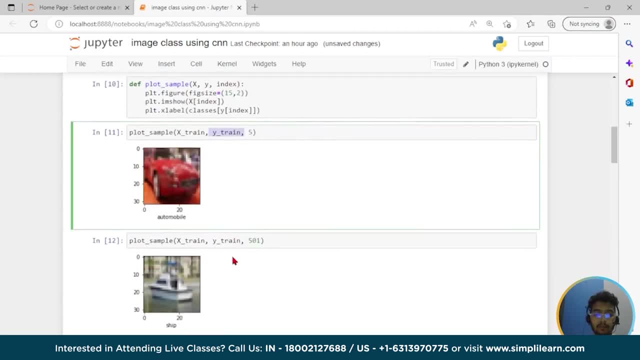 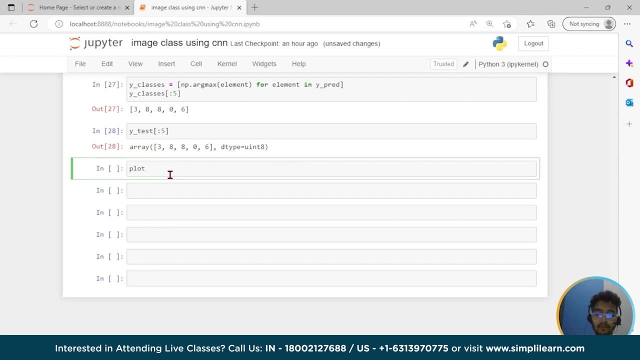 we predict from the training data y-training x-train. okay, now let's predict the training data y-training x-train. okay, now we will predict from the test data. so here i will write plot underscore sample, then x underscore test comma, y underscore test, and you can write the random one. so here i will. 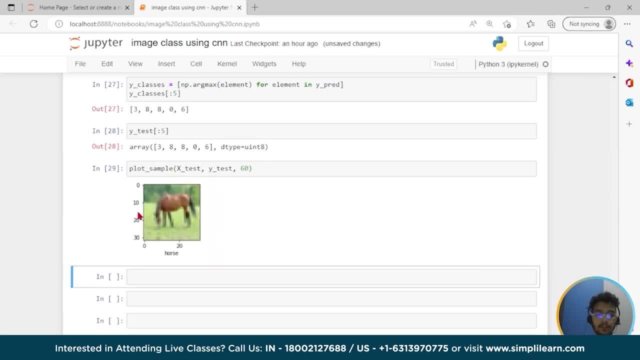 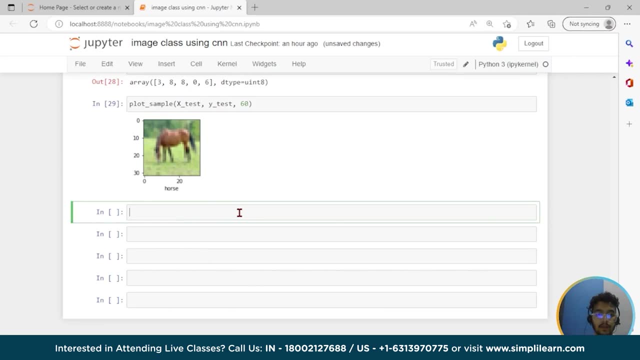 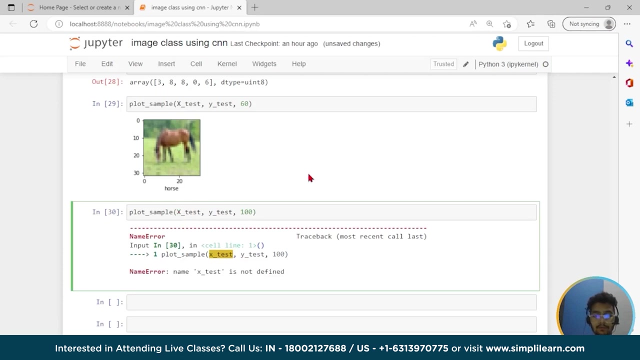 write 60. let's see, so you can easily see here this is odd and it is predicting right horse. and let me okay plot sample. then: x underscore test comma. y underscore test comma 100: okay, let's enter. okay, x is capital. yeah, so you can see. this is dr. okay, so 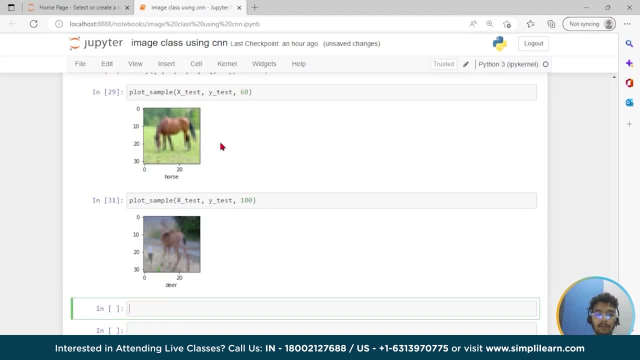 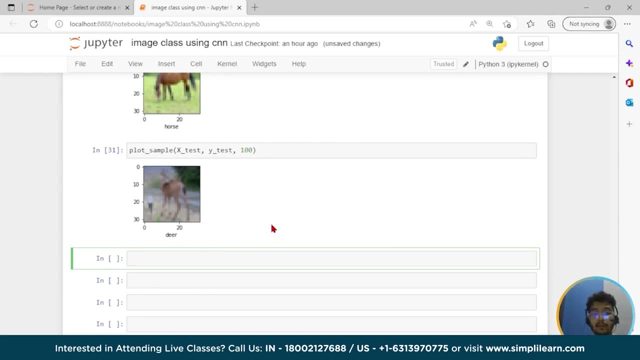 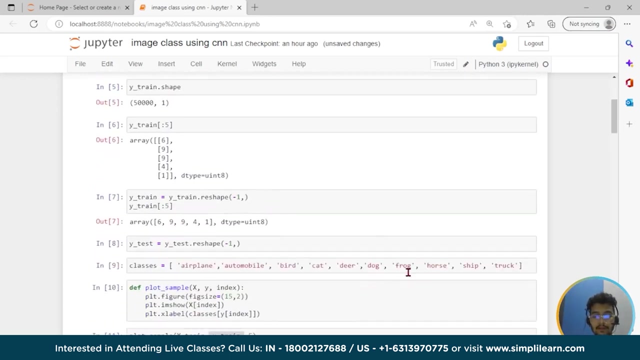 our model is predicting the correct image. okay, then, what we like. let's see it is predicting the right class or not. okay, we made the classes like random classes. okay, where are these? these? so let's see. it is predicting right or wrong. okay, for that i have to write classes. 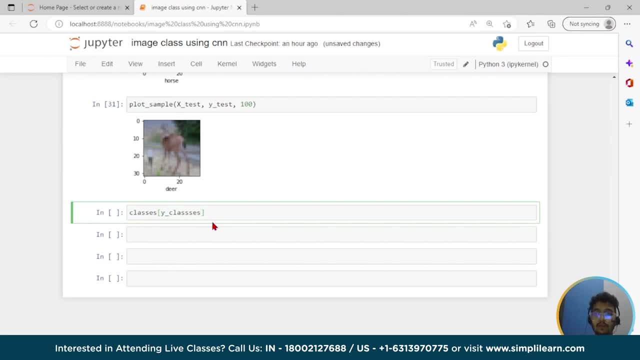 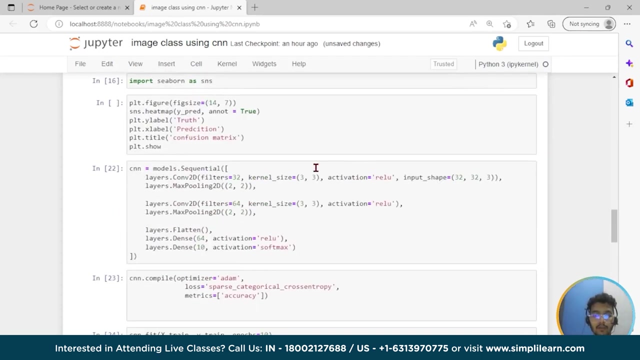 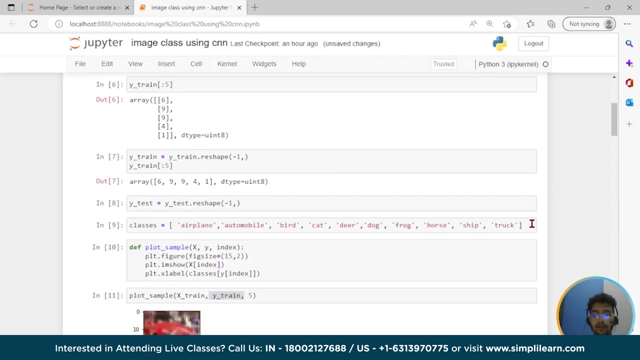 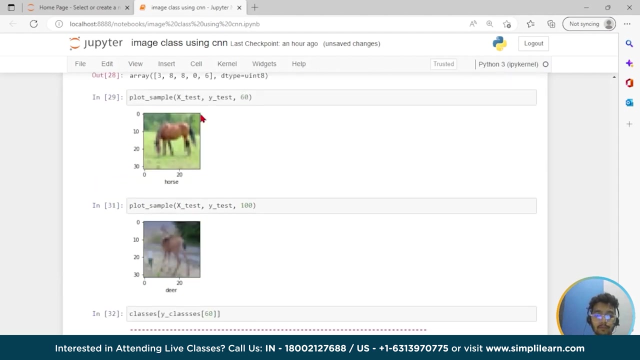 y underscore classes. yes, like which number? 60, okay, 60.. the 60 is not defined because like number of classes, okay, okay. so there are one, two, three, four, five, six, seven, nine, okay, zero to nine. i can choose. so here what i will do. i will take this small one, i will five, okay, this is frog. 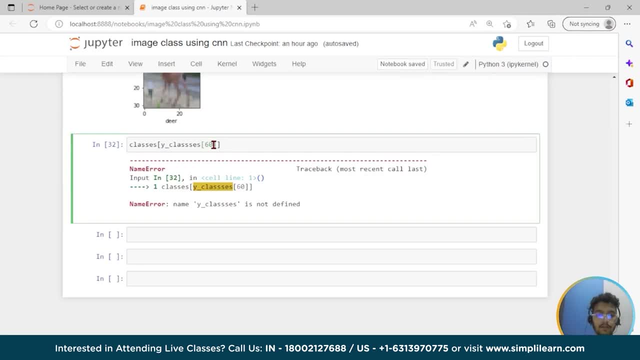 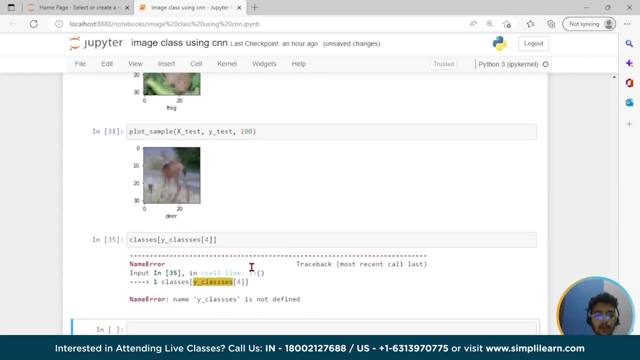 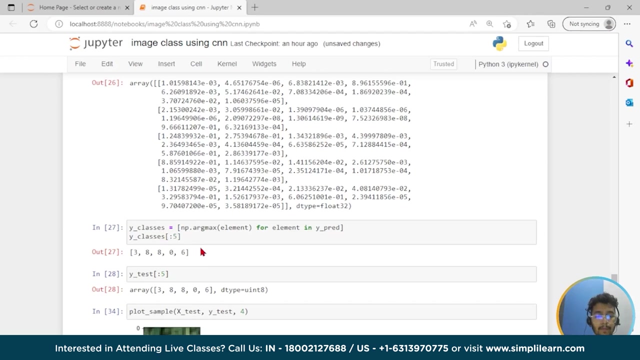 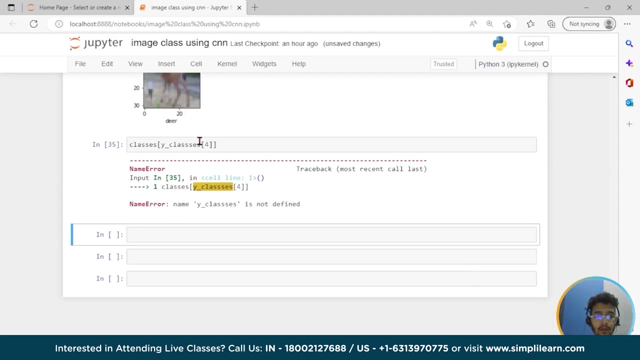 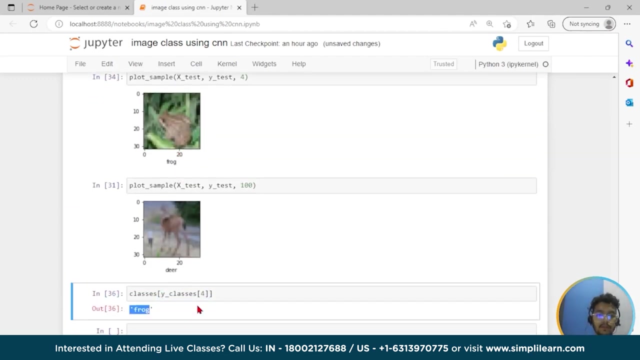 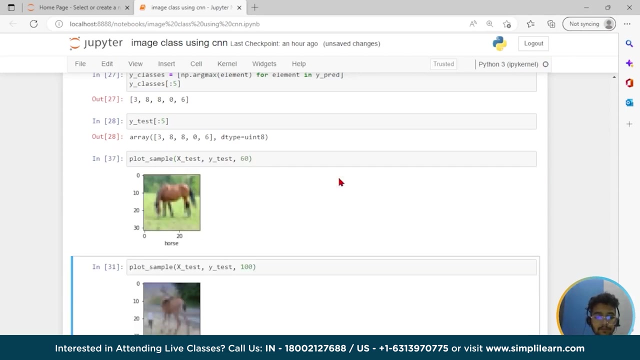 it's frog, right, so i will take instead of 60. here i will see: frog. okay, y class is not defined. y underscore classes is defined. see, okay, there are three s. yeah, so, as you can see, frog, this is frog. so our classes depending, right. so here i will write it again like 60 it was horse and let me write here 60. 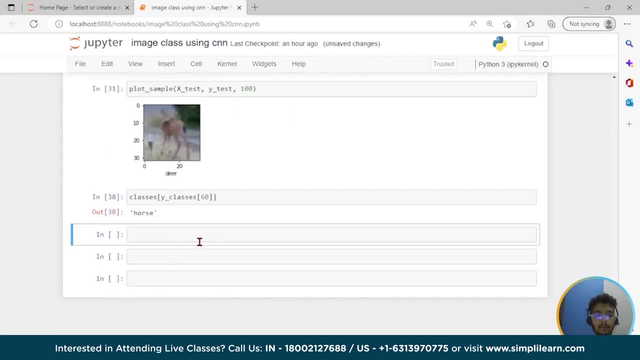 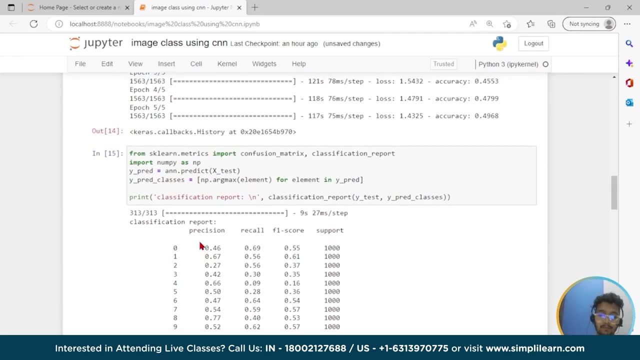 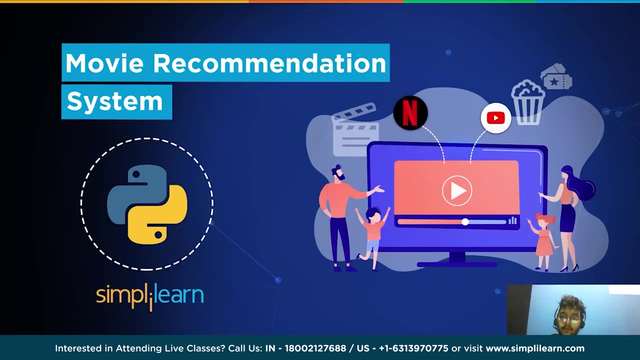 you can see the right prediction. okay, so this is what- how you can you do image classification using cnn. i hope you guys must have understood this concept like how to do image classification using cnn. in today's session, we will go through what is movie recommendation system. after that we will 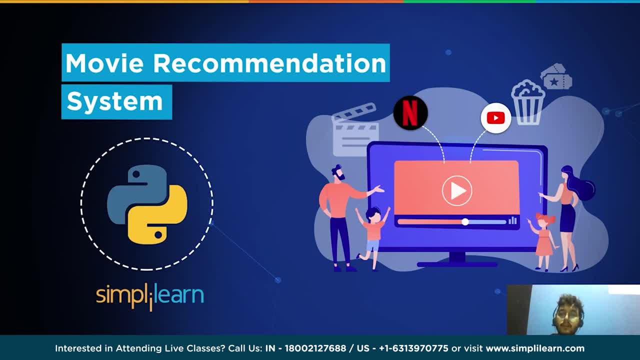 see how movie recommendation system work. moving forward, we will see filtering strategies for movie recommendation system and at the end we will see hands-on lab demo like how to create movie recommendation system using python and how to create movie recommendation system using python in detail. we already have data set with us. we will perform different function and implement. 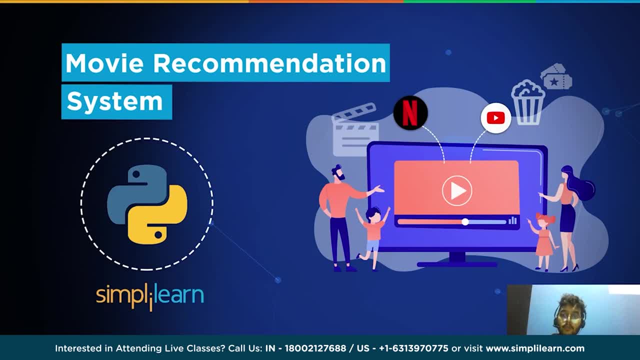 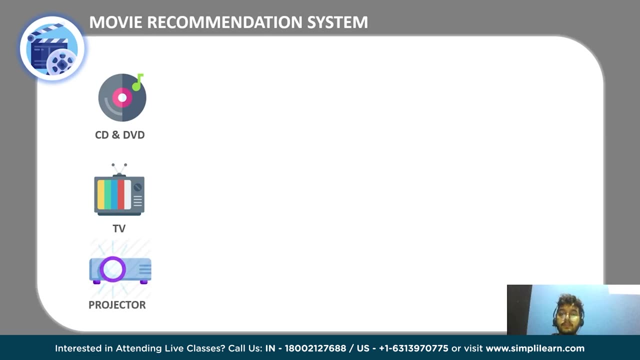 a movie recommendation system using python. before we move on to the programming part, let's discuss what is movie recommendation system actually is and proceed further for the same. so renting cds and dvds, reading local tv, listenings, watching film strip projectors or recordings- all of this is a thing of the past. today, all of the world's biggest film collections, 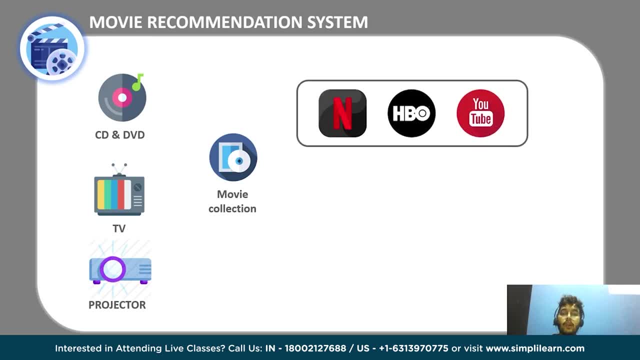 have been digitized and moved to the online streaming services like netflix, hbo or youtube. these platforms can now help us with what is possibly the most difficult task of all: choosing a movie. they have been enhanced with ai powered capabilities. well, that is no longer a. 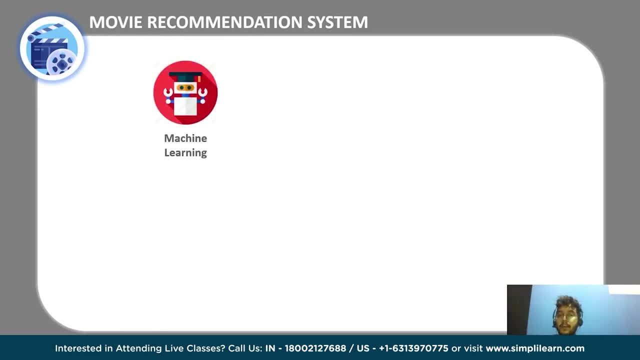 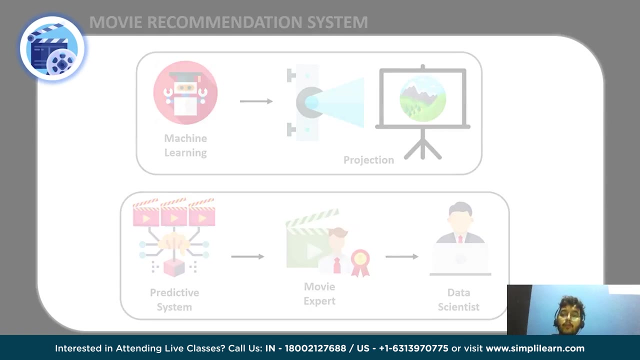 concern for you. it is finally time for machine learning to put its skills on display in the modern cinematic landscape to create advanced predictive system for true movie action. so let's take a look at what is movie recommendation system. movie recommendation system is a system that uses machine learning to predict or filter user. 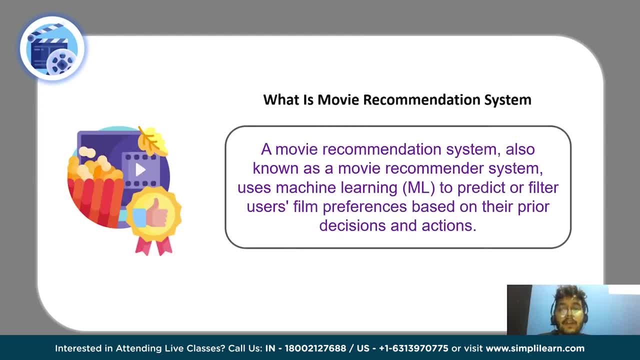 feel, preferences based on their prior decision and actions. it is an advanced filtration system that anticipates the consumer in question potential like selection for a domain, specific item, a movie. so after seeing what is movie recommendation system, we can now move on to the next part of the video. 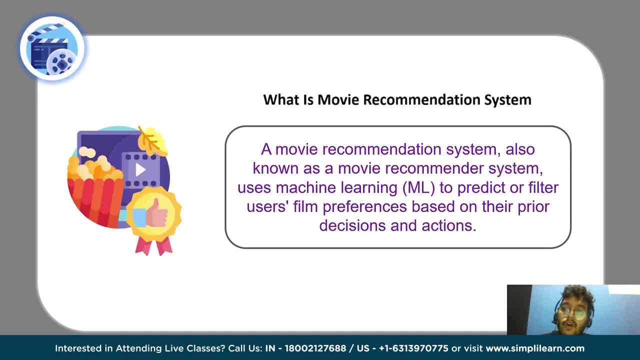 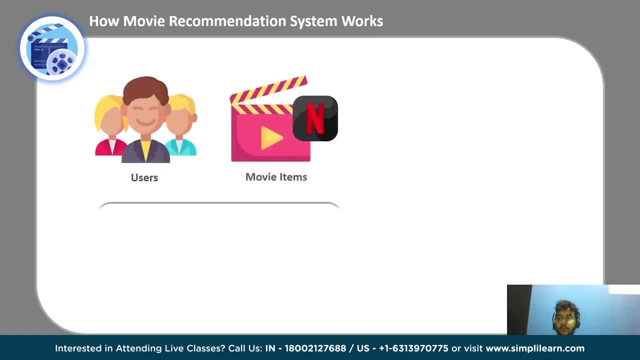 after seeing what is movie recommendation system, let's move forward and see how movie recommendation system actually works. a movie recommendation system fundamental idea is a pretty straightforward. every recommender system primarily consists of two components: users and items. user receive more prediction from the system and the actual movies are the products filtering and predicting only. 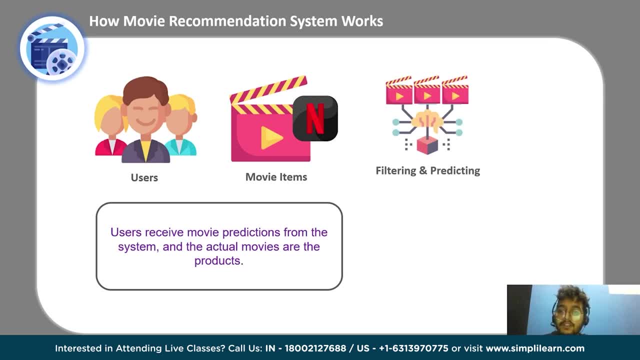 the movies that are matching users is most likely to wish to see. in the main objective of movie recommendation system, the user information from the system database is used by the ml algorithm for these recommendation system. based on information from the past, this data is used to forecast the user in questions behavior in the future. data should be handled by experts because 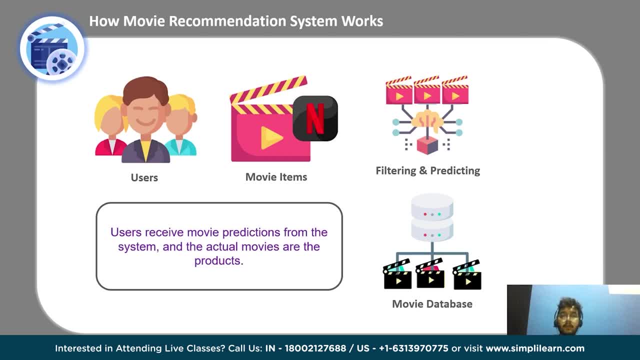 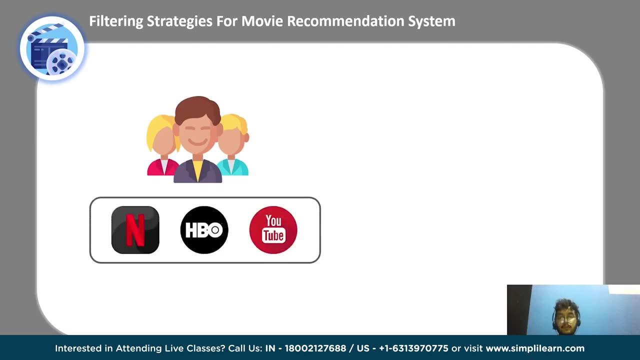 it is so crucial to ml projects, including the movie recommendation system. after seeing how movie recommendation system works, let's see some filtration strategies for the movie recommendation system. to assist user in finding the most relevant films, movie recommendation system employ a variety of filtration techniques and algorithm: the content based filtering and the collaborative filtering. 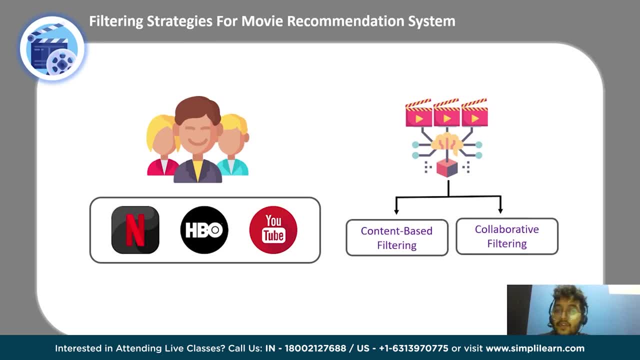 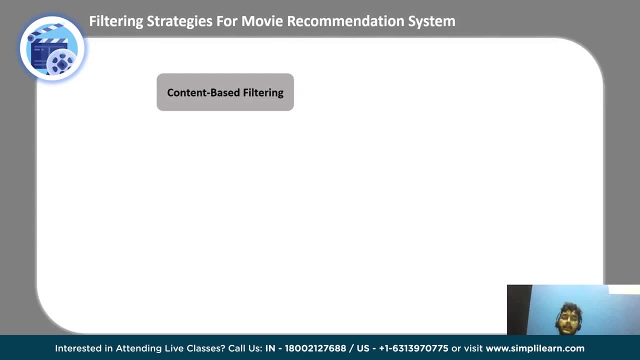 system. subcategories of the ml algorithm used for the movie recommendations are the most well liked ones. filtering based on content or content based filtering: a method of filtering movies in a movie recommendation system that makes a different movie recommendation system. and the content based filtering system. that makes a different movie recommendation system. and the content based filtering system. 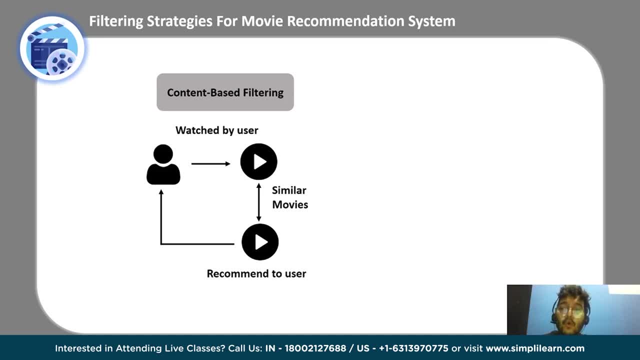 this information, which is taken from the just one user, is quite important in this case. this technique uses an ml algorithm to suggest movies that are comparable to the user's past choices. therefore, the information about the prior movie choices and likes just one person is used to generate. 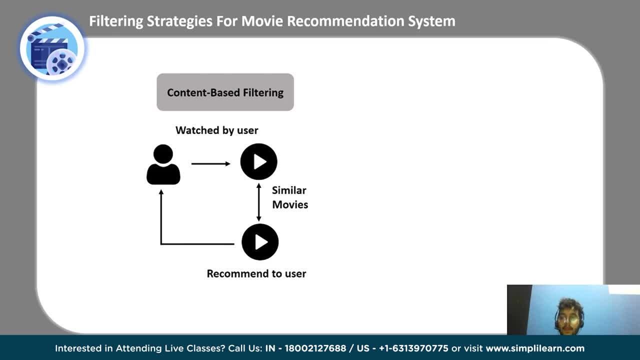 similarity in content based filtering and the second one is collaborative filtering, as the name techniques is based on the interaction between the relevant person and the other user. for the best outcomes, the system contrasts and compares these behaviors. it combines the film choices and uses patterns of several people like. there are two types of collaborative filtering algorithm: the 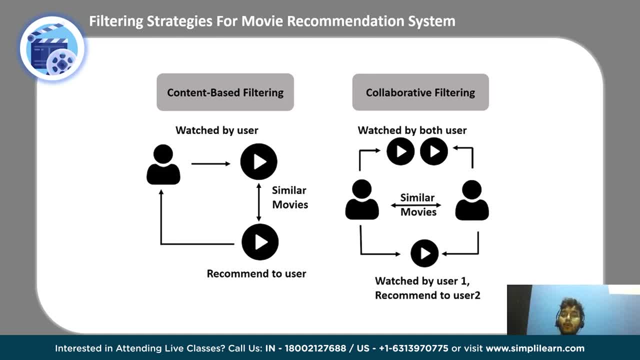 first one is collaborative filtering based on users. the goal is to find patterns in target users and other database users, like movie preferences. and the second one is collaborative ideas. the third one is item based filtering. the fundamental idea behind this is to find comparable products, products like movies that target users rate or interact with after seeing. 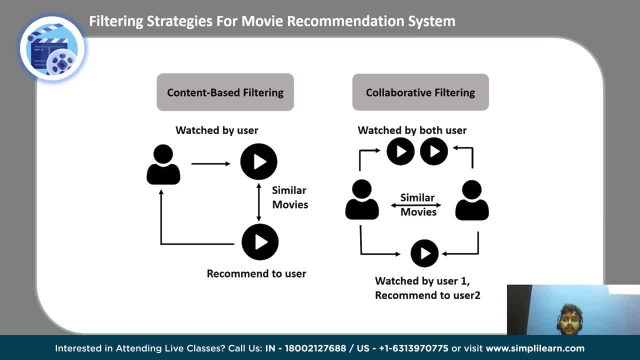 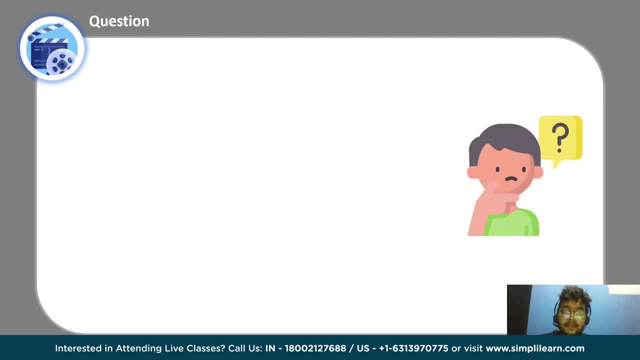 the filtering strategies for movie recommendation system. so here is one question for you guys. i will give you one minute for this. you can comment or you can give answer in chat section so i can see if the answers given by you are right or wrong. i'm repeating again. so here is one question for you guys. 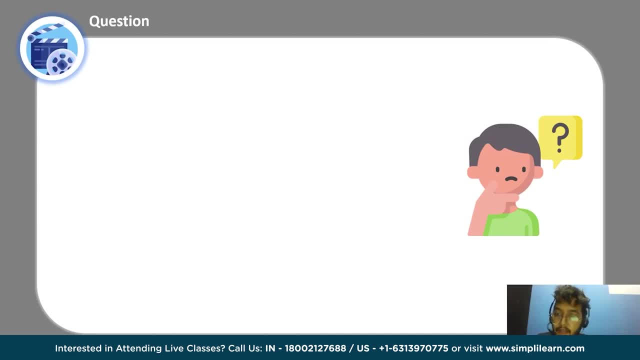 i will give you one minute, exactly one minute, for this. you can comment or you can give your answer in chat section so i can see if the answers given by you are right or wrong. so the question is: which is the best language for machine learning, programming? which is the best language for machine? 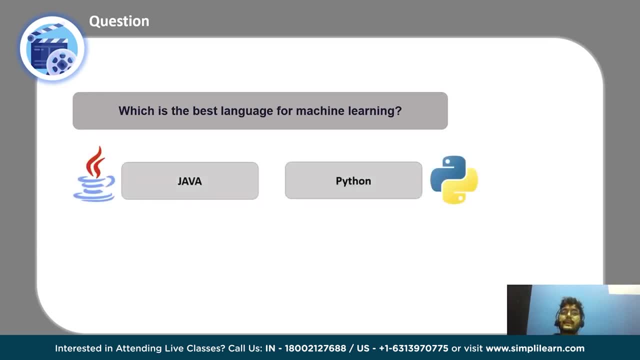 learning. the first one is java, the second one is python, the third one is r language and the fourth- so this is the question i am repeating again- which is the best language for machine learning? the option one is java, second, python, r language and c plus plus. so i'm starting timer of one minute. 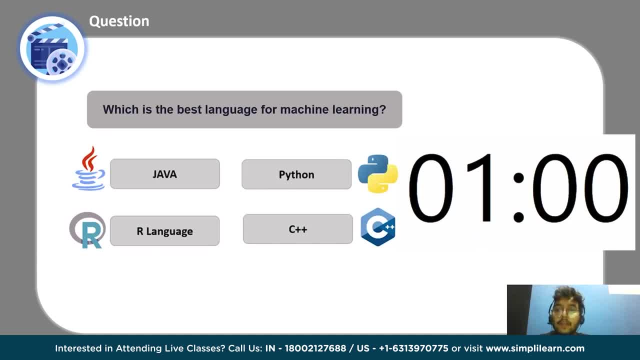 just type your answers in comment section or in a chat section. do let me know your answers, please. i want that everyone should participate in this and make this live session interesting. so i am starting timer, so your time starts now. please, guys, do let me know your answers in chat section or in you can comment down. 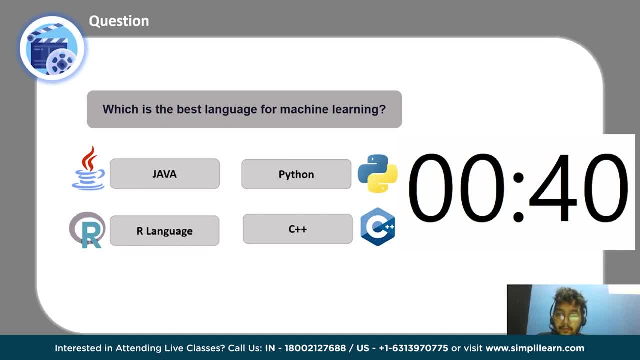 42 seconds to go. you can comment or you can give your answer in the chat section so i can see if the answers given by you are right or wrong. 30 seconds more, which is the best language for machine learning. you can give your answer chat section or you can comment. 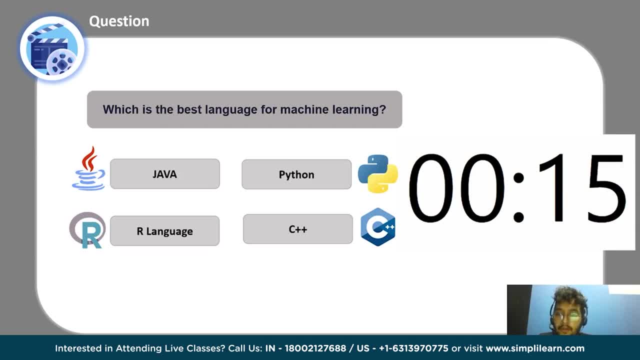 so i can see if the answer is given by you are right or wrong. guys, come on please. i want that everyone should participate in this and make this live section interesting. come on, guys. five second more. one yep time up. so time is over. we will give reply those who gave correct answer. 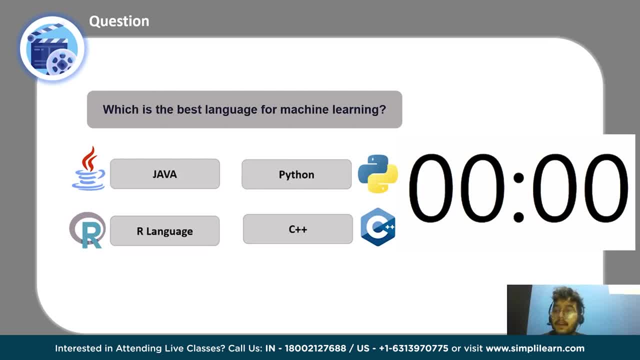 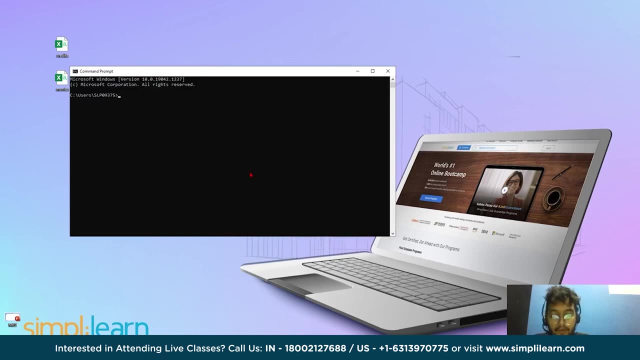 and those who didn't give correct answer. we will give you a reply with the correct answer. so now let's move to our programming part. to perform movie recommendation system using python. so first we will open command prompt to write command to open jupyter notebook. so we will write. 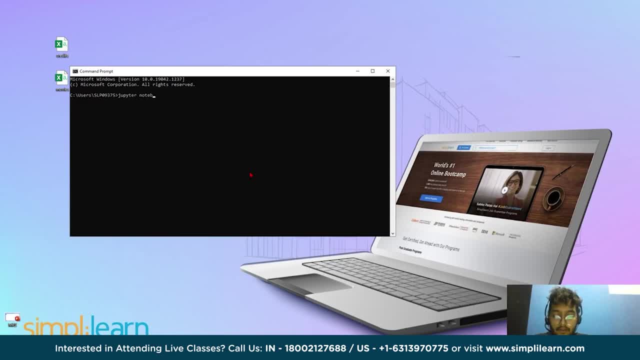 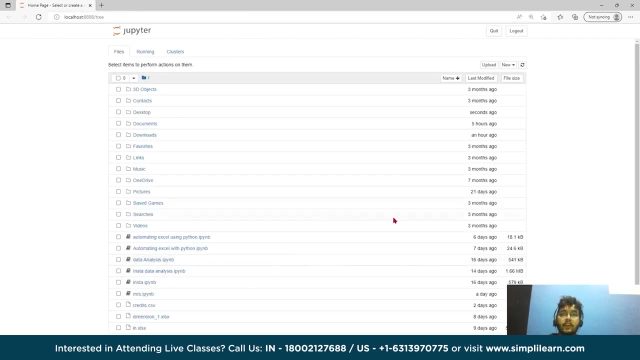 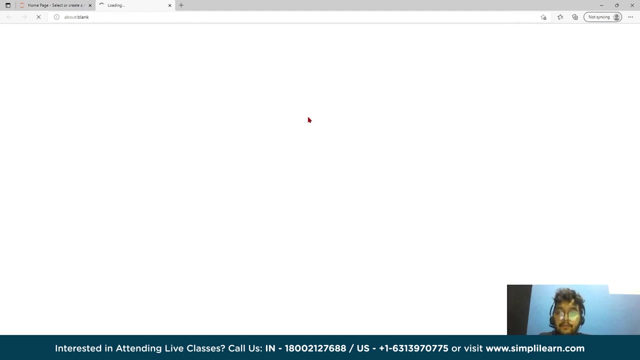 jupyter notebook, press enter. so this is the landing page of jupyter notebook, and select here new, new python file. so this is how jupyter notebook ui looks. look at your final super lagger llevavu over here. we applied jupyter目 taxonomic normal ui tutorial to that. let me those who have watched web 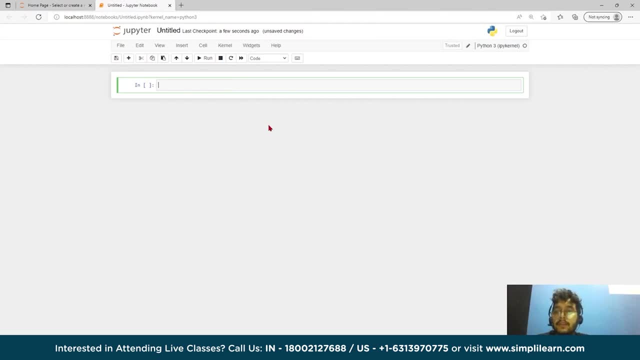 So at first we will import some major libraries of python which will help us in mathematical functioning. So the first one is numpy. Import numpy as np. So numpy is a python library used for working with arrays. It also has a function for working in the domain of linear algebra and matrices. 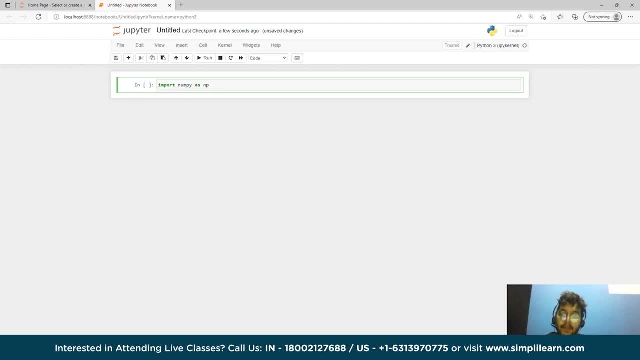 It is an open source project and you can use it freely. Numpy stands for numerical python, So here np is denoting numpy, So we will import the next library. import pandas as pd. This should be space, yap, So pandas is a software library written for the python programming language. 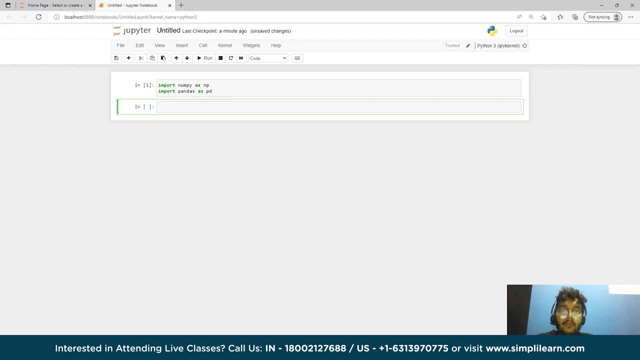 For data manipulation and analysis. In particular, it offers data structures and operations for manipulating numerical tables and time series. So after importing libraries we will move ahead and import data set. So for importing data set we have to write like: we have two data set with us. 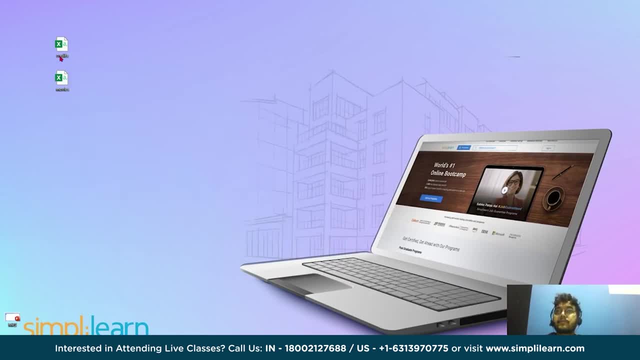 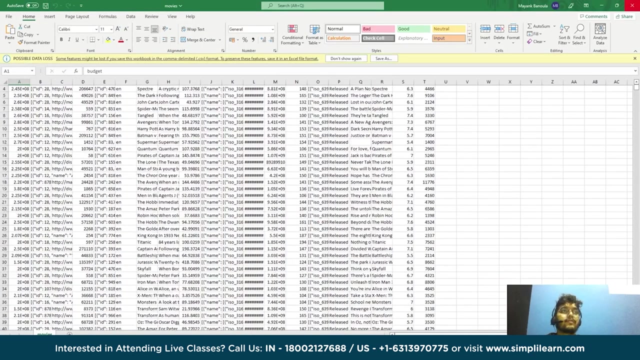 Let me show you the data set. We have two data set with us. The first one is credits- This one- And the second one is movies one, Movies one. So don't worry, you can get these data set link in the description box. 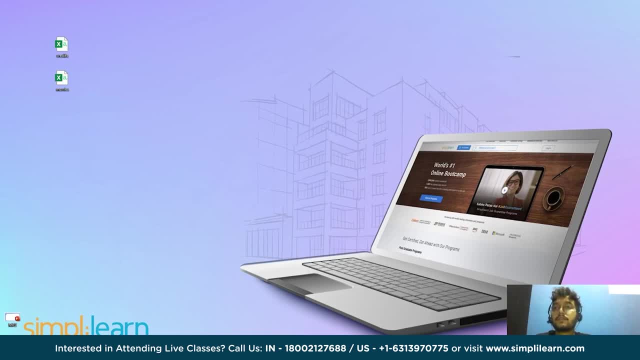 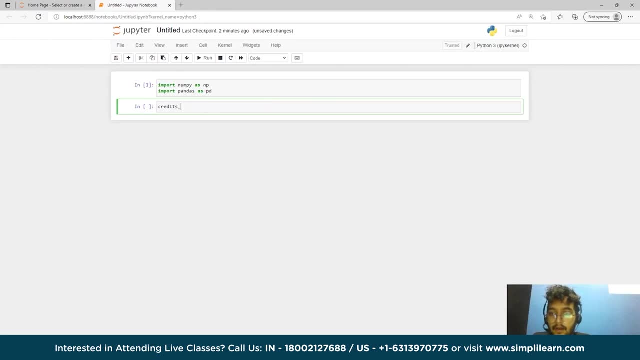 So let me write credits, Credits, Credits, Let's go. data frame equals to pdread, underscore, csv. Here you have to give your location of the data set: creditscsv. The second one is movies- Let's go. data frame. This is for movie data frame. 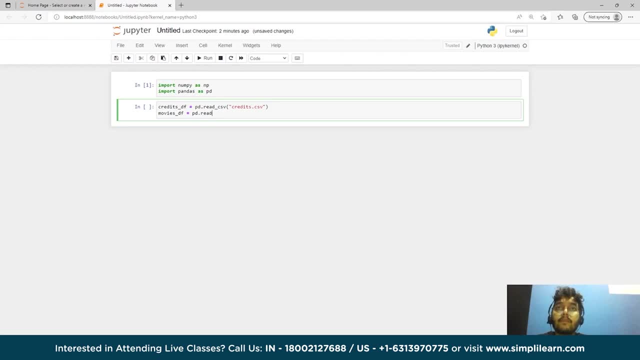 So here you have to give the movie location movie data set, location movies, dot, csv. Okay, everything seems good, Let me run this, Yeah Here. pd is for the pandas library, Read is used for reading the data set from the machine and csv is used for the type of 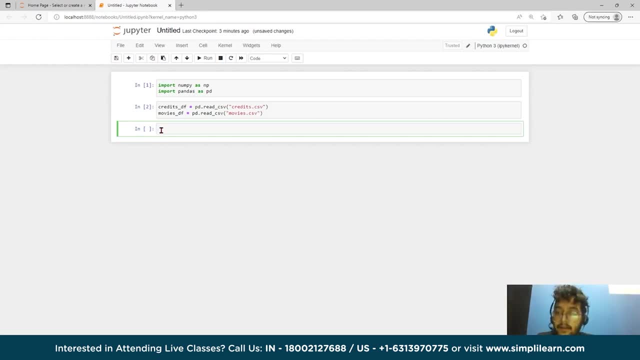 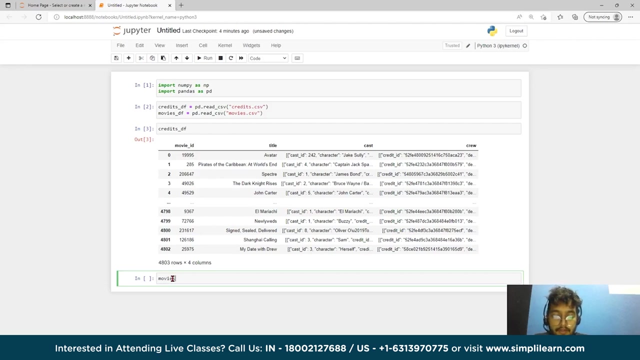 file which you want to read. So after this, let's write code to see the data set. So we will write here credits, underscore df and we will run it. So this is our, so this is our credit data set And next one is movies underscore. 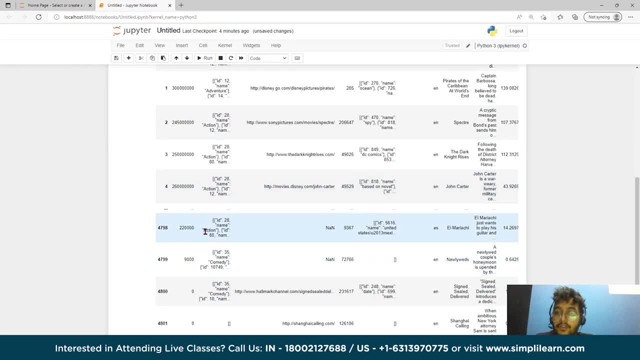 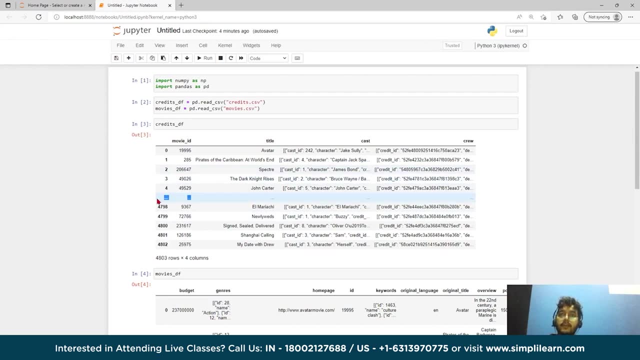 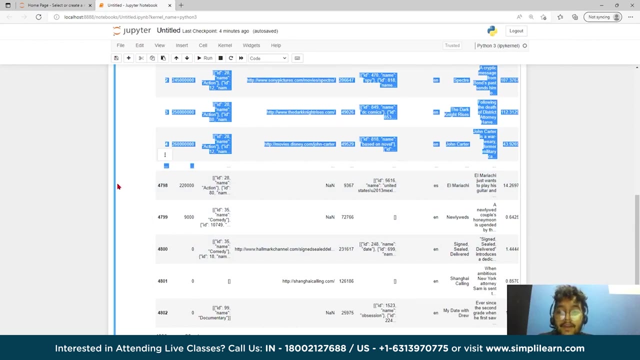 So this is our movie data set. So this is how our board data set look like. So here you can see three dots: This one and here also This one. So we are unable to see our full data set. Like what if we want? like full a 4803 rows. 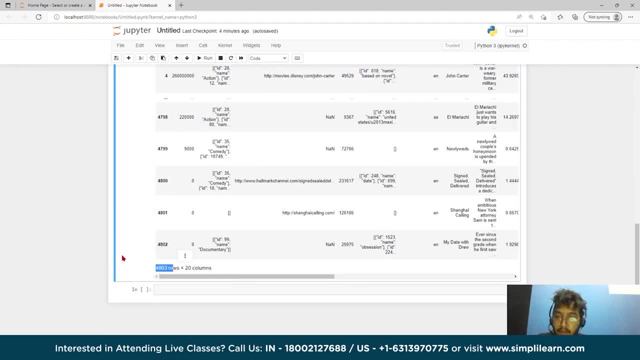 This one. So we are unable to see our full data set. Like what if we want, like full a 4803 rows? So at that case we can write here: PD dot set underscore option: Okay, And here we will write display dot max underscore columns: this: 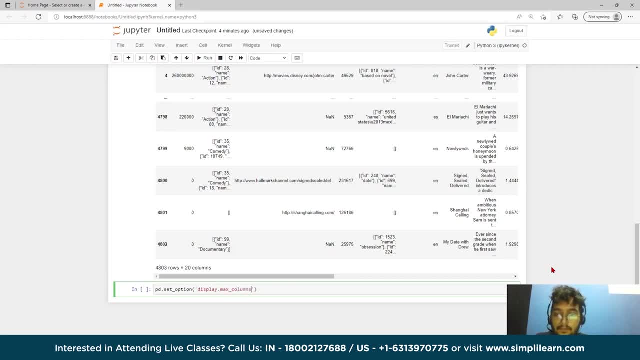 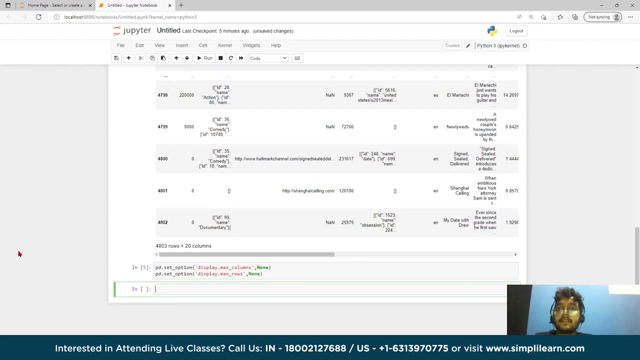 And here we will write display dot max underscore columns this. And here we will write display dot max underscore columns: Okay, So here we will write none same for the rows PD dot set option: display dot max underscore rows none. let's run this. so now, if we will write credits underscore. 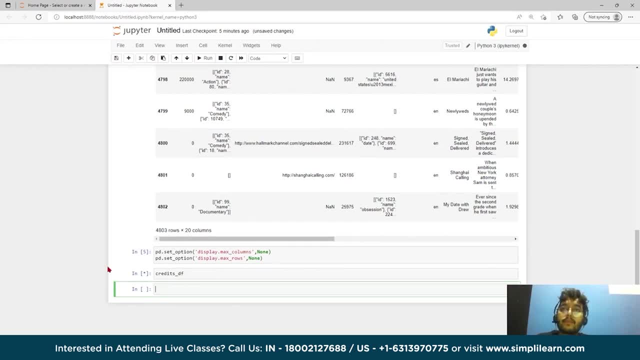 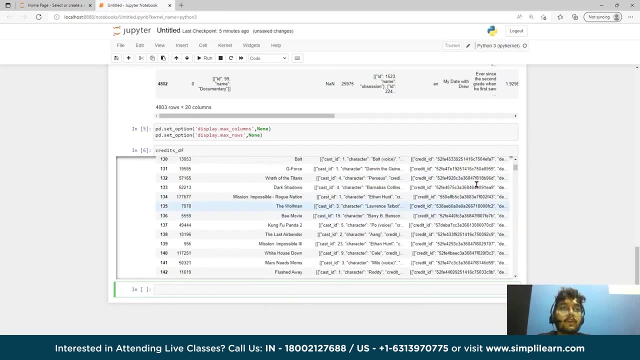 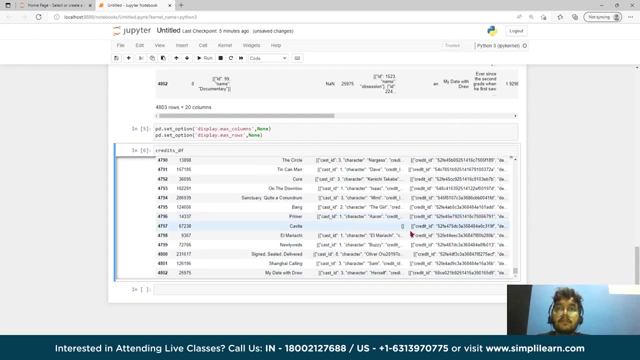 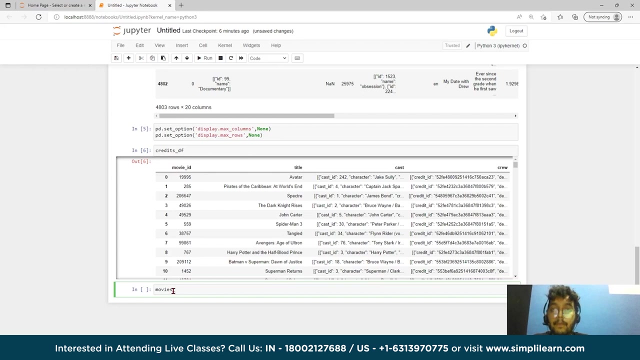 DF, it is running. yeah, now you can see your full data set, like full credit data set, with 4 8 0, 3 rows of 4 8 0, 2 rows, because there is this is starting from 0, that's why. so what about movies data set? 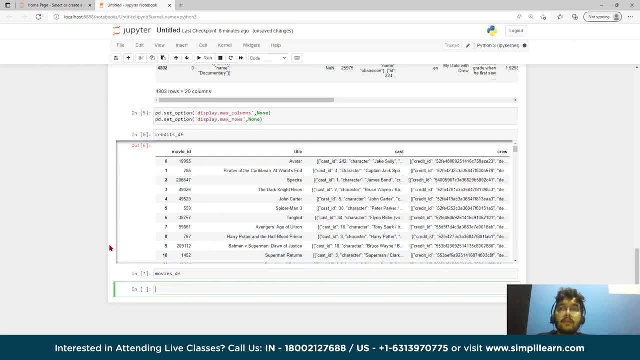 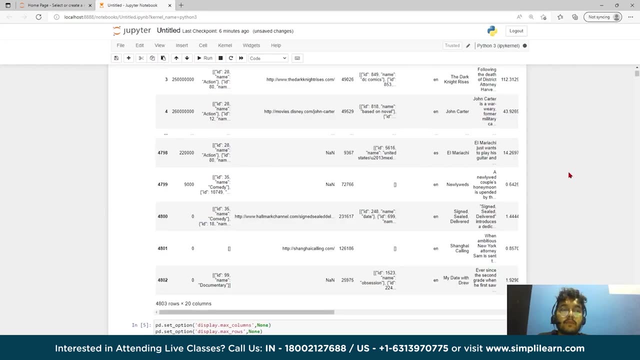 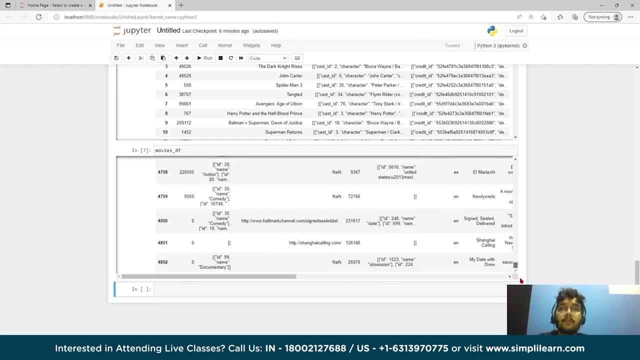 give it running. this is still running. you can see here. so here you can see the full data set, movie data set with 4, 8, 0, 2 rows, or if you want to see only five top rows, so you can write here: credits: underscore DF. 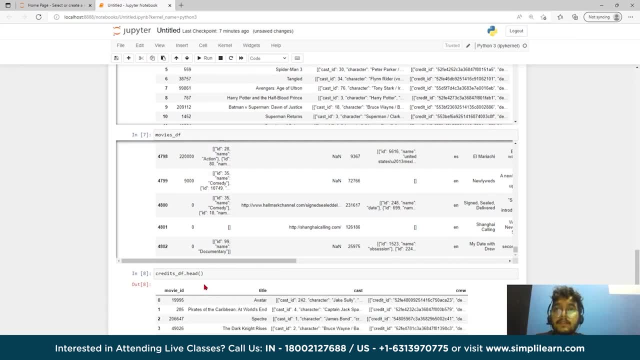 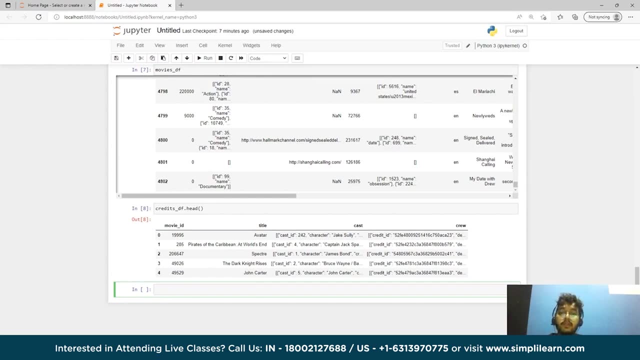 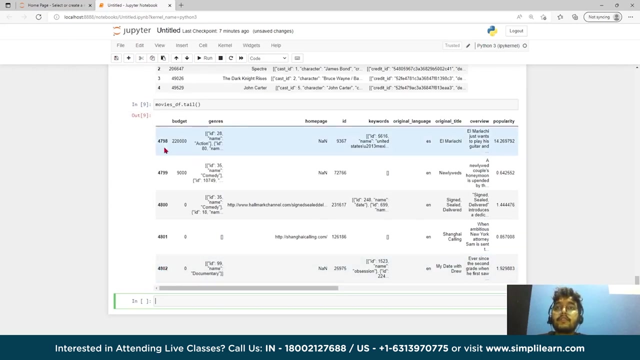 dot head. so by this only five top rows. so from head you we can see our five top rows, and if we will use tail instead of head, we see our last five rows. so here let me do with the movies. one df dot tail, yeah. so here you can see. 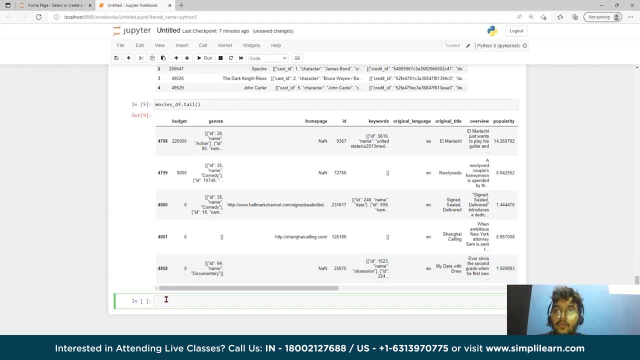 4798, row 4799 till 4802. so with tail we can see our last five rows. so, moving forward, let's merge the credit data set to movie data set, because if we will combine them the confusion will be less and at the end it will be better for us. so we will write here: movies underscore equals to movies. 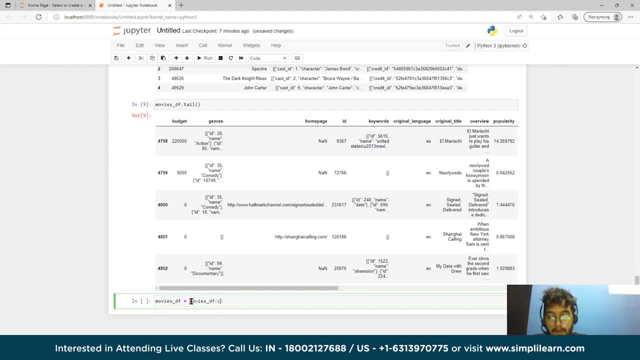 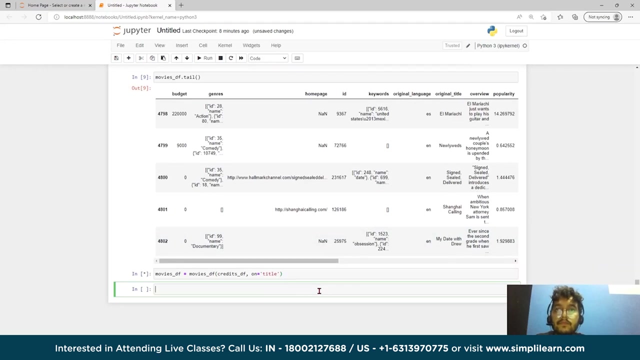 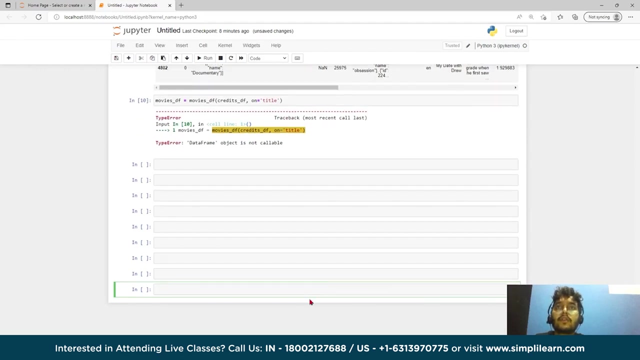 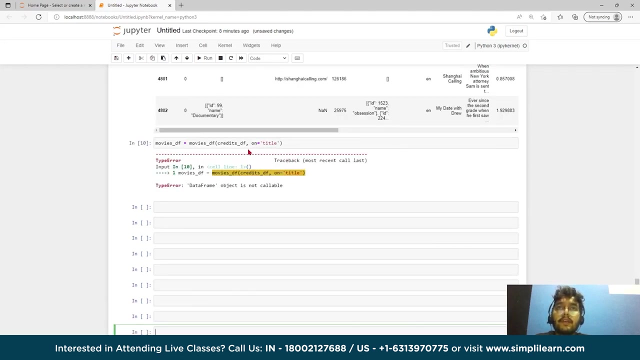 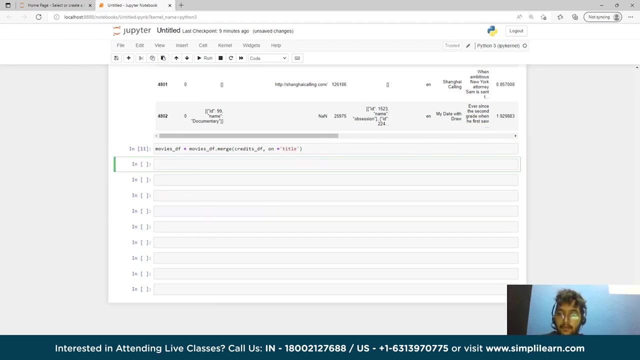 underscore data frame and credits underscore df on it tell: okay, t is small, i guess. yeah, perfect, you title, let me do something something like this: okay, it is saying data frame object is not callable. credits underscore df: okay, and transaction data set: no. get this name correct, sure. 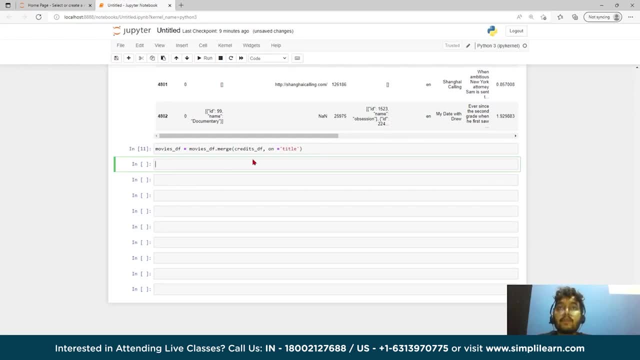 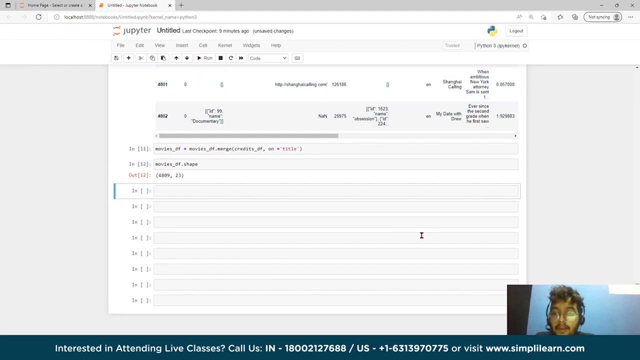 yeah, there you go. so with rgu set we will wait till this point. so keepith our days, zero, what's time? charge kov's charge only one. so movies, underscore, df, dot shape. okay, let's run it: 4809 and 23, 23. but if we see here, 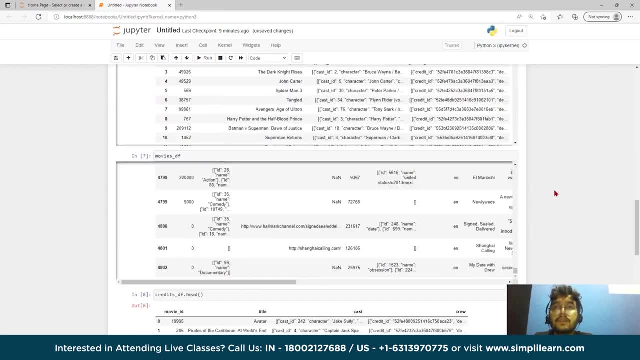 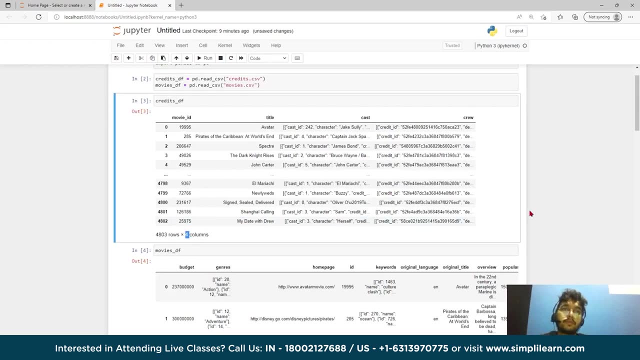 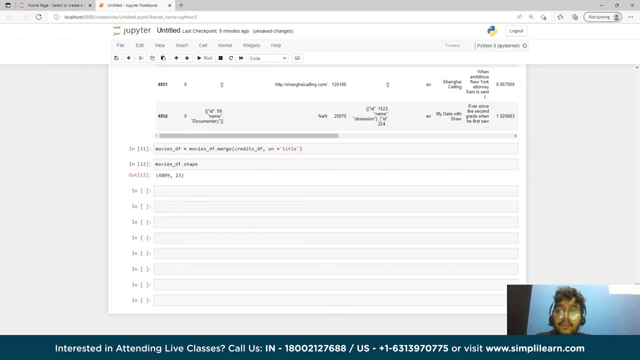 like in movies data set. so in movies data set, here here, yeah, yeah, there are 20, and in here we are four columns in credit data set, so like. so you will be thinking that's why not 24, why only 23 columns? that is why, on title- you can see here on title, the titles in both titles are same you. 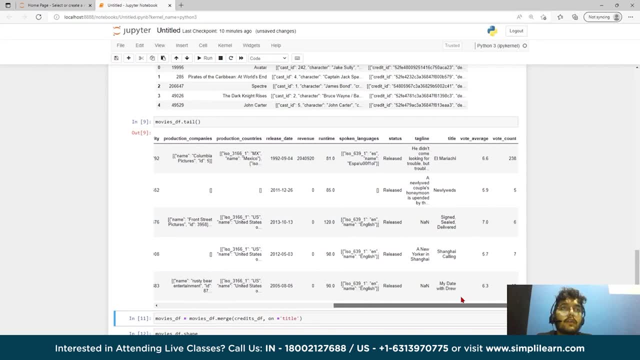 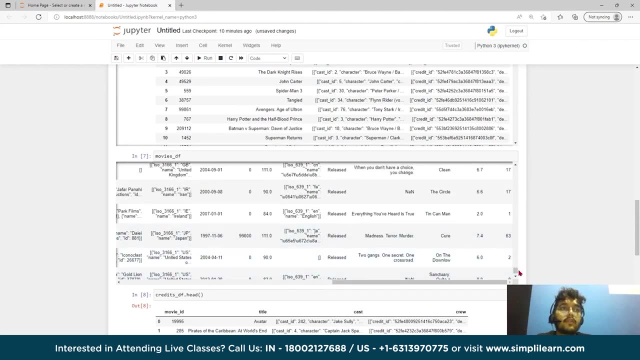 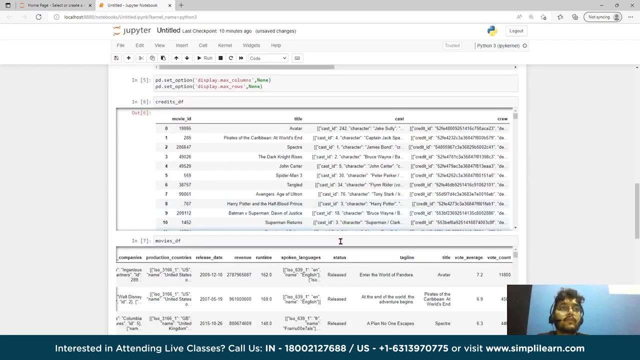 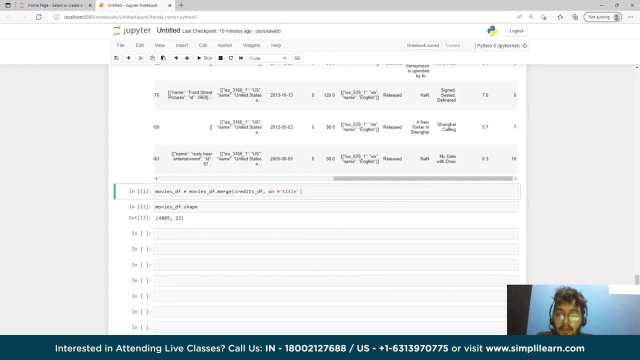 can see here both titles are same in both. okay, let me show you like this: okay, after Pirates of the Caribbean spectra and so on. here you can see after Pirates of the Caribbean spectra and so on. so that is why on title written while merging: so title are same. so, moving forward, let's see our merge data set so we will write only movies. 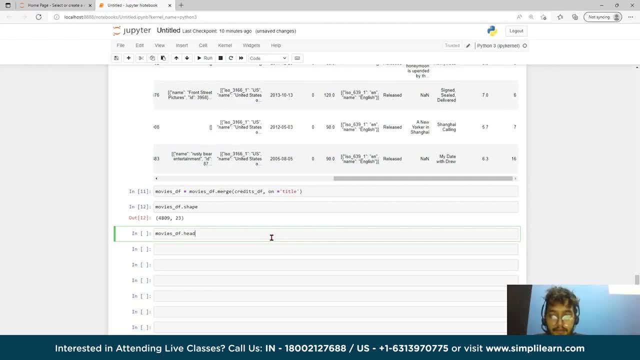 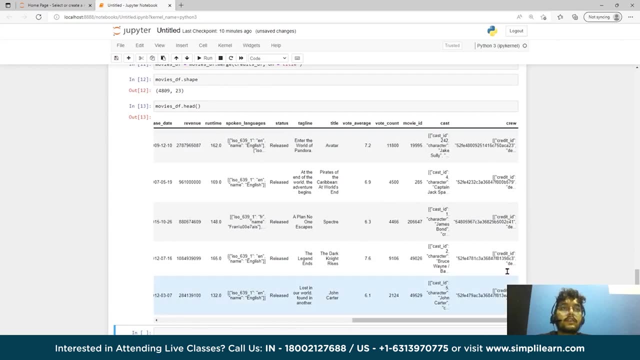 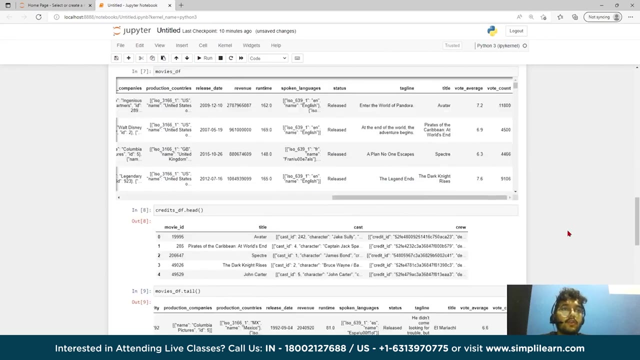 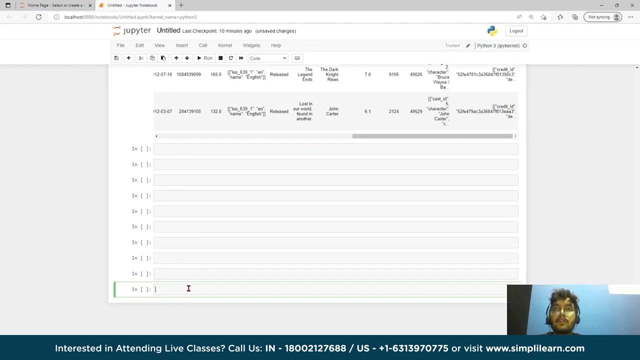 underscore data frame dot head. yeah, so our data is merged. you can see the last cast crew movie ID: yeah, you can see here. movie ID title are the same. they are merged. cast crew. okay, guys, let me give some more for the better view. yeah, so you can see. all columns of credit data set are added to movies one. so moving forward, let's see. 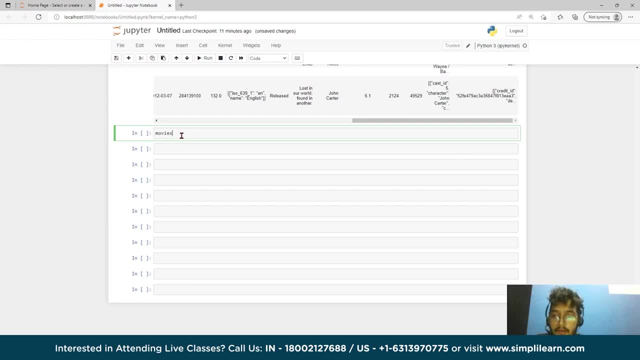 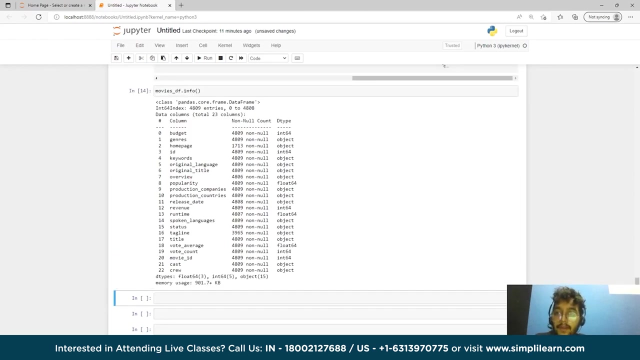 another function like movies, underscore, df, dot info. so by this- yes, you can see. so by this, the data frame information is printed via the info method. the data includes the total number of columns, their labels, data kinds, memory use, rage, index and the number of cells in each columns, like non-null values. note that info method. 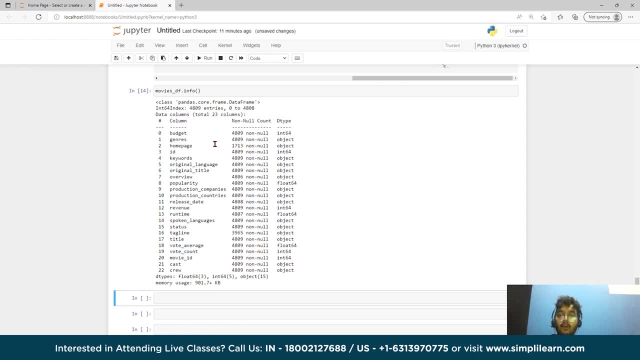 just indeed print the information. so here you can see the. all the information is printed okay, like columns, name and the all null values count, and data types too, like this int object and in which we are working most. so after this, let's move forward and select some main. 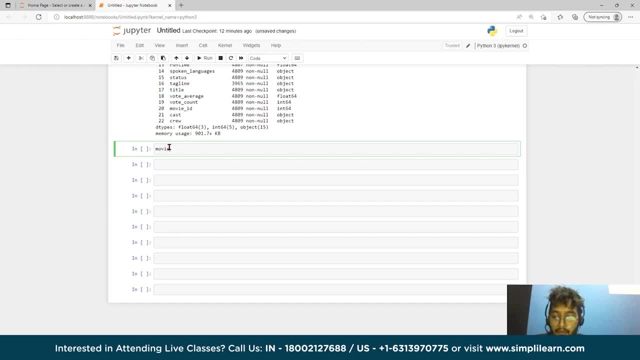 column in which we are working most. so we will write: movies underscore df equals to movies. underscore df title comma, and another one is overview. okay, okay, here we have to like this. yeah, so here we have to write: genre journal is complete and we will work on what keywords. keywords are the main. 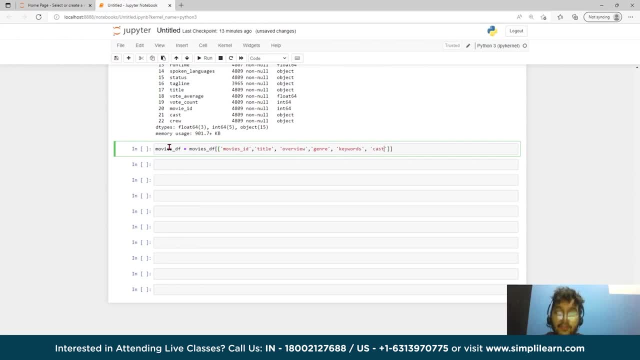 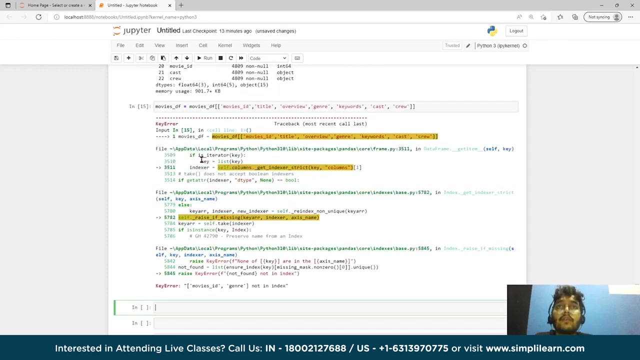 keywords. okay, keywords then to cast. then we will. we will do recommendation with the crew as well. okay, by running this, let me see our data again with seven. okay, okay, there is one error. okay, this is movie. the movie, the idea of genre. no, yeah, not index. okay, got it, got it, why not genre? 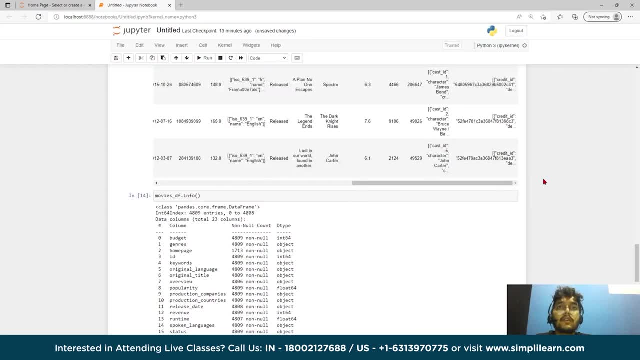 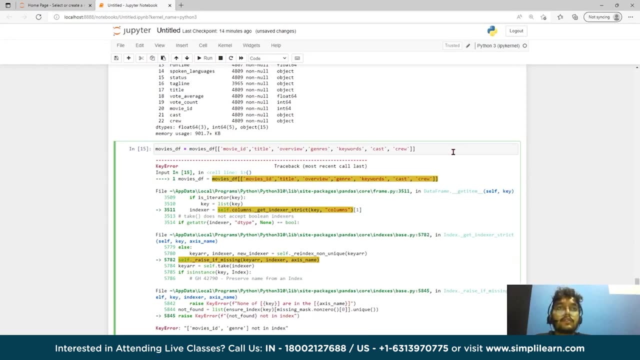 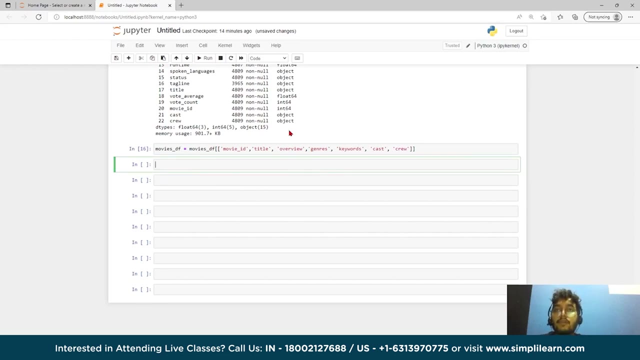 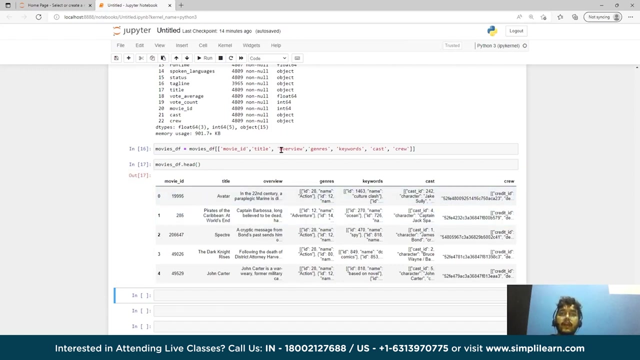 it's jonas. i guess what it is. it's jonas, that's why it's jonas. okay, yeah, so let's see our data again with seven columns. so i will write. so i will write here: movies underscore: df, dot, head: yeah, so you can see only our. we have like movies: id: same title: overview, genres, keywords. 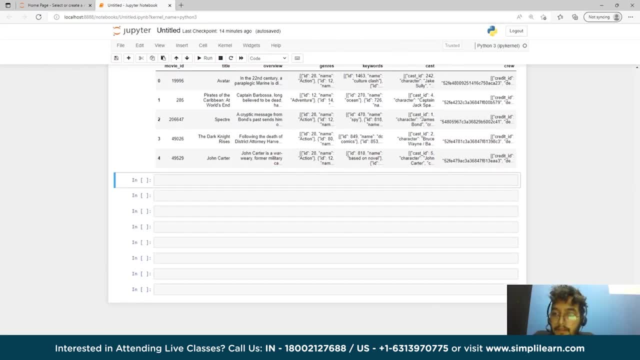 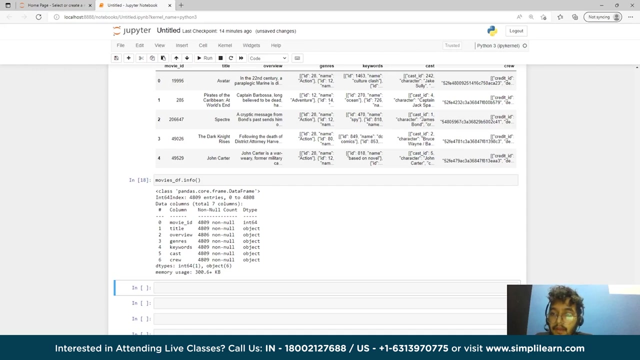 cast and crew, only so. So here you can see the selected columns, okay. So let's move forward and once again, let's see the info again, Like movies, underscore, df, dot. Info has come with selected columns And let's move forward and see how many missing values are present, in particular column. 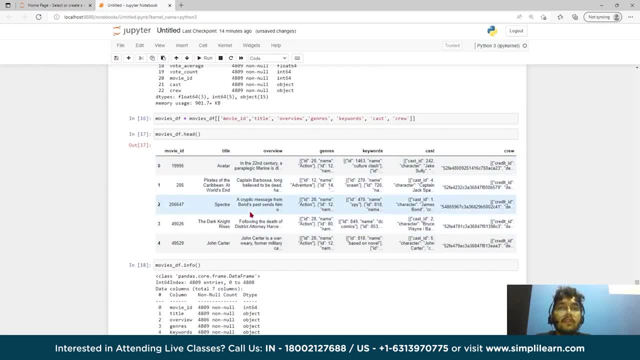 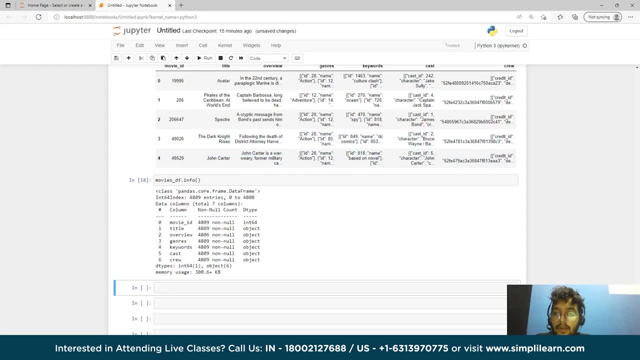 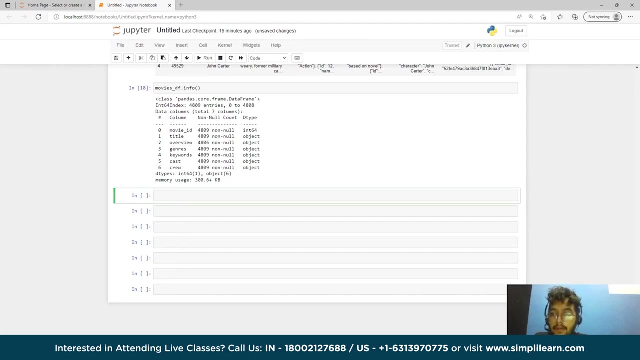 So, like the columns is full, we can see here, But we don't know about that: 4803 values are filled or not. So what, we will do it, we will see how many missing values are present there. So here we will write like movies: underscore df: dot is null, dot sum. 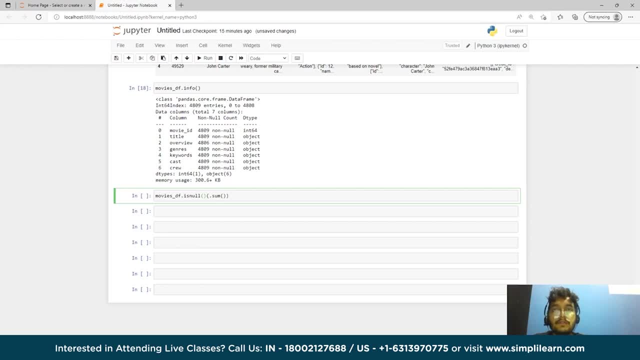 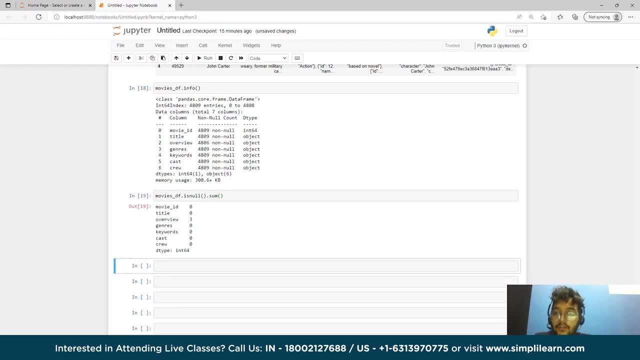 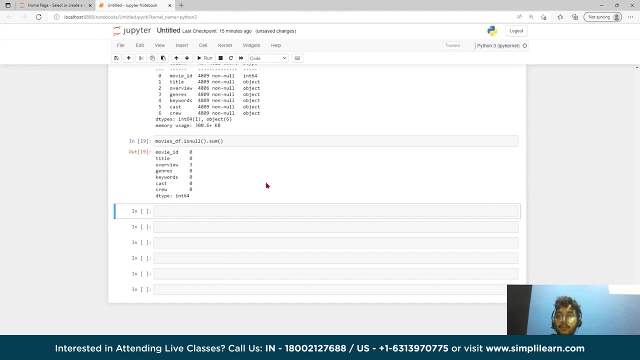 Not like this. Yeah, perfect. So the function data frame is null. This one is null dot sum. dot sum returns the number of missing values in the data set. So here you can see overview. have three missing values. So what we can do is we can write here movies: underscore df. 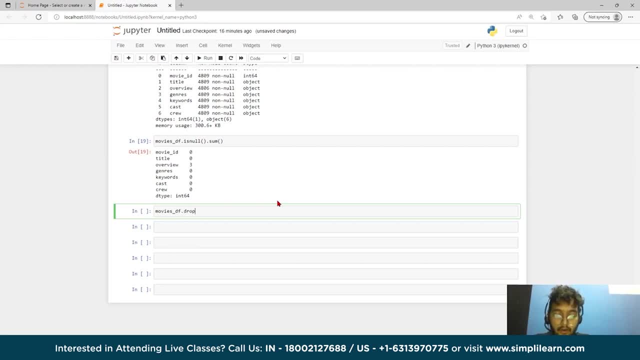 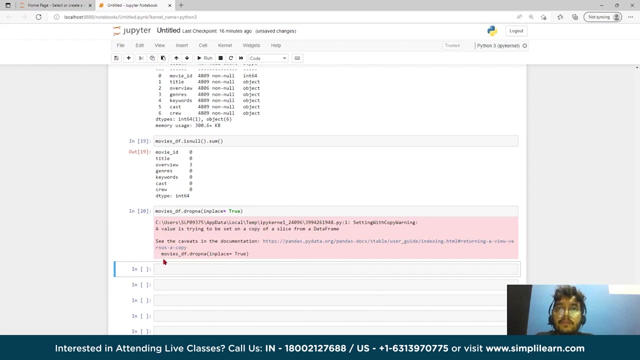 df Dot Drop N A. This Equals to True. Okay, We will run it. It's saying: Okay, let's document Drop N A. This is true, Okay, fine. So if you set in place equals to true the drop, any method will modify your data frame directly. 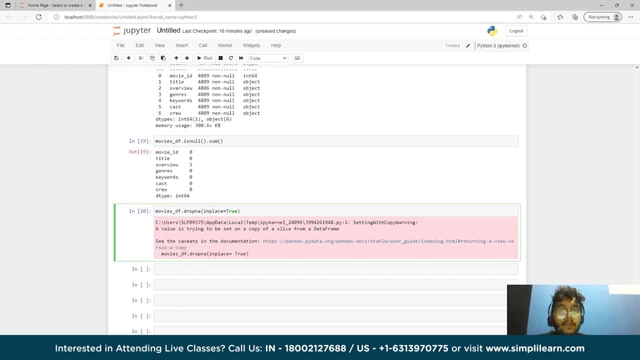 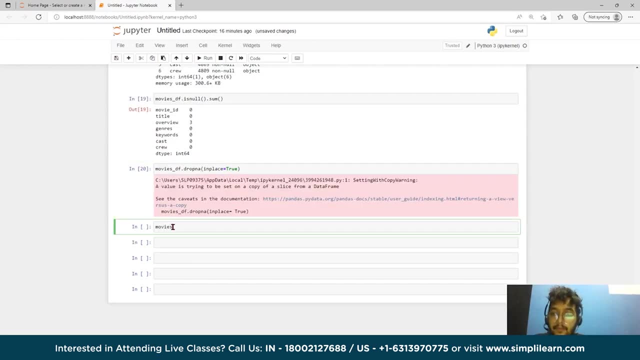 That means that if you set in place equals to true, the drop, any will drop all missing values from your original data set. Let's move forward and see movies Underscore: Df Dot, Duplicated- Duplicated. So the duplicate method returns a series with true and false values that describe which rows in the data frame are duplicated or not. 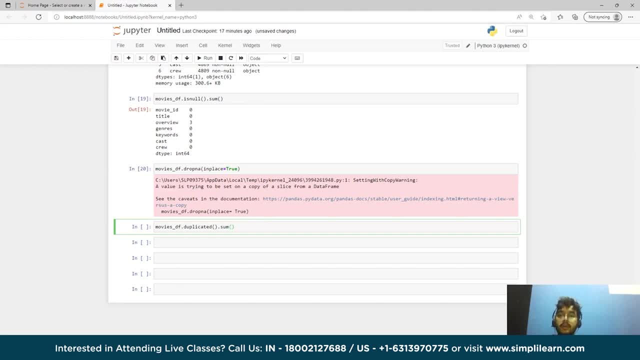 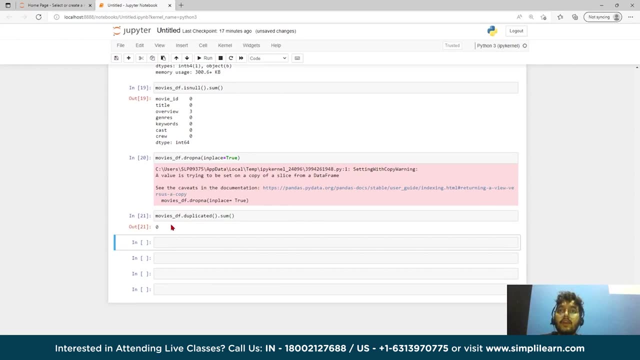 Use the subset parameter to specify if any column should not be considered when looking for duplicates. So here let me run this first. So here we are getting zero. Why zero? So if you are Like thinking, there is no true or false return, 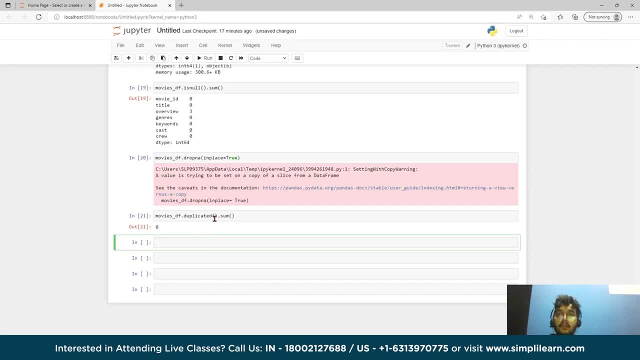 So if you write it without sum, Like if I will write it without sum, Okay, let me copy from here. Yeah, And I will run this. So here you can see False, false, false in whole data set. 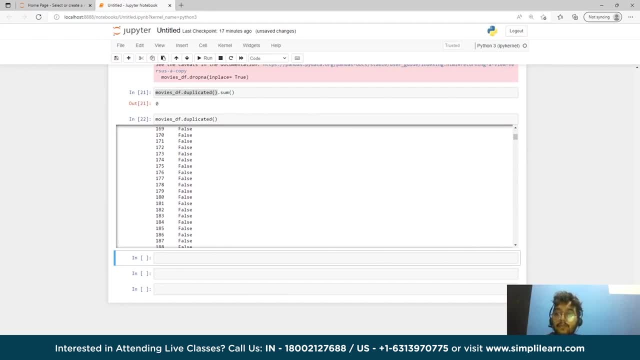 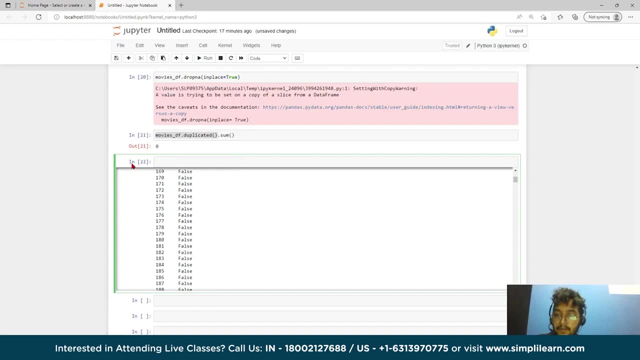 So sum will combine them and return you a value At the end. zero represent false itself. So we need, Do not need this, So we will write something else. So moving forward, Let me write first. movies. Underscore Df. 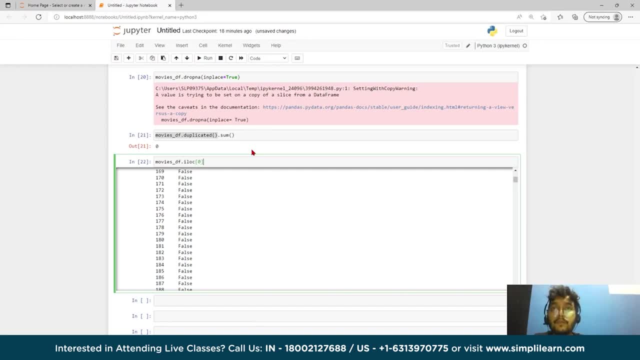 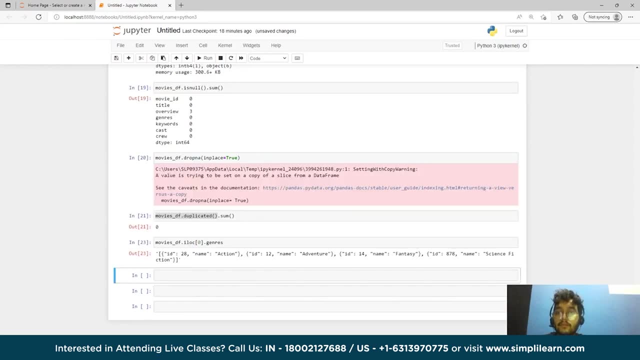 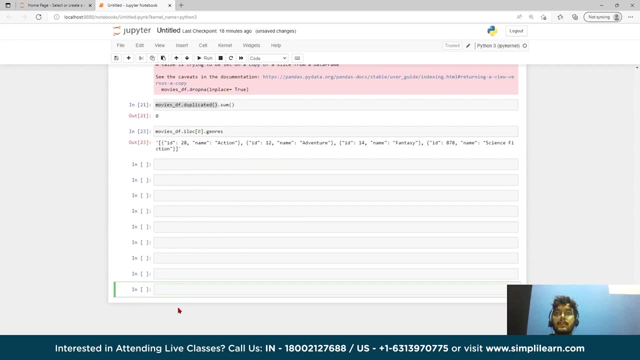 Dot I, location Zero, Dot Jonerts. Let me run this. So the ilog function, This one Ilog function, First. let me do something like this. It will go up. Okay, Huh, Okay. 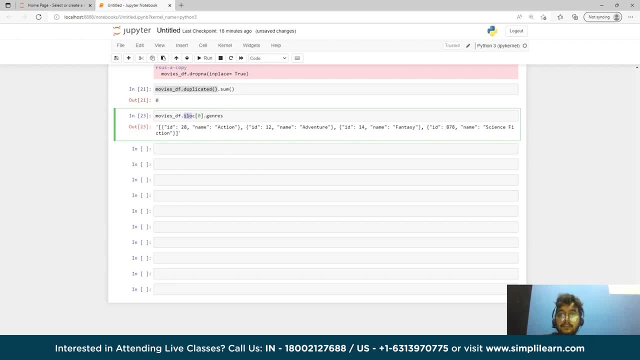 So From ilog function in Python is defined in the Pandas module that helps us to select a specific row or column from the data set. using the ilog method in Python, We can easily retrieve any particular value from a row or column by using index value. 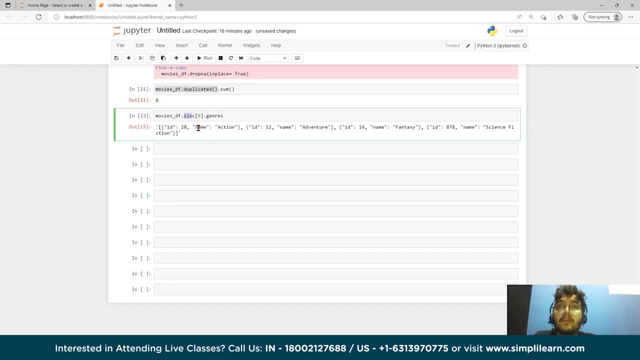 So here zero position line is coming. It is here You can see. So name action like name action, name adventure, name fantasy, This side fiction, This one science fiction. Yeah, So this is because I am giving here genre. 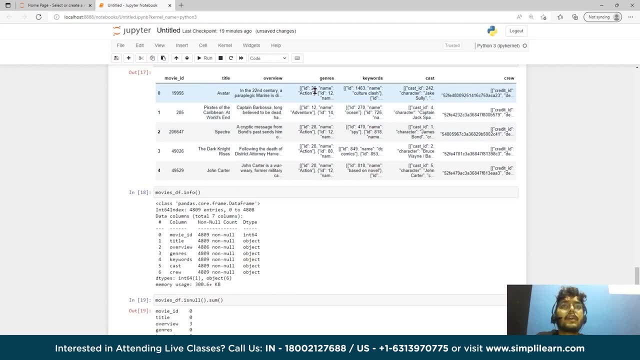 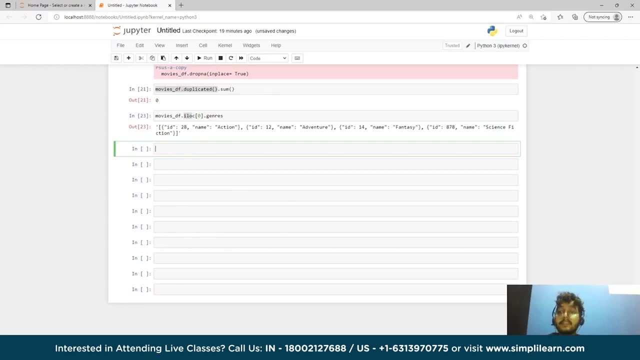 That is why you can see here: See, I did want your name, action, name something, something, something like that. Okay, So Let's import something called AST- abstract syntax for tree. So this is one of the major library import AST. Let me run this. 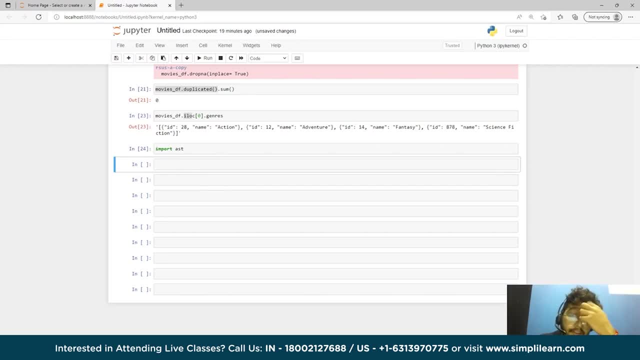 So import is a class defined is the AST module that is used to express the import statement in Python in the form of abstract syntax tree. So so an abstract syntax tree, or just syntax tree, is a tree representation of the, of the abstract syntactic structure of text written in a formal language. 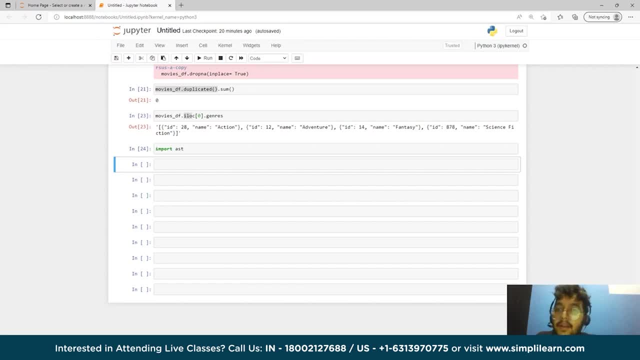 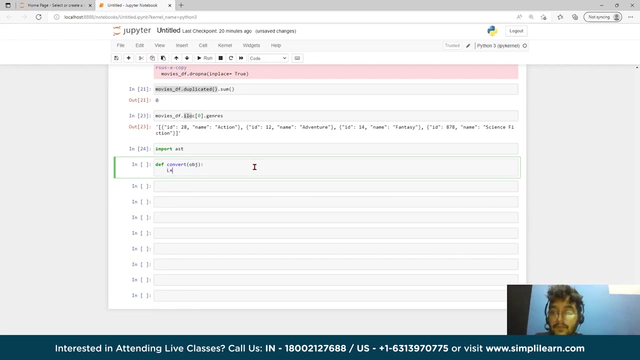 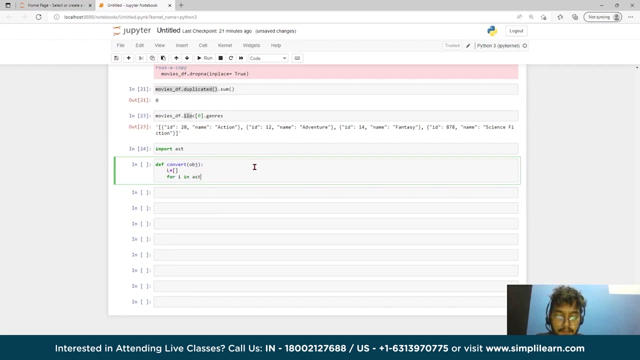 Each node of the tree denotes a construct occurring in the text, So let's convert some like literal to objective. I will pass some of the verb to the subject and append them, So here I will write: def. convert object Like L equals to blank array, for I in AST dot. 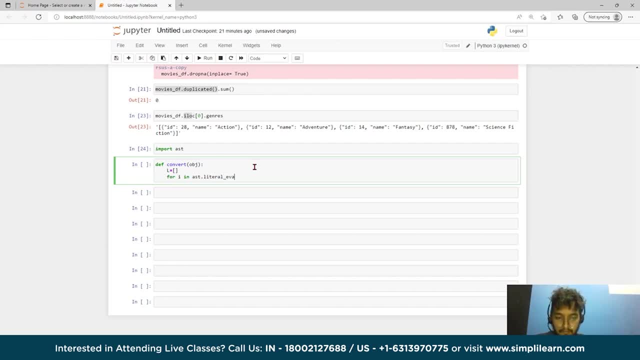 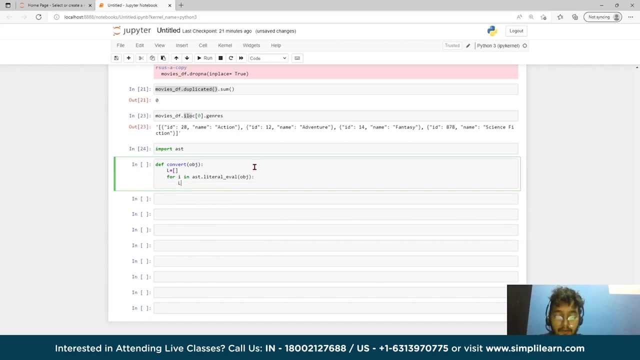 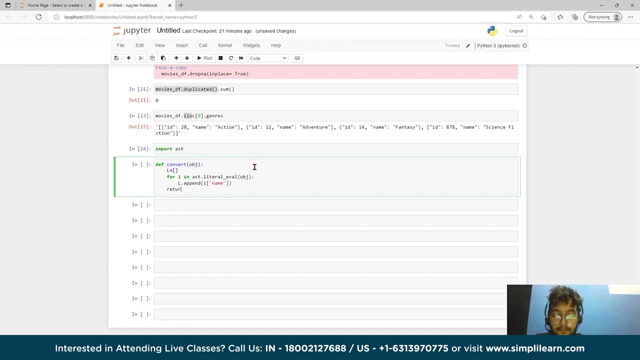 Well, bitvgObject: lappend return. Here we are converting is like: here is a convert is a function and l is an array to append. by using for loop We can append them to name. So let me write code, then I will explain like what is happening. 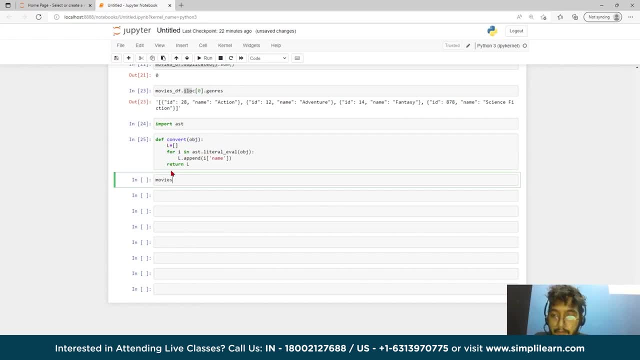 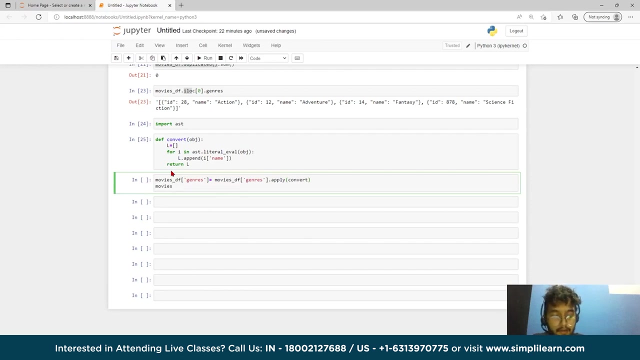 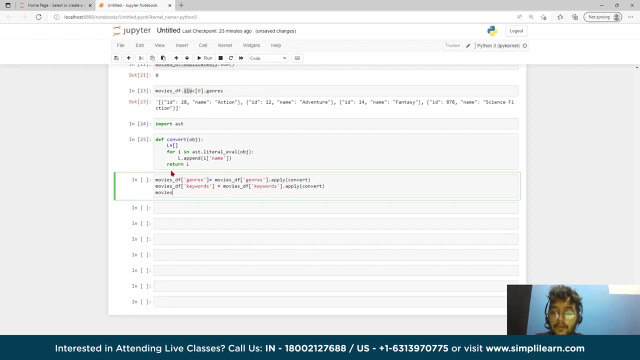 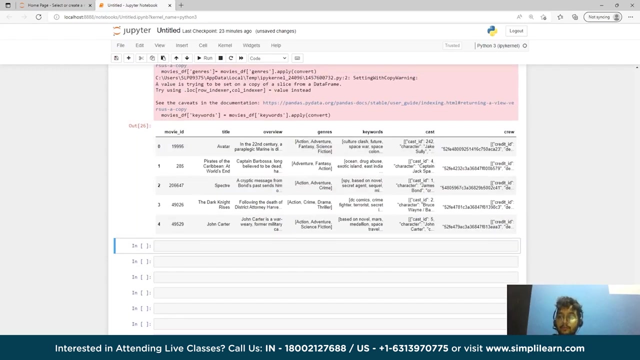 So let me write full code. So movies underscore df: like, like, like, like and then dot apply. So then movies underscore df, then I will write keywords to movies underscore df keywords. so if we will see our old data set in that, like if we will see our old data set in that, 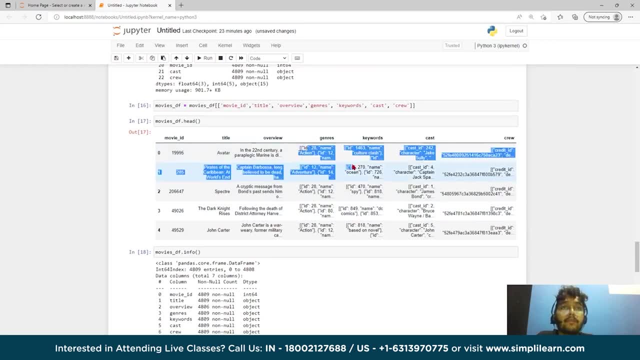 we will see old data set in that genre and that's keyword, this keyword, id name and so on, like id, that name, like this type of things. so it will create a mess in retrieving them. so by using AST library we just convert them to the normal one, like: 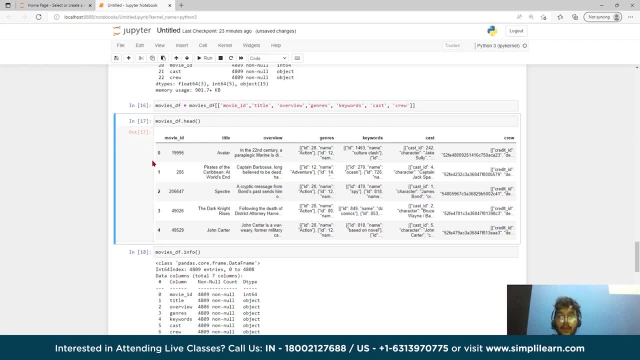 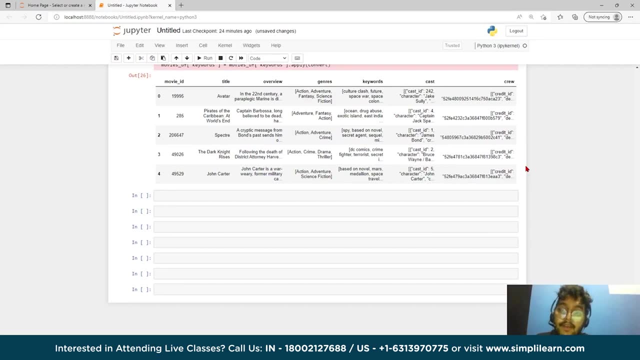 title. so got it guys. so I hope you guys understand till here. if you have any question or any query regarding any code or question, just put as in comment. our team will shortly provide you the correct solution. abbreviating again, I hope you guys understand till here. if you have any type, 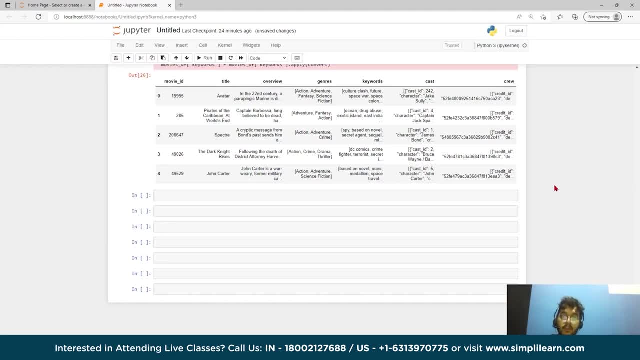 of questions regarding any code or something, so just put as in comments. our team will shortly provide you the correct solution. so, moving forward, let's convert cars to and like same as previous way, like like this. only so what we will do here we will. 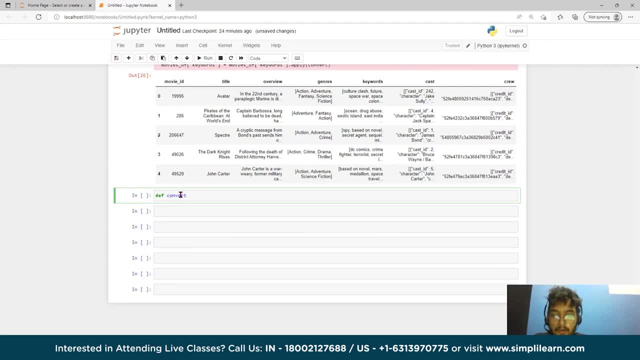 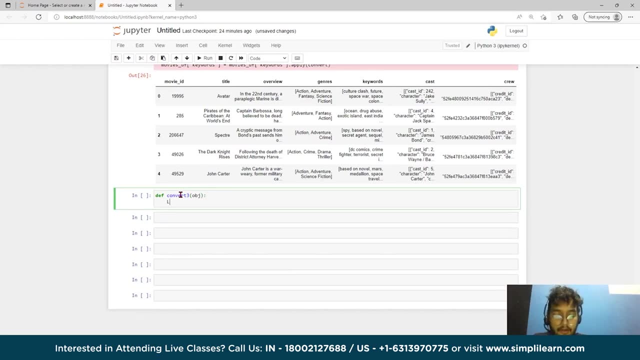 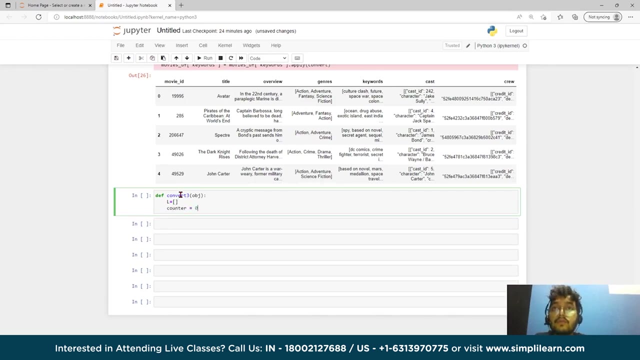 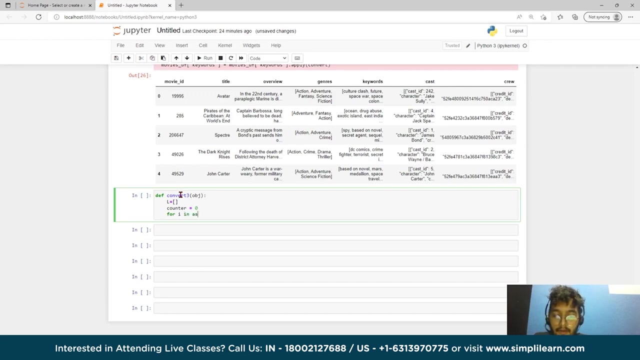 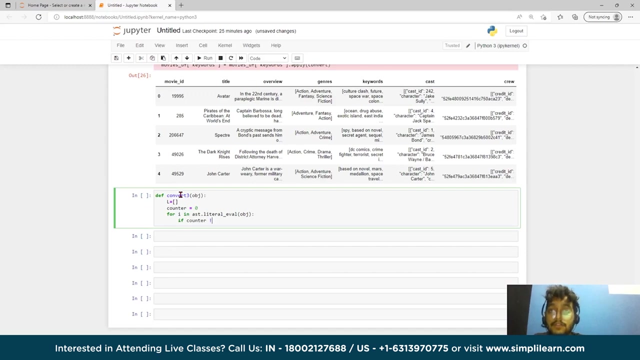 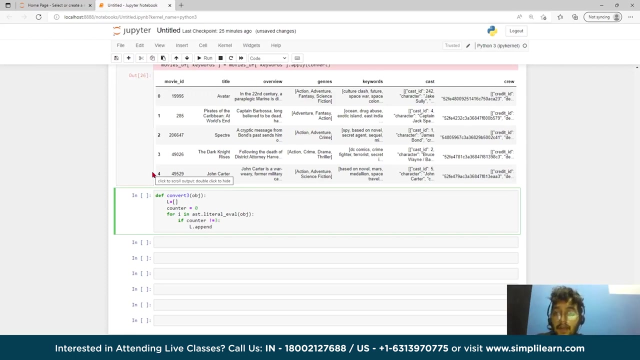 write def convert here I am using: so L equals to counter, equals to 0, AST dot, literal. if counter does not equals to 3, then L dot, L, dot, dot. append. okay, then here. 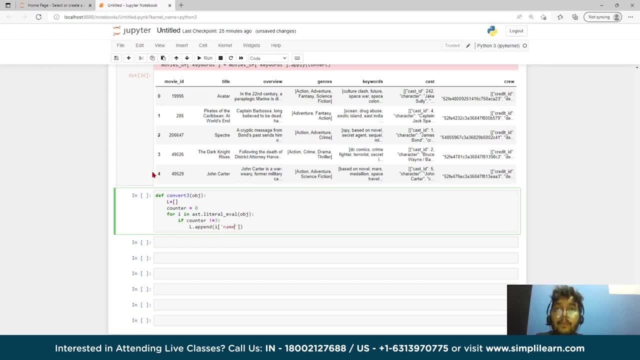 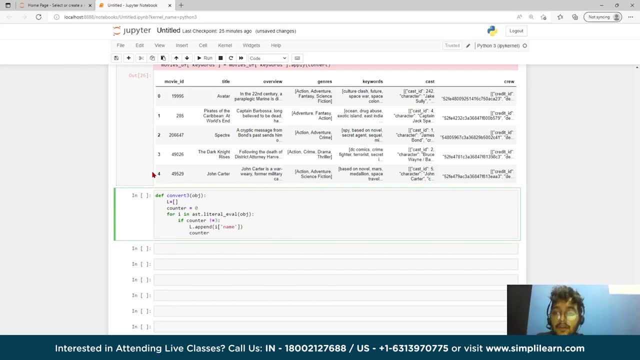 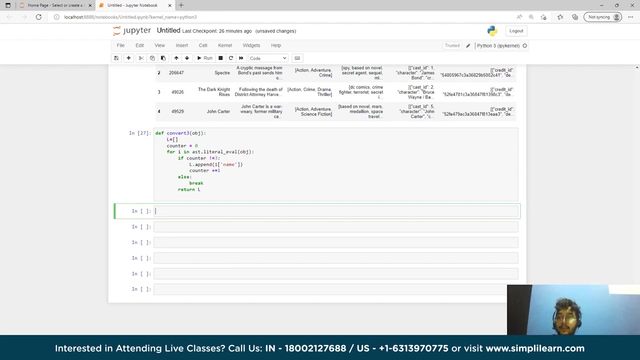 I have to write I to name. okay, counter equals to 1,. if you want to write like: counter equals to counter plus 1, it is like both the same. else, take turn L. so let me run this. let me run this, okay. so after this small code, we have to assign: 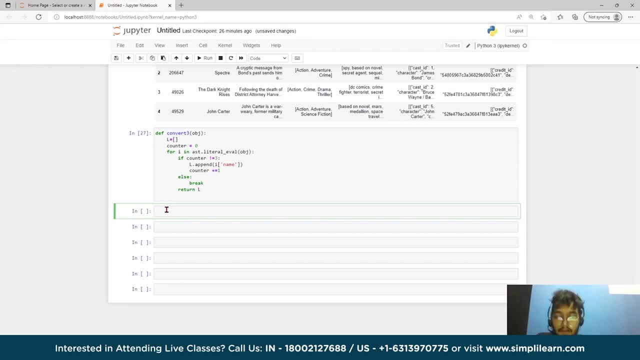 the values, like we are doing it for cars now. so movies, okay, movies underscore DF, then cars. so movies underscore DF cars, so movies underscore DF cars. so we kind of show the table: okay, this guys is telling us to write movies and movies. 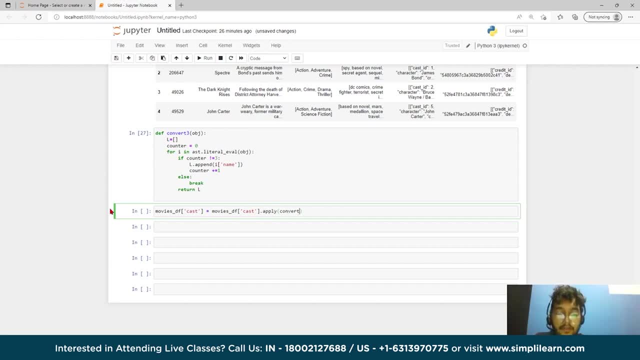 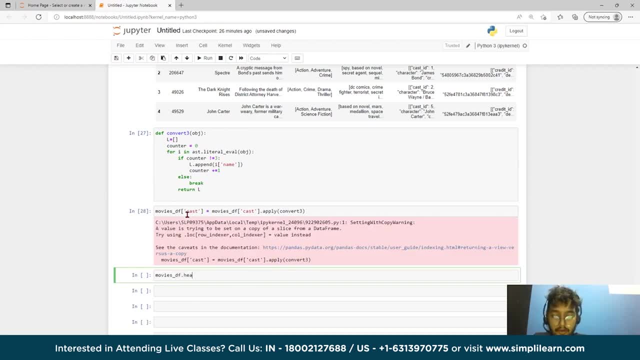 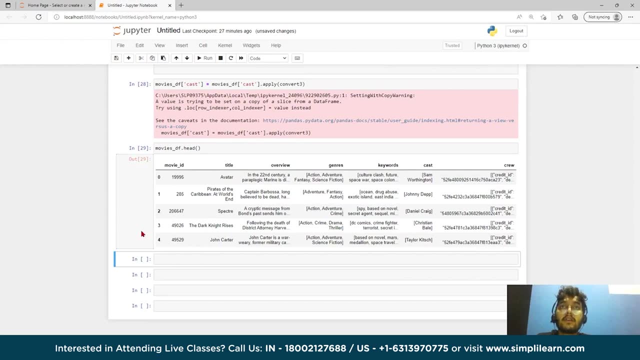 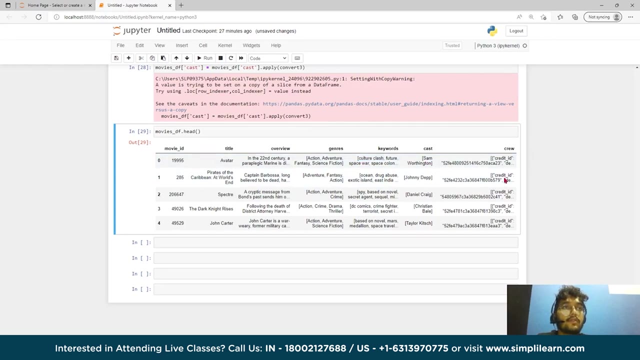 movie movie moviem movie. Carnival movie movie movies, movie movies, cinema movie movie movies, movie films, movie movies. ay, like this is nothing, so here you can see. cast is also same, like keyword and journal. so like let's do for the crew too. so like we are converting, you can. 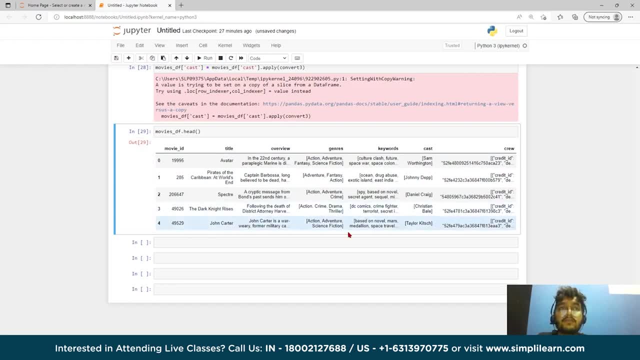 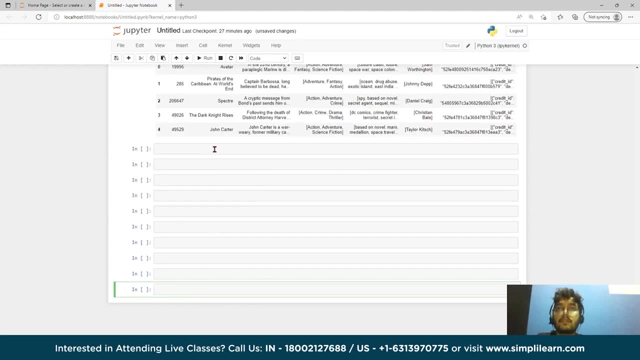 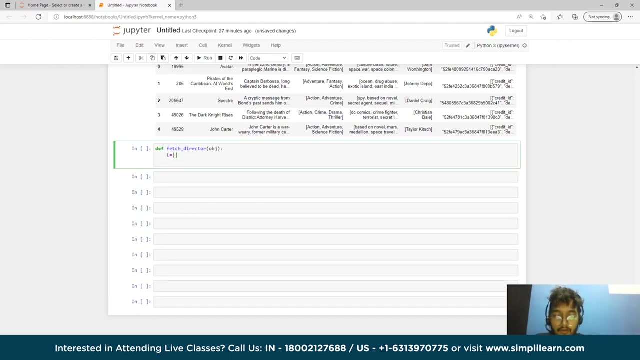 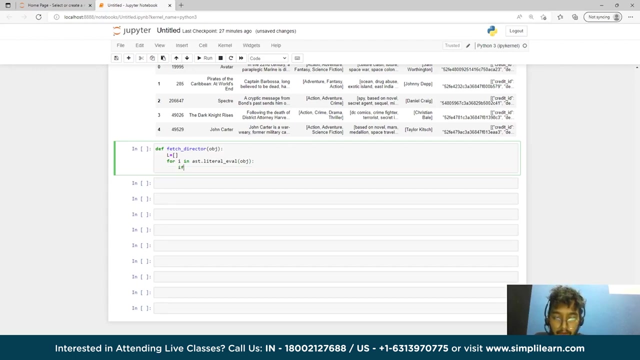 say in a structured way. so let's do for the crew one too. so let me put some yeah. so here we will add dev like fetch, which is nothing like a function name as director OBJ. okay, colon L equals to, or I in AST, dot literal OBJ if I job. 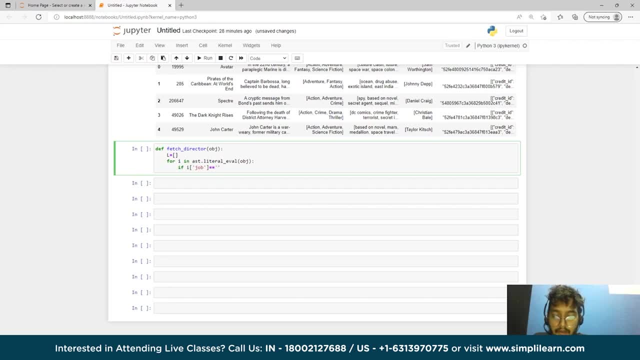 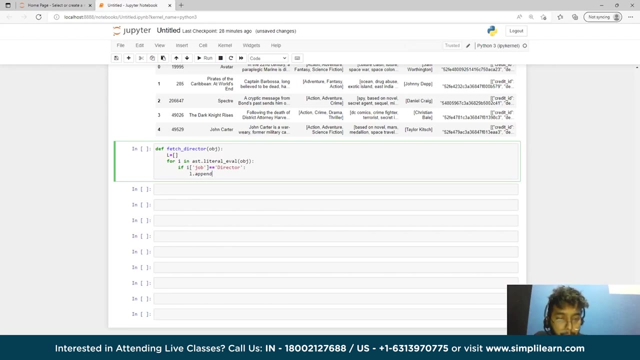 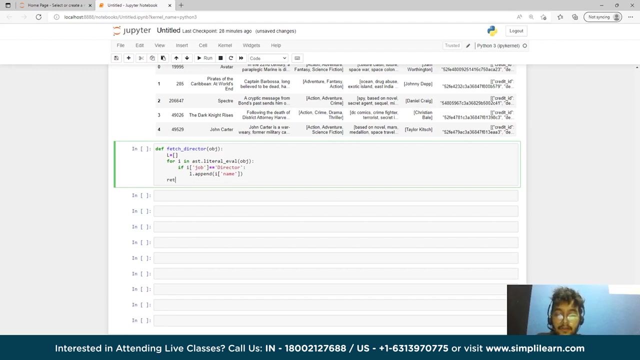 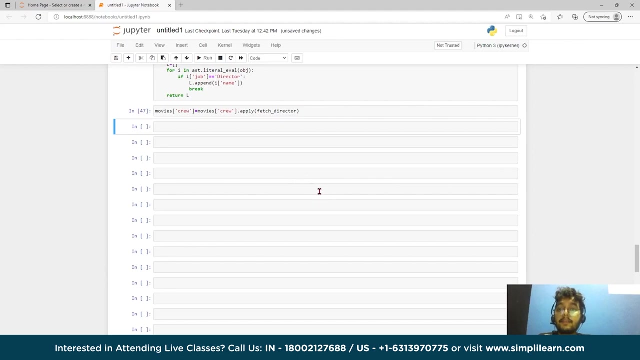 procedure equals to like we can hit director. so then L dot append, L dot append, hmm dot append to the same name but returned a capital L. so we have to again write that movies, that movies, movies. Just remember, fetchDirector is a function name. Lets see changes. 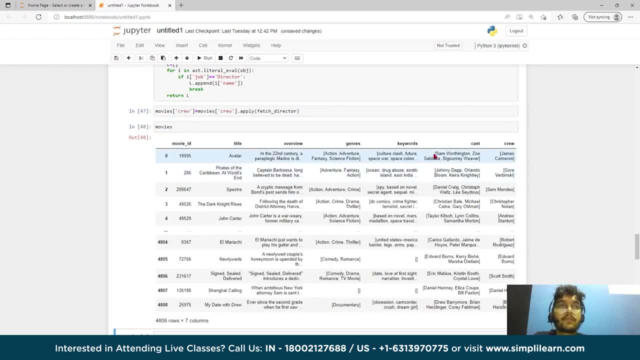 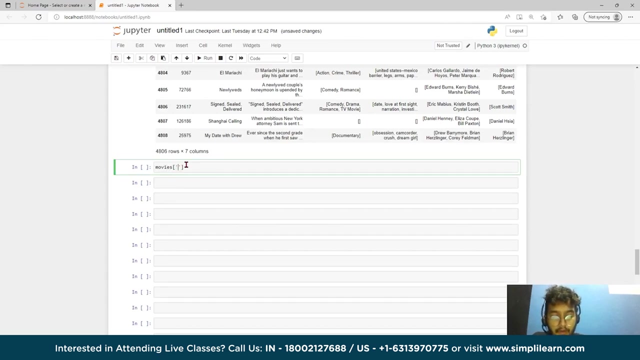 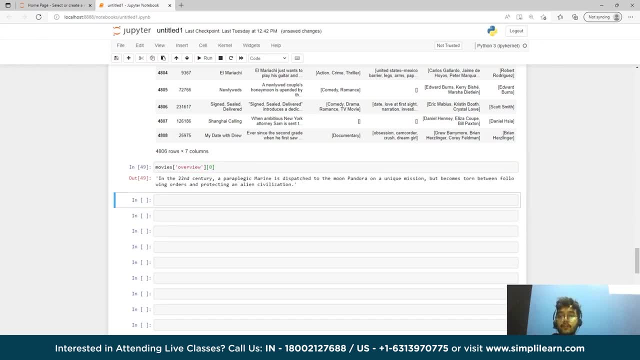 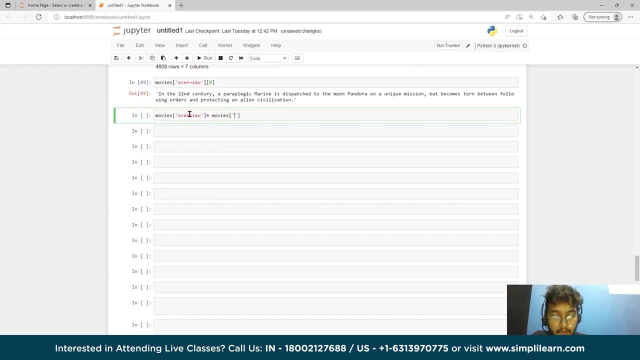 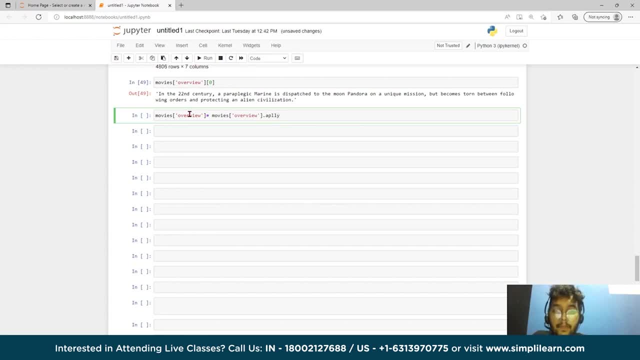 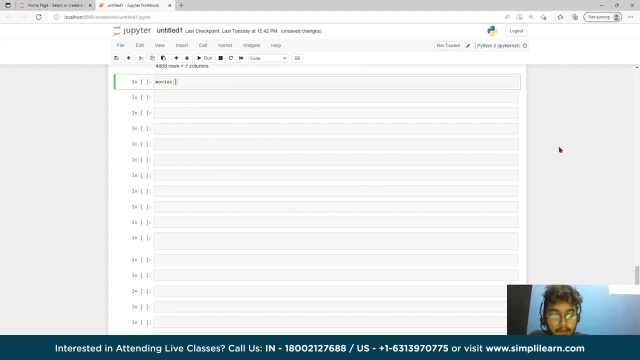 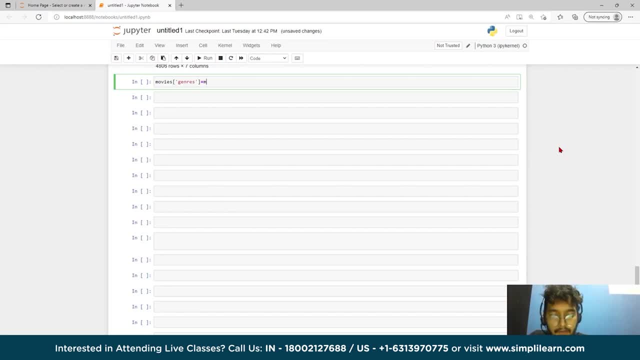 movies Like genres, movies Like genres, movies Like genres, So movies, So movies, So movies, And again genres And again genres And again genres. But apply. 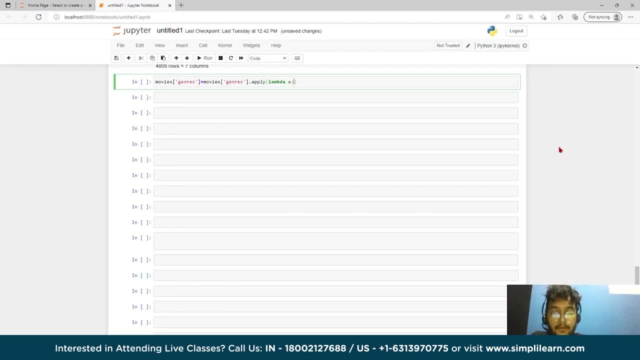 But apply, But apply lambda, lambda, lambda x, x, x, i, i, i replace, replace, replace, replace, replace, replace space, replace space, replace space ma. 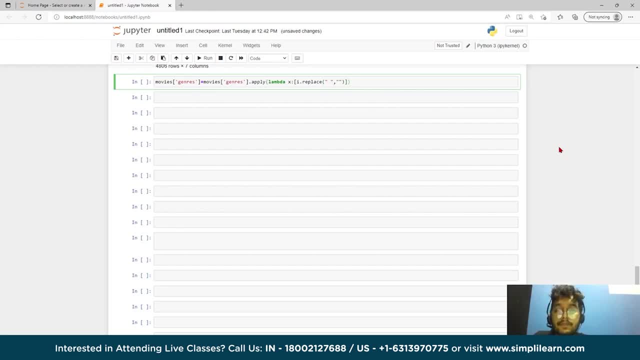 ma, ma to no space, to no space, to no space. Oh, it seems good, Oh it seems good, Oh it seems good. Then I have to write, Then I have to write, Then I have to write, for everywhere. 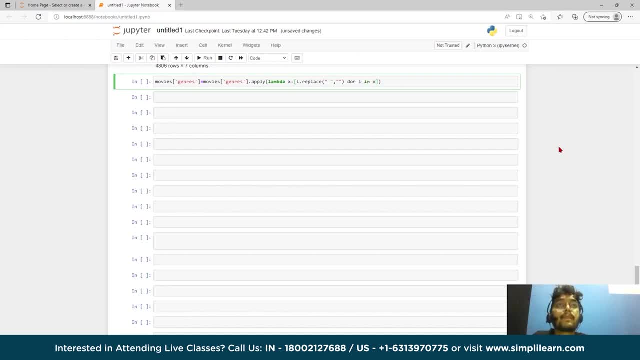 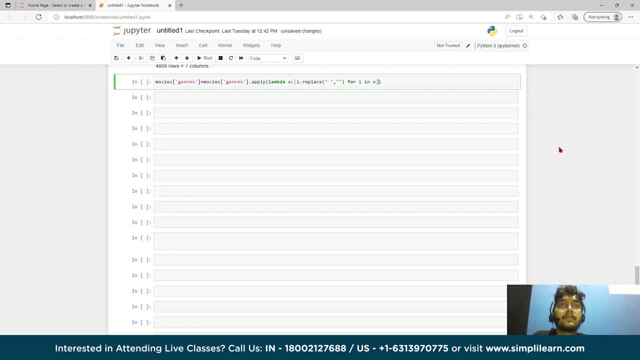 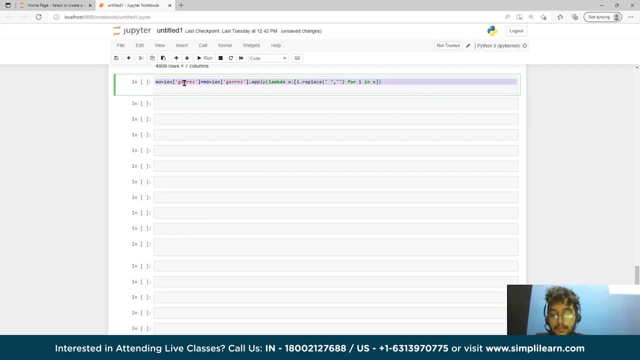 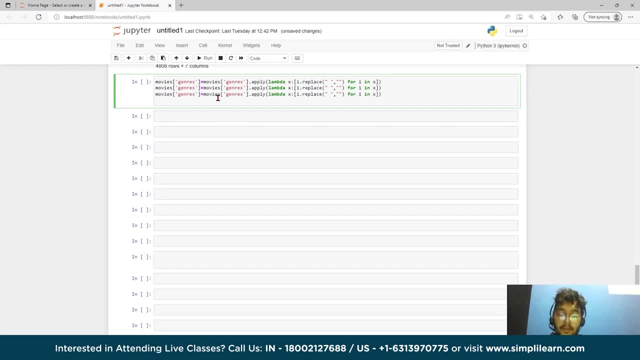 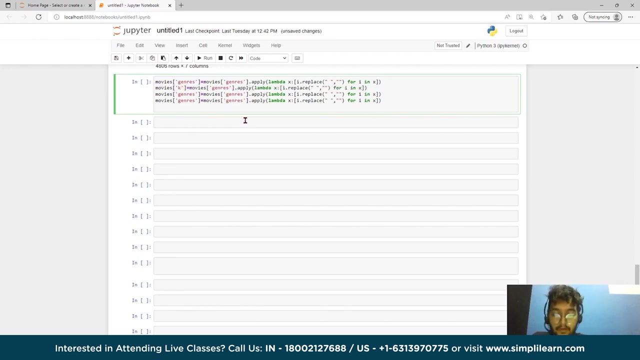 Seems good, Seems good, Seems good. So let's copy-paste this, So let's copy-paste this, So let's copy-paste this, See See See. One for keywords, One for keywords, One for keywords and one for cast and crew. 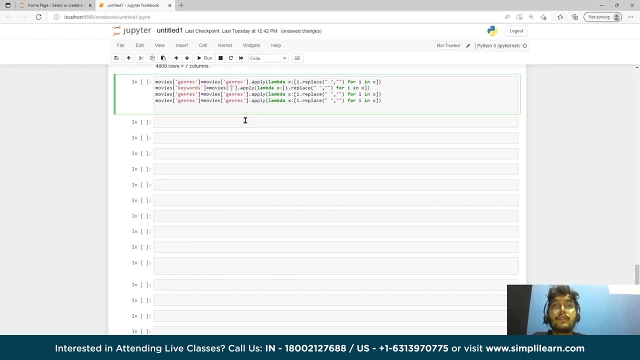 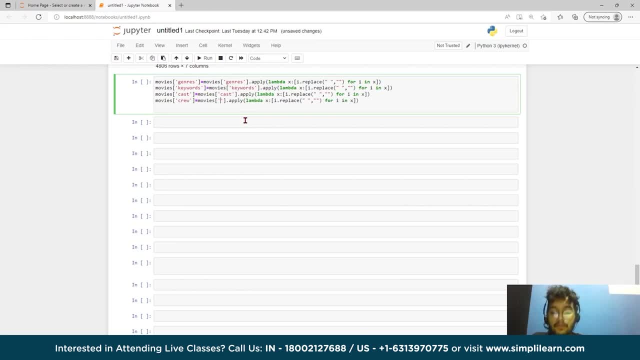 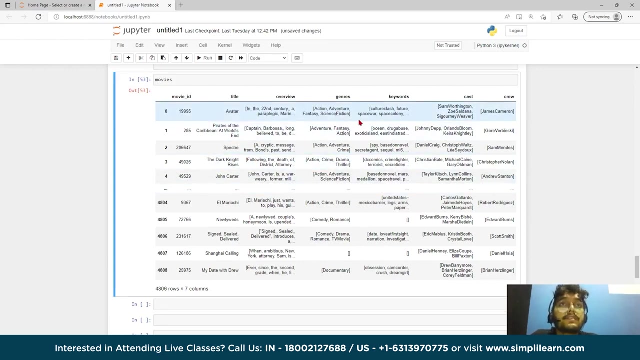 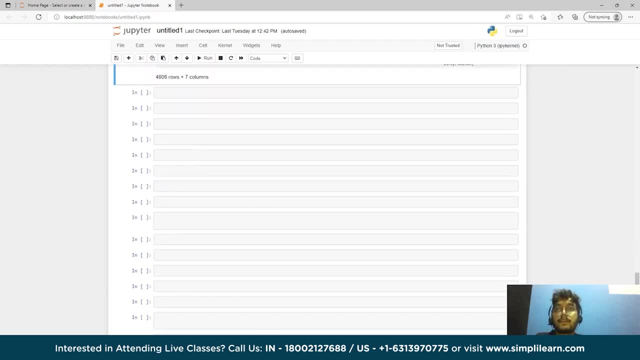 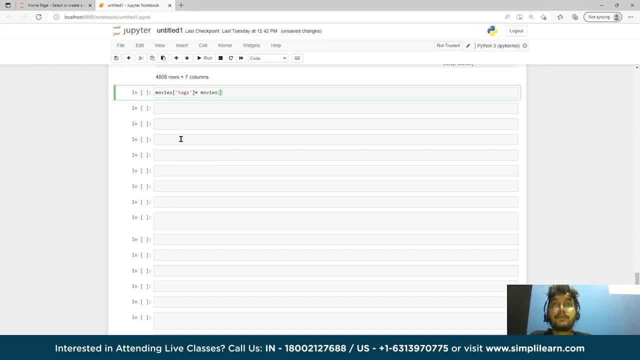 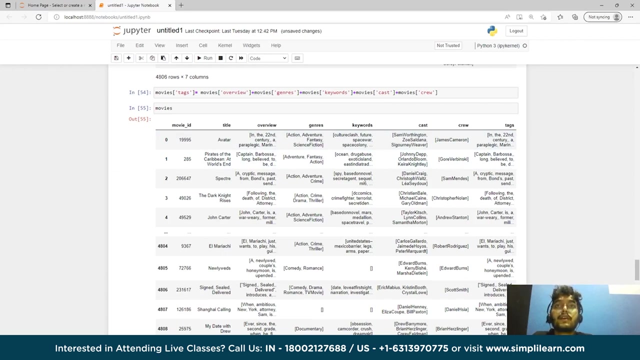 movies, and first we will put overview plus movies and genres and movies and what we have to give keywords, keywords, then again movies. then asked he'd run this. okay, so let's see the data frame. okay, still coming. so there is one problem. I guess yeah, no, no, no. so here, 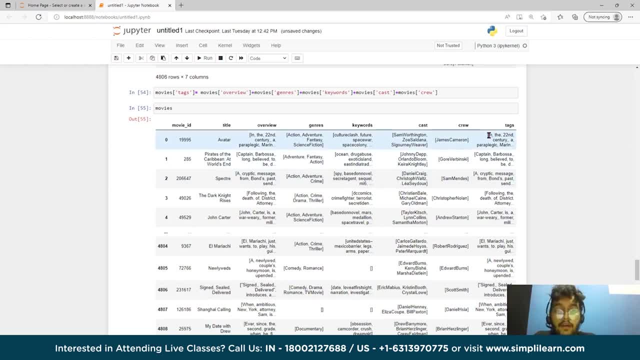 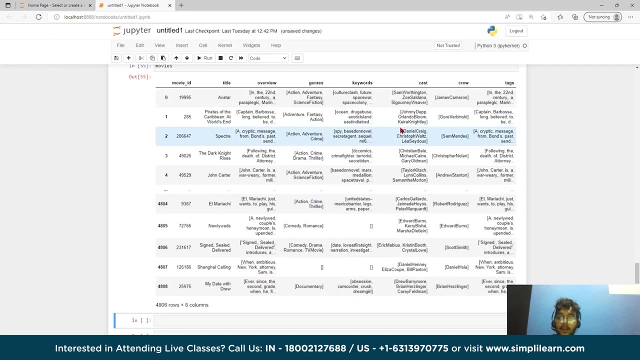 you can see all the data is merged in a under tag column. yes, you can see like in the second century, blah, blah, blah. so I hope you guys understand till here. if you have any question or any query regarding any code or anything, just put as in command or our team will. 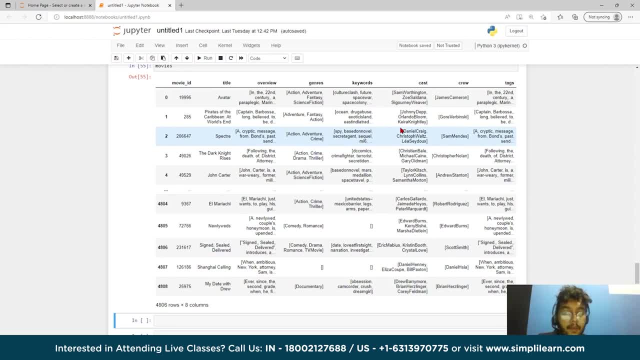 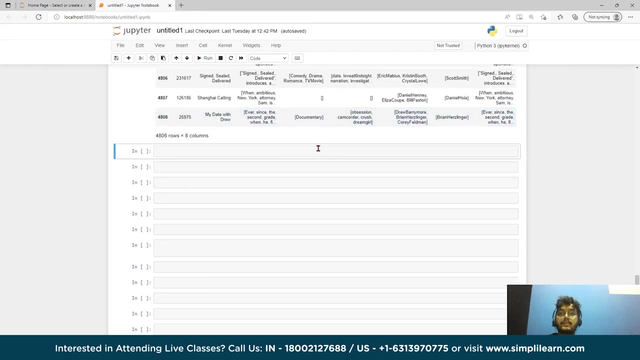 shortly provide you the correct solution. okay, so I'm repeating again. I hope you guys understand till here. if you have any question or any query regarding any code or like any question, just put as in command. our team will shortly provide you the correct solution. so from here, let's create a new data frame, okay, so 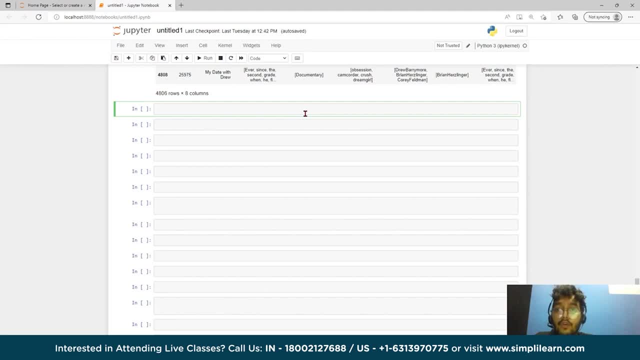 let me create new data frame because now we don't need this overview house crew genre. like columns like this. we have already merge into a 1 one column, like tag column, so we will write here: neo df equals to movies, so movies- we need, movie ID. you data frame we need. 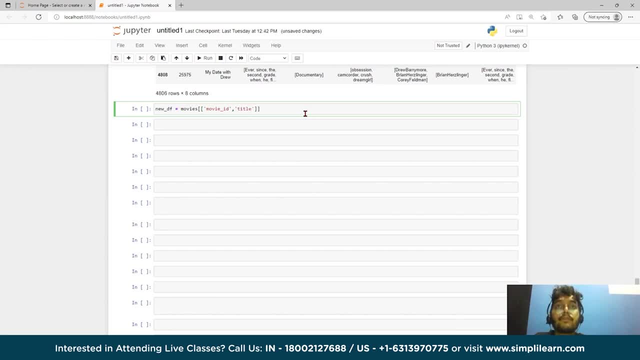 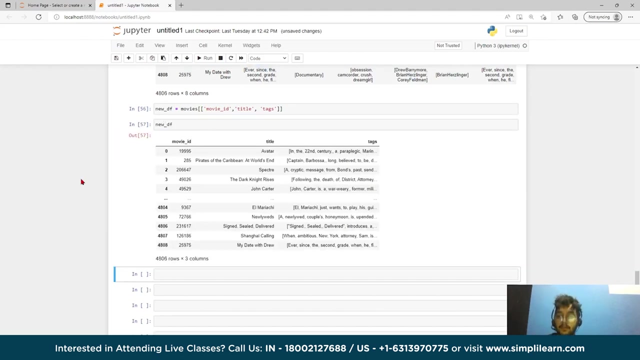 movie ID comma. we need title and we have everything in tag column- tags column. so we need tags column. okay, run this. let's see our new data frame. so this is our new data look likes with only three columns like movie ID, title and tags. so here you can see array brackets like this, this array brackets, so, and we are. 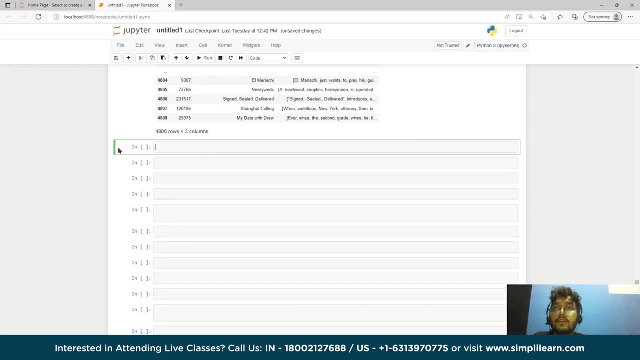 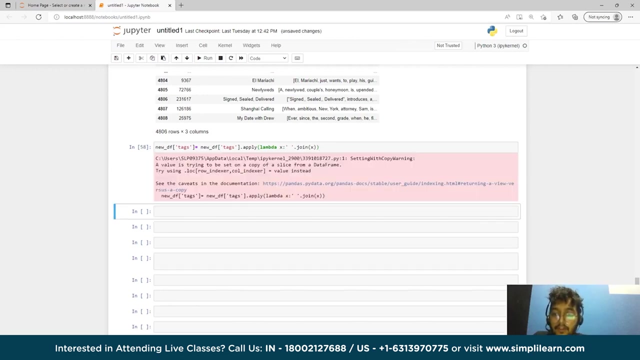 gonna remove them, so we will do what we will write here. we will write new data frame that in tags equals to new data frame. X dot apply and X space dot join. seems good, everything is okay, okay, fine, yeah, so let's see the results. so we will write here new underscore. 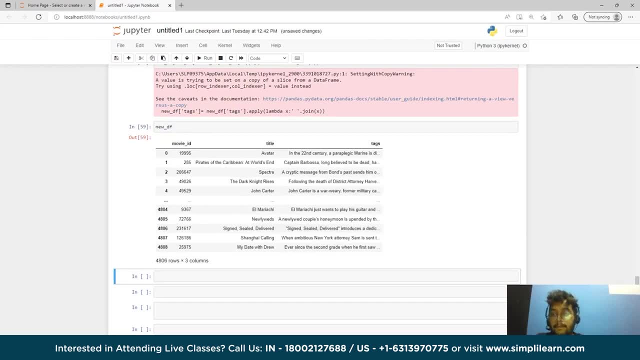 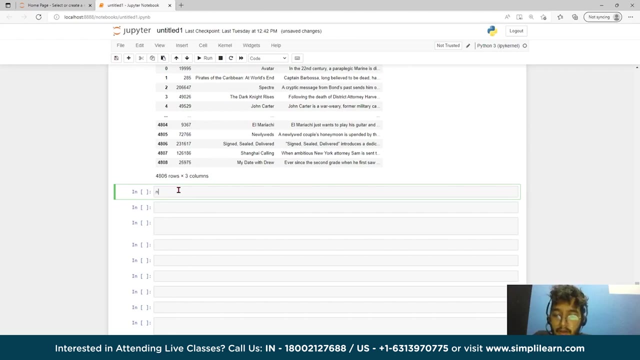 data frame. so you can see the brackets are removed. now let's see the data which is present in the 0th index in tag column, like this: dot dot dot in the same. okay, for that we have to write here a new data frame tax. we did it before, like for the overview. 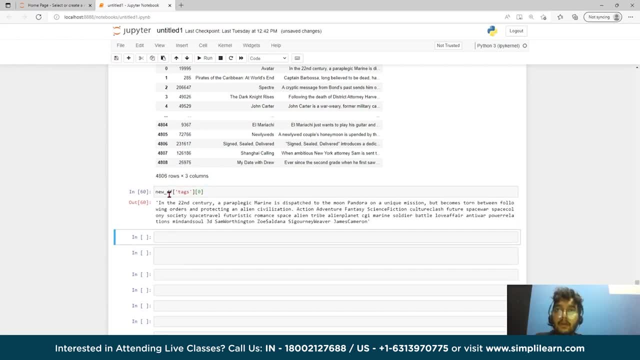 are. so yeah, so this is the whole data in the first, like first index, 0th index. so some part of the overview, like from civilization and some are you can see this action at winters, fantasy, science fiction. these are some like John and a, like you can see like these are some creos members and like Sam Worthington, like they are some. 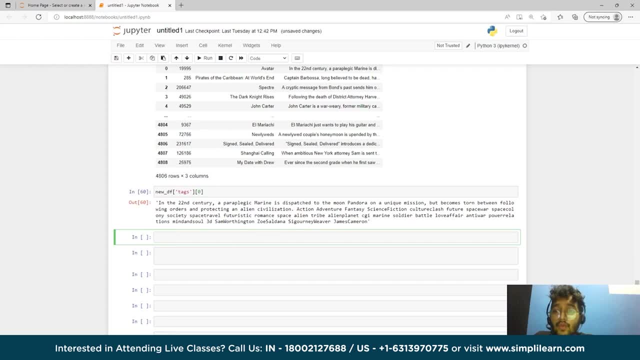 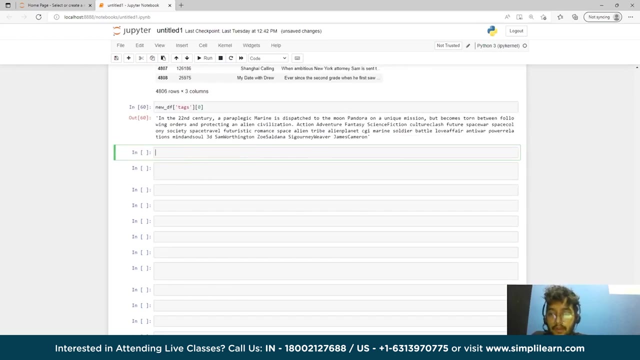 cast crew. ok, so like moving forward, like what we are going to do is just make them in lower case, for the better prediction likes something in capital, something like smaller, so let's make it to lowercase. so new underscore df tax equals to new underscore df tax. dot apply. 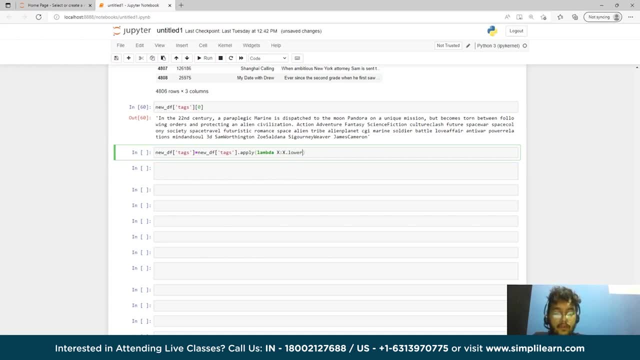 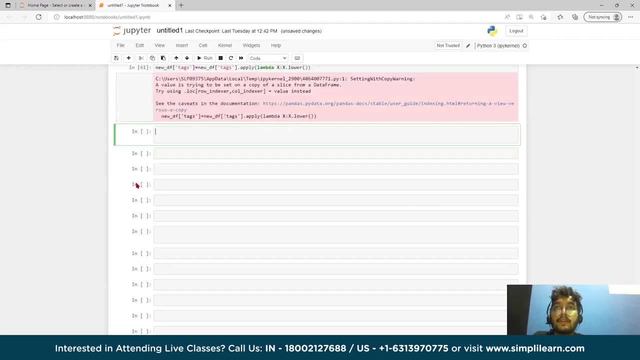 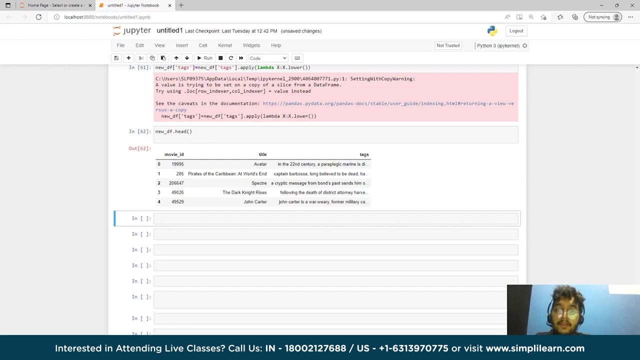 x dot lower. ok, So don't worry about this error. let's see the result. new underscore: df dot. yeah, now all the data present at tag column is in small case, or you can say lower case. Moving forward, let's do some feature extraction using count vectorizer. 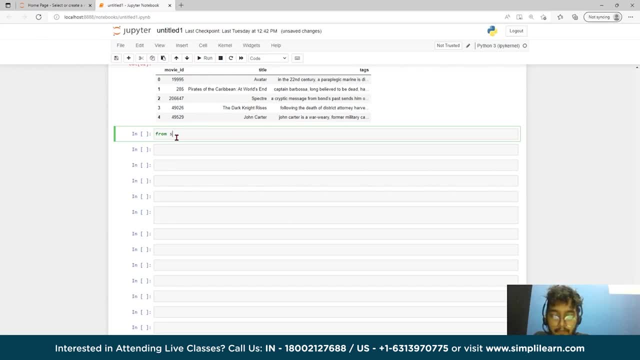 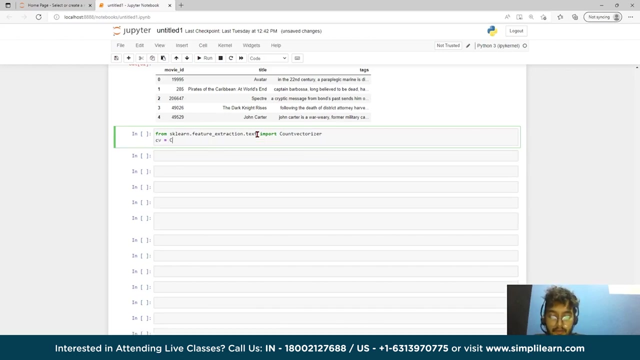 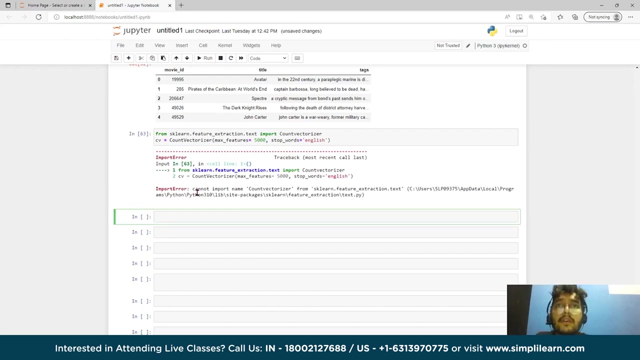 So let let me write first from sklearn dot feature extraction. feature extraction: ok, cool dot text. import count vectorizer. dv equals to count vectorizer, underscore features. features equals to 5000, top words equals to English And this yeah, so count vectorizer: ok, there is a I cannot import count vectorizer from. 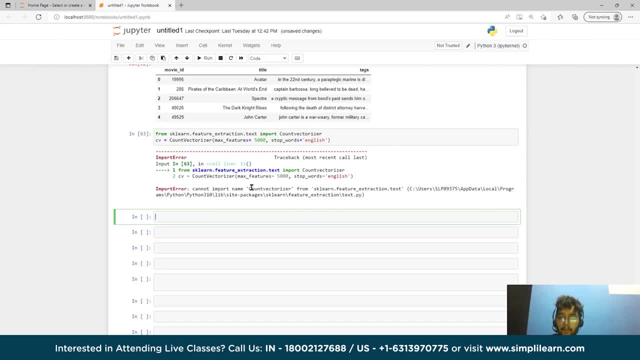 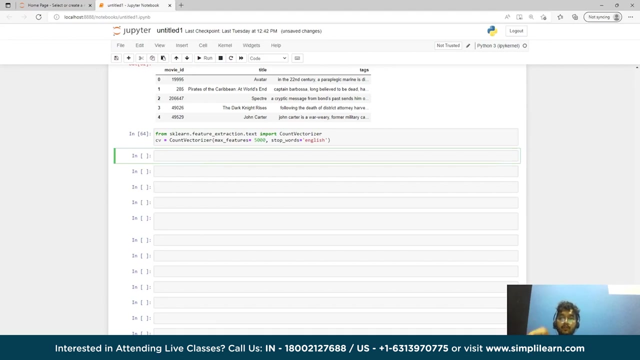 sklearn from user. ok, ok, sorry, sorry, my bad, here v is capital. ok, guys, I'm sorry, sorry, Sorry, Sorry, Sorry, Sorry, Sorry, Yeah, sorry. So he v is capital, So no error. 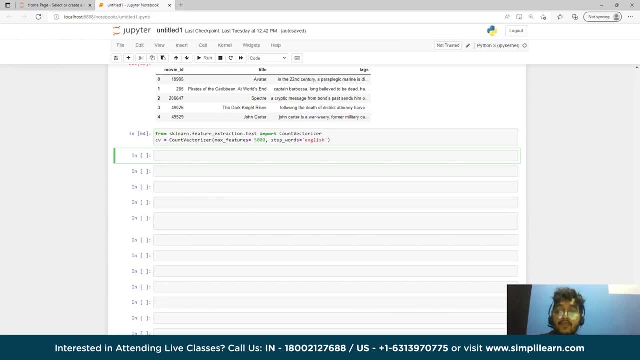 So count vectorizer is a great tool provided by the scikit-learn library in python. It is used to transform a given text into a vector on the basis of the frequency count of each word that occurs in the entire text. So let me write something. 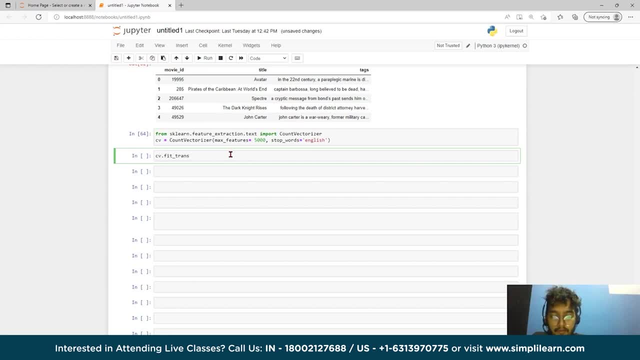 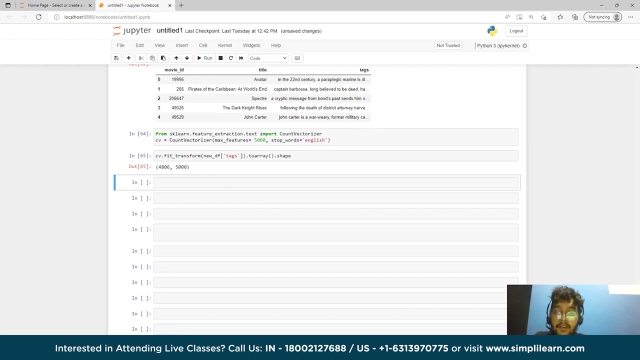 CV: dot ID underscore form f at x like dot to array shape. ok, so the fit method like learns a vocabulary dictionary of all tokens in the raw documents, that is, it creates a dictionary of tokens. by default the tokens are words separated by spaces and like punctuation, so that maps each single. 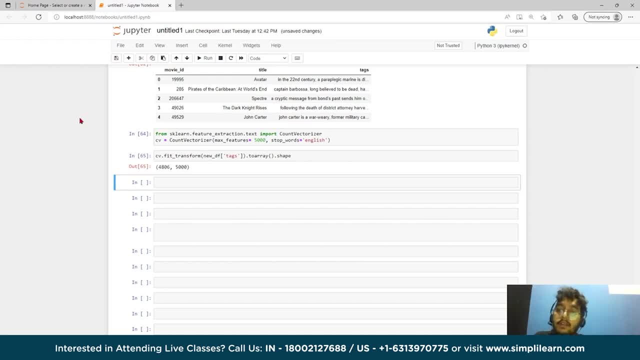 token to a position in the output matrix. so here cv is a like, here cv is a counter vectorizer. so let's convert into vector to array. so for this we have to write vectors. vectors equals to cv, dot fit. so yeah, then transform x sin. so here we have to write dot to array. 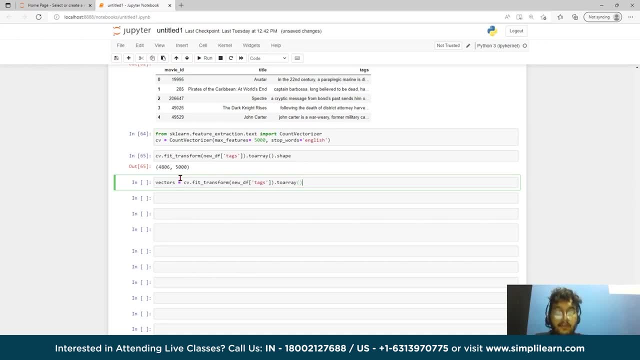 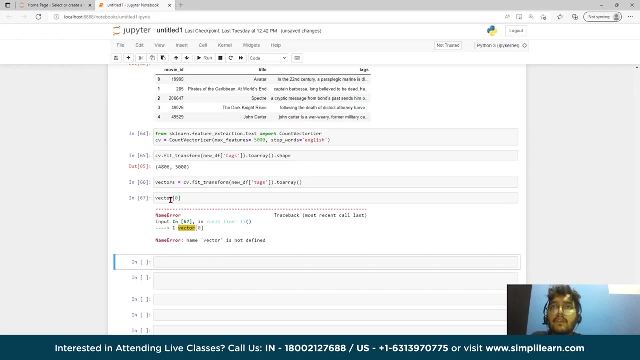 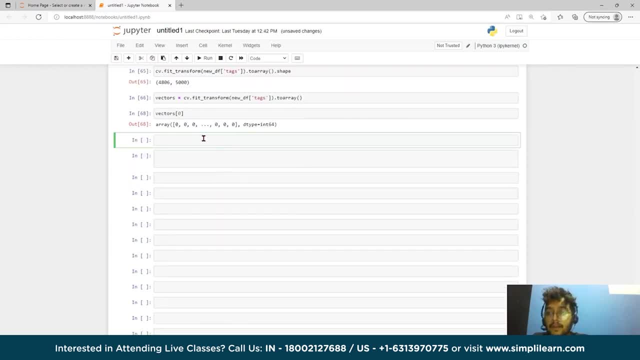 so we will write here: vector 2 r, order 8, global formed pastor Module and product sheet. so answer these question. now it is like a string, which is like a string, so anything like that can be done in Excel. so, mycom, if first of all I want to stove, now I don't want to solve. 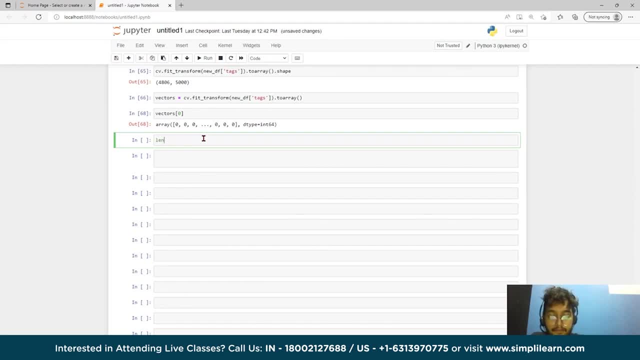 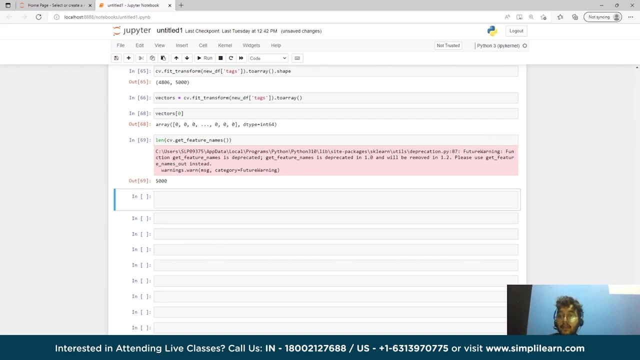 and then CV dot get feature names names. okay, then bracket, yeah, so okay, we have like 500 feature names. so I'm repeating, I'm saying again like I hope you guys understand till here: if you have any question or any query regarding any code, whatever it is, so just put as in comments. our team will. 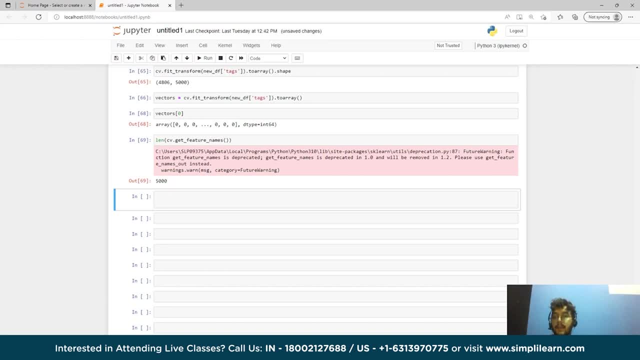 shortly provide you the correct solution. okay, guys, like any code or you are not understand anything, just put as in comment. our team will shortly provide you the correct solution. so let's import some major library which is import NL TK. so what is NL TK? so what is NL TK? 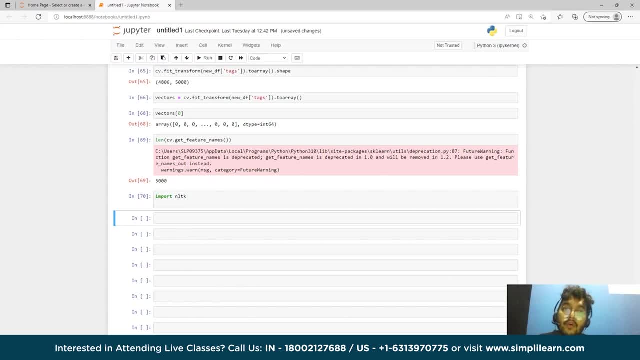 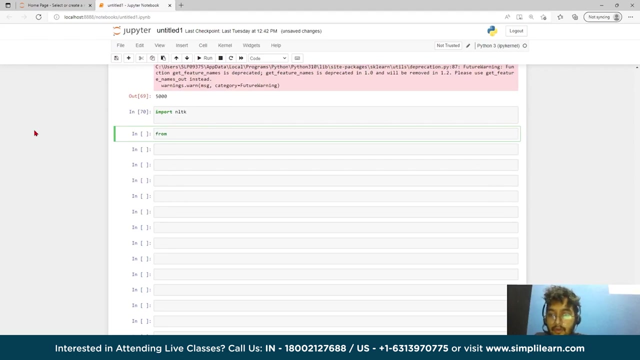 the natural language toolkit. NL TK is a platform used for building Python programs that work with human language, for applying any statical natural language processing NLP. it contained text processing libraries for tokenization, parsing, classification, stemming, tagging and semantic reasoning. so, moving forward like from, let me write first from an NL TK dot. 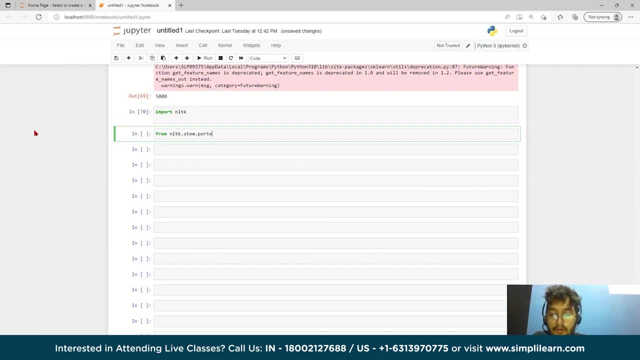 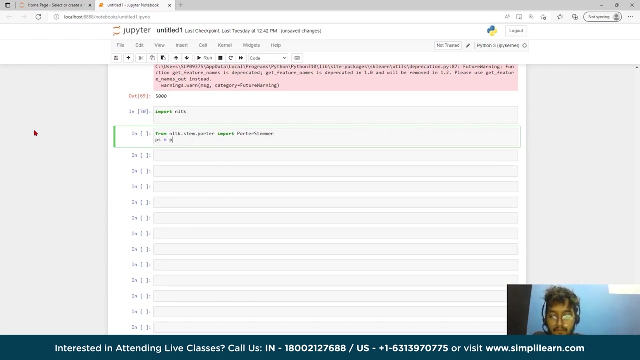 stem dot Porter. import Porter. yes, equals to water. you, you, you, you. Stemming is a process for reducing a word to its word stem, that suffix and prefix, or to the roots of words, known as a lemma. Stemming is important in natural language understanding and natural language processing. 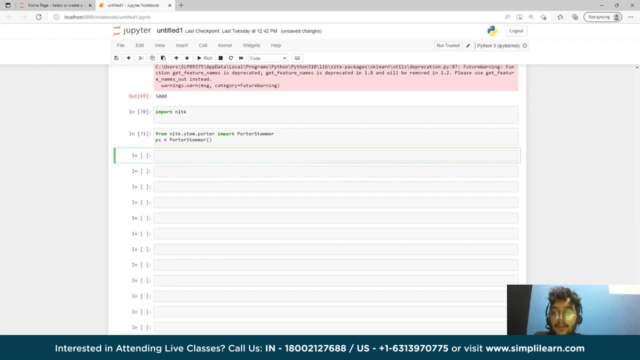 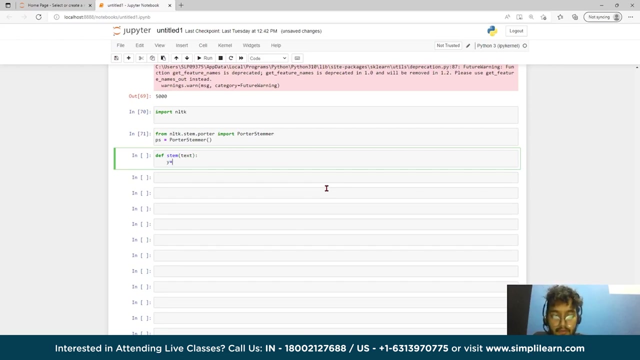 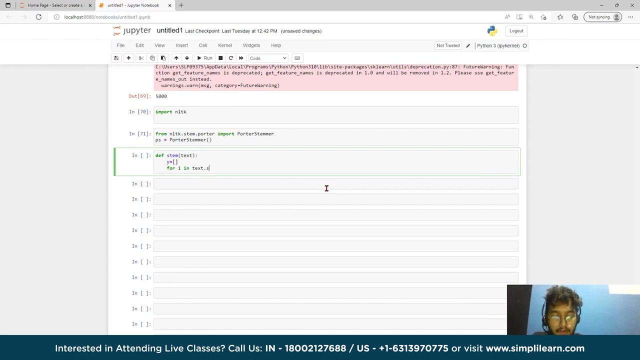 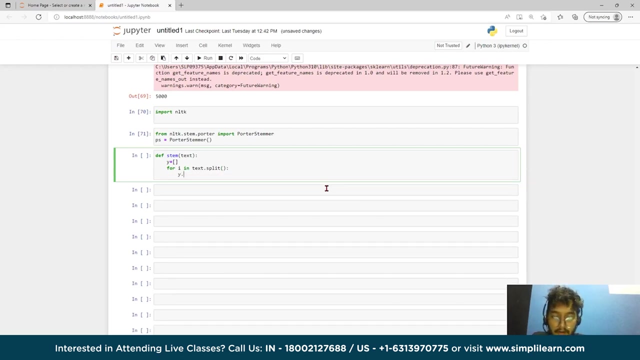 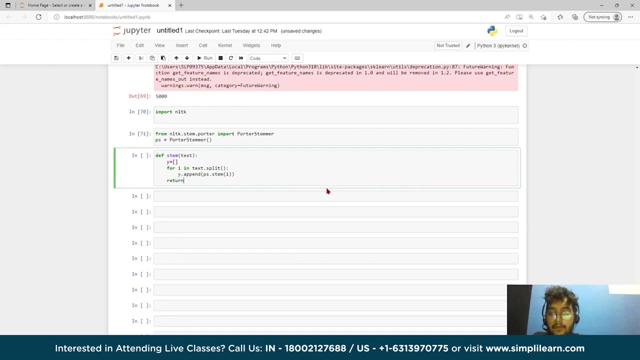 So here, like I have to write, so here I will write def stem to text. y equals to for i in text. dot split y, dot append dot stem done. dot join y. So let's apply stemming to a tag column. So here we will write new df tags. equals to new df tags. dot apply stem. 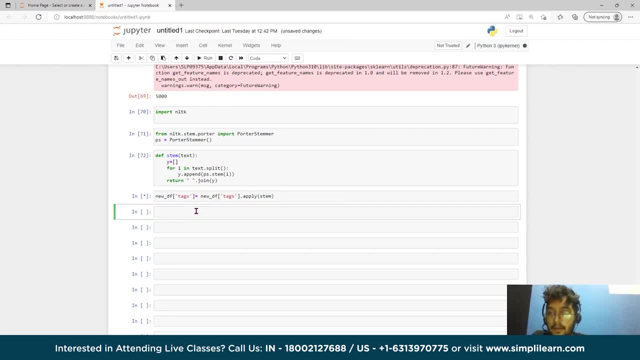 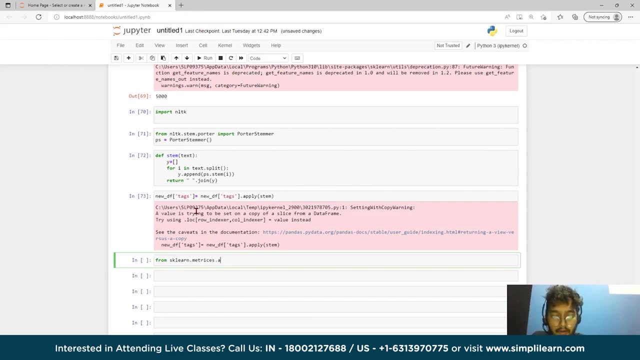 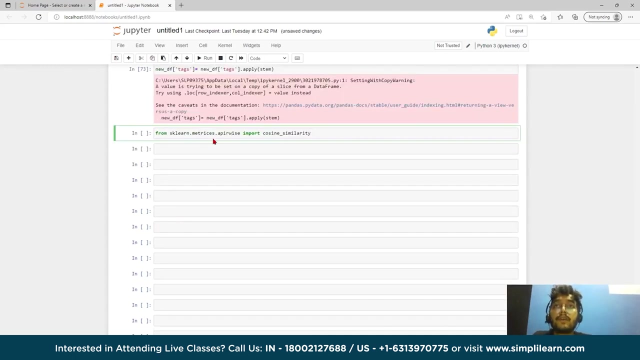 So let's import a cosine similarity from sklearn. So here will write: from sklearn dot, matrices dot. pairwise, import cosine underscore similarity. okay, it seemed good. from sklearn matrices matrix. sorry, matrix dot pairwise, it is pairwise, pairwise import cosine similarity. okay, let's run this no. 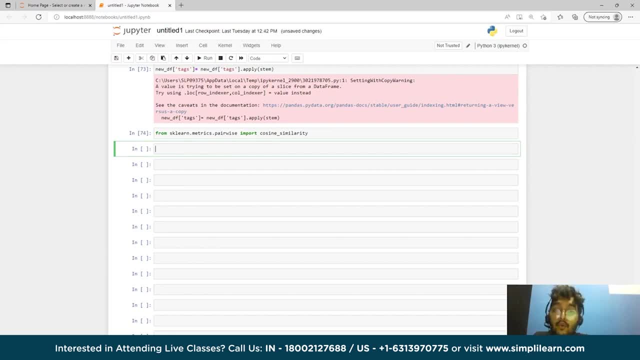 error. so cosine similarity measures the similarity between two factor. I repeat: cosine similarity measures the similarity between two vectors of an inner product space. it is measured by the cosine of the angle between two vectors and determines whether two vectors are pointing in roughly the same direction. it is often used to measure the. 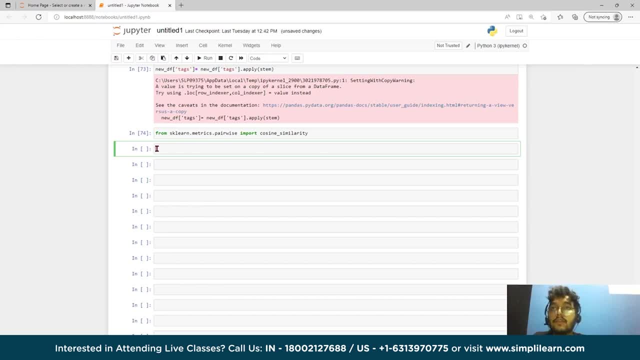 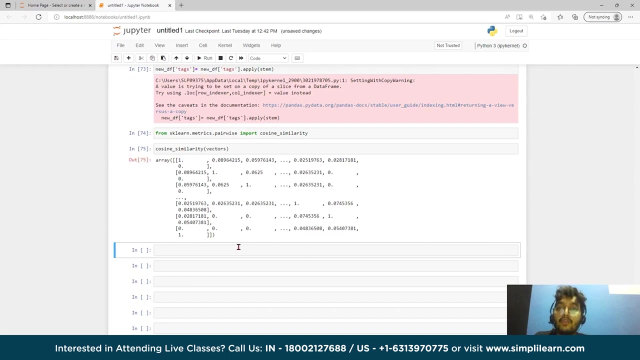 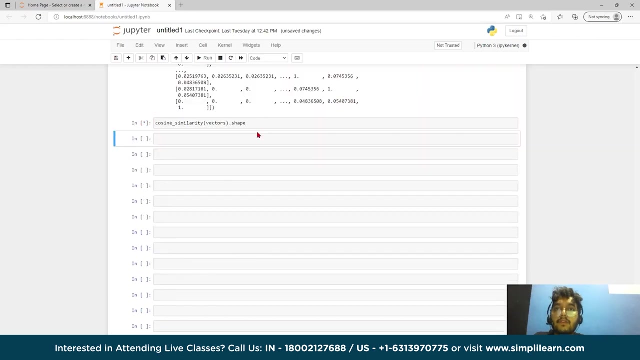 document: similarity in text analysis. so here we will write: cosine underscores- see me Larry T vectors. so these all are the vector present. let's see the cosine similarity vector, column and row using space. so here I will write: cosine similarity vectors: dot shape. it's still running. you can see a. yeah, so for 806 rows and for 806 columns are 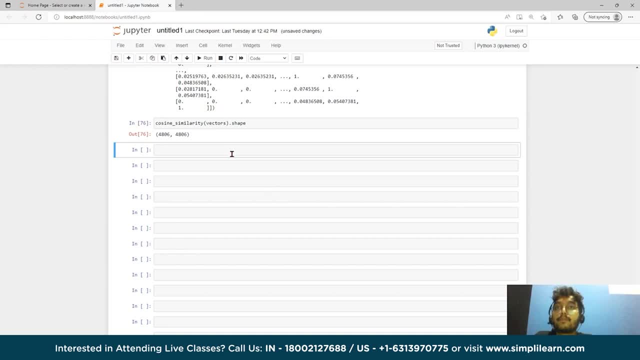 there. yeah, so for 806 rows and for 806 columns are there. so for 806 rows and for 806 columns are there. let's assign variable similarity to this. okay, so let's similarity will write like this: thank you, so cosine similarity underscore here. yeah, I did this because we don't have. why I did this? because we don't have. 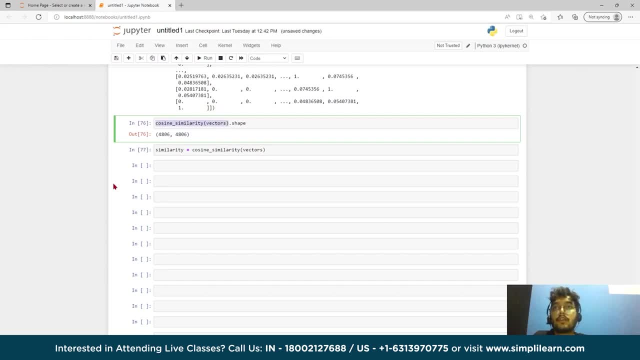 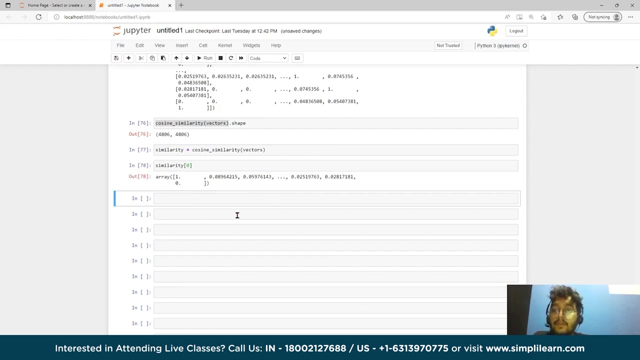 to write always this long sentence, a long keyword. you can say. so moving forward, let's see first column like we will add similarity. so this is our first column. so let's see the rows only. so we will write here: clarity zero, dot shape, 48606. okay, so let's move forward and let's create some like sorted. 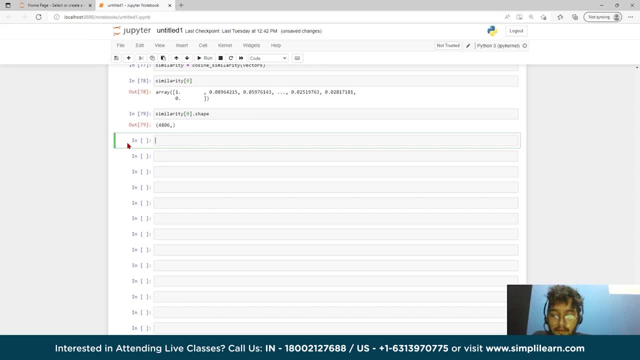 list. so for that sorted list, enumerate spelling is fine. okay, one more like similarity, similarity zero. then i have to write numbers equals to true comma key equals to lambda colon x, not capital x, x. to write one, one colon six, one colon six, one colon six, one colon y. 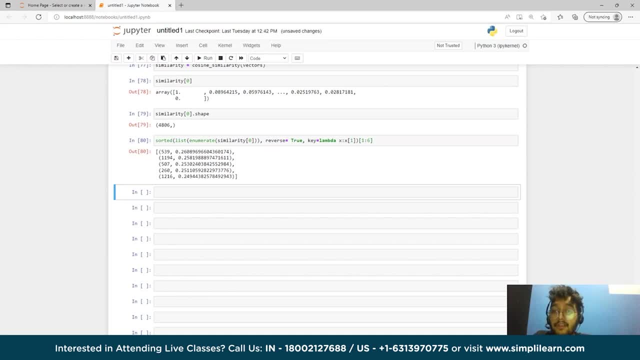 so the enumerate function in python converts a data collection object into an enumerate object. an operate returns an object that contains a counter as a key for each value with an object making inserted in a collection easier to access. so finally, let's create the recommend function to check the movie documentation system. ok, so, so let's start so count the. 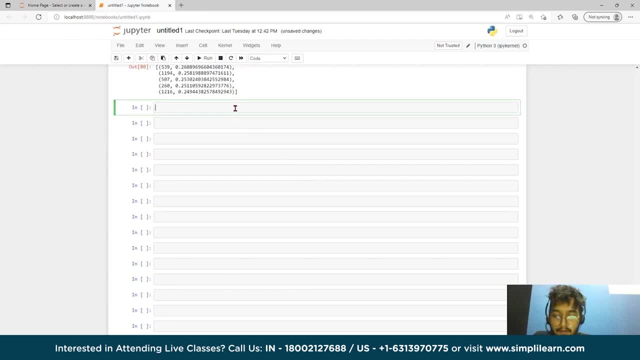 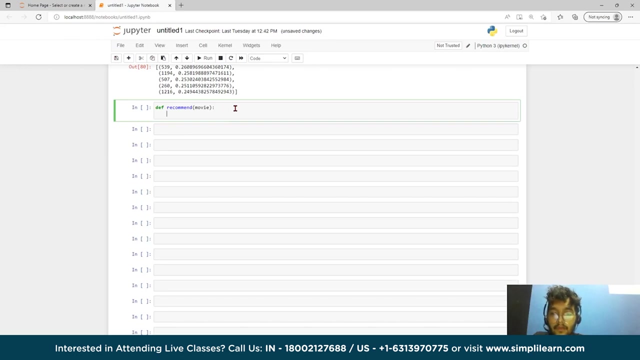 johnson, close the writeränger file and complete all this steps and will prepare um, so let's add an object to it. ok, in floating art, we will add document to it and a number sign got um, So let's write here. df the command v x. 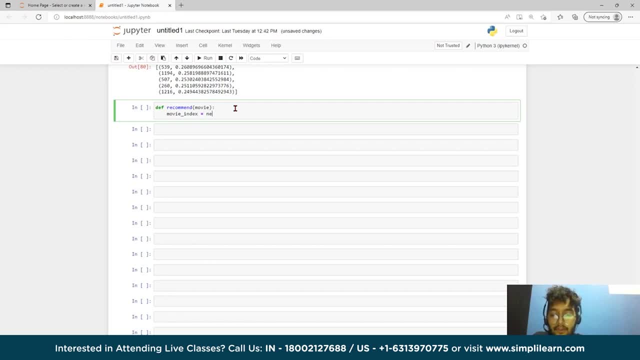 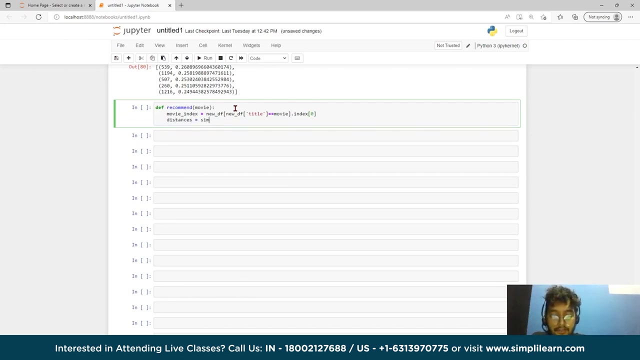 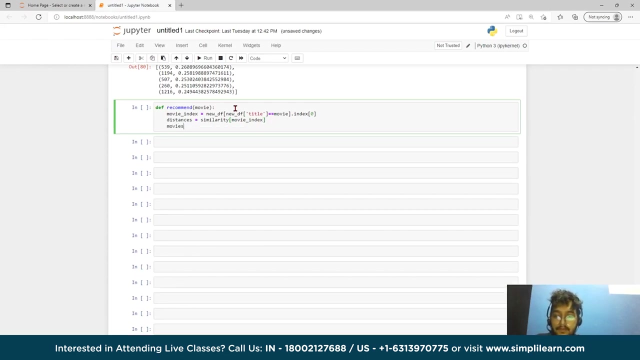 So new df. in the df, title x x, movie x: 0. Tenses Versus similarity and movie. so movies list equals to sorted list. numerate list: r d, t. numerate distances. comma reverse equals to true keyword. sorry, key only. 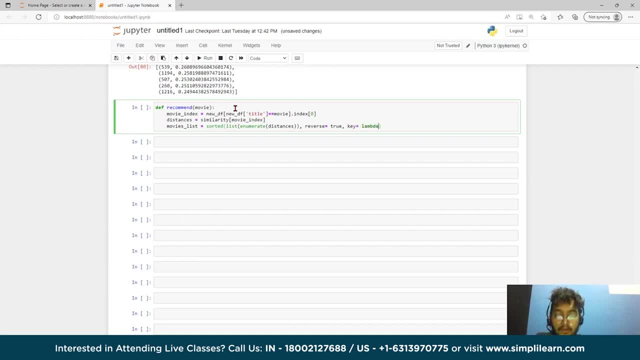 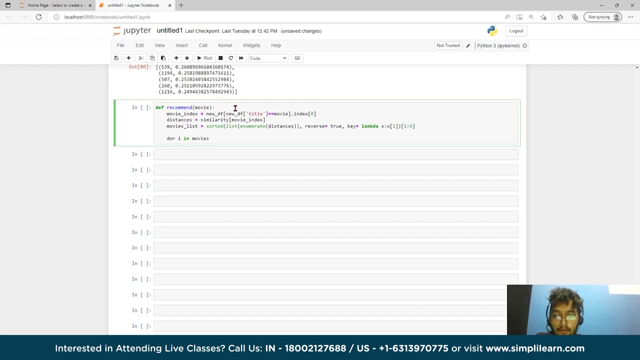 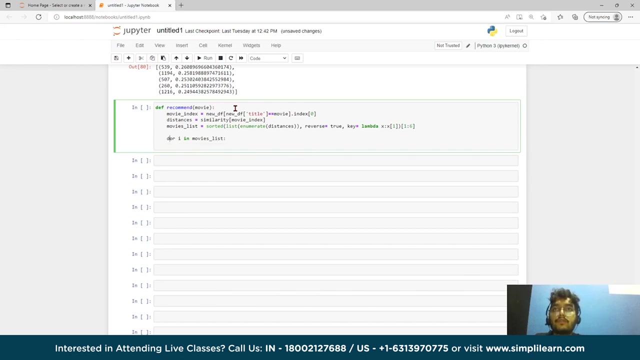 key equals to lambda x, colon x 1, colon six For I in movies list: End, End if dot, I lock I 0 zero dot title because we need title only. so yeah, it seems good, okay, so. 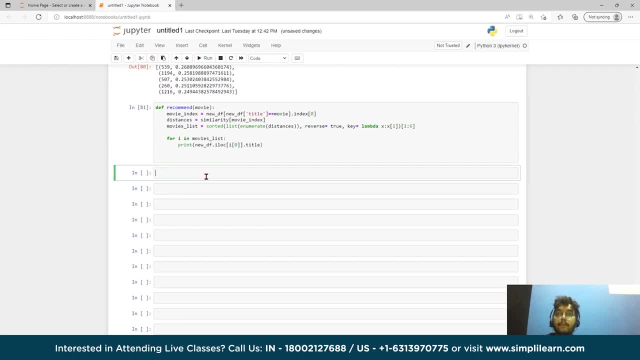 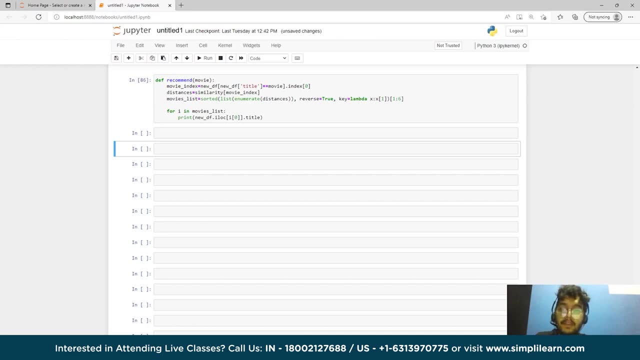 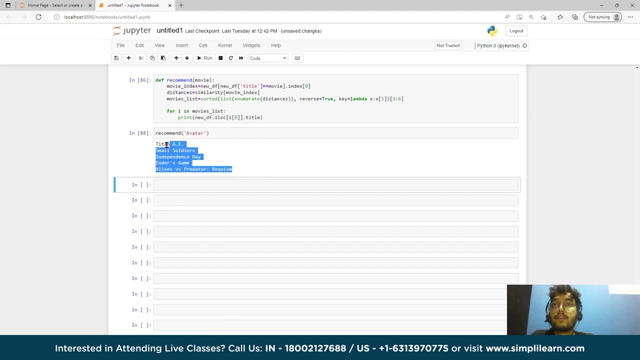 finally that, like time is came. so finally the time has come to check the recommendation of your favorite movies. so you can comment in the chat section, so I can check. so let me write first. recommend recommend for movie Avatar. okay, so here you can see the recommendation system is working fine. so Titan a dot e. 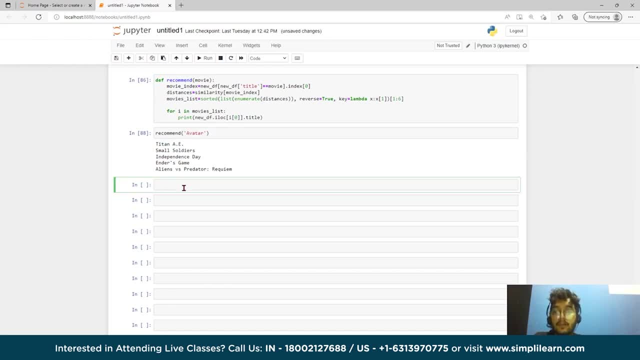 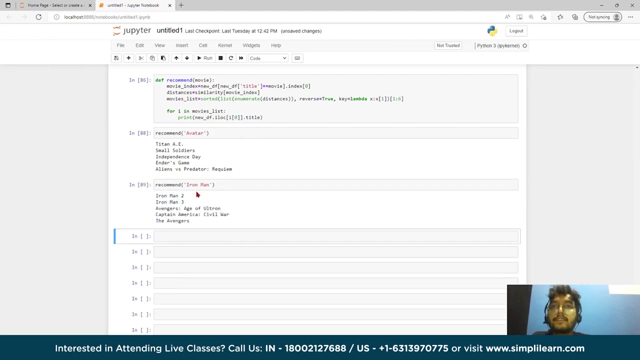 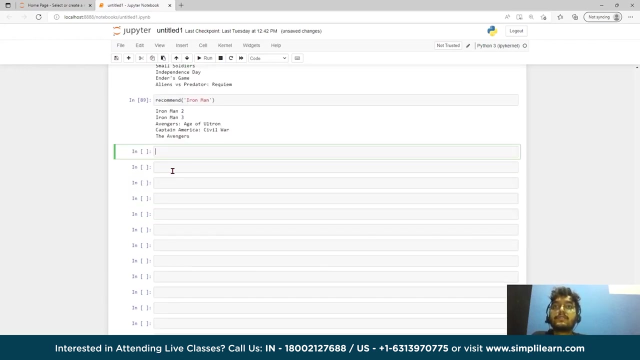 small soldier, independence. they are the recommendation for the movie. after so let me check for the another one recommend like for one of my favorite movie, Iron Man. so here you can see: Iron Man 2, Iron Man 3, Avengers, Age of Ultron. Captain America and the Avengers are the recommendations for the movie. 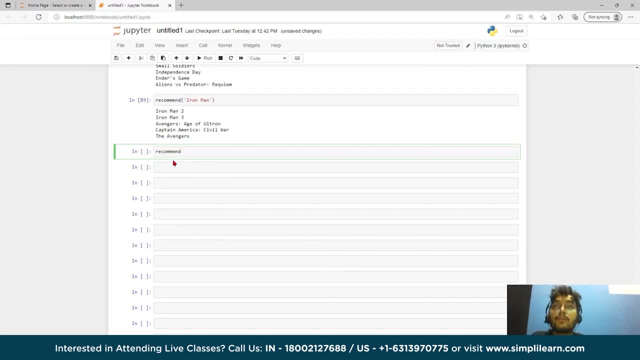 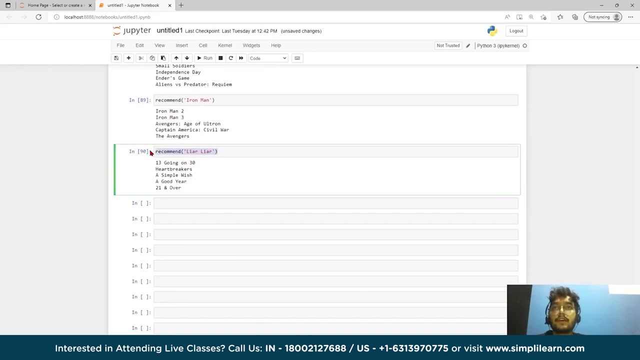 Iron Man. so let me check for the one more recommend della liar queen their eyes. and the last one is started. I want to check: is captain america's Civil War that you can see the captain america the first time inject the winter? so update them three-year-old, wrongly avengers. 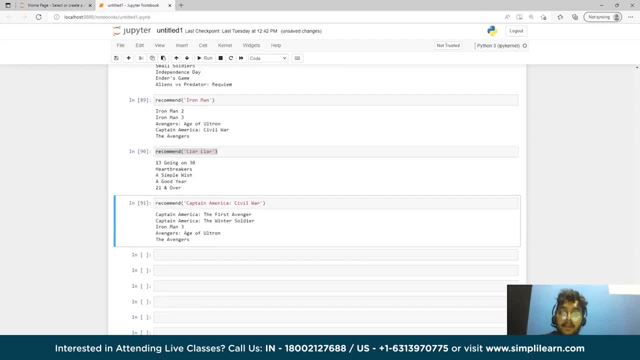 So I hope you guys understand till here. if you have any questions or any query regarding any code or question, just put as in comments. our team will shortly provide you the correct solution. If you want to become an AI expert and gain handsome salary packages, look at the wide 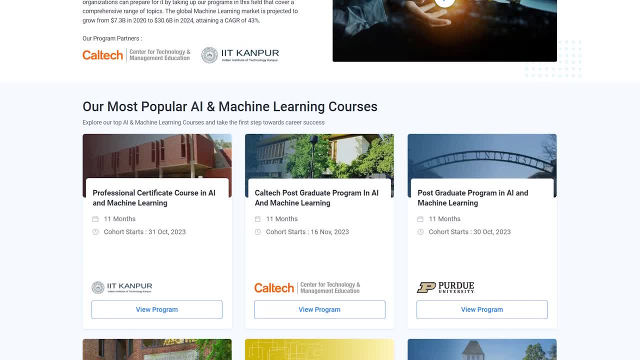 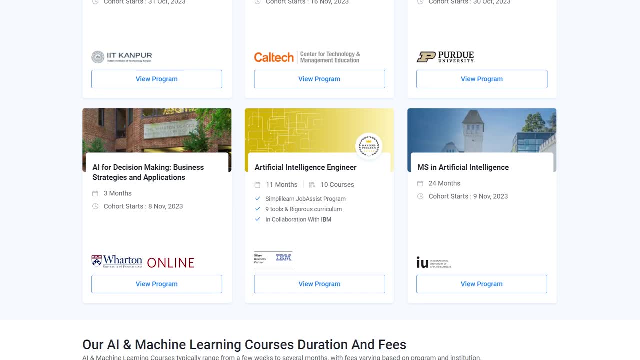 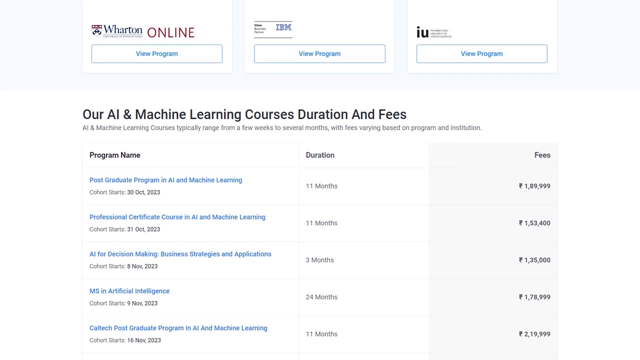 range of AI ML courses by Simrelang, in collaboration with top universities across the globe. By enrolling in any of these certification programs, you will gain expertise in skills like Generative AI, Prompt Engineering, ChatGPT, Explainable AI, Machine Learning Algorithms. 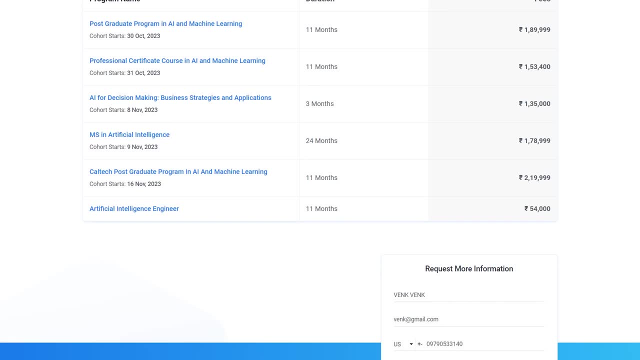 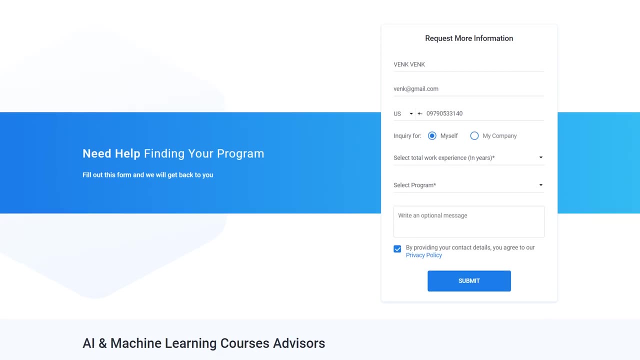 Supervised and Unsupervised Learning, Model Training and Optimization, and there is much more on the list. With hands-on experience in the tools like ChatGPT, DALI, Python, OpenCV and TensorFlow, you will catch the eyes of top recruiters. 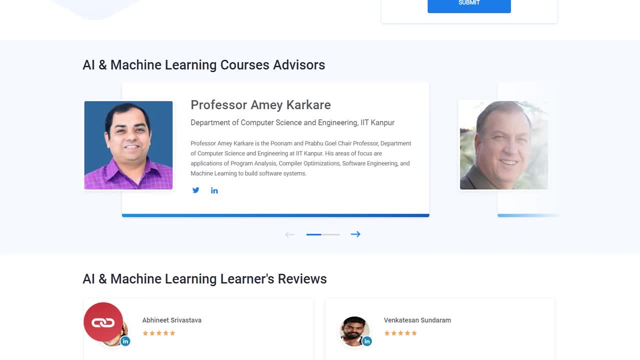 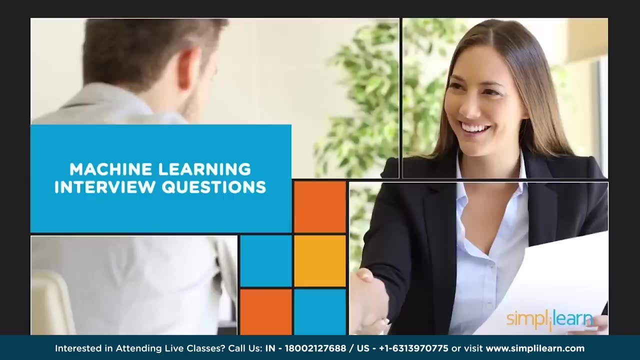 So what are you waiting for? Hurry up and enroll now. An year of experience is preferred to enroll in these courses. Find the course link in the description box. Interview questions for machine learning Now. this video will probably help you when you are attending interviews or machine learning. 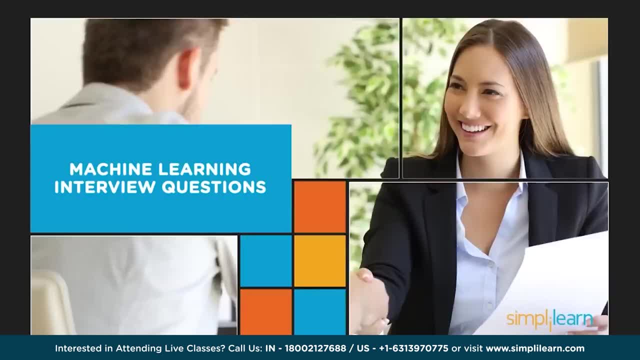 positions, and the attempt here is to probably consolidate 30 most commonly asked questions and to help you in answering these questions. We tried our best to give you the best possible answers, but of course what is more important here is, rather than the theoretical knowledge you need to kind of add to the answers, or 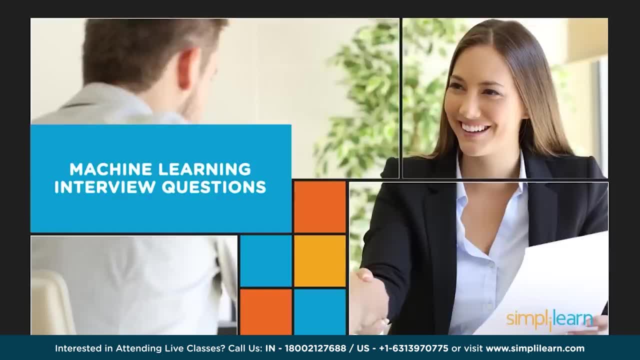 supplement your answers with your own experience. So the responses that we put here are a bit more generic in nature, so that if there are some concepts that you are not clear, this video will help you in kind of getting those concepts cleared up as well. but what is more important is that you need to supplement these. 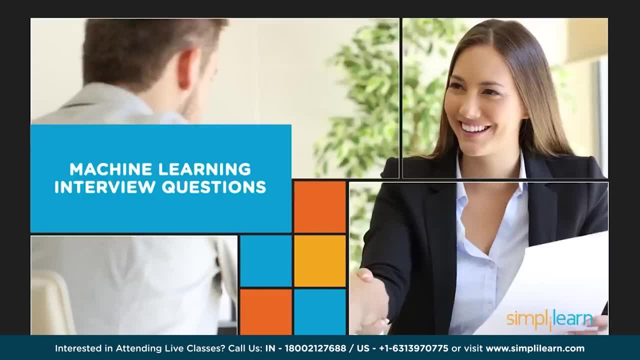 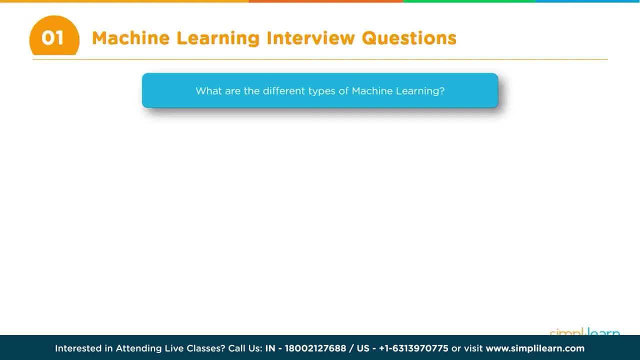 responses with your own experience. So let's get started. So one of the first questions that you may face is: what are the different types of machine learning? Now, what is the best way to respond to this? There are three types of machine learning. 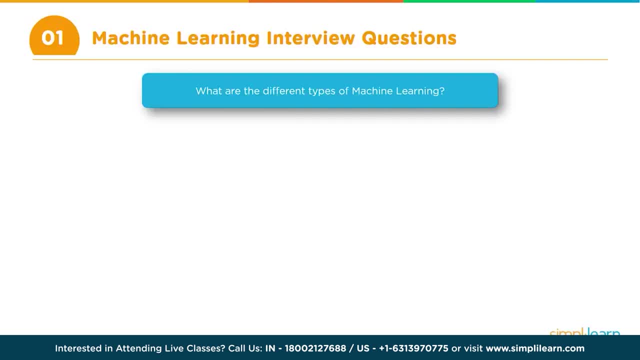 If you read any material, you will always be told that there are three types of machine learning. but what is important is, you would probably be better of emphasizing that there are actually two main types of machine learning. So the first one is machine learning. 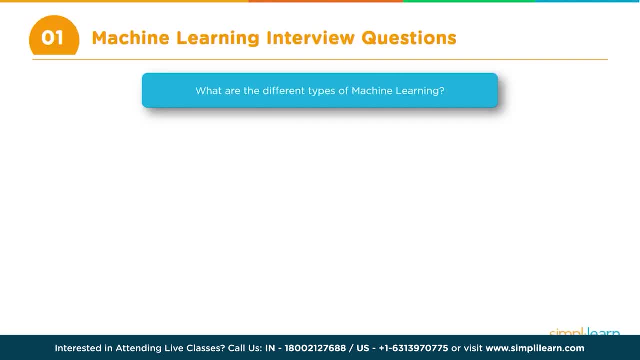 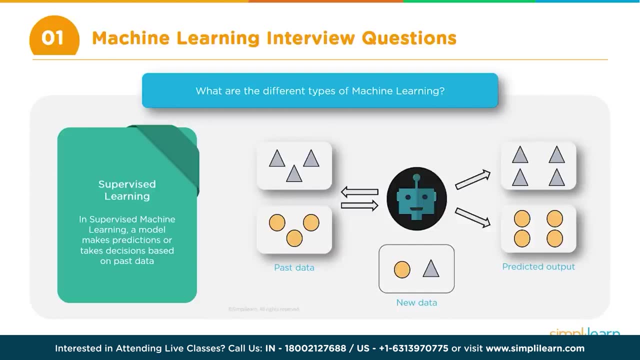 Which is supervised and unsupervised. and then there is a third type, which is reinforcement learning. So supervised learning is where you have some historical data and then you feed that data to your model to learn. Now you need to be aware of a key word that they will be looking for, which is labeled. 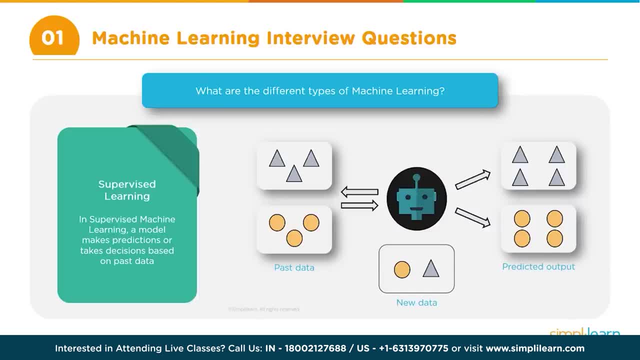 data. So if you just say past data or historical data, the impact may not be so much. you need to emphasize on labeled data. So what is labeled data Basically? let's say, if you are trying to do training model for classification, you 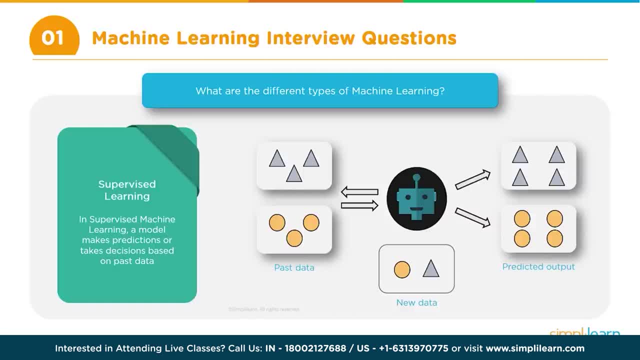 need to be aware of all your existing data. which class each of the observations belong to right. So that is what is labeling, So it is nothing but a fancy name. you must be already aware. But just make it a point to throw in that keyword labeled, so that will have the right. 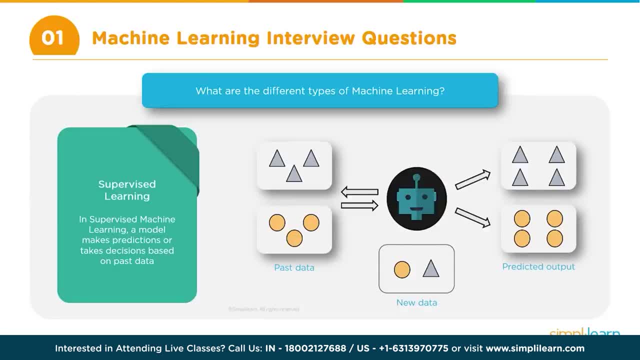 impact. Okay, So that is what is supervised learning When you have existing labeled data. So that is what is supervised learning When you have existing labeled data, which you then use to train your model. that is known as supervised learning. 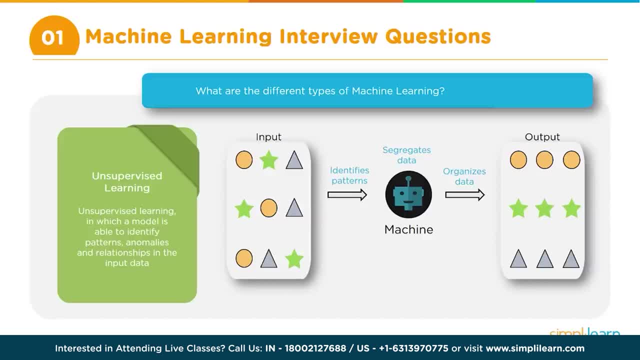 And unsupervised learning is when you don't have this labeled data. So you have data. it is not labeled, So the system has to figure out a way to do some analysis on this. Okay, So that is unsupervised learning. 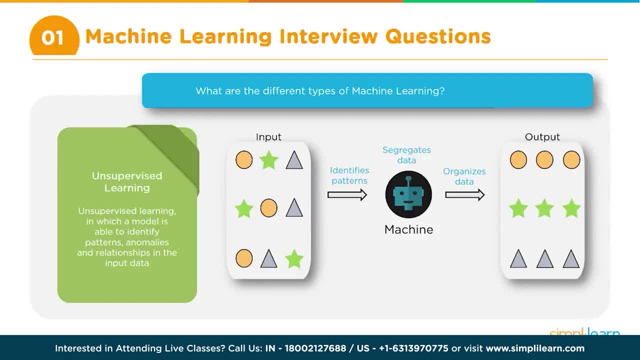 And you can then add a few things like what are the ways of performing supervised learning and unsupervised learning, or what are some of the techniques. Okay, So we perform or we do regression and classification and unsupervised learning, we do clustering. 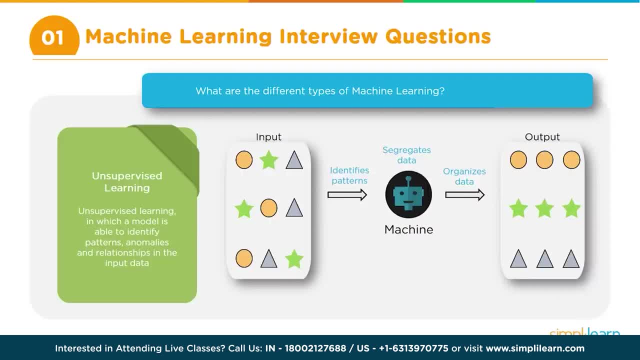 Okay, And clustering can be of different types. Similarly, regression can be of different types. but you don't have to probably elaborate so much If they are asking for just the different types. you can just mention these, and just at a very high level. 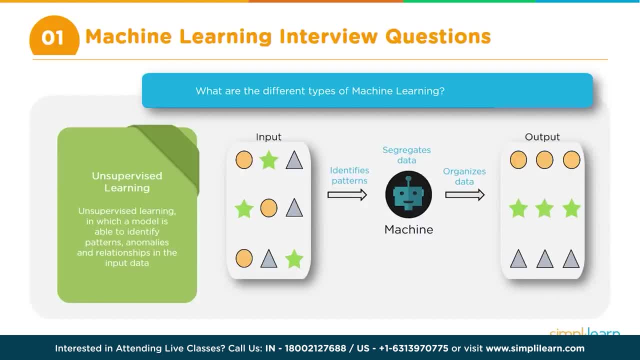 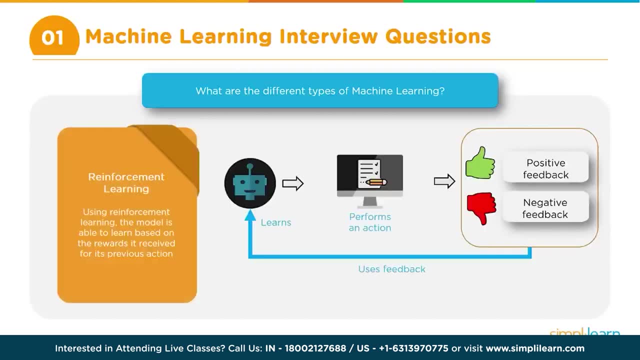 But if they want you to elaborate, give examples, then of course I think there is a different question for that. We will see that later. Then the third: So we have supervised, then we have unsupervised, and then reinforcement you need to provide. 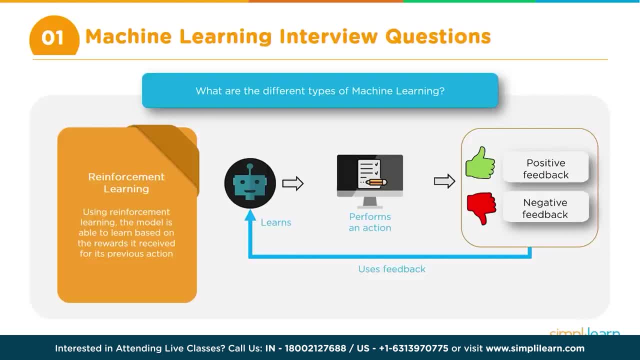 a little bit of information around that as well, because it is sometimes a little difficult to come up with a good definition for reinforcement learning, So you may have to a little bit elaborate on how reinforcement learning works, Right? So reinforcement learning works in such a way that it basically has two parts to it. 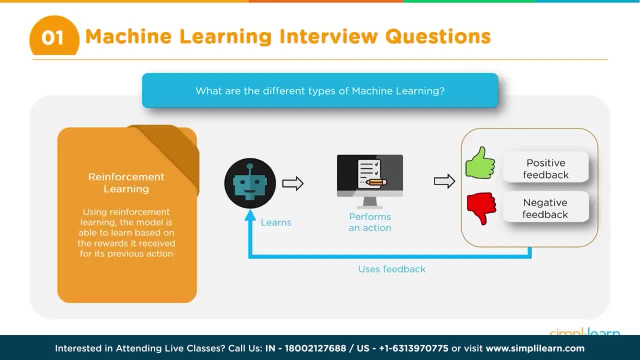 One is the agent and the environment, and the agent basically is working inside of this environment. So the agent is given a target that it has to achieve and every time it is moving in the direction of the target, so the agent basically has to take some action and every 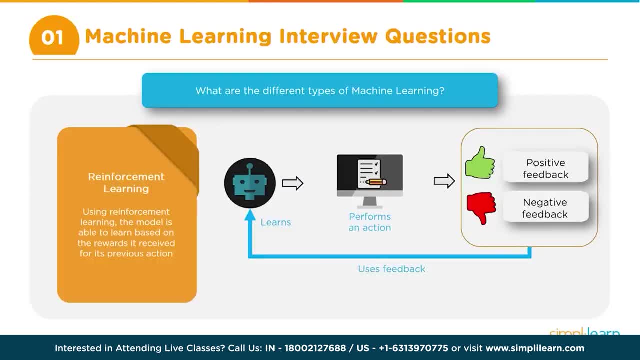 time it takes an action which is moving the agent towards the target, towards a goal- a target is nothing but a goal- then it is rewarded, And every time it is going in a direction where it is away from the goal, then it is. 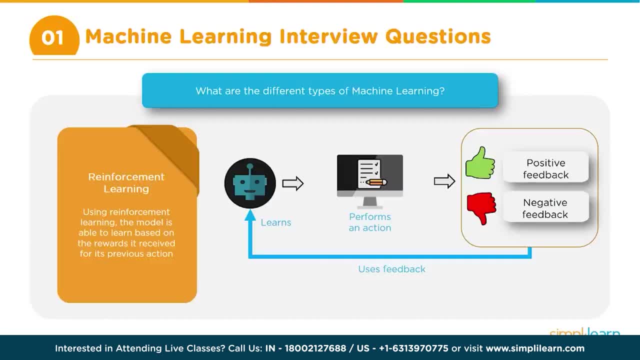 punished. So this is the way you can leave it explained and this is used primarily or very, very impactful for teaching the system to learn games and so on. Examples of this are basically used in AlphaGo. You can throw that as an example, where AlphaGo used reinforcement learning to actually learn. 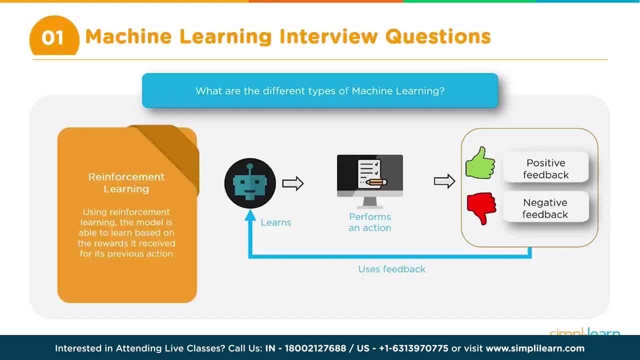 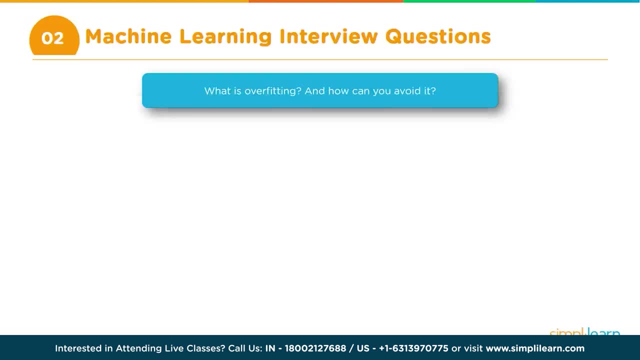 to play the game of Go and finally it defeated the Go world champion. Right, This much of information? that would be good enough. Okay, So there could be a question on overfitting. So the question could be: what is overfitting and how can you avoid it? 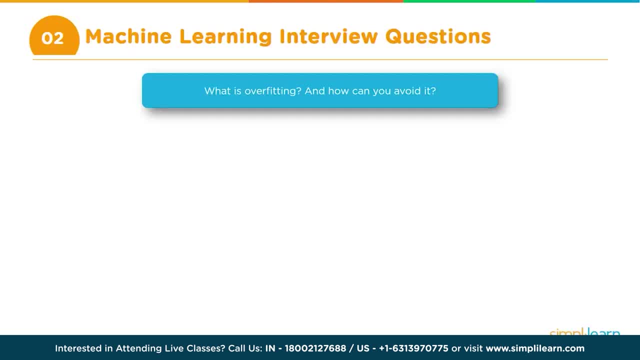 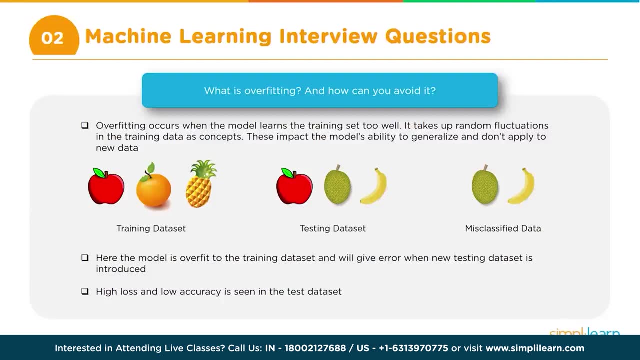 So what is overfitting? Let's first try to understand the concept, because sometimes overfitting may be a little difficult to understand. Overfitting is a situation where the model has kind of memorized the data. So this is an equivalent of memorizing the data. 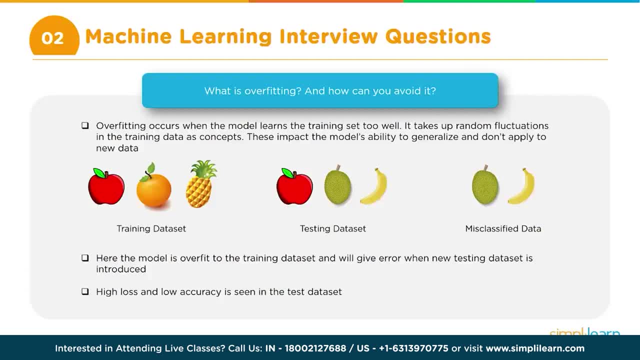 So we can draw an analogy so that it becomes easy to explain this. Now, let's say you're teaching a child about recognizing some fruits or something like that. Okay, And you're teaching this child about recognizing, let's say, three fruits: apples, oranges. 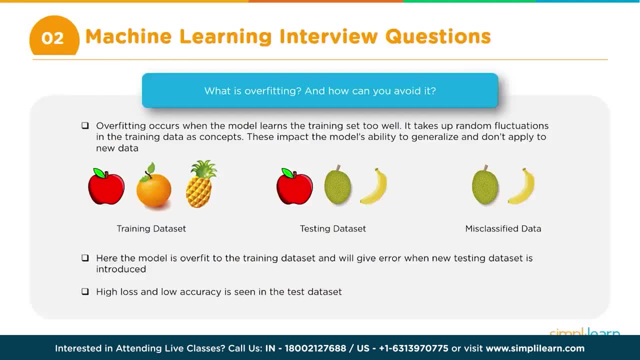 and pineapples. Okay, So this is a small child and for the first time, you're teaching the child to recognize fruits Then, so what will happen? So this is very much like that is your training data set. 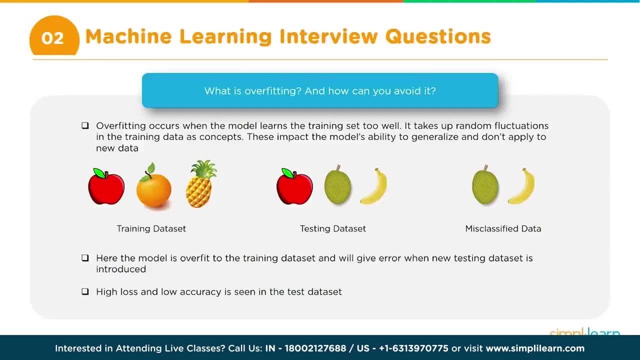 So what you will do is you will take a basket of fruits which consists of apples, oranges and pineapples, Okay, And you take this basket to this child, and there may be, let's say, hundreds of these fruits. 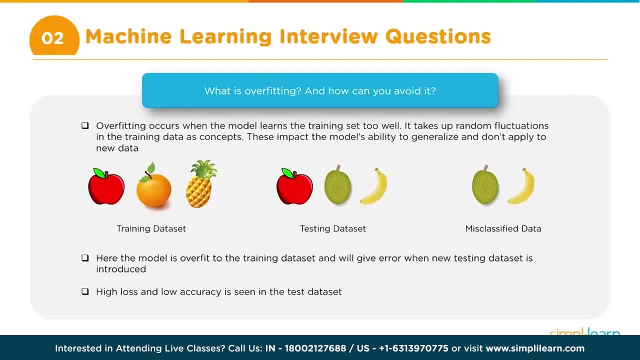 So you take this basket to this child and keep showing each of this fruit, and then first time, obviously, the child will not know what it is. So you show an apple and you say: hey, this is apple. Then you show maybe an orange and say: this is orange, and so on and so forth. 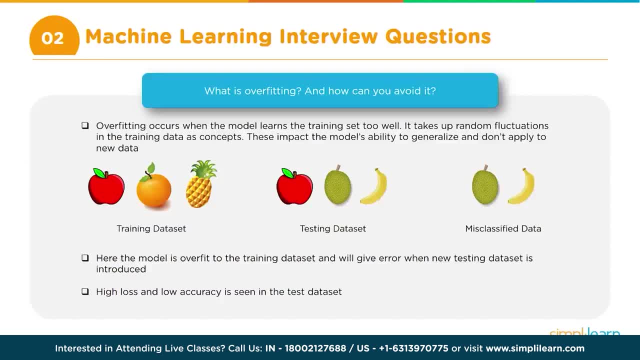 And then again you keep repeating that right. So until that basket is over. This is basically how training works in machine learning also. That's how training works. Until the basket is completed- maybe 100 fruits- you keep showing this child. 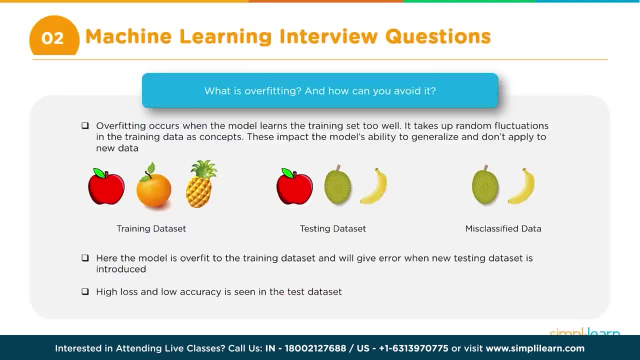 In the process. what has happened? The child has pretty much memorized these. So even before you finish that basket right, By the time you are halfway through, the child has learned about recognizing the apple, orange and pineapple. Now what will happen after halfway through? 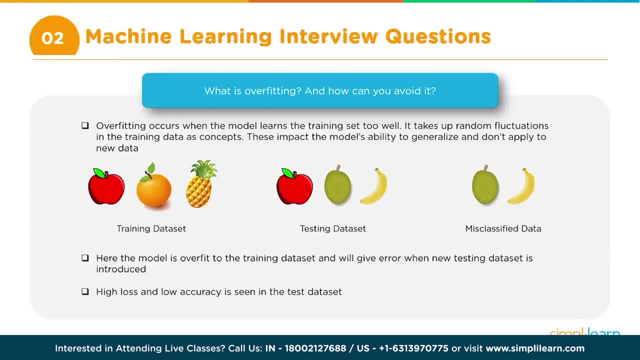 Initially, you remember, it made mistakes in recognizing, but halfway through now it has learned. So every time you show a fruit, it will exactly, 100%, accurately, It will recognize it. Okay, It will identify it. It will say the child will say: this is an apple. 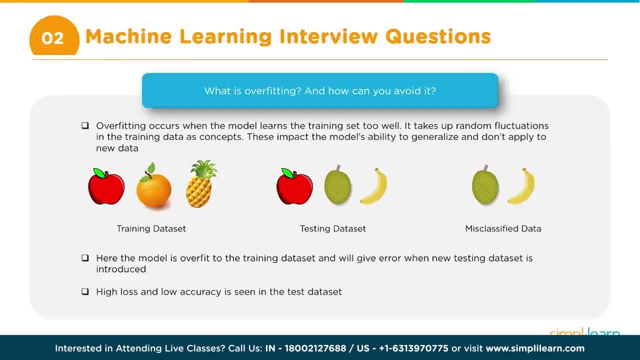 This is an orange, And if you show a pineapple it will say this is a pineapple, right? So that means it has kind of memorized this data. Now let's say you bring another basket of fruits and it will have a mix of maybe apples. 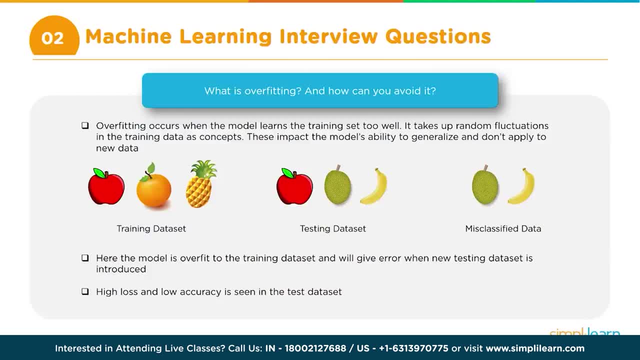 which were already there in the previous set, But it will also have, in addition to apple, it will probably have a banana or maybe another fruit like a jackfruit, right? So this is an equivalent of your apple, This is an equivalent of your test data set, which the child has not seen before. 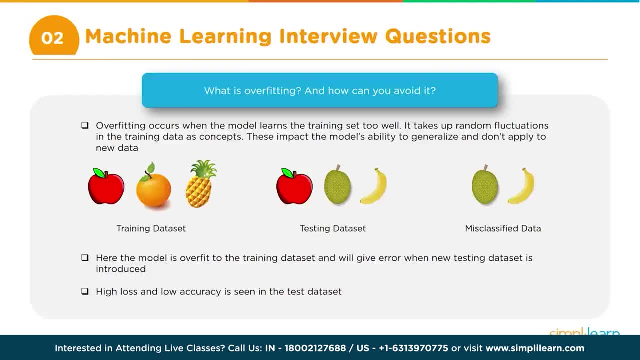 Some parts of it it probably has seen, like the apples it has seen, But this banana and jackfruit it has not seen. So then, what will happen In the first round, which is an equivalent of your training data set towards the end? 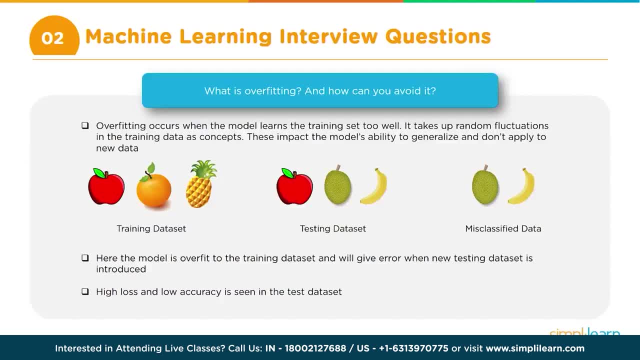 it has 100%. it was telling you what the fruits are right: Apple was accurately recognized, orange was accurately recognized and pineapples were accurately recognized, right. So that is like 100% accuracy. But now, when you get another fresh set which were not part of the original one, what will? 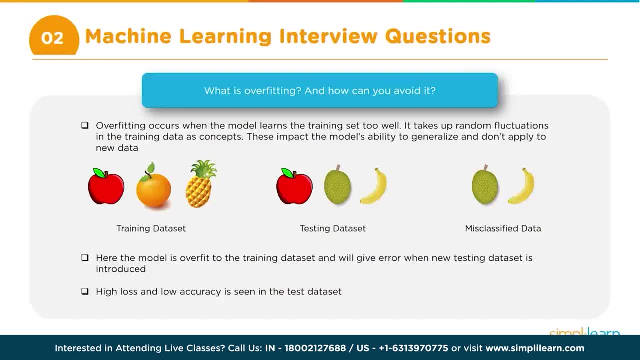 happen. All the apples maybe it will be able to recognize correctly, but all the others, like the jackfruit or the banana, will not be recognized by the child, right? So this is an analogy. This is an equivalent of overfitting. 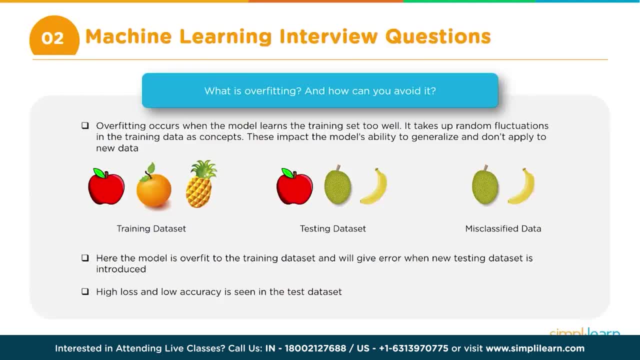 So what has happened During the training process? it is able to recognize or reach 100% accuracy, maybe very high accuracy, okay, And we call that as very low loss, right? So that is the technical definition, So that is the technical term. 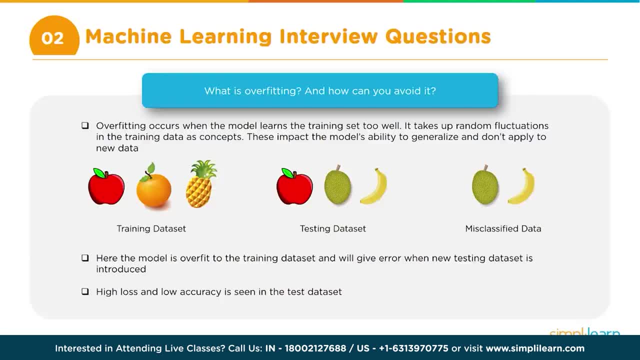 So the loss is pretty much zero and accuracy is pretty much 100%, Whereas when you use testing, there will be a huge error, which means the loss will be pretty high and therefore the accuracy will be also low. okay, This is known as overfitting. 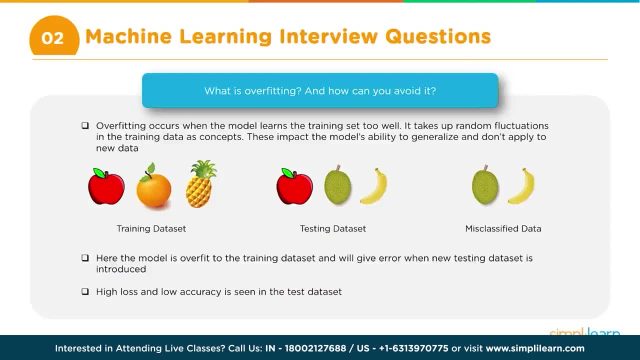 This is basically a process where training is done. training processes. it goes very well, almost reaching 100% accuracy, but while testing it really drops down. Now how can you avoid it? So that is the extension of this question. 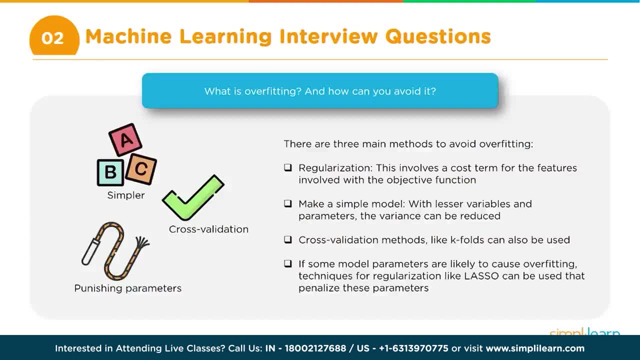 There are multiple ways of avoiding overfitting. There are techniques like what we call regularization. That is the most common technique that is used for avoiding overfitting, And within regularization there can be a few other subtypes, like dropout in case of. 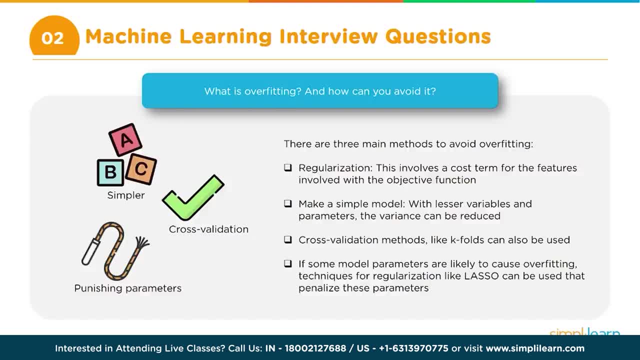 neural networks and a few other examples. But I think if you give example or if you give regularization as the technique, probably that should be sufficient. So there will be some questions where the interviewer will try to test your fundamentals and your knowledge and depth of knowledge and so on and so forth. 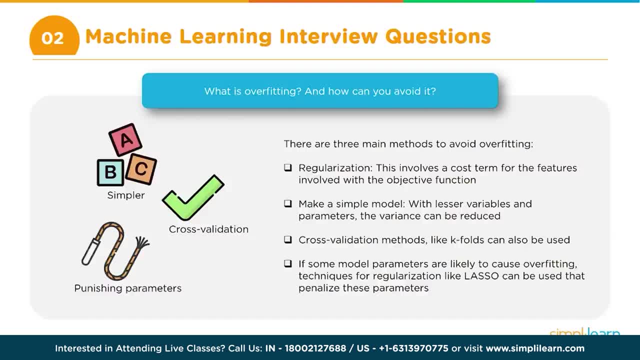 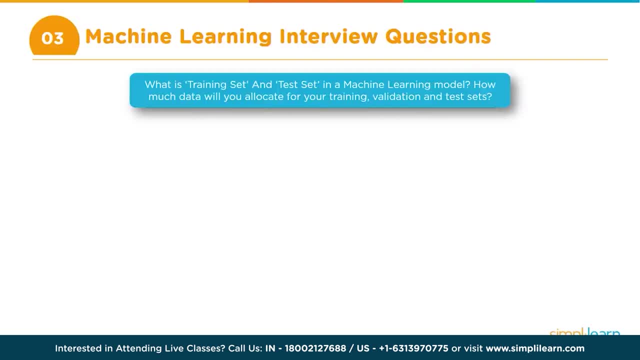 And then there will be some questions which are more like quick questions. that will be more to stump you. Okay, then the next question is around the methodology. So when we are performing machine learning training, we split the data into training and test, right? 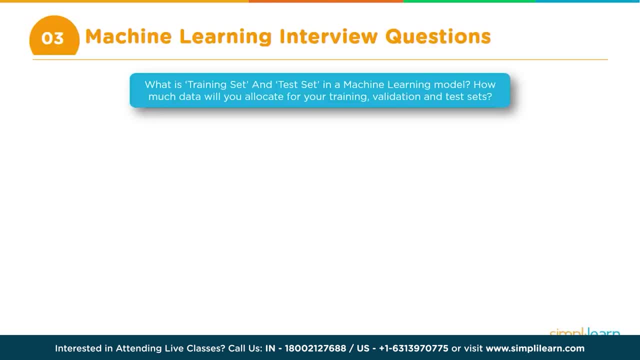 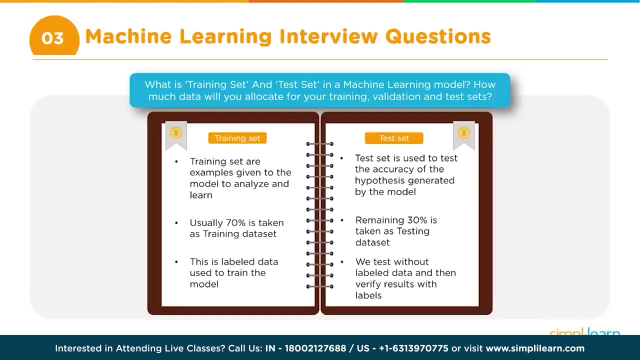 So this question is around that. So the question is: what is training set and test? What is training set and test set in machine learning model And how is the split done? So the question can be like that: So in machine learning, when we are trying to train the model, 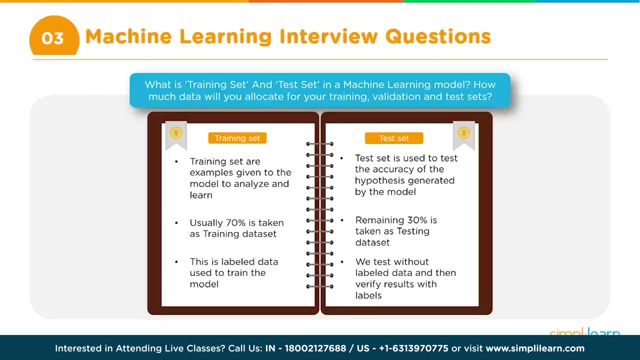 So we have a three-step process: We train the model and then we test the model And then, once we are satisfied with the test, only then we deploy the model. So what happens in the train and test is that you remember the labeled data. 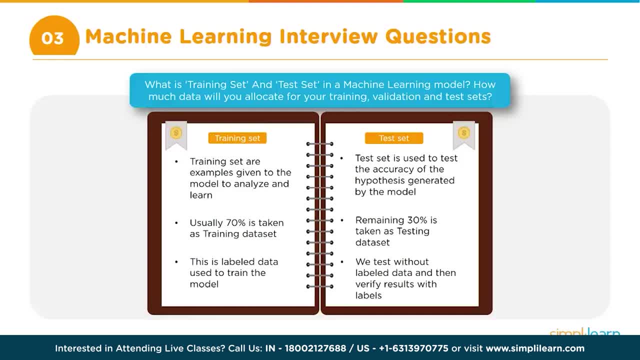 So let's say you have- Let's say you have- thousand records with labeling information. Now, one way of doing it is you use all the thousand records for training and then maybe right, Which means that you have exposed all this thousand records during the training process. 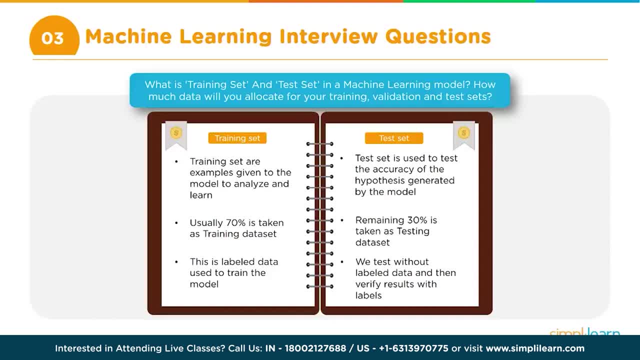 And then you take a small set of the same data and then you say, okay, I will test it with this, Okay, And then you probably what will happen. You may get some good results right, But there is a flaw there. 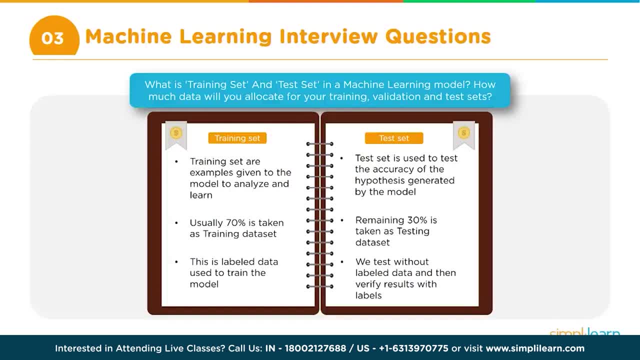 What is the flaw? This is very similar to human beings. It is like you are showing this model, the entire data, as a part of training. Okay, So obviously it has become familiar with the entire data. So when you are taking a part of that again and you are saying that, I want to test it. 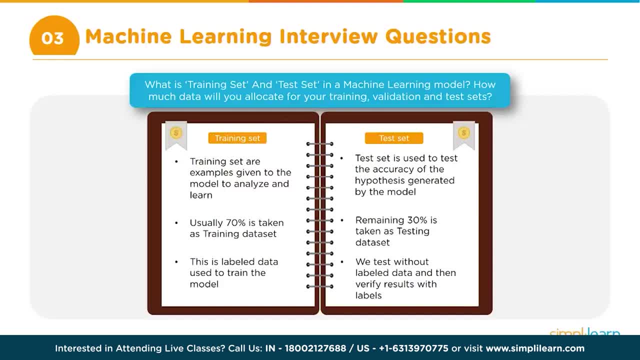 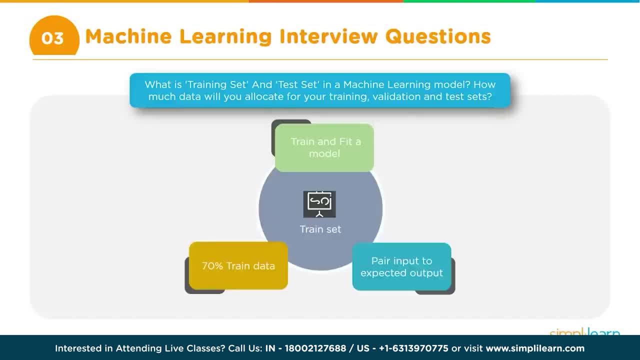 obviously you will get good results. So that is not a very accurate way of testing. So that is the reason what we do is we have the label data of this thousand records or whatever We set aside before starting the training process. 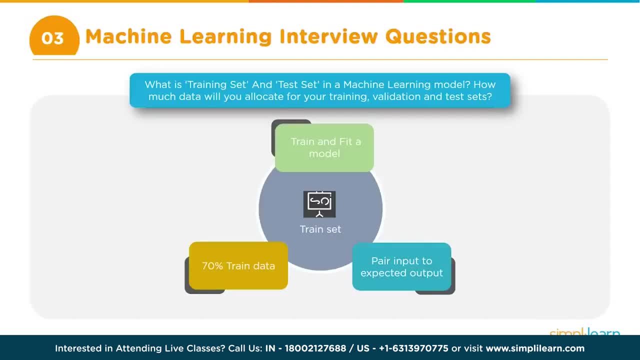 We set aside a bunch, We set aside a portion of that data and we call that test set and the remaining we call as training set and we use only this for training our model. Now, the training process, remember, is not just about passing one round of this data set. 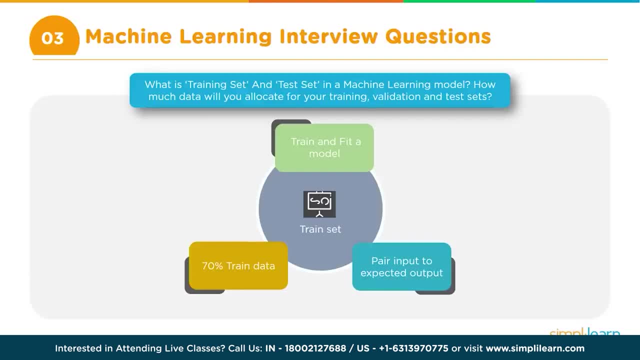 So let us say now your training set has 800 records. It is not just one time you pass this 800 records. What you normally do is you actually, as a part of the training, you may pass this data through the model multiple times. 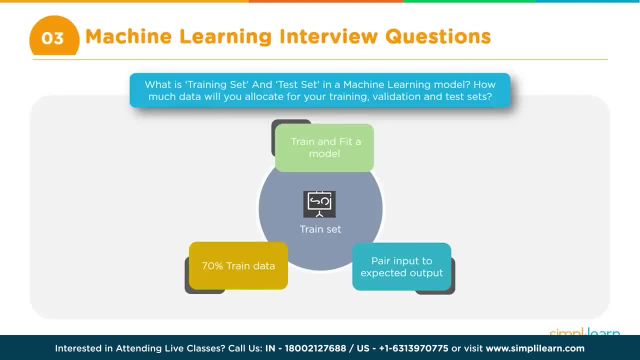 So this thousand records may go through the model, maybe 10,, 15,, 20 times. till the training is perfect, till the accuracy is high, till the errors are minimized. Okay Now so, which is fine, which means that your- that is what is known as the model- has seen. 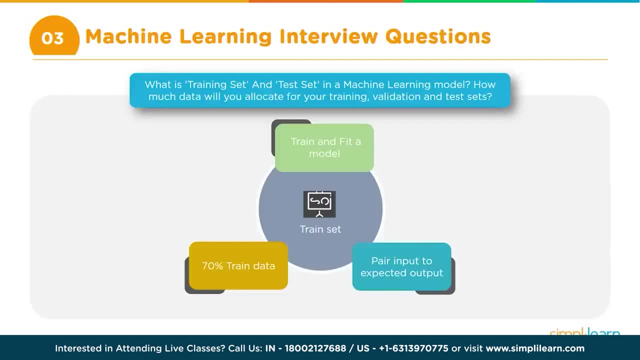 your data and gets familiar with your data. And now, when you bring your test data, what will happen is: this is like some new data, because that is where the real test is. Now you have trained the model and now you are testing the model with some data. 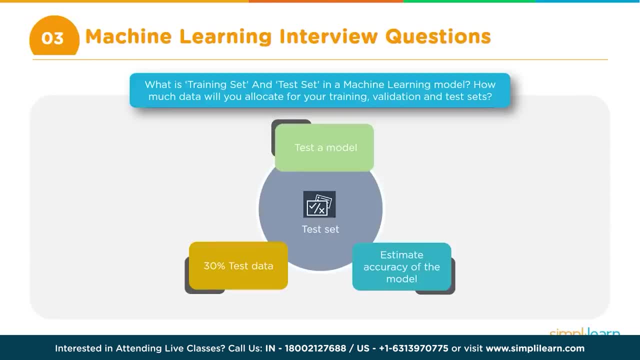 Which is kind of new. That is like a situation, like a realistic situation, because when the model is deployed, that is what will happen: It will receive some new data, not the data that it has already seen. Right, So this is a realistic test. 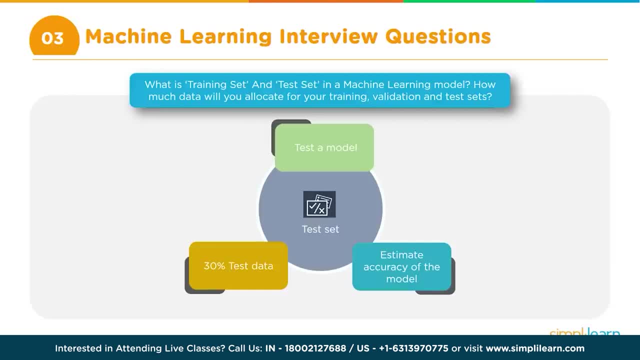 So you put some new data. So this data which you have set aside is for the model. It is new And if it is able to accurately predict the values, that means your training has worked. Okay, The model got trained properly. 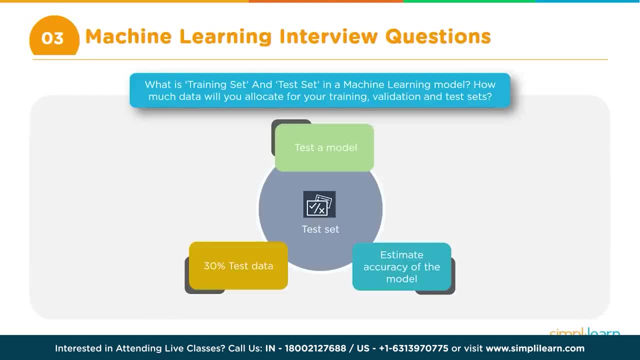 But let us say, while you are testing this with this test data, you are getting a lot of errors. Okay, That means you need to probably either change your model or retrain with more data and things like that. Now coming back to the question of how do you split this. 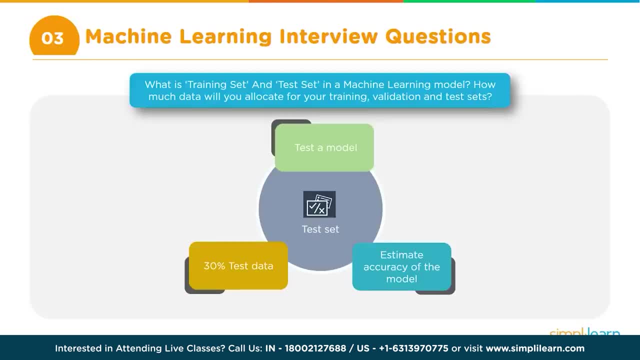 What should be the ratio? There is no fixed number. Again, this is like individual preferences. Some people split it into 50-50.. 50% test and 50% training. Some people prefer to have a larger amount for training and a smaller amount for test. 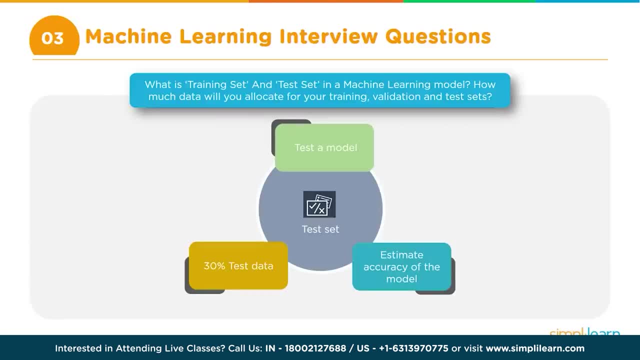 So they can go by either 60-40 or 70-30.. Or some people even go with some odd numbers like 65-35 or 63.33 and 33, which is like one-third and two-third. So there is no fixed rule that it has to be something. 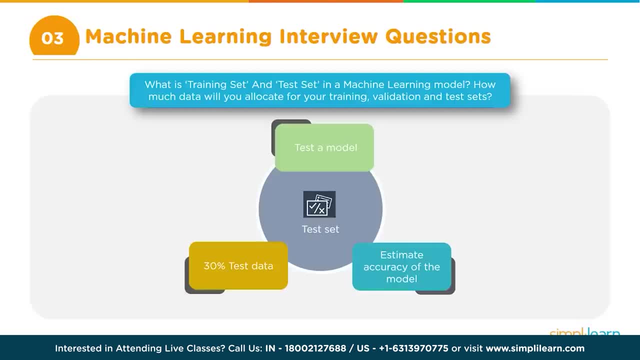 The ratio has to be this: You can go by your individual preferences, All right. Then you may have questions around data handling, data manipulation, or what do you call data management or preparation. So these are all some questions around that area. There is again, no one answer. 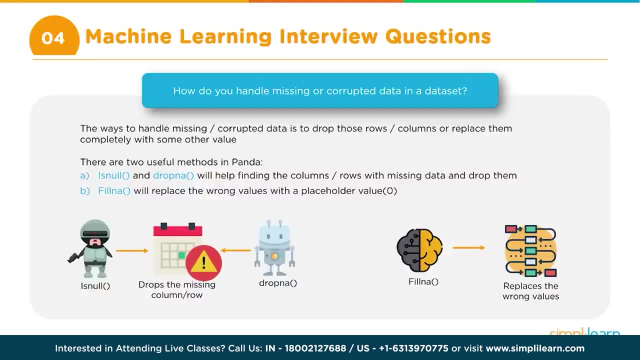 One single good answer to this. It really varies from situation to situation And depending on what exactly is the problem, what kind of data it is, how critical it is, what kind of data is missing and what is the type of corruption. So there are a whole lot of things. 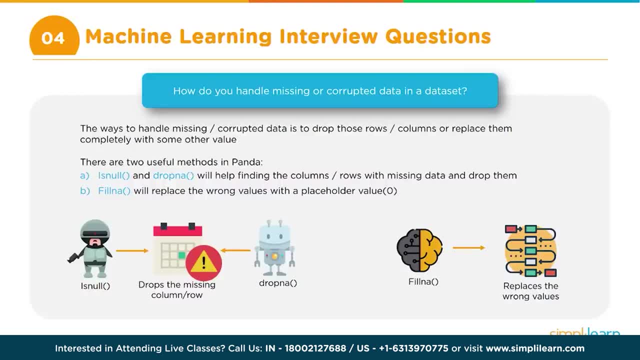 This is a very generic question And therefore you need to be a little careful about responding to this as well, So probably have to illustrate this again. If you have experience in doing this kind of work in handling data, you can illustrate with this. 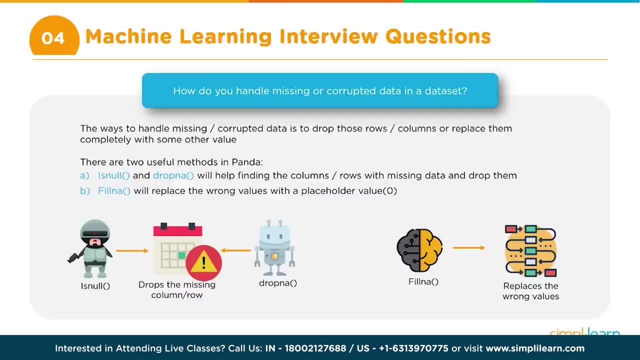 For example, saying that I was on one project where I received this kind of data. These were the columns where data was not filled, or these were this many rows where the data was missing. That would be, in fact, a perfect way to respond to this question. 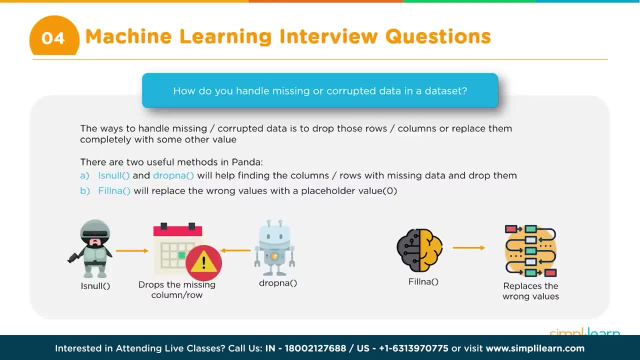 But if you don't have that, obviously you have to provide some good answer. I think it really depends on what exactly the situation is, And there are multiple ways of handling the missing data or corrupt data. Now let's take a few examples. 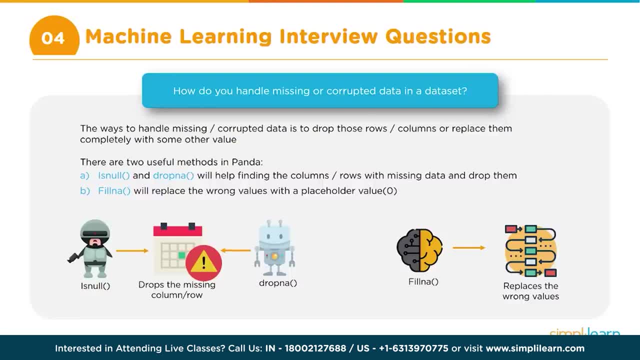 Now, let's say you have data where some values in some of the columns are missing and you have pretty much half of your data having these missing values in terms of number of rows. Okay, that could be one situation. Another situation could be that you have records or data missing. 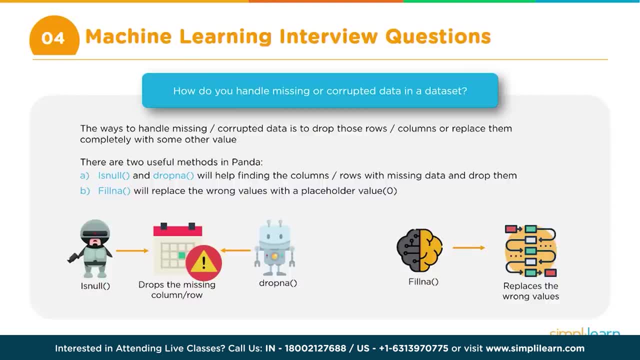 But when you do some initial calculation, how many records are corrupt, or how many rows or observations, as we call it, has this missing data? Let's assume it is very minimal, like 10 percent. Okay, Now, between these two cases, how do you? 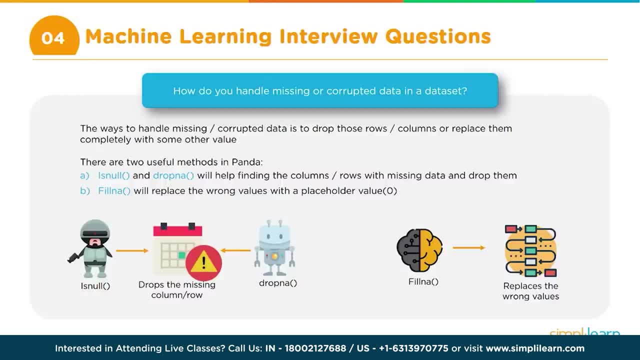 So let's assume that this is not a mission critical situation And in order to fix this 10 percent of the data, the effort that is required is much higher And obviously effort means also time and money, Right? So it is not so mission critical and it is okay to, let's say, get rid of these records. 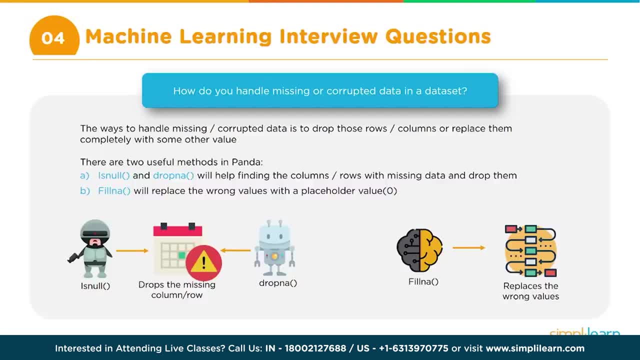 So obviously one of the easiest ways of handling the data part or missing data is Remove those records or remove those observations from your analysis. So that is the easiest way to do. But then the downside is, as I said in, as in the first case, if, let's say, 50 percent of your data is like that because some column or the other is missing, 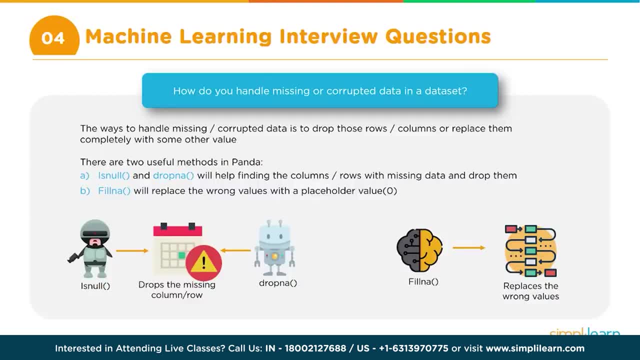 So it is not like every in every place, in every row, the same column is missing. But you have maybe 10 percent of the records. Column one is missing and another 10 percent. column two is missing, Another 10 percent. column three is missing, and so on and so forth. 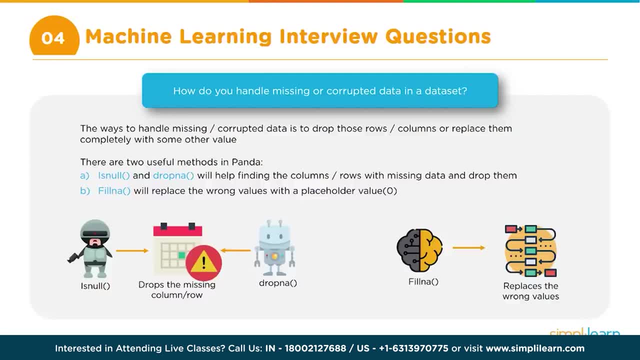 So it adds up to maybe half of your data set. So you cannot completely- You cannot completely- remove half of your data set. Then the whole purpose is lost. Okay, So then how do you handle? Then you need to come up with ways of filling up this data with some meaningful value. 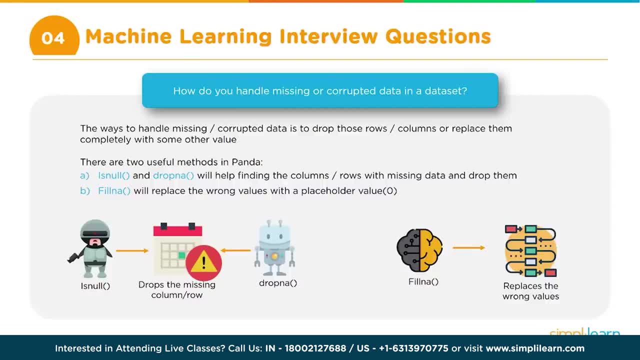 And that is one way of handling. So when we say meaningful value, what is that meaningful, Let's say, for a particular column? you might want to take a mean value for that column and fill wherever the data is missing. Fill up with that mean value so that when you're doing the calculations your analysis is not 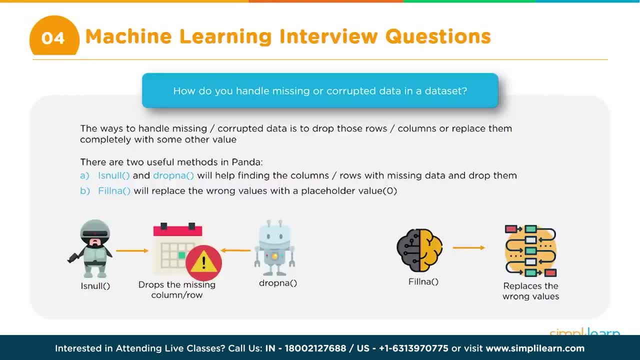 Completely way off. So you have values which are not missing, First of all, so your system will work. Number two: these values are not so completely out of whack that your whole analysis goes for a toss. There may be situations where, if the missing values, instead of putting mean, may be a good idea to fill it up with the minimum value or with a zero. 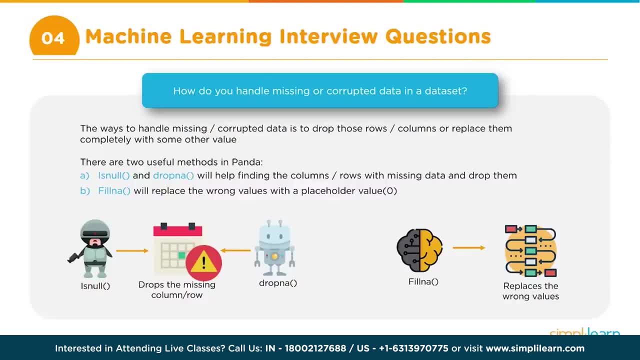 So, or with the maximum value. Again, as I said, there are so many possibilities, So there is no like one correct answer for this. You need to basically Talk around this and illustrate with your experience, As I said. that would be the best. 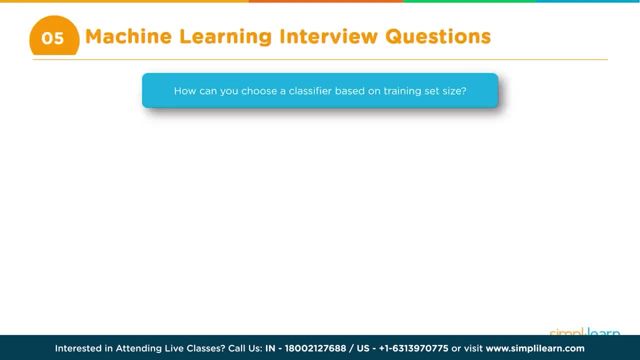 Otherwise, this is how you need to handle this question. OK, so then the next question can be: how can you choose a classifier based on a training set data size? So again, this is one of those questions where you probably do not have like a one size fits all answer. 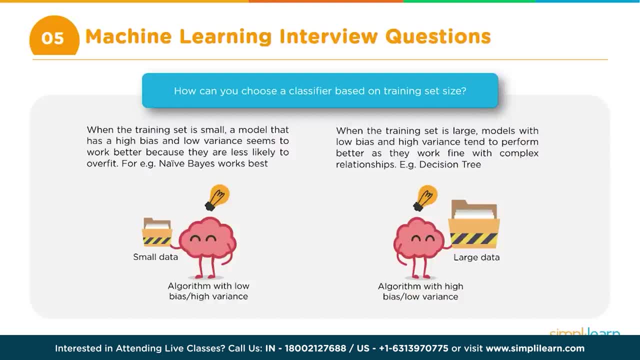 First of all, you may not, let's say, decide your classifier based on the training set data size. Maybe not the best way to decide the type of the classifier, And even if you have to, there are probably some thumb rules which we can use. 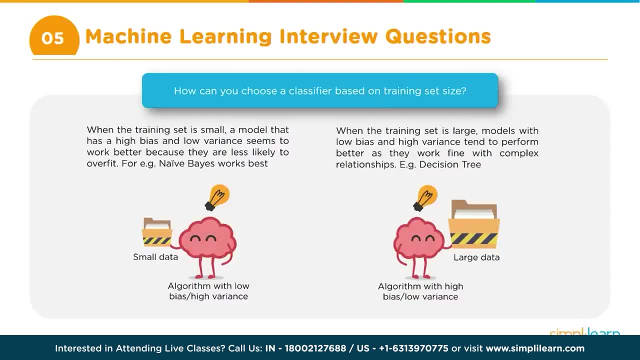 But then again every time. So, in my opinion, the best way to respond to this question is you need to try out a few classifiers, irrespective of the size of the data, And you need to then decide, on your particular situation, which of these classifiers are the right ones. 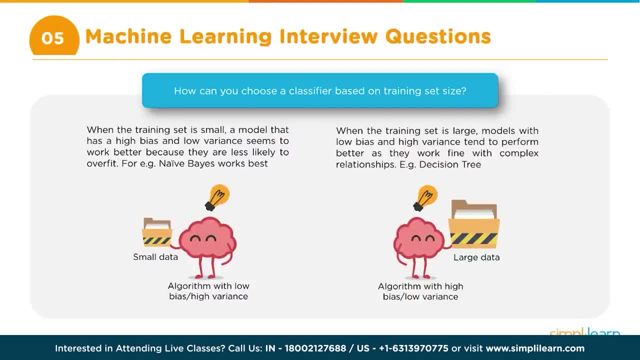 This is a very generic issue, So you will never be able to Just by. if somebody defines a problem to you and somebody, even if they show the data to you or tell you what is the data or even the size of the data, I don't think there is a way to really say that yes, this is the classifier that will work here. 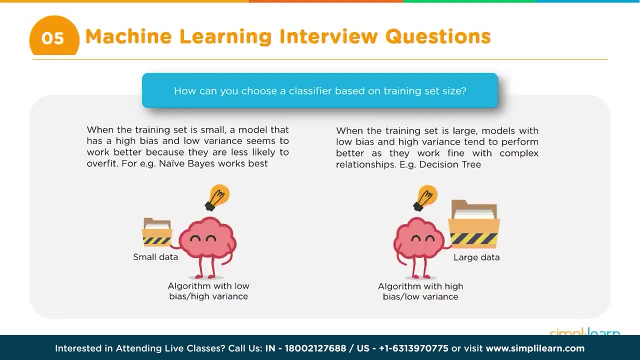 No, that's not the right way. So you need to still, you know, test it out, get the data, try out a couple of classifiers and then only you will be in a position to decide which classifier to use. You try out multiple classifiers. 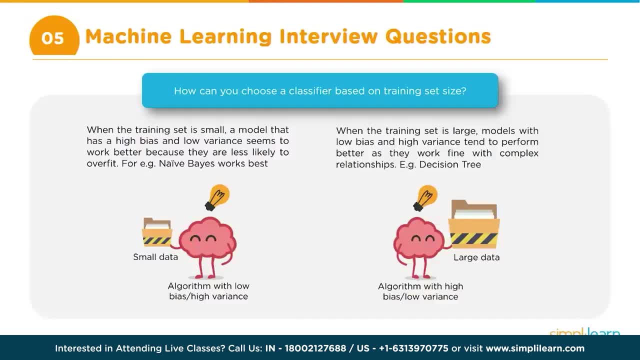 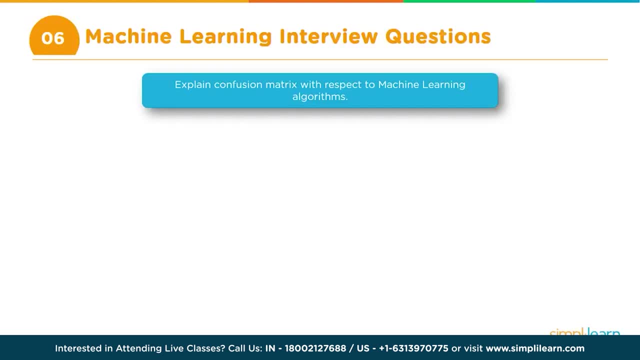 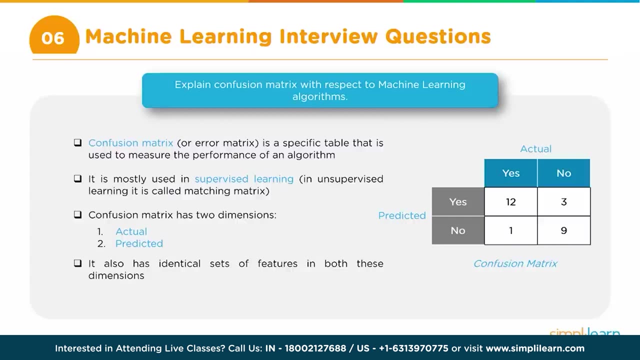 See which one gives the best accuracy And only then you can decide. Then you can have a question around confusion matrix. So the question can be explained: confusion matrix, So confusion matrix. I think the best way to explain it is by taking an example and drawing like a small diagram. 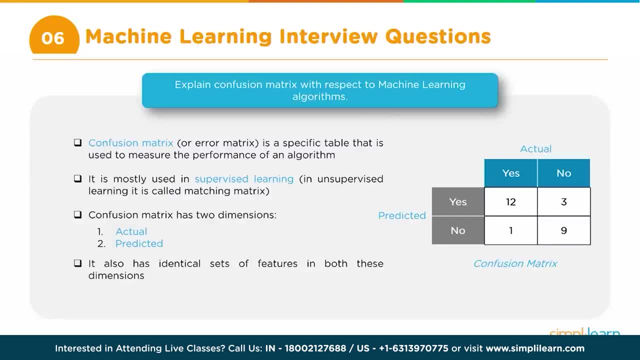 Otherwise it can really become tricky. So my suggestion is to take a piece of pen and paper and explain it by drawing a small matrix. And confusion matrix Is about to find out. this is used specially in classification learning process, And when you get the results- and our model predicts the results- you compare it with the actual value and try to find out what is the accuracy. 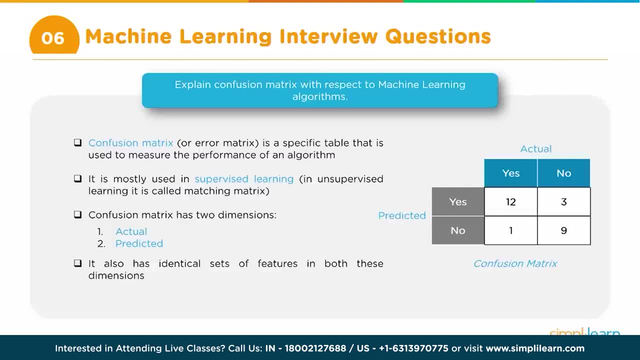 So in this case, let's say this is an example of a confusion matrix and it is a binary matrix, So you have the actual values, which is the labeled data And which is So you have how many yes and how many no. 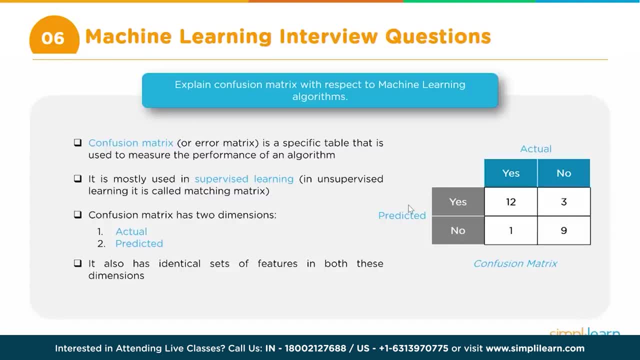 So you have that information And you have the predicted values: How many yes and how many no. So the total actual values, the total yes is 12 plus 1, 13.. And they are shown here. And the actual value no's are 9 plus 3, 12.. 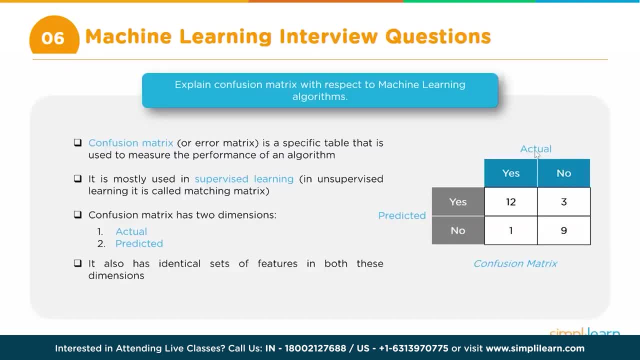 So that is what this information here is. So this is about the actual and this is about the predicted. Similarly, the predicted values there are: yes are 12 plus 3, 15 yes And no are 1 plus 9, 10 no's. 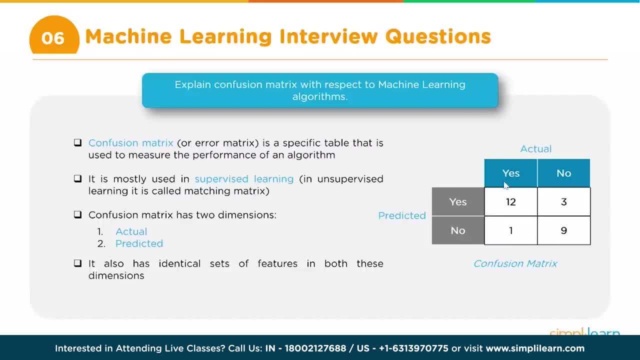 So this is the way to look at this confusion matrix, And out of this, what is the meaning conveyed? So there are two or three things that needs to be explained outright. The first thing is, for a model to be accurate, the values across the diagonal should be high, like in this case. 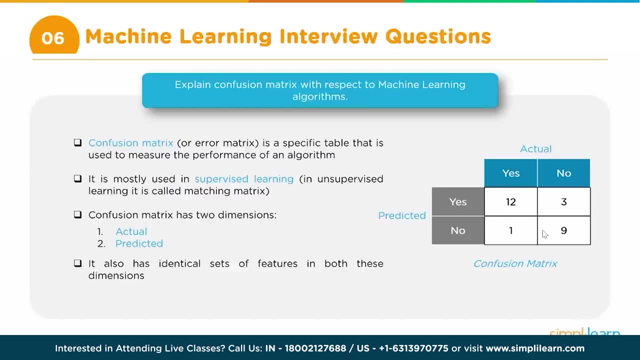 That is one Number two. the total sum of these values is equal to the total observations in the test Data set. So in this case, for example, you have 12 plus 3,, 15 plus 10, 25.. 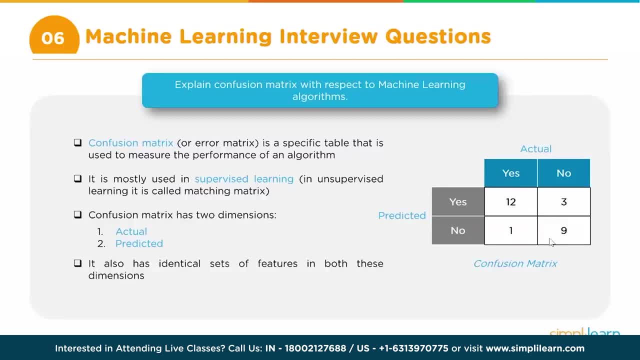 So that means we have 25 observations in our test data set. OK, so these are the two things. you need to first explain that the total sum in this matrix the numbers is equal to the size of the test data set And the diagonal values indicate the accuracy. 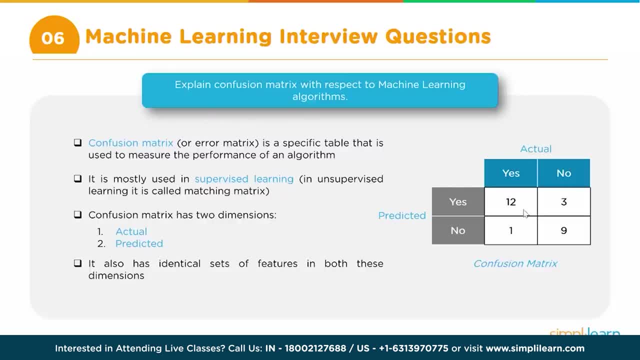 So by just by looking at it, you can probably have an idea about: is this an accurate model? Is the model being accurate? I mean they're all spread out equally in all these four boxes. That means probably the accuracy is not very good. 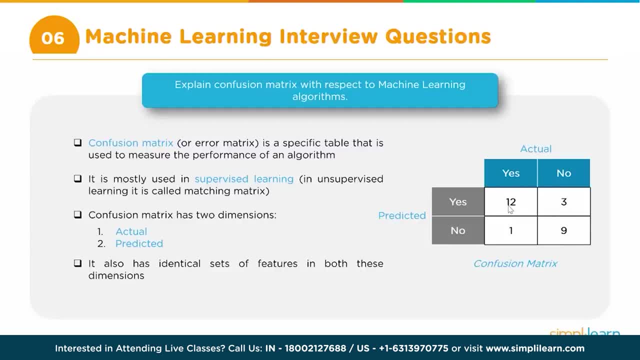 OK, now how do you calculate the accuracy itself? Right, How do you calculate accuracy? So it is a very simple mathematical calculation. You take some of the diagonals, So in this case it is nine plus 21 and divided by the total. 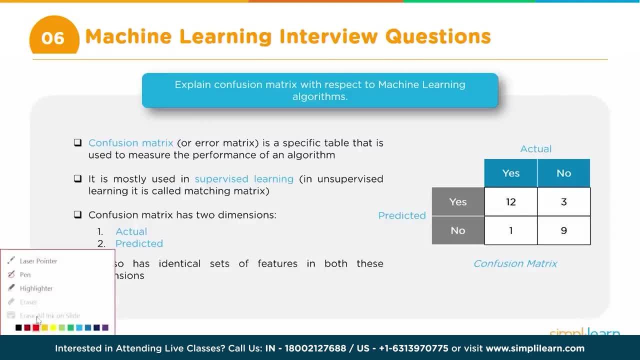 So in this case, what will it be? Let's me take a pen. So your, your diagonal values is equal. If I say, D Is equal to 12 plus nine, So that is 21.. Right, And the total data set is equal to. 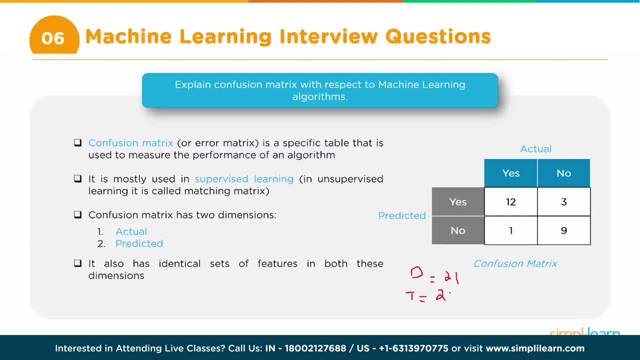 Right, We just calculated it is 25.. So what is your accuracy? It is 21 by your accuracy is equal to 21 by 25. And this turns out to be about 85 percent, Right? So this is 85 percent. 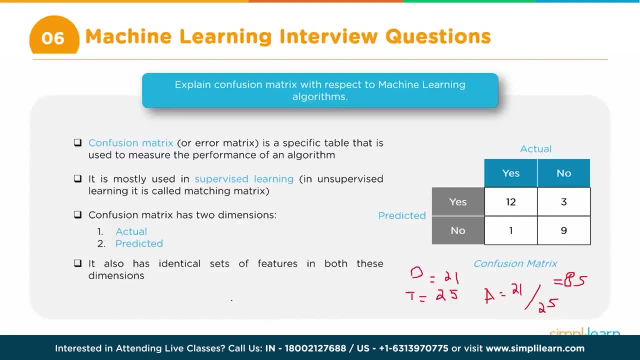 So that is our accuracy. OK, So this is the way you need to explain your diagram. Give an example. Maybe It is a good idea to be prepared with an example so that it becomes easy for you. You don't have to calculate those numbers on the fly. 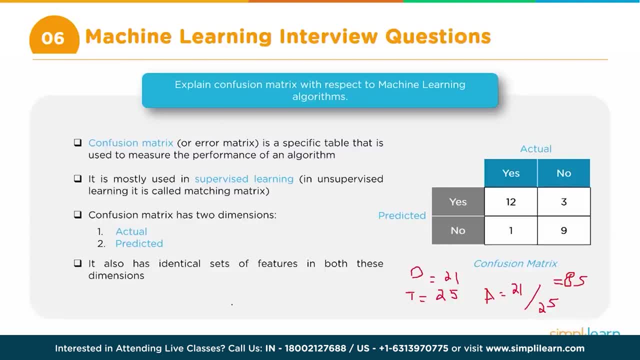 Right. So a couple of hints are that you take some numbers which are with, which add up to 100. That is always a good idea, So you don't have to really do this complex calculations. So the total value will be 100 and then diagonal values. you divide once you find the diagonal. 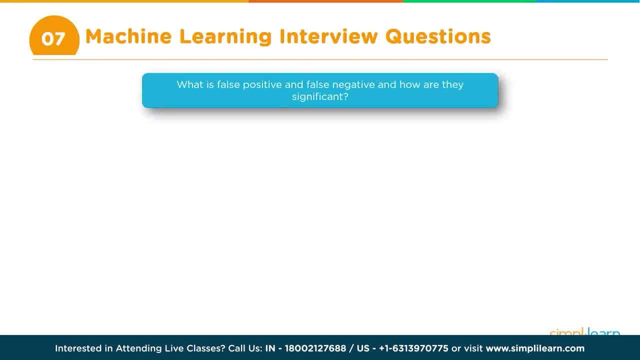 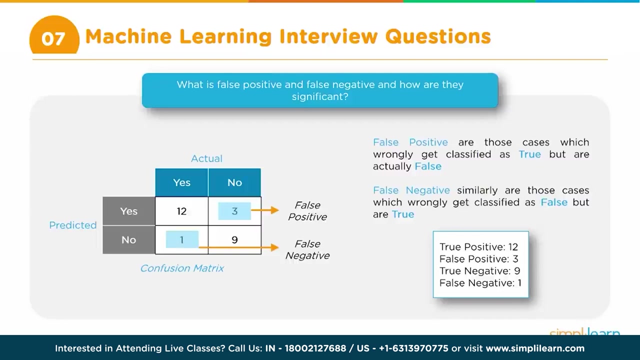 values. that is equal to your percentage. OK, All right, So the next question can be a related question about false positive and false negative. So what is false positive and what is false negative? Now, once again, the best way to explain this is using a piece of paper and pen. 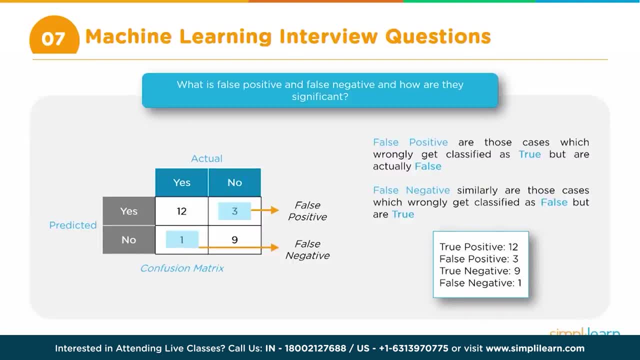 Otherwise it will be pretty difficult to explain this. So we use the same example of the confusion matrix and we can explain that. So a confusion matrix looks somewhat like this, And then we just look somewhat like this And we continue with the previous example. 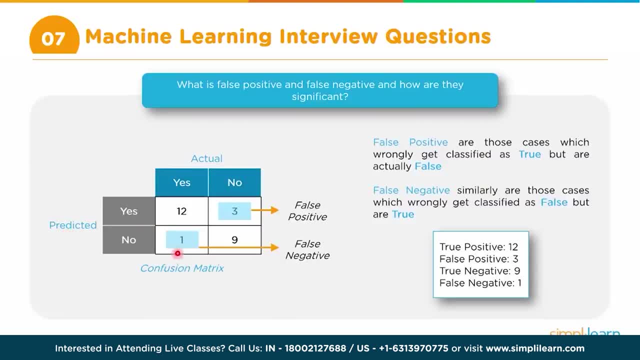 The previous example, where this is the actual value. This is the predicted value And in the actual value we have 12 plus 1, 13 yeses and 3 plus 9, 12 nos, And the predicted values there are 12 plus 3, 15 yeses and 1 plus 9, 10 nos. 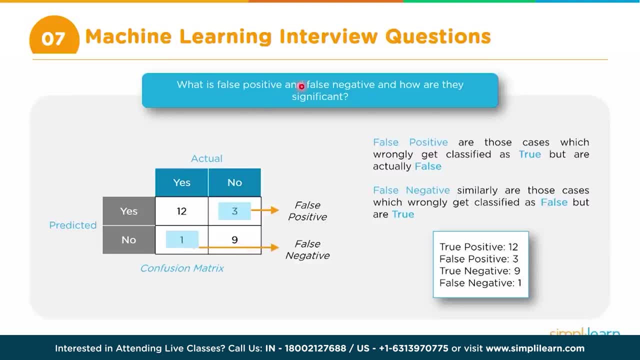 OK, Now this particular case, which is the false positive. What is a false positive? First of all, the second word, which is positive. OK, This is referring to the predicted value, So that means the system has predicted it as a positive. but the real value? 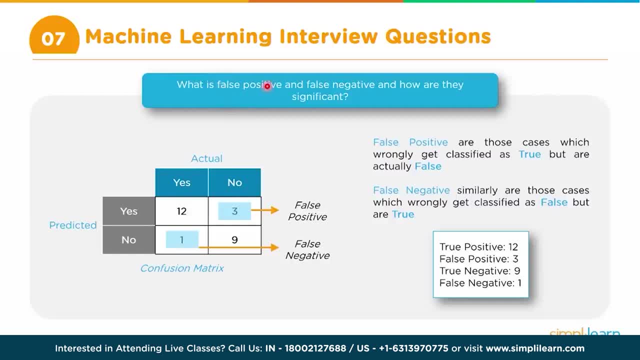 So this is what the false comes from, But the real value is not positive. OK, That is the way you should understand this term: false positive or even false negative. So false positive, So positive is what your system has predicted. So where is that system predicted? 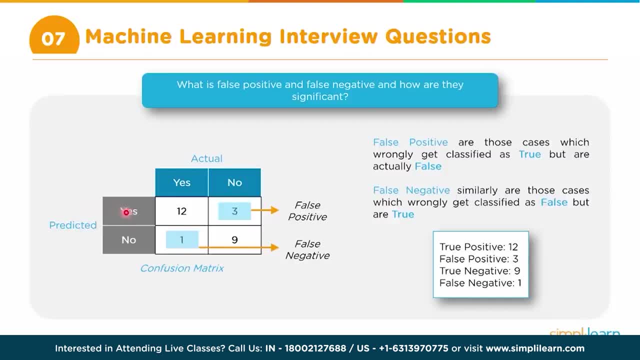 This is the one Positive is what? Yes, So you basically consider this row. OK, You consider this row. So this is, this is all positive values. This entire row is positive values. OK. Now the false positive is the one with where the value- actual value- is negative. 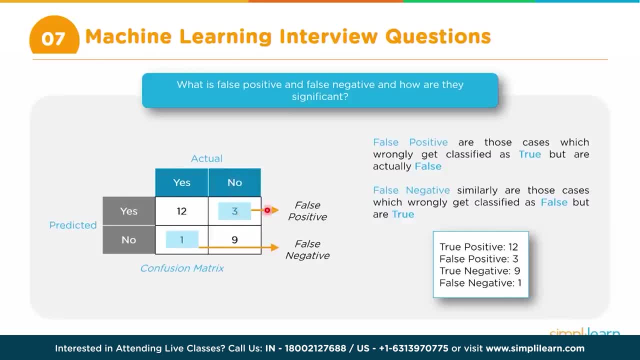 Predicted value is positive, but the actual value is negative. So this is a false positive Right And here is a true positive. So the predicted value is positive and the actual value is also positive. OK, I hope this is making sense. 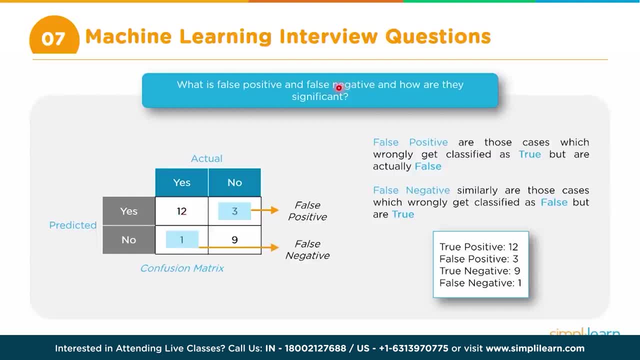 Now let's take a look at what is false, negative, False, negative, Negative is the second term. That means that is the predicted value that we need to look for. So which are the predicted negative values? This row corresponds to predicted negative values. 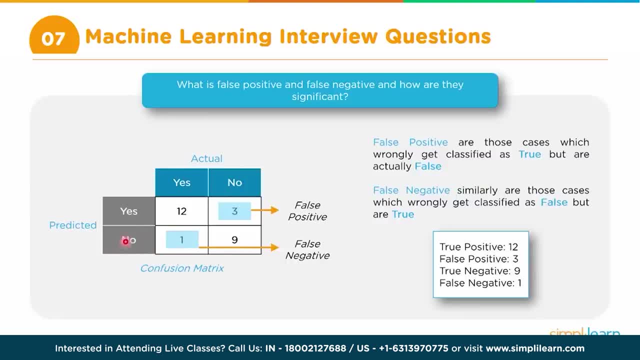 All right, So this row corresponds to predicted negative values And what they are asking for- false. So this is the row for predicted negative values And the actual value is this one. Right, This is predicted negative and the actual value is also negative. 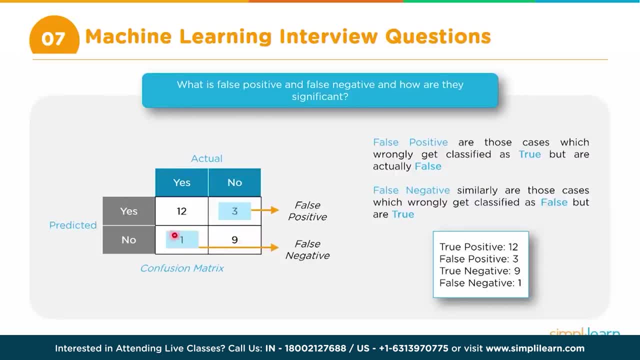 Therefore, this is a true negative. So the false negative is this: one Predicted is negative, but actual is positive, Right? So this is the false negative. So this is the way to explain And this is the way to look at false positive and false negative. 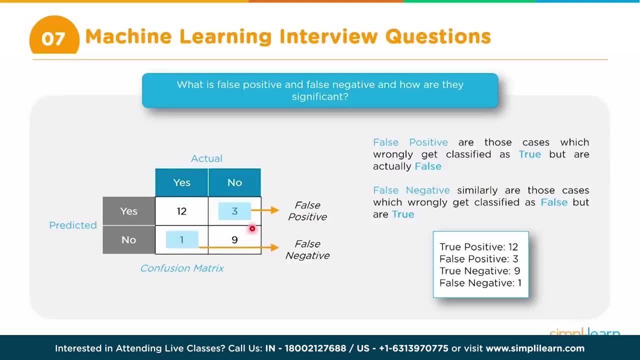 Same way, there can be true positive and true negative as well. So, again, positive, the second term you will need to use to identify the predicted row Right. So if we say true, positive, positive we need to take for the predicted part. 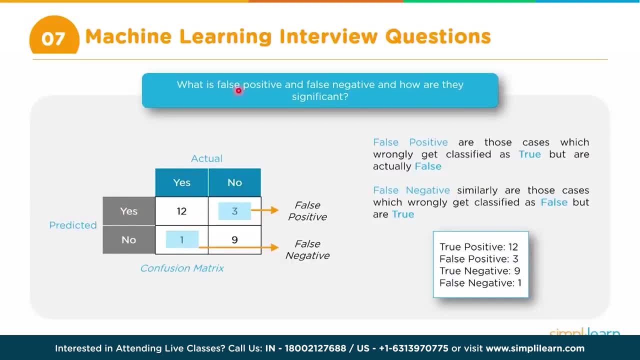 So predicted positive is here Okay. And then the first term is for the actual: So true, positive. So true, in case of actual, is yes, Right. So true, positive, is this one, Okay. And then, in case of actual, the negative. 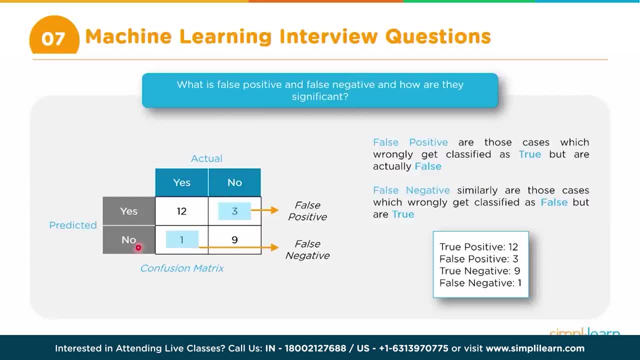 Now we are talking about, let's say, true, negative, True, negative, Negative is this one, And the true comes from here. So this is true, negative. Right Nine is true, negative. The actual value is also negative and the predicted value is also negative. 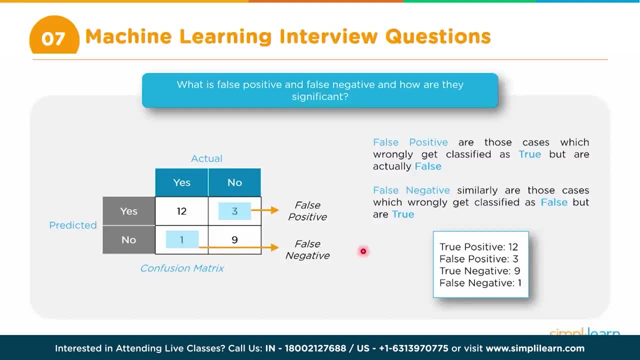 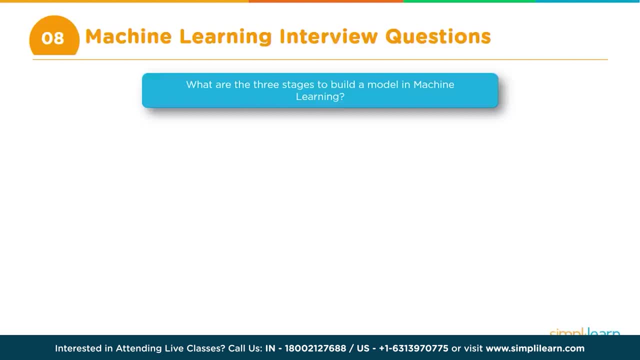 Okay, So this is the way you need to explain this: The terms false positive, false negative and true positive, true negative. Then you might have a question like: what are the steps involved in the machine learning process, Or what are the three steps in the process of developing a machine learning model? 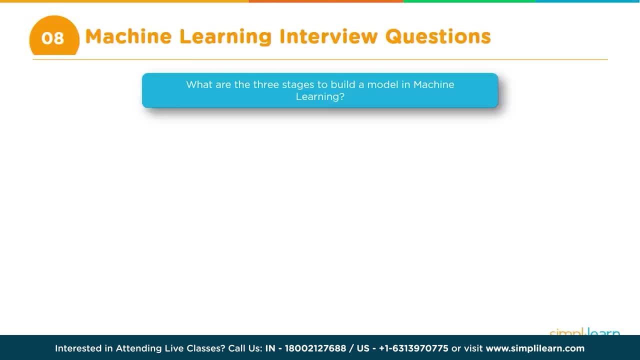 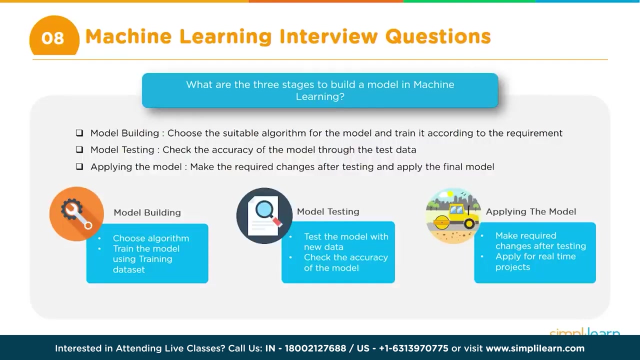 Right, So it is around the methodology that is applied. So basically, the way you can probably answer in your own words, but the way the model development of the machine learning model happens. So first of all you try to understand the problem and try to figure out whether it is a classification problem or a regression problem. 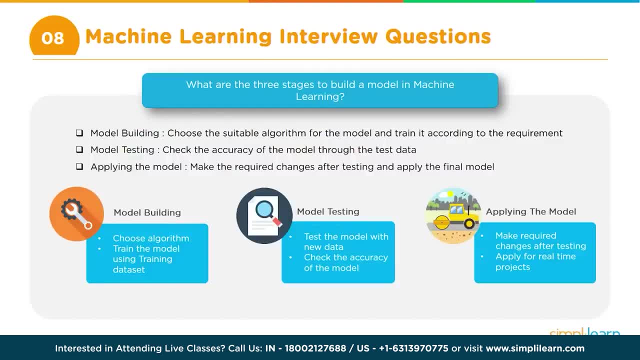 Based on that, you select a few algorithms and then you start the process of training these models. Okay, So you can either do that or you can. after due diligence, you can probably decide that there is one particular algorithm, that which is most suitable. 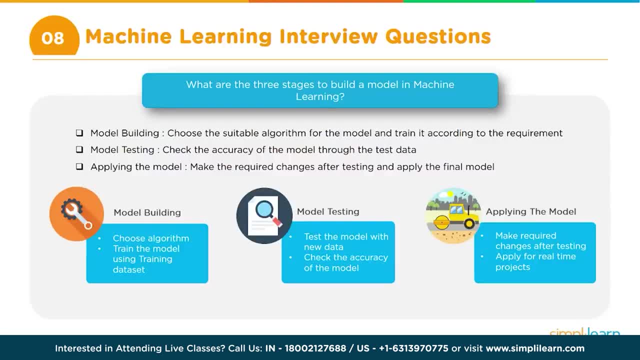 Usually it happens through trial and error process, But at some point you will decide that, okay, this is the model we are going to use. Okay, So in that case we have the model algorithm and the model decided, And then you need to do the process of training the model and testing the model. 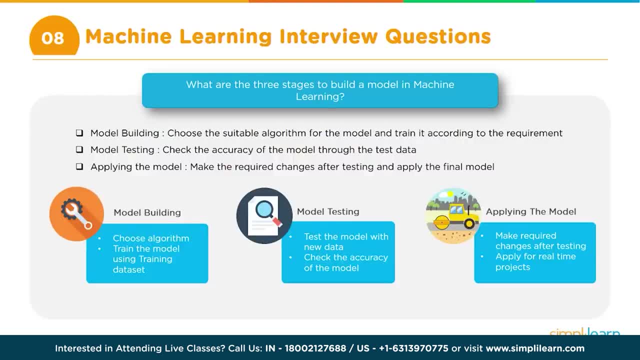 And this is where, if it is supervised learning, you split your data- the label data- into training data set and test data set, And you use the training data set to train your model And then you use the test data set to check the accuracy. 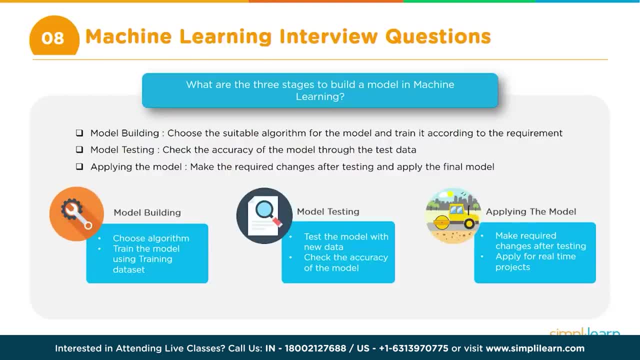 Whether it is working fine or not. So you test the model before you actually put it into production, Right? So once you test the model, you're satisfied it's working fine. Then you go to the next level, which is putting it for production. 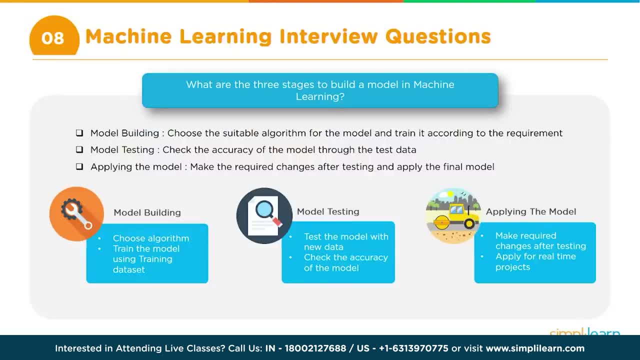 And then in production, obviously new data will come and the inference happens. So the model is readily available And only thing that happens is new data comes and the model predicts the values, whether it is regression or classification Now. so this can be an iterative process. 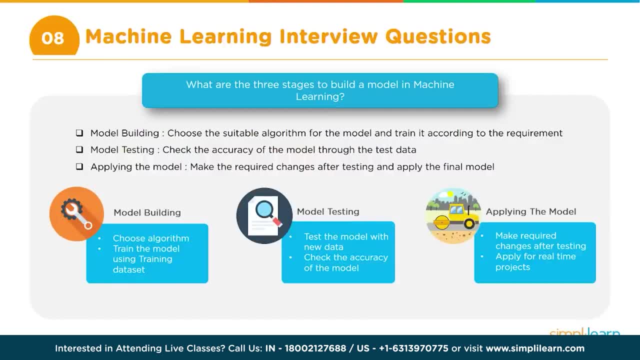 So it is not a straightforward process. You do the training for the testing and then you move it to production now. So during the training and test process, there may be a situation where, because of either overfitting or things like that, the test doesn't go through, which means that you need to put that back into the training process. 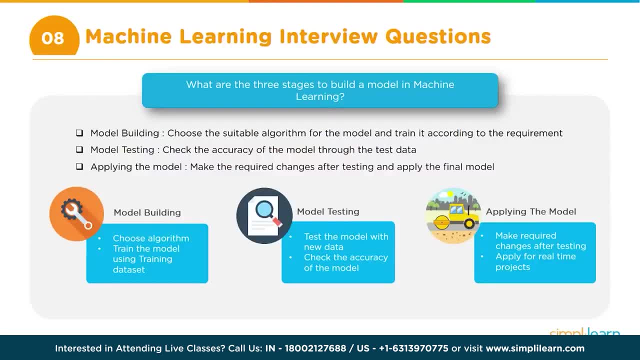 So that can be an iterative process. Not only that: even if the training and test goes through properly and you deploy the model in production, there can be a situation that the data that actually comes, the real data that comes with that, This model is failing. 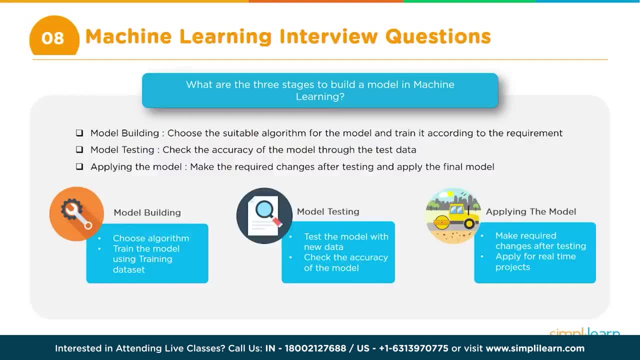 So, in which case you may have to once again go back to the drawing board, or initially it will be working fine, But over a period of time, maybe due to the change in the nature of the data- once again the accuracy will deteriorate. 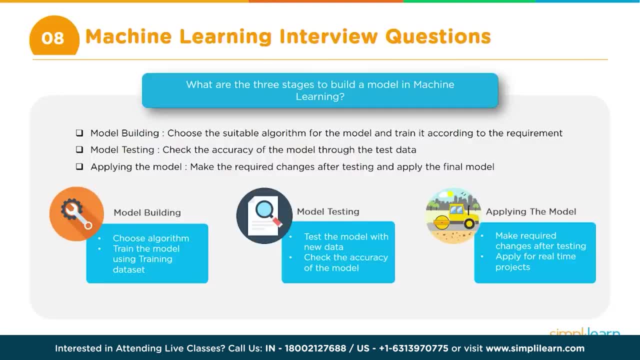 So that is again a recursive process. So once in a while you need to keep checking whether the model is working fine or not And, if required, you need to tweak it and modify it, and so on and so forth. So this is a continuous process of tweaking the model and testing it. 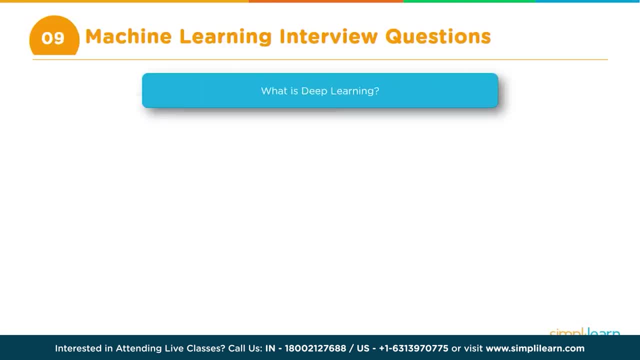 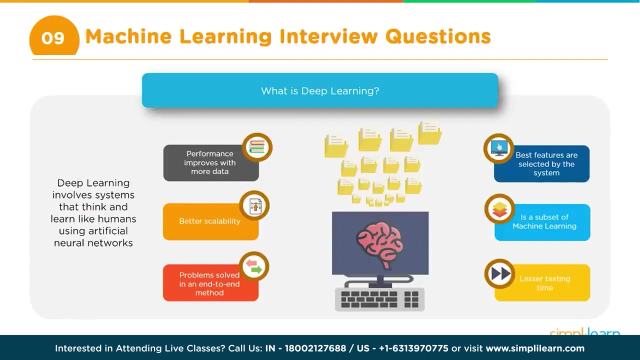 And making sure it is up to date. Then you might have question around deep learning. So, because deep learning is now associated with AI, artificial intelligence and so on, So can be as simple as what is deep learning? So I think the best way to respond to this could be: deep learning is a part of machine learning. 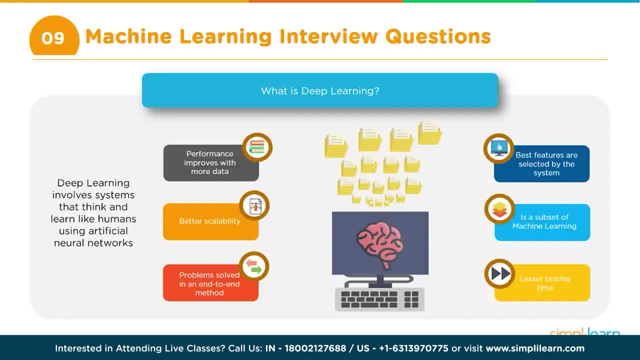 And then obviously the question would be: then what is the difference? right, So deep learning, you need to mention there are two key parts that interviewer will be looking for When you are defining deep learning. So first is, of course, deep learning is a subset of machine learning. 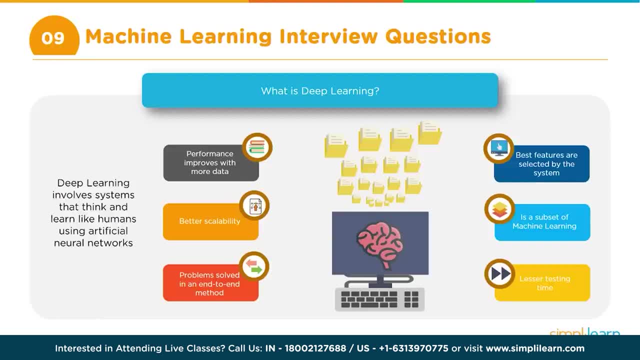 So machine learning is still the bigger, let's say, scope, and deep learning is one part of it. So then, what exactly is the difference? Deep learning is primarily when we are implementing these, our algorithms, or when we are using neural networks for doing our training and classification and regression and all that right. 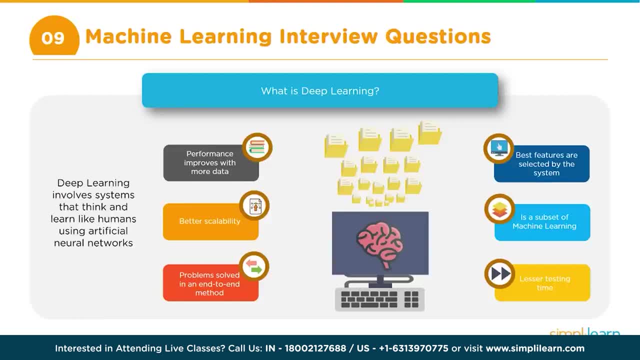 So when we use neural network, then it is considered as deep learning And the term deep comes from the fact that you can have several layers of neural networks and these are called deep neural networks and therefore the term deep learning. The other difference between machine learning and deep learning, which the interviewer may be wanting to hear, is that in case of machine learning, the feature engineering is done manually. 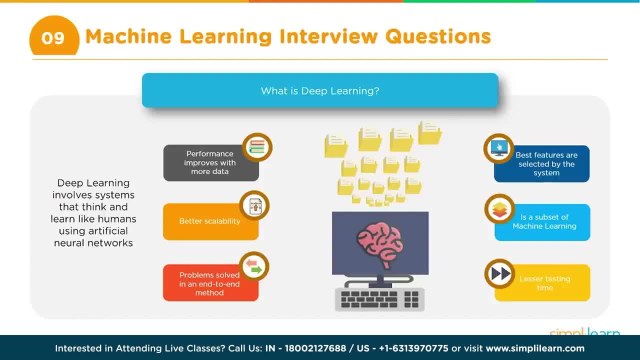 What do we mean by feature engineering? Basically, when we are trying to train our model, We have our training data right. So we have our training label data and this data has several. Let's say, if it is a regular table, it has several columns. 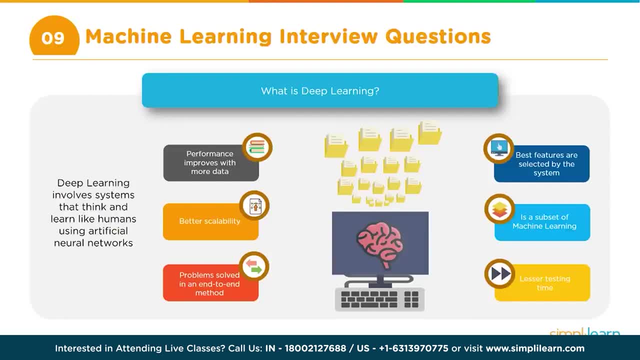 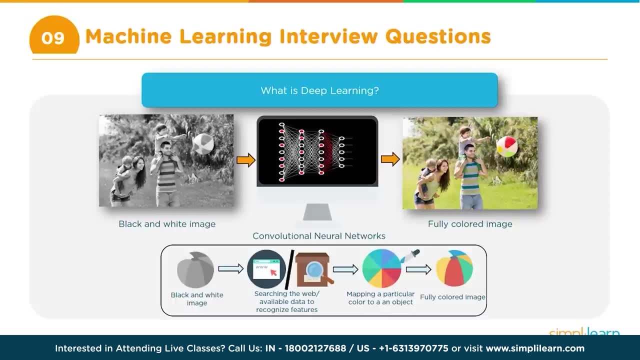 Now, each of these columns actually has information about a feature, right? So if we are trying to predict the height, weight and so on and so forth, So these are all features of human beings. Let's say, we have census data and we have all this. 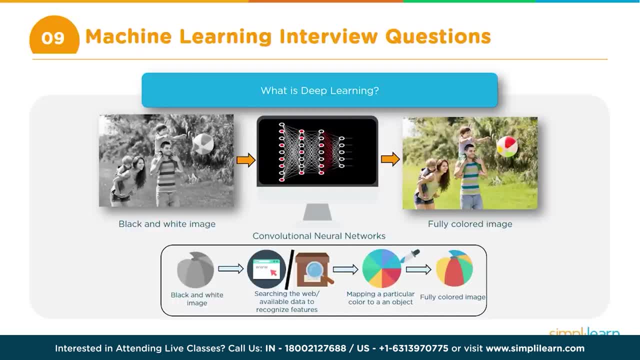 So those are the features Now. there may be probably 50 or 100.. In some cases there may be hundreds of them. There may be hundreds of such features. Now, all of them do not contribute to our model, right. 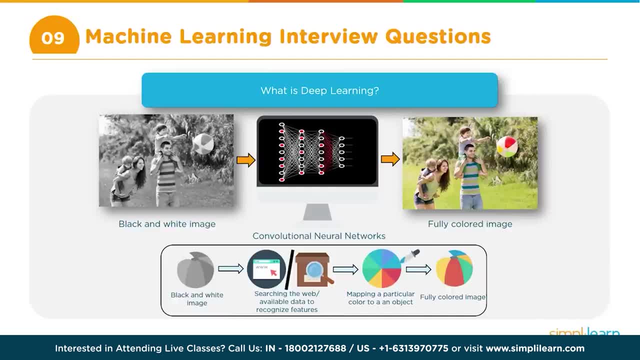 So we, as a data scientist, we have to decide whether we should take all of them, all the features, or we should throw away some of them. Because, again, if we take all of them, number one of course- your accuracy will probably get affected. 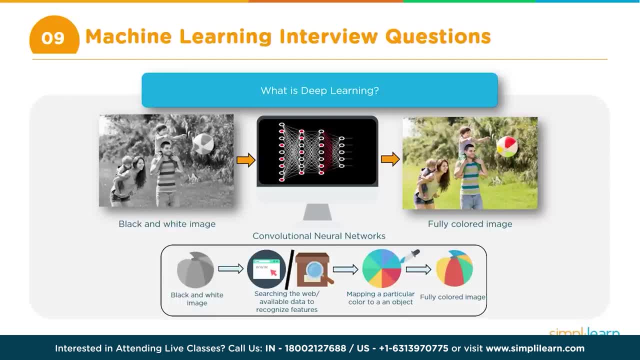 But also there is a computational part. So if you have so many features and then we have so much data, it becomes very tricky. So in case of machine learning, We take care of identifying the features that do not contribute to the learning process, and thereby we eliminate those features, and so on. 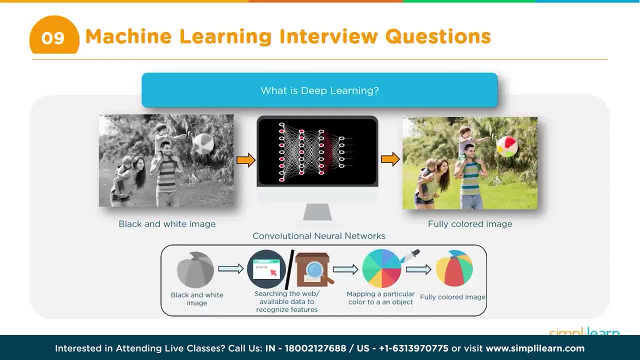 So this is known as feature engineering, And in machine learning we do that manually, Whereas in deep learning, where we use neural networks, the model will automatically determine which features to use and which to not use, And therefore feature engineering is also done automatically. 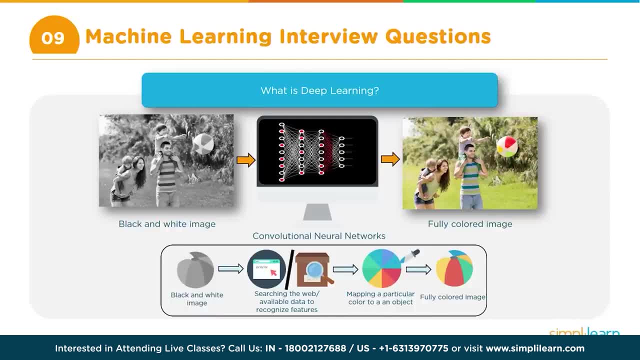 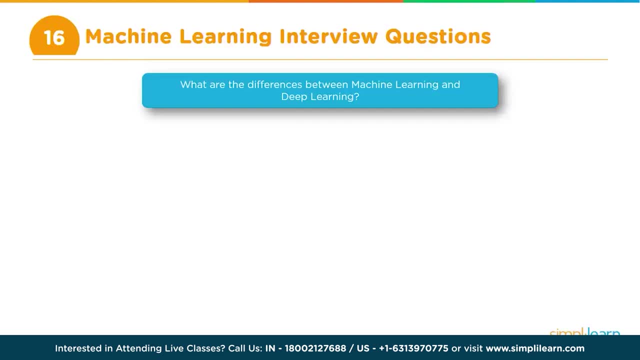 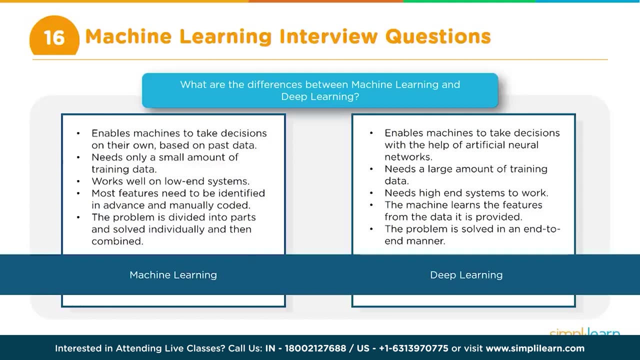 So this is an explanation. These are two key things. They probably will add value to your response. All right, So the next question is: what is the difference between, or what are the differences between, machine learning and deep learning? So here this is a quick comparison table between machine learning and deep learning. 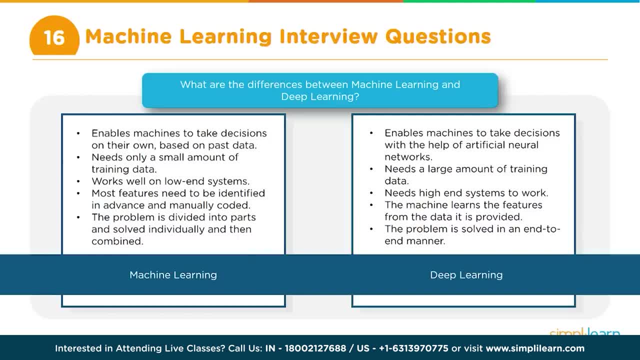 And machine learning enables machines to take decisions on their own based on past data. So here we are talking primarily of supervised learning, And it needs only a small amount of data for training And then works well on machine learning, Works well on low-end systems. 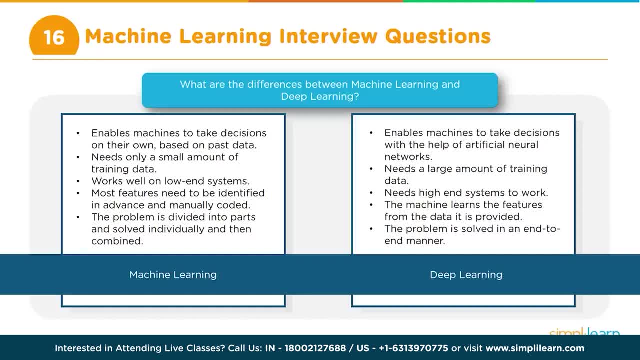 So you don't need large machines And most features need to be identified in advance and manually coded. So basically the feature engineering part is done manually And the problem is divided into parts and solved individually and then combined. So that is about the machine learning part. 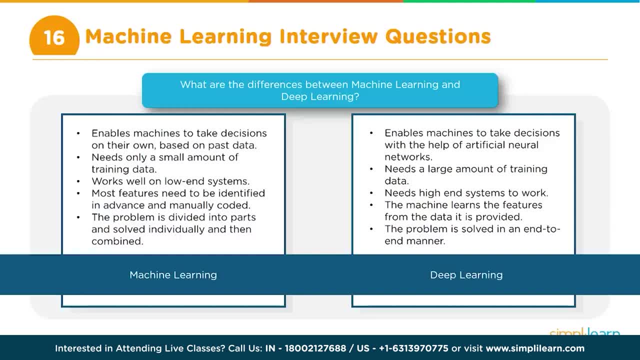 In deep learning. deep learning basically enables machines to take decisions with the help of artificial neural networks. So here in deep learning we use neural networks. So that is the key differentiator between machine learning and deep learning, And usually deep learning involves a large amount of data. 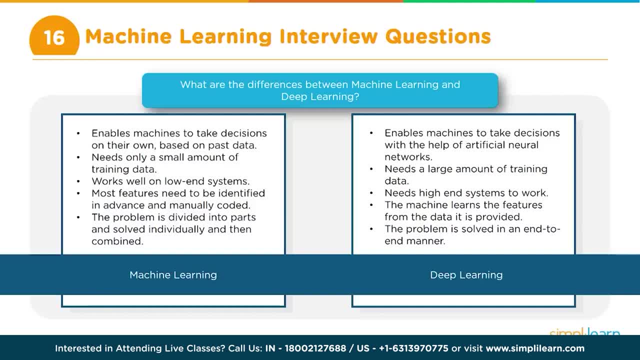 And therefore the training also requires. usually the training process requires high-end machines Because it needs a lot of computing power And the machine learning features or the feature engineering is done automatically. So the neural networks takes care of doing the feature engineering as well. 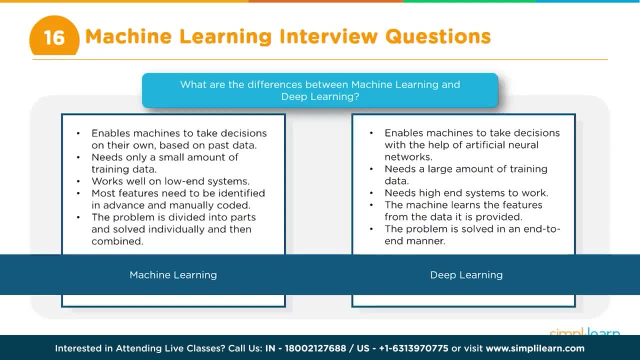 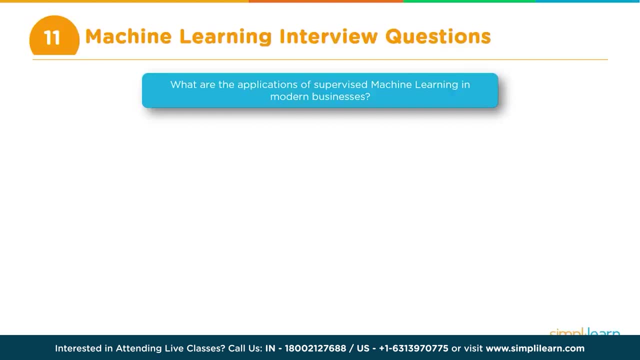 And in case of deep learning, therefore, it is said that the problem is handled end-to-end. So this is a quick comparison between machine learning and deep learning. In case you have that kind of a question, Then you might get a question around the uses of machine learning or some real-life applications of machine learning in modern business. 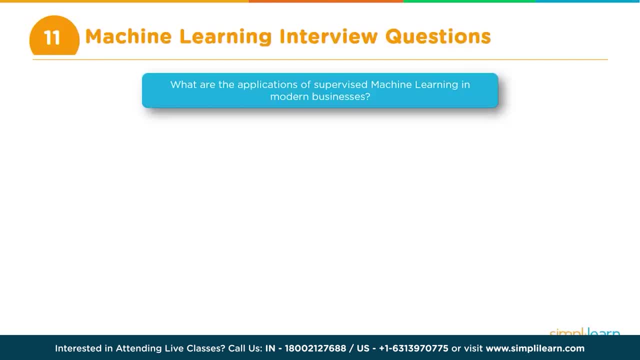 The question may be worded in different ways, But the meaning is: how exactly is machine learning used, or actually supervised machine learning? It could be a very specific question around supervised machine learning, So this is like give examples of supervised machine learning, use of supervised machine learning in modern business. 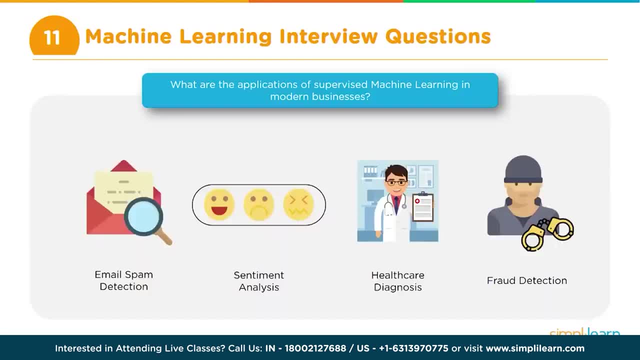 So that could be the next question. So there are quite a few examples, or quite a few use cases, if you will, for supervised machine learning. The very common one is email spam detection. So you want to train your application or your system to detect between spam and non-spam. 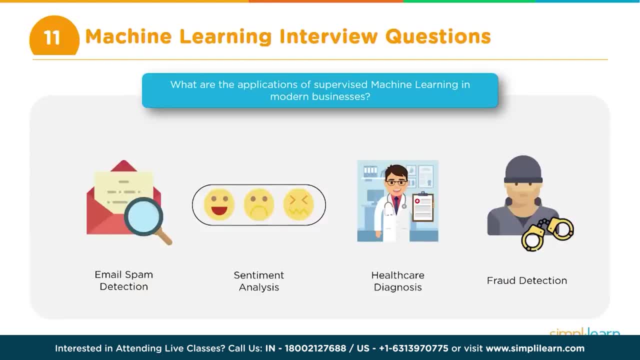 So this is a very common business application of supervised machine learning. So how does this work? The way it works is that You obviously have historical data of all of your emails And they are categorized as spam and not spam. So that is what is the labeled information. 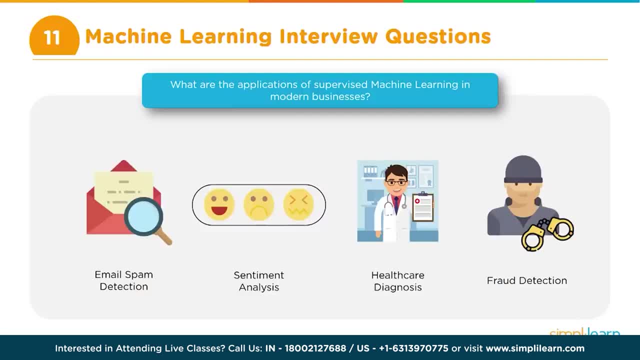 And then you feed this information or all these emails as an input to your model And the model will then get trained to detect which of the emails are to detect which is spam and which is not spam. So that is the training process And this is supervised machine learning. 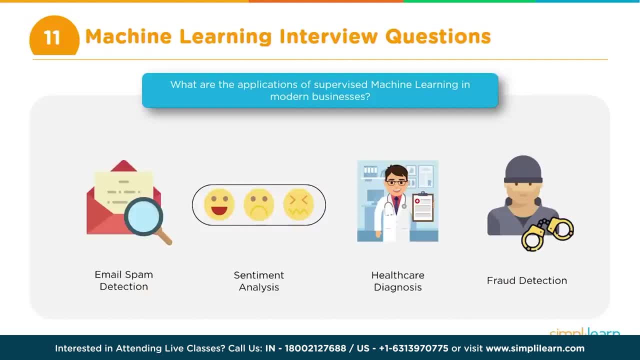 So you have labeled data, You already have emails which are tagged as spam or not spam, And then you use that to train your model. So this is one example. Now there are a few industry specific applications for supervised machine learning. One of the very common ones is in healthcare diagnostics. 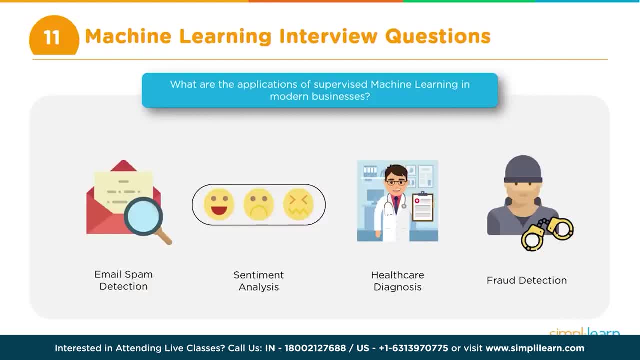 In healthcare diagnostics. you have these images and you want to train models to detect whether from a particular image, Whether it can find out if the person is sick or not, Whether a person has cancer or not. So this is a very good example of supervised machine learning. 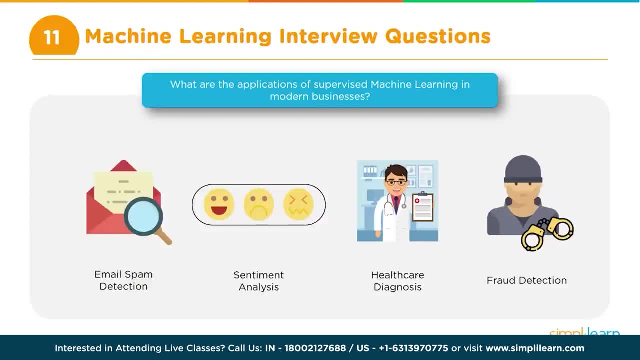 Here the way it works is that existing images- It could be x-ray images, It could be MRI or any of these images- are available And they are tagged saying that this x-ray image is defective or the person has an illness Or it could be cancer. 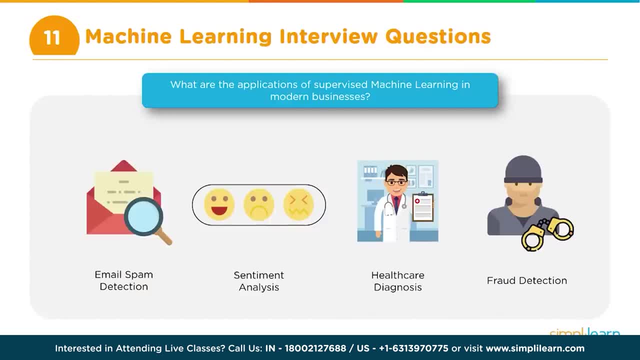 Whichever illness. So it is tagged As defective or clear or good image And defective image, Something like that. So we come up with a binary- Or it could be multi-class as well- Saying that this is defective to 10%. 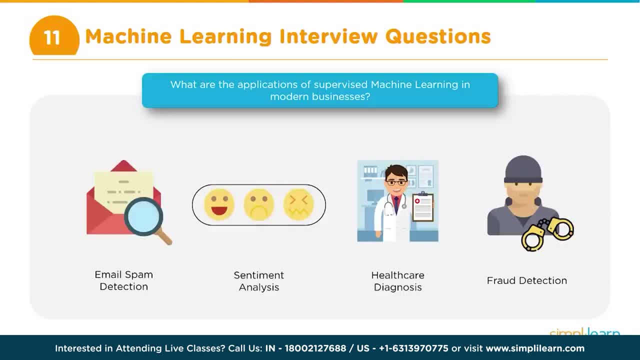 This is 25% and so on. But let's keep it simple. You can give an example of just a binary classification. that would be good enough. So you can say that in healthcare diagnostics using image, we need to detect whether a person is ill or whether a person is having cancer or not. 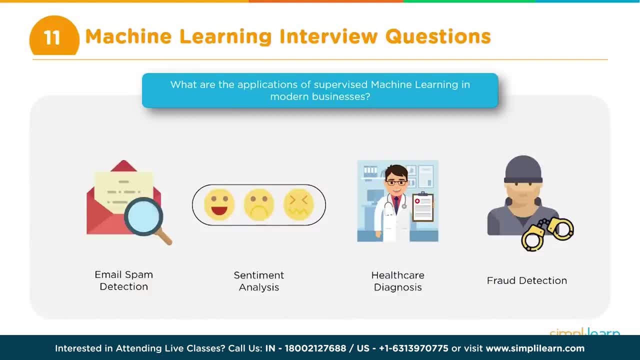 So here the way it works is You feed labeled images And you allow the model to learn from that So that when new image is fed It will be able to predict whether this person is having that illness or not, Having cancer or not. 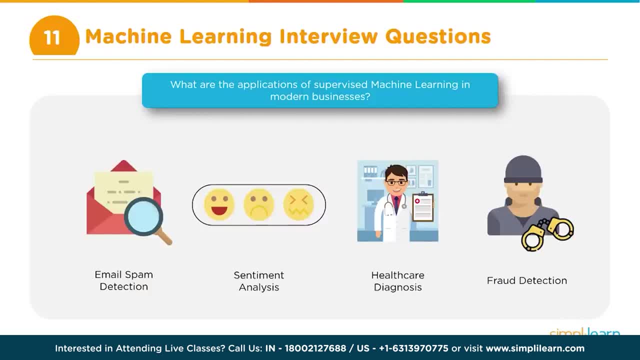 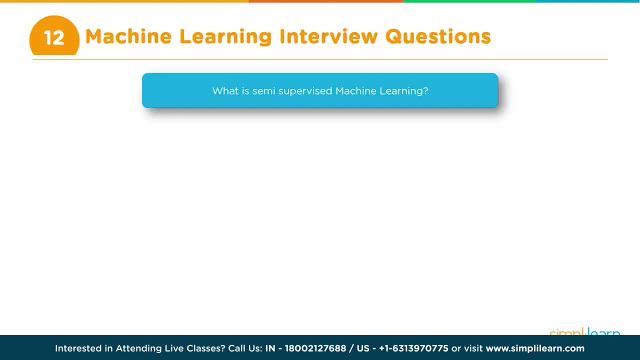 Right. So I think this would be a very good example for supervised machine learning in modern business. All right, Then we can have a question like: So we've been talking about supervised and unsupervised, And so there can be a question around semi-supervised machine learning. 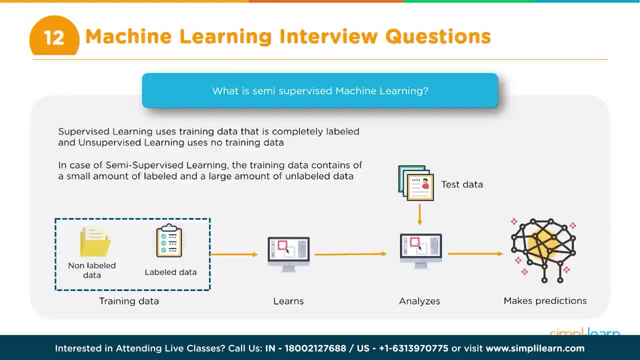 So what is semi-supervised machine learning Now? semi-supervised learning? as the name suggests, It falls between supervised learning and unsupervised learning, But for all practical purposes it is considered as a part of supervised learning, And the reason this has come into existence is that in supervised learning you need labeled data. 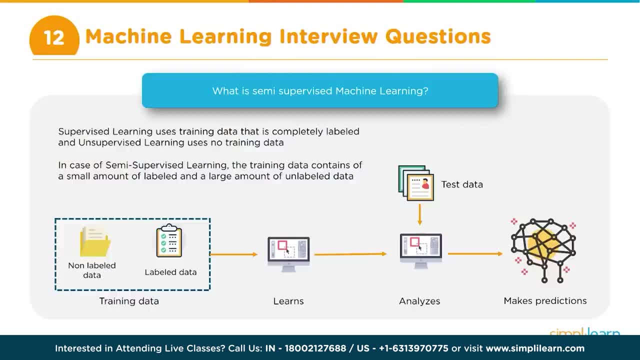 So all your data for training, your model has to be labeled. Now this is a big problem in many industries or under many situations. Getting the labeled data is not that easy, because there's a lot of effort in labeling this data. Let's take an example of diagnostic images. 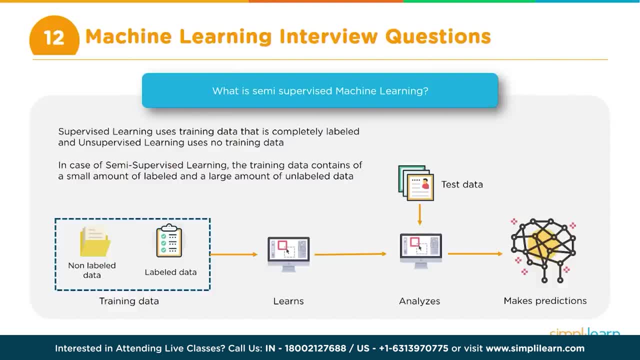 We can just, let's say, take x-ray images. Now there are actually millions of x-ray images available all over the world, But the problem is they are not labeled. So the images are there, But whether it is defective or whether it is good, 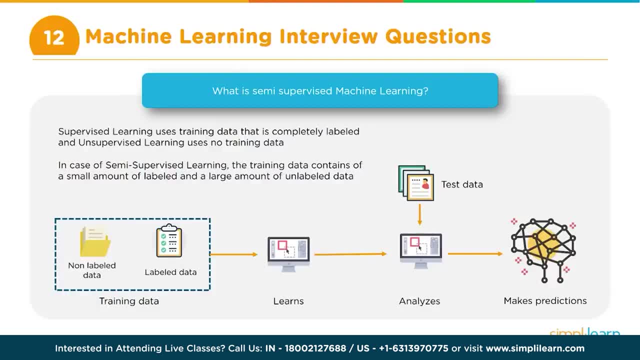 That information is not available. It is available along with it In a form that it can be used by a machine, Which means that somebody has to take a look at these images- And usually it should be like a doctor- And then say that okay, yes, this image is clean and this image is cancerous, and so on and so forth. 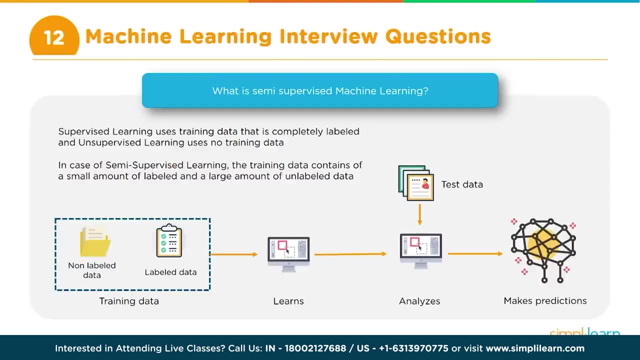 Now that is a huge effort by itself. So this is where semi-supervised learning comes into play. So what happens is there is a large amount of data. Maybe a part of it is labeled. Then we try some techniques to label the remaining part of the data. 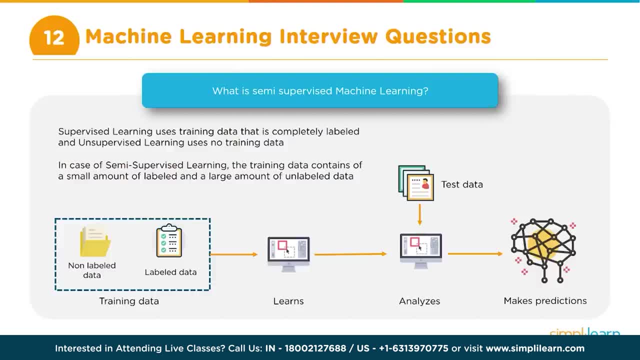 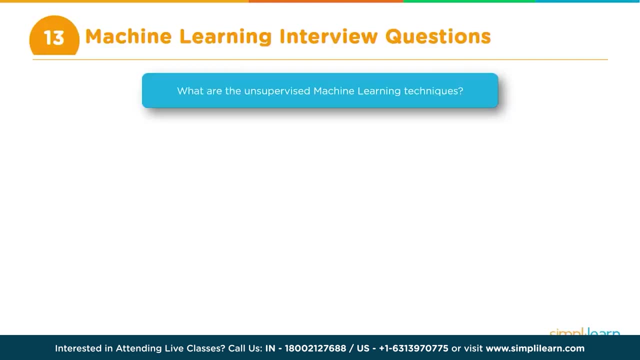 So that we get completely labeled data And then we train our model. So I know this is a little long winding explanation, But unfortunately there is no quick and easy definition for semi-supervised machine learning. This is the only way probably to explain this concept. 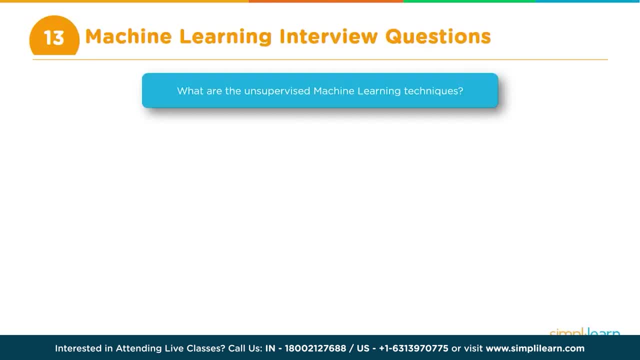 We may have another question, as what are unsupervised machine learning techniques, Or what are some of the techniques used for performing unsupervised machine learning? So it can be worded in different ways. So how do we answer this question? So, unsupervised learning, you can say that there are two types. 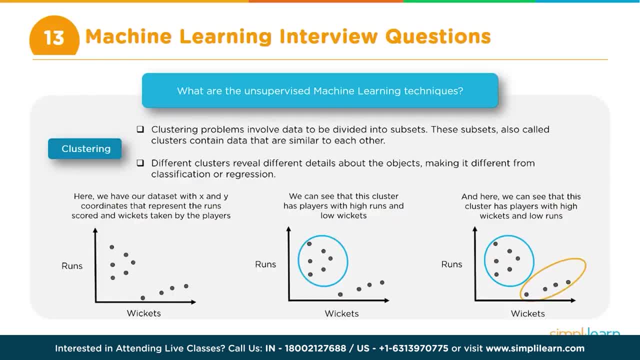 Clustering and association And clustering is a technique where similar objects are put together And there are different ways of finding similar objects. So their characteristics can be measured And if they have most of the characteristics, If they are similar, then they can be put together. 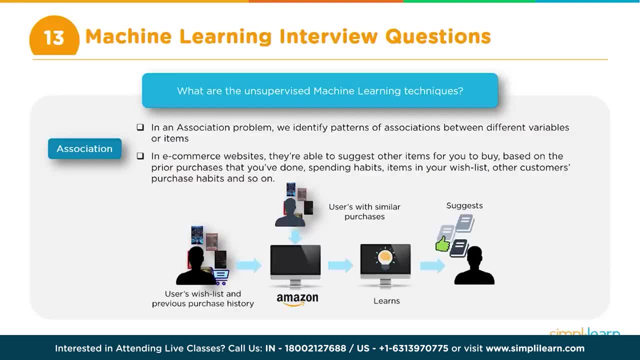 This is clustering, Then association you can. I think the best way to explain association is with an example. In case of association, you try to find out how the items are linked to each other. So, for example, if somebody bought, maybe, a laptop, The person has also purchased a mouse. 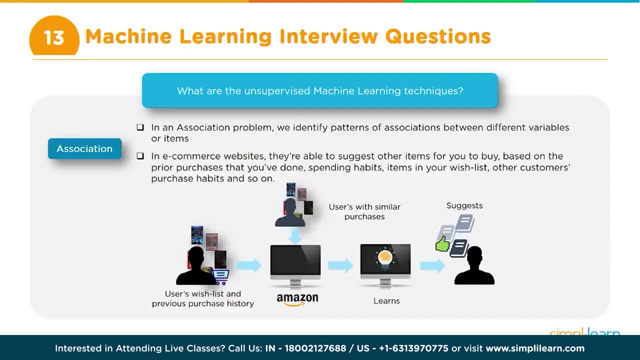 So this is more in an e-commerce scenario, for example, So you can give this as an example. So people who are buying laptops are also buying a mouse, So that means there is an association between laptops and mouse. Or maybe people who are buying bread are also buying butter. 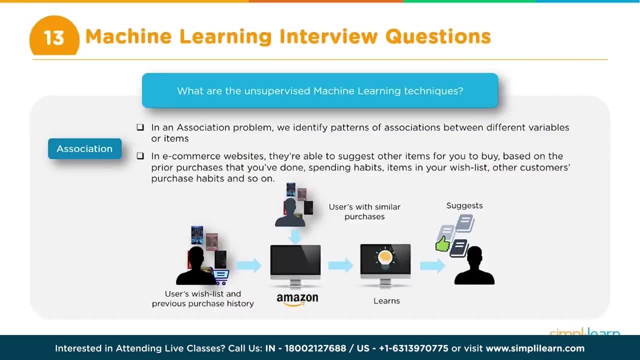 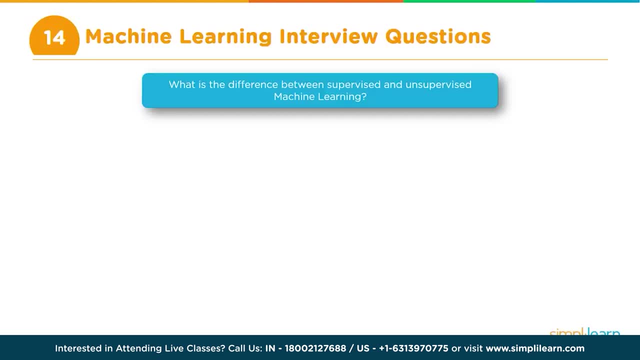 So that is an association that can be created. So this is unsupervised learning, One of the techniques. Alright, then we have a fundamental question: What is the difference between supervised and unsupervised machine learning? So machine learning, These are the two main types of machine learning. 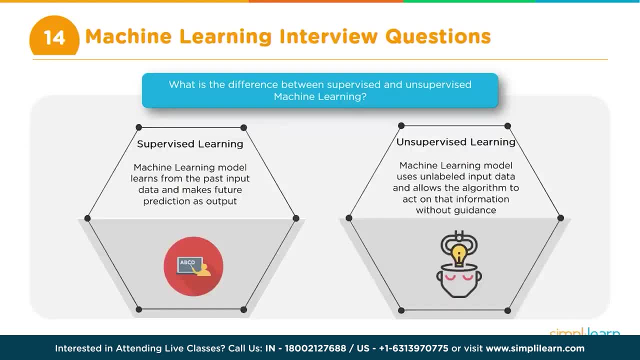 Supervised and unsupervised And in case of supervised- And again here probably the key word that the person may be wanting to hear is labeled data. Now, very often people say we have historical data And if we run it it is supervised. 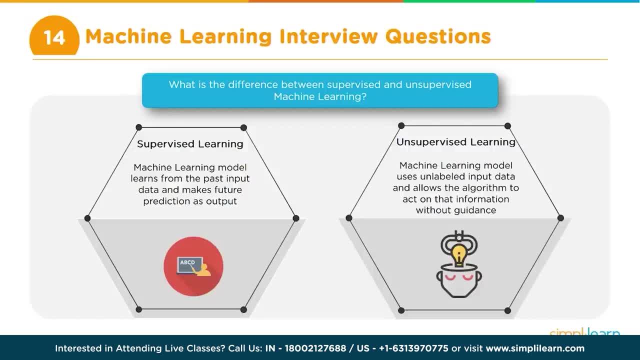 And if we don't have historical data, yes, But you may have historical data, But if it is not labeled, then you cannot use it for supervised learning. So it is very key to understand that we put in that key word labeled. So when we have labeled data for training, our model- 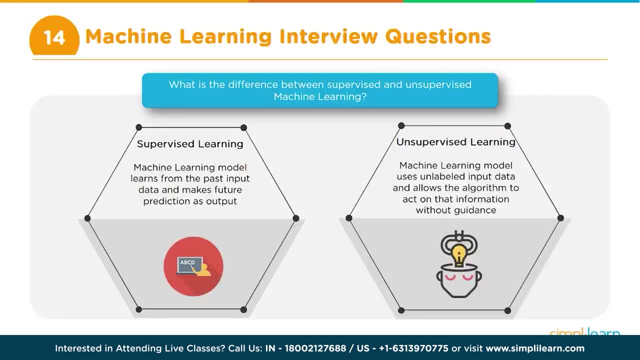 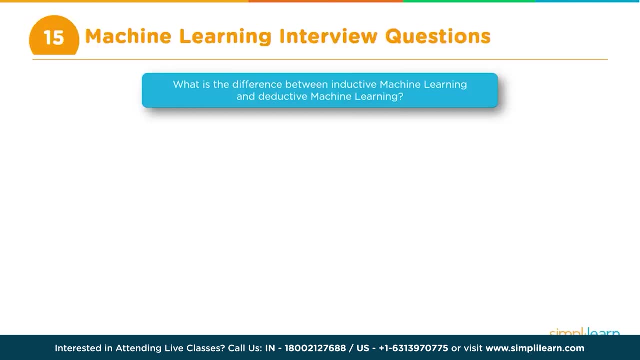 Then we can use supervised learning, And if we do not have labeled data, Then we use unsupervised learning, And there are different algorithms available to perform both of these types of trainings. So there can be another question A little bit more theoretical and conceptual in nature. 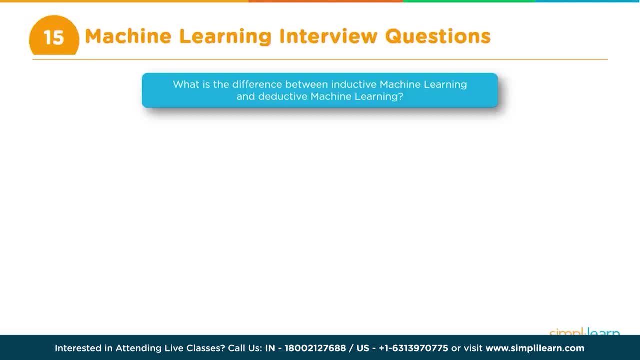 This is about inductive machine learning and deductive machine learning. So the question can be: what is the difference between inductive machine learning and deductive machine learning, Or somewhat in that manner, So that the exact phrase or exact question can vary And they can ask for examples and things like that. 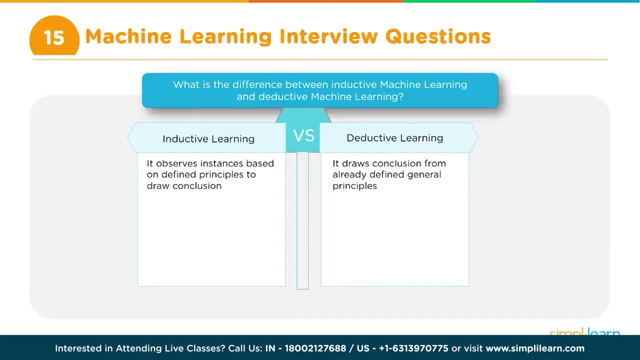 But that could be the question. So let's first understand what is inductive and deductive training. Inductive training is induced by somebody And you can illustrate that with a small example. I think that always helps. So whenever you are doing some explanation. 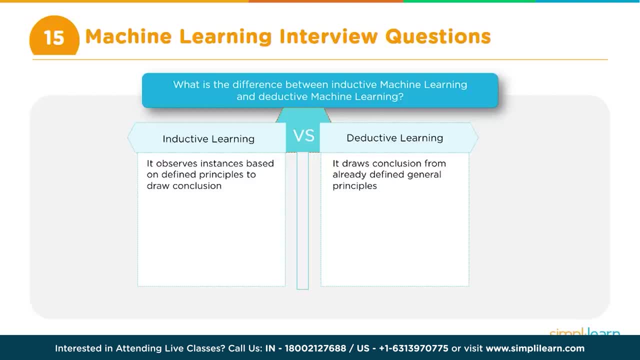 Try as much as possible, as I said, Take some examples from your work experience Or give some analogies, And that will also help a lot in explaining as well And for the interviewer also to understand. So here we will take an example. 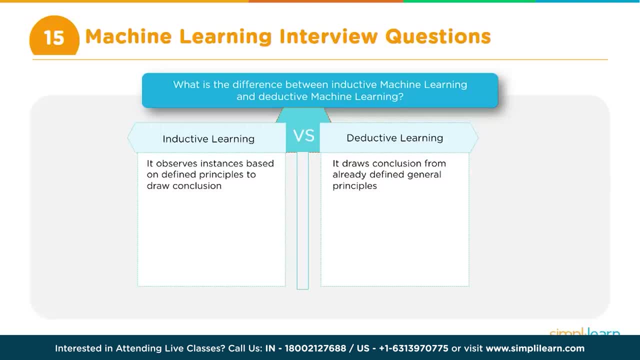 Or rather we will use an analogy. So inductive training is when we induce some knowledge or the learning process into a person Without the person actually experiencing it. What can be an example? So we can probably tell the person Or show a person a video. 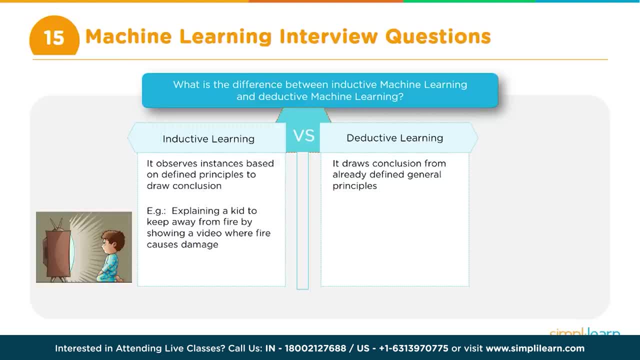 That fire can burn his finger Or fire can cause damage. So what is happening here? This person has never, probably, seen a fire Or never seen anything getting damaged by fire, But just because he has seen this video, He knows that fire is dangerous. 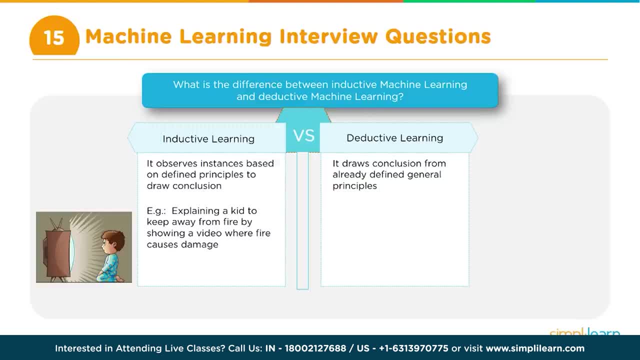 And fire can cause damage. So this is inductive learning. Compared to that, What is deductive learning? So here you draw conclusion, Or the person draws conclusion Out of experience. So we will stick to the analogy. So, compared to showing a video, 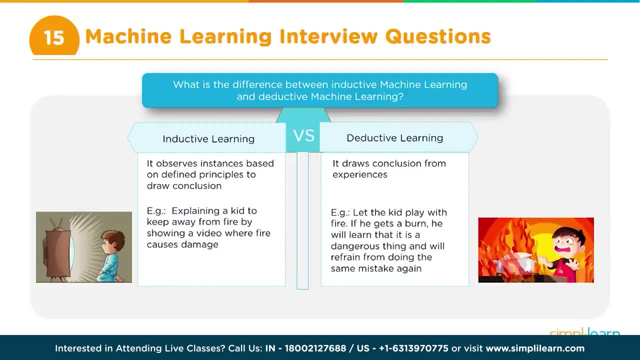 Let's assume a person is allowed to play with fire And then he figures out that if he puts his finger It's burning, Or if he throws something into the fire It burns. So he is learning through experience. So this is known as deductive learning. 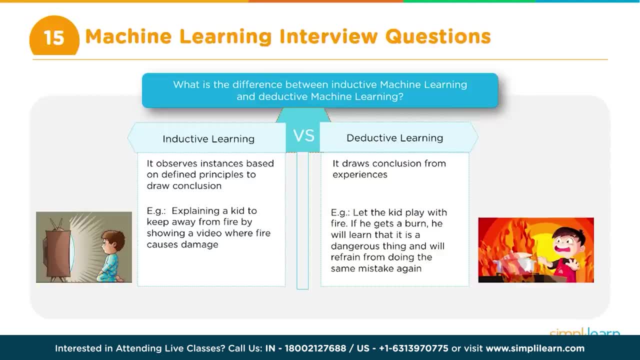 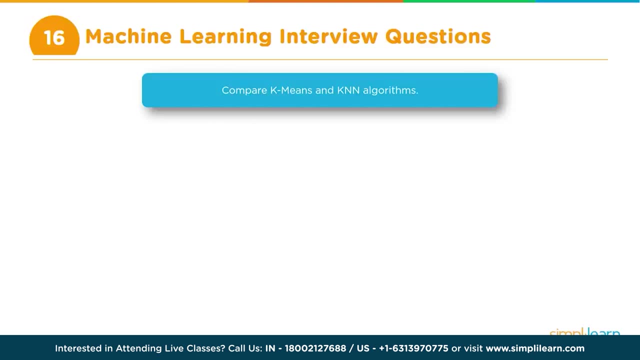 So you can have applications Or models that can be trained using inductive learning Or deductive learning. Alright, I think probably that explanation will be sufficient. The next question is: Are KNN and K-means clustering similar to one another? 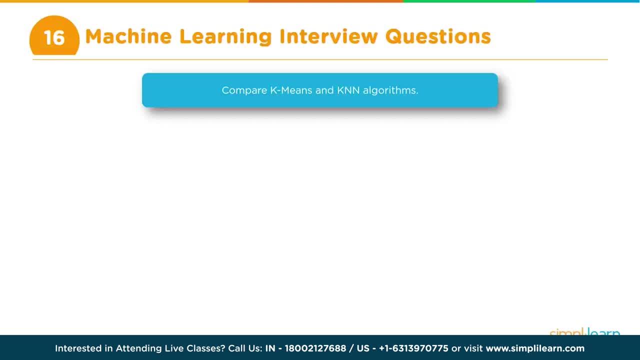 Or are they same? Because the letter K is kind of common between them. So let us take a little while to understand what these two are. One is KNN, Another is K-means. KNN stands for K-nearest neighbors And K-means, of course, is the clustering neighbors. 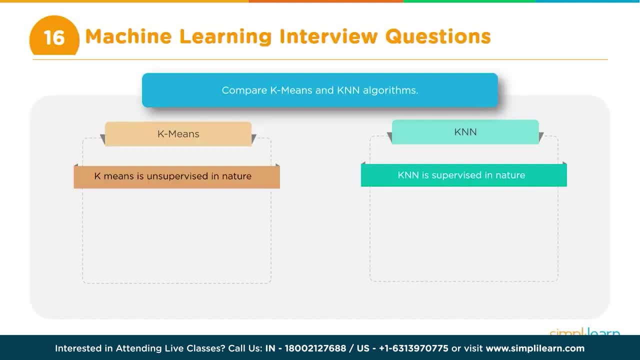 Now, these two are completely different Except for the letter K being common between them. KNN is completely different. K-means clustering is completely different. KNN is a classification process And therefore it comes under supervised learning, Whereas K-means clustering is actually unsupervised. 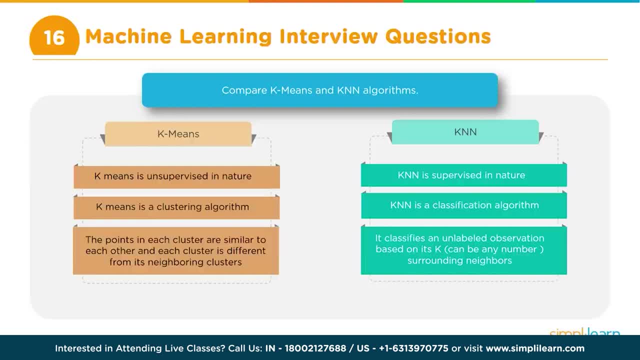 When you have KNN, When you want to implement KNN, Which is basically K-nearest neighbors, The value of K is a number, So you can say K is equal to 3.. You want to implement KNN with, K is equal to 3.. 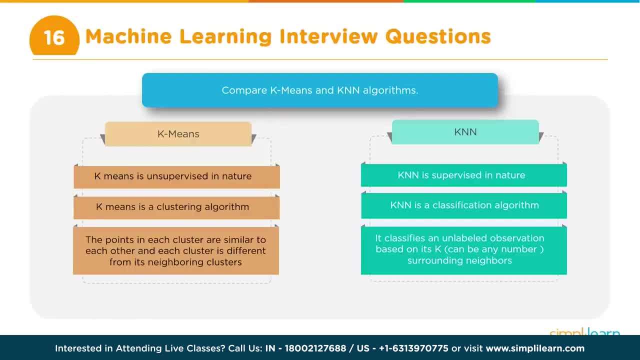 So, which means that It performs the classification In such a way that: How does it perform the classification? So it will take 3 nearest objects And that is why it is called nearest neighbors. So basically, based on the distance, It will try to find out its nearest objects. 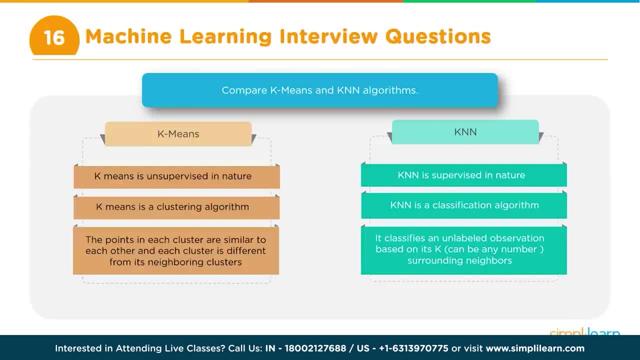 That are 3 of the nearest objects And then it will check whether the class They belong to which class. So if all 3 belong to one particular class, Obviously this new object Is also classified as that particular class. But it is possible that they may be. 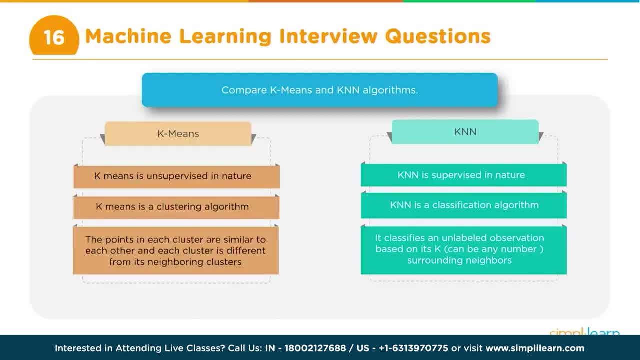 From 2 or 3 different classes. So let us say they are from 2 classes. And then, if they are from 2 classes, Now usually you take an odd number, You assign an odd number to. So if there are 3 of them, 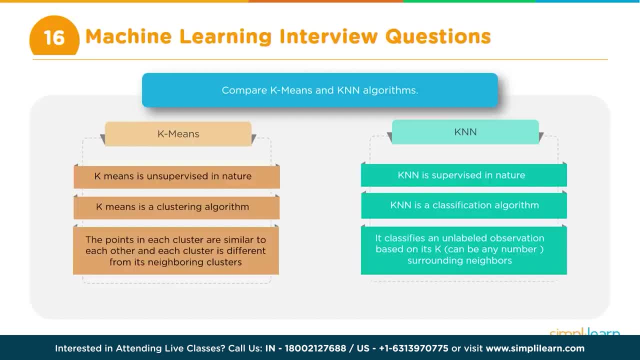 And 2 of them belong to 1 class, And then 1 belongs to another class, So this new object is assigned To the class to which the 2 of them belong. Now the value of K is sometimes Tricky. whether should you use 3.. 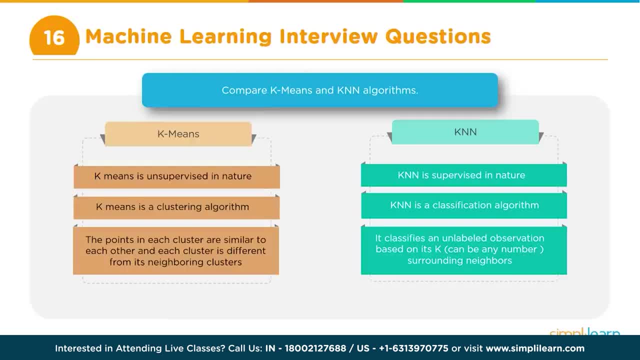 Should you use 5.? Should you use 7.? That can be tricky because The ultimate classification can also vary. So it is possible that if you are taking K as 3. The object is probably in one particular class, But if you take, K is equal to 5.. 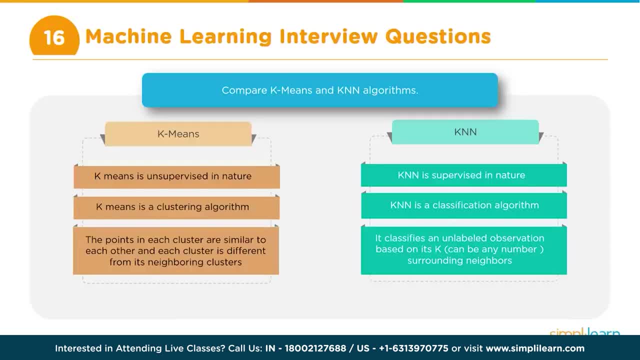 Maybe the object will belong to a different class, Because when you are taking 3 of them, Probably 2 of them belong to class 1. And 1 belong to class 2. Whereas when you take 5. It is possible that only 2 of them. 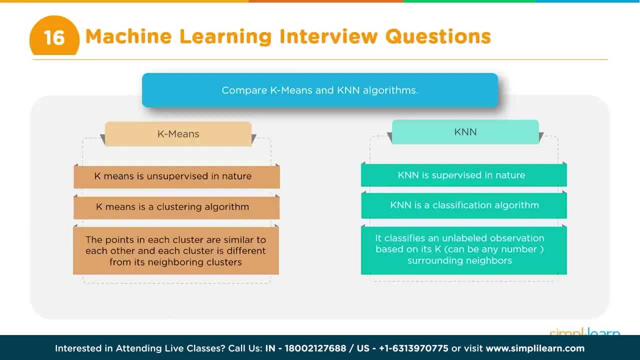 Belong to class 1. And 3 of them belong to class 2.. So, which means that This object will belong to class 2.. So you see that. So it is. the class allocation can vary Depending on the value of K. 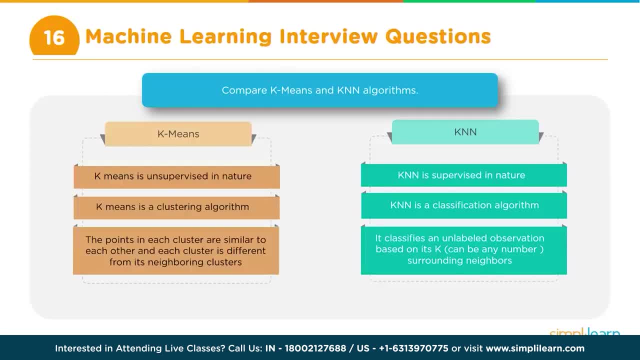 Now K means, on the other hand, Is a clustering process And it is unsupervised, Where what it does is The system will basically identify How the objects are, How close the objects are With respect to some of their features. 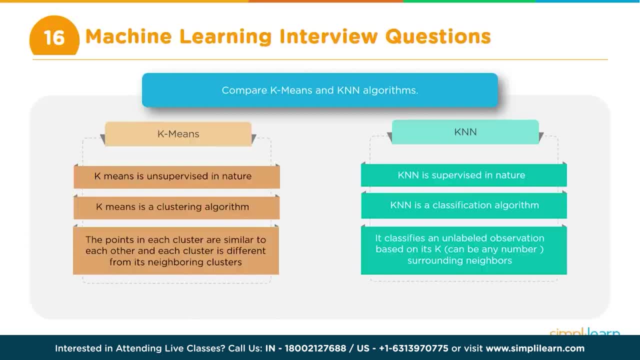 Okay, And the system will basically Identify The objects. Okay, And, but the similarity, of course, Is the letter K, And in case of K means Also we specify its value, And it could be 3 or 5 or 7.. 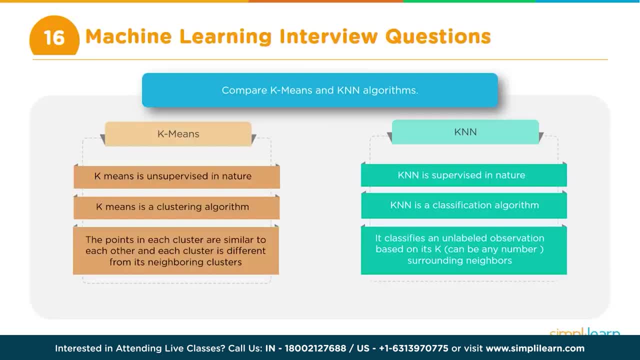 There is no technical limit as such, But it can be any number of clusters That you can create. Okay, So based on the value that you provide, The system will create that many clusters Of similar objects. So there is a similarity to that extent. 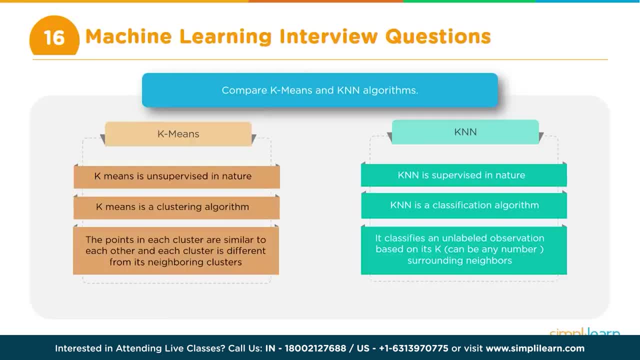 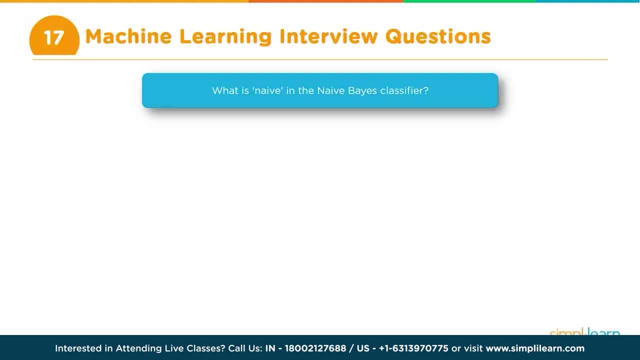 That K is a number In both the cases, But actually There are two completely different processes. We have what is known as naive base classifier, And people often get confused, Thinking that naive base is the name of the person Who found this classifier. 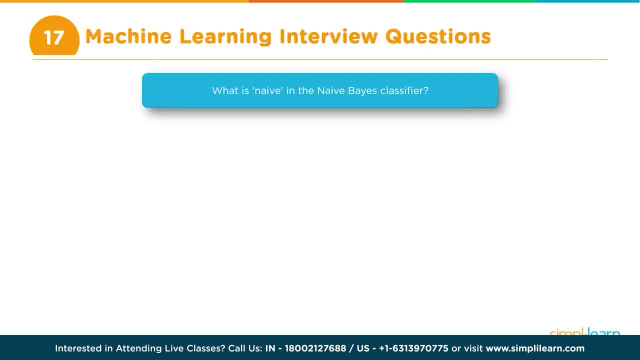 Or who developed this classifier, Which is not 100% true. Base is the name of the person, B A, Y, S is the name of the person, But naive is not the name of the person, Right? So naive is basically an English word. 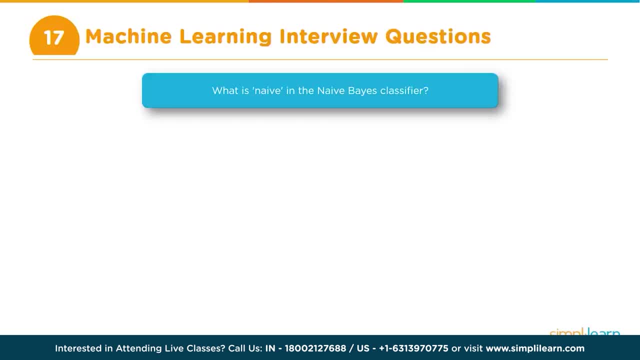 And that has been added here Because of the nature of this particular classifier. Naive base classifier Is a probability based classifier And it makes some assumptions That presence of one feature of a class Is not related to the presence of any other feature. 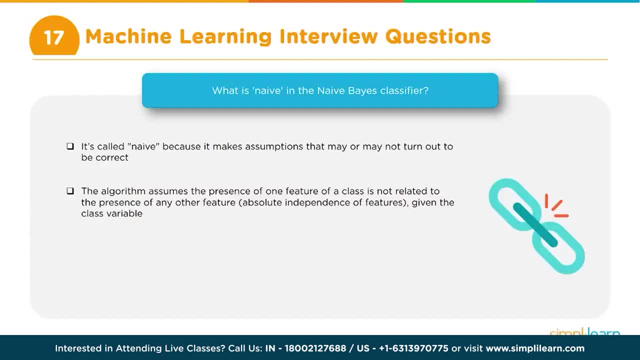 Of maybe other classes, Right? So which is not a very strong Or not a very, What do you say, Accurate assumption, Because these features can be related and so on. But even if we go with this assumption, This whole algorithm works very well. 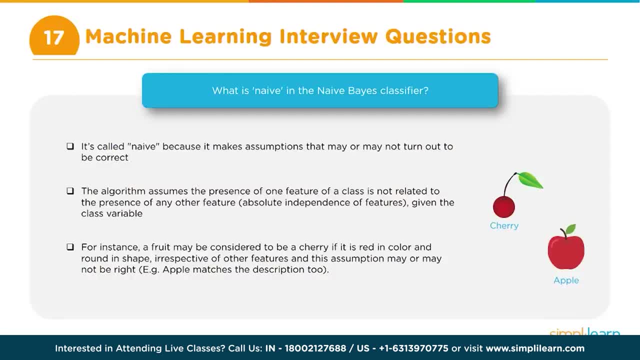 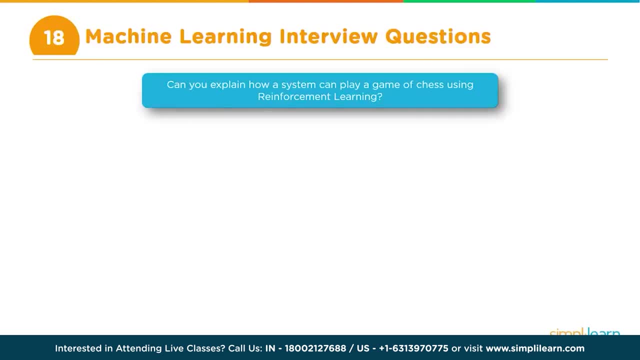 Even with this assumption, And that is the reason, And that is the good side of it, But the term comes from that, So that is the explanation That you can give. Then there can be question around Reinforcement learning. It can be paraphrased in multiple ways. 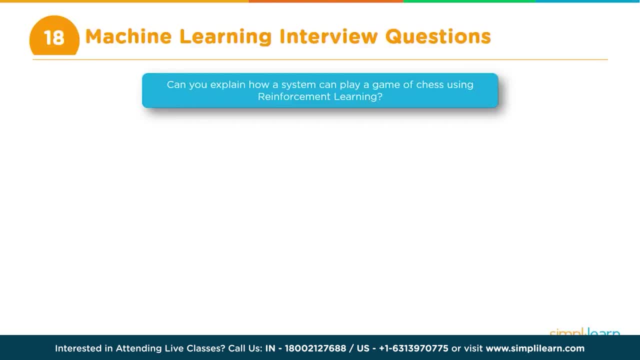 One could be. Can you explain how a system can play a game of chess Using reinforcement learning, Or it can be any game. So the best way to explain this is again To talk a little bit about What reinforcement learning is about. 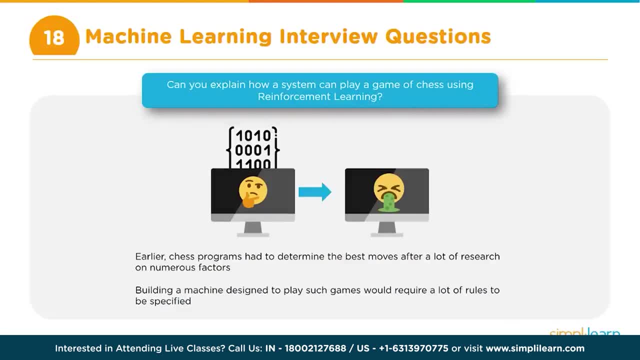 To explain the process. So, first of all, Reinforcement learning has an environment And an agent, And the agent is basically performing some actions In order to achieve a certain goal, And these goals can be anything, Either if it is related to game. 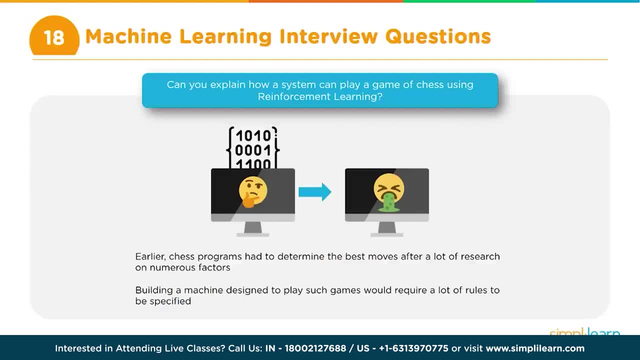 Then the goal could be that You have to score very high. Score a high value, High number. Or it could be that your number of lives Should be as high as possible. Don't lose lives. More advanced examples could be For driving. 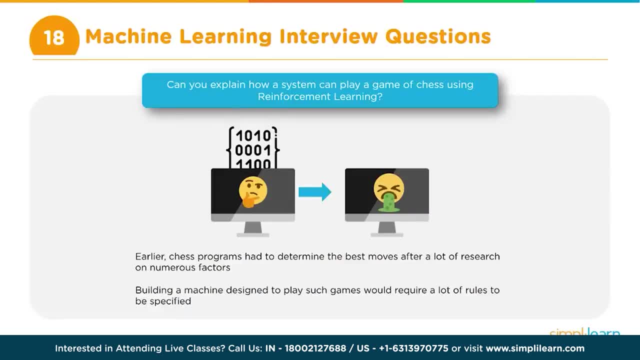 In the automotive industry- Self driving cars. They actually also make use of reinforcement learning To teach the car how to navigate through the roads, And so on and so forth. That is also another example. Now how does it work? So, if the system is? 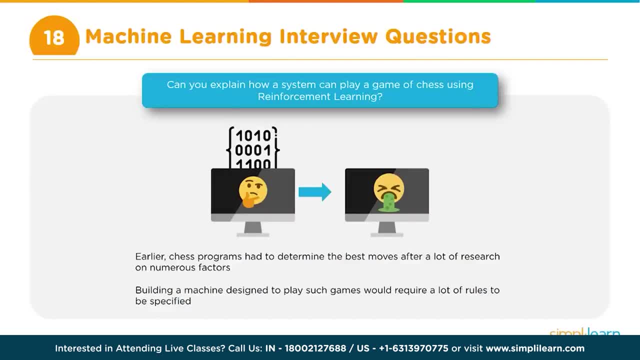 Basically, there is an agent in the environment And every time, the agent takes a step Or performs a task Which is taking it towards the goal, The final goal, To minimize the number of lives and so on, Or minimize the deaths, for example. 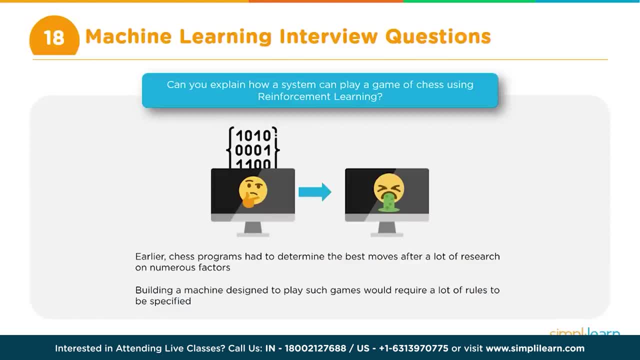 It is rewarded, And every time it takes a step Which goes against that goal, Contrary or in the reverse direction, It is penalized. So it is like a carrot and stick system. Now how do you use this To create a game of chess? 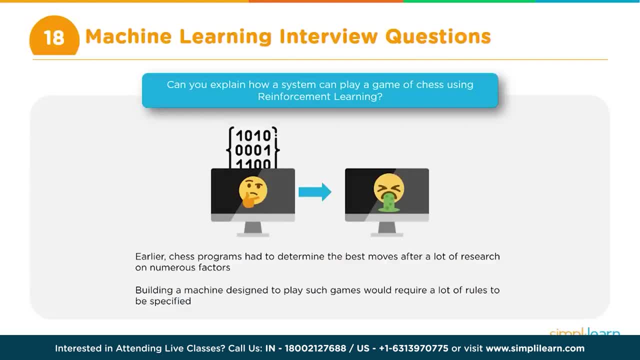 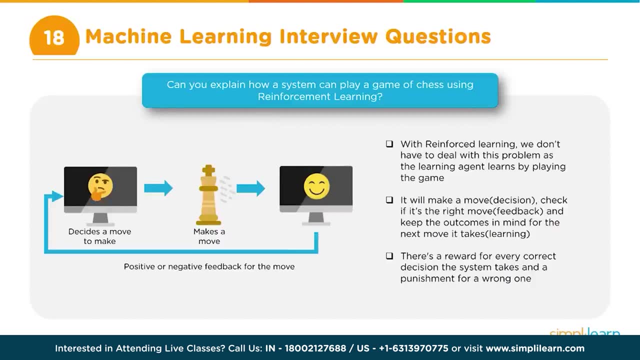 Or to create a system to play a game of chess. Now, the way this works is- And this could probably go back to this AlphaGo example, Where you created a human champion- So the way it works is in reinforcement learning, The system is allowed. 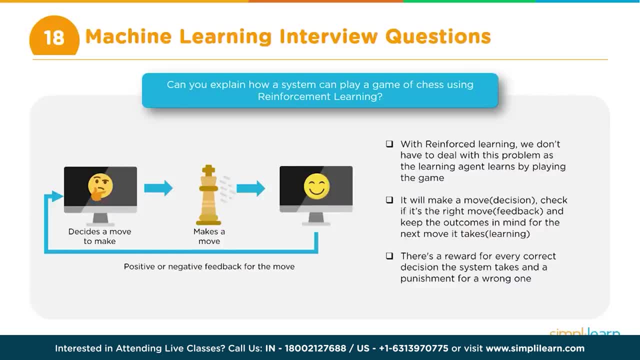 For example, in this case We are talking about chess, So we allow the system to first of all Watch playing a game of chess. So it could be with a human being, Or it could be the system itself. There are computer games of chess. 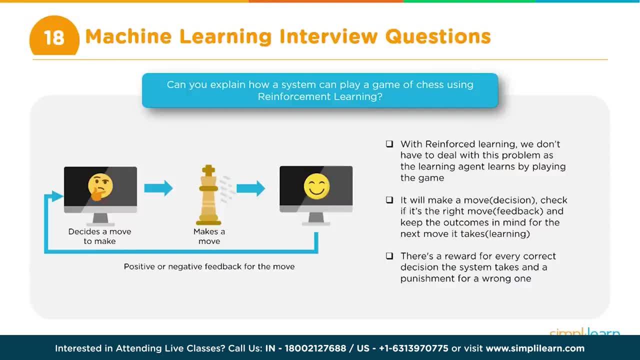 Right. So either this new learning system Has to watch that game Or watch a human being play the game, Because this is reinforcement learning And reinforcement learning is Pretty much all visual. So when you are teaching the system To play a game, 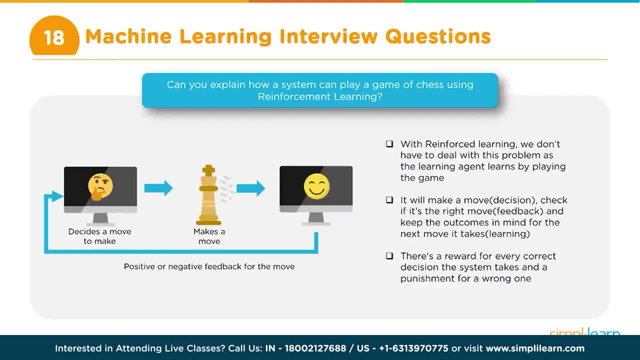 The system will not actually go behind the scenes To understand the logic of your software, Of this game or anything like that. It is just visually watching the screen And then it learns. So reinforcement learning to a large extent Works on that. 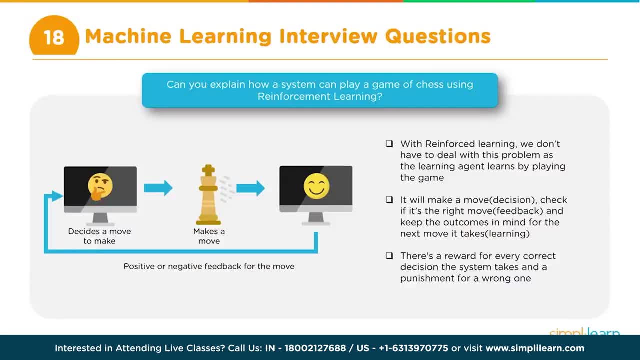 So you need to create a mechanism Where, by your model, Will be able to watch Somebody playing the game And then you allow the system Also to start playing the game. So it pretty much starts from scratch, Okay, And as it moves forward, 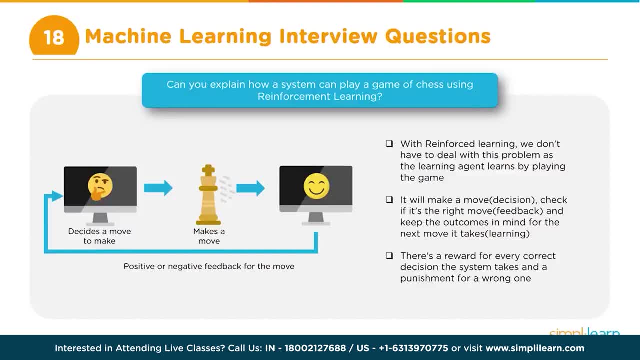 Right at the beginning, The system really knows nothing About the game of chess. Okay, So initially it is a clean slate. It just starts by observing How you are playing, So it will make some random moves And keep losing- badly. 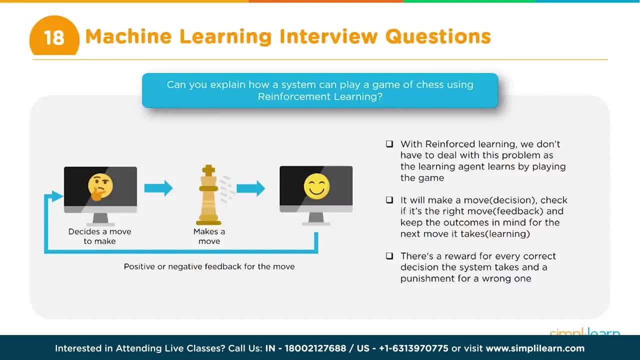 So you need to now Allow the system Or you need to play with the system, Not just one, two, three, four or five times, But hundreds of times, Thousands of times, Maybe even hundreds of thousands of times, And that is exactly how AlphaGo has done. 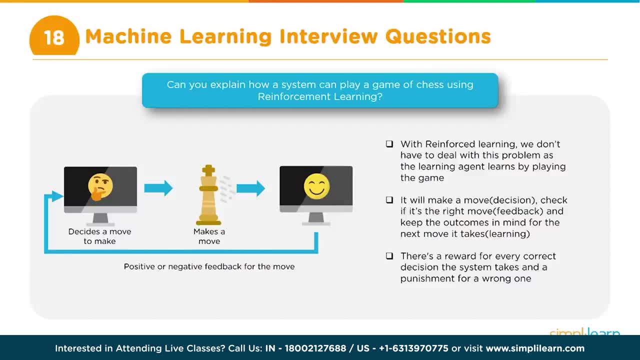 It played millions of games Between itself and the system Right. So for the game of chess also, You need to do something like that. You need to allow the system to play chess On its own Over a period of repetition. So I think you can probably explain it. 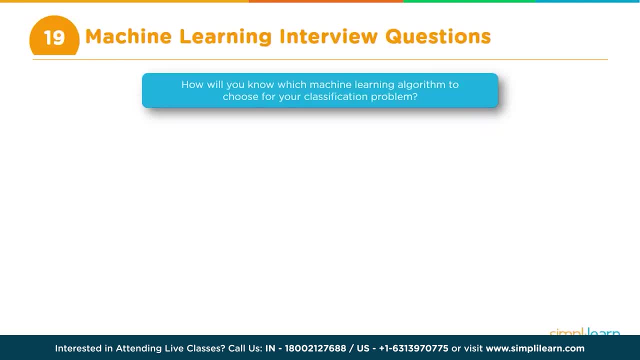 To this much, To this extent, And it should be sufficient. Now this is another question Which is again somewhat similar, But here the size is not coming into picture. So the question is: How will you know which machine learning algorithm to choose? 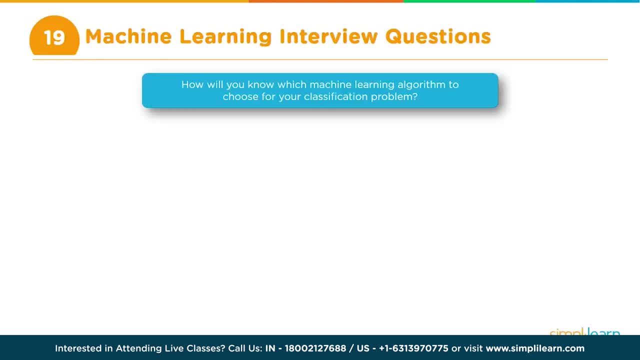 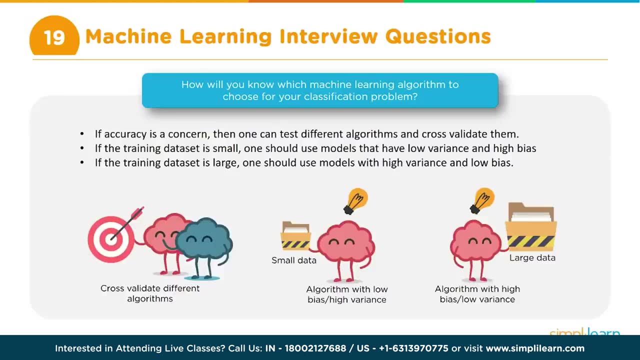 For your classification problem. Now, this is not only classification problem. It could be a regression problem. I would like to generalize this question And I am going to use The simple answer is: There is no way you can decide Exactly, saying that. 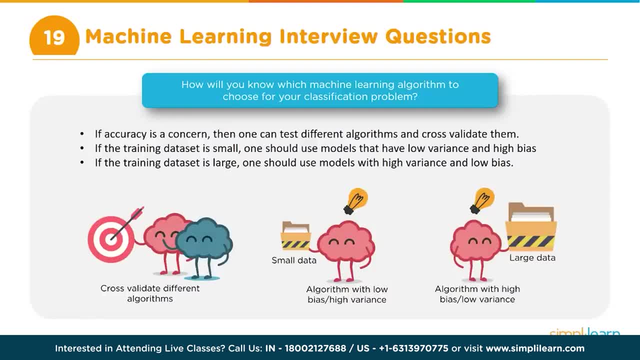 This is the algorithm I am going to use In a variety of situations. There are some guidelines Like, for example: You will obviously, depending on the problem, You can say whether it is a classification problem Or a regression problem And then, in that sense, 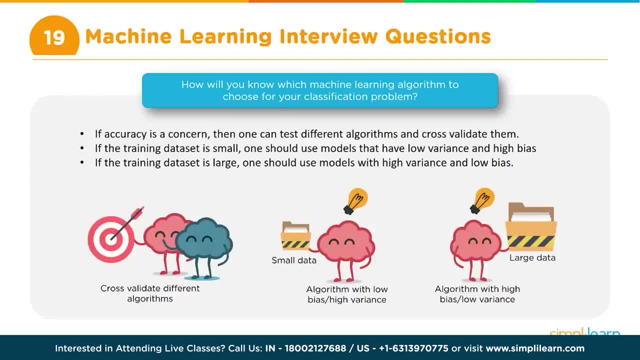 You are kind of restricting yourself to If it is a classification problem There are, You can limit the number of algorithms. But now, Within the classification algorithms You have decision trees, You have SVM, You have logistic regression. Is it possible to outright say yes? 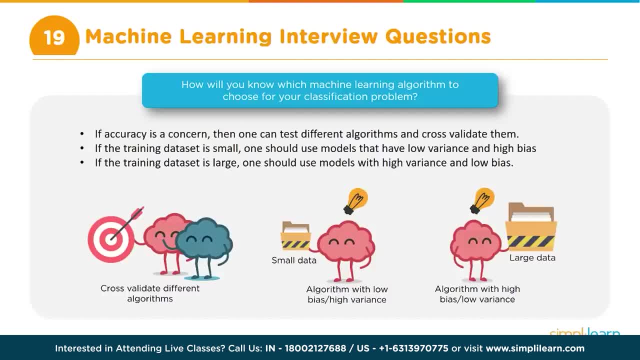 For this particular problem, Since you have explained this, Now, this is the exact algorithm that you can use. That is not possible. So we have to try out a bunch of algorithms, See which one gives us the best performance, Best accuracy, And then decide to go with. 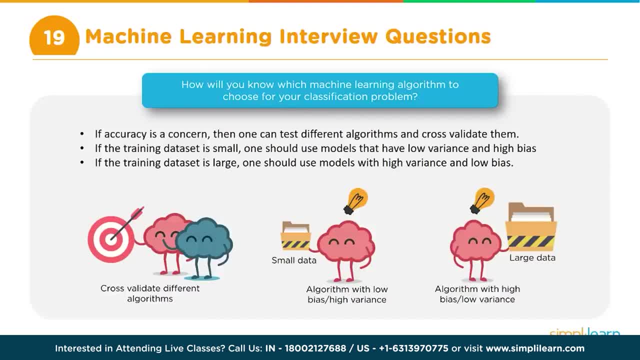 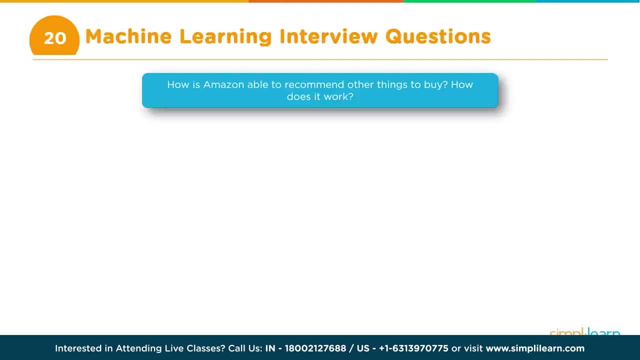 This particular algorithm. So in machine learning, A lot of it happens through trial and error. There is no real possibility that anybody can, Just by looking at the problem Or understanding the problem, Tell you that, okay, In this particular situation, This is exactly the algorithm that you should use. 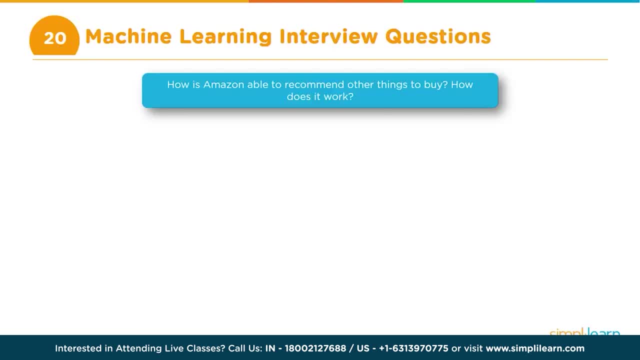 Then the questions may be around Application of machine learning, And this question is specifically around How Amazon is able to recommend Other things to buy. How does it work? How does the recommendation engine work? So this is basically the question is all about. 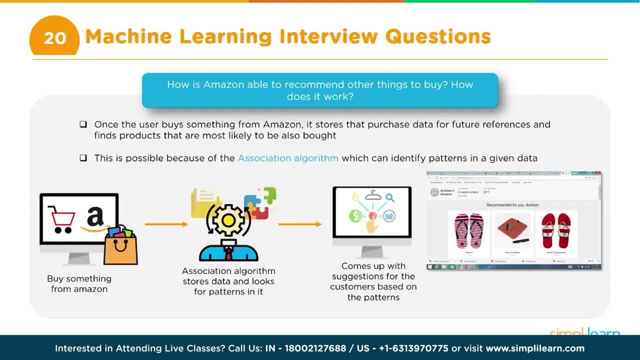 So the recommendation engine again Works based on various inputs That are provided. Obviously, something like Amazon website or e-commerce site Like Amazon collects a lot of data Around the customer behavior- Who is purchasing what, And if somebody is buying a particular thing. 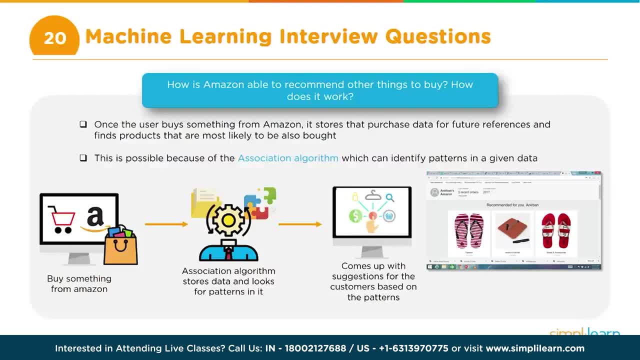 They are also buying something else. So this kind of association- So this is the unsupervised learning That we talked about- They use this to associate and link Or relate items, And that is one part of it. So they kind of build association between items. 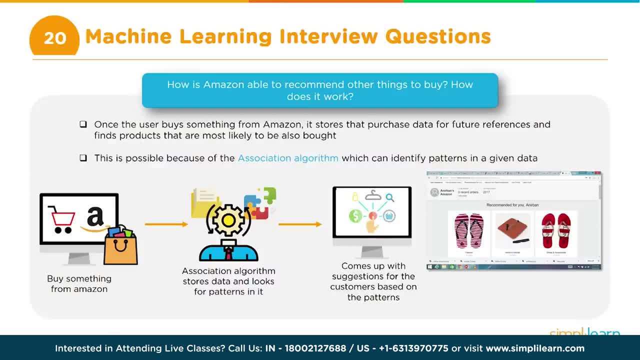 Saying that somebody buying this is also buying this. That is one part of it. Then they also profile the users Based on their age, Their gender, Their geographic location. They will do some profiling And then, when somebody is logging in And when somebody is shopping, 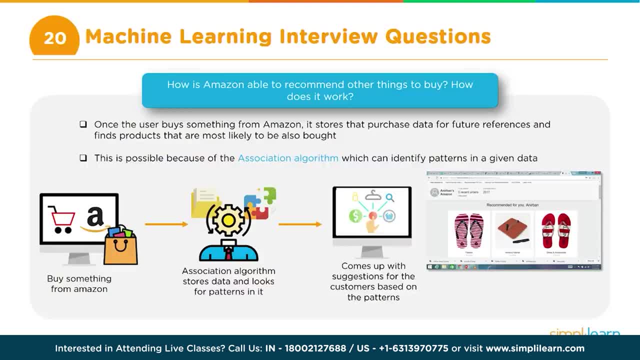 Kind of the mapping of these two things are done, Obviously, if you have logged in, Then they know who you are And your information is available, Like, for example, your age, maybe Your gender, And where you are located, What you purchased earlier. 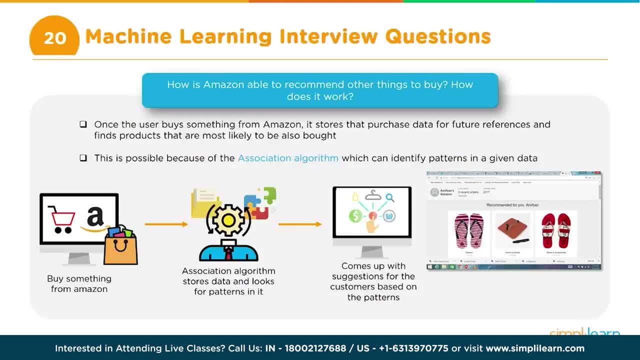 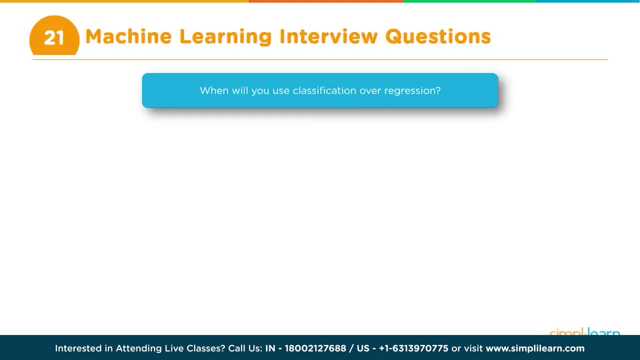 So all this is taken And the recommendation engine basically Uses all this information And comes up with recommendations For a particular user. So that is how recommendation engine works. Alright, So this is basically something very basic Like: when will you go for classification? 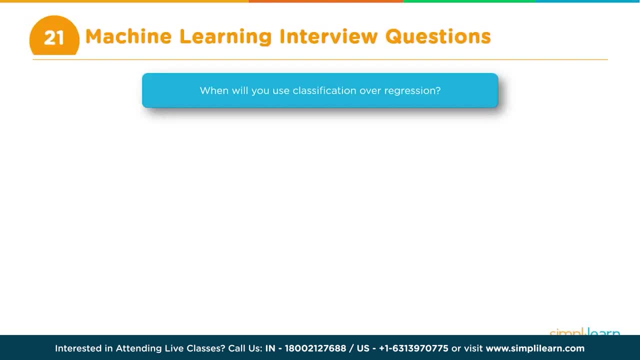 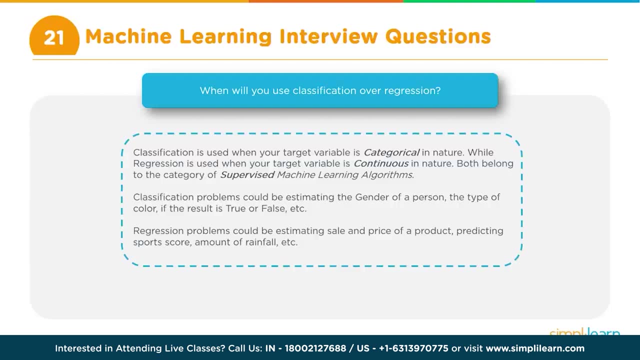 Versus regression? When do you do classification Instead of regression, Or when will you use classification instead of regression? Now, yes, So this is basically going back to the understanding Of the basics of classification and regression. So classification is used When you have to identify. 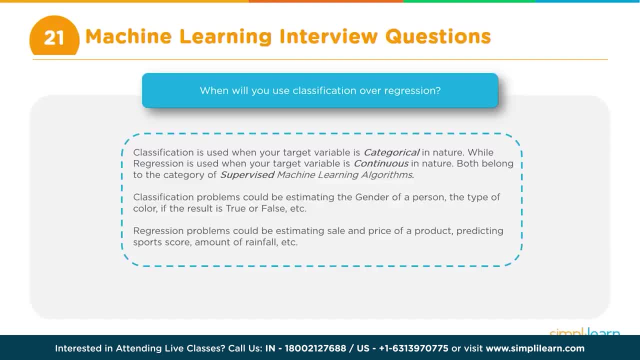 Or categorize Things into discrete classes. So the best way to respond to this question Is to take up some examples And use it. Otherwise it can become a little tricky. The question may sound very simple, But explaining it can sometimes be very tricky. 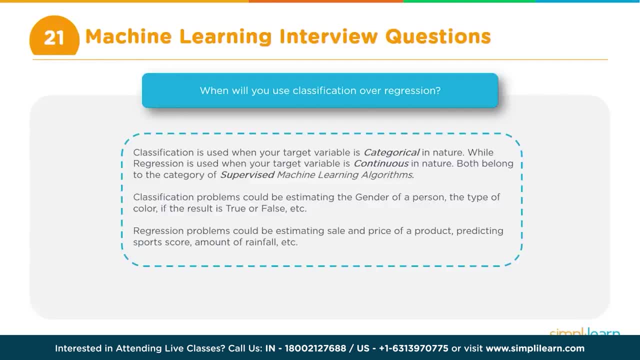 In case of regression We use. of course there will be some keywords That they will be looking for, So just you need to make sure you use those keywords. One is the discrete values, Another is the continuous values. So, for regression, If you are trying to find some continuous values, 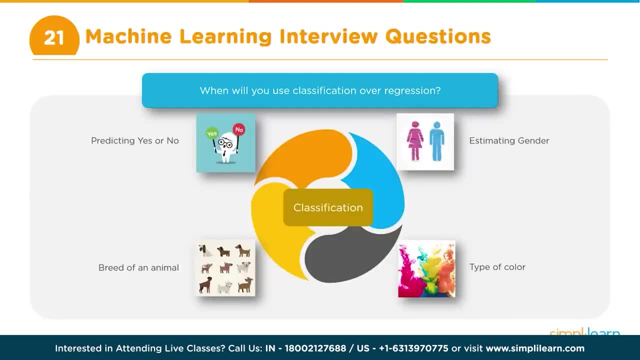 You use regression, Whereas if you are trying to find some discrete values, You use classification. So classification is like, Let's say, there are images And you need to put them into classes Like cat, dog, elephant, tiger, Something like that. 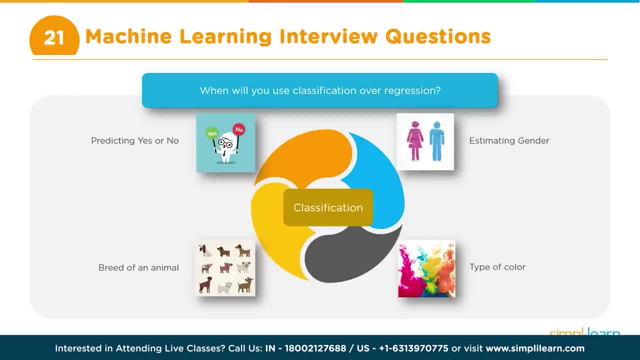 So that is a classification problem, Or it can be That is a multi class classification problem. It could be binary classification problem, Like, for example, Whether a customer will buy or he will not buy. That is a classification, Binary classification. It can be in the weather forecast area. 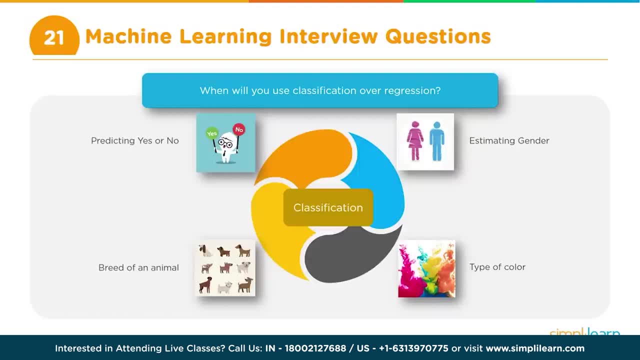 Now weather forecast is again A combination of regression and classification, Because on the one hand, You want to predict whether it is going to rain or not. That is a classification problem, That is a binary classification: Whether it is going to rain or not rain. 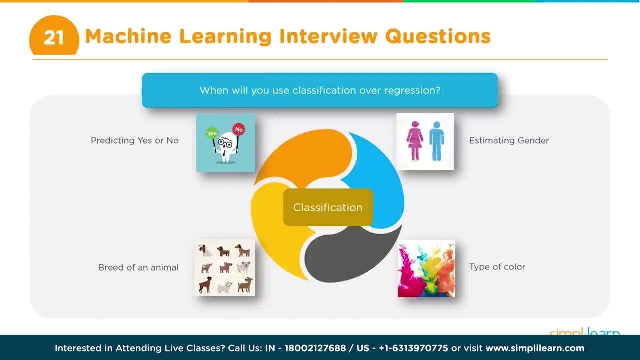 However, you also have to predict What is going to be the temperature tomorrow. Now, temperature is a continuous value. You can't answer the temperature In a yes or no kind of a response. So what will be the temperature tomorrow? So you need to give a number. 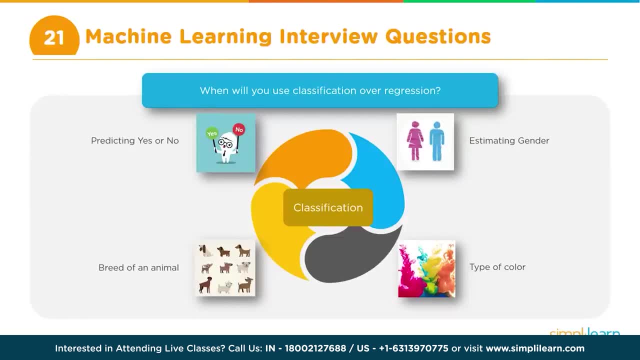 Which can be like 20 degrees, 30 degrees or whatever. So that is where you use Regression. One more example is stock price prediction. So that is where, again, You will use regression. So these are the various examples. So you need to illustrate with examples. 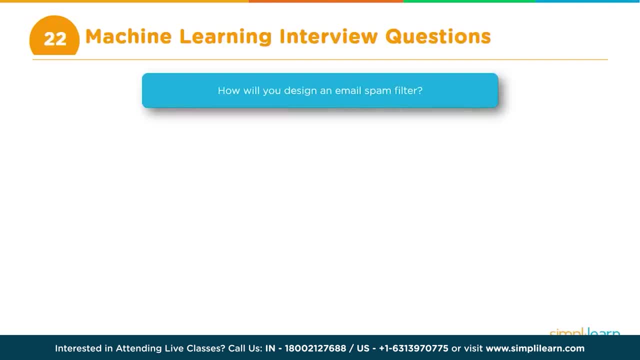 And make sure you include those keywords Like discrete and continuous. So the next question is more about A little bit of a design related question To understand your concepts And things like that. So it is: how will you design a spam filter? 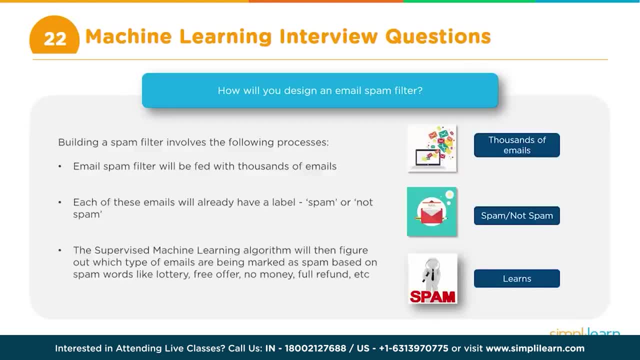 So how do you basically design Or develop a spam filter? So the first thing here is He is looking at probably understanding Your concepts in terms of What is the algorithm you will use, Or what is your understanding about Difference between classification and regression. 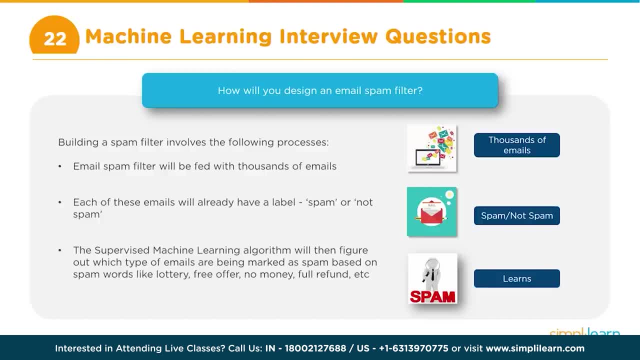 And things like that, And the process, of course, The methodology and the process. So the best way to go about responding to this Is we say that, okay, This is a classification problem, Because we want to find out Whether an email is a spam or not spam. 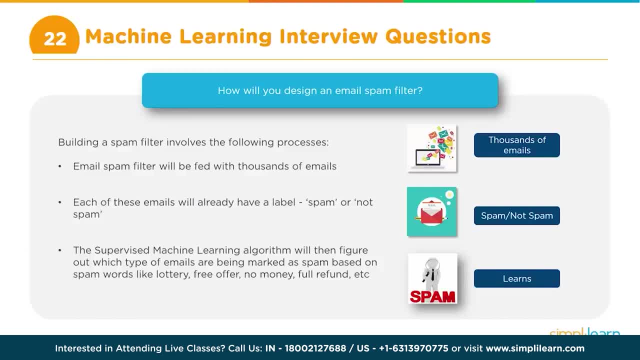 So that we can apply the filter accordingly. So the first step is to identify What type of a problem it is. So we have identified that it is a classification. Then the second step may be to find out What kind of algorithm to use. 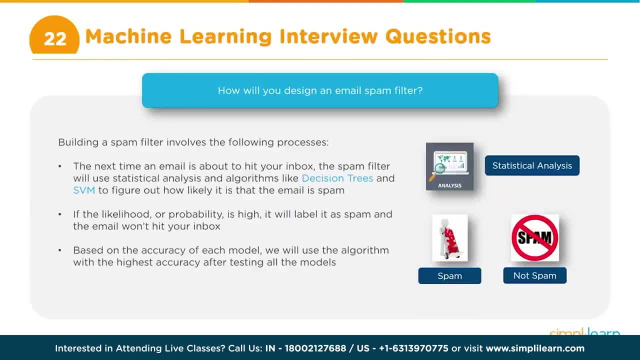 Now, since this is a binary classification problem, Logistic regression is a very common, Very common algorithm, But however right- As I said earlier also, We can never say that okay, For this particular problem, This is exactly the algorithm that we can use. 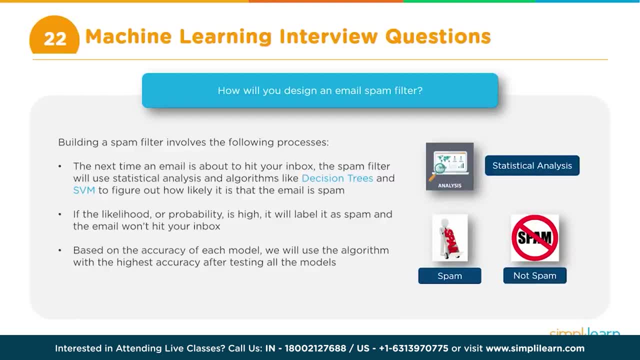 So we can also probably try decision trees Or even support vector machines, For example SVM. So we will kind of list down A few of these algorithms And we will say, okay, We would like to try out these algorithms, And then we go about taking. 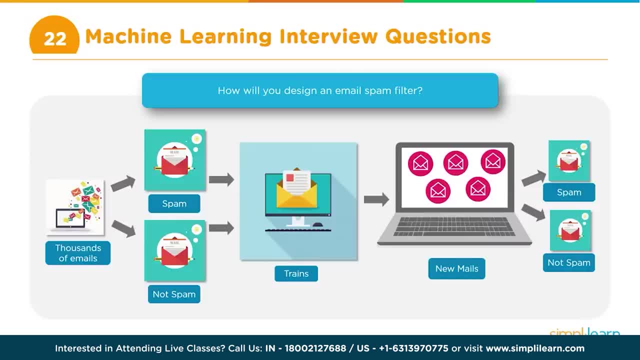 Your historical data, Which is the labeled data Which are marked. So you will have a bunch of emails And then you split that into training And test data sets. You use your training data set To train your model Or your algorithm that you have used. 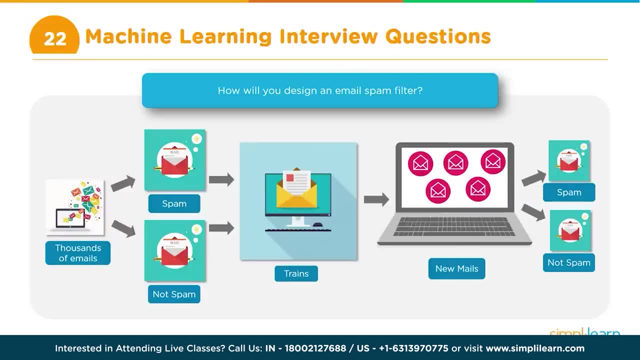 So and you actually Will have three models. Let's say you are trying to test out Three algorithms, So you will obviously have three models. So you need to try all three models And test them out as well, See which one gives the best accuracy. 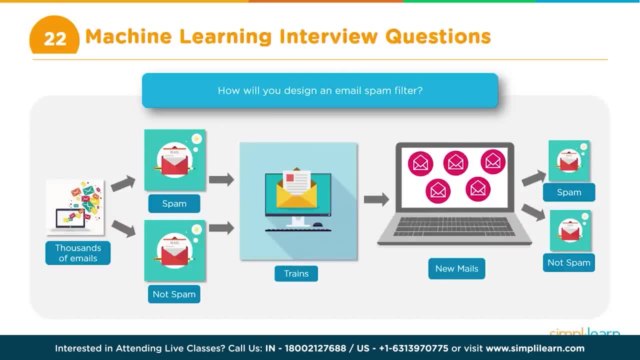 And then you decide that you will go with that model. Okay, so training and test will be done. And then you zero in on one particular model And then you say, okay, This is the model we will use And then go ahead and implement that. 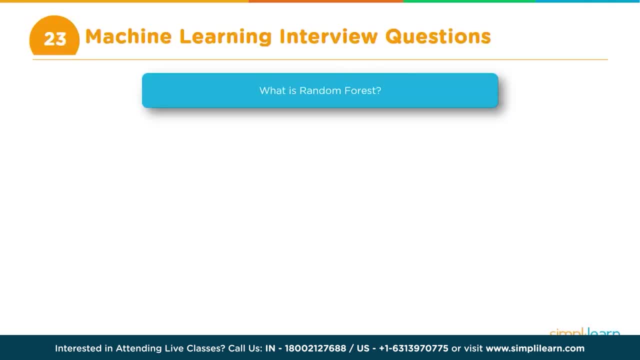 So that is the way you design a spam field. The next question is about random forest. What is random forest? So this is a very straight forward question. However, the response You need to be, again, a little careful. While we all know what is random forest, 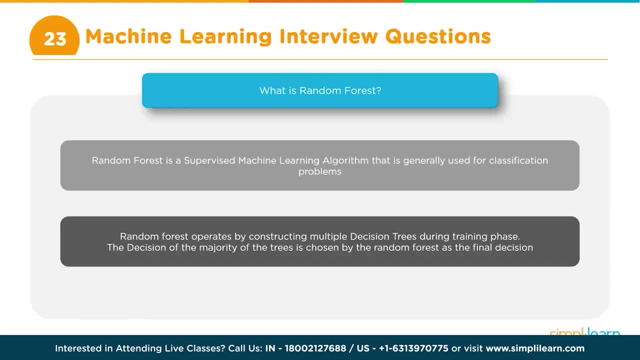 Explaining this can sometimes be tricky. So one thing is Random forest is kind of, In one way it is an extension Of decision trees, Because it is basically nothing but You have multiple decision trees And trees will basically You will use for doing. 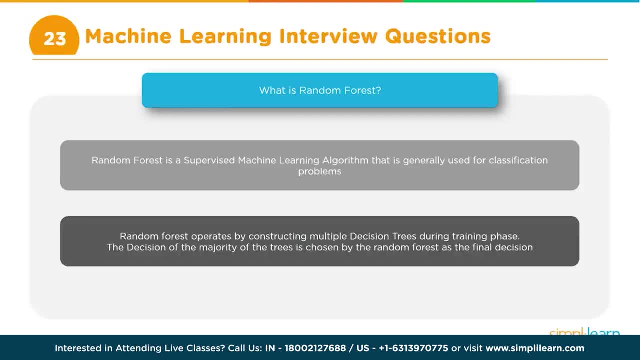 If it is classification- Mostly it is classification- You will use the trees for classification And then you use voting for finding the final class. So that is the underlines. But how will you explain this? How will you respond to this? So, first thing, obviously, 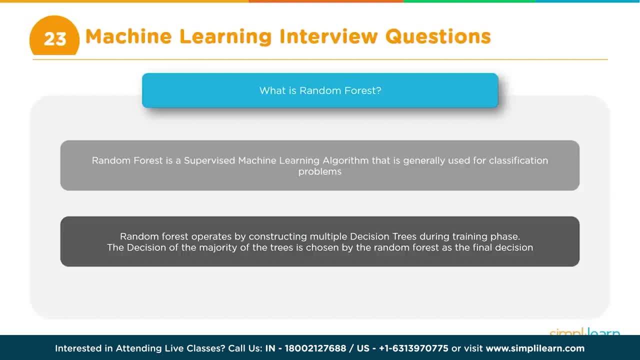 We will say that random forest is one of the algorithms, And the more important thing That you need- to Probably the interviewer is waiting to hear- Is ensemble learner. So this is one type of ensemble learner Is like a combination of algorithms. 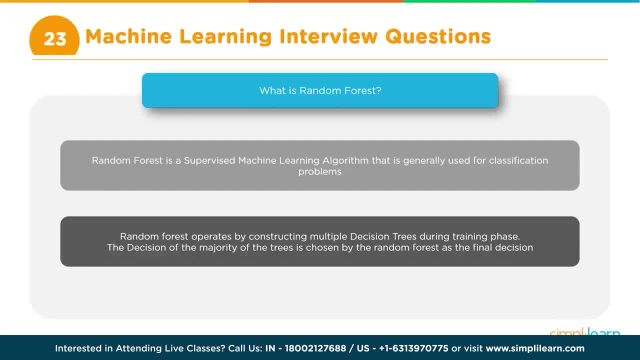 So it is a learner Which consists of more than one algorithm, Or more than one, Maybe, models. So in case of random forest, Algorithm is the same, But instead of using one instance of it, We use multiple instances of it, And we use 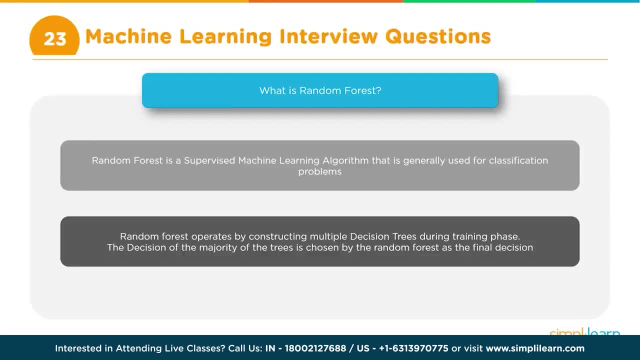 So in a way that is, a random forest is an ensemble learner. There are other types of ensemble learners Where we have, Like we use different algorithms itself, So you have one And a decision tree combined together, And so on and so forth. 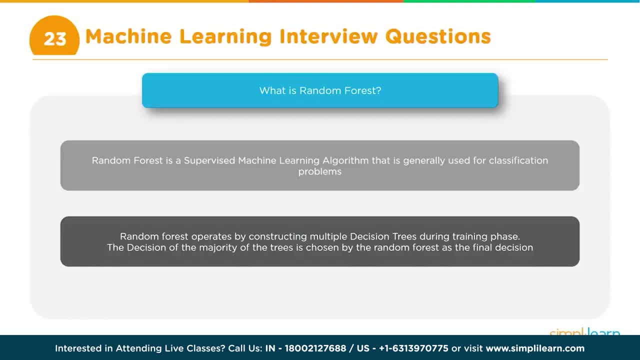 Or there are other ways Like, for example, splitting the data in a certain way And so on. So it is all about ensemble. We will not go into that, But random forest itself. I think the interviewer will be happy to hear this word. 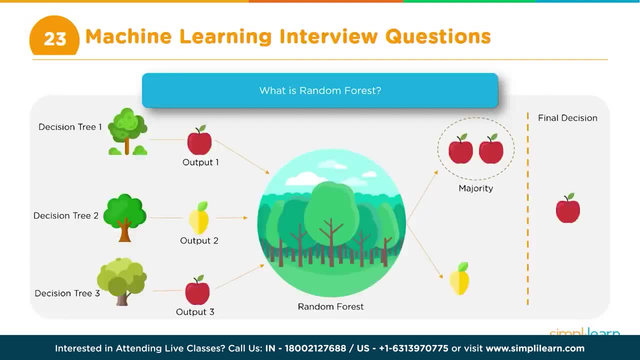 Ensemble learner. And so then you go and explain how the random forest works. So if the random forest is used for classification, Then we use what is known as a voting mechanism. So basically, how does it work? So random forest consists of 100 trees. 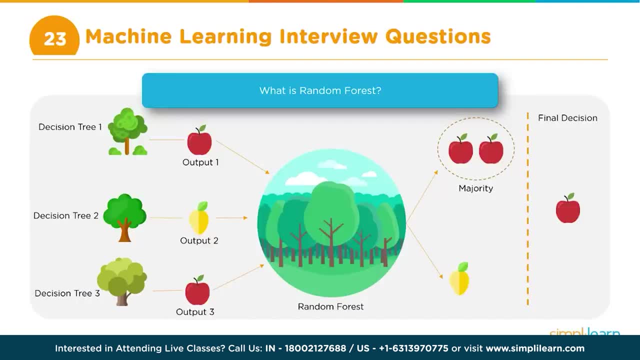 And each observation you pass through this forest, And each observation- Let us say it is a classification problem, Binary classification, 0 or 1.. And you have 100 trees. Now if 90 trees say that it is a 0. And 10 of the trees say it is a 1.. 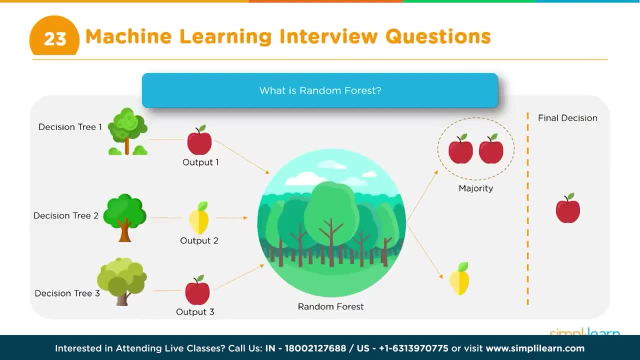 You take the majority, You may take a vote, And since 90 of them are saying 0. You classify this as 0. Then you take the next observation, and so on. So that is the way random forest works For classification. 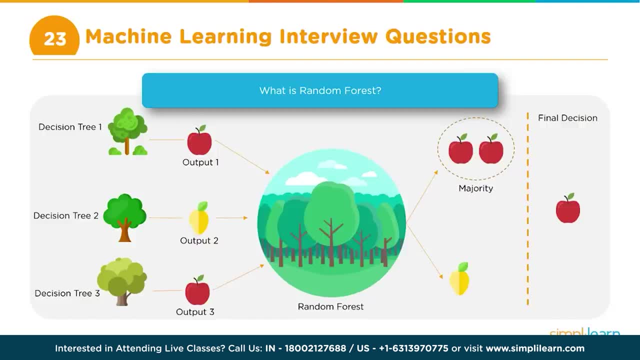 So this is the regression problem. It is somewhat similar, But the only thing is, instead of vote, What we will do is So, in regression, remember what happens- You actually calculate a value. So, for example, you are using regression to predict the temperature. 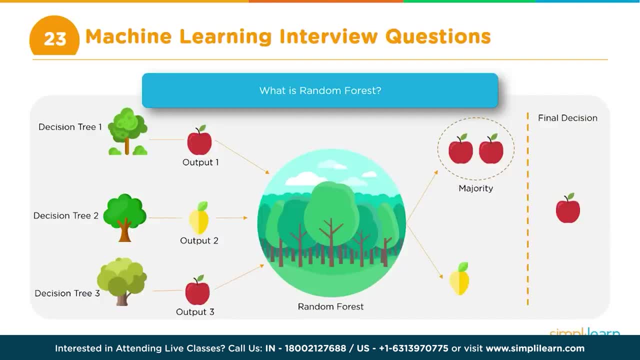 And you have 100 trees, And each tree obviously will probably predict a different value of the temperature. They may be close to each other, But they may not be exactly the same value. So these 100 trees. So how do you now find the actual value? 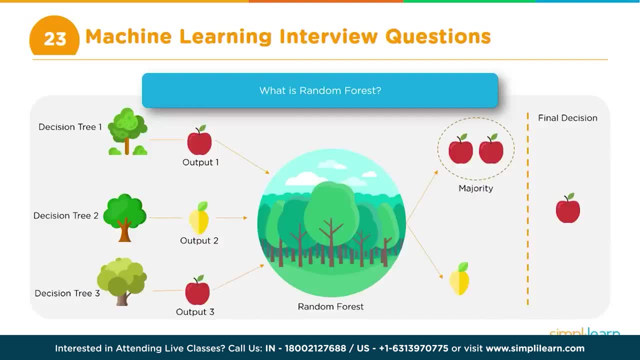 The output for the entire forest. So you have outputs of individual trees Which are a part of this forest, But then you need to find the final output of the forest itself. So how do you do that? So in case of regression You take like an average or the mean. 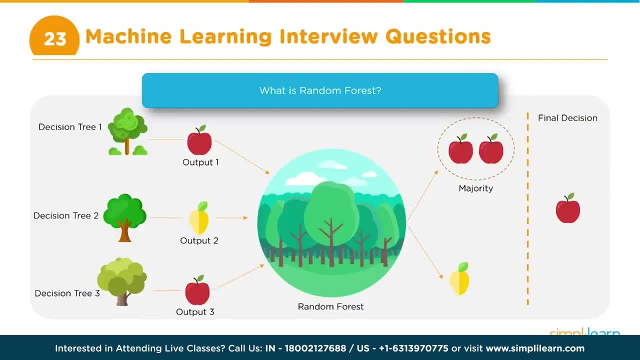 Of all the 100 trees. So this is also a way of reducing the error. So maybe if you have only one tree, And if that one tree makes an error, It is basically 100% wrong Or 100% right. But if you have, on the other hand, 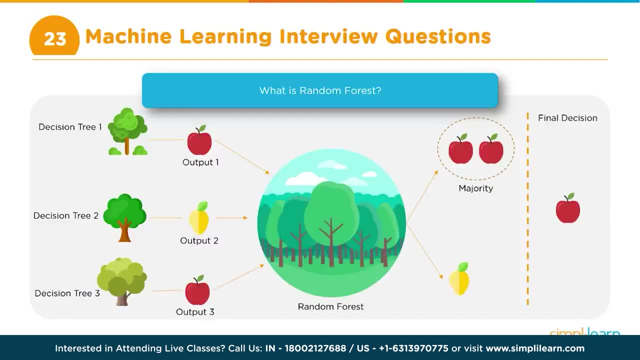 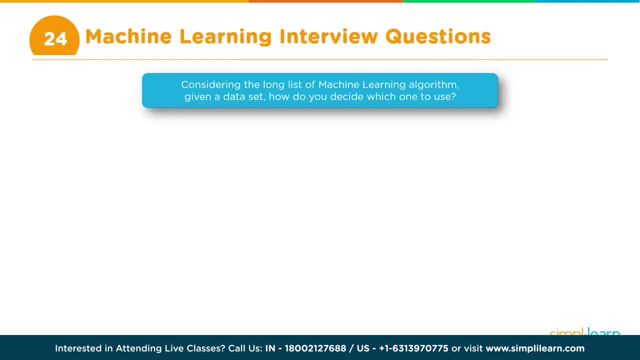 If you have a bunch of trees, You are basically mitigating the error, Reducing the error. So that is the way random forest works. So the next question is: Considering the long list of machine learning algorithms, How will you decide on which one to use? 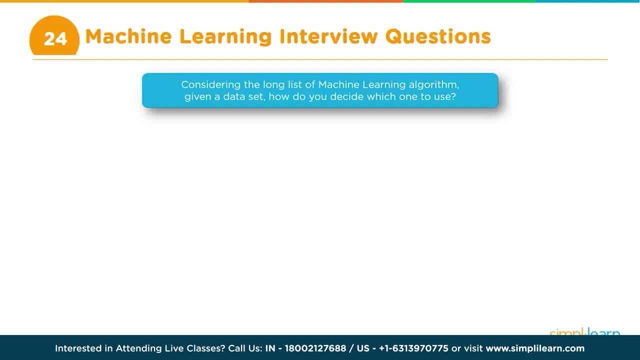 So once again Here, there is no way to outright say that This is the algorithm that we will use for a given data set. This is a very good question, But then the response has to be like again: There will not be a one size fits all. 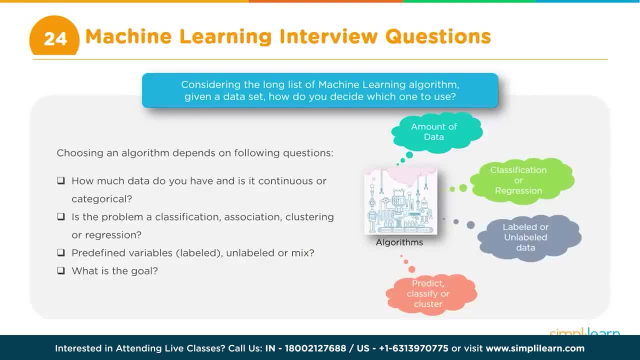 So we need to, First of all, Probably shorten the list In terms of by saying Whether it is a classification problem Or it is a regression problem. To that extent you can probably Shorten the list Because you don't have to use all of them. 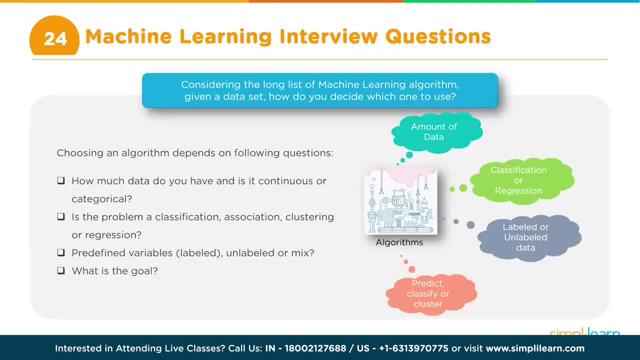 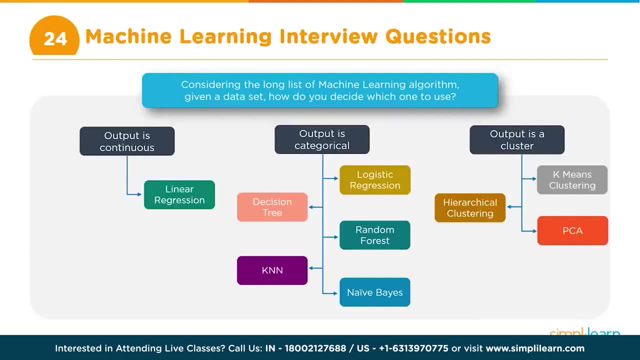 If it is a classification problem, You only can pick from the classification algorithms. So, for example, if it is a classification, You cannot use linear regression algorithm. Or if it is a regression problem, You cannot use SVM. Or maybe no, you can use SVM. 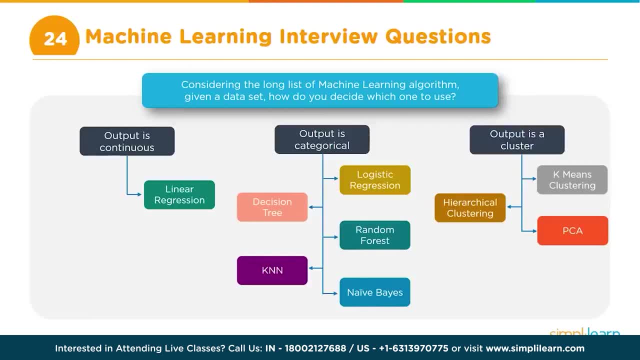 But maybe a logistic regression. You can probably shorten the list, But still you will not be able to 100% decide on saying that This is the exact algorithm That I am going to use. So the way to go about is: 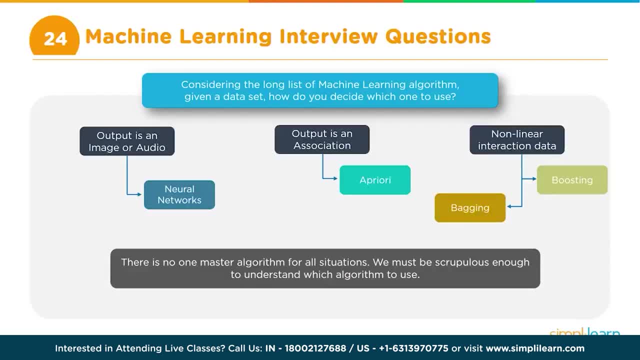 You choose a few algorithms Based on what the problem is. You try out your data, You train some models of these algorithms, Check which one gives you the lowest error Or the highest accuracy, And based on that You choose that particular algorithm. 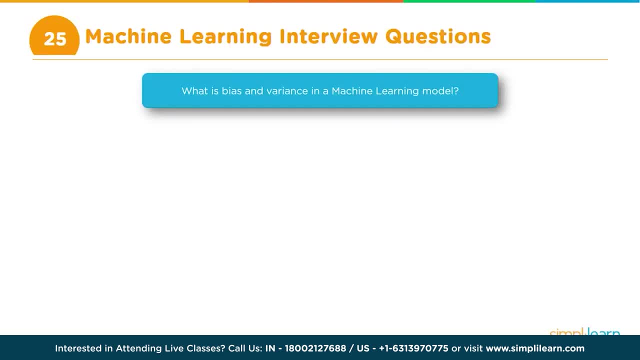 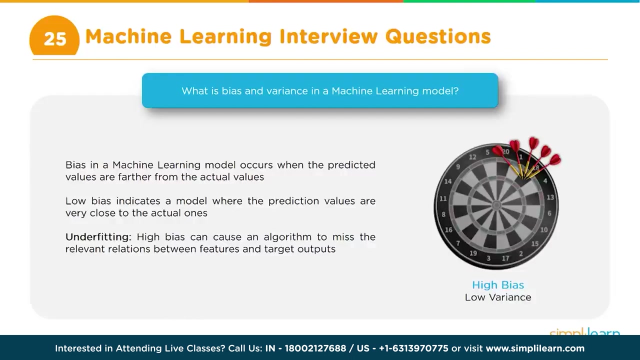 Okay, So the question is around Bias and variance. So the question can be: What is bias and variance in machine learning? So you just need to give out a definition For each of these. For example, bias in machine learning: It occurs when the predicted values are. 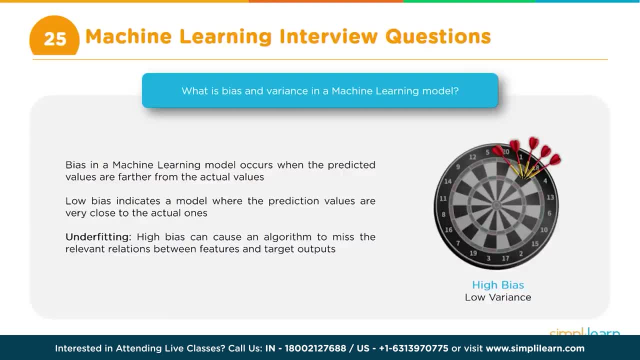 Far away from the actual value. So that is a bias, And whereas they are all, All the values are probably. They are far off, But they are very near to each other, though The predicted values are close to each other. You see the difference. 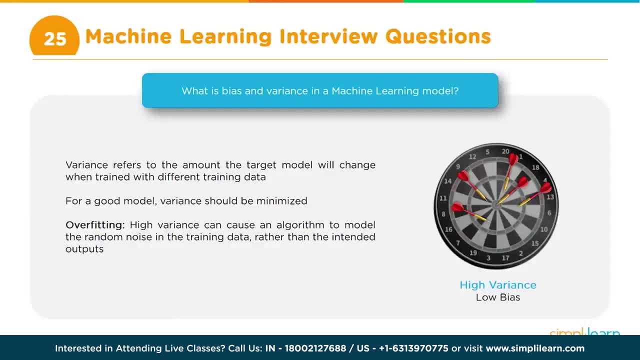 So that is bias. And then the other part is your variance. Now, variance is when The predicted values are all over the place, Right. So the variance is high. That means it may be close to the target, But it is kind of very scattered. 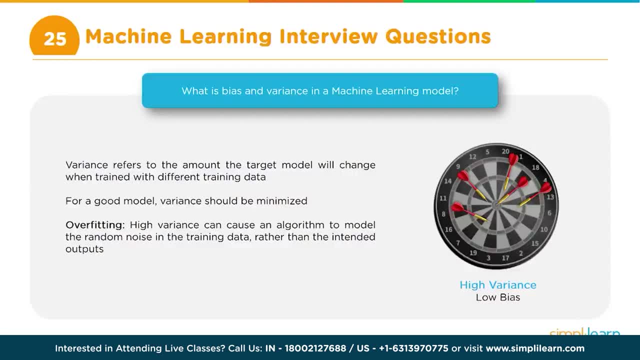 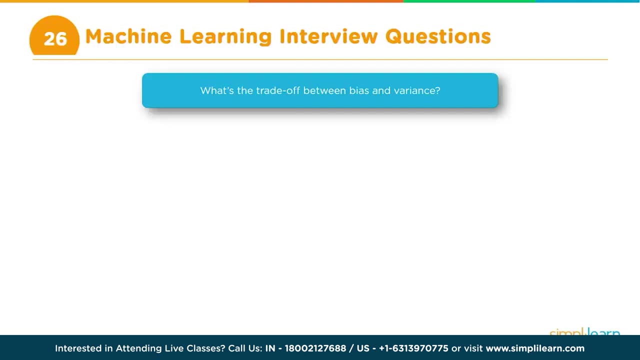 So the point: The predicted values are not close to each other. Right, In case of bias, The predicted values are close to each other, But they are not close to the target. They are more scattered. So that is what In case of variance. 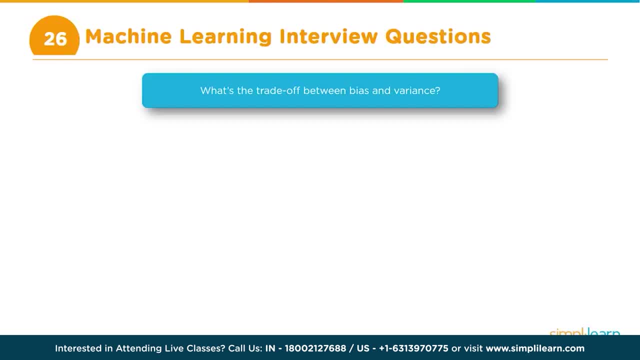 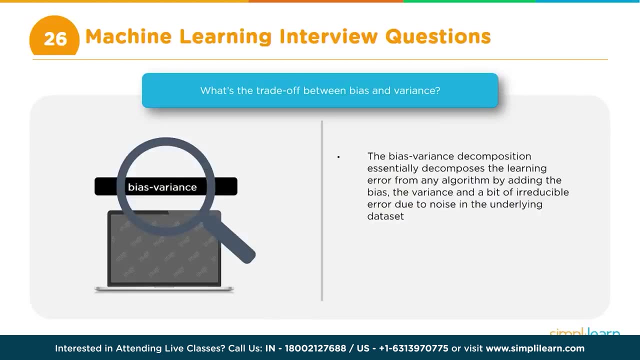 Okay, Then the next question is about, again related to bias and variance. What is the trade off between bias and variance? Yes, I think this is an interesting question Because these two are heading in different directions. So, for example, If you try to minimize the bias, 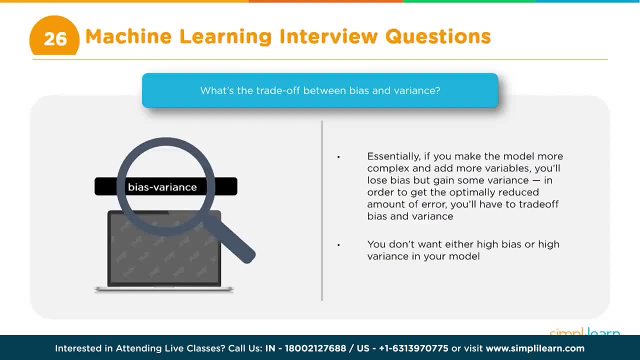 Variance will keep going high And if you try to minimize the variance, The bias will keep going high And there is no way you can minimize both of them. So there is a trade off Saying that, okay, This is the level at which I will have my bias. 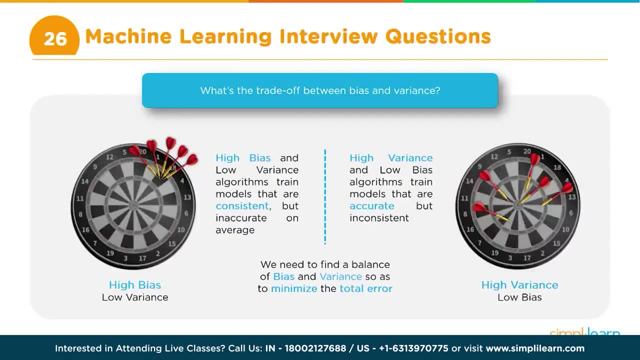 And this is the level at which I will have variance. So the trade off is that Pretty much, that You decide what is the level you will tolerate for your bias And what is the level you will tolerate for variance And a combination of these two. 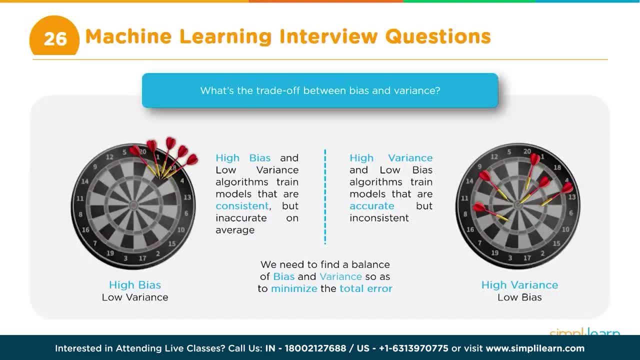 In such a way that Your final results are not way off, And having a trade off Will ensure that the results are consistent, Right? So that is basically Consistent, and which means that they are close to each other And they are also accurate. 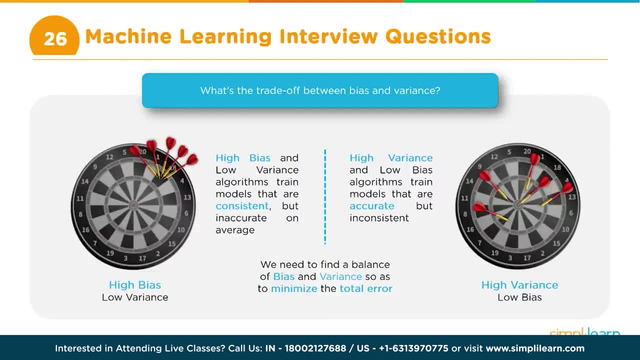 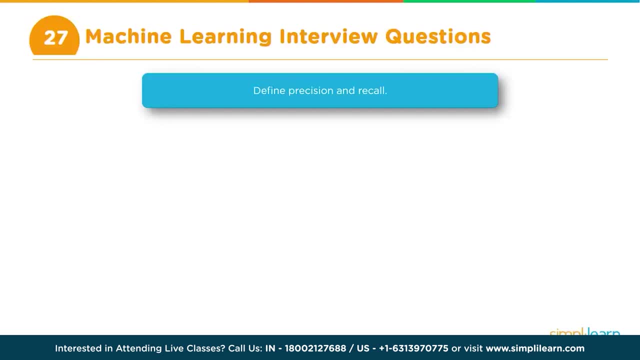 That means they are as close to the target as possible, Right? So if either of these is high, Then one of them will go off the track. Define precision and recall Now again, Here, I think it would be Best to draw a diagram. 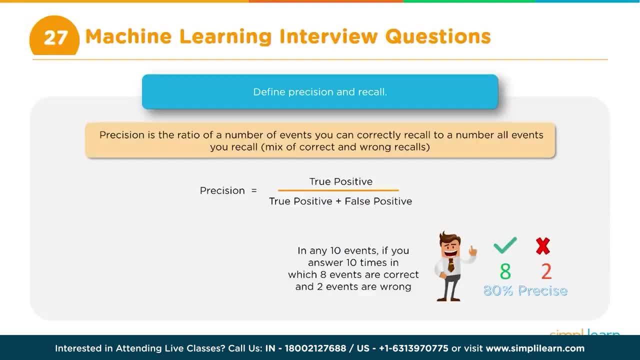 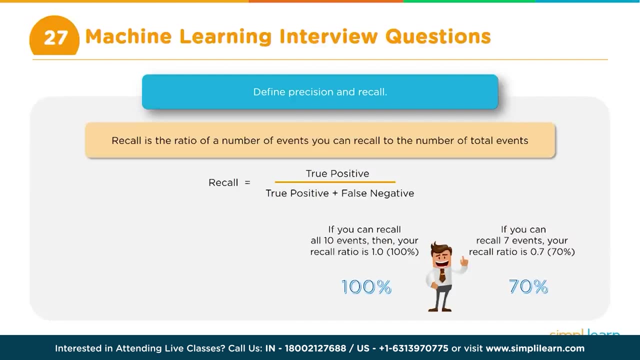 And take a confusion matrix, And it is very simple. The definition is like a formula. Your precision is True positive By true positive Plus false positive, And your recall is True positive by true positive Plus false negative. So that is, you can just show it in a mathematical way. 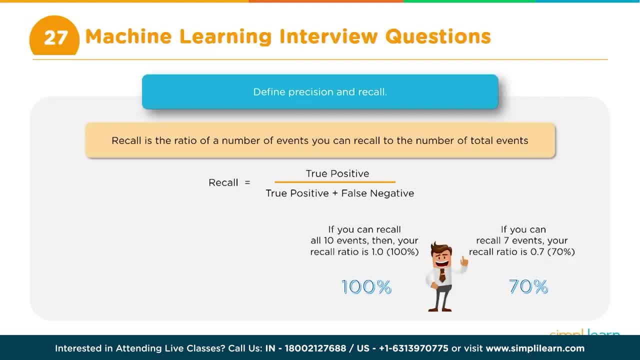 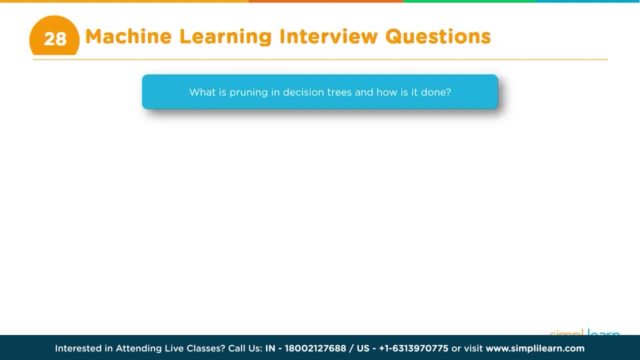 That is pretty much That can be shown. That is the easiest way to define. So the next question can be about decision tree. What is decision tree pruning And why is it So? basically, decision trees are Really simple to implement And understand. 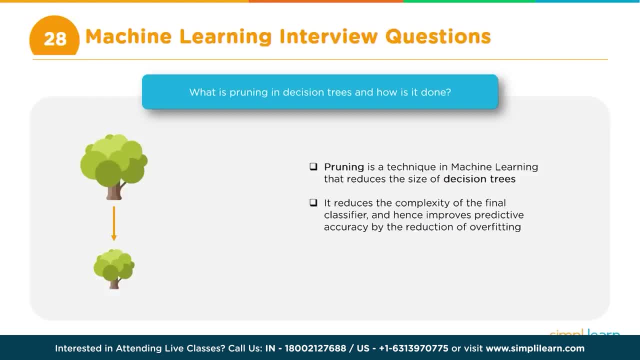 One of the drawbacks of decision trees Is that it can become Highly complicated as it grows Right, And the rules and conditions can become very complicated, And this can also lead to Overfitting, Which is basically that during training, You will get 100% accuracy. 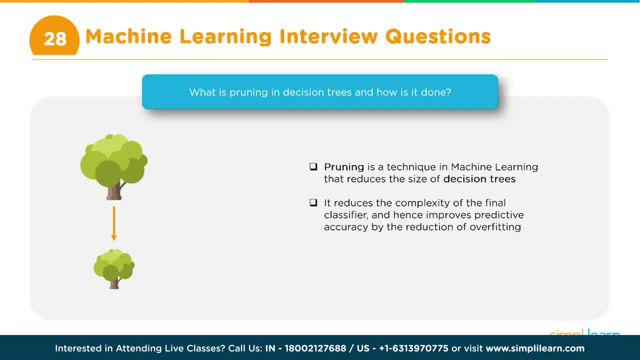 But when you are doing testing You will get a lot of errors. So that is the reason Pruning needs to be done. So the purpose or the reason for doing Decision tree pruning Is to cut down on overfitting Or to cut down on overfitting. 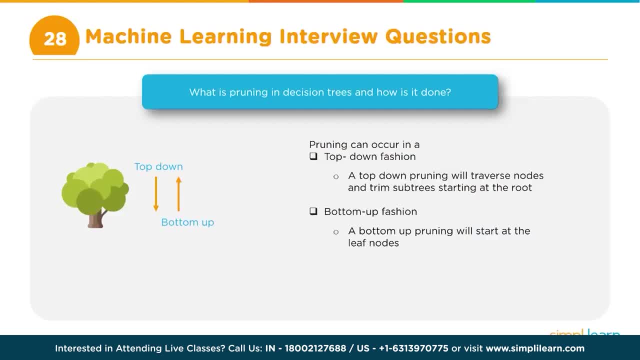 And what is decision? tree pruning? It is basically that You reduce the number of branches Because, as you may be aware, A tree consists of the root node And then there are several internal nodes And then you have the leaf nodes. Now, if there are too many of these internal nodes, 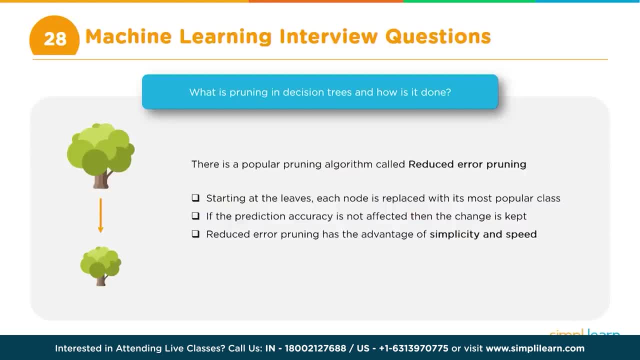 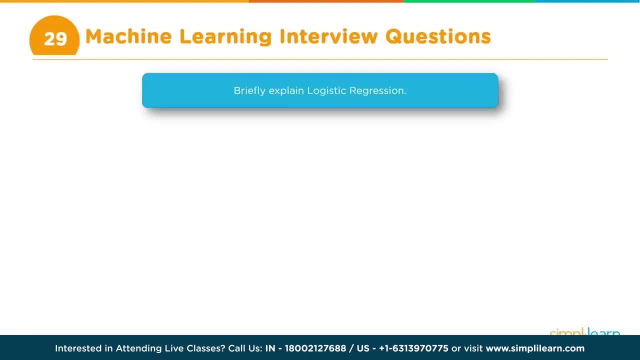 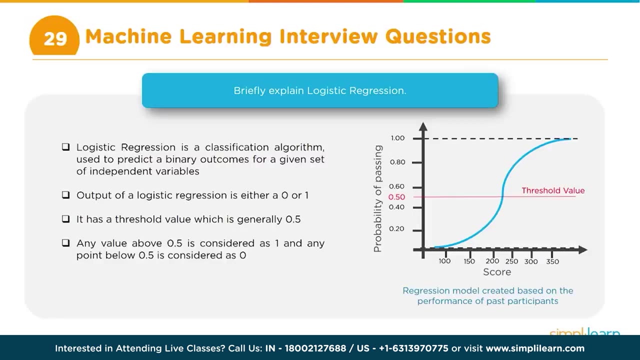 That is when you face the problem of Overfitting, And pruning is the process of Reducing those internal nodes. Alright, What is logistic regression? So, basically, logistic regression Is One of the techniques Used for performing classification, Especially binary classification. 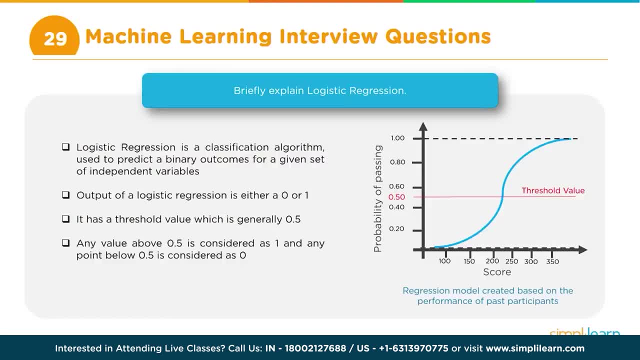 Now there is something Special about logistic regression, And there are a couple of things You need to be careful about. First of all, The name is a little confusing. It is called logistic regression, But it is used for classification, So this can be sometimes confusing. 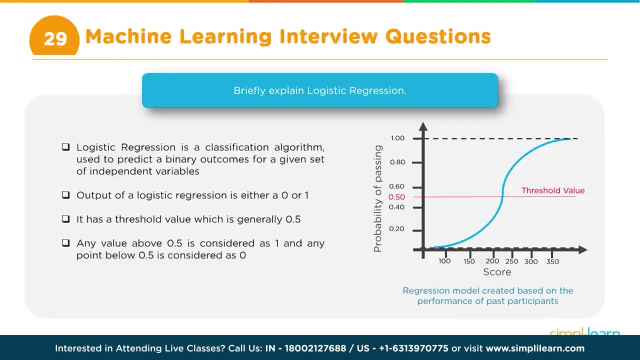 But you can probably clarify that To the interviewer If it is required, And they can also ask this like a trick question. So that is one part. Second thing is The term logistic has nothing to do with The usual logistics that we talk about. 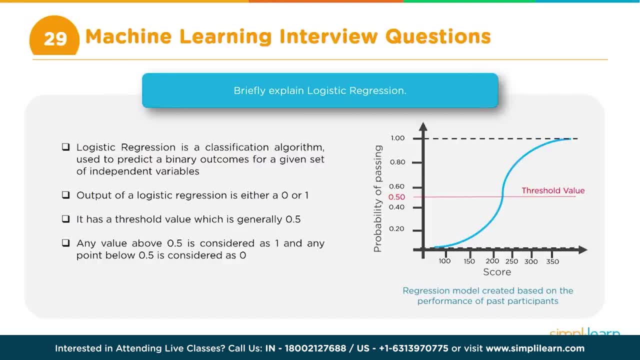 But it is derived from log, So that the mathematical Derivation involves log And therefore the name logistic regression. So what is logistic regression And how is it used? It is used for binary classification And the output of a logistic regression. 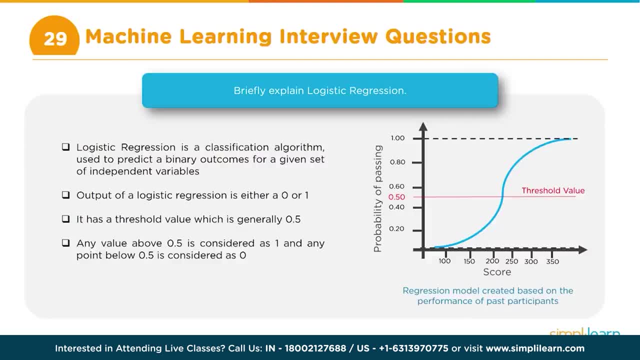 Is either a 0 or a 1. And it varies. So it is basically. It calculates a probability between 0 and 1. And we can set a threshold That can vary. Typically it is 0.5.. So any value above 0.5. 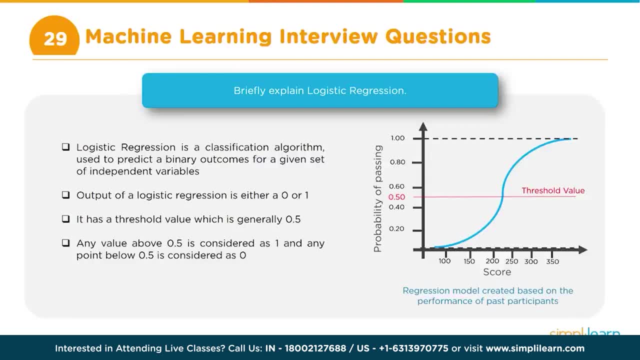 Is considered as 1.. And if the probability is below 0.5. It is considered as 0.. So that is the way we calculate the probability, Or the system calculates the probability And, based on the threshold, It sets a value of 0 or 1.. 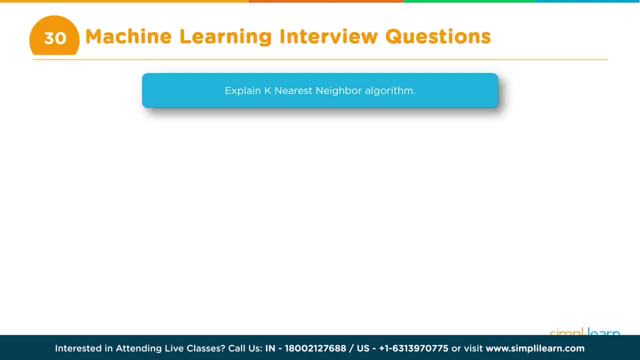 Which is like a binary classification- 0 or 1.. Okay, then we have a question around K nearest neighbor algorithm. So explain k nearest neighbor algorithm. So, first of all, What is a k nearest neighbor algorithm? This is a classification algorithm. 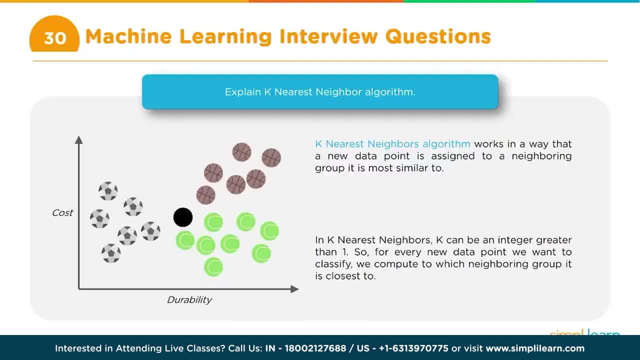 So that is the first thing we need to mention, And we also need to mention That the k is a number, It is an integer And this is variable And what the value of k should be. It can be 2,3,5,7.. 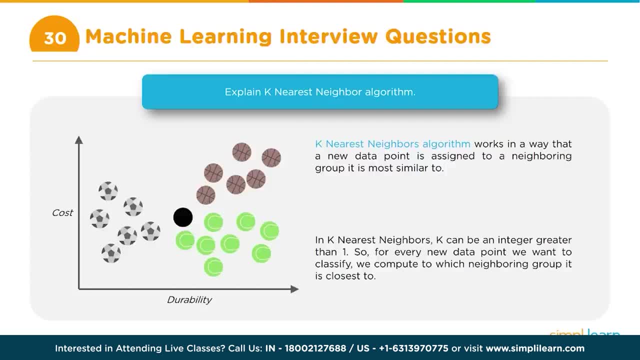 And usually it is an odd number. So that is something we need to mention. Technically it can be even number also, But then typically it would be odd number And we will see why that is So. based on that, We need to classify objects. 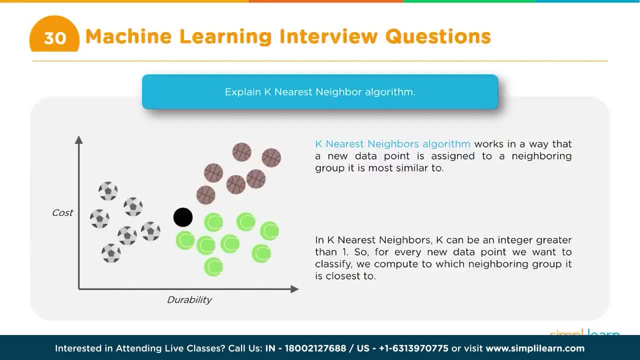 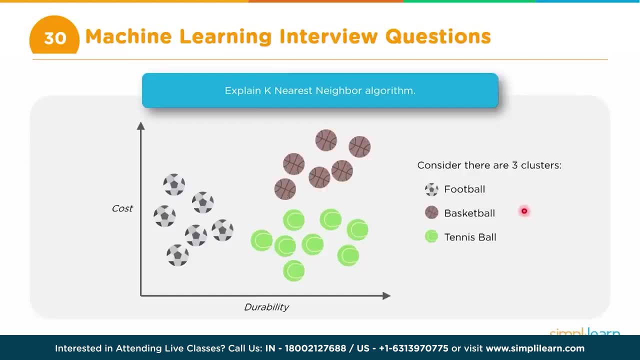 We need to classify objects. So, again, it will be very helpful To draw a diagram. You know, if you are explaining, I think that will be the best way. So draw some diagram like this: So you have 3 clusters or 3 classes existing. 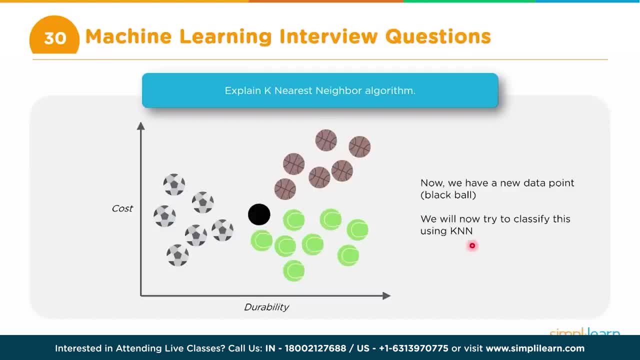 And now you want to find For a new item that has come. You want to find out Which class this belongs to. So you go about as the name suggests. You go about finding the nearest neighbors, The points which are closest to this. 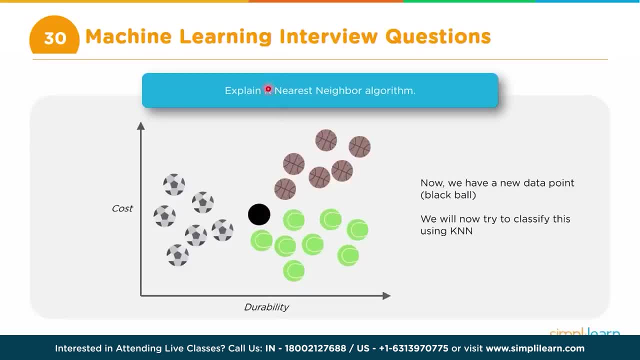 And how many of them you will find. That is what is defined by k. Now let us say Our initial value of k was 5.. So you will find the k, The 5 nearest data points. So in this case, As it is illustrated, 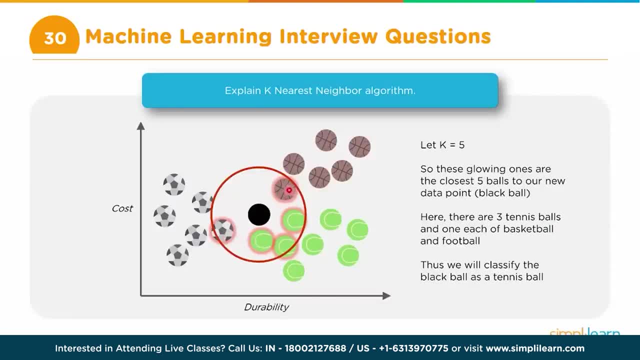 These are the 5 nearest data points, But then all 5 do not belong To the same class or cluster, So there are one belonging To this cluster, 1. The second one belonging to this cluster, 2. 3 of them belonging to this third cluster. 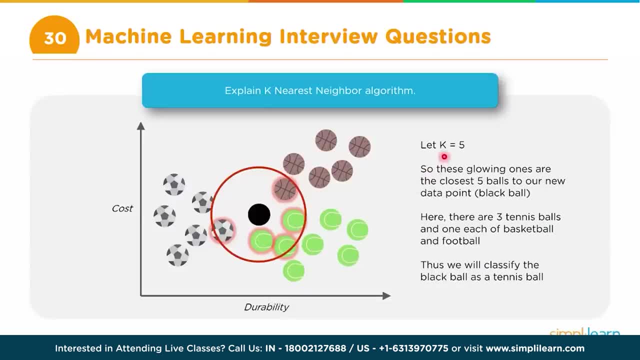 So how do you decide? That is exactly the reason We should, as much as possible, Try to assign an odd number, So that it becomes easier to assign this. So in this case, you see that The majority actually, And you go with the majority. 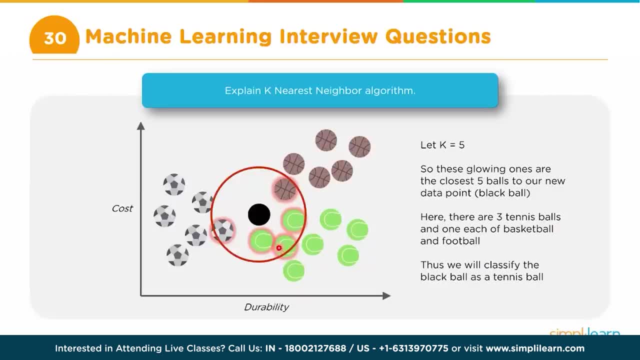 So, since 3 of these items Belong to this class, We assign, which is basically the, In this case the green, Or the tennis, or the third cluster, As I was talking about. So we assign it to this third class. So in this case it is. 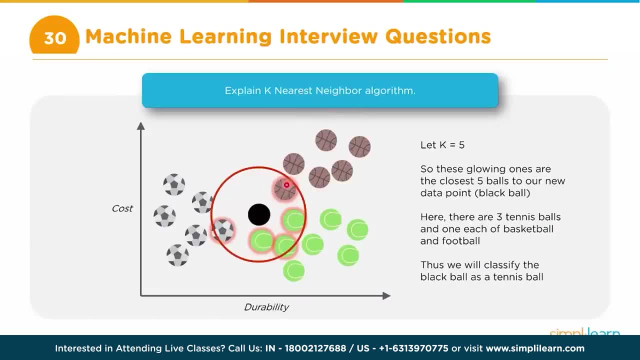 That is how it is decided. So k nearest neighbors. First thing is to identify the number of neighbors That are mentioned as k. So in this case it is: k is equal to 5.. So we find the 5 nearest points And then find out. 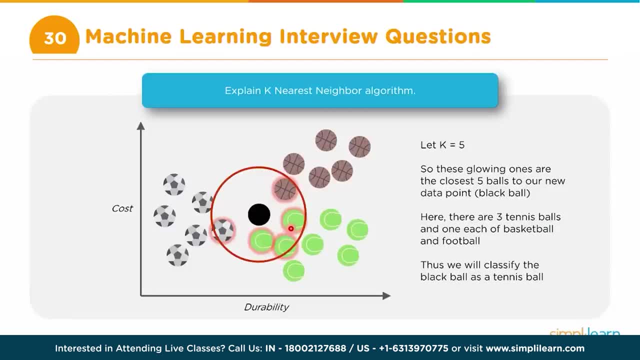 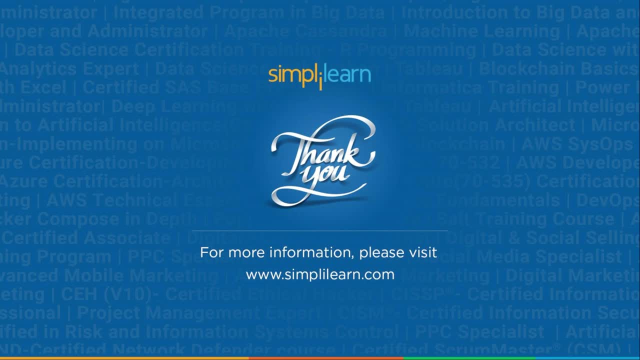 Out of these: 5. Which class has the maximum number in that? And then the new data point is assigned to that, And with that We have come to the end of machine learning: Beginners to advanced full course. I hope you found it valuable and entertaining. 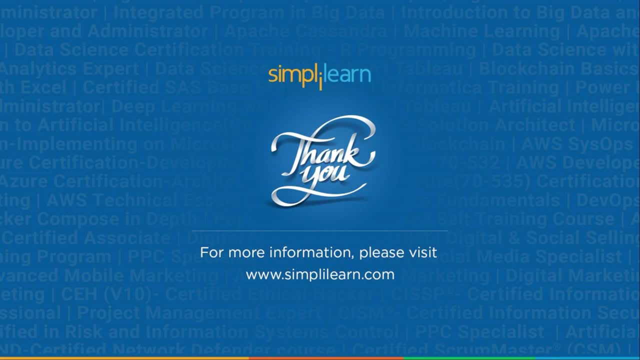 Please ask any questions About the topics covered in this video In the comment section below. Our experts will assist you in addressing your problems. Thank you for watching. Stay safe and keep learning. Staying ahead in your career Requires continuous learning and upskilling. 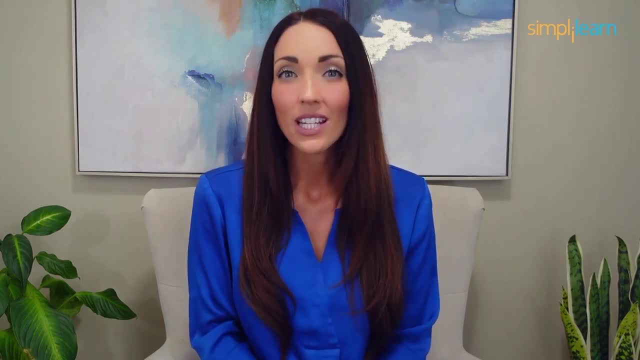 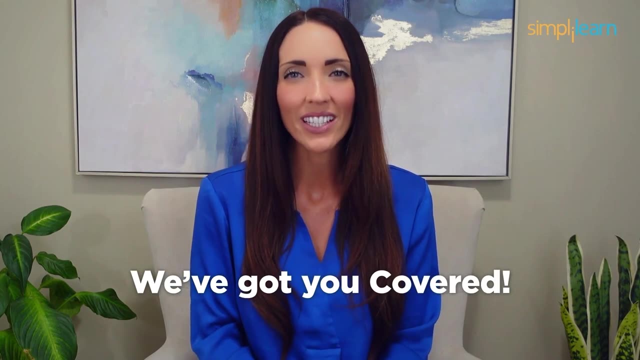 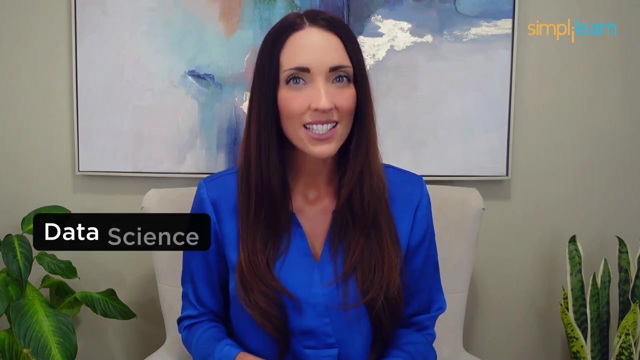 Whether you are a student Aiming to learn today's top skills, Or a working professional Looking to advance your career, We've got you covered. Explore our impressive catalog Of certification programs In cutting edge domains, Including data science, Cloud computing. 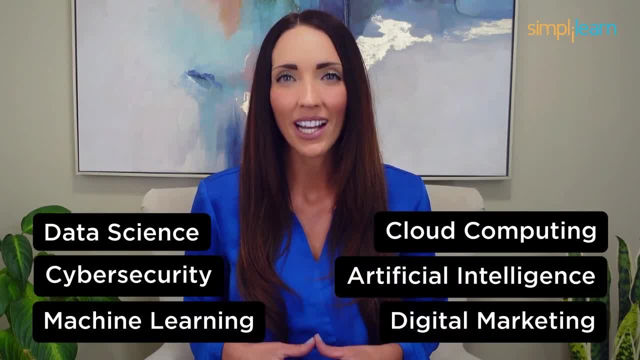 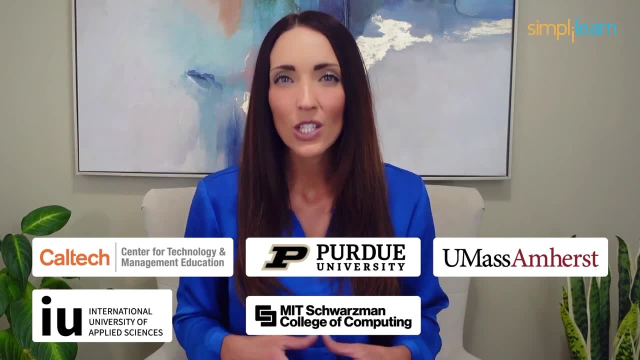 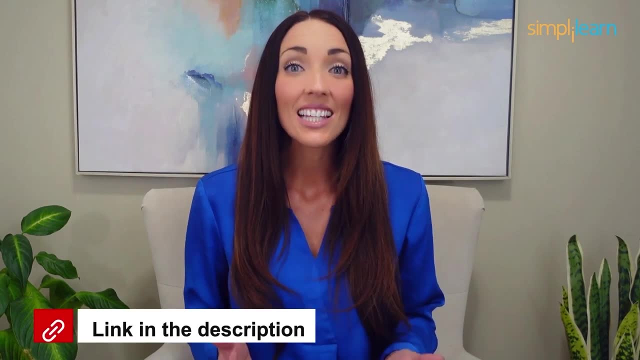 Cyber security, AI, Machine learning Or digital marketing Corporations, And delivered by industry experts. Choose any of our programs And set yourself on the path To career success. Click the link in the description To know more.